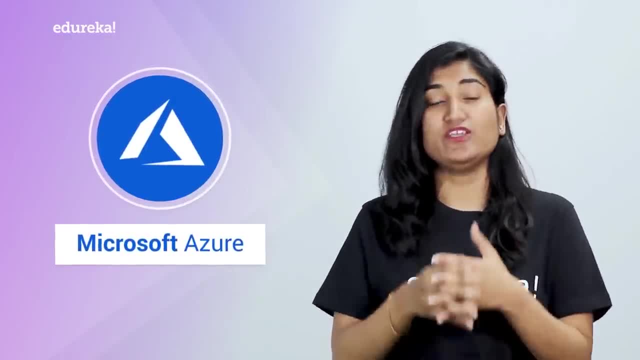 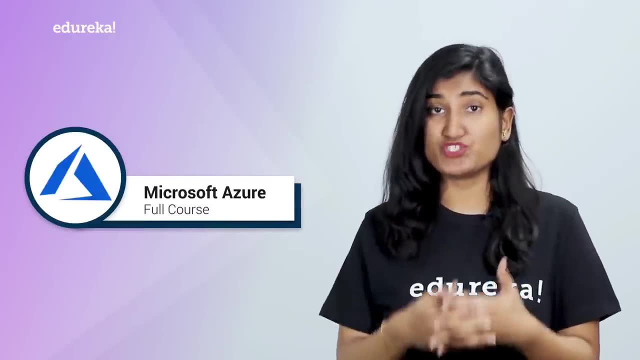 of top cloud computing skills that one must have If you want to make a career in this domain, then you've landed at the right place. Hi, I welcome you all to this full course on Microsoft Azure, which not only talks about Azure fundamentals, but will also take you deep. 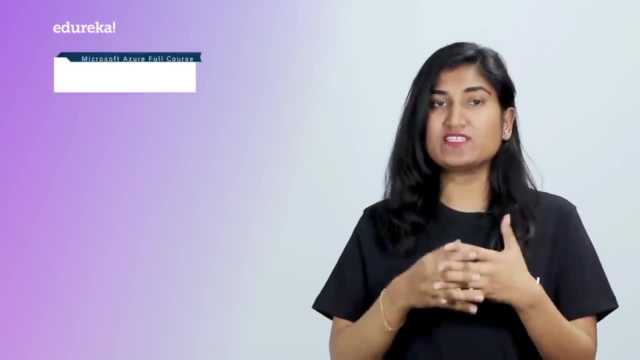 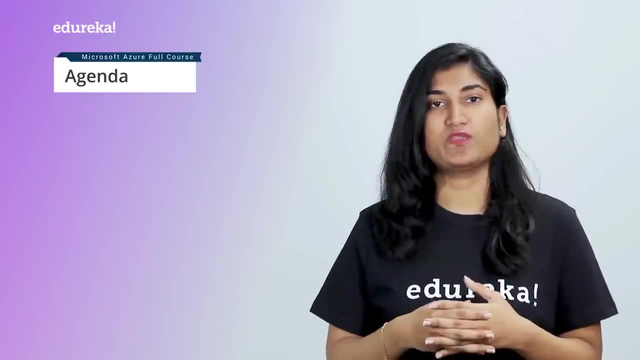 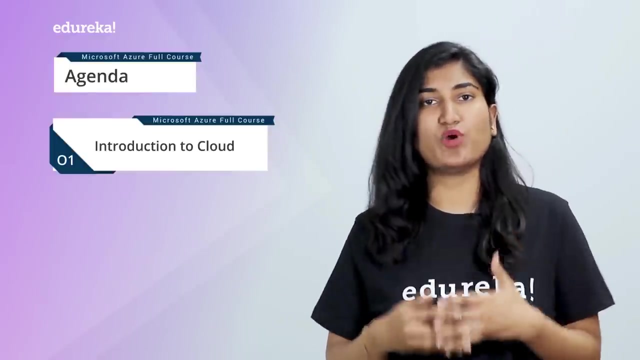 at conceptual levels. Before we get into details, let's look at our agenda for today. For better understanding and ease of learning, entire course is divided into multiple modules. First module, introduction to cloud, is about what exactly cloud computing is. different kind of deployment and service models in cloud computing. 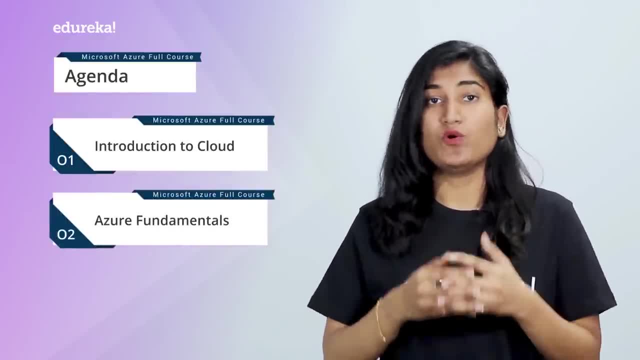 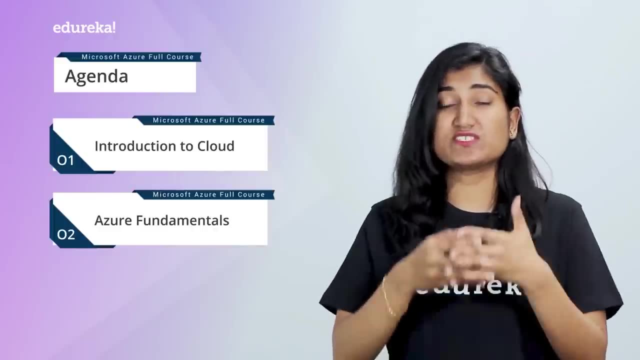 Second module is about Azure fundamentals. Well, in this module we will learn how to create Azure free TAR account and we'll also discuss one of the core computing service, which is Azure virtual machine. Next up in the third module, we'll discuss Azure storage services and database. 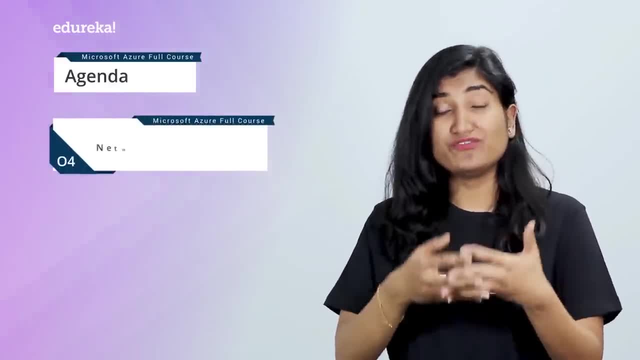 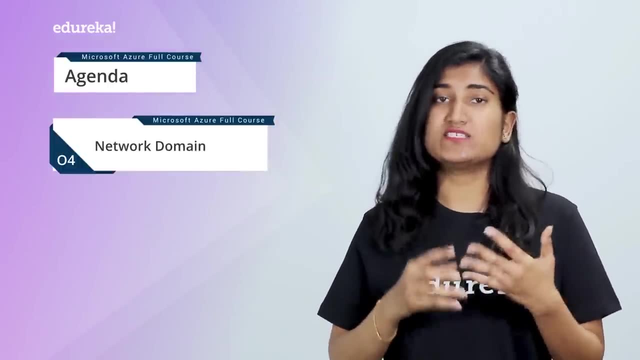 features in detail. Fourth module is about different network services offered by Azure. In here we'll discuss Azure virtual network and related concepts like subnets, security groups and many more. In fifth module we will learn how to secure your access to your resources. 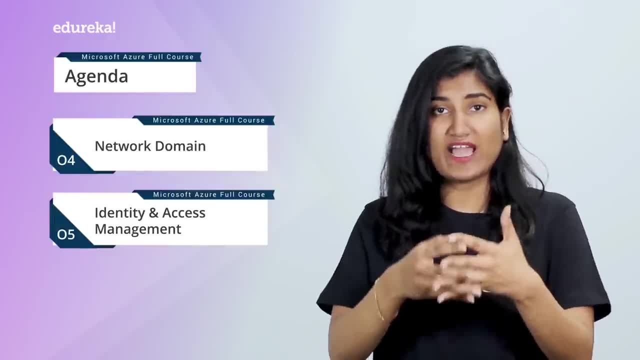 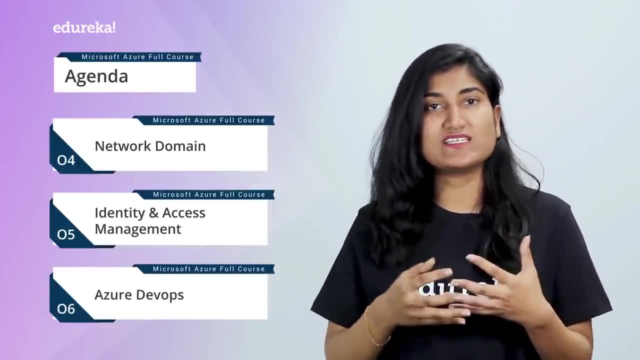 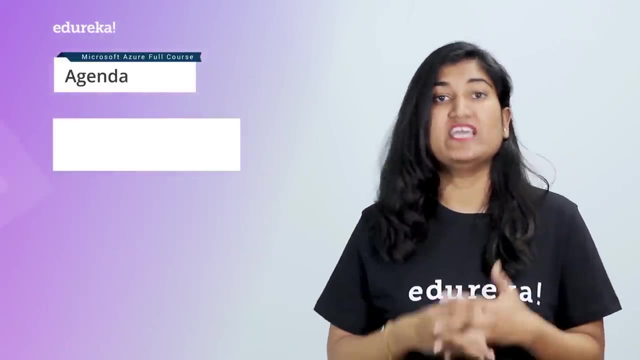 using identity and access management services like Azure Active Directory. Sixth module is all about Azure DevOps. In this module, we'll learn how to simplify and accelerate entire DevOps process using Azure DevOps services like Azure Pipeline, Azure Boards, etc. In seventh module, we'll talk about different services offered by Azure. when you are dealing 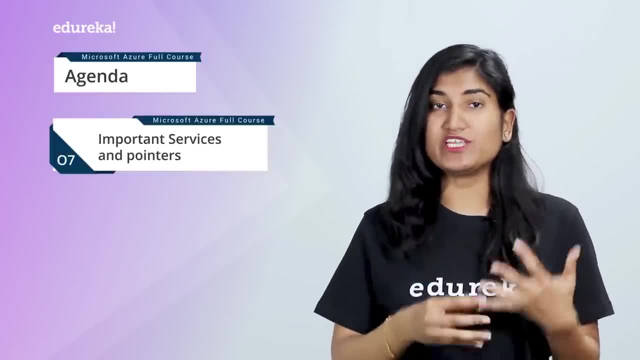 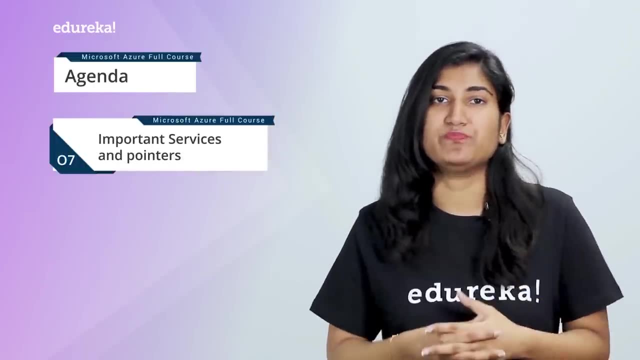 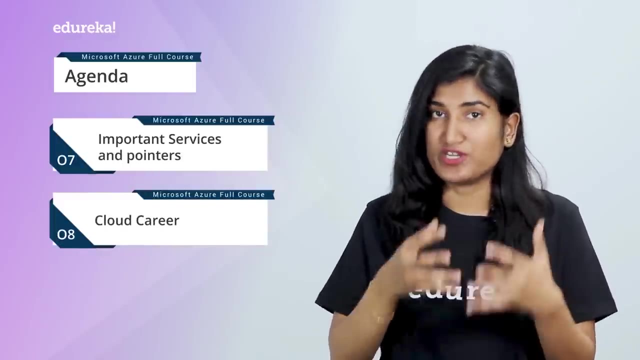 with current trending technologies like machine learning, AI, IoT and many more. Also, we'll be comparing Microsoft Azure with other leading service providers like AWS and GCP. Final module is mostly career related. In this module we'll discuss most frequently asked interview questions in Azure interviews. We'll also 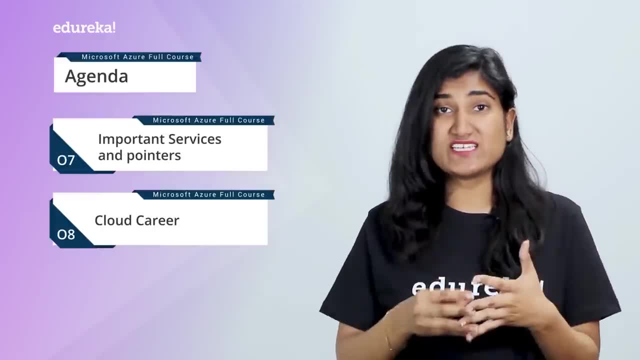 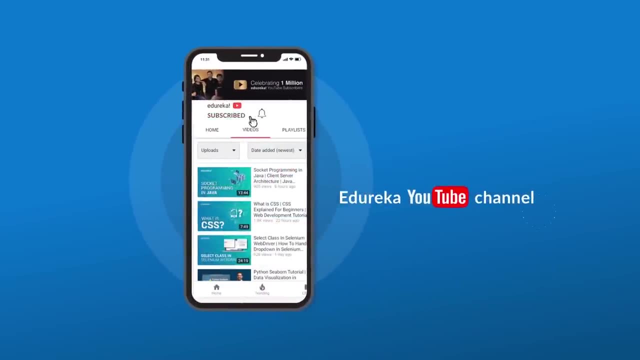 discuss roles and responsibilities, job trends and skills that you should have to ace your interview. Thank you, everyone. While you are at it, please do not forget to subscribe at Eureka YouTube channel and hit the bell icon to stay updated with current trending technology. 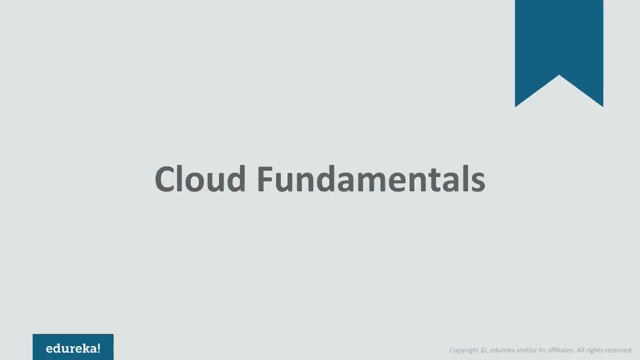 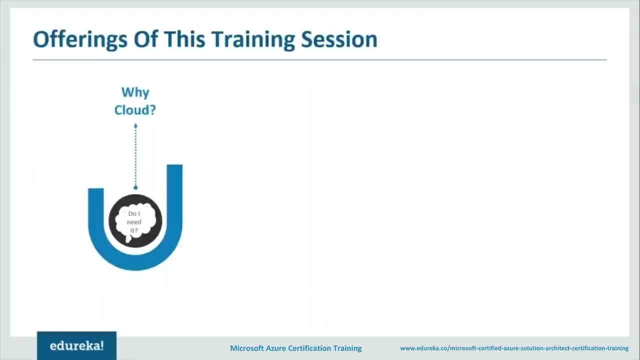 Thanks. So let us move further and quickly take a look at today's agenda first. Firstly, I would be discussing the basics of cloud, as in why it is needed and what it is exactly. I would also discuss the different models that cloud has to offer to you, like its service models and also. 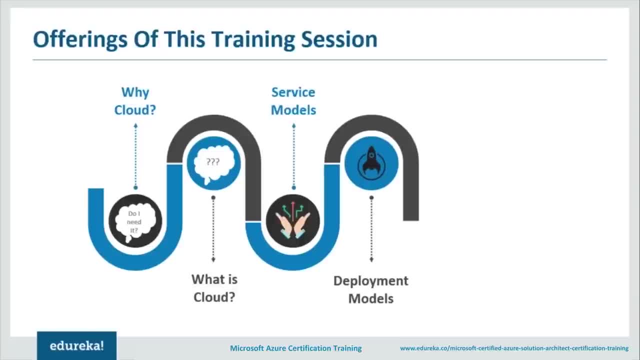 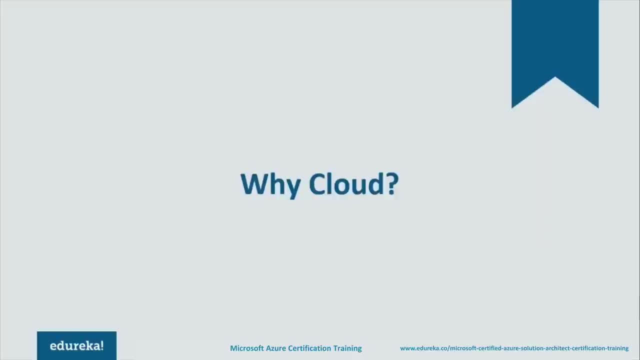 its deployment models. I would also discuss the different cloud providers that are there in the market And finally, I would finish things off with the demo part. I hope this agenda is clear to all of you. Firstly, let's understand why cloud. to understand this: 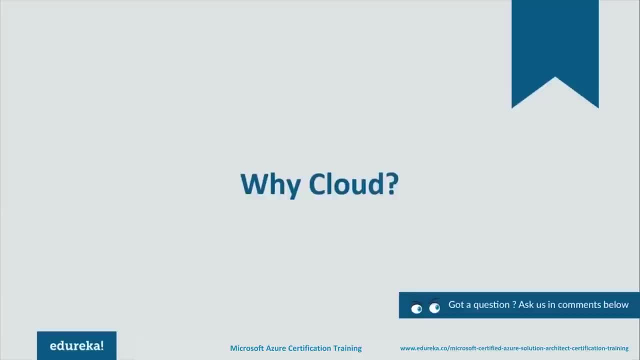 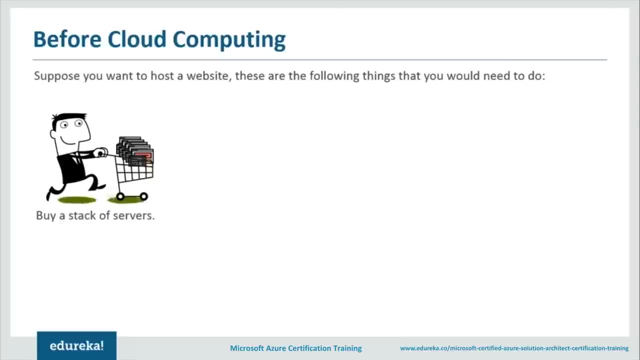 We need to understand the situation that existed before cloud came into existence. So what happened back then? and firstly, in order to host a website, you have to buy a stack of servers, and we all know that servers are very costly, So that meant we ended up paying a lot of money. next was the issue of traffic. 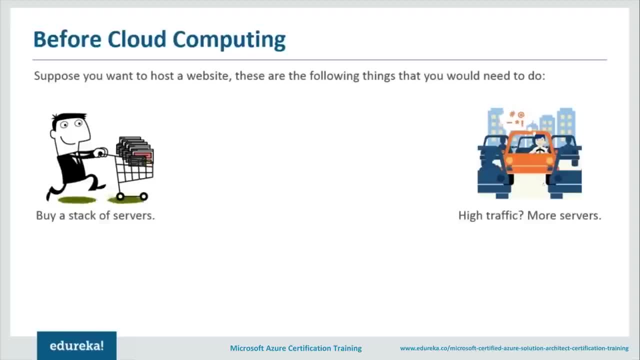 Now, as we all know, if we are hosting a website, we are dealing with traffic that is not constant throughout the day and that meant more pain. would understand that as we move further. And the other thing was monitoring and maintaining your servers. Yes, This is a very big problem. 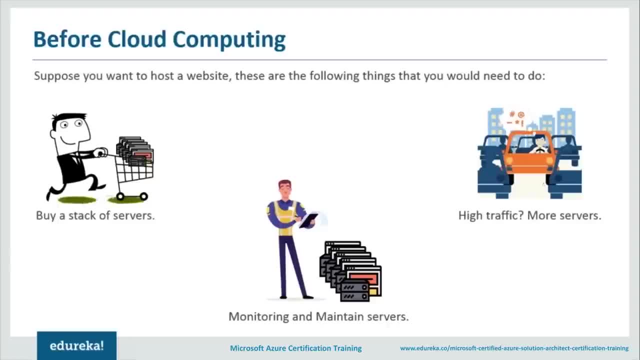 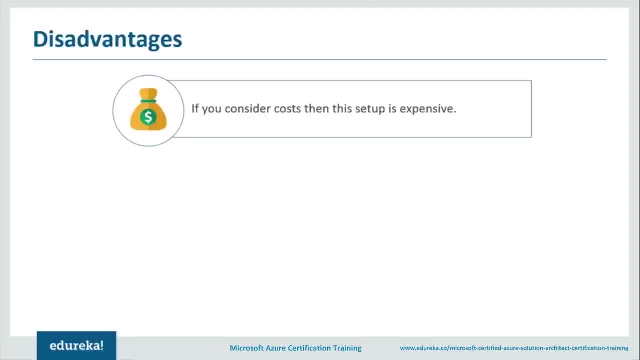 Now, all these issues. they led to certain disadvantages. What are those? as I mentioned, servers are very costly. Yes, the setup was again costly, and thus you ended up paying a lot of money, and there were other factors contributing to this point. Let's discuss those as well. one troubleshooting was a big issue. 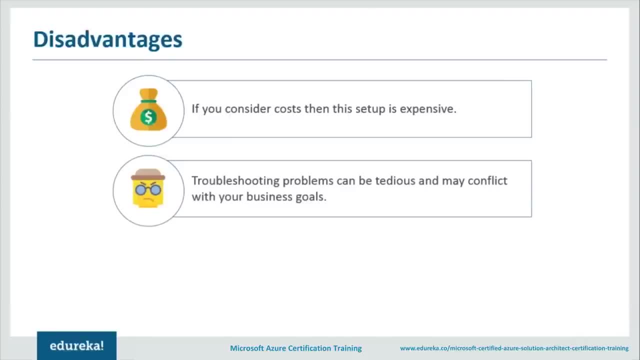 since you're dealing with a business, your prime focuses on taking good decisions So that your business does well. but if you end up troubleshooting problems or you focus more on infrastructure related issues, then you cannot focus more on your business, and that was a problem. 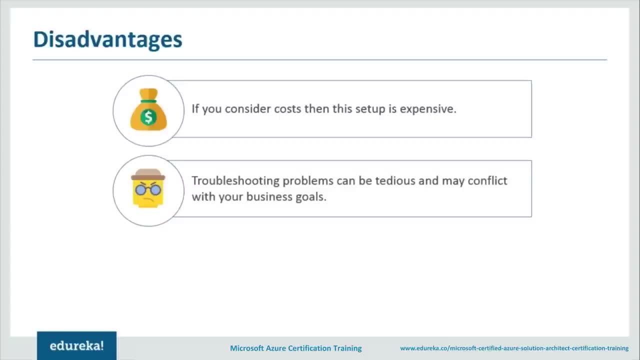 So either you had to do multitasking or you had to hire more people to focus on those issues. Thus, again, you ended up paying more money. as I've discussed, the traffic on a website is never constant and since it varies, you are not certain about its patterns, say, for example, 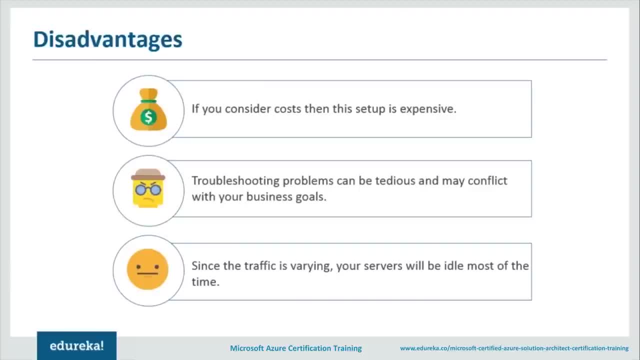 I need to host a website, and for that, what I decide is I'm reserving two petabytes of total memory for my usage, based on the traffic, but as the traffic varies, there would be times when the traffic is high and my whole two petabytes of data is consumed. 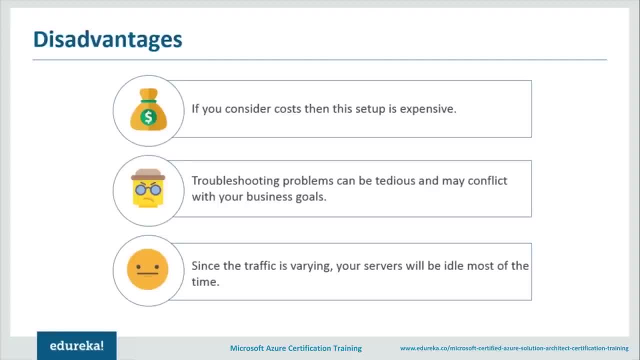 or space is consumed, rather, But what if the traffic is very low for certain hours of the day? I'm actually not utilizing these servers, So I end up paying more money for the servers than I should be. So yes, upscaling was an issue. 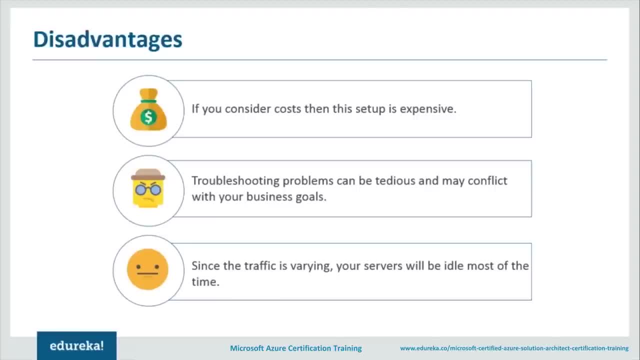 So all these things were an issue because we were paying more money, We did not have sufficient time to take our decisions properly, There was ambiguity, There was more trouble monitoring and maintaining all these resources and, apart from that, one important point which we need to consider is the amount of data. 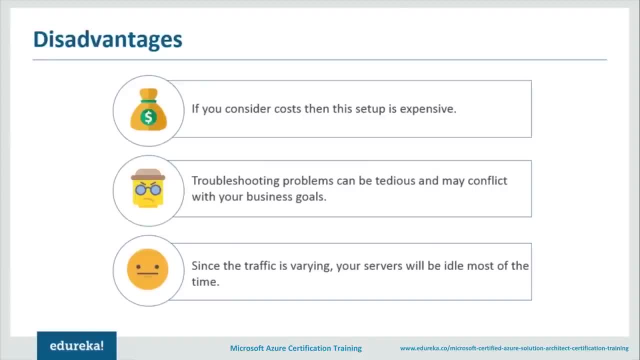 that is being generated now and that was being generated then, then it was okay, But nowadays, if you take a look at it, the amount of data that is generated is huge, and this is another reason why cloud became so important. Yeah, as I've mentioned the data now. 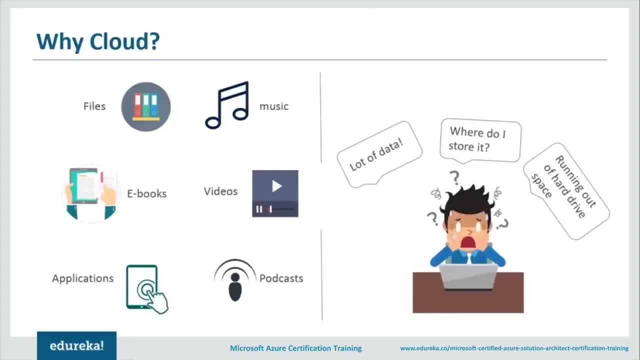 we all know that everything is going online these days, and what that means is we shop online, We buy food online, We do almost everything that is required, as in whatever information we need to get everything online- your bookings or reservations- everything can be taken care of. 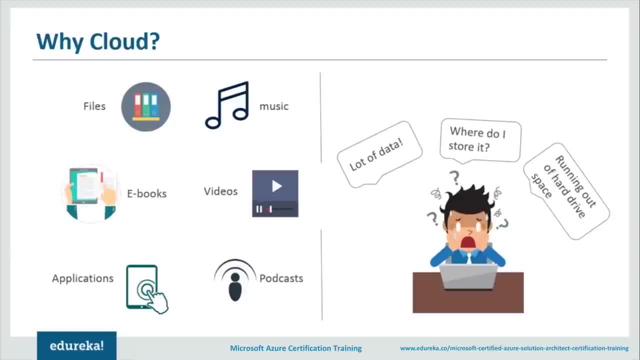 That means we have a lot of data that is being generated these days and this is digital data. back in those times, We were communicating through verbal discussions and all those things, so through paperwork, and that was a different data to maintain. since everything is moving on cloud or moving online, the amount 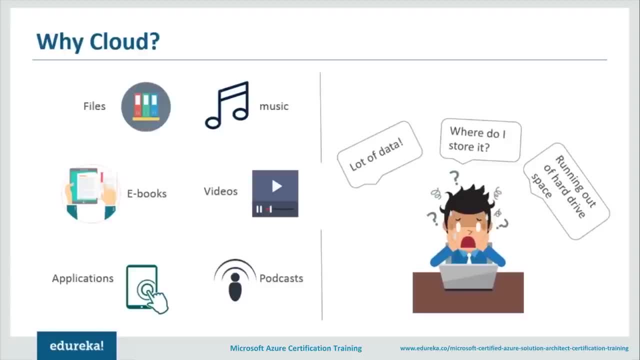 of data that we have is huge these days, And then, when you have this huge amount of data, you need a space where you can actually go ahead and maintain this data. So, yes, again, there was a need of this space and all these issues. that is, your cost, your monitoring. 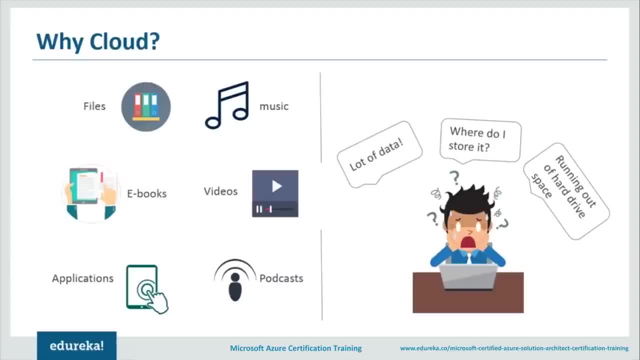 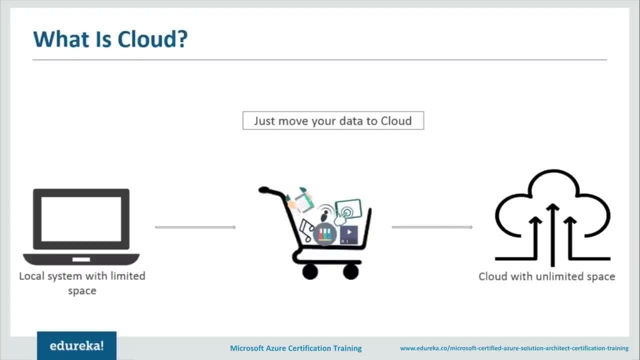 your maintenance, providing sufficient space. Everything was taken care by cloud. So let us try to understand what this cloud is exactly. Well, think of it as a huge space that is available online for your usage. Now, this is a very generic definition to give you to be more specific. 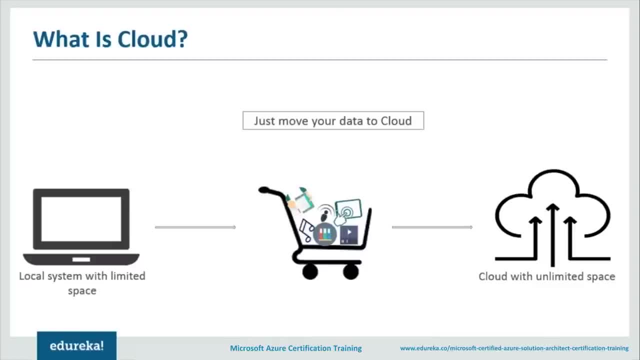 I would be saying that think of it as a collection of data centers, now data centers again at a place where you store your data or you host applications, basically. So when you talk about these data centers, they were already existing. So what did cloud do differently? 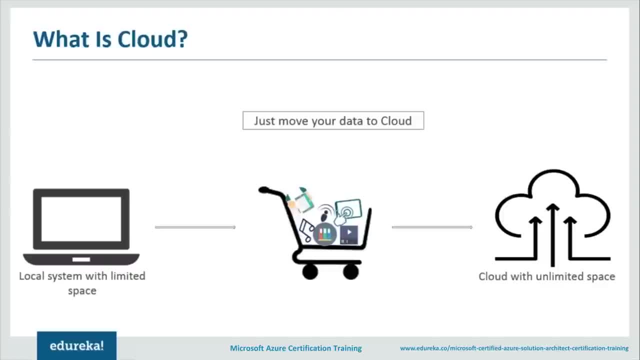 Well, what cloud did, was it made sure that you are able to orchestrate your various functionings, your applications, managing your resources properly, by combining all these data centers together Through a network and then providing you the control to use these resources and to manage them properly. 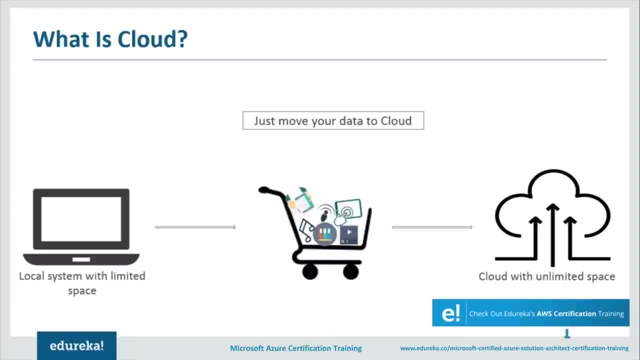 to make it even more simpler, I would say there was a group of people or organizations, basically, that went ahead and bought these servers, these compute capacities, storage places, compute services and all those things, and they have their own channel or network. All you have to do was go ahead. 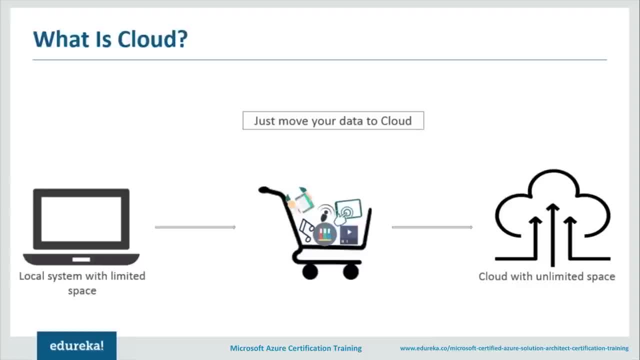 and rent those resources only to the amount you need it and also for the time that you need it. So, yes, this is what cloud did? it let you rent the services that you need and use only those services that you need. So you ended up paying for the services that you rented. 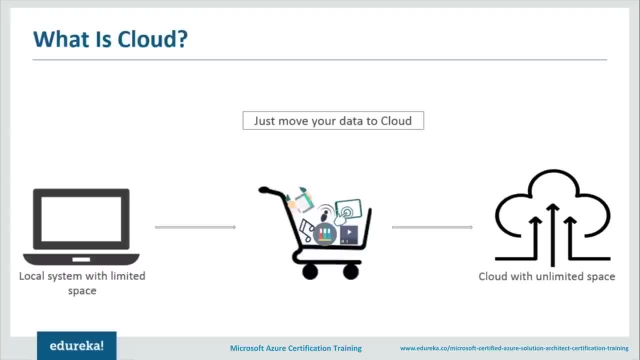 and you ended up saving a lot of money. The other thing is these service providers: They take care of all the issues like your security, your underlying infrastructures and all those things, so you can freely focus on your business and stop worrying about all these issues. 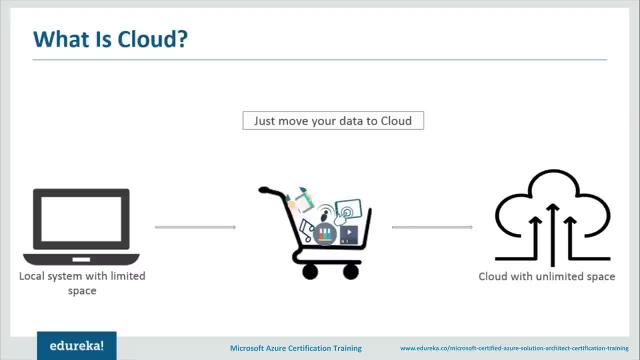 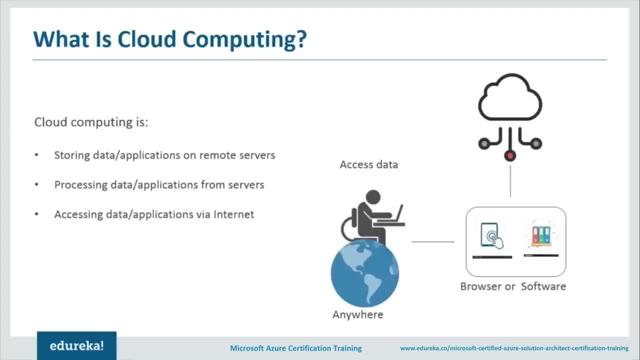 So this is what cloud is in simple words, It's a huge space which has all these services available and you can just go ahead and pick and rent those services that you want to use. So what is cloud computing? Well, I've already discussed that. just to summarize it, 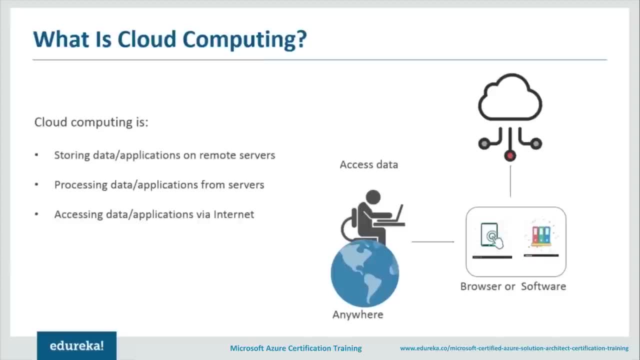 I would say it is nothing but an ability or it is a place where you can actually store your data, You can process it and you can access it from anywhere in the world. Now, This is an important point. Say, for example, you decide to choose a reason for your infrastructure somewhere. 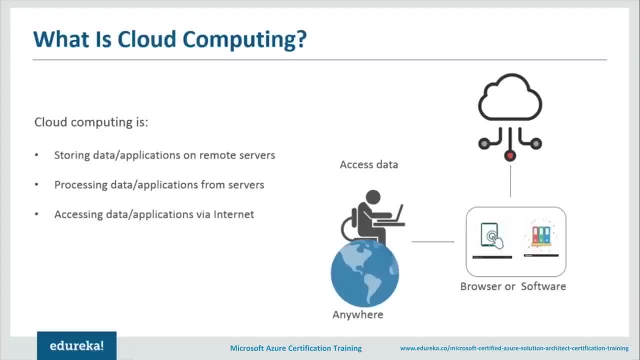 in us. you can sit in maybe China or maybe in India and you can still have access to all your resources. that is there in us. All you need is a good internet connection. So that is what cloud does: it makes the world accessible. It lets you have your applications wherever you want to. 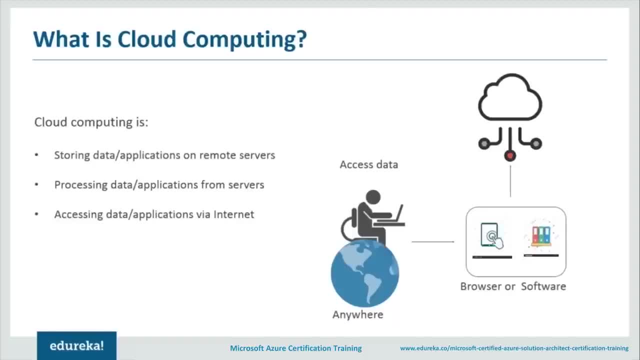 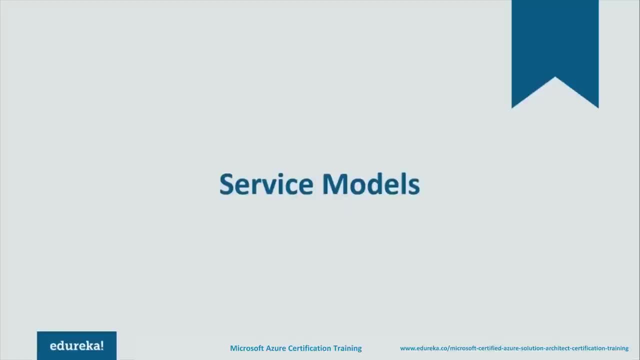 and manage them the way you want to. so this was about cloud computing, guys. next we would be discussing different service models. Now you need to understand one thing: you are being offered cloud services, the platform to use your services or your applications, basically- but then different people have different requirements. 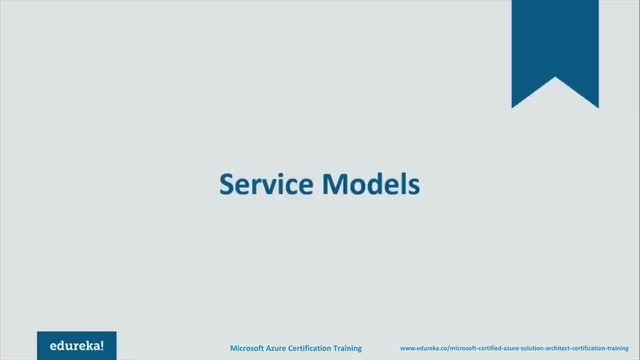 There are certain people who just want to consume a particular resource, or there are certain people who actually want to go ahead and create their own applications, create their own infrastructure and all those things. So, based on these needs, we have particular service models, that is, your cloud providers provide you. 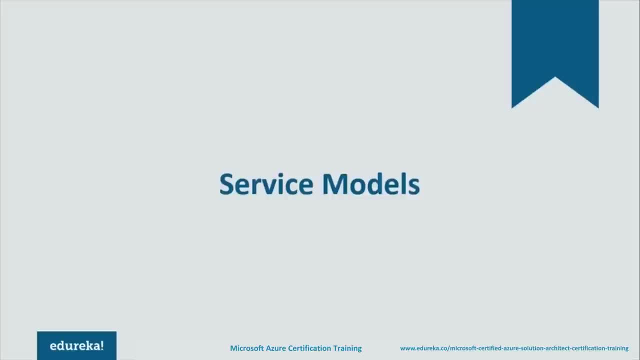 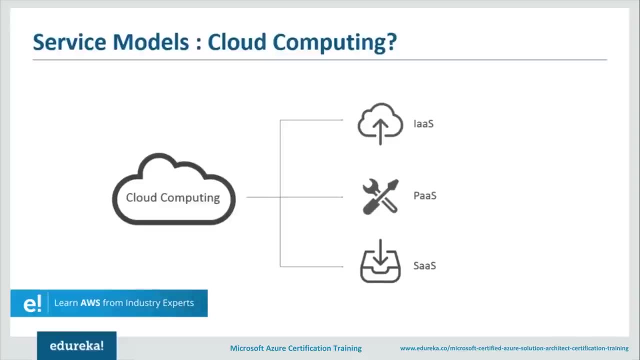 with a particular model which suits your needs. So let us try to understand these models one by one. Well, we have these three models, that is, your IAS, your PAS and your S AAS. I would be discussing them in the reverse order, that is, I would be talking about S AAS first. 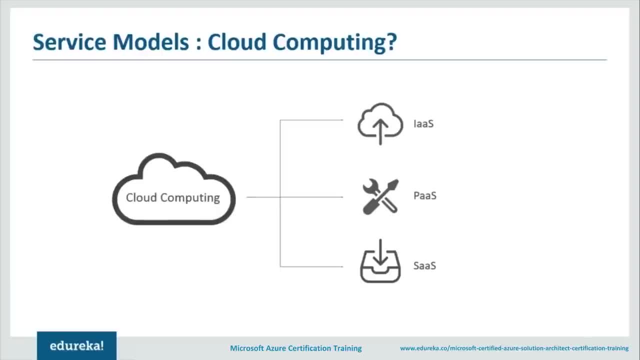 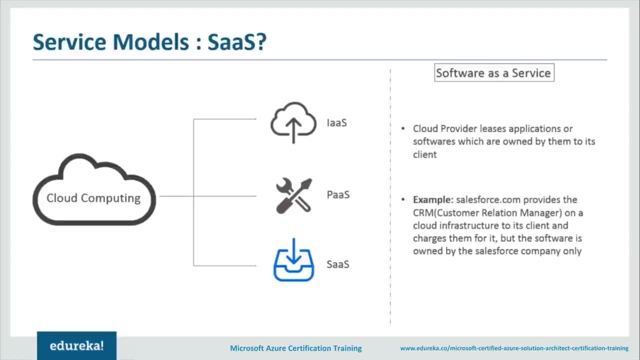 and then I would go upwards. So let us start with S AAS or SAS. S AAS is nothing but a software as a service. Now, what happens here is basically you are just consuming a service which is already being maintained and handled by someone else. to give you a valid example, 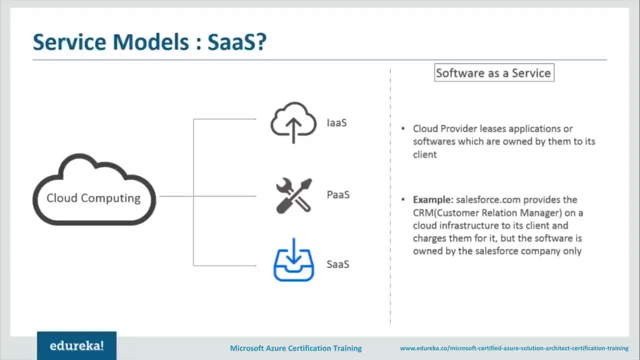 We have a Gmail. all you do is you send mail to people and you receive mails, and whatever functionality you do is you just use the service that is there. You do not have to maintain it. You do not have to worry about upscaling, downscaling, security. 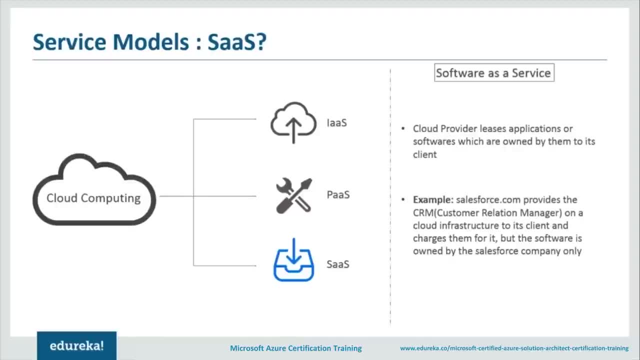 issues and all those things. everything is taken care by Google. say, for example, your Gmail is what I'm talking about. Google manages everything here, So all you have to worry about is consuming that service. Now, this model is known as software, as a service. that is S AAS. 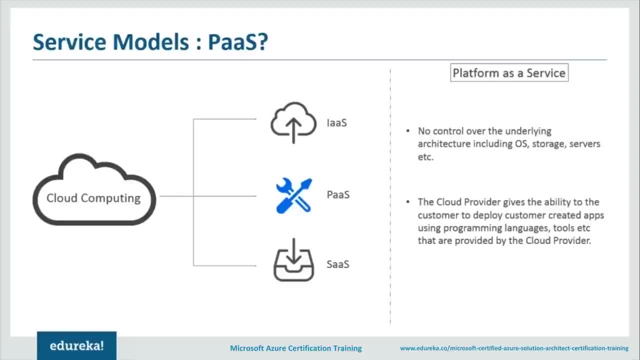 Next, we have pass, that is, platform as a service. Now, here you are, provided with a platform where you can actually go ahead and build your own applications. to give you an example, We have our Google App Engine. Now, when you talk about Google App Engine, 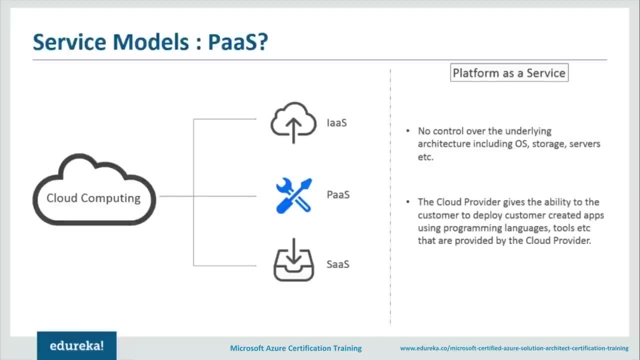 what you can do is you can go ahead and you can create your own applications and you can put it on Google App Engine so that others can use it as well. So, in short, you are using that platform to create your own applications. And, lastly, we have IAS, that is, infrastructure as a service. 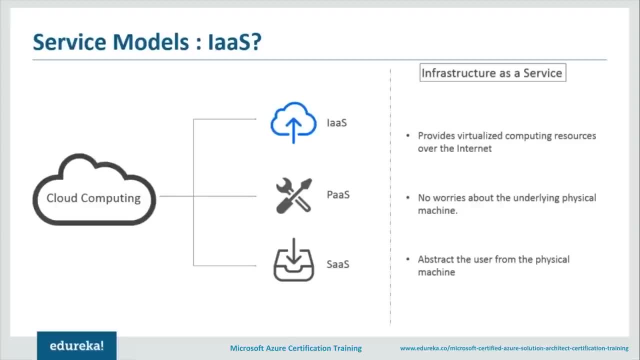 Now, what do I mean by this? Well, the whole infrastructure is product to you, so that you can go ahead and create your own applications. that is, an underlying structure is given to you based on that, So you can go ahead and choose your operating systems. 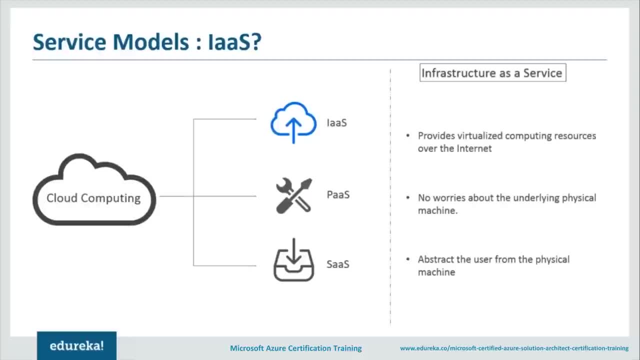 the kind of technology you want to use on that platform, the applications you want to build and all those things. So that is what an IAS is: infrastructure as a service, basically. So these were the different models that I wanted to talk about. So let us move further and discuss the next topic. 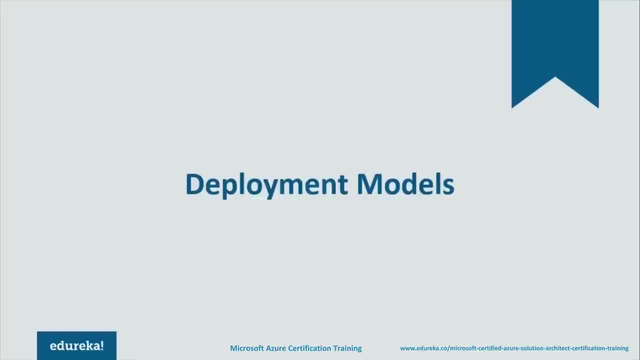 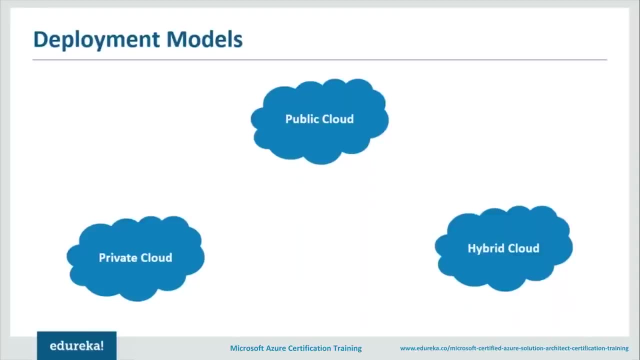 that is, the different deployment models that are there. Now, when you talk about deployment models, you can also call them as different types of clouds that are there in the market. We have these three types, that is, your public cloud, Your private cloud and your hybrid cloud. 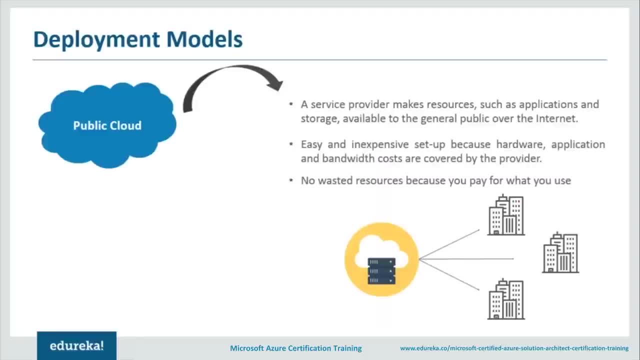 Let us try to understand these one by one now. as the name suggests- the public cloud- It's available to everyone. you have a service provider who makes these services or these resources available to people worldwide through the internet. It is an easy and very inexpensive way of dealing. 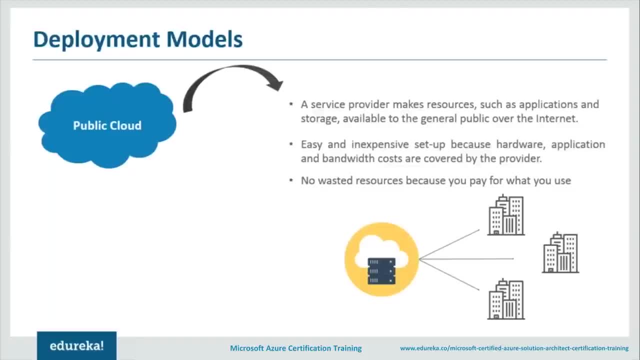 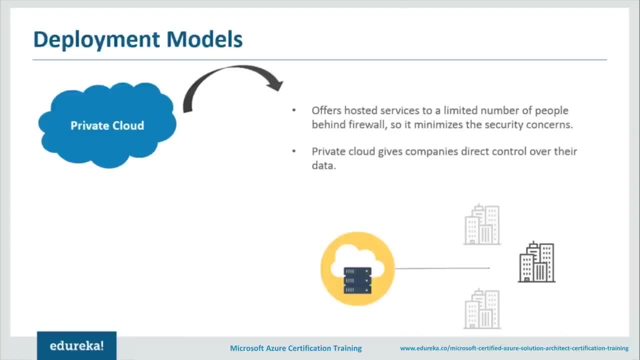 with the situation, because all you have to do is you have to go ahead and rent this cloud and you're good to use and it is available publicly. next We have the private cloud. now this is a little different. here, you are provided with this service. 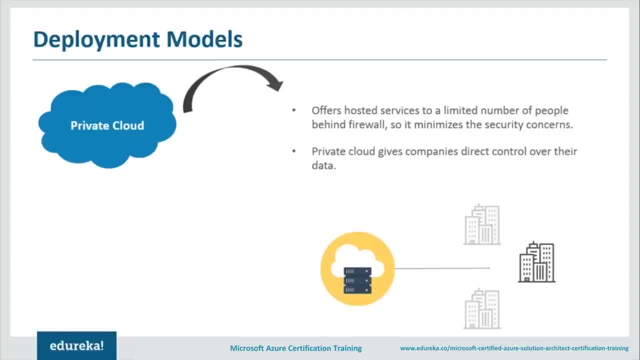 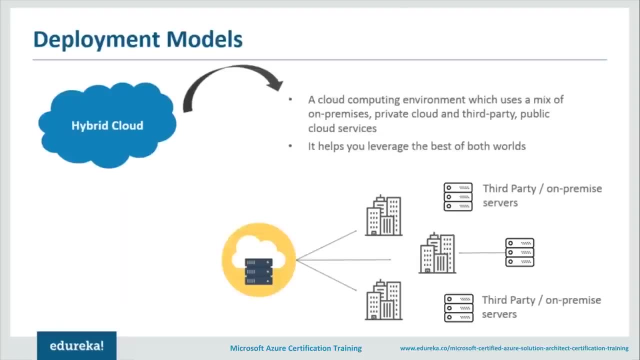 and you can actually go ahead and create your own applications. and since it's a private cloud, you are protected by a firewall and you do not have to worry about various other issues that are there at hand. and next we have our hybrid cloud. Now it is a combination of your private cloud. 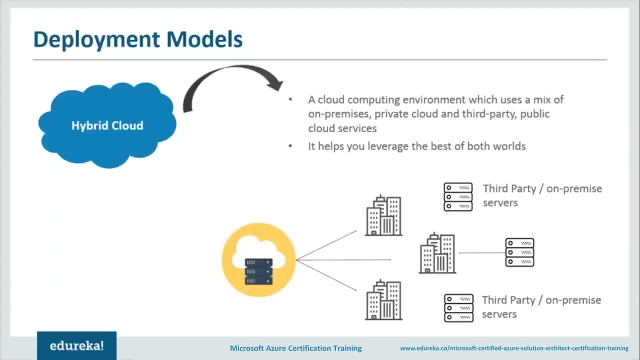 and your public cloud say, for example, you can go ahead and build your applications privately, You can use them, you can consume them, You can use them efficiently. when you sense that peak in your traffic, you can actually move it to the public, that is, you can move it to the public cloud. 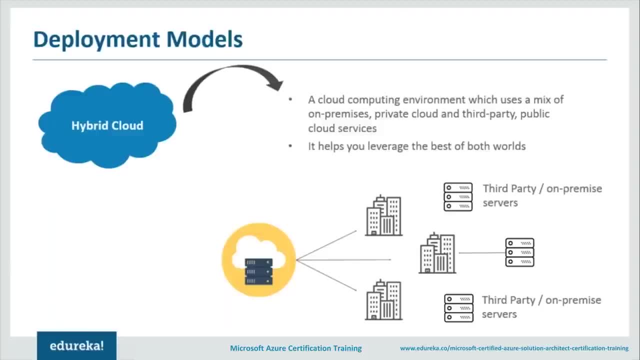 and even others can have access to it and they can use it. So these are the three basic deployment models that are there for your exposure, or your usage, rather, and you can go ahead and use those as well. I hope this was clear to all of you. 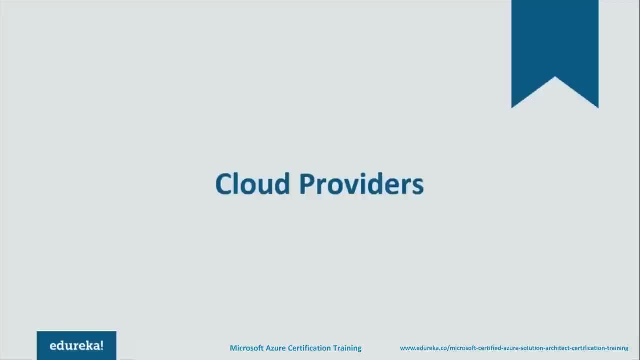 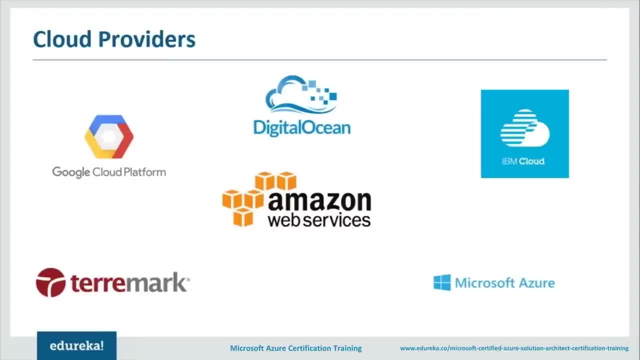 So let us move further and try to understand the next topic, that is, different cloud providers that are there in the market. Now, as I've mentioned, what happened was, since cloud came into existence, quite a few people went ahead and they bought their own infrastructure, and now they rent these services to other people. 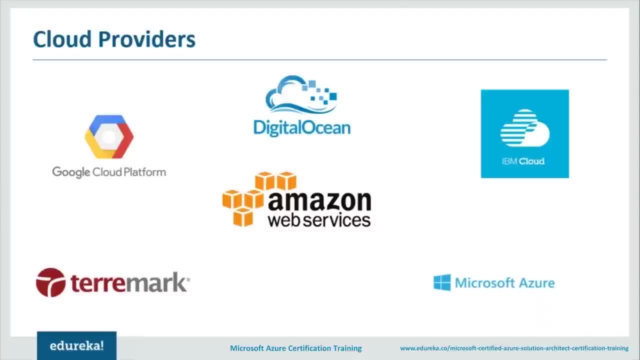 and when you talk about this infrastructure, they're quite a few people out there who are actually providing these cloud services to different people across the globe. Now, when you talk about these cloud providers, the first thing that should come to your mind is Amazon Web Services. 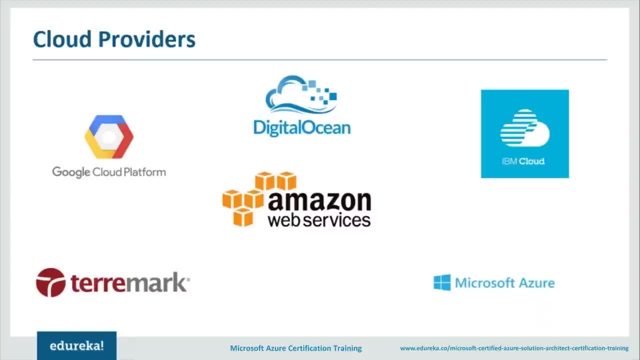 because it is highly popular and it leaves other cloud providers way behind. the reason I'm saying this is the numbers that talk about Amazon Web Services. to give you an example, If you talk about its compute capacity, it is six times larger than all the other service providers that are there. 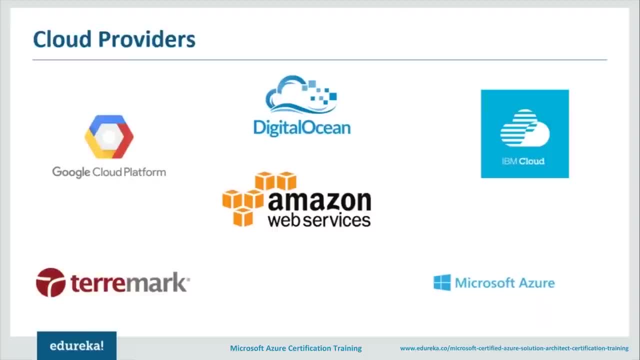 in the market. say, for example, if you talk about the other service providers in the market, if their compute capacity combined was X, Amazon Web Services alone gives you a capacity of 6x, which is huge. apart from that, it's flexible pricing and various other reasons that has the services it provides. 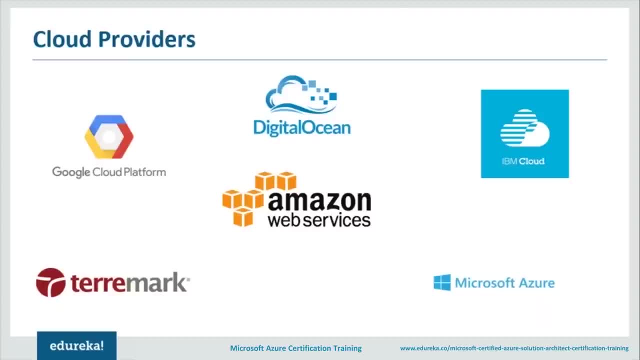 and all those things, it is rightly a global leader and the fact that it had a head start- that is, it started way before many of the services that are there in the market. it actually gained popularity And now we see quite a few organizations going ahead and using Amazon Web Services. apart from that, 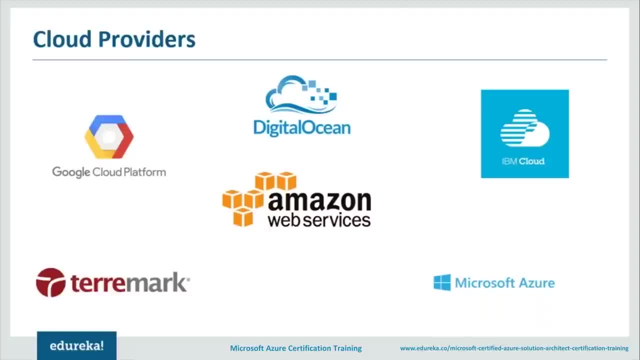 We have Microsoft Azure, which is a Microsoft product, and we all know that when Microsoft decides to do something, they expect that they kill all the competition that is there in the market. It is still not in terms with Amazon Web Services or few other service providers that are there in the market. 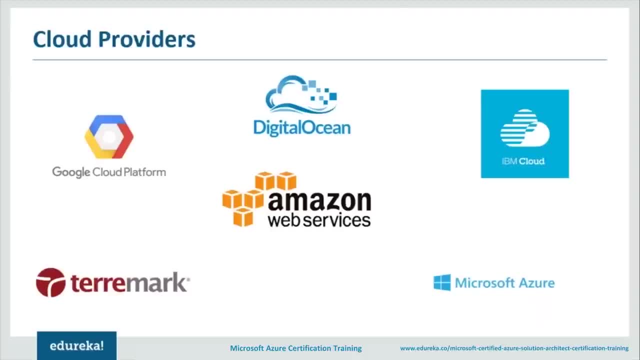 but not very neck-to-neck, but it is probably the second best when you talk about Amazon Web Services or the cloud service providers in the market. So, yep, it has a lot of catching up to do when you compare it with Amazon Web Services. 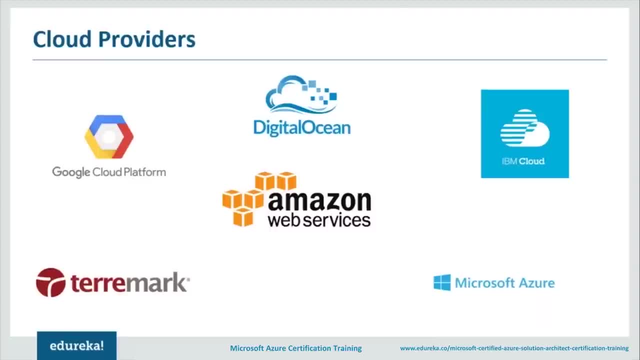 but it is still a very good cloud service provider that is there in the market. Then we have something called as Google Cloud Platform, again a very good cloud provider in the market. Now, why am I saying this? We all know the infrastructure that Google has to offer to you. 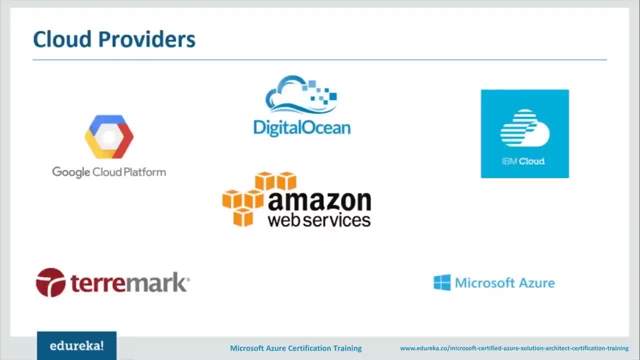 It is one of the best search engine that is there in the market and the amount of data they deal with every day is huge. So they are the Pioneers when you talk about big data and all those things, and they know how to actually handle this amount of data. 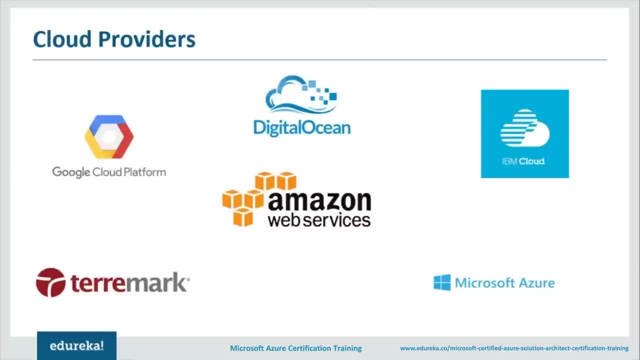 And how to have an infrastructure that is very good. That is why they have a very good facility and that leads to it being one of the cheapest service providers in the market. Yes, there are certain features that GCP offers which are better even than Amazon Web Services. 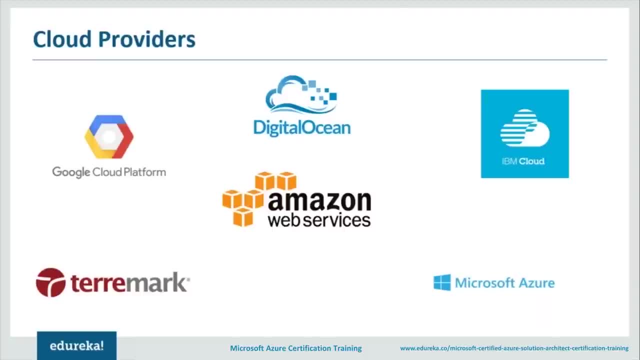 when you talk about its pricing, and the reason for it is it has various other services that are there. What it does is it helps you optimize various costs, how it uses analytics and various other ways by which it can optimize the amount of power you use, and that leads to less usage of power. 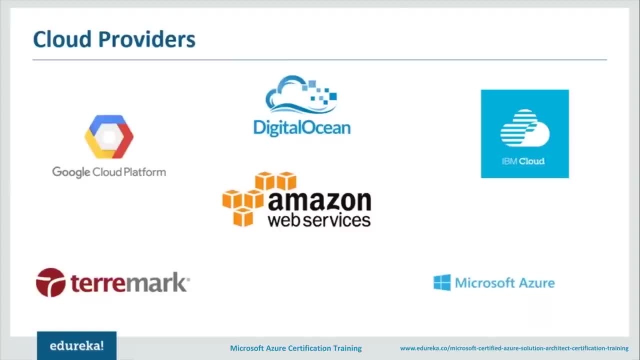 And since you are paying less for power- that is, providers are paying less for power- You end up paying less for your services as well. So that is why it is so cost efficient. Then the other service providers, that is, we have distillation, We have to remark. we have IBM, which is again very popular. 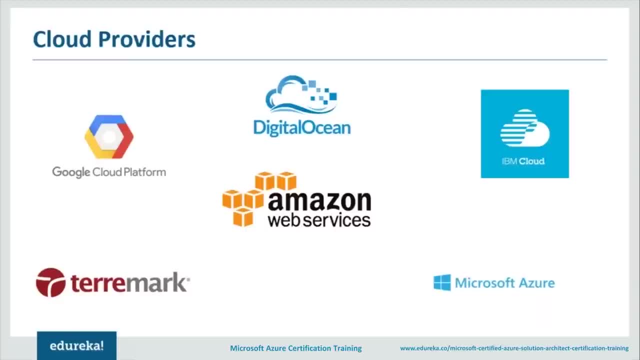 but that is a discussion for some other time. as far as these service providers go, These are the major ones that, as we have Amazon Web Services, We have Microsoft Azure, We have GCP, which are talked about a lot. This was about the basic lot riders. 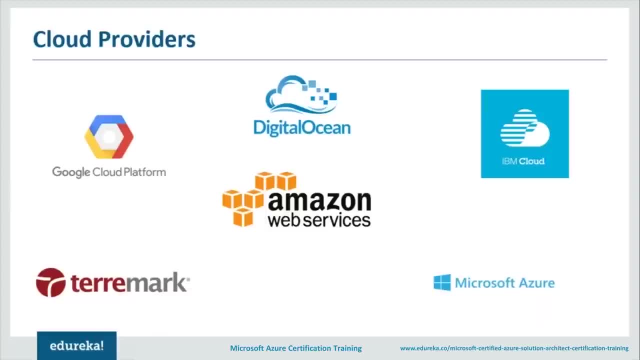 and the basic intro which I wanted you all to have. I hope you all are clear with whatever conscious we've discussed in time. So let us move further and switch into the demo part. Let us try to explore few of these services or cloud providers, as Natalie is the introductory part. 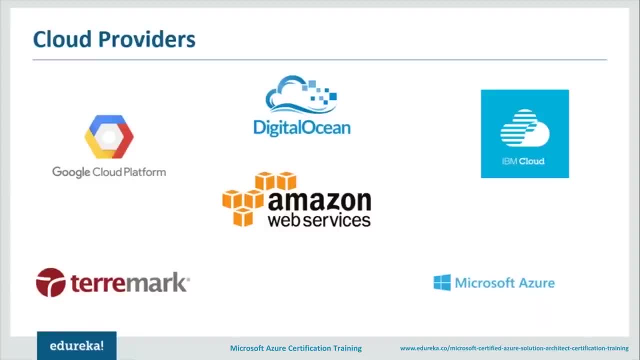 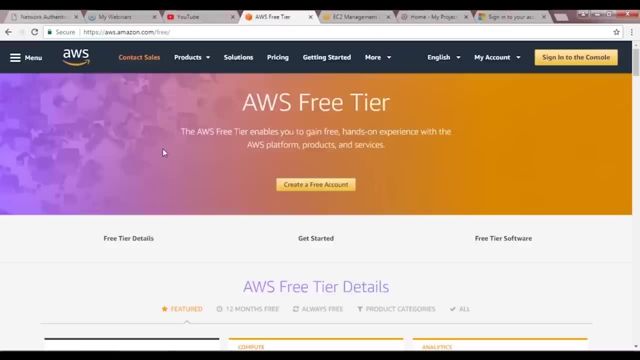 Okay, guys, what I'm going to do is I'm going to switch into the console, basically, where we can take a look at these services one by one. So, yes, guys, what I've done is I've gone ahead and I've logged into my AWS account. now, AWS provides. 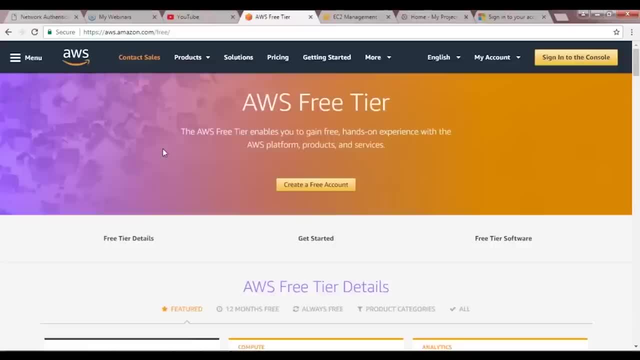 you with a free tier, and then they have their paid services as well. Let's discuss these one by one. first I would talk about AWS, then I would talk about GCP and to some extent I would also discuss a juror as well. but let's focus on AWS for first. one point: 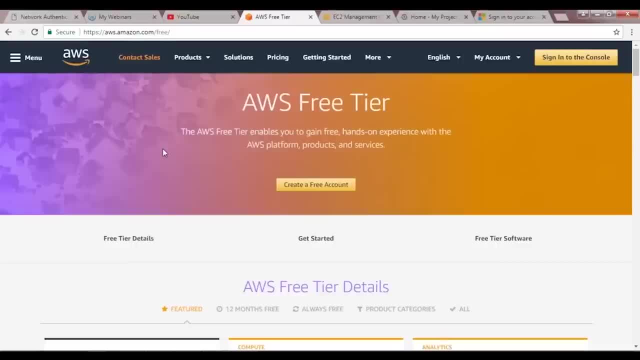 which I did not mention while going through the concepts was: AWS provides you with a free tier. Now, when I say a free tier, this is where you do not have to pay any upfront money. You can actually go ahead and have access to AWS services. 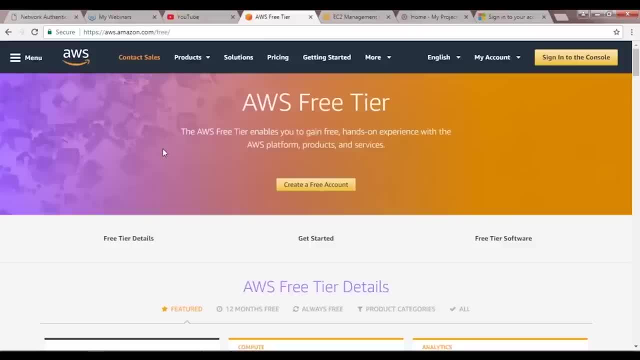 and see how they work, And once you are confident and comfortable with them, you can actually go ahead and decide whether you want to buy those services or not. So yes, these services are made available to you for free for one complete year. Yes, there are certain restrictions on it. 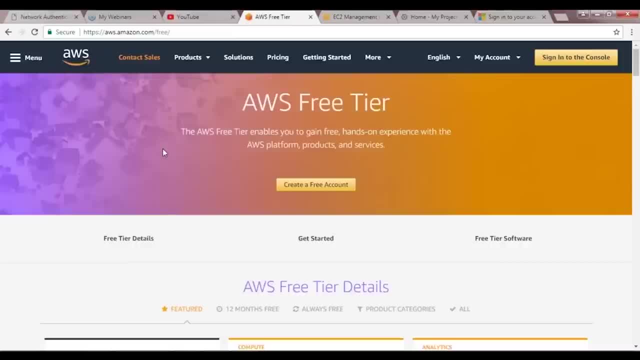 But as long as you stay in those restrictions, you won't be charged anything. if you cross those restrictions, Yes, AWS will charge you. Now how does AWS do that? Well, when you create an account, you have to give in your credit card details or debit card details. 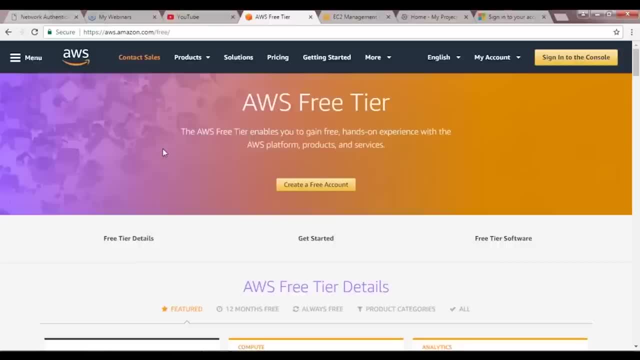 when you do that, AWS will cut a lump sum amount from your account, verify your account and reinstate that amount back into your account so that none of your money is used, but just a verification is done that this is your valid credit card or your debit card. 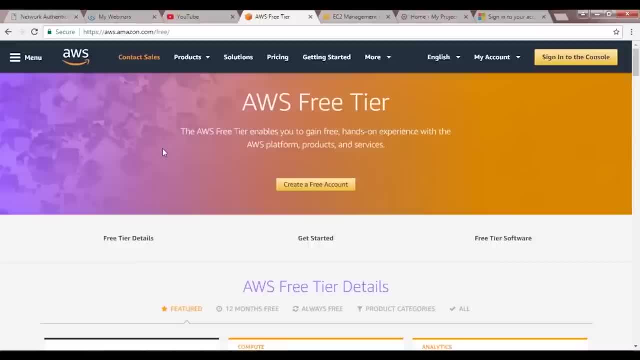 and once your 12-month free trial expires, then they would notify you that your free trial is over. Would you want to go ahead and continue using our services? If you say yes, then they would charge you. Meanwhile, they won't charge you. 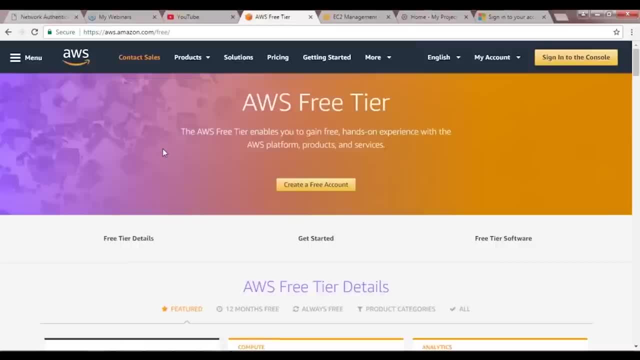 so you can stay relaxed and you can actually go ahead and give your credit card or debit card details. but just make sure that you set an alarm and, once your free trial gets over, you kind of either revoke your access or go ahead and continue with the paid services that AWS has to offer. 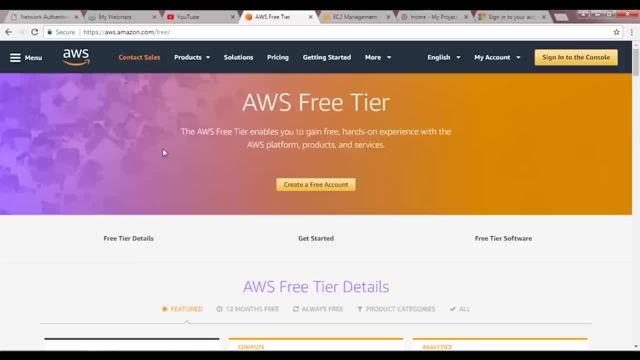 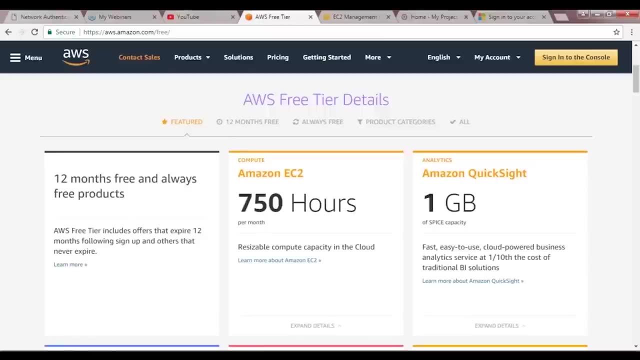 to you. So what does this free tier has to offer to you Basically? let's take a look at those. Well, firstly, we have compute services. when you talk about AWS, and to name a few, we have easy to. we have Lambda, which are popular services. now, easy to is something. 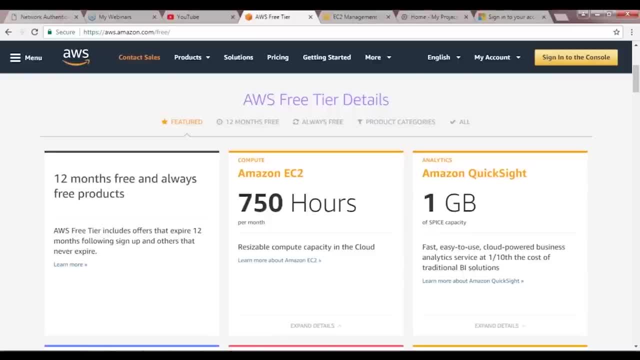 like a raw server where you can actually go ahead and host your websites and applications. It is very popular And if you want to use it, AWS gives you 750 hours per month for free. then you have some service called as Amazon quick set, which is basically an analytics service. 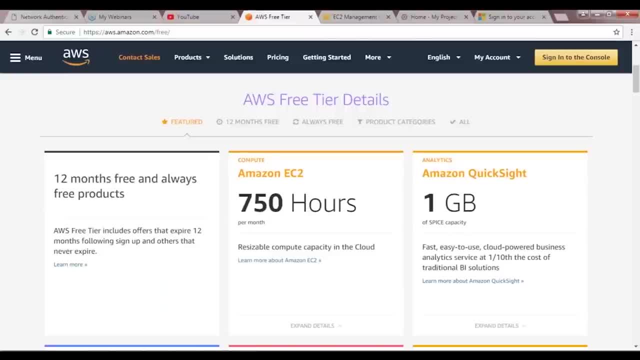 and I won't get into the details of what it does basically, but you have a space of 1gb available to you. That is nothing but spice capacity Basically. again, I won't get into the details because I want to stick to the surface as far. 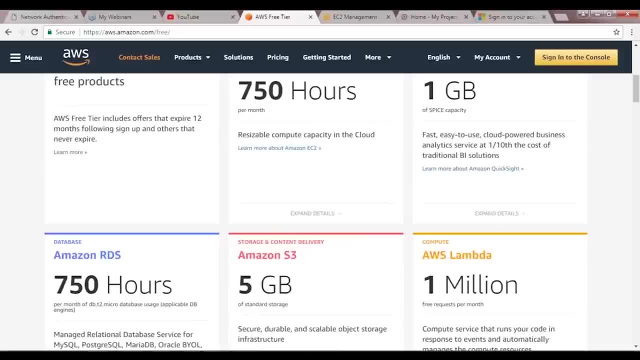 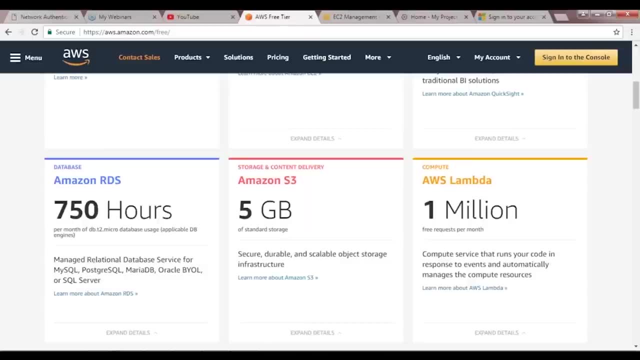 as this session goes. then you have other services, like your database service, which is an RDS. You have your storage service, which is s3, Amazon Lambda. Now, Lambda is another compute service which is similar to your easy to, but easy to is more. 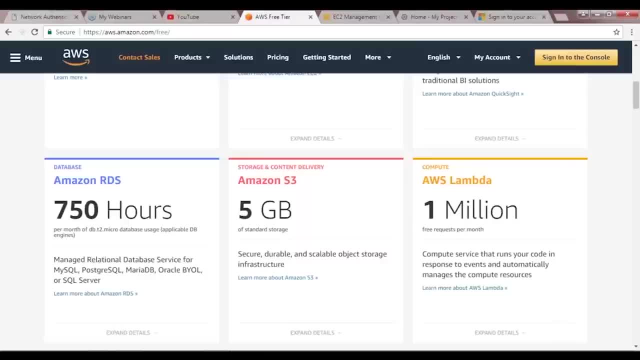 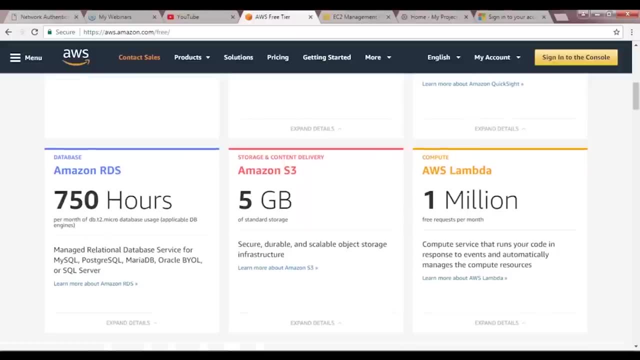 of a place where you can host a website It's, whereas Lambda does not let you host your websites. But yes, you can definitely go ahead and do a lot of background application work when you talk about AWS Lambda. apart from that, AWS also provides with various videos. 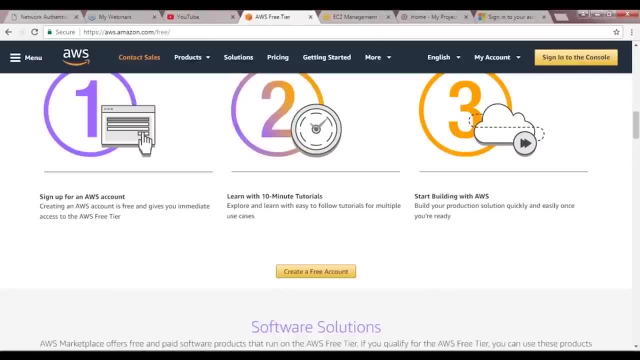 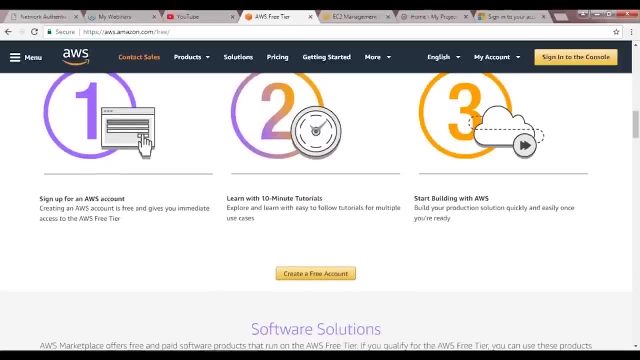 that talk about? how do you want to go ahead and get started with using these services, how to create an account, how to create instances and all those things? So this was about the free tier. Let us end up move further and see how the console looks like. 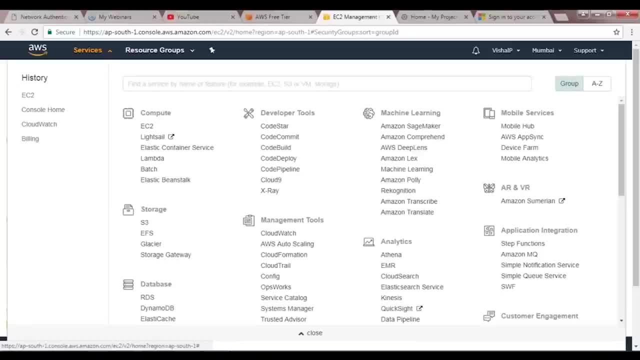 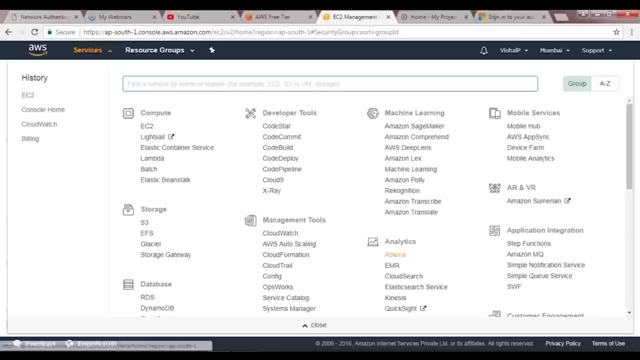 You can actually go ahead and create your own instances. You can do a lot of things. So this is what the different services that a device has to offer to you. You have your compute services, developer tools, machine learning, and I'll text your storage database services. 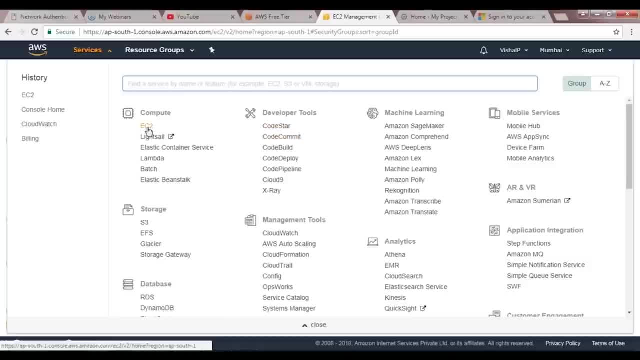 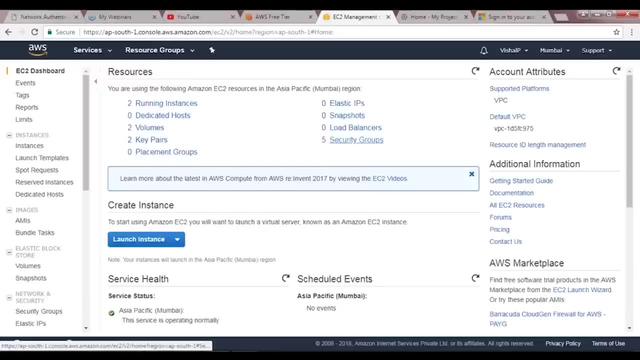 You can actually go ahead and use these on your own. You can go ahead and create certain instances here. Now, once you click here on easy to you get to see the number of instances that are active, the security groups that are there, the key pairs that you have. 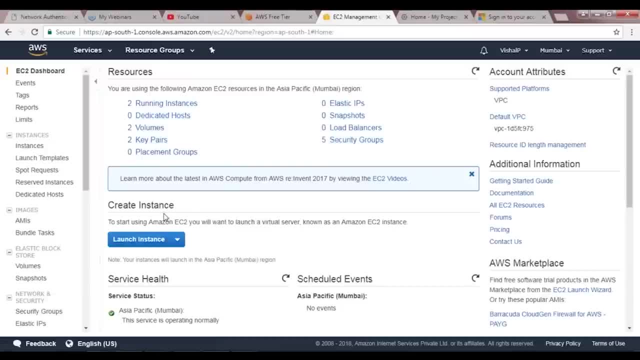 Let us see, or take a look at, an instance. Basically, I would tell you how to create one. I won't create one myself because I have certain ones running already. I would just walk you through how the process works when you click on that launch instance. 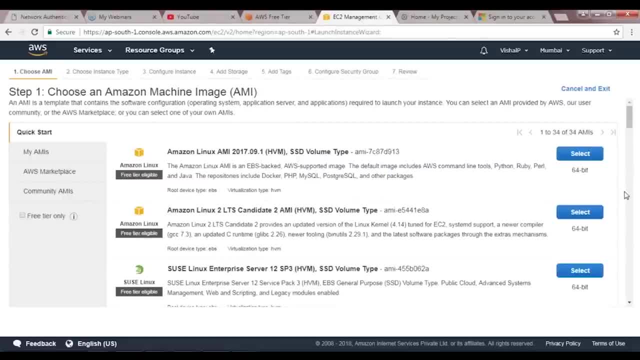 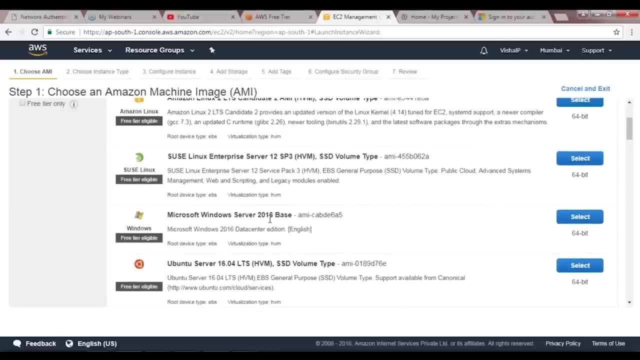 it will give you options, as: in what kind of an instance Do you want to create so you can actually go ahead and pick the one that suits your need, based on the OS you're using and stuff like that. Since I'm using a Windows OS, I'll be picking one for Windows. 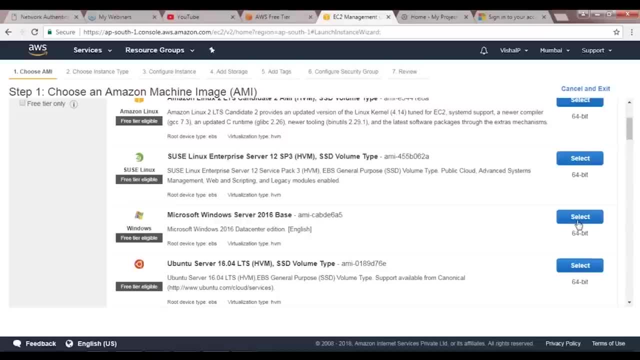 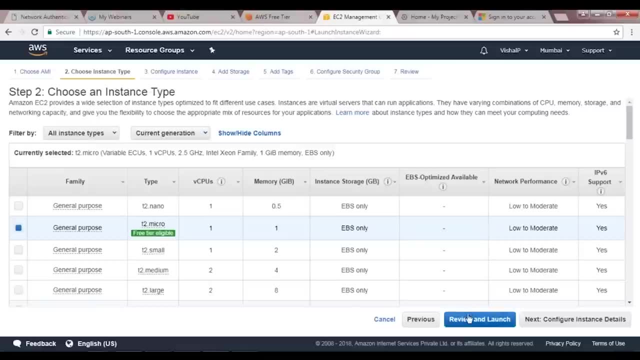 and I would be using the one that is freely available to me or eligible for my free tier. So when I say select, I see that a free tier, eligible t2 micro instance is available to me. I can either click on this and directly go to the final step of creation. 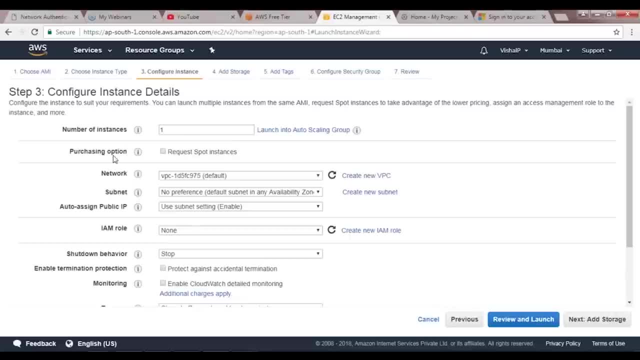 or I can take a step-by-step approach, that is, if I want to modify it, I can go ahead and given these details, as in the number of instances, my purchasing options, Network subnet, or to assign public IP and all those things. So let's click on next and we can also put in these details. 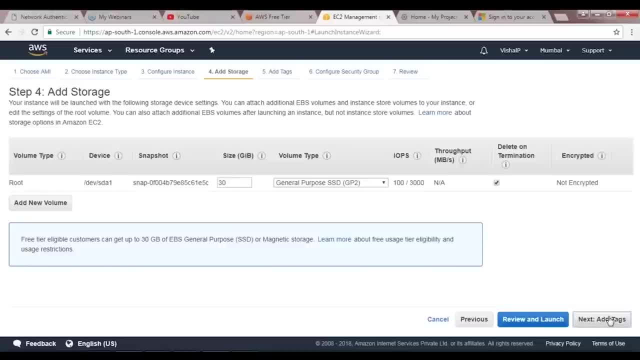 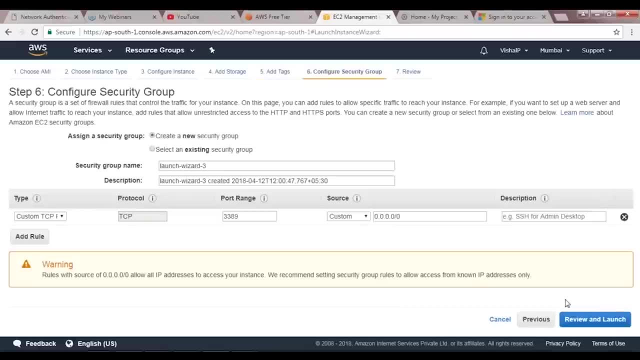 but I'm going to stick to the default decisions or the selections. you can also go ahead and configure your security groups. I would talk about that as well, Do not worry. And finally, it would say: do you want to review and launch it? Once you click on this, you would have a new instance. 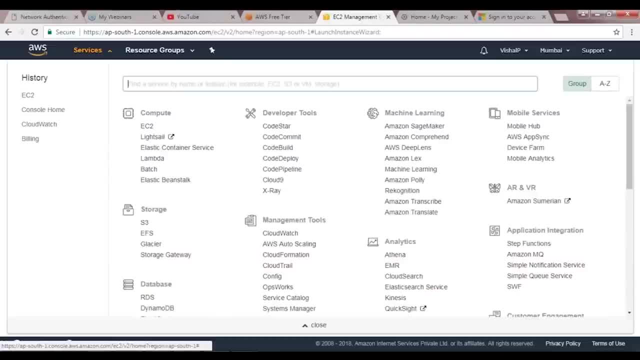 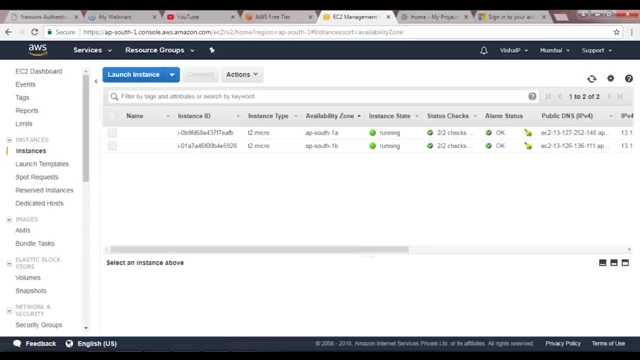 There would be couple of statistics and you would have your instance available for use. to give you an example, Take a look at this. as you can see, I have two instances running and the security checks are done, and I can actually go ahead and do a lot of things with it. 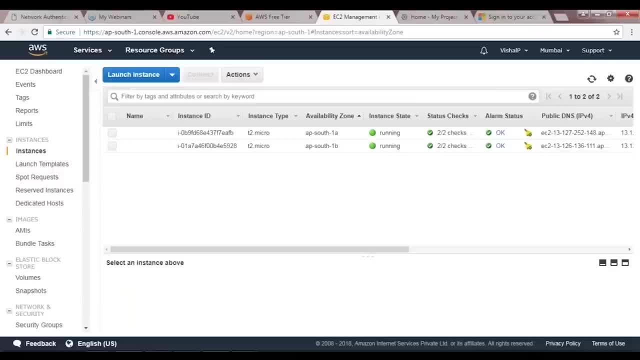 I can actually go ahead. I can connect to a server, I can have my security group, security policies and, when you have an instance, you can do so many things: hosting a website and the other things that are there now. I just mentioned key pair values and I mentioned security groups. 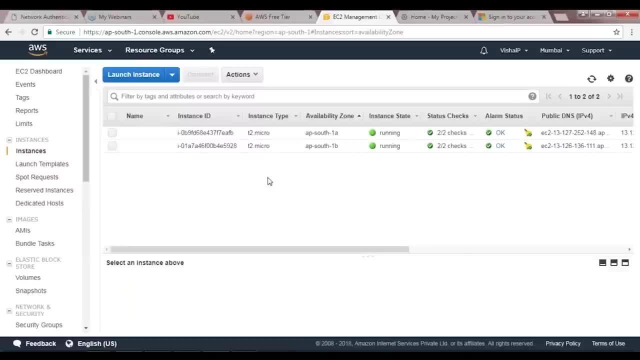 Now, when you talk about the key pair, it is nothing but an authentication process that lets you use your instance. It is a verification process. Basically, it varies when you talk about using it on your Linux and using it on your Windows. Windows, you would need it. 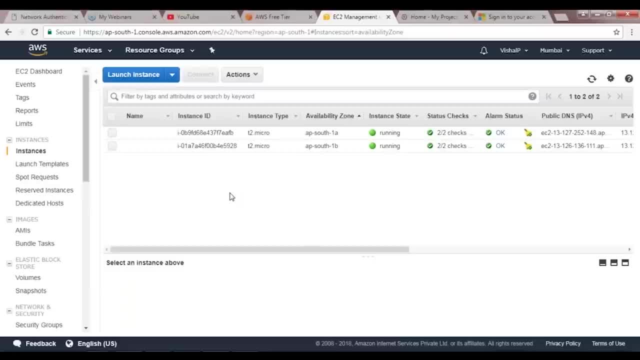 for an external login, as far as when you talk about Linux, you'll have to go ahead into your terminal and generate those SSH or your secured server keys, basically, or secured cell keys, rather- and then log into your website and then go ahead and use it on your server, basically. 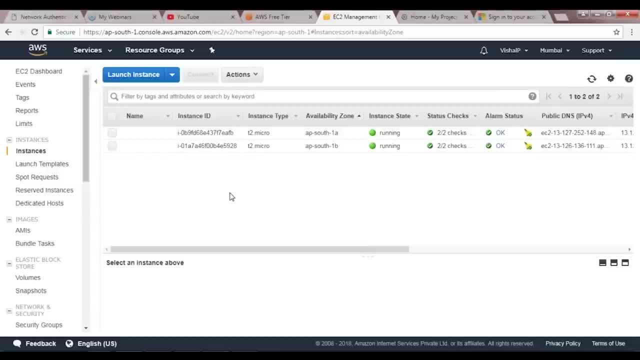 So this is what happens. So that is something called as a key pair value. when you talk about AWS, a key pair value, once created, it is unanimous, or it is not unanimous, or that it is primary to a particular instance, and you should not lose it because if you do, that instance becomes useless for you. 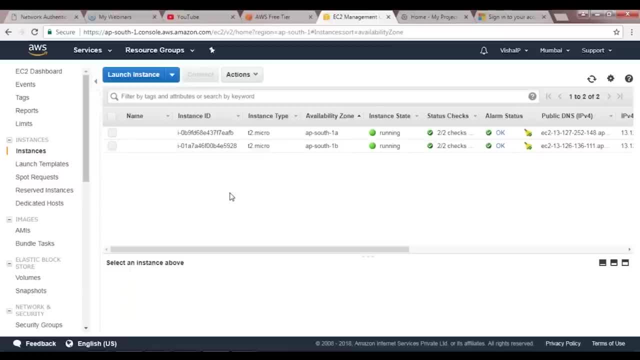 So you have to make sure that once you create a key value pair, that key value pair, it stays with you And when you do try to connect to a server, that key pair value or its value is available with you so that, basically, you can switch to your server and connect to it. 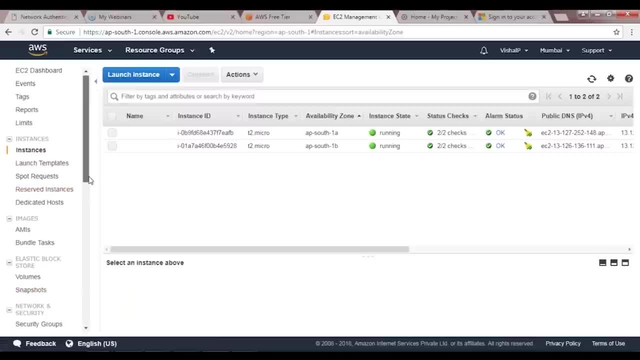 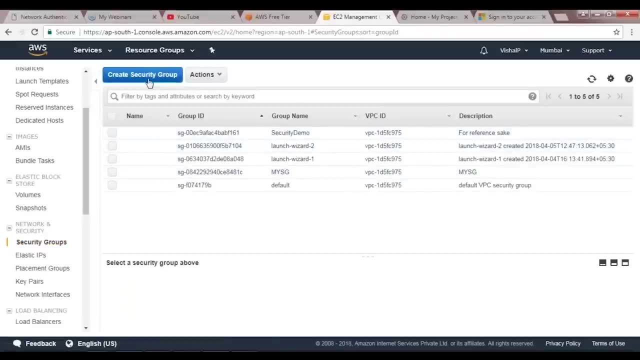 And then you have something called as your security groups as well. Now, if you come down here, you can go ahead and set in your security group policies, whatever those are. you can create a new security group and you can just go ahead and add rules. 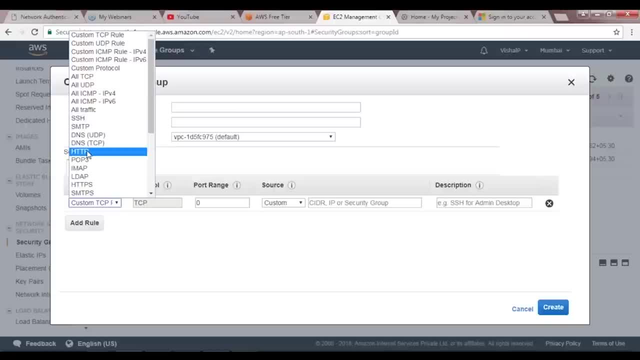 as in what kind of security policies you want. Say, for example, you have your HTTP, HTTP, PS. Now, if you're using Windows, you'd be needing RDP and those kinds of rules. you can go ahead and select a source you want to and accordingly, you can set in your security rules. 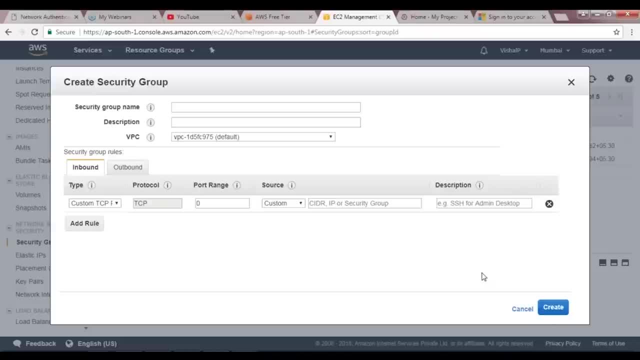 Once you create on- click on create- you'd be having your security group up and running for you and you can like stay assured that your so-called services are more than secure here. So yeah, this was about Amazon Web Services and how its interface looks like. then you have something called. 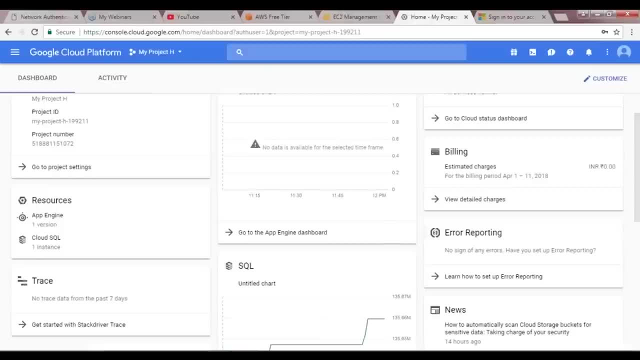 as your GCP. now, GCP 2 has a free tier. The only difference is GCP gives you an, a balance amount, as in say, some amount of US dollars, and you can. the services are paid services, but you can use this balance to go ahead and use those services. 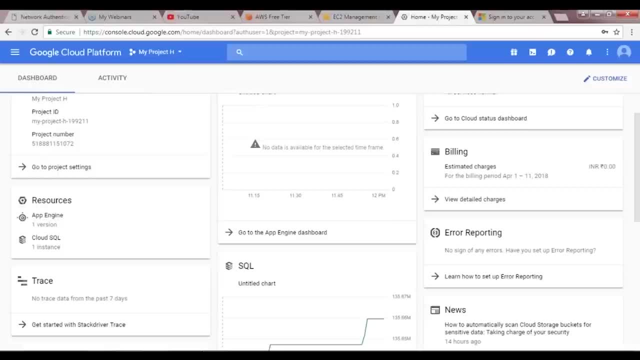 So it pans out to similar approach which AWS takes in. but if you talk about their pricing, AWS charges you on Ali basis, whereas your Google Cloud platform charges you on second basis, So it is more affordable. say, for example, you stop using a particular instance at two minutes. 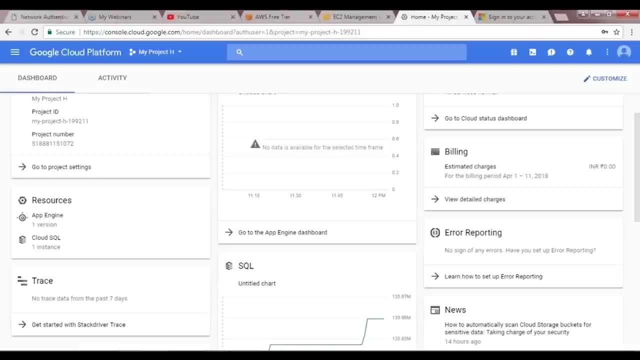 You'd be charged only for those two minutes. But if you stop using an instance for two minutes in AWS, you'd be charged for a complete hour. So that is the difference between the two. as far as logging in is concerned, again, you'll be going ahead and giving in your credit card details here. 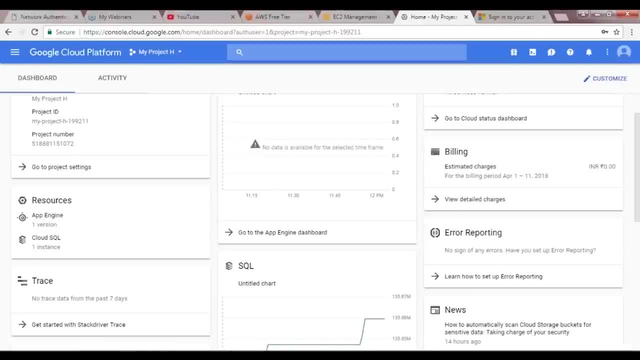 as well the differences. here You have to make sure that you do not enable your billing, because once you do that, trust me, you're going to end up paying a lot of money, because I accidentally left few instances open the last time I logged in and I was charged heftily without me being noticed. 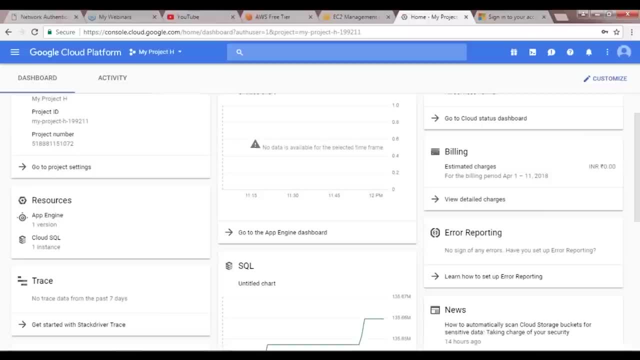 So when you see a button there saying that enable billing, make sure that you use it carefully, because you do not want to be charged for something that you are not using. So when you talk about GCP, this is how the interface looks like. you have all the services. 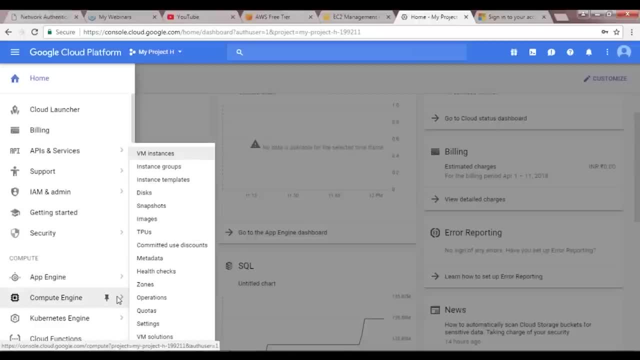 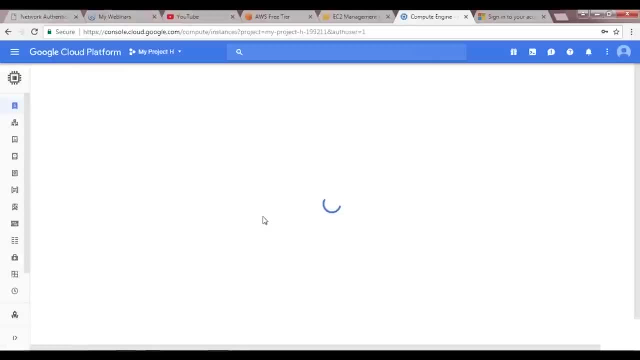 here as well. there, If you had your compute services, you have your compute engine, basically, and you can to come here and create your instances. You can click here and you can go ahead and go through the process of creating your instances, but I won't be creating an instance as far as your GCP is concerned. 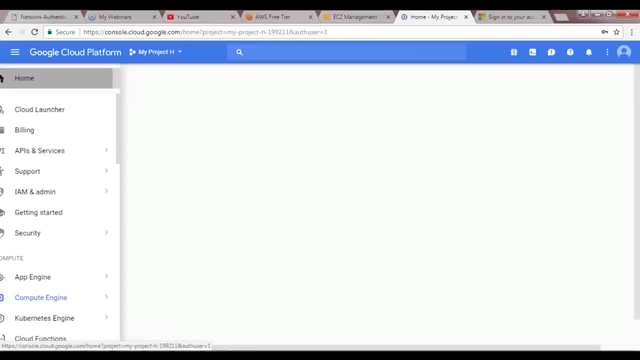 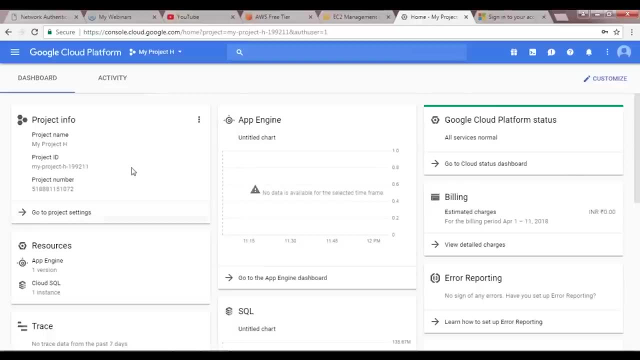 because I've given you a reason already. I'm happy working with AWS for now. This is your dashboard, where you get in all the information as in whatever is happening as far as your account is concerned. So this is one of the accounts managed by a person. 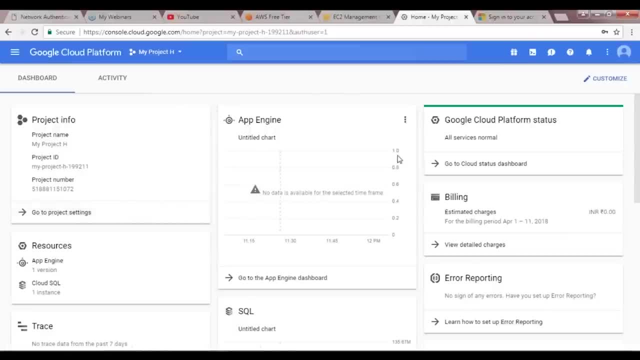 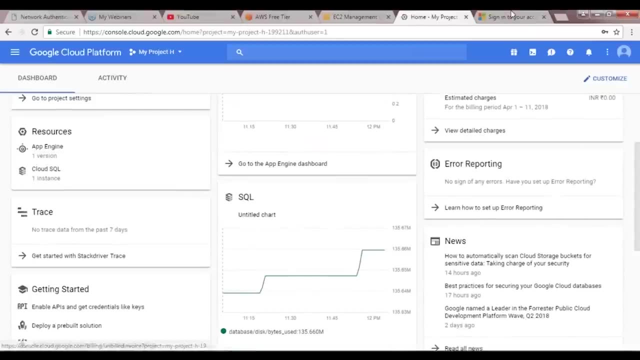 I know who works with me and the certain projects which he has gone ahead and created. So it's the information for those details, or the details for that projects, basically, and then you have something called as your Microsoft Azure. Now, I won't log in and get into the details. 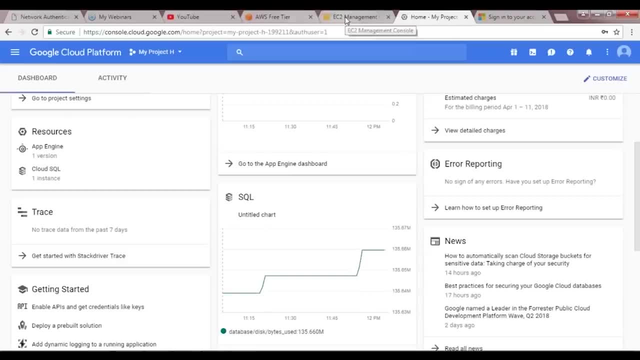 But, yeah, it to provides you with similar services. So, yes, this was about the different cloud traders that are there in the market, and I just wanted you all to have some understanding as in how do these things work and what do these services have to offer to you. 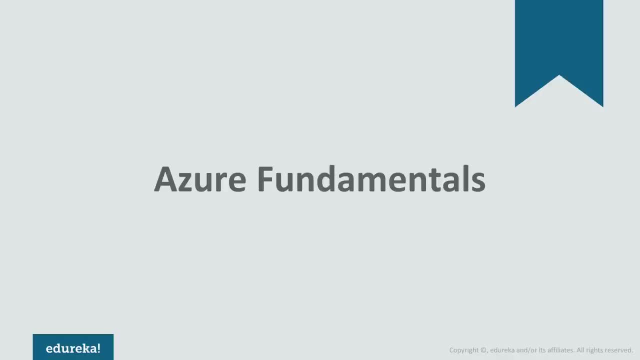 I hope this is clear to all of you. Why Microsoft Azure? Why are you guys so interested in Microsoft Azure? Now, one thing is that Microsoft Azure is actually becoming pretty big. I mean the cloud leader on papers it is AWS right now, But if you see the growth that has been happening the past few years, 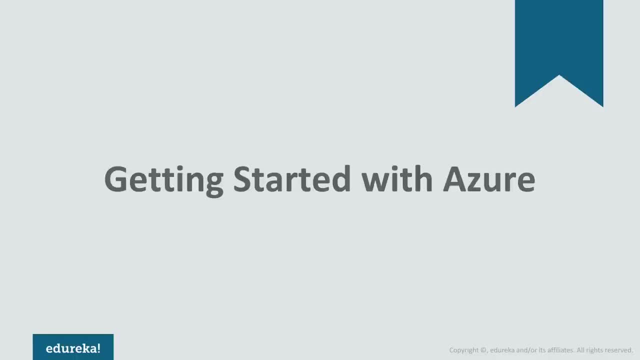 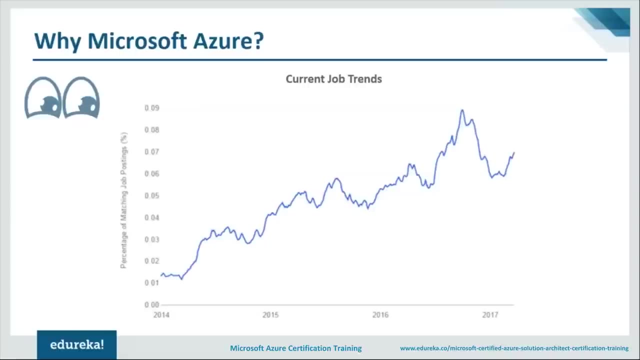 Microsoft Azure is actually coming out pretty big right. So- and that is the reason if you look at this graph, there are the job opportunities, for Azure has been on a rise and that is like. this is the primary reason that you guys want to learn about Microsoft Azure. 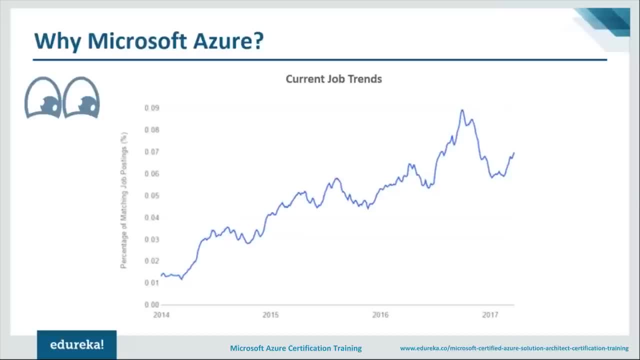 because obviously you want to make a career shift into the cloud industry, right, And for that availability of jobs should also be a factor. And if you see the graph- this graph is has actually been taken from indeedcom, right, And as you can see, the graph is rising. 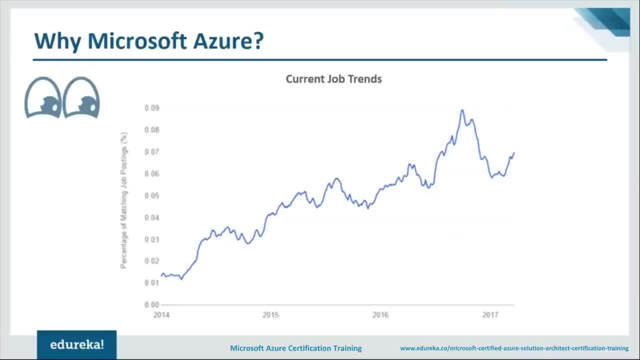 So if you see, at 2014, it was around point zero one percent in the middle Mid, in the late 2016, it's reached around point zero nine. It came down to a fall, but then again it is at a rise. 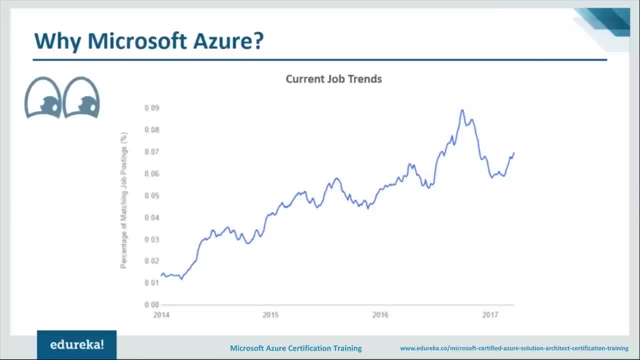 So this is a partner that you see, but if you take my advice, because I have seen the industry, as far as I know, these jobs are going to increase multiples in the future as well. right, It's not only restricted to Azure. If you talk about AWS, if you talk about any cloud technology, 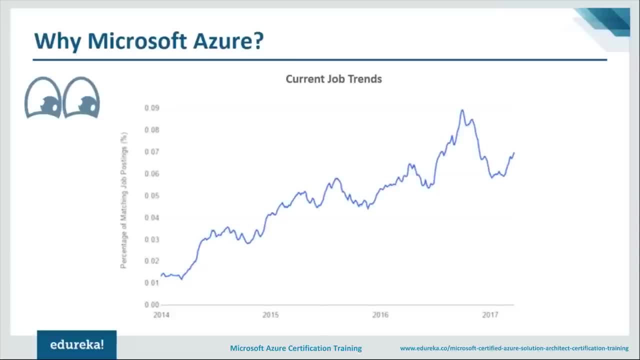 it has become imperative for you to learn about cloud, because it is the thing. everything in the next 10 or 15 years is going to be on the cloud, right? Any company which is still on its on-premise servers will move to the cloud one day or another, because that is inevitable. 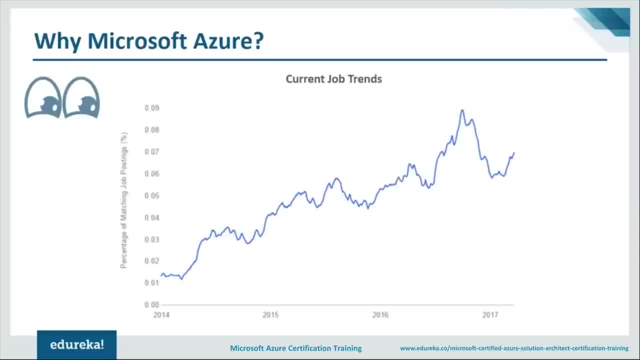 That is something that has to happen, and that is the reason it becomes very important for you guys to skill up to the cloud level right now, talking about Azure, like I said. so jobs are increasing Every day. jobs are there for you, So what needs to be done from you guys is prepare for the exam. 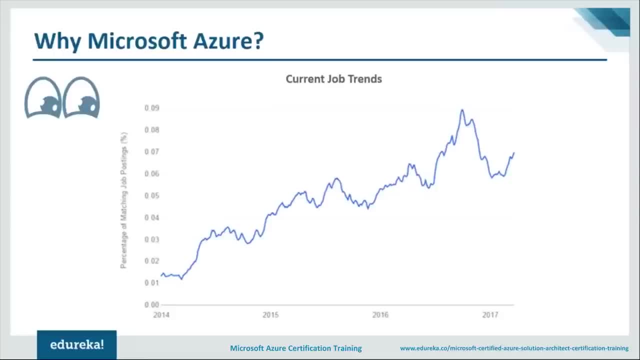 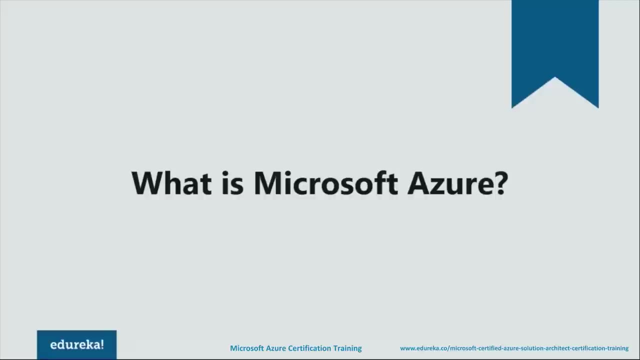 that is there for us. your give that exam, get the certification, get hands-on experience and get the job. This is the course. This is the path that you should have for taking a cloud computing role, right? having said that, so, guys, this is the reason why we learning about Microsoft Azure today. moving on, 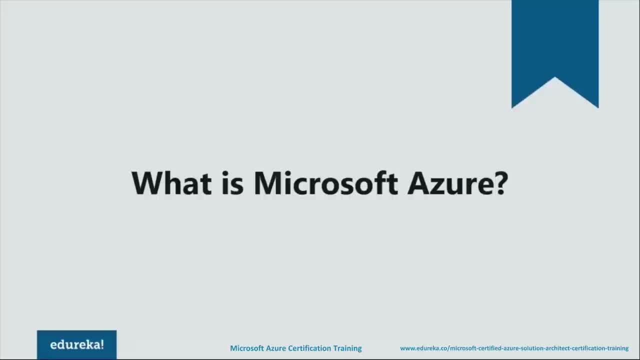 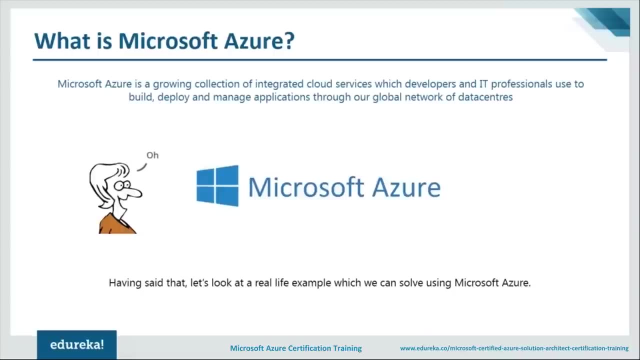 Let's understand what Microsoft Azure is exactly. So Microsoft Azure is a growing applications through Microsoft's global network of data centers. right, So, by using the Microsoft's infrastructure, you build, deploy and manage applications on the Azure environment and, like Azure- like I said, it's a cloud provider- provides you the cloud. 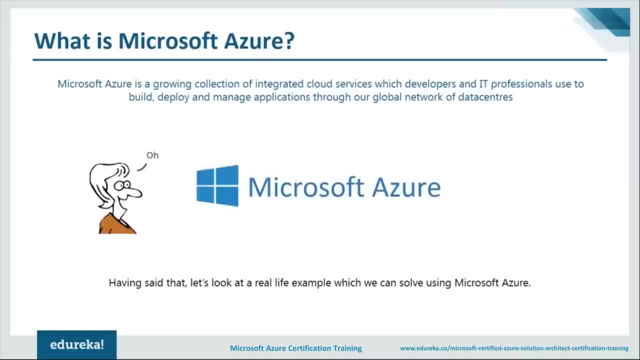 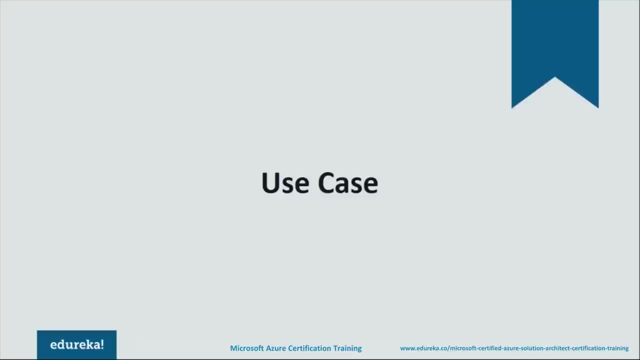 services. you are using those cloud services, but those cloud services are actually on the Microsoft's infrastructure and that is what you are paying them for. All right, So this is what Microsoft Azure is all about, guys. Now let's see a use case. now, guys. my philosophy is that, rather 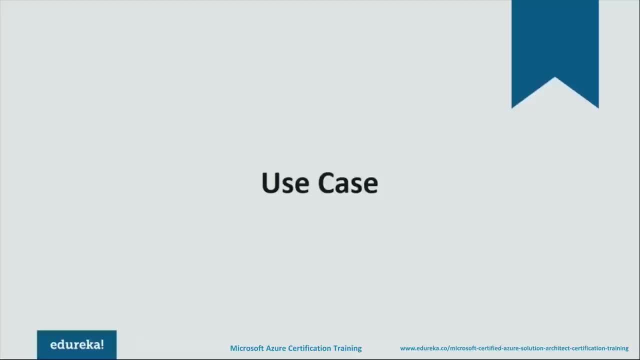 than doing all the theory first and then going on to the practical, I would like to follow the reverse approach right. I would like to begin from practicals, because that is what your exam will be based on. your exam will be based on real-life example. 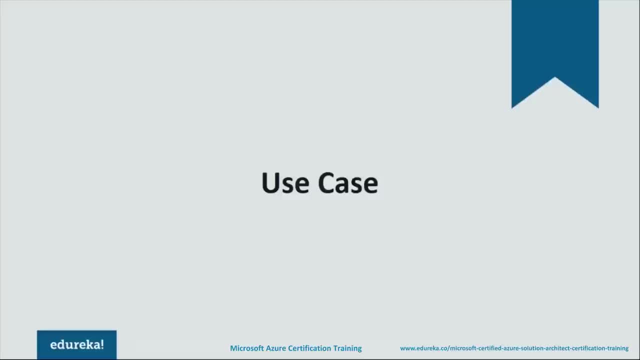 that you based on real-life scenarios. It will be based on what kind of hands-on knowledge you have in your as your domain. All right, and that is a reason every session of ours will have a use case through which we will try to analyze how we can implement. 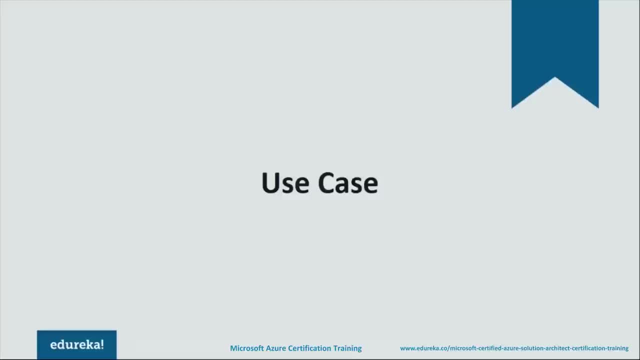 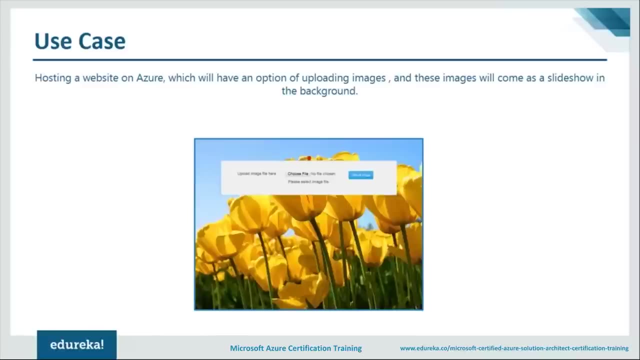 it in the cloud, right? So this is your first use case. This is kind of simple, guys, So please pay attention. So we are trying to make a website which is something like this, right? So what happens here is you have a set of images and these images 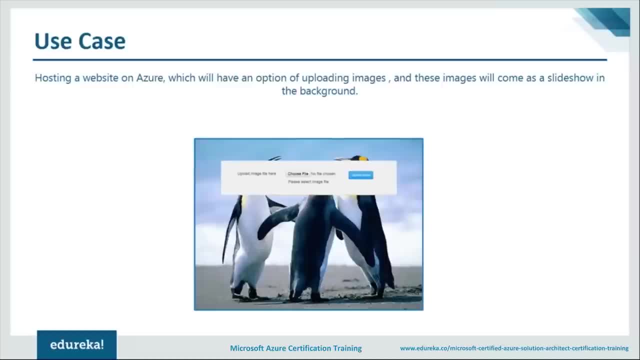 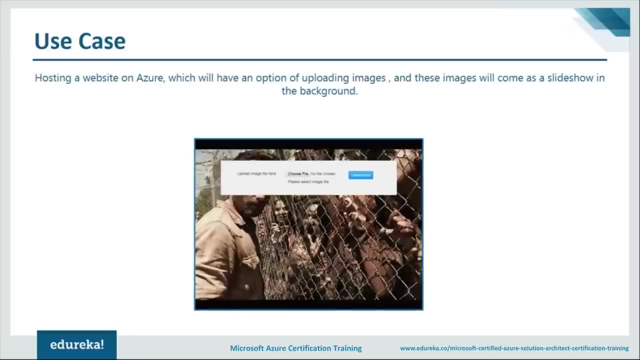 are actually being played in the background And in this website you have a functionality to upload more files to the cloud And once you do that, those files will automatically be added in the slideshow and will start running All right. So this is our use case and we have to implement it on the cloud. 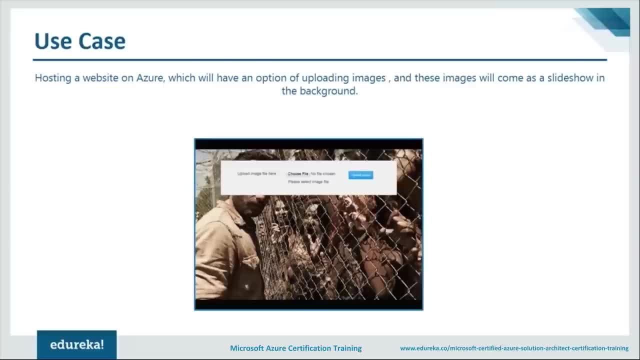 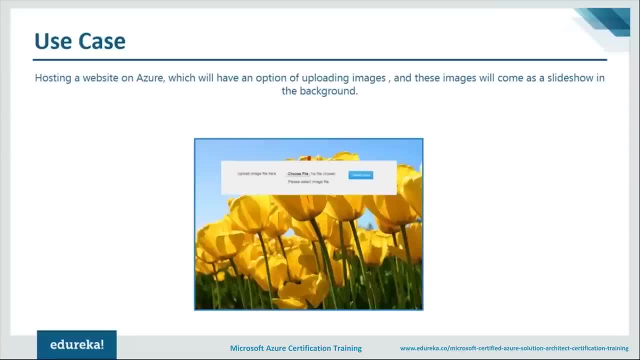 So there are two stages in the way We are going to take this use case. the first stages: We're going to apply pure logic, right, We are going to understand how we can actually deploy It on any cloud service, right? Not only Azure, but any cloud platform which is out there. 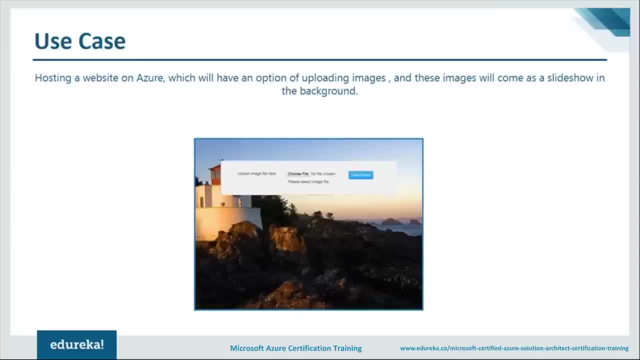 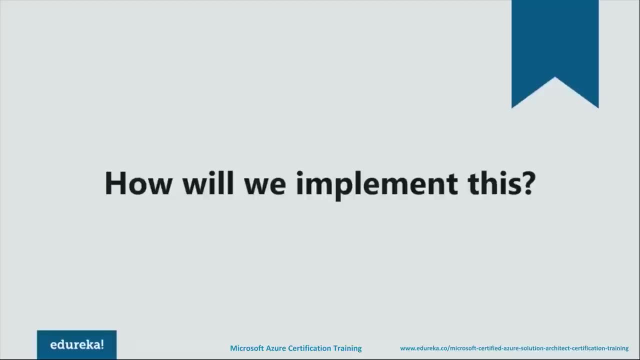 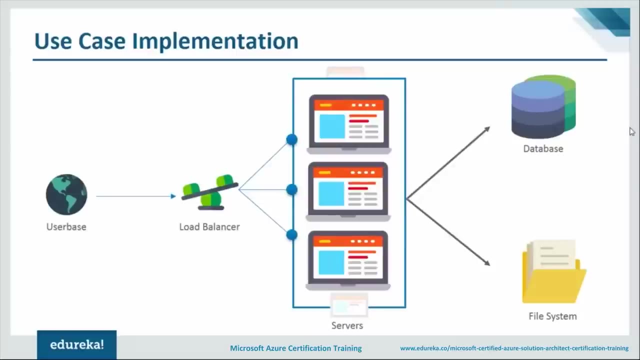 How can we implement this use case. So let's see that first, and after that, once you have understood that, we'll try implementing it in Azure. So first let's see how we will implement this in a general scenario, by pure logic. So your user base will be accessing the internet, right? 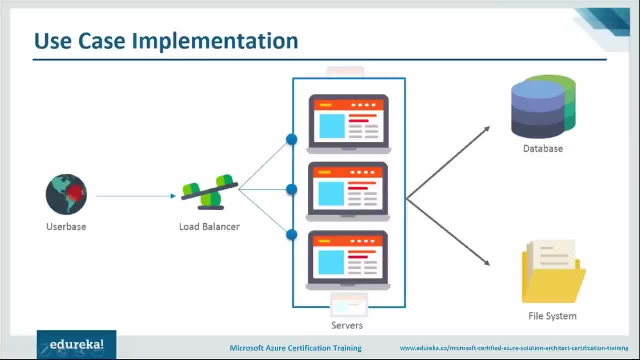 Now, when your user will try to access the website, he will enter the website name right. So all of that traffic will come at this point, which is called a load balancer. Now, what is a load balancer? A load balancer is basically a service which distributes your 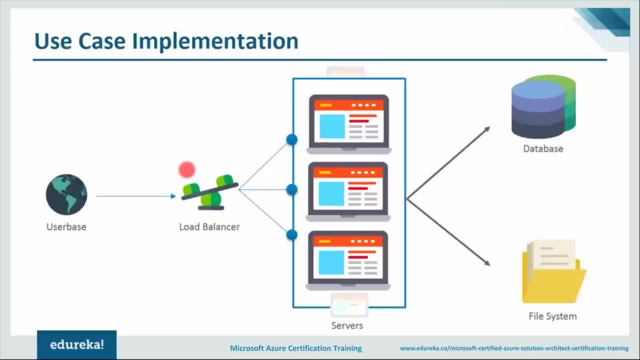 traffic equally among the servers running at that time. So say there are like five servers running or your website, then, and if traffic is coming on to your servers, that traffic will be distributed among those five servers by the load balancer. So So the job of the load balancer is to distribute the traffic equally among the servers, right? 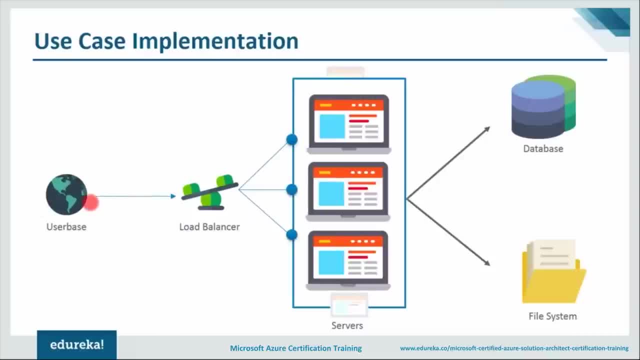 So this is what the load balancer is all about. So your user base from the internet is trying to access your website, So the traffic comes to the load balancer and the load balancer separates, or it segregates, the traffic into equal proportions and give it to the servers, right. 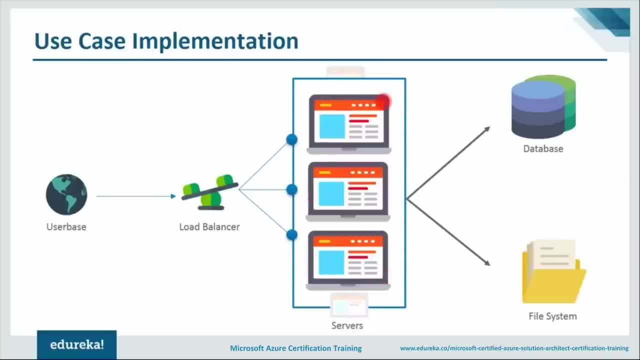 So once the traffic comes on to the servers, the servers process the request and if you talk about our website, so our photos are actually stored on a file system, right? So whatever files you are uploading or whatever files are there which are already been uploaded, 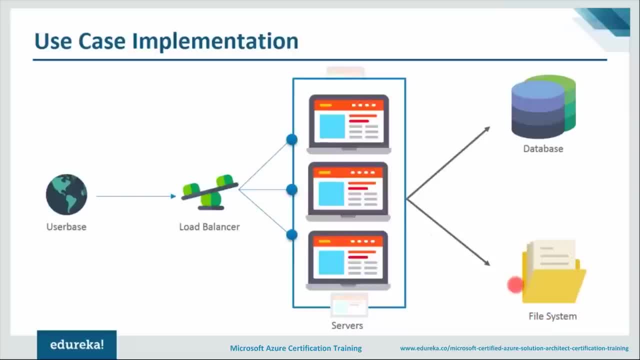 are there on a file system, right? So it will access that file system for fetching those files. But our servers, they don't know what files do we want, right? What are the like? say, for example, I upload a file and before uploading the file there, 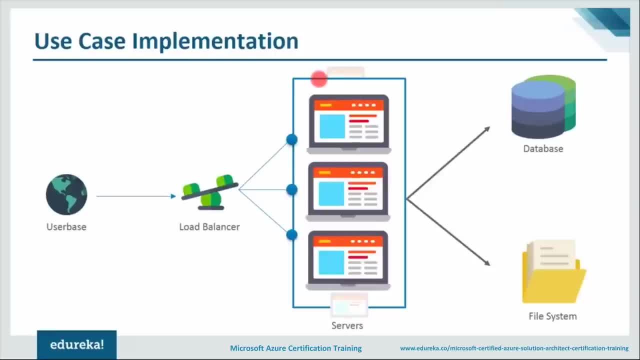 were three pictures running in the background, So my server should know what are those three files. There should be a list of those files that the server has to play in the background. Now that list of files is actually stored in a database, right. 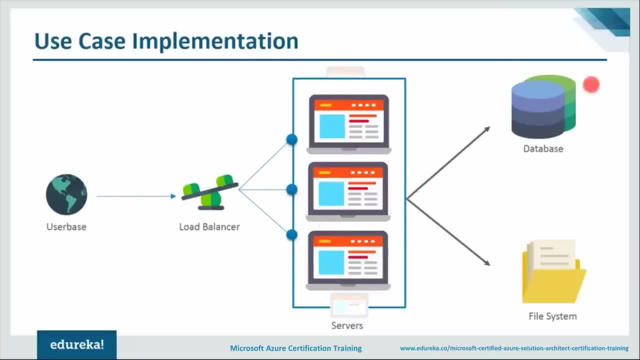 So what my servers will do is it will first get that list from the database right And once it gets that list it will fetch that list of files from the file system. Say, there are around five files in the database. So my server will interpret the addresses of those five files from the database and 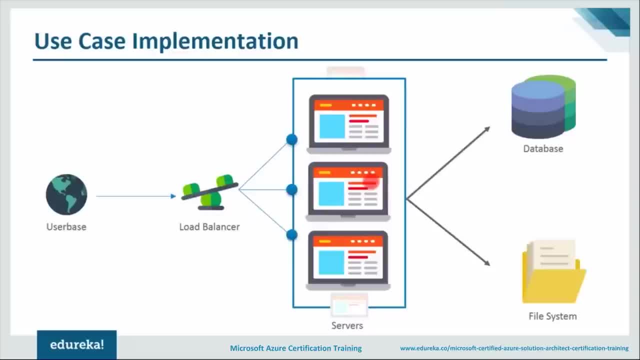 then it will call the file system And get those addresses or get those files from there and try to show that in the slideshow in the website. Now, when we upload the file, what happens is first your database is updated, right. So whatever file is being uploaded to your servers, that file is renamed according to. 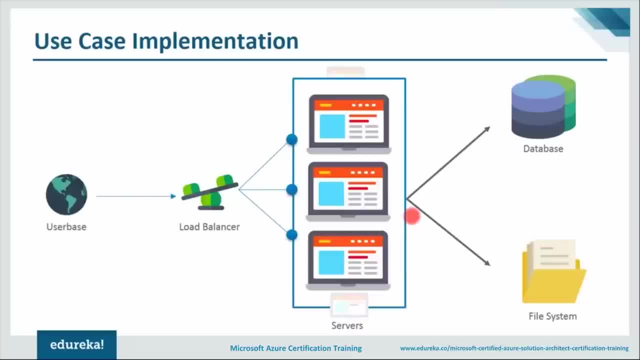 whatever parameter you have set, because it has to be unique right. Each file has to be identified with a unique name, right? So it renames that file to that unique name, Then stores it on the database. Once entry has been made on the database, then it gets uploaded onto the file system. 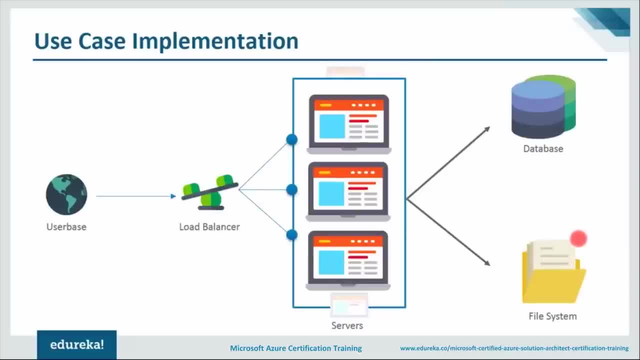 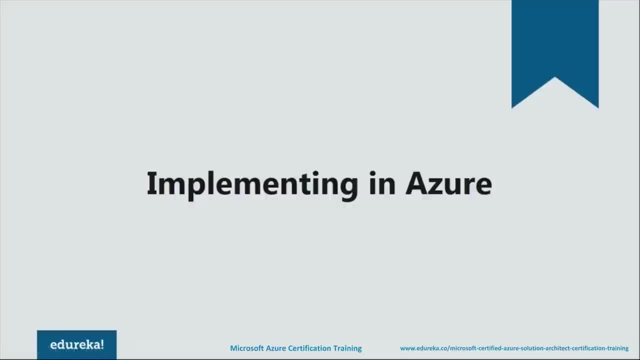 right? So, guys, this is the architecture of your application. This is the logic that we'll be following today, So let's try to implement this architecture in Azure now. So we understood how we can actually architect this use case in a general way, right? 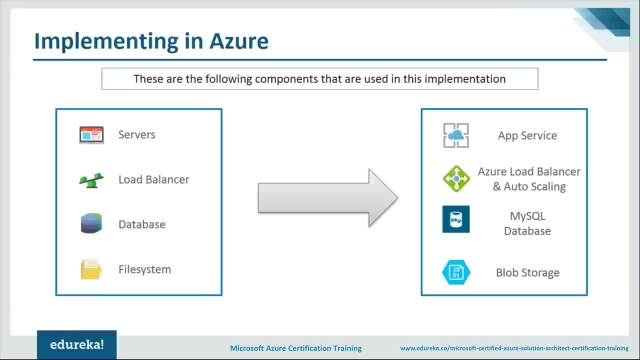 Let's see how we can implement it in the Azure environment. So in the Azure environment, The servers that you're trying to implement is actually provided to you by a service called the app service. What is app service? We'll be discussing in the further slides. 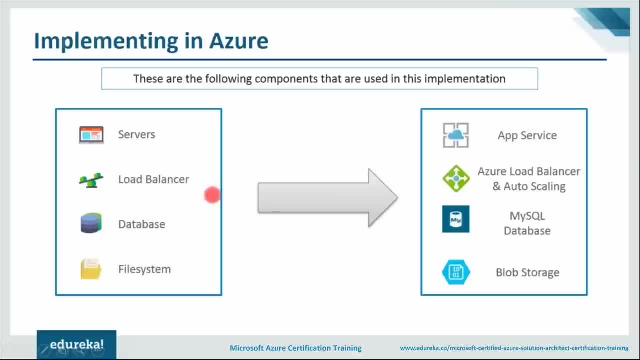 Then let's talk about the load balancer and auto scaling. So the load balancer is actually implemented by the Azure load balancer and auto scaling, right? Having said that? then we talked about the database. So database is the MySQL database that we'll be using in Azure. 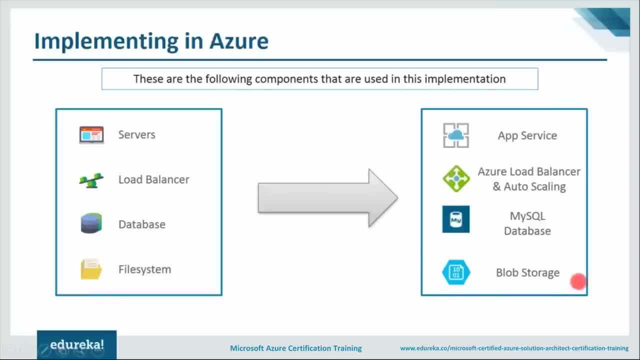 And then you have the file system, which is called blob storage. Okay, In Azure, what are these services? You might be confused. Okay, What is your load balancer? What is the app service? What is MySQL database? What is blob storage? 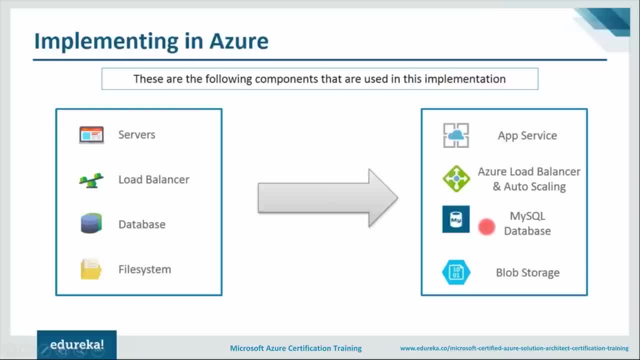 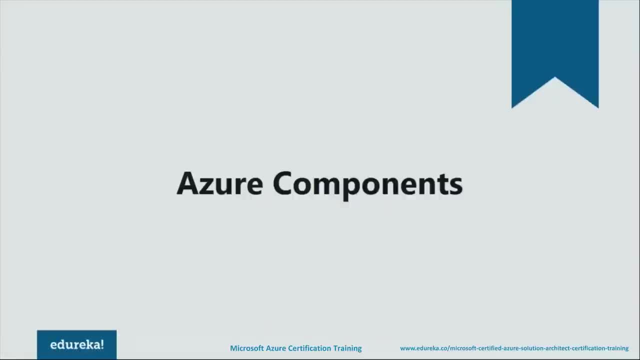 Don't worry, I will explain everything to you in the coming few slides. So let's go ahead then. So these are the services that you'll be using in Azure. Now let's go ahead and understand these services one by one. So let's talk about the app service first. 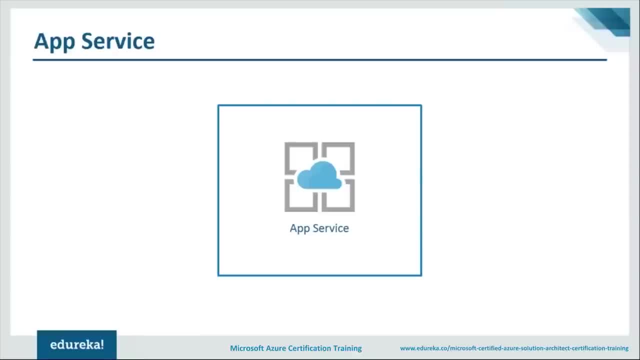 So the app service is basically a part of the compute domain, right, And in the compute domain you have a lot of services. But why are we using the app service? Let's understand that. So there are basically three kinds of services in the compute domain, if you talk about in. 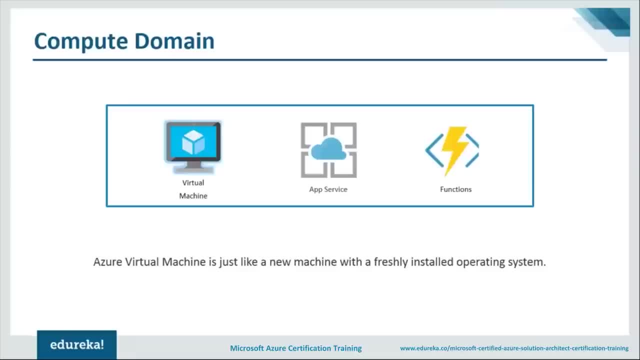 a very broad sense. The first service is called the virtual machine. Now, what is a virtual machine? A virtual machine is just like your traditional computer that you have in your in-house data house. It is a computer that is accessible to you and you can do anything with that computer. 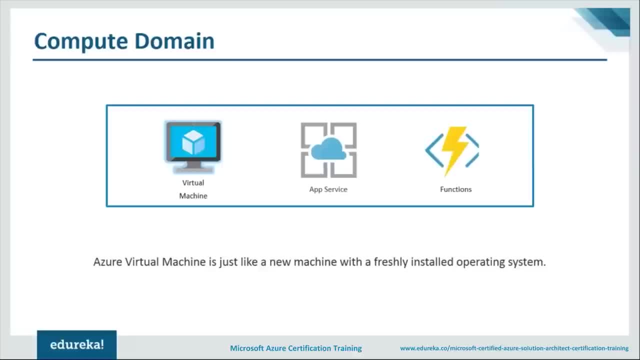 You have all the rights to that computer. All you have to do is, Basically, what you will do with a virtual machine is. you will say that I need this much RAM, I need this much storage and I need this much configuration. Please give me a computer. 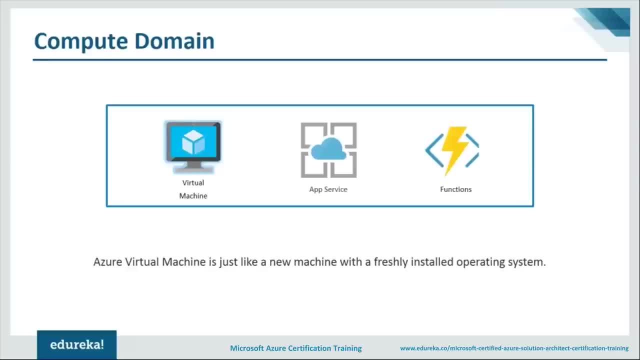 So Azure will create that virtual machine for you, right, And it will give you the IP address and the password for that machine. What you can do is, by remote desktop connection, you can enter that IP address, enter the password and you'll be able to connect to that computer. 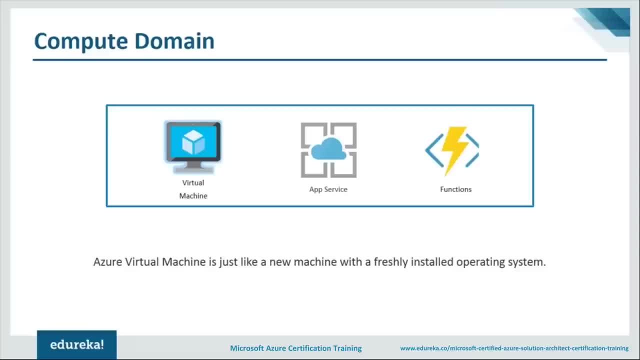 Now, once you connect to that computer, it is your computer. now You have the access to the user interface. You can do anything on this computer. You can make it a website server, You can make it a work at your environment, You can use it for image processing right. 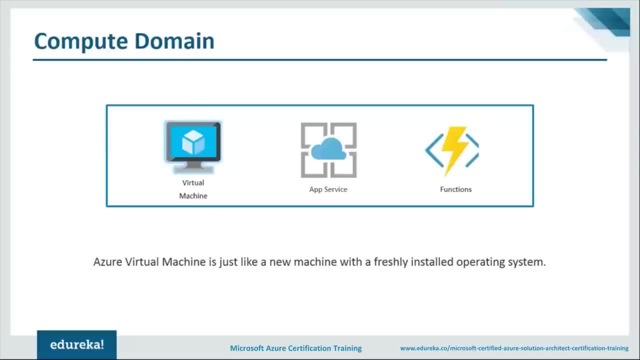 You can do multiple things on a server, like you might be doing on your server as well. Right, So this is what virtual machines is all about. You can configure it to become anything. Our next service is called the app service, So it is basically an automated version of a virtual machine, but with limited possibilities. 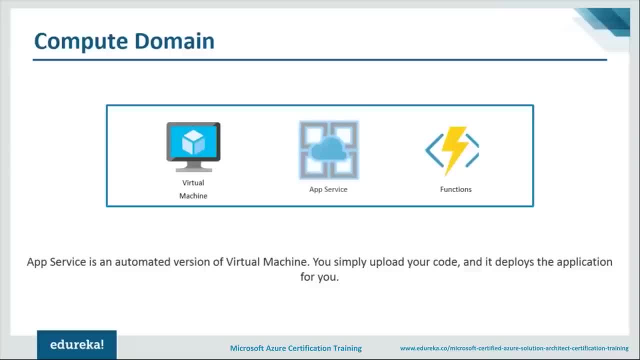 When I say limited possibilities, Limited possibilities, this service is actually very more focused, right? So app service. basically, it doesn't give you the access to the user interface, alright, But that gives you a more simple interface to deal with, because if you were to host a, 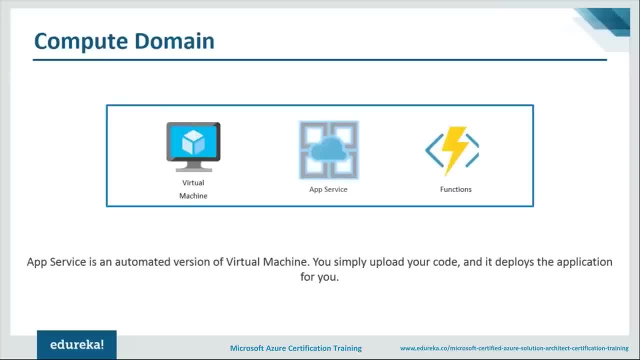 website in virtual machine. you would have to configure the virtual machine, You would have to configure the firewalls, You would have to install the necessary software. like say, for example: you have a PHP website, right, You would have to install the PHP software on your virtual machine and then you would. 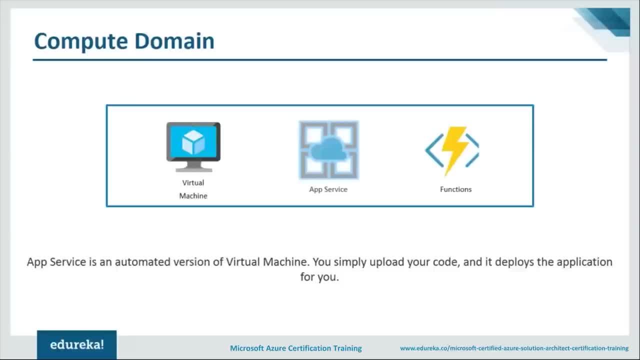 have to copy those your website files, or the files that you have coded into a specific folder, and then you would have to specify the configuration for your firewall and everything right. So there were a lot of things that you had to do in your virtual machine. 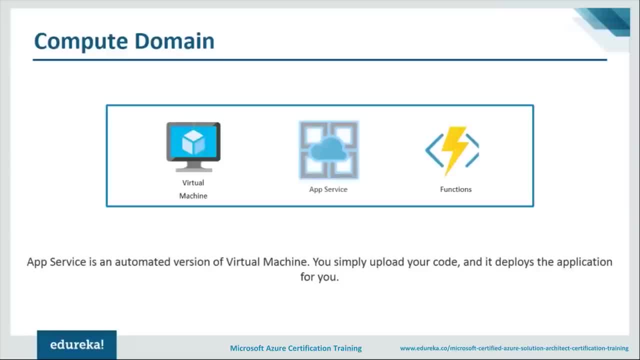 With app service. you don't have to do anything. You just have to specify what language you want. Say, for example, I want a PHP website, so I'll select PHP, I'll do next. Then it'll ask me what kind of configuration I want. 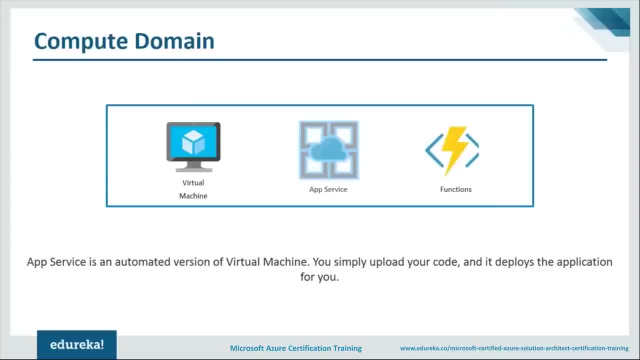 I'll specify the configuration, I'll click next and that is it. My website will be deployed automatically. it'll ask me to upload the files. I'll upload the files. It'll automatically send it to whatever folder it is required. and it is done, right. 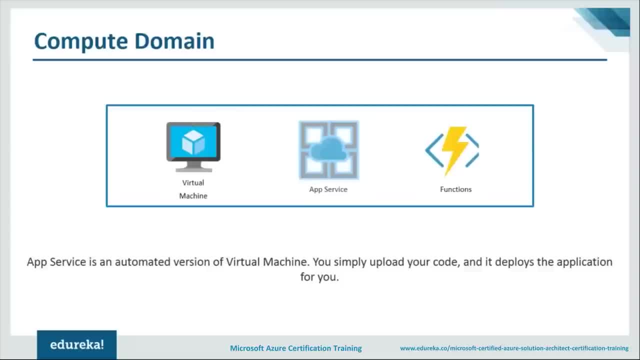 So this is the part of app service, right? It is more automated, because with virtual machine, everything had to be done manually, but with app service, everything happens automatically. I just have to upload my files, right? So this is what app service is all about. 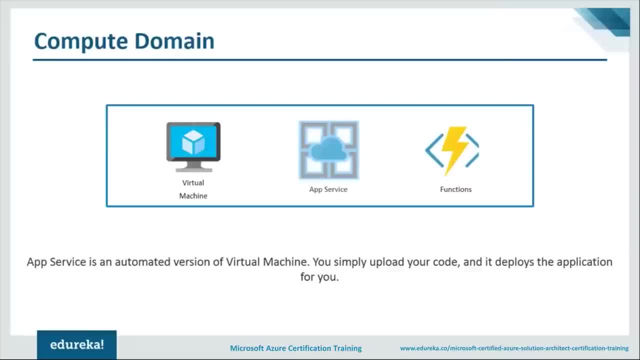 So, like I said, so app service is basically used to deploy an application. all right, You cannot do anything else with it, You cannot use it to process a customized workload or something like that. You can just use it to deploy an application, and that is why it is called an app service. 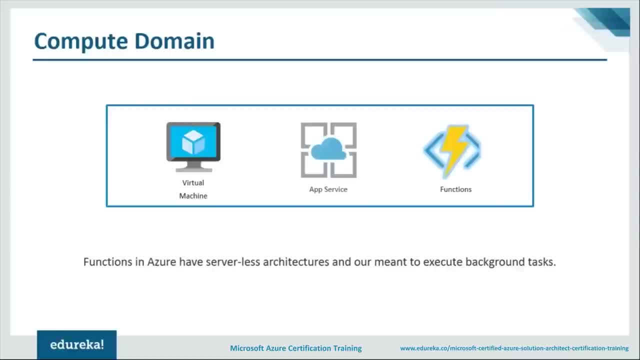 right. Moving on, let's talk about functions. So functions is basically a very new technology. It's called the serverless architecture. It's basically what it does is: you don't have to specify the configuration, You don't have to specify anything. 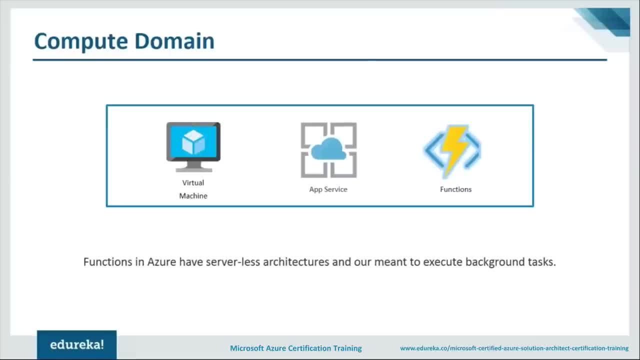 You just have to upload your code and it executes it for you, but it will not deploy any application for you. For example, you want to host a website. it will not do that. It just does processing, in the sense it will only do background tasks for you. 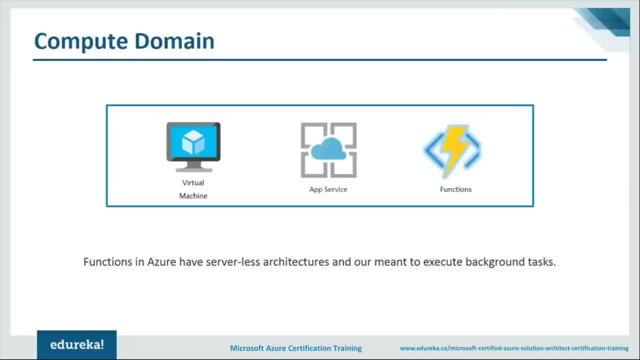 For example, if you have- let me take an example which uses both these services- If you have, say, an application like Instagram, right so user uploads his image on your application and then your application has to store that image. Now, before storing that image, maybe you want to compress the image or you want to apply. 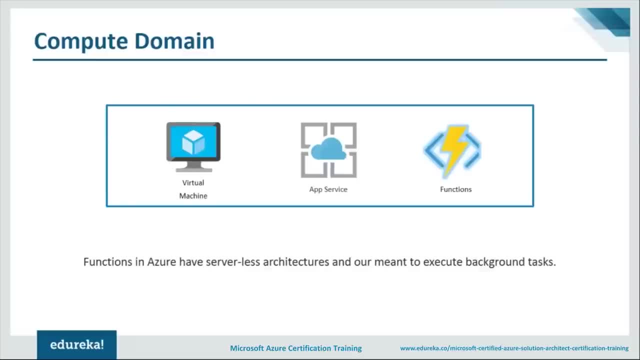 a filter to it or whatever right. So from your application the file is uploaded, and now these many tasks have to be done. If these tasks are actually configured in your code, which is actually uploading the file as well, it will actually increase the overhead on the server which is hosting an. 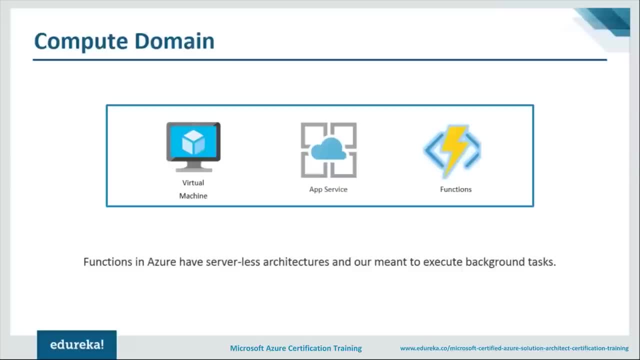 application. But what we can do is The way things happen today is everything is distributed right, So from your application, only the file will be uploaded. Once the file is uploaded right, the tasks will be the tasks like renaming the file. 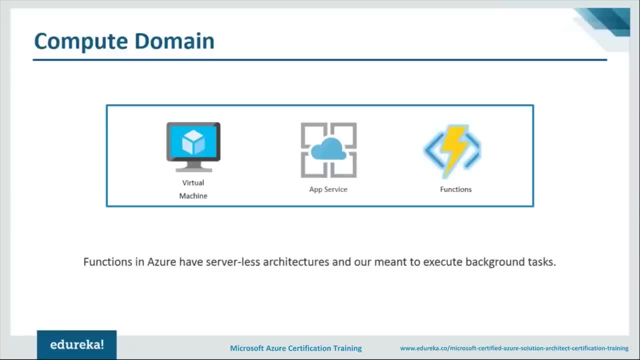 or compressing the file or applying the filters. everything will be done using the functions. So the function will get invoked whenever the file is uploaded using the app service and the function will execute all the tasks that have to be done on that particular image. 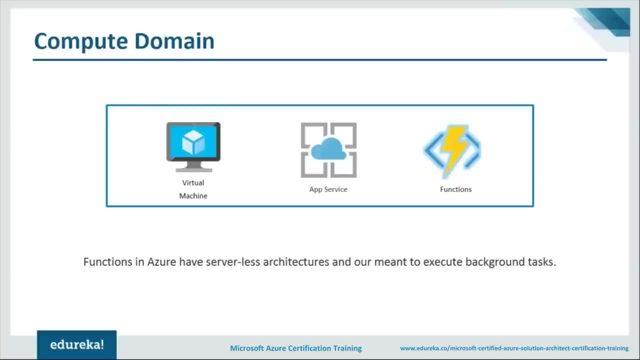 This reduces the overhead on the server. This reduces the overhead on the server which is hosting your application. right, And you have your background. tasks will be implemented by your functions and then will be stored in the respective file system, whatever you have coded your function to do, right. 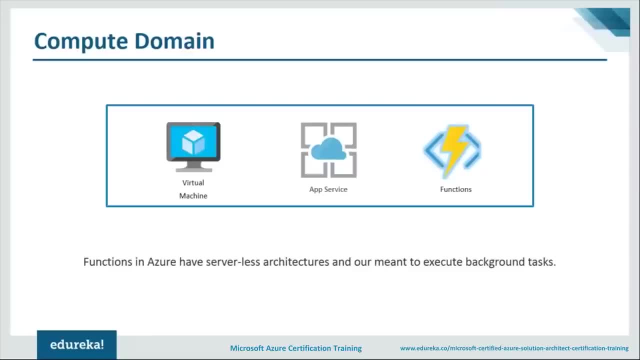 So this is basically a reference. So recapping again: virtual machine is basically a computer. You can configure it to do anything. You can actually use app service in a virtual machine manually. For example, you want to deploy an application, you can use it by configuring a virtual machine. 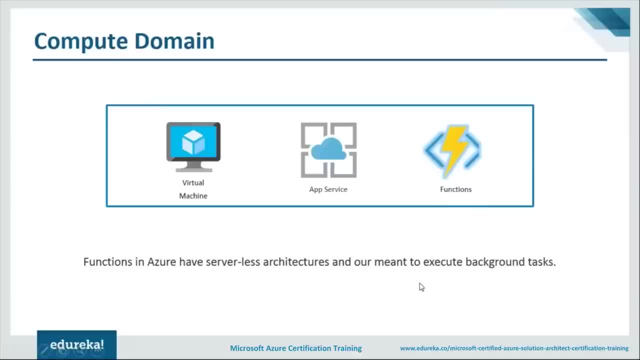 right, You can also use it as a function. your virtual machine, that I mean to say as in. you can configure it to only execute background tasks. But the thing is you have to configure everything manually. If you want an automated version, you can go with app service. 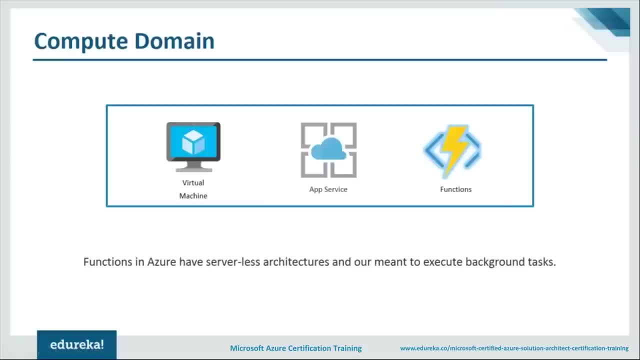 App service is used to deploy an application, right, But if your use case is not about deploying application, you want to do some raw processing, you might as well opt for functions, which is a service which is not useful to deploy an application, but is used to execute background tasks. 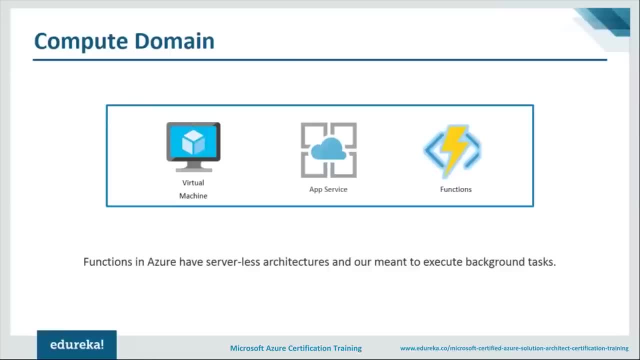 All right. so, guys, any doubt in whatever we have discussed, like we discussed virtual machine, we have discussed app service and we have discussed functions. All right, like I said, we are using the app service. why? Because we are deploying a website, right? 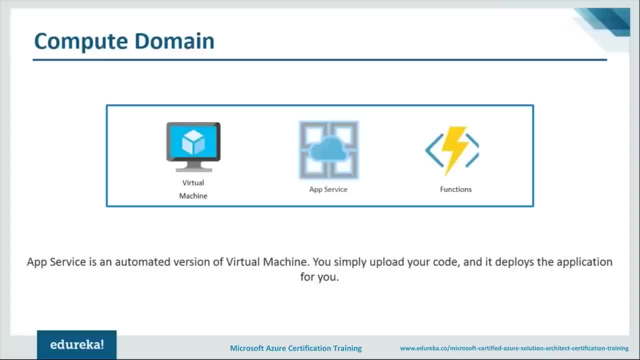 So for deploying a website, I need app service, So it cannot be done using functions. can be done with using virtual machines as well, but it will need a lot of manual work, And our job is to make it work. We need to make everything faster, right? so cloud computing is all about speeding up. 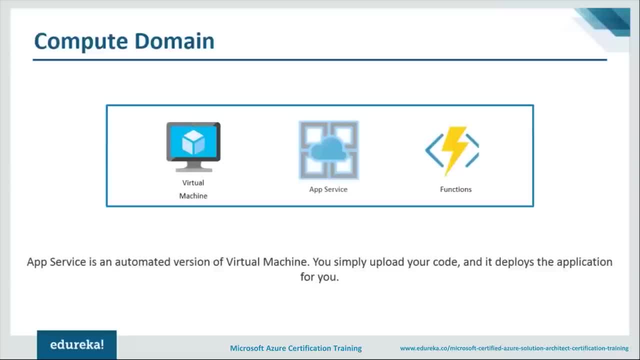 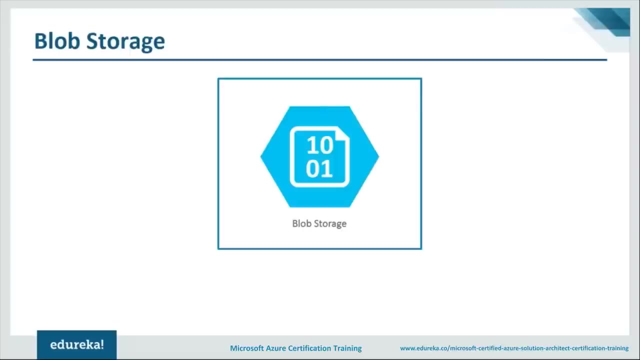 things. the speed of implementing is increased, right? So I'd rather use an app service and upload my code on the app service and it will deploy the website for me, right? It's that simple, guys. Let's move on to the next topic of today's discussion, which is the blob storage. 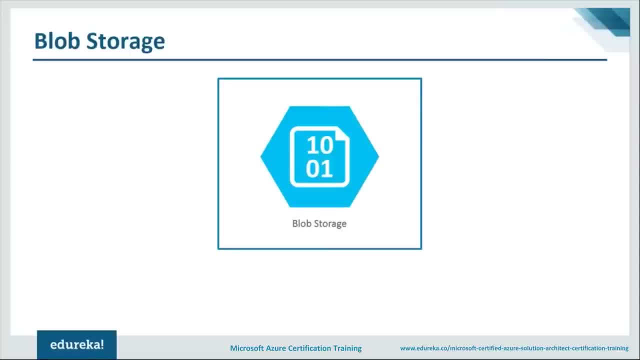 So the blob storage is basically the file system that you need to upload your files. right? You definitely need a file system. There is no alternative to this, right. So your blob storage is the place where you'll be storing your image files. 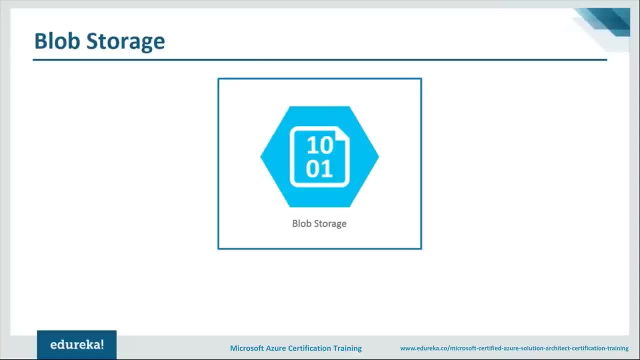 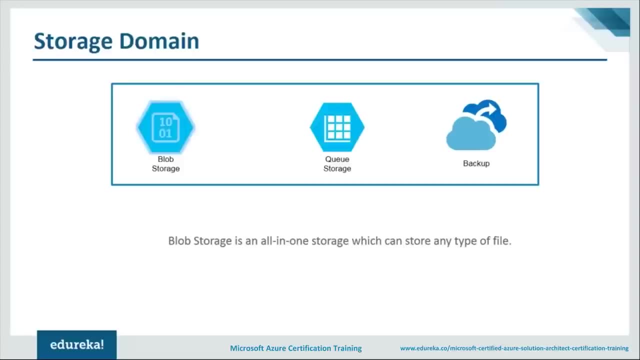 But why did we choose the blob storage? Why not some other service from the storage domain? Let's discuss that. So in the storage domain, basically you have three kind of services. You have more services as well, but these are the three main services in the blob in. 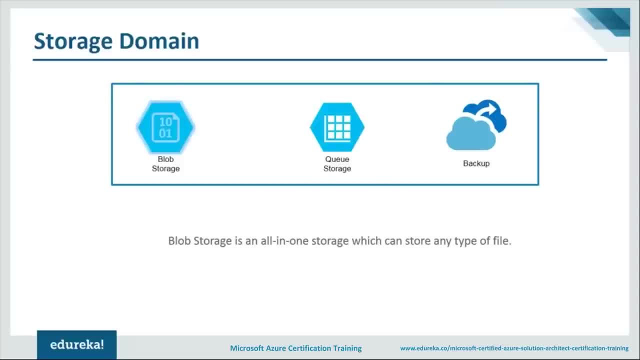 the storage domain, You have the blob storage, you have the queue storage and then you have the backup right. So the blob storage is, like I said, is, a file system on which you can upload your files, upload any kind of file right. 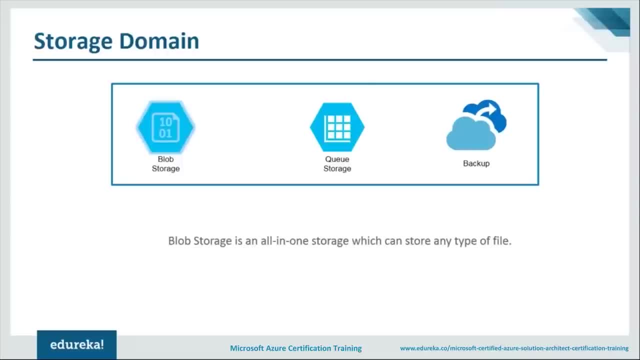 And that's about it. There is nothing more to blob storage. This is the thing. Next is queue storage. So queue storage is basically a queuing service. Whenever you have to synchronize tasks, say, for example, process, one has to be done before. 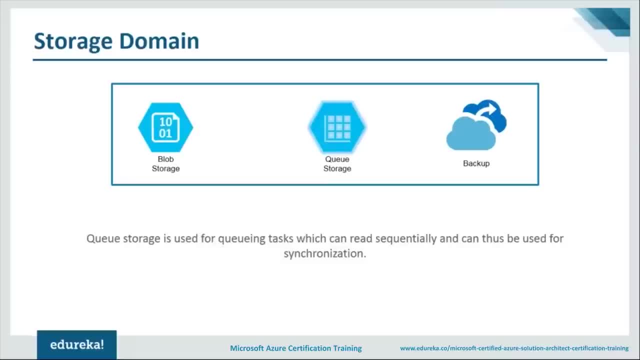 process two, and process two has to be done before process three. So what you can do is you can bundle these tasks in a sequential manner and you can add it to the queue storage right? What the queue storage will do is it'll actually. 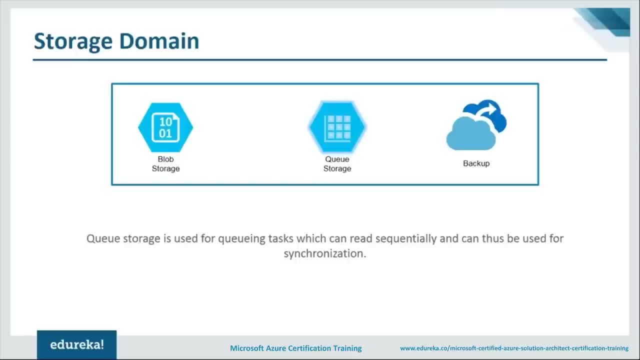 Hold these tasks according to the sequence that you entered right, and whenever the queue storage is accessed, it'll give them only the first task, not the second task and the third task first. So the way it functions is like this. Say, for example, like I said, the image processing application: I want to rename file first. 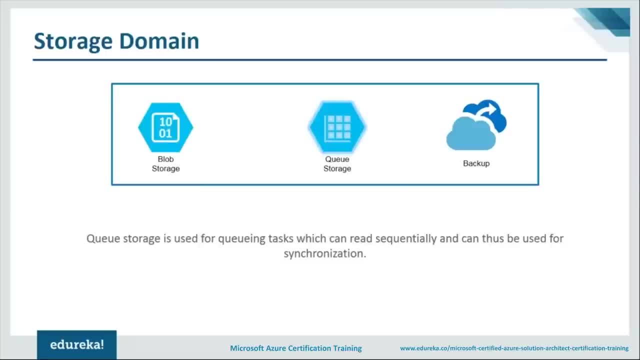 Then I want to add filters and then I want to store it on the file system. So these three tasks I will write it down and I will add it into the queue storage. Now say, these tasks will be done by my functions. all right, 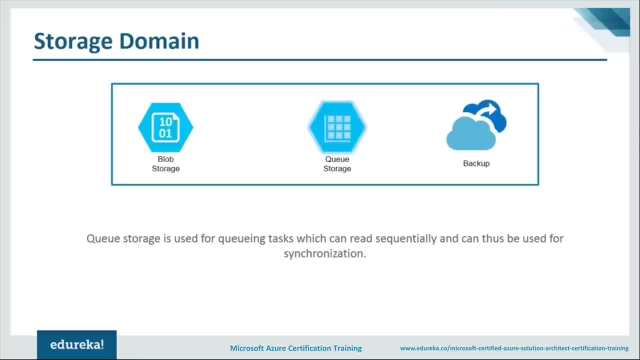 So what functions will do is it'll try to interact with queue storage and it'll ask for a task. All right, so queue storage will give the task to functions in a very sequential manner, in the sense that it'll first give it the task to rename the file, so it'll rename the. 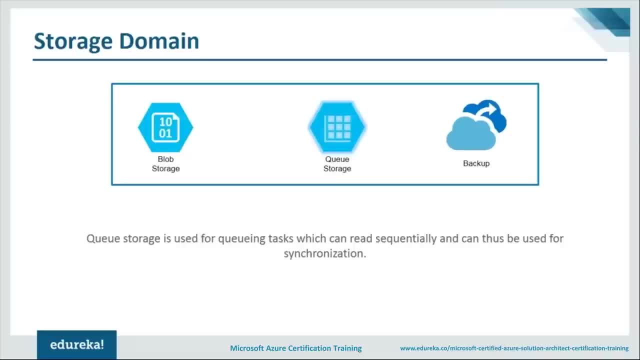 file. Once that task is done, it'll again try to access queue storage and then queue storage will give it a task to filter the image or apply filter to the image. right? Then it'll apply a filter to the image and then it'll ask for a task to filter the image. 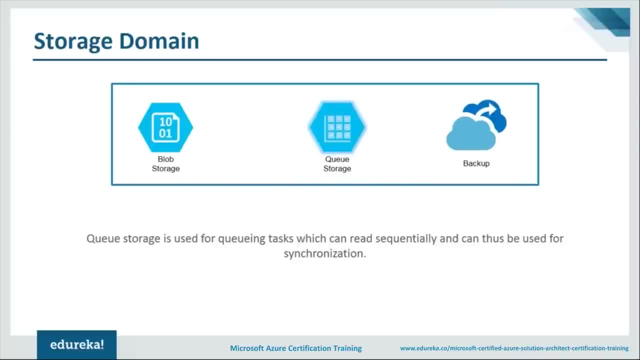 All right, So that's it. It'll be done with that and then it'll try to again the queue storage and then it'll see that. okay, now it has to store that file in a file system which is specified in the 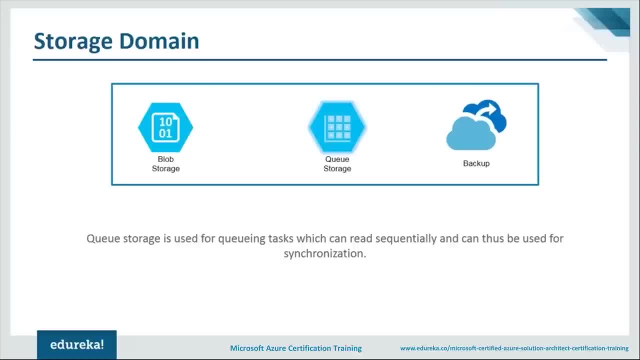 code right And it'll pick that task, do it and be done with the first file, And then it'll again access queue storage and the process goes on right. So, basically, queue storage is used to give a sequential manner to the processes that 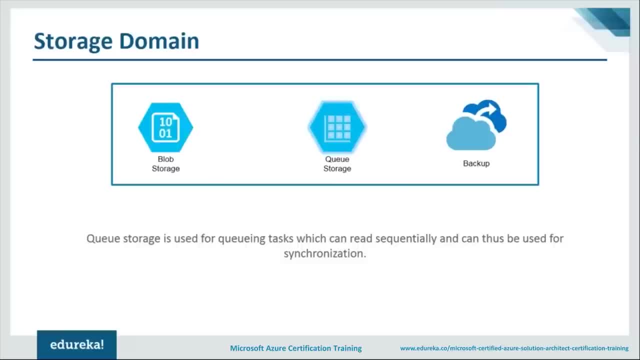 you're trying to execute. Having said that, this is about queue storage. Then comes backups. So backup is a service wherein you can store your infrequently accessed data, right? What is your infrequently accessed data Could be? for example, in my company, we take a record of everything, right. 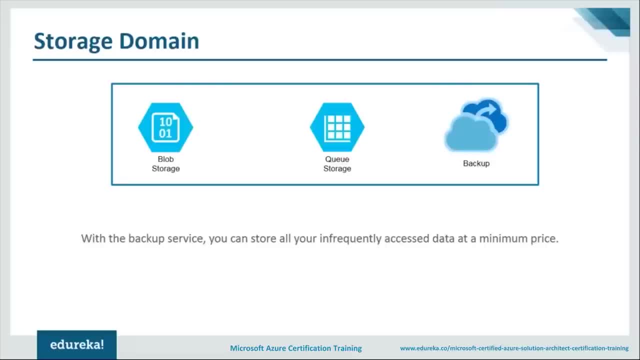 We take a record of every class that we do. we take a record of every query that you guys raise. Now, say, the classes that were taken, say like two years ago, right, and obviously I cannot delete those classes because they have to be kept for record. but what is the point? 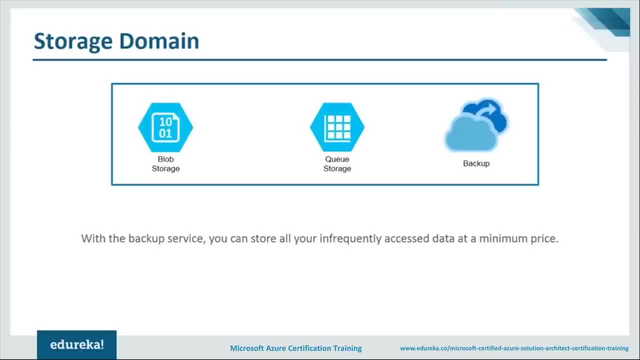 of keeping them on my data. What is the point of keeping them on my live hard drive? because my live hard drive is where I do my current tasks right. So rather than keeping it on my live hard drive, I say, okay, let me keep it in a CD. 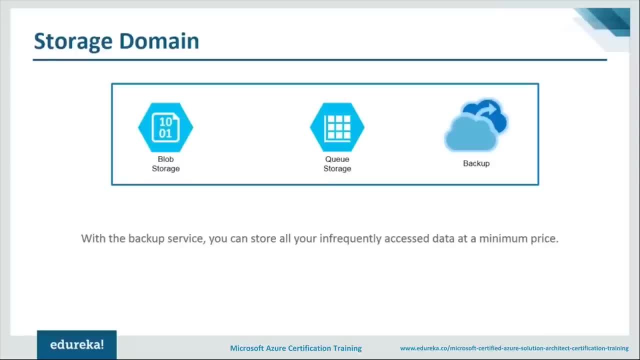 or a pen drive and keep it somewhere where I can take it out when I actually need them, right? So this is the concept of taking a backup Now. similarly, if you want to take a backup in Azure, say, you have your virtual machine. 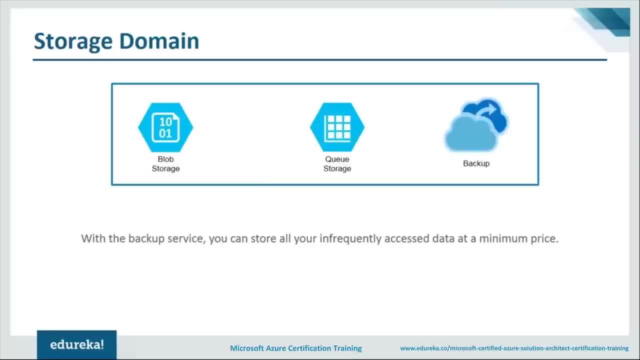 and you have stored a lot of files on your virtual machine, but you think, okay, I don't need these files anymore, Or maybe I don't need these files As of now. I might need them later, So why do spend that much on the storage that you're taking on the virtual machine, right? 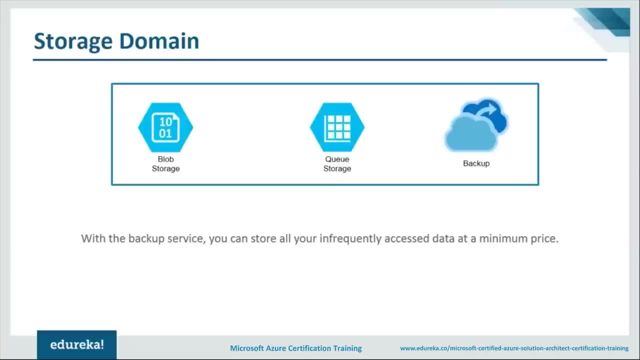 rather than storing the infrequently accessed data, why not put more frequently accessed data? So what you can do is the infrequently accessed data that you have in your machine on the cloud. you can actually take a backup of that and store it in the backup service. 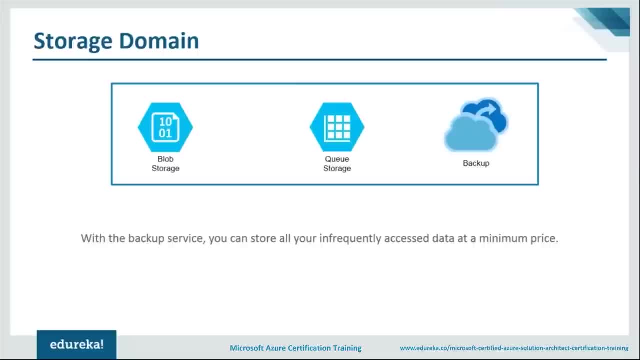 Now, why will you store it in the backup service? is because storage is more cheaper. when you talk about the backup service, Because obviously first of all they'll use magnetic tapes or they'll use SSDs or something like that to store your data. 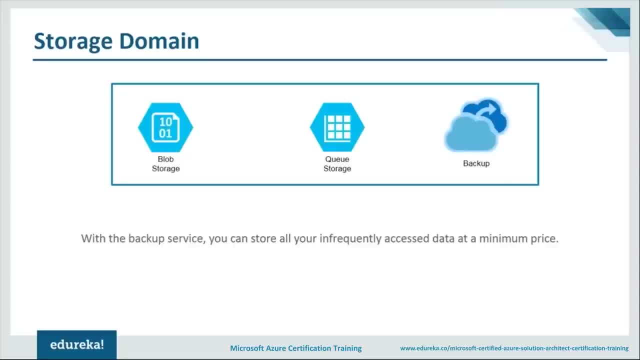 Now why is it cheap? is because obviously it has a downside, that the response time or the time to retrieve the file from a backup service is obviously more. For example, if you have stored everything in your virtual machine you can like go to that particular folder, access that file and that is it right. 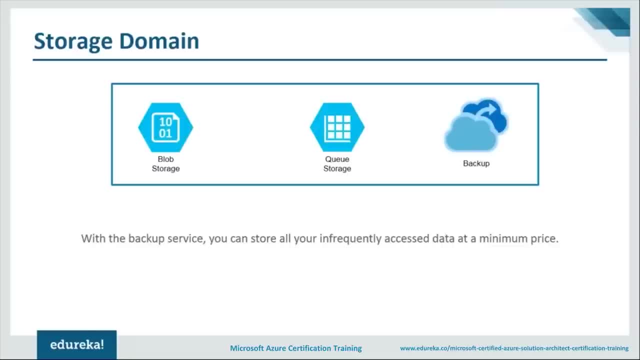 But if you have stored it in the backup service, the retrieval actually takes time, But it is worth it because you don't use that file every day, right, You won't be using it and also you're paying less, So it doesn't pinch you that much because you're paying less and you are not using that. 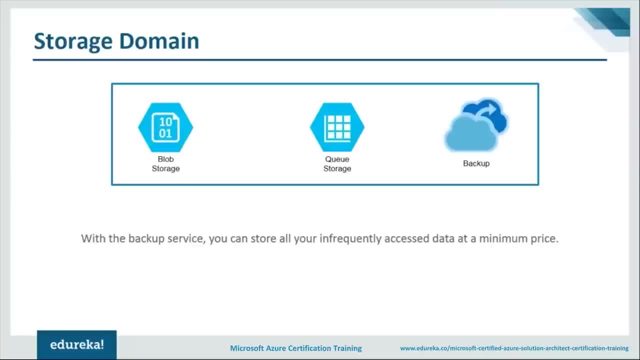 file very frequently as well, So why not put it in the backup service? So this is what the backup service is all about. Now, today, in our implementation, we are using the blob storage for obvious reasons that I want to store my image files, right. 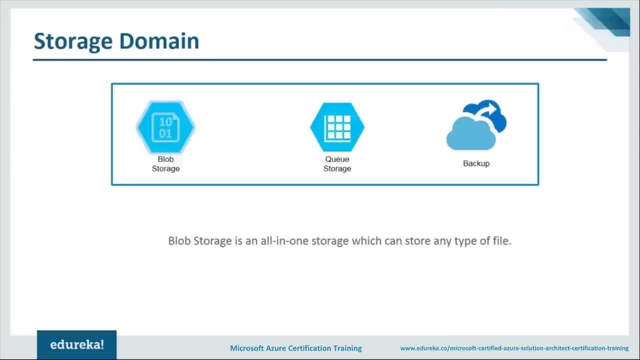 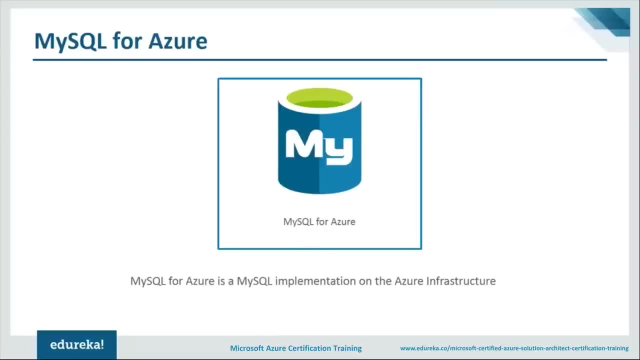 So I'll not store it on the backup. obviously I'll not store it in the queue storage. I'll store it in the blob storage, because that is what that service is meant to do. Now, our next service from Azure is the MySQL service from Azure. 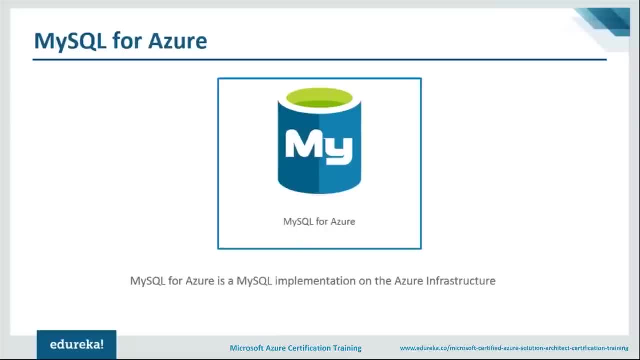 It is basically a MySQL implementation on the Azure infrastructure, right, So you can use any database you want. In Azure, you have an SQL service which is purely SQL, So if you're comfortable with that, you can use it. I am using MySQL for my use case today because that is the way I have coded my application. 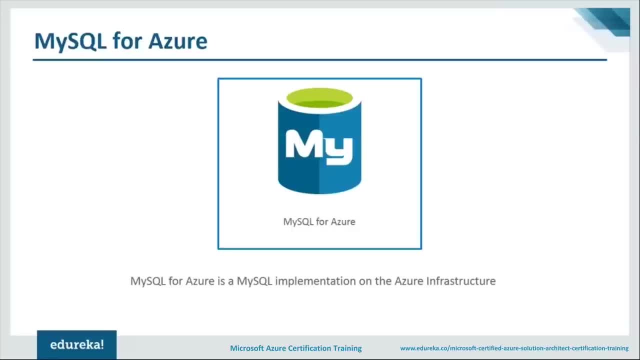 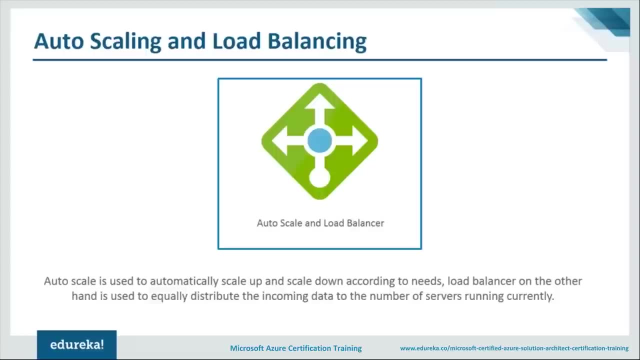 to be right, So it is just personal choice. The next service that we are going to talk about is order scaling and load balancing. So, like I said, load balancing is when you want to equally distribute your traffic among the number of servers that are running that time, and order scaling is actually scaling. 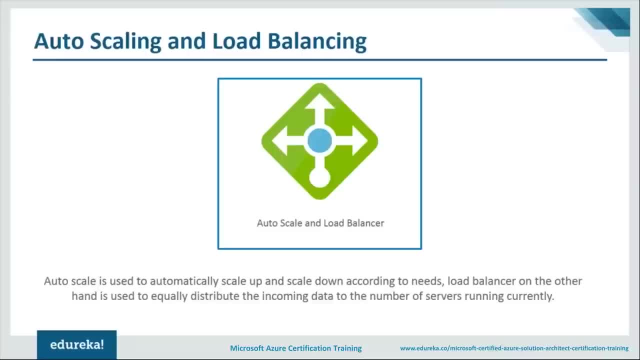 up the number of servers that you're using according to the traffic that is coming onto your website, So you can actually set a metric that. So obviously, when more traffic is coming onto your website, your CPU utilization will increase because you have to process more requests now. yeah. 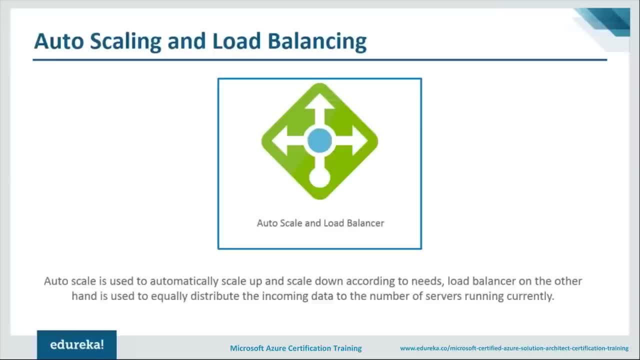 So your server will be processing more requests and that is the reason your CPU usage will increase. So you can actually set a metric. Let's say my CPU usage, when it increases 60 or 70 percent, increase one more instance, or increase three or four more instances, right? 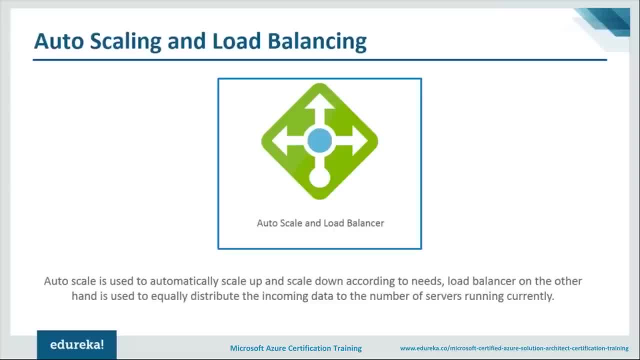 So it is based on your personal use. So this is what order scaling is all about And obviously, when you're using it, you're going to be using it for a lot of different purposes. So if you're using order scaling, the number of servers is changing constantly. you need 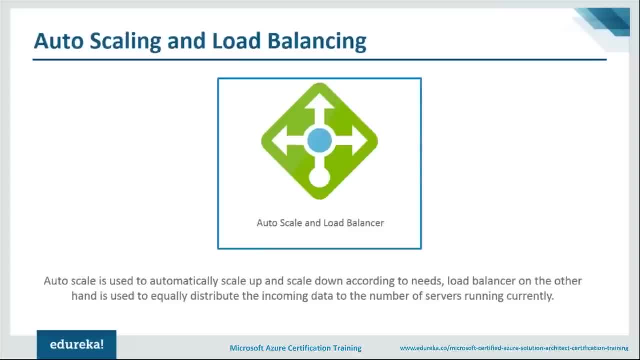 a load balancer along with it, right, The load balancer? so that say, you have six or seven servers which are running right now and say the traffic decreases and it sees, okay, now the CPU utilization is going down, so it will reduce the number of servers, right? 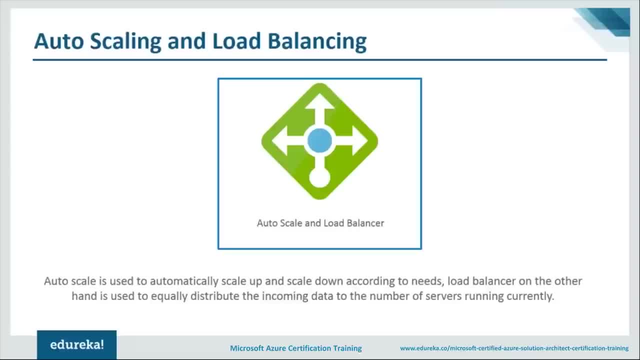 So when it will reduce the number of servers, the load balancer should identify: okay, there were seven servers before. now there are like three, So you'll be distributing the traffic according to those three servers, Okay, So the load balancer actually plays a very important role in the order scaling process. 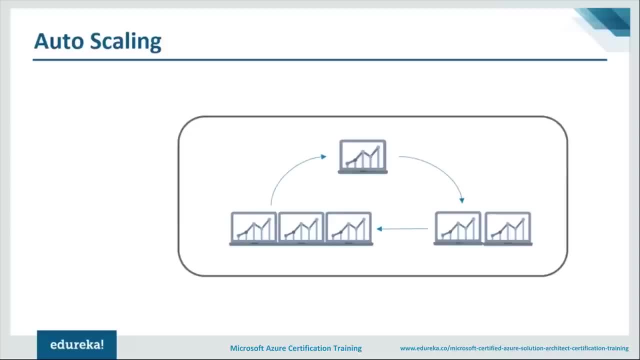 Having said that, so this is how order scaling actually works. So say, you have one server, right, and the usage increases. it goes on to become two servers and then again the usage increases, it becomes three servers. right Now, when the usage decreases, these three servers can be reduced to one server, or can? 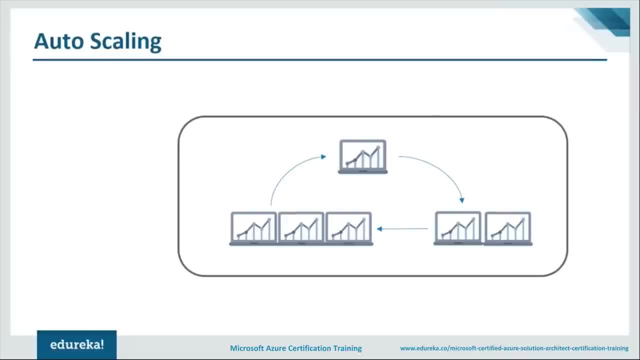 be reduced to two servers. So this is a diagram representation of what order scaling is. We talk about load balancers. Okay, So load balancer, like I said. so load balancer is a very crucial part of order scaling process, because load balancer is the part which actually distributes the traffic according to the number. 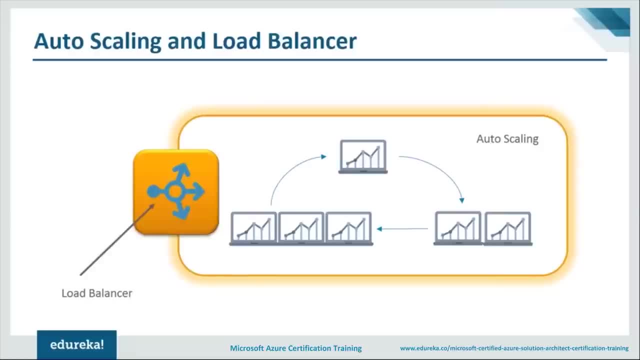 of servers that are running at that time, right? So this is how the process works. The traffic comes on to the load balancer and the load balancer sees how many servers are running and distributes traffic according to that. All right, Okay. 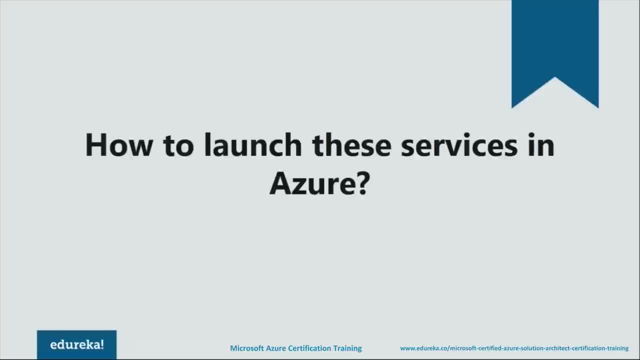 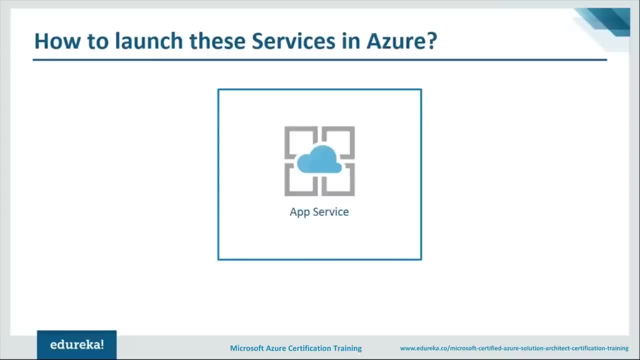 So we are done with the services. These are the services that we'll be using today, So now we'll see how we can launch these services. Let's see how we can launch these services in the Azure user environment. So, guys, we'll talk about the app service first. 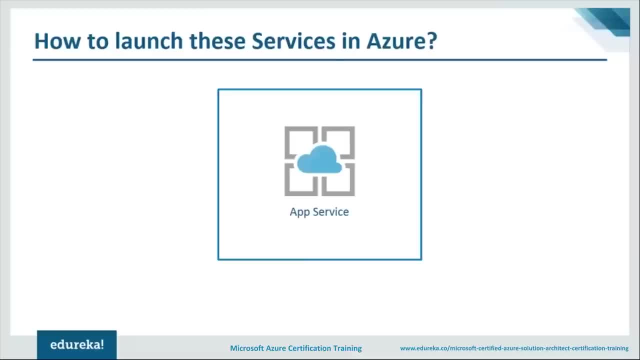 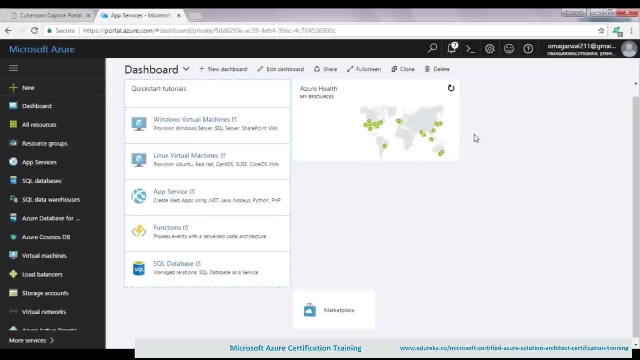 We'll see how we can launch an app service in the Azure UI. Okay, Let me show you the user interface for Azure now. So, guys, this is how the user interface for Azure looks like. You have all the services listed there on the left side right, and this is the dashboard. 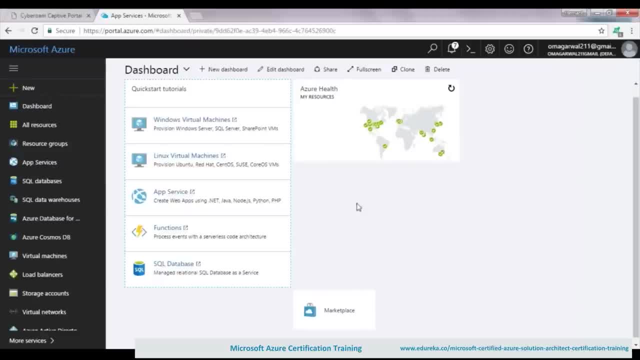 This is called the dashboard. Whatever services you launch, you can pin it here for basically getting access quickly. It is just like a desktop on your computer which has all the shortcuts and everything, and this is what the dashboard is actually used for. All right, 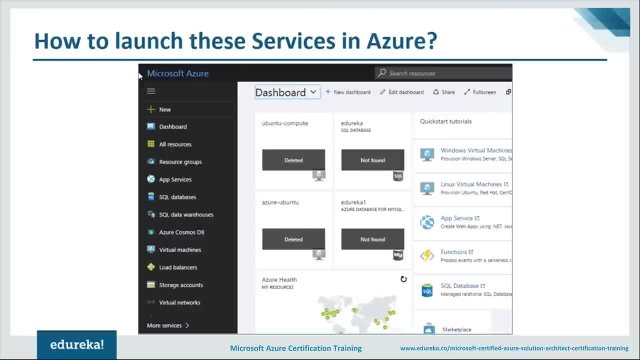 Having said that, let's see how we can launch the app service in Azure. So first you will click on app services. as you can see from here, You can click on app services and moving ahead once you have clicked on app services, you. 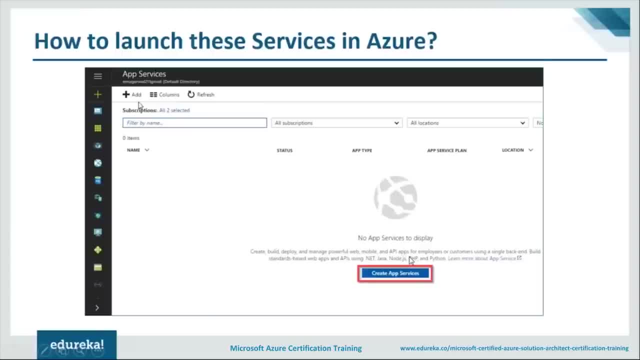 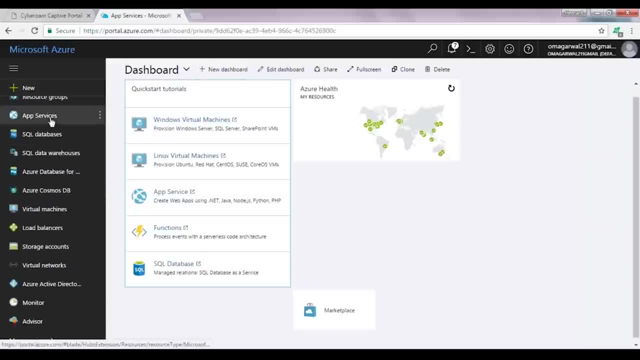 will reach this page. Click on create app services And then you'll click on web app. And that is it. Let me show you how you'll do that. So you'll click on app services. click on create app services, you'll scroll down click. 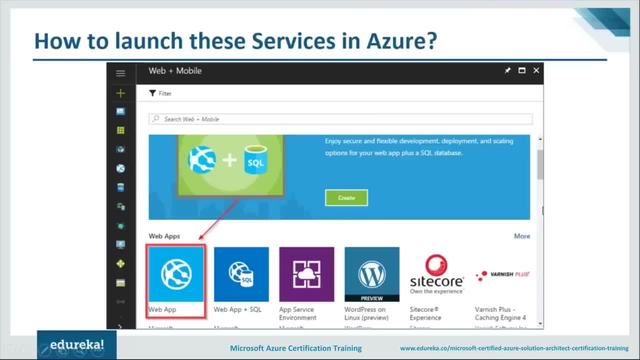 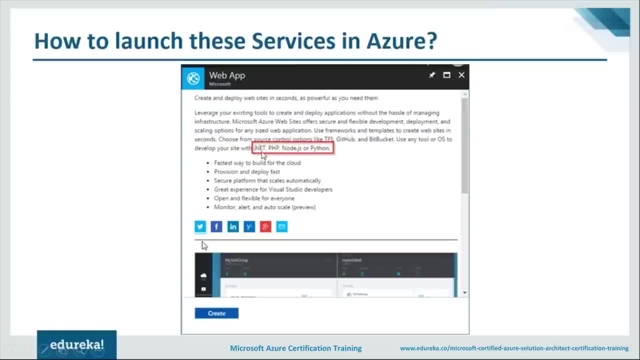 on web app And over here, as you can see. after this, you will reach the screen wherein you will see that you have four options. You can either code your website in NET, PHP, Nodejs or Python, So if it is either of these four languages, you don't have to do anything. 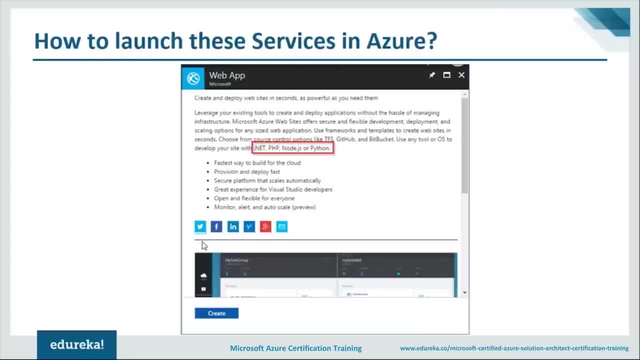 You just have to upload your code. Then this web app that you'll be creating and your app will be deployed automatically, without installing any software, without doing any configuration, just this, All right, Okay. So once you have reached this page, you will click on create. 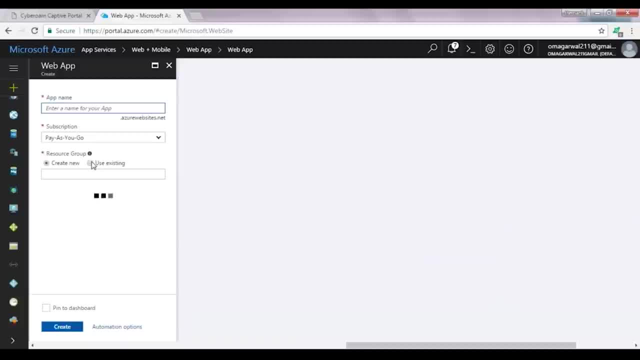 So let's click on create And then you will reach the screen. So now you have to give your application some name. So let us give us this name as Edureka-01.. So let's see if everything is fine. Okay, So everything is fine. 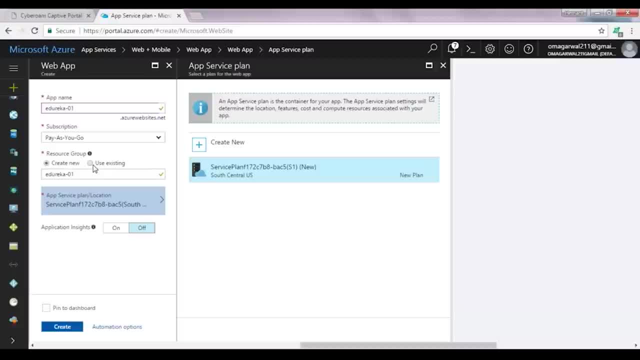 Everything is fine, So we have a little bit of extra stuff. My name is Edureka. I'm going to call myself Edureka. Where is Edureka? Ok, Edureka, It's all good, So I will give you the password. 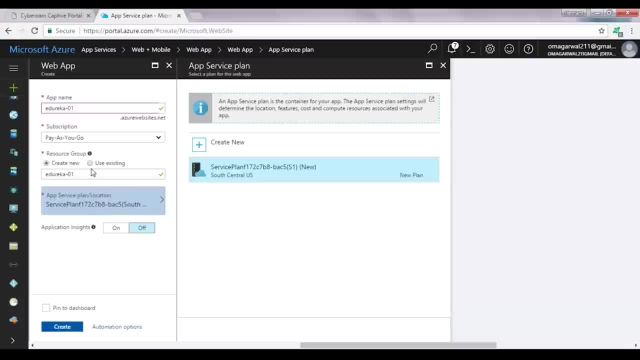 So for now, I'll just go ahead and give you the password. You will be given your password, You will be given the name and you will see that it is Edureka here And then right there, if you click on it, you will see the name. 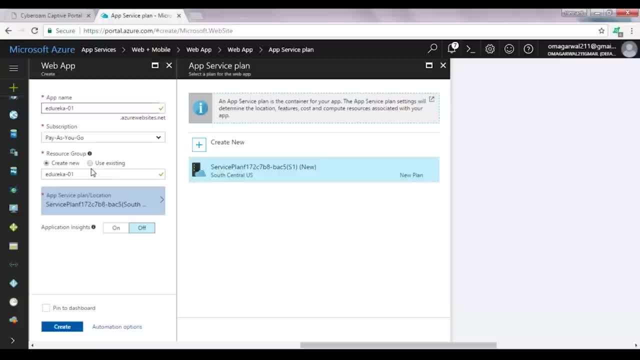 We have to click on create. So I am going to say Edureka Edureka, So Adureka Edureka. So for now we are going to show you this, So you see this here, And then you have the resource group. 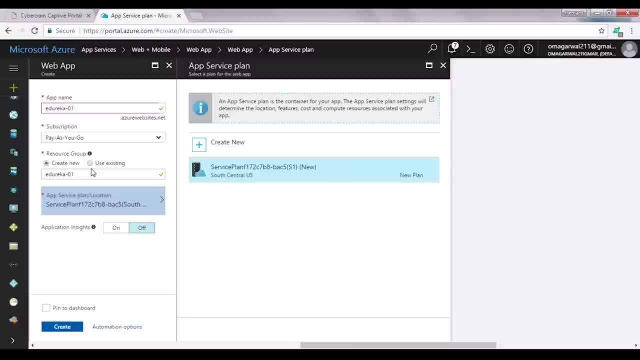 and it will be called a resource group. So any changes that you want to put across the group you can do to the resource group. Alright, we'll be discussing in detail what a resource group is in the further modules, but for now all you should understand is that a group. 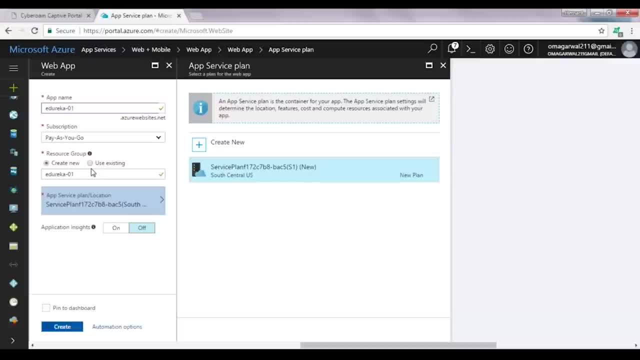 of resources is called a resource group. So if you have an application and it's utilizing, say, three or four resources, it's better to put those resources under one group, Alright, so this is about that. Then you have the app service plan. So app service plan is something. 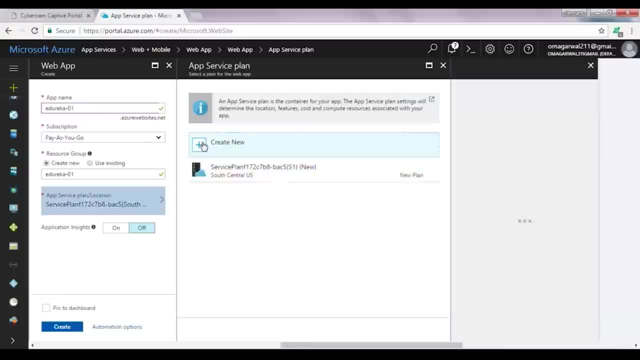 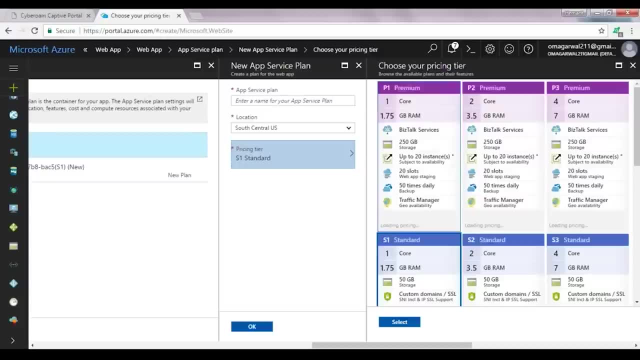 as in what kind of computers you use and everything. So let's create a new plan for you so that you understand it better. Under the pricing tier, this is the main part that you have to select, guys. You can select the app service plan. you can give it some name. 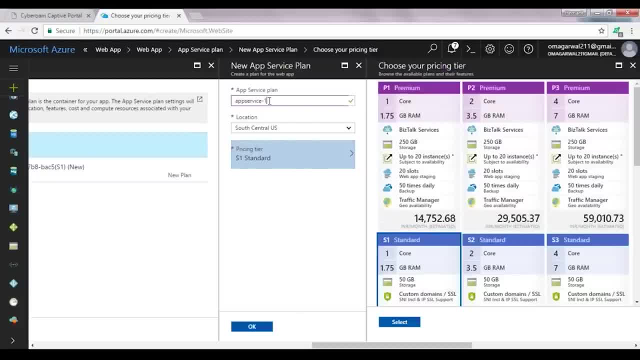 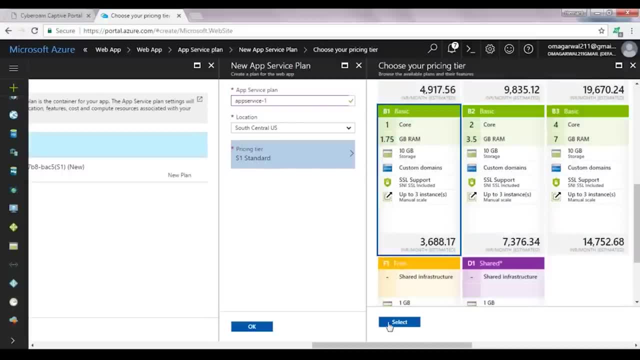 Let's give it as app service hyphen one. Alright, and this is my app service plan. You can select what kind of plan you need. Let me select the basic plan as of now and click on select Alright and then click on OK. 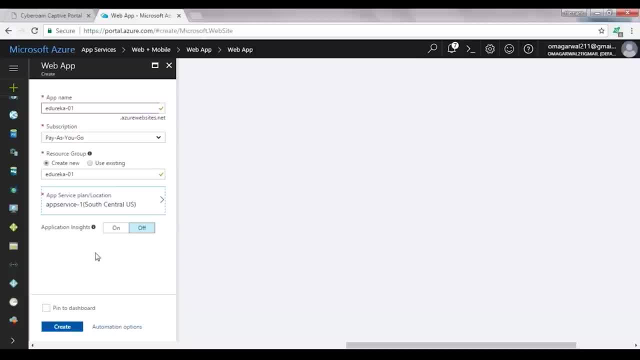 So this is about app service plan. You can click on application insights, which basically gives you the monitoring tools. For now, let's not discuss it, Let's not go into it. We'll be discussing it later. and now let's click on create. So I am taking the Pinto dashboard. 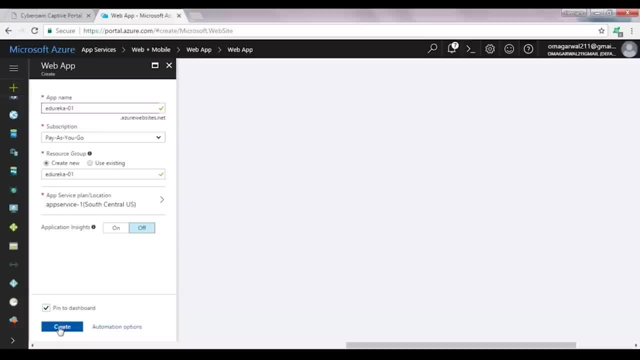 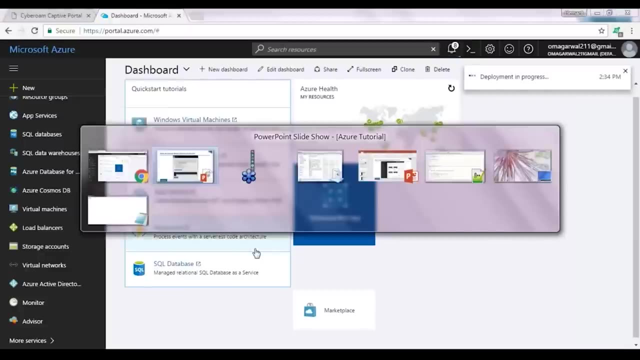 which will basically create a shortcut on the dashboard to this application, Comes in handy. and that's it, guys. You will click on create Alright. so now my application is being created, Okay, so alright. Alright, my web app is deploying. Let me go back to my slide and let's jump on to our 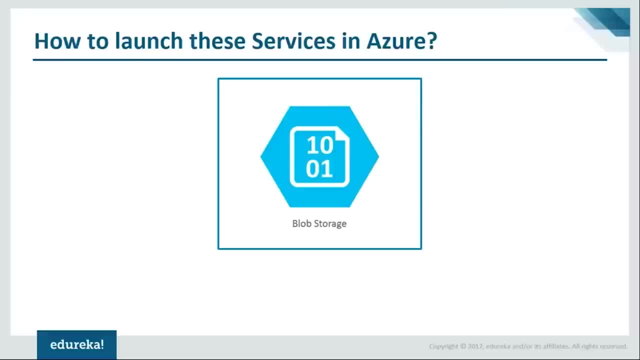 next service, which is blob storage. So, like I said, blob storage is just like a file system. You need a file system to show your files right. So that is what the blob storage is all about. Let's see how we can create a blob storage instance in Azure, So you will reach. 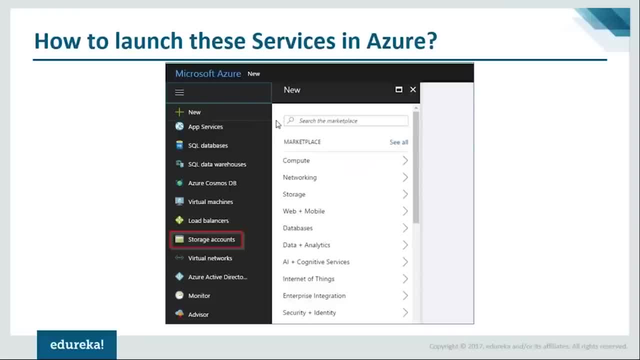 this is the dashboard. You reach the screen and you will click on storage accounts. Once you have clicked on storage accounts, you'll click on add And that's it. This is the dashboard. You'll reach the screen and you will click on storage accounts Once you have clicked. 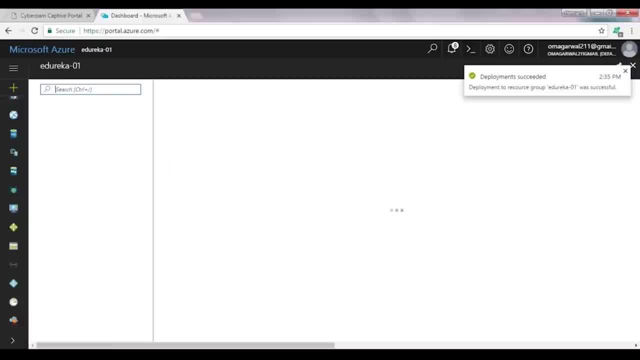 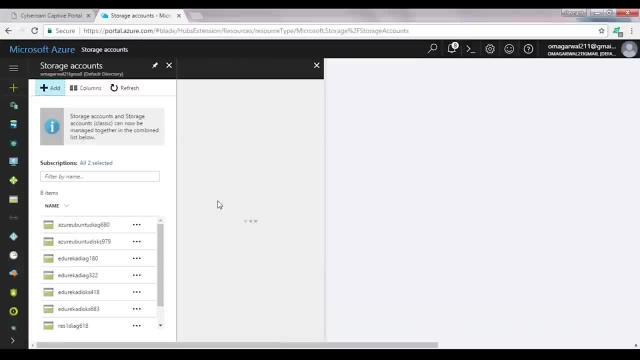 on storage accounts, you'll click on add And that's it. You'll see that you have created And that is it, guys. Nothing much required. Let's go ahead and do this. I'll go here, I'll click on storage accounts, I will reach the screen and click on add, And I will start. 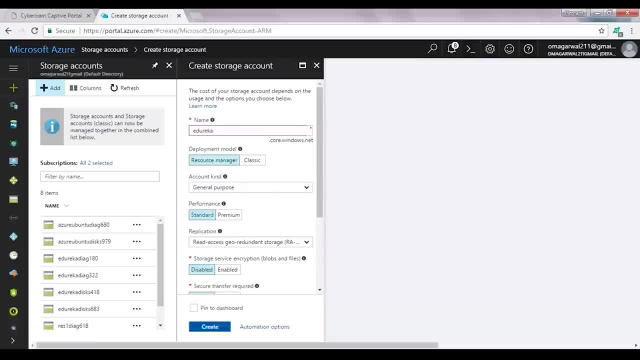 entering the value. So let's give it the name called edureka-01.. So this is taken. Let's give it name as Azure edu. right, This name is available. Alright, so the performance would be standard because this is a demo. 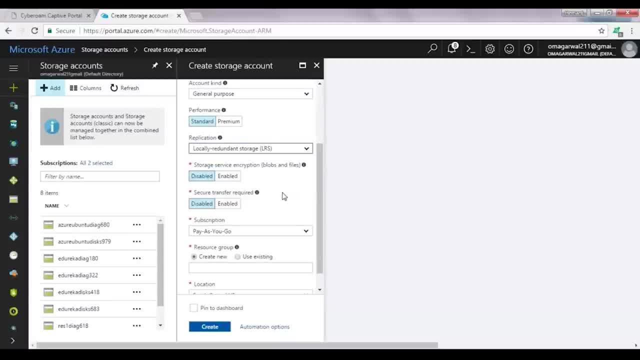 Replication is not required. So I'll say locally redundant storage Storage service. encryption is not required, Secure transfer is not required And subscription is pay as you go. Okay, Resource group: Let's select edureka-01, because this is the resource group. 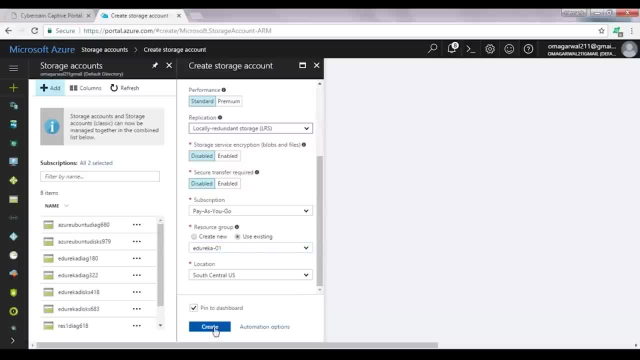 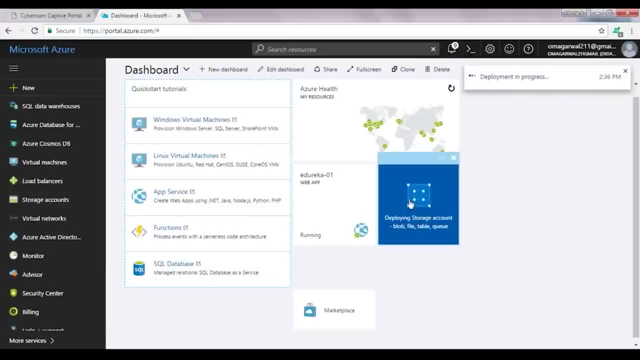 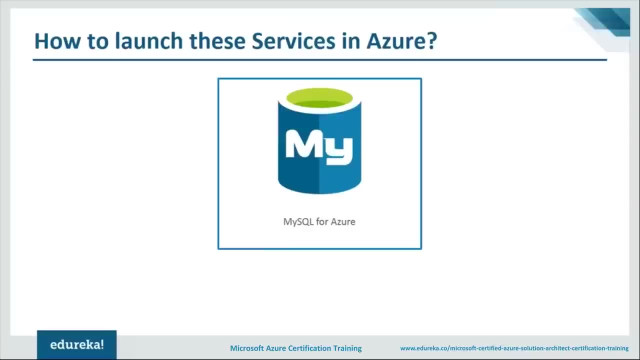 that I selected earlier. right, And let's spin it to dashboard. So we'll click on create. Alright. So my web app has been deployed already and my storage account is also being deployed. Alright. So this was about it. Let's go on. Let's see for our MySQL now. So for MySQL. 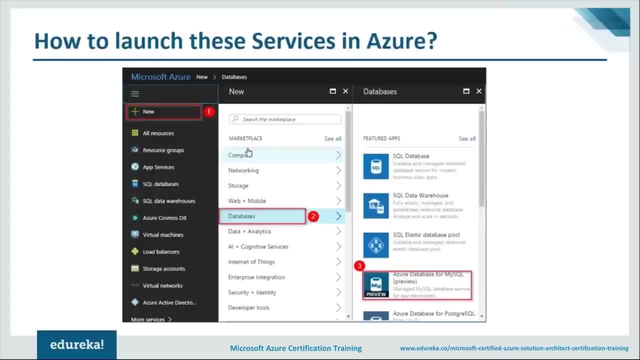 let's see what all we have to do. So we will click on new. We will click on databases and then we'll click on Azure database for MySQL. Alright, And that is about it. Let's go back and do that. So we'll click on new. 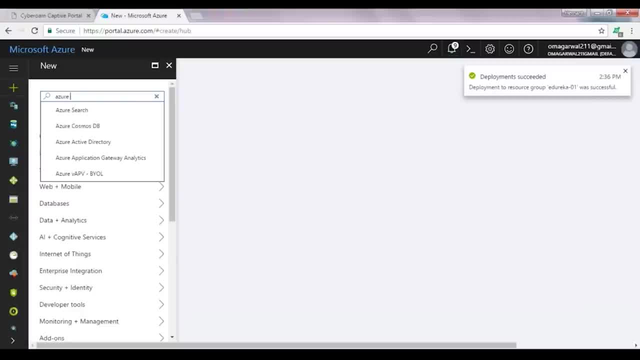 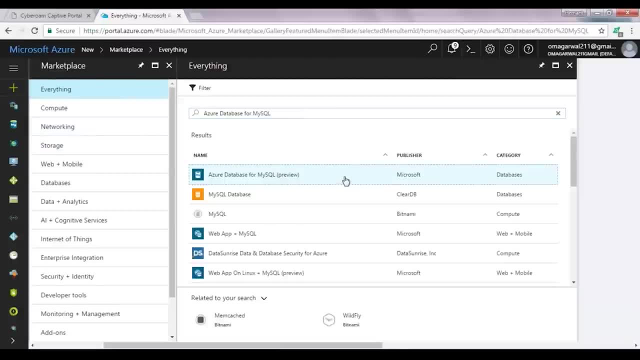 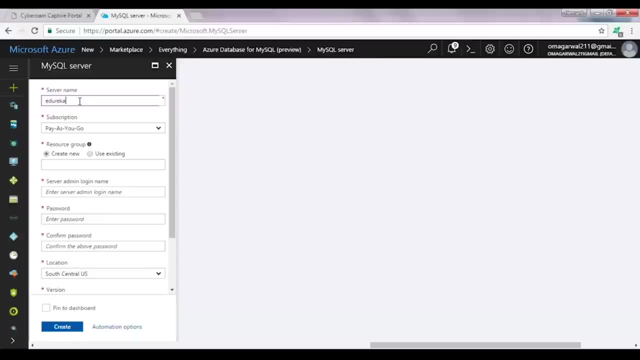 We'll search for mysql. Alright, Here it is. So I'll click on this and I'll click on create. So here it is. I have to enter the server name. Let's enter the server name as edureka-01.. It is available, It's. 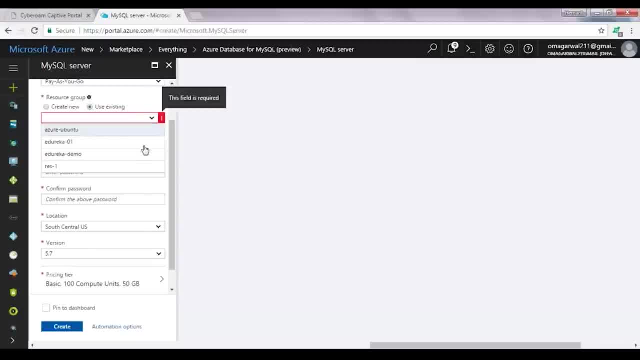 good, The resource group should be the same. So let's select edureka-01.. Server admin login name. Let's give it as edureka Password. Let's give it edureka-1234.. Confirm the password: edureka-1234.. And it is asking. 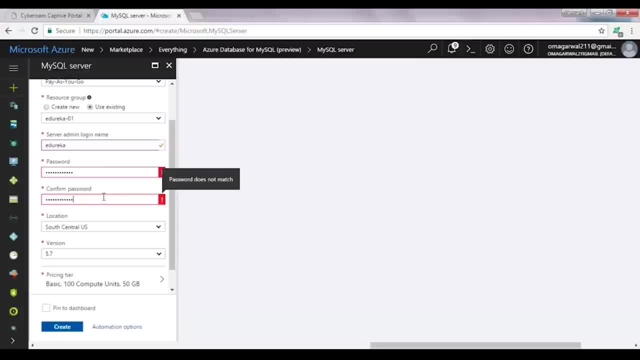 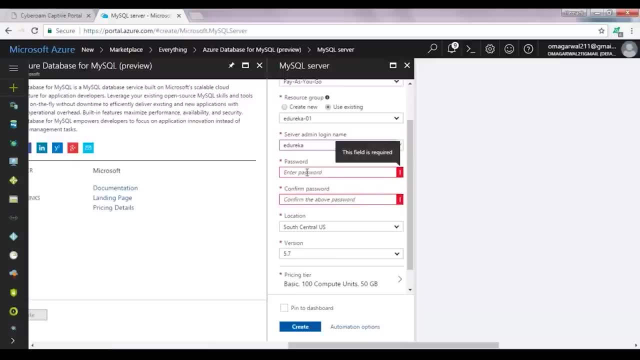 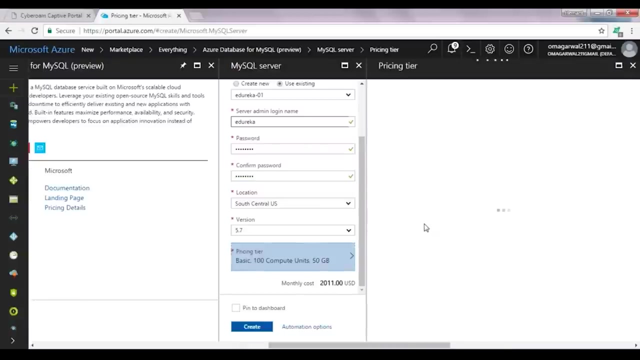 me some special character, So let me add the special character as well. Okay, So basically, you cannot have the login name in your password, So let me change the password to edureka-1234!. Same in the confirmation. Alright, So this is available now. The location is South Central US. Version is 5.7.. Pricing: 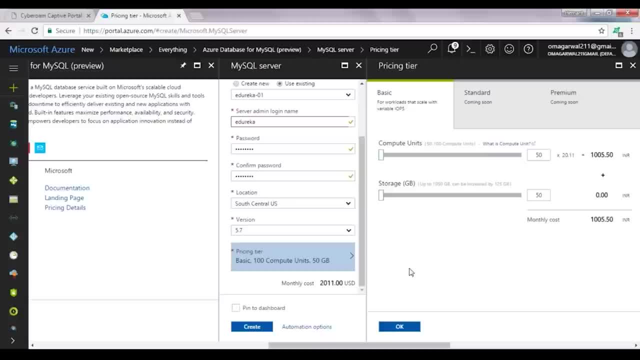 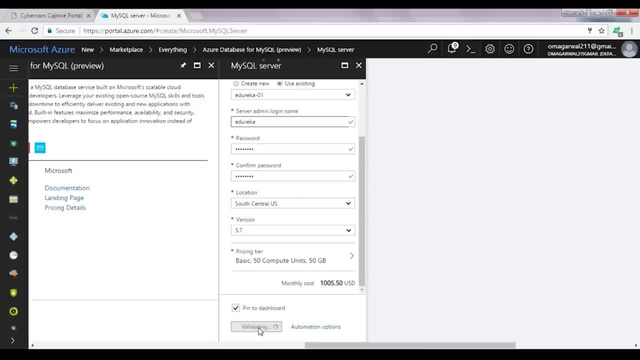 tier. Let me see if there is something more or less. Alright, I'll take this, I'll click on. okay, Pin it to dashboard and click on create. It's pretty simple, guys. You would know when you will do the hands-on on yourself. So the pricing tier can be the minimum if you are using it. 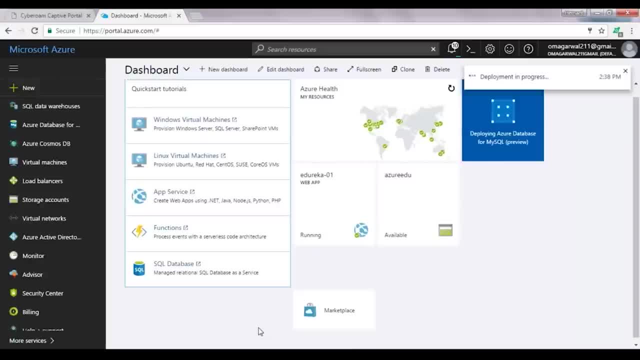 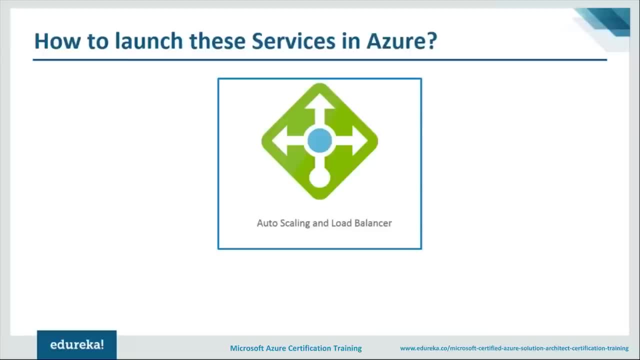 for demo, or if you are creating an application which is for global scale application, So you can choose the pricing tier according to that. Alright, While it is applying, let's move ahead. So let's come on to the auto scaling part now. So, basically, we have to configure our web app to auto scale as and when required. 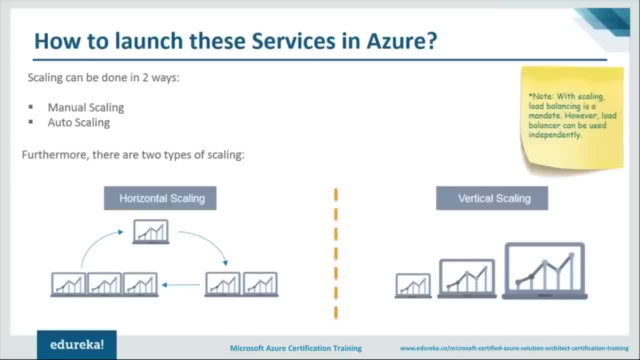 So let's see how we can do that. So let's understand the types of auto scaling first. So basically, there are two types of scaling. One is called horizontal scaling and one is called vertical scaling. So horizontal scaling is when you are increasing your order types. This is slightly different in Manchester, and 330 if you're in Mexico, because when you're buying a product from you, you're getting a further specific order right. So if you're getting a unit hourly or a unit or per month- something like�� inamı in Casous- you're. 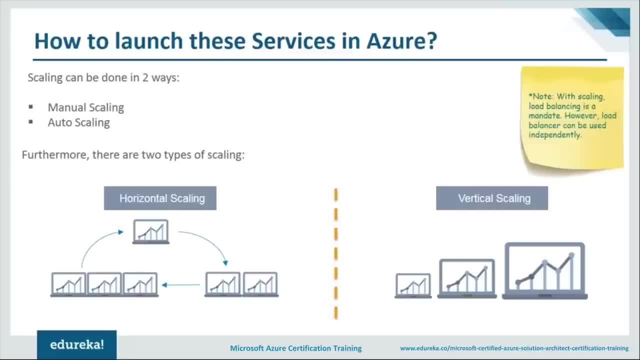 getting additional orders at the drop-down, and that makes all that easy to do. So we let's learn a bit more. Let's stay increasing the number of servers that you require. Say, you have an i7 server, for example. all right, 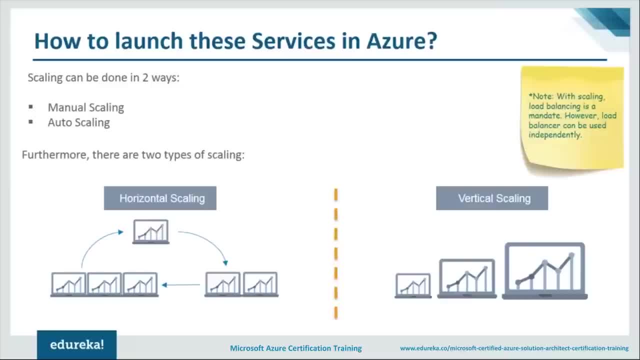 Now the usage goes up, so you take two i7 servers, and if it again goes up, you take three i7 servers, right? So this is what horizontal scaling is all about, right? Let's come on to vertical scaling now. 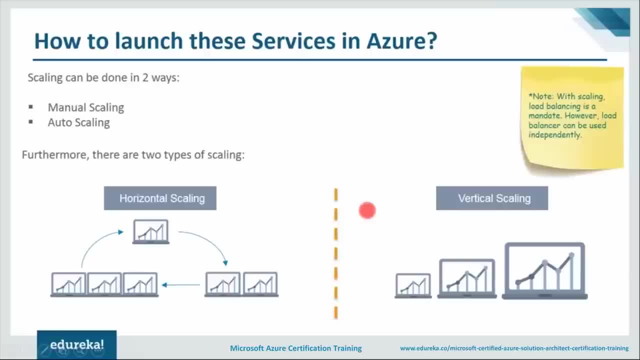 So vertical scaling is when you are increasing the capacity or the configuration of your system. Say, you were using an i3 system before right the traffic increases. so now you're using an i5 system, The traffic increasing. now you're using the i7 system. 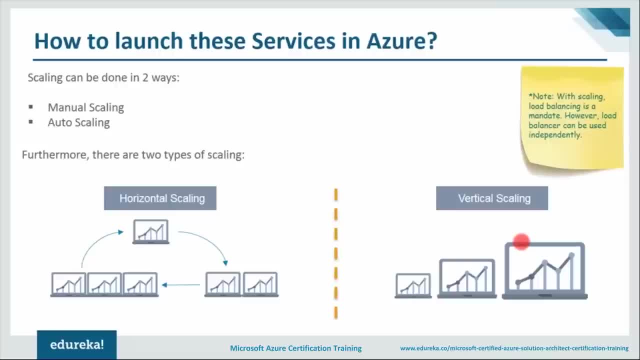 So you are having only one machine, but you're increasing the configuration of your system, Right? So these are the two types of scaling which exists in auto scaling Also. the other way is manual scaling, So you can also manually scale up your number of instances. 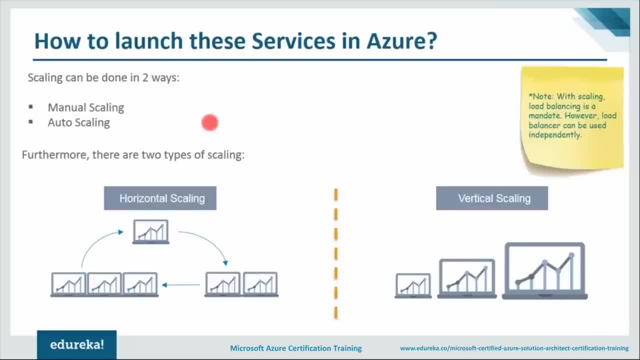 or the configuration of your system right. So the way to do that is to manually go into the servers, change the pricing tier and you are set. This is how you manually scale Auto scaling. I'm going to tell you in a couple of few slides. 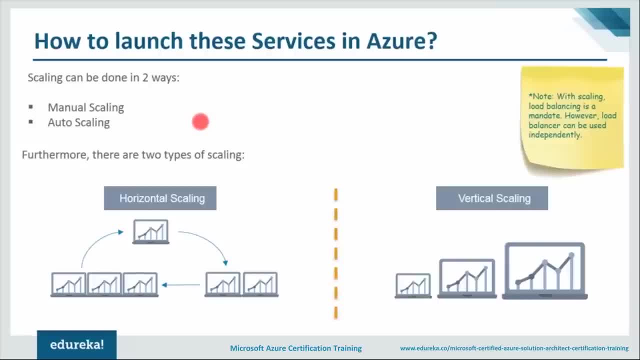 Also, guys, when you are auto scaling, like I said, load balancing is automatically attached to it. All right. so when you will be auto scaling in a web app, you don't have to configure the load balancer. The load balancer is configured automatically. 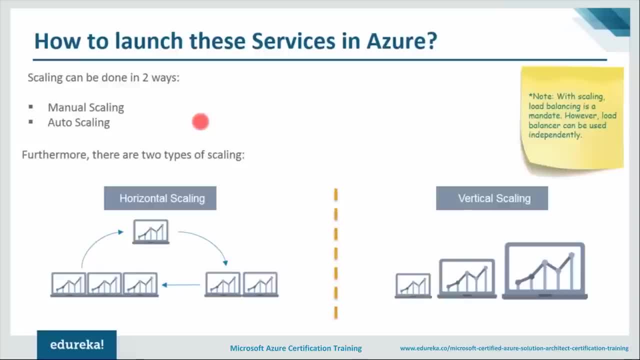 and set automatically for you to be used. all right, Because it doesn't make sense to use auto scaling and not use load balancer, And that is the reason Azure has automated the process of attaching a load balancer when you're using auto scaling. 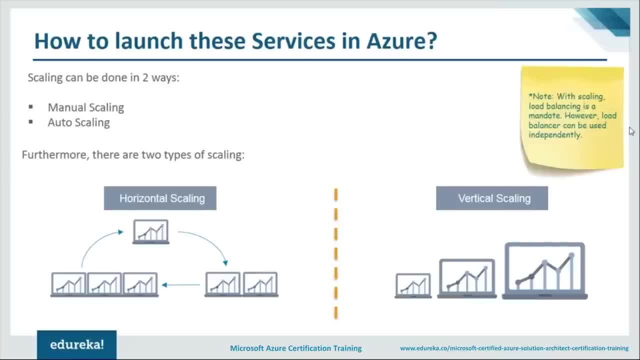 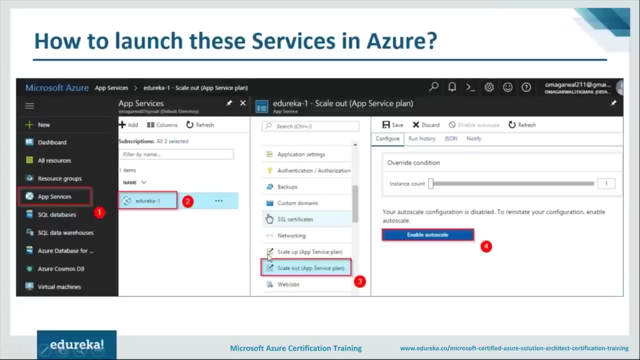 All right, moving ahead, guys. Let's see how we can launch this instance. So, guys, first you will click on app services, You will go to your particular instance that you have launched, You will go to scale out and you will click on enable auto scale. 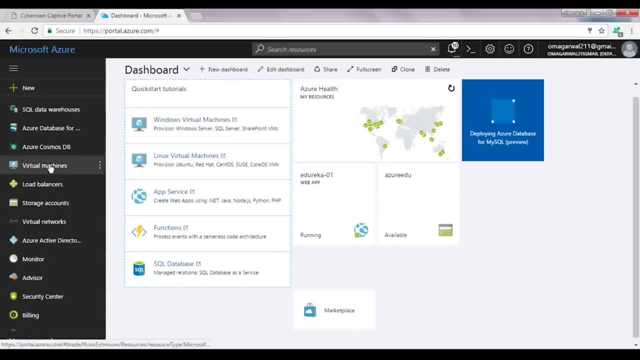 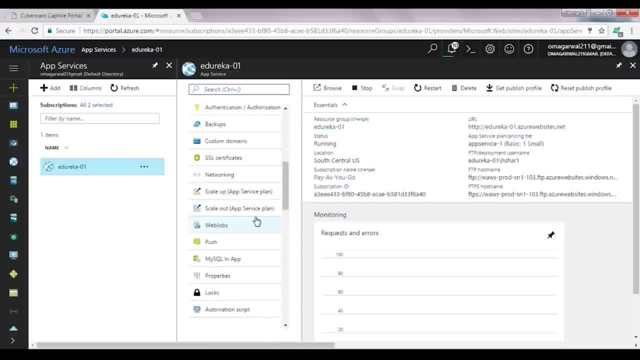 All right, so let's do that. We will go to app services, which is here. So this is my instance that I've launched. I click on edureka-01.. I'll go down and, as you can see, I have two options. 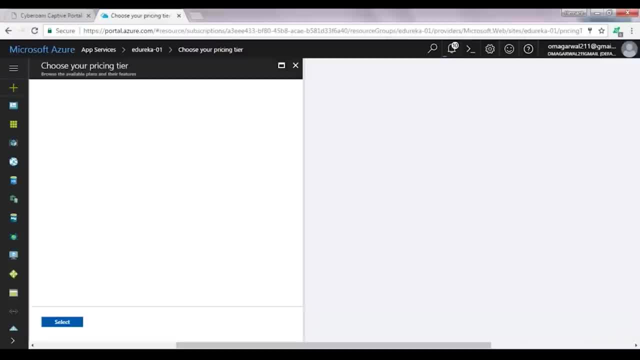 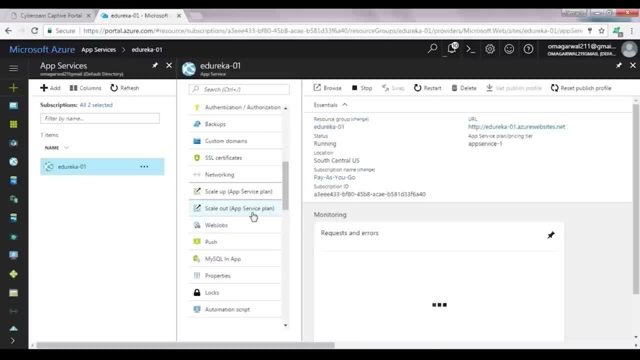 I have scale up and I have scale out. When I click on scale up, you will see the pricing tier, so I can increase the configuration of my system. right, But this is not what I want. I want to scale out, which is: I want to increase. 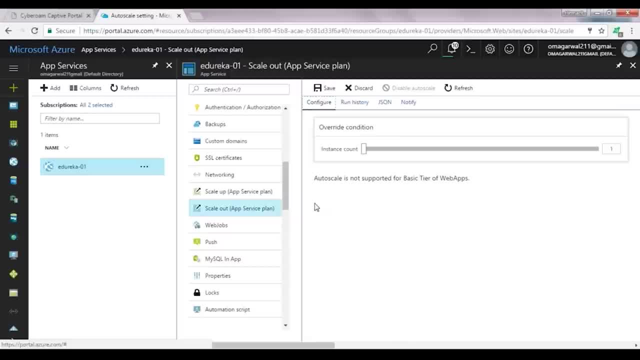 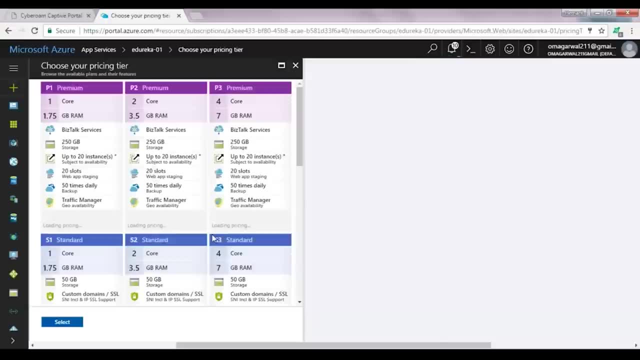 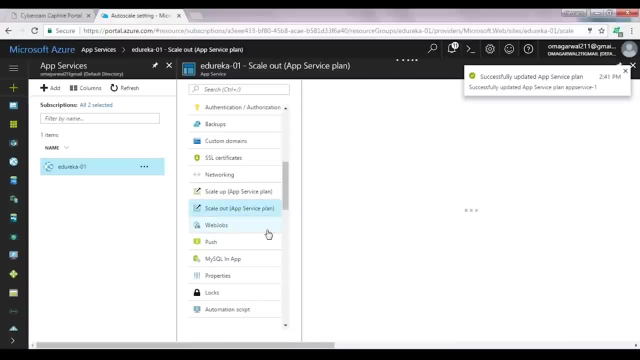 the number of instances running right now. right, So it says auto scale is not supported for basic tier of web apps. Okay, so let me change my, let me change my configuration, All right, so if I go to scale out now, 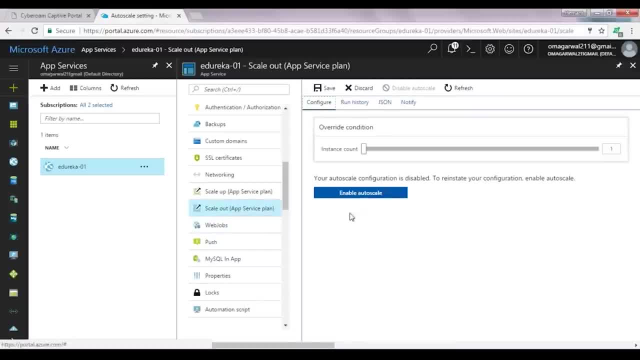 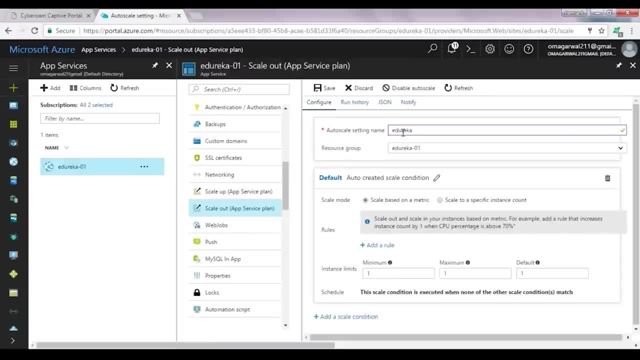 you can see that I have the option to enable auto scale, So I will click on enable auto scale and then let's give it a name. Let's give it a name as edureka-auto, All right, so my auto scaling property name is edureka-auto. 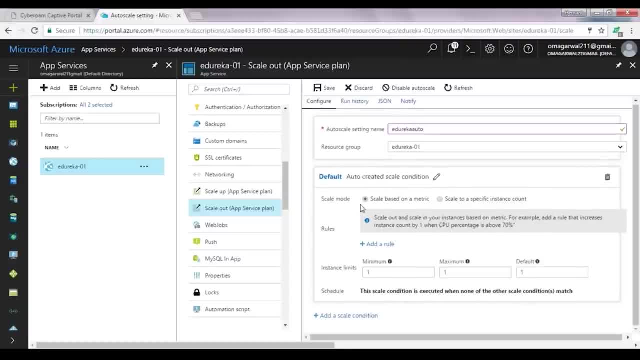 The resource group is edureka-01, right. So now you have an option to scale based on a metric, which is based on, you know, some statistics, like the CPU usage or the memory usage or anything, right. And the other one is scale to a specific instance count. 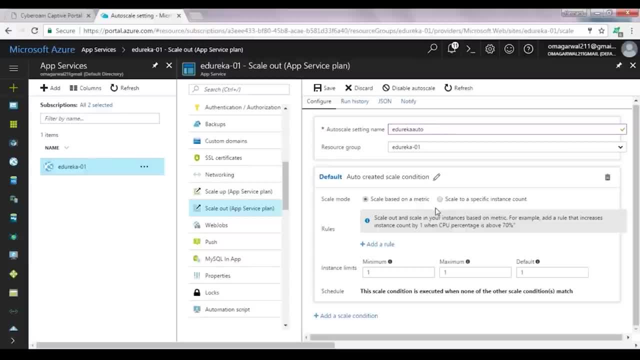 So, for example, whenever the traffic increases, say you were one instance, now like increase to five instances, all right. So these are the two options. We'll go with scale based on a metric and scale out and scale in your instances based on metric. 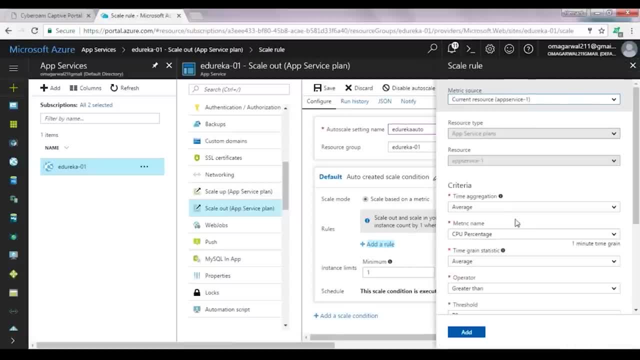 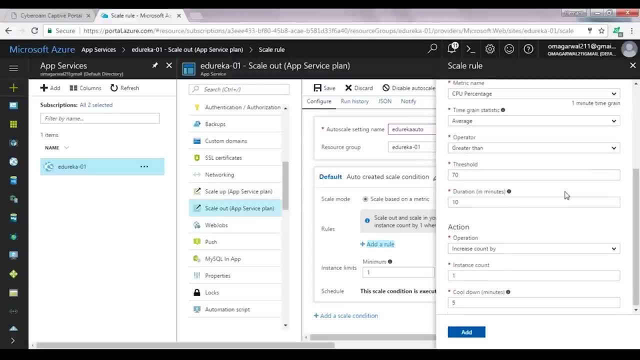 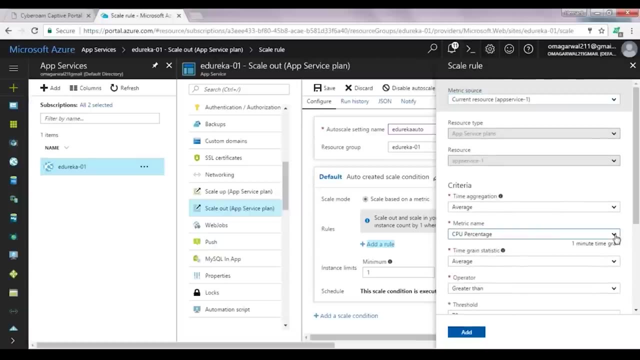 All right. so let's add a rule. Let's add the rule as in: what we want, what kind of metric Do we want to monitor and scale according to right? So, as you can see, the time aggregation is not something we should be worried about. 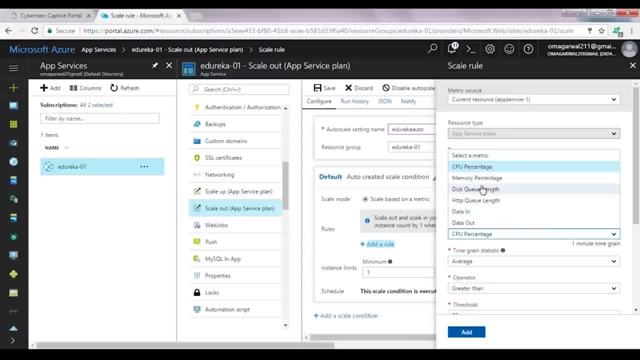 Okay, guys, so these are all the metrics that you can actually monitor and scale according to. You can scale according to the memory percentage. You can scale according to disk queue, HTTP queue, data in and data out, right, So let's, for now, keep it simple. 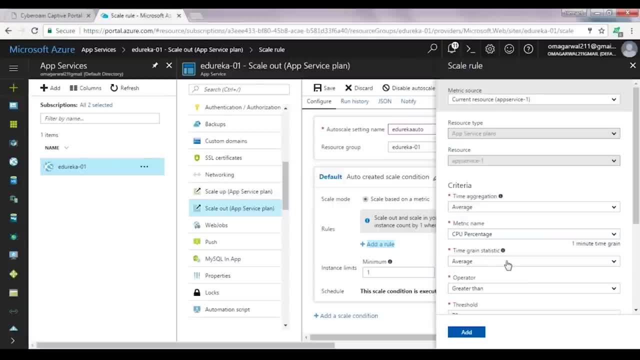 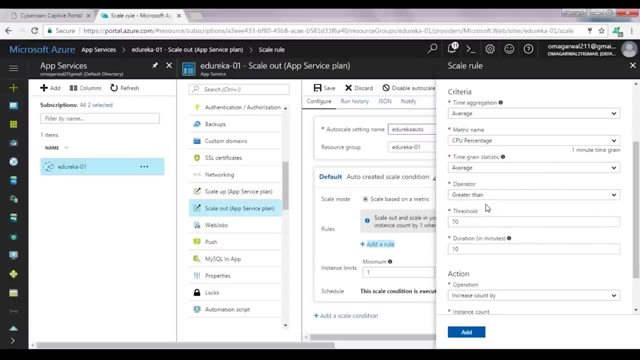 and scale according to CPU percentage, right? Uh, the time is not something you should be worried about, and the operator All right. so what should be the conditions? So should it be greater than, or should it be greater than or equal to? lets keep it at. 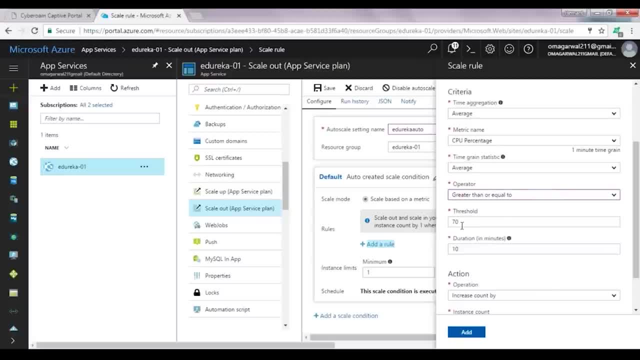 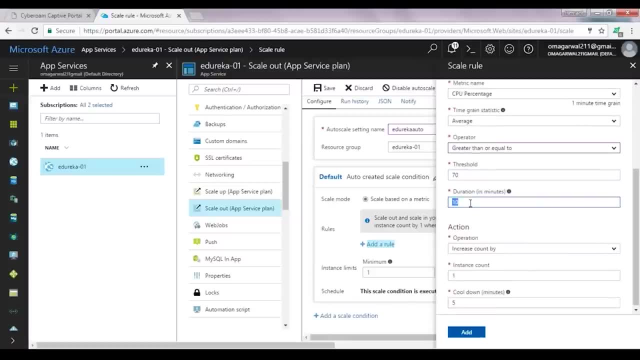 greater than or equal to. So whenever the threshold is greater than whenever the CPU use, it will go greater than or equal to 70 for ten minutes. So you can set this as, say, two minutes. all right, Okay, let's. so it says that. 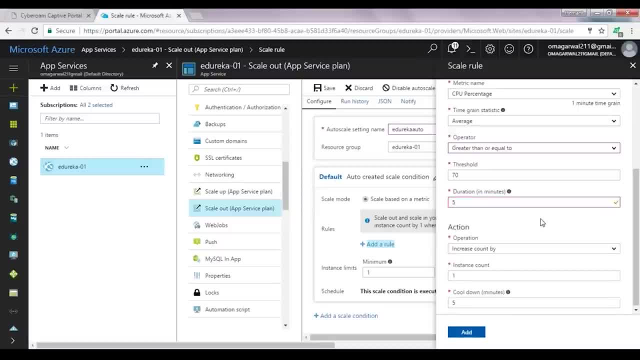 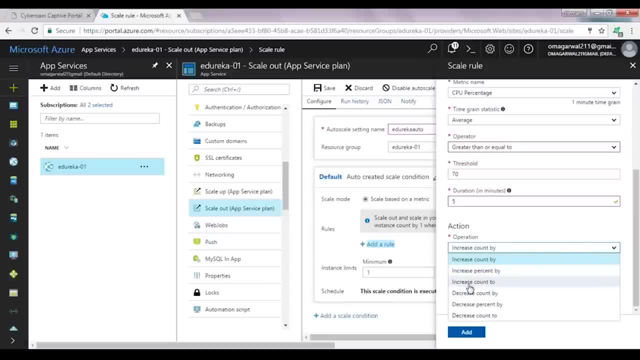 it should be between 5 and 7.20,. okay, So let's keep it at 5.. Increase count by. so let's see what all options we have here. So you can increase by percentage. you can increase by count to, as in: if you were 1, you can increase it to 10, right? 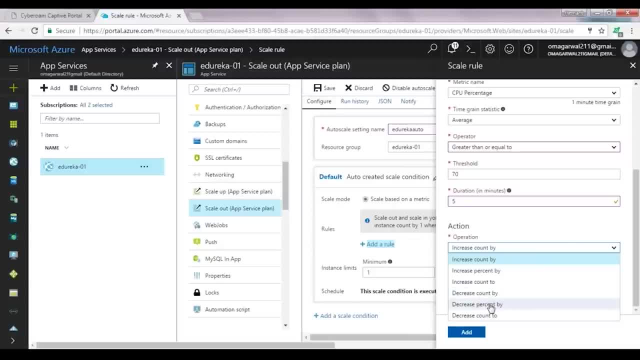 and you can decrease the count or you can decrease the person by as well. Alright, so when you are auto scaling guys, you have to set two rules. One is the rule to increase and obviously one rule is there to decrease. So whenever the traffic goes down, you have to decrease your instances as well. So for 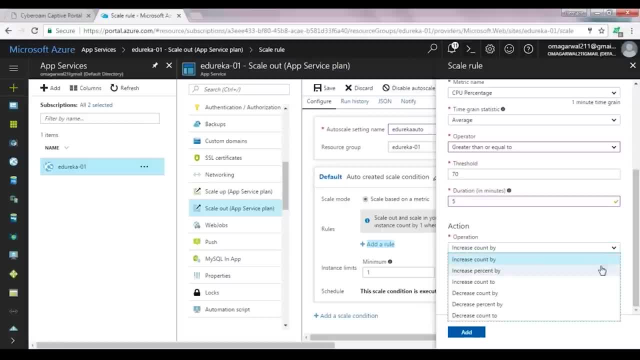 now we are setting the increase rule, So let's set the increase count by option. So how many instances should it increase? I think one is a fair number and cooldown is something that is actually there. when you are say you auto scale right, now right, and then say you auto scaled one min back and again the CPU. 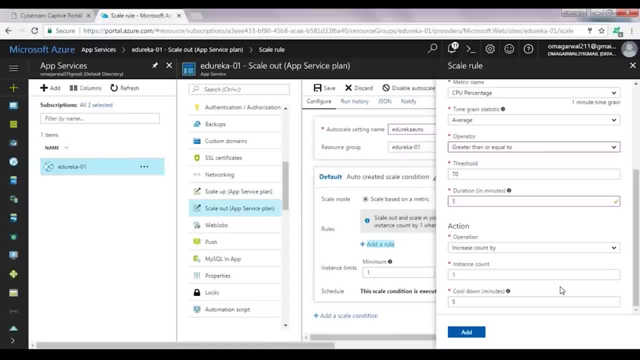 usage goes up. So, rather than going on and scaling up again, what you can do is you can wait for 5 minutes and watch the metrics, right, because it doesn't happen in a second that your CPU usage will go down, because there are a lot of services. 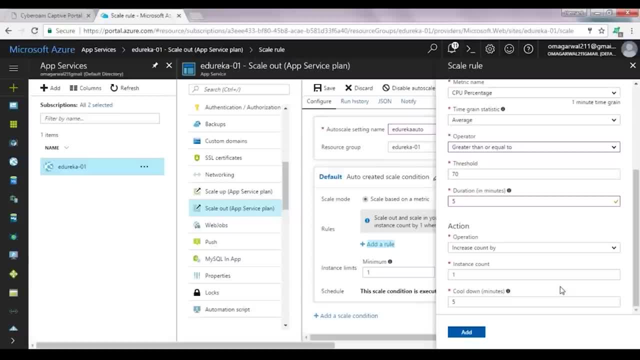 which are actually running right. So you can wait. once your new server has been deployed, you can wait for the traffic to be transferred to that server as well, and then you can see the metrics go down. Alright, for that we keep something called cooldown minutes. 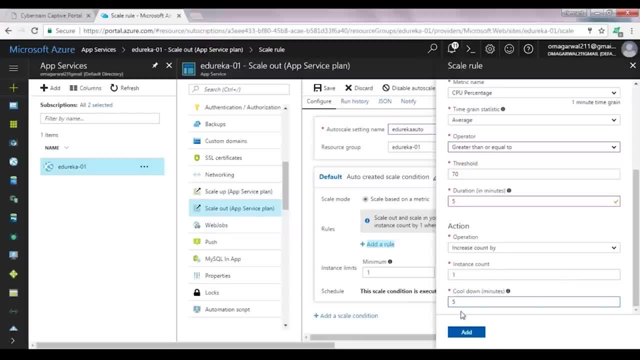 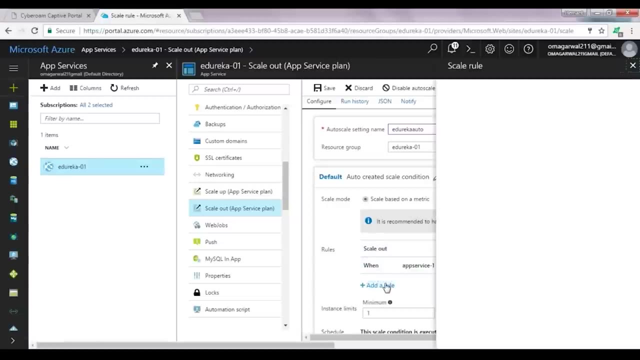 Right, so we have. the default is for five. let's keep it at five only. and now, this is it, guys. there's nothing else to configure. let's click on add. all right, so, as you can see, this rule has been set. let's add one more rule to decrease, so the CPU. 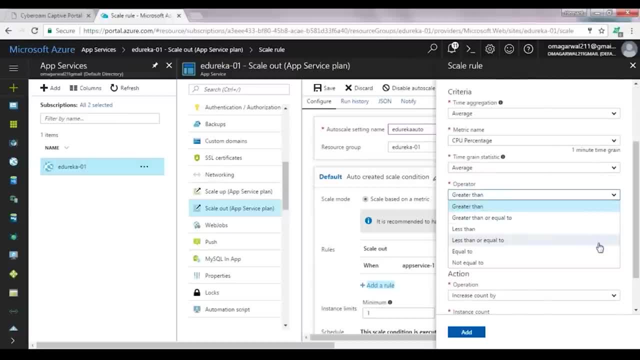 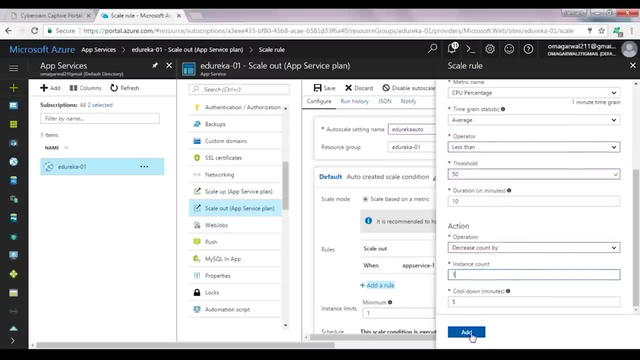 percentage is fine. the operator should be less than or less than right. so whenever the threshold is less than 50%, decrease, count by one instance and let the cooldown be this much, all right. so again the cooldown logic goes here as well. say you decrease an instance and again your CPU is still low because it. 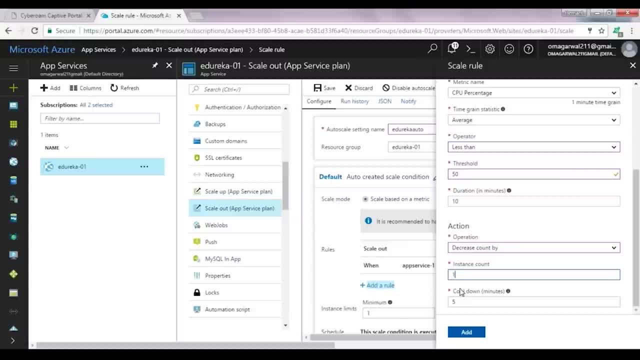 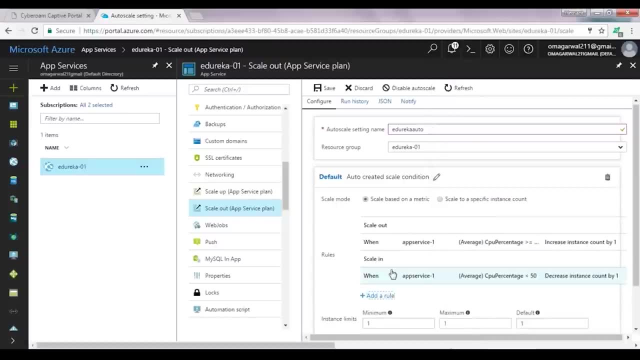 takes time for your traffic to get transferred to the server number. it has decreased down to right, so let's keep the cooldown minutes. so we click on add now. all right, so we have added the auto scaling rule. guys, this is it. there's nothing much to configure, actually, if you think about it. 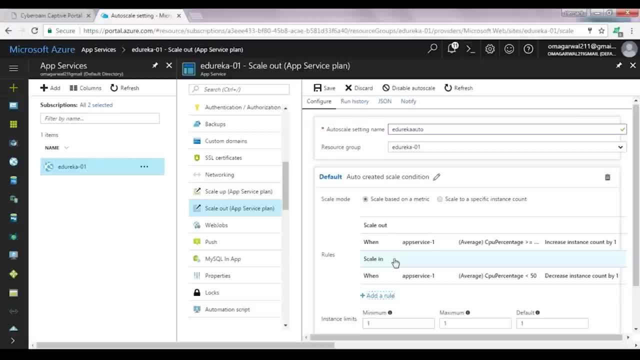 it's a very complex process but as your has given you the simplicity to do it very simplistic or a very English manner, because you just say, like I said, if the CPU this is above 70%, increase the number of servers by one right. so if you 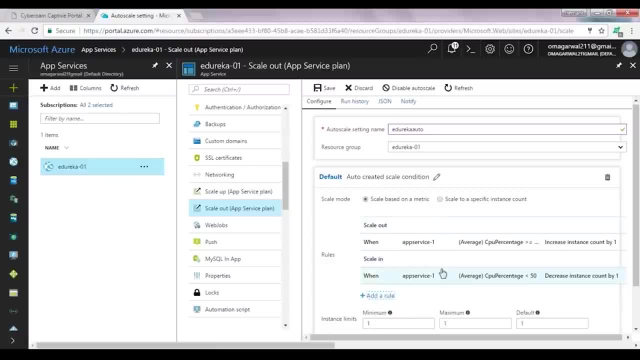 go here and if you don't know about auto scaling, you'll actually figure out what is happening. right and same is the case with scaling. so whenever your CPU is less than 50%, decrease the count by one, right. so, as you can see, you can actually read it here that this is what we have. 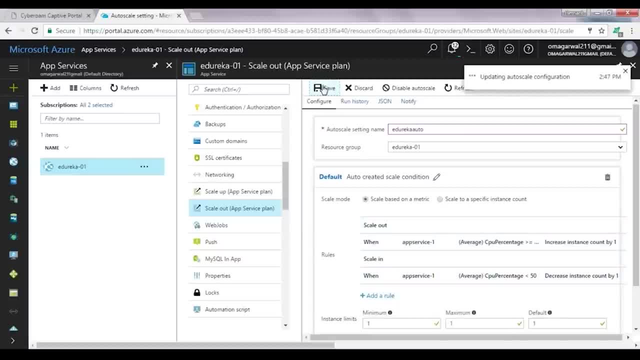 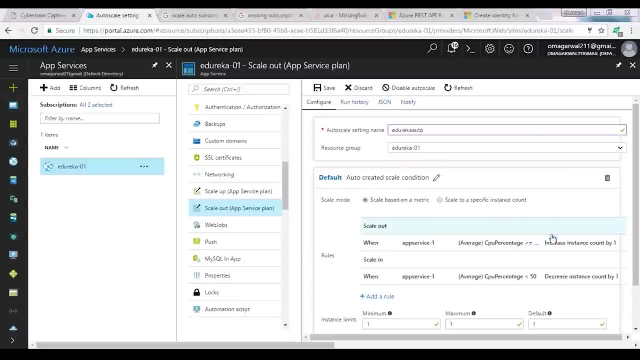 configured all right, so let's save this now. all right, guys. so this is how you auto scale your web app instance. now, since we are doing a demo, guys, we don't require the auto scale module for my application, so I'll just discard it for now, because I can't even demonstrate. 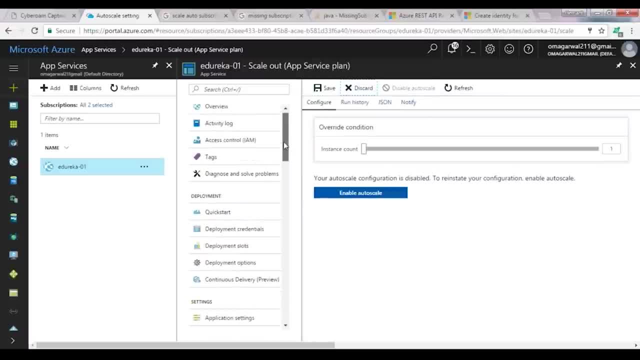 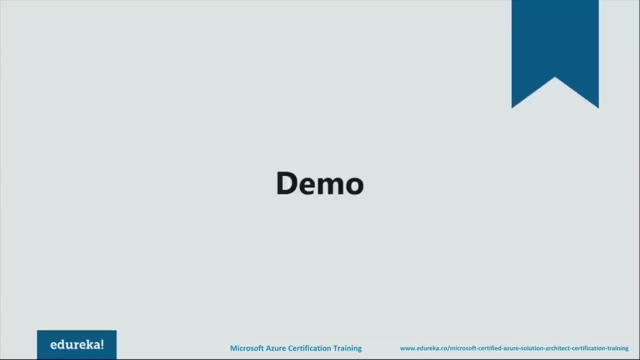 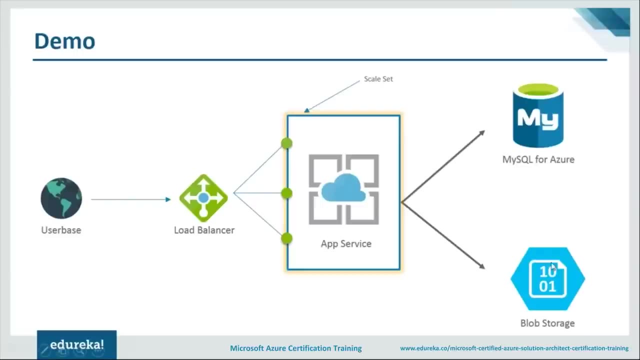 this to you, right? so I just showed you how you can auto scale. now let's go back and see what all is left. all right, so now we are going to do the demonstration. so we have launched each and every service. we have launched the app service, we have launched a blob storage and we have launched some mysql for azure. 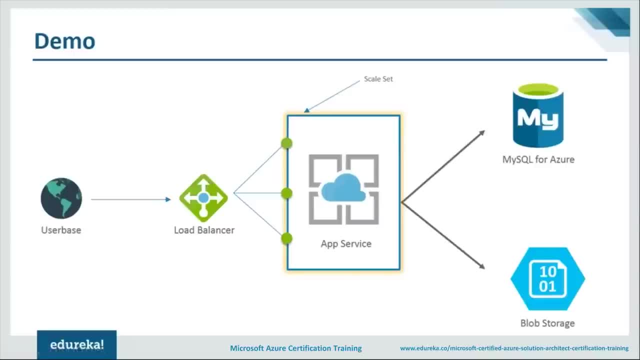 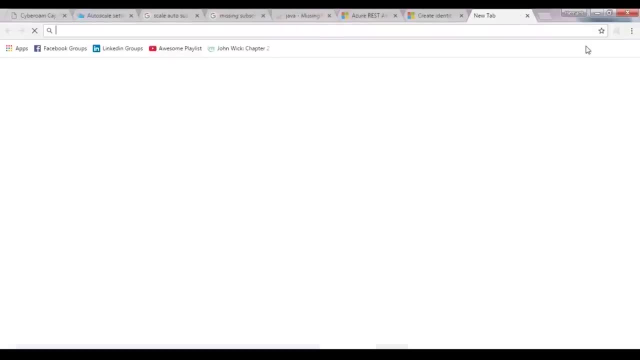 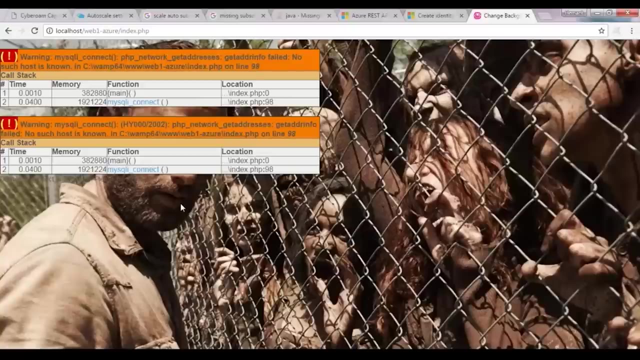 right now let's go back and check and deploy our website. so let me show you how the website looks like in my localhost. so my localhost is this: all right, okay, so this is showing me an error because, as of now, my code is not connected to my azure instances. 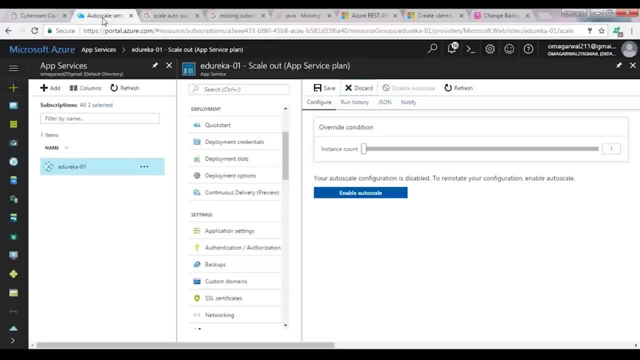 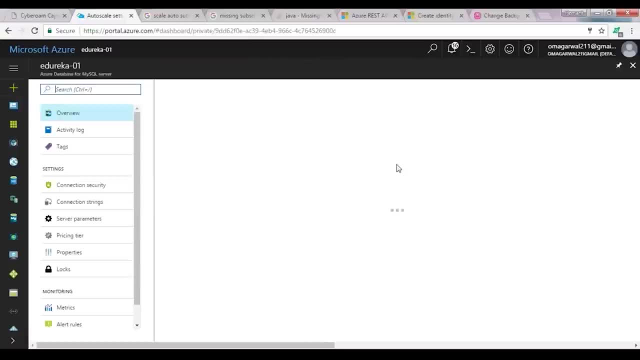 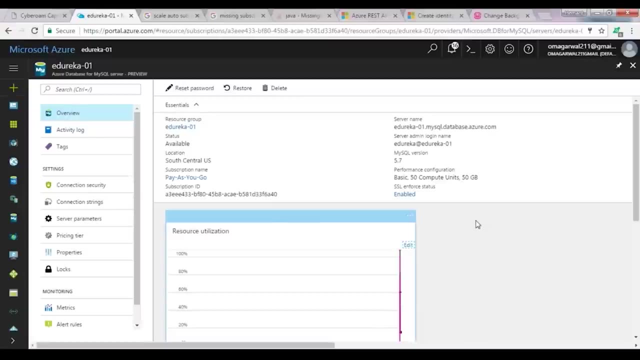 all right, so let's first configure our instances. so let us go to the dashboard and let's first configure our database. all right, now for configuring your database. the first thing that you have to do is connect to it. right now. the way you can connect to it: 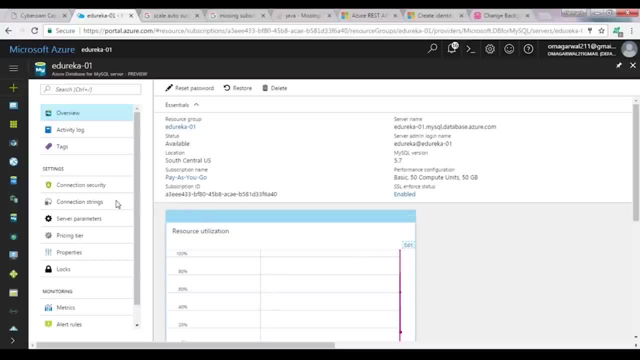 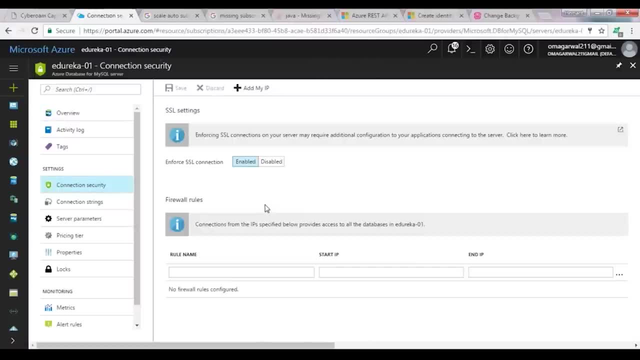 is using the command prompt. for that you have to click on connection security. now you cannot connect to your database just like that. you have to configure your IP address in the set of rules that are there for the firewall of the database, and when your IP address is listed there, then you can connect to the database. let. 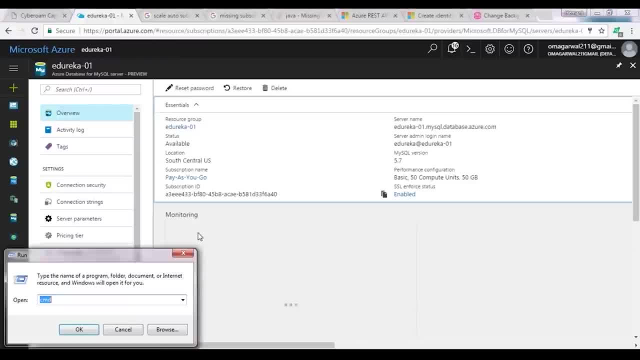 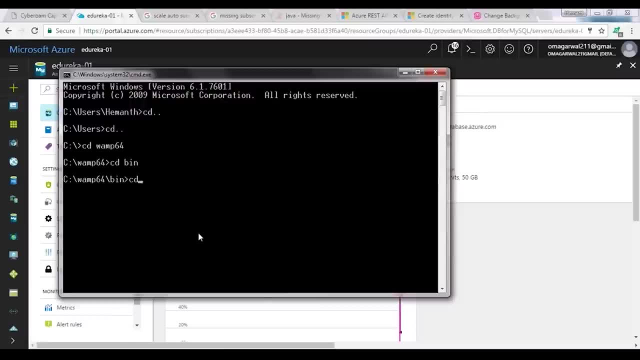 me show you how. let me show you that you cannot connect as of now. so I will launch the command prompt. I will go to my mysql installation, all right, all right, so this is my mysql installation, guys. so I will type in the command mysql-h paste and then the server name, which is this: I'll paste it. 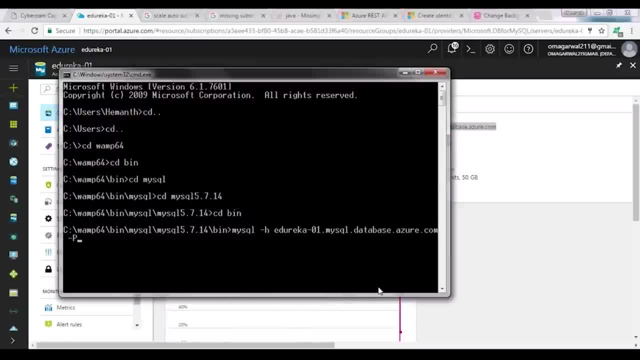 here. all right, then I will give the port number. so the port number is hyphen capital P. guys, don't forget its capital P. it's different than small p, right? small P is for password, capital P is for the port number. and then I'll give the username. 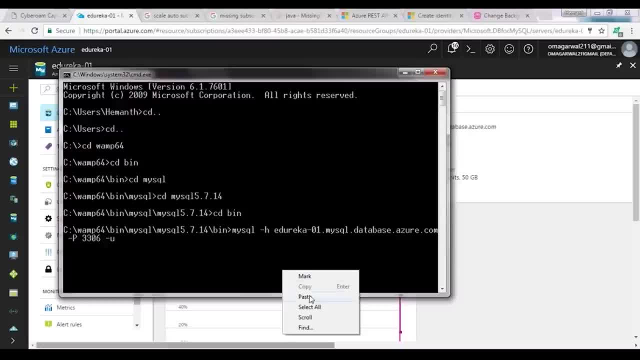 so the username is this. I'll paste it here right, and then I will type in the password and hit enter. enter the password, which is edu1234. exclamation: hit enter. see. as you can see, client with the IP address is not allowed to access the server. all right, so now what I'll do is I'll go to. 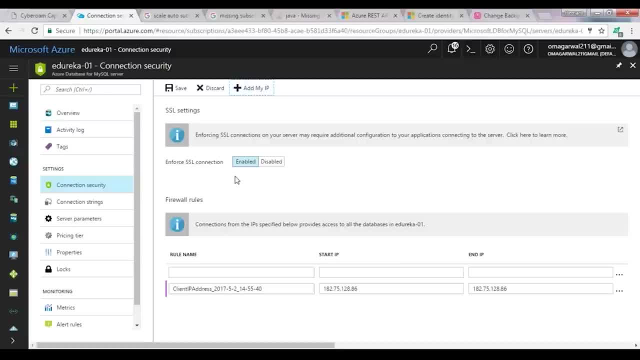 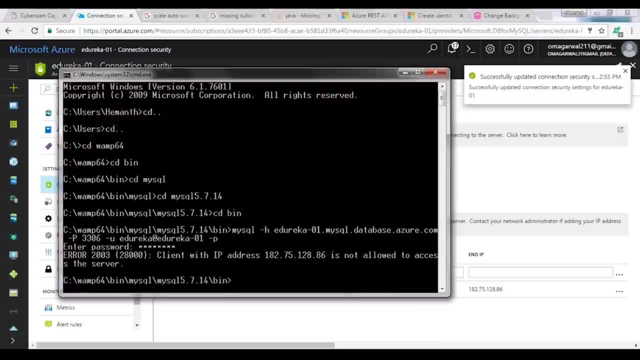 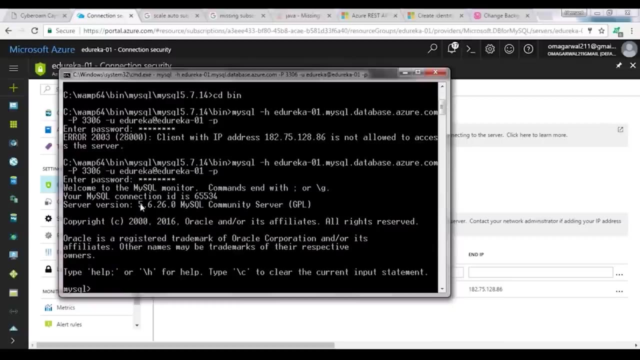 connection security. I will add my IP and I'll click on save so it says successfully updated connection security. let's go back to our command prompt, execute the same command again, type in our password and now, as you can see, I have successfully connected to my database. now I can create a database. 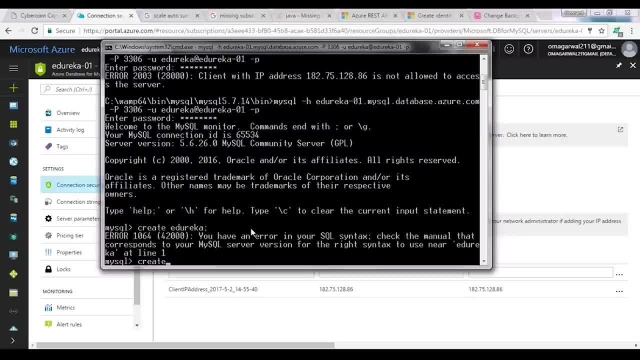 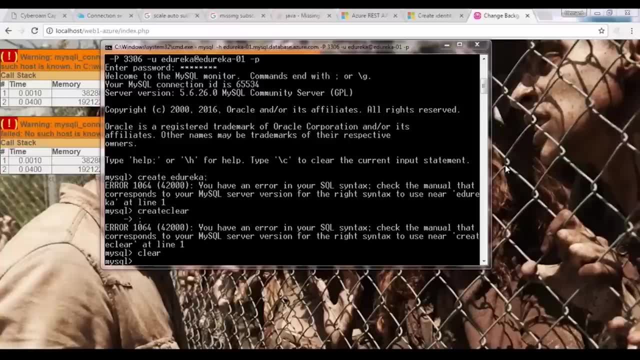 here called edureka. let me create a database, let me clear the screen. oh guys, I forgot, I'm working on Windows. so in Windows you cannot clear your MySQL screen. what a sham. all right, so if you are using Linux, you could have just typed in ctrl L and it would have been fine. all right, guys. so, as I was saying, 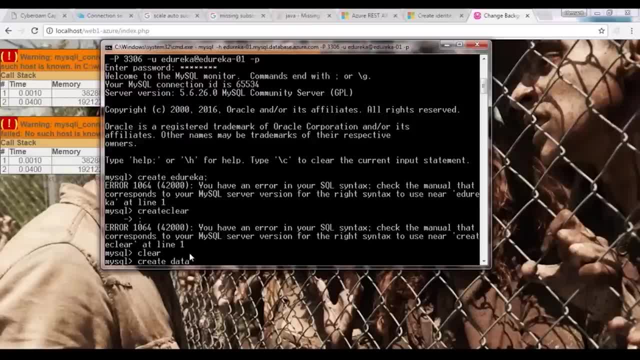 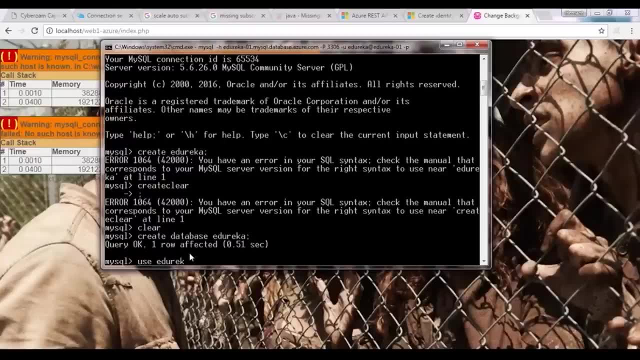 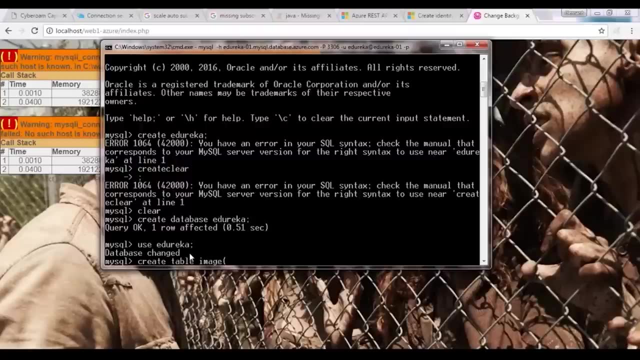 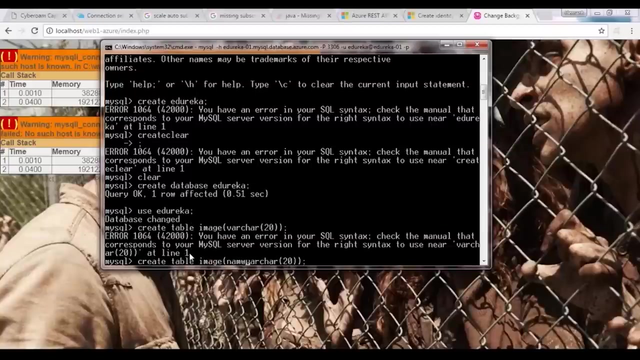 let's create a database called edureka. so create database edureka and that is it now type in use edureka, I'll create a table. let's create a table called image right and title name, as this one. second, my column name is name. alright, so I've created a table. so if I type in show: 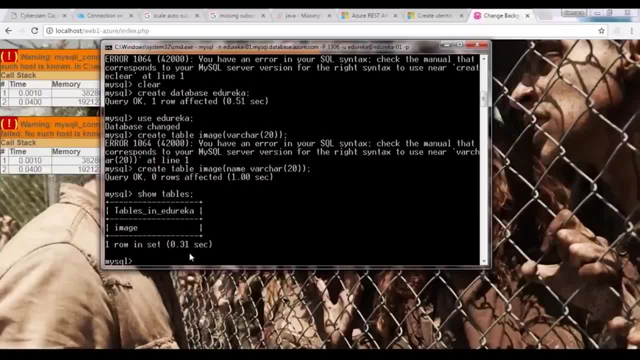 tables. it will show me the table name, which is image. alright, guys, so this is done. now I have created a table. at first, I created a database called Edureka in my MySQL, which is hosted on Azure, and then I created a table called image in it, and the table has one column called name. alright, so this is it. this is my. 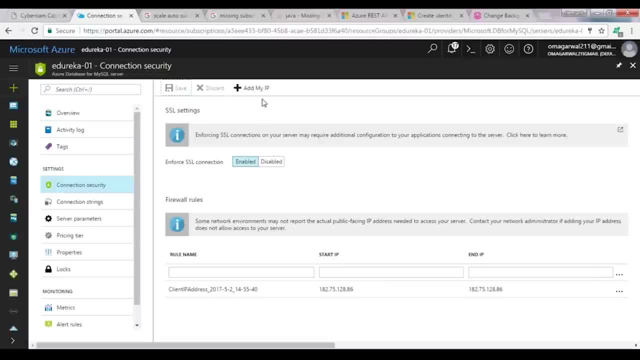 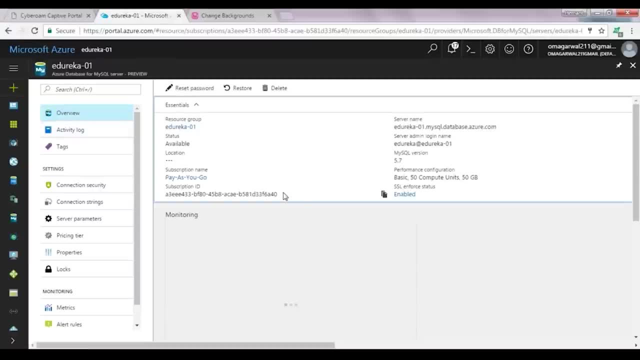 MySQL. so my MySQL has been configured now. alright, so my MySQL has been configured. now let me go back to the overview. alright, so my MySQL has been configured now let me go back to the overview. alright, so my MySQL has been configure. As you can see in the databases, it will show that there's a. 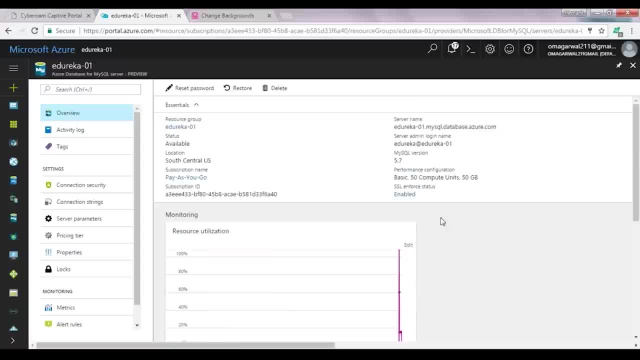 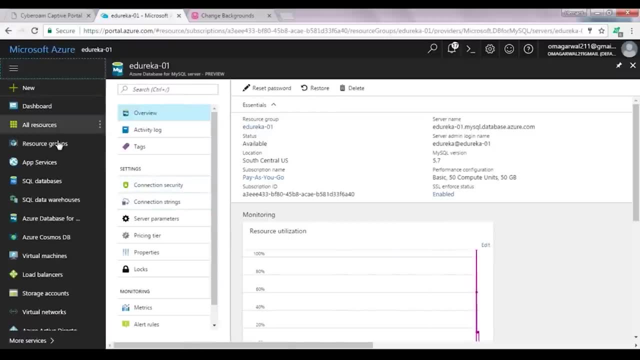 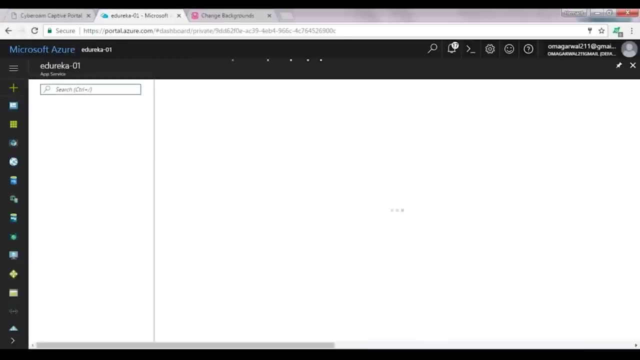 database called Edureka, which I just created. Alright, let's go back. You might have to add the web apps IP address as well. We'll do that later. Let's go to our web app now. Awesome. So we'll go to our web app and, guys, this is a web app. This. 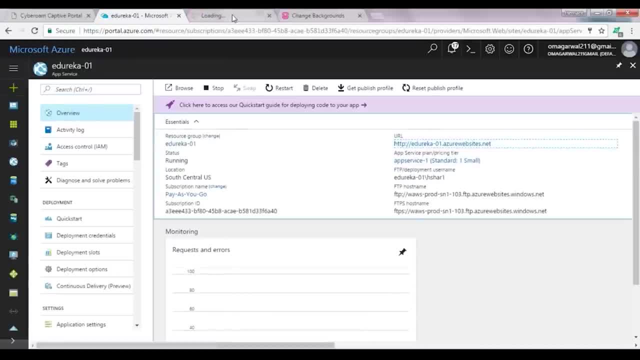 is the URL for your website. We'll click on this URL and you will see a welcome page. This is your welcome page. So now what you have to do is you have to upload your code over here. Alright, So the way you can do this is using GitHub. 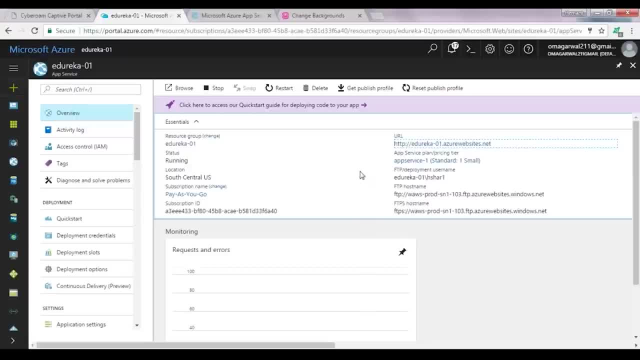 or you can do it using FTP as well. Now, I know most of you are from non-technical background, so you might not be knowing what GitHub is. So for now, what I'll be doing is I will be using a FTP software called FileZilla. 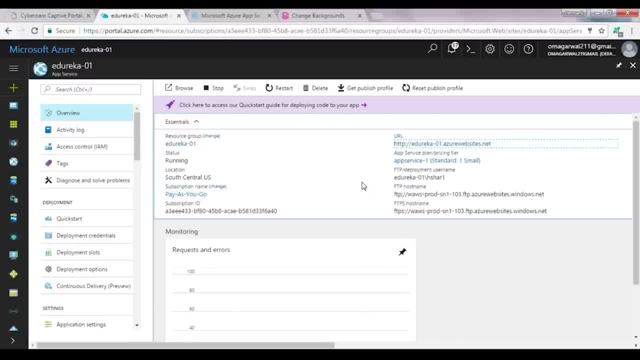 For transferring my files from the next session onwards, I'll be using GitHub, and for that I have actually there is a video in your LMS which is a short tutorial on GitHub, how to use GitHub, which is enough for a demonstration So you can go through that video before coming to the next session and then we 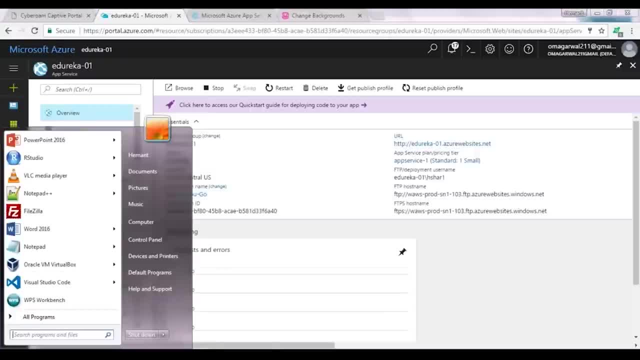 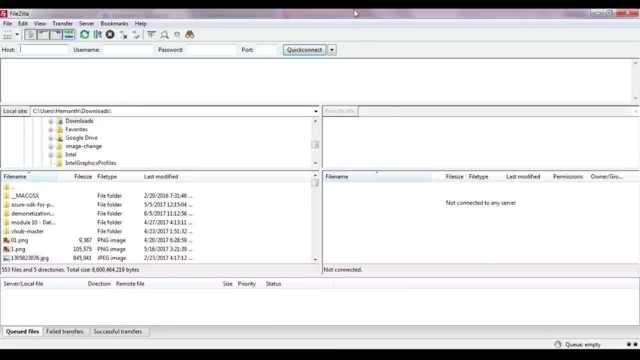 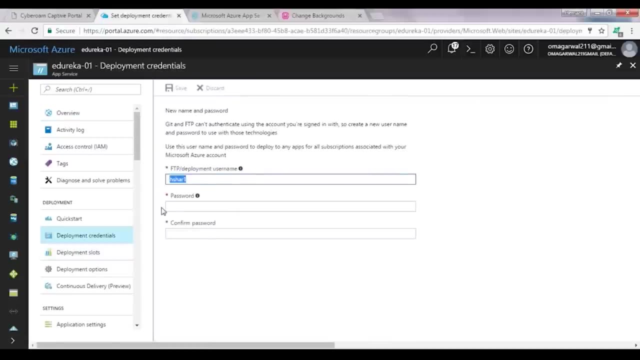 will be using GitHub. Alright. for now, let's use the FTP software, which is called FileZilla. Alright, so the way you can connect here is like this: So you have to create a deployment credential. Alright, so my deployment credentials is hr1.. Let's give it a password and the password could. 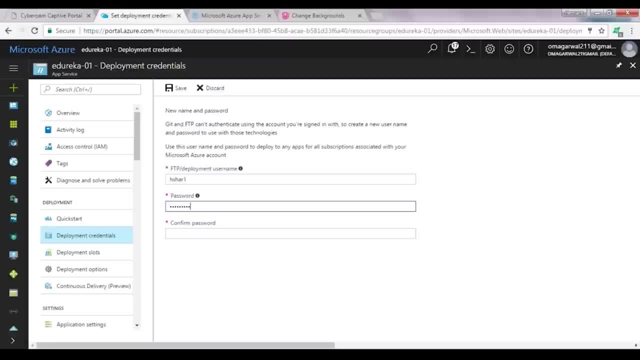 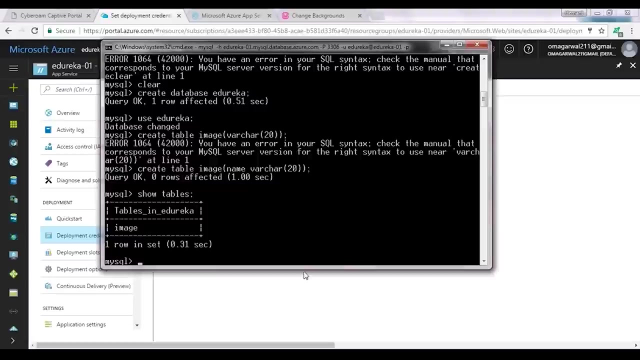 be okay, let me give as: heymonth199.. Alright, and over here also heymonth199.. Alright, let's click on save. or maybe this username is not available, so let me give it: hr12.. Click on save. Okay, let's try this again. hr12.. Alright, maybe I'm 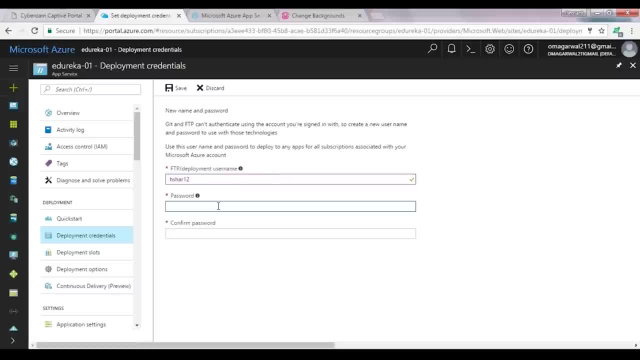 connected here. maybe that's why Let me exit it: Heymonth1994.. Hmm, let's click on save. Alright, so I get the error out of here. Right, so like we have successfully reset the deployment credentials now, Alright, so what we can do is 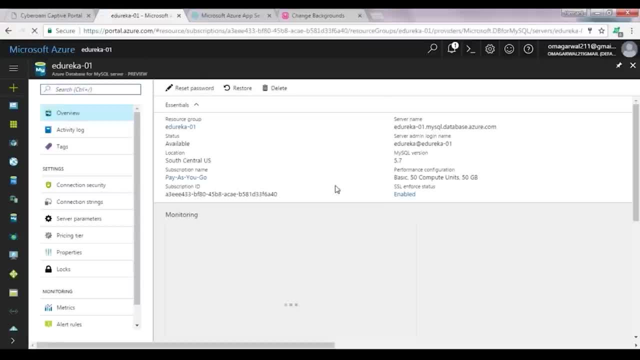 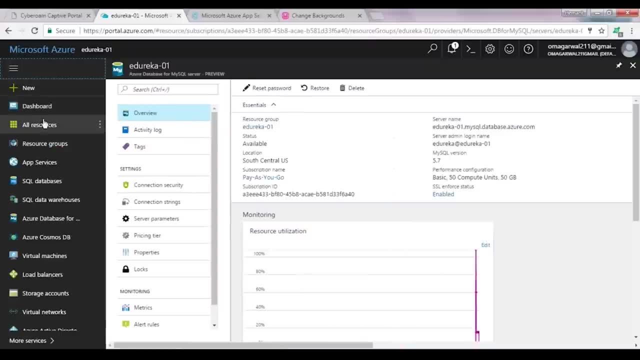 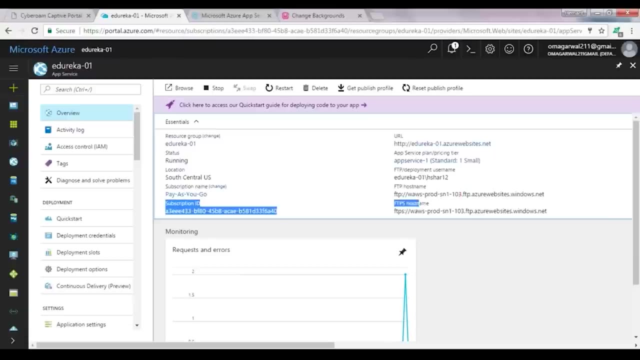 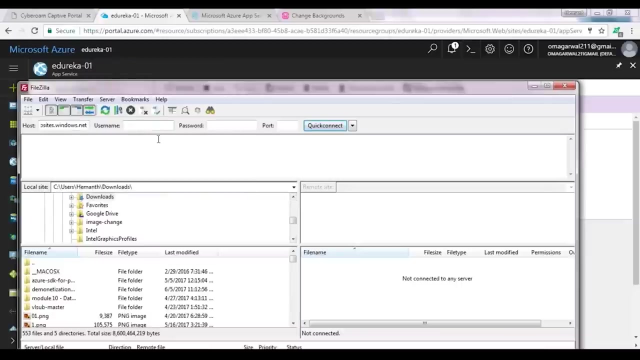 I will go back to my web app. Alright, so now I can get connected to my web app. I'll have to enter the FTP hostname, So it will go here One second. Alright, the hostname will go here. The username is hr12.. Password is: 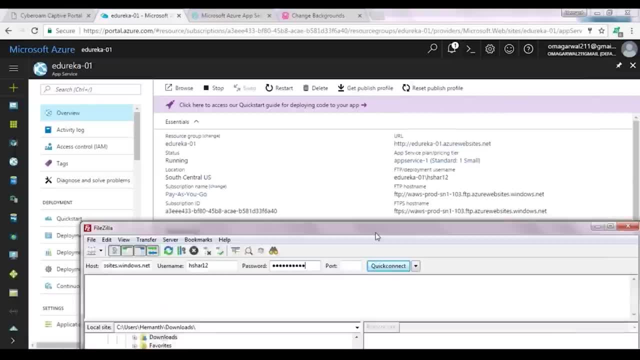 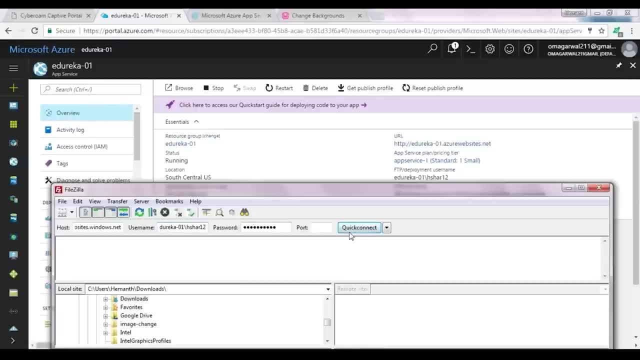 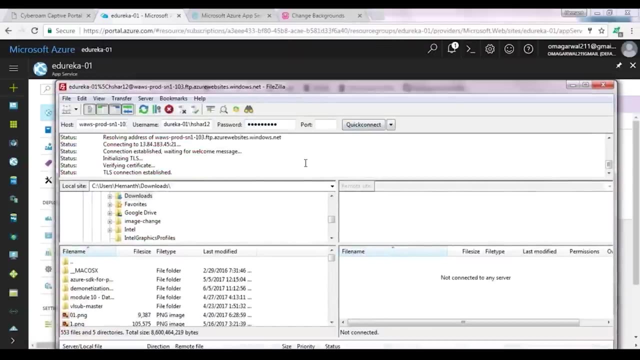 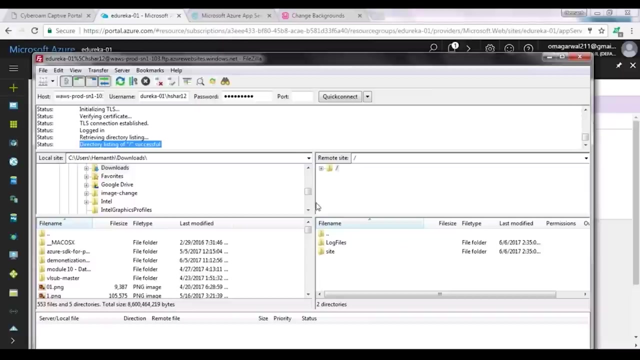 this Right and what else? Alright, the username is this. I'm sorry, The username will be this: Alright, let's click on quick connect. Alright, so, as you can see, we have successfully logged into our FTP channel. So over here you'll go on site. 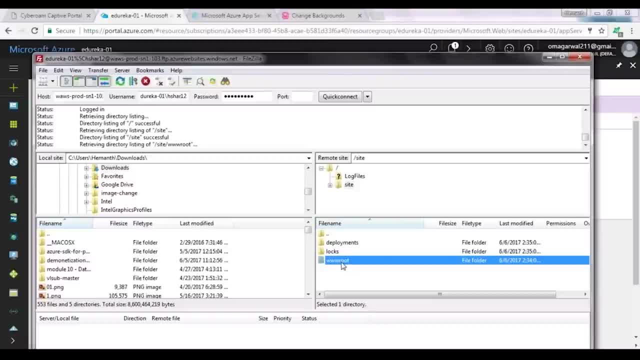 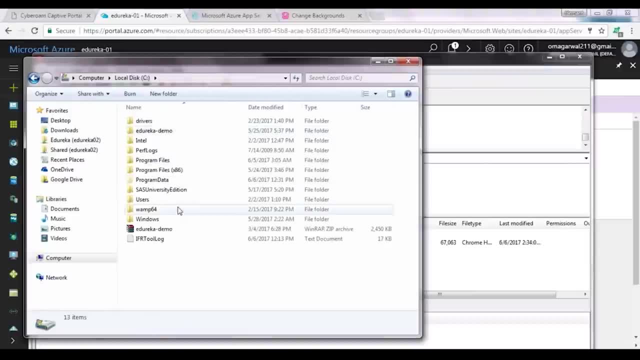 So over here you'll go on site. So over here you'll go on site. Alright, we'll go on wwwroot And then you can copy all your website files over here. So let us do that. My files are somewhere here, Alright, so let's copy the files now. 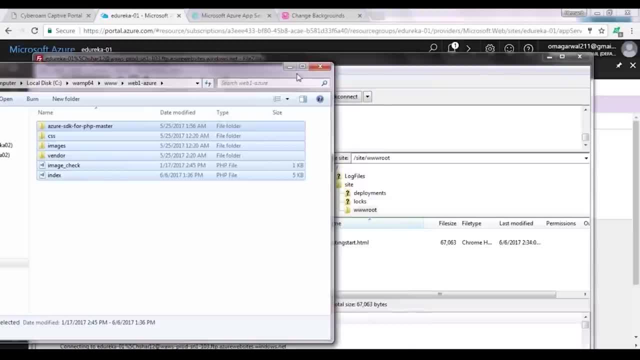 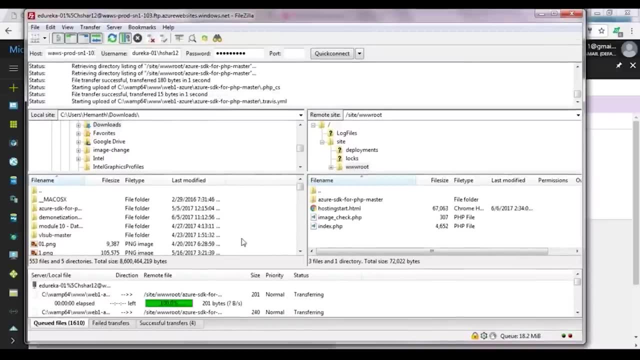 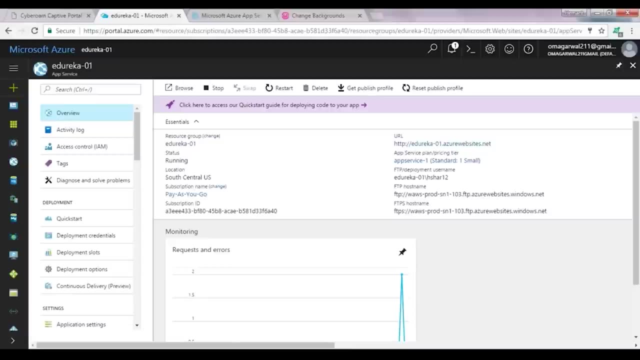 I can just drag and drop it over here And the process will start Now. it might take a while, So let us configure some other files while my website is being copied. Okay, so now what we can do is we will go to our dashboard and we can configure our 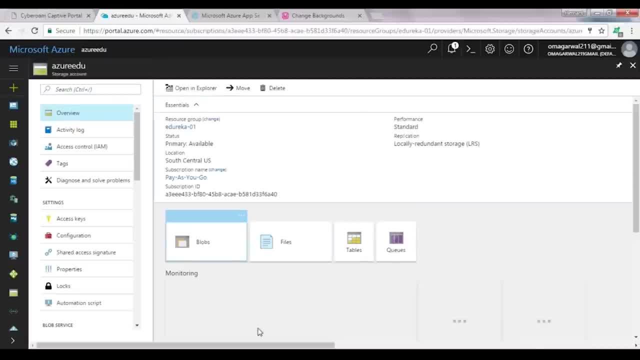 storage. Mind you guys, I might have to upload my code which in my web app, because there are some things that I have to change in the code, because the addresses and I'm creating new services right, So I'll have to change the services address in my code. So I'll do. 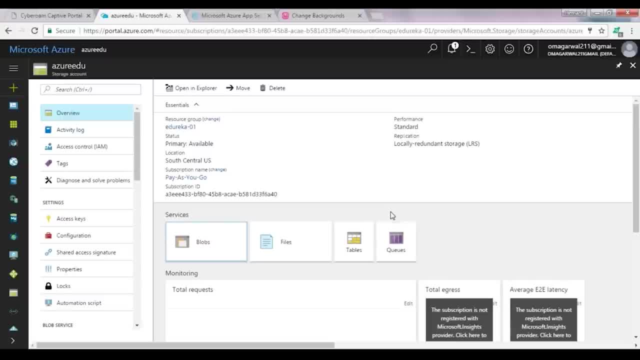 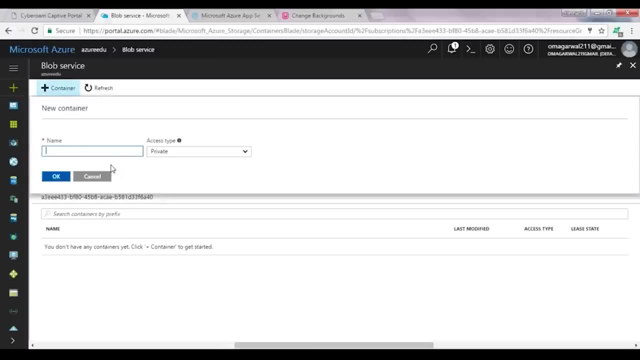 that, and then I will update the particular file that I'll be changing in in my web app. So let me just give me a minute, Okay? so now what I'll do is I will create a blob over here, I'll create a container, and the container name shall be hello and 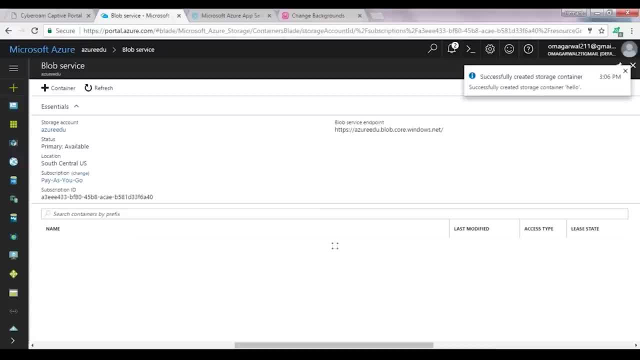 the access type will be container. All right, I click on okay. So I have successfully created a container called blob. If you go in properties, you will see that this is the URL for it, right? so let me show you the code for my website, guys. so 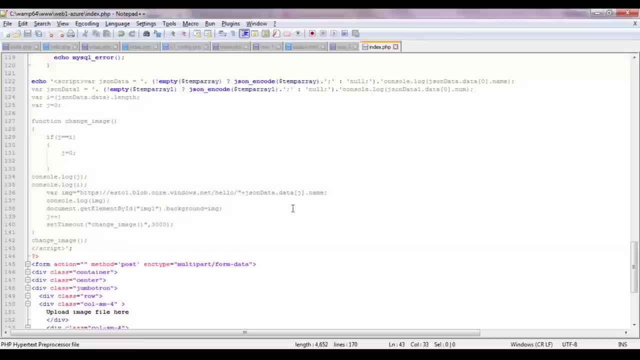 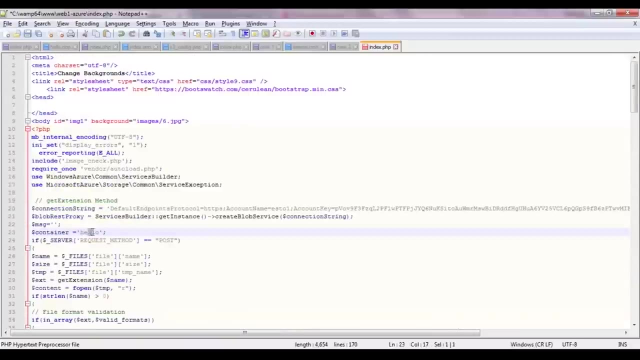 this is the code for my website. all right, now I'll have to change the URL at places, so let me do that, so it will get changed here. all right, then. my container name is hello, so that is okay. and now one more thing, guys. so whenever you are, 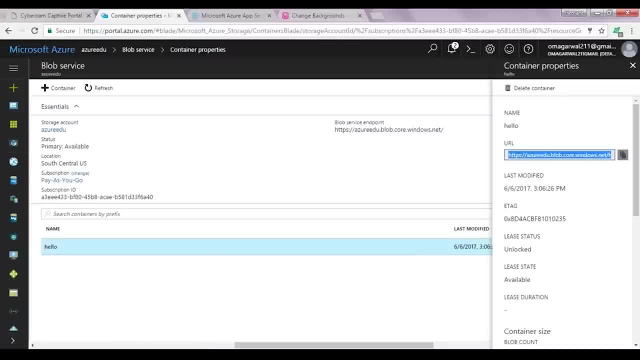 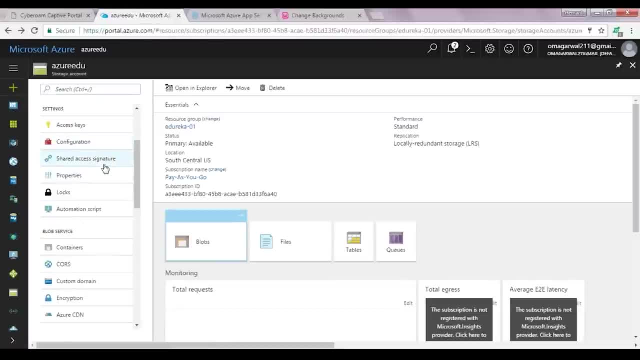 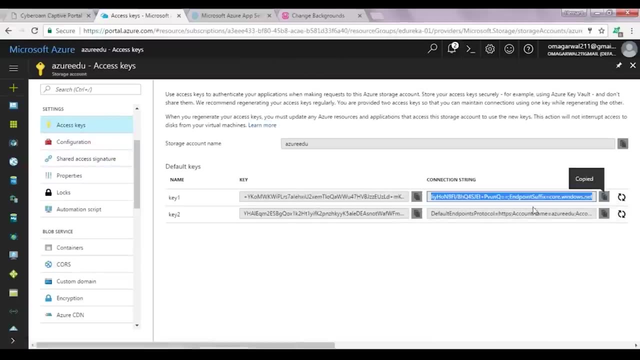 basically going to connect to your storage account, the order, your blob storage. you have to go here. I will show you. we'll have to go to access keys. so here is a key, right? so you, this is the connection string that you have to include in your code. I have copied it, I'll go here and I will include it in. 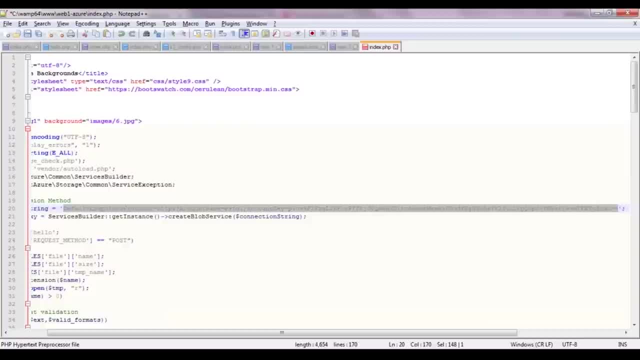 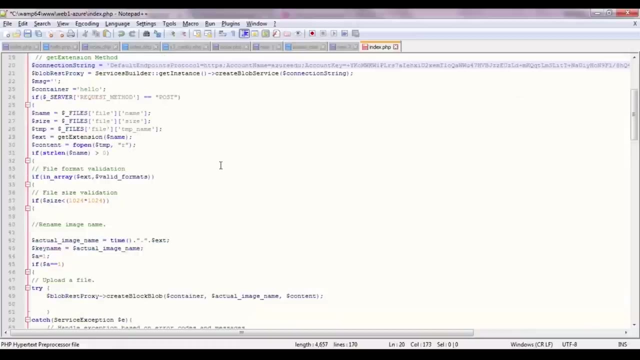 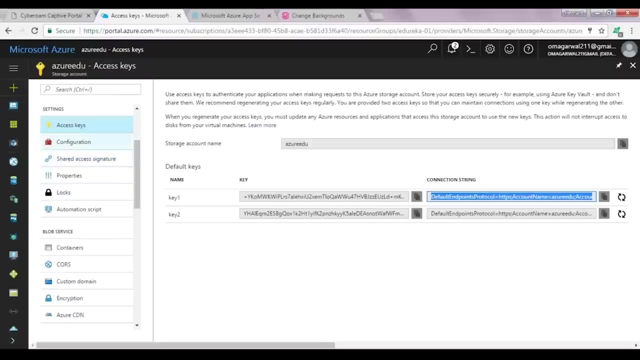 the connection string code. all right, so I'll control V and over here. you have to remove the endpoint suffix, all right, so this is not required. if you put this, it will not work. okay, I don't think anything else is required. oh yes, I have to change the database credentials as well, so let's do that as well. so your. 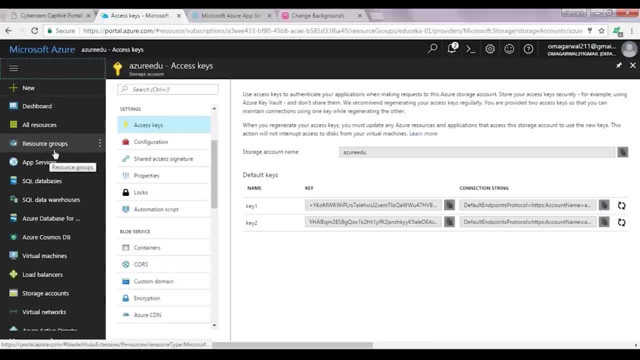 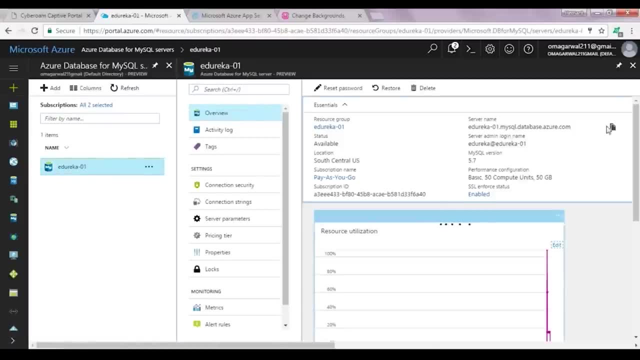 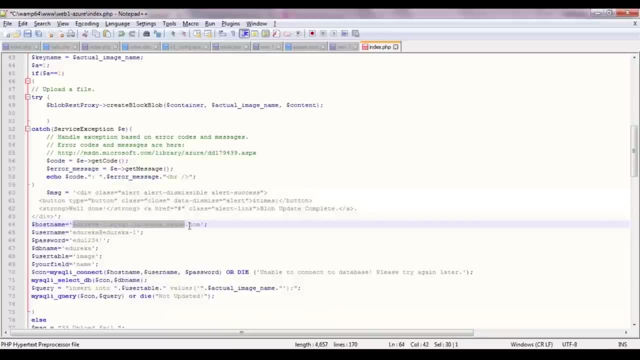 storage account is set, you don't have to change anything else. let's go to the my SQL. but all right, here it is. so the server name has to be changed. let's copy the server name and give it here. so the host name is this, all right? 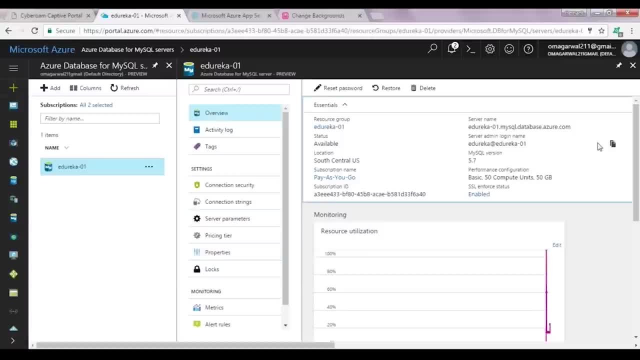 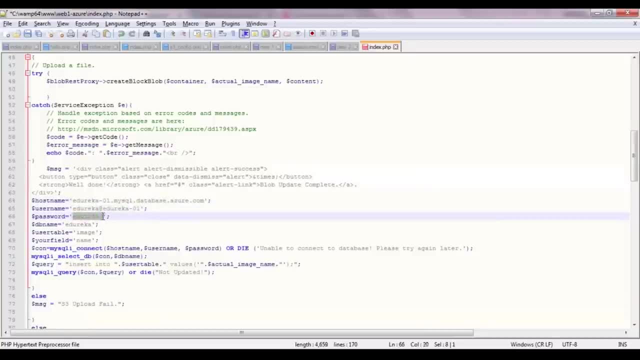 and let's see. so our login name is this. let's put the login name here. password is edu1234, exclamation, which is right. our DB name database name is edureka, which is nice. username, user table is image, which is right, and the field name is name. 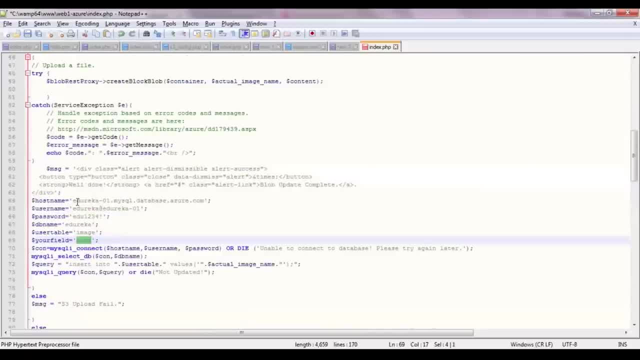 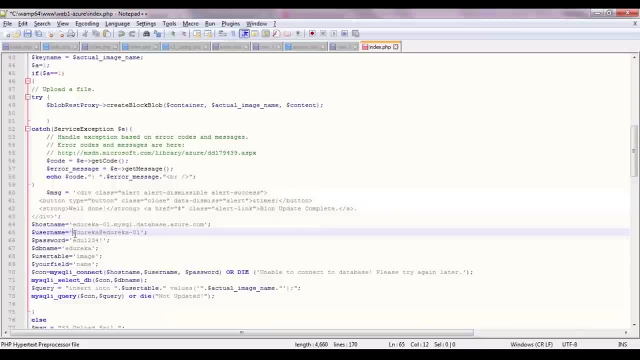 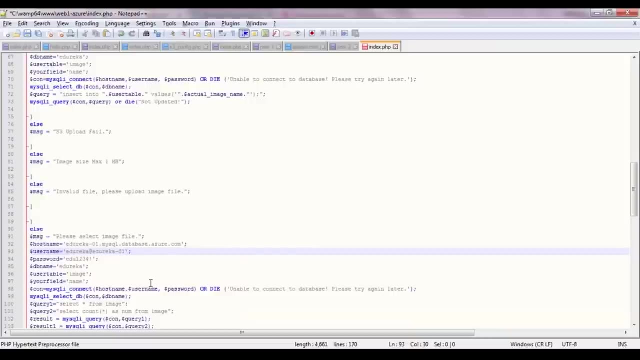 all right, everything seems fine. one more place I have to change it, so let's do that as well. so let's copy this, paste it here. copy our username, paste it here, and everything seems fine now. so now, when I try to run the code, it will run. 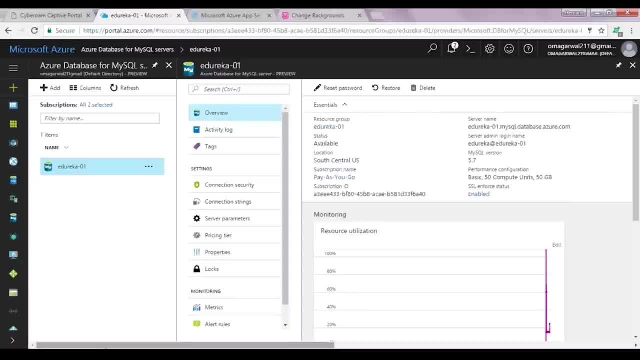 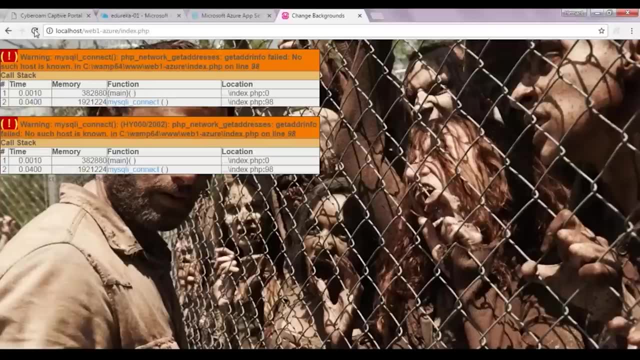 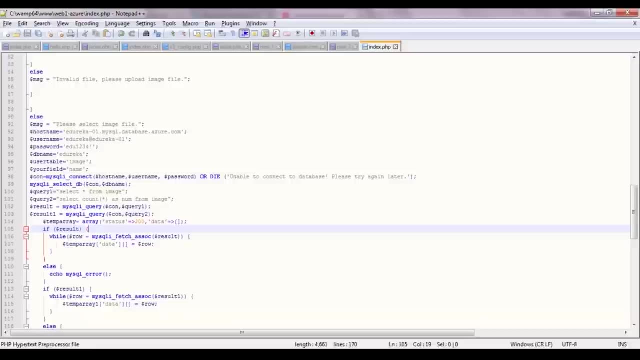 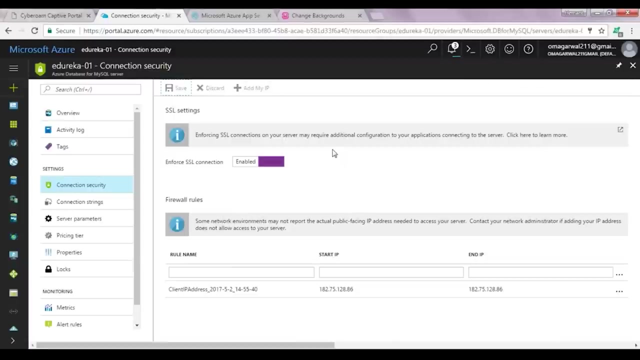 on my localhost, but it will not run on my web app. why? because I'll tell you so I was getting these warnings right, so let me refresh. wait, let me save it, so let me refresh it now. okay, one second. okay, so say: successfully updated. let's go back and check whether it's working. 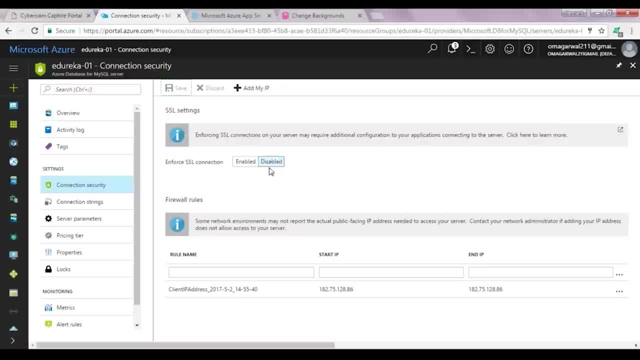 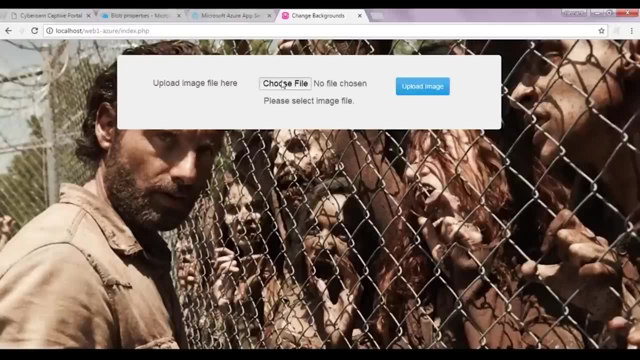 all right, so basically, you have to disable the enforce SSL connection in your MySQL. that would be it I for to do this. all right, so now I will choose in a file and I'll be uploading this particular file, which is desert. I'll click on upload image and it will take some time to upload the image. 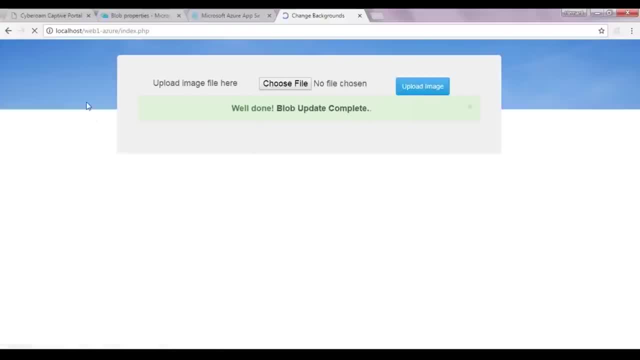 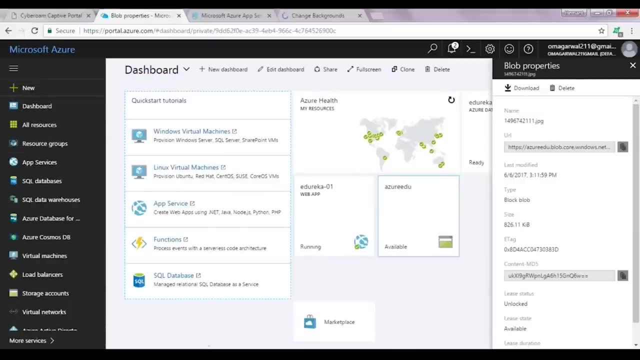 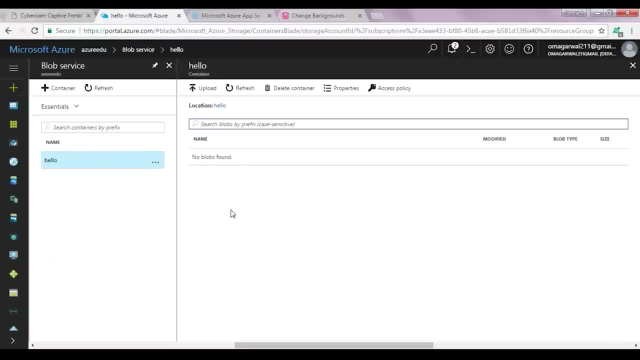 and it says: well done, blob, update complete. and, as you can see, my image is loading. let's check whether we have it in our dashboard as in in our storage. the. we'll go to zero edu, we'll click on blobs, we'll go to hello container and you can refresh it. 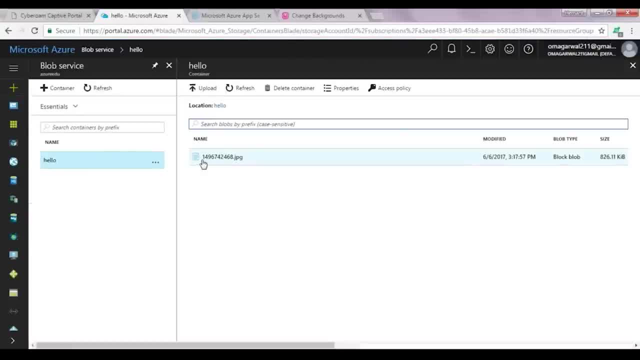 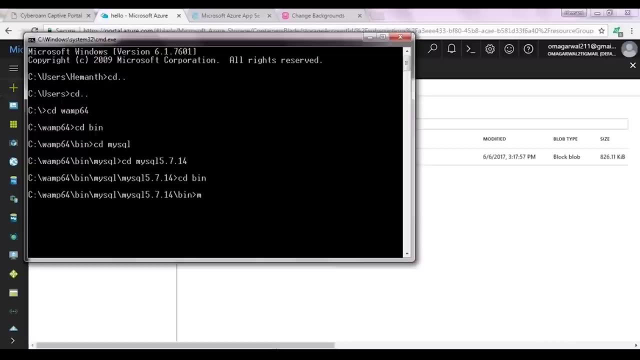 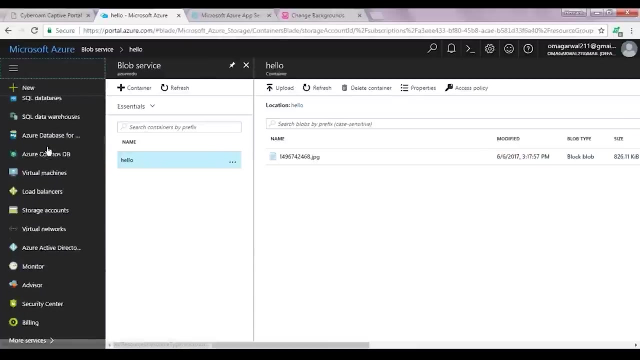 and, as you can see, there will be a file here which says one four nine six, seven, four, two, four, six, eight. all right, so let me connect to my mysql now again. all right, just give me a second. i will type in mysql-h and then the username. 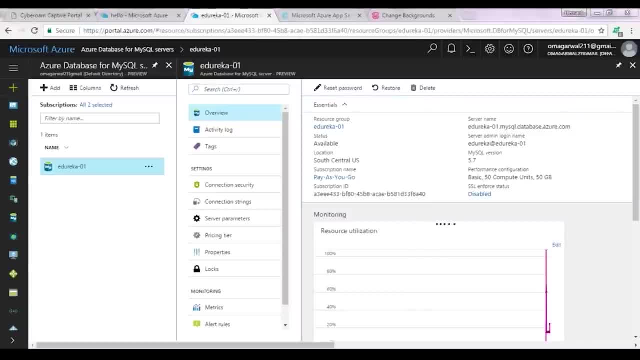 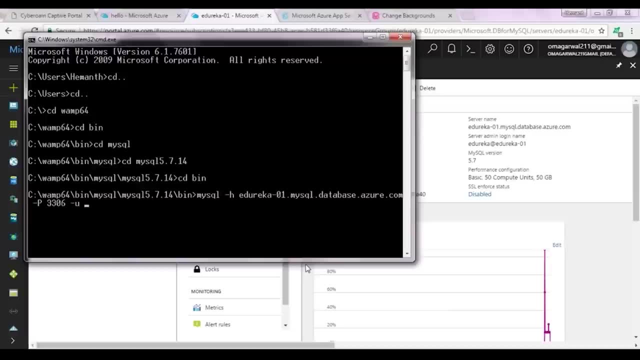 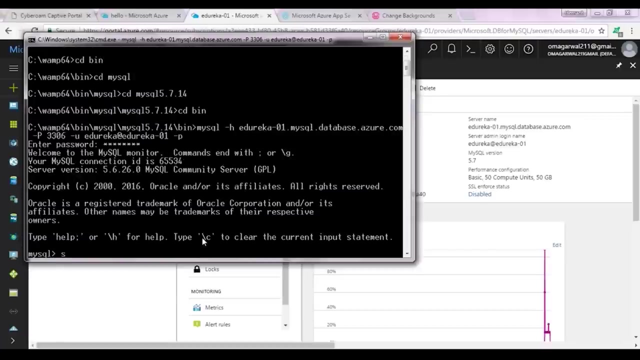 so this is my hostname, guys. so i'll copy this hostname, paste it here, and then my port number, which is 3306, my username, which is this: i paste it here- and then the password, which is, as of now this: edu1234. exclamation: i've connected to my database. i'll use the database. 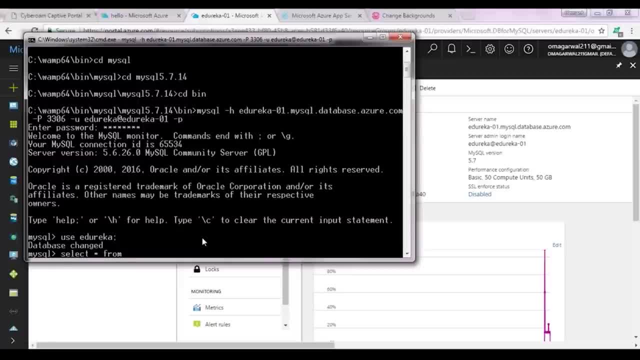 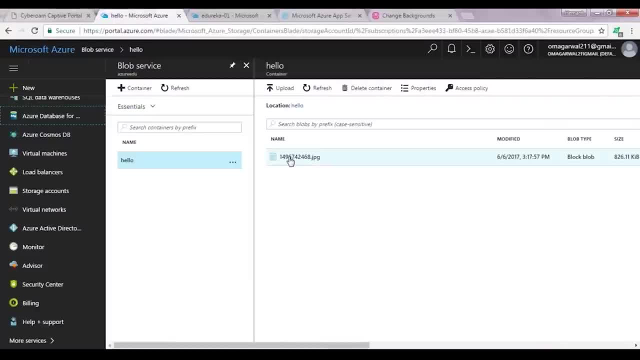 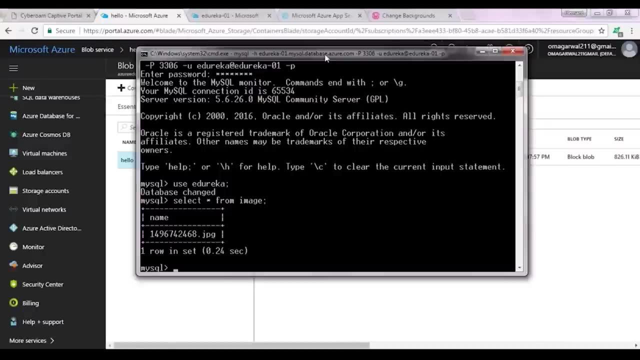 that i've created select table and i will show you the record. now. let's compare it with what is there. it's one, four, nine, six and four, two, four, six, eight, and it's one, four, nine, six, seven, four, two, four, six, eight. so, guys, as you can see, the same file has been uploaded here and it has been mentioned here. 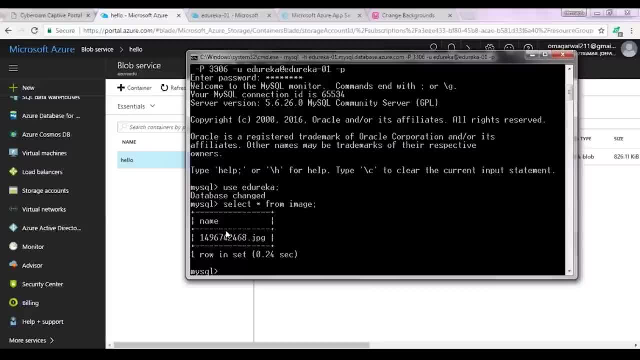 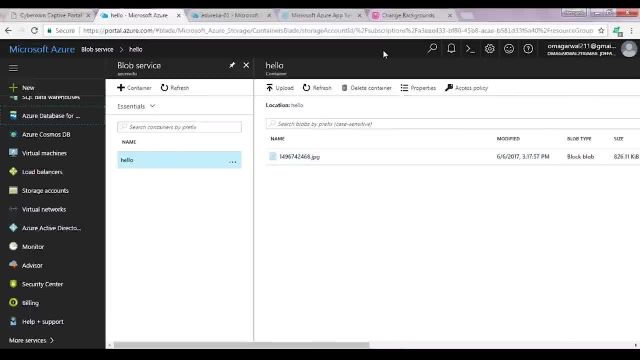 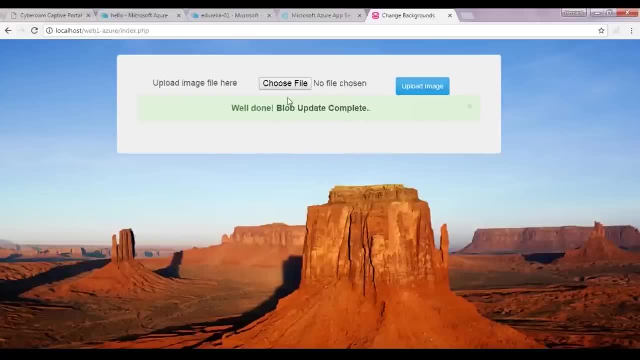 so what my website is now doing is it is basically fetching the file from my database and then accessing that file over here in my file system and hence displaying it in its background. so, as of now, this, since there is only one image, it is not showing the slideshow. let me choose one more. 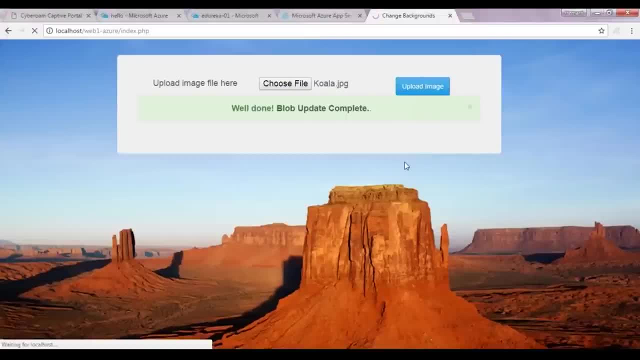 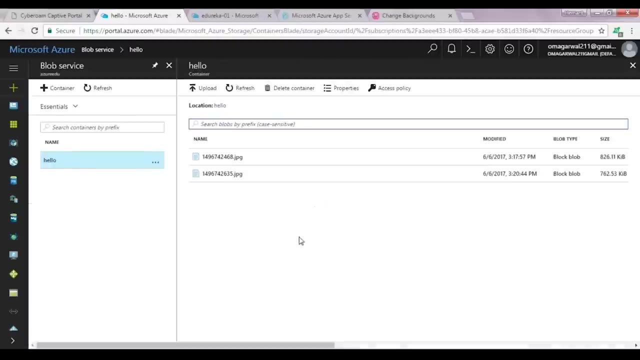 file. let's upload the koala image and click on upload image. so now, when you will see, that's the image which is being loaded and if i go here and i refresh it, i can see that there are two images now here right and in my database as well. if 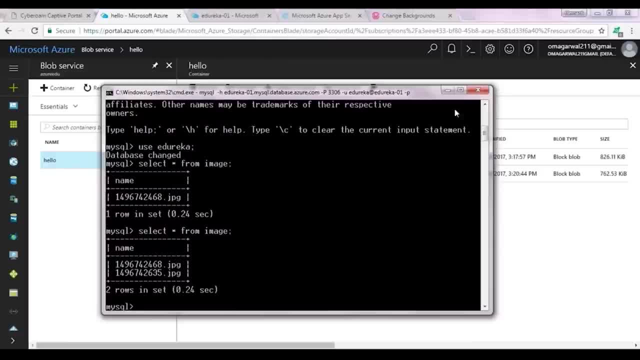 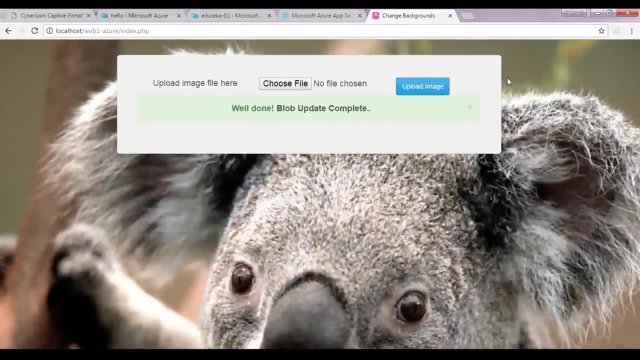 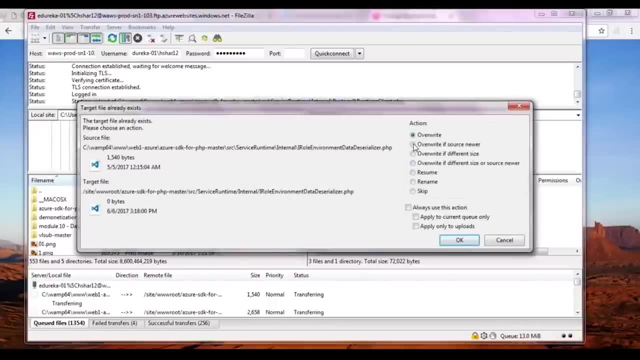 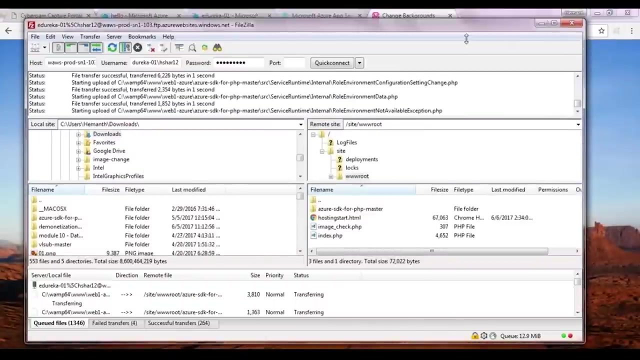 i refresh it, i can see two images. all right, guys. so this website seems to work fine. it is connecting with my storage account. it is connecting with my database on azure. now let's check if my files have been uploaded. so it says: okay, this might take some time, guys, so let's wait, because we are all set here. we are done with. 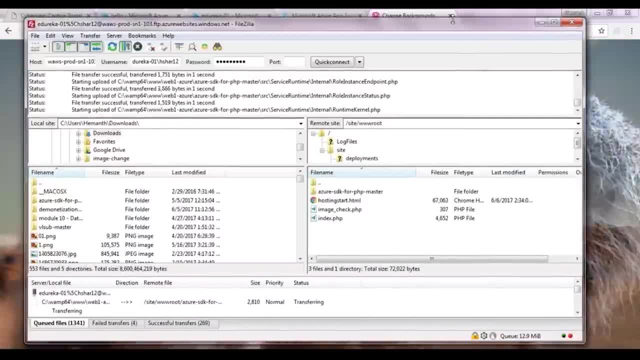 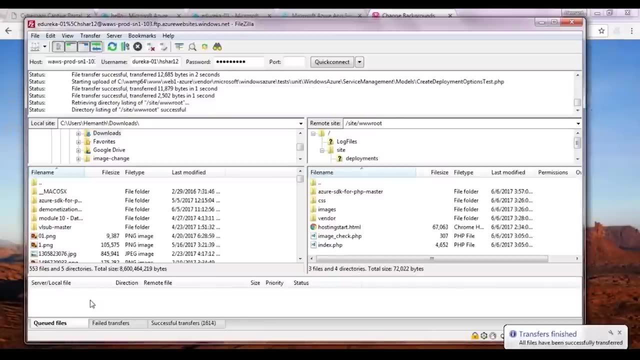 everything. we are just waiting for our files to be transferred here, and then i'll show you how it works over there. all right, so let's wait. all right, guys, so my transfers are finished, so now let's check whether my web app is working or not. all right, so i'll go to my system. 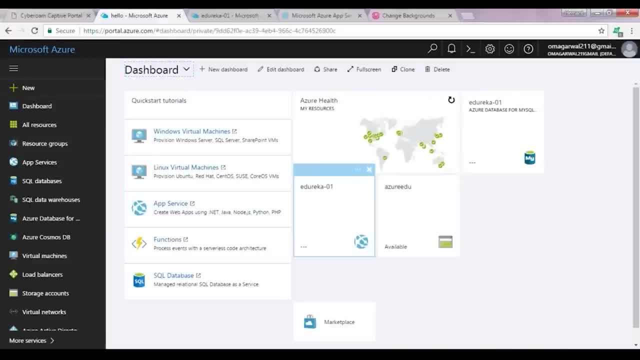 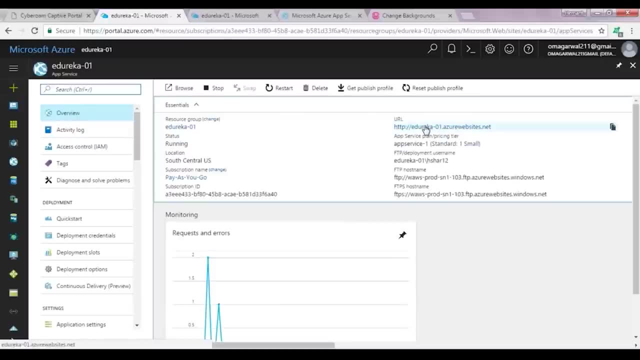 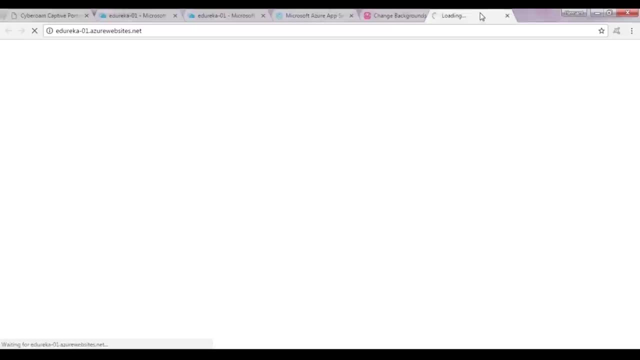 to the dashboard. I'll go to my web app and this is the link. I'll click on this link. Now, guys, like I said, you have to add the IP address of the web app in the MySQL as well. So when I go here you'll see an error. right and now, like I said, 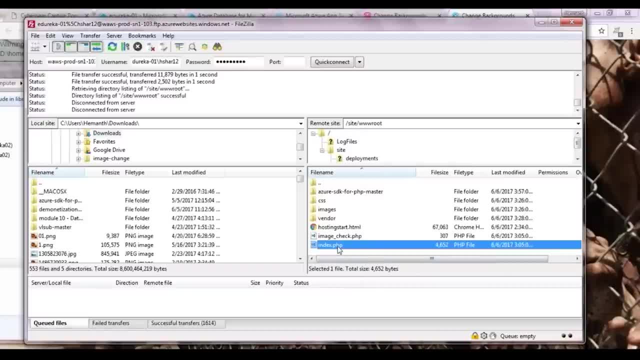 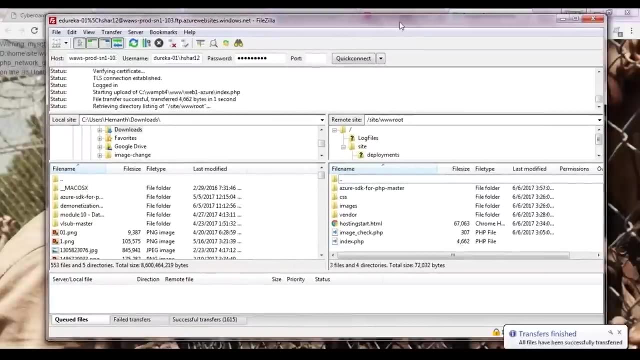 we have to send the index file again, So I delete the index file from the server from here. Alright, copy the index file again, because it's been updated. Alright, and now I will refresh this. So, as you can see, it says the IP address is not allowed. 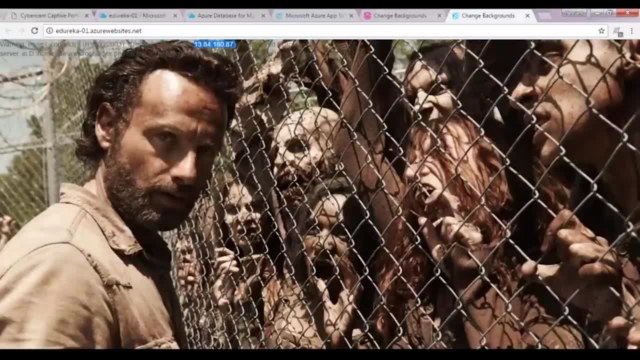 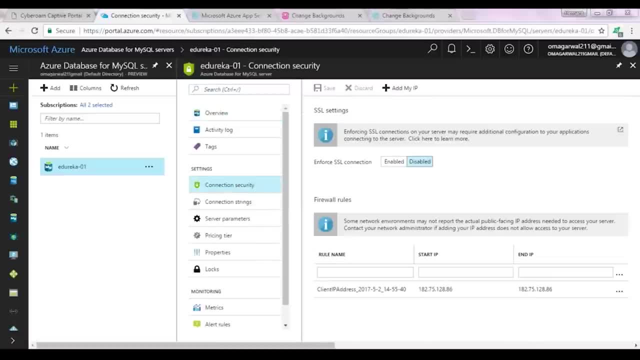 to access the server. So what we'll do is we will copy the IP address, We will go to our database, Go to connection security. Alright. so here we are. We will select the web app, give the start IP and the end IP. Alright, so let's get rid of. 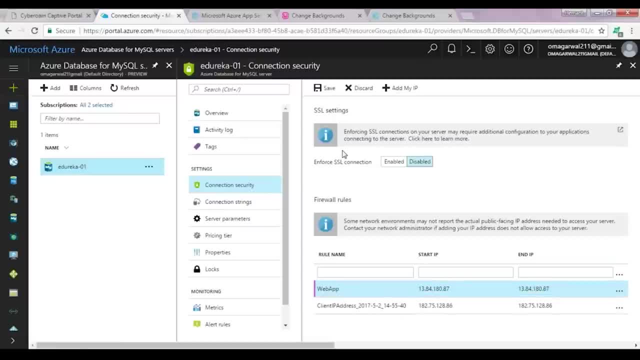 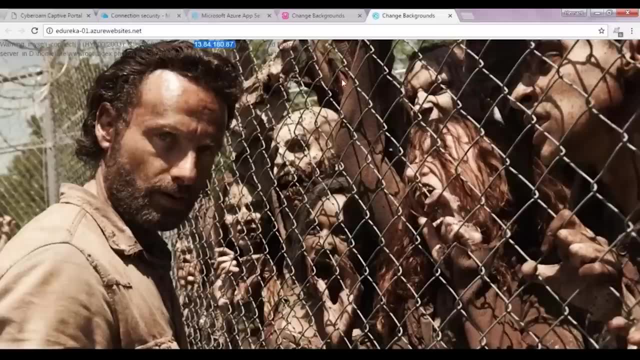 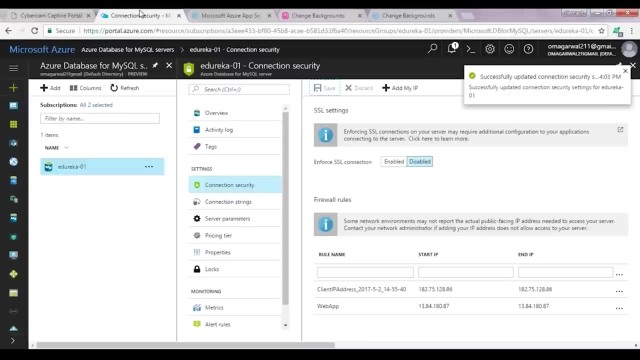 the spaces. and this is it. Now we'll click on save. Now why are we doing this? We are doing because here we got an error that this IP address is not validated With the MySQL, So we have added this IP address over there. 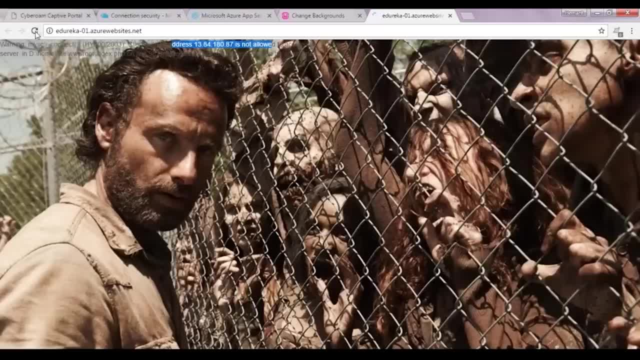 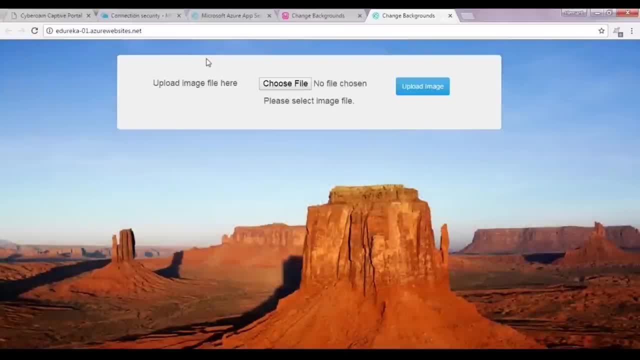 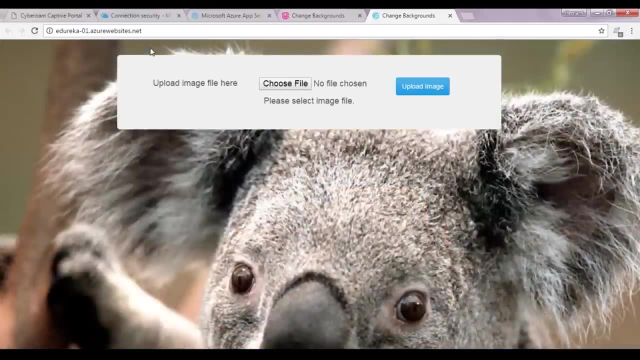 updated security settings. Let's refresh it and check. Okay, awesome guys. so now my website is working. So I have successfully updated my website in the web app, Alright, and I didn't have to configure anything. I didn't go to the UI, I just transferred my files and my website is up and ready. 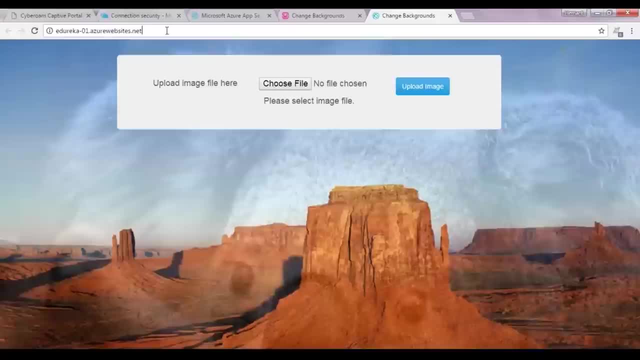 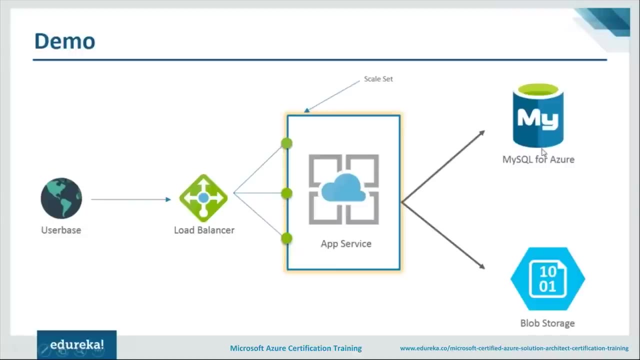 This is the address which is being used to get to the website. Alright, so, guys, this was the demo. Let me get back to my slide. So let me recap what I did. I configured my app service with the code. I configured MySQL with the IP. 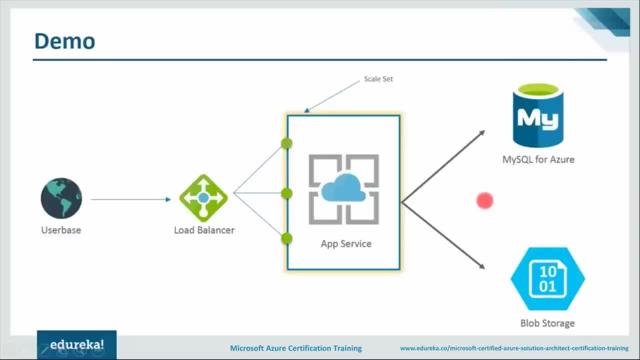 addresses of my own computer to configure it, and the IP address of my app service, so that the app service can communicate with MySQL. I configured my blog storage and I configured its address in my code, my PHP code, and I configured the hosts name and the password for the created MySQL service in my PHP code as well. So 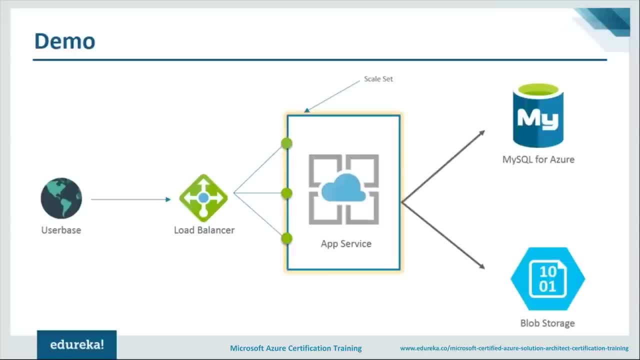 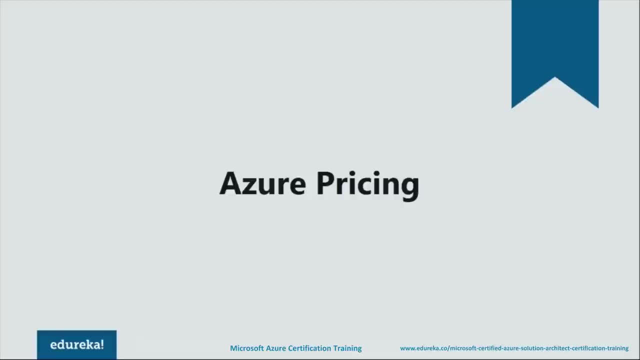 guys, this is what we did, Alright. having said that, let's go ahead, guys. so we're done with the demo. let's get on with Azure pricing now. Now, whatever services that we have used, what if I tell you that you can use them for free? Yeah, so. 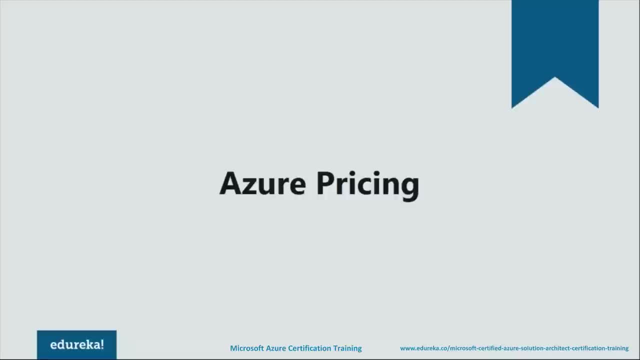 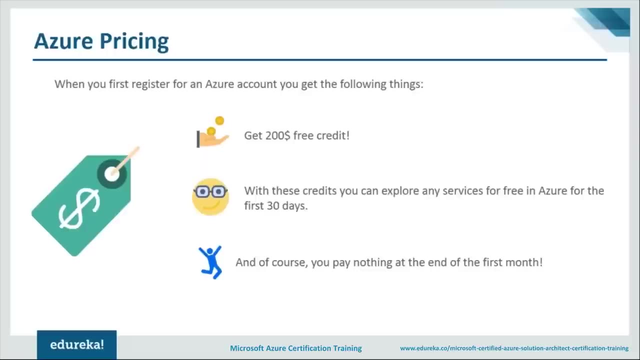 let me teach you guys how you can do that in the Azure pricing section. So the Azure pricing sections has these three features. alright, So for the first time you register on Microsoft Azure as a new account, you first of all get $200 worth of free credits in an account. Now what you can do with this $200 is you can use 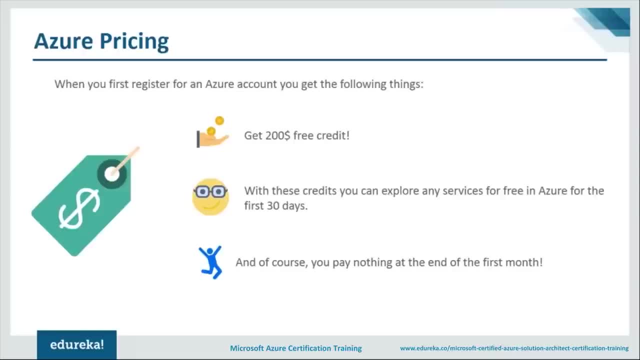 it to deploy application as and when you want. So this is a one-time free credits that are allotted to you on registration. Also, with these credits you can explore any services for free in the Azure for the first 30 days. So in Azure you can use these credits to be to launch any kind. 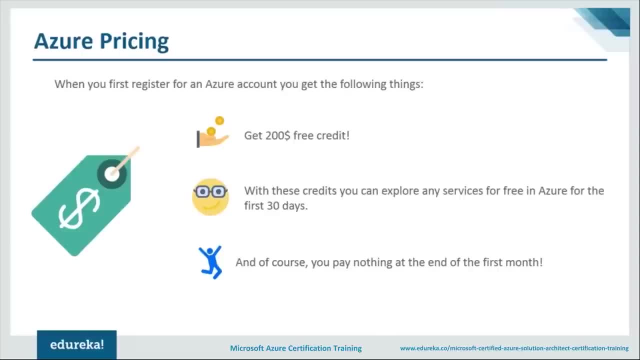 of service for the first 30 days and, of course, after you use the services, you don't have to pay anything. alright, but you might have to register your credit card with them, because that is how it works. they'll charge you one rupee in that and then they'll refund the one rupee afterwards. This is just for. 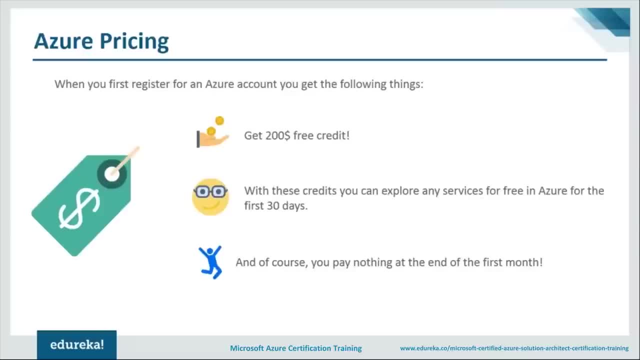 verification purposes, because once your free trial ends, you have to upgrade your plan, to pay as you go or whatever that you are looking for. right, But the good thing about Azure is that sometimes it happens that we start using the free thing and we forget to see that it is only valid for 30 days, and we forget that and after. 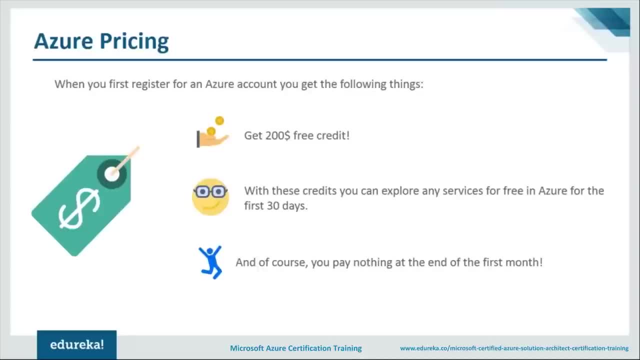 30 days. if you use another services, you get charged right, But with Azure that is not the case. With Azure, what happens is you are given a pricing tier which is free trial, right. So at the end of 30 days it says free trial. 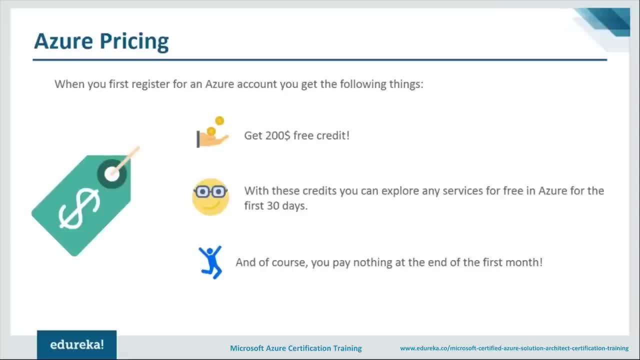 expired and you're not allowed to do, or you're not allowed to access, any of your services. It is only when you manually change your plan from free trial to pay as you go that when you can actually start using your services again. So- which is a good thing- by Azure, because you have control of your finances in your 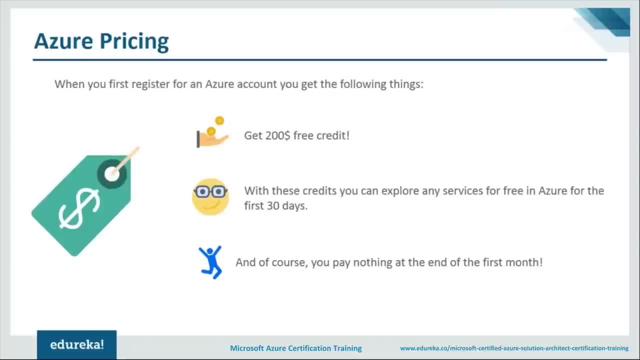 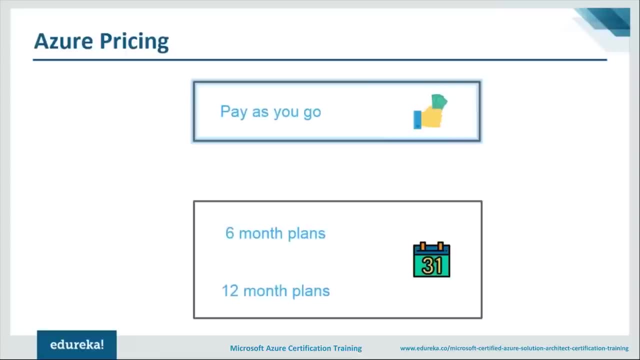 hand right, You will know what you get charged for, and that is something very transparent about Azure that it has come up with, so it is a very good thing. Having said that, let's go ahead and understand that the two plans which are there- So one plan is called pay as you go plan and the other plan is: 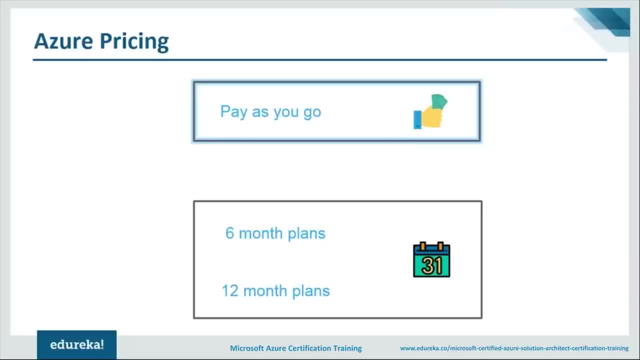 called six month or 12 month plan. So basically with pay as you go plan. the thing is that you take a service or you take an instance and you use it for one day or two day or a week or two weeks and you pay for that amount. only, all right. But when you want longer commitments, say for example, 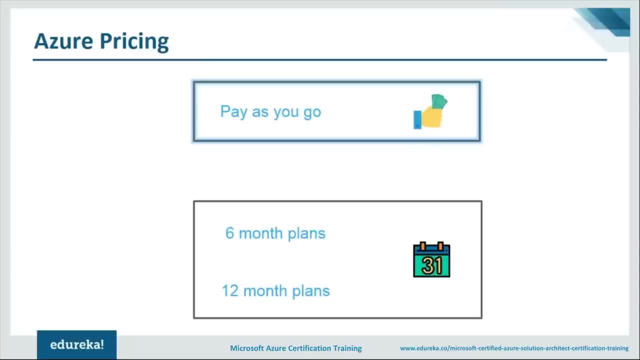 our website, right, our company's website. it's called edurekaco, So it will be there until the company is there, right? So for those kind of cases it is better to go for long-term plans, because with long-term plans you get discounts, right? So if you compare it with pay as you go, if you're 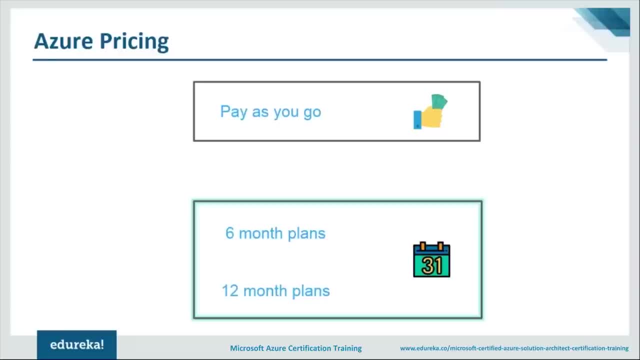 using an instance with pay as you go plan for, say, six months and you compare it with a service or instance in which you have opted for a six months plan or a 12 months plan and you have gone through the six months, the amount of money that you're paying in that and the amount of money that you're 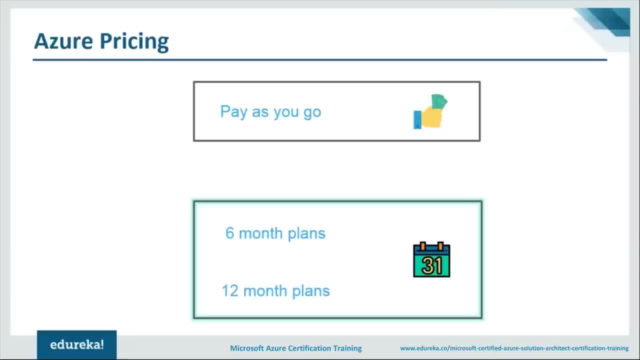 paying through the pay as you go service is obviously less right. So the other thing is with the plan. the catch here is that you have to pay a full upfront or a partial upfront payment for the six months or 12 months or whatever term that you want the instance to be. 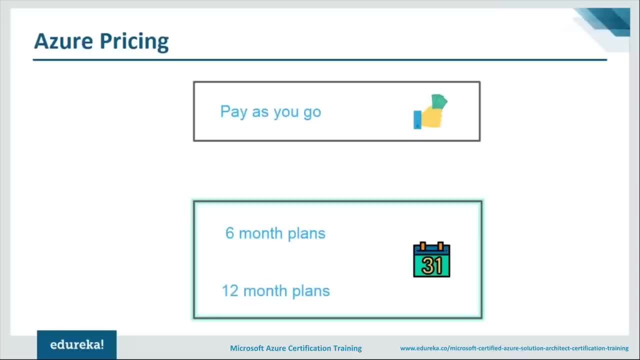 running on right. So this is the thing that you have two kind of things: you have pay as you go plan and then you have a plan wherein you pay in future. So it's basically like prepaid and postpaid. with prepaid, you have six months and 12 months plan. with postpaid, you have pay as you go. 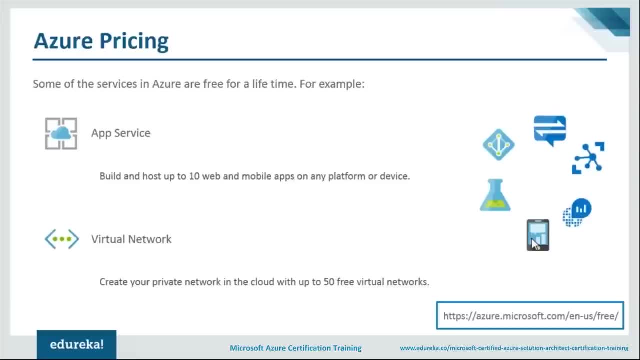 This is the which I've added in my slide, So this link will take you there, and it lists all the services on my website that are available on this website for free, which are there? Some of the services that we have not discussed today are: 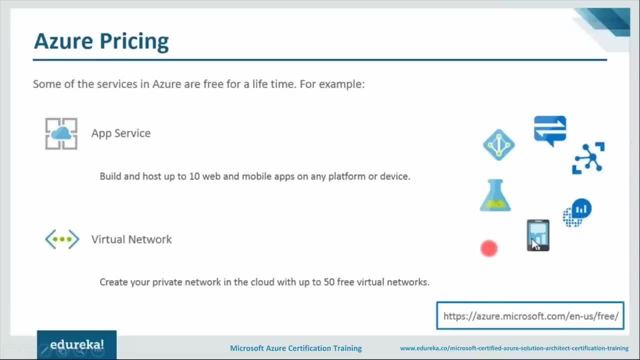 also included under the free subscription. Now, the good thing with Azure is, guys, that even if your free trial ends, these free things will be there for you. right? You can use these free things. even if the free trial ends, These free things are there for life. So the first 10 app services that you use. 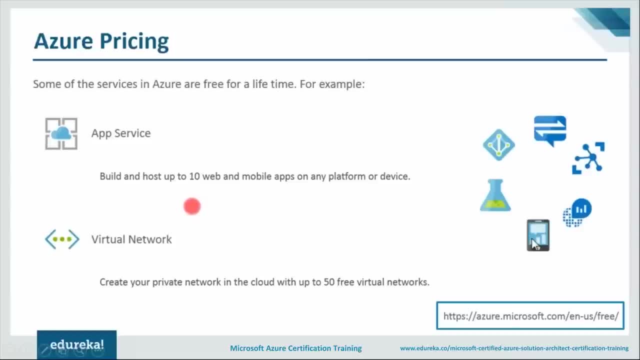 in Azure, they are free. Similarly, with the case of virtual networks, you can actually create 53 virtual networks with Azure right After the 50 virtual networks that you have would have created, the 51st would be charged for you as one virtual Network. That is again a cool thing, right? So like app service. 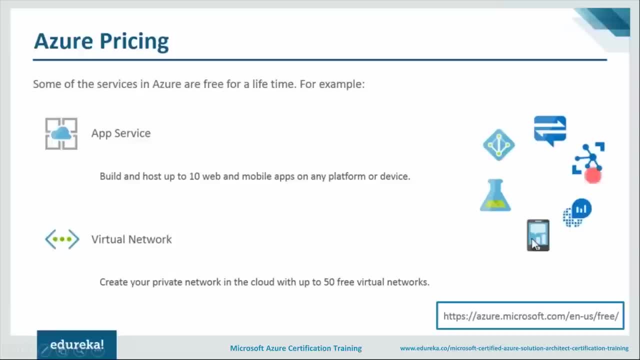 and virtual network. like I said, there are other services as well: one, two, three, four, five, six, 6 in all which have free with a seer for a lifetime. So there are some restrictions, like, for example, in App Service. you have, you can. 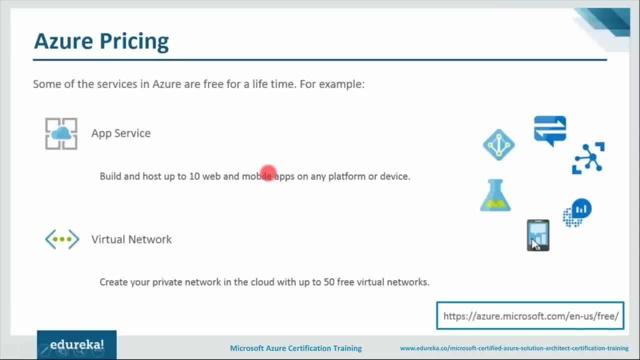 only run 10 apps in Rsoule for 3 weeks, because more than 10aszure devices can run 10 applications per unit without any fee. So you can run 10 apps inuplig in Azure services for free. similarly, you have these services as well. all right, so this. 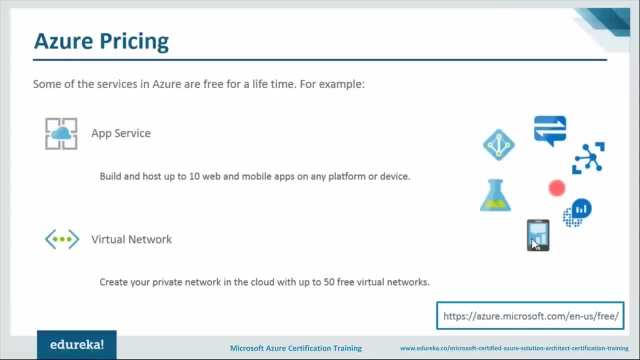 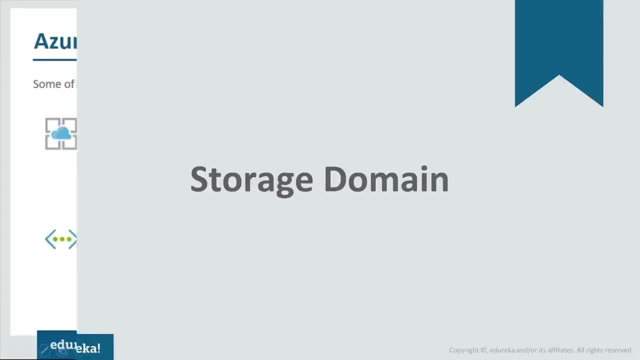 is a cool thing about Azure that, even of the field trial ends, they give you free services. having said that, guys, okay, so that brings us to the end of our session. so today, in this session, we'll be understanding Microsoft Azure storage components. all right, so let's go ahead and see what is our agenda for today. so 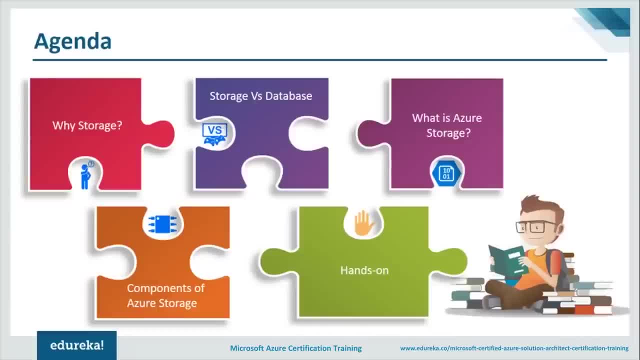 we'll start off by discussing: why do we actually need storage? all right, and then we'll move on to a question which is frequently asked, that when do we use storage versus when do we use database? all right, after that we'll move on to see the topic of the day, which is what is as your storage, and then we'll move. 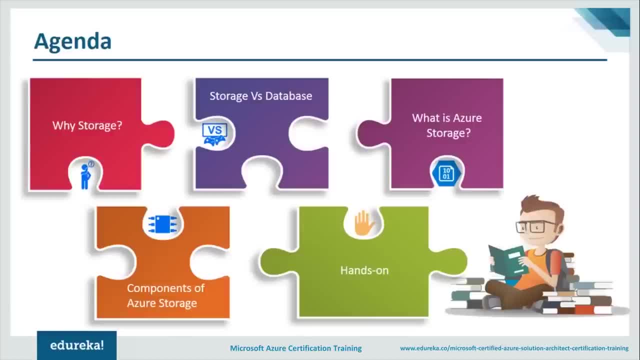 on to discuss the components of as your storage and, towards the end, we'll be doing a hands-on on you, each and every service that we'll be learning today. all right, so, guys, I hope the agenda is clear to you. I welcome you all to the live session. any doubts that? 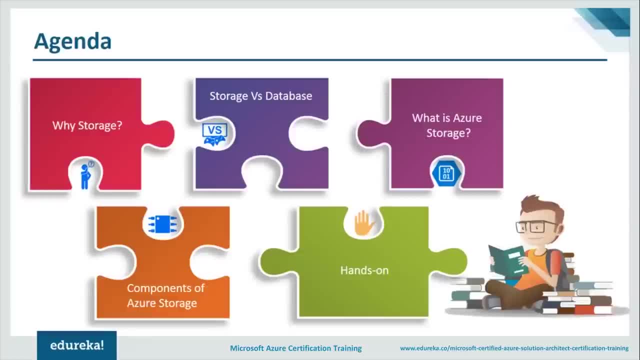 you have, please put it in the comment section. I am a team with me here. they'll be answering all your queries here today. all right, so with that, let's begin today's session with our first topic, that: why do we actually need storage? alright, so for this, let's take an example. first, let's take a use case and 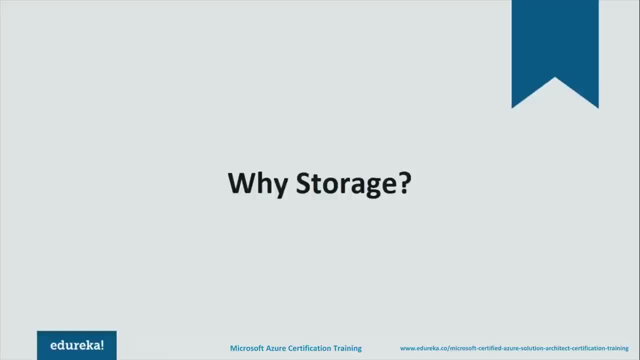 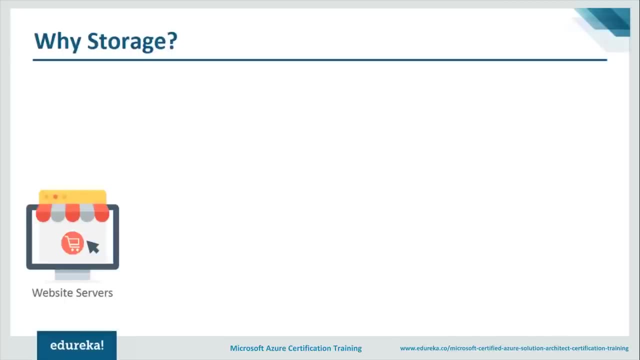 see and understand what is the need of storage in today's data. all right. so, for example, we have an image processing application. right for support this image processing application, we have given the user interface as a website, so around a million people can access my website and put in their request to process their image. alright, so we don't want the 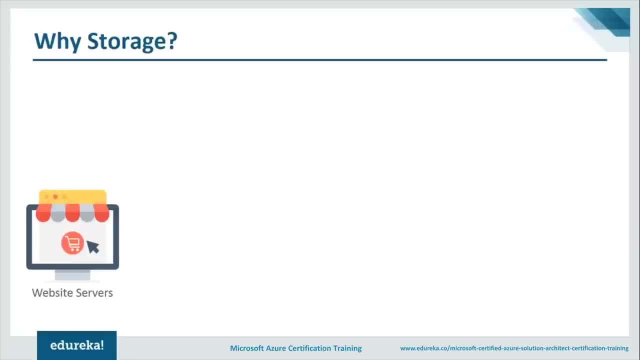 processing of the image to happen on this server which is проводing by my website. I wanted to be happening on some other solo right. I want the processing to happen on a backend server, so for that we have some backend servers. now my request for the processing will come in from website servers, so I need a place. 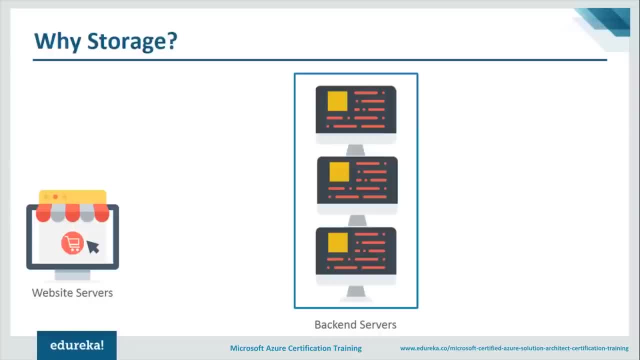 where in I'll be storing all the jobs right which can be accessed by the backend server as well. so for that I need an entity where I, wherein I can dump in all the jobs which are there which are to be done by the backend servers. now, obviously, all the jobs cannot be done simultaneously by the. 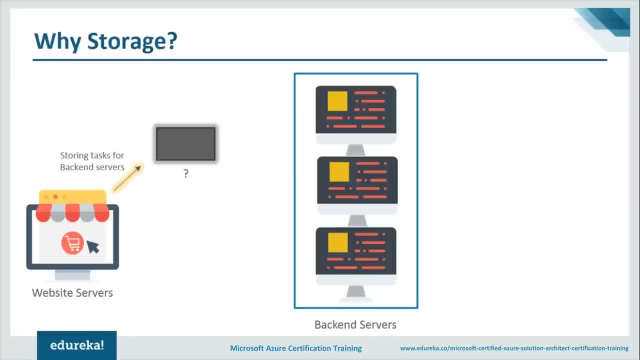 backend servers right. so say, like I said, there are like million people who are accessing your website at once and they put in a million requests, right, and your backend servers cannot process all the requests at once, so they will do it one by one, right, and they can do that with the help of this entity. they will. 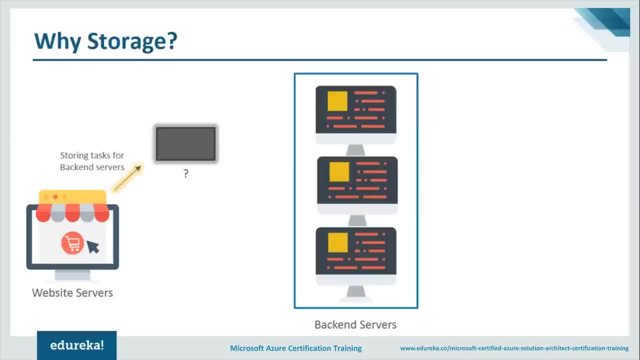 they will pick up a job, do that job and then go again back to the entity, pick up another job, go back to the entity, and so on. all right, so now, when you have all the jobs in this entity, these jobs have to be distributed equally to the backend servers right once that is done, 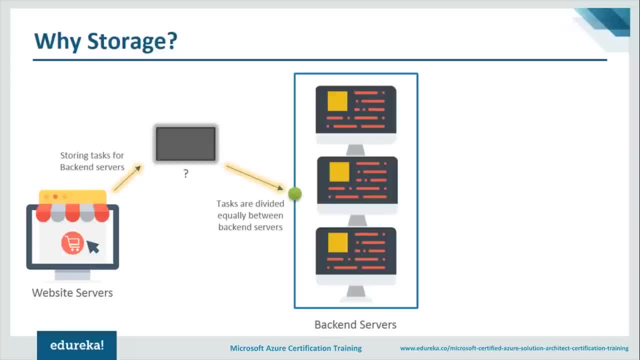 once your backend servers process all the images which are there, or process an image which had, which had some operations to be done on it, then the image has to be stored somewhere. right, because you have to store the end result somewhere. so you will store all the properties, like the name, the location of. 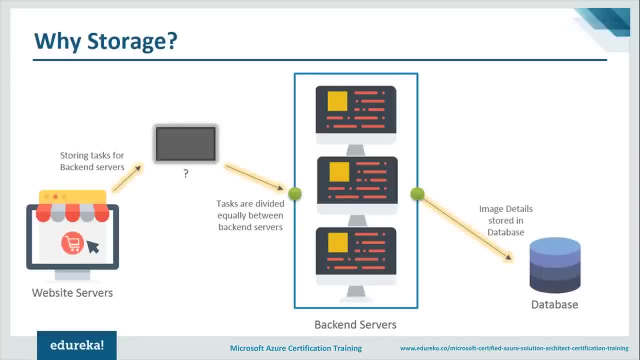 the image, everything on the database. but here comes a change. you cannot store a an image on a database. i mean you can actually do that, but when you look at the data that an image contains, it is all randomized, it is. there is no structure in the data that an image has or for. 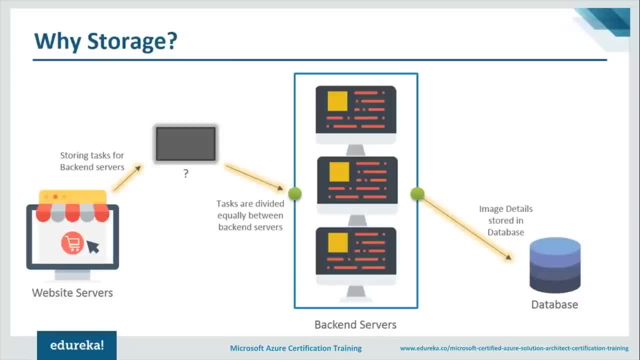 that matter, any video file has, or any any kind of file has, right. so that is the reason we need an entity to actually store this kind of data, so that the processing that is required to query this kind of data, which would have been there in the case when you would have stored your image. 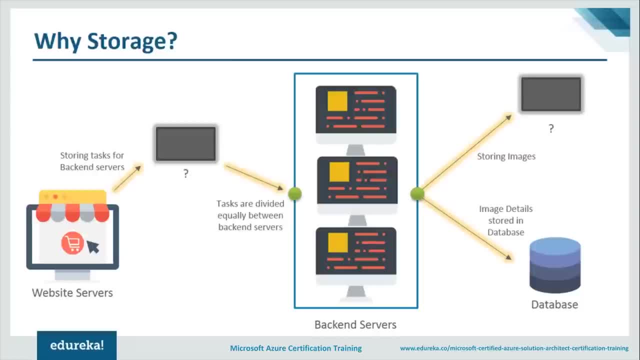 in a database, right? so in, in that case, process, a lot of processing is required if you try to query them. so we wanted the processing part to become less, the processing burden to become less, and hence we, hence we wanted an entity we can do, which can actually store any kind of file. let it be. 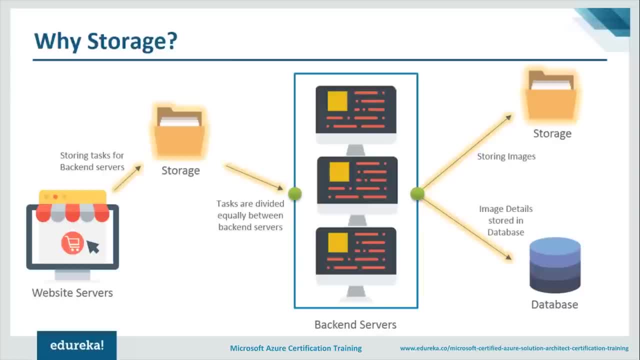 images, let it be video, files etc. came in storage. so let's discuss the first case wherein we had to store the jobs, right? so when storage came in, now we can actually put in, say, 10 000 jobs per second in the database. right, so we can actually store any kind of file, let it be images, let it be video. 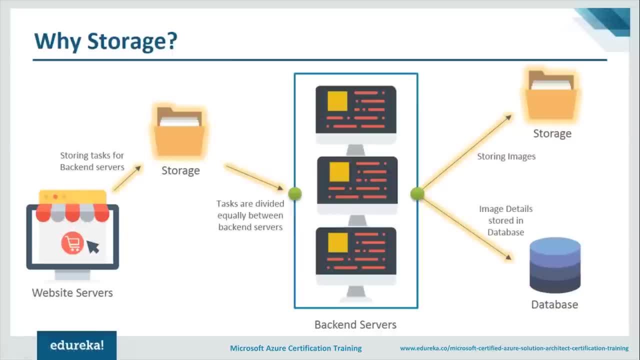 inside uh this storage, uh this storage service, without any uh overburden on any of the servers, be it back-end servers or be it website servers. right, so the processing time has drastically reduced and the jobs are now listed uh in the queue. so a queue is actually a service which is 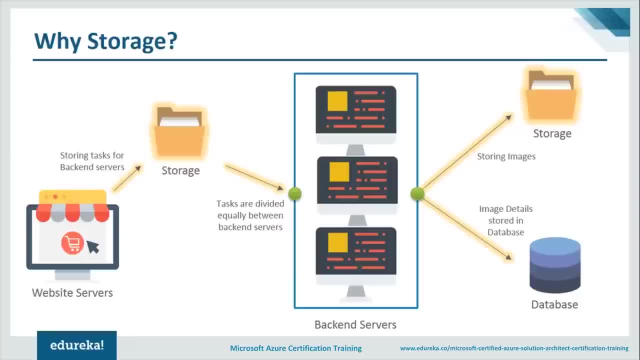 offered by storage, right. so now, what back-end servers will do is it will take up the job from there and execute it, and once they have executed, that job will be deleted and the next job will be queued next. uh, when we talk about this section wherein we had to store images. so uh, now any kind of uh file. 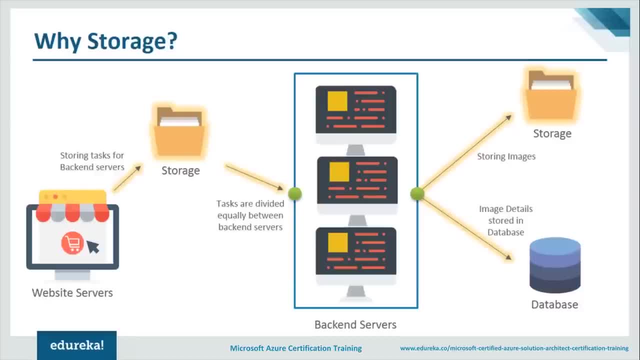 uh can be stored on the storage service which is offered by cloud. uh, it's not only limited to the cloud. if you uh think about it in your computer, in your own local computer, on your mobile, you store some pictures or you store some video files, right, and you store it inside a file system. 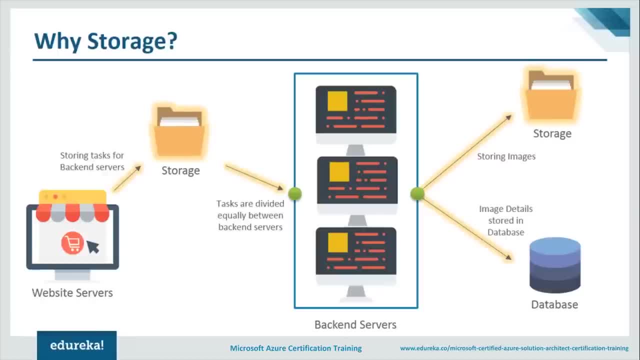 it is not a database. it is a file system, and it can contain all the objects that you want to store. you don't? uh, you do not store your objects inside a database, all right, so this is why storage is needed. uh, let's go ahead and understand. what is the difference. 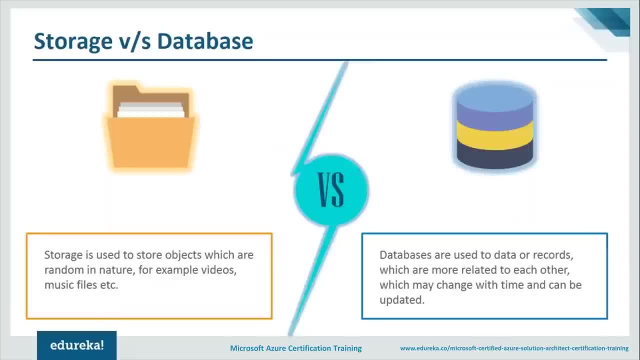 between storage and a database. so a storage is basically needed, uh, whenever you have objects, like i said, so you have. when you have music files, when you whenever you have video files, whenever you have images, right. so in all these kind of cases you use a storage, uh, kind of service. but 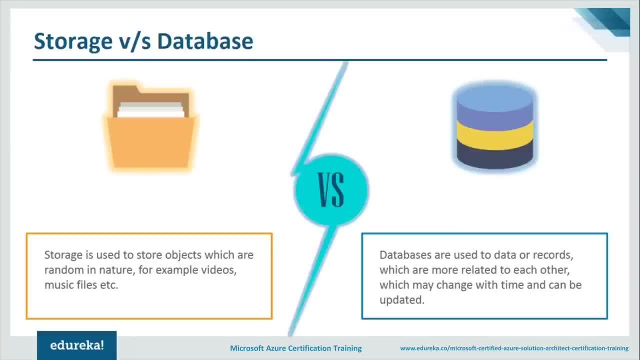 say something related to the metadata of a file. for example, when you store the file in in the storage, you need to have the location of that particular file, you need to have the properties of that particular file. so all these things, all the properties, all the uh, any location column. 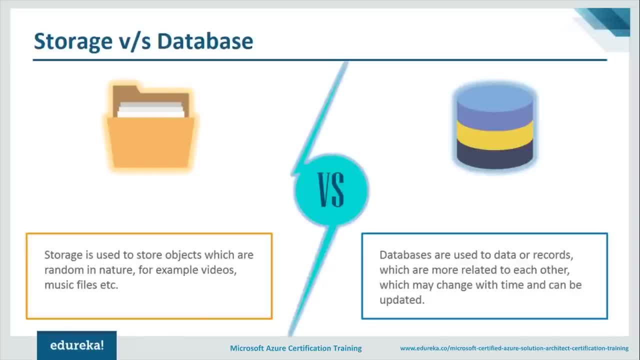 that you want to add. all these are structured right. they are not randomized and hence they can be added inside a database, be it sql or no sql, it can be added right. so this is the main difference, uh. this is, uh, how you'll differentiate between using a storage and a database moving. 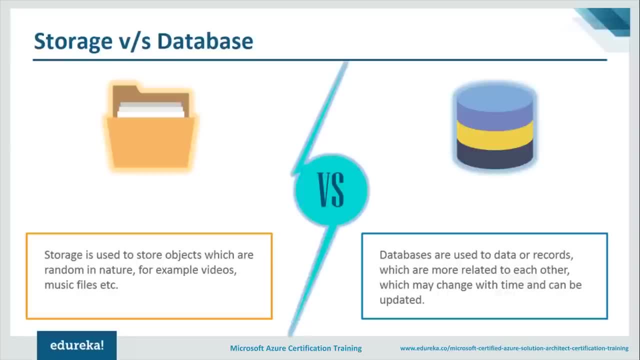 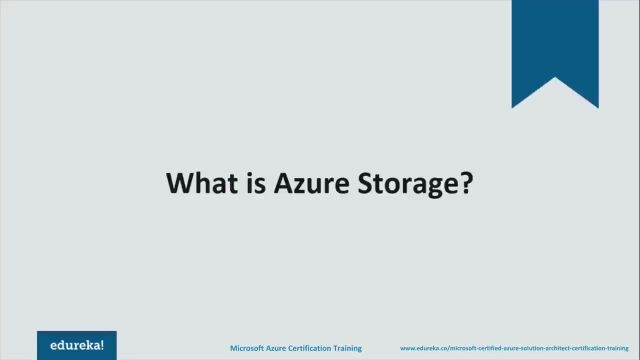 along, guys. so now we have understood what a database is, what a storage uh services. when do we use the storage service? when do we use the database service? let's move on to the topic of the day, which is azure storage. so what is azure storage? so azure storage is a service, uh from. 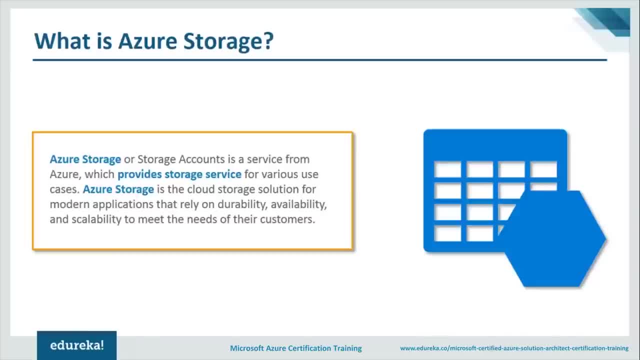 azure, so you use it whenever, uh, you want to store something on the cloud and since we are using the azure, we'll be using the storage service from azure, and that storage service is called the azure storage service. now, when you begin to use the azure storage service, first of all you should 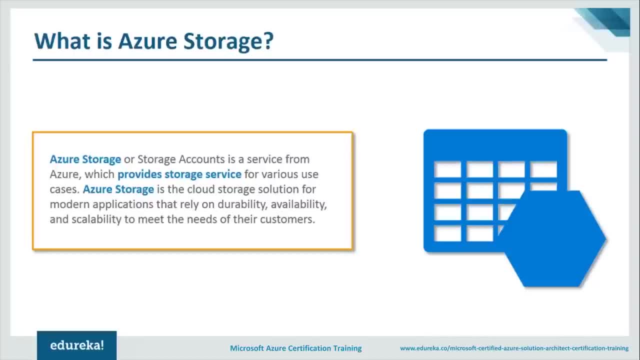 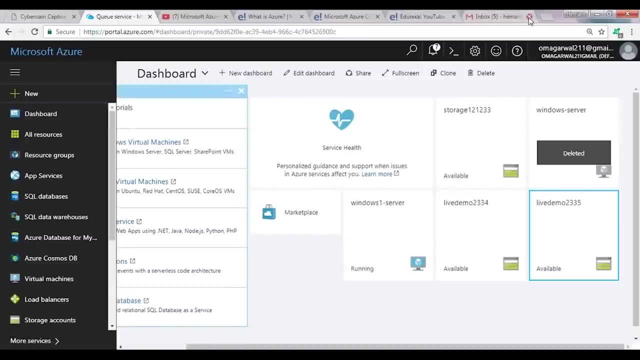 have a storage account which you can create in the azure management portal. so let me show you how you can do that. so let me quickly jump on to my browser so that i can show you my azure dashboard. so, guys, this is how my dashboard actually looks. like, right? so, as you can see on my dashboard, i 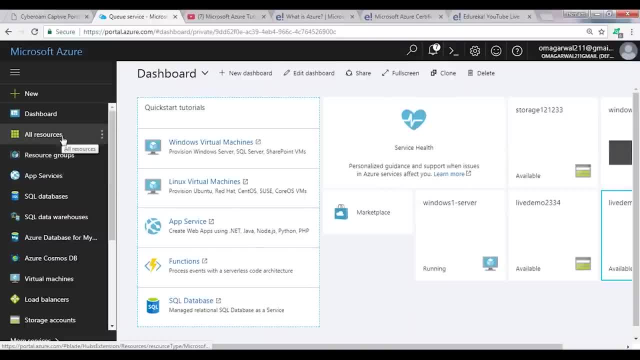 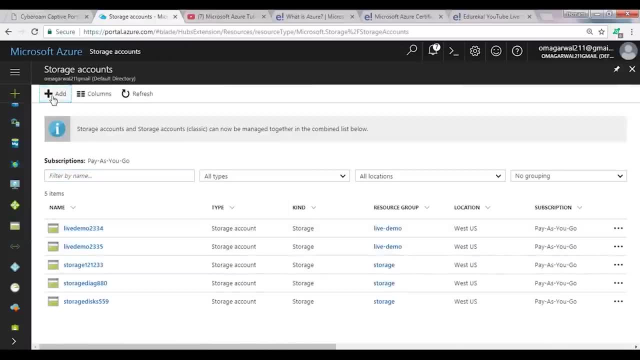 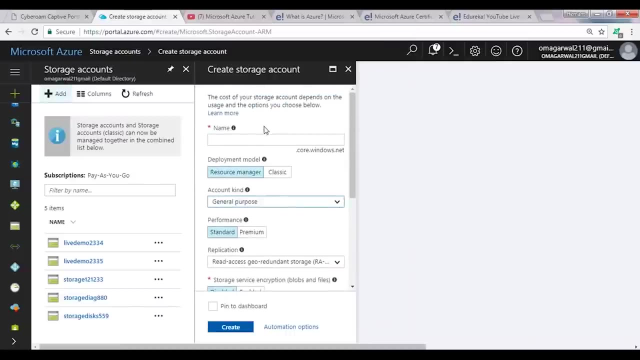 have all these services listed. so what i'm interested in today is the storage account. so i'll click on storage accounts- so i have some deployed already over here. i click on add to add a new storage account and then i'll have this page. now, uh, you will enter the name of the storage. 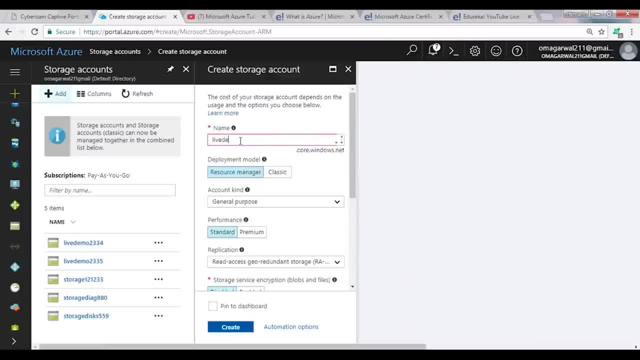 account here. so that name has to be the name of the storage account, so that name has to be, uh, unique. so let me enter a name, say live demo, two, three, two, double, three, six. all right, so that seems to be available. then comes the option of account kind. all right, so how do you want that? 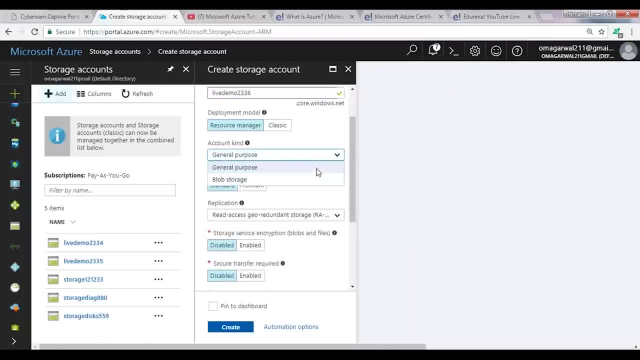 account to be what? would it be a blob storage or would it be a general purpose? so we don't want to restrict our account to only blob storage. we want a general purpose account, right? so we'll choose that. and then comes the replication part. how do you want your data to be replicated? now, there are 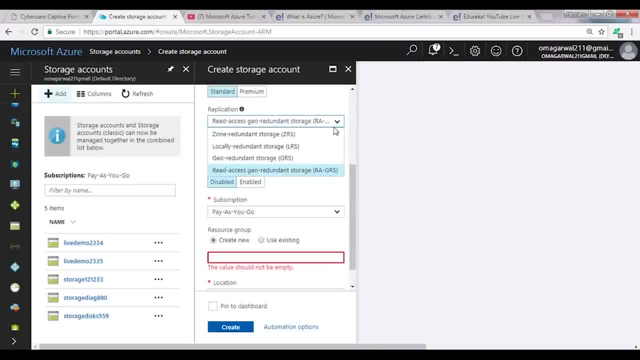 a few, uh, good options that we have here. one is called the locally redundant storage. so when we have the locally redundant storage, what this basically means is- so understand it like this- that there are regions and inside a region there are zones. so, for example, we have the us and inside us we have cities like chicago, new york. right now say new york and chicago are 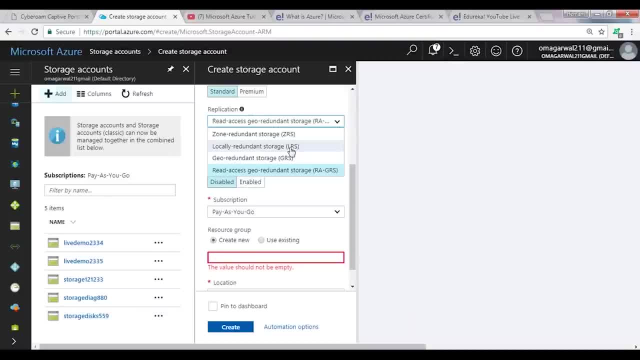 two zones and the region is us all right. so when i say locally redundant storage, what that basically is that inside a zone that is inside in, say, new york, you have a data center for for azure. in in that data center you are, your storage account has been created. so when you select the options or 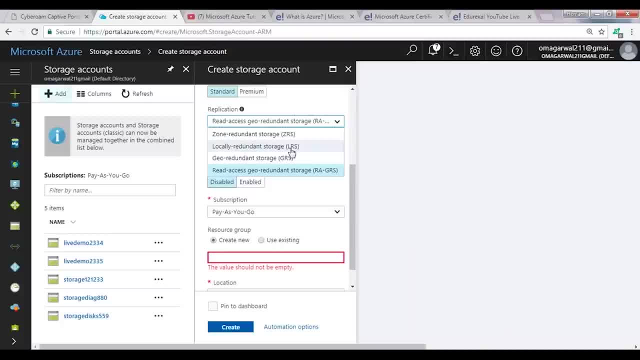 option of locally redundant storage. what basically it does is it'll: it'll replicate your data inside the data warehouse. it will replicate the data inside uh, the data center in which you have actually deployed your storage account, so that if one server cracks as you, you have your storage account in other server in that same particular uh premise, right? 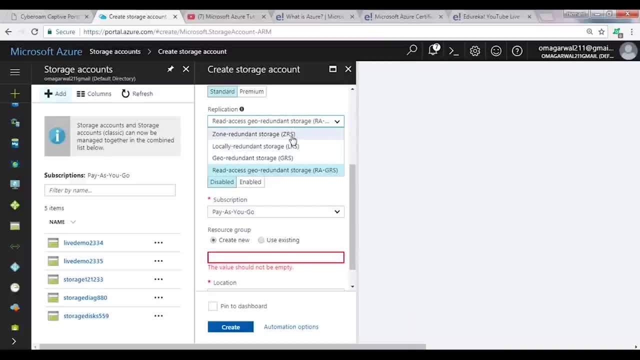 but when we choose zone redundant storage, what that basically means is: so our zone was chicago or new york, right? so in chicago, if you have a data center, and in new york if you have a data center, so whatever is there in the new york data center will be replicated to the chicago data center as. 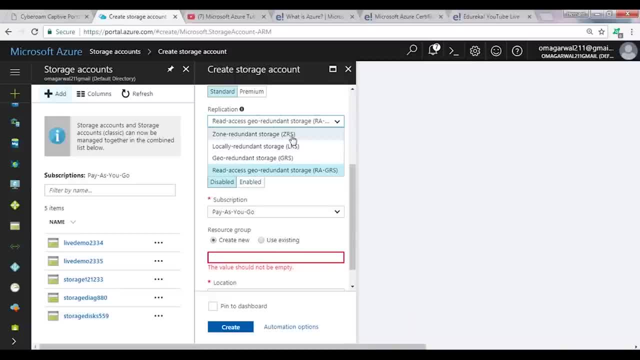 well, so that if one zone goes down, so if this, if the data center in new york goes down, chicago would be up, and hence your storage account can still be used all right. so that's one of the things that you have to be aware of. so that is what the meaning of uh zone, redundant storage- is. 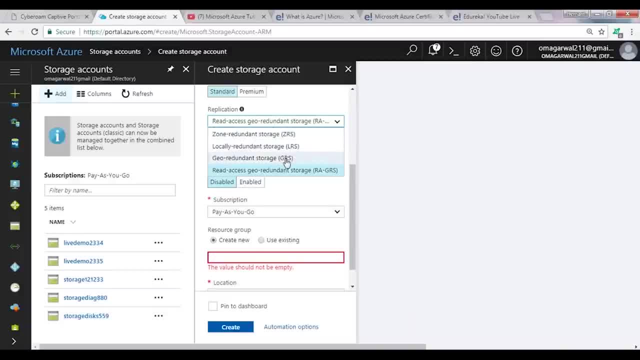 when we talk about geo redundant storage, what we basically mean is: you have different regions. so, for example, we have the us region and we have the india region, so inside, so inside india region, we have different zones, right. so if it's select the geo redundant uh option, we will have the read. 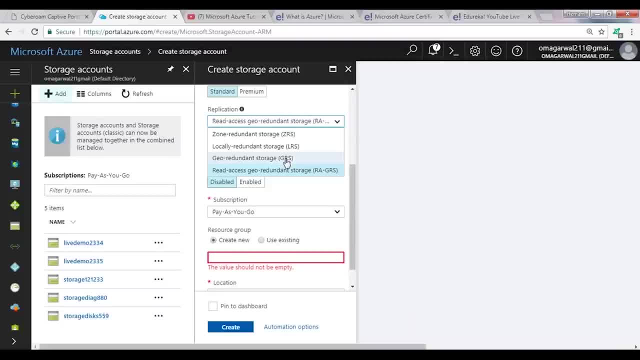 write access to both these regions, that is, in the us region and the india region as well. so whatever you have deployed in the us region, in the chicago zone, uh will be replicated across india region as well, whatever zones you ever deployed in india regions also all right. so this is what the meaning uh, what is the meaning of geo renin storage? 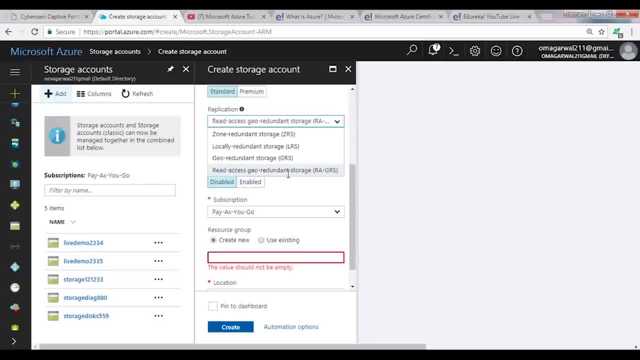 and then we have the read access geo redundant storage, which is a very interesting option wherein you only get the read access of the redundancy. for example, your main server is in new york, right, so it's a zone inside the us region. so if you select read access geo redundant storage, 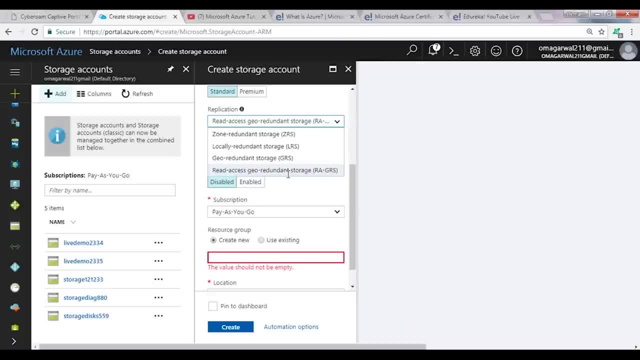 in the uh your, your data will be replicated to india as well. but when a failover happens, that is, when your new york server is down and when you are accessing, when you are redirected to the india region, in that case you can only read the data, you cannot write on it. all right, so it is useful. 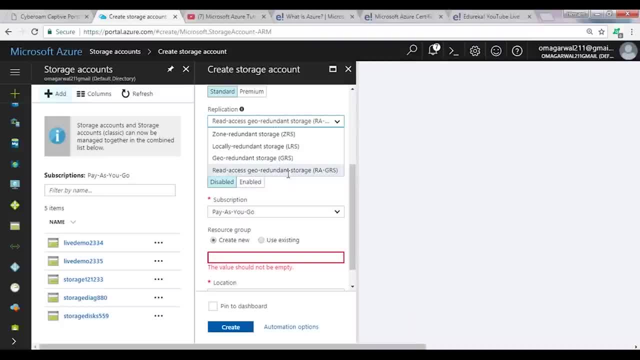 for those applications which only fetch data and there is nothing to write. so in that case geo redundant storage would actually be pretty costly for you. but if you select the read access geo redundant storage, it is a little less cheaper than the geo redundant option. since you are not 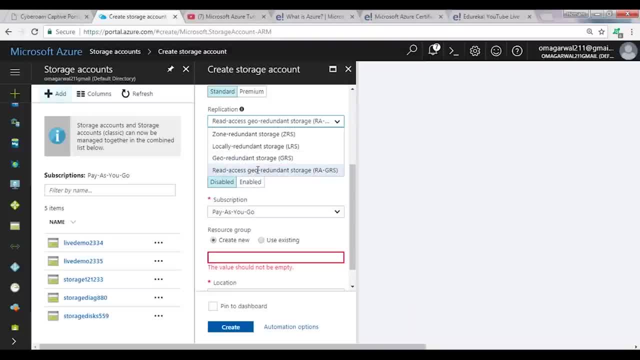 writing on it. you don't want your data to be replicated whenever you write uh a thing right and that, uh. so this is the reason that read access geo redundant storage is kind of cheap, but since ours is the demo today, so i'll select locally redundant storage and then the subscription. 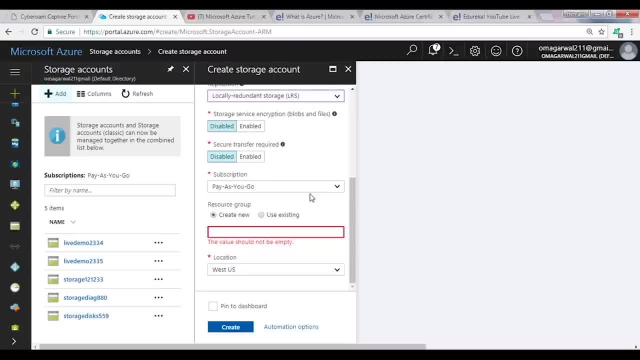 you can choose uh, pay as you go or free tier in your option if you have created a new azure account. and then comes the resource group. so resource group is nothing but a group of resources. so it is basically created to manage your resources uh more efficiently in the case uh when you have. 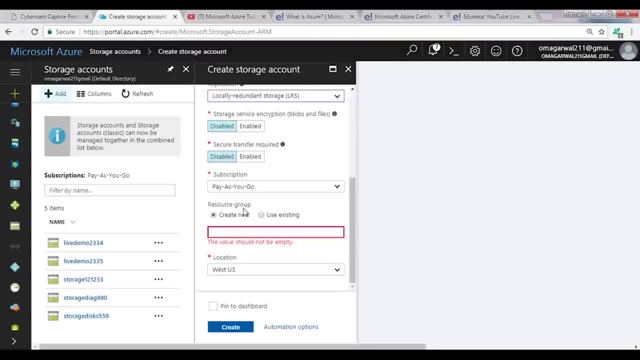 a large use case wherein you're deploying a host of different services. if you include them inside one group, it becomes easier to manage, because if you want to delete all the resources, you just have to delete the group, and all the resources and the dependencies will be deleted automatically. right, 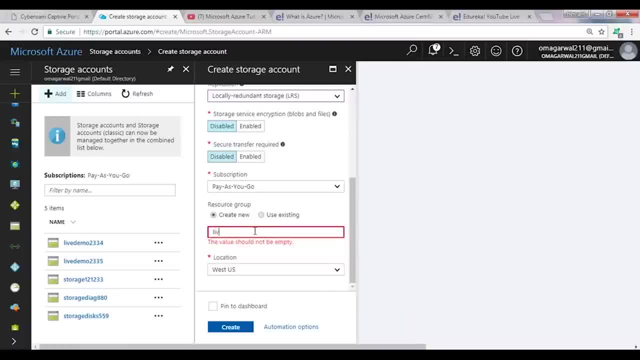 so you can see that the resource group is helpful. so we'll create a new uh resource group today. let it be live hyphen demo one, right, and we'll pin it to dashboard and we'll click on create. so when we pin it to dashboard, it basically uh has a shortcut on the desktop, uh for azure, so let me uh. so while 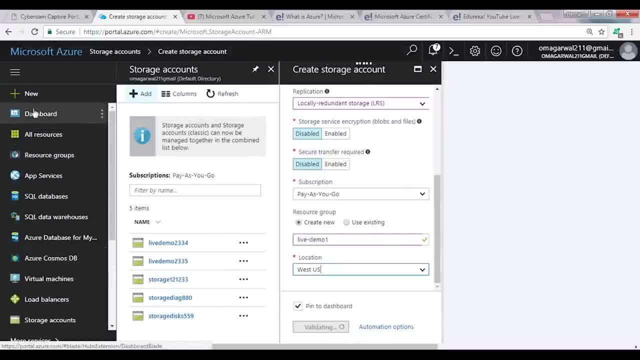 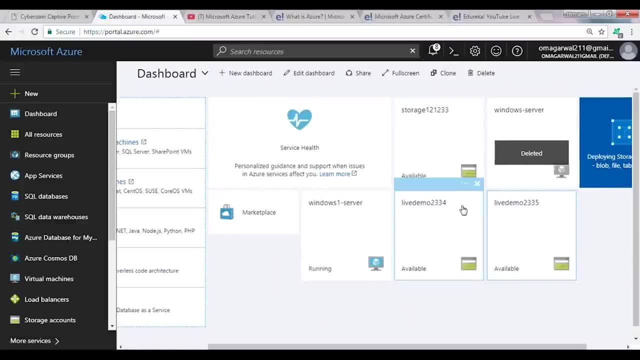 this is being created. let me show you how that dashboard actually looks like. so that dashboard basically gives you all the shortcuts that you want. so this is the dashboard, guys. so you get all the shortcuts that you want to your services, right? so my uh live. so my, my storage account. 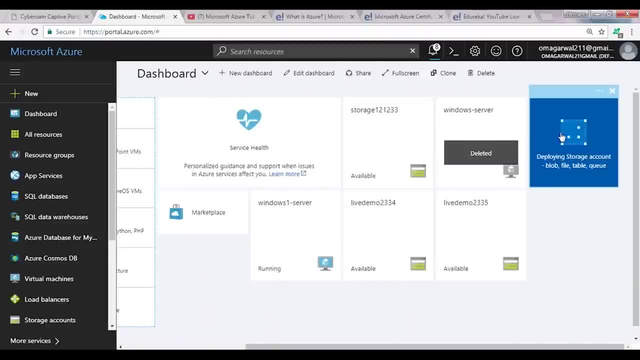 is now being created. it is called live demo 2336, so i can quickly access it from here, rather than to go to my store particular storage account over here and then accessing it all right. so while this is being created, guys, this was about azure storage. this is how you create a storage account. let me 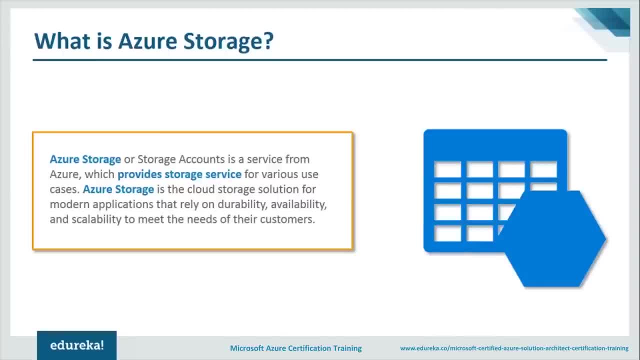 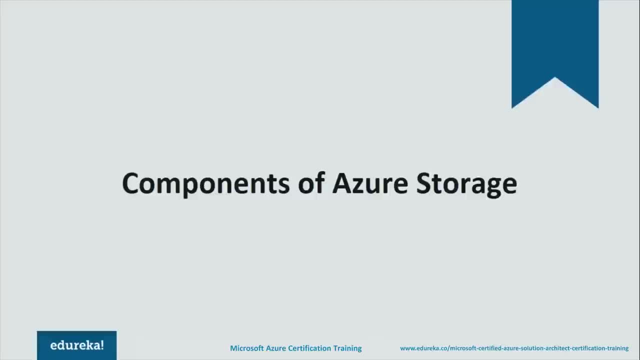 come back to my slide. so this is what an azure storage is. let's move on to discuss the components of azure storage. so right till now, we have discussed how you can create a storage account, but inside a storage account you have a host of different services which you can make use. 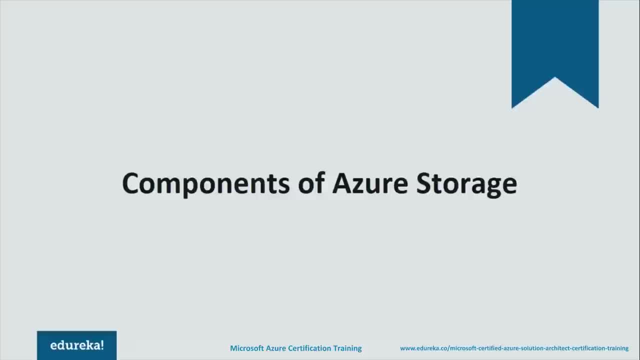 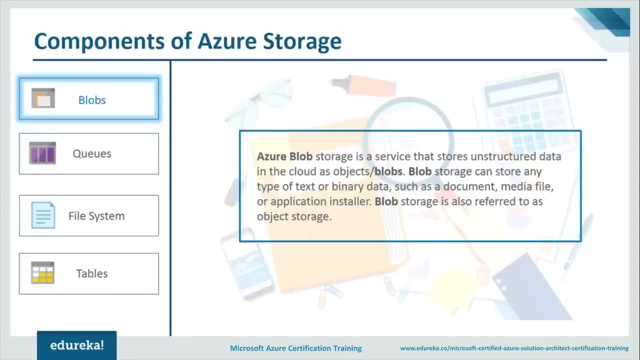 according to your use case. all right, so the first service is called the blob service. so what a blob service? so a blob service is nothing but a file system service wherein you can upload any kind of file, right? so for those of you who know about aws, so aws has a service called s3, right? 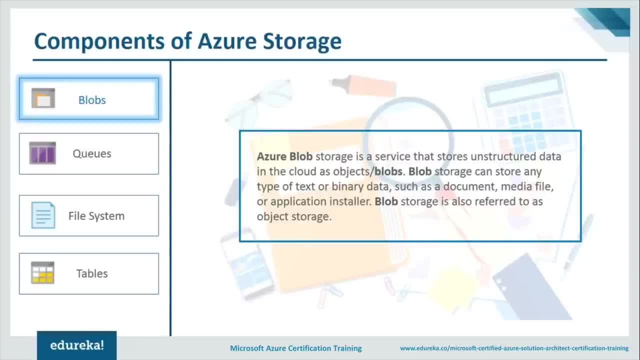 like s3. right, there is nothing changed into it, just the name of the service is called blob. now, inside blob, you can upload any kind of file and then that file can be accessed by. depending on the permissions that you're going, it can be accessed by any anyone on the planet. 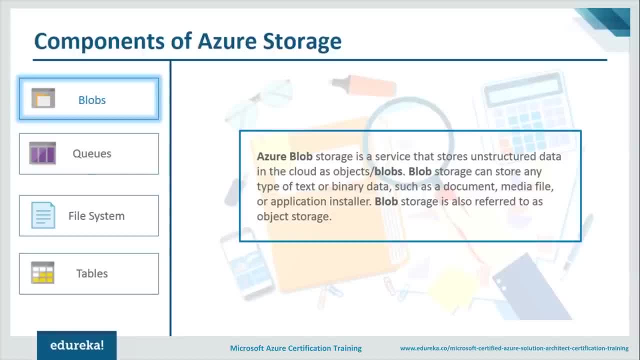 for example, you have created a website and it's showing some images. so those images rather being on the website's server, it could be there on blob and can be accessed directly through the link of any object that you actually upload in the blob. all right, having said that, guys, let me quickly show you. 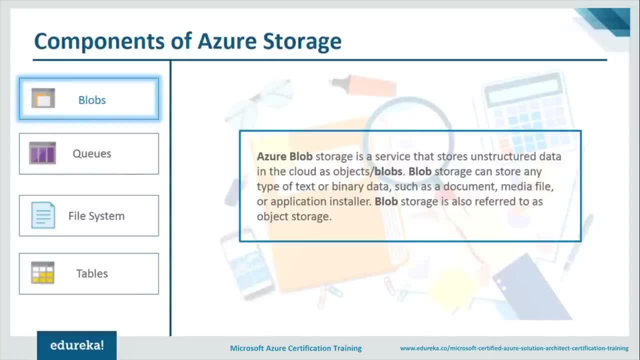 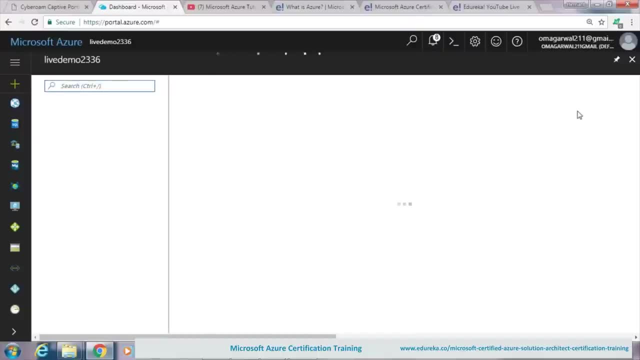 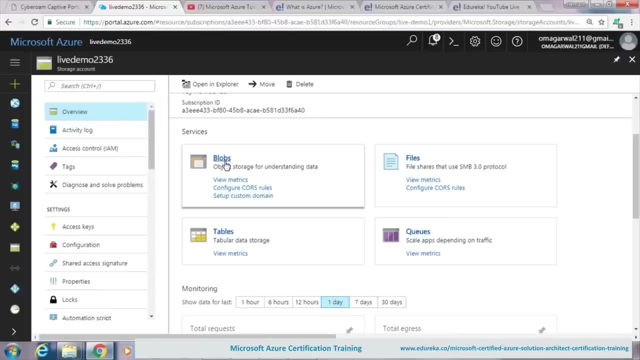 how you can create a blob storage. so let me go back to my dashboard. so, as you can see, my storage account has now been created. so if i go into my storage account, i'll get the screen wherein i have to choose a service. all right, so let me click on blob. so, because that is what i want to create, i 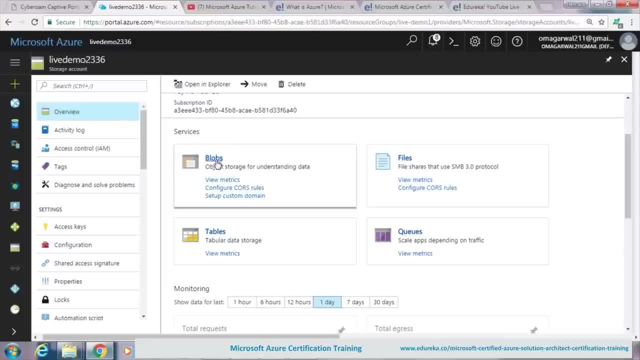 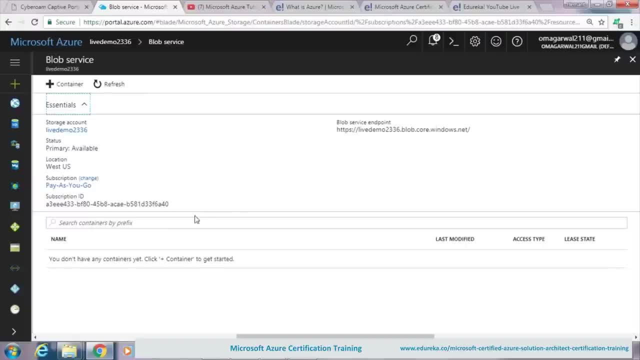 click on blobs, i'll open. open it in a tab. okay, i'll open it in the same tab, and then it will show me a screen where it will show me that there has nothing been added right. so there are no containers yet. so what are containers? containers- 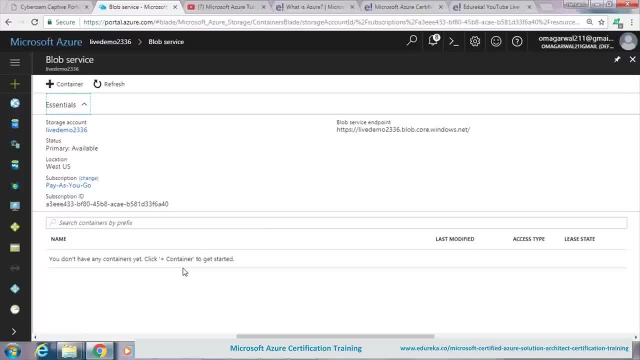 are nothing but folders that you have inside the blog. all right, so you cannot store anything in the root directory, that is, you cannot store, upload any file over here. you have to have a folder inside which you will be uploading your files. all right, so the folders are nothing but containers, don't? 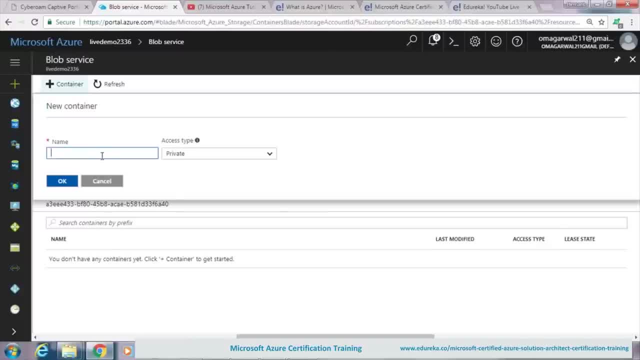 get confused with the right. so inside this I will create a container called live-demo. right, so it's done. the access type is blob, so what that basically means is: if it's private, it cannot be accessed by anyone. if it's blob, inside this particular container, all the files can be accessed, and if if it's container. 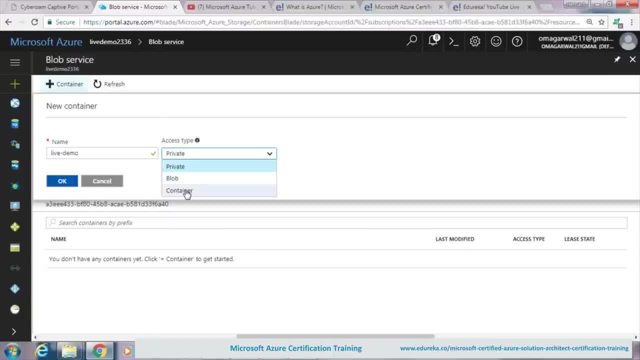 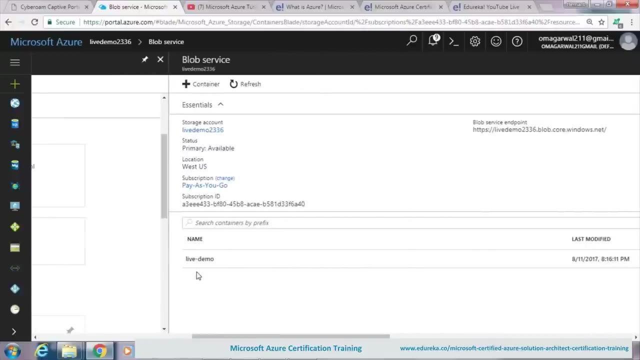 this basically means that if it inside this container you have created one more folder, that also can be accessed. but when we select blob, only the files can be accessed. so we'll select blob and we'll click on OK, and it will hardly take a second to create a container in the blob service. alright, 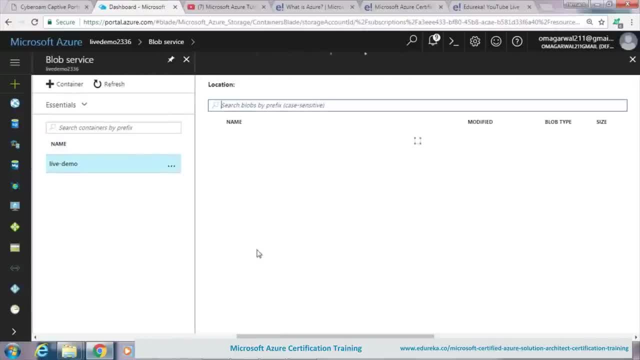 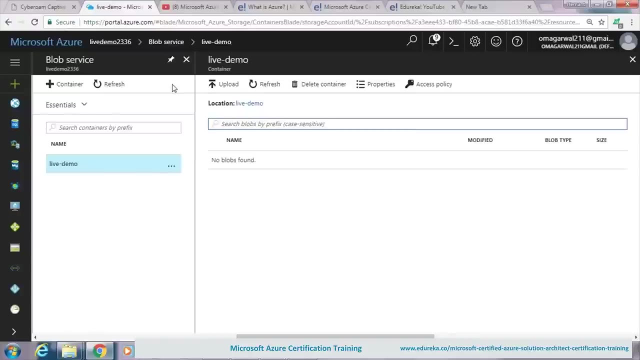 so we have a container now which is the live demo, and if you go inside this container, there is nothing in it as of now, right. so now I have actually created a website which can interact with the blob service. so let me show you how that website actually looks like. or, before that, let me show you the queue service. let us 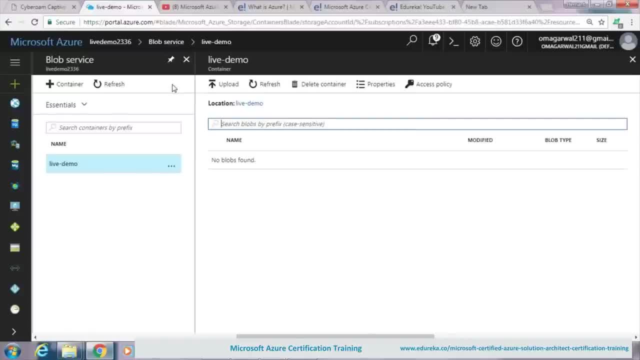 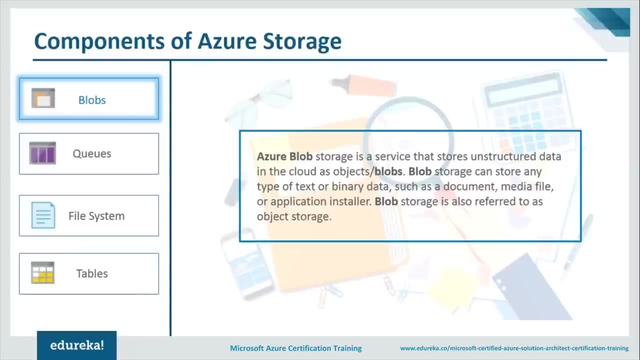 cover the queue service first, and then we'll come back and discuss the blob. alright, so let me come back to my slide. so, blobs, like I said, you have created a blob. you can upload any kind of file inside a blob using a website, or you can read the files as well from a website. alright, let's move on. 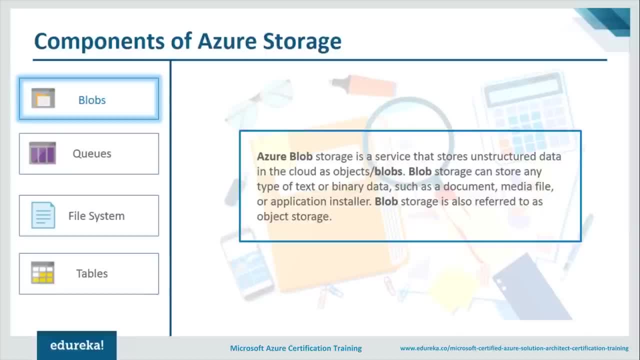 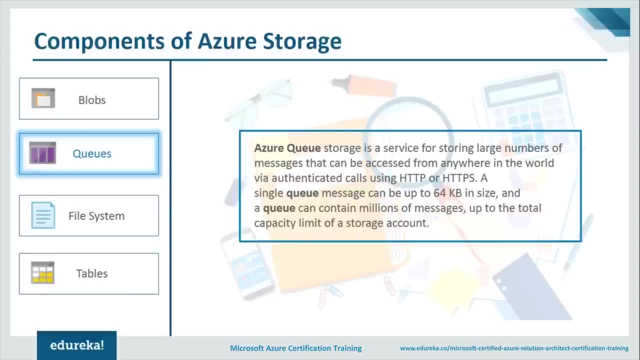 and discuss queues. so what are queues? queues are basically. it's exactly like a data structure wherein you, whatever information goes first, is the first to come out as well, alright, so you use queues to basically list jobs. so in our use case- we discussed that- we have an image processing application which has 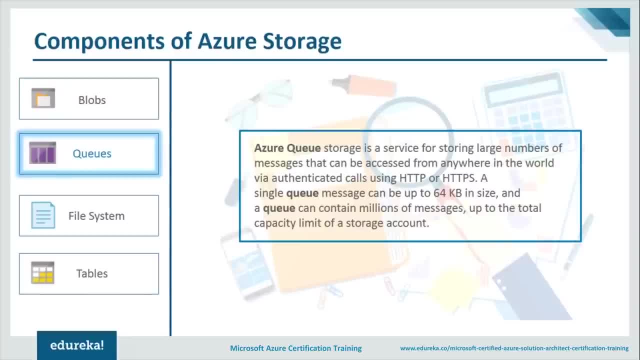 millions of users accessing it, and since millions of jobs cannot be executed at once, they are listed inside the queue so that the server, at its own pace, can fetch the jobs and execute it alright. so this is what a queue is all about. as simple as that. now, the way you can. 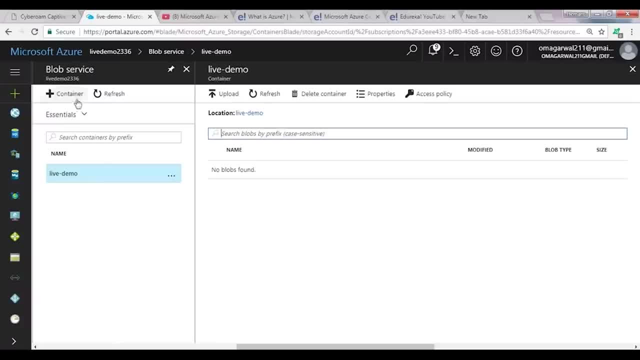 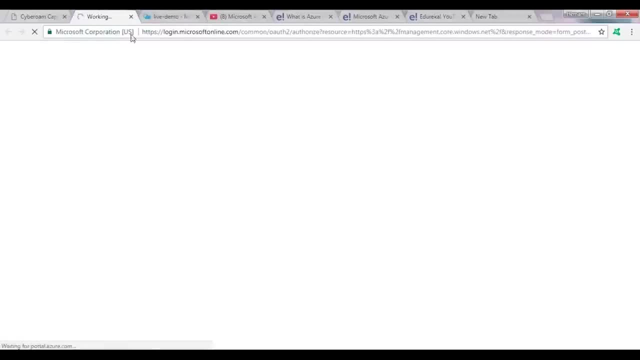 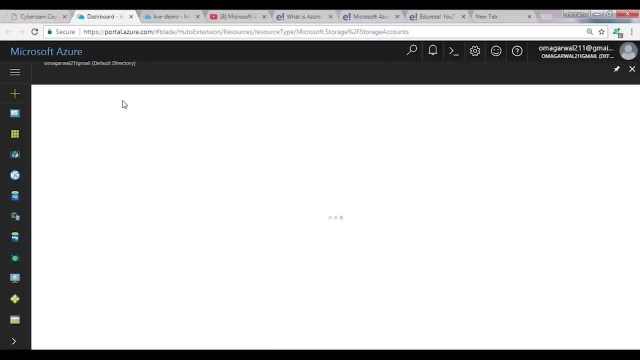 create queues in the azure dashboard is something like this: that you have your storage account right, so let me go to my storage account. so my storage account is now being opening alright. so inside my storage account, with the blob service as well, I had queues option right, so I'll go to that queues. 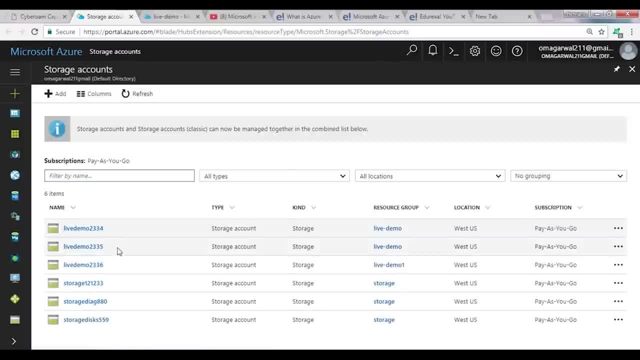 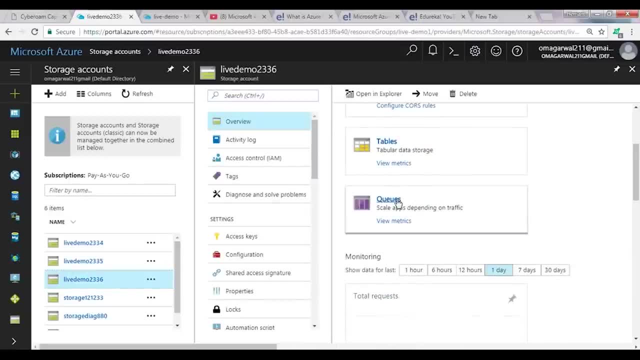 option and create a new queue. so my storage account was livePorHope, Demo 2336, right, and now I'll Ah قال choose. i'll go inside queues and i'll go to the existing queueスト signe. let me create some queuestores and then i'll go to this and this and this eye. so here, based on the 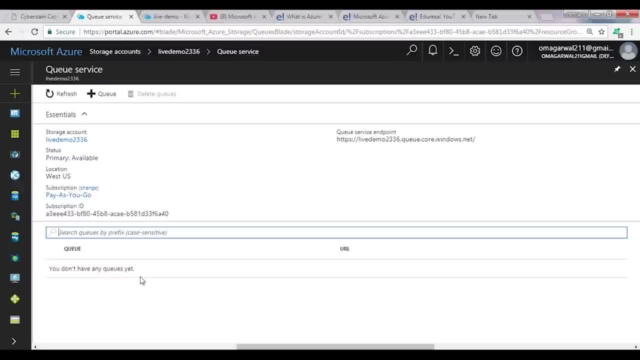 as you can see, as of now, there are no queues that have been created, so i'll create a new queue and let me call it hello123. all right, so i'll create the queue now. so my queue has now been created. now, if i go to my 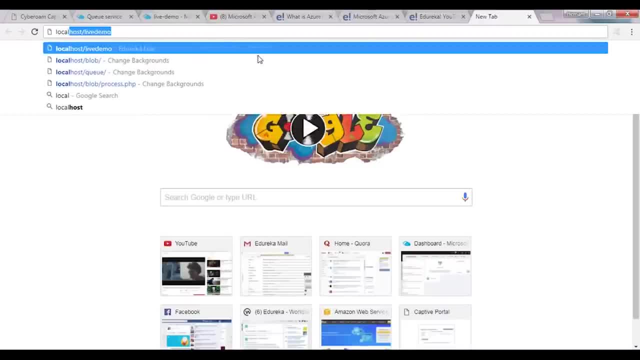 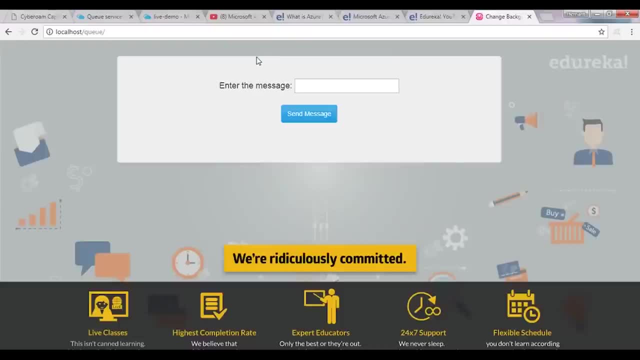 website, which is there for queue. this is how my website will look like if i want to upload some data into queue. so this is a sample website, guys, that i have created. now this website has to have the has to know how to interact with your queue service. for that you. 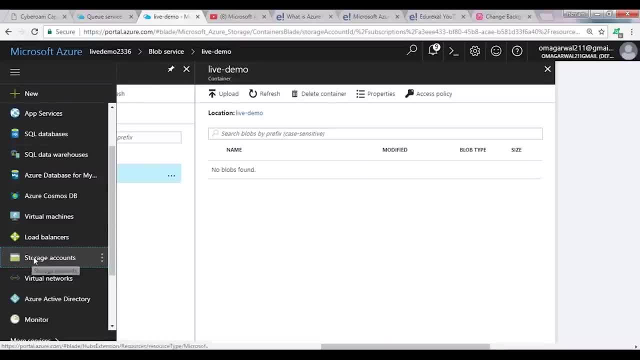 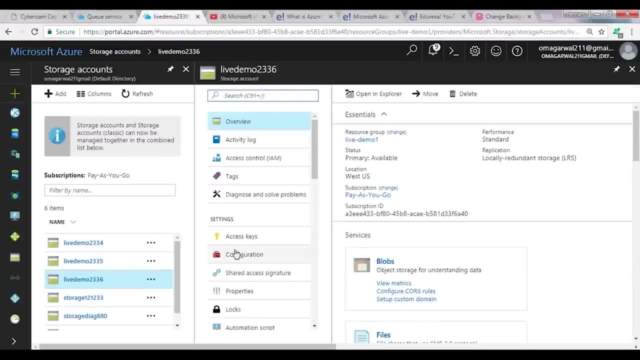 have a thing called your connection string. so every storage account that you create will have a unique connection string that you have to include in your code. now, if i click on access keys here, you'll go to your storage account and then you'll have this pane in that you have to go. 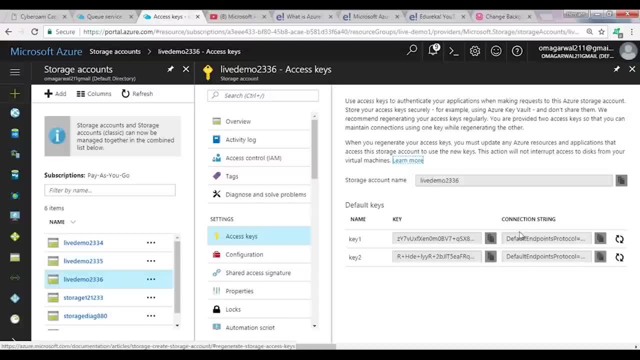 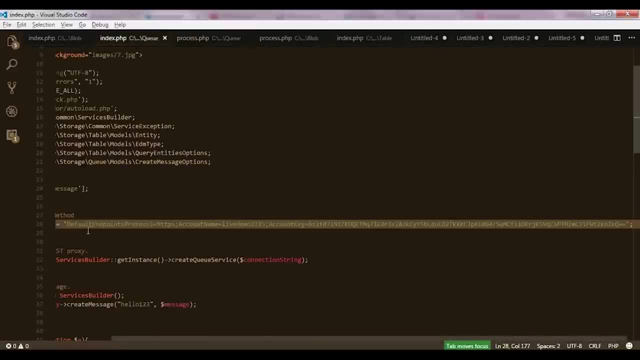 to access keys. once you go to access keys, you will have a connection string and a key, so you have to have the connection string in your code included so that your code can interact with the particular service. all right, so i'll go to my queues code. so my queue code is this and, if you can see, this is the connection string that i have to specify. 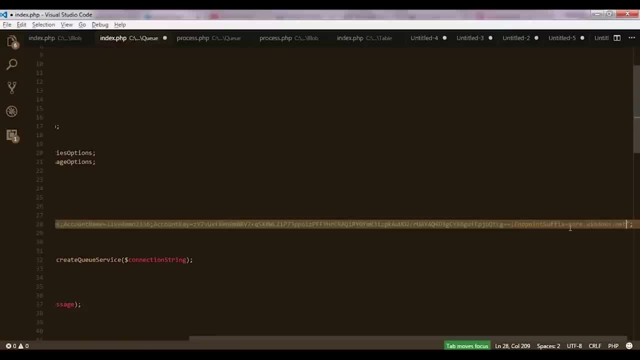 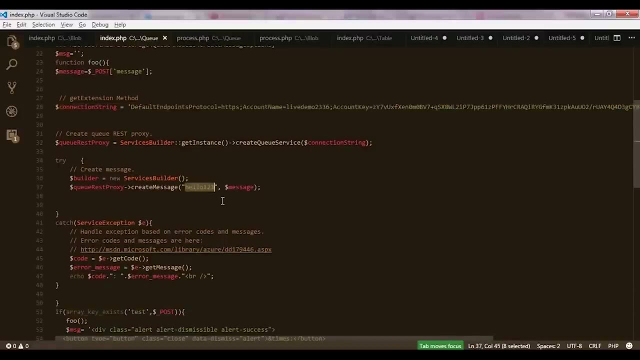 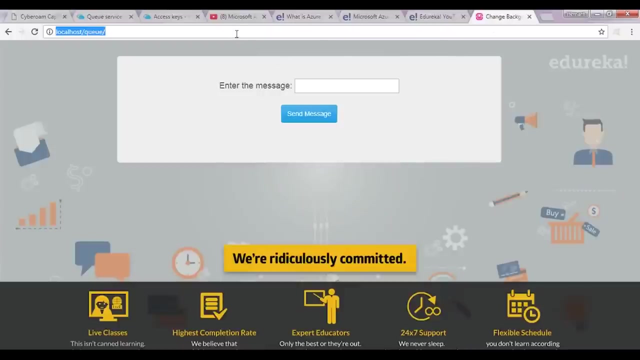 i'll copy paste this connection string over here, and this endpoint has to be removed because it is not required in the connection string. once you do that, you will save it. my queue name is hello123, so it has been already specified here. right now i'll go back. i will go to my uh website, which is this, right, so i've already specified. 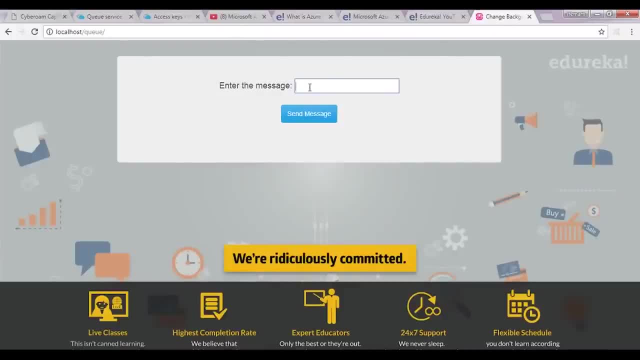 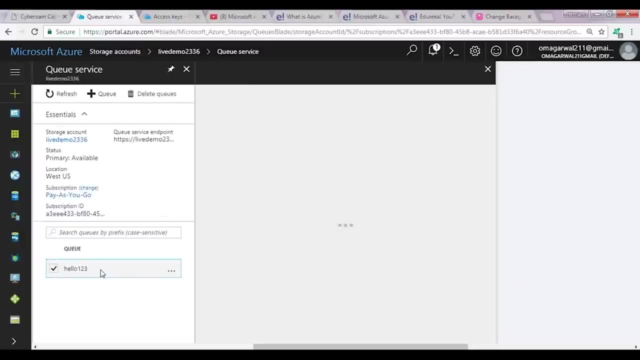 to it: uh, for it to send messages to my queue, right? so if i send a message saying, uh, hello world, right, and i click on send a message, it'll actually send that message to my queue, which can be seen in here. so as if you, if i go to my queue, you can see that a message has been added which says: 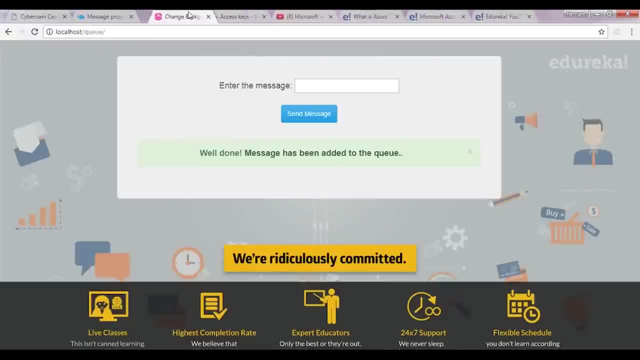 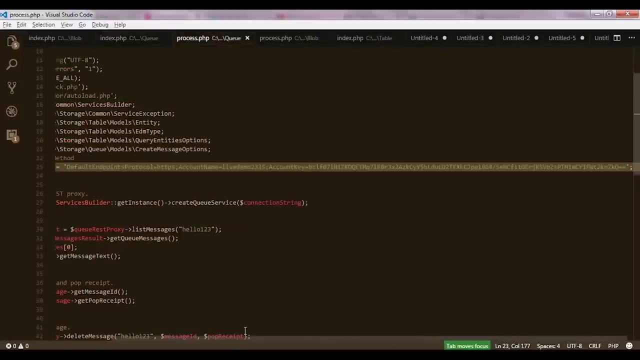 hello world. all right, so this is what i just entered. now, if i uh go on and process this queue, which is i want to receive message now, so i'll have to change uh this in the php as well. so i'll go to my process php for my queue. i'll change my connection string so that it can interact. 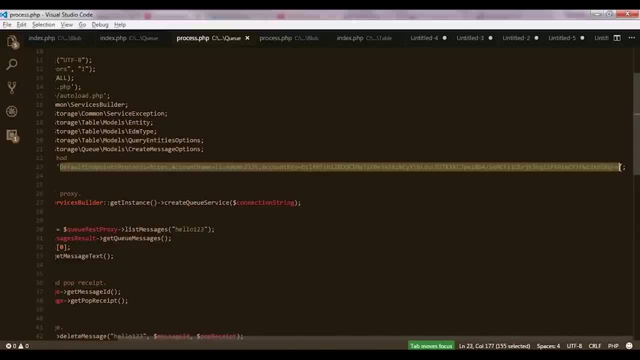 with the queue and fetch the messages from over there. right, i'll go to my connection string so that it can interact with the queue and fetch the messages from over there. right, i'll change it here. i'll change the endpoint as well, and now my code will be able to interact. 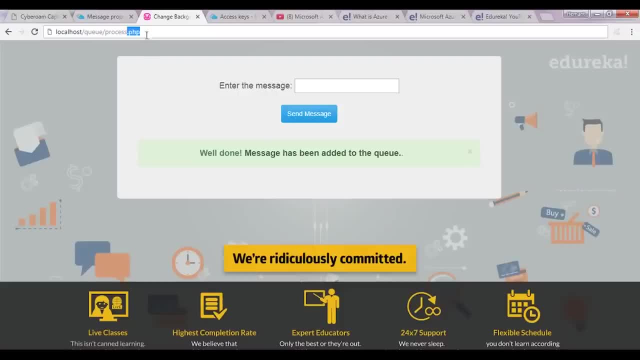 with my queue that i've just created. all right, so if i go to processphp, it will basically fetch the message from that queue and display it here. all right, so, as you can see, the message received is hello world. if i enter any other message, say: uh, edureka. 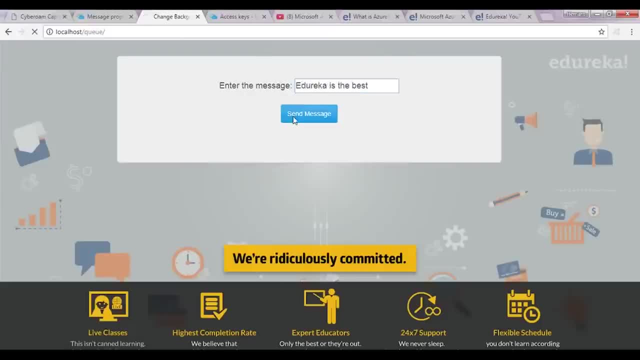 is the best right. i entered this message, i send it to the queue, all right, and now when i process it, i'll get the same message back and if you will see over here, guys, i'll just refresh it now. as you can see, the message has been processed and it has been deleted from the queue. so, as and when the message is processed, 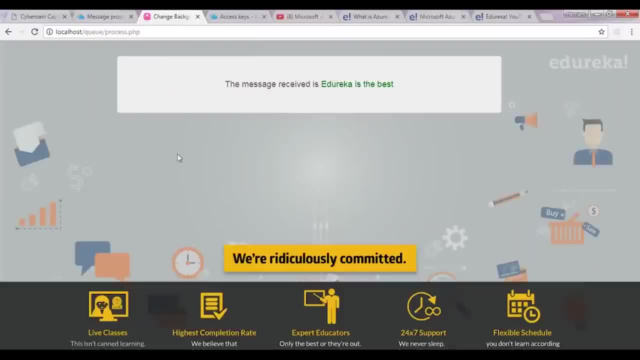 it is automatically deleted from the queue. all right, so this is how my queues work. let me quickly show you how how the message is processed. so let me show you how the message is processed. the blobs work right. so let me go to my uh blobs website. so this is where i'll be uploading a file. 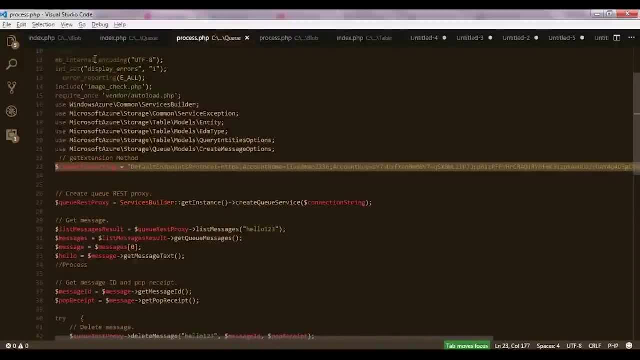 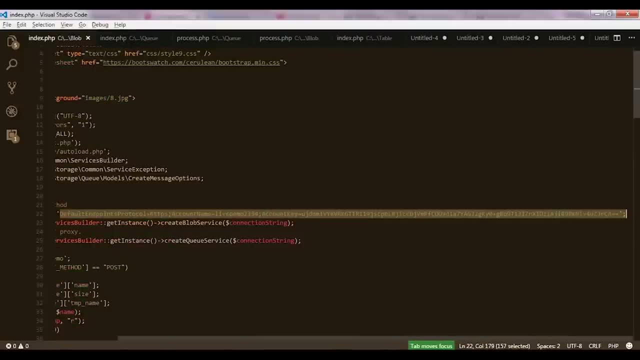 onto blobs and again i have to change the connection string again. right, so i'll go to my blob code and change the connection string which is here. all right, i'll change the connection string to my current storage account and my container name. i've already specified it to be: 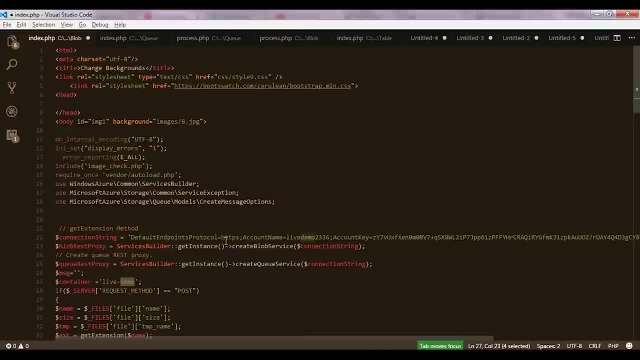 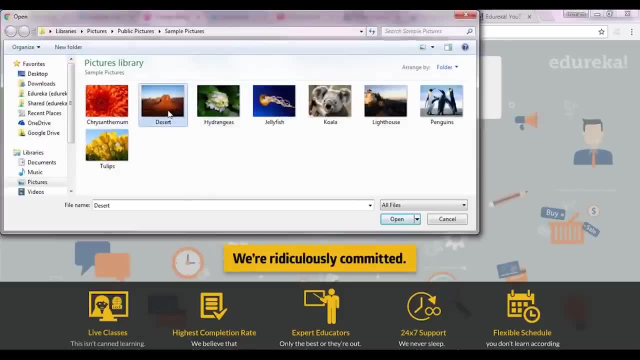 demo. right, i created a live demo container. now, if i'll save this code and if now i choose a file and say i upload the desert file, all right. so what it does is it basically renames the, the, the name of that file, automatically according to system time, so that there is no clash when two or 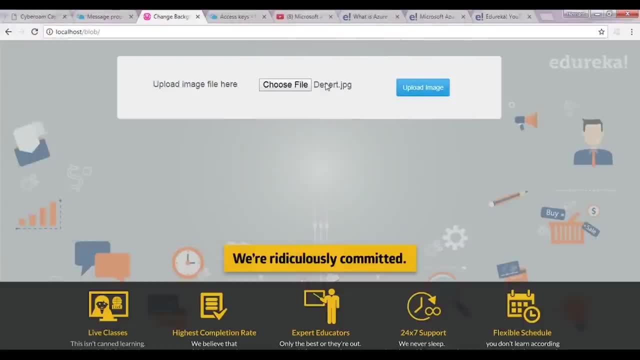 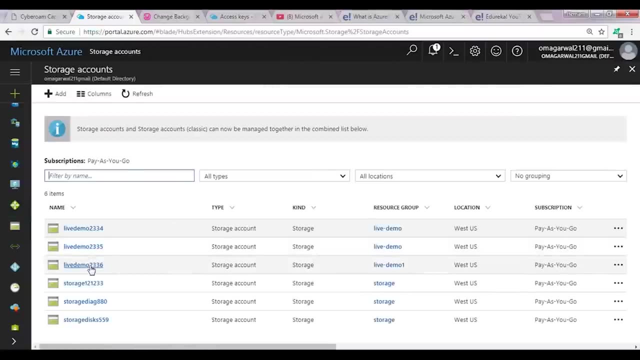 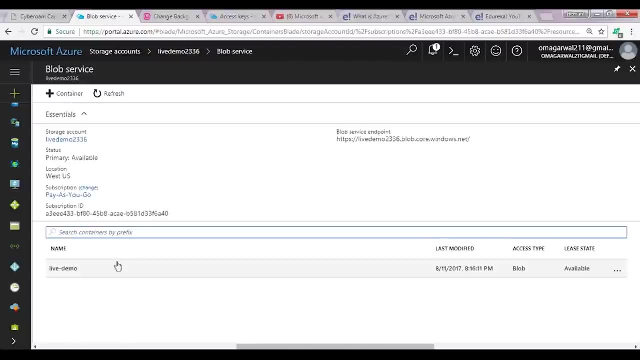 three files are updated with the same name. all right, so i'll upload this file now. so as of now, as you can see, if we go into our blob, there are no files, right. if i go inside my blob, which is here, there's no file in it, right, but the moment i upload the file from this particular website, 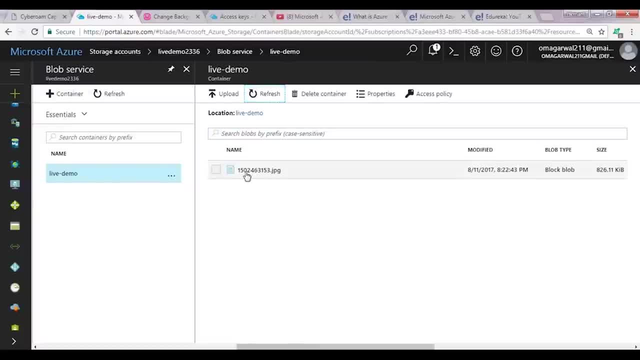 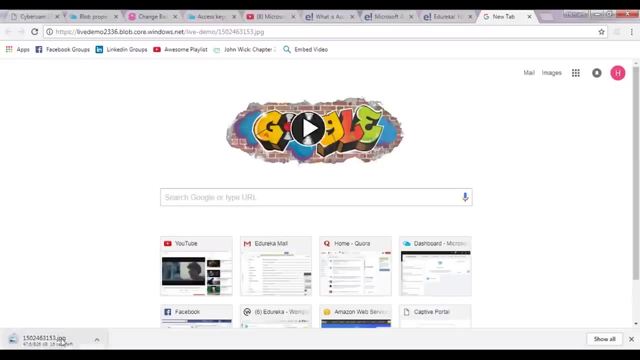 my file will be listed here. so, as you can see, my file has been successfully added over here, and now, if i go to the particular link of this file, i'll be able to download the file, to download my file, right. so my down. my file is now being downloaded, and once it is downloaded and 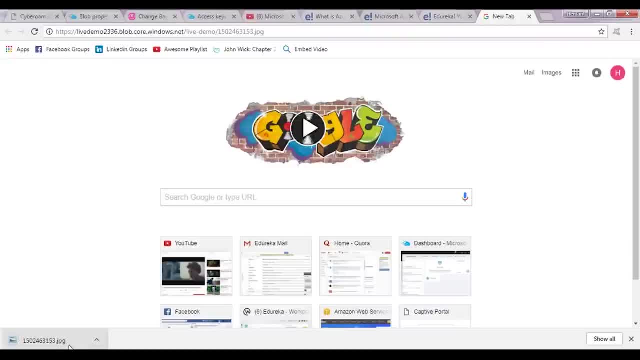 if i try to open it, it'll be the same file that i just uploaded, right? so if i open it now, you can see this is the file that we uploaded in the blob and it is now accessible on this particular link by everyone in the world. all right, so this is how cool blob is now. 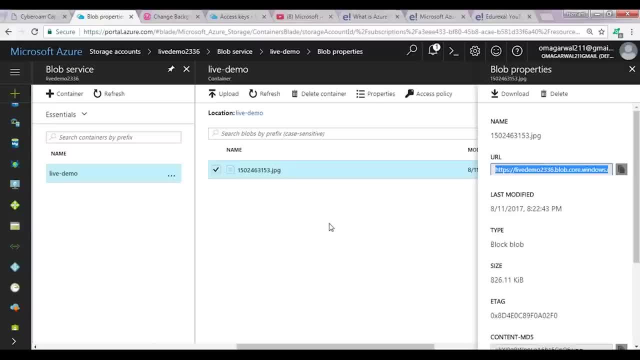 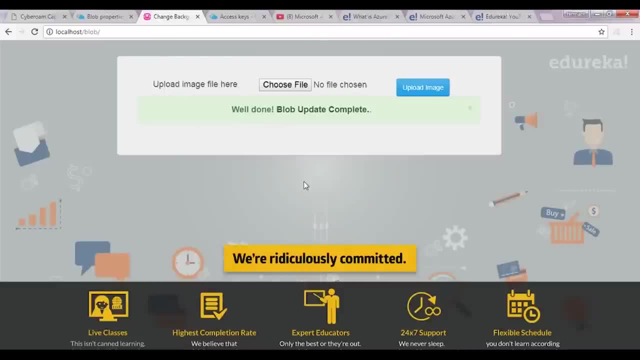 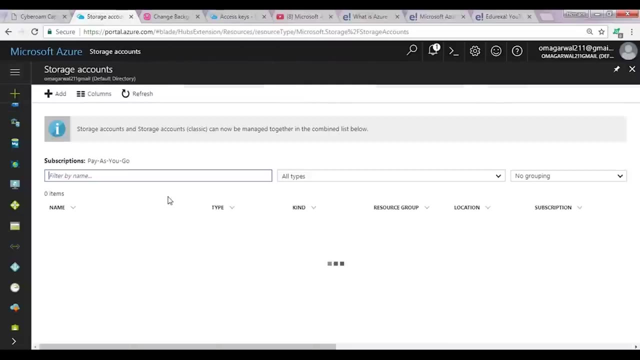 Now I'll be using Blob and Queues together. Let me show you how. So what I'll basically do now is this image, or this image that I've just uploaded has also been added to the queue that I created, So let me show you the queue. 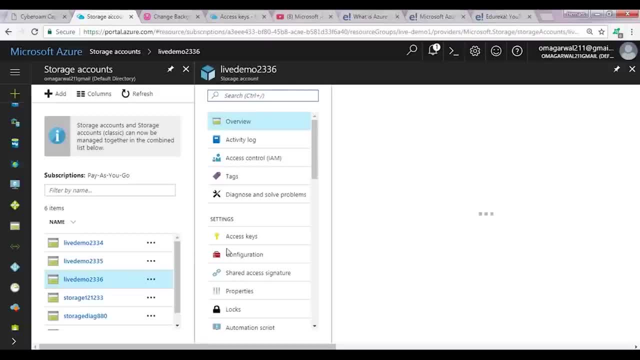 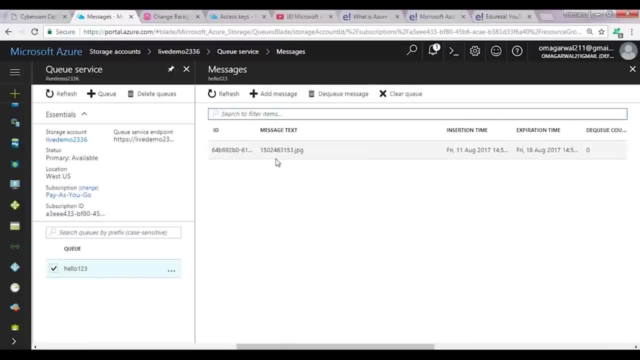 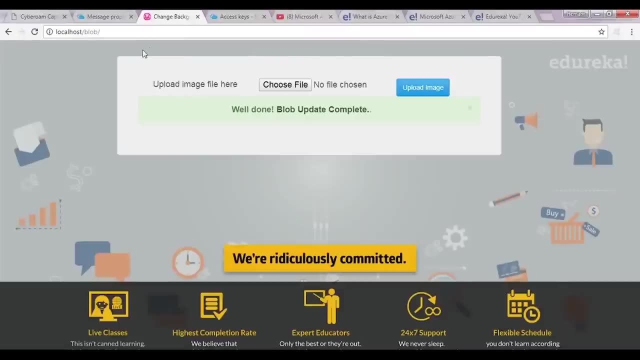 So if you see the queue, it'll list the message or the file name that we've just uploaded. We'll go into Queues. This is my queue And, as you can see, this image has been added to the queue. Now I'll process this image and the way I'll do it is like this that the image will be. 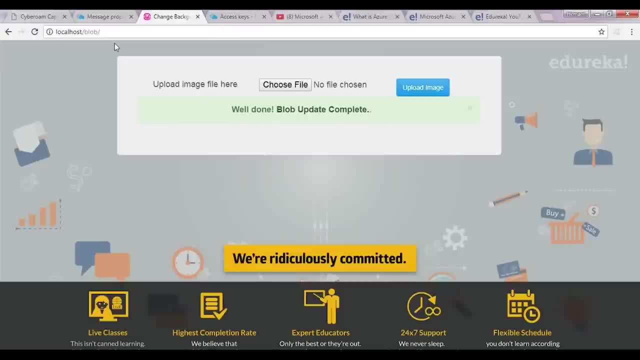 fetched from the queue and then the link of that image will be gone to and that image will go into the background of the website, right? So for that, first I have to change the code, obviously. So I'll go to my Blob Process website, right? 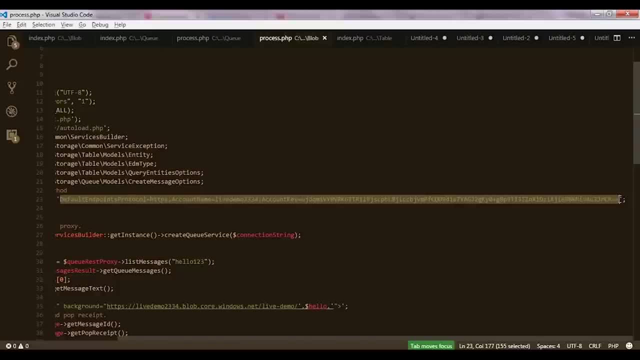 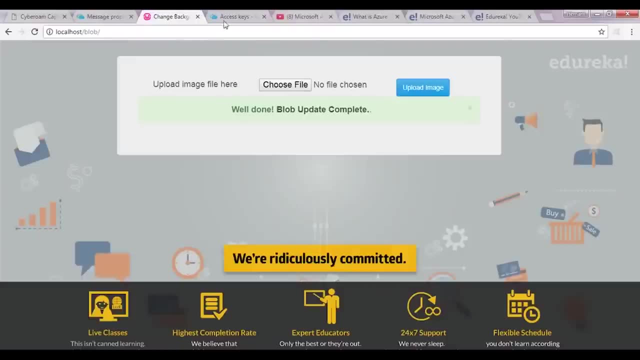 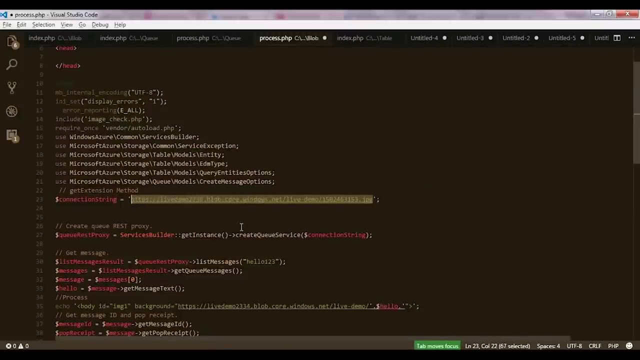 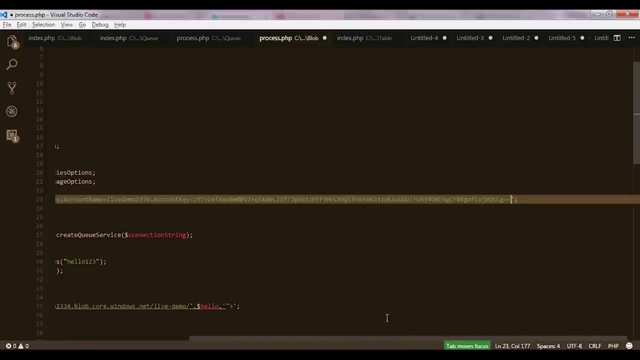 And I will change the connection string To the one that we are using right now. One second Right. So this is my connection string. I'll change it to what we are using right now, Right. And then also I have to change the link that will be accessing the file. 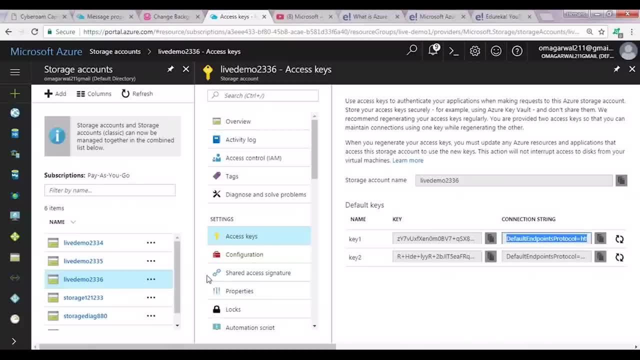 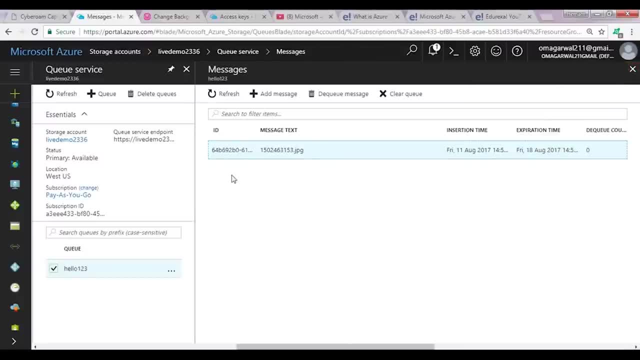 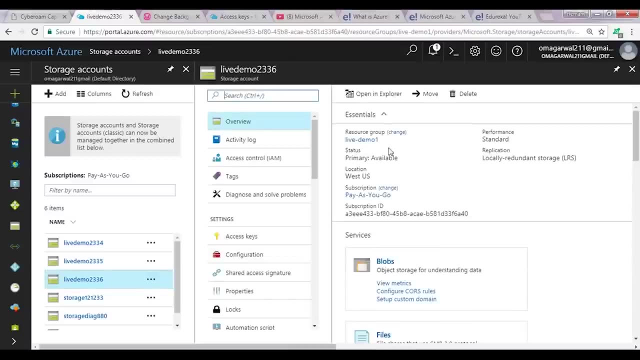 Right, So this is the link that it is accessing. So the link has changed now because the storage account has changed. Okay, All right, so let me select the link for it. So I'll go inside Blobs and I'll go inside the container. 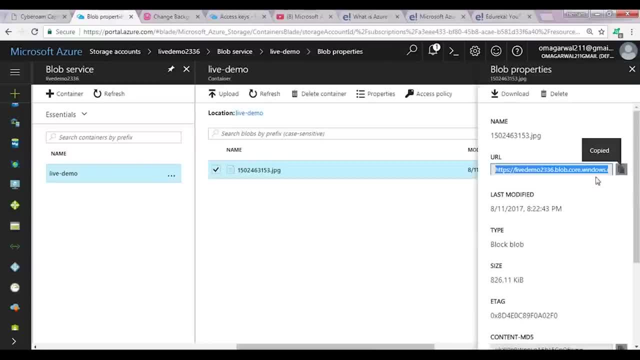 So this link is going to. so, from from this point onwards, till this point, that is, till the container name, the link will be same right. So let me copy the link and paste it in my code and I'll show you what I mean. 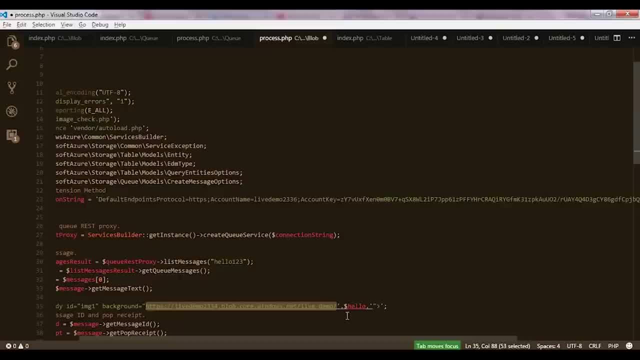 So if I paste the link here, so the link to live demo will be same and just a file name has to be fetched, Right? So this is the this file name I'm fetching from the queue and what we'll do now is it? 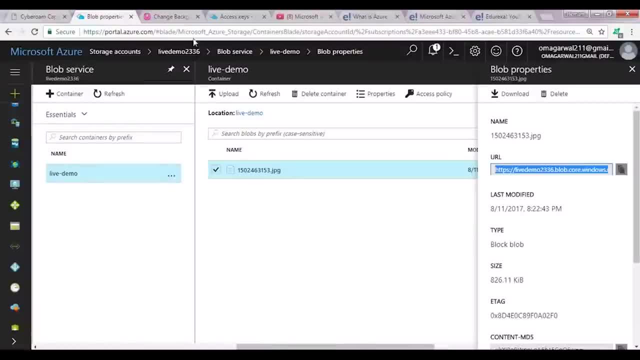 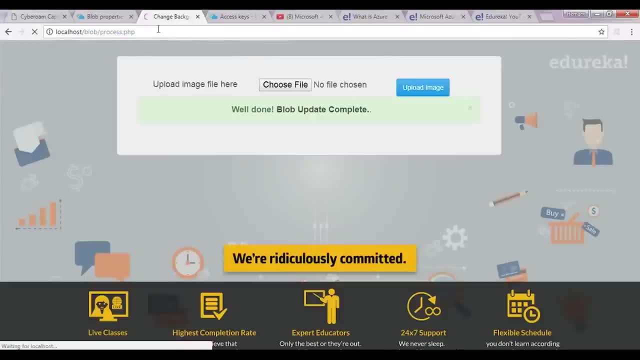 will fetch the file name from the queue and we'll change the background of the particular website, Right? So if I process the page now- that is processphp- what will happen is it will fetch the file from the queue and will change the background. 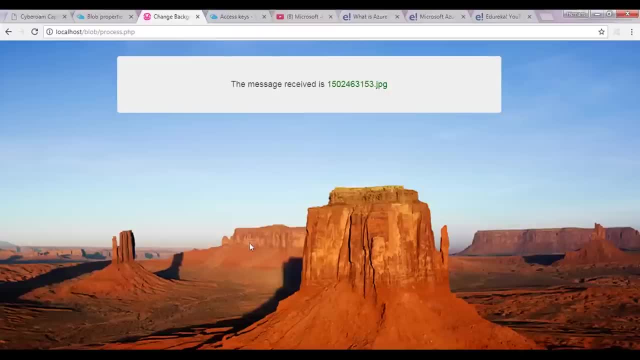 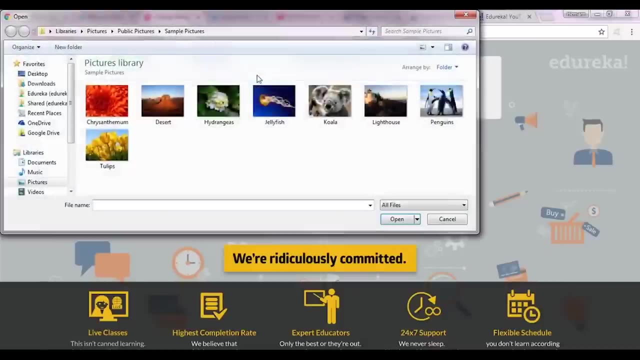 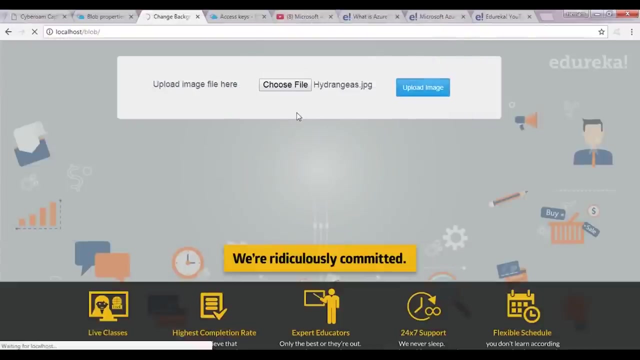 All right, So I have updated the, the desert file, right, So it is showing the desert background now. Now I'll show you how exactly queues are basically used. So, say, I upload, say, three, four files. right, I upload this flower image and, mind you, the file, the message that we just received would. 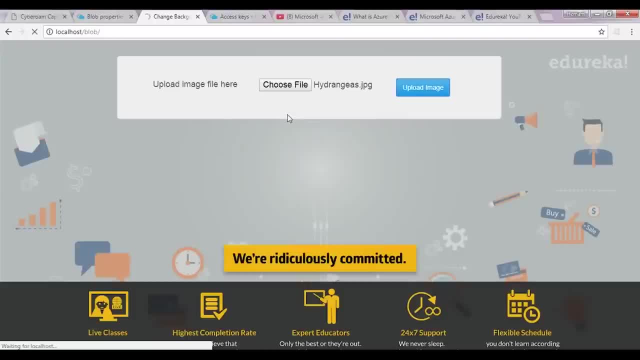 have been deleted from the queue, All right, And I'll just show you whether that is working or not. So I'll upload this flower file. Uh, it might take some time because of the files are kind of large, right? So, uh, the file will be uploaded. 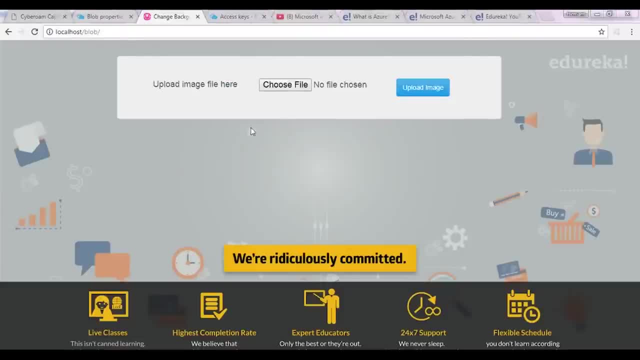 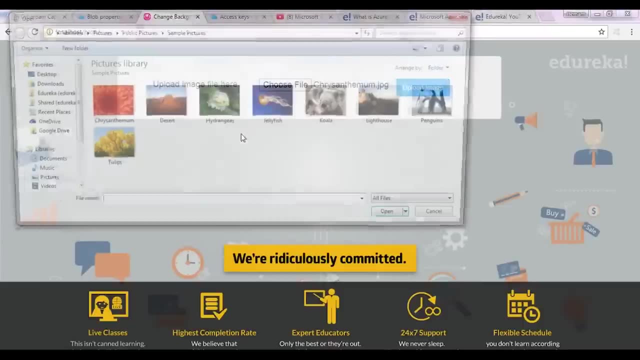 Okay, It gave me an error. Let me upload it again. So I'll choose a file. So sometimes when the size uh, when the uh, uh, the size of the file is more, it throws you an error, right? 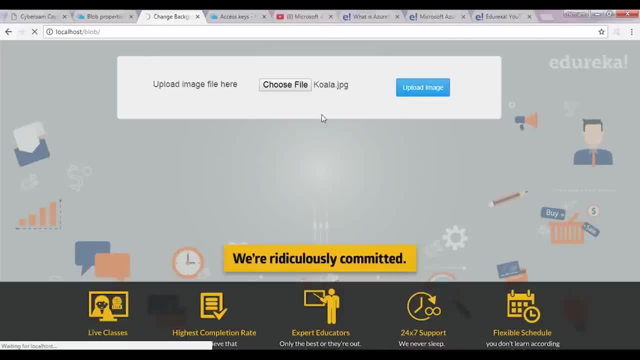 You can't do anything about it. So let me uh upload the file again. So once it is uploaded, guys, I, I I'll be able to see it. I'll be able to see it here, right? So I have like three files right now. 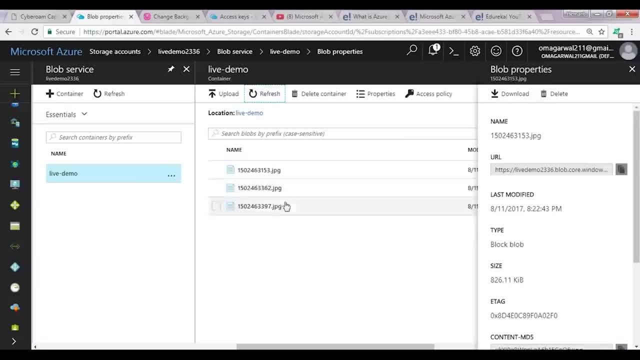 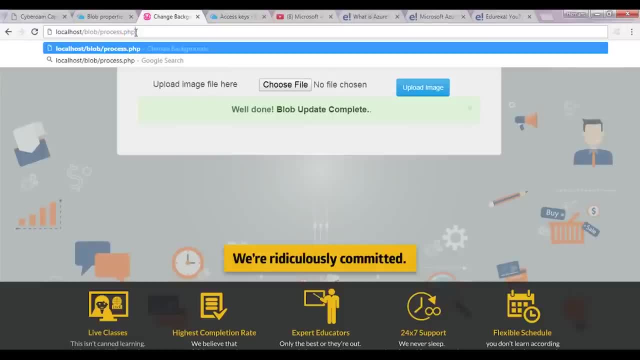 So it says a well done, blog date complete. And if I refresh it I'll be able to see four, three files now, Cool. So if I go to processphp now it will not list me the previous file that I uploaded. 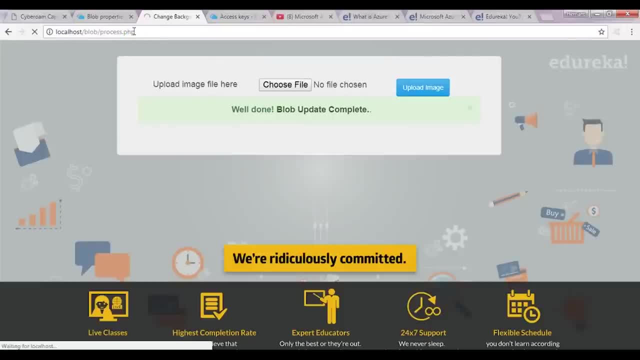 but the recent file that I just uploaded. So let me go to process, and now it'll show me the image that I've just uploaded. All right, We'll fetch it from the queue, the file name, And then it'll show me in the background. 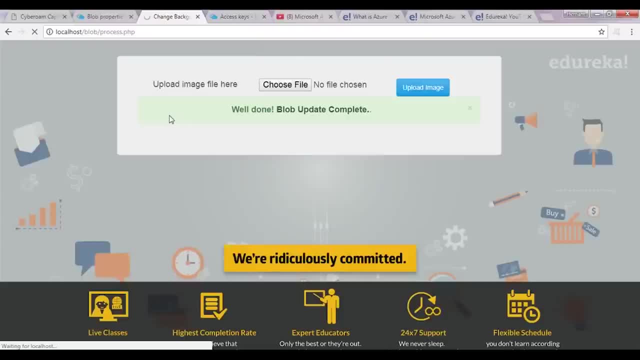 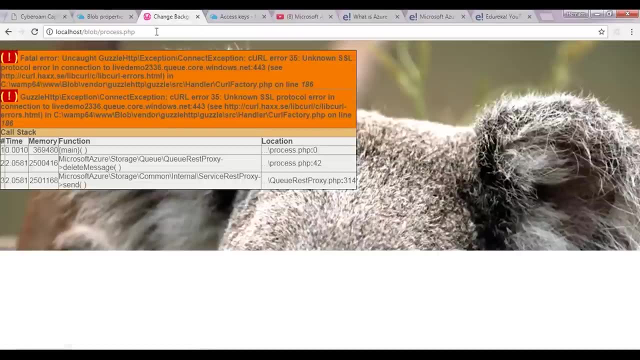 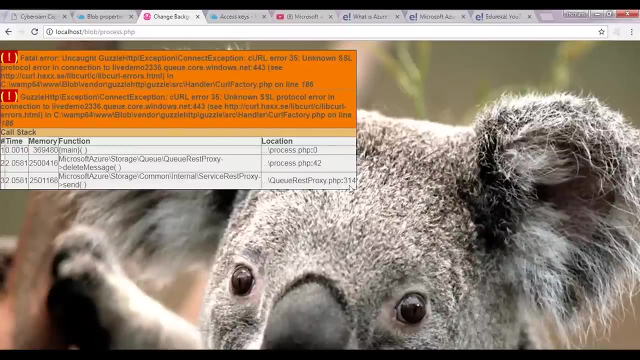 All right, The net is a little slow. bear with me, All right. So, as you can see, the file has been there. I'm getting some weird error where, just because the net is not working, but forget this error, guys. You can see, you. you get the image in the background. 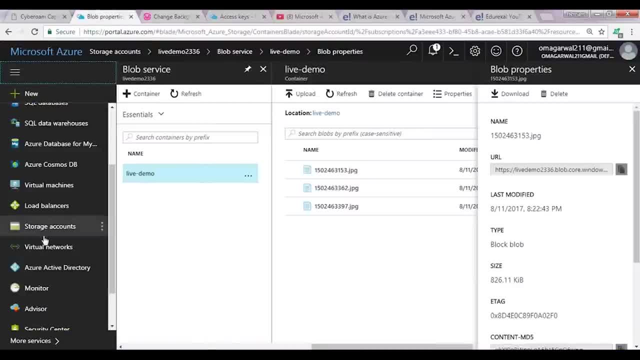 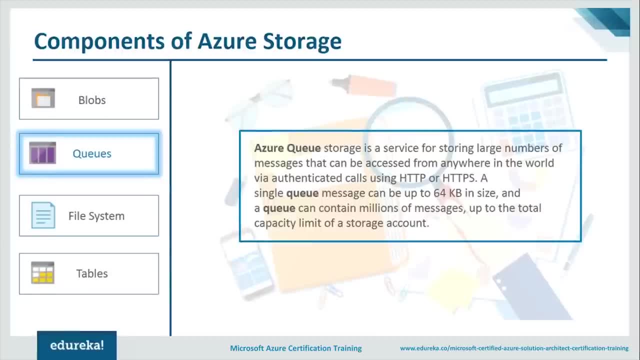 Right, So similar as a case. Now let me go to my storage accounts. So we have discussed queues and blobs. now Right, go to my slides. so we've discussed what blobs are. we have discussed what queues are. let me go to my 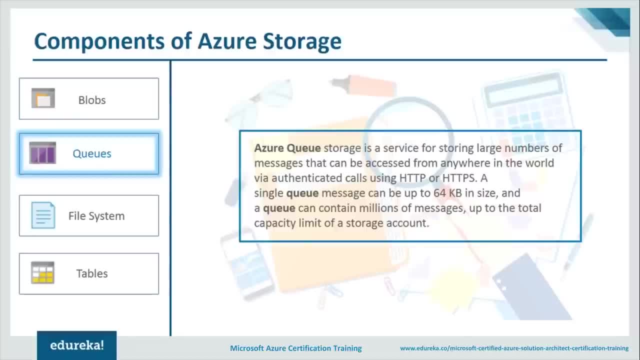 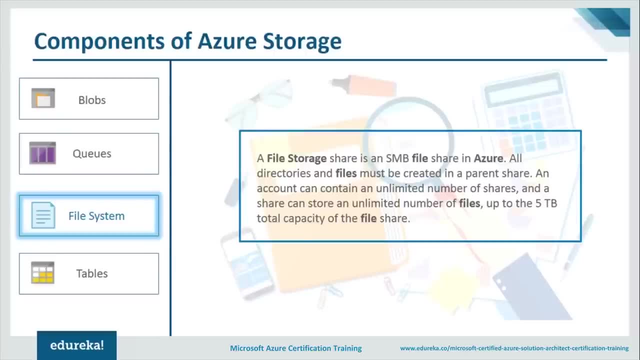 file system, which is the best thing that i've figured out in azure. so with file system it is exactly like blobs: you can upload any kind of file, but with file system you can actually mount it as a drive on your computer. all right, you can use it as it, as if it was an extended drive in your own. 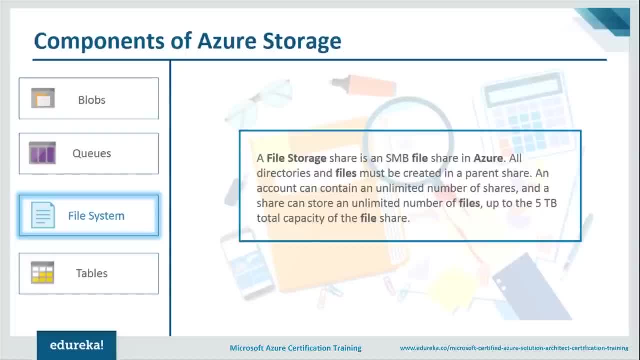 computer right. but and also you get an authentication protocol with it, which is called the smb 3.0 protocol, which is used by servers when, whenever, there is a file transaction, so that authentication you'll also get when you're using the file system and to and how you can mount it. 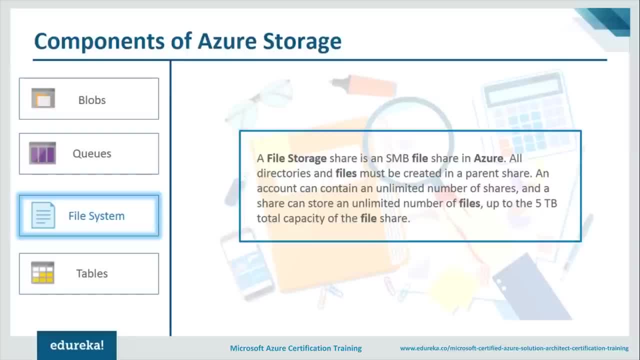 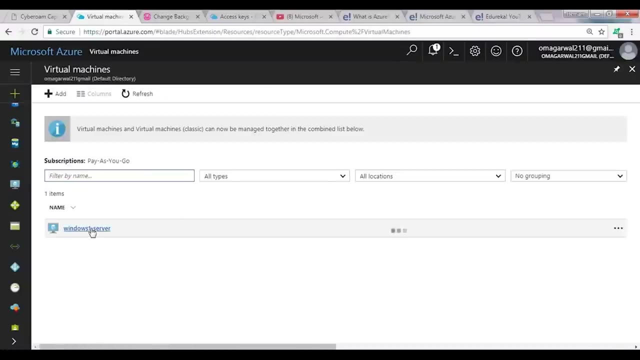 let me show you how. so, first of all, this mounting process is not available in windows 7. it is only available in windows 10 and above. so what i've done is i've deployed a virtual machine in azure. let me show you the virtual machine, right? so this is my virtual 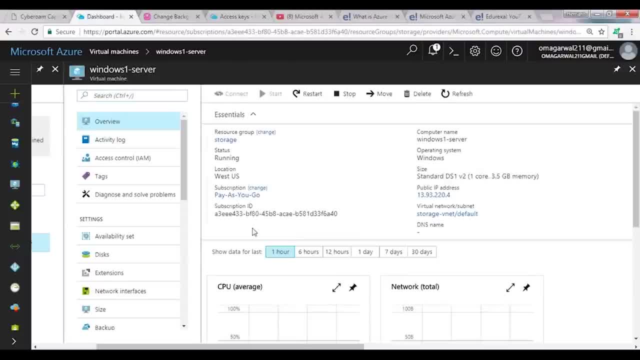 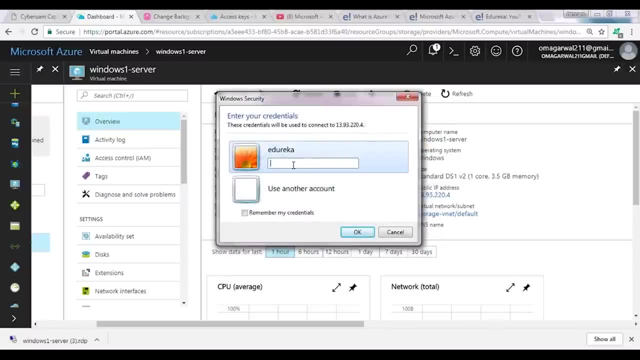 machine. so i've deployed windows 2012 server on this. now what we'll be doing is we'll be mapping the file that we'll be creating in our storage account in this particular system. all right, so i'll connect to it and now it'll ask me the username and the password, so i'll 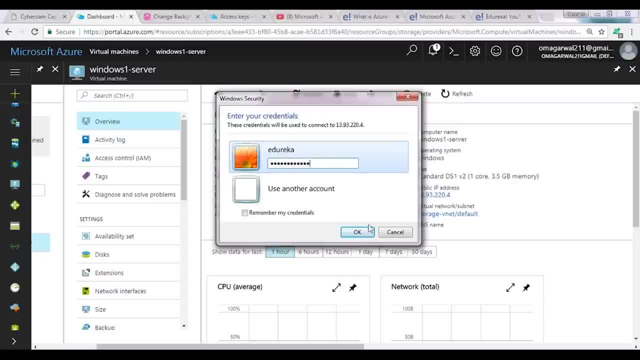 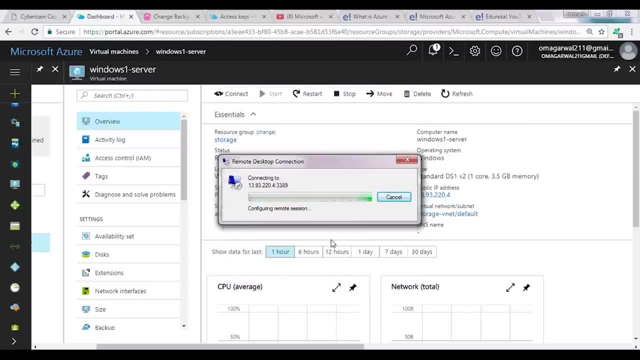 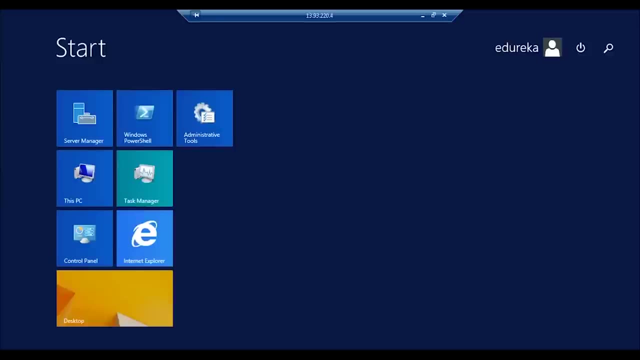 specify the password and i'll click on ok, okay, yes, and then i'll be connected to my system. so i'm in. so this is my system, guys. so if i go to my computer right now, as you can see, there is no drive that is listed right. so we'll be creating a network drive over. 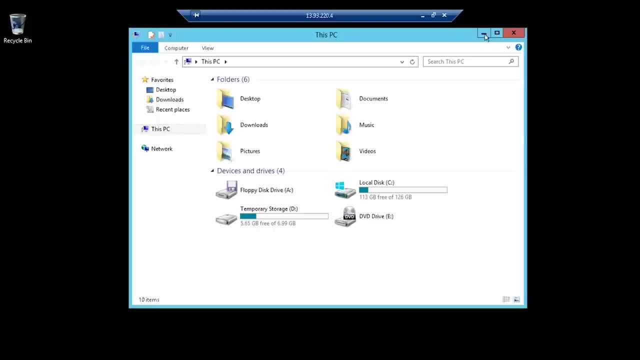 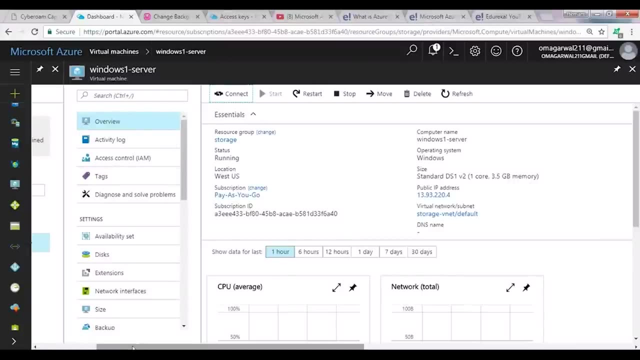 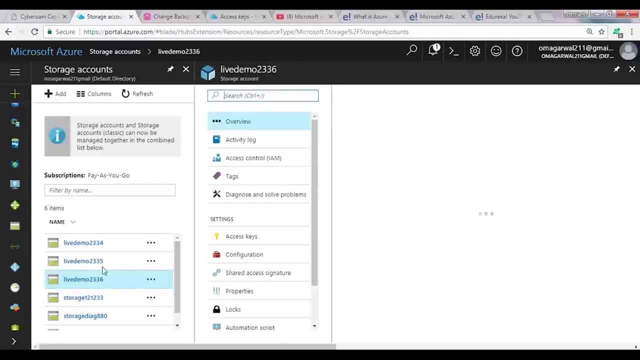 here on which we can upload any kind of file. now the way to do that is to first go to your azure dashboard and create a file over there, create a file system directory over there, right? so we'll go to our storage accounts. so it is in live, demo 2336, and then we'll be going to 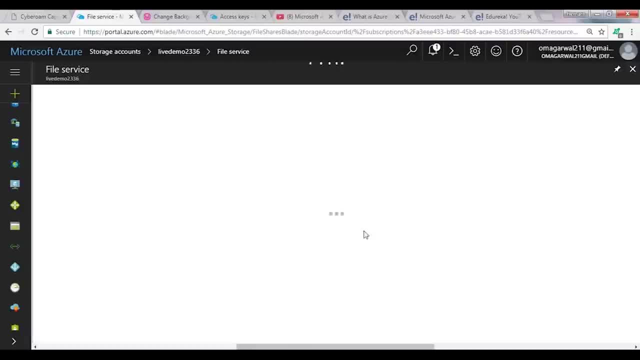 files, right? so as of now, as you can see, there is no directory which has been listed here. so i'll create a file share service and let me name it something as my drive, right? and the quota is basically: how many gbs of drive do you want, right? it can go to terabytes, but since the drive is 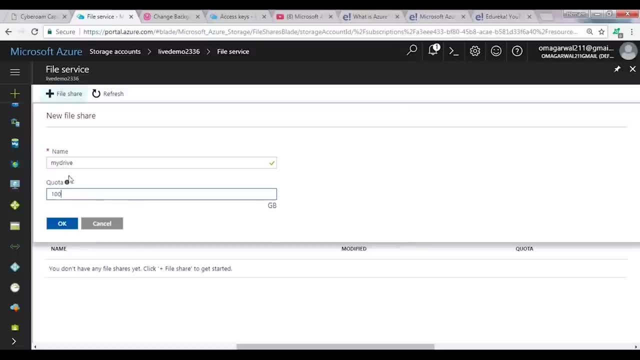 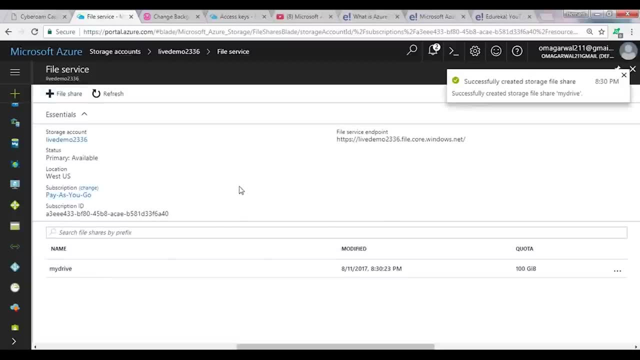 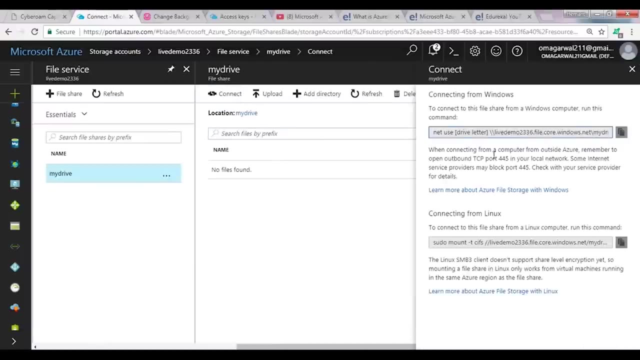 i'm doing a demo. let me create a 100 gb drive right now. right, so i'll create a 100 gb drive and i'll click on ok. all right, so my drive has been successfully created. right, so i'll go to this drive, i'll click on connect and then i will get this command to connect to it. all right, i'll copy. 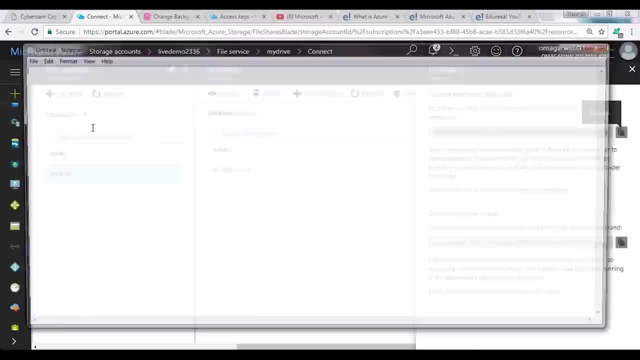 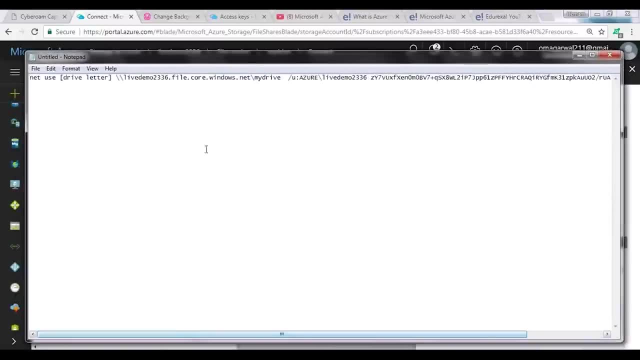 this command and i'll paste it in the notepad. so i'll use this in my server that i've just deployed. now, how will i use this now? if you look at this command, guys, this is the address of your server. all right, so this is the. 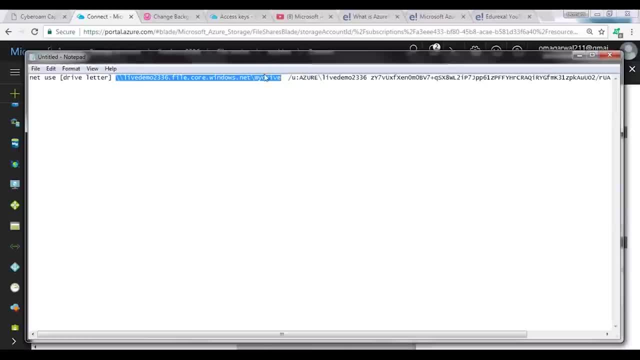 address of your storage account and this is the file share that you have just created, which is called my drive right. the username to access this would be azure slash live demo 2336, all right, and the password for this would be the key which has been specified here. now i have to specify. 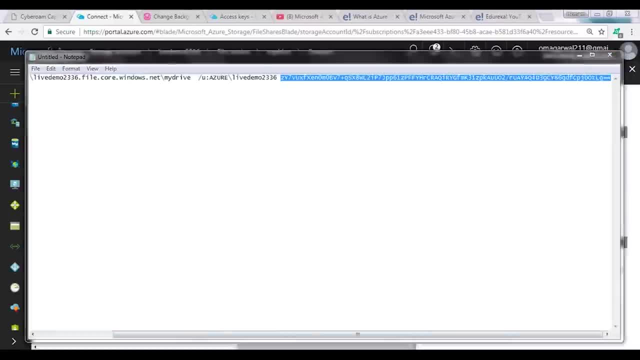 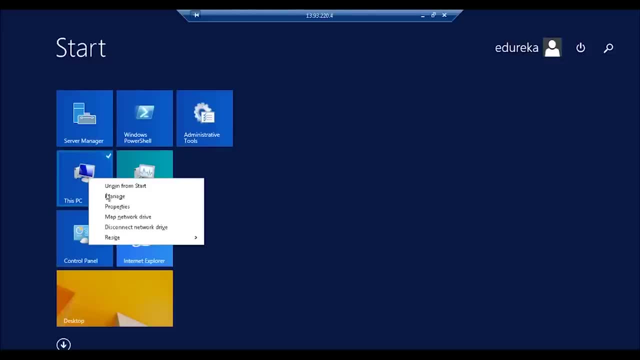 everything in uh that i've just mentioned in this server that i've created. so i'll just copy this and i'll just copy it, all right. so the way you'll map the network drive is like this: you'll go to pc, you will right click it and you will click on map network drive. 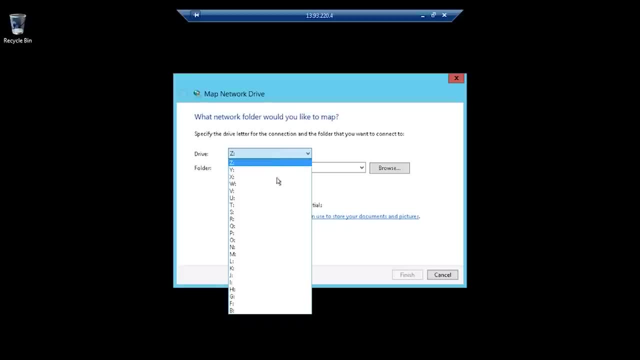 all right. now it will ask us the drive name that we want to allocate it. so, for example, we want to allocate the k drive to it, all right, and in this particular thing, you will be putting in your address of the server, right? so let me copy the address of the server, which is this: 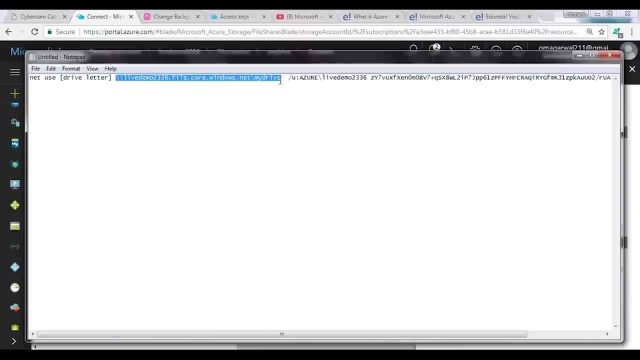 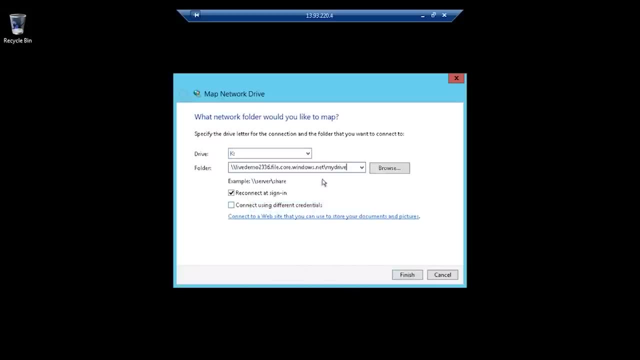 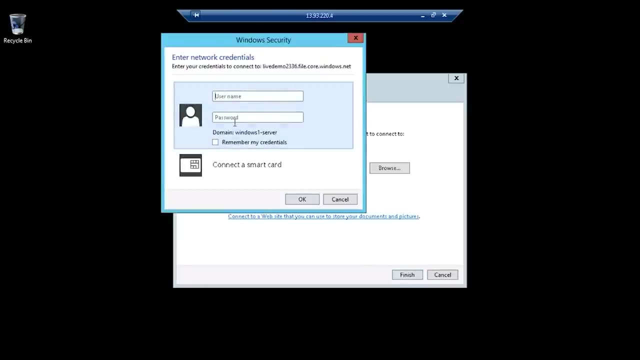 all right, i'll copy the address and i'll save it over here. all right, so it has saved it and now i'll click on finish. so, if everything goes well, guys, it'll ask you for the username and the password now. the username would be this: that is, azure slash. 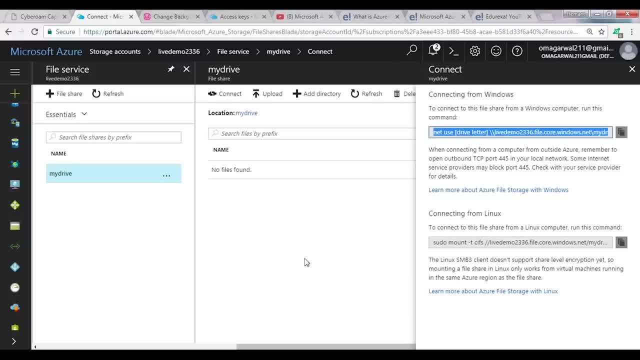 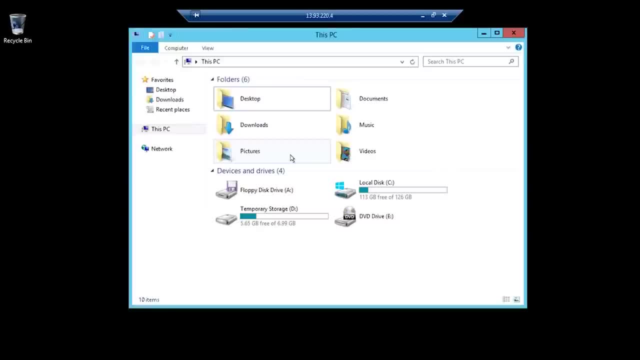 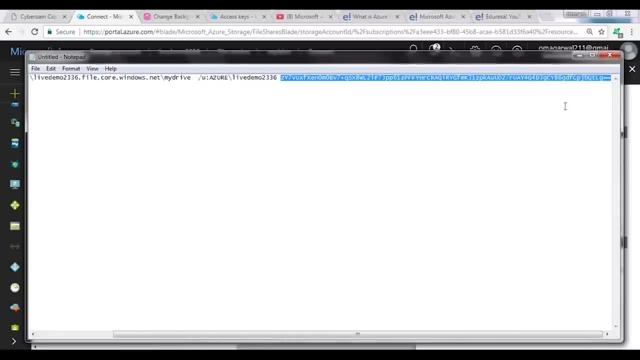 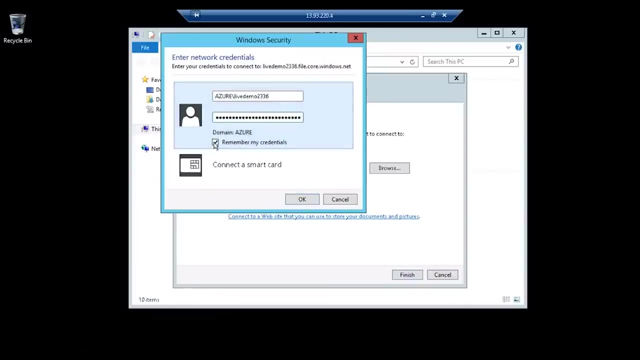 live demo: 2336. right, so i'll go to my server, paste the username here and then it'll ask me the password. so, like i said, the password would be this: your key. so i'll copy the password, i'll paste it here, that is in this particular field, and i'll click on. remember my credentials and click on ok. 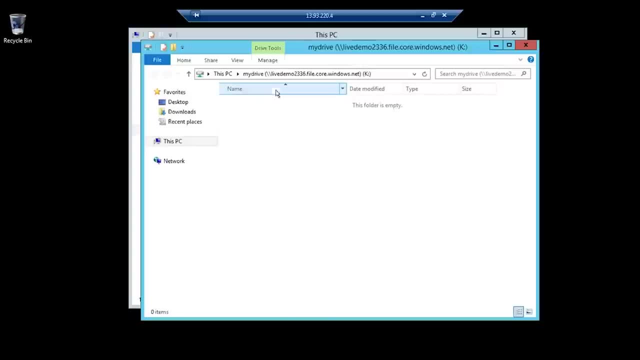 so now, if everything is authenticated, it will go inside my drive. so, as you can see, i am inside my drive right now and if i go to this pc- that is my computer- i can see that a drive has been added over here. now this is my computer and i can see that the drive has been added over here now. this: 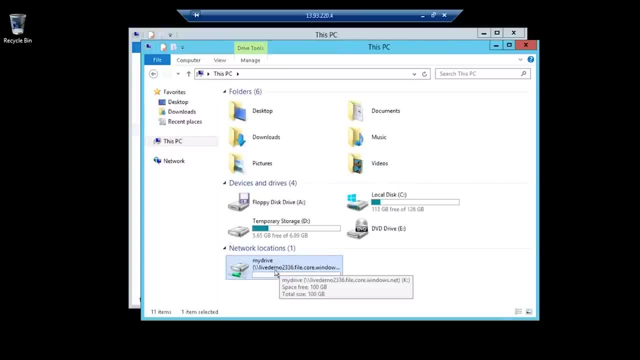 drive. in this drive, as you can see, the total size is 100 gb and the space free is 100 gb, so this is the quota that we assigned in file share while creating it. right now, if i want to copy any file over here, i can easily do that. i'll just copy this particular file and paste it here, right so? 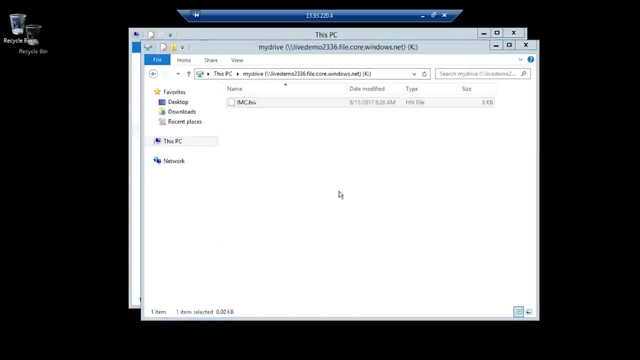 it will easily copy it and say: i want to. i want a shortcut to be copied here. i can shortcut copy the shortcut as well, because i don't have any files on this particular server that i can show out that i can copy it over on my dashboard, right? so, um, i don't have saved any text inside this csv. 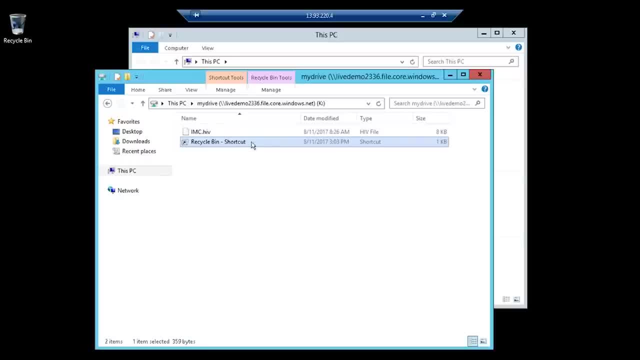 page at this point because i have refused to show any parts of the Librefilter that are up here currently here. so, as you can see, the files have been copied here and these actually have been uploaded to the azure account as well. right, so let me show you on the dashboard if these files are visible. 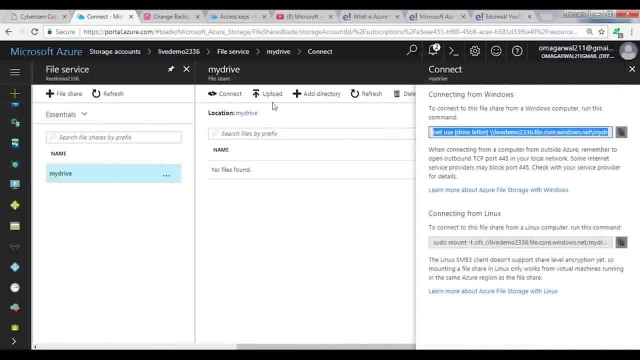 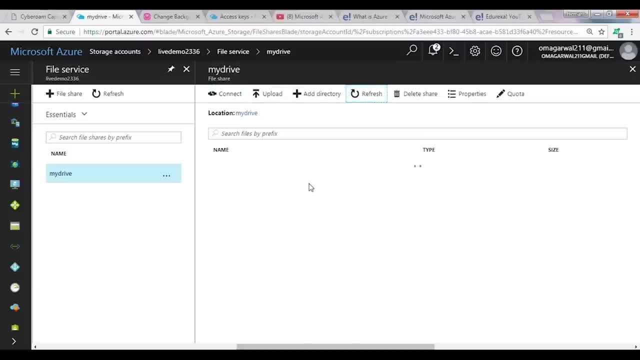 so i'll go to the azure dashboard and this is my drive if i refresh it right now. refresh so it will list me all the files that i've just uploaded. all right, so it is taking some time, and so, basically, when you uh create a network drive in your own computer, it is as if you're using your. 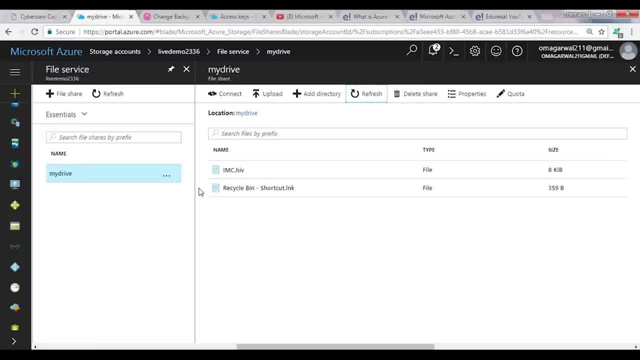 own driver on your local computer if your internet network is good, right? so, as you can see, we have added these two files in our directory in the server and you can view it here as well and you can download it from here. you can click on it, you can download it and anyone can down. 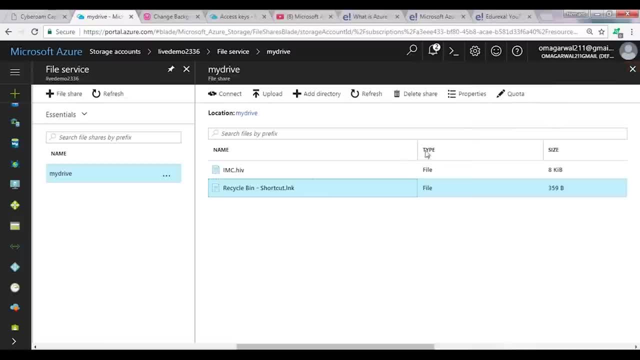 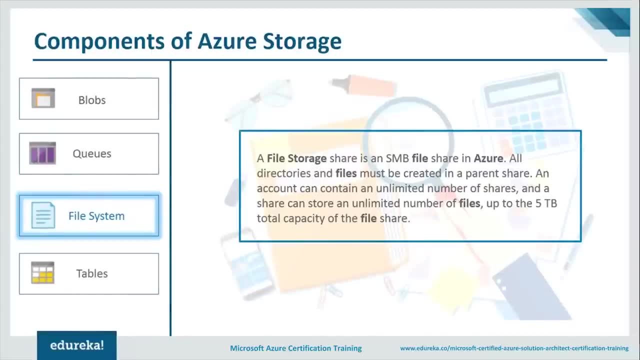 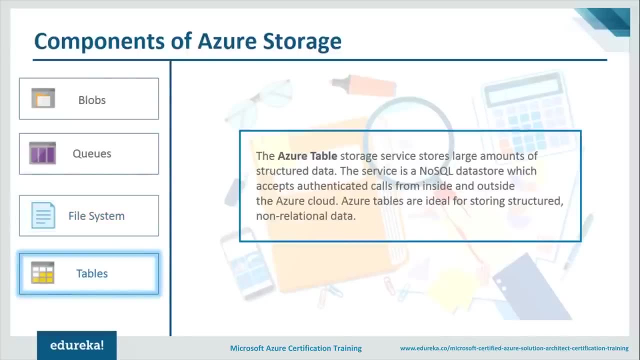 down it if they have the link, all right. so we are done with file system. let us come back to a slide and discuss our last component of today, which is tables. now, tables is again an amazing service from azure, so it is just like no sql, but it is basically you can say, a child of no sql. you cannot. 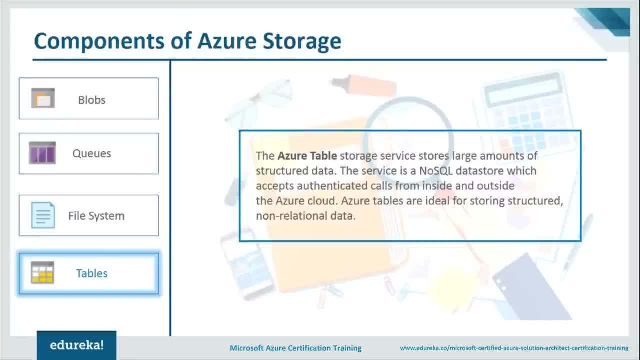 do complex queries on it. now, the way or the advantage of using tables is that, say, you have a data in which the structure is changing dynamically. what i mean by that is, say, you are enter, you have a form, you have created a website in which it accepts three things: it accepts your name. it accepts your. 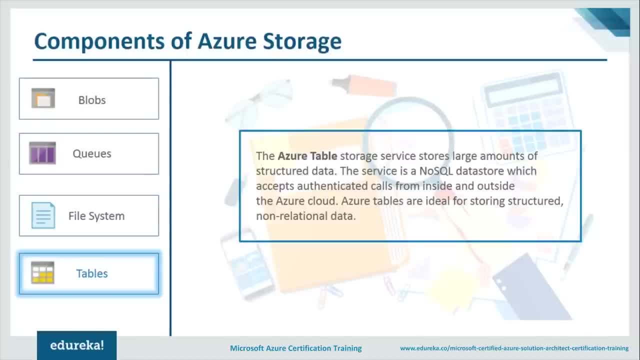 mobile number and it accepts your location. all right. so once it does that, it will upload it in the database, right, normal as usual. but what if, tomorrow, i a use case comes in wherein i want to add one more field, which maybe is asking for your credit card number, right, so? 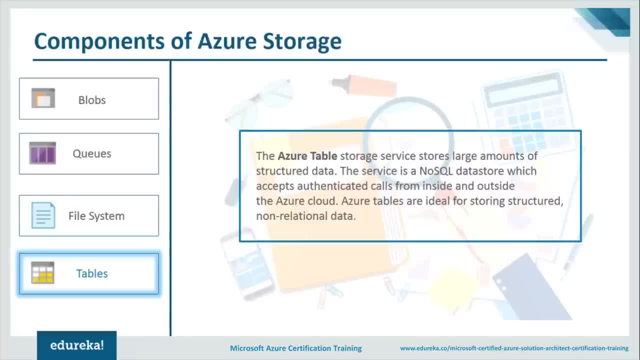 if it is asking that if you were using traditional systems, you would have to go to your database and add one more column and then go on to change your user interface and your php or whatever scripting language you're using, but with tables the thing is that you don't have to change anything in the 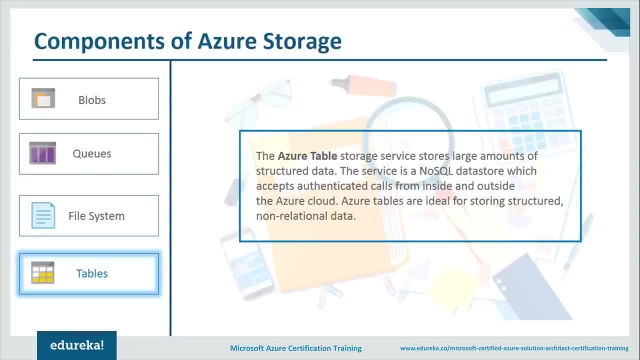 back end, as in, you don't have to change anything in your database. it'll. it'll automatically adjust according to your data and create one more field which is uh, basically, which is basically you're trying to ingest. for example, in our case, we are trying to ingest the credit card number as well. so 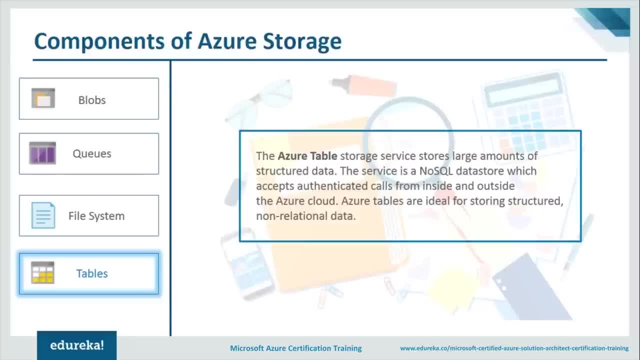 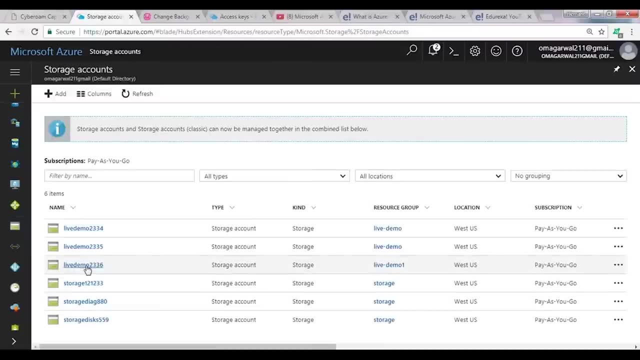 it will do that automatically. so let me show you, uh, how you can use the table service. so we'll come back to our dashboard and go to storage accounts right and again in in your storage account. you'll have all the services listed, so we will select tables. we'll go inside tables. 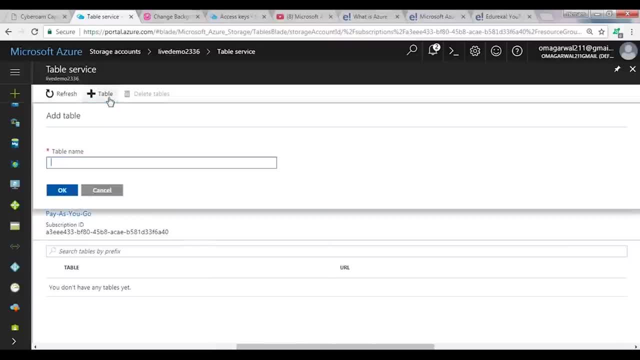 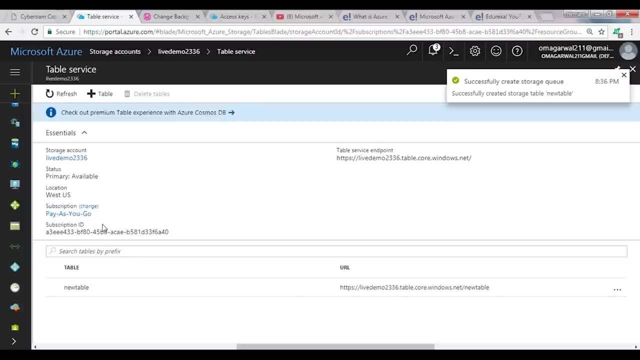 right, and once we are inside tables, we'll have to create a new table. so let's name this table as say, um new table, right, and we'll click on ok, so my table has now been created. all right, now the way you can upload your data to this table. 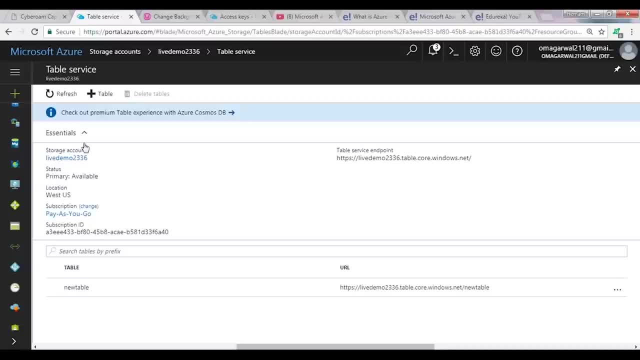 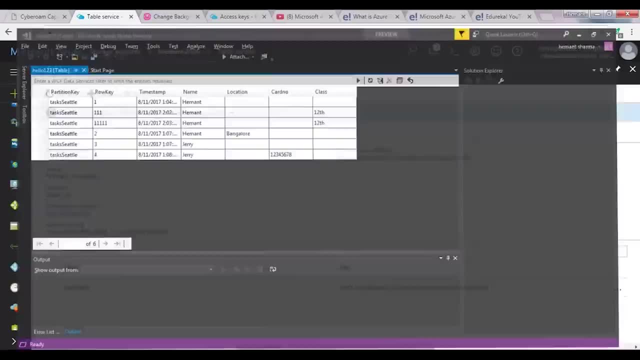 is the same. you just copy the connection string, you call the api and you can upload your data. but to view the data in the table, you will need your visual studio. all right, so let me, for this is a one table that i can use to create a new table. so let's go ahead and create a new table. 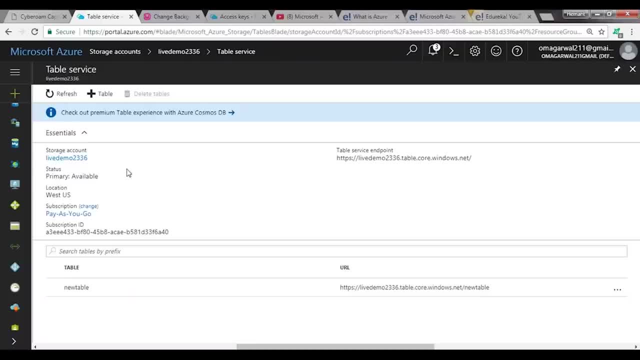 so let's go ahead and create a new table. so for adding it, i'll show you how to add it, but first let me add some values inside this particular table. that is my new table, right? so there is nothing inside it because i just created it. so, uh, what i'll be doing is i will be going 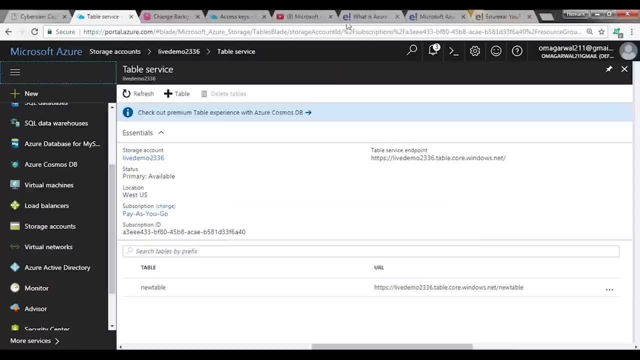 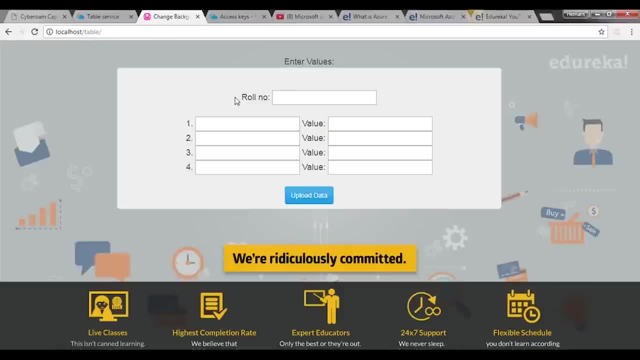 i'll be showing you the website through which i'll be uploading the data into the table. so it is this. so this is my website, using which i'll be updating the table right now. the way i'll be doing it is i'll be first changing the connection string, so the 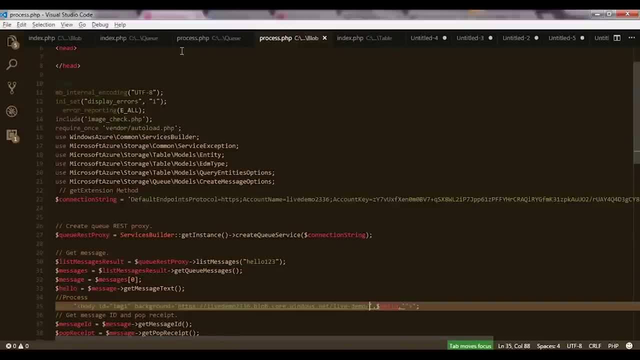 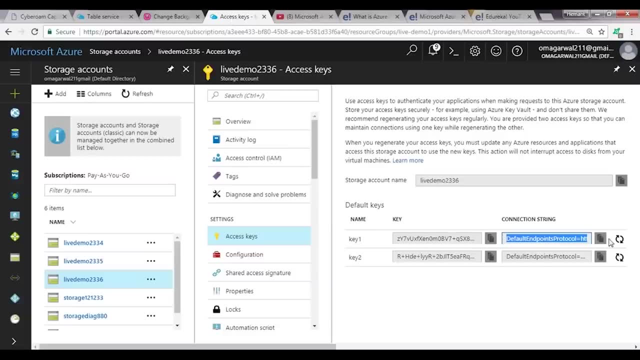 connection string can be found here. right, i'll have to change this. uh, this is my connection code for table, so i'll have to change the default connection string. so let us quickly change it. this is my connection string. i'll come back to my code. paste it here. 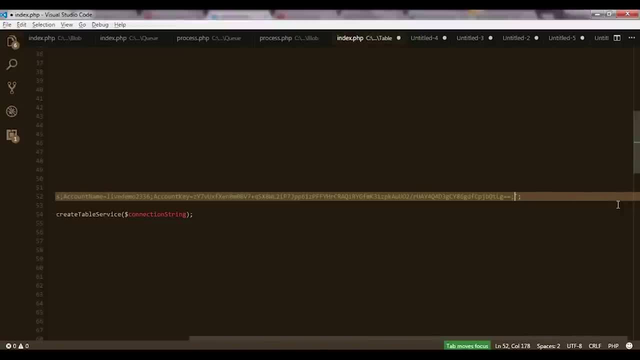 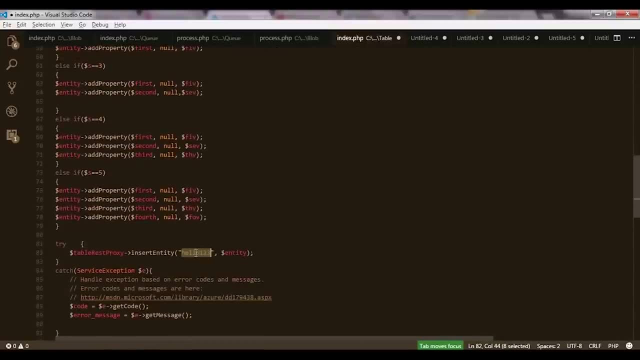 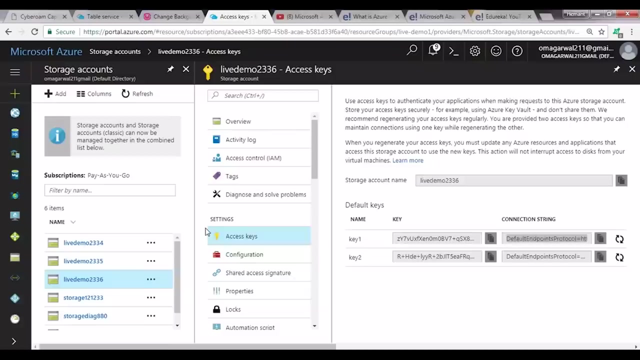 right and remove the endpoint. cool, so my connection string has been given. now i have to change the table name as well. so my table name is new table. right and all right, so nothing else has to be changed. cool, so our code is done. now i'll come back to my slide. 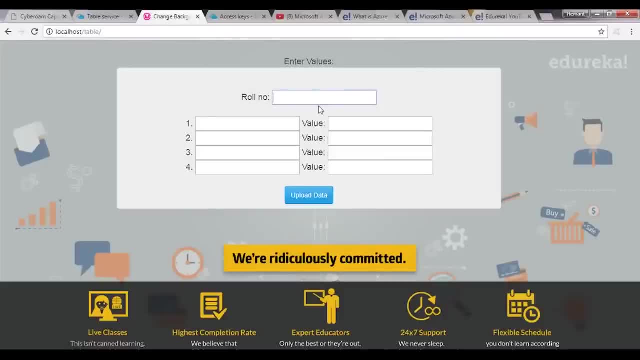 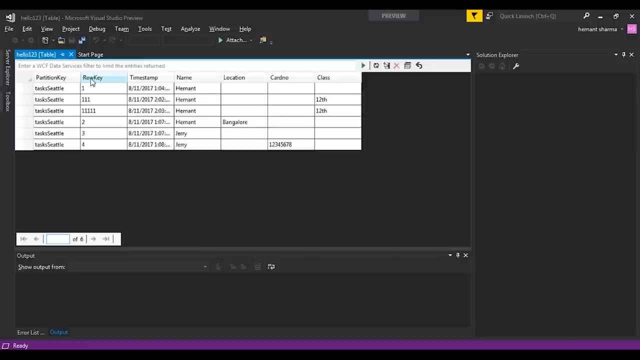 and refresh it. all right. so now, uh, there are two things that you have to understand that are there in a table. one is called the partition key and one is called the row key. all right, so what is partition key? what is row key? let me explain you. so, uh, whatever, uh files that you're. 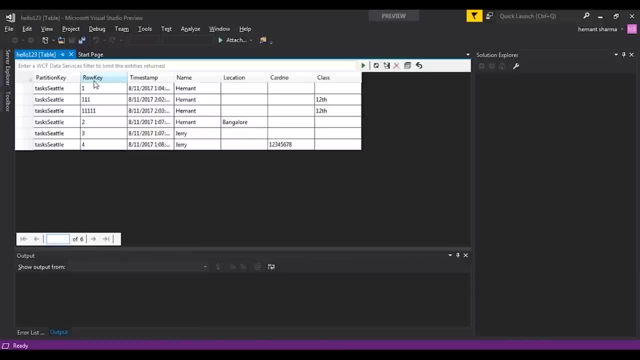 trying to store in your table are stored in different nodes. when i say nodes, there are basically different servers. all right, now each server will have a partition key which can identify it. so say, there is server one, server two, server three and server four. all right, so i want. 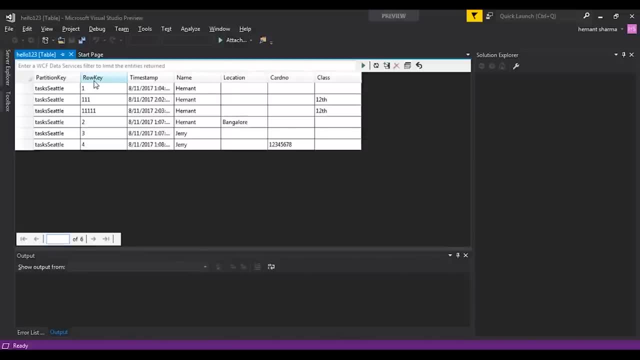 to store my data in server one, all right, so my particular type of data that i want to store in server one, so for that the partition could be key- would be one: all right, now, inside my server, every row has to be identified by a unique identifier and therein comes in the row key. so this row key should be unique to each and. 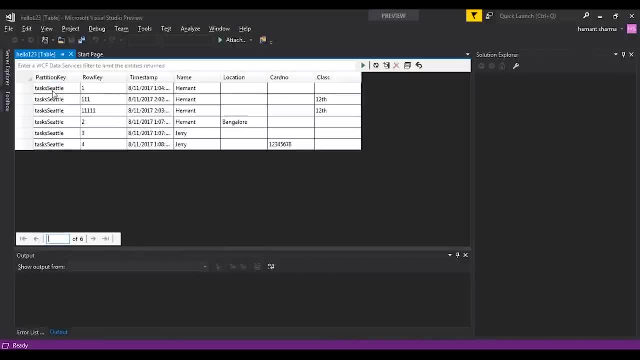 every record that you will be putting inside a partition key table that is inside that particular server. if you change the server again, the row key can be same as that of the previous server, but when you're you are creating records inside, uh, one particular partition key, the rows. 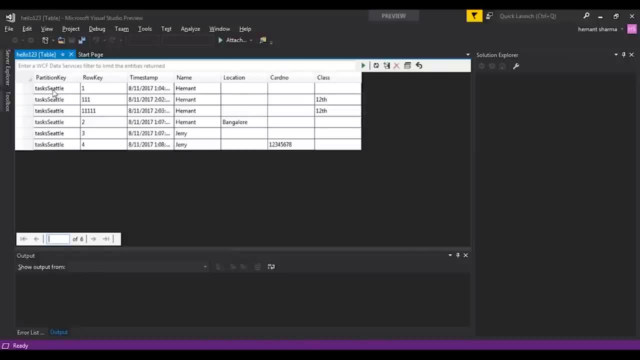 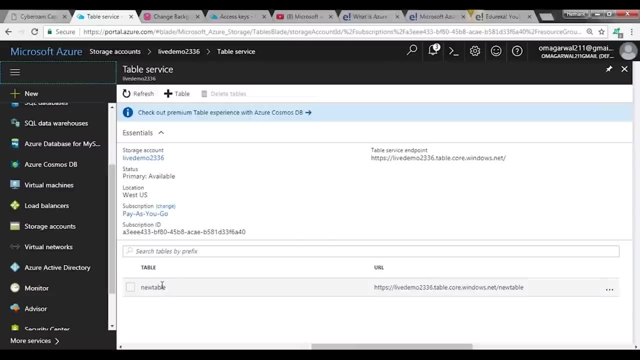 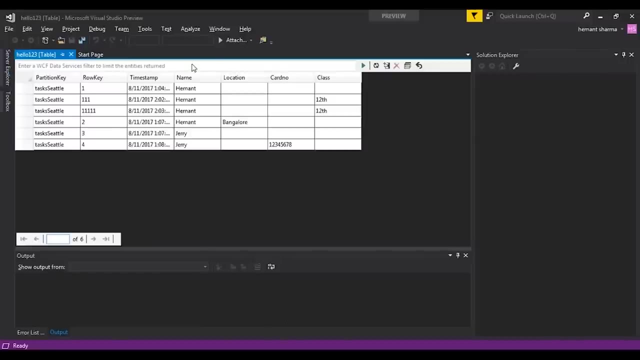 should be different. all right, having said that, guys, uh, so we have uh this website and we have created our new table over here. all right, now what i'll be doing is i will be mapping this new table in my visual studio now. the way to do that is open your visual studio, go to server explorer and uh. 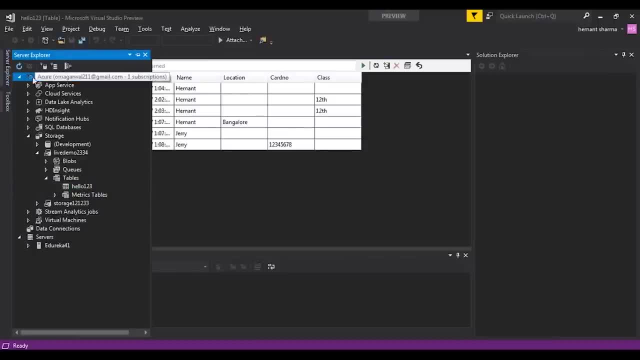 once you have uh you, you'll be listed your azure service over here. all right, now i'll have to map my particular storage account on this uh visual studio as well. so the way to do that is in the storage section, click right, click it and click on attach external storage. all right, so once that is done, it will ask me the account name and 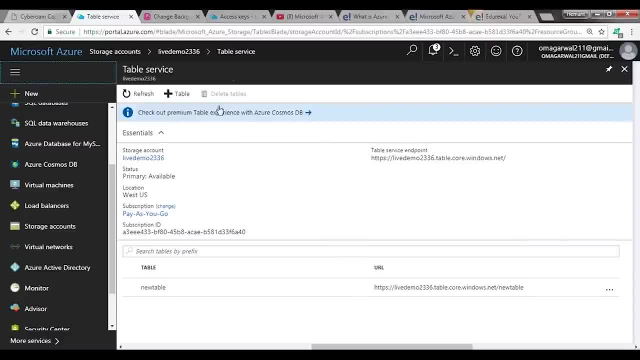 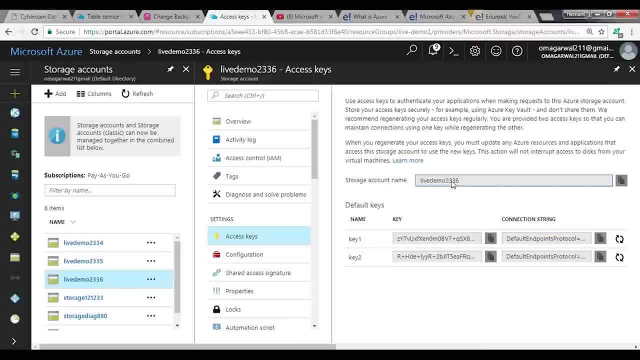 the account key. now the way to attach. it is like this that you will go to the table service: uh, sorry, your storage account. you will copy the name, paste in the account name and then your connection string, sorry, your key, right, right. and in this case you will be copying the key and you have to paste the key here. 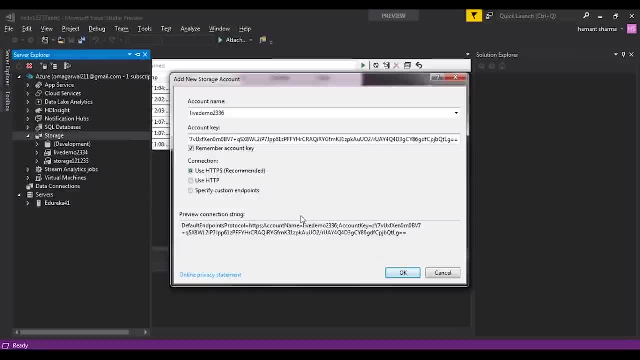 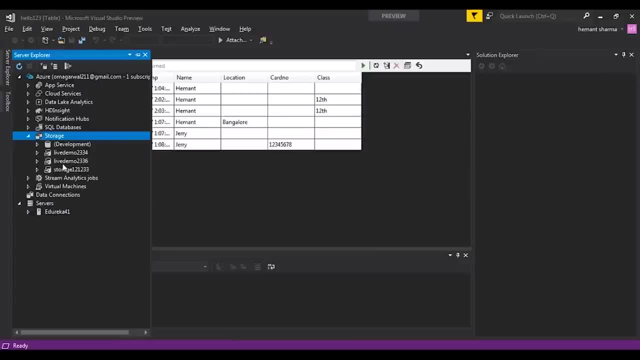 remember the account key so that you don't have to enter it again and again and click on ok, so this will add your storage account over here, right? so this is my storage account, live demo 2336. right? so my storage account has now been added and inside it i have created a table. 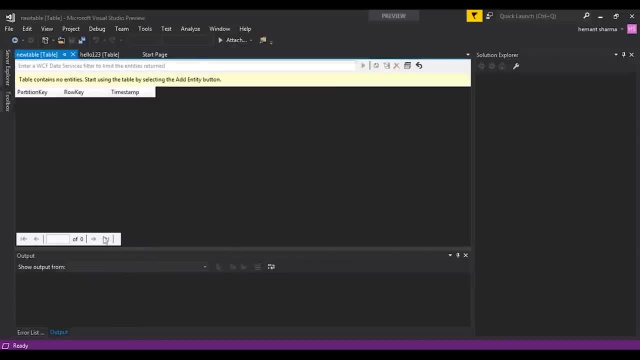 called the new table, all right. so if i click on the new table, i've called it new table, all right. so if i click on the new table, i have got a new table. right now you can see there is nothing that has been added as of now. so what i'll do is uh from my website. 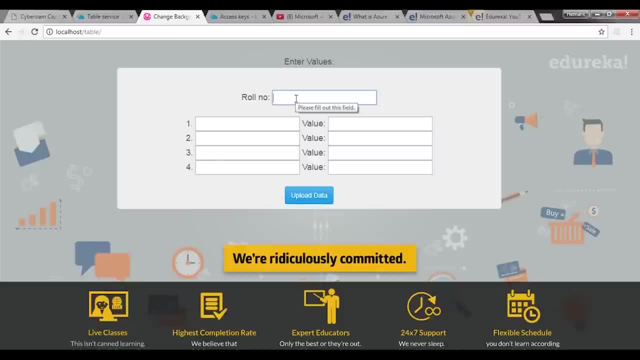 now i'll add a new value. so i've already specified the partition key. as default, it is called task seattle. right, all i'll be doing is i'll be entering the name over here, entering the row key over here, which will be unique. all right, so as as of now, there are no records, so i'll enter one. 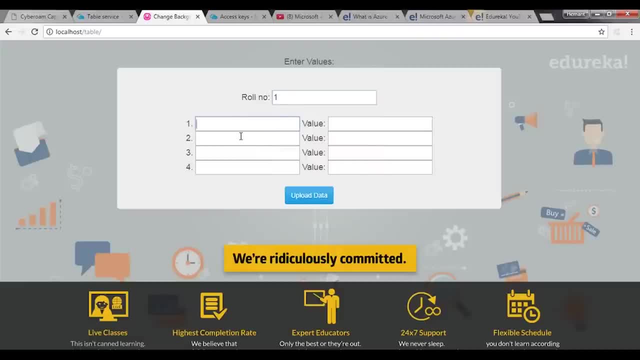 as my, uh, as my row key, and now i'll enter the columns that i want. so this row, this particular row, is the number, is the columns and this is the values that that i want for that particular column. so for that i, for example, i want the name column to be there, right inside the name column. i want. 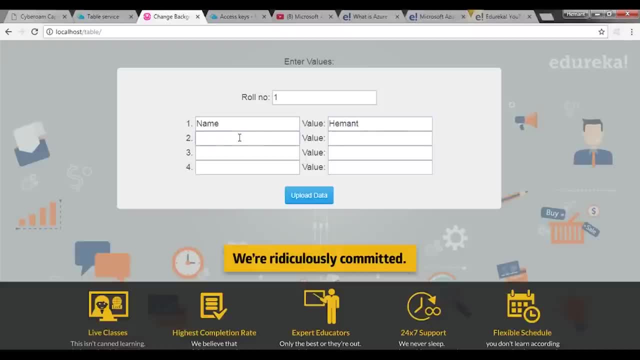 the name hey month. all right, i'll specify that and say i want, uh, my mobile number to be there. i'll specify mobile, i know right, and i'll specify the mobile number here. that is one, two, three, four, five, six, seven, eight, nine, say. and now i'll click on upload data, so this will upload the data to the. 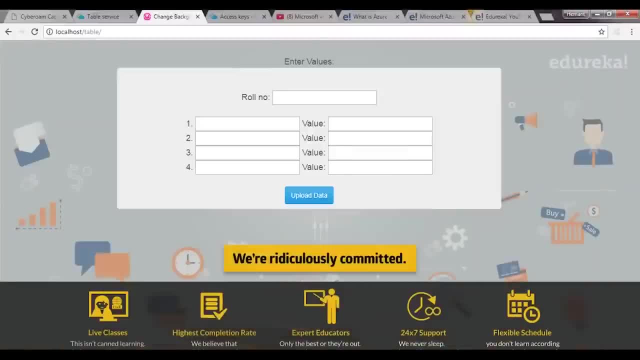 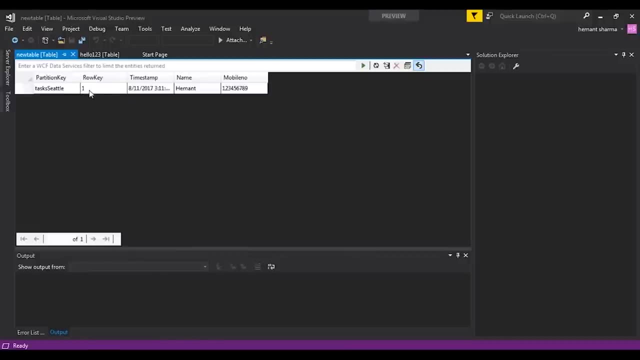 table i've just created. so if i go here, go back to my visual studio and i refresh it, i'll be able to see that a new record has been entered in which the row key is one right, the name is hemant and the mobile number is this: now, say, i want to add one more field, which is asking for my credit card. 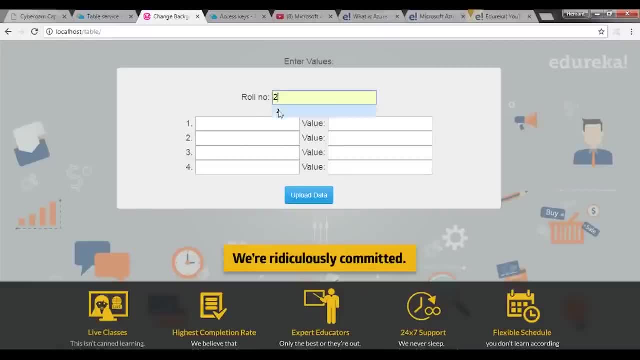 number. all right. so, as i said, the row key would be different. now i'll enter the name. so whatever column you have already specified, it will go inside the same column. so i have already specified name, right? so if i enter the value hemant here, it will not create a new column and enter the value. 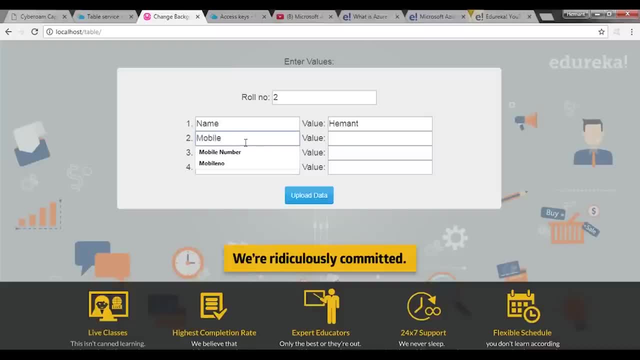 hemant over there. it will just create then column which is new to the data. all right, so the mobile number is again, say, five, six, seven, eight, and. and now it will ask me for my credit card number. right, so the credit card number could be this: all right, so now, if i upload the data, 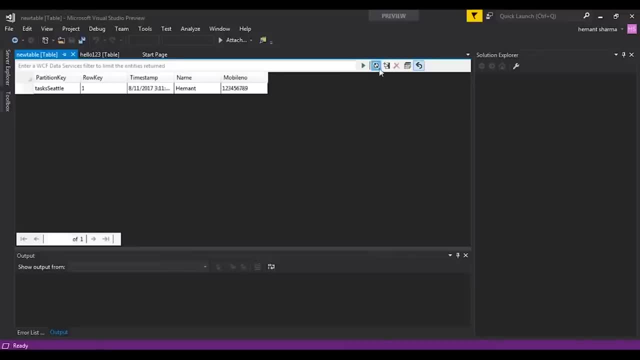 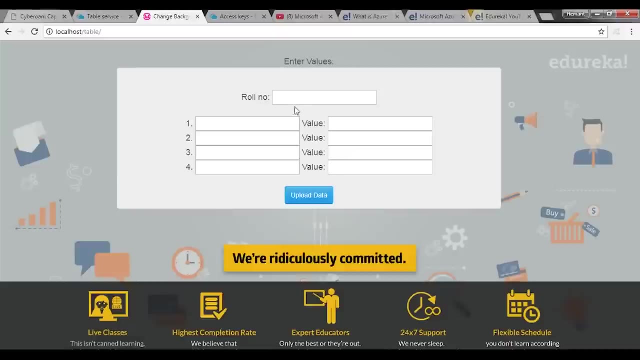 and i'll show you how it looks now. so, as you can see, now the credit card number of field has been added. so the for the first record there is nothing there in the credit card number field, but in the second record i have added that i want this data. all right, also, guys. um, you can specify. 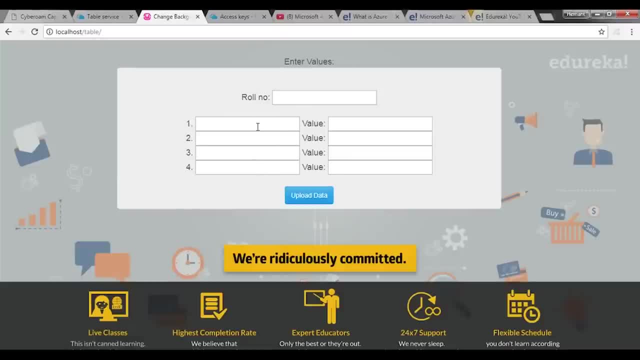 in any order. there is no specific order that you have to specify right, so i can enter the name for first right and then i can enter the credit card number, say this is the credit card number that i want to add right, and say i'm entering the mobile here. 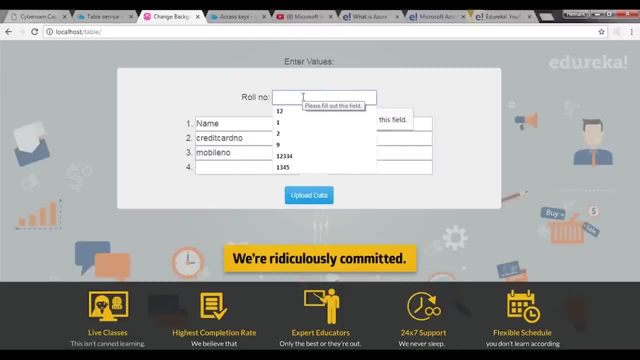 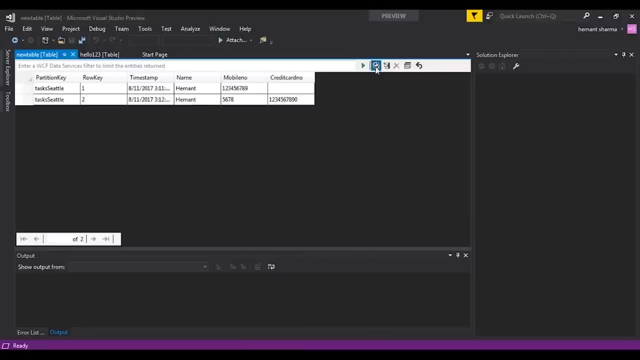 right if i upload the data now. so this is required. sorry, three upload data will be updated and if i refresh it now, you can see that uh. okay, so m capital and i'm small. you have to be careful of the uh, of the indentation, of the uh, sorry, your syntax as well. so whatever. 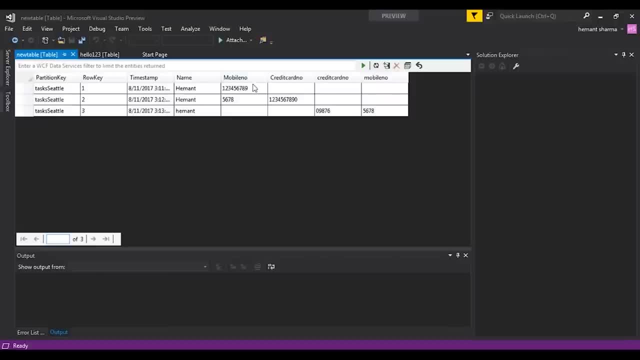 column names you're specifying. it is case sensitive. so, like you can see, i made a mistake here by specifying a small c and it created one more column. all right, but, as you can can see, the name is in the same column now. all right. so what? in in whatever, sorry, in whatever. 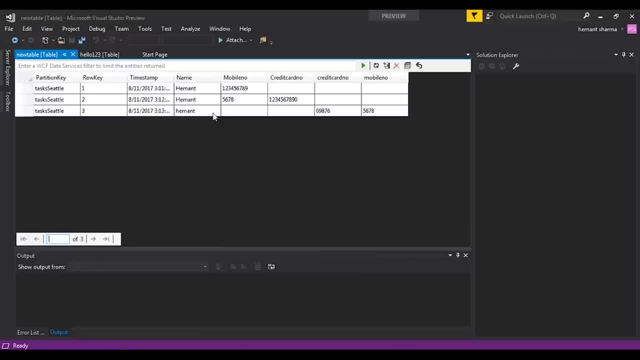 sequence. you can add your record and that record will be added automatically in its respective column. all right, so this is how tables can be used. all right, guys. so with that, i think we are done with our services. so we discussed what are blobs. we discussed what are queues. we discussed 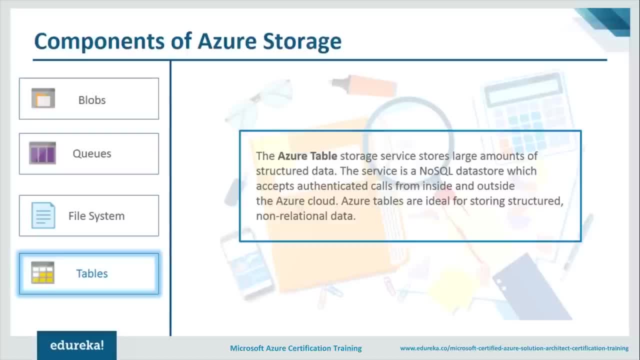 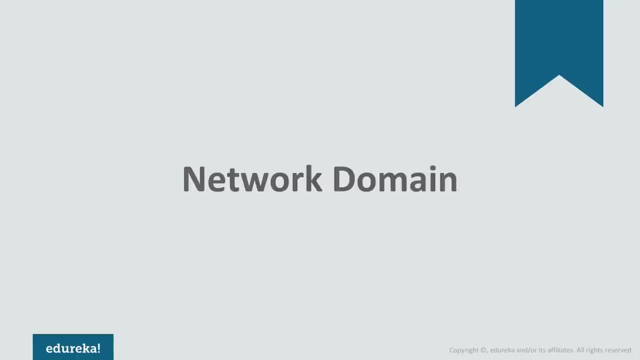 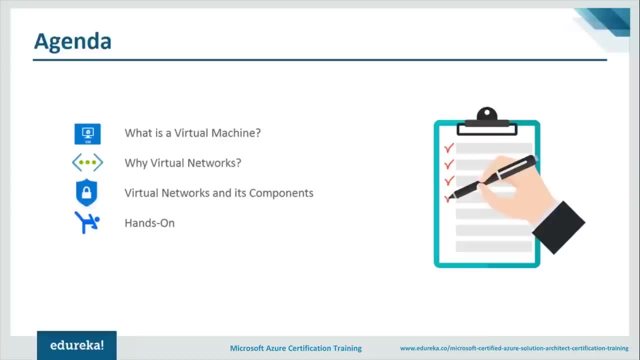 what are file systems? we discussed what are tables, and for each of the service we saw how we can use them in azure and how we can deploy them as well. all right, so let's go ahead and see what all we are going to learn in just today's session. so today, in this session. first, we'll start off with 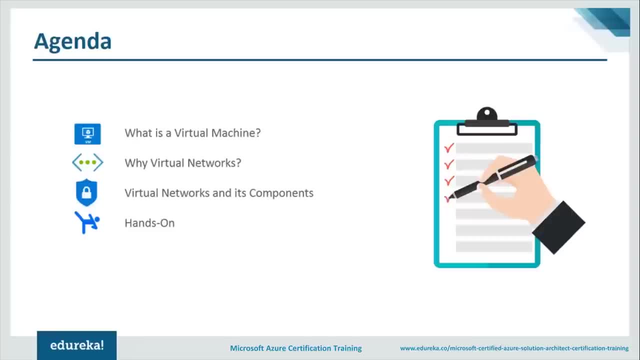 what is a virtual machine? right, we're going to understand what is a virtual machine, how we can configure it, how we can launch it in azure. once we have done that, we'll move on to virtual network. so before understanding what is a virtual network, we'll first understand why do we actually need a? 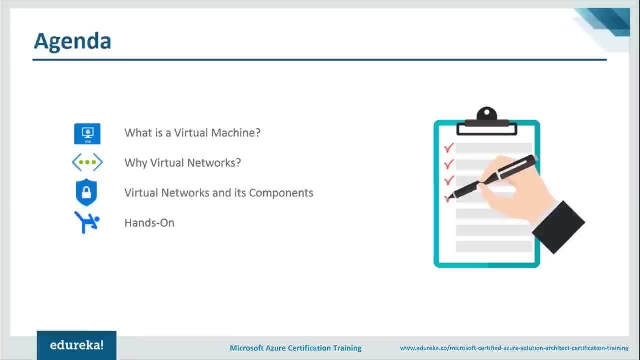 virtual network right. once that is done, we'll move on and see what is a virtual network exactly and its components right, and towards the end we'll be doing a demo wherein, like i said, we'll be deploying two servers which we'll be configuring from scratch, that is, a web server and a database server- right, and we'll 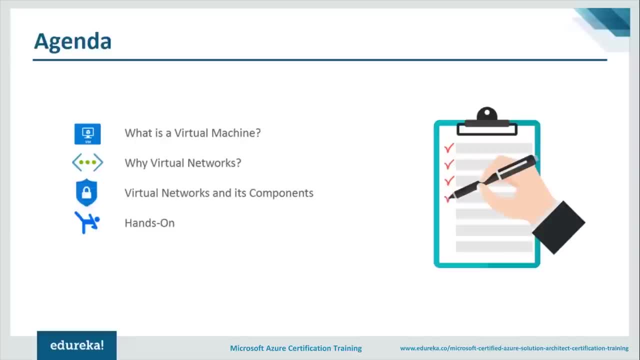 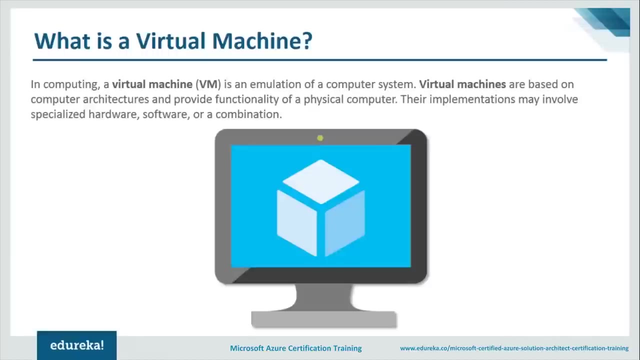 be deploying them in virtual networks and configuring their properties, right? so, guys, i hope this agenda is clear to you. let's move ahead and start off with the first session, which is: what is a virtual machine? right? so what is a virtual machine? so, a virtual machine is basically a raw. 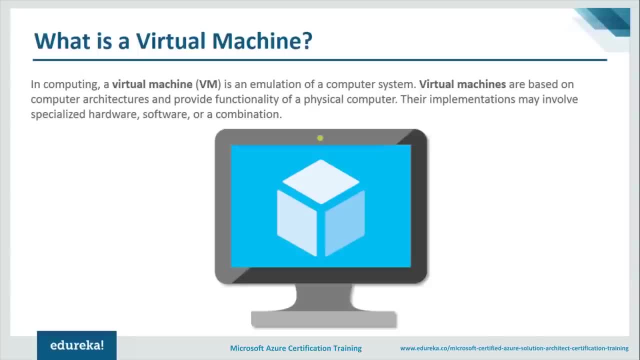 server that you get from your cloud provider. that raw server could, could- be an ubuntu machine. it could be a windows machine, right? so it's basically just like your own personal computer. rather than purchasing it, you're renting it out on cloud, right? when you're renting it out on cloud now, it is the 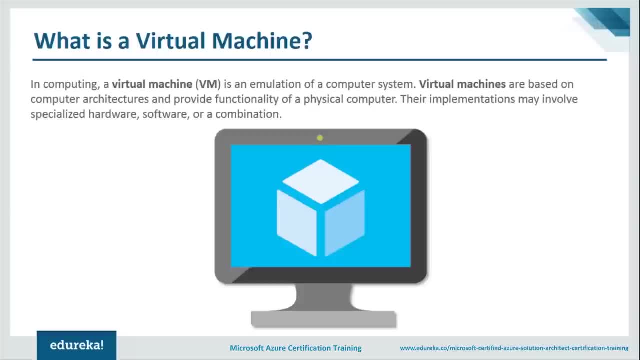 same as if it was you on your own computer, right? so it's a fresh piece of operating system. you can install office as you want. you can want it to be, make it to be a web server. you can make it to be a, a worker tier environment. you can configure it to be anything right? so today we are going to make it. 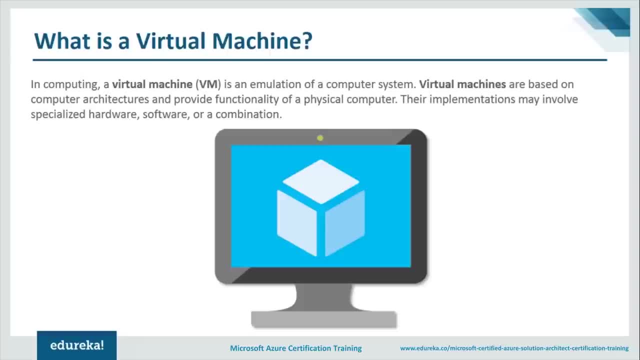 a web server and a database server. moving on, guys. so this is what virtual machine is all about. and also, if you compare it with aws, which is also a popular cloud computing service, with in aws, this, this same service, is called ec2. all right, in azure it's called virtual machine. in aws it is called ec2. 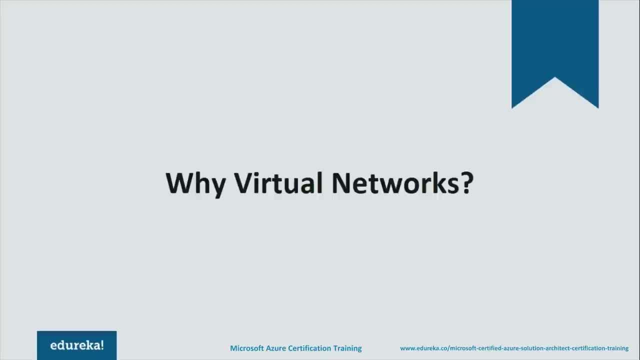 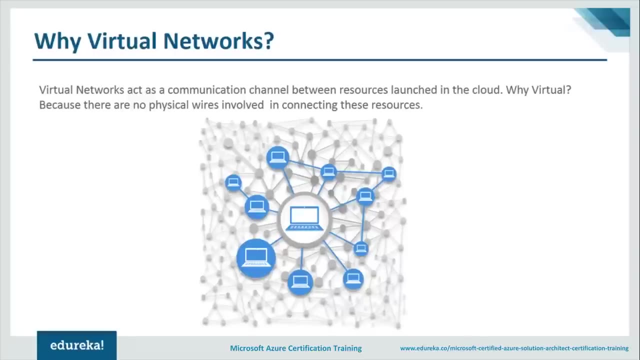 all right, moving ahead, guys. now let's start with virtual networks and first understand why do we actually need virtual networks? all right. so, like i said, we have virtual machines. right. so if you say, launch two virtual machines and you want both of them to communicate with each other, for example in: 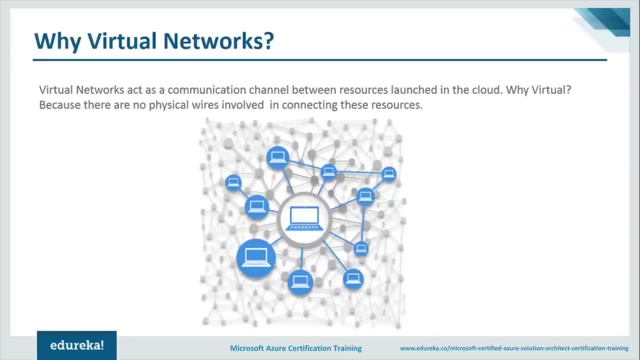 our session today, in our demo session, what we'll be doing is that we'll be deploying a web server and we'll be deploying a database server, and we want the web server to talk to the database server. right. for this, for this communication, we need a channel and hence we need a network. right, but why virtual networks? so, if you guys, 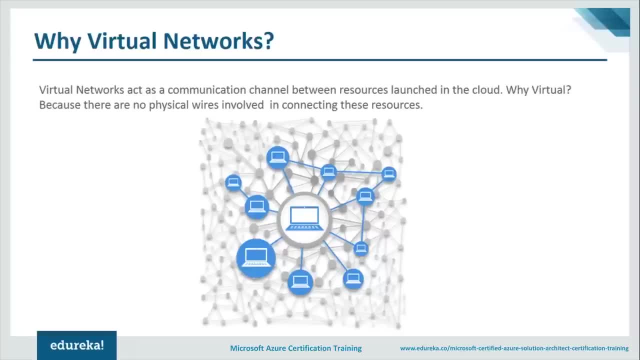 would have noticed, in cloud there is no. there, there are no wires, there are, there are no switches, there are no routers. all right, so your virtual machine is connected using a logical connection. right, it is logic. these two servers are logically isolated and that is why we call it virtual right. 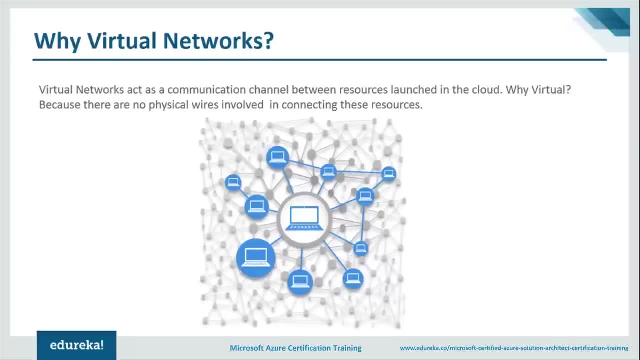 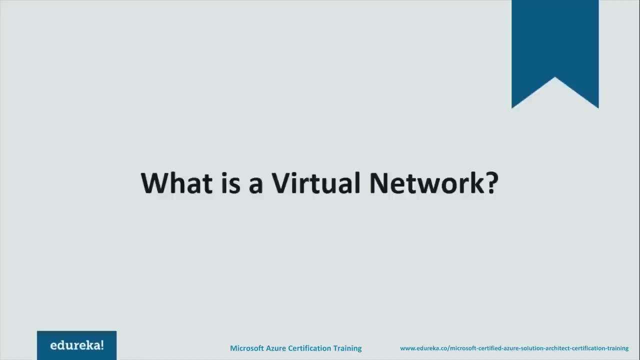 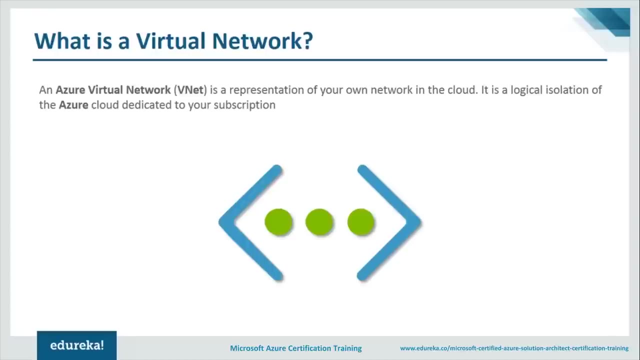 so this is so. we understood that for the communication scale, uh sake, we need a virtual network. let's now understand what a virtual network exactly is. right, so a virtual network is just like a representation of your network, but on the cloud. right, for, for example, we launched a server on the cloud and we connect to a virtual network. 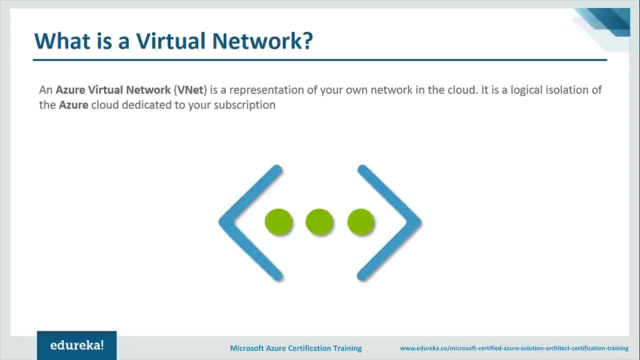 right. when we connect to our virtual network. that is on azure, our network will include that server as if it's on our own network. that is on on-premise right. that is what a virtual network is. that is what a virtual network is right. your server will be on the cloud, but your company or your company's- 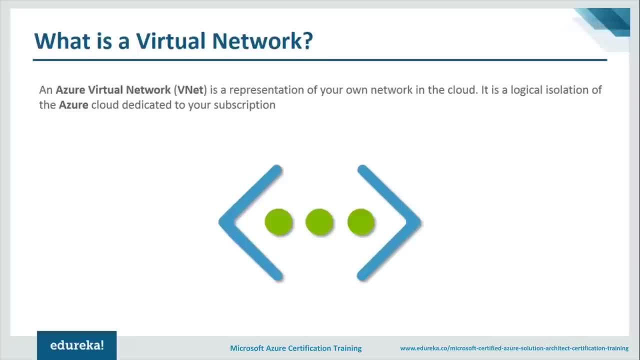 network will feel as if the server is on your own network, right? um? and it, like i said, it's a logical isolation of the azure cloud dedicated to your subscription. that is, uh, whatever, uh resources that you have launched in the cloud. it logically isolates it from the rest of the resources that 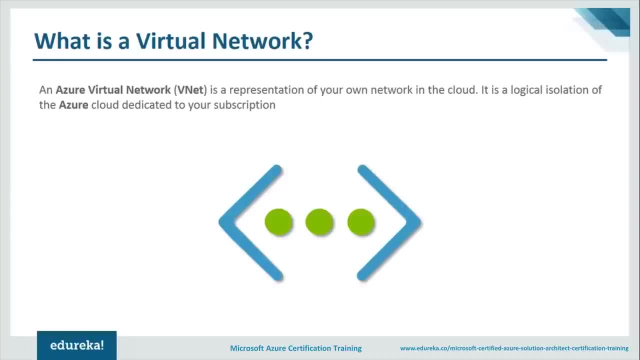 are there on azure that maybe it could be your resources or someone else's resources as well. it are insulated to other resources. it doesn't matter if the other resources are failing or doing anything right. they are all isolated. so this is what a virtual network is all about. now, when we 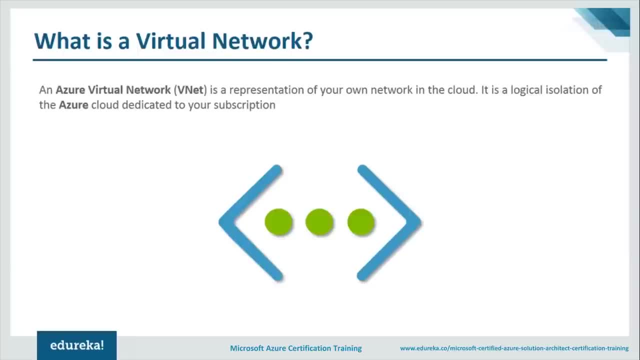 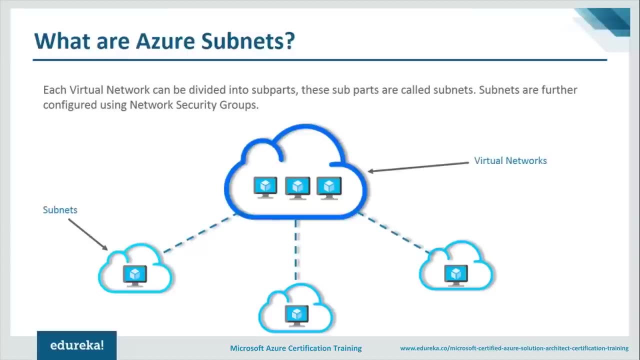 say virtual network. it basically has a lot of components. let's understand these components. so the first component is an azure subnet. now, what is an azure subnet? basically, when you divide a network into subparts, it is called an azure subnet. all right. so when you divide your virtual network, 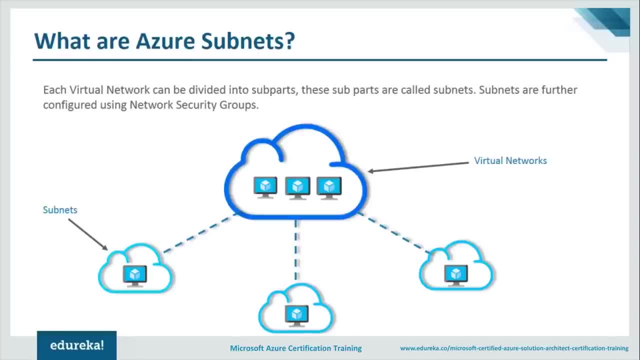 into parts. it's called a subnet. now this subnet can actually be given unique properties. for example, in this same virtual network you have three virtual machines, right? one virtual machine is in one net, one subnet, and the other virtual machine is another subnet. but this subnet you can configure, uh, to be unique. for example, we wanted to, we want to create a public subnet. 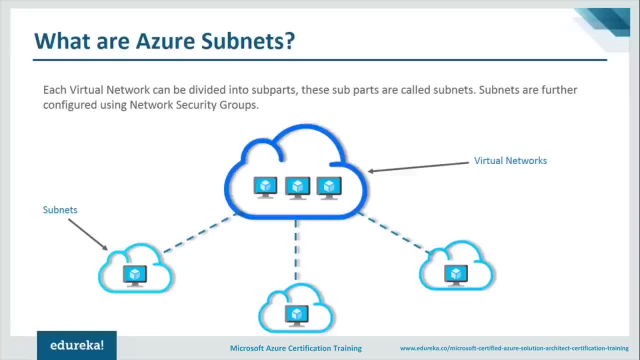 so a public subnet is basically a subnet which has internet access. all right, so we can configure the properties in a way that this particular net, the machines in this particular subnet, will have the internet access and the other particular subnet will not have the internet access. 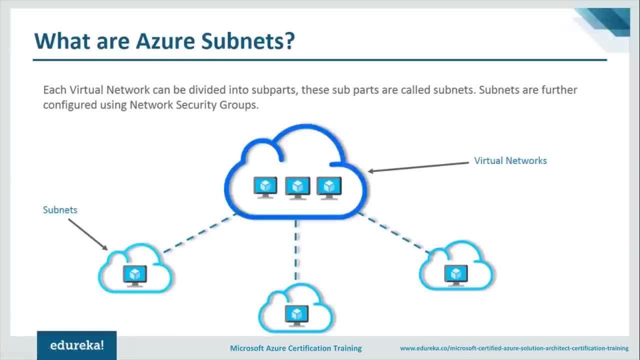 So a subnet which doesn't have the internet access is called a private subnet. So the virtual machine in this particular subnet will not have internet access. but when you actually see it from a broader perspective, all of these servers are on the same network, But because of the subnets, because the properties of subnets, they reflect different properties. 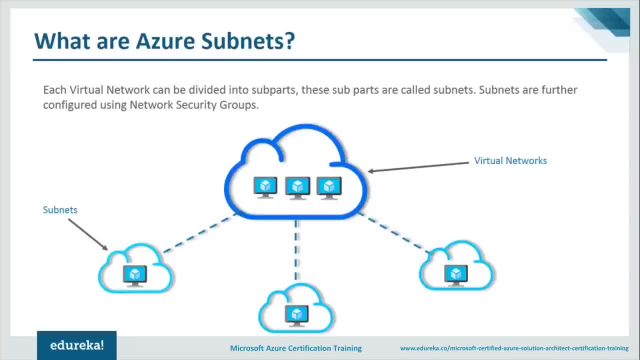 So, being on the same network, they have different properties and using subnets, this is how subnets are actually useful. So this is all you need to know about subnets, guys. Now, with subnets, the properties that I was talking about. say, I want to connect to a 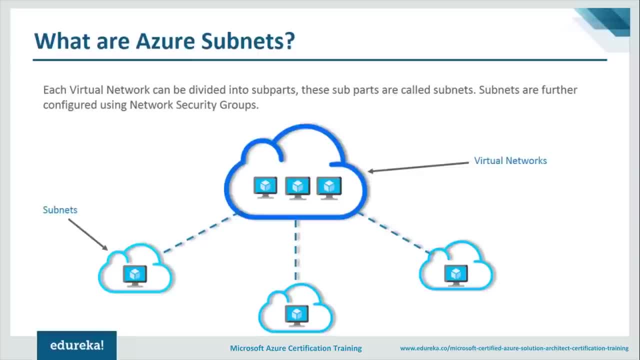 web server. so for connecting to the web server, for accessing that website, I need to go through the HTTP protocol, right? So all of this is configured in a firewall. Now what is that firewall called? That firewall is actually network security groups. 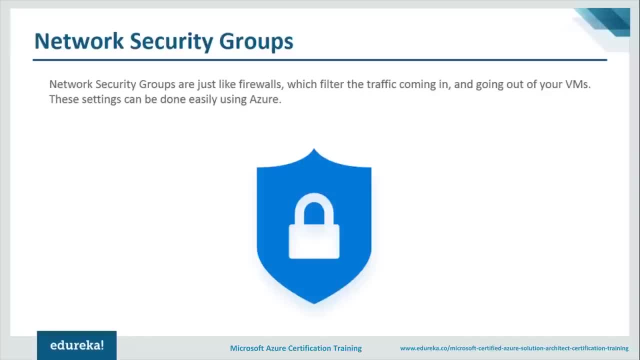 Now, what are network security groups? Like I said, they are just firewalls in which you put in the properties that you want the subnet to reflect. For example, I want to connect to my web server, so I have to allow all HTTP traffic on that. 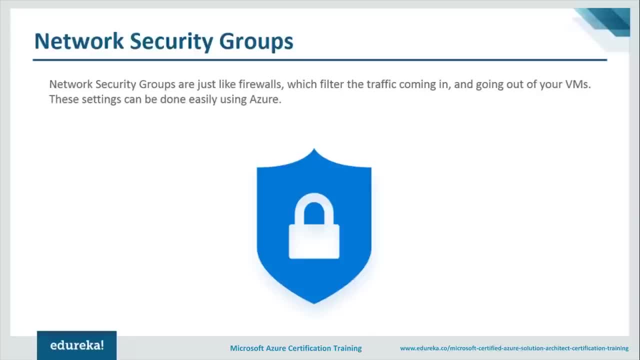 subnet and for that I'll have to attach that particular network security group to that subnet. Now I know it's a lot to take. I just explained it. I gave you three components and you might be thinking which component goes where. right, 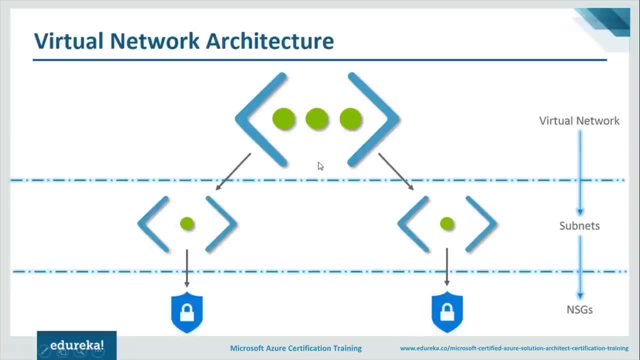 And so I have this diagram. So I'll just summarize what I just explained it to you. So we have this virtual network. In the virtual network we have subnets, and a subnet is attached to a network security group, right. So this network security group is where you will be configuring all the protocols, all. 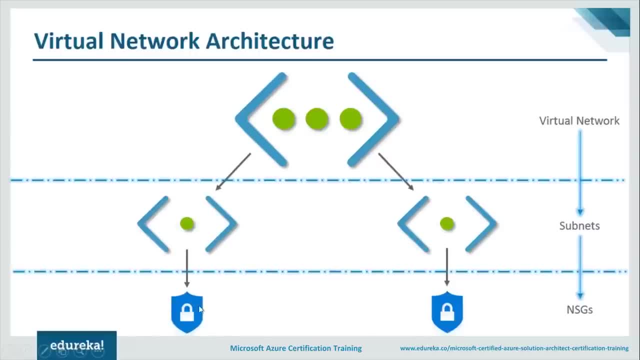 the properties that you want your particular machine to reflect. This firewall will be attached to the subnet in which you'll be deploying your virtual machine, right? So this is a place where you'll be deploying your virtual machine and it will be attached to the subnet. sorry, your network security group. 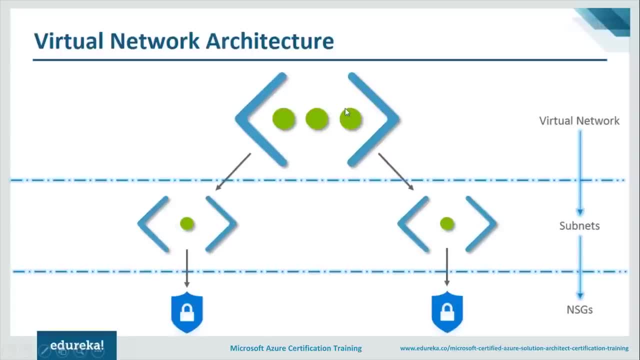 And this subnet is actually included in your virtual network, right? So both these subnets are actually in your virtual network. So one virtual network will have as many subnets as you want, and each subnet will have different properties because of its network security groups. 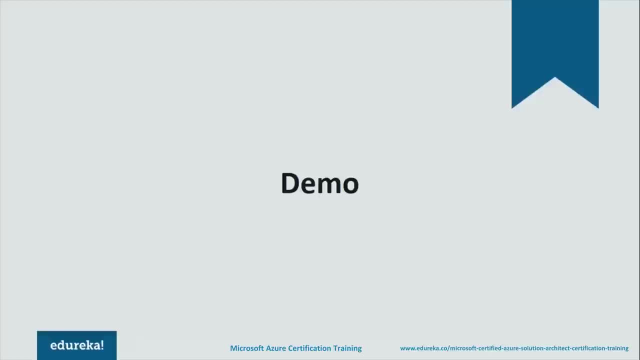 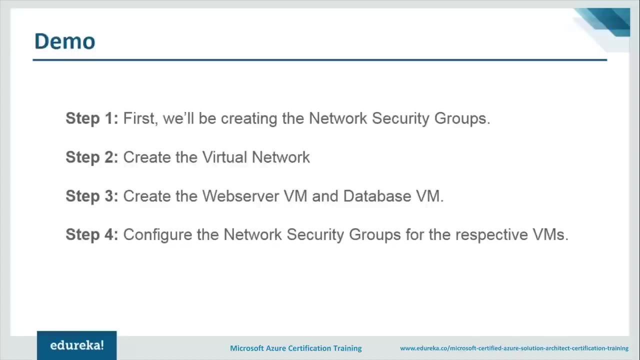 Moving along, guys. now let's so. enough of talks. I have explained to you everything you need to know. Let's go ahead and start with a demo, And for that let's look at the steps that we're going to do. 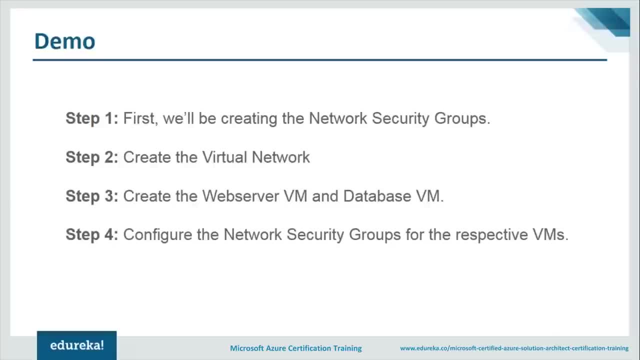 So first we'll be creating a network security group. That is the firewall that is required for our server. So basically, we'll be creating two firewalls: one for our web server and one for our database server. Right, So let's go ahead and do that. 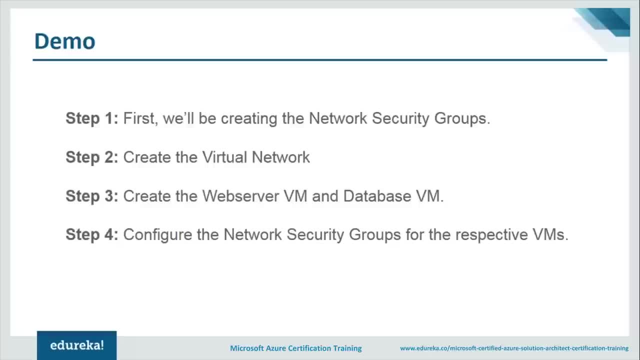 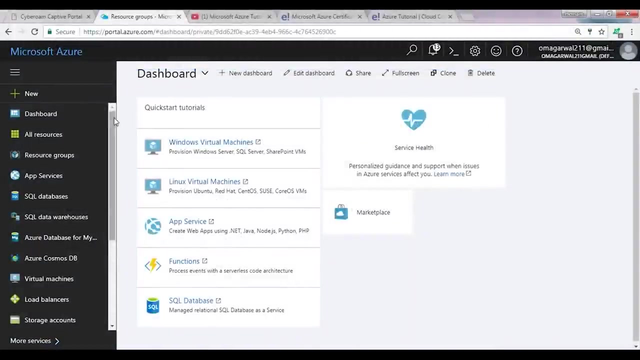 So just give me a second, I'll go to my Azure dashboard. Okay, All right. so, guys, this is how my dashboard actually looks like. Now, on this dashboard, the first job that I have to do is to create a network security. 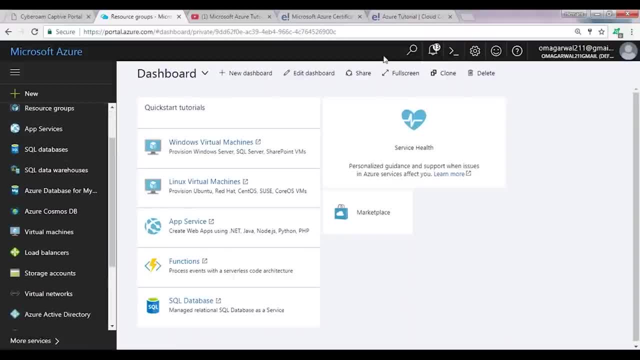 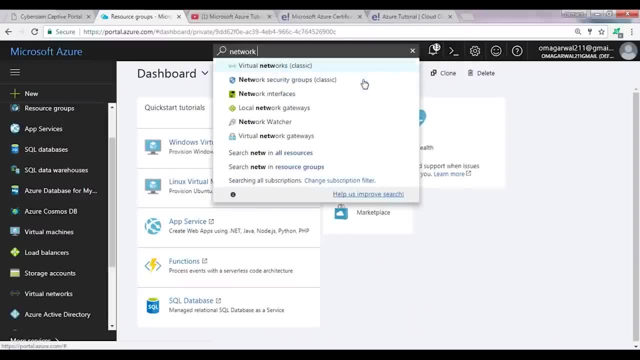 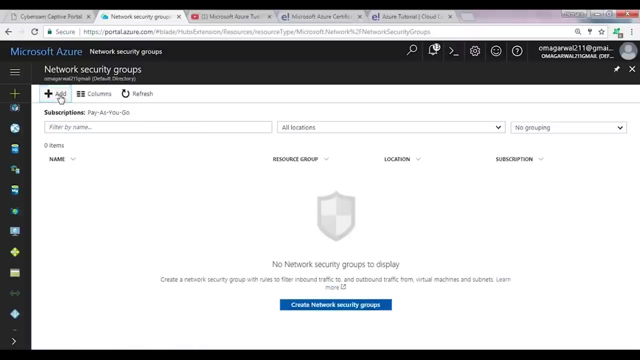 group. So let us do that. Let us go to the search bar and type network security group, Network security groups, right, And once you have done that, you will see it is listed over here. We'll click on it and then we'll click on add. 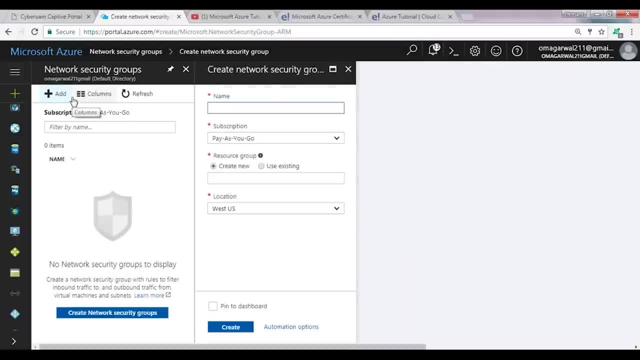 Now, when we click on add, we first have to add the firewall for web server, right? So it is your choice. Either you could deploy the web server first or your database, So you'll type in the name of the network security group. 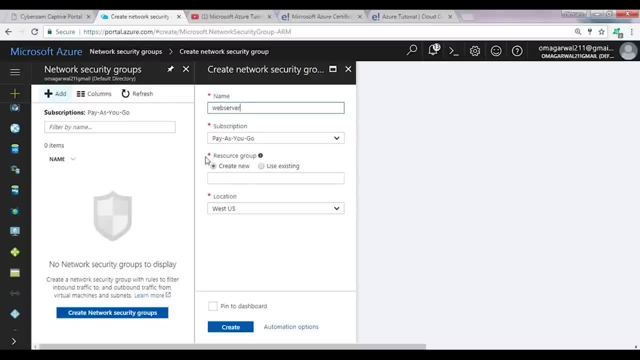 This is for my web server, so I'll type in web server, Then I'll have to assign a resource group. Now, what is a resource group? So basically, like for our use case today, we'll be deploying a lot of resources, right? 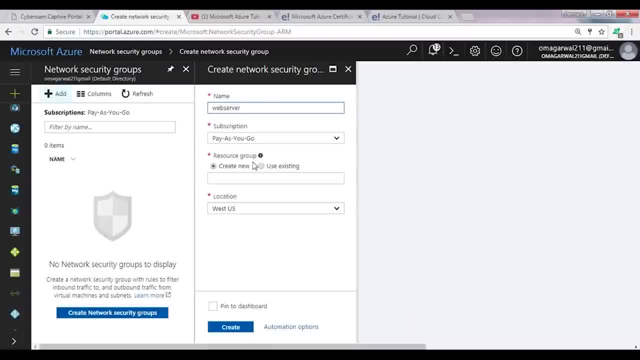 So it becomes easier for us to manage it. if it comes under one group, All right, So we'll be creating that group over here. So, say, I'll name the group as live-demo. All right, So this becomes my resource group And all the resources that I'll be launching today, I will include them in this particular. 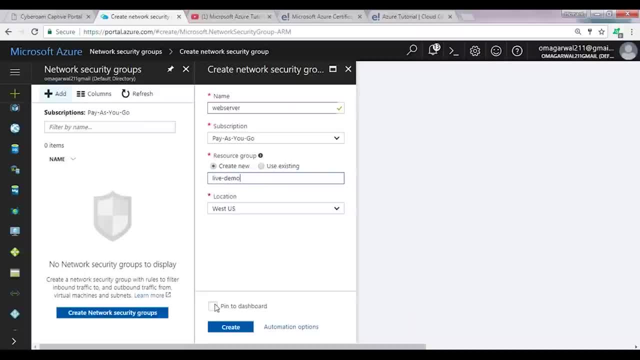 group so that it becomes easier to manage for me. All right, And I'll pin it to dashboard and I'll click on create Now while it is being created. you would have noticed that I've pinned it to dashboard. Now. what is the dashboard, guys? 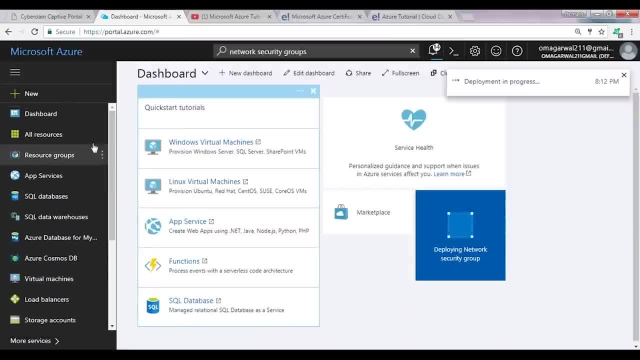 So for those of you who are not acquainted with the Azure dashboard, so dashboard is just like a desktop guys that you have on your computer. So all the shortcuts are created here, Because I would be configuring all the properties. So I'm going to create a dashboard. 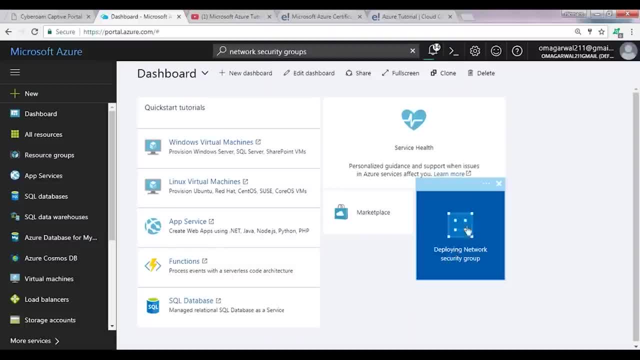 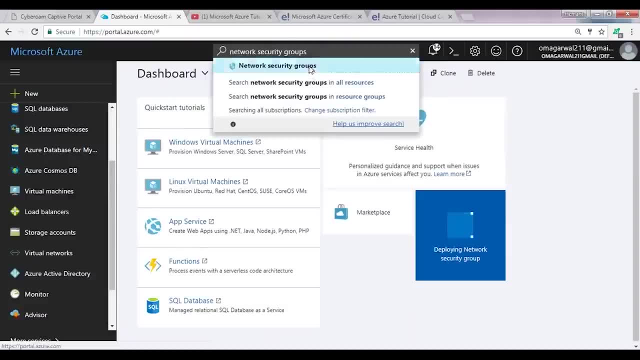 I'm going to create a dashboard, So I want it to be listed here, and that's why I have created a shortcut on the dashboard. All right, So while it is being deployed, let's deploy our second network security group as well. 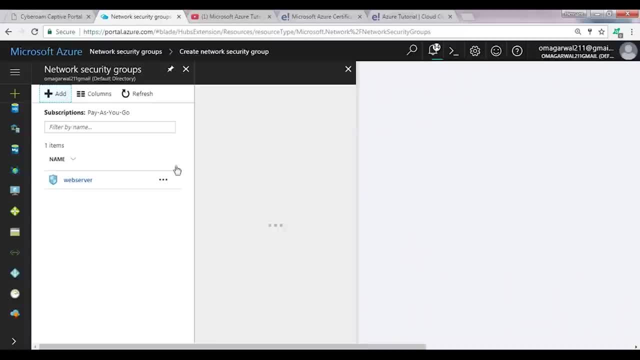 which is for my database, right? So I'll click on add and I'll type in database. I'll include it in the resource group that I've already created, which is live-demo. I click on this, I'll pin it to dashboard and I'll click on create, right. 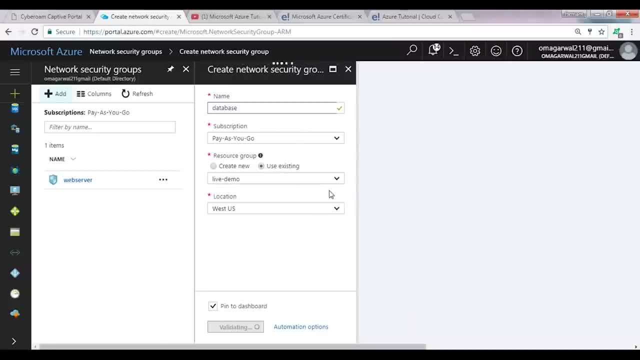 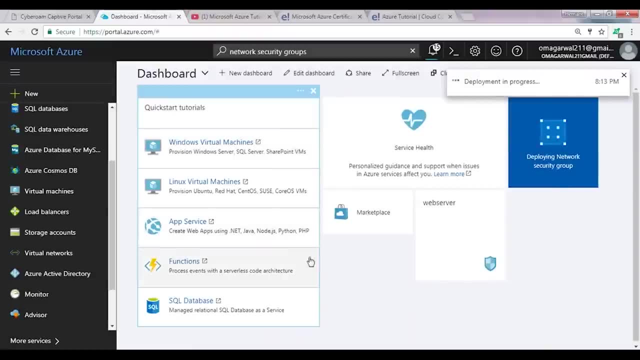 That is it. It's pretty simple. You just enter the name, the resource group that you want to enter it in, and create it right Now. one thing that I want you to notice is, guys, I have not configured any property as. 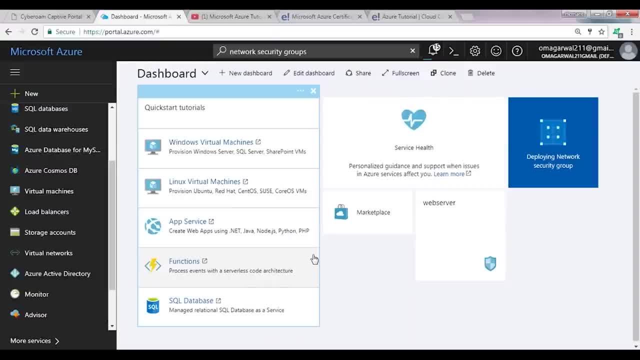 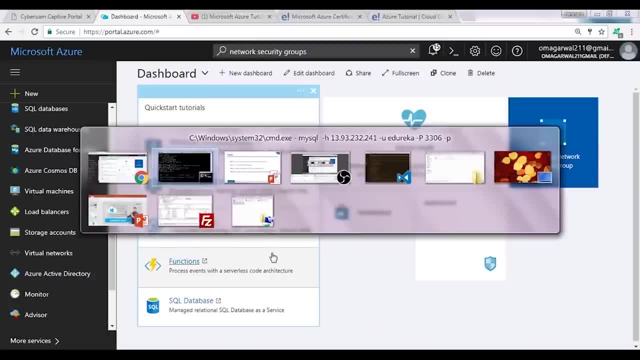 of now. right, I'll do that later. So, as of now, I've just created two firewalls with the name web server and database. Now what I'll do is let me come back to my slide to see what we'll be doing next, right? 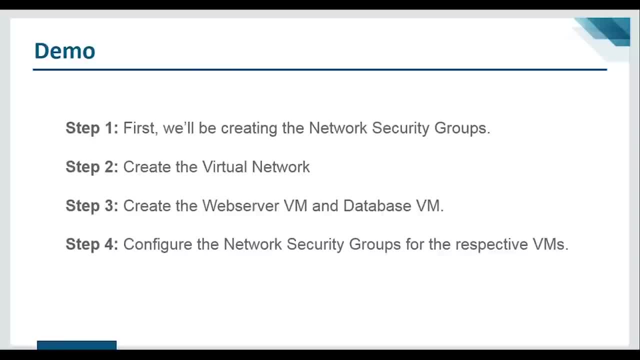 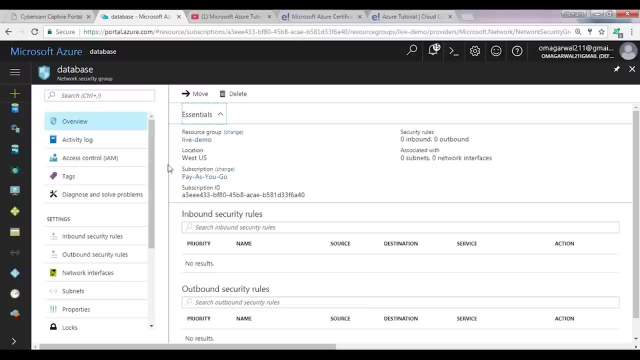 So step two is create the virtual network. Okay, So now I'll be creating the virtual network in which I will be deploying my servers, right? So let's do that, Let's create a virtual network. So I'll click here, I'll go to virtual networks. 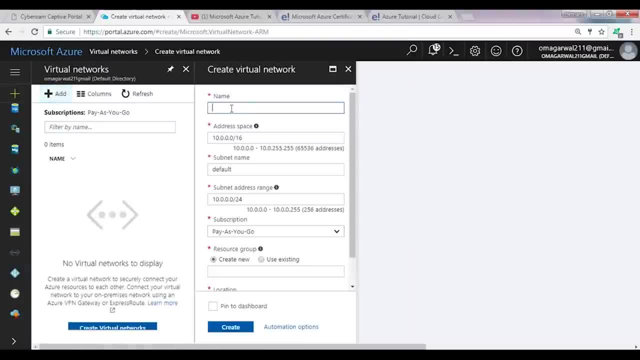 I'll click on add and I'll give the virtual network name, say VNet, right, And then comes the address space. Now what is the address space? Address space is basically the number of IP addresses that your network can hold. 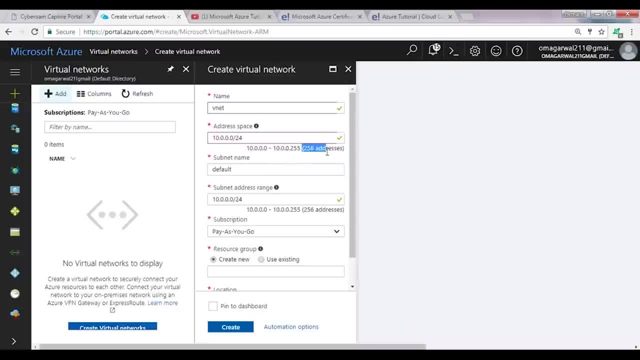 So as of now, this virtual network is the address space. Okay, So this virtual network can hold 256 computers right, or 256 virtual machines. Now, since I'll be creating more than two subnets, I want an address space which will be more. 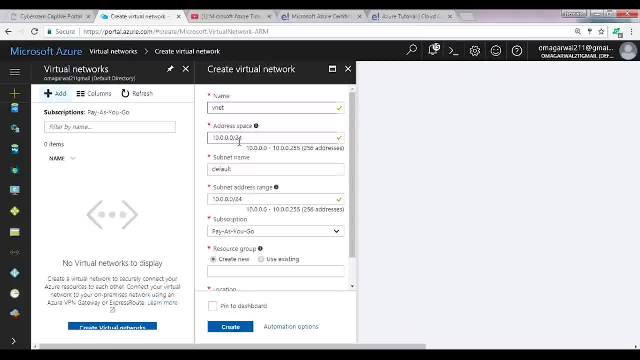 because each subnet will take some minimum value, right? So let us give it a more elaborate address space. Let me type in this right and edit this part, And this will give you a bigger setup. So let's go ahead and create a new set of addresses to deal with. 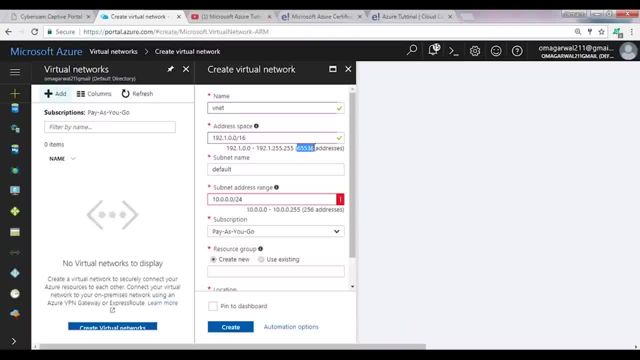 So now my address. my virtual network will be capable of having 65,000 addresses, which is kind of cool, right. Next, we have the subnet name. So by default, when you create a virtual network, there will be a default subnet will be created. 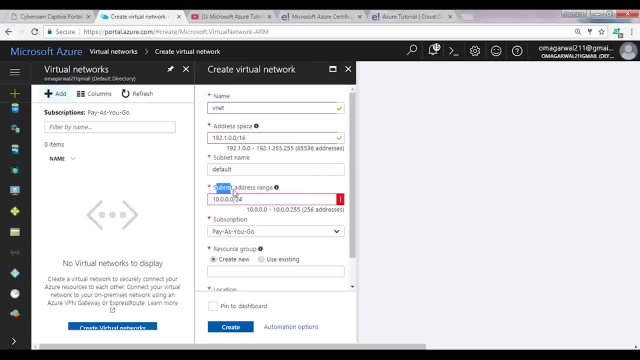 which will be created, right? So this is the address range for that default subnet. so it should be in the same range that we have specified for our virtual network. Okay, So let's create a virtual network, So let's give it this address. 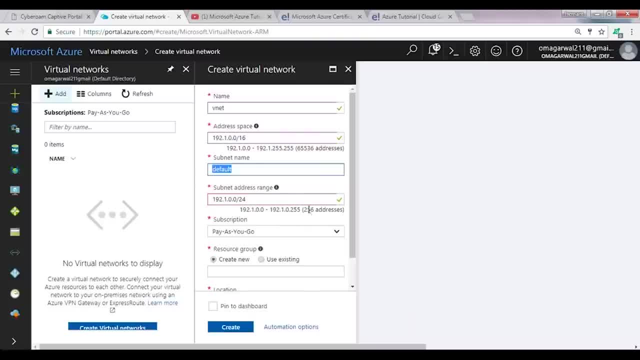 And, as you can see, in this particular subnet- that is the default subnet- I'll have around 256 machines right. So that is it. Nothing else needs to be configured. I will include it in the resource group that I've already created. 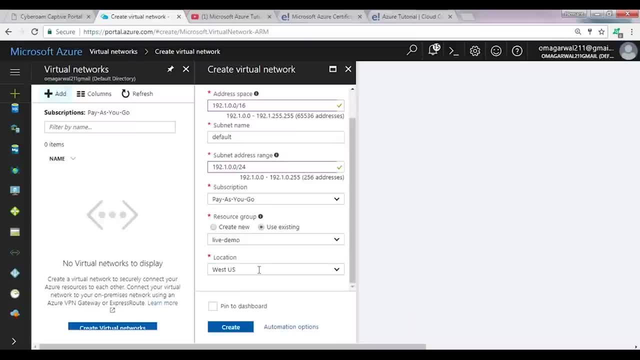 That is live demo, And location is basically the place where the servers are being deployed, right? So by default it's best US. We'll keep it at that right And we'll create this virtual network. That is it, guys. 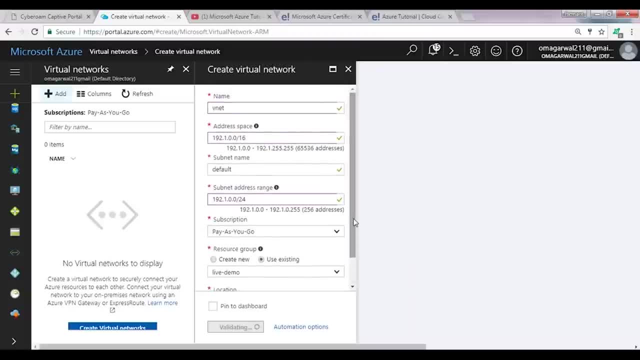 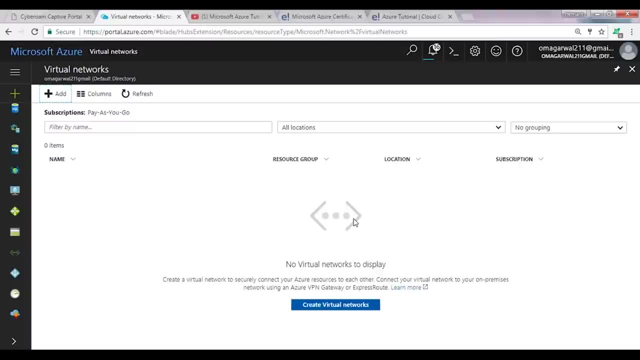 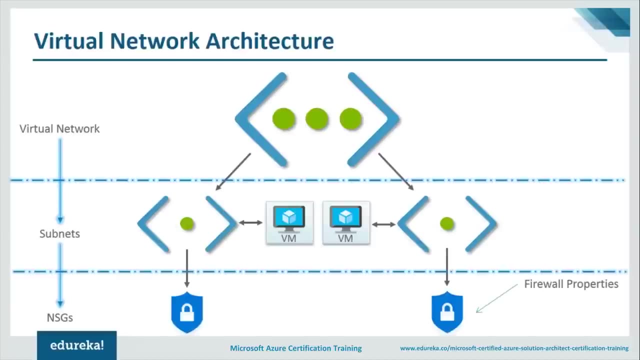 Nothing else to be configured For as of now. this virtual network does not have any subnets, right? We want a web server subnet and we want a database subnet that we'll be deploying now, once the virtual network is ready. right? Let me come back to my slide and show you this diagram. 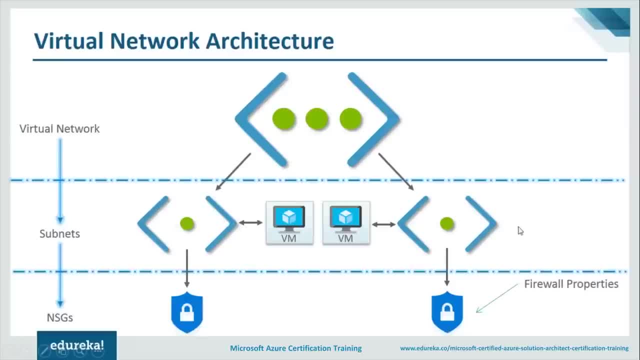 So this diagram basically talks about a virtual network, two subnets. Now what I'll be doing is I'll be launching two virtual machines and I'll be attaching these virtual machines with this subnet. all right, And this is basically your network security group. 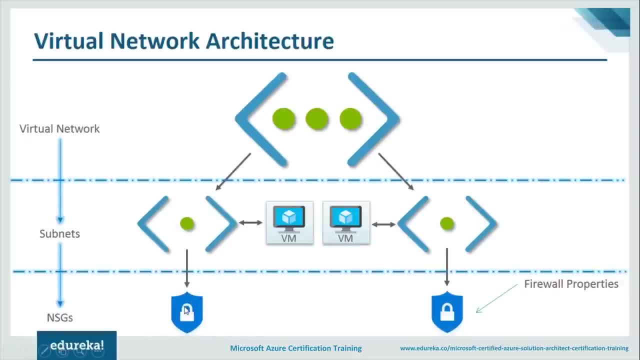 This is where you'll be configuring your properties, and this also I'll attach to the subnet Now. this VM will then reflect the properties of this particular firewall, right? I'll not be attaching this firewall directly to this VM, but I'll be attaching it to the 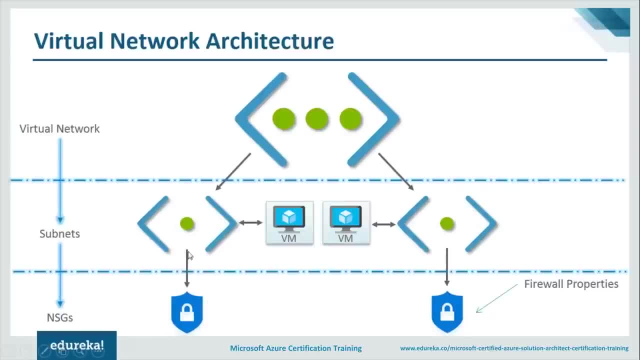 subnet. Now what advantage do I have in this is that, say, I launch three servers in the subnet, All of them will reflect this property right, So I don't have to configure them separately. So I don't have to configure them separately. 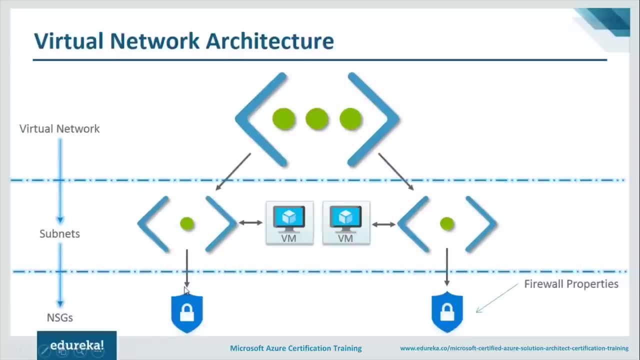 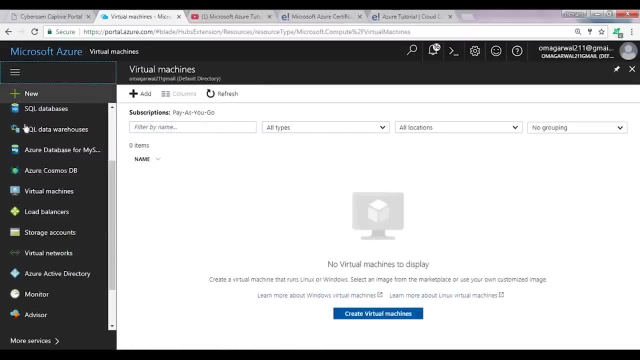 All of them will be reflecting the security group's properties of this particular subnet. All right, I think our virtual network is ready. Let's see. So if I go to my virtual networks, I'll see that I have my virtual network ready. 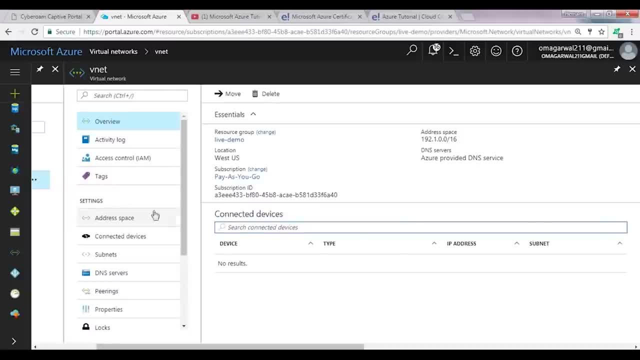 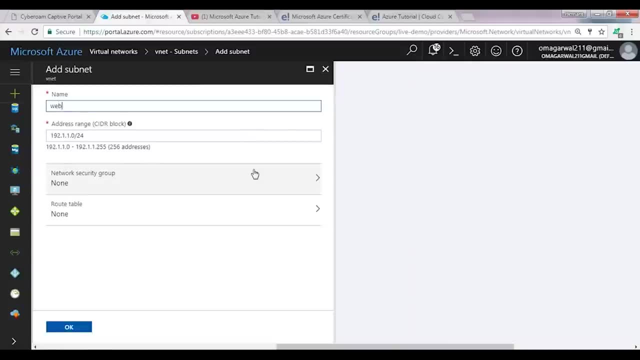 All right, Now I'll go inside my virtual network and now I'll be deploying the subnets. So we'll go to the subnets pane, We'll click on add and let's add our first subnet, which is the web server subnet right. 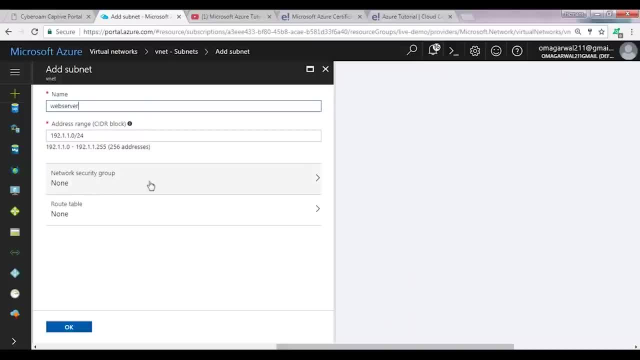 Now this web server subnet will be attached to a network security group, which will be for the web server, right? So we'll attach a network security group for the web server and we'll click on OK, That is it. It's that simple. 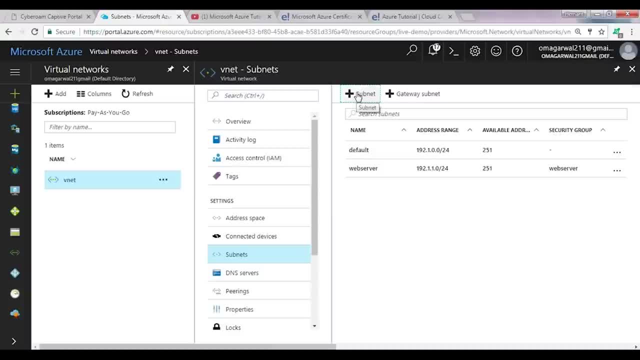 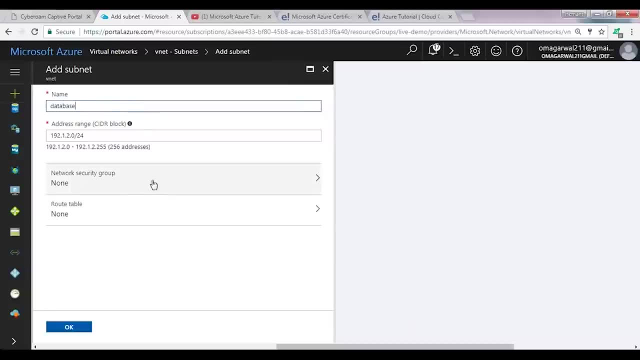 Just add the subnet, attach the network security group to that and you're done Right. Similarly, I'll be deploying the database subnet now and I'll go to network security groups. I will click on the database subnet. Database subnet. 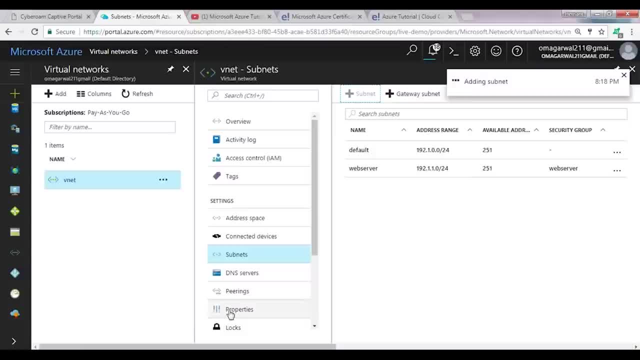 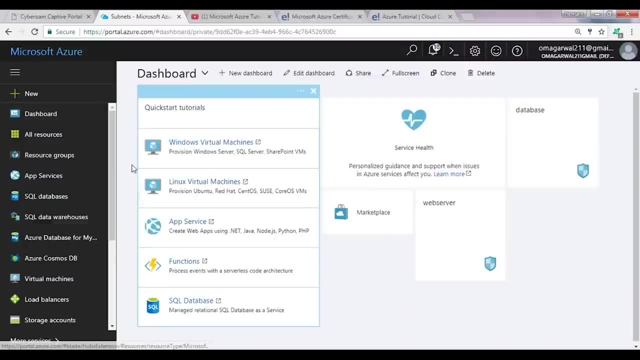 Database network security group. I'll click on OK and bam, I have one more subnet. Let me go back to my dashboard and see what all do I have. So I have the two network security groups. I have deployed the virtual network. 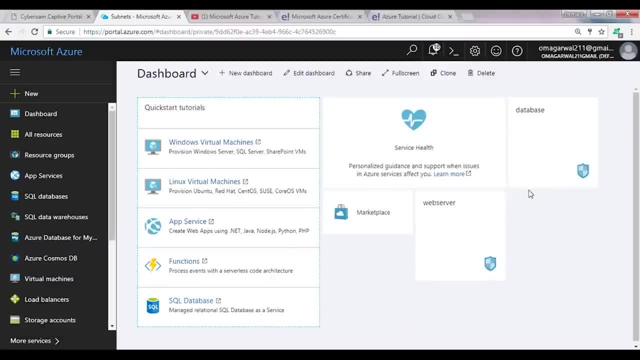 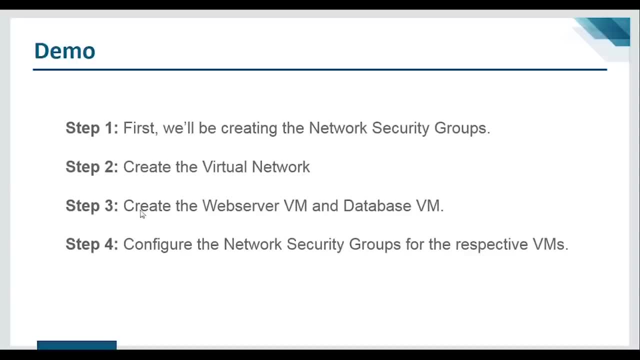 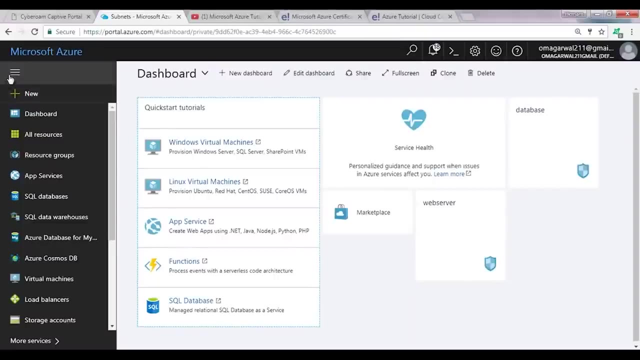 I have deployed the subnets in it and I have attached the firewall to the subnet. All that is left is now the VM. So step three is create the web server virtual machine and the database virtual machine. So let us do that. We will go to our pane. go to virtual machines, right. 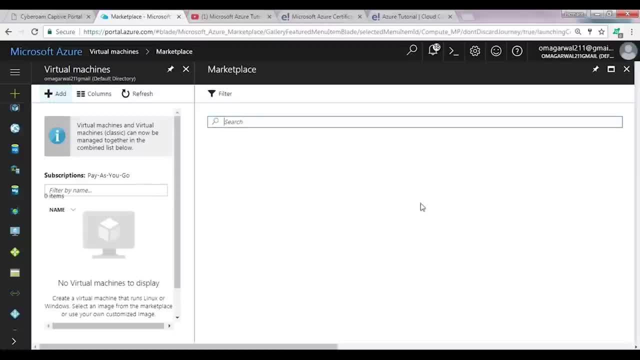 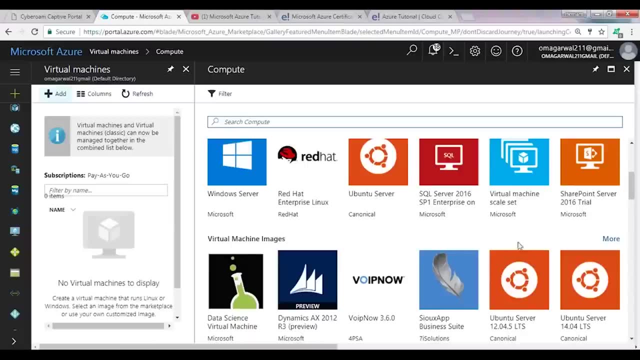 Click on add and with this you will get this page wherein you have all the operating systems that you can set in your virtual machine. Now you can set a Ubuntu operating system. You can also configure a Windows server, but we'll be dealing with Ubuntu today, right? 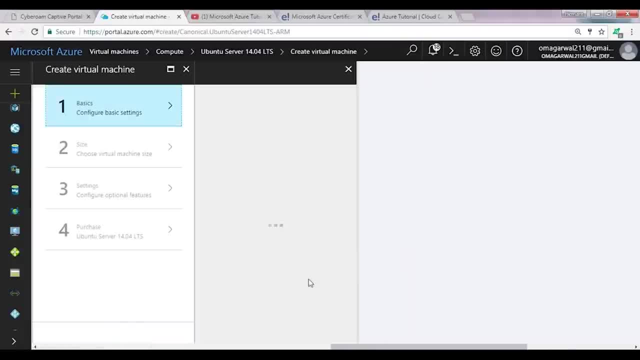 So I'll select Ubuntu, I'll click on create And then I'll get this page where I have to enter the general properties. So I'll name the server as web server, right? I'll give the username, the username that will authenticate me to this particular server. 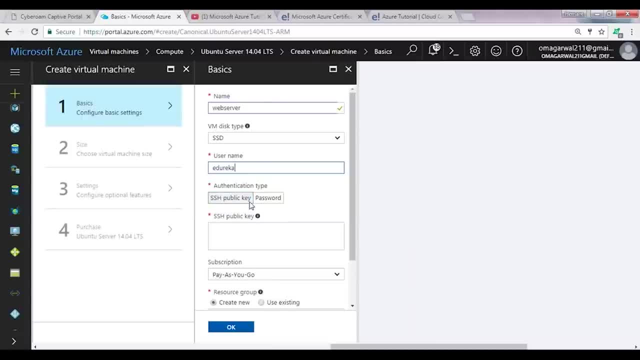 Now, when you talk about the password or the way you will authenticate yourself, you basically have two options. You can either authenticate through a public private key or you can authenticate through a password. So password is more easier and since we want our things to be done quicker, I'll give a 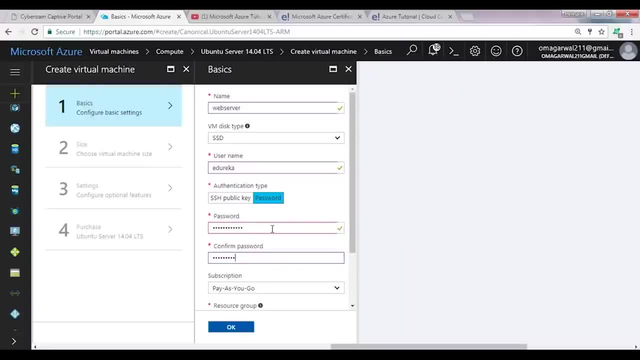 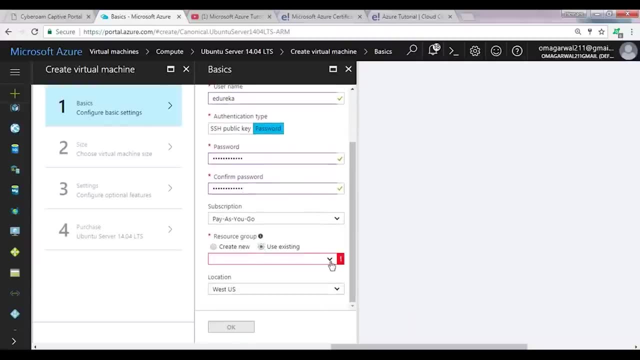 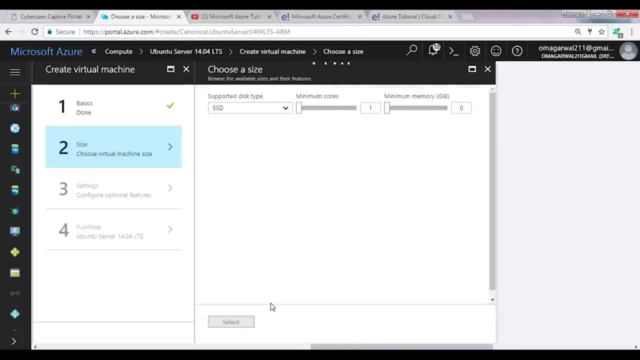 password. And this is the password. I'll configure it now And that is it, guys. Nothing else needs to be configured. Resource group: I'll give the resource group that I've already created. that is live demo And I'll click on OK. 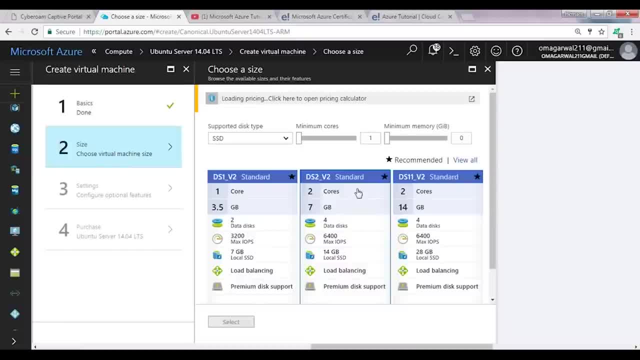 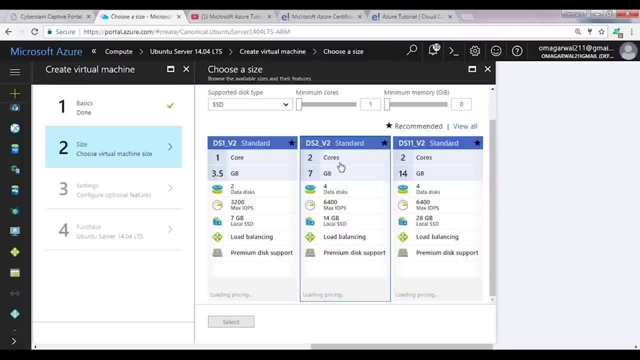 On the next page it will ask me the configuration of my server that I want, right? So do I want a one-core CPU and a 3.5 GB RAM, or I want a two-core CPU and a 7 GB RAM? 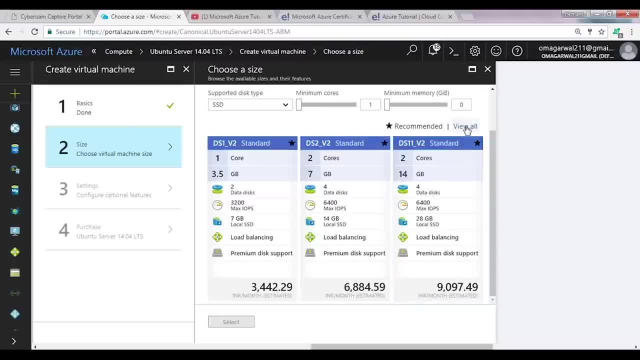 I can choose all the configurations which are available here in the view all page, But I'll stick to the first configuration, which is the basic one, because I'm doing a demo right, So I don't need a big machine for it. 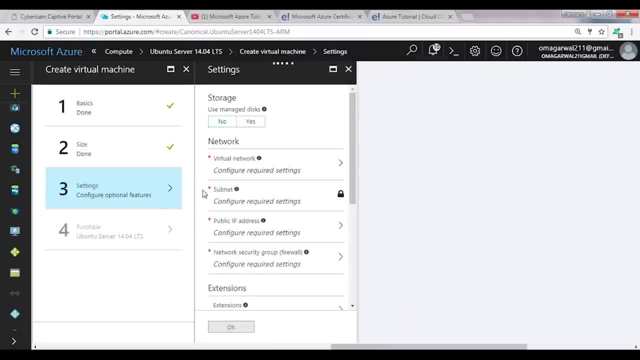 I'll click on select. Next comes the optional features that I have to configure. right. So the storage. and then what virtual network do I want my server to be deployed in? So we have created the virtual network called VNet, So we'll be deploying it in this. 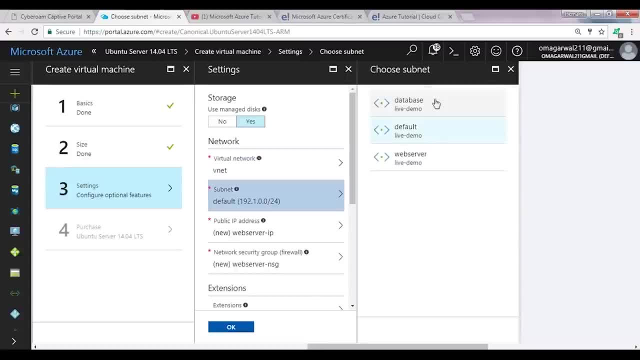 Then comes the subnet. So inside this virtual network there are three subnets. Like I said, one is default, That is created by default, And then we have the database and the web server subnet. So since this is a web server VM, we will be deploying it under the web server subnet. 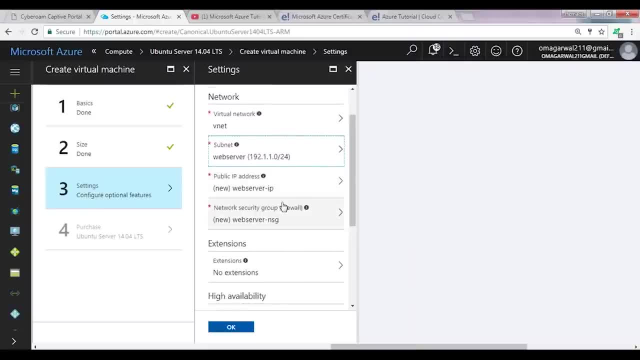 Then comes the public IP address, so it'll assign it a public IP address through which we can access it. That is going to be new. And then comes the network security group. So, since we have already assigned it to the network security group, we'll be deploying. 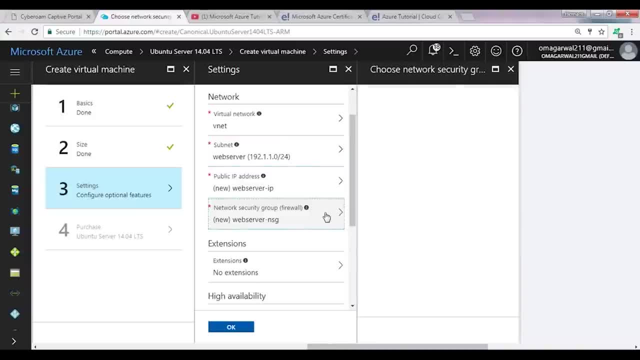 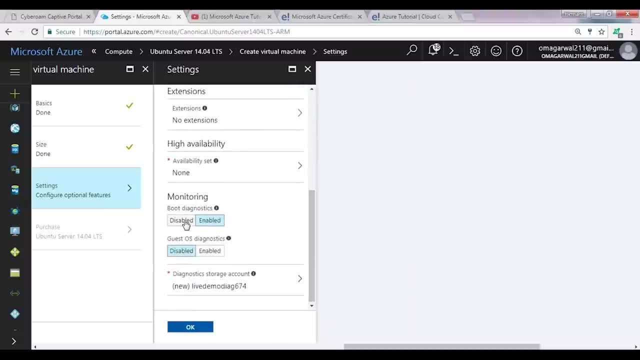 it. So once we have assigned a network security group in the subnet, we don't need any network security group to be attached over here. So we'll click on none And then monitoring. Do you want it or not? I would prefer to be disabled because I won't be needing the server after the session. 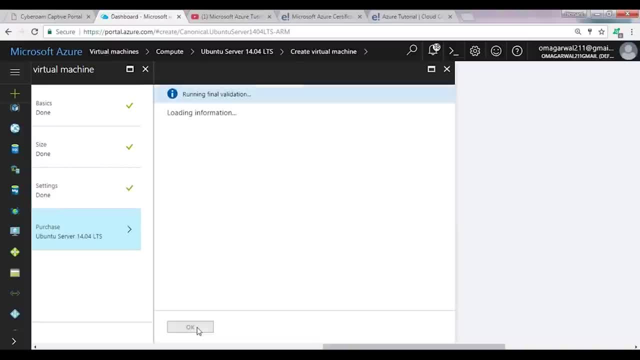 So I'll click on disabled and I'll click on okay, All right. So now what will happen is it will validate all the properties that I've entered And, once it has entered, it will give me a page wherein I have to agree with it. 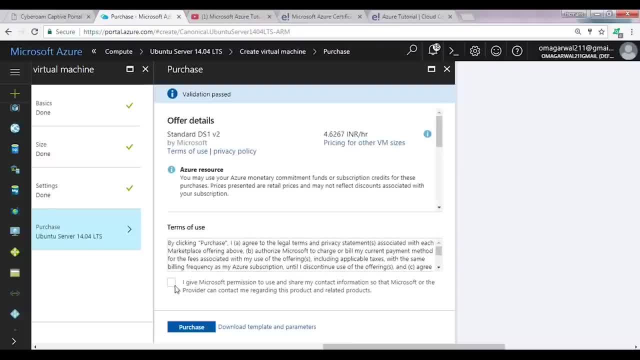 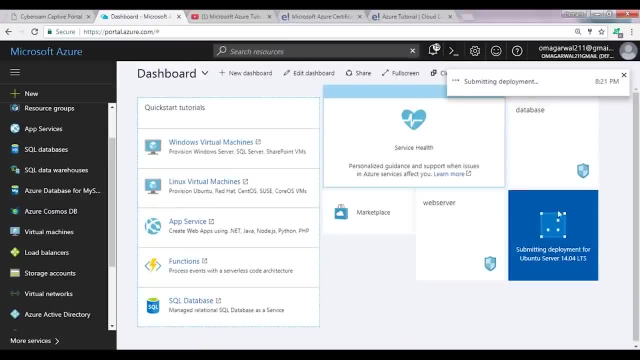 Okay, So I'll agree to the terms and conditions and that is it. So I'll agree to the terms and conditions and I'll click on purchase And that will deploy my server. That is it, guys. So this is my web server being deployed. 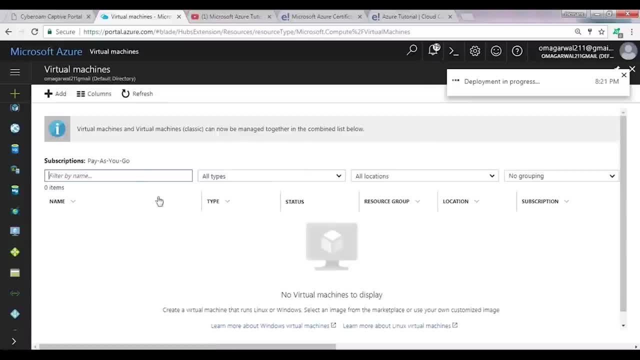 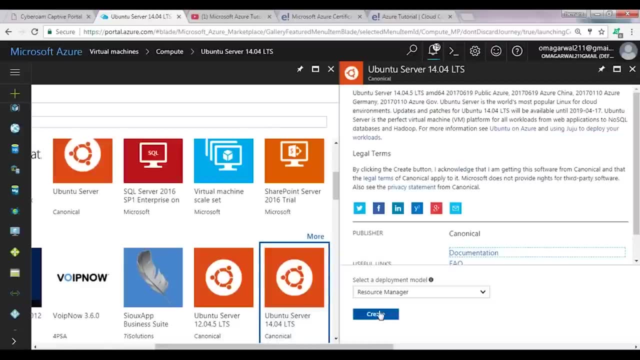 Let's quickly deploy our database server as well, following the same steps that we have followed now. right, So I'll choose Ubuntu machine. I will click on create, I will go to this page and type in the name of the server, which is database. 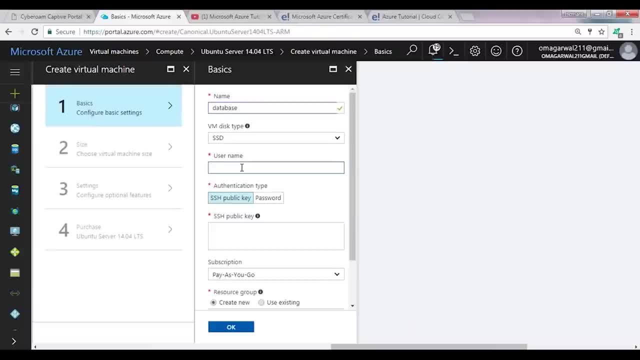 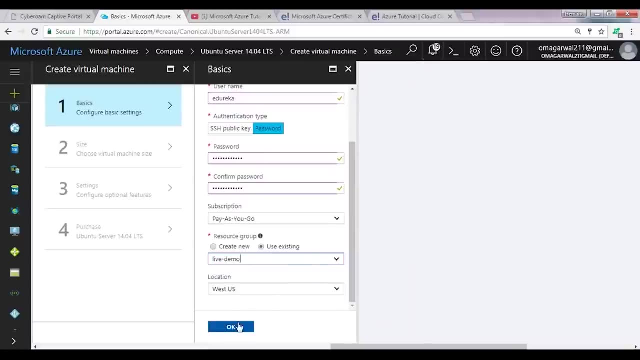 Okay, Right, The username. So it's Eureka. Authentication type is password, So I'll type in the password now. Confirm the password. And then comes the resource group. So it's live demo, Right, And the location is West US. 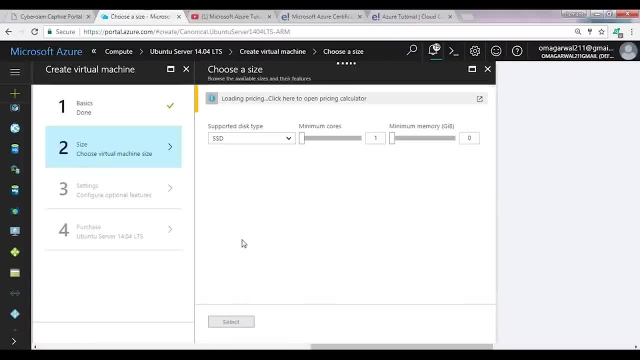 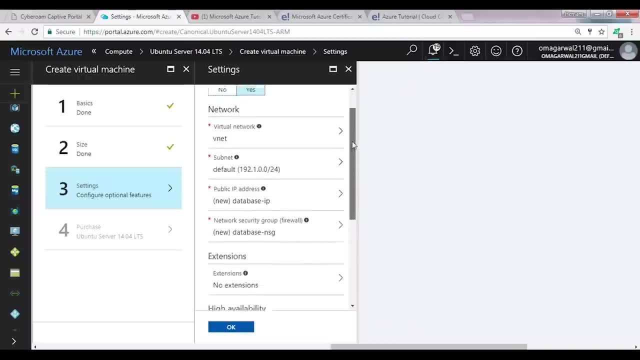 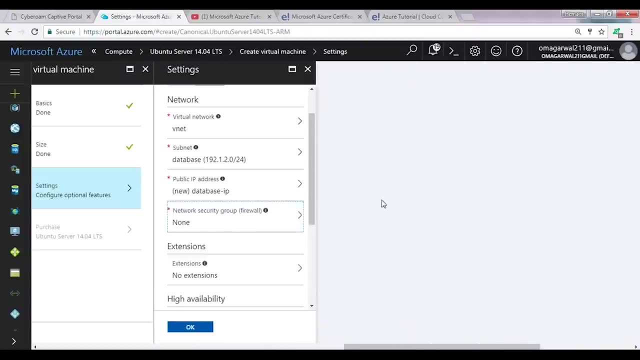 I click on okay, Select the most basic configuration, which is the first one. Click on select. Now I'll be configuring the virtual network settings. So subnet would be database Right. Network security group will be none, And that is it. 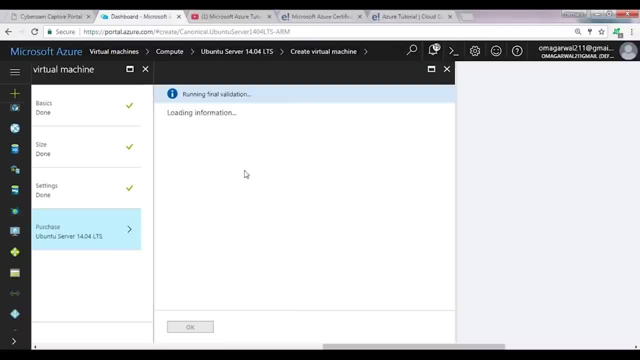 Monitoring will be disabled. Click on okay. It will validate all the properties And then I shall purchase the server, which will be deployed. Right, If you're talking, if you're thinking, how much is it going to cost me? so each server? 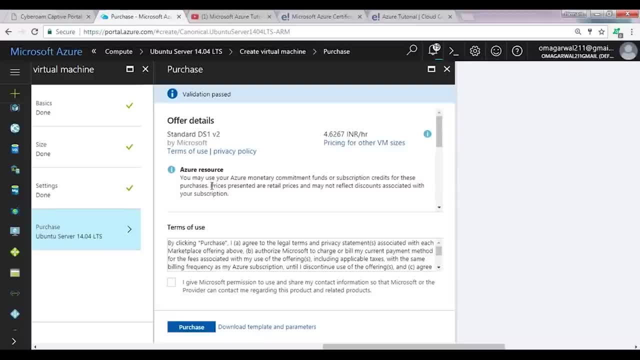 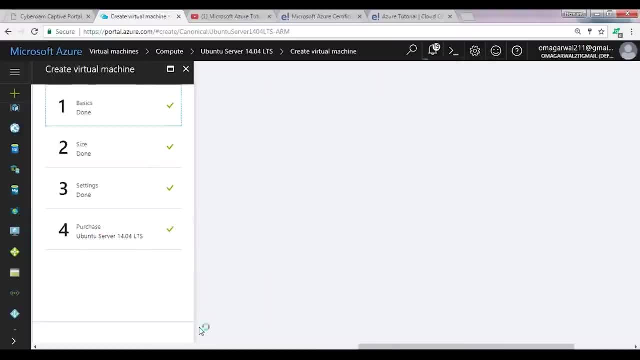 is going to cost me around 3.5 rupees per hour, Right? So that's like a fraction of a dollar. So I think if you're learning Azure, that is worth it, Right? So my servers are being deployed, guys. 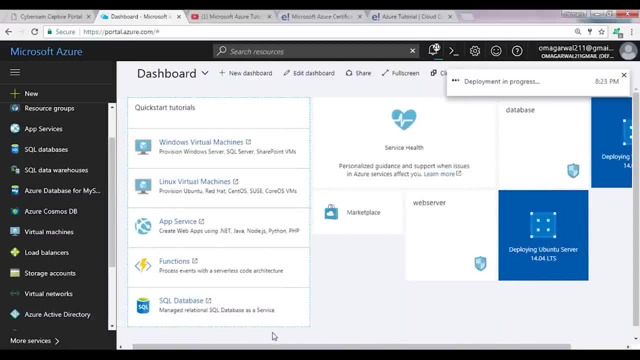 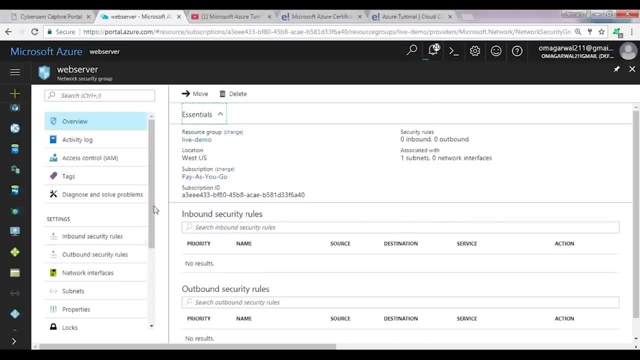 Now, while my servers are being deployed, let me configure the properties of each server, Right? So let me go to the web server firewall and configure the properties. So, basically, what I what I'm looking at is the inbound security rules, So I click on inbound security rules. 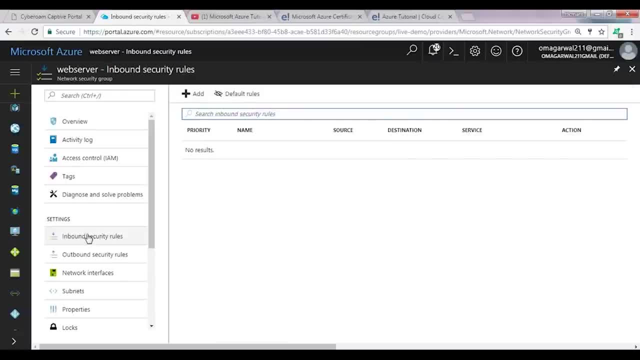 So inbound security rules are basically the rules which are created for the connection Right, The connections which are incoming to the server Right. So this is a web server Right. So for a web server, first you have to enable the HTTP connection. 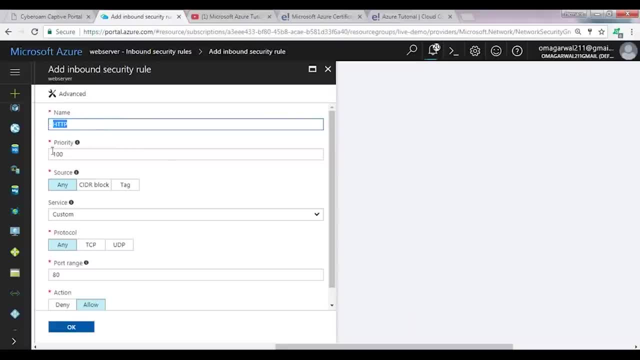 So I want the HTTP connection through HTTP protocol to be enabled over here. Right, And the source is any. what? what kind of people can access the server? So I want the whole world to access my internet website. So the source is any, the service is HTTP. 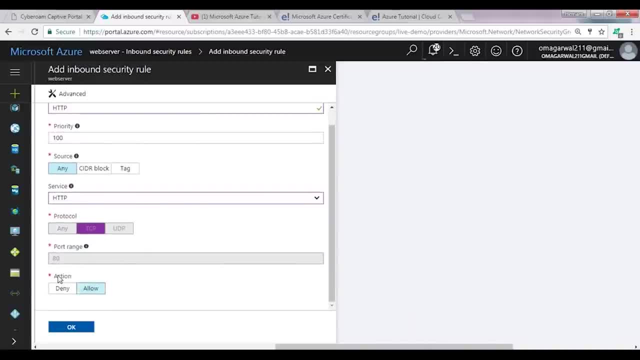 Right, And everything else is default. The action: What do you want? What do you do? you want to deny it or you want to allow it? So I want to allow the connections. So I'll select allow and I'll click on okay. 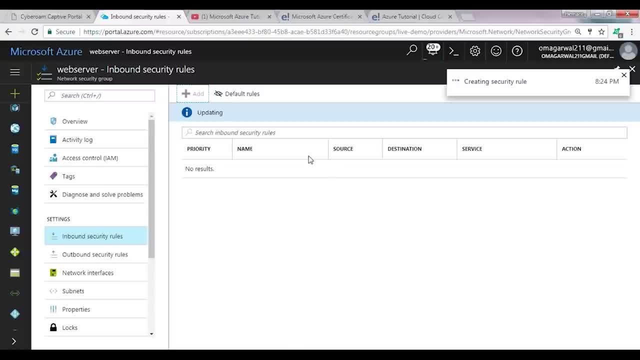 All right, So my security rule is being created. So, while this is being created, guide guys let's. we'll have to add one more security rule, which is the HTTPS security rule, Because Our websites connect through two protocols, which is HTTP and HTTPS. 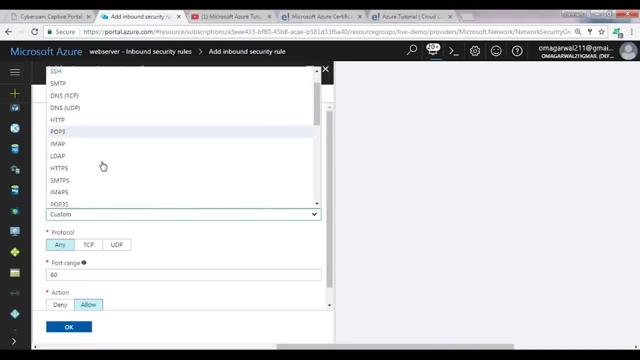 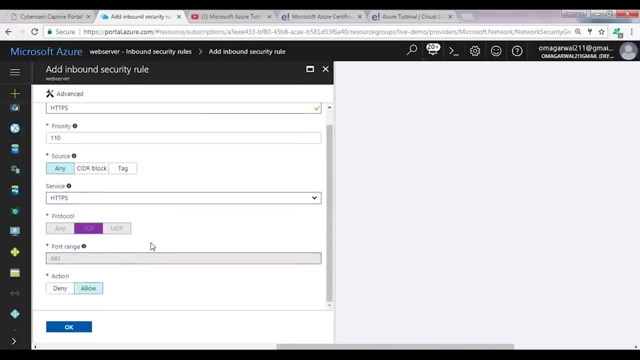 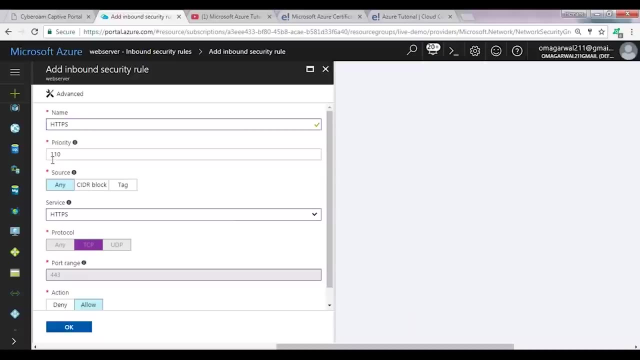 So we will configure HTTPS as well. So let us select HTTPS from the list. Here it is, And then the action is allow. And you might be wondering what this priority number is right. So priority number is basically the number which will be given to your rule. 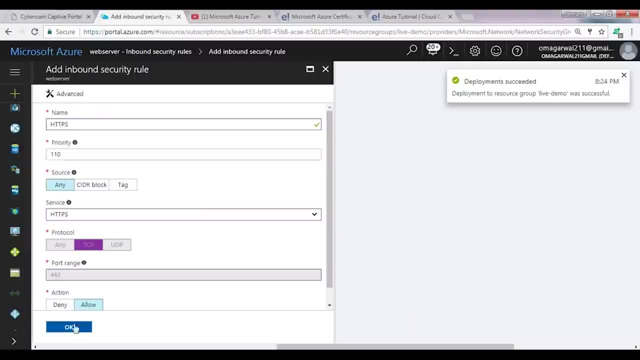 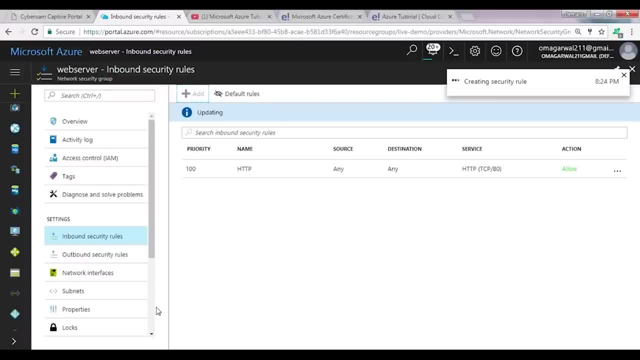 So, say example, in my previous rule I gave the priority number as hundred Right. So when it reads the set of rules that are given in the firewall, the first rule would be the least number which is there. So the least number is hundred and it goes up to, I think, 900. 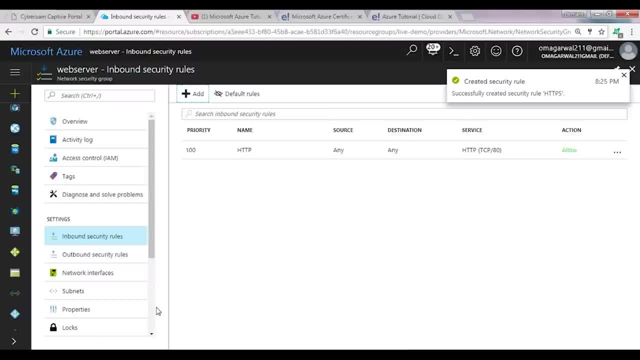 Right, So it will read all the rules according to the numbers and then configure them. So we have added the HTTP rule and the HTTPS rule is also being added, And that is it. That is all is which is required. So let me just refresh it and I can see their HTTP. 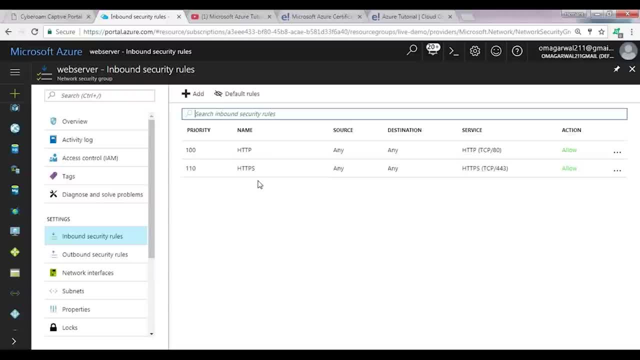 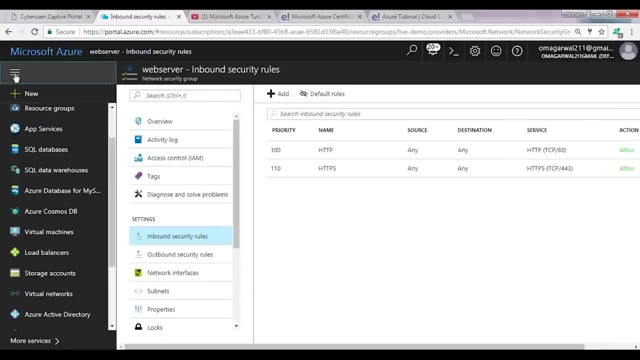 And HTTPS rules are already been given. Now I also want to SSH. I should be able to SSH into my server, But before that, let me show you what if I don't configure the property here. Let's see what then happens, Right? 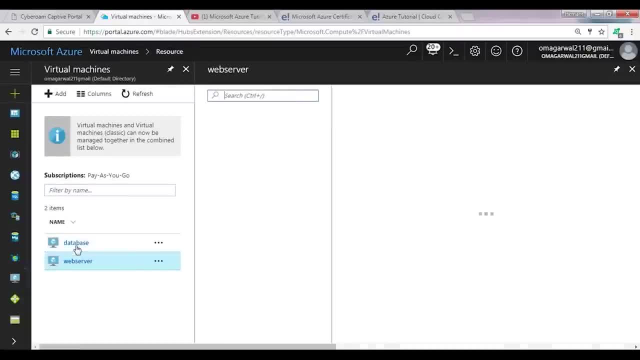 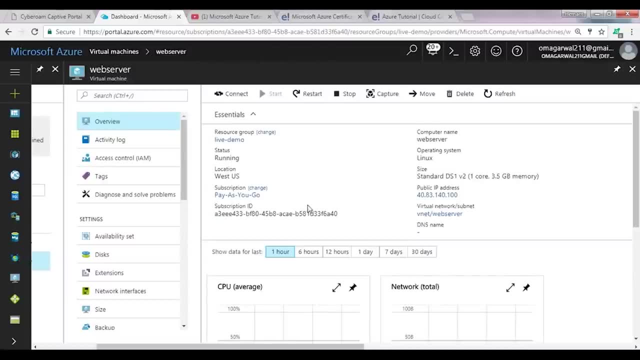 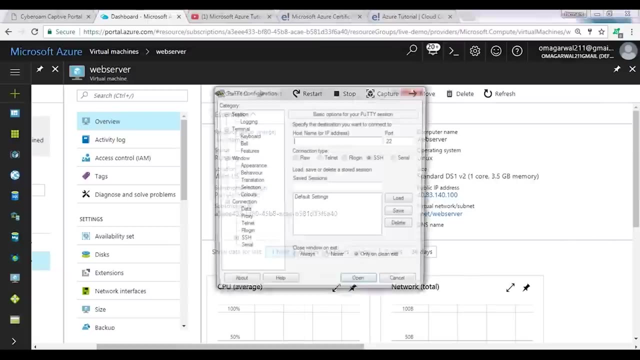 So for configuring my web server, I'll have to SSH into the web server to see to install all the softwares which are required for that particular server Right. So let's connect to this server. So the way I can connect is using a software called Putty. 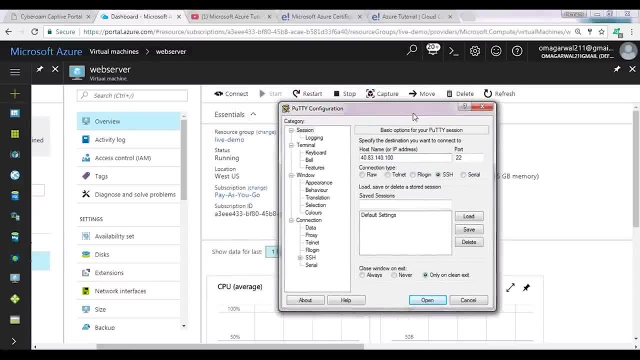 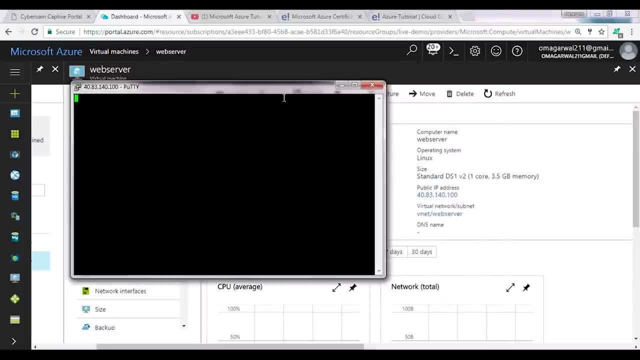 So I launch the software, I paste the IP address here And as of now, guys, I have not added the SSH property, Right? So if I try to connect, it will show the screen and it will keep on pointing here, Right? 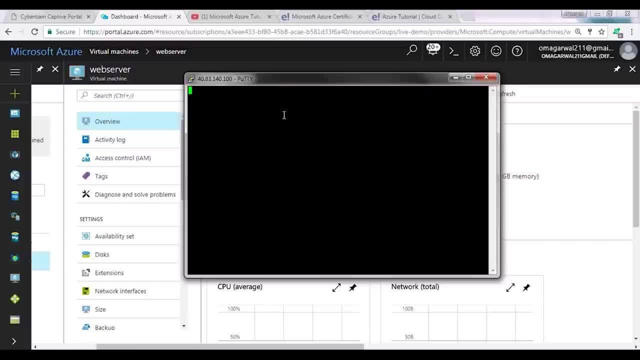 So the connection will time out after a few, say 30 or 40 seconds, And that basically means that the server is refusing any connection to it, And the reason for that is that I have not configured it in my firewall So to do that. see, as you can see, it has given me an error which says connection timed. 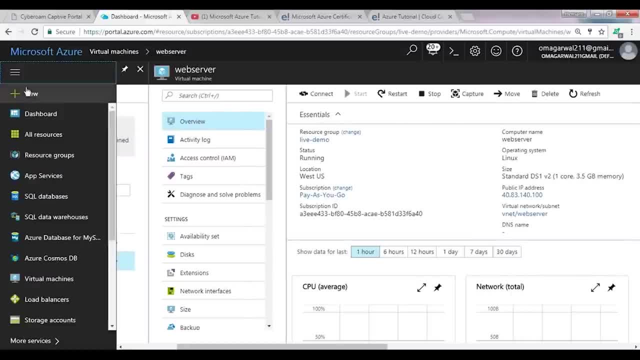 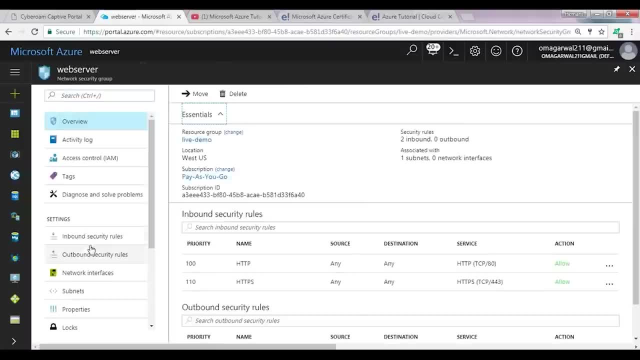 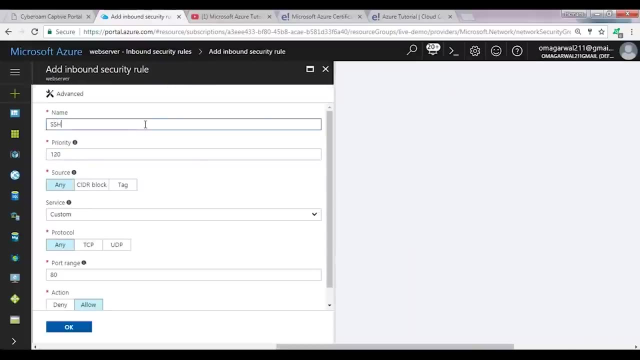 out. So to do that I'll have to go to my firewall, which is the network security groups of my web server. Right, I'll go to the inbound security rules And now I'll add a rule for SSH. So once I add the rule, I'll be able to connect to my service. 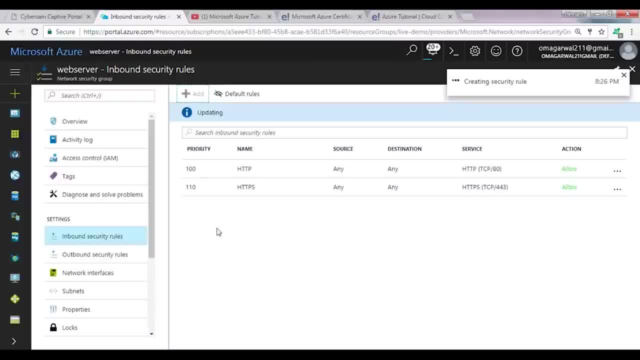 So it's done. My security rule is being created, And once it is created, I'll be able to SSH into the server. Also, it takes some time for that rule to actually be applied. Right, It says that it created a security rule, but sometimes it takes time to reflect. 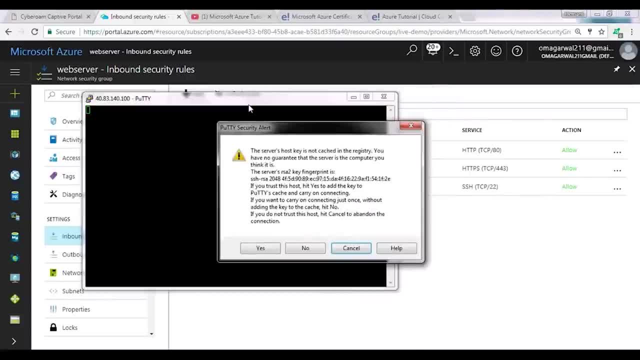 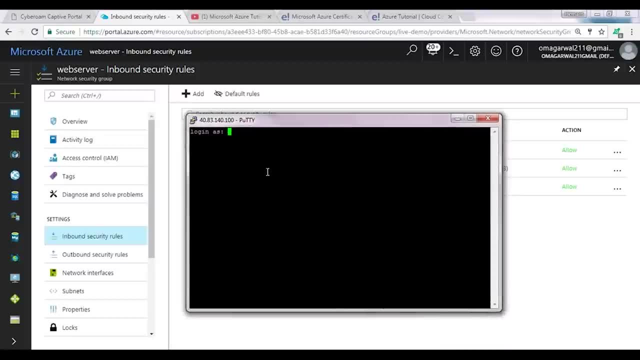 Let's see if the rule is being reflected here. And yes, the rule is being reflected. So, as you can see, I've added the SSH rule And now it is giving me the login page. So I log in into my server, which, with the username Edureka, I configured the username. 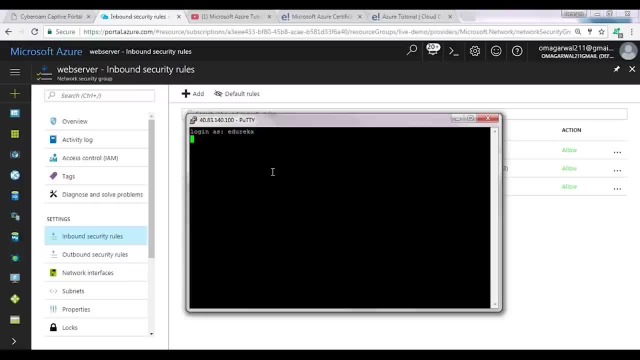 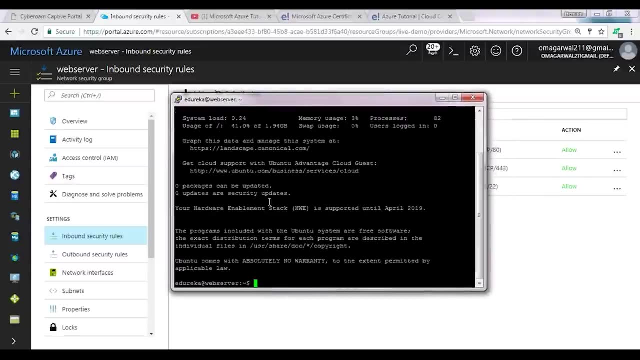 to be Edureka, And now it'll ask me the password after authenticating the username. So I'll type in the password And, if everything goes well, I'll be authenticated to my server, Right? Yes, So I am in my server. 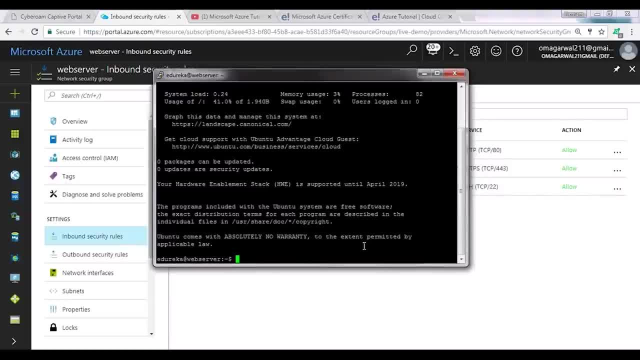 So this is my Ubuntu server, which is running on Azure cloud. Now I need to configure the softwares in it so that it becomes a web server. Alright, So as of now, there's nothing installed on it. It's a fresh piece of software. 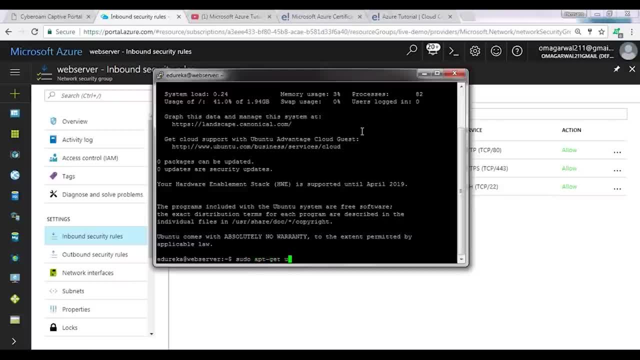 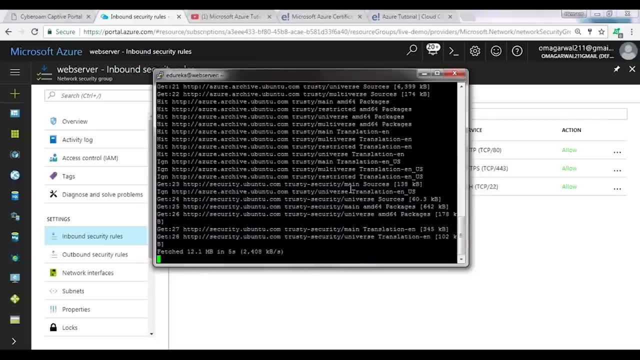 So let me first update this Ubuntu. So I'll type in the update command. It's sudo apt-get update Right Now. it'll take some time to update. Meanwhile, guys, let me quickly show you if I can access my web server as of now or not. 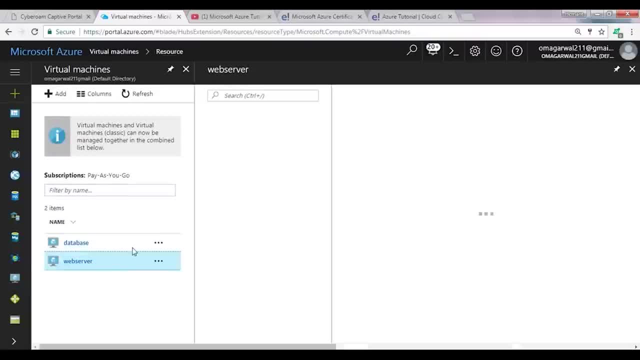 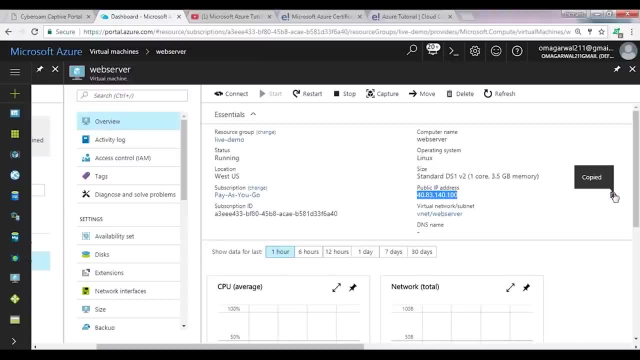 Right, So I'll go to virtual machines. I'll go to web server. Now. you might ask me that we have already configured it to accept HTTP connection, But still, if I try to connect to this server, I'll not be able to do so. 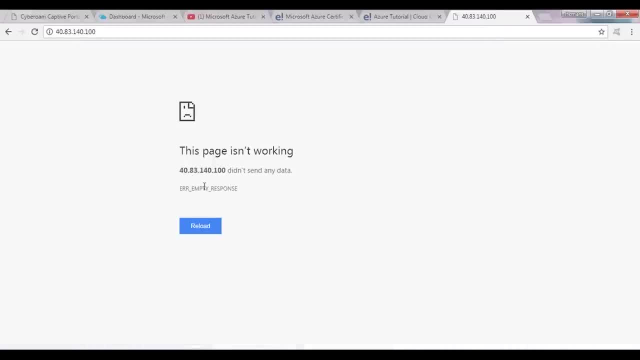 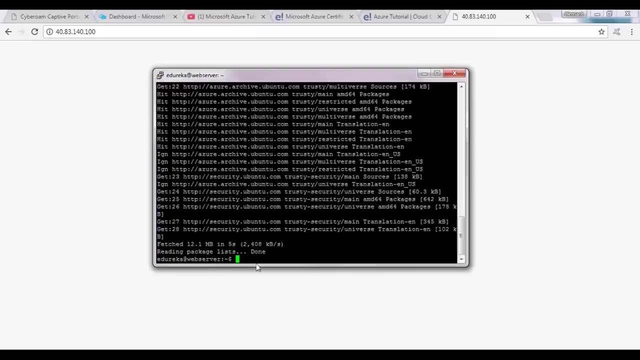 It'll return me an empty response screen. So this basically means that there is nothing configured on my server as of now. So what I'll do is so my Ubuntu is now updated. So what I'll do now is I'll update it with the. 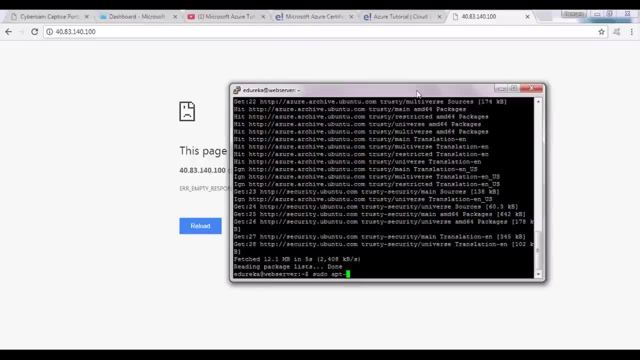 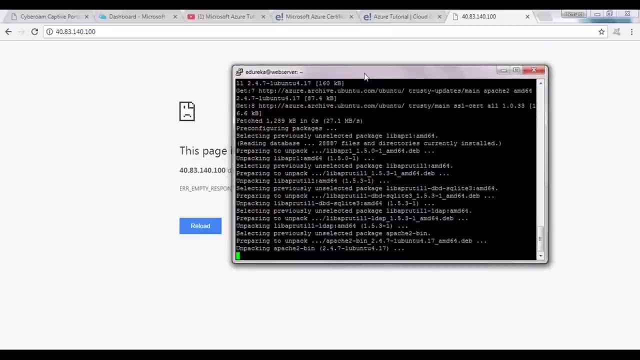 Apache software. Right, So I'll type in the command for Apache, So: sudo, apt-get- install apache2.. All right, Once I've done that, it'll install the Apache software here And within seconds you can see that I'll be able to connect to this server. 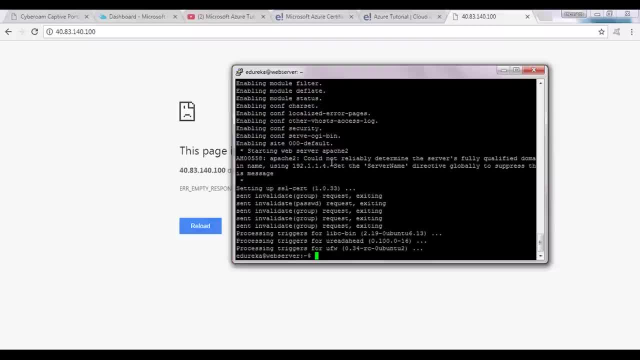 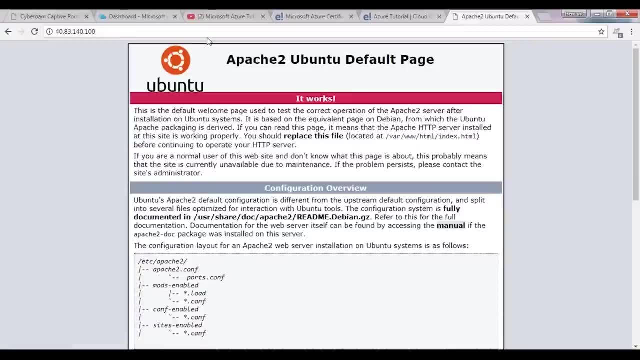 So it's starting the service processing. Yeah, So Apache is installed. So if I try to connect to this server, you'll be able to see that I'm getting the Apache screen. So if you want, you can connect to this server. 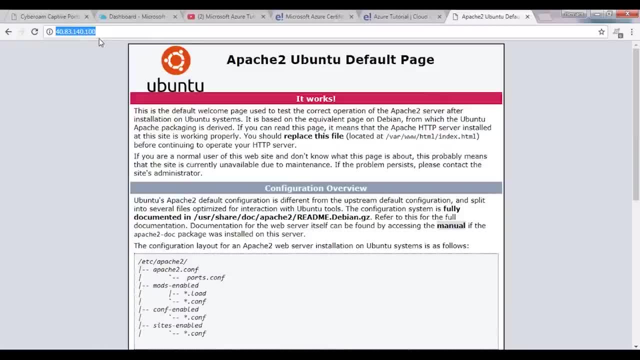 The IP address is 40.83.140.100.. My team will be handing you out this IP address, So I'll repeat it again: It's 40.83.140.100.. You can go to this link and you'll see the Apache page as of now. 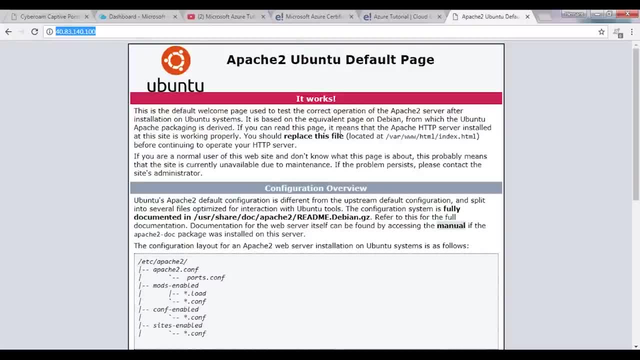 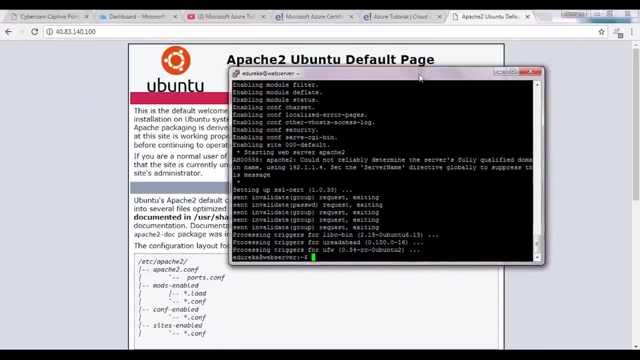 Now, as we'll go along and we'll update this thing, this website, You'll see that this page will be updated. All right, So I have the Apache working on my server now. Now my website that I've created. it is actually a PHP website. 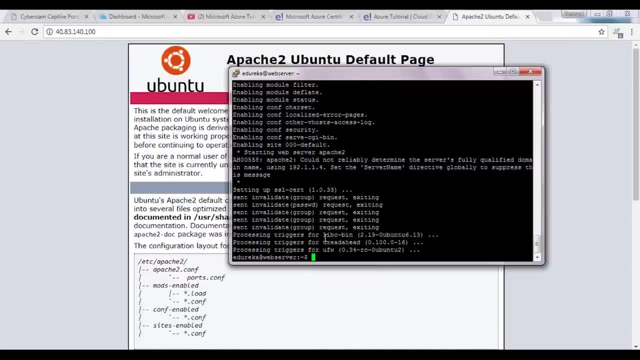 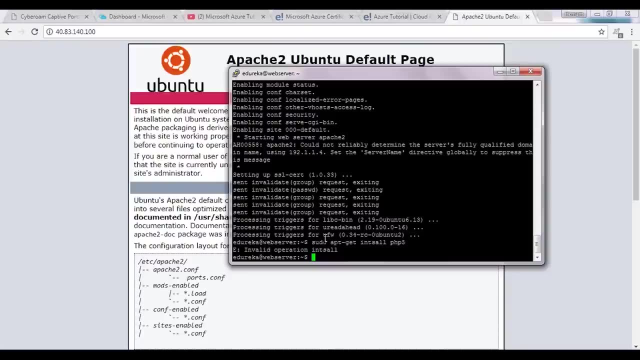 So I'll have to install PHP on this server as well. So I'll write sudo apt-get- php5.. And I'll have to install it. So that's it. This is it One second. So I mis-installed my badge. 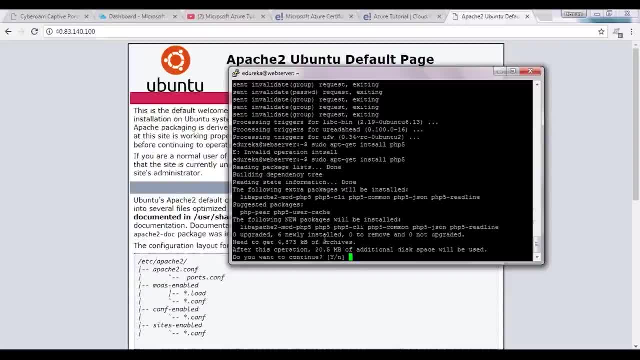 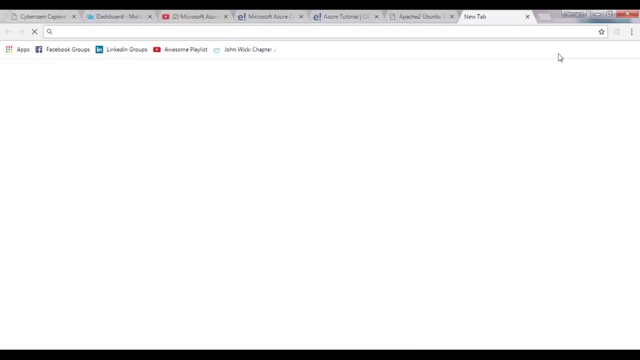 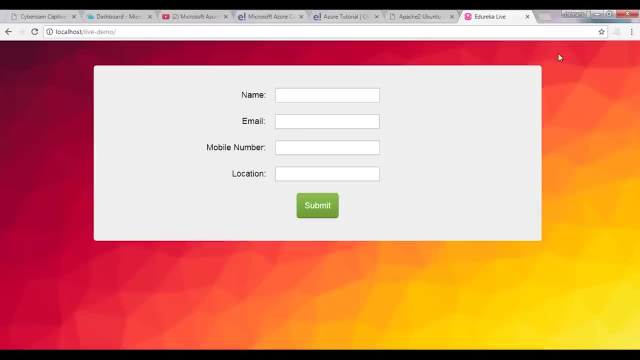 Sorry, Right. So now my PHP will be installed on this system, And while this is being installed, guys, let me show you how my website actually looks like. So I'll go to localhost and I'll type in the address for my website. 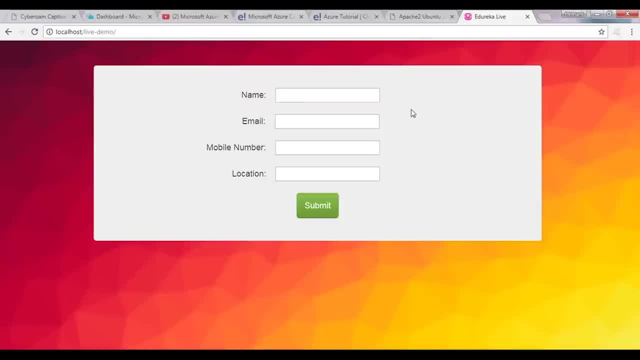 All right. So this is how my website actually looks like. It's pretty simple. You just have to enter your name, your email, your mobile number, your location, And once you click on that, it will show you the address. And once you click on submit, all of this address will go to MySQL. 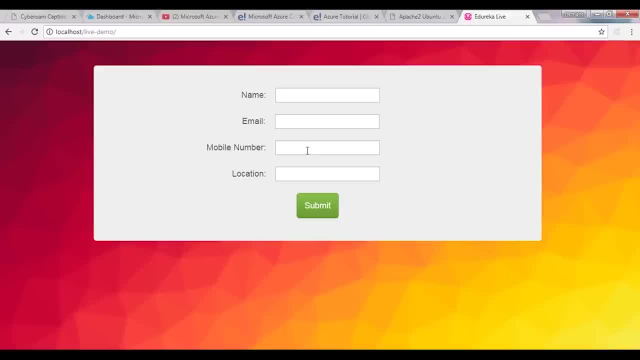 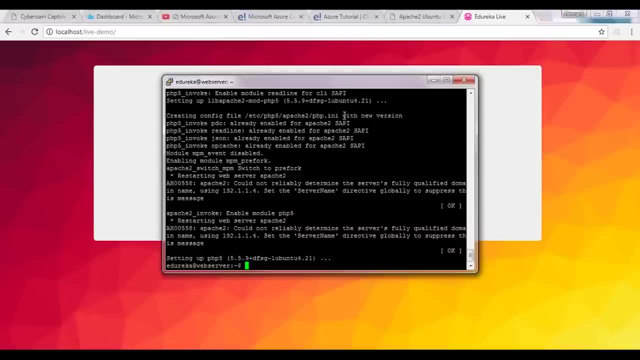 Now MySQL is in a different server. This will be in a different server, And what we're trying to do is we're trying to authenticate them to each other using watchmill networks. All right, So if I go to my web server, so my PHP has been installed. 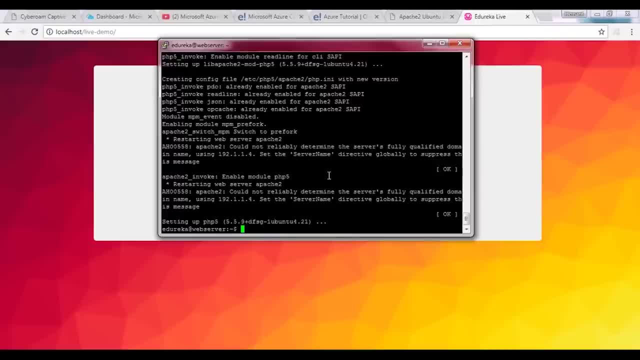 And with PHP I also need an extension which will allow it to connect to MySQL. So for that I'll have to install that extension as well. So sudo apt-get install. So with this my extension will get installed on the system. 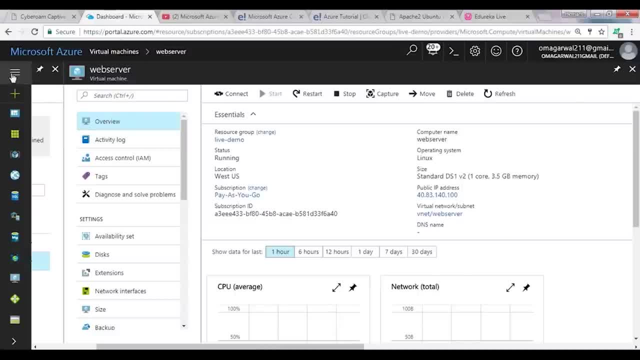 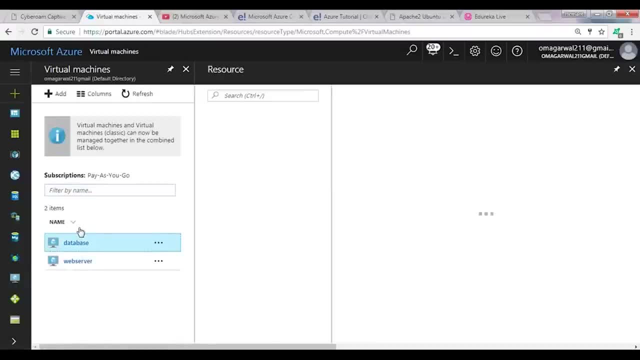 And that is it All right. So my web server is configured. now Let's go on and configure our MySQL now, All right. So MySQL is a bit tricky, guys, because there is a lot of configuration that you have to do. 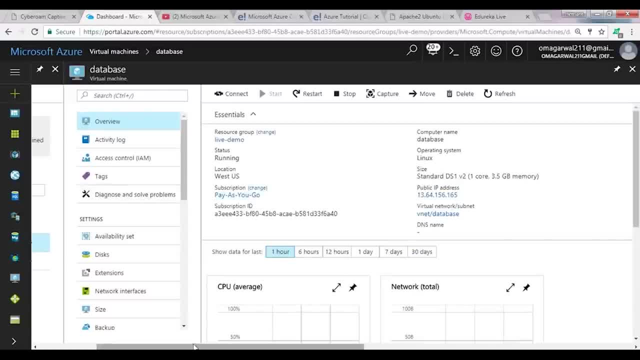 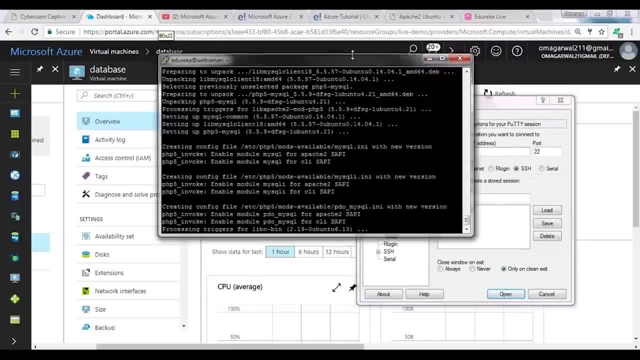 But let's hope for the best and see if we can connect to it. All right. Also, guys, if you would have noticed, I have not configured anything for my server, for my database server. So, as we did in web server, I'll show you. 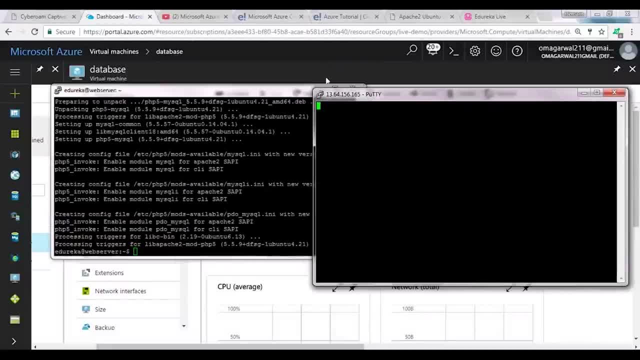 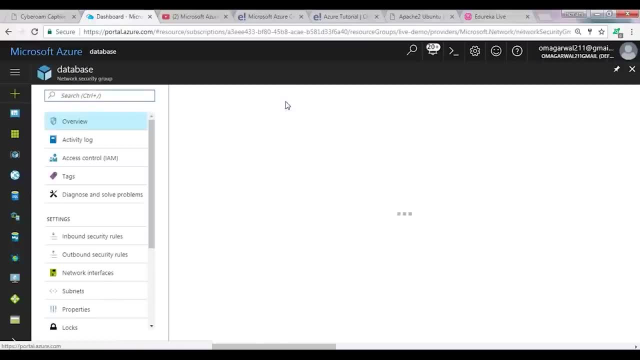 If you try to connect to it as of now, we'll not be able to. So while this is being loaded, let me quickly go to the properties of my database server Right And include the inbound security rules, according to what I want. 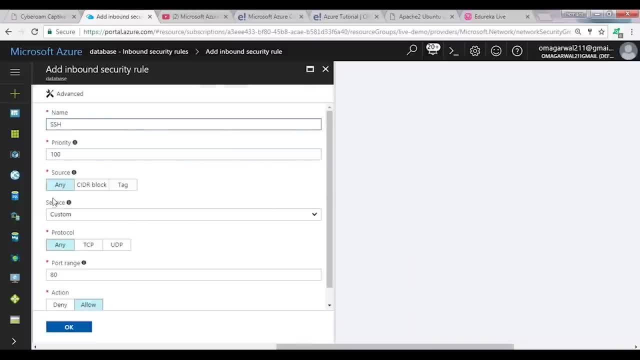 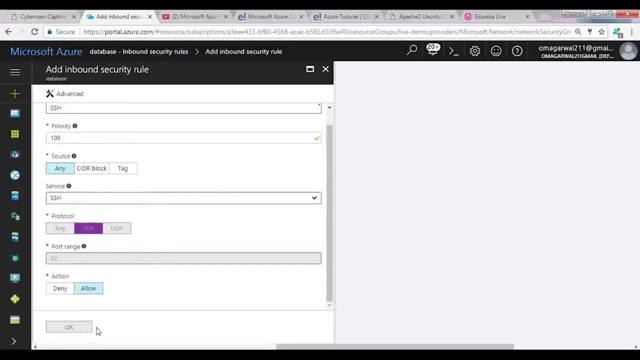 So I'll first have to enable the SSH rule Right. So this is how I'll be able to connect to my server. So I'll select the SSH service. The action is allow, I'll click on OK And my security rule will now be created. 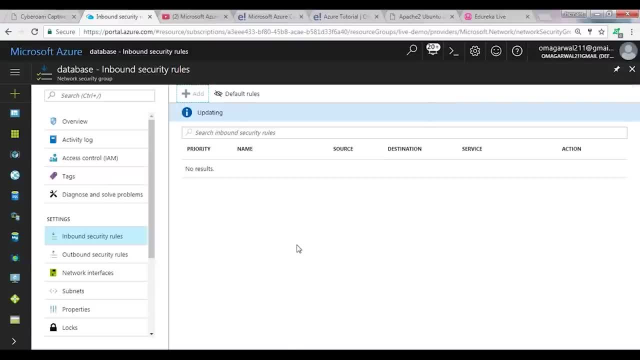 Also, I should also be able to create a MySQL connection to the server, because I want this server to be accessed through my computer. Right, For example, I'll be creating a database, I'll be adding the table Right, So I want to do all of that through my computer. 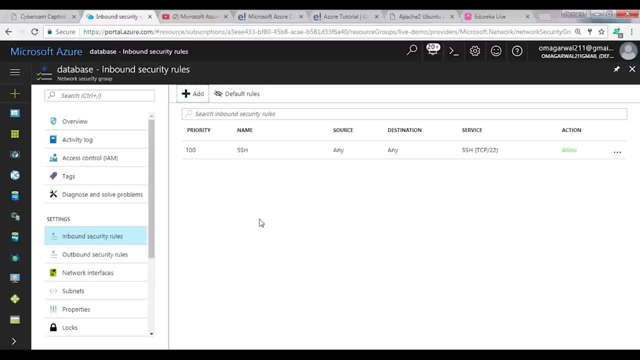 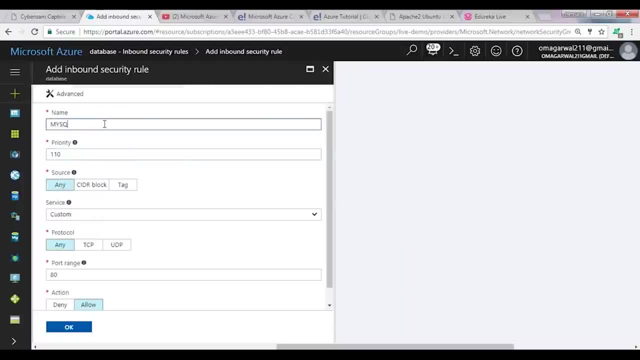 I don't want to SSH into the Ubuntu again to configure anything, So we'll be doing that. So we need a MySQL connection as well. So let's add that. So it would be MySQL And the service would be MySQL. Action is allow. 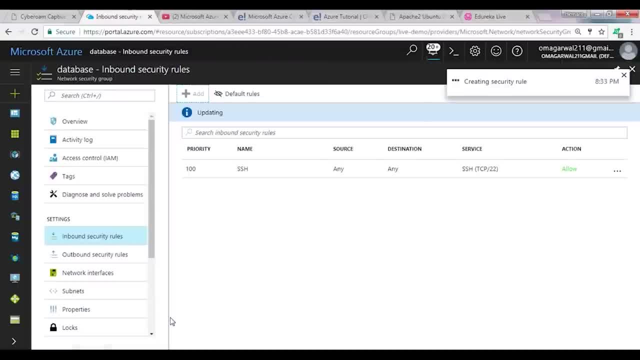 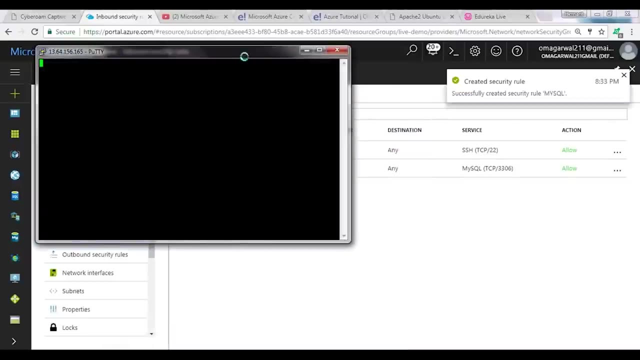 I'll click on OK. And this is it, guys. So now the security rule will be created And if we try now to connect to our database, So I'll be able to do so. So I'll copy the IP address, I'll click on open. 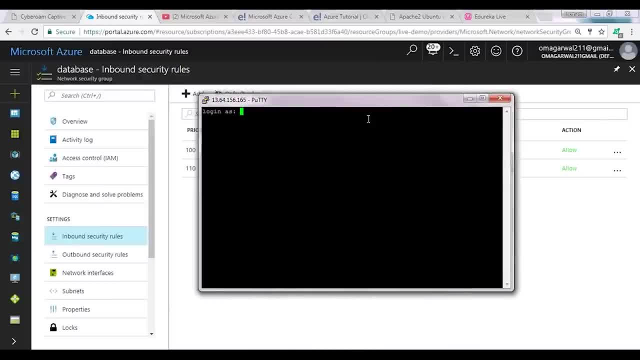 I'll say yes, And now it'll ask me for the login name. So, as you can see, the security rule worked. It is asking me for the login name and now the password. So I'll give the password for this And done. 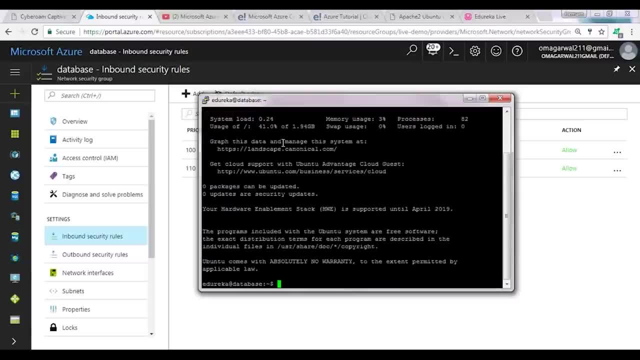 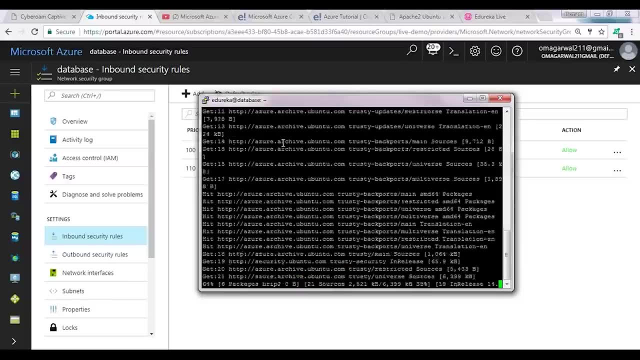 With this, I'll be authenticated to my Ubuntu server. First of all, I'll update this. So first of all I'll update this machine with the update command, Like we did in the previous server as well. So now it will be updated. 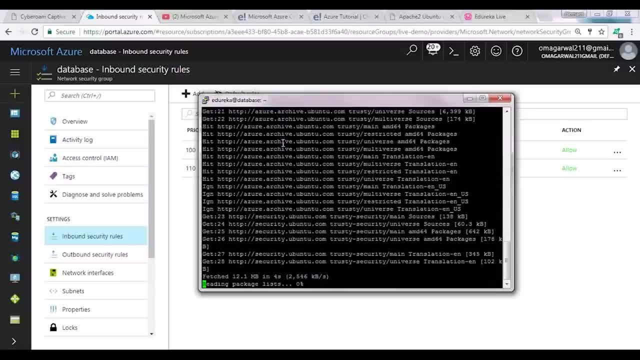 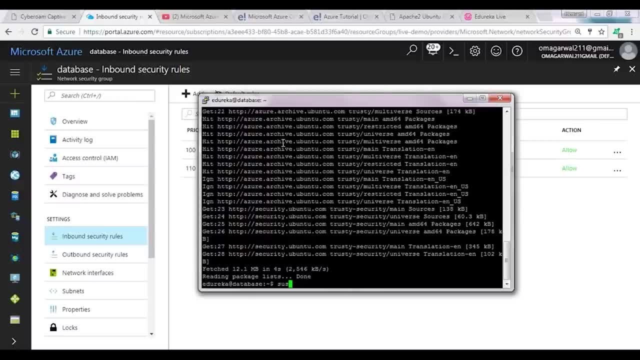 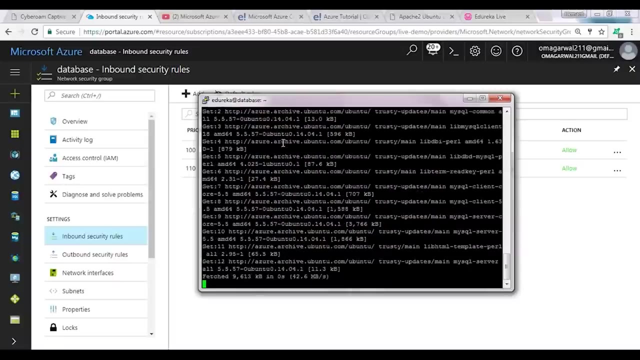 After this, I'll install the MySQL service that we'll be using to connect our website from. So I'll now install the MySQL service, which is sudo, apt-get. install mysql-server. Right, This is it. I'll type in y, which means yes. 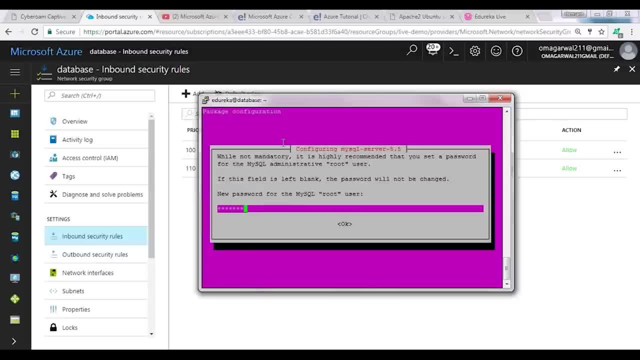 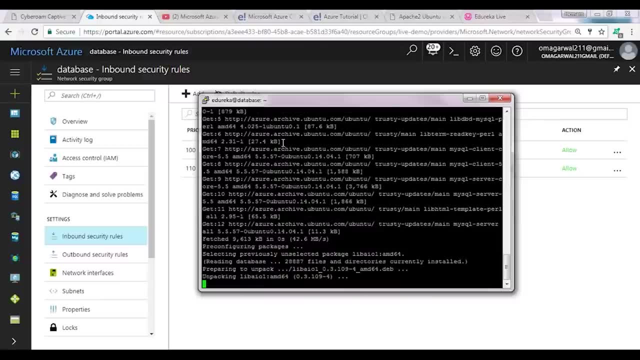 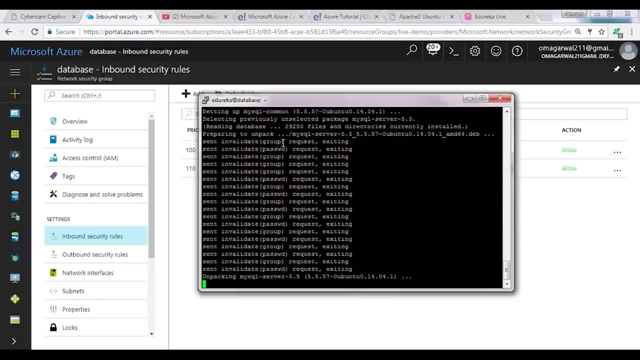 And now it'll ask me for the password. I'll type in the password and confirm it again, Hit enter And that is it Okay. So now I've configured MySQL. I've installed MySQL on my system. The next thing is: by default, MySQL only allows the local host to access the root user. 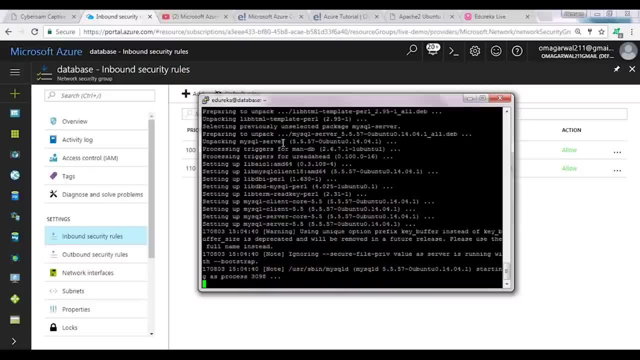 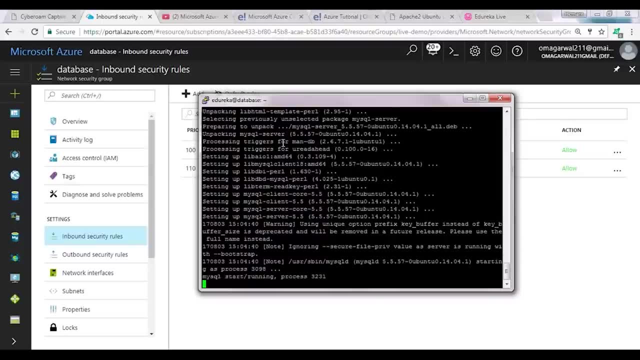 Right, If I want to connect to my machine, I have to create one more user for MySQL for me to access it. Right? So once my MySQL is installed, I'll show you what I mean. Right? So we'll be doing that. 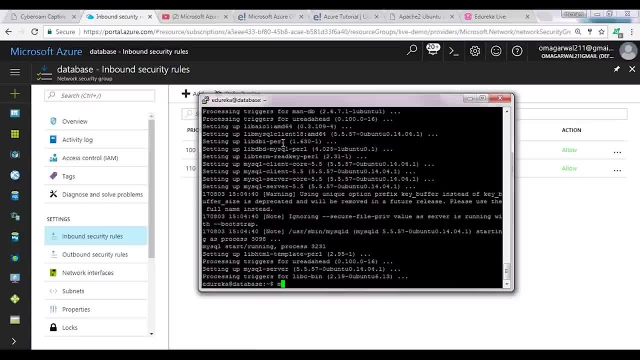 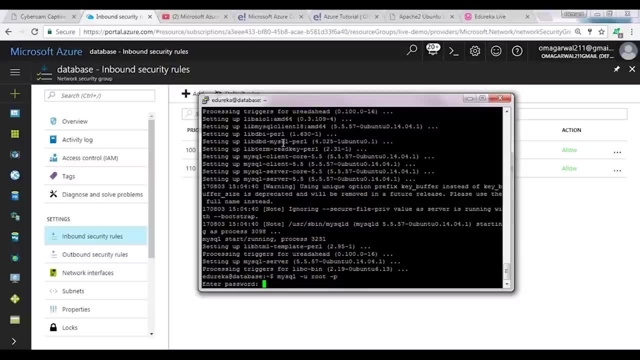 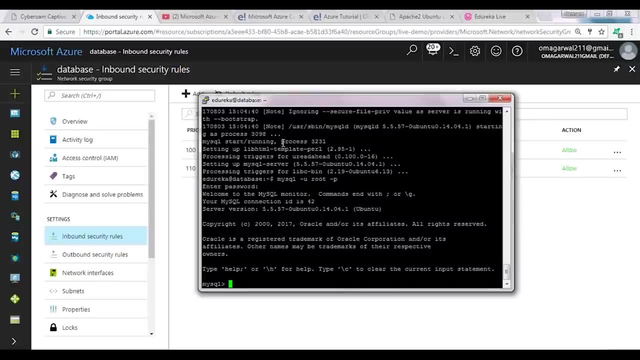 And I think we're done. Yeah, So we're done. So let's connect to our MySQL service now. So the user is root And the password was edureka123 to connect to my database, And we are in. So, like I was saying, we have to create a user that we'll be accessing from. 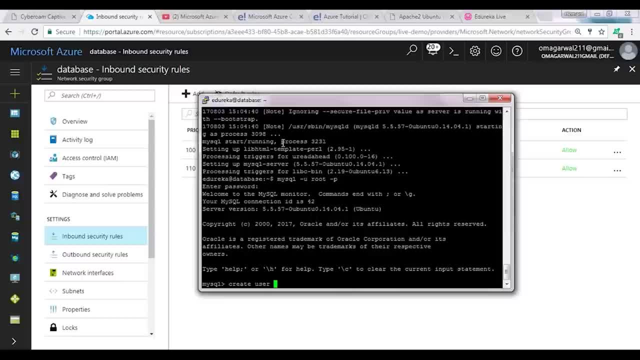 So let's create a user for MySQL. So I type in create user. Say the username is edureka for my database. Where is it? It is on localhost And I should add the password for it. Let me add the password as edureka123. 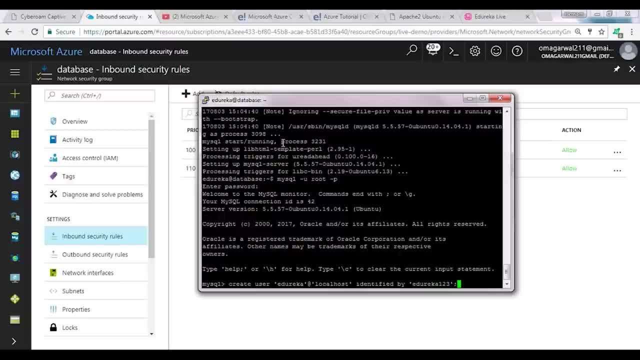 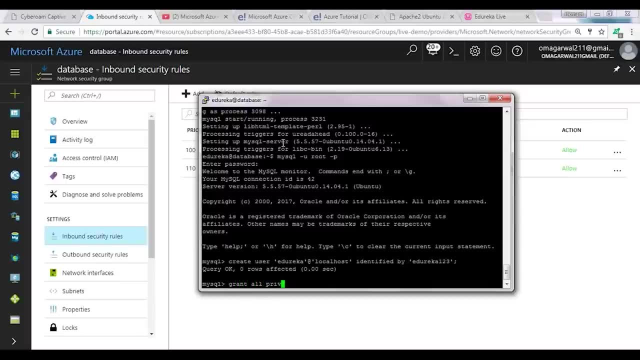 Right And let me deploy this server. So I've created the username. Now I'll have to grant all the privileges to this particular server. So let me give this, Let me give the command for that, So it's grant all privileges on everything that is there on this database to this particular. 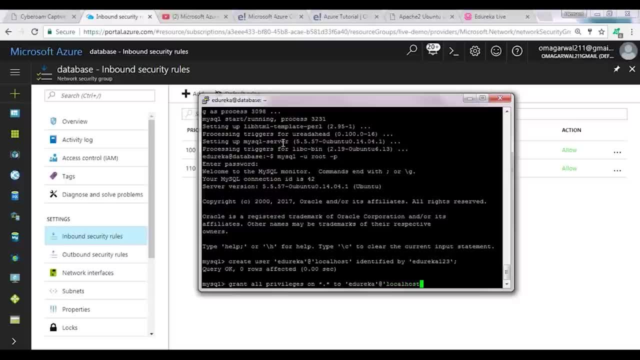 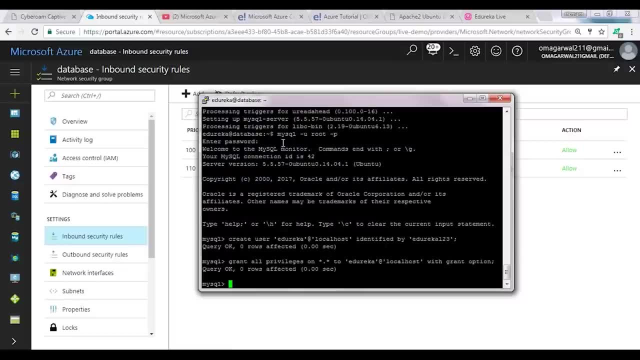 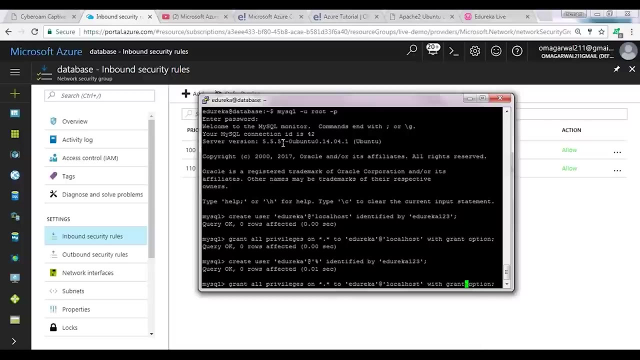 username which resides on localhost. So this is a command that we'll be configuring, All right. Now, same set: we'll be configuring for the percentage Host. So let us do that as well, All right, And then grant all the privileges for the same. 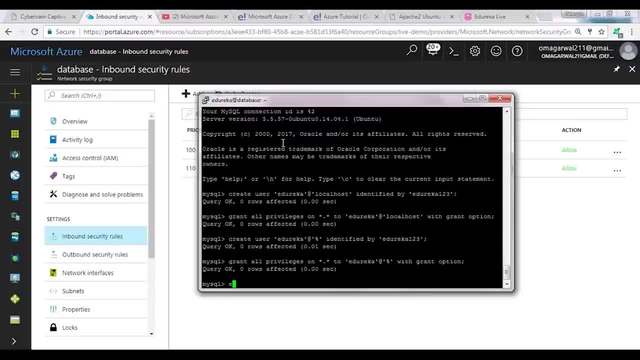 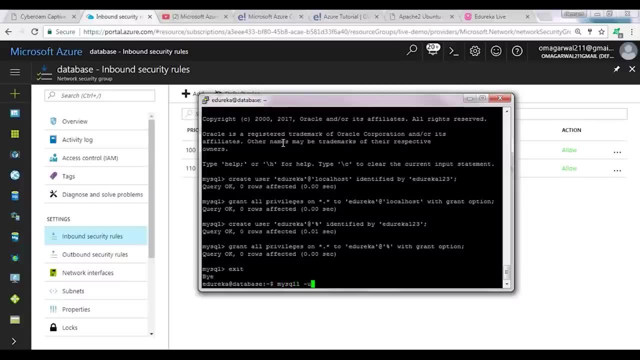 All right, So done. So we have created successfully a new user. Now, if I try to connect to this database using this user, let's see how we can do that, So I'll type in MySQL. So previously I authenticated myself using root. 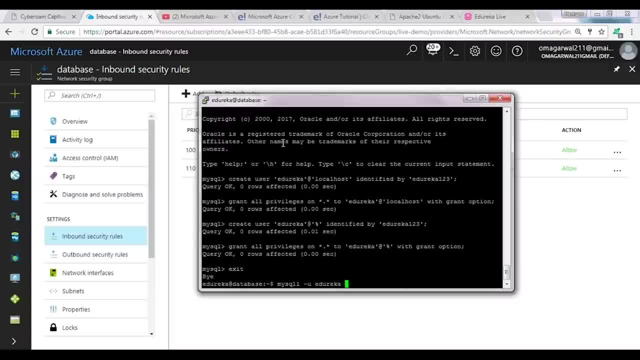 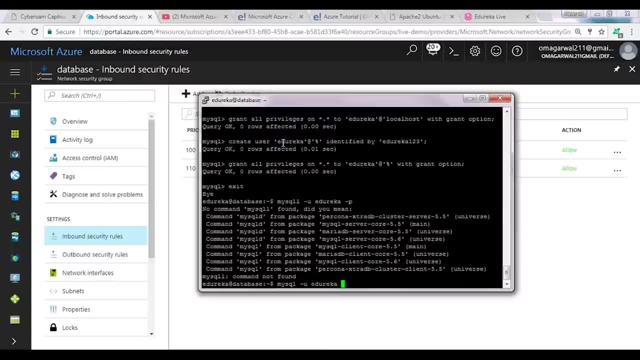 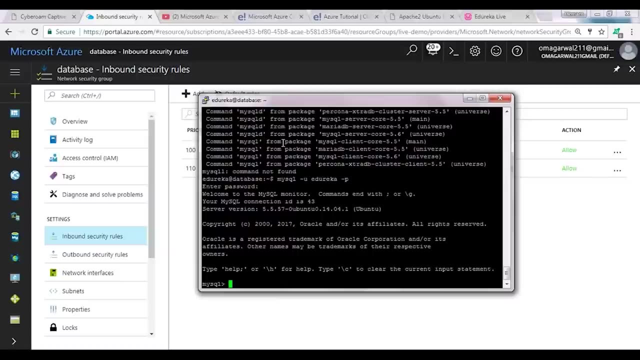 But now I'll use the edureka username And see if I can connect to it. Sorry, I misspelled it, So it's edureka-p. And now the password. So, as you can see, I can authenticate through, All right. 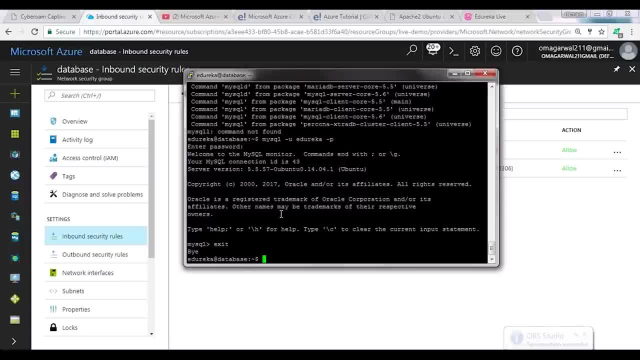 Sorry for that glitch, All right, So now what we'll be doing is like I was saying. so we have to configure one more file for our MySQL to get configured. All right, So for that let us go to our directory, that is, etc. 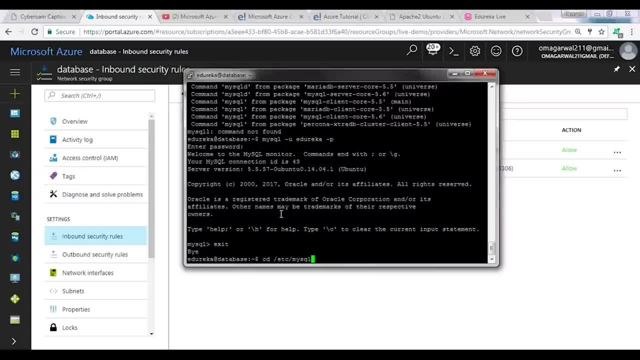 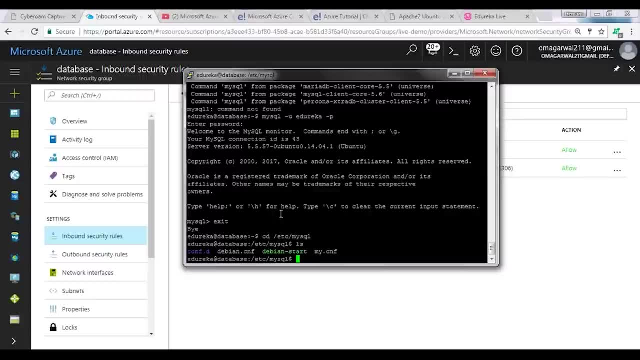 And in that MySQL, All right. And now in this particular directory I have a file called mycns. So this is a configuration file that I'll have to configure for connecting to my MySQL, So I'll sudo nano into it. 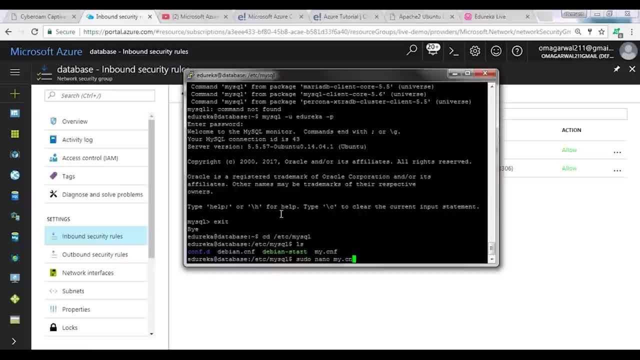 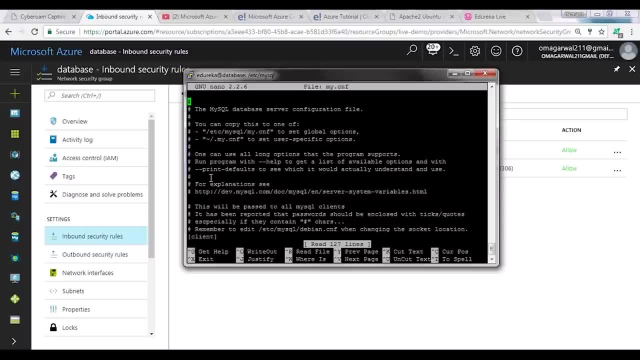 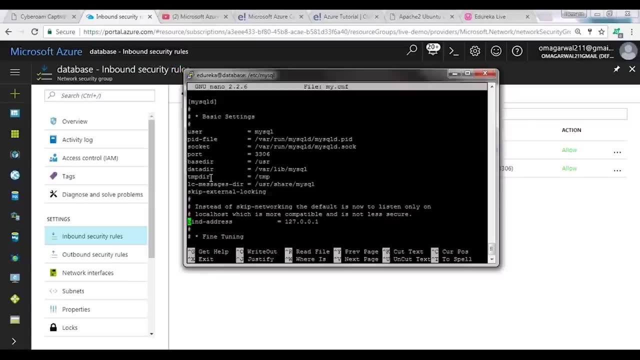 And then I will get To this particular statement which says bind address. So this bind address statement basically says that only localhost connections are allowed to my MySQL Right. So I'll have to comment this part out And then I'll save it. 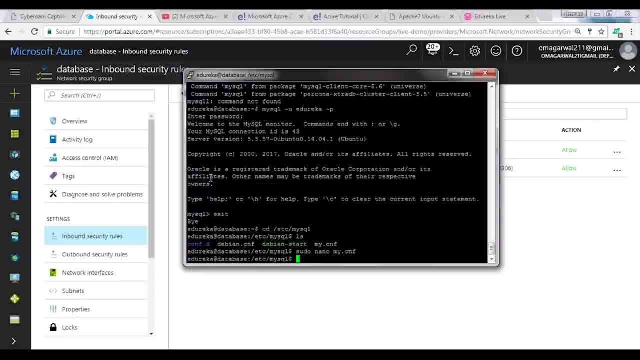 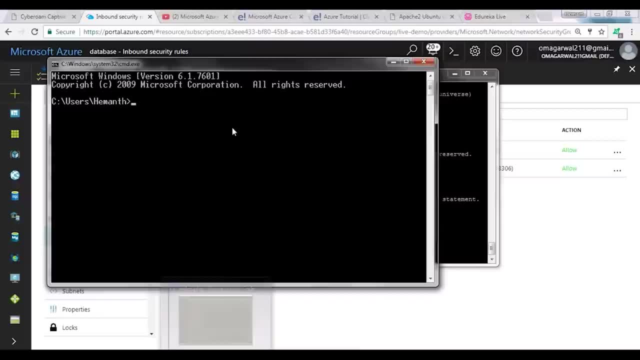 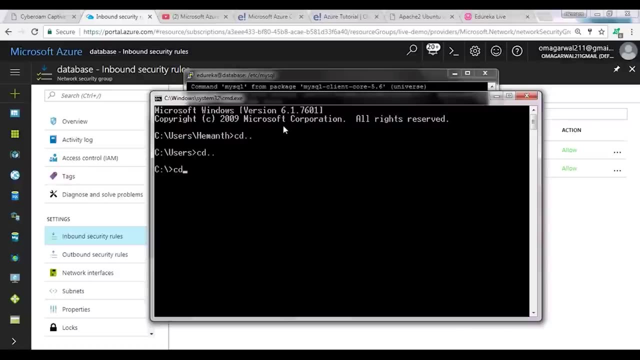 And that is it, guys. So this was the last setting that I had to do. Now, if I try connecting it through my computer, I'll be able to connect to this particular MySQL instance. So how to do that? First, I have to go to my MySQL installation folder, which is somewhere here. 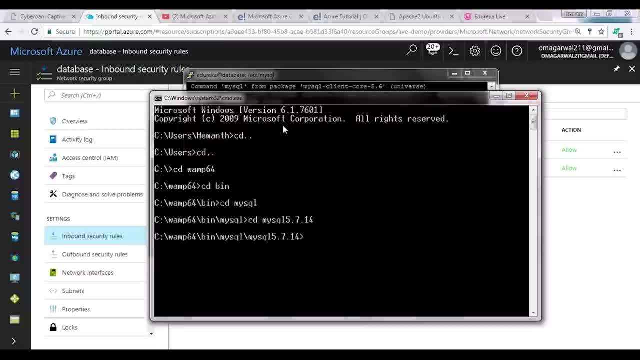 Right, So let me quickly go to my folder. So this is the folder where MySQL resides. So now I'll connect it using this particular command Which says MySQL, hyphen H. Now I'll paste in the IP address The username, which is edureka. 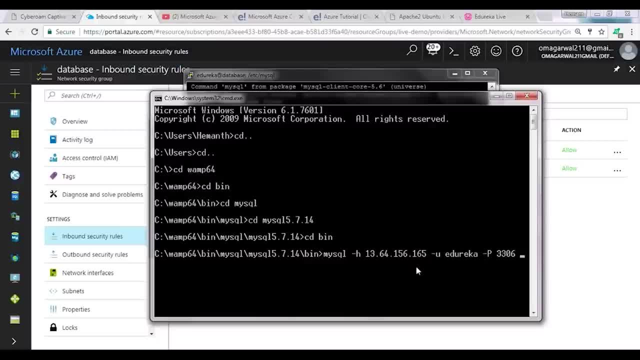 The port number, which is 3306.. And then the password. It'll ask me for the password, So the password is edureka123.. Now, mind you guys, it will not connect right now. It'll give me an error that it can't connect to MySQL service. 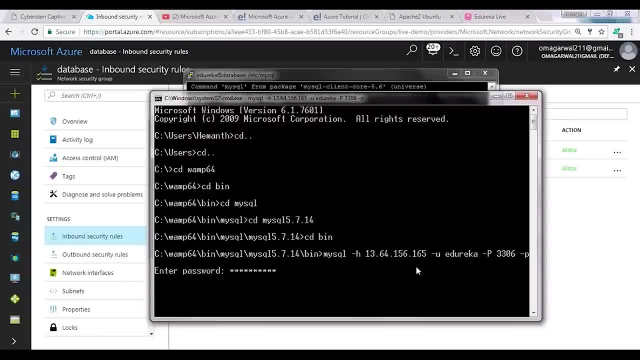 And the reason for that is that we have configured everything after the MySQL service started on my server, So now I'll have to restart my server to connect to it Right. So it'll take some time and then it'll throw an error that it can't connect to the particular. 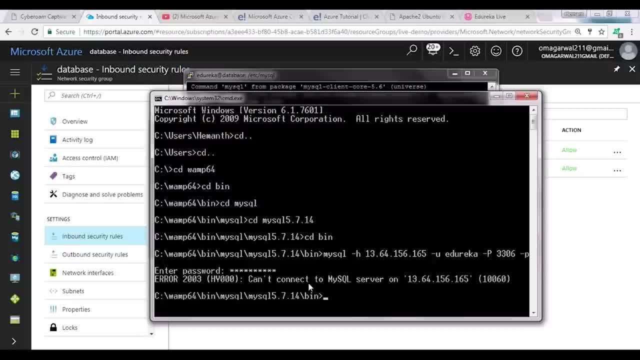 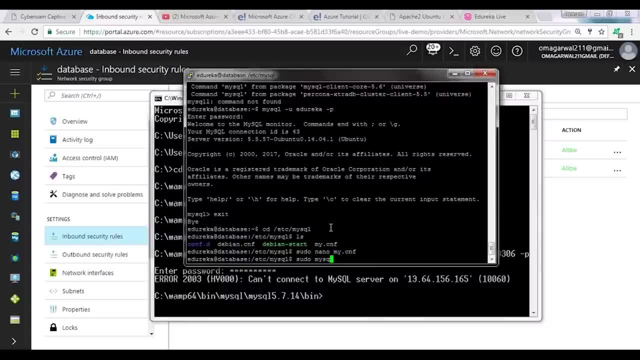 MySQL server, Right, So, as you can see. So for now connecting to it, we will have to restart the service. So let me restart it by typing in sudo service MySQL restart. All right, So with this command, my MySQL will get restarted. 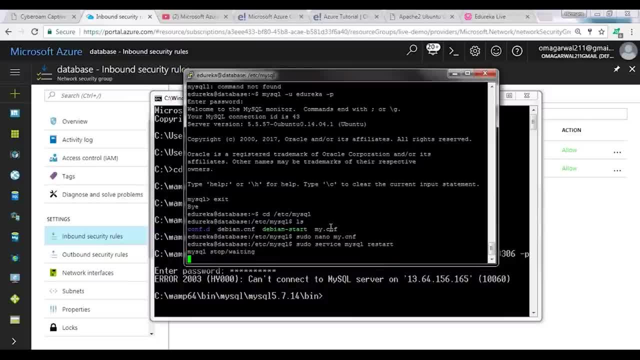 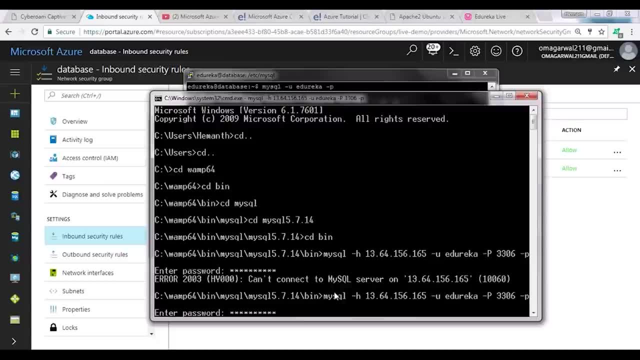 So let's see. So my MySQL has stopped and now it has restarted, And now if I try to connect to my MySQL server, I'll be get. Yes, So I have it on my computer. Now I'm able to connect to my MySQL server. 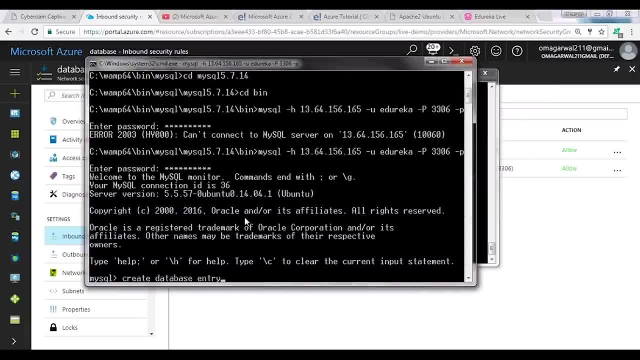 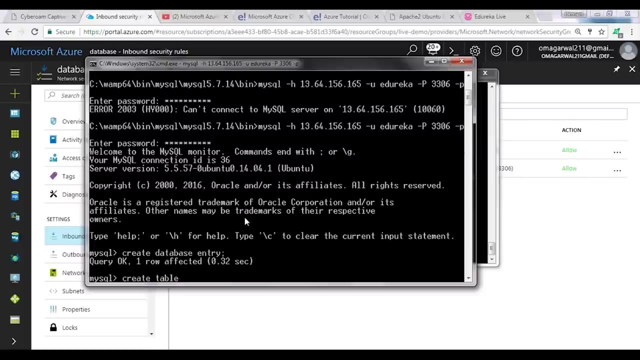 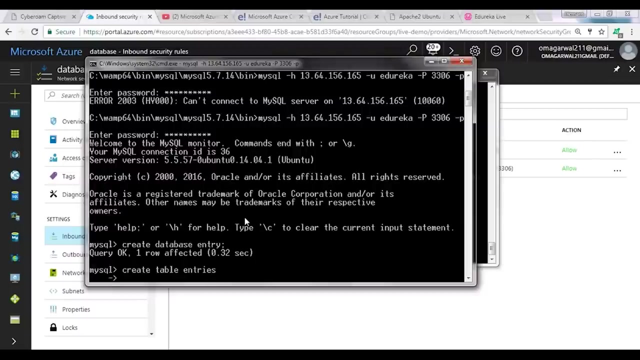 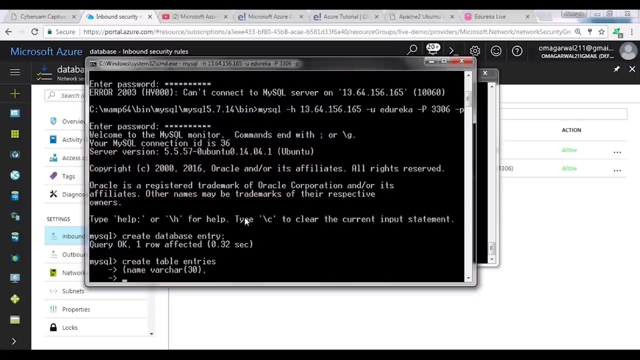 Let's quickly create a database for my website, which says create database entry. So I'll quickly create a database and I'll create a table for this Right, Which is create table entries. I'll give the name Yes, And then the second entry is email address. 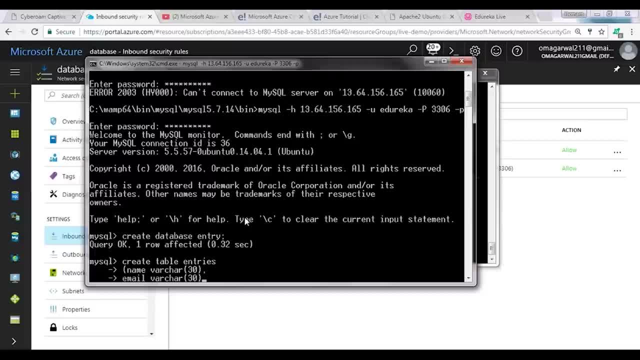 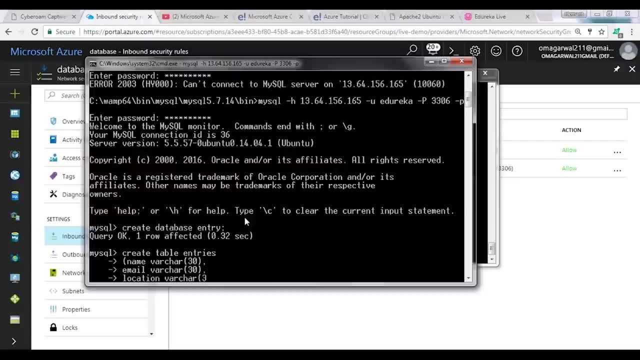 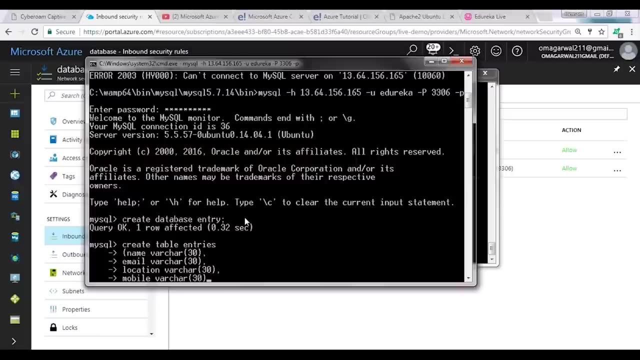 So that is varchar30.. Right, And then the location, which is again varchar30.. And then my mobile number, which I'll be feeding here. All right, So I think the net is giving some problems. All right, So I didn't select the database. 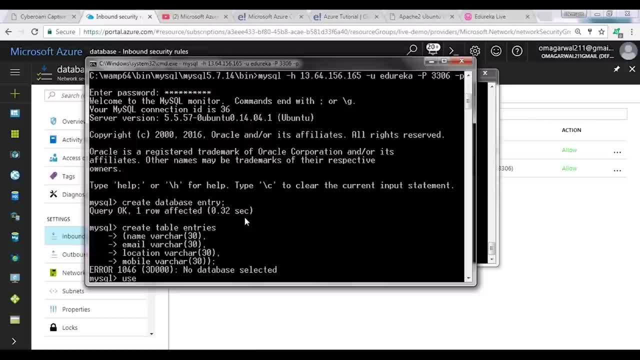 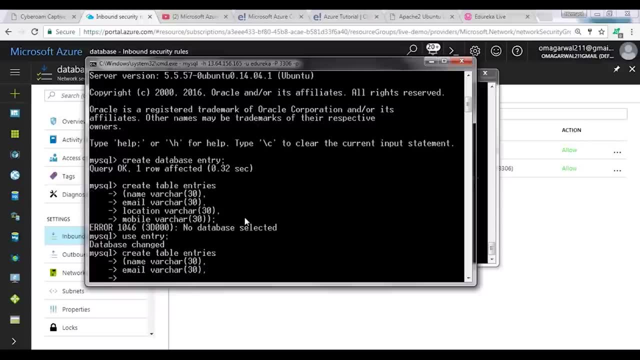 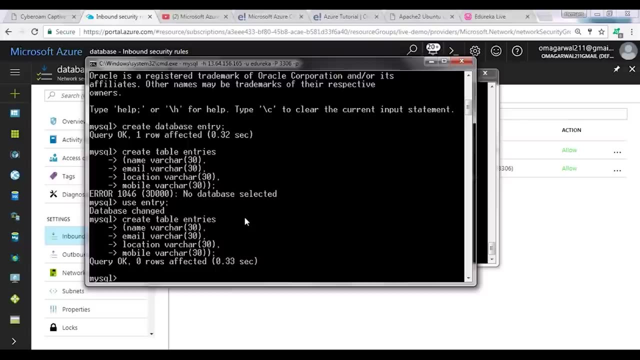 So use entry, And then I'll create the table. So, guys, there is some problem with our internet connection. I think it is residing on your end as well, So what we'll do is we'll continue this session in our next video. 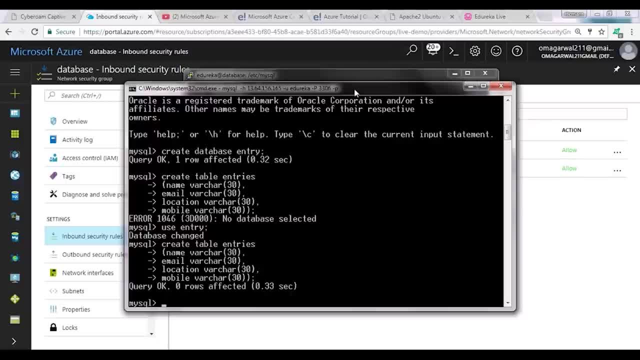 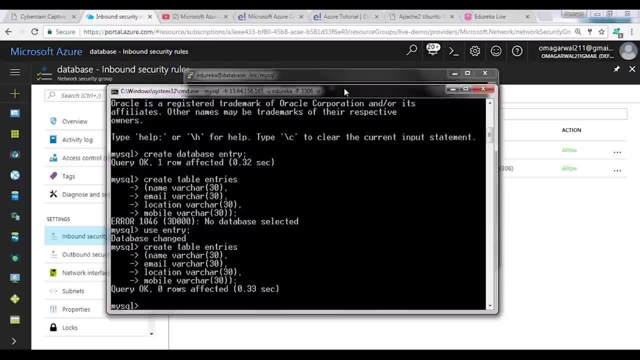 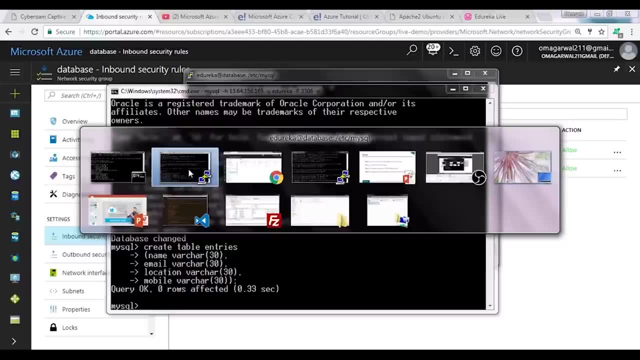 So we have created the database Now. next is creating a web server Now. next is creating a web server Now. next is creating a web server. that we'll do in our next session. So let me quickly come back to my slide, which is here. 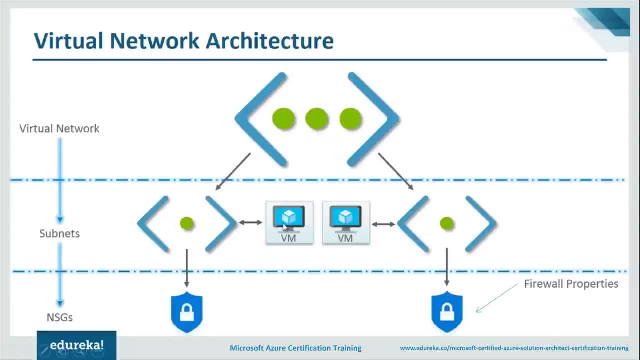 So we have created a VM for the web server. we have created a VM for database. we have configured a database. we can connect to a database to our computer. all that is left is configuring the web server. So we'll do that in the next section and I'll show you how you can configure the properties. 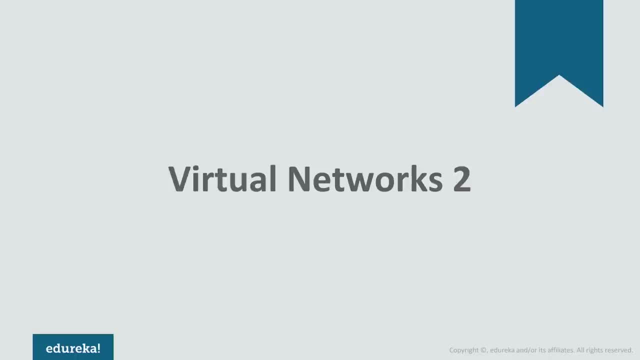 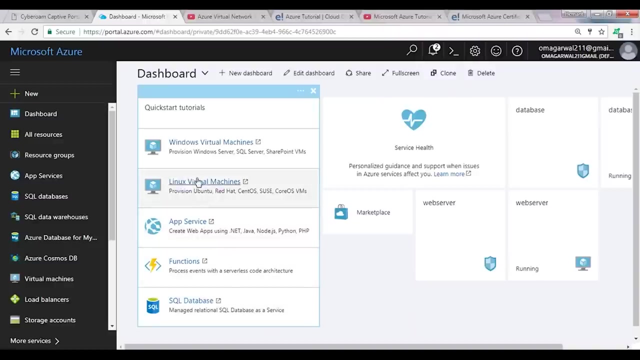 for it. Today, in this session, I will show you, guys, how you can configure the web server. Alright, so let me quickly go to my Azure dashboard. Alright, guys, so this is my Azure dashboard And, for those of you who are new, I will show you how you can deploy a virtual machine. 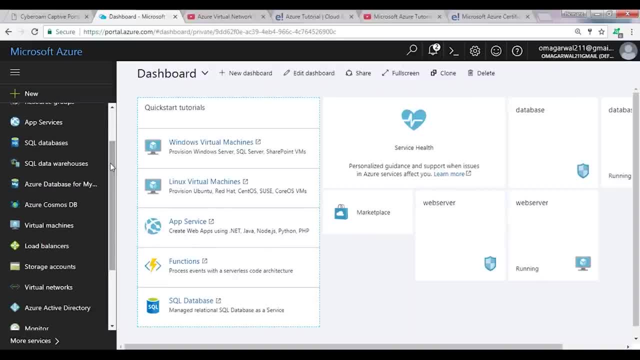 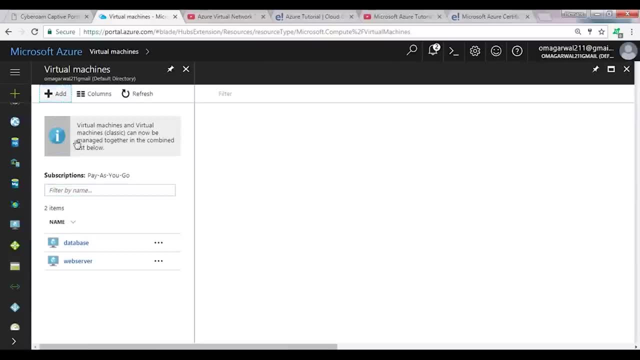 I've already deployed one, But let me quickly show you how you can deploy another virtual machine. So in the, in the dashboard, you will go to virtual machines, you will click on add and then you can give the nerve, the. you have to choose an operating system. you'll choose. 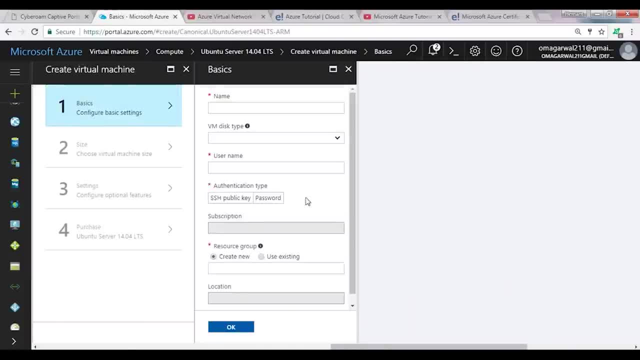 the operating system. you will click on Create And then you'll have the screen where you can fill all the information right. Once you fill in all the information, you just have to click on OK And in the last part it will ask you to agree to the terms and conditions. you can do that. 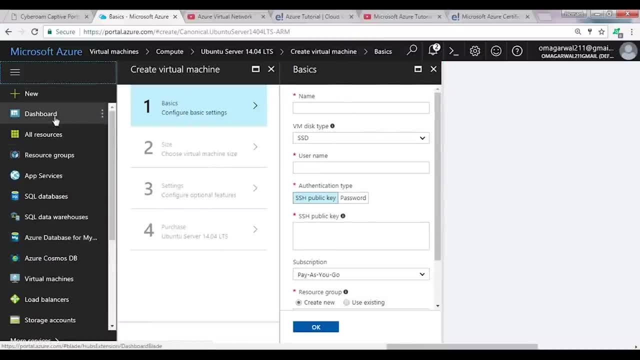 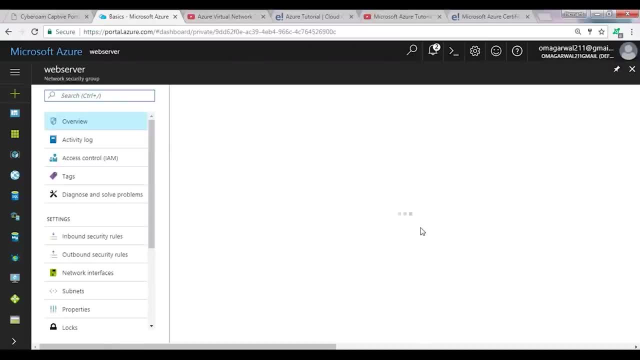 and your virtual machine will be deployed. Alright, So I've already deployed one virtual machine. that is for my web server. Now in the web server you can see these are the properties that I have attached to my web server. So this is basically my network security group for my web server. 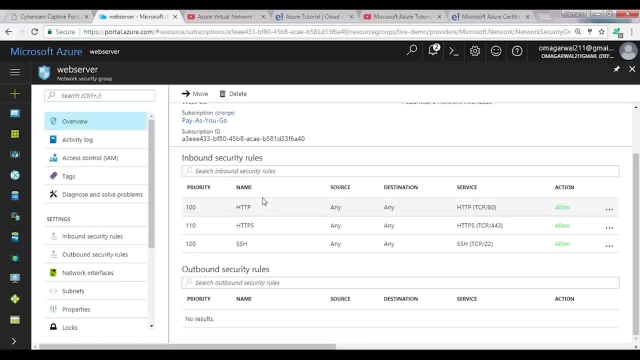 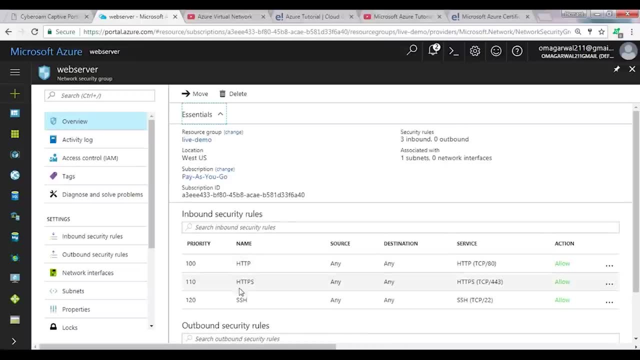 In this. I've configured that my web server can. we should have HTTP connections. it should have HTTPS connections and an SSH connection right Now. if I want to add more properties to it, I can add by clicking here that, as that is inbound security rules. 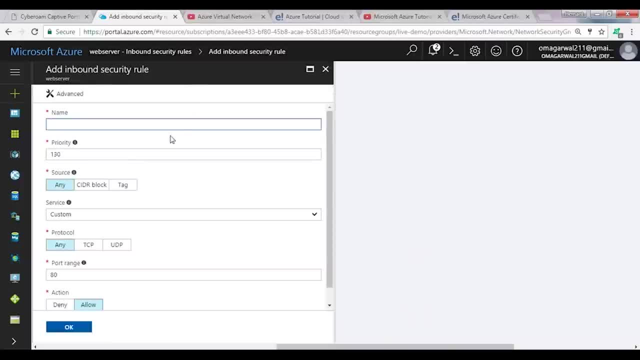 I'll go here, I'll click on Add And then I can add any property that I want from this list that is available here, right? So I've already added the properties. Now what I'll do is I'll SSH into my web server and see how we can configure it. 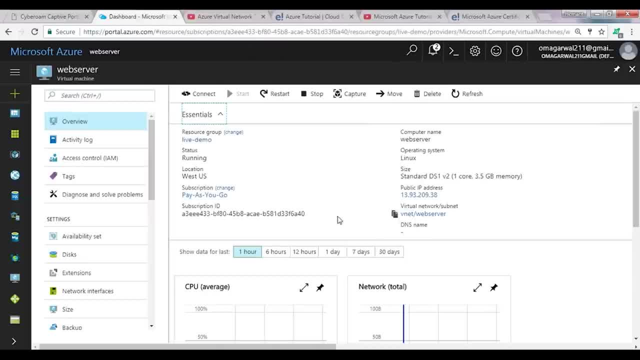 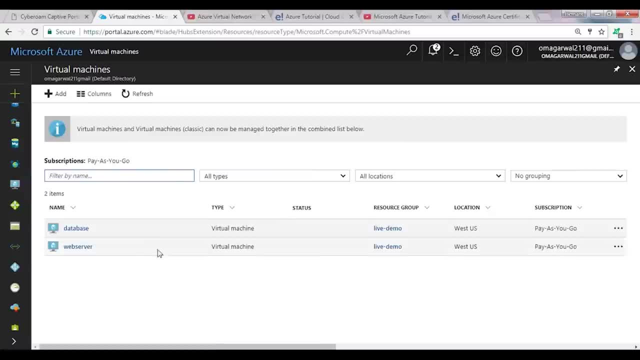 Alright, so this is my web server page. So I've just gone to virtual. So if you go here in the virtual machines tab, you will find all the virtual machines that are deployed over here. I selected my web server And then I reached this page. 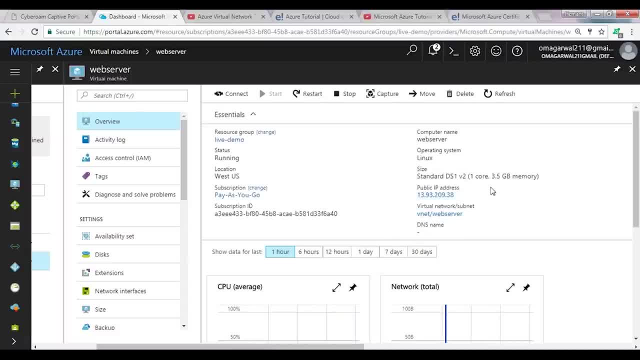 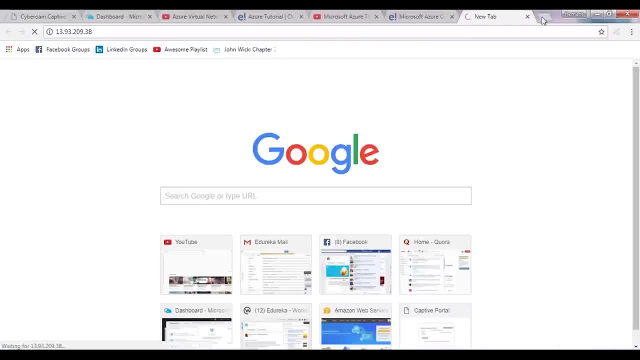 Now I need the IP address of my virtual machine to connect to right. So as of now, if I copy this IP address and paste it here, you can see I cannot connect to my virtual machine as of now because there is nothing installed on this web server. 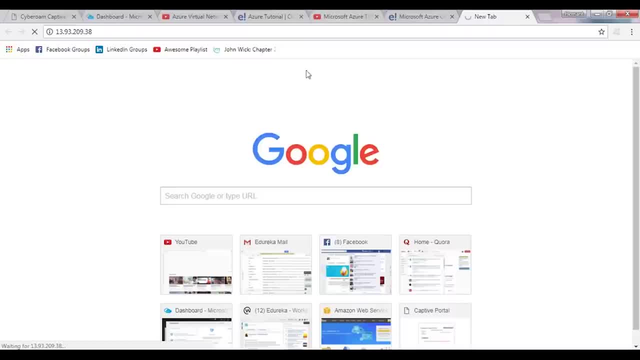 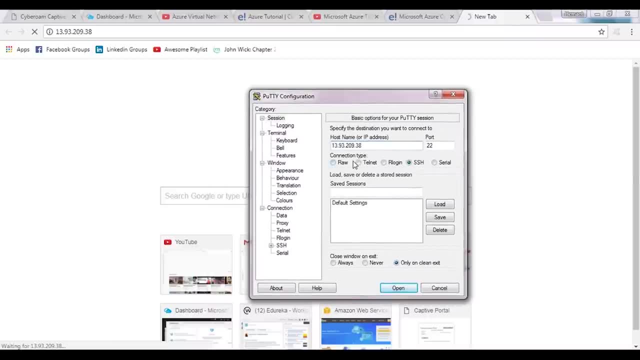 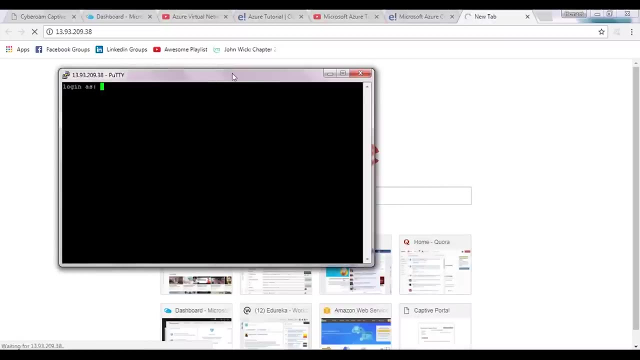 So what we'll be doing now is we'll be installing the necessary softwares for my virtual machine to work Alright. So I will enter the IP address here And I'll click on open And it'll ask me the login name. So I'll give the login name that I've configured, that is, idreca. 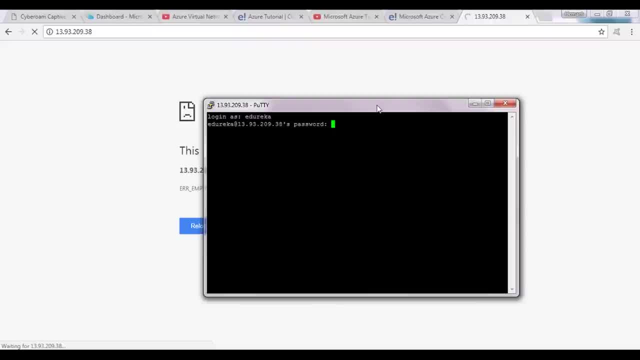 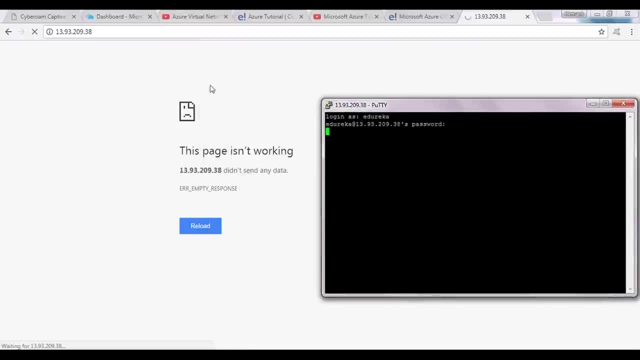 Now it'll ask me the password, So I'll enter the password. that is this. And while it is connecting, let me show you that, as you can see, the page is not working as of now, So we will install the necessary softwares here and then we'll try again to connect. 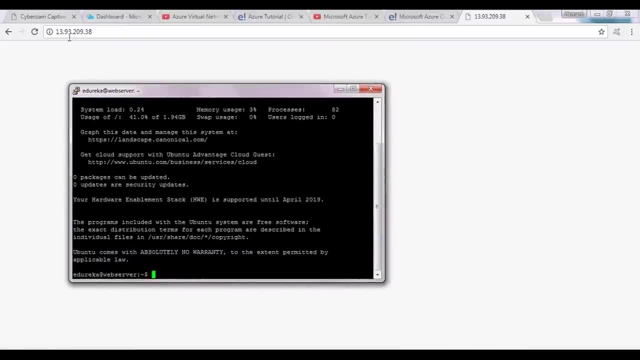 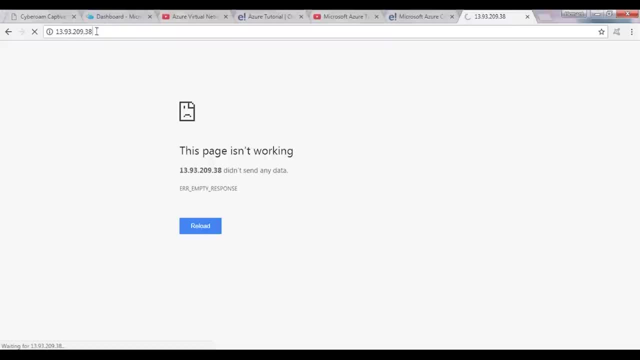 So if you guys want, You can actually connect to this website. The IP address is 13.93.209.38, right, So my team here, they will put it in the comment box for you to access. You can go to this IP address and you can see that as of now, we cannot connect to this. 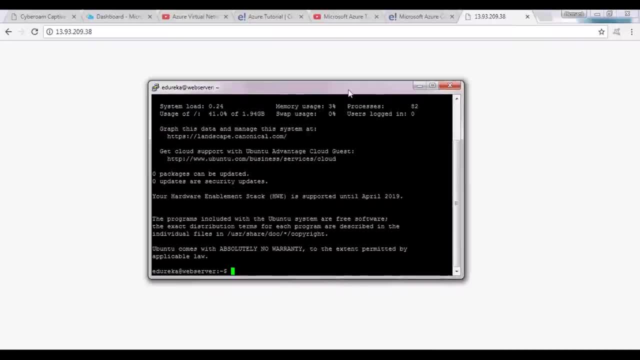 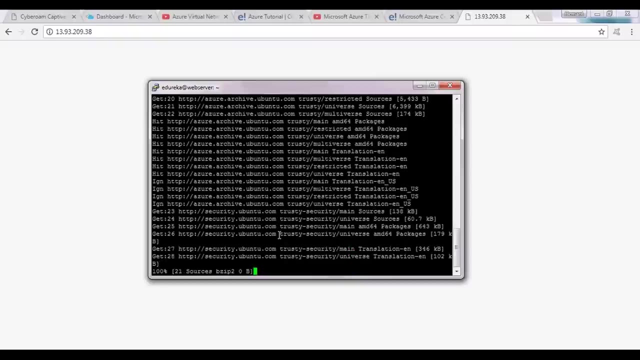 particular website. Alright, So now. so this is the Ubuntu machine. This is my server. I will install the necessary software, So I'll sudo, update it first. Alright, So now Okay, Let's go. Alright, So my updation is being happening, and now I will install the PHP software. 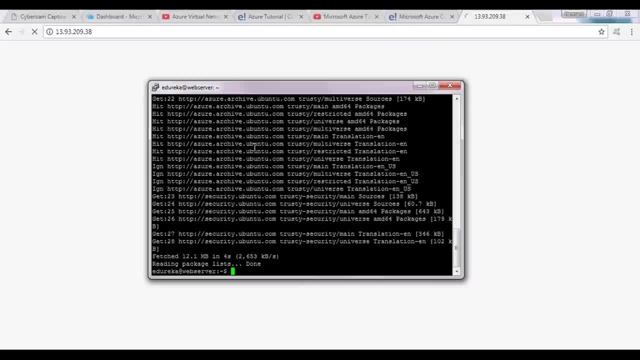 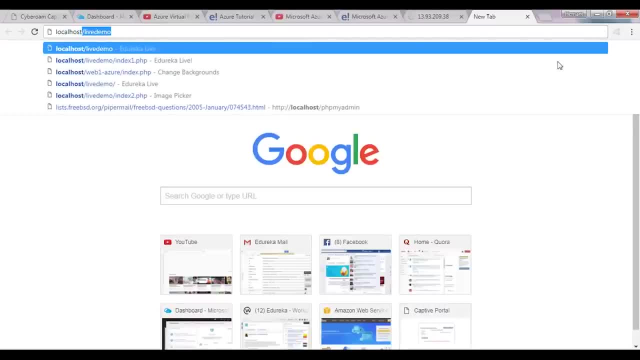 So my website for that I want to deploy on this particular server. Let me quickly show you the website that I want to deploy. So it's hosted on my local host as of now. right, So let me go to my website. So here it is. 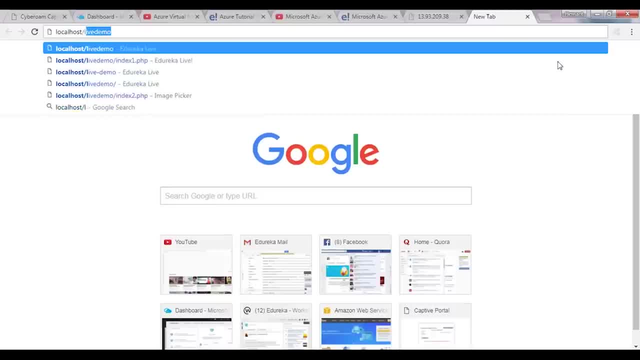 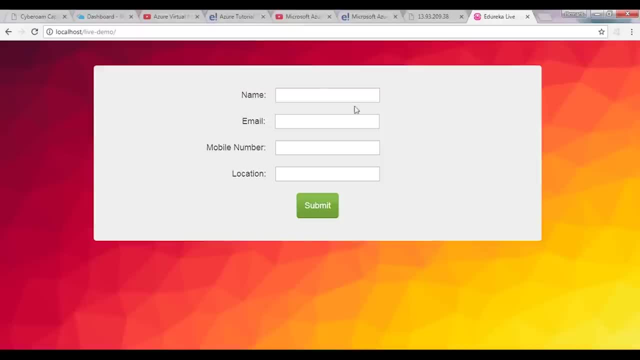 Alright, So this is my website, guys. I'll enter a name, an email address, a mobile number and a location, I'll click on submit and it will enter all these values into the MySQL database that we created yesterday. Alright, So I'll show you how the values that will be reflected in the MySQL. 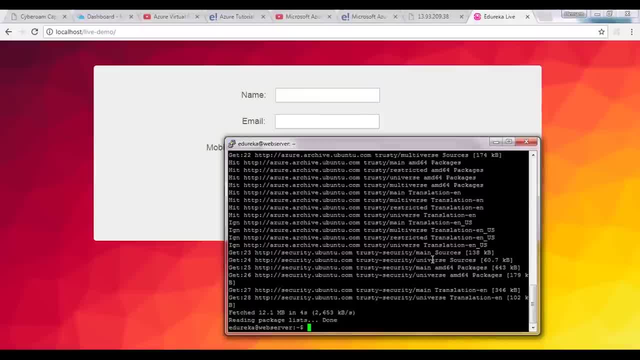 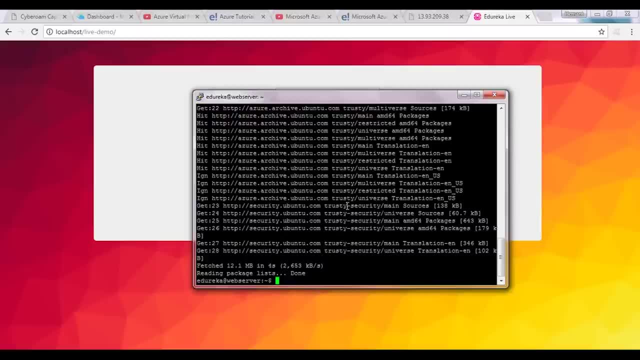 But for now let's configure our web server first. So this is the MySQL database. So this is the website that I'll be uploading to my web server. But first I have to install the necessary software. So this is the PHP website, guys. 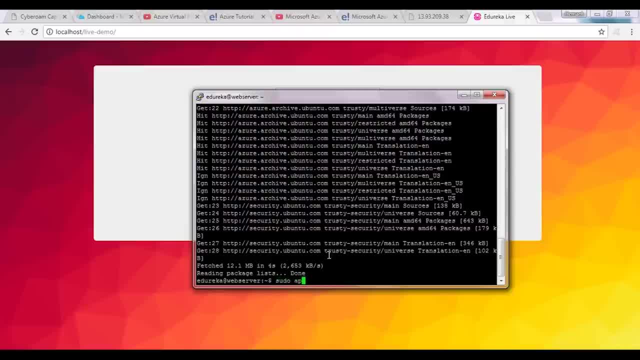 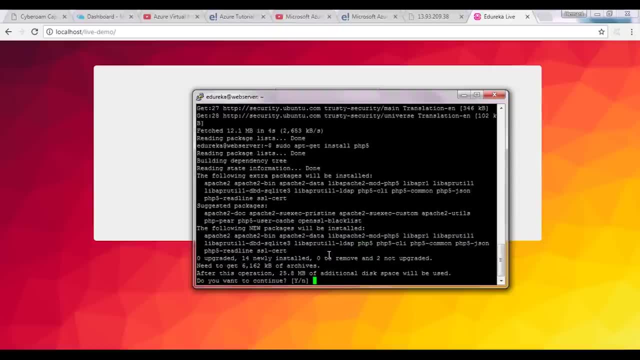 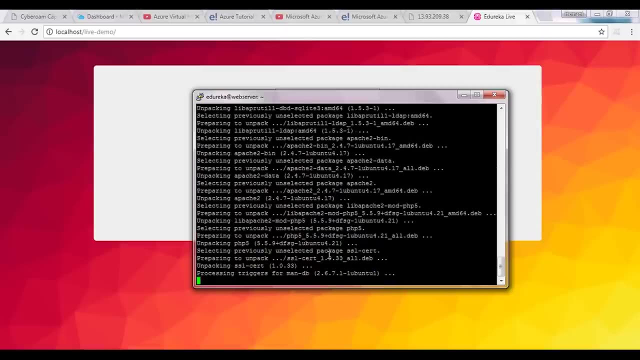 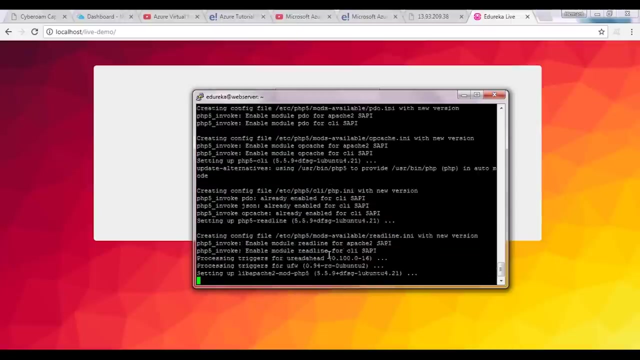 So I'll install the PHP software now. So I'll sudo: install the PHP. Alright, So it will install the PHP now And then we can go ahead. Now, since my website has to interact to MySQL, Okay, I also have to install an extension for my MySQL to work. 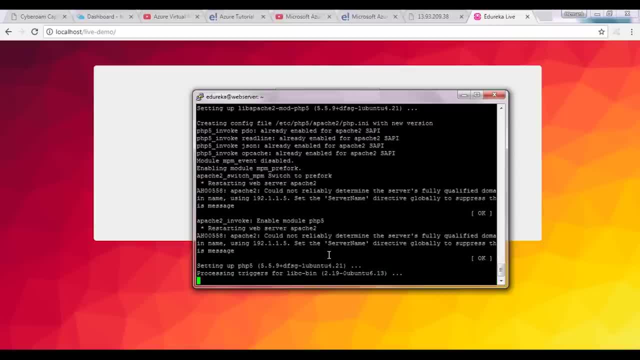 So I'll do that as well once this is done. So yeah, So my PHP is installed. Now I'll install the extension for my PHP MySQL. So to do that, I'll sudo: install the PHP extension, which is this: Alright, So you can see that my PHP now is intending to run on the iPhone as well. 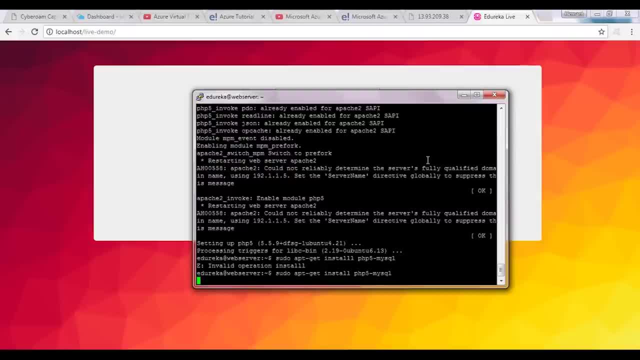 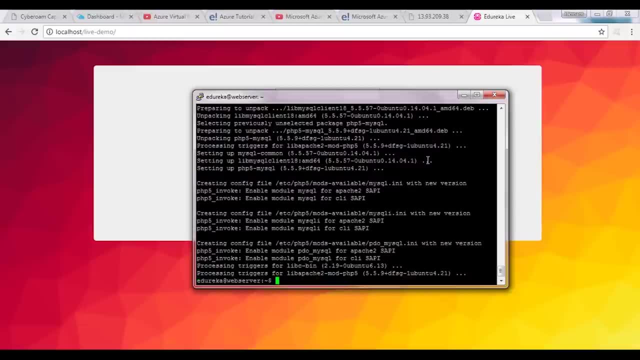 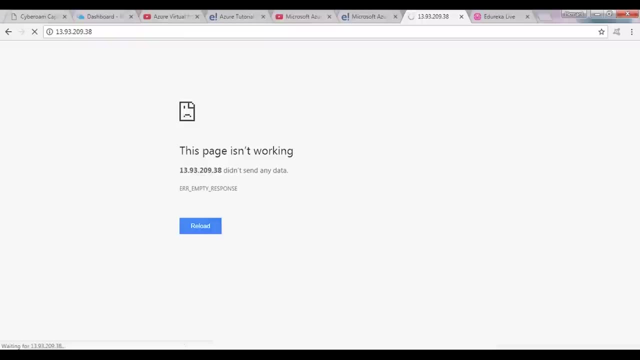 So I just have to install the Apache server. and let's say, let me say so, So mySpell won't work, My unearthing is not working, So I have to install the Apache server. So let's install the Apache server. So let's see what this is now. 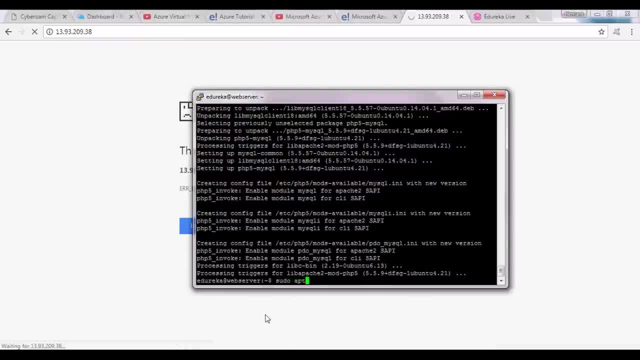 So let's say: let's install the Apache server. So let's say: you have all thisじゃあ You have to install the Apache server. So let us install the Apache server. So, like I said, as of now we cannot connect to it. 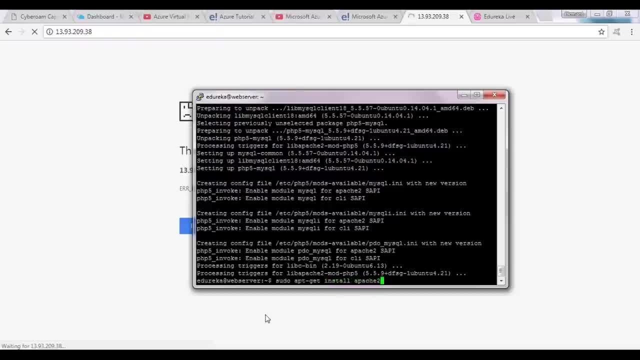 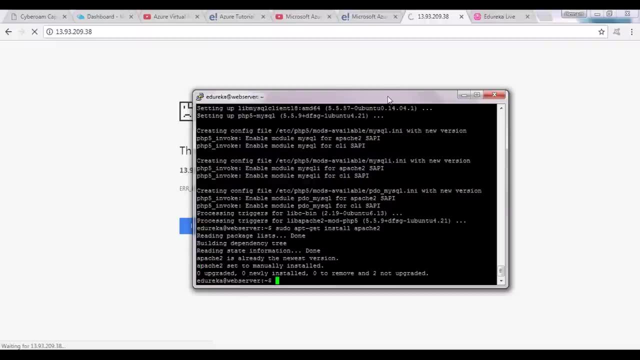 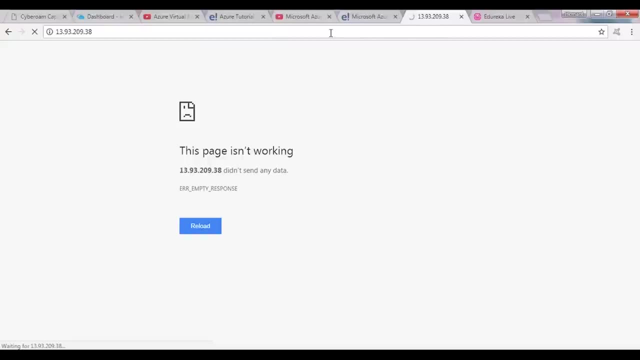 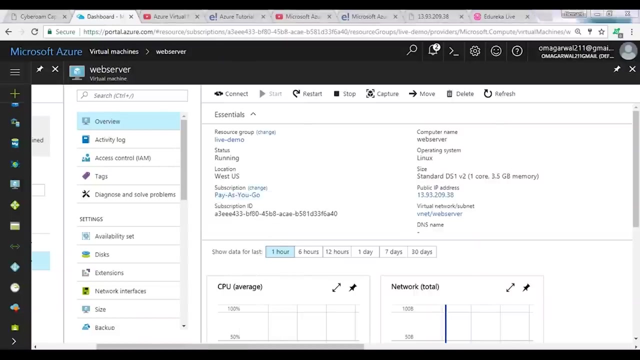 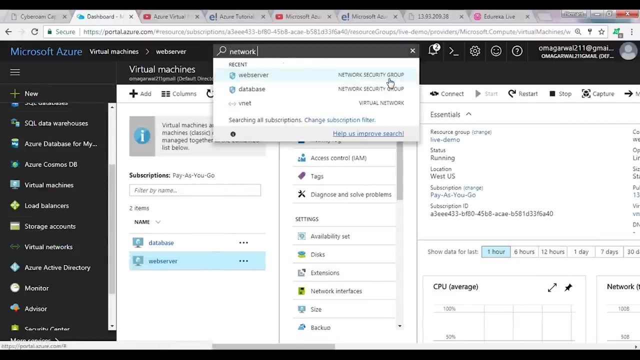 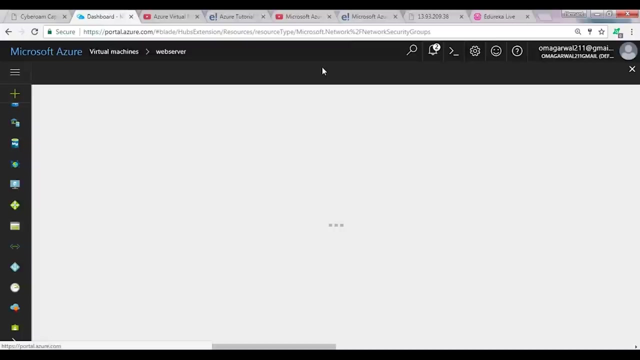 install Apache. all right, so now, if I try to connect to my website, I'll be able to do so. so let me quickly check my network security settings. so I'll go here, I'll type in network security groups and that will list me all the network security groups which are present as of now. all right, so I 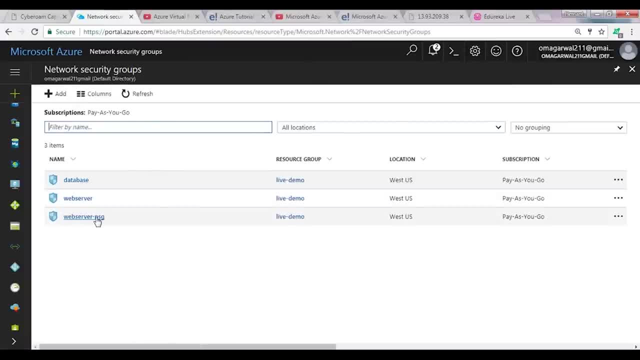 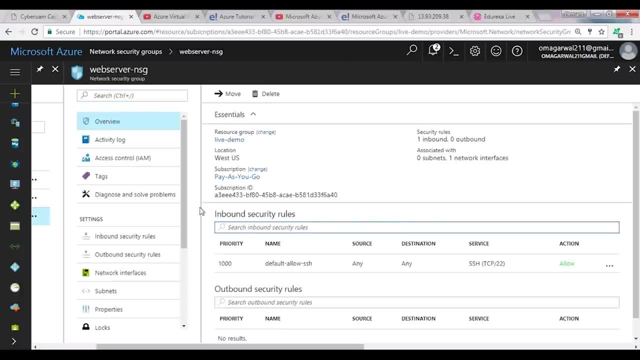 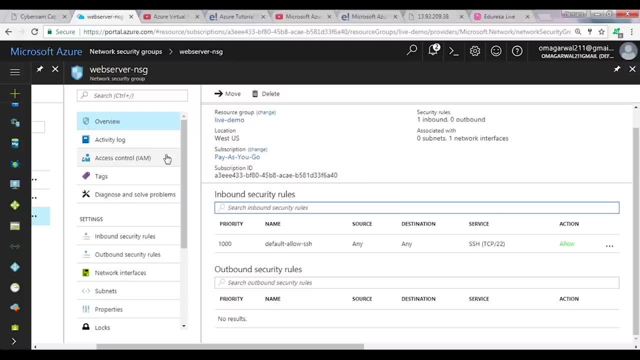 have two network security groups. this is the new web server network security group that I have configured. so I'll go here and as of now you can see, only the SSH rule is there. so what I'll do now is I'll install the Apaches. I'll 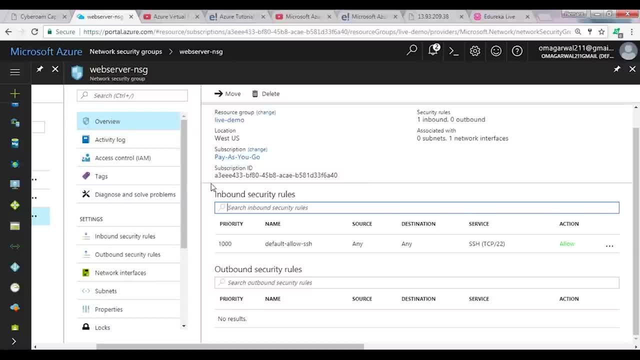 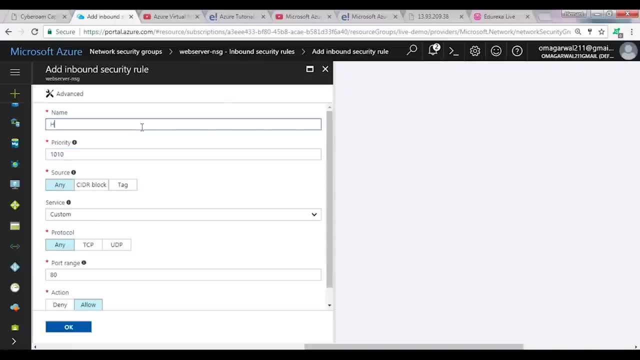 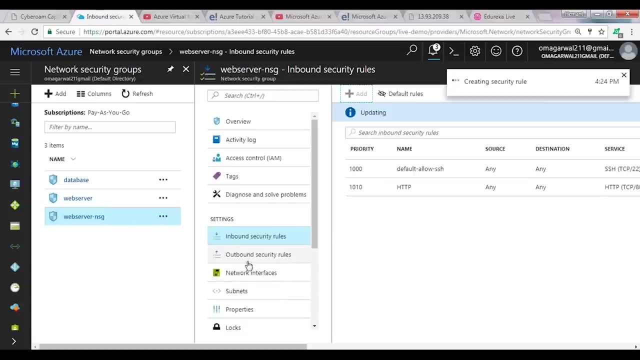 configure it to allow HTTP connections. so to do that, I will go to inbound security rules. I'll click on add, I'll add the HTTP rule. here it is, I will click on allow and I'll click on ok. all right, so my security rule is being deployed. I also have to configure it to have the HTTPS rule as. 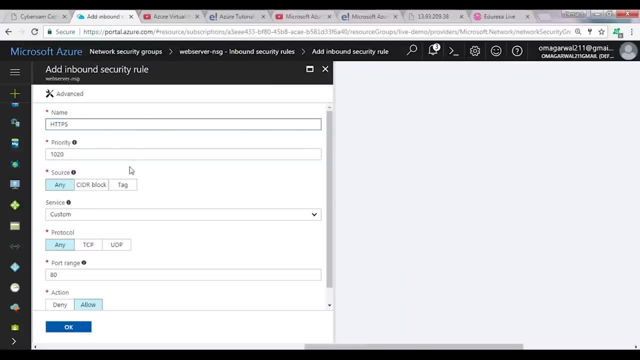 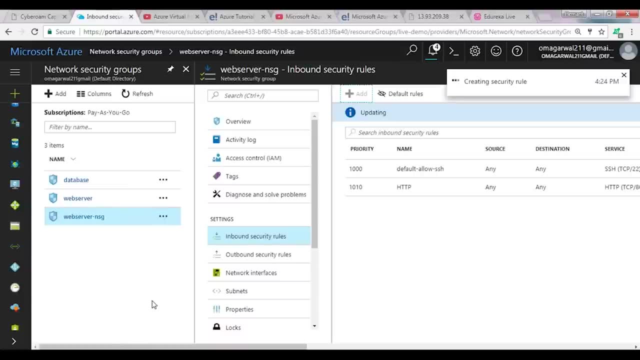 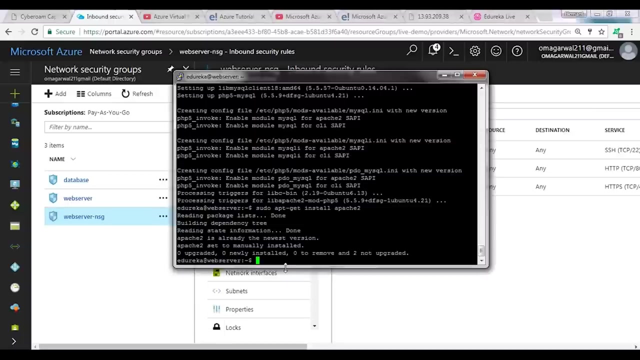 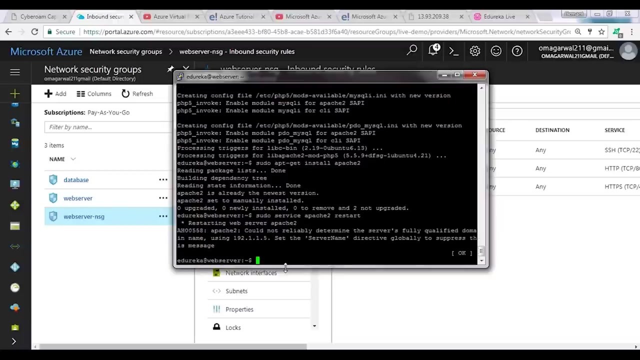 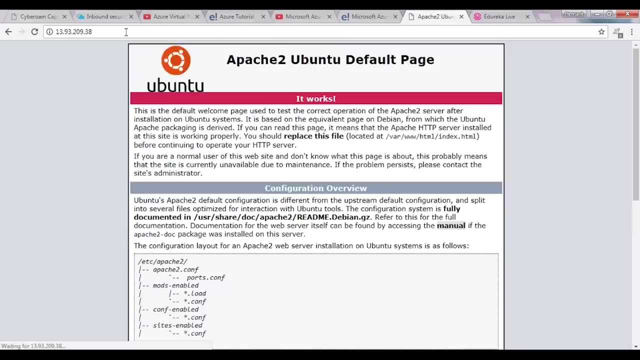 well, so I'll configure it to have the HTTPS rule as well. so I'll configure it to have the HTTPS rule. I'll click on ok and yes, I have the security rule for this as well. now let me restart the Apache to service, pseudo service Apache to restart: right, and if now I try to connect to my website, yes, so I. 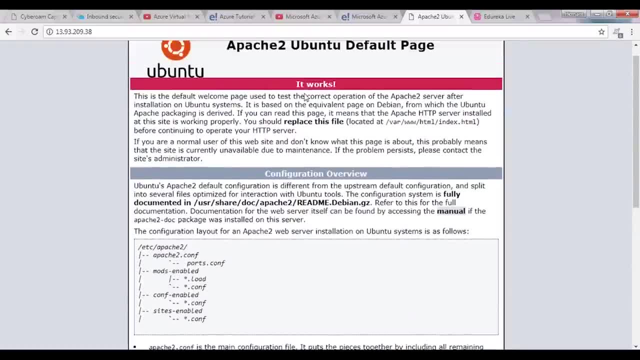 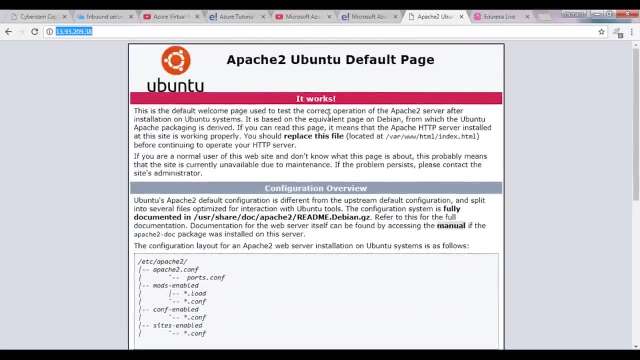 can see that Apache to page is now working right. so if you guys will now try to access this IP address, the Apache to page will start working. all right, guys. so now, since our page is working, the the next task is to connect through ftp and upload my website. so to do that, i'll have to first add 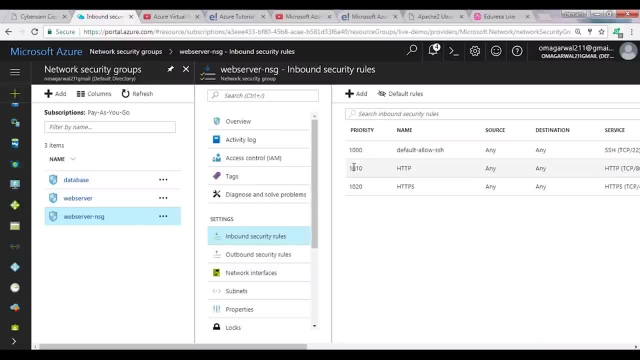 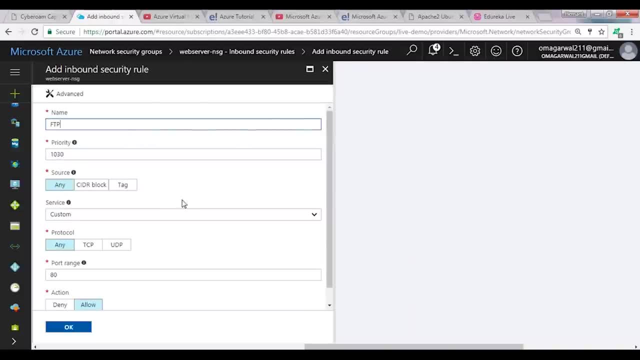 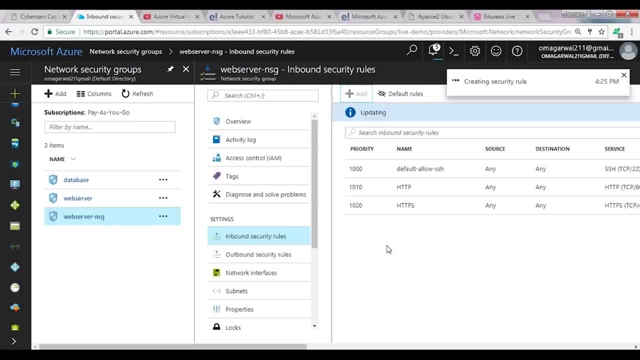 the ftp rule in the inbound security rules. so to do that, i'll click on add and in the name i'll type in ftp. right, the service would be ftp, and then the action is allow and i click on ok. so it is now creating the security rule. 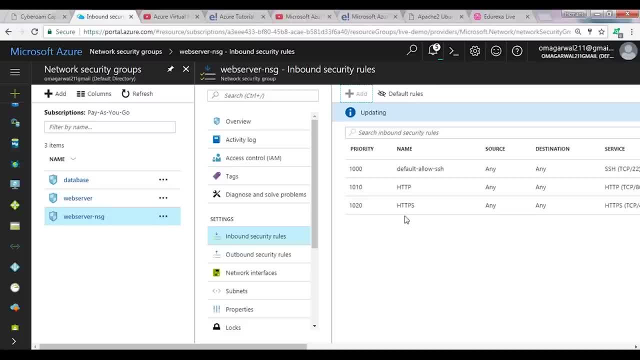 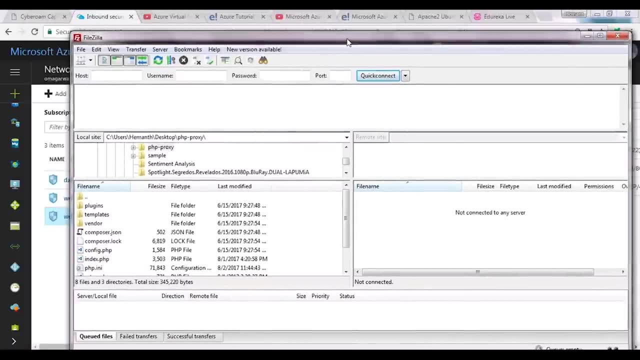 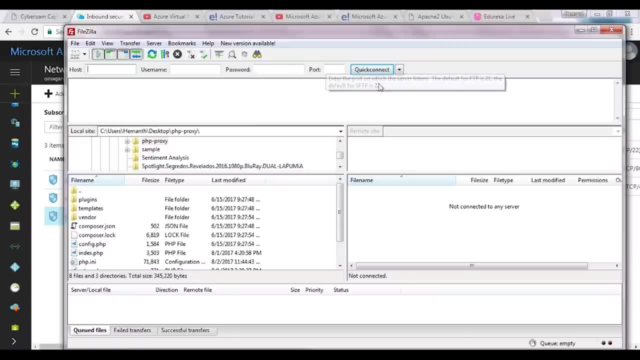 and once this is done, i'll be able to connect through an ftp software that i had. this is called filezilla. all right, so you'll enter the ip address here, your username, your password, port number for ftp connections- it's 22- and then you'll click on quick connect and then we'll have the all. 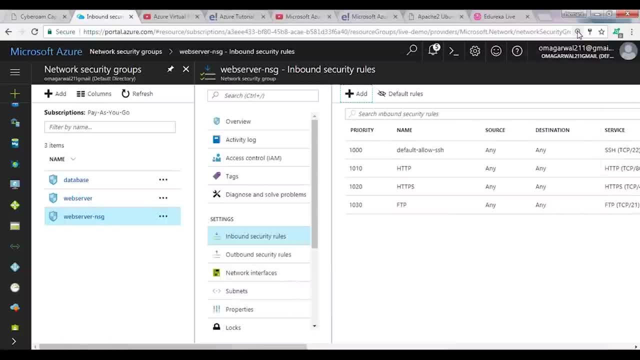 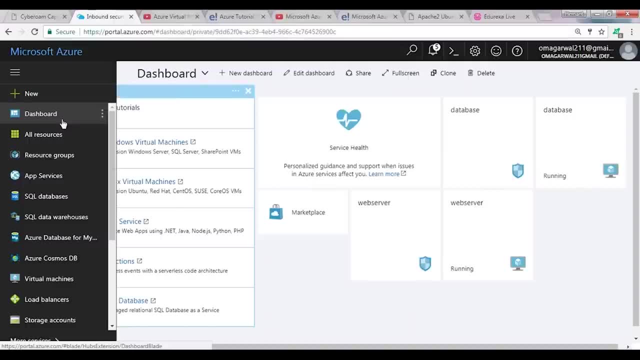 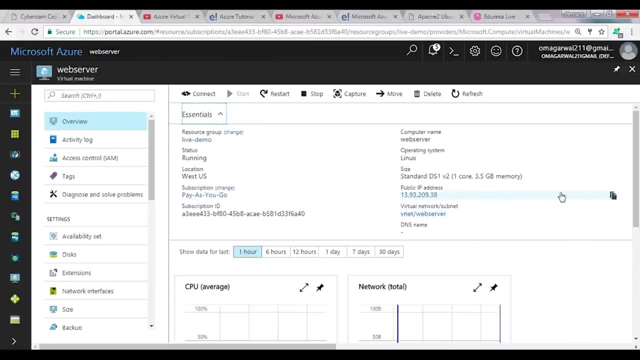 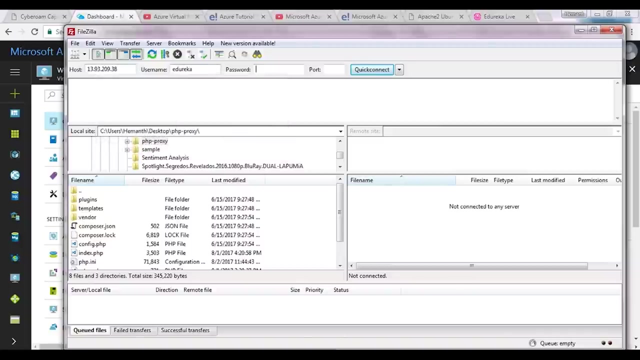 all the directly listing of that server over here. all right, so as i can see, the ftp rule has been added, so now i'll go to the dashboard. i'll go to my web server, i'll copy the ip address, i'll paste it here in the host. the username for it, that is edureka. 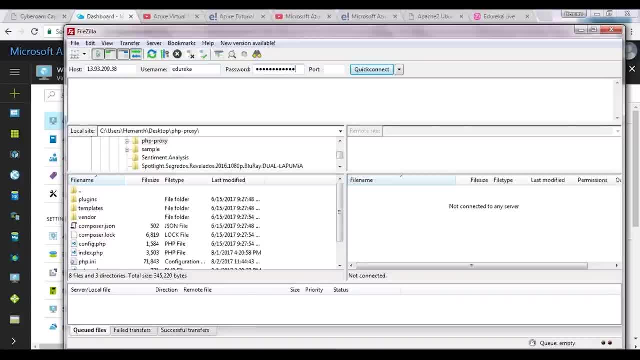 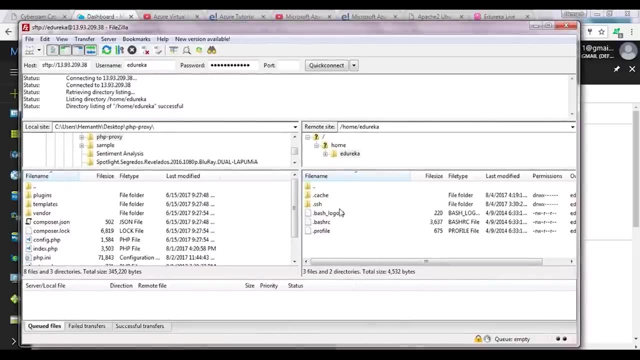 password. let me enter the password and now the port number. i'll click on quick connect. now. it'll take some time to connect to the directory of my server. so now i have the directory all right. so now i'll have to upload my website, right. so for. 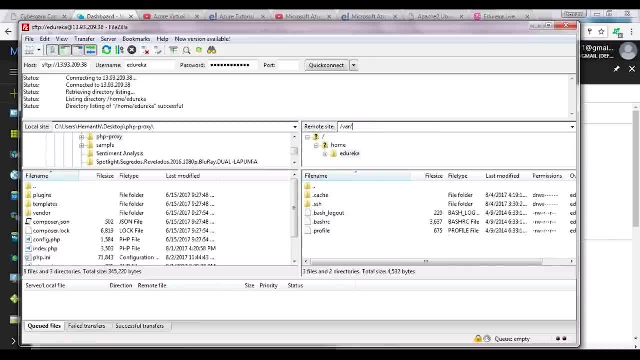 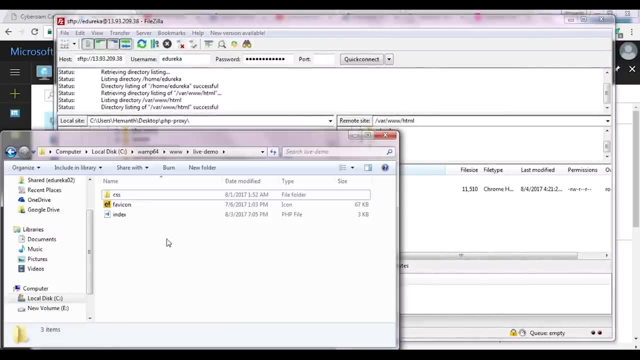 doing that, i'll have to go to this particular directory, that is, slash bash, slash www, slash html. all right, so this is the directory where you will be uploading your website. now, by default, you cannot upload your website, so let me show you what i basically mean if i try to upload my files here. 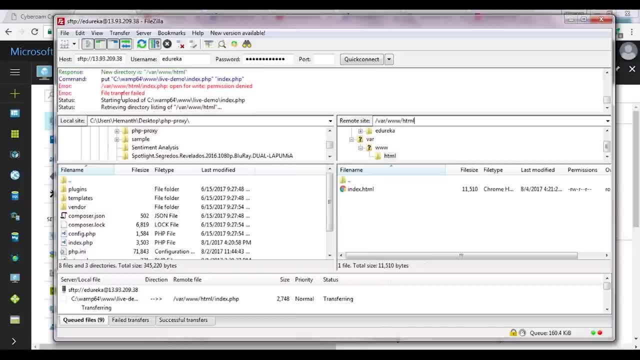 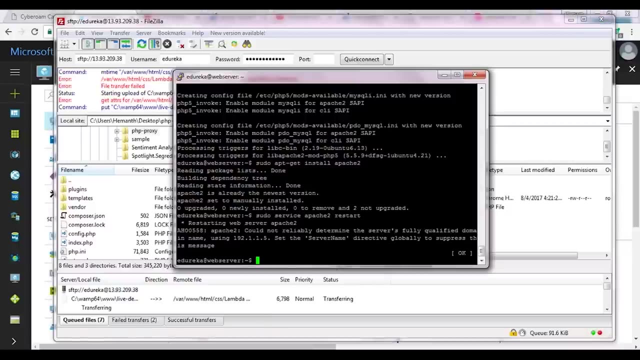 you'll see that i'll have an errors, that file transfer has failed. so that is because, um, over here we don't have the uh access rights i've been. i cannot read right in this directory. now for doing that, i'll have to allow myself to uh, allow myself from the shell. so i'll do that. let me cancel all. 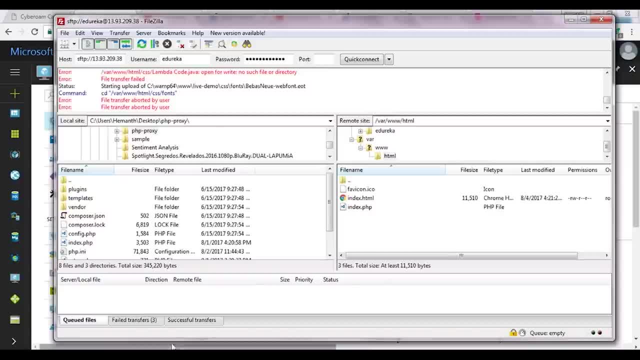 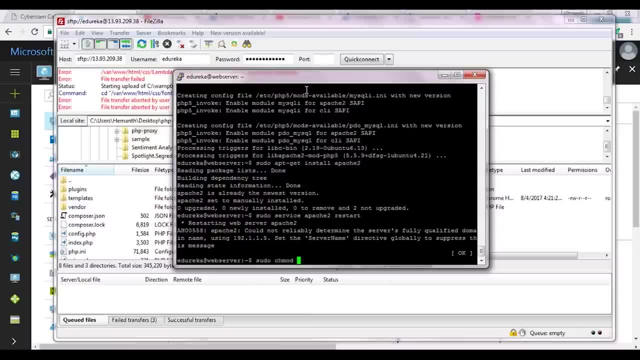 the uh file transfers that are happening. all right, so now i'll go here. i will type: sudo c hmod, hyphen capital r triple seven. so this will basically give me the rewrite access to this particular directory and once i have that i can upload my files. 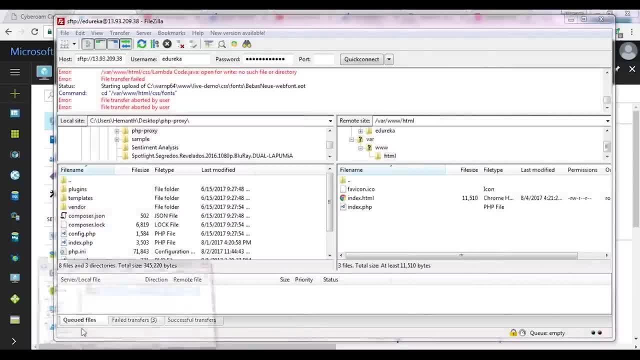 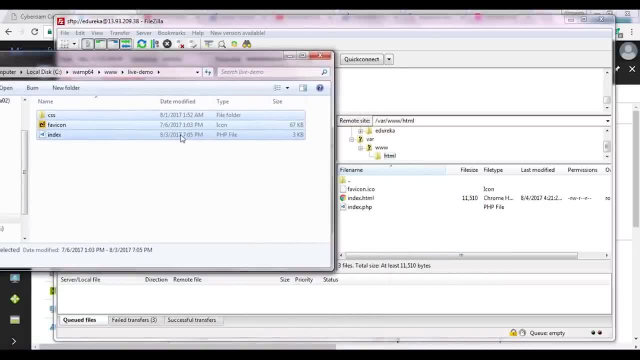 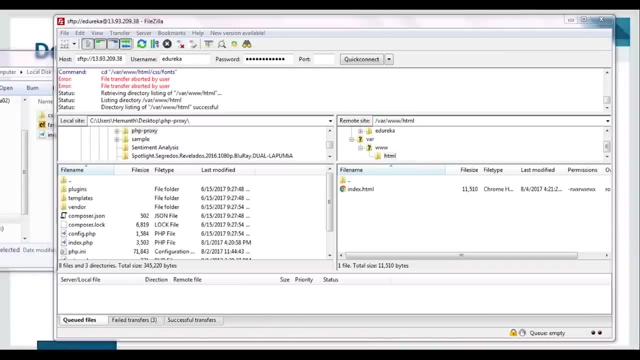 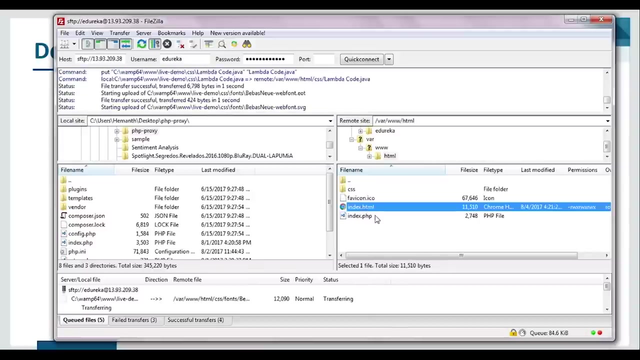 all right, so this should be it now. if i try to upload my files over here, all right. so now, like i said, if i'll try to upload my files, it should upload it successfully. so, as you can see, the file transfer has now started. all right, i don't need the indexhtml. so basically, this is. 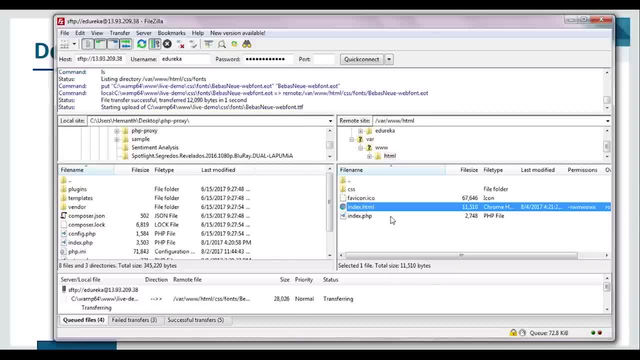 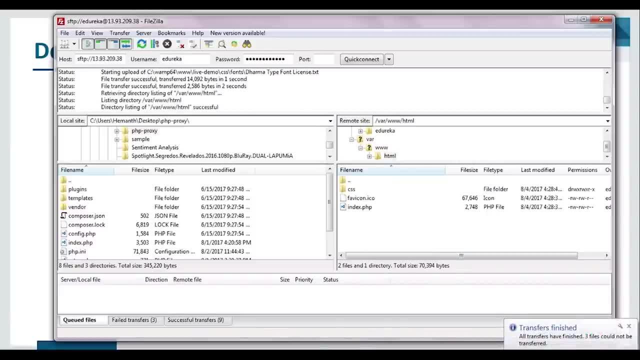 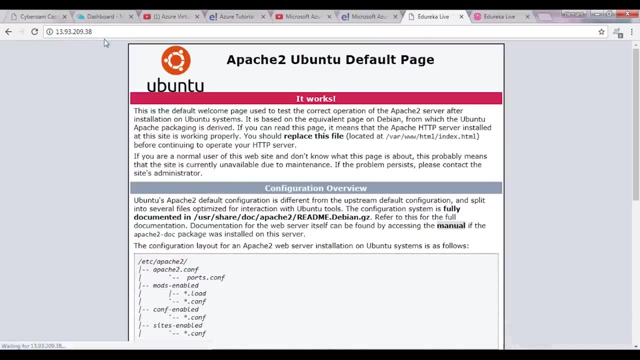 the apache page that you were seeing, so we can delete this page. okay, so my transfers have finished. so now, if i go back to my website and i try accessing it, i will be able to see the website that i just uploaded. right? so this is the website that i just uploaded. 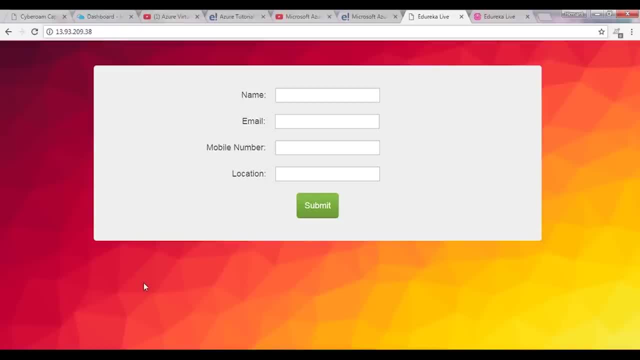 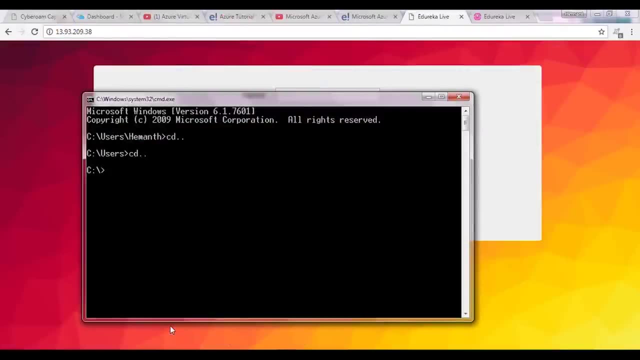 now, um, let me show you the database server that i configured yesterday. so for that, let me open my command prompt, go to my mysql installation. so this is mysql installation. guy, i'll type in the command mysql, hyphen h, and now the host name. right? so for the host name i need the ip address of my server. 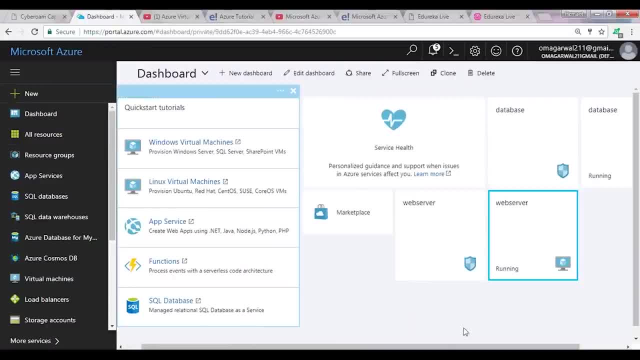 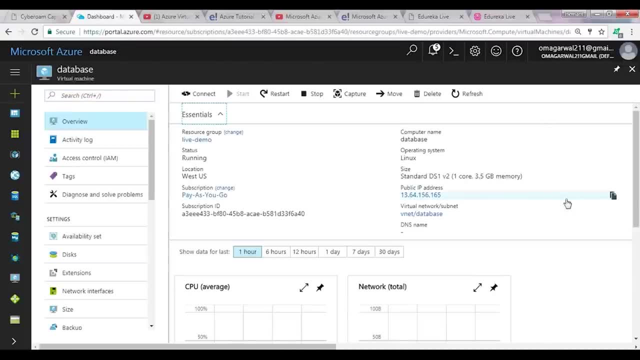 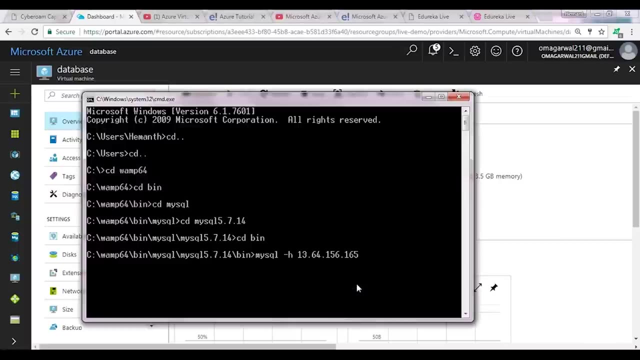 so for that i will go back to my dashboard and my database server, which is here. i'll copy the ip address for my database server, i will paste it here, and then the username, which is edureka, the port number, which is 3306, and then the password. all right, so it'll ask me the password. 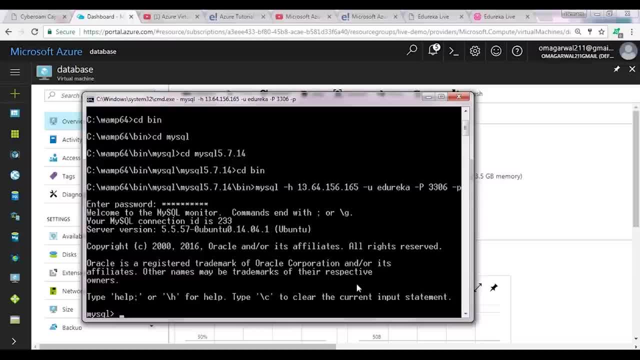 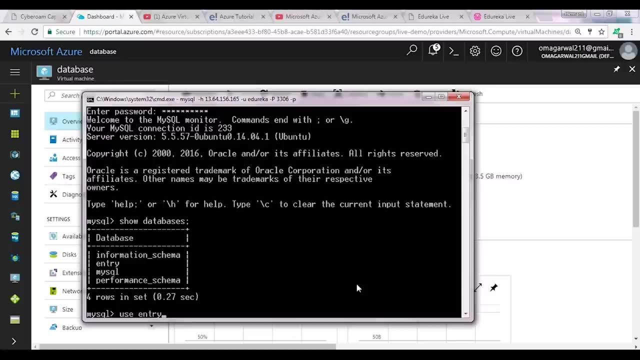 and with this i'm there in inside my mysql shell. now this mysql shell, uh, i have created a database called entry, so let me show you so as you can see, there's a database called entry. in this, my all my website data will go right, and inside entry there's a table called entries. 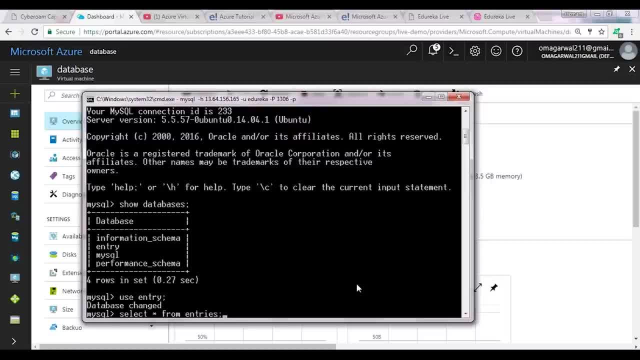 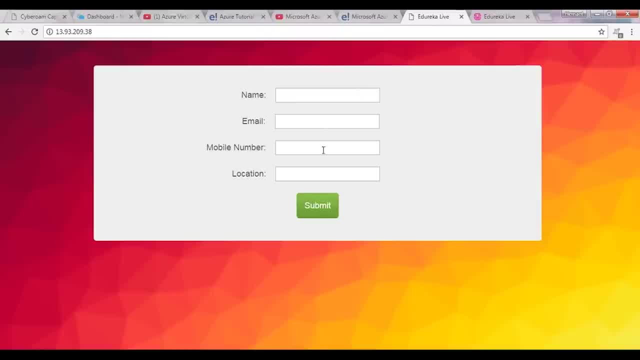 so as of now, if you can see, this table would be entry empty, right? so this table is empty. now my website will, uh, actually upload all the information that i'll be typing in here to this mysql shell. so if you guys want you want to try this website out, you can go to. 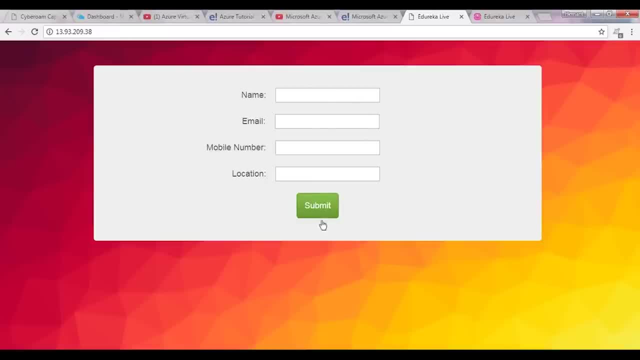 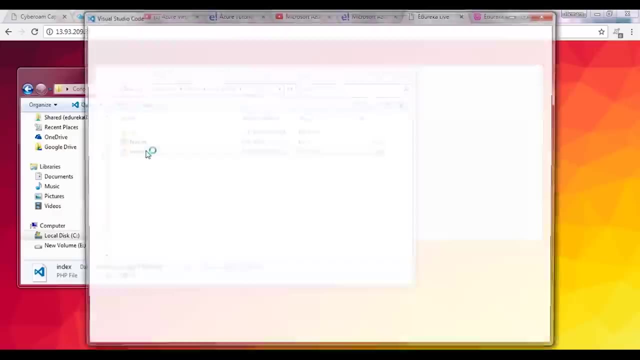 this ip address you can type in all your information, click on submit and it will get reflected over here right. so before that, before you could actually do that, let me change the index uh file, so i'll have to update it with the ip address of my server. 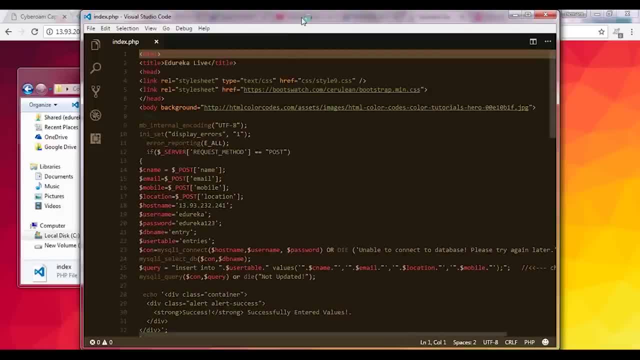 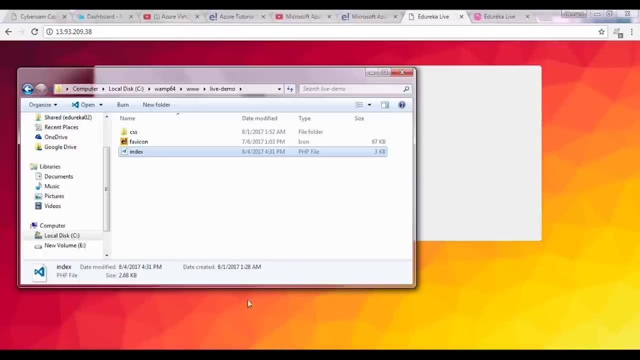 of my database right. so for doing that, give me a second. i'll go here in the host name, this is the ip address that i have to change. i'll change it with the ip address of my server, my database server, so i'll save it. and now i'll override this in my server. so i'll take. 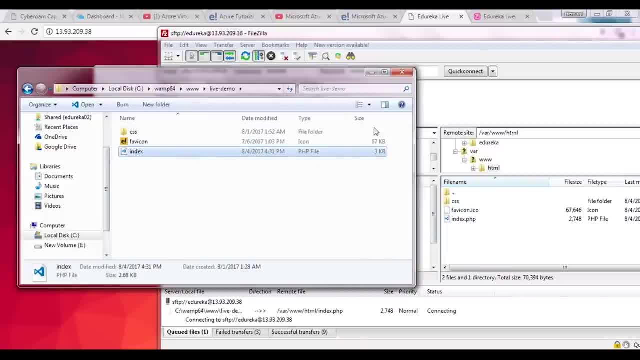 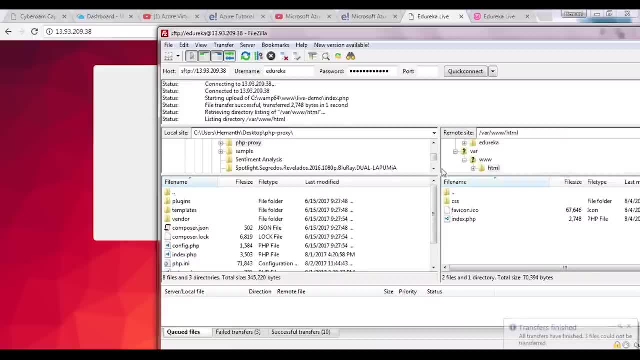 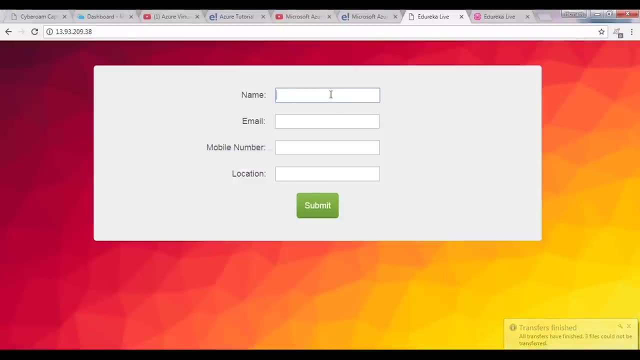 this file, indexphp, paste it here. now it'll ask me whether i want to override the file, so i'll say okay, and now it has transferred my file, all right. so now, if i enter details in my name, my email address, my phone number- all right, and then my location. so now if i click on submit, it will enter the values in the mysql. 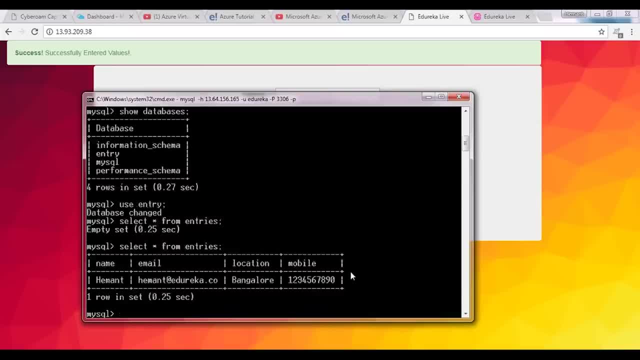 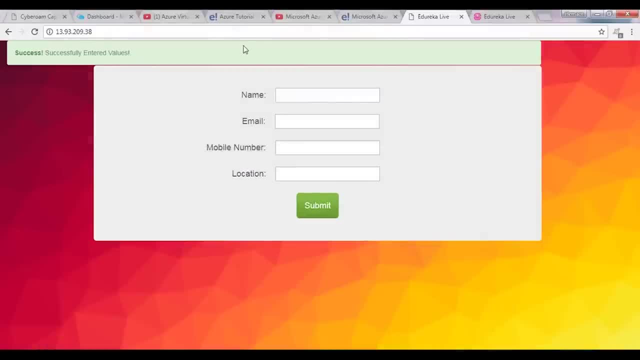 so now, if i refresh my mysql, i'll be able to see the entry which i just made, right? so this is it, guys. i have configured my web server on the azure vm and we have configured it from scratch, or so you'll find there's a service in azure called. 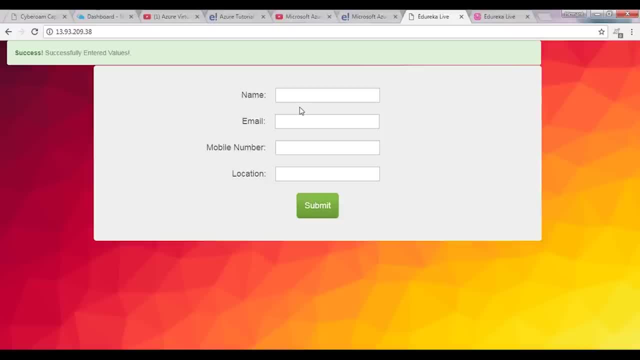 app service so you could do that automatically. all of this, that is, configuring your web server and everything. you just have to upload your code. it would have installed everything, but it's good to have, it's good to learn from scratch, right? you should understand how things happen in the. 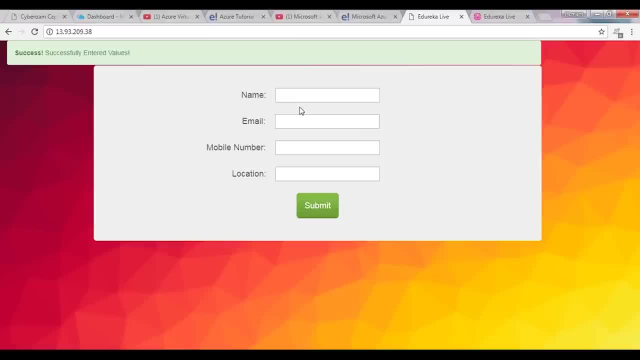 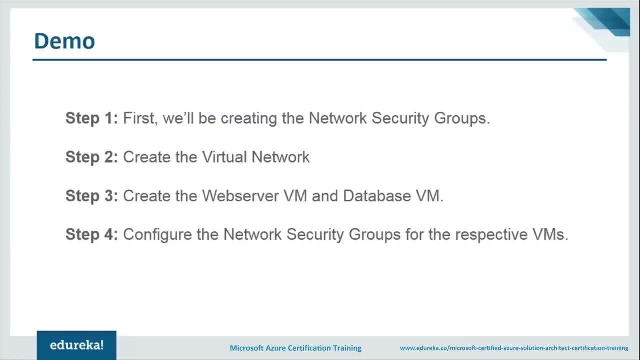 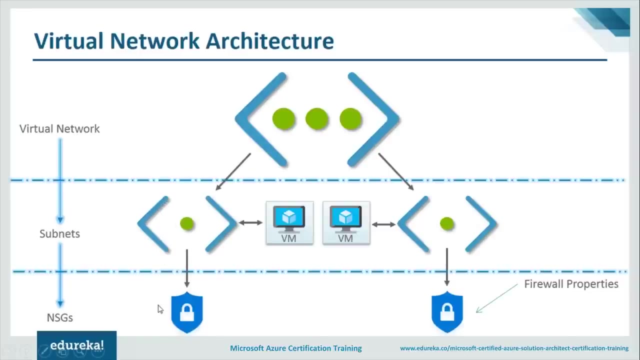 background, and that is the reason that is the motive behind today's demonstration today. all right, so with that, guys, i will end today's session, right? so let me summarize what all we did. so we created a virtual network, we created a subnet, we created a network security group. 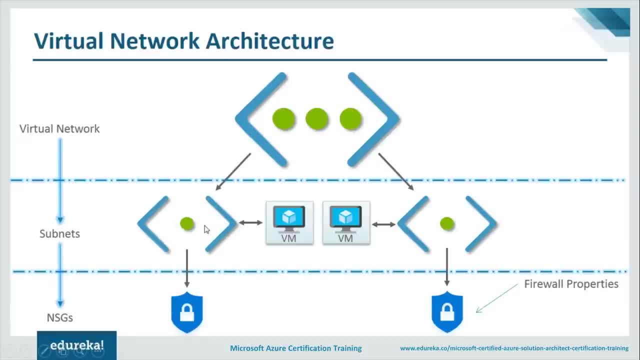 we created a vm. we attached the vm through the subnet and since the network security group was attached to the subnet, our vm could access the properties in the uh in my network security group. in my network security group, i allowed all the http connections right. i allowed the ssh connection and that is the reason i could connect through ssh. 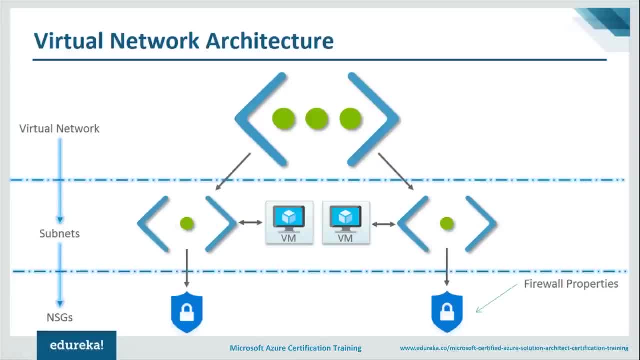 right, and that is the reason you guys could also connect to this website. if you try to open it, and in case i would have denied all the traffic from http, you guys won't have been able to access the website, and that is the reason we need firewalls. 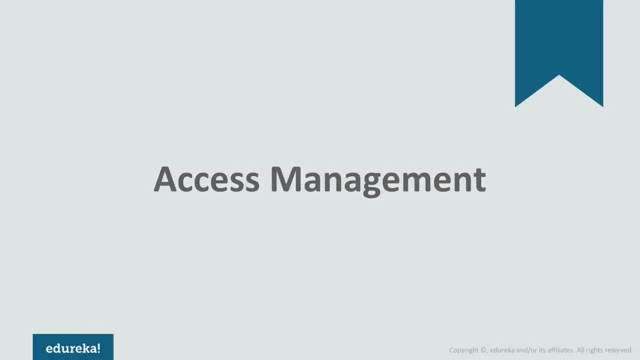 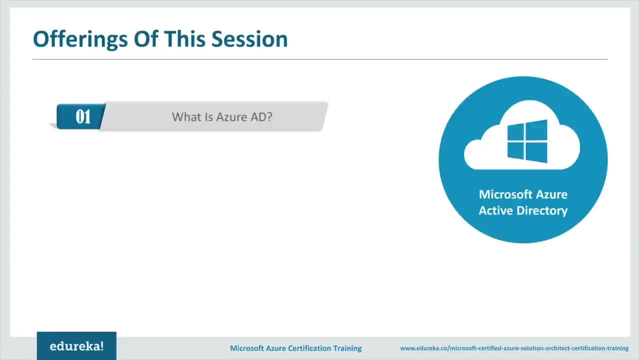 today's topic of discussion is azure active directory. but before we do go ahead and understand what an active directory exactly is, Let's start by taking a look at today's agenda first. So what do we have here? first and foremost, we would be starting things off by understanding. 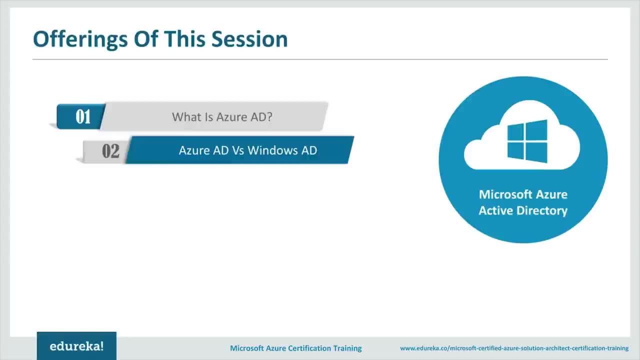 what an azure active directory exactly is and why it is needed. you would also understand what is the difference between Azure Active Directory and windows Active Directory. would also understand what are the different audiences this Active Directory caters and discuss what are its different additions. I would also talk. 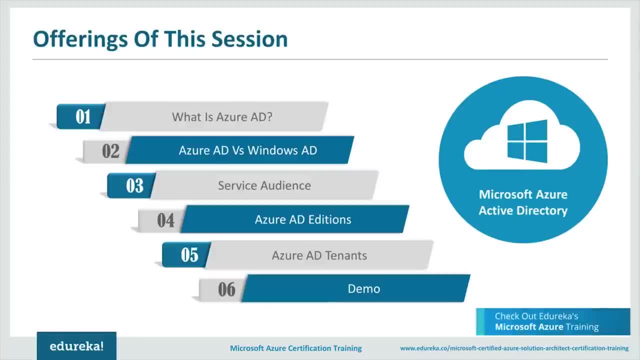 about what are Azure Active Directory tenants? Finally, I would finish things off with the demo part. Now, when we talk about the demo, I would be talking about how do you go ahead and create users and how do you go ahead and create an active directory. 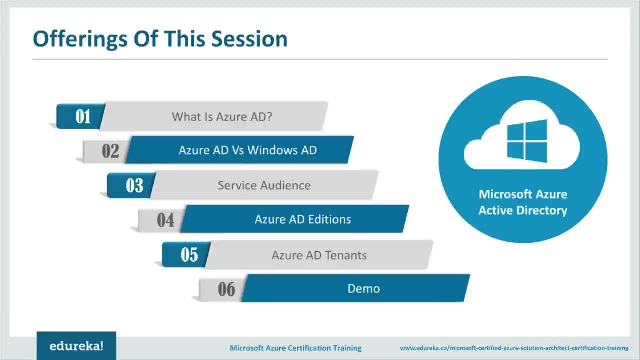 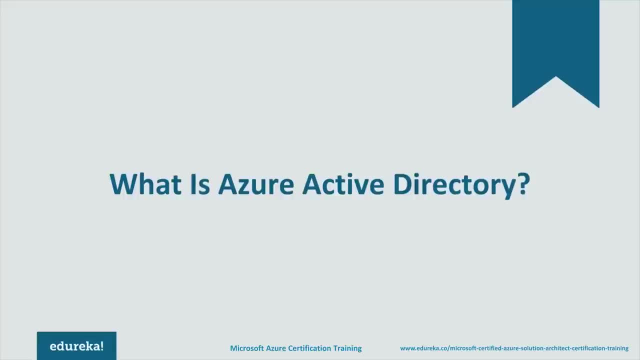 I would also be discussing quite a few other terms as well, but that is for the later part. Let's start by understanding what an Azure Active Directory exactly is. Let us start by taking a look at the definition first. Now, if I talk about the definition, 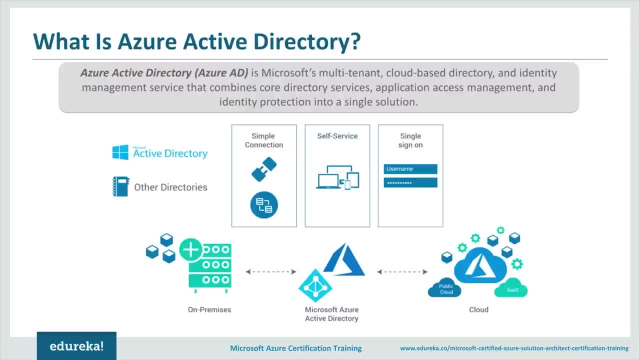 this is what we have. It is Microsoft's multi-tenant cloud-based directory and identity management service that combines core directory services, application access management and identity protection into a single solution. Now, there's so many terms in it and so many things to understand. 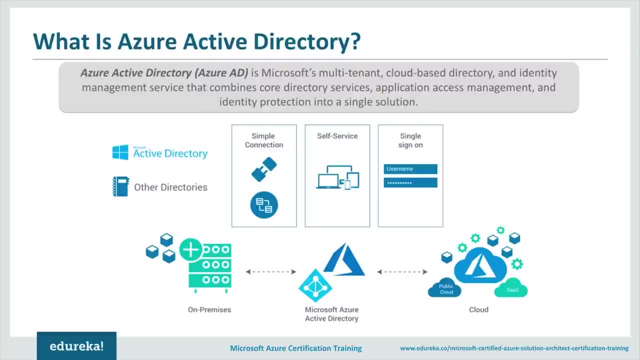 Let me simplify this definition so that you understand it in a much better way. to do that, I would be giving you an example. think of it in this way: Suppose I am a cloud vendor or not a cloud vendor. I am a service vendor and I reside on a cloud. 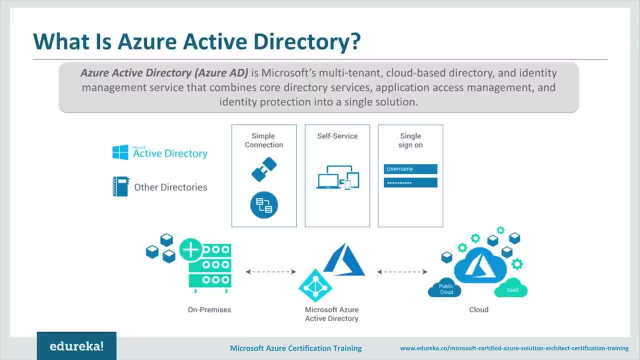 That means I have a particular application that runs on cloud. Now. this service is used by quite a few customers. Plus, there are quite a few organizations that I have to interact with now, in this case, all these medias or customers and organizations. They have to communicate with me. 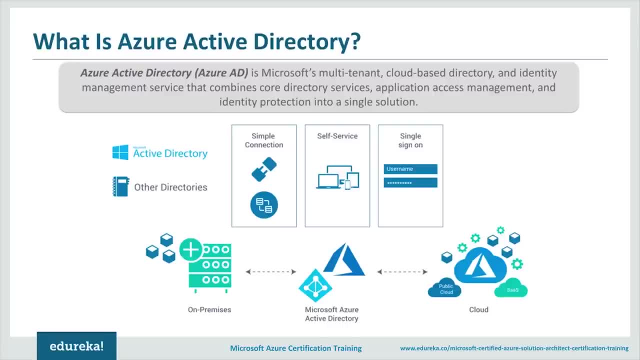 So how do they do it? Well, what they would do is they would go ahead and create an account, or maybe have some user IDs through which they can actually communicate with me. now, This is okay, If the number is countable or manageable, suppose. 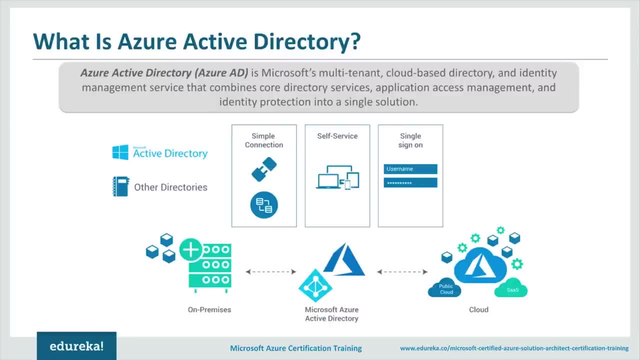 there was a situation where we had a number of people and the number of people was constantly increasing. suppose I have somewhere around thousand, two thousand people now. these many logins and these many credentials: managing all these can be a huge problem. Let me give you an example. 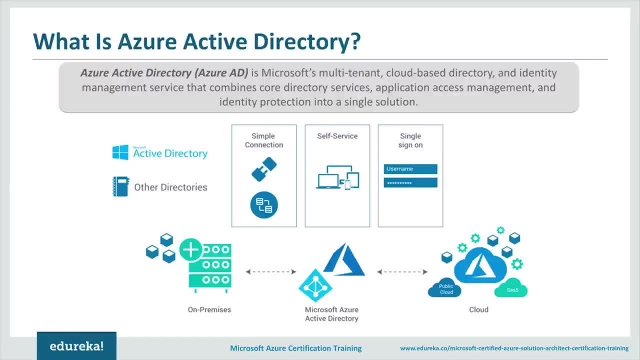 How does this happen exactly or what problems do you face normally? suppose I have 10 organizations. now to log into all these or give access to all these 10 organizations can be a use problem Why all these organizations might have different kind of accesses based on that. 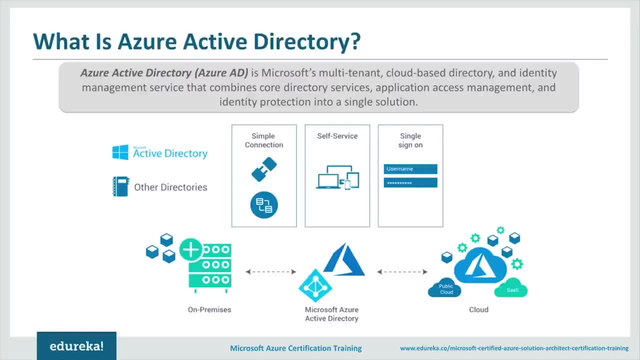 I have to set in different security protocols as well. If certain organizations have an easier protocol, what if they get an access to other organizations as well or to the data that other organizations have to correspond to? in that case it can be a huge problem apart from that. 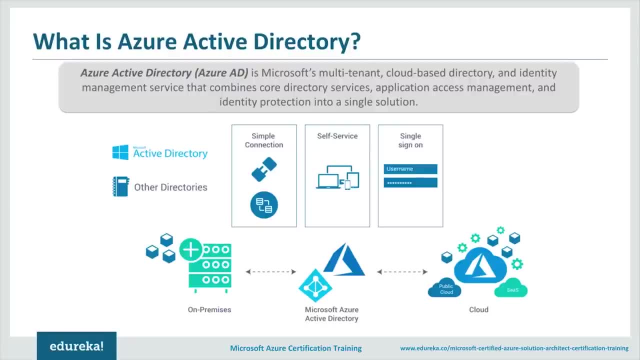 I might have n number of customers, and keeping track of so many customers can again be a problem when you talk about creating credentials. So all this is a huge problem. So what happened was Microsoft Azure. it went ahead and created something called as Azure Active Directory. 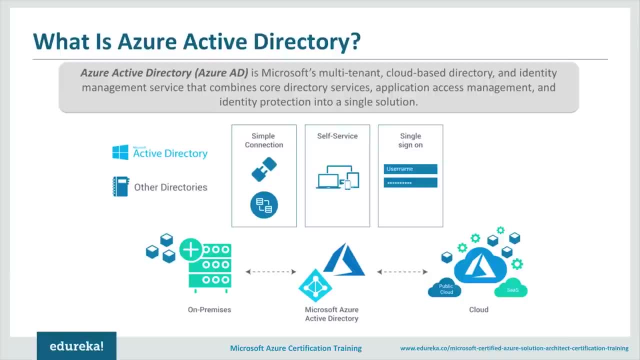 It is nothing but something that acts as a middleware. It takes care of all the sign-ins and all these things. how now the users will have a single sign-on process. That means they would sign in only once. plus, they can have access to the applications that are there, which I provide them. 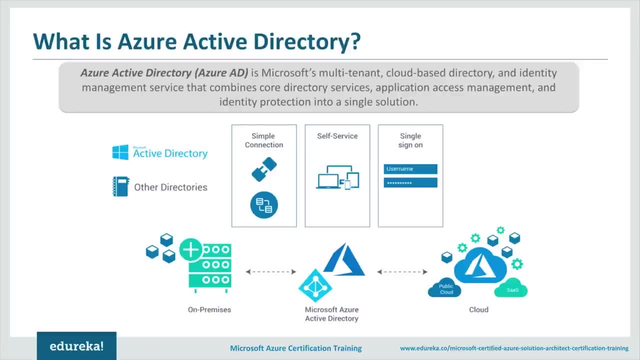 Now this intermediary that is your Active Directory. What it does is it federates all the responsibilities of taking care of access and all those things. that is the way I set all the rules. It just incorporates those rules and, accordingly, it gives access to all the users. 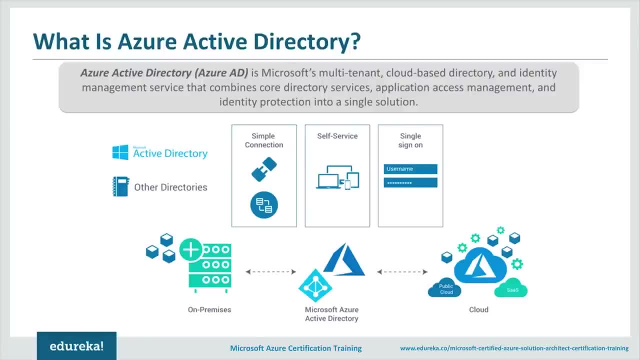 thus simplifying all the complexities that I would face otherwise. So this is what an Active Directory exactly is: It basically goes out and simplifies all the signing in and user authentication processes, or identification processes. Rather, now, as we move further, we would be discussing quite a few other terms. 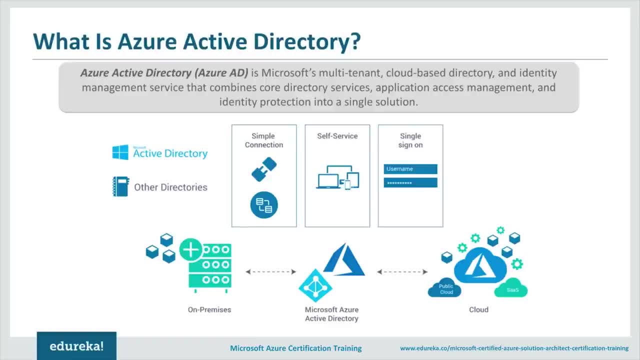 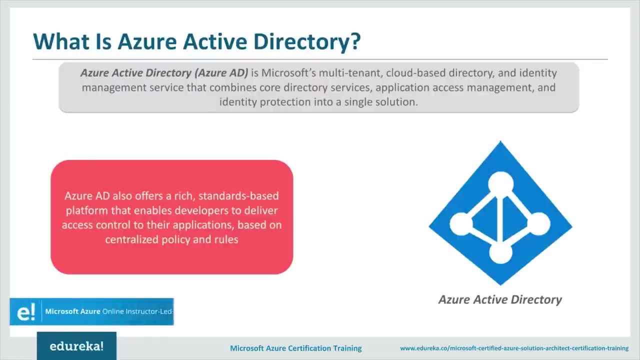 and you'd be having a clearer picture as to what I'm saying exactly. But meanwhile, you just bear with me and let's move further and try to understand What are the other points that we need to talk about. Okay, Yes, I did miss out on this point. 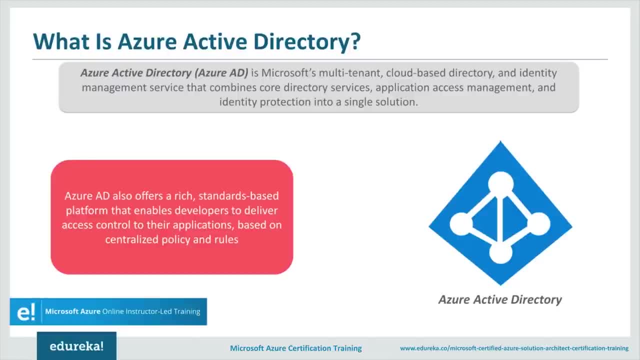 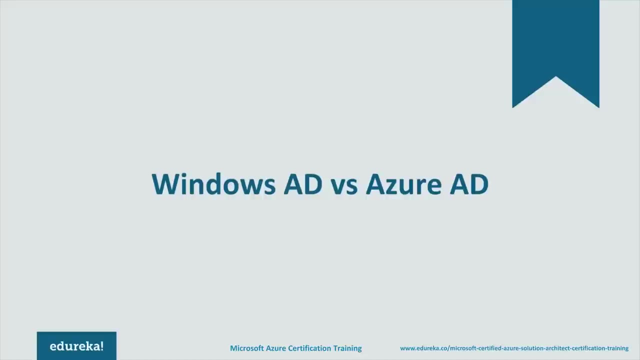 What Microsoft Azure does is. it also gives you something called as a better platform, where developers can develop the applications with lot more ease again as we move further. We'd be understanding this point as well. So what is the exact difference between Windows AD and Azure AD? 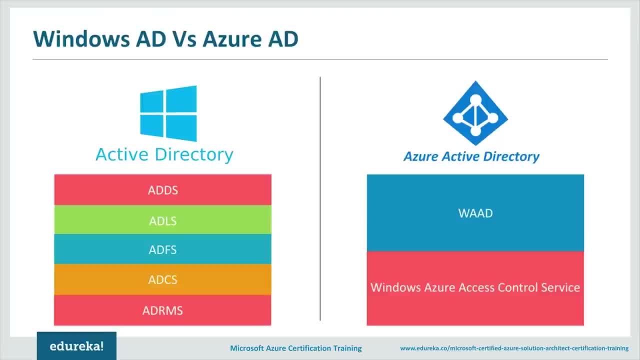 Let's try to understand that as well. And when you talk about Windows AD, that is, Active Directory. These are the layers It has to take care of. you have something called as your domain services. You have your lightweight directories. You have your Federation Services, certificate services, 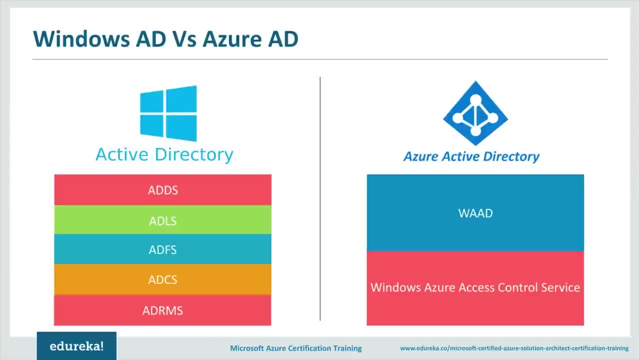 and rights management services as well. Now, these are so many things to take care of when you talk about your Active Directory with Microsoft Azure. it combines all these layers into two. Firstly, you have your Windows Azure Active Directory now. it is something that takes care of all the services. 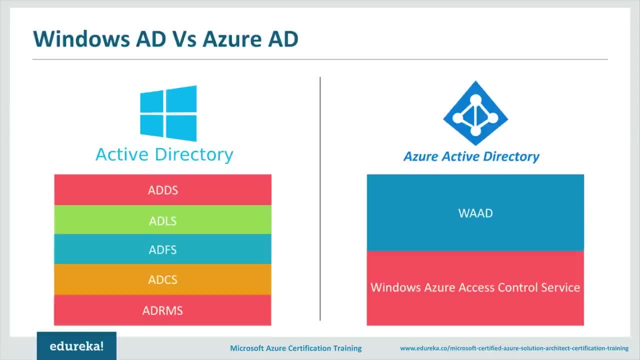 that surround or revolve around identity problems. That is when you talk about identification management. This is the part that takes care of it. That is your w-a-a-d, and then we have the other part where you have to actually go ahead and communicate with other organizations. 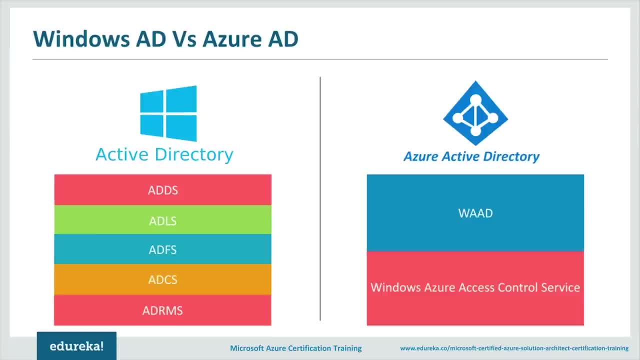 I give you an example of 10 different organizations needing 10 different things. that is, federating all these organizations. your Windows Azure access control services. It takes care of all those things. So both these so-called Active Directories- they more or less serve similar purposes. 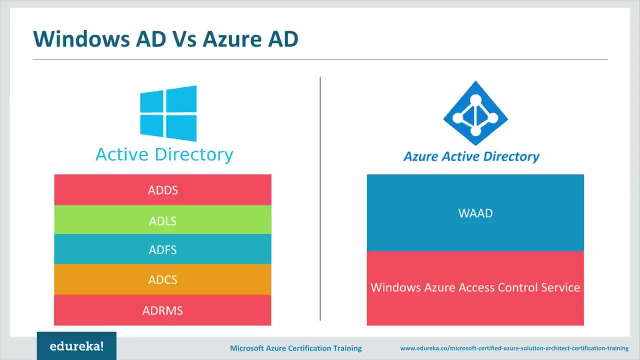 but the approach in which they do is is completely different. Your Active Directory has more layered approach where every service is given a different layer or different way of handling it. But when you talk about your Microsoft Azure Active Directory, it simplifies things. your first layer takes care. 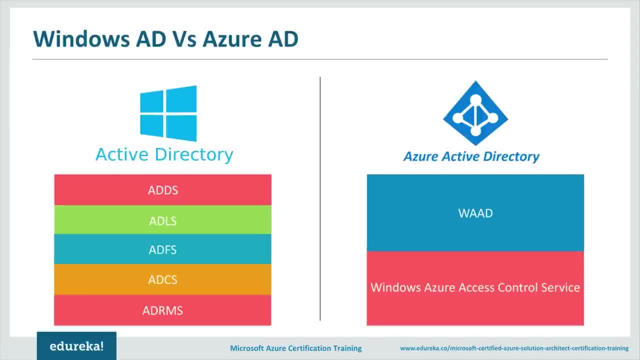 of most of the things, and the remaining things are something that is taken care by your Windows Azure access control service. Also, when you talk about Active Directory, it uses something called as LDAP for various other communications, But when you talk about your Azure Active Directory here, 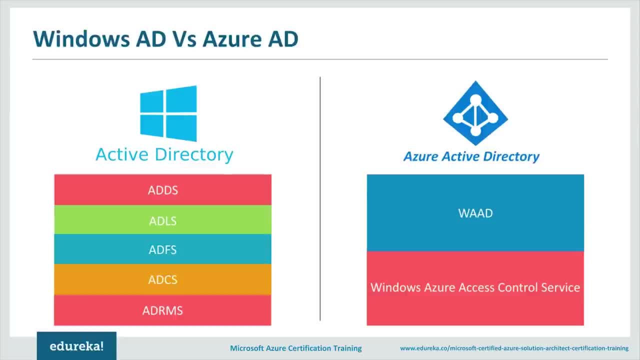 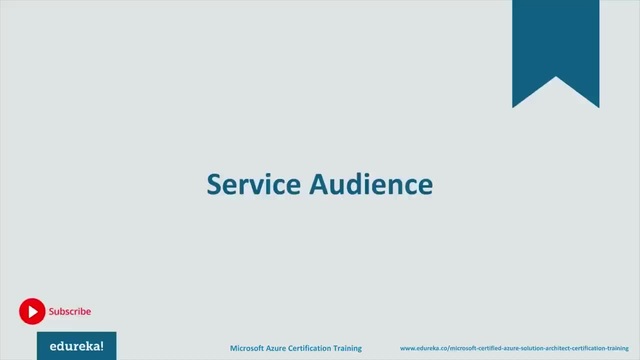 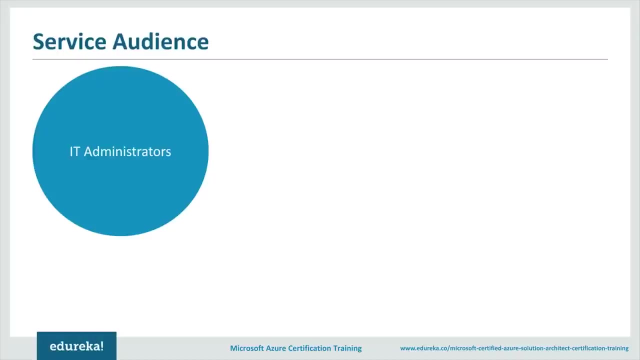 you use something called as your rest APIs. again, the approach is completely different. So what are the audiences that are catered by this directory? But first and foremost, we have IT admins. now, when I talk about IT admins, what Microsoft Azure Active Directory does is it provides. 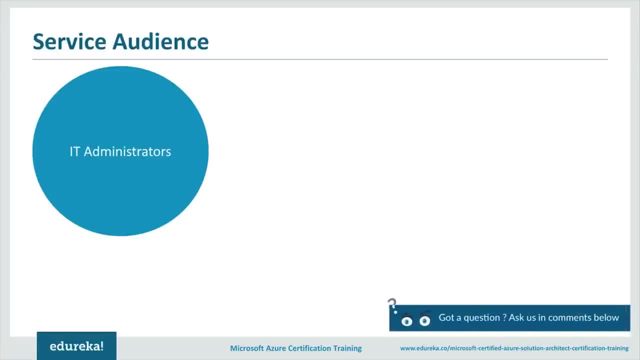 in single sign-on for various applications. Now there are quite a few SAS applications, that is, software as a service applications and various on-premise applications to which you have a single sign-on. You do not have to log in every now and then. now I've worked. 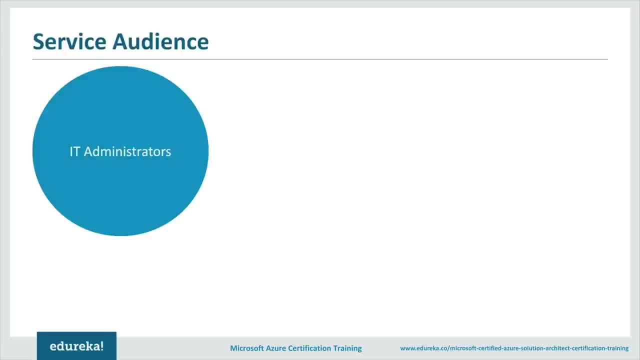 on quite a few applications and places where you have to log in every now and then. you have a lot of trouble because you have to remember so many passwords and so many logins, and these different credentials can be a problem. Now, this is something your Microsoft Azure takes care. 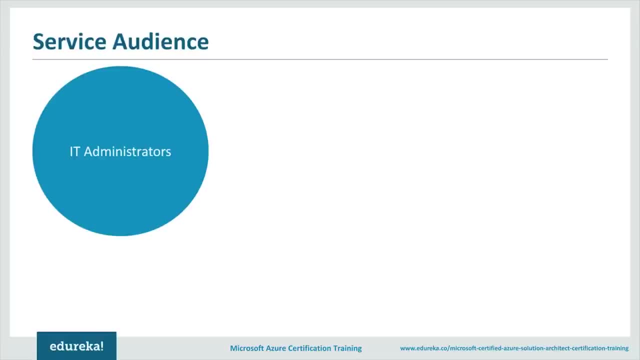 of single sign-on is very convenient. apart from that, It ensures strong identification and the quite a few processes that ensure this. now I won't be discussing those points in detail. Yes, when you talk about identification, Microsoft Azure ensures that it happens in a very good manner. 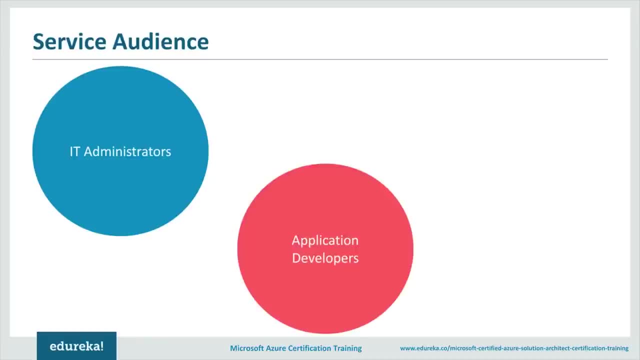 Plus, it automates quite a few processes, again easing up this process. apart from that, It also caters quite a few developers as well. Now I'm talking about quite a few organizations, and since sign-on becomes easier here, your application developers can focus on building applications. 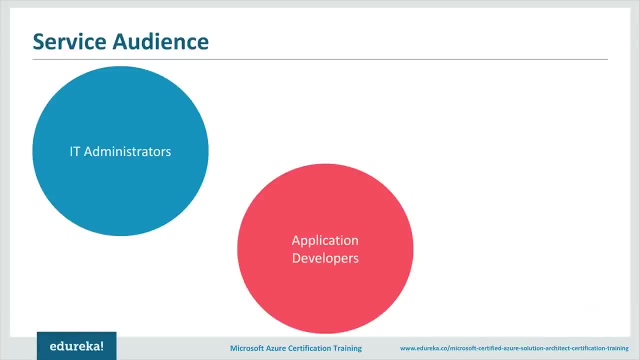 and since they have access to so many organizations and so many resources, application development definitely becomes easier. online customers, now people who have been working for quite a while- You might know that we have things like Office 365, or you have your CRM services as well. 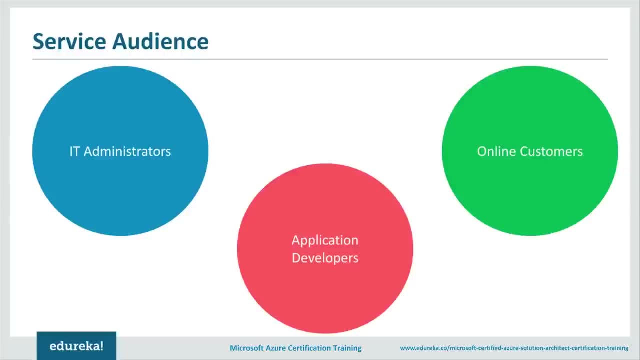 Now, you had an access to all these things by using your Windows Active Directory, but your Microsoft Azure Active Directory also gives you access to all these services. That means, if you are using or have account on any one of these things, you can have access to all these services. 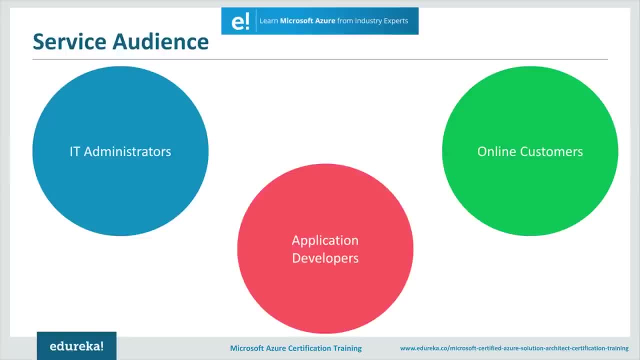 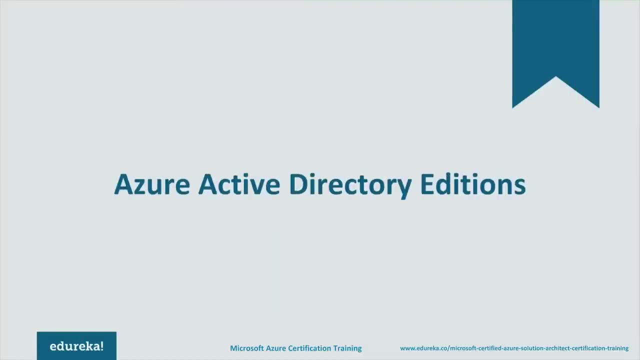 or have access to all the Active Directory services that Azure has to provide to you. So what this does is it caters the needs of various online customers as well. So let us try to understand the next point, that is, Azure Active Directory additions. for that? 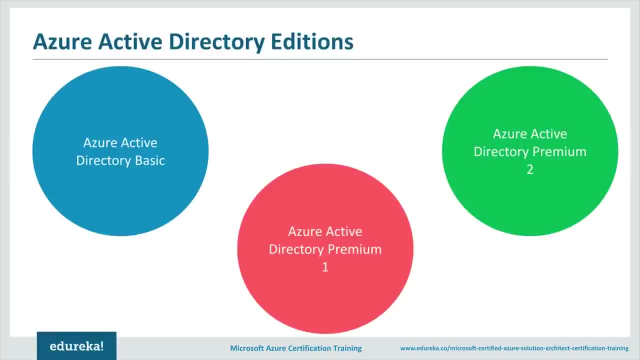 What I'm going to do is I'm going to go ahead and switch into the Microsoft's web page, basically, or I'm going to switch into my browser and move to their website and talk about all these points. So instead, what I would do is I would first discuss the last point. 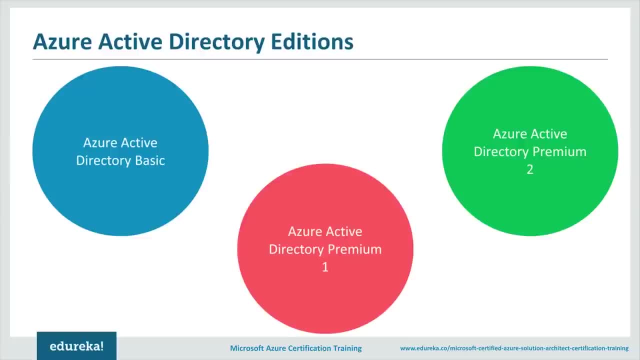 and before we do go ahead and take a look at the demo, then we would just go ahead and talk about these points as well, so that we can directly switch into the demo part. So let's move further and try to understand the next point and then come back to this point. 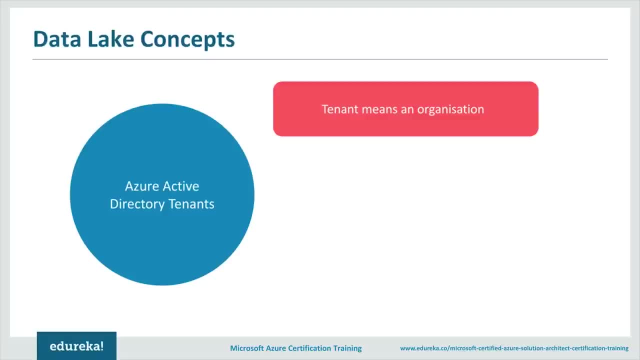 So what are tenants basically? now, when you talk about a tenant, it is nothing but an organization. I just mentioned that we have tens of organizations that a particular application might cater. now All these organizations are treated as tenants. All these tenants can have access to a particular Active Directory or more than one Active Directory. 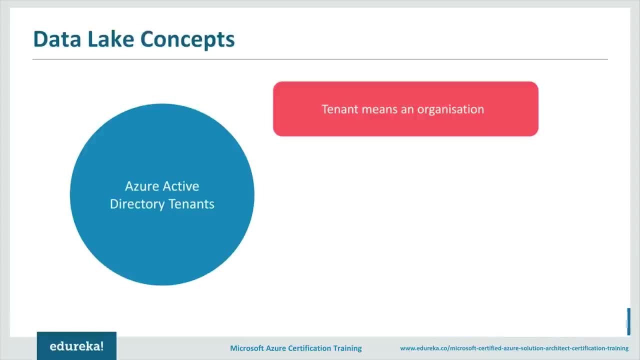 as we move into the demo part, I would be talking about how to create multiple directories as well. Yes, We have more than one Active Directory. will discuss this as we move into the demo part, But before that, you just understand these points as in what I'm trying to say exactly. 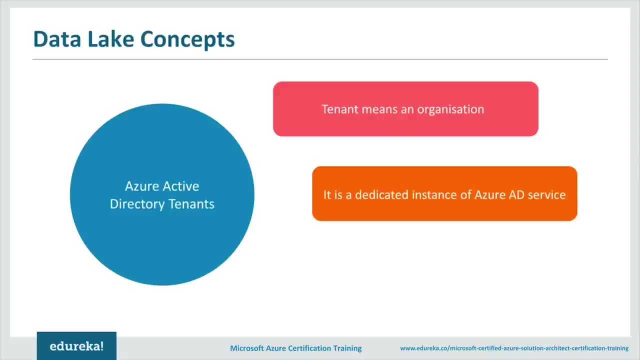 Yes, what happens here exactly is, when you talk about a tenant, first and foremost it is nothing but an organization and it is a dedicated instance of your Azure Active Directory service Plus. these are isolated instances. That means, as I mentioned, we have 10 organizations or five organizations. 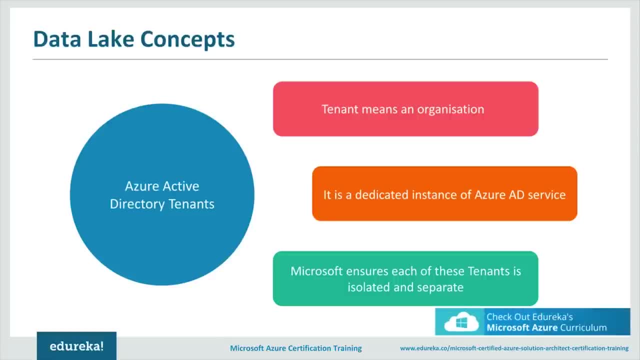 You'd be having isolated instances for each of these organizations, ensuring that they stay aloof and their services and their protocols are maintained differently. This is where your Azure Active Directory steps in. it takes care of all these things. It ensures that nothing is ambiguous or nothing is intermixed. 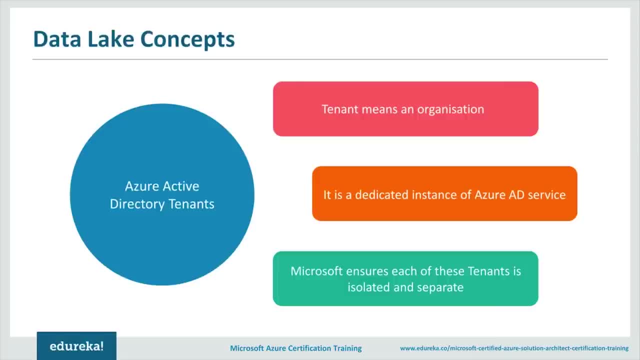 Everything stays separate, plus, each and every platform or organization gets serviced equally Well. as you move further, we would be creating users, and then I would give you the differences as in what a tenant is. How do you go ahead and create all the domains and all those things? 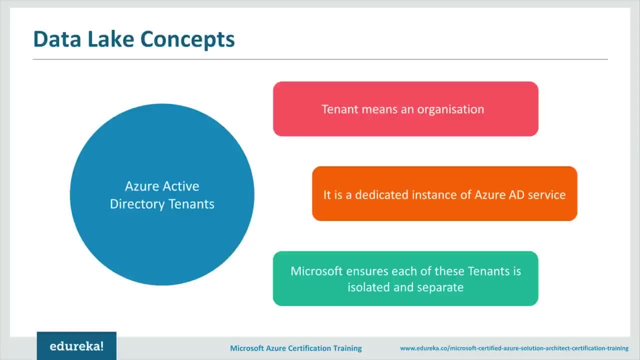 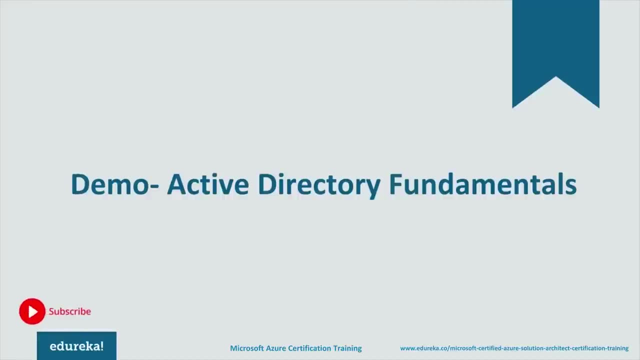 So again into the demo part. you'd be understanding these topics with little more clarity or more understanding. rather, This is the demo part, But before that, as I've already mentioned, let me quickly switch to the website of Microsoft Azure and I would be discussing the additions. 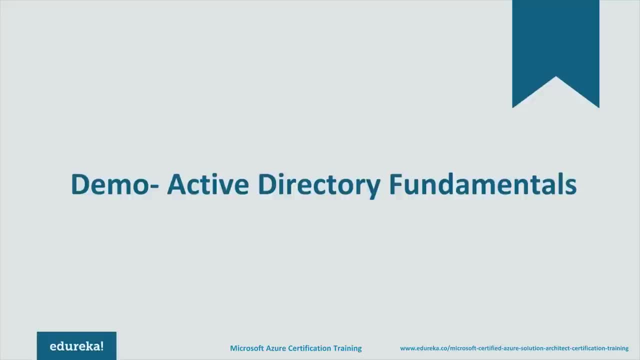 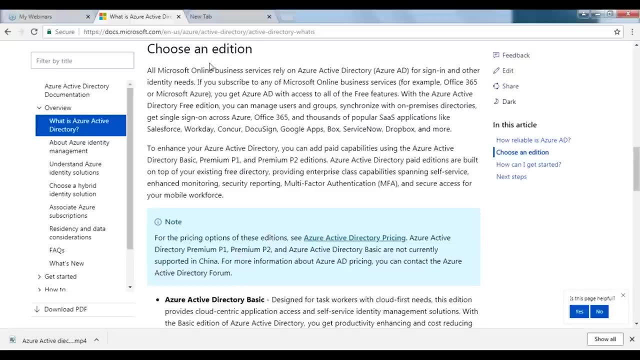 that you can choose from, and then we can directly jump into the demo part. Okay, guys, so this is a Microsoft dog, basically, which talks about choosing an addition. So these are the options you have. We would be finishing this quickly and then we would be switching into the demo part. 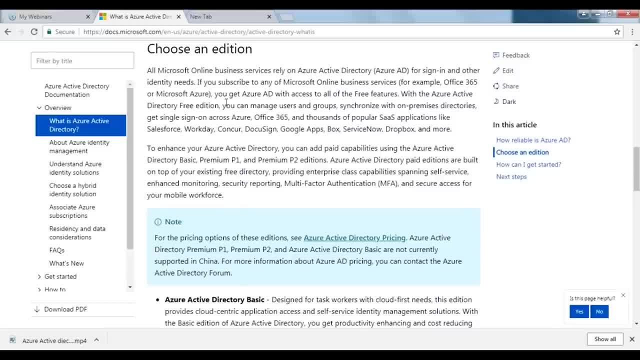 So let's understand this now, what Microsoft Azure does, as it gives you various options. first and foremost, you have three options to pick from and out of these three options, The first one is your basic option, that is, your Active Directory basic. Then you have your premium, which is P1. 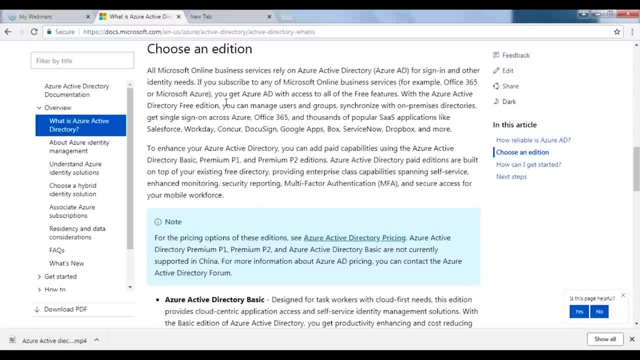 and then you have one more premium, which is P2. all these things provide you with different options that you have. first and foremost, your main job is to have your access, that is, your identity management, Your security and your single sign-on and all those things. 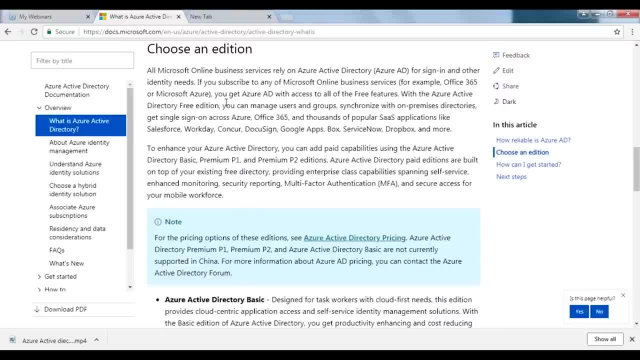 Now, these are some of the services that come with your basic account as well, and also with your free account. what Microsoft Azure does is. for people who are completely new to the session and Microsoft Azure, Let me tell you that you have a free sign-in. 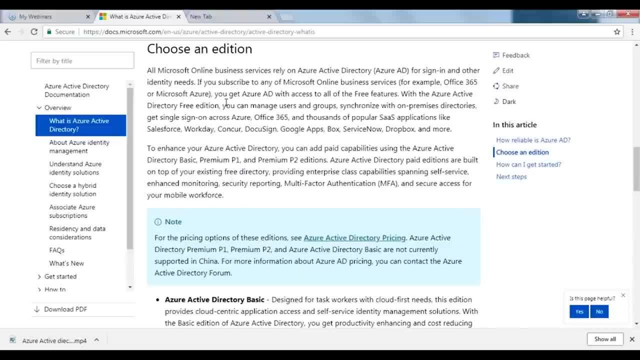 to Microsoft account. That means you can go ahead and create your account there and avail these services for a certain duration, which are available to you for free. So yes, you do not have to pay anything there. You have a free account in that. 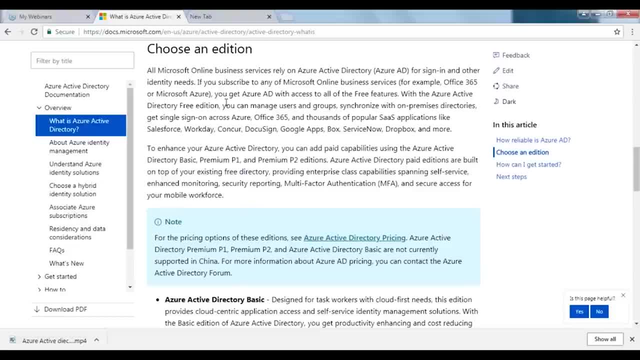 You'll be having access to some of these services, but if you need Advanced Services, then you have to pay for it, And for those things you have three options, that is, your basic premium P1, and premium P2.. Let's try to understand these one by one, as in: what are these? 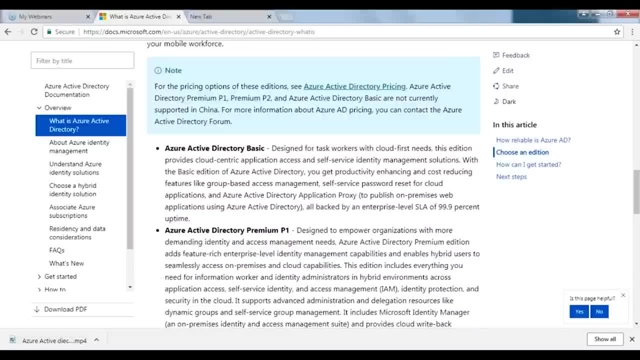 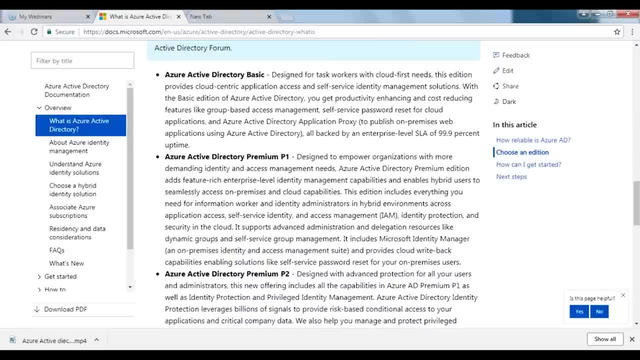 and what do they have to offer to you? Now, if you scroll down and if you take a look at this thing, you have your Azure Active Directory basic. Now, this basic is nothing, but it is designed for people who are task workers or who are focused on a particular application of on cloud. 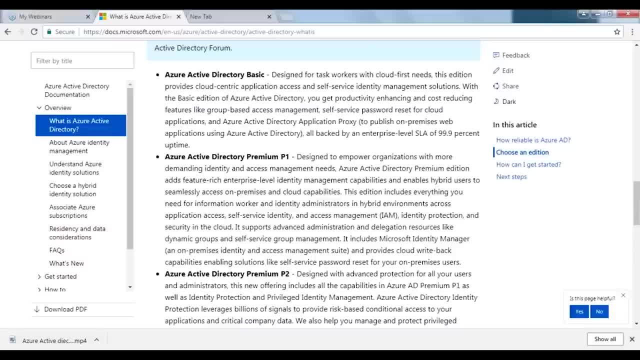 Now it takes care of everything- your single sign-ons, your SLS- and it ensures that the security is 99.9% and it provides you with all these features which you can see here, That is, your self-service, password resets and all those things. 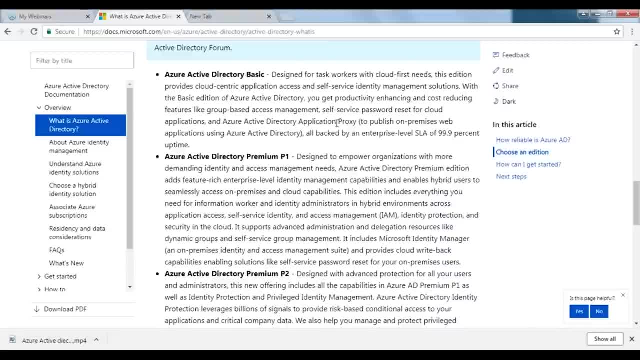 You also have access to quite a few things, like your proxies and all those things. I won't be getting into the details of what proxies are and all those things, But yeah, for people who are admins and who have worked on these topics or in these domains. 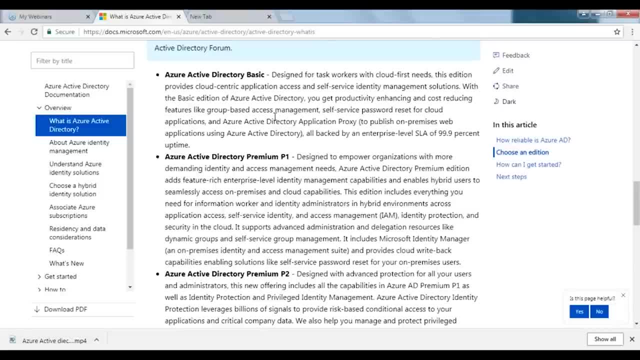 they would understand. what do these things mean? So, yep, you have access to all these things which fall under your basic option. apart from that, You have something called as your premium P1.. Now, this is for people who want to scale up. 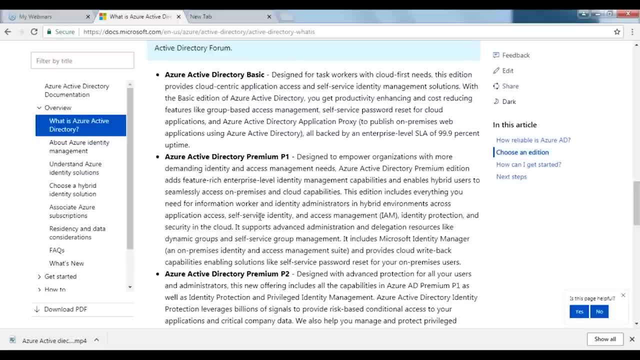 So when you try to scale up, you'd be dealing with quite a few things and terms like your I am and all those things would come into picture. Now I am is nothing but your identity and access management, basically, which is a very important point when you talk about Active Directories. 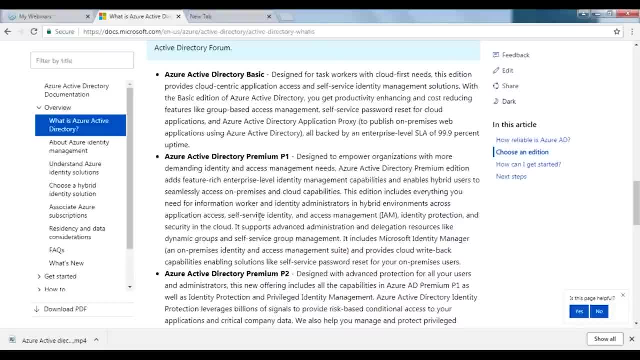 So, yes, it provides you with these things as well, or these facilities as well, like identity protection, your security in the cloud and all those things. Everything is taken care of for this particular model. Now, when you talk about premium P2, if I scroll down, this is what you have. 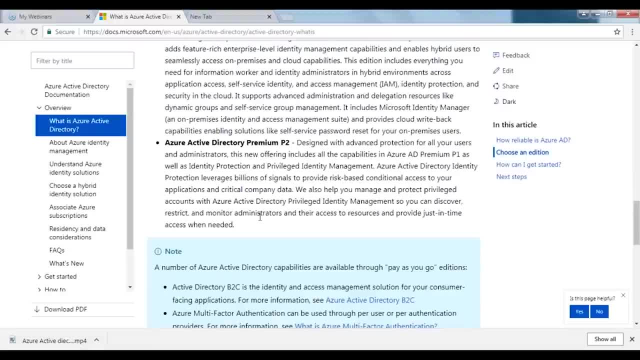 It is designed for more advanced protection. That means you'd be getting all the services that were provided in basic and P1. apart from that, You'd be having some additional services which ensure more security. That means it focuses more on privilege identity management. 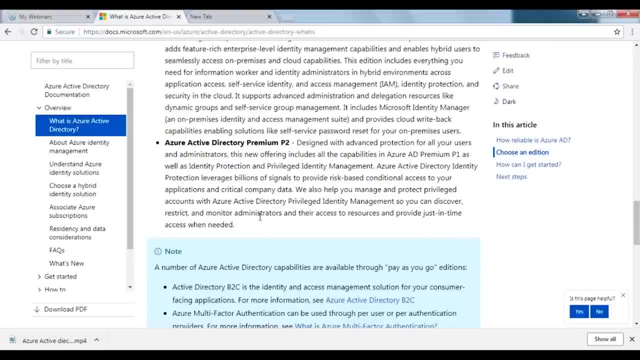 Now again, this is something that you can read and understand. it is very easy. But to give you a basic difference, your first thing provides you with your basic services, That is, your basic access. gives you basic Active Directory service access. Then you have your premium version. 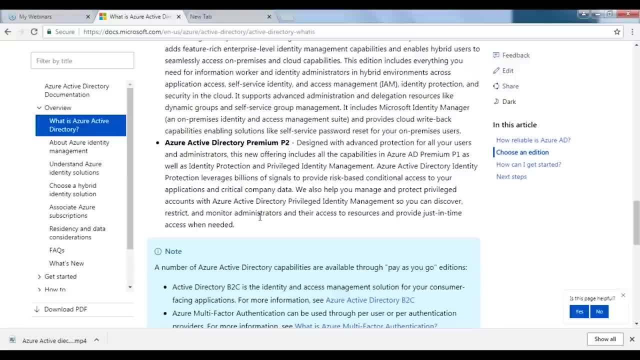 which is focused for scaling up, and when you talk about P2, it focuses more on advanced security. So these are the three different editions that you can choose from now, if you are somebody who is belonging to a particular organization and wants to go ahead and use these services. 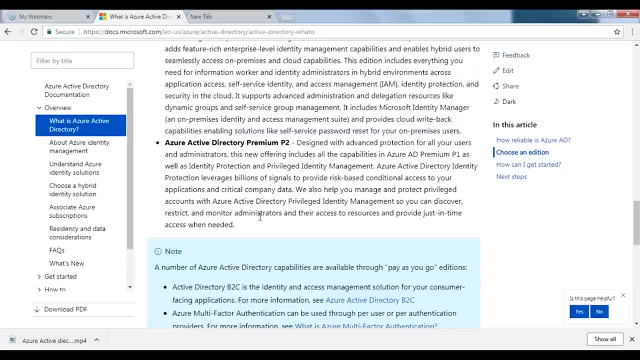 He can actually go ahead and read all these things and then go ahead and take a decision accordingly. Now what I'm going to do is I'm quickly going to go ahead and switch into the demo part. for that I need to go ahead and open my Microsoft Azure account. 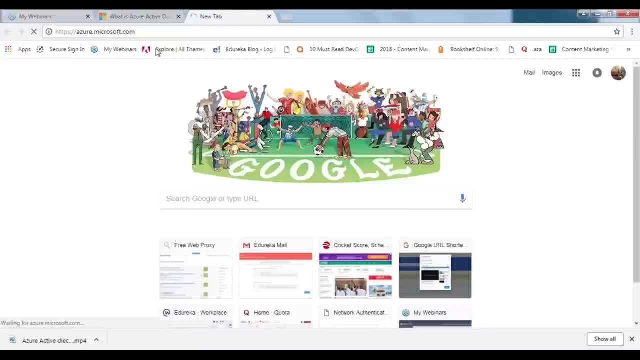 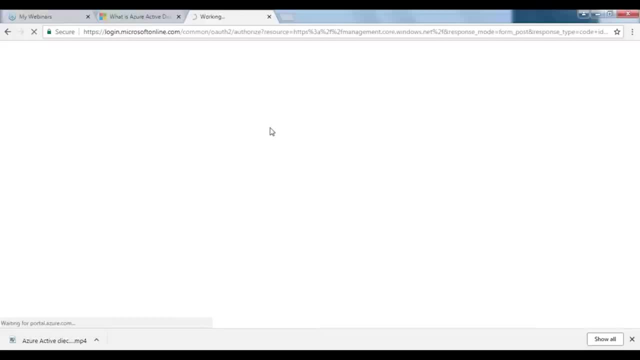 So let's do that. Well, my internet is kind of slow today, So it might take a little longer while than normal. I can click here on portal and there you go. It would ask me to sign in. I would be using a dummy account today for this so-called demo. 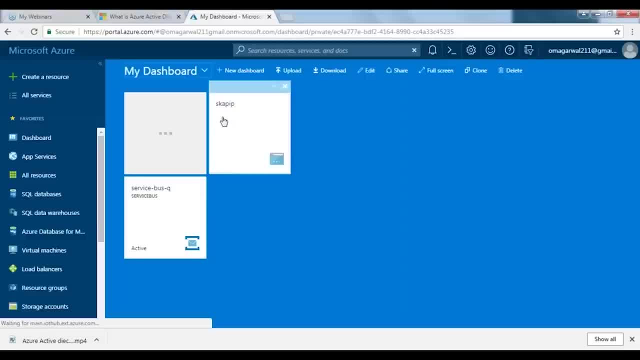 I wanted to give you an access to our view, to quite a few directories and all those things. So that is why I did go ahead and create an accountant, or certain Active Directory is created, or, basically, certain accounts created. Now this is how the Azure portal looks like for people. 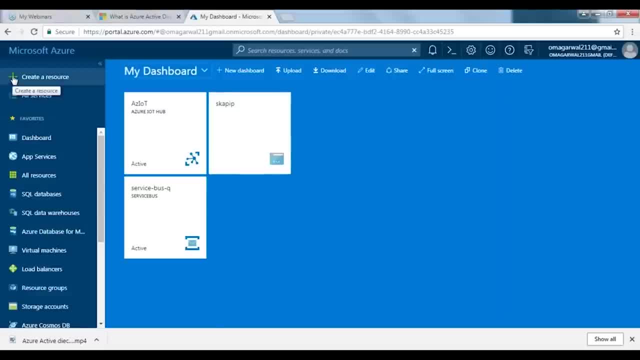 who are completely new. again, You have your dashboard here. apart from that, You can actually go ahead and create quite a few things, that is, your virtual machines, your data factories and all those things. for people who want to know all those things, They can actually go ahead and refer the other videos. 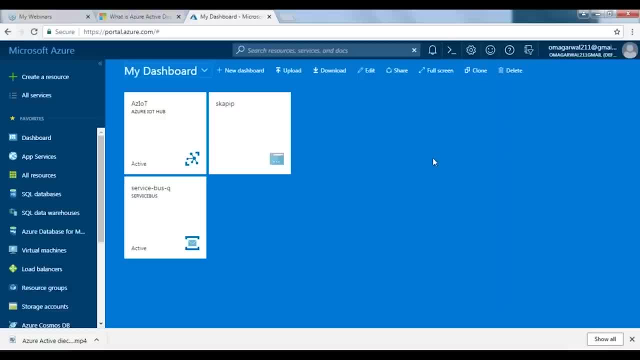 that are there in this series, and you would know quite a few other things as well, But as far as this session goes, we are here to talk about Active Directory, So let's head into it and try to understand. how do you go ahead and create Active Directories? 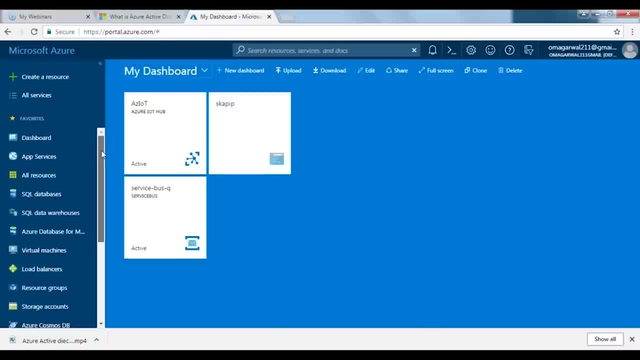 and all those things. now, how do you navigate to a particular Active Directory? now, if you scroll down here, you would be seeing an Active Directory here for people who have an account on Microsoft As your and have access to all these things. They would have an Active Directory by default. 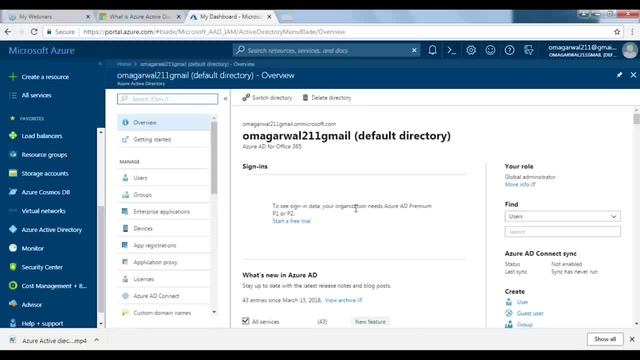 So you just have to come here and click on it And a particular dashboard would open up for you people as well. Now, this is how it looks like. you have all these things and overview getting started. you have users groups which you can manage and monitor. you have devices. 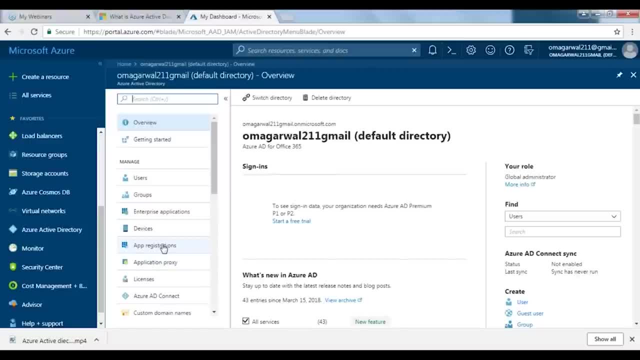 You can connect to your various app registrations. as I've told you, you can manage multiple applications as well. Now, in that case, what happens is, as I mentioned, you might be dealing with multiple applications. So a particular user- what applications should he have access to? what domains does he have access to? 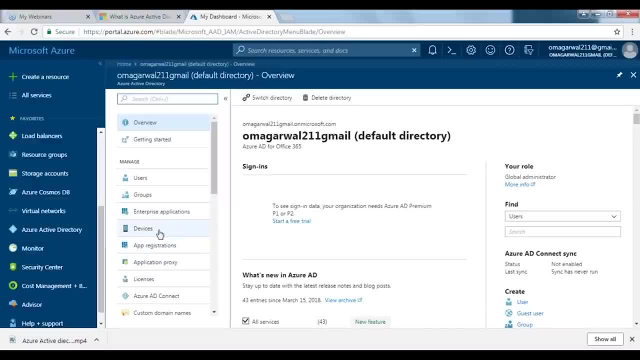 What are the devices that are configured? all these things can be controlled or managed from here, basically. So this is what your so-called Active Directory does. Now let's move further and try to create some users. Now, how do we do that? 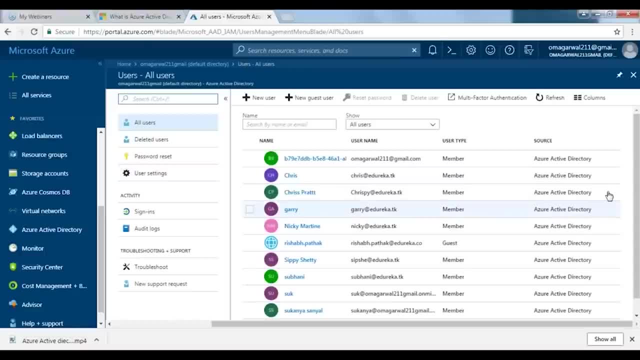 Well, I can click on this icon here and it would give you the list of users that already there. as you can see the quite a few users here. This was a demo account, So we did go ahead and create so-called users so that you can have a look at them. 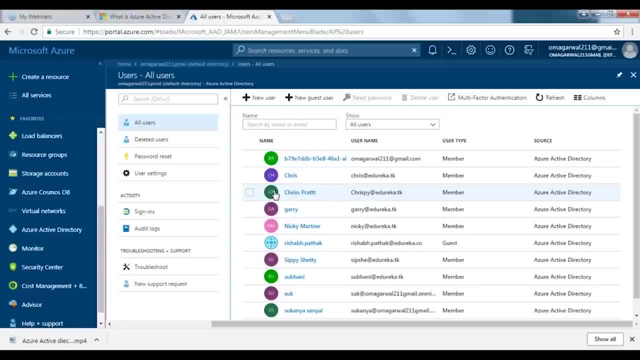 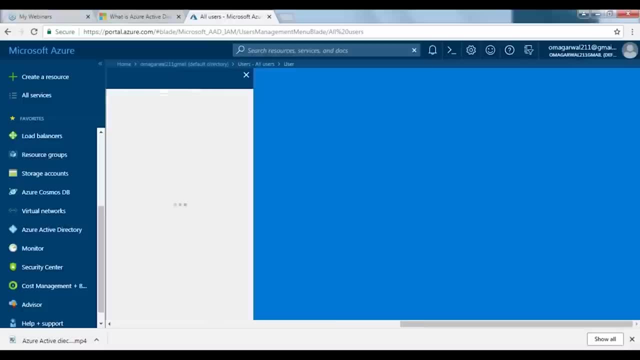 This is something that I created yesterday, That is, Chris Pratt. Now, how do you go ahead and create an account? I would be talking about all these things. to give you a start, You have to click on this thing- new users- And this window opens up. now again. 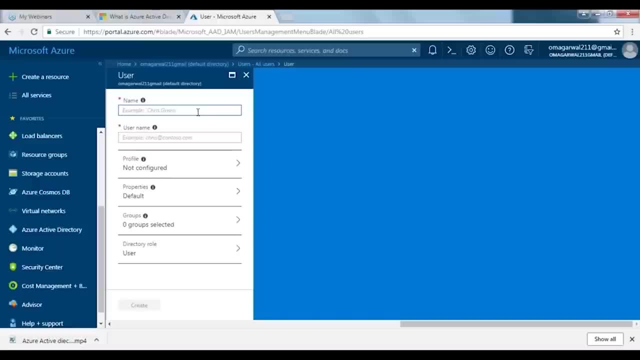 I'll have to go back and show you something else. How do we deal with all these things? Well, first and foremost, you need to give in a pseudo name or a name of the person for which you want to create a user. apart from that, you need a particular domain name or, yes, a domain name. 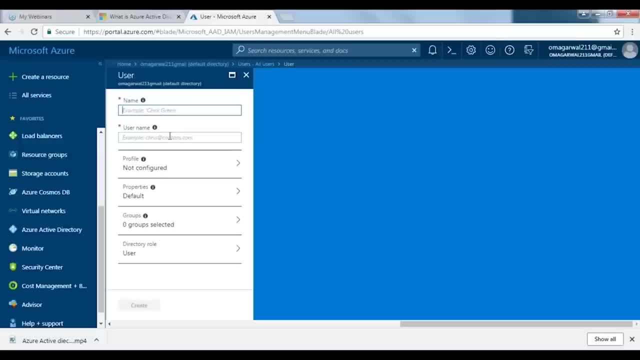 for a particular domain service. Now, how do we get that? now these domain services have to be registered with your so-called Azure Active Directory. So I have these accounts here, right? So I can use one of these accounts to just go ahead and create a particular user, suppose. 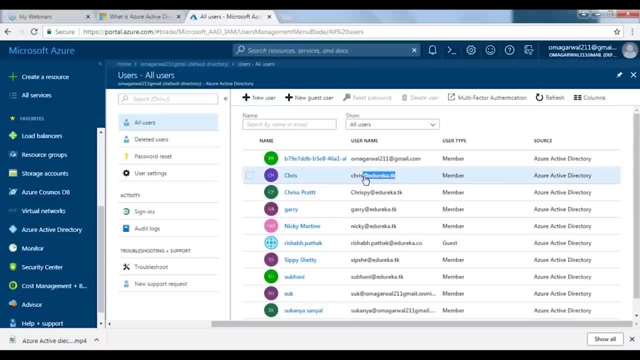 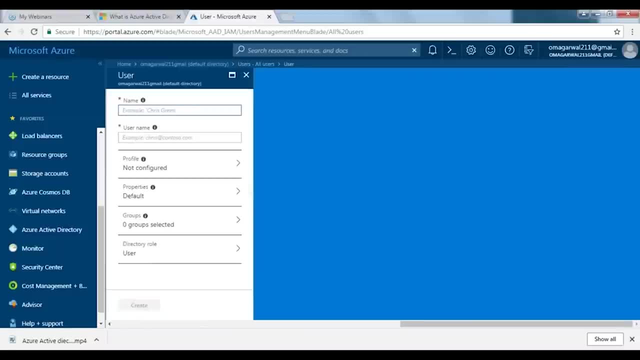 I want that user to be assigned, or maybe associated with this ID so I can select this domain service extension. basically, again click on new user. So what name should I give to this particular user? now, I am a huge cricket fan and recently I watched England's match. 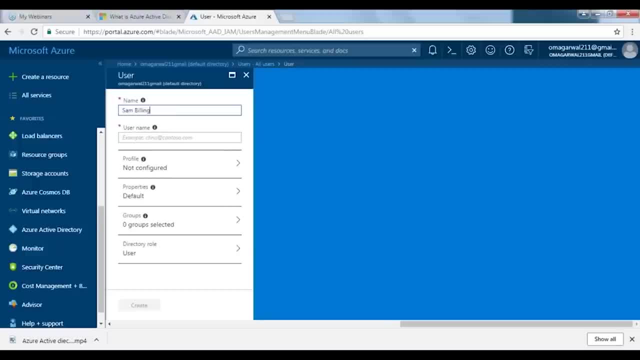 So let's pick the name of one of the players that belongs to England team. So some Billings and again, this is where I would be creating the user, say I say sample as a pseudo name and I given this domain details that is at the record, dot TK. 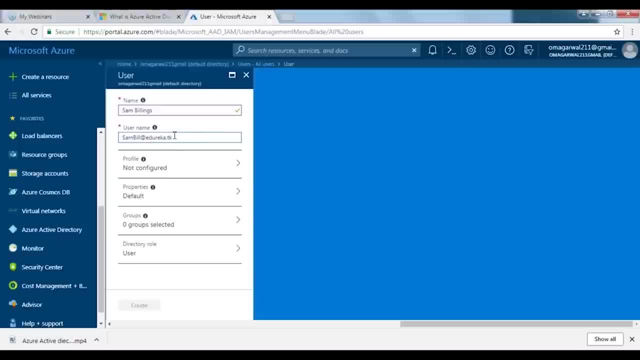 Now, this is something that is configured already. That is why I can use it and I can have an account. if I used an ID that was not registered with this as your account, I wouldn't have been able to create this user, because it would have given me a particular error. 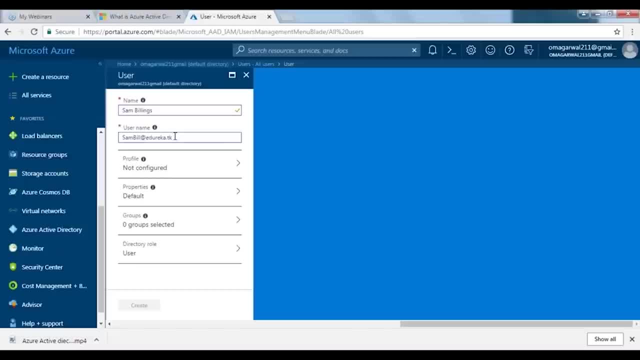 as we move further. So I would be taking a look at that as well, But for now, let's go ahead and create a legitimate user. that is this one now. It verifies whether the name is proper or not. name is something you can use in any which way you want to. 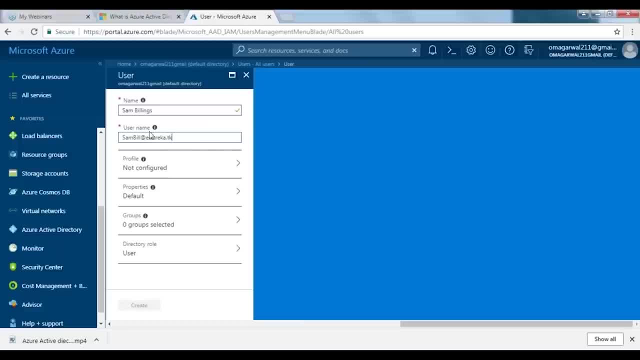 but your username has to be legit and valid. So I have these details which I've entered. configuration: not required properties can be default, and if I have to assign him a role, I can click here. You can see the name is verified here as well. 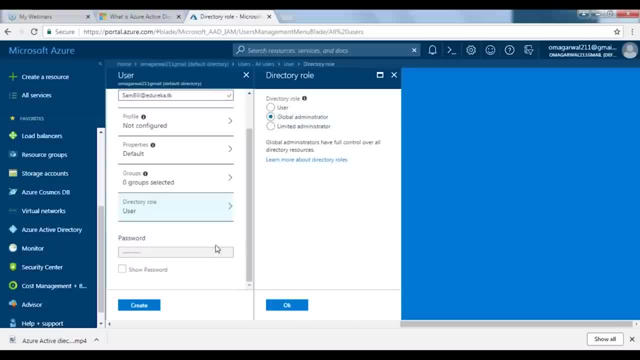 Let's make him a global admin. maybe- and again, you'd be given a password here. If you say show it would show you the password and I would suggest that you note it down, because you would be required to go ahead and login and in that case you might be needing this password. 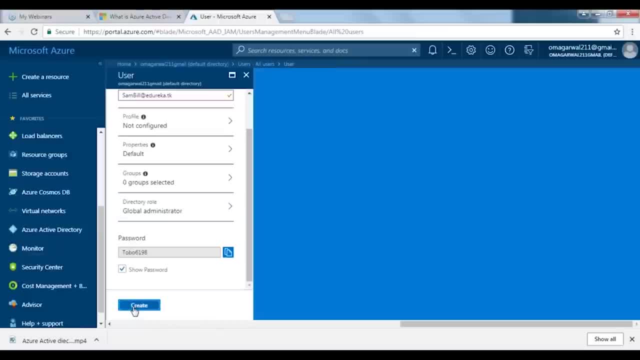 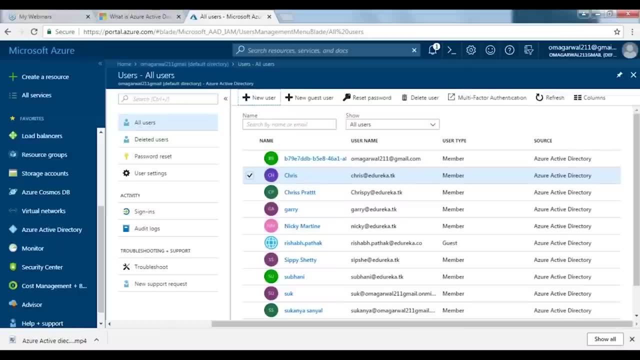 So, a suggestion that you noted down, I say okay here and I create the user now. it might take a while, because at times there are certain things that take a while, but in this case it has happened pretty quickly. So, as you can see, we've gone ahead and created a user. 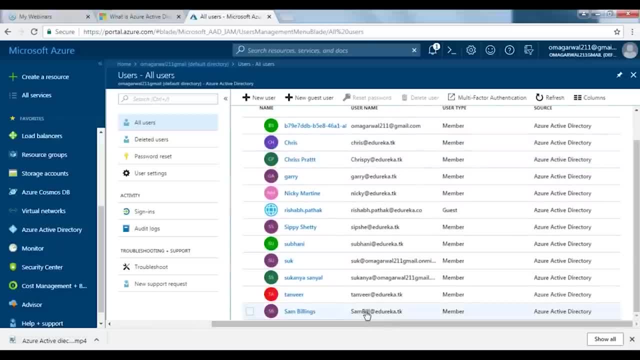 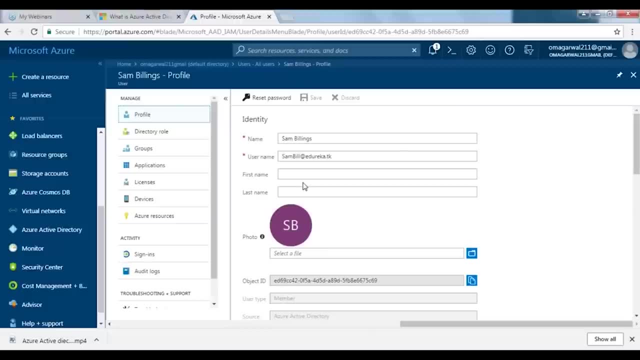 His name was sampling, if I'm not wrong. So yes, there you have this account which is sample, and if you click on it and open it, you can have access to that account where you can enter in other details What applications that are there under this user. 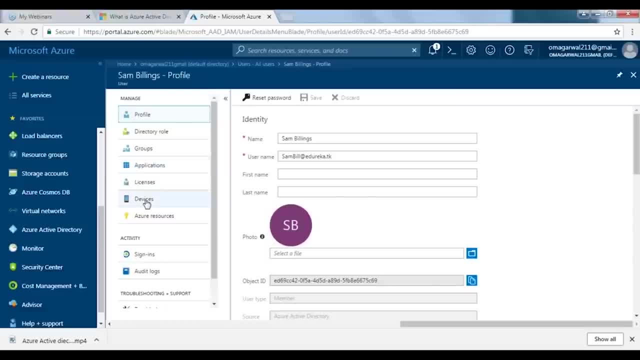 and what applications do you want to assign, which devices do you want to configure and all those things. if you scroll down, you have some other options as well: sign-ins and audit logs. now I won't get into the details of these things, but you can assign all these things to this particular user. 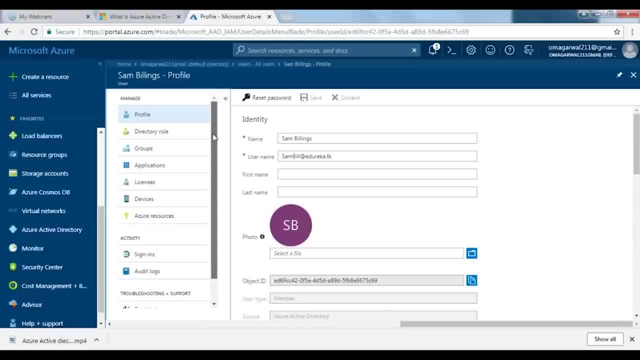 as well. So, yeah, this is what the user looks like, and you can actually go ahead and log into this as your account through this user profile As well. we can do that. what I'm going to do is I'm going to go ahead and create or open an incognito window. 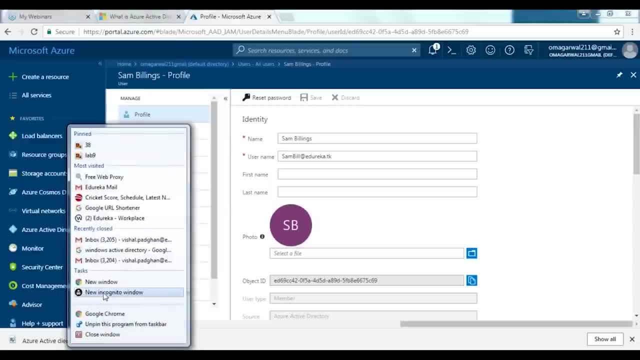 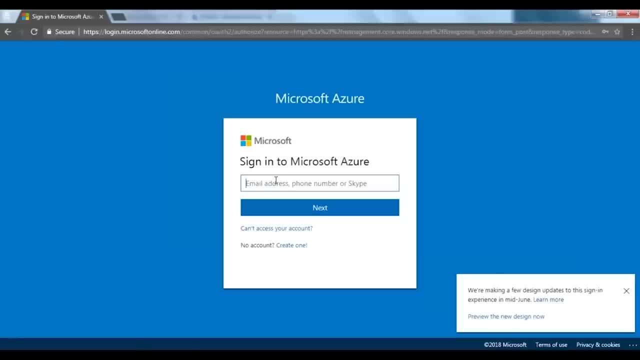 where I'm going to go ahead and log in as this user- Let's just say cognito- and Now, if I try to log in, I would have to enter in the details. I've actually gone ahead and tried logging in, but I've forgotten the credential details. 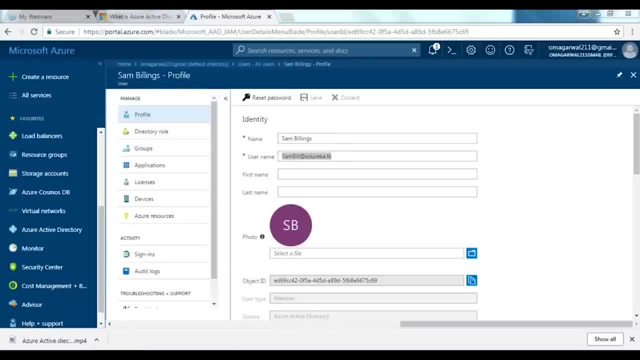 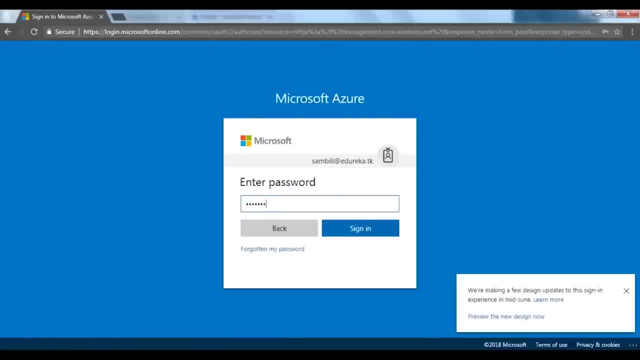 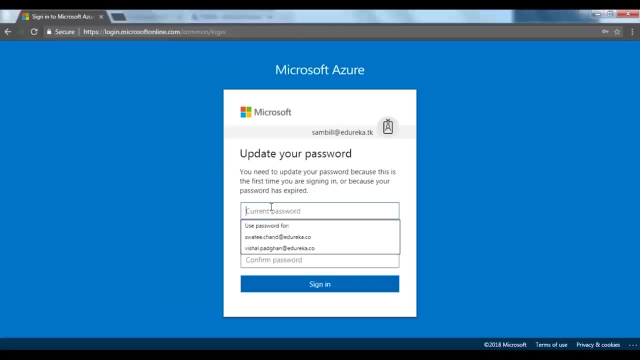 So let me just quickly switch to this window, copy this email ID and again switch here. So this is the email ID which we have, sample next, and my password was: I hope it is right. Yes, So when you log in for the first time it would ask you. 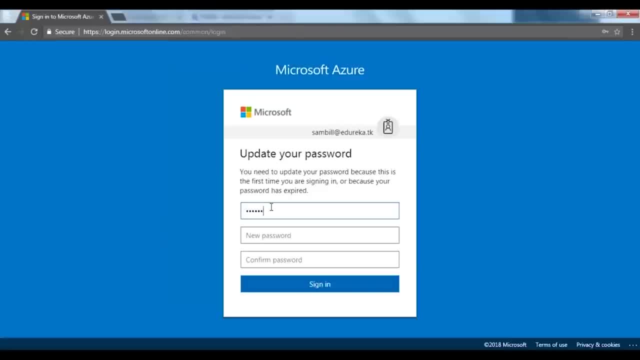 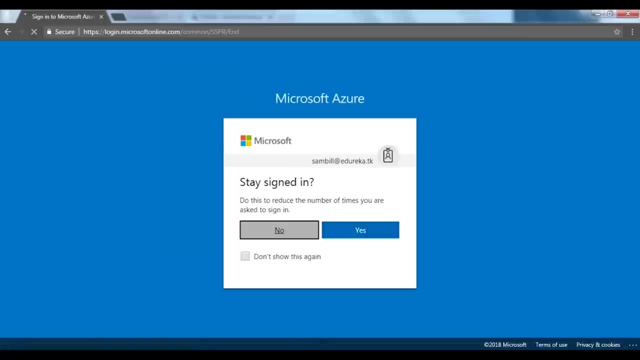 to enter the current password And then you can enter the new password, Let's say, and then you re-enter the password They were and you sign in. So what happens is you enter into this portal as a fresh user. See, I'm a completely new user. 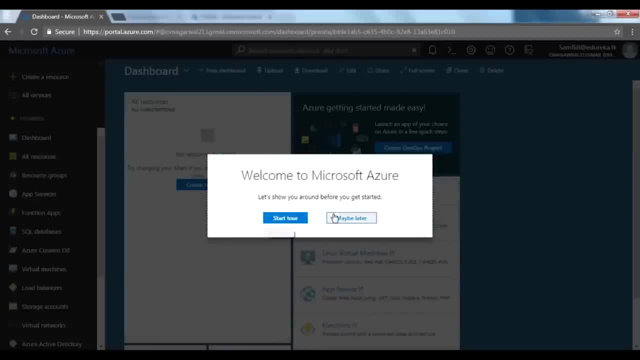 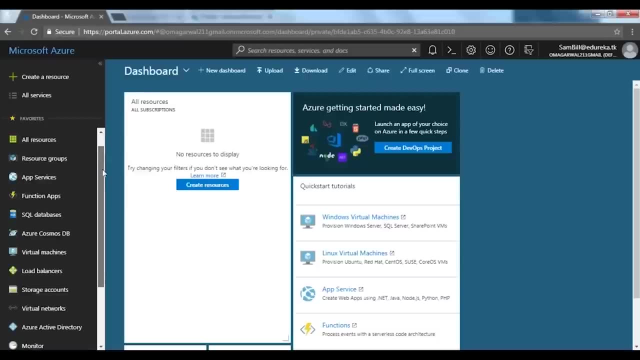 and it says: do you want to start a tour? but I don't want to do that, So I would just say, maybe later. there you go, You have your fresh dashboard, There is nothing pinned here and everything is completely new. So, yep, you've entered in as a completely new user. 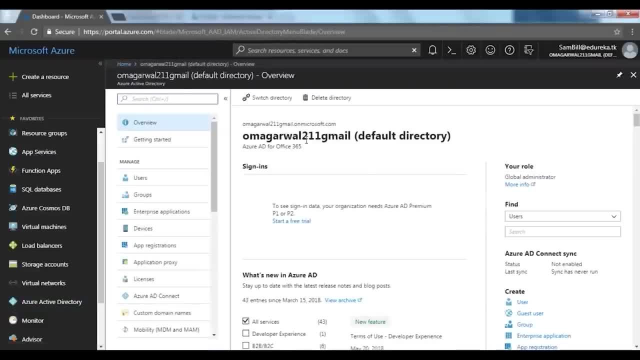 And this is the Active Directory where I'm assigned to. that is my previous Active Directory. as you can see, This is what we have here to offer. So, yes, as a user, I have certain privileges and I can have access to this so-called portal. 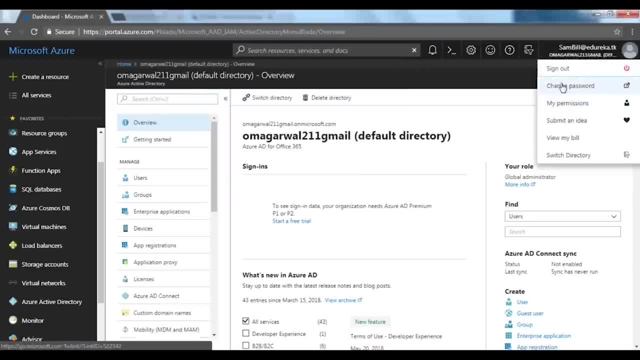 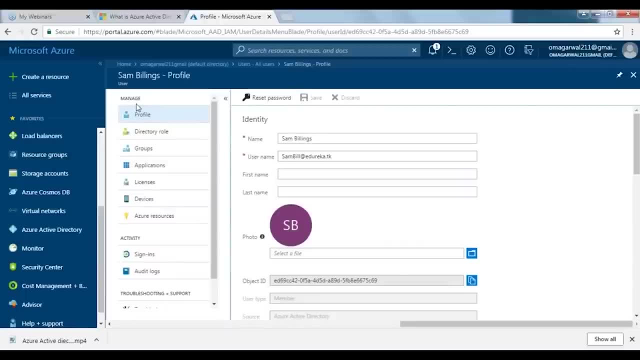 So this is something I wanted you all to see, the quite a few other things which we are going to go ahead and take a look at it, But for now, let me just log out and close this tab. back here The other things I want you to understand. 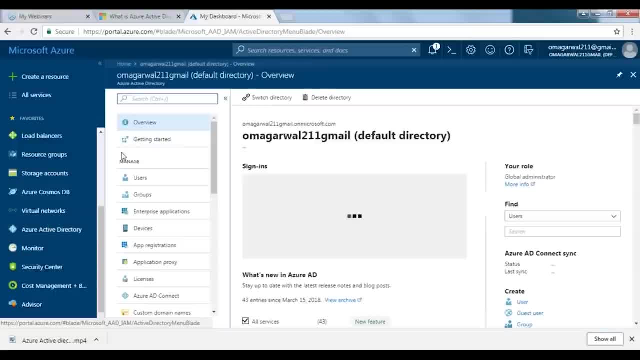 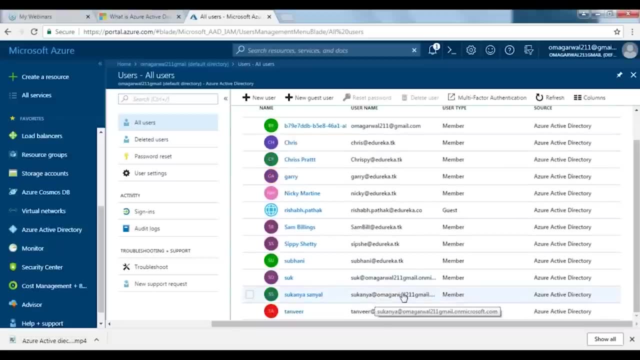 and those things are. if I come here, what you can see is we have certain users here, right, There you go. Now, if you take a look at certain email IDs, you can see these email IDs. Now, these are quite huge email IDs, right. 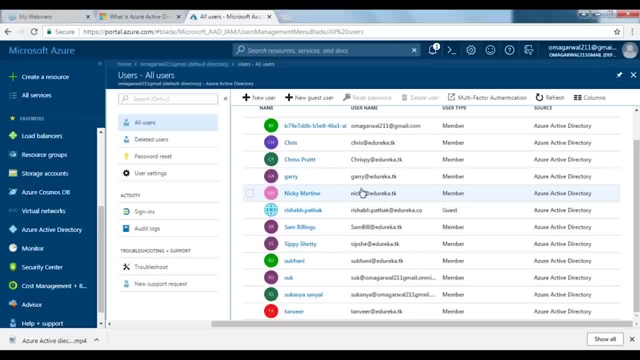 What happens is when you do go ahead and register your domain service, you register that domain service with Microsoft Azure account, and when you do, when you do go ahead and create users, you would not want to have such use names. That is say, for example: 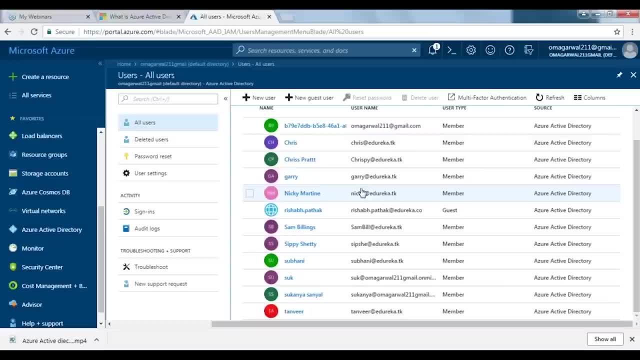 we shall at Microsoft something, something, something, something that can be long right and that is complicated to handle our manage. So instead, what you can do is you can provide them with pseudo identities or pseudo IDs as well, so that the process becomes easier or simpler to handle. 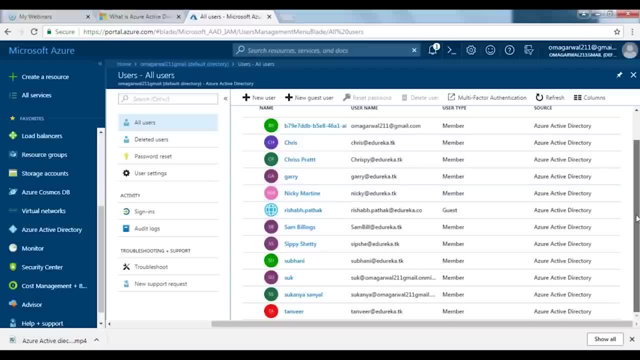 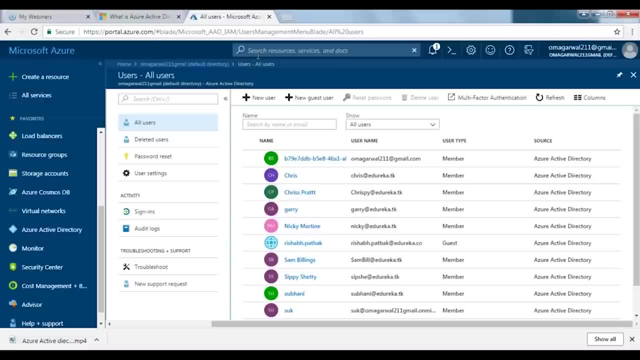 Let's try to do that and see how can we do that. Can we just go ahead and assign a particular domain name or a domain service when we just go ahead and create a new user or all those things? so in order to add a particular domain? 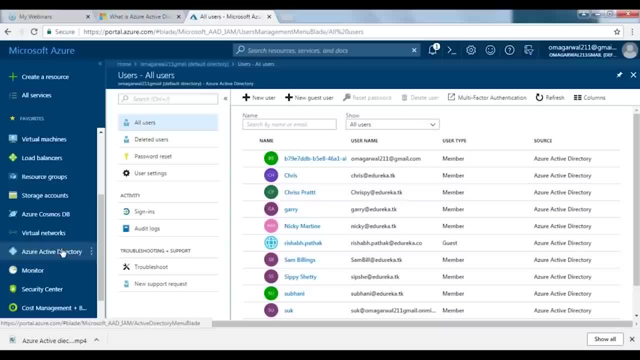 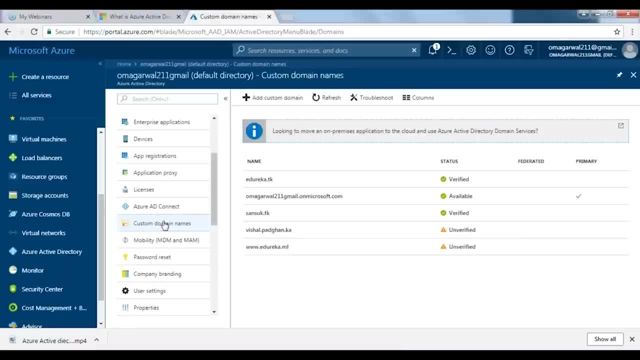 what you have to do is you have to go ahead and again, where is my Active Directory? here it is, and I just kind of scroll down. You can see custom domain names, where you can actually go ahead and add domain names, but there are certain catches to it. 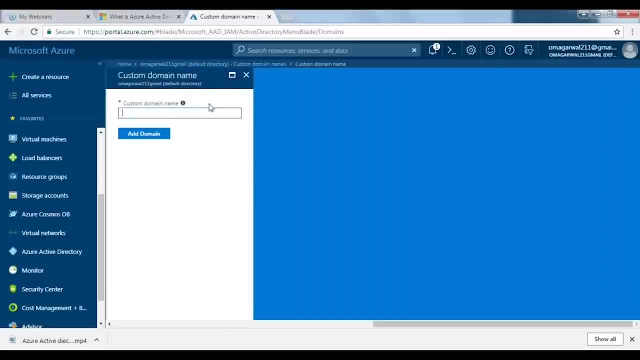 Let's try to understand those. now it would ask me to enter a custom domain name and I say demo domain Maybe, yeah, and let me give it some extension. now again, let me tell you that this is a demo practice and it won't take in this particular domain name. 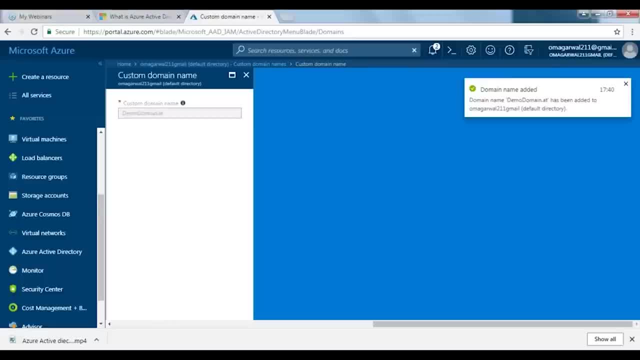 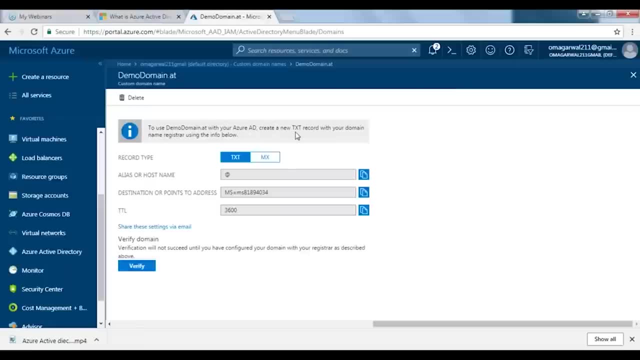 I'll tell you why, but first let's just try to add this domain. Yeah, the domain name is added, But, as you can see, to use demo domain dot at with Azure AD. create a new text record with your domain name registrar using the info below. 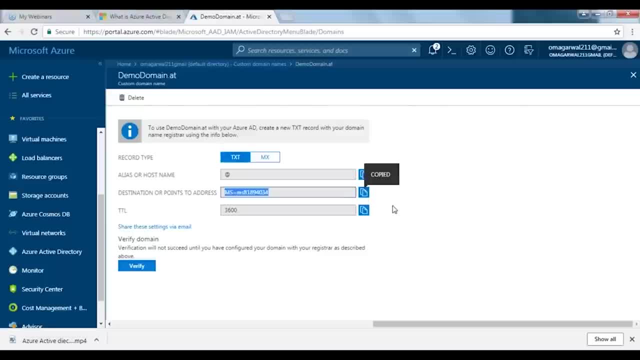 So if I say text, I need to copy this part and I have to actually go ahead and add this to my particular domain name. now I won't be going ahead and doing that because that is something that we are not discussing here, because for that we would be needing some. 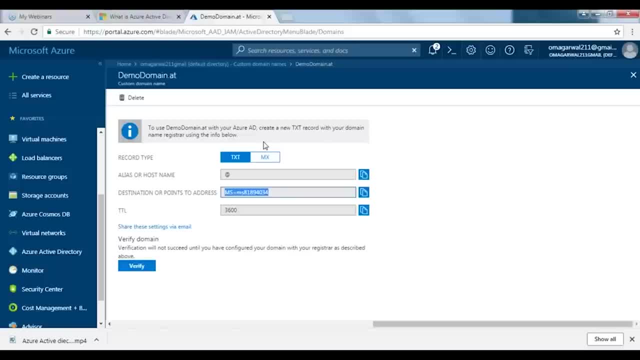 of the domain name, which I do not have right now with me. So if you do go ahead and try to add a particular domain name, you need to have that particular domain. that is suppose I'm using a particular website or I have a particular organization. 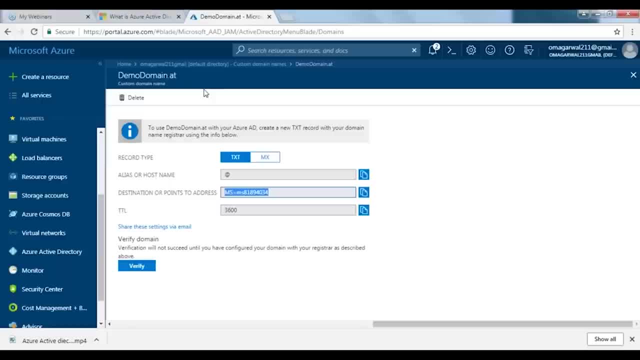 which has a particular website or a domain name that is XYZ at XYZ, dot-com or something like that. So I need to make sure that I go ahead and register or have access to that particular domain and then I need to go ahead and attach this particular text to it or authorize this text. 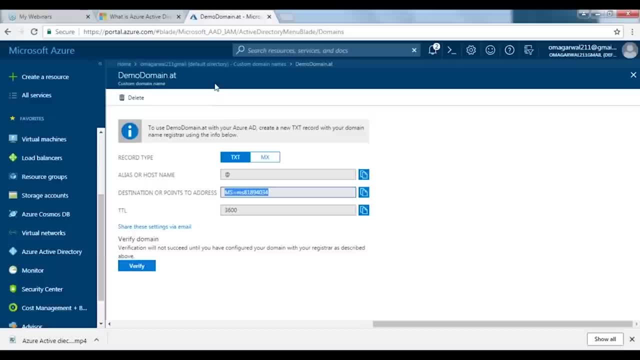 with it so that I can actually go ahead and confirm with Microsoft Azure that, yes, I have an access to that particular domain, and only then can I go ahead and use this particular domain with my Microsoft Azure. If I click here on verify, it would give me an error. 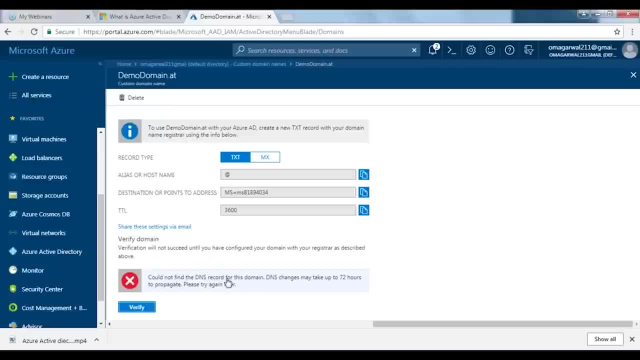 that I'm very sure of see could not find the DNS record for this domain. DNS changes may take up to 72 hours to propagate. That means I have 72 hours to go ahead and add this particular text message to that domain and so that I can verify that, yes. 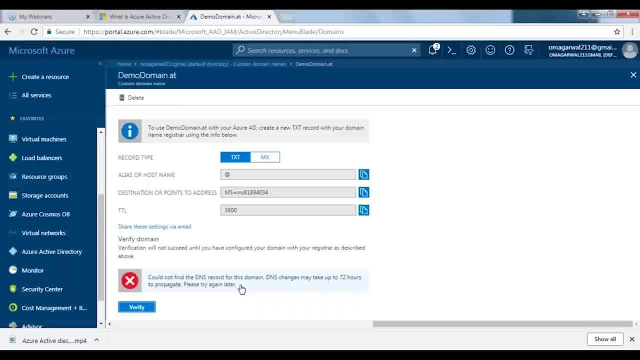 this domain is legal, But in this case it isn't. I just took something for the demo purpose or for the reference sake, And this is the domain that I might have or which I can actually go ahead and use. So, yeah, this is how you actually go ahead. 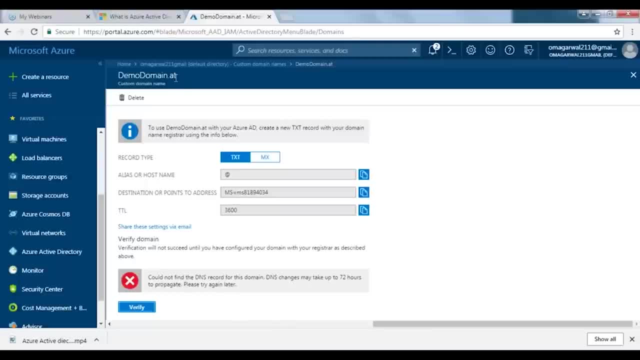 and add a particular domain and you can actually go ahead and create a user as well. What you have to do is, when you do go ahead and register this particular domain, you can just go ahead and follow the processes, like creating a user, which we did in the previous case. 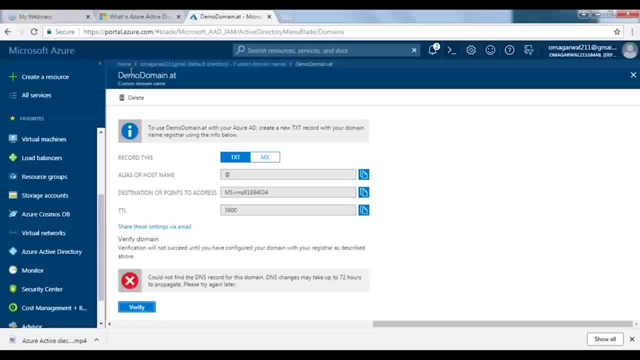 because that was the registered domain when I use that so-called edurekatk. It was registered with my so-called as your account and I could actually go ahead and register that particular user, But in this case I cannot. but yes, if you do go ahead and create a particular domain. 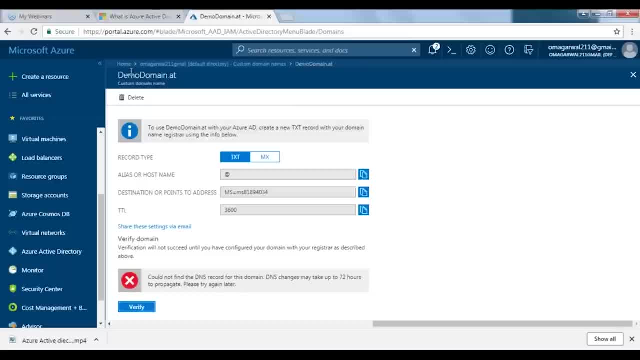 or you want to go ahead and create a particular domain or register a particular domain. make sure that it is valid and it is under use, and you can actually go ahead and register that particular domain by using this particular process. So yeah, this is how you actually go ahead. 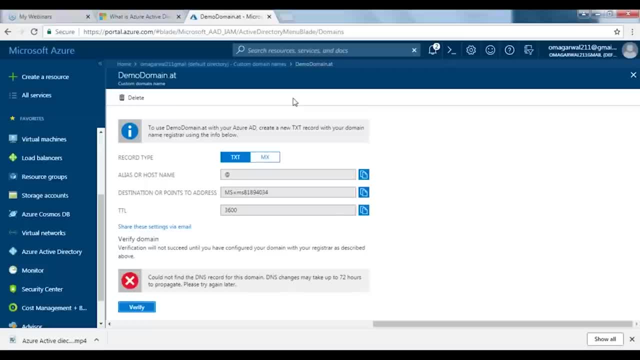 and do all these things. now, when you have this particular domain which is not registered, and if you do go ahead and create a particular user on it, what happens is your Microsoft Azure would let you create that user, but the credentials or the access that user has is as a guest user. 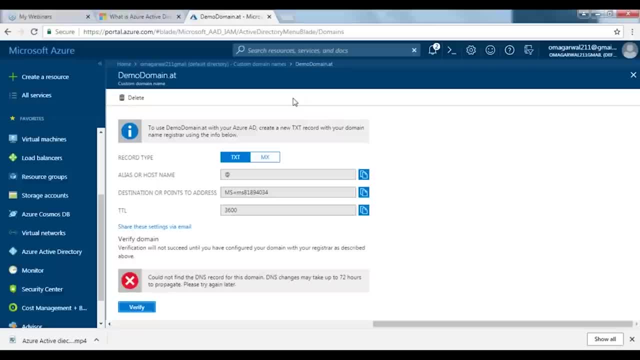 because your Microsoft isn't sure that this domain which you just created is actually registered or something that you can actually go ahead and use. So that is one point which you need to consider. now let me just quickly go back to my active directory and see if there are anything. 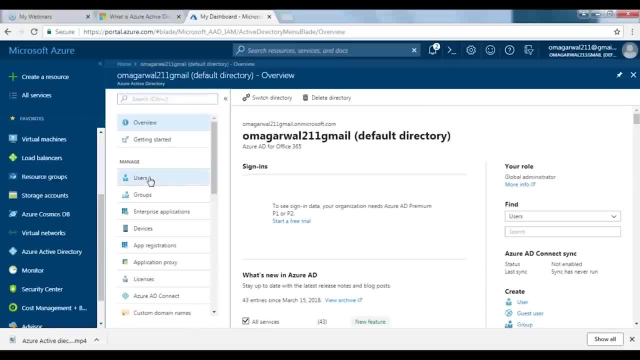 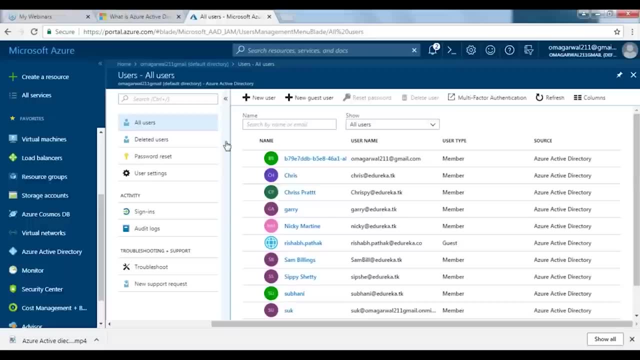 or any points that I need to discuss with you, or something that we have messed up on. So what I'm going to do is I'm going to talk about something else called as creating an active directory, or can we create multiple active directories? That is a question. if you ask me, I would say yes. 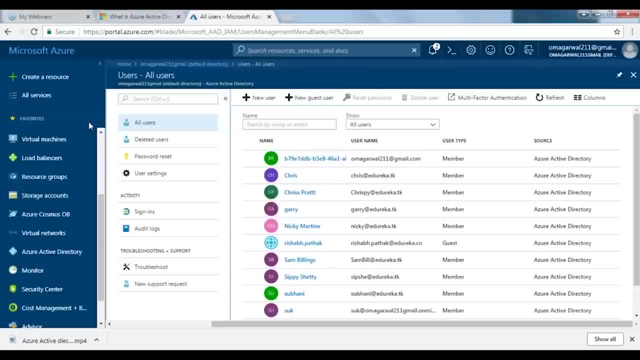 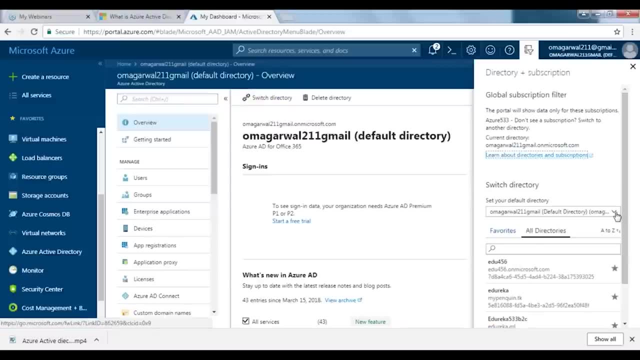 definitely, You can create multiple directories. Now, as you see here, if I go to a particular directory, I would be having an option called as switch directories. Now, if I click here, I have certain options from which I can pick a default directory. 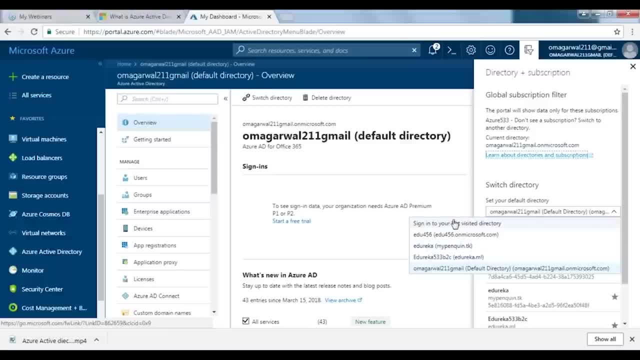 now, in my case, I have quite a few directories which I can actually go ahead and choose from, but I want to give you all a demo as in how do you go ahead and create one, because these are something that we have created for the practice purpose. 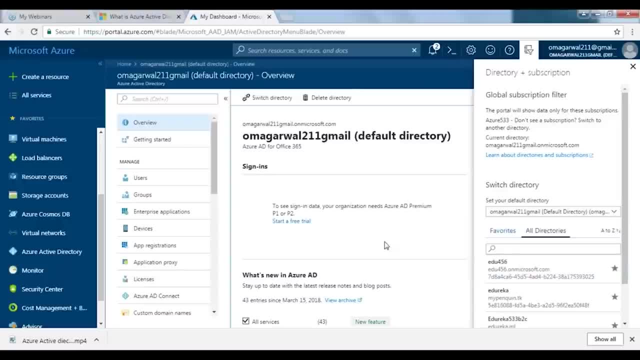 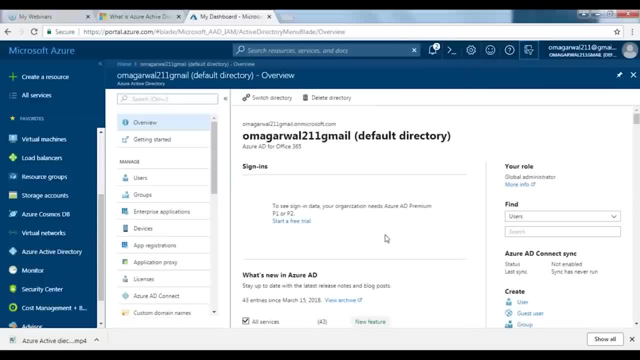 or certain usage purpose. So let's go ahead and create a fresh one. So how do we do that? Can we just go ahead and create one? Yes, definitely We can create one. If you just scroll down, you have certain options here. 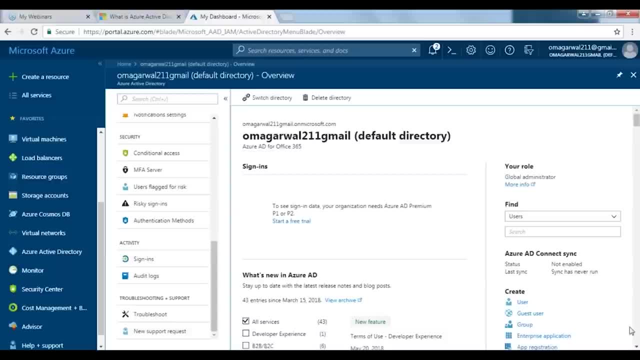 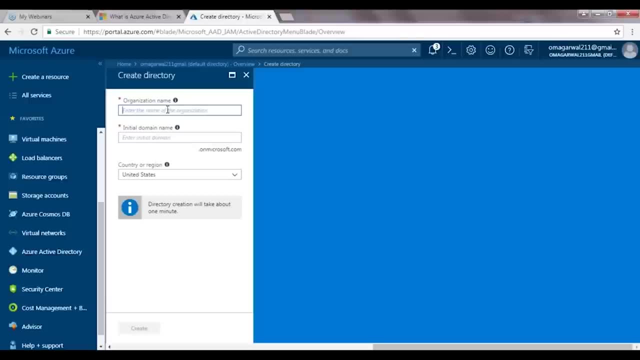 We had an option of creating a new directory. Let me just go ahead and see where that option is. See as this option create a directory, So let's start by giving it certain names. a edureka- 1, 2, 3, 4, not 1, 2, 3, 4.. 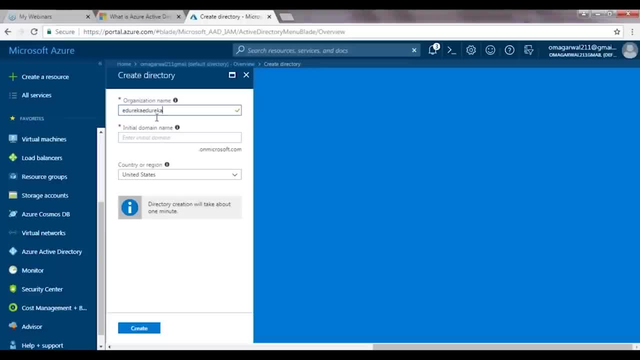 Let's call it say: edureka, edureka- Maybe is it there Yep, and what should be the domain name: edureka 1 2 1. edureka 1 2 1 state. well, since I'm from India, that stick to India. 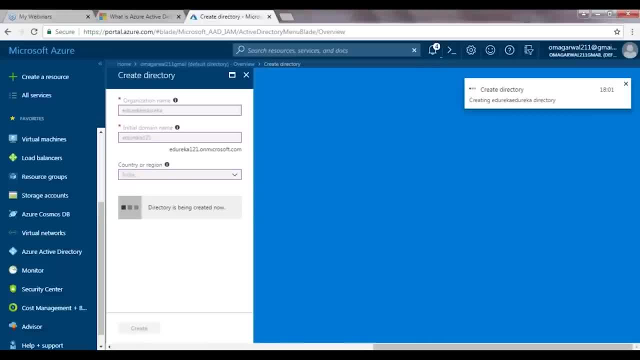 and I say create now. it might take a couple of minutes when you just go ahead and create this so-called directory. So, yep, meanwhile you bear with me and there you go, You have your directory here. You can just click on this thing to manage your directories. 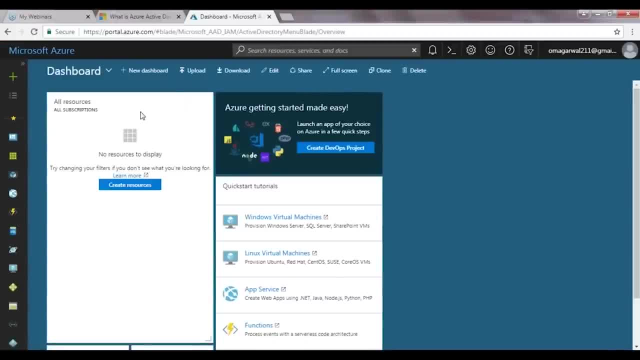 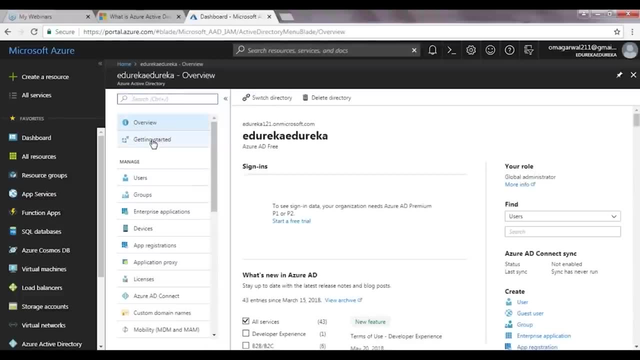 As you can see, it's a completely new directory, which is fresh and new to use. that means, as you can see, it's edureka, edureka, and if you click on any one of these things, you won't be having anything else. now, in my previous Active Directory, 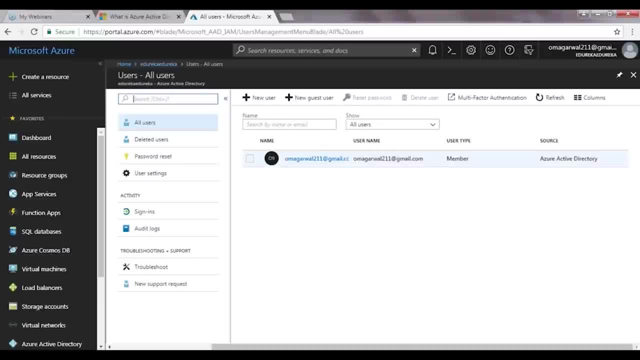 I had so many users and if you come here you would see there's just one user: main admin. I do not have anything else or no other user whatsoever. That means this is a fresh directory, like as you can see if you just go back to the direct edit option. 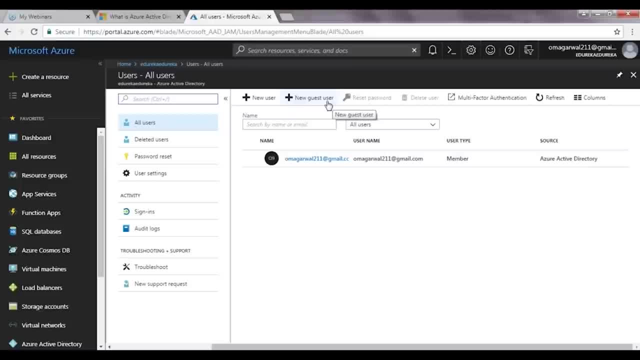 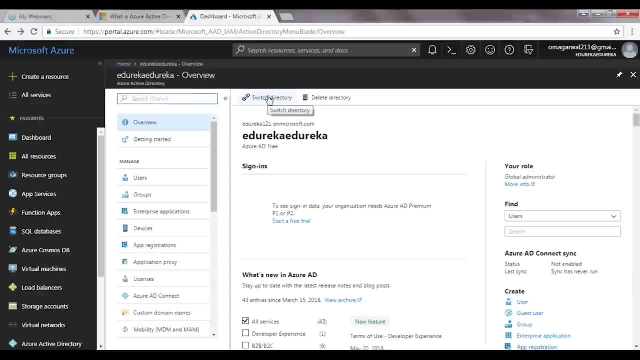 you'd be having an option of resetting your so-called directory, and you can do that as well, but I do not want to do that for now. I can just click on this and I go back. see, here's the option. You can click on it and you can switch the user. 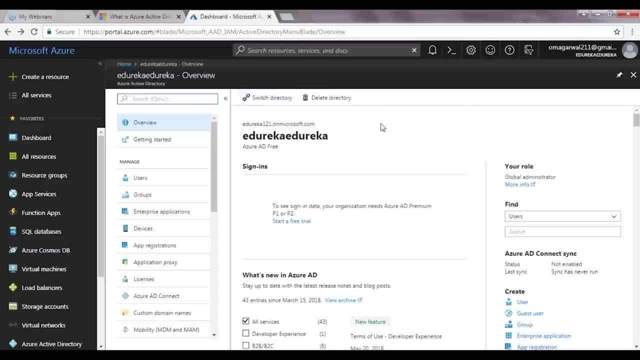 So, yeah, you can use multiple directories and you can have multiple users for these directories as well. Now I can just go ahead and create users for this directory as well, but I won't be doing that now, since I do not need this directory. 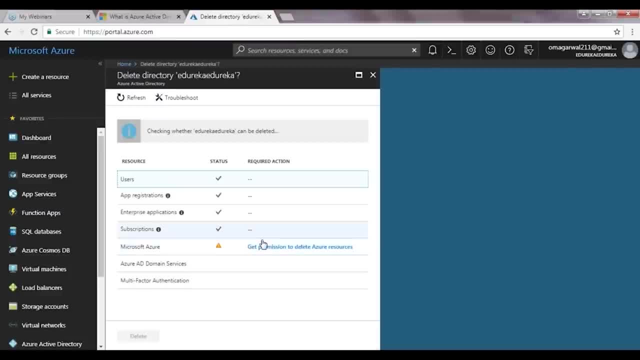 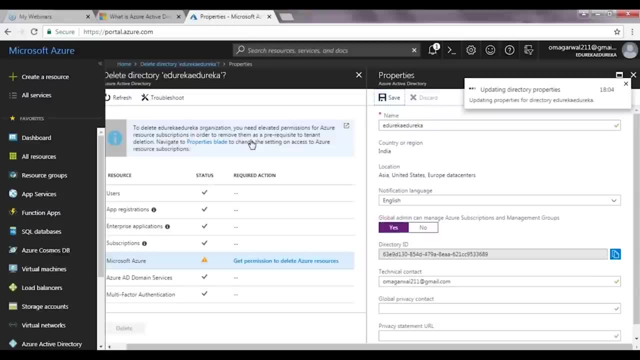 I'm just going to go ahead and delete it. So I click on this I can. I do not have permissions, probably, so I click on it and I ensure that permission is granted, I say yes And I save changes. it might take half a minute. 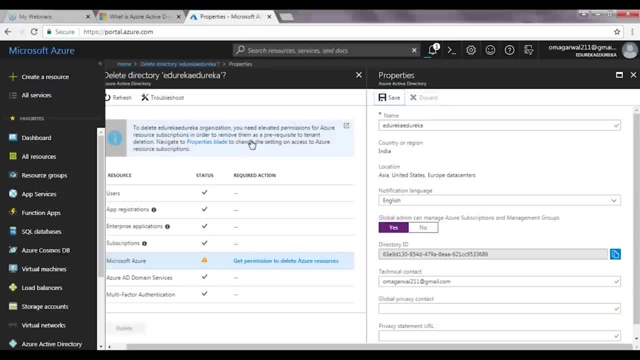 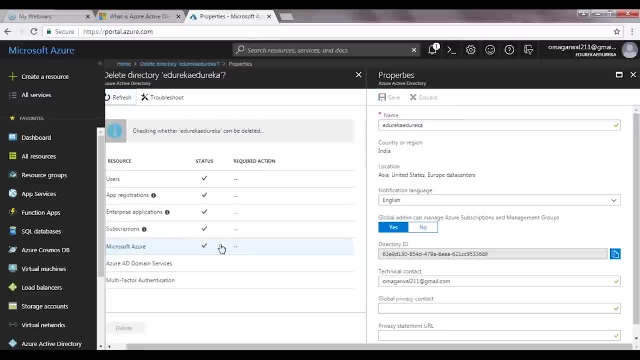 to update these properties, or if the internet is slow, it might take a longer as well. They see the changes have been updated. If I refresh this thing, the access is given to me. I can just. I don't want to delete the dashboard. 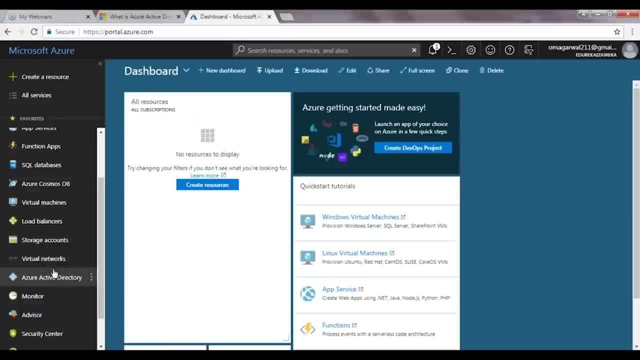 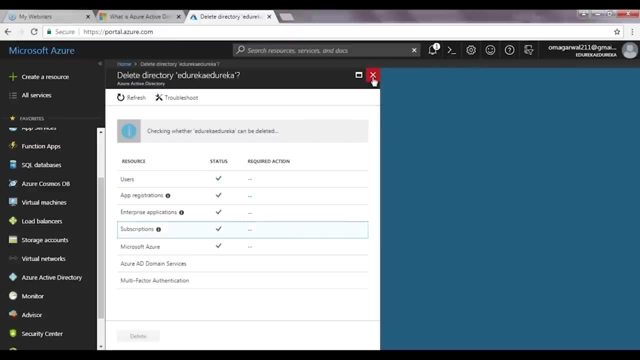 I just want to go ahead and delete my so-called active directory. So I do not have an access to my domain services, because of which I'm not able to delete this account. But yeah, you normally have an option where you can actually go ahead and delete this directory. 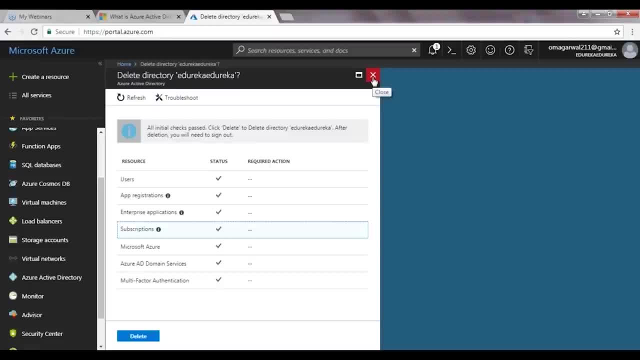 So, yep, you can go ahead and do that as well. So this was the demo about active directory as in, how do you go ahead and create a user, How do you create a particular domain space or domain service? Basically, how do you go ahead? 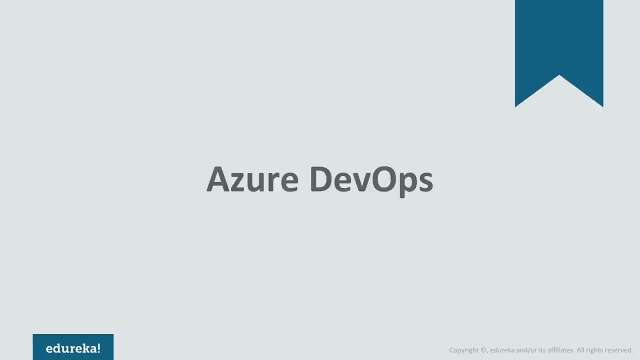 and create multiple active directories. We want to know about what is devops. What are the services available in Azure to handle the devops? So let's first learn about what is devops, All right. So first thing is, when we say what is devops, 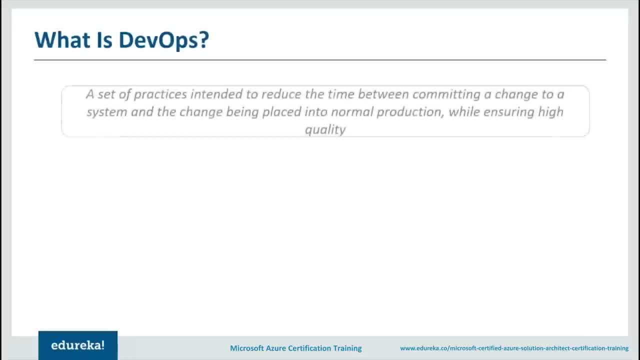 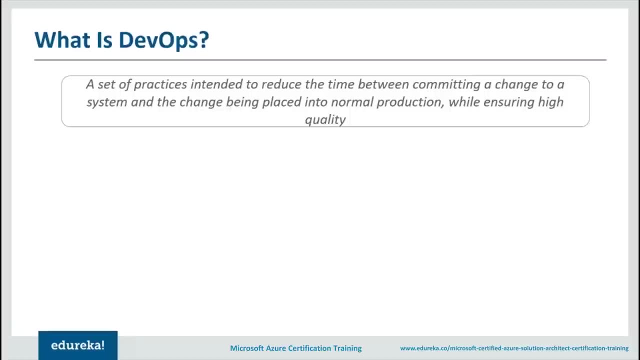 So basically, just for the definition perspective, it's a set of practices intended to reduce the time between committing the change. So let's say you are building an application, if you commit a change, committing this change and taking it to the production is a very long process. 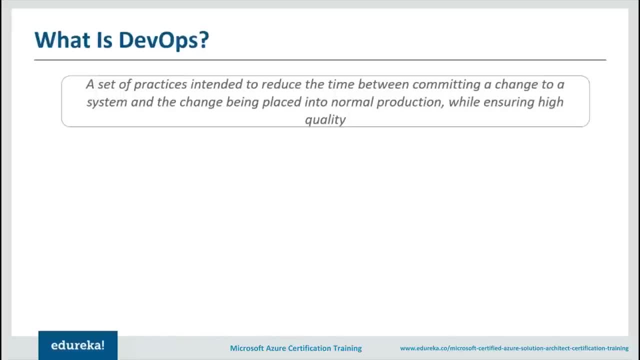 But then devops means that once you commit a change and finally taking that change to the production, devops is something which can help you reduce the overall time and provide you a standard set of practices using which it makes your deployment very, very smooth. Of course, it can help you maintain high quality. 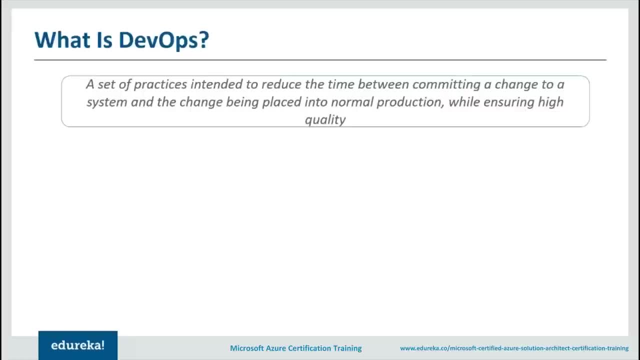 in your application. This means if you want to do testing, if you want to do some reviews- all these things basically, are covered in the devops. some of you guys might be coming from the development background, some of you might be coming from the operations background. 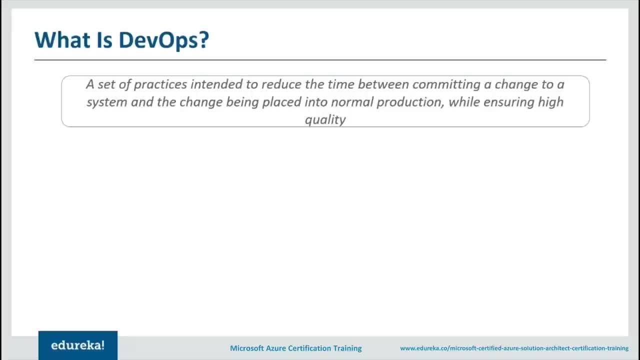 So this is a place where both of us meet together: the developer, the operation guys. They come together and work together. so far, in a normal work environments. If we are not into devops, what do we do? the developers have the responsibility of, you know, doing some coding, building that. 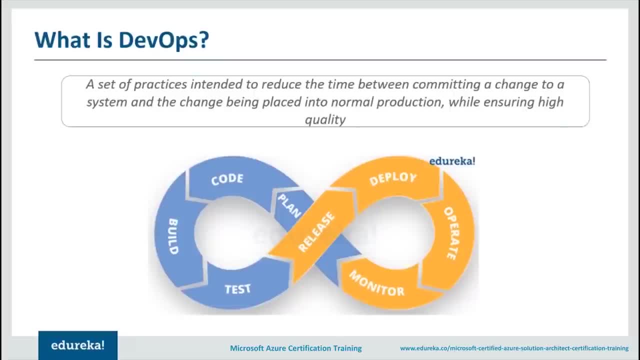 and finally putting it into a source control. Once you put it into a source control, the test team will actually take that source code, do their own builds and start doing the testing on top of it. Now, once they are doing this testing, they'll do some test stuff. 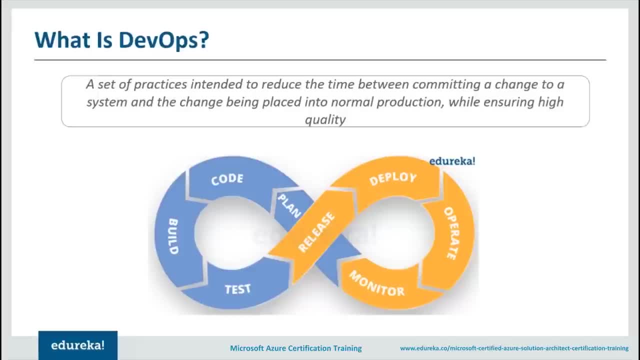 push it back to the development team, and this to and fro keeps happening. once all this testing is complete, Then you put everything into the operations bucket. Then you tell them that yes, we are done, We have completed everything. now you go ahead and make a release of it, do the deployment, do the operations. 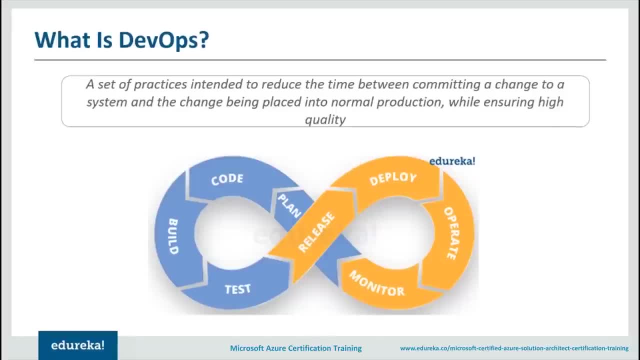 on top of it, Keep monitoring the stuff. if you face any challenges, then inform the development team. Now this used to be a very siloed approach, So developers and testers working separately, the operations guys are working separately, and there used to be a lot of friction between these two areas. 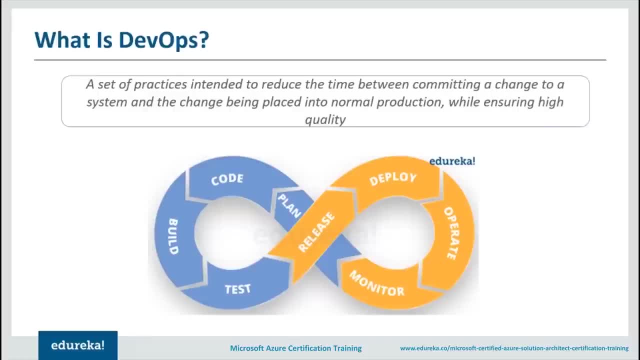 So now, when we come to the devops environment, these two set of people, they have actually become one, which means you together do the development, you together put it into the source control, you do the testing and finally you go ahead, because it's not just individual people. 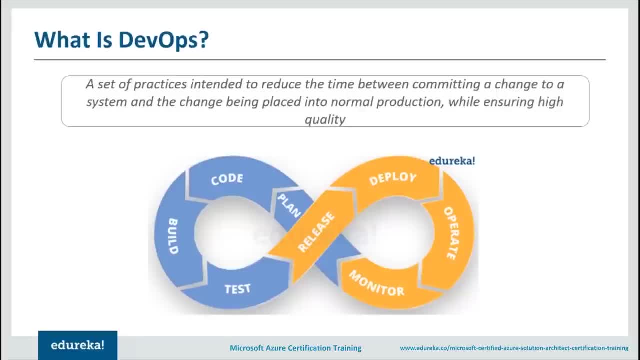 It's a team, So you go ahead and do the release, you do the deployment and finally do the monitoring, so that you know- because if you have started developing something, you know that- what is the best thing you have developed and how you need to handle that. 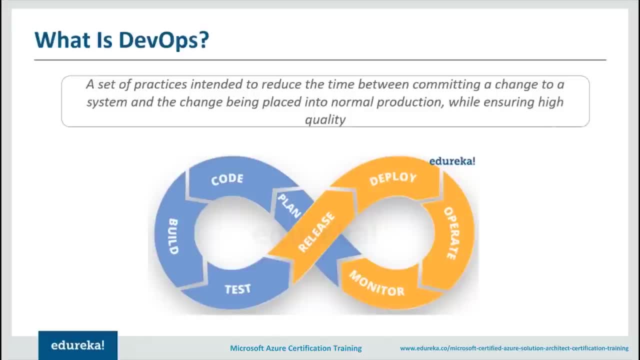 So this is one area where the developers and operations- They come together and work as a team, friction can be reduced, the time to Market becomes faster and the quality even becomes much better. do not worry if you do not get the hundred percent of what is happening. 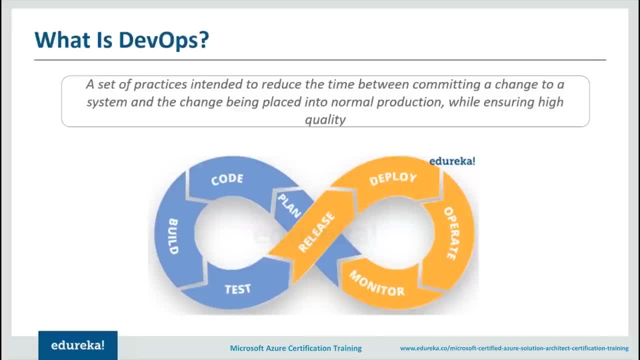 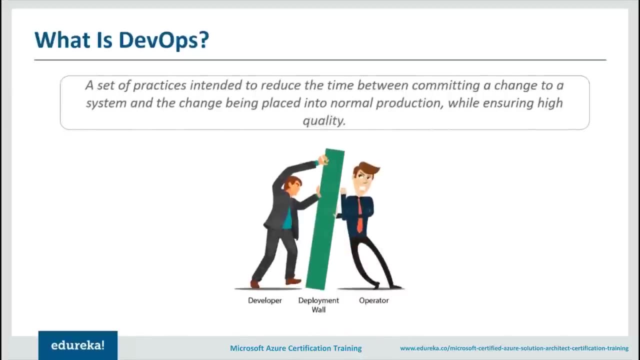 but then the overall idea to understand is that now the developers and the operation, they come together and work together as one single team. just for this, you know a very small diagram: the developers, they'll build something, they'll start pushing it to the operations team. 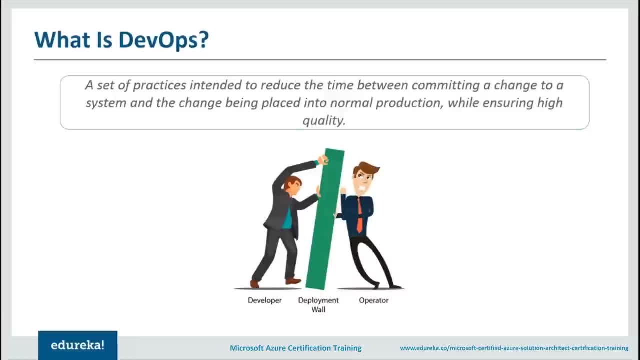 So you do the deployment, you take care of everything, the operations. if they'll face any challenges, they'll start pushing it back to the developers team looking at a very small thing. Okay, if I can solve something very quickly, that's fine. Otherwise I'll start pushing it back to the developer team, saying: 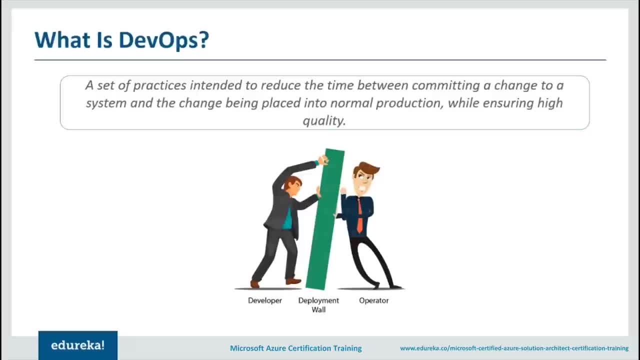 that this is not working. So there is a lot of friction and there is a lot of miscommunication. that happens in this kind of environment. way to solve it is that both of us, the developers and the operations- work together as a team. Okay, I hope you got some glimpse of what is devops. 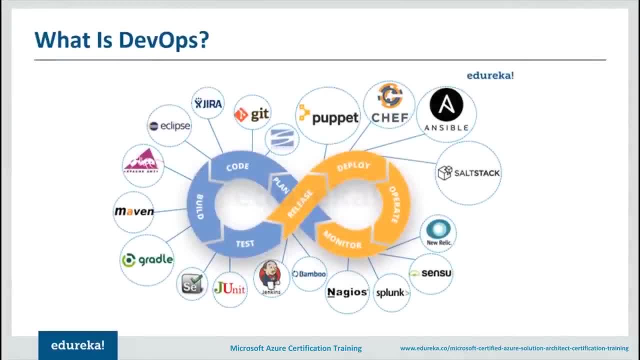 and now we're going to talk about some tools which are available in devops. when we say devops, Each of these areas are covered by different kinds of tools. So if you are doing some development, you might use, let's say, Eclipse. You might use, let's say, Visual Studio. 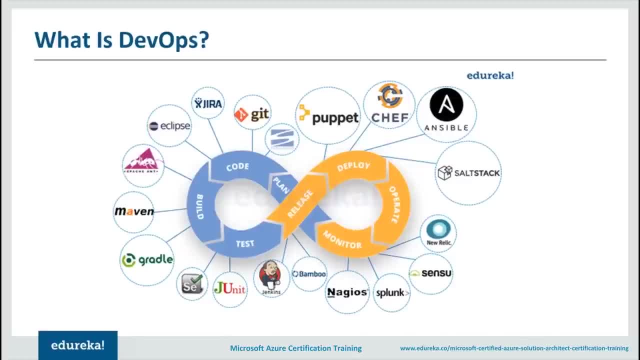 You might use Visual Studio code and then you are checking in your code in TFS team foundation services. You might be checking in your code in Jira and get a lot of different repositories. Now this is one area. Of course, if you have to do some builds, you can use a kudu server. 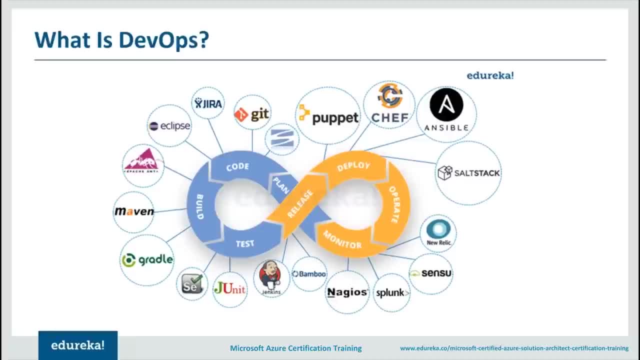 You can use Maven, you can use Gradle, So all these different tools are used to build your applications. Finally, if you are done building your code and if you have done all the check-ins, then the testing happens. you might be using selenium, you might be using selenium. 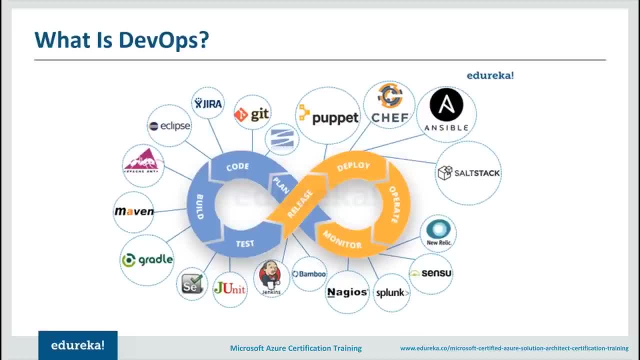 or J units to do the testing of your applications. Now again, you can see here: all these different areas required different kinds of tools, and if you are releasing something then of course you can use Jenkins and bamboo to release your stuff. Finally, you do the deployment. 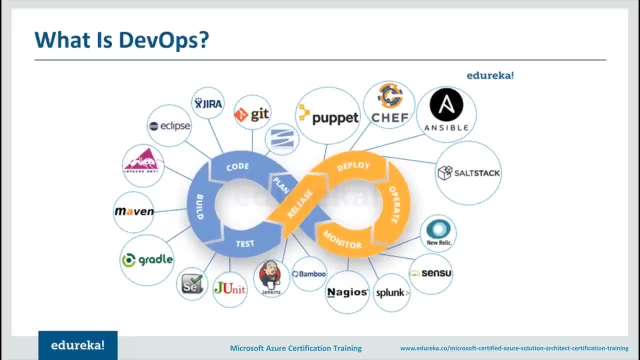 All right. so there are different tools to do the deployment and then you do the operations, which means your operations team is sitting there and doing all these operations stuff and they are monitoring this stuff using different tools. when we say that we want to build a devops platform, 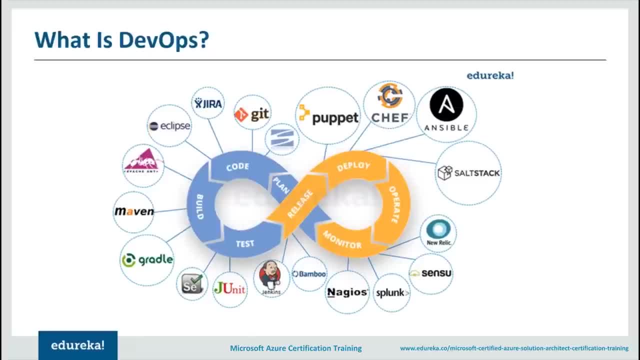 We want all these tools, what you see here- to work together so that you can do this activity without having to do any manual intervention. Okay, and this is where we are going to spend our time- into looking at how these tools can be used when we go to Azure devops. 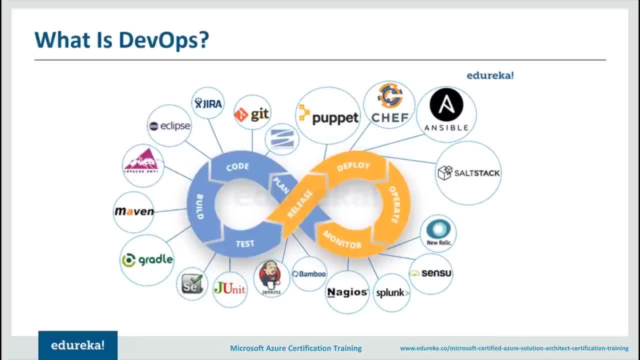 I guess you guys have learned about what is Azure, some basics. I guess you guys have learned about what is Azure. I guess you guys have learned about what is Azure, some basic stuff and what is devops. now we are going to look into if I have to do all this devops activity in Azure. 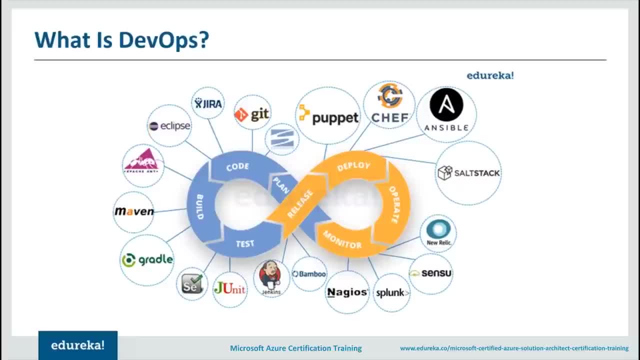 Okay, so what is it that is available to us? and now let's learn about what is as your devops. So, as your devops is something which is providing us all these set of tools integrated into one single environment. This means that, if you know how to work with Eclipse, 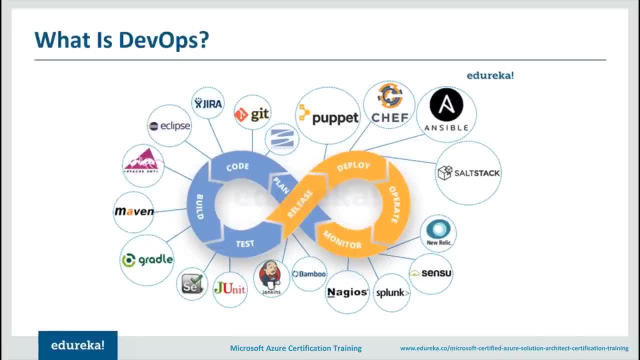 if you know how to work with TFS, if you know how to work with git, selenium, all these different tools, then you can use Azure devops. or, in fact, in my case as well. I didn't do you know a lot of tools, but still, when I started learning about Azure devops, 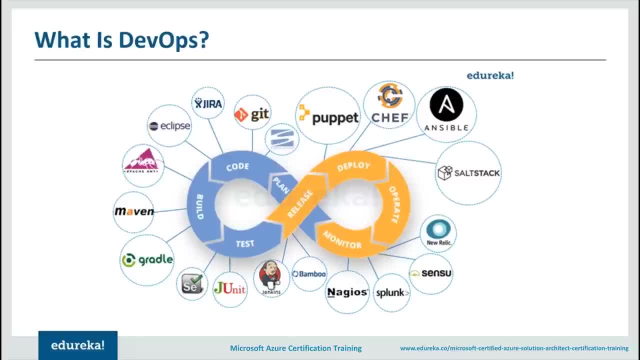 I started learning about all these things as well, So you don't have to worry that if you are not a part of any of these particular areas- for example, if you're not part of right now how to do the deployment, or if you're not part of how to do monitoring- 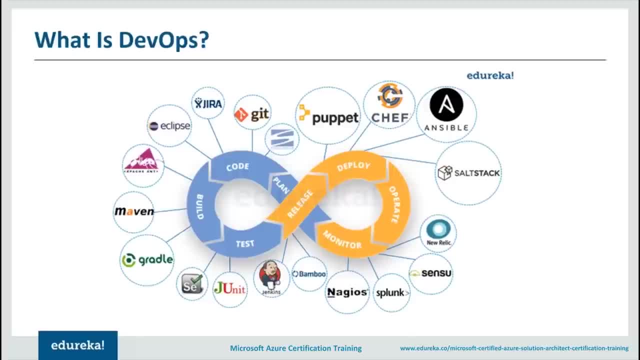 and you are on the developer side, or basically you are into the development side, then you don't have to worry that. will I be able to use devops or not? So the answer to that is yes, you will be able to use the devops, or, in fact, 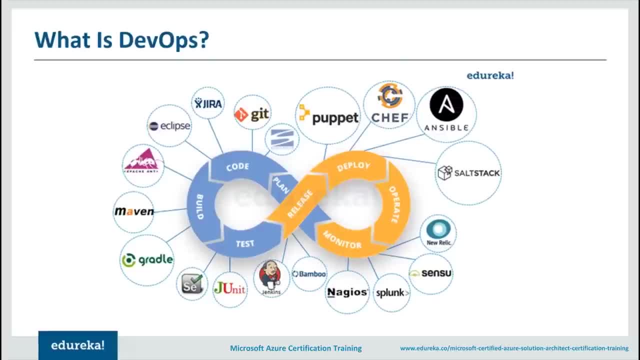 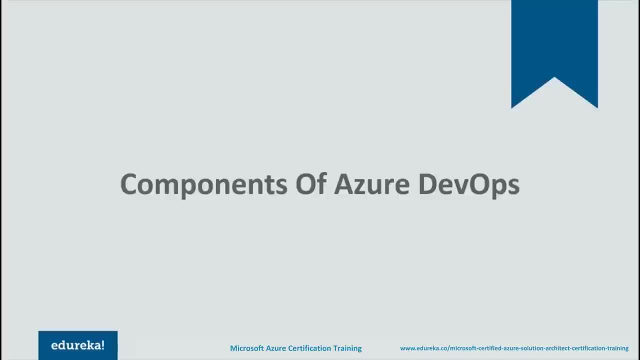 that will help you move towards the devops, Even if you know maybe a couple of parts of it. So now we are going to talk about what are different components of Azure devops and once we'll see some demos, you will be very clearly able to understand. 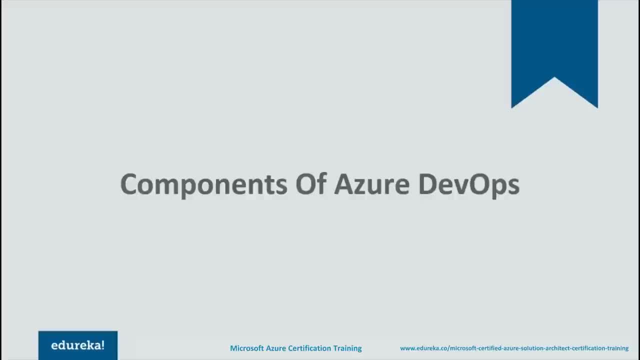 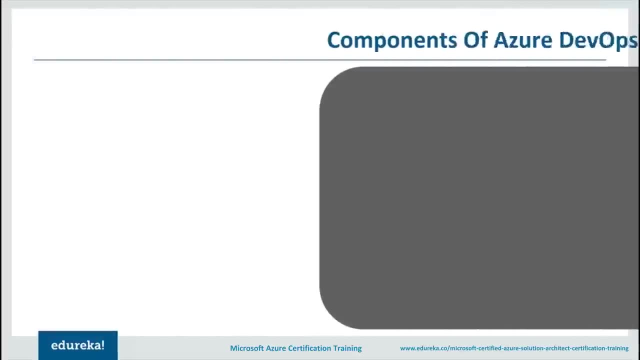 how you can take your application from the planning stage up to the deployment and monitoring stage using the tools in Azure. Okay, so let's learn about what are different components of Azure devops which are available. Now let me just show you all five, actually. 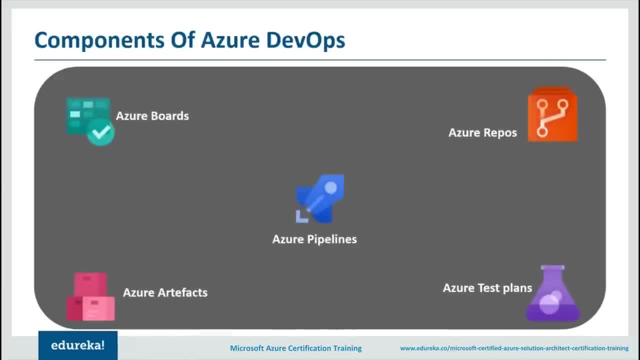 So there are five different components which are available as part of Azure devops. First thing that we need to know is about Azure boards. There are people who come from the scrum background. They are coming from the project management background. They know how to create some features. 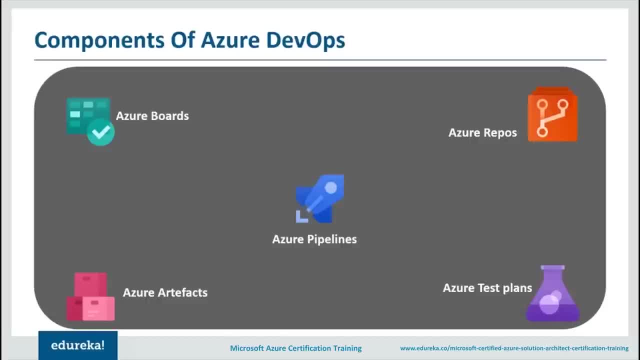 They know how to create epics, They know how to create the stories, They know how to create tasks and all that stuff. and then there are developers who themselves go and create the task on which they are going to work, And there are resters who just want to create some test cases. 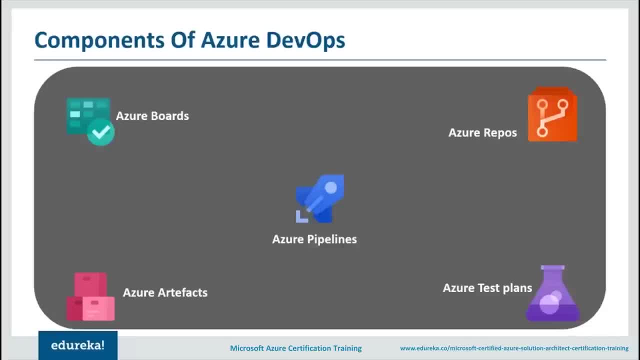 and after the test cases are done, they want to create the bugs which they find in the system. Now, all these activities can be done as part of the Azure boards. Number two is, of course, after you have done all the planning, after you have created all the epics. 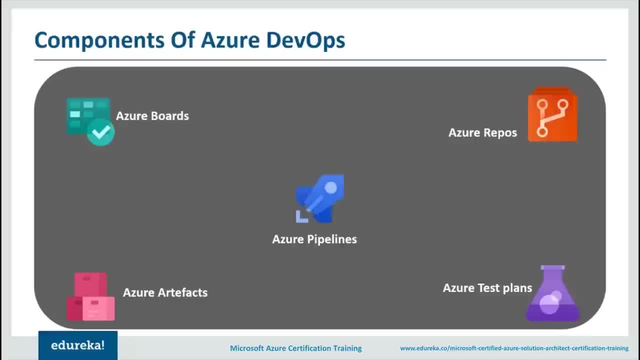 all the features, all the stories, tasks and everything. Second thing you want to do is development. For example, you start doing development in TFS, You start doing development in Eclipse. Any ID that you want to use, you can do the development. 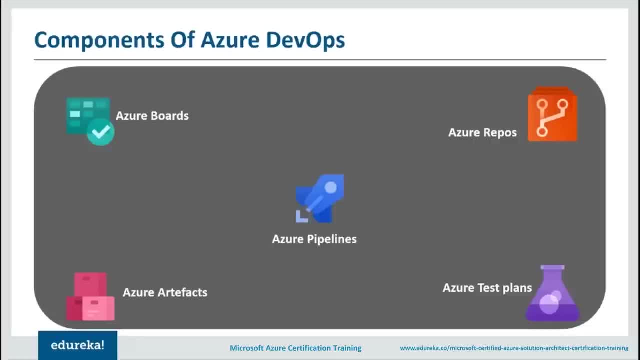 Once you are done with the development. now you want to push all this into a source control. Now this is where Azure repos will come in and it will help you store all the information. So in the source control, you check in your code and Azure repos is a place which provides us. 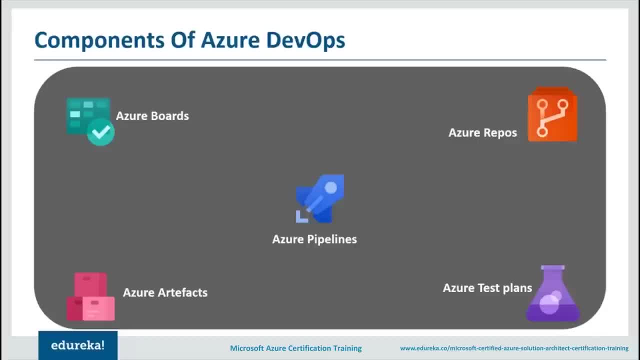 with a lot of different repositories- In fact right now it's two- if you want to use team foundation services or if you want to use git. So basically, you can provision that in Azure repos and you can start checking your application code in Azure repos. 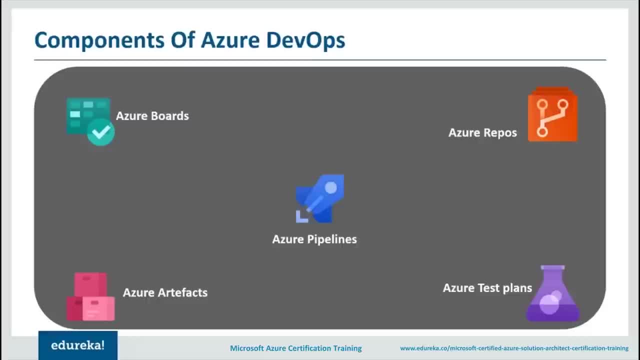 So again, we are going to see all these things in action today. The third thing is: once you have checked in your code, what do you want to do next? So there are two things that you want to do. First thing is that you want to run something called. 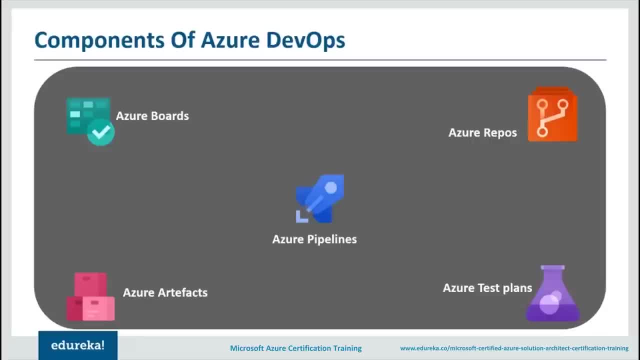 as a build pipeline. When you have checked in your code, you want to make sure that nobody has checked in some wrong code, So this is where you build your code. Of course, the developers have the responsibility to build the code on their local machines. 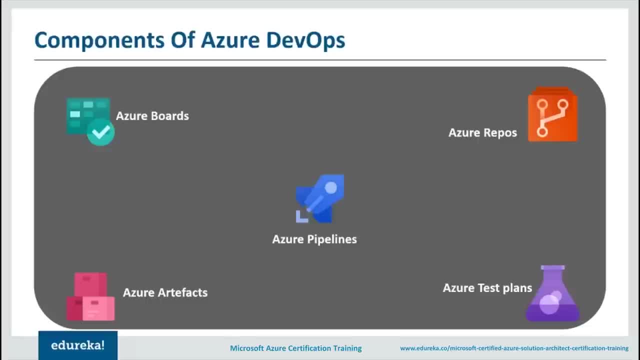 This is not a good practice. Now, if developers is just building it on their local machine, this means that maybe some of the dependencies on that machine are not correct or maybe it's not in sync with the other team members. So this means that if person says that, yes, 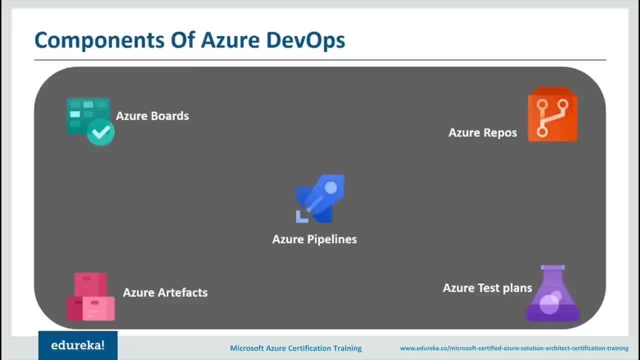 it is building on my machine and I just want to push it in the source control. Is that good? The answer is no, because this means that if somebody will have a special dependency in the application which is installed locally but it's not installed, 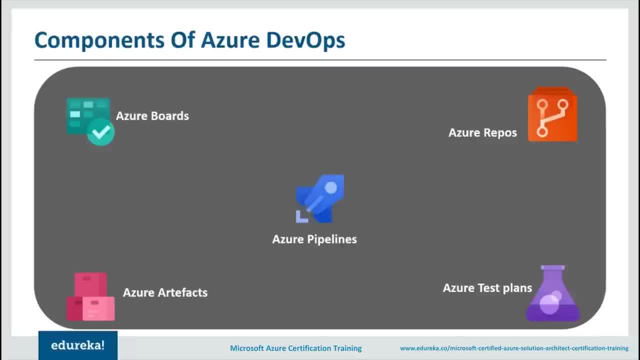 you know for everyone, for others, when they will download that code, it will fail. So that is why, whenever the developers push something in the repose or basically in the source control, it is going to be taken by the Azure pipeline. It is going to do something called as a built. 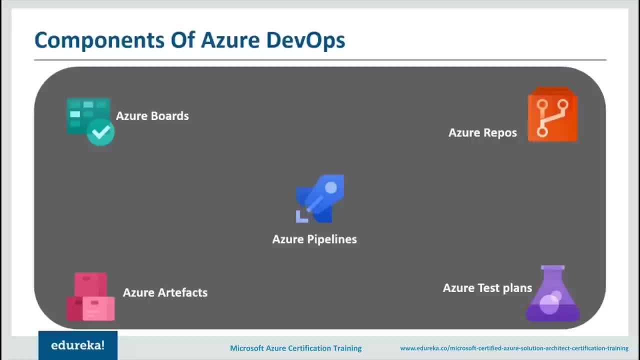 Okay, So the building of code happens in the Azure pipeline. Now next thing is: the build has already happened. What do we need to do next? The next thing we need to do is release this code Now. I can release it in the dev environment. 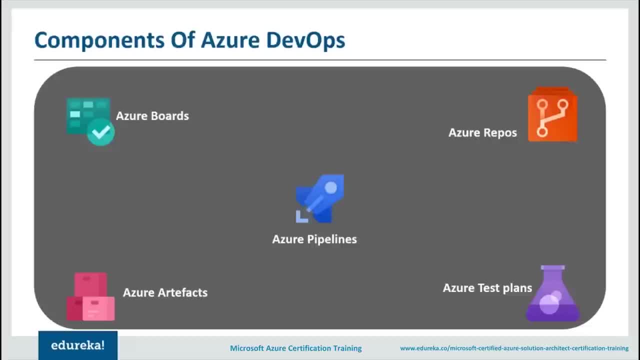 I can release it in, let's say, pre prod or you at environment, or I can also release this code and stuff in production environment. But normally what do you do if developers check in something? We do the build of the code and then we release it in the dev environment. 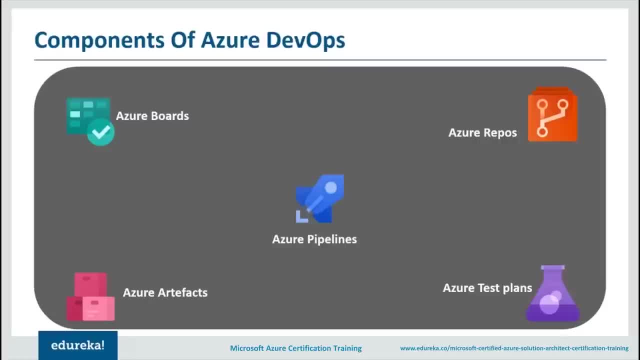 Now, once it goes to the dev environment or maybe in a test environment it is going to run, after it run completes, Then you would want to run some kind of you know some tests on top of it. Let's say you have deployed a web service. 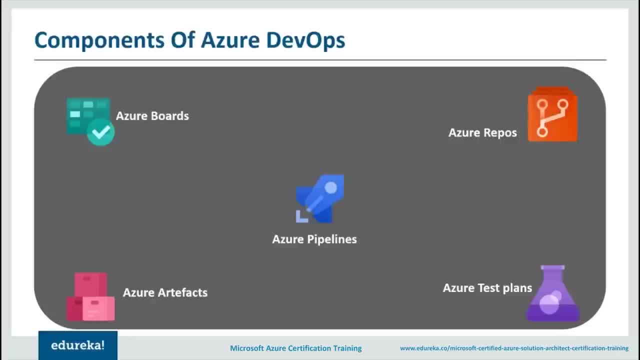 So if you have deployed a web service, you would want to test if it's behaving correctly. or if, let's say, you have deployed a web application, You want to check if everything is looking fine in that web app or not. So there you can run manual test cases. 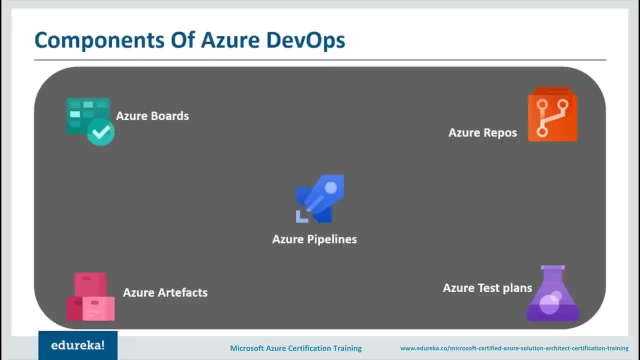 automated test cases. You can even do the exploratory testing. All that stuff can be done as part of the Azure test plans, All right. And finally, once all this test plans is done, we can again use basically the pipelines to release something to different environments. 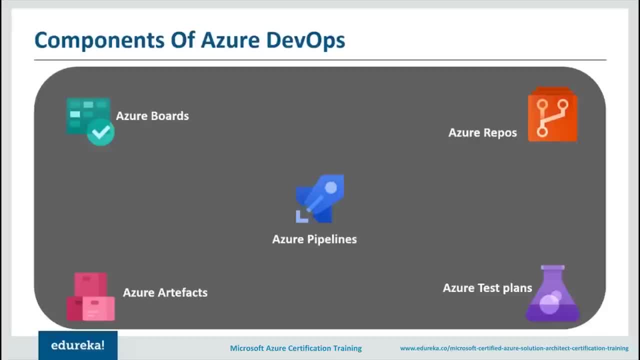 like you at production and all that stuff. While all these things are going on, there are a lot of things you can configure, like workflows or in fact, let's say, approval workflow. So if you are checking in something, you want to make sure the review happens. 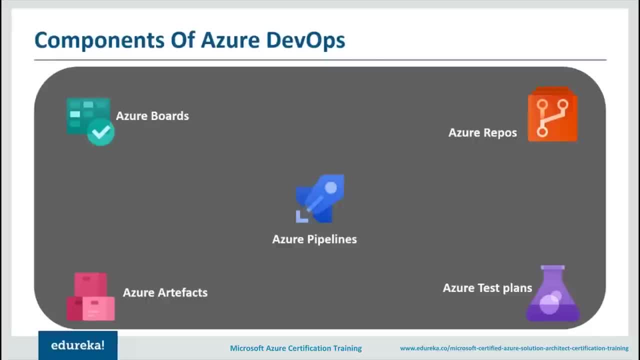 so that can be taken care in the Azure repose. If you are releasing something to the uat environment, you need, let's say, an approval from your team lead, or you need an approval from the program manager. So all these approvals are by default built. 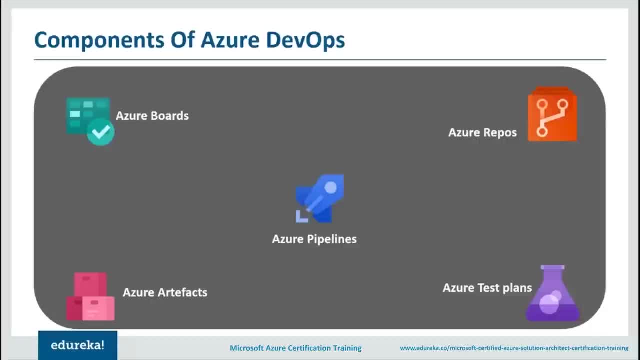 in into all these services. Now, one thing which I haven't touched upon is as your artifacts. Now this is something. for example, let's say you have got 10 projects and all these 10 projects have got common dependencies. it may not be common in all. 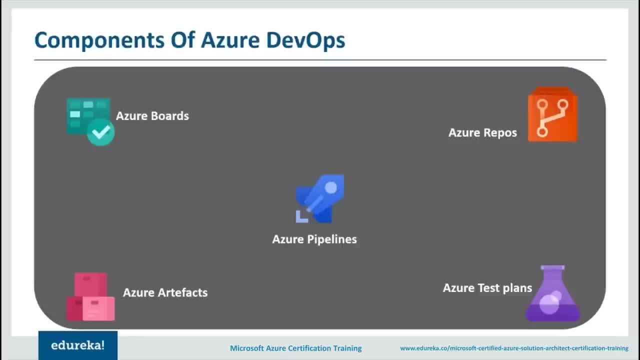 but let's say, three projects are using one dependency, five projects are using some other dependency. So what you can do, you can collect all these dependencies and put it into a one single location called as your artifacts. So I'm going to show you few of these things in demo today. 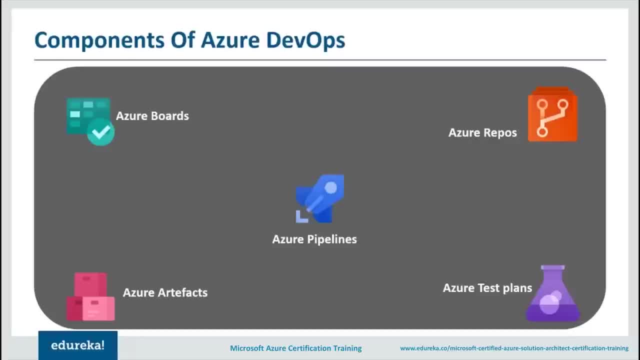 that, how you can use as your boats, as your repose, as your pipelines, And of course I'm not going to touch in the demo on test plans and artifacts Now. I hope everybody understood this overall infrastructure We have got as your boats to create our work items. 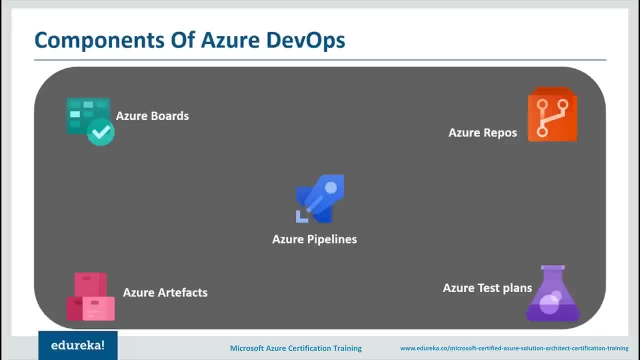 We have got as your repose to store our code. We have got as your pipelines which can help us do the build of the code, release of the code into a particular environment. Then we have got as your test plans which we can use to do our testing. 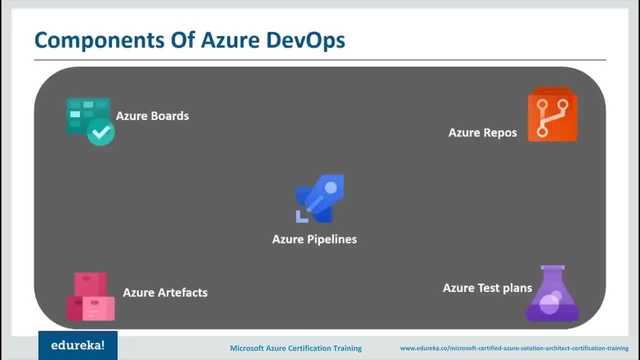 which could be a manual test cases, automated test cases, exploratory testing. all that can be done as part of the Azure test plans And, finally, if you have got some common DLLs or common jar files which you want to store it as part of your repository. 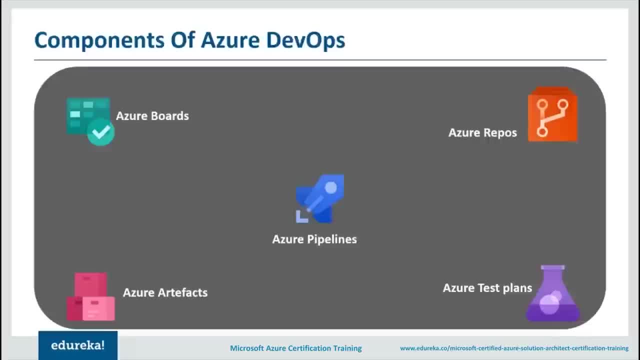 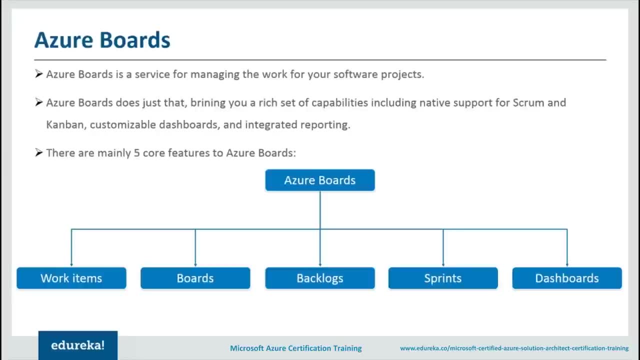 then you can use as your artifacts. Now let's look at some of the more things now. First thing, as I said, is as your boats. So we have got five different components as part of as your boats, All right. So, as I said earlier, as your boats is a service. 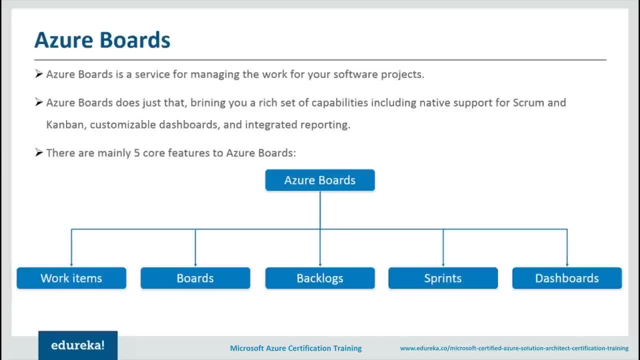 for managing the work of your software project, which means you want to create some, let's say, epics. You want to create some features, basically some tasks, some product backlog items. You want to create some bugs. all this can be handled in as your boats so you can set up that I want. 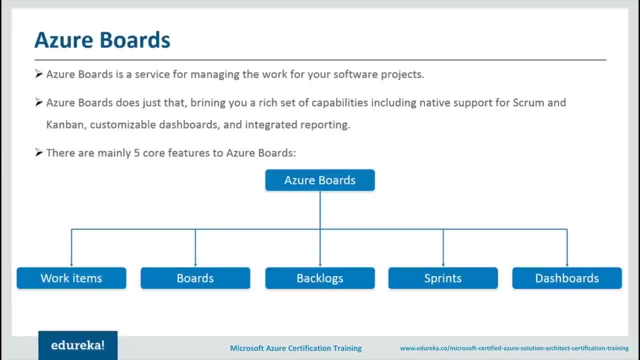 to follow the agile process, I want to follow the scrum process, I want to use the Kanban, So all these things are available as part of the Azure boats. So it does not matter that what kind of process you want to follow. 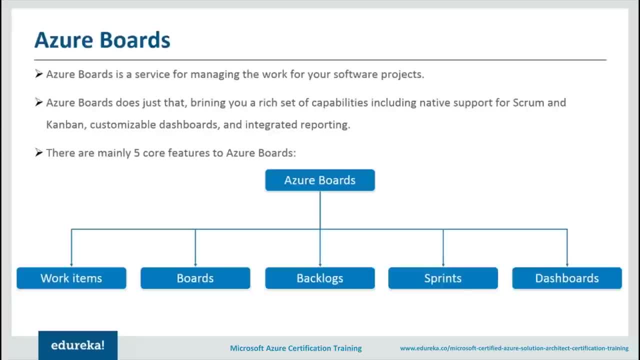 I know that a lot of people know about agile. So, guys, I am also an agile and safe certified, So I know there are different processes and all these different processes can actually being handled by as your boats. So what you can do, you can go ahead. 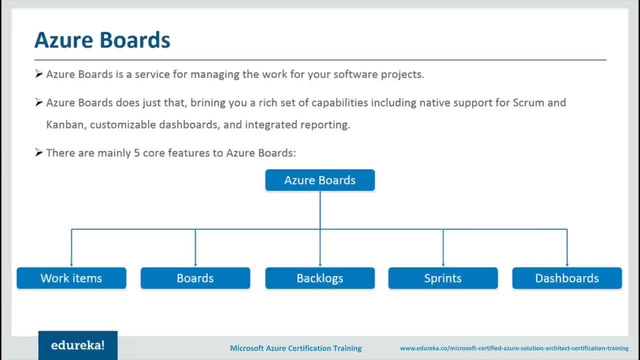 and create work items. then you can have the backlogs. Now I'm going to tell you what is a work item and what is a backlog, and then we have as your boats- In fact board is something. very basically, you can run some queries and see that what is something. 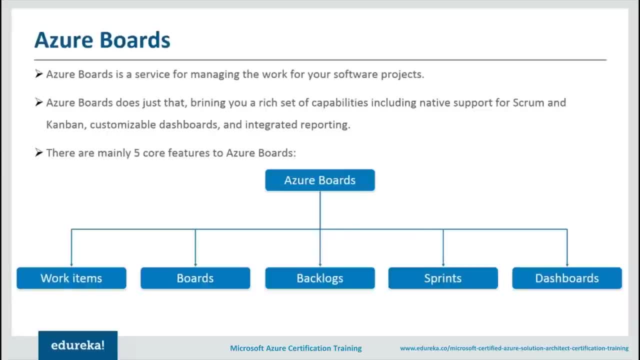 in particular Sprint, or let's say what other tasks which are active or what are the tasks which are closed, if you just want to say that, what were the tasks which were released in this particular Sprint? So all this information you can get it from the boats. 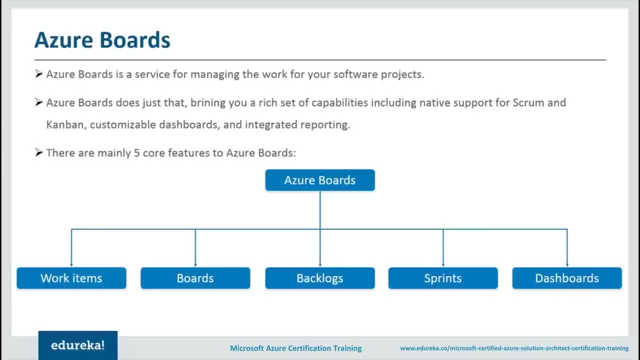 Next thing is about Sprint. Now, let's say a Sprint is of 15 days, So in 15 days, what other work that we are going to accomplish? So those things are basically those tasks or features. They go into Sprints. 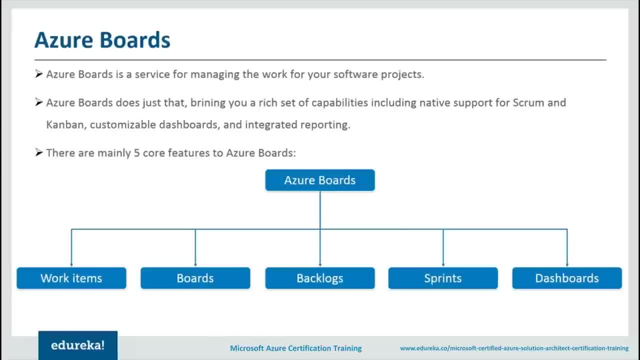 All right, And finally, we have the dashboards, which can help you have the overall picture of what is the progress of your particular Sprint or what is the overall progress of a particular release. Okay, So this is what is covered as part of the Azure boards. 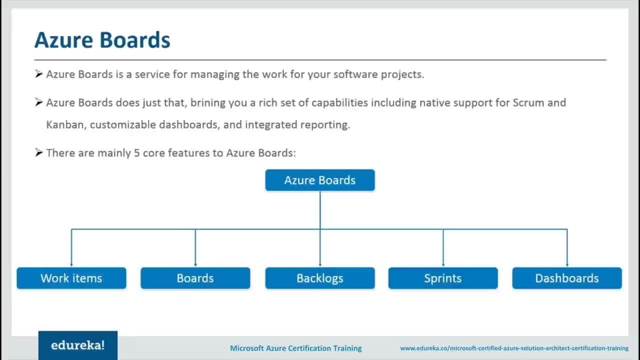 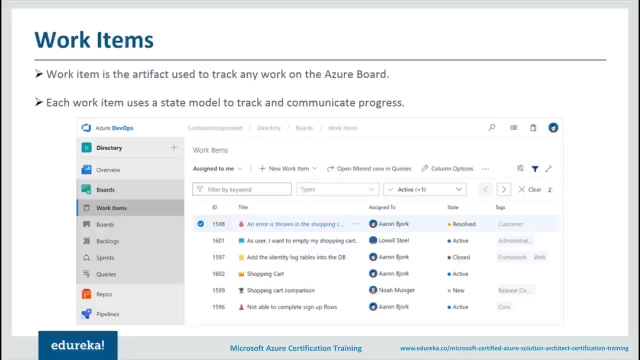 We can just talk slightly more on this and then we'll see that in the demo. Now what do we see here? We have got work items, pretty simple stuff, create, Let's say. you can see here, This is a bug being created. 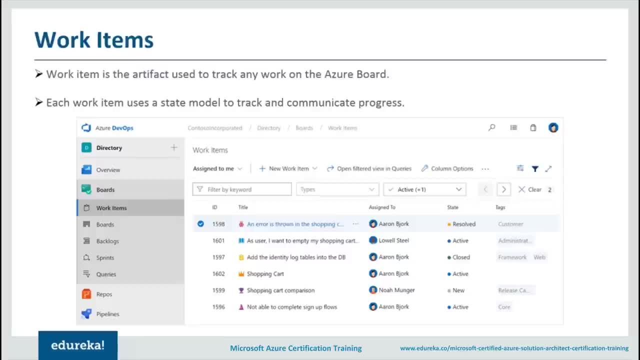 This is a user story which is created, or basically the backlog item which is created. Then we have the tasks which are getting created and, the same way, we have got features. We have got epics which we can create as part of the work items. 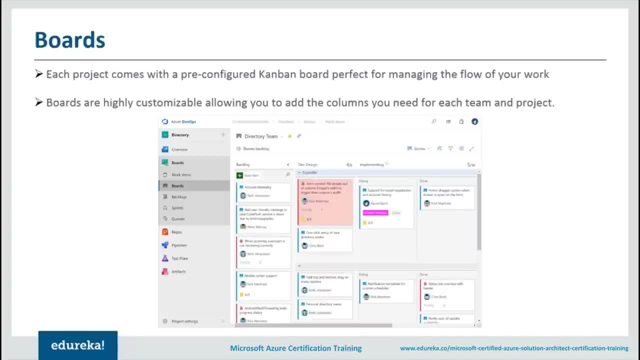 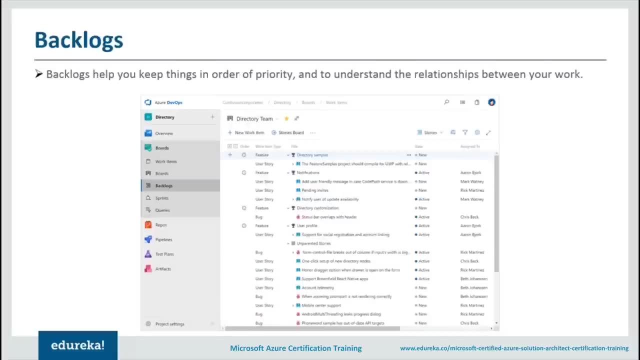 Then we have got boats, So you can see that what is basically the particular flow of your current Sprint or what is the flow of your project? Of course, we have got backlogs. now we can arrange. what do we want to do as part of the backlog? 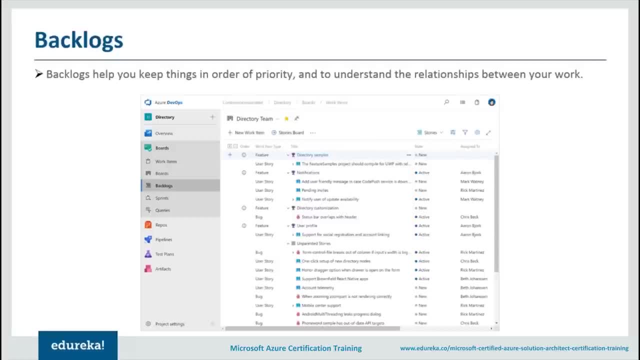 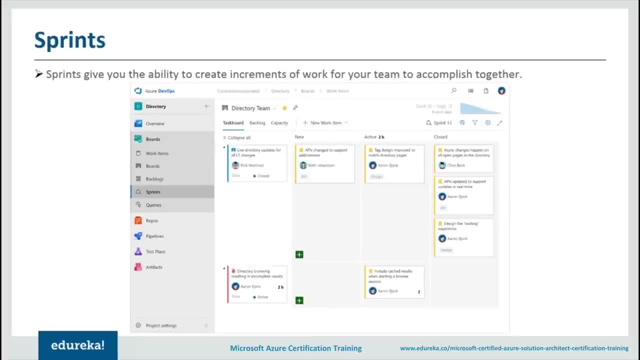 How do you want to prioritize your different work items so you can deliver your software on time? Next thing is about Sprints. if you guys have not worked with Sprint, So do not worry because we don't want to go into that. What are the details of Sprints? 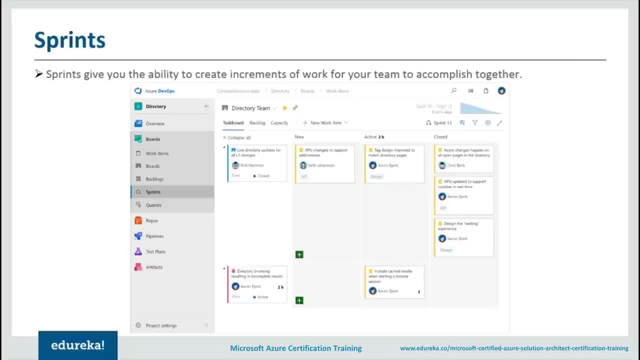 But then Sprint is basically, let's say, a small time box window in which you can go ahead and deliver a particular part of your product In your e-commerce application. If you say that we want to deliver the checkout functionality, So let's say if you are ready to deliver the checkout functionality. 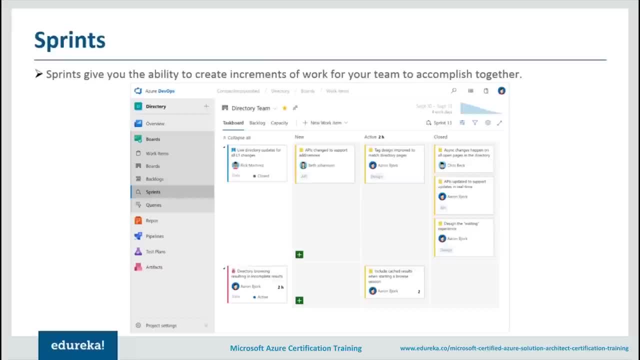 in two weeks as part of the Sprint. So your checkout feature or your checkout epic will go inside that particular Sprint. So once it goes inside that particular Sprint, the whole team starts working towards that particular area. and what they do they try to complete all that stuff. 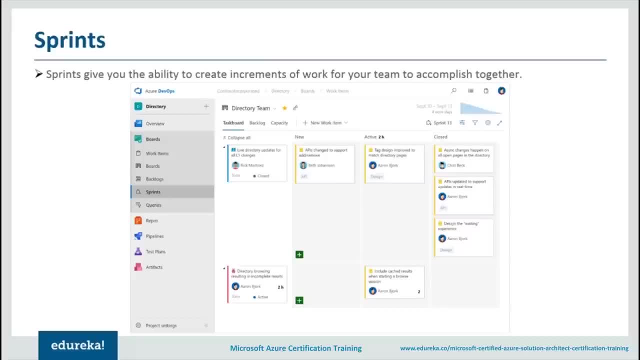 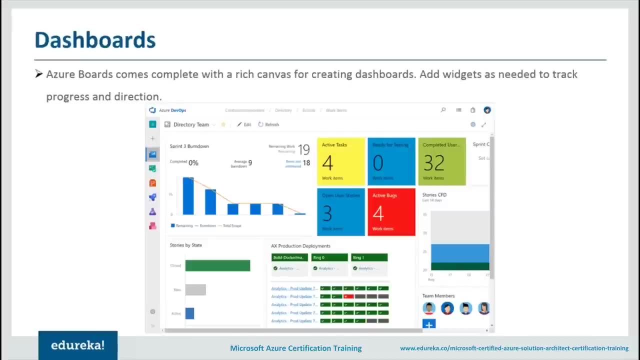 during that 15-day time box window, and that is what you can build as part of the Sprint. All right, So then we have the final dashboards where you can see what is the current status of your project before we go further and look into other different aspects. 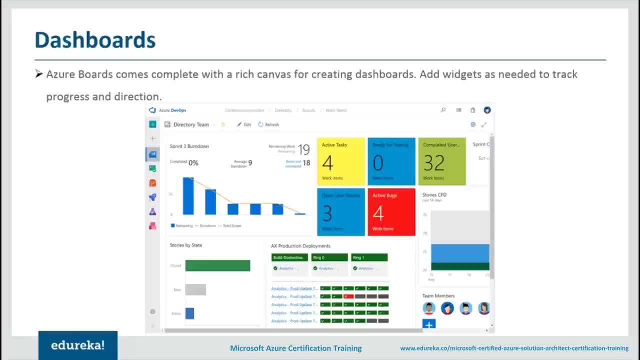 like pipelines and stuff. I just want to give you a small demo of how you can create the work items, how you can create the backlog items and how you can use the boats. So let me stop here for a while, Okay, and what I'm going to do now is going to go. 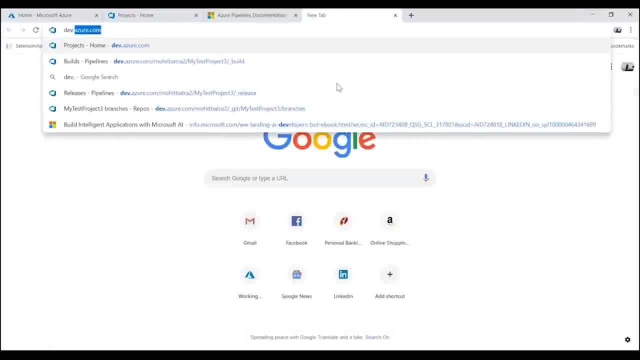 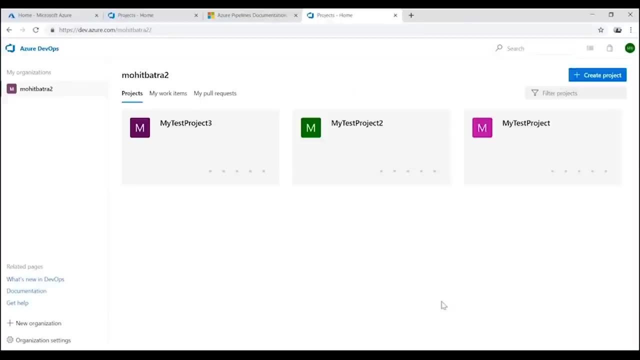 to something called as devazurecom. what you need to do here is, if you are not signed in, they'll ask you to sign up or sign in, and once you sign in, this is the kind of basically the dashboard. you will see what you can do here. 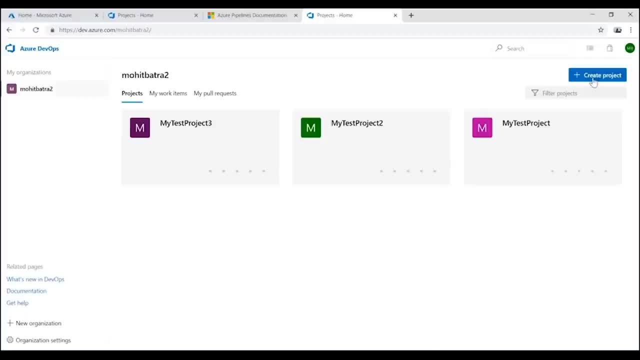 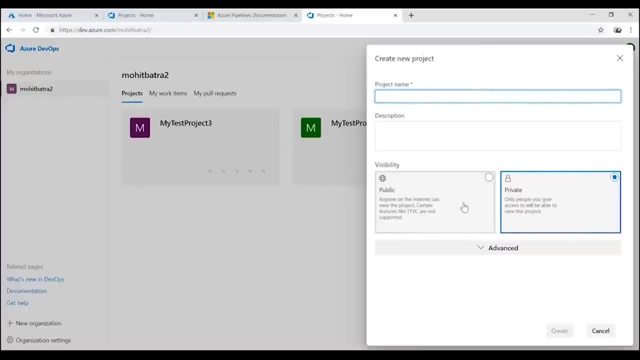 The first thing you can do here is create a new project. All right, So let me create one. What do you see here? It is asking me that is it a private project or is it a public project? Now, let's say, if I want to create a project called 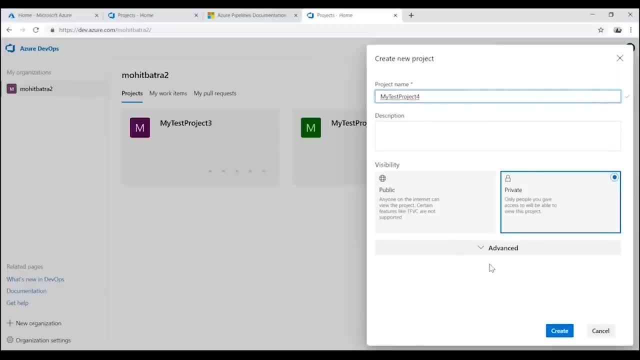 my test project, for I'm not going to create it. It takes some time, you know, to set up everything, but what I can show you here is that now it is asking that: what is the version control? So, basically, where do you want to keep your source code? 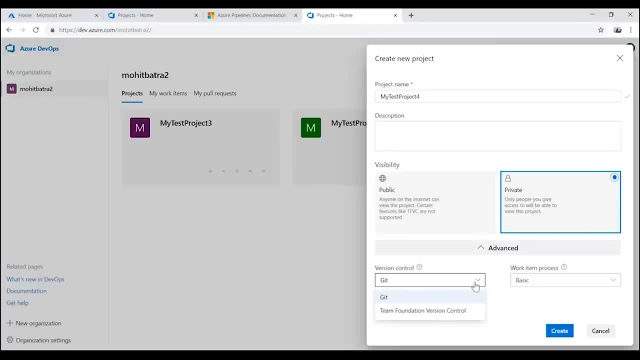 Do you want to keep it in git or do you want to keep it in TFS? Okay, so you can go ahead and select the different version control options which are available Now. of course, I think with time they will keep adding more. 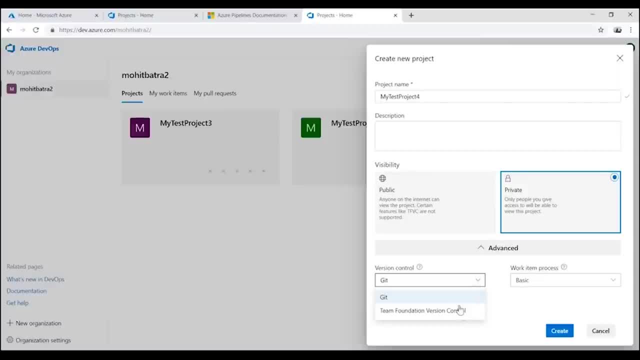 and more. you know source controls or the version control repositories here which you can use, but most common ones, which we everybody knows, is git. We also have GitHub, which is again a repository for storing the git based version control. Of course there is something from Microsoft. 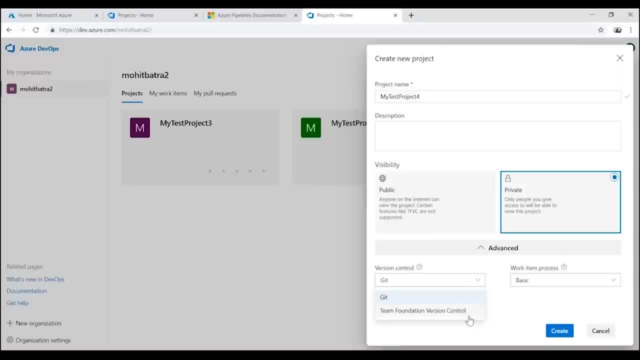 which is available, which is the team foundation. If some of you guys have worked before with TFS or the team foundation services, This is the one. it is totally up to you. How do you want to store your code? So I'm going to select git right now. 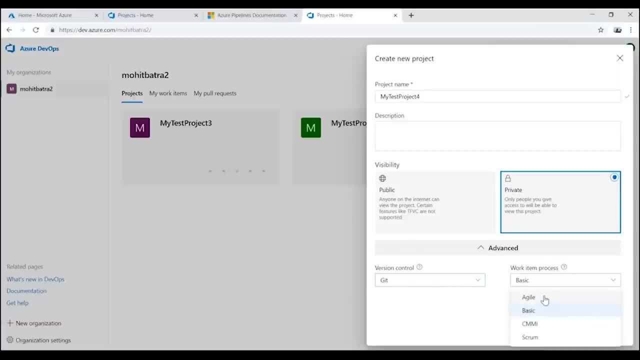 The next thing is about work item process. So if you want to follow the agile process, you can use this one. If you want to use a scrum process, you can follow this one. Then, of course, you have got CMMI and a basic one. 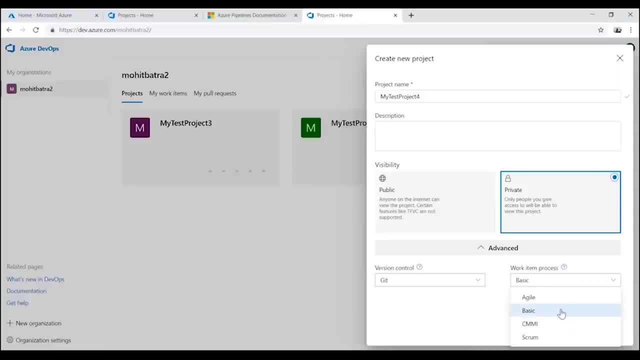 Now, basic is something which does not follow a particular process, but this is something which can help you set up either the agile process or the scrum process. It's like a kind of a blank template, but if you are comfortable working with agile environment, 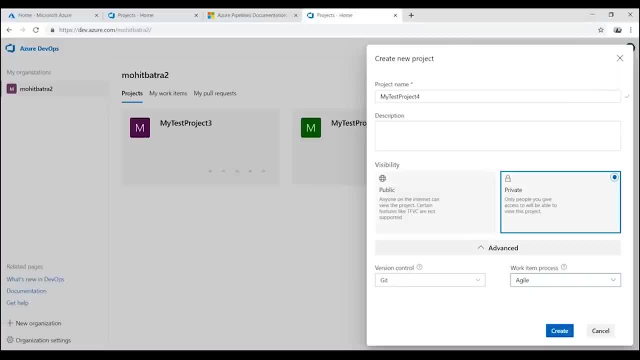 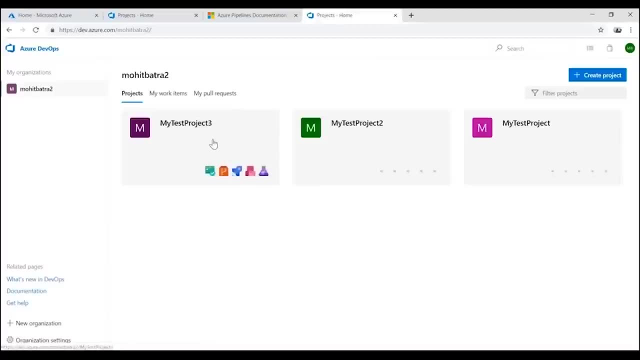 you can select this one and you can click on create Now. as soon as you do that, what you will see it's something like this one, my test project 3, because I created this one and I added few things here, So I want to show you that. 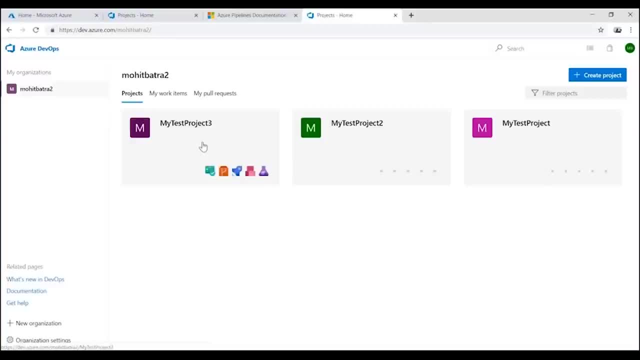 All right, before we go into inside this particular, my test project 3, what are the things you can see here? something called as Azure boards, which we have already talked about, the repositories, Azure repos, Then we have the Azure pipelines. We have got the test plans and then we have got the artifacts. 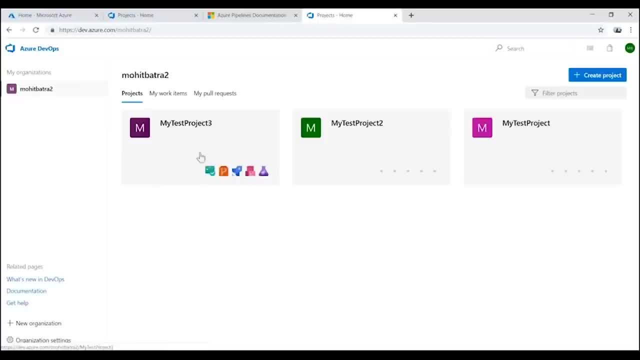 the same stuff that we have seen in the slide. It's available on devazurecom once you create a project. Now let me go ahead and first of all, click on this project. what I have done in as part of this project. I am using agile plus, I am using git. 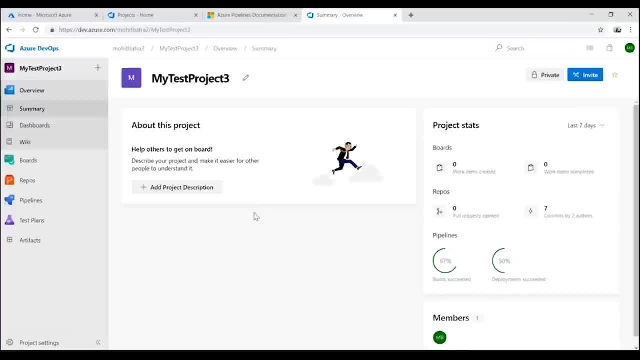 So I've selected this one, and this is now showing up in my test project 3.. The first thing, as I told you, that I want to show you about is boards. Now let me go here. on the left hand side, You can see boards, repos, pipelines, test plans and artifacts. 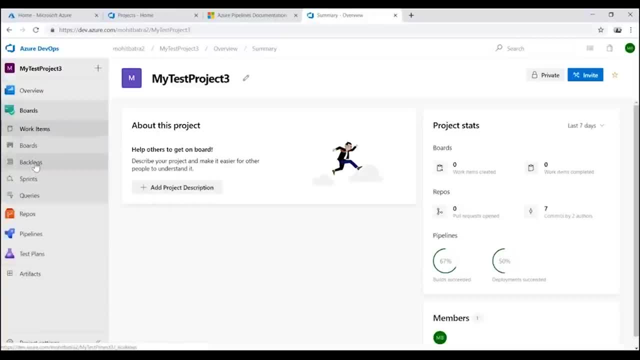 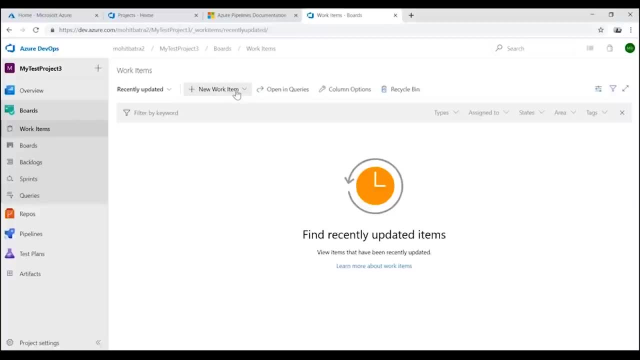 So I'm going to go inside boards right now and straight away show you what you can do in the boards. First thing is, of course, pretty simple if you want to do the planning. So what do you do? you create something called as a, let's say: 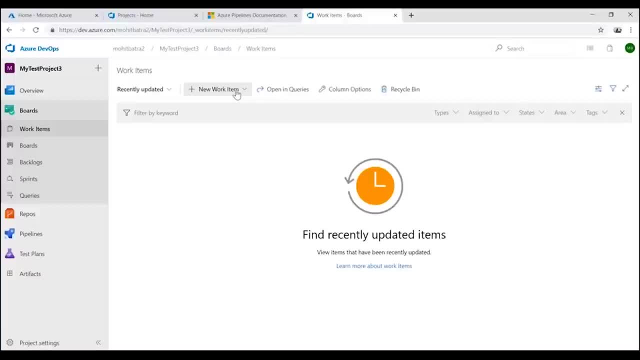 a task or basically, you create a work item. Now, work items are of different types. You can have something called as an epic. Now, epic is something which is very, very high level. So, let's say, your leadership team comes up and they define something called as an epic. 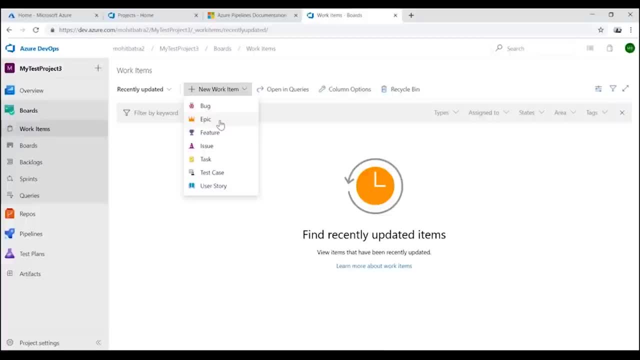 Now they will say that we want to deliver this kind of project. All right, So there they are, defining a particular epic. Now, inside the epic, what you can do, your product owners or, let's say, your project managers, They will go ahead and decide on the number. 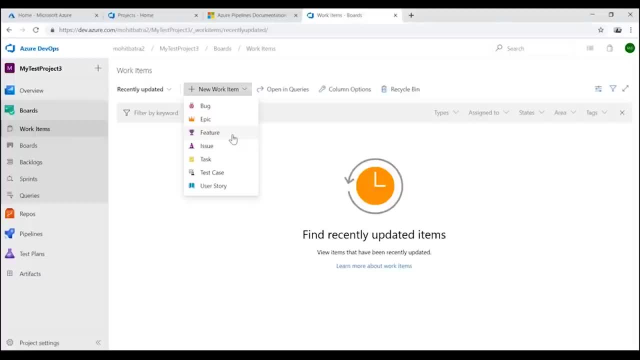 of features that you want to have as part of the epic. Let's say you want to build an e-commerce site. So in e-commerce site the business says that we want to set up some e-commerce set up for our, this business. That's an epic. 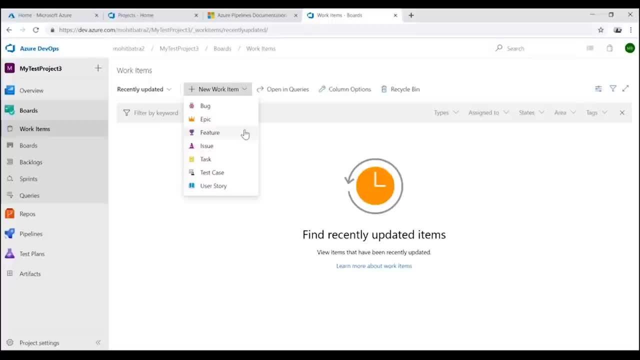 Once you go inside that epic, you will say that I want to create a feature. Now, what is the feature here? I want to deliver the card functionality, I want to deliver the product page, I want to have a recommendation engine, or maybe I want to have a search engine. 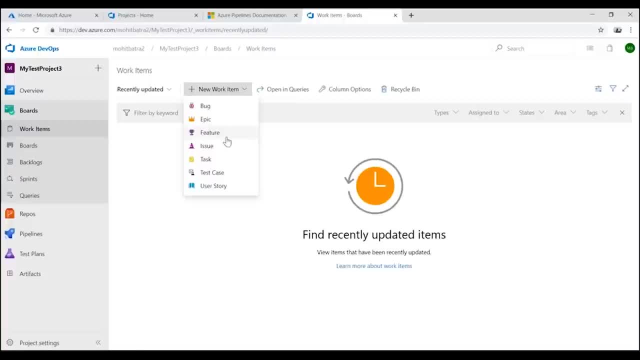 in my e-commerce portal. Now, this is what will be created by product owners or they will be created by the project managers. Now, when you say I want to create, let's say, and search service in my e-commerce site, So as part of the search service, 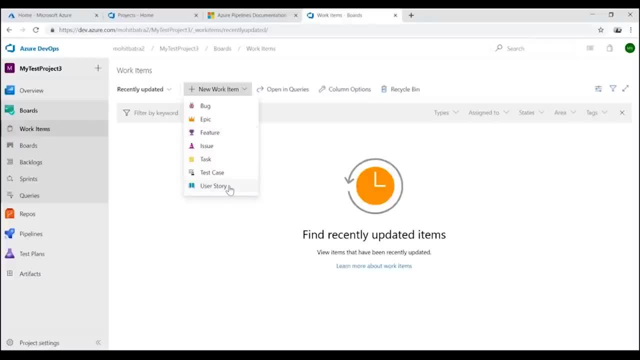 what do you need? You will go ahead and create some stories. So in the story, what will you say? you will say that I want to have some database ready which will contain all the information of my products. Then I'm going to have, let's say, one more story. 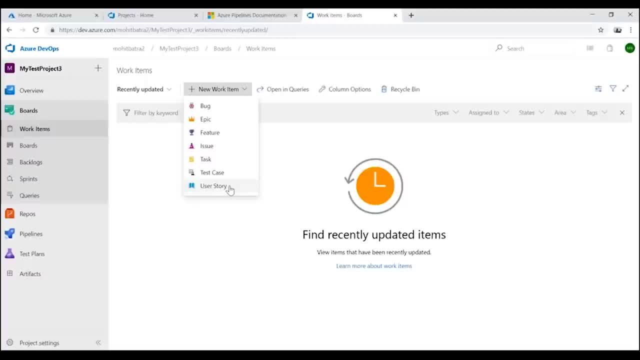 for building up a middle layer which can help me- you know some- building some api's which can help fetch this information from my database and show it to the end users. Then I'll build another story to say that I want to show it to the end customers. 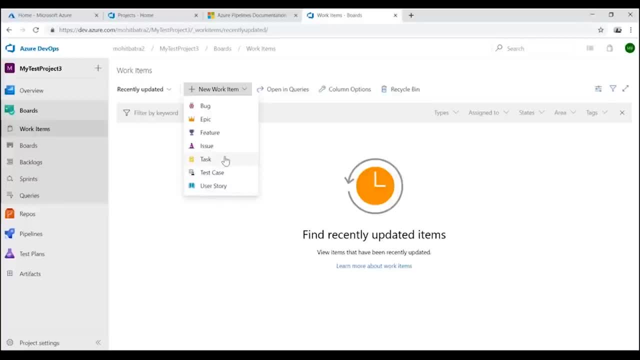 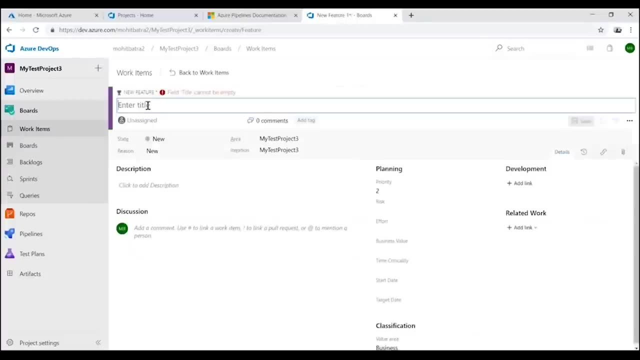 and once you have these user stories, then you go ahead and create task inside that particular story. So let me start building up. Let's say, one feature. I'm not going to, you know, go into the complete agile model, but right now I'm just saying 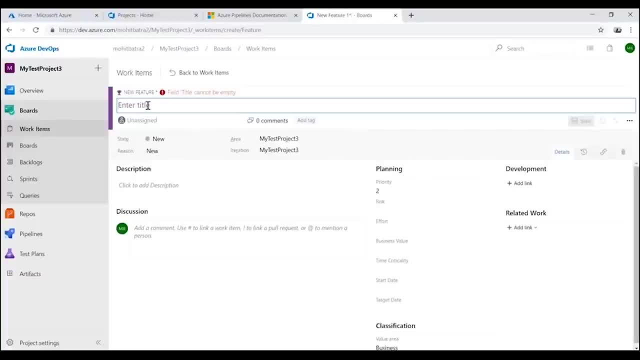 that we want to create a feature for, let's say, search in e-commerce. Okay, just remember, guys, This is not the way we write in agile format. So if you want to, you know, just create a new feature. There is a particular format. 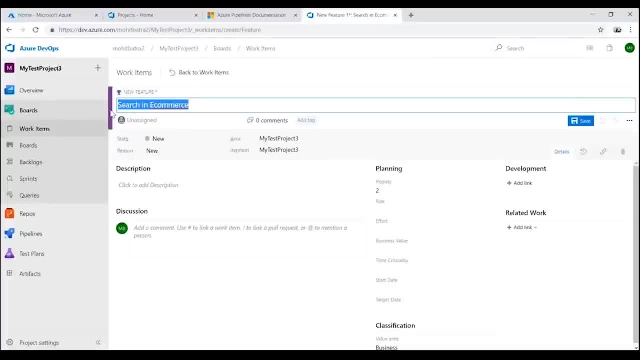 in which you should create the feature. Basically, the text has to be in a particular format, but that's not the agenda for today. The agenda is to show you that you can create a new feature. You can provide a particular iteration path. This means I want to do it in this particular time frame. 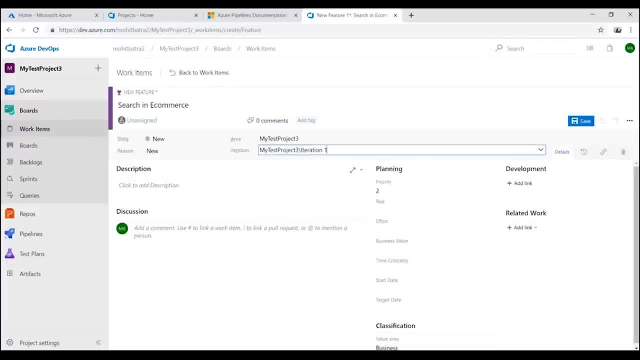 Okay, I can create multiple iterations. Okay, and I can put up the iteration here. Now, next thing, what I can do here: I can link it to some existing item. All right, so we'll do it later, but then we'll say what is the business value of this? 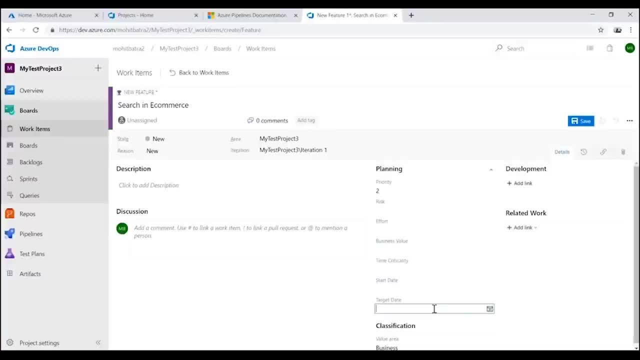 What is the time criticality? What is the start date? What is the target date which we want to complete this particular feature? This feature is new right now, So let me save it. You can go ahead and provide description. You can use the discussion board to do some discussion. 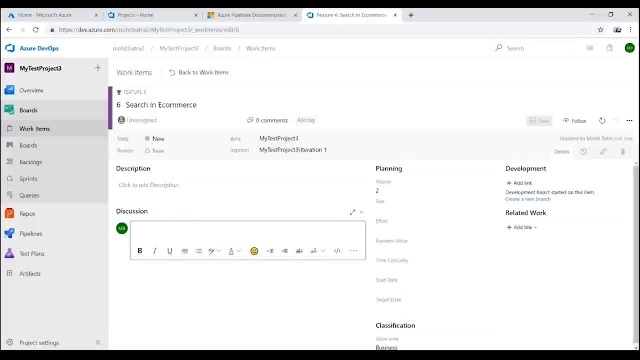 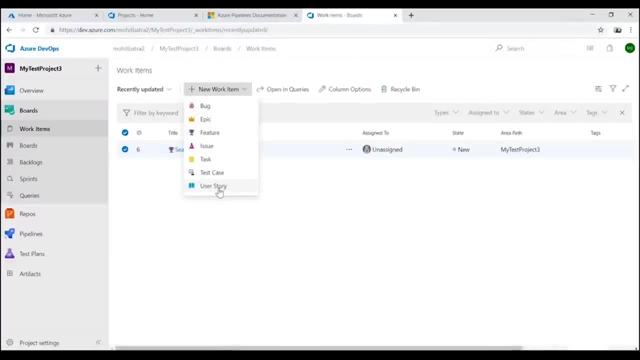 on top of this particular feature And once you are final that yes, our feature details are ready, Then what is the next thing? Let me go back to work items and let's say I want to create a particular user story. What will I do? 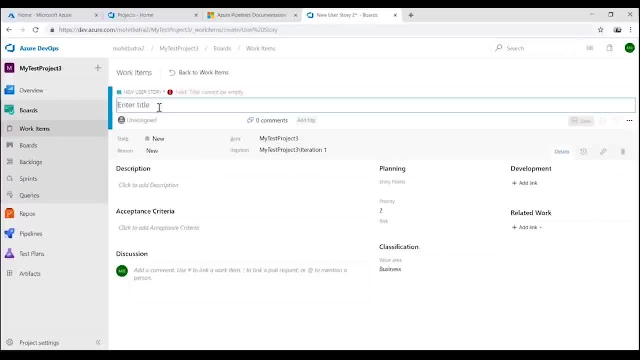 I'll say that I want to create, Let's say, in the search, I want to create the API's. And what do I need to do? I need to link it to the epic, or, in fact, I'll need to link it to the feature. 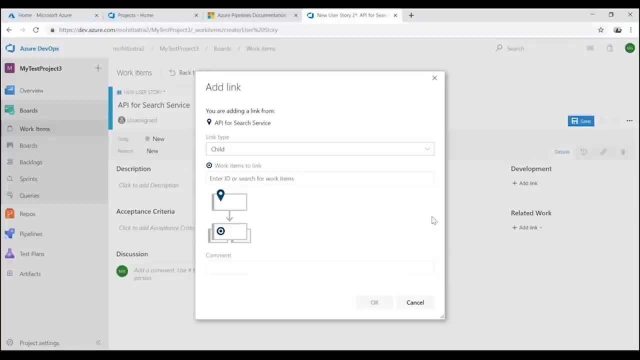 on the right side, Add link existing item. and I can also say that: what is the parent here? So the parent is research for it. So the parent is search in e-commerce. Okay, so I'm going to link this one and say that I'm creating a user story. 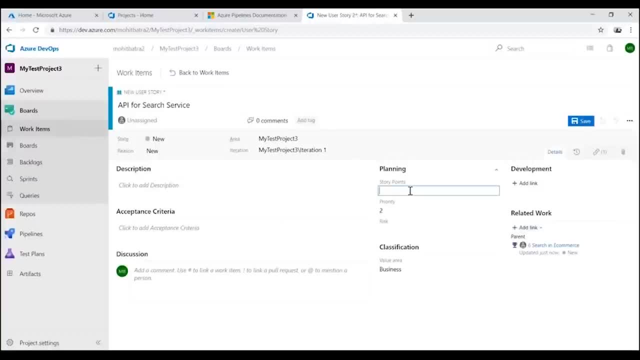 Let me save it. In fact, you can see that if you know about what a story pointing, so you can add story points here. or in fact, let me tell you this: if you go for, you know, for any kind of course or not just from here, 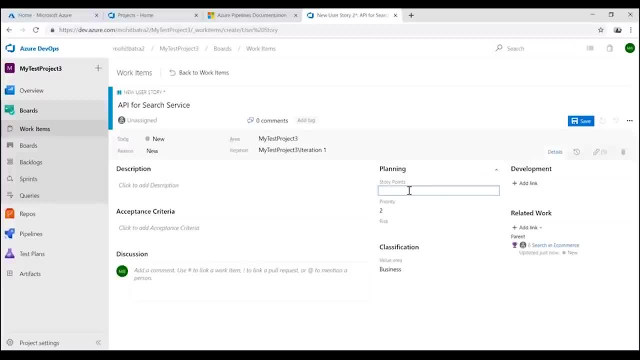 but if you go for any kind of course about how do you handle agile, So there you will learn more about story pointing, So you can also provide the risk. Let's say this is a medium risk. What is the priority here? All these kinds of 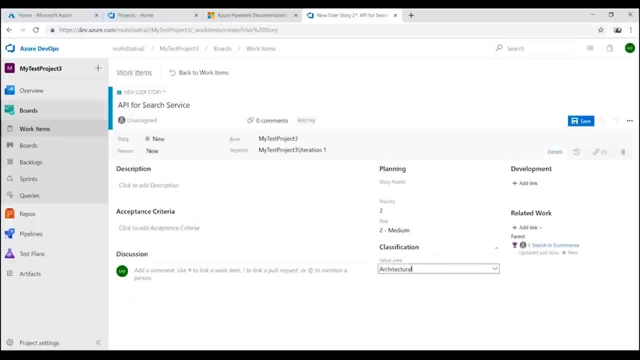 setup. you can provide here that you want to do some architectural thing or you want to. is it a business feature? All this information is provided as part of the user story, So let me save this one. Go back to the work items. So right now this is showing is separately. 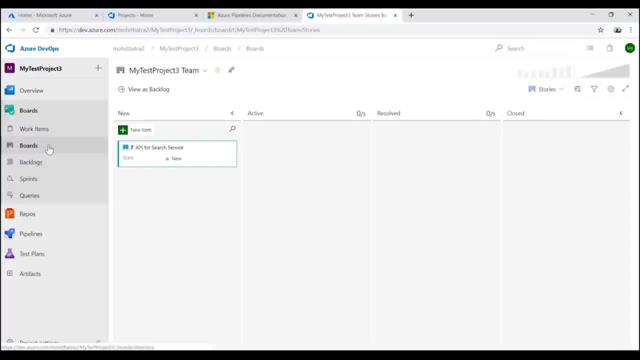 but once we'll go to the boards, Let me go to the backlogs first. what you will see here, all the different stories which are available Now. this is something on which we want to work. Let me add one more Story here. new work item. 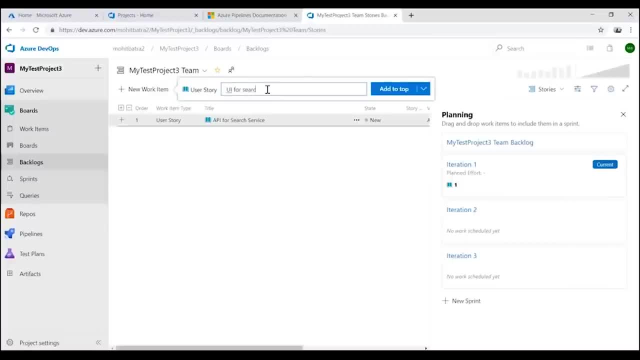 and, let's say, UI for search. Okay, let me add this one Now. What you see here is we have created now two stories in the first print, or basically in the planning side. Let me just open it up and so, as part of the iteration, what we are going to do. 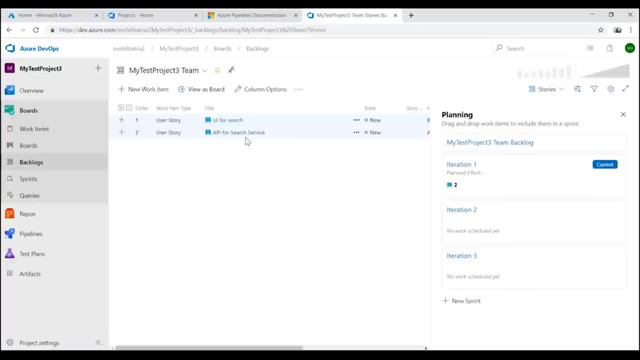 in the first iteration, or let's say in the first 15 days, what we are going to deliver. We are going to deliver API for search service, Or in fact actually both of them have got into the same iteration. So now you can see, here we have got one story. 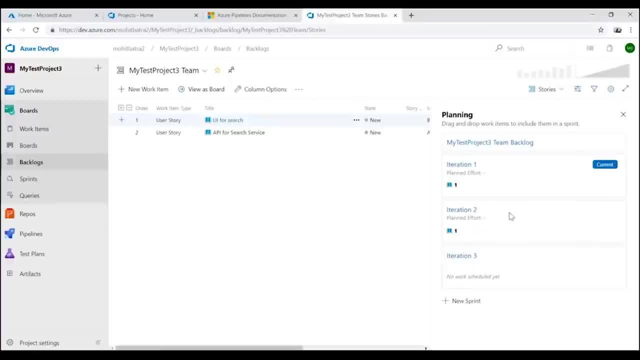 which we are going to cover in iteration one, which is right now the current one, and one story We are going to cover as part of the second iteration. Now, in fact, if you go ahead and add more tasks to it, say if I click on. 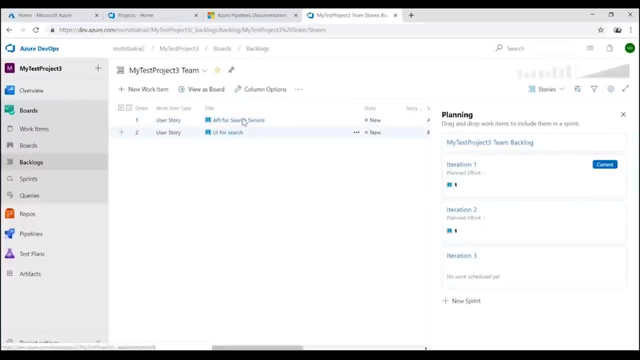 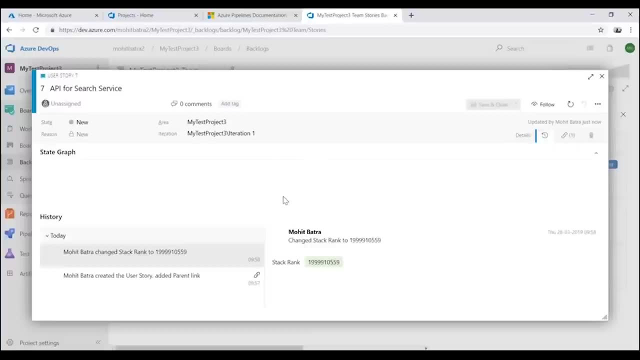 I can even change the priority for this one by dragging and dropping. now click on API for set service. I can go ahead and click on, or in fact I can see the whole history of that particular feature or, in fact, that particular user story. I can also go to this particular link. 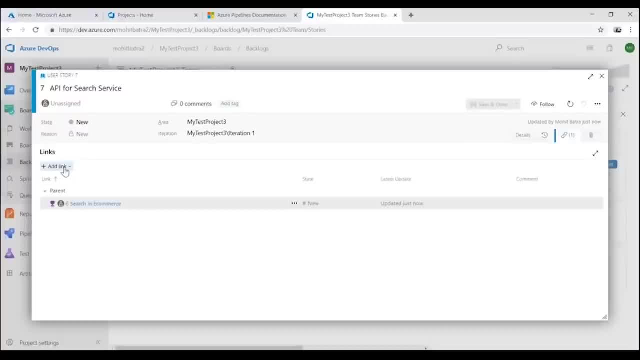 and I can say that I want to add some child items here. Okay, so I can say, add a new item and that is a child item which is of type task, and then I can say that I need to do some basic setup or maybe let's say some design of my search service. 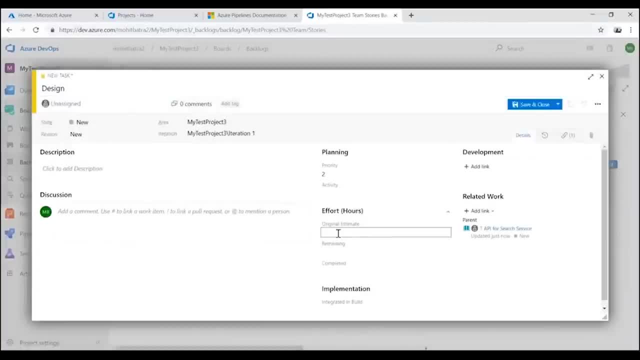 So that is one task I'm creating, All right. So what is the original estimate for creating this particular task? I can say 10 hours. What is the remaining time? 10 hours completed, 0, and I'll provide some description here and save it. 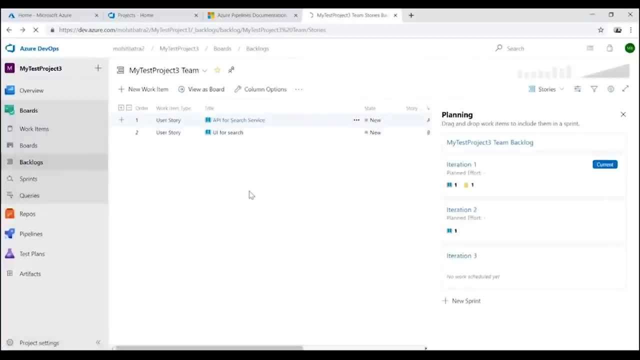 So this means, if I close this one- and in fact I'll just refresh this page- You will get a complete idea of what are the tasks which are, or what are the stories on which you are going to work on, or, basically, what are the backlog items. 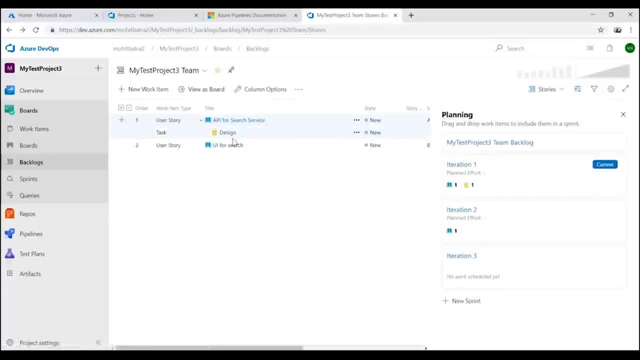 on which you are working in and what are the tasks under that. So this is the kind of thing that you can set up with Azure DevOps. I hope this stuff is clear to you guys. So we have got different iterations. Let me click on Sprints. 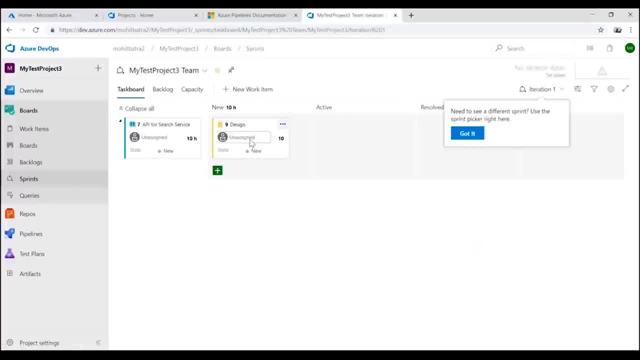 So you can see, right now The first iteration is going on and the design is here. Once I start working on this, I can even see use the visual editor to make it active. Once this stuff is done, I can even move it to the result state. 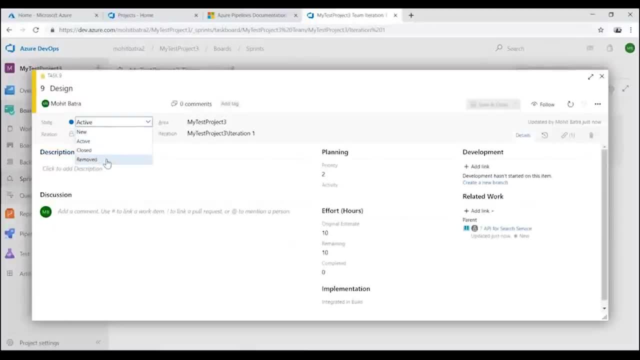 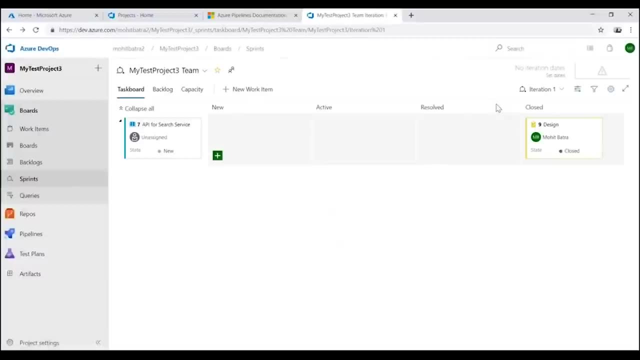 Okay, let me just open this one. I can just close this task and say that's it. So this is how my overall flow of basically the work items work Now. next thing which I want to show you is repositories. Repositories: We mentioned that we can use either git. 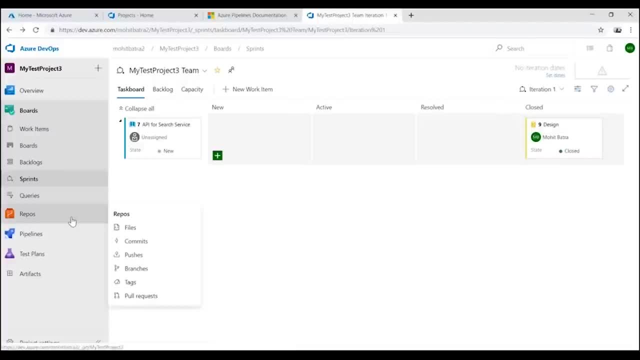 or we can use TFS to basically maintain our source code. I'm just going to show you a demo right now to show you how all this stuff works. So what you will do here. you can set up a repository which is like a git or a TFS. 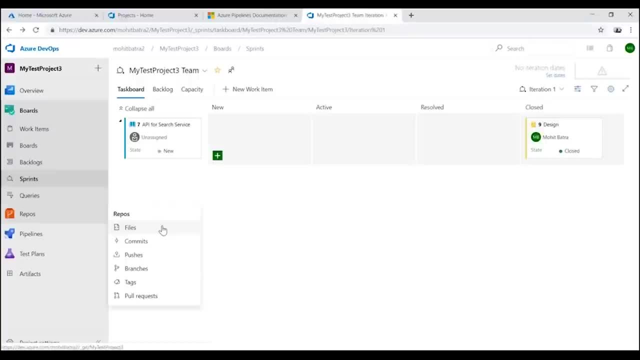 Then you can go ahead and start checking in your code. What first thing you will see here is because we are using git, So I'm clicking on something called as branches, and in the branches there is a default branch which is always available. Now that's called as a master branch. 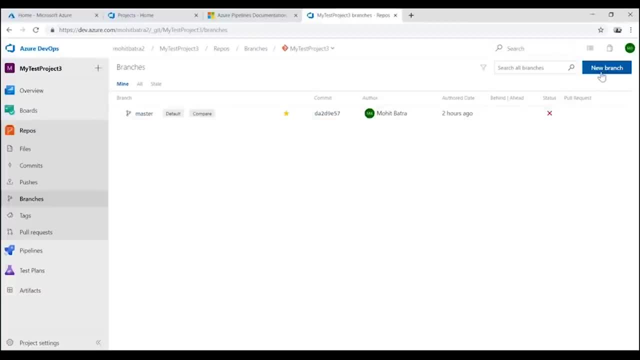 In fact, you can go ahead and create more branches in some of the source controls, like TFS. You will have one single place where everybody is checking in the code. Now, in case of git, it does not work the same way. It's a very different structure. 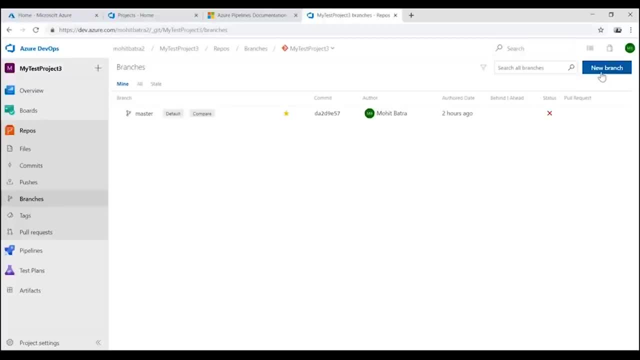 So what you do is you create your own branch. You work in that branch, which means branch is basically a copy of a master branch, So you will go inside that branch, You will make your check-ins. Now, that is your branch in which you are making the changes. 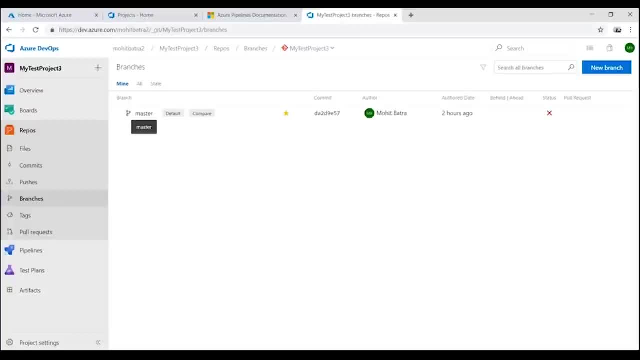 You will do the testing. Once you are completely fine, that everything is running fine, then you are going to push those changes from your branch to the master branch. Remember that if you haven't worked with git before, so there is nothing to worry about. 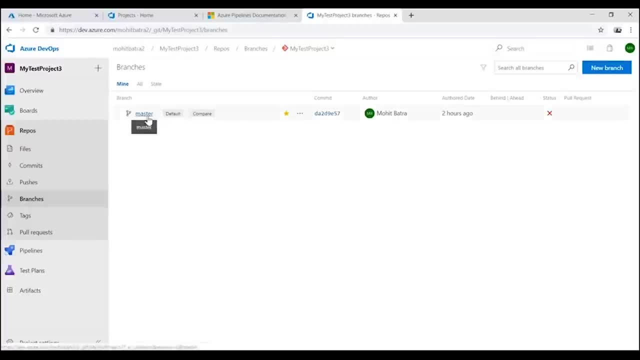 because this is not something specific to Azure DevOps. What I'm talking right now about the branches, this is something specific to the git. So let me show this thing: that we have right now a default master branch. If I'll click on this one, 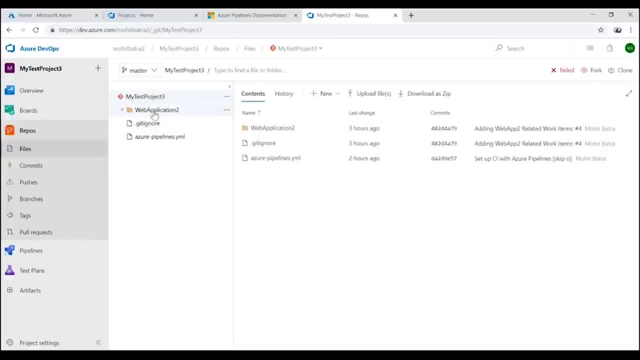 what you will see. I have already check-in one particular project into my repository. Okay, that's called as a web application too. If I click on this one, it's a very simple MVC application that I've created and added it into the source control. 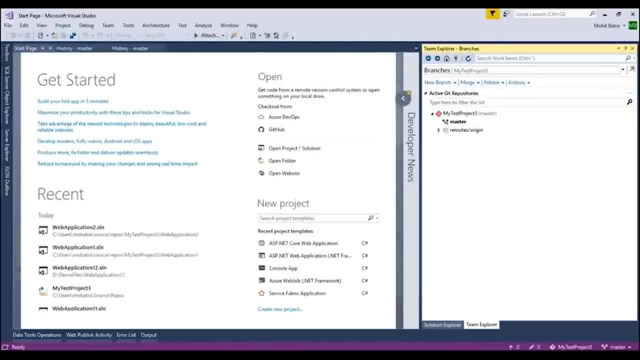 I'll go to the visual studio Now. in the visual studio, you can again see that I am using git tools for visual studio And this is showing me that I have got a master branch. Now what I can do, I let me create one more application. 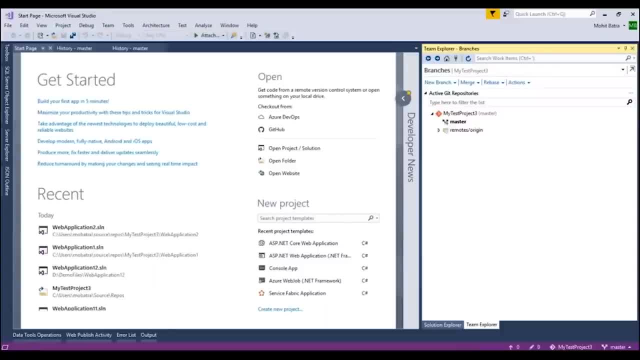 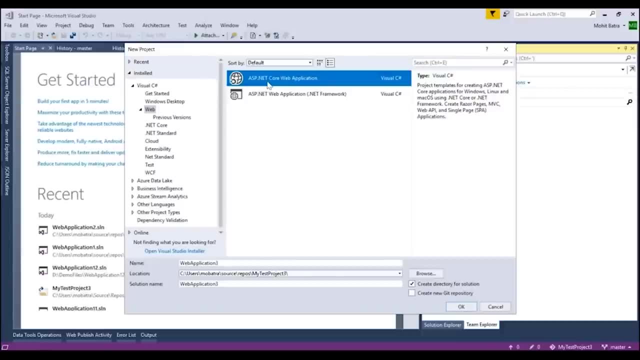 and check that in. So let me create a simple application file. new project: aspnet core web application. Remember you can use Eclipse, You can use IntelliJ or you can use any other ID to do the development. Okay, So this is not restricted to dotnet or visual studio. 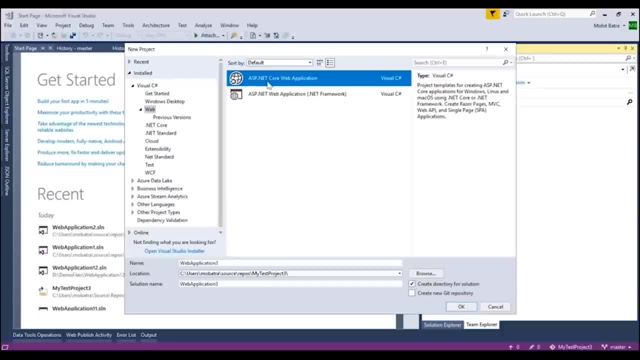 You can do. use any kind of platform or any framework to build your application, or it can be in any ID, Eclipse, IntelliJ- Anything will work here, All right. So what I'm going to do is create a new application called web application 3.. 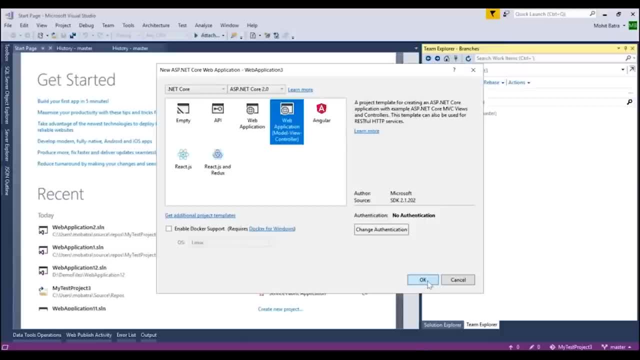 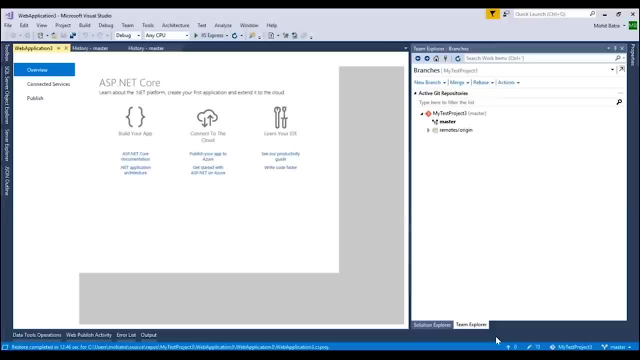 Let this application being created. All right, Now that we have created our application, what do we need to do? You can see here that my project is ready. I'm going to simply push this code into the source control. Okay, How do I do this? 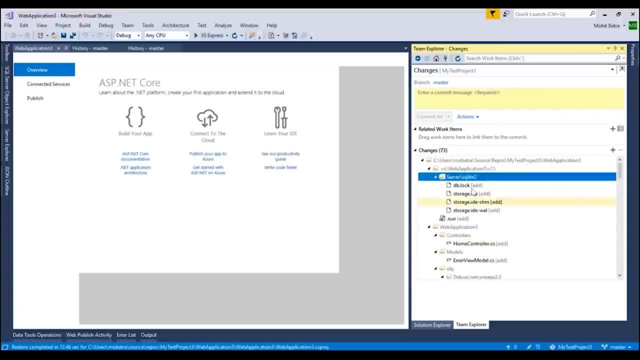 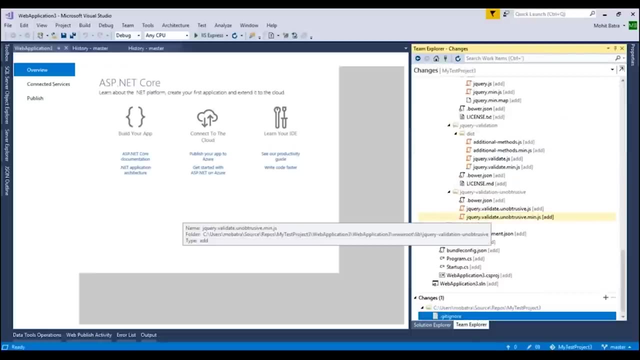 Let me first of all ignore few of these items, and what I'm going to do is: Okay, I'm going to state these items Now. this is something very specific to git, So if you are not comfortable with git, do not worry, because this is something you can learn very quickly. 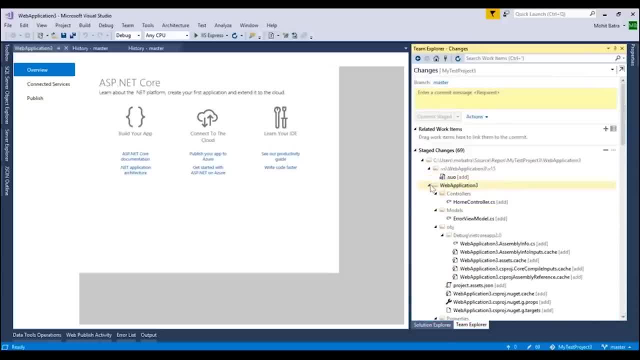 All right. So what do I have here? I have got my full application, which is web application 3. I can go ahead and check in into a git repository which is managed by Azure DevOps. So I'm going to say checking in. 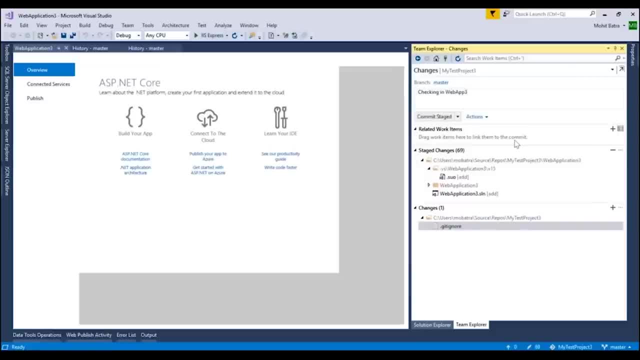 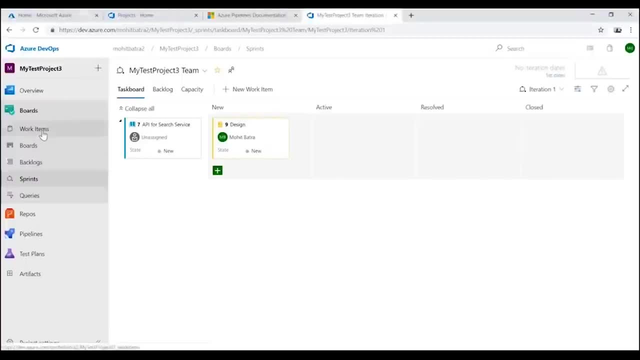 Web application 3.. Okay, Also, I can actually go ahead and map it to a work item. Let me click on this one and go back to portal, to my work item. In fact, we do not have a work item for development. 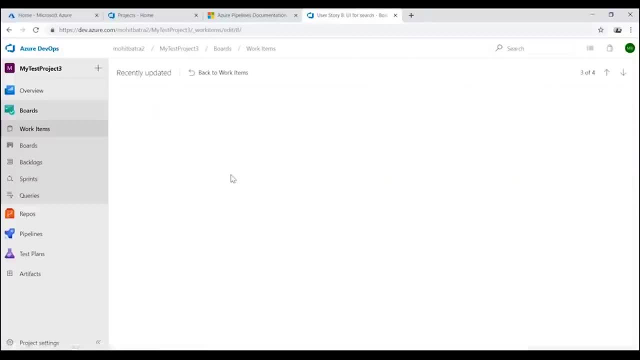 Let's create one. So UI for search service. Let's go back to the links. I hope you guys remember. now You can click on add link, new item and let's say we call it build web app 3.. Okay, let's call it create. 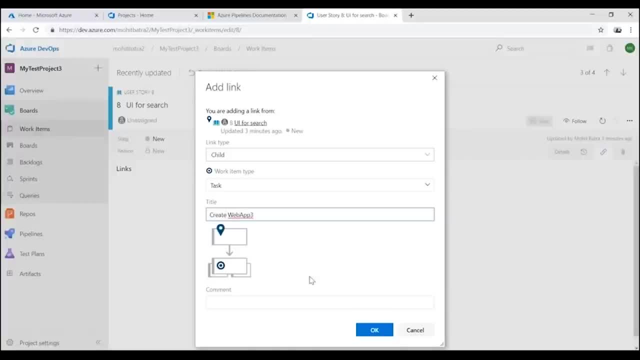 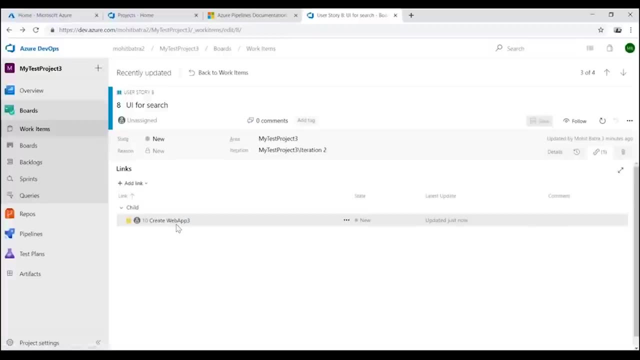 I know this is not the way we write the task, but just to give you an idea, that I'm just creating a new task called create web app 3.. That's it. So it is going to give me create web app 3. task is ready. 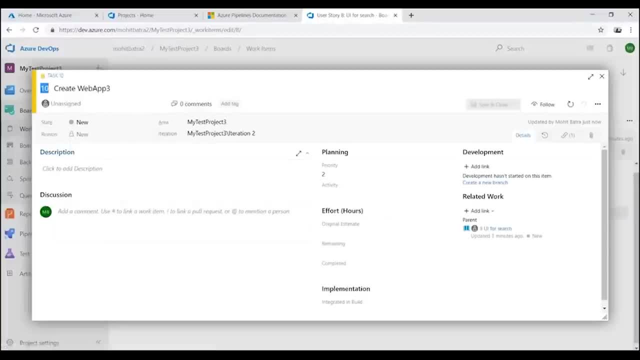 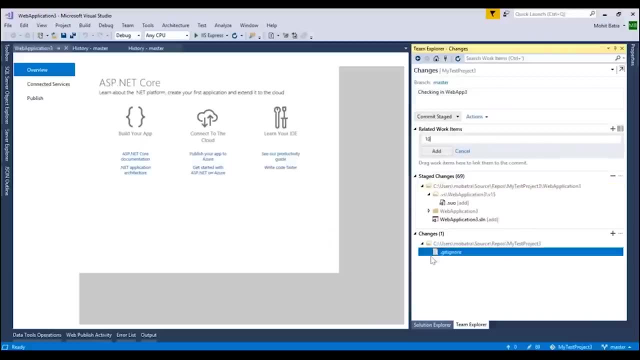 I can click on this one And the task number is 10.. Okay, so I'm going to copy this one. go back to Visual Studio, enter the ID of the work item. Okay, so I'm going to say 10 is the ID. 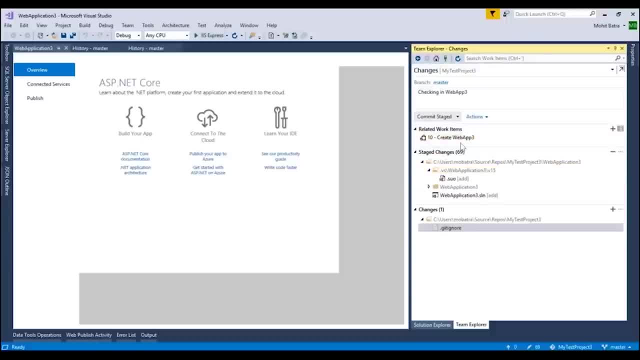 And you can see basically the related work item. Now, what we are doing here, We are creating a new application. when we are checking in the code, We are also specifying What is the related work item. All right, So let me commit all this stuff in the code. 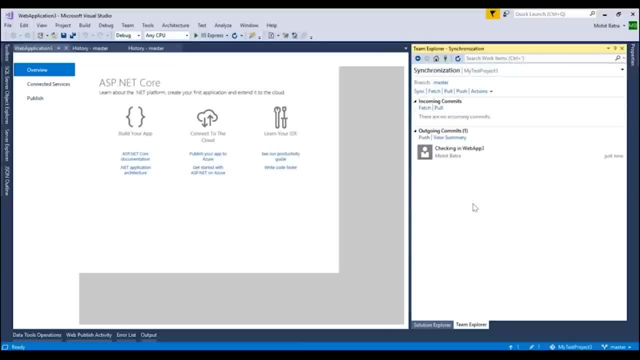 Sync it back to the cloud, which means now I have checked in into my local environment. I just want to push these changes into the cloud environment. So again, this is specific to git. You do not have to worry about this, Just give me a second. 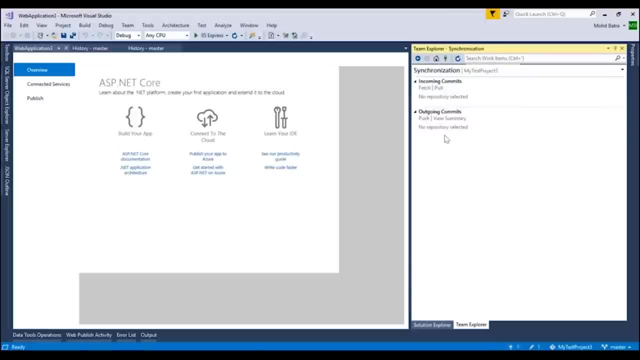 I'm just something related to, you know, git I need to. Okay, so I think this should work. Now it push these changes. Okay, so now this is going to push my changes to the source control. All right, so you can see here. 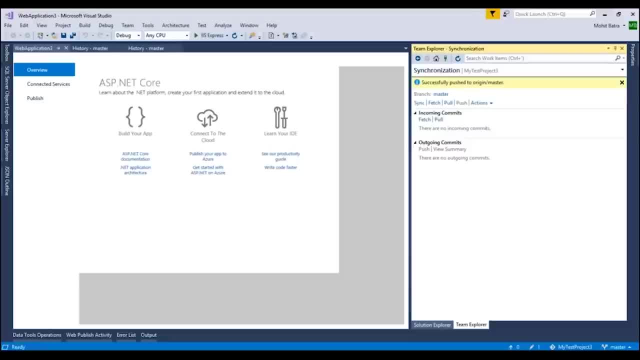 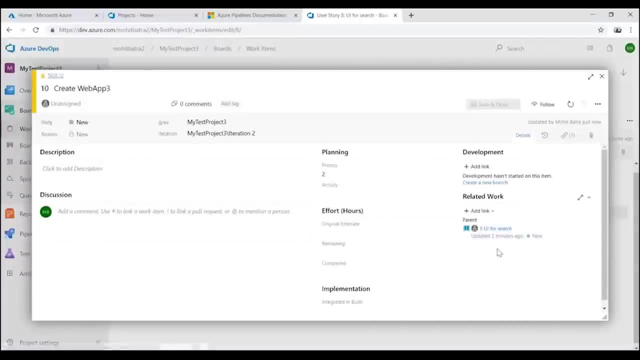 It has been successfully pushed to the master branch. If I go back to the devops environment, what you will see here, In fact, if I just open up the application as well, so you can see here This is the parent side and in fact. 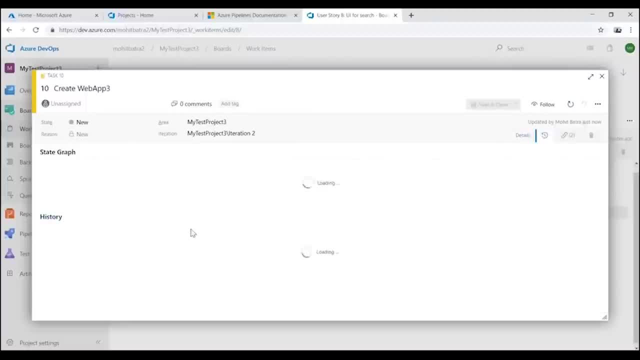 let me just refresh this one, Okay. so what do you see here in the description, Or basically in my history? I can see that I have done some check-in here, So it is linked to that particular chicken. Now you can start visualizing this stuff. 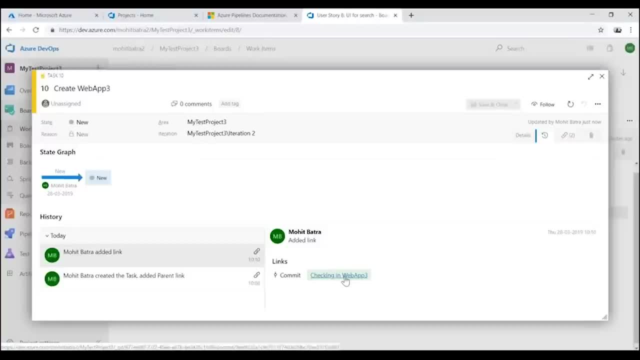 So you have got tasks, you have made your chickens. from those chickens It is coming in. Once you make a check-in and attach it to a particular work item, it will be linked to that particular work item. So if anybody is going and looking into what changes, 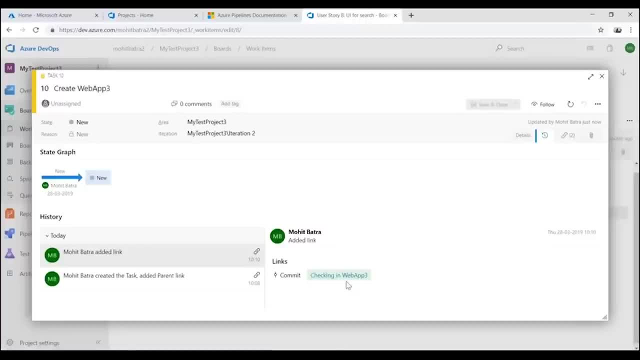 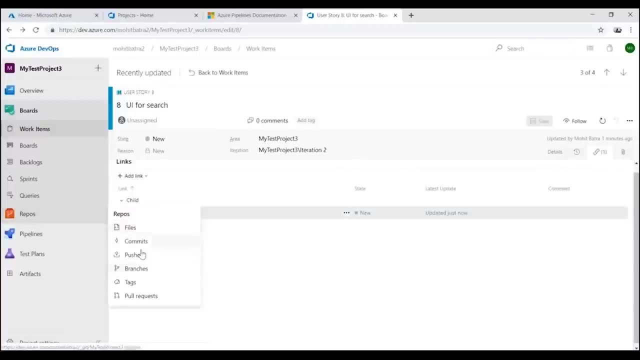 you have made as part of this task, you can actually go ahead and see all that stuff. Now, this is a part of the task. Next thing is let's go back to the repos and see the commits. Okay, we have made a commit into the repository. 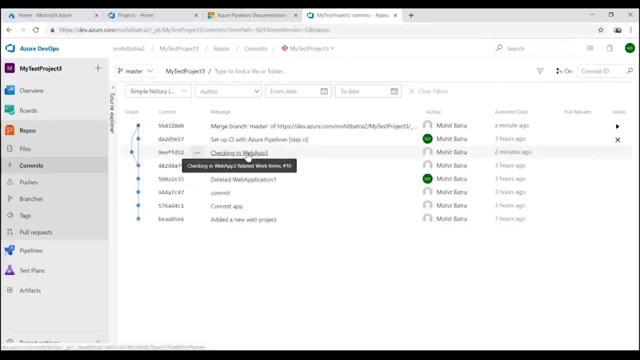 What do we see here? We have got check-in web app 3.. Okay, So this is what we have checked in as part of the web application 3 that we just created. Now The next thing is: I want to build this application. 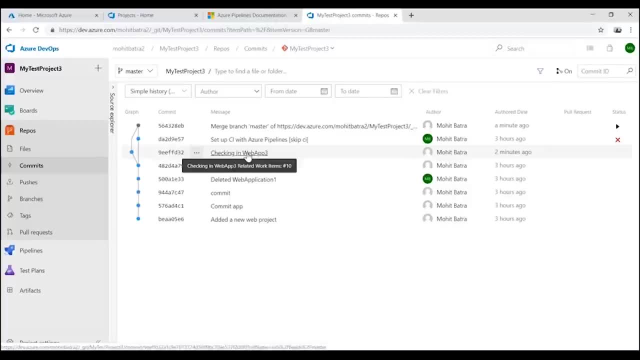 Okay, So if you guys remember, the second thing was checking in the source code. after checking in the source code, I want to automatically build this particular code. So what do I need to do here? I need to go to the third component called pipelines. 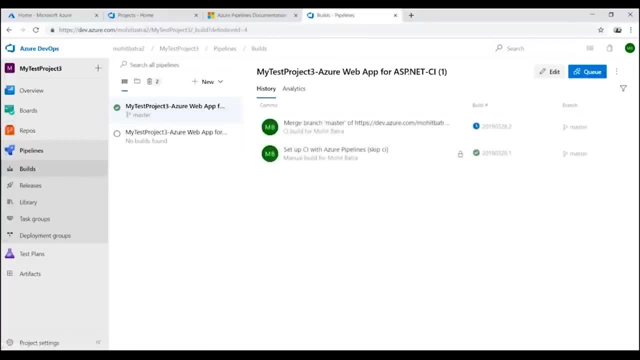 I see something called as builds, which means I want to take up this particular source code and do an automatic build of that. So what I can do, I can click on something called as new build pipeline. I've already got to create it. 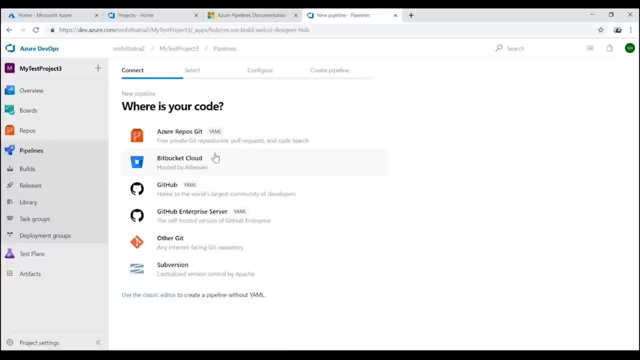 but I just want to show you from scratch how this is done. So where is your code? It is asking me. So my code is present in a git repository, So I'm going to select this one. And what is asking me that? where is your source? 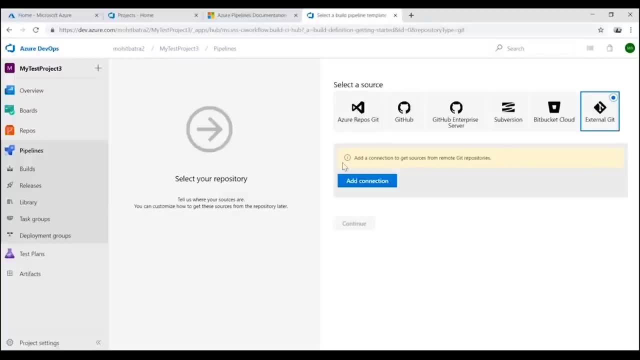 Okay, or where is your git repository? All right, So my repository is in Azure repos, git. Okay, so I'm going to select this one. You can even select GitHub, For example, if you just want to pick up the code from GitHub directly. 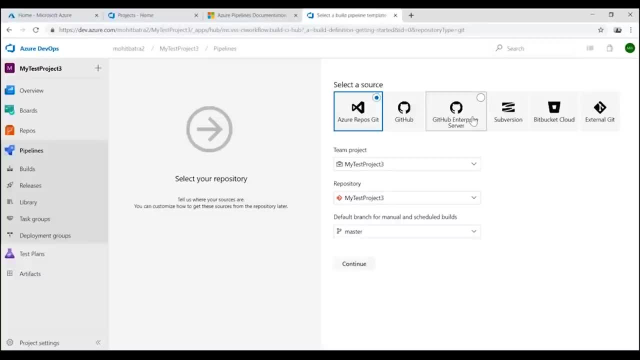 and use it. you can do it here, or you have the GitHub Enterprise server. If you have got GitHub deployed in your local environment or in your Enterprise environment, you can use subversion, or you can, in fact, if you have got TFS, there's a different way to use it. 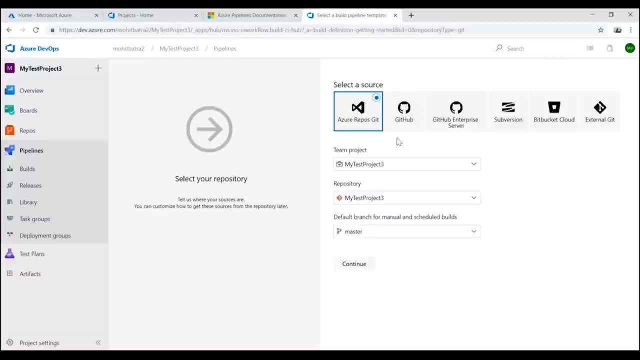 But then right now we are focusing on using the git in Azure repos. All right, So here you can see it. I have got my test project 3, which is my- basically my- repository and my team project. Then I'm going to pick up all the code from master branch. 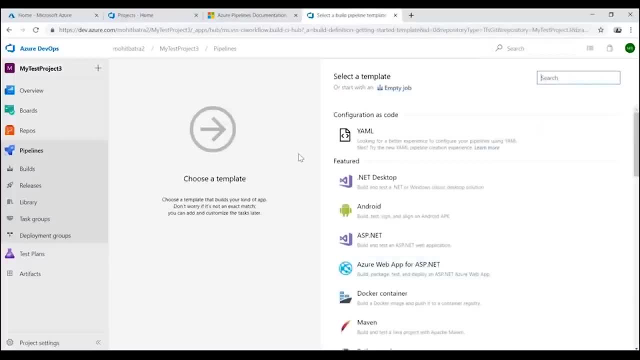 Okay, so I'm going to click on continue and the first thing that I need to do is tell Azure how to build my project. So how do I want to build my project? I want to build this project as part of Azure web app. 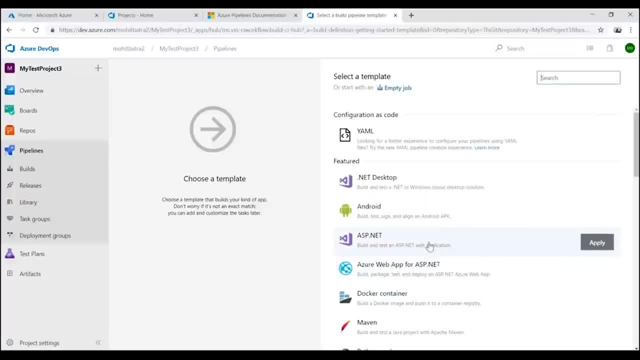 This means I want to take my code and finally, I want to deploy it in a service in Azure called Azure web app. When we say as your web app, then I want to build my project as part of the Azure web app, Okay, So if you want to do a normal build, for example, 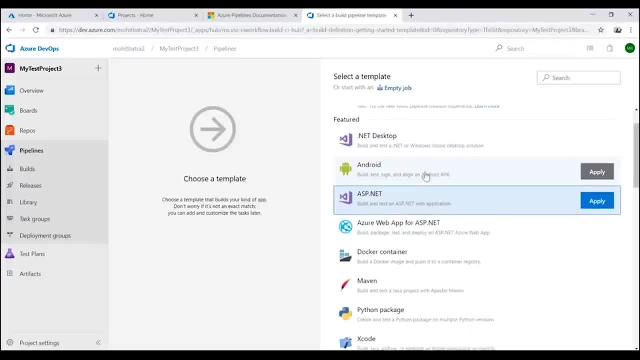 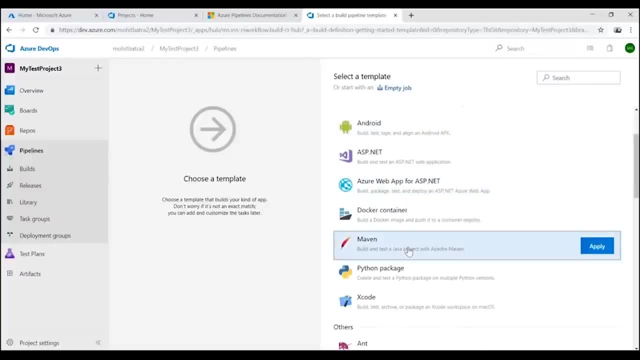 of your aspnet application. you can do it. If you have a got an Android project, you want to build it. If you have got Maven, let's say you have a Java project and you want to use Maven to build your projects. 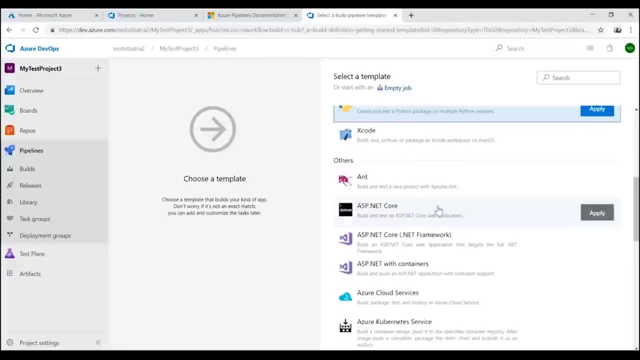 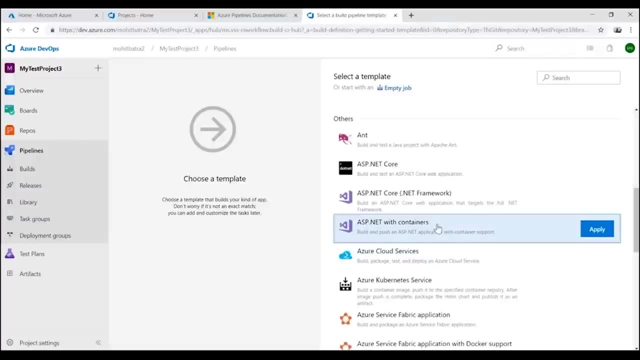 You can do it. You have got python packages, You have got aspnet core, Then we have got. if you have know what is a container, if you want to build docker containers, you can do it from here. If you want to deploy, basically build. 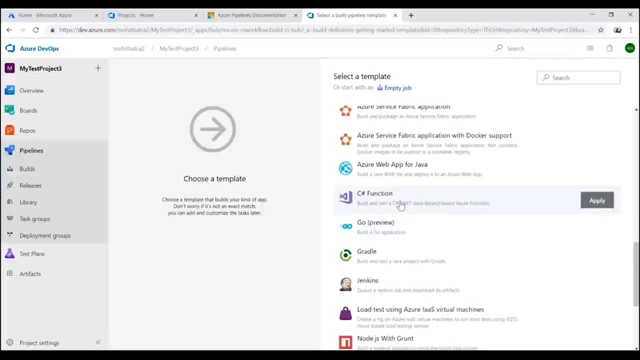 and deploy for Azure Kubernetes Services. you can do it. Then, if you have got just a function, you can build a C sharp function. You have the Azure web app for Java, So all these things can be done as part of the Azure build pipelines. 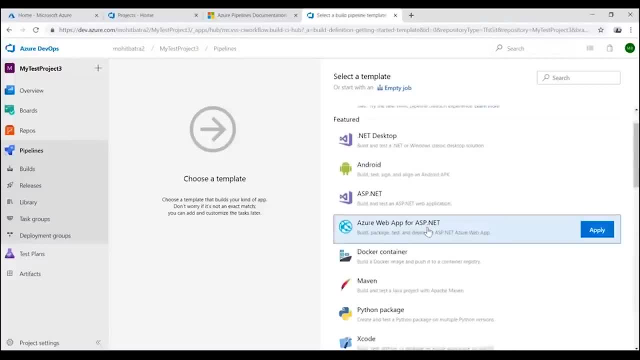 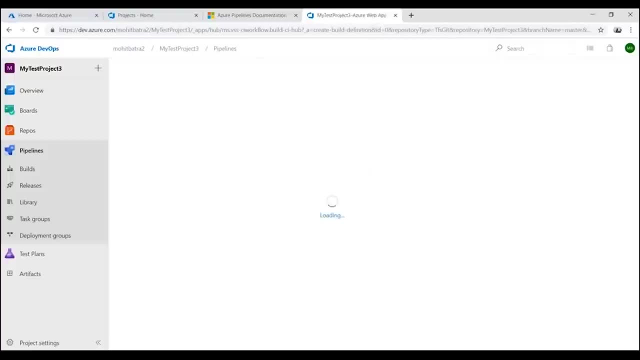 Okay, So what I'm going to do right now is select a service in Azure. Basically, I want to deploy in this particular service called Azure web apps, and that is why I'm going to select this one to build my code. Now, if I have to build my code, 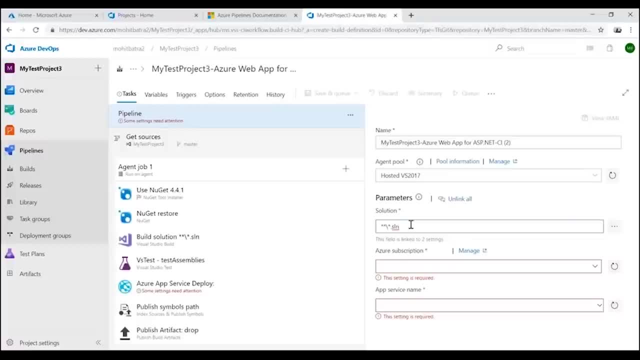 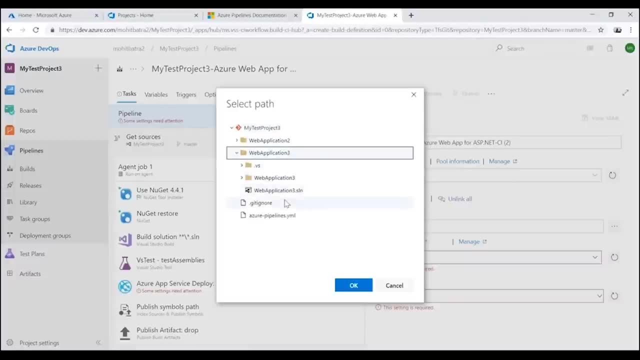 what do I need to provide? I need to provide: where is my solution? All right, so I'm going to click on this one and tell the system, or basically tell my build pipeline, that it resides in web application 3.. Okay, This is my new project that I picked up. 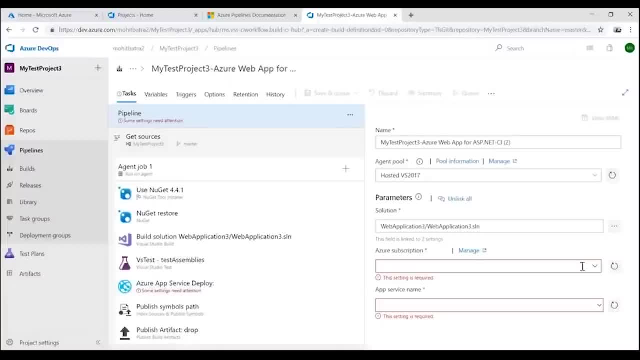 I'm going to select this one and click on OK. Then finally provide where is this as your subscription in which I want to deploy? So I'm going to select: this is my subscription in Azure and what is the name of the app service. again, 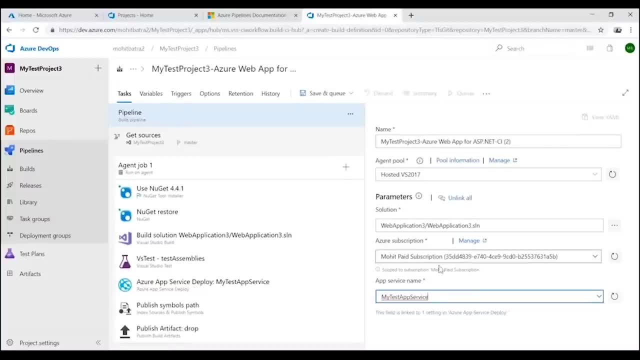 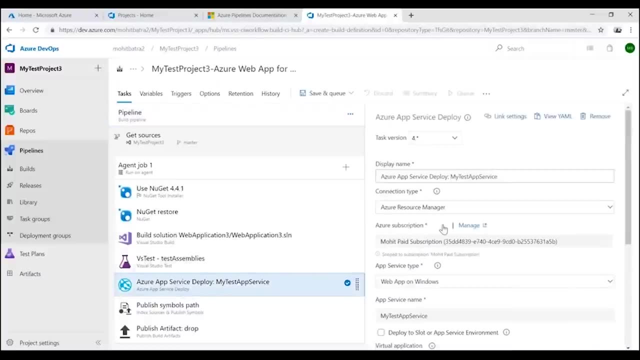 There are a few things that we are rushing through. Okay, So this is what we can select, and next thing is: I can go ahead and select. So this is what we are going to do. We are going to build as part of the build pipeline. 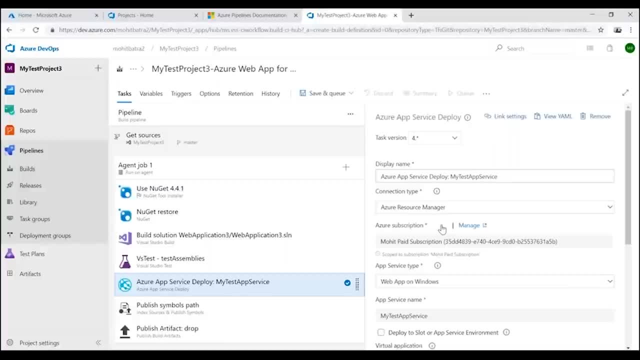 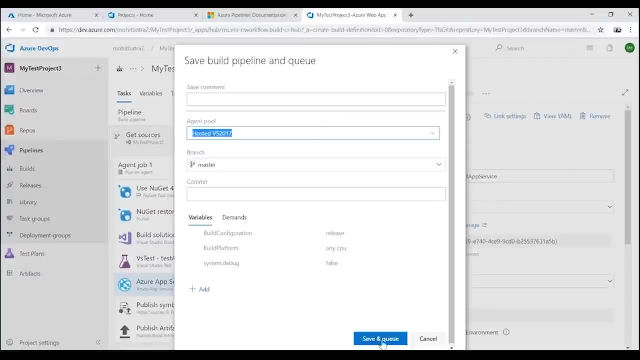 So we are going to take the source code from the git repository, do a build of it automatically. Let me save this one And cue it, which means I'm going to save this pipeline and start doing the build of my project. So now that we are built, pipeline is ready. 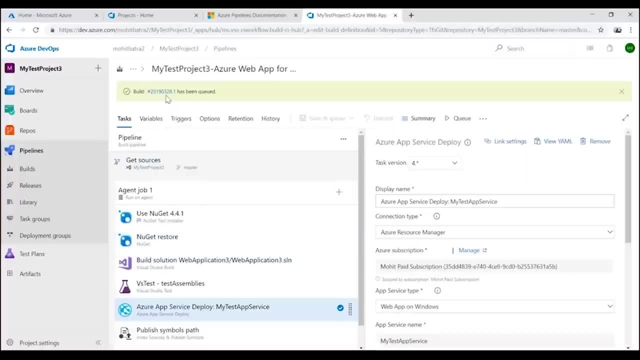 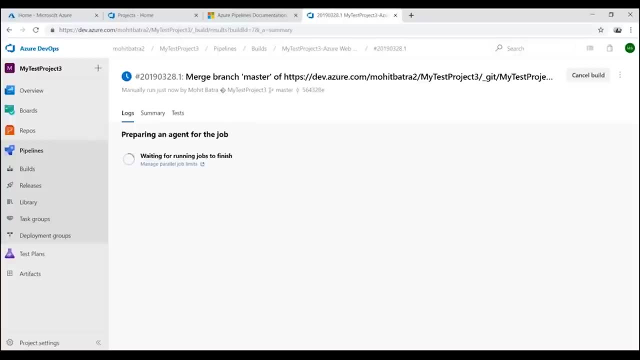 which means our code is going to be get built. Let me show you when the build is happening, What is going on. So it is does going to take some time to do the build, because this is the first time it is happening, but I'm going to show you that I already have one pipeline. 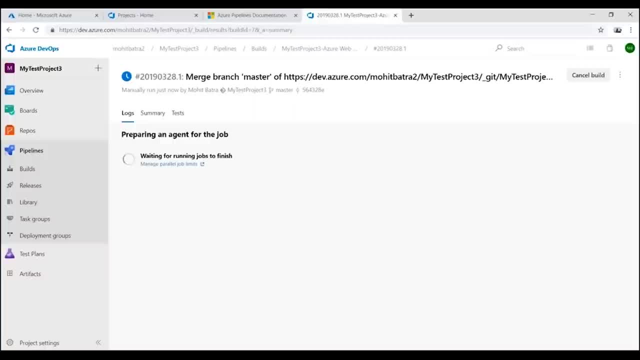 which is already built for my web application 2, which was very similar. So while this is running, let me go to builds. And this was a pipeline which was completed successfully, So let me select this pipeline. So this is how the build happens. 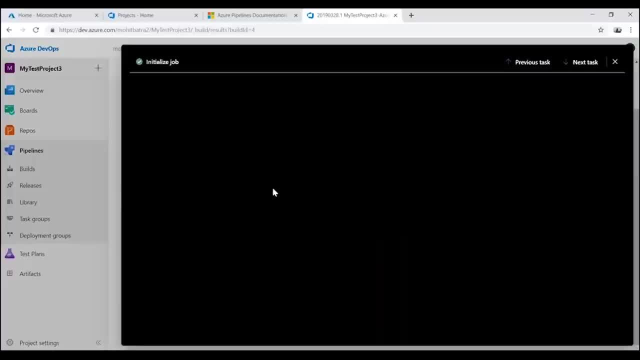 So if you open up anything, it is going to give you the detailed logs of how the build happened. So it picked up the code from your source control, It did a build and you can see all the build activities which happened as part of this pipeline. 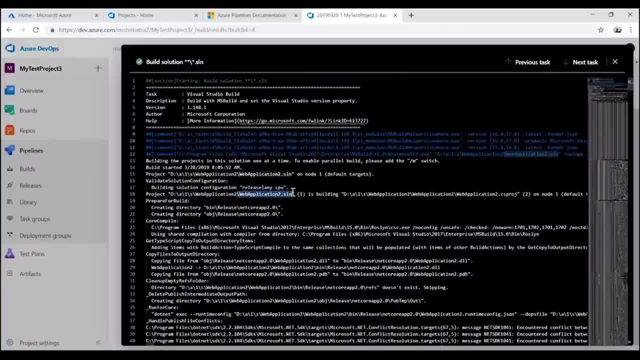 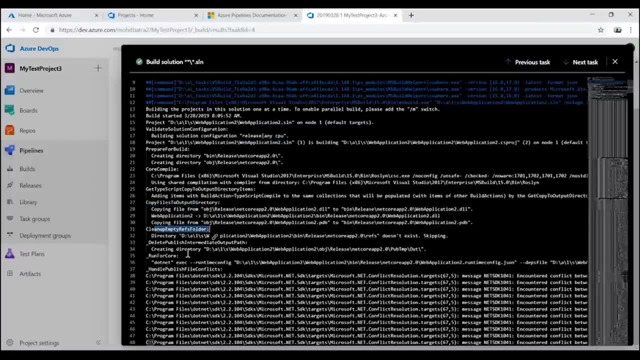 So you can see here: it picked up the web application 2 project And it started doing the build. It did all the copied files to output directory and cleanup and all that stuff And finally it did a build of my project. Now, once I did a build of my project, what next? 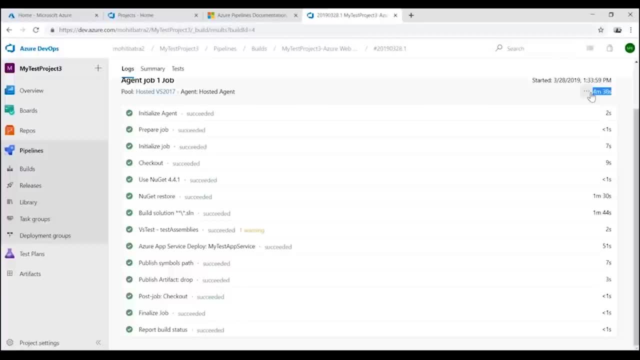 so you can see here it approximately took 5 minutes to do the build. So what you can do as part of your Azure DevOps: as soon as somebody checks in the code, it will automatically trigger a build pipeline using which your application will be built. 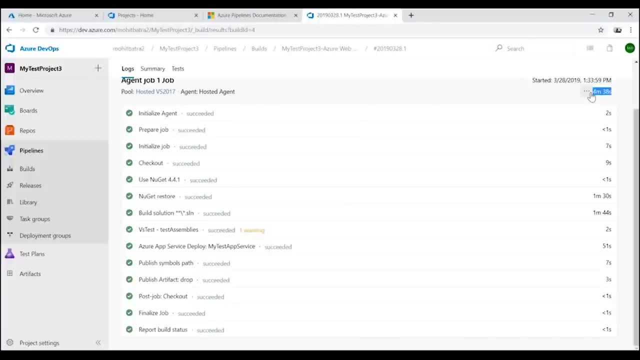 And if there is a failure, then the person will be informed back using a mail that your code is not correct. Okay, so you have to rectify your code as soon as possible. Now, once we have done all this build activity, what next do we need to do? 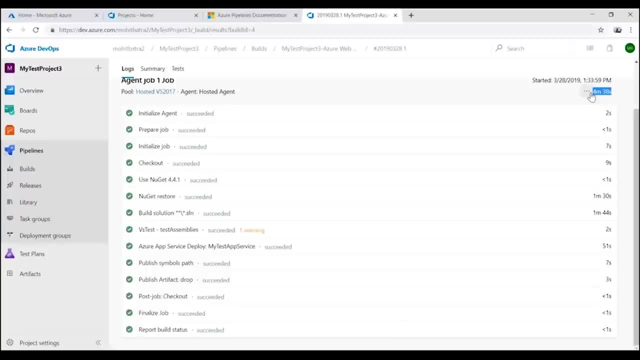 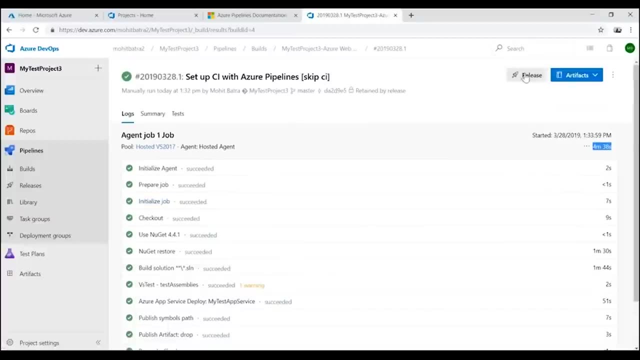 We need to release it to a production environment, or maybe to a UAT environment. How do we do that? We do it using something called as releases. So now that this one is ready, either I can click on release and build up a new release pipeline. 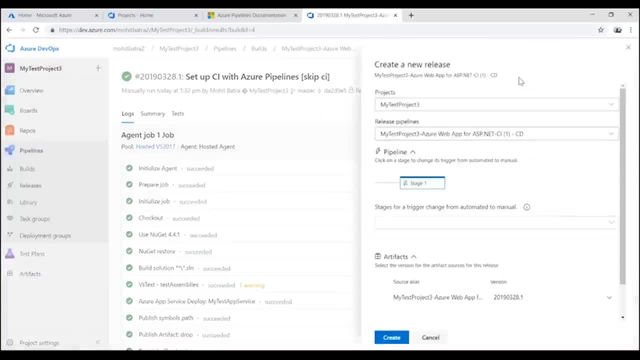 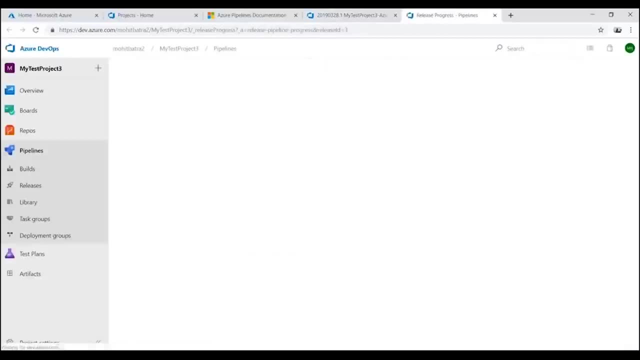 So let me click on this one And I'll say I want to create a new release. So I'll click on release to, and what you will see here Now that the complete build which happened. now it is asking me that where do you want to release it? 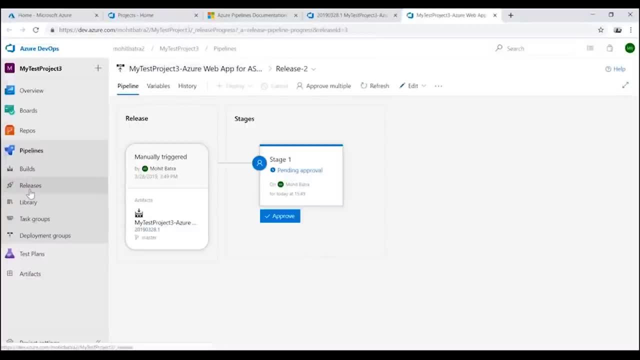 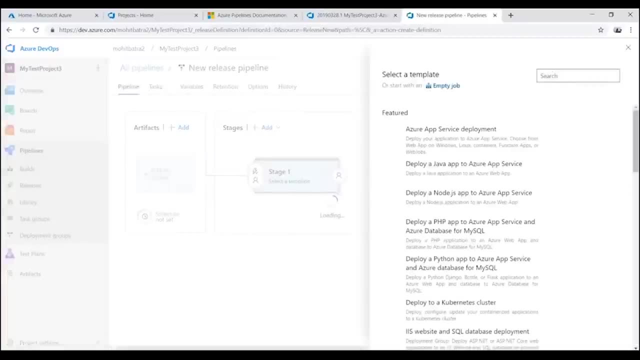 So I've already created a release pipeline. In fact, we can let me click on this and let's create a new one as well. releases new pipeline And is asking me: where do you want to do the deployment? So I'm telling Azure that I want to do the deployment. 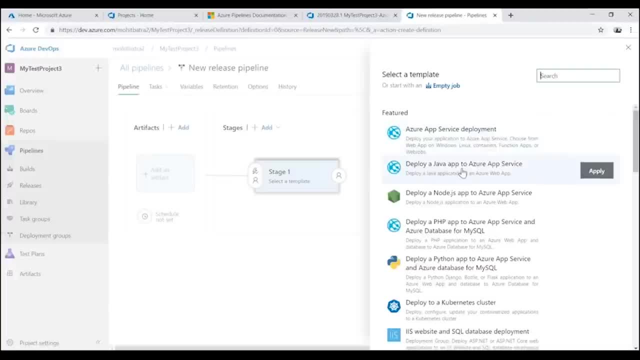 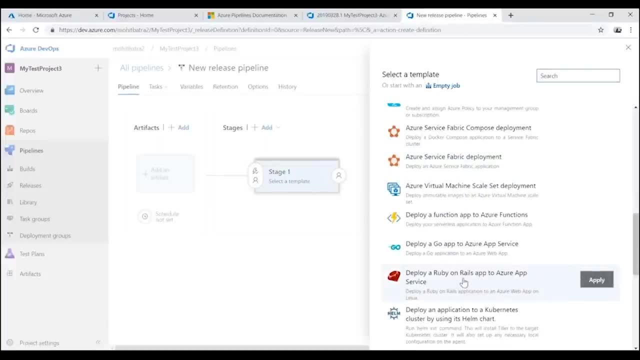 in Azure app services You can deploy a Java application. You can deploy a nodejs application. You can install it in service fabric. You can install it, you know, deploy a rails on Ruby application. on app service, You can deploy an is website. 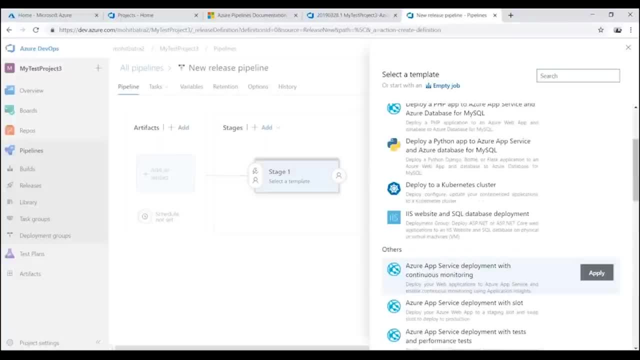 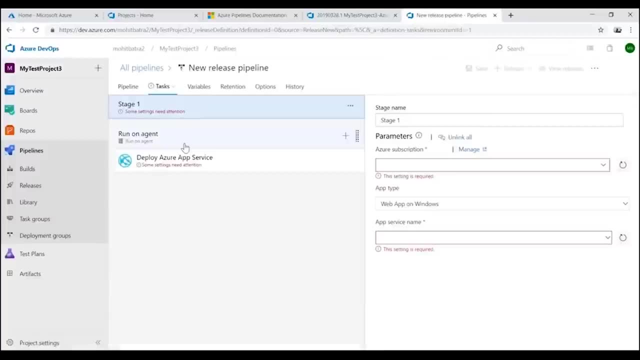 All right. so all these things you can do And I'm going to deploy in Azure app service, All right. So once I select this, I just need to provide what is the application basically which I want to build and what is the Azure subscription. 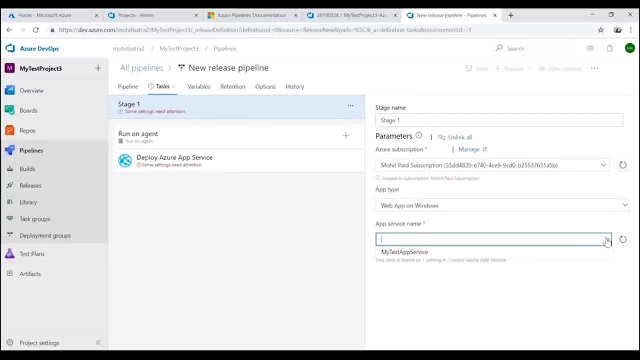 in which I want to deploy the application. Let me select this one. So there is one. I've already created my test app service. Once I've done this, I can save it. So this is my release. pipeline is ready. So now my code has gone into source control, my build pipeline. 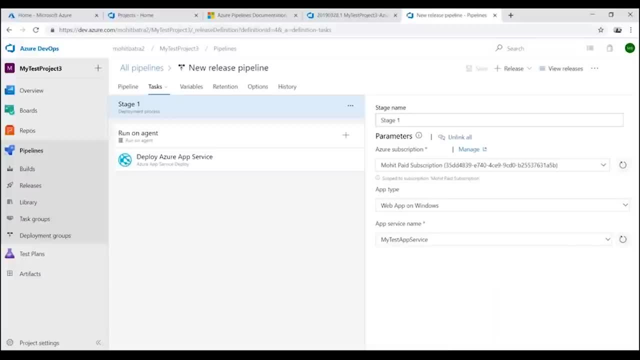 which is picking up that source code and building it. that is ready. Now This is my release pipeline, which is going to take that build code and going to do the deployment. Okay, so I can click on here and say: create a release and that's it. 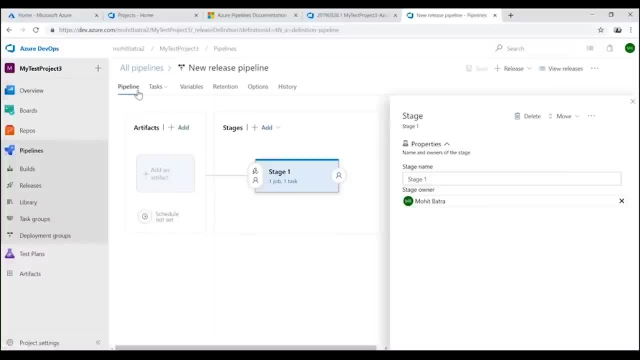 Or in fact one more thing I can show you: if I go back to the main pipeline, I can even set up who will approve it before it goes into a particular environment. So I can click, for example, pre-deployment conditions And say who is going to do the pre-deployment approval. 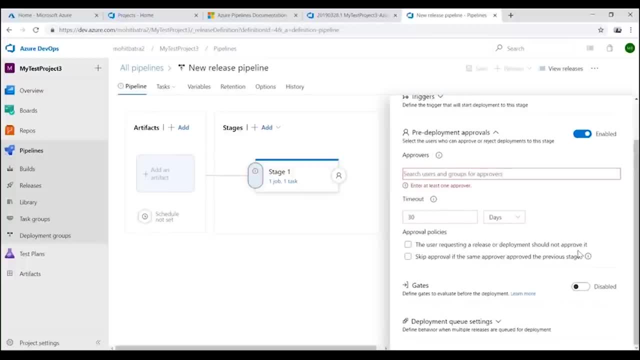 if your team lead needs to approve the overall release before it goes into you at or production, then you can specify who is the approver. So in this case, I'm going to put in my name, All right, and I'm going to save this one. 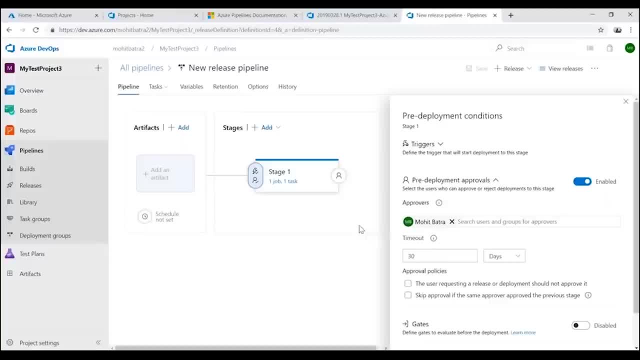 So this means as soon as the deployment will start happening, It is going to ask me for the approval. I'll get an email that please approve the release deployment. Then only it can go to production. So I'm going to click on now create a release. 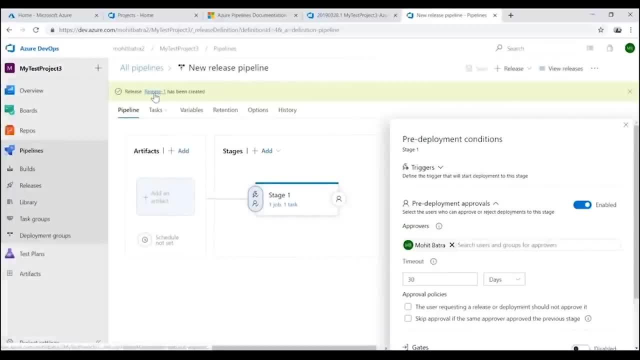 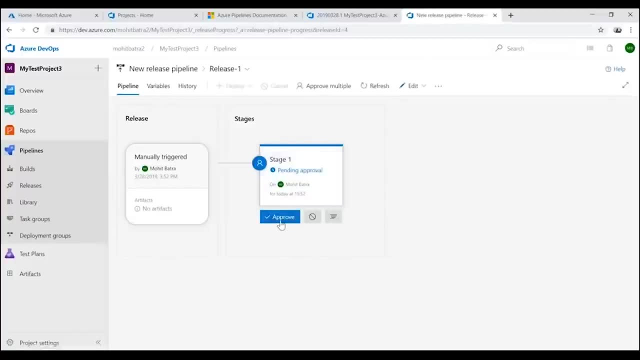 and click on create, So go to the release which has been created now and you can see it is saying pending approval. What I can do is because right now I am the owner, So I can click on approve and say yes, I want to approve. 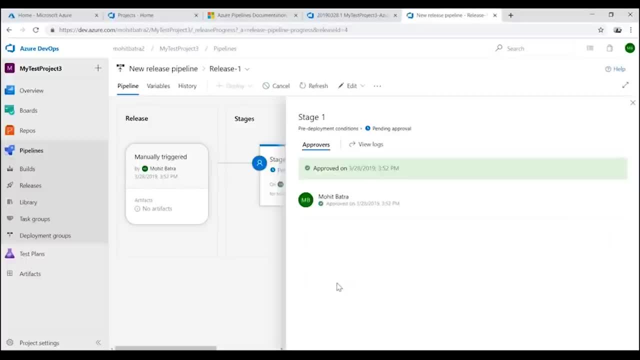 Basically approve this particular release And then it will continue further to do the deployment. Now you can see here The approval is done And right now this is under queue, which means as soon as the resources are available in Azure it is going to start the release deployment. 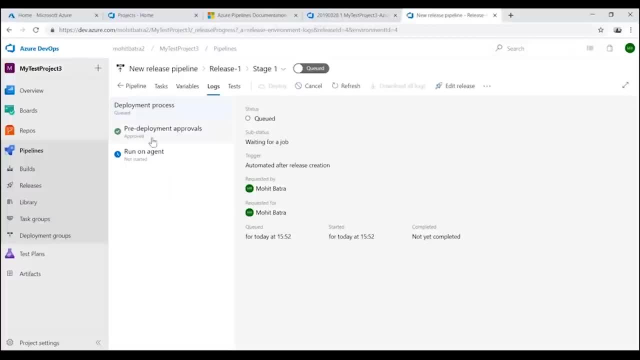 And while this is right now, it's in a queue state. I can show you the one which I deployed for web application too, So I'll go back to the releases. Okay, So this one is already done. In fact, not this one. 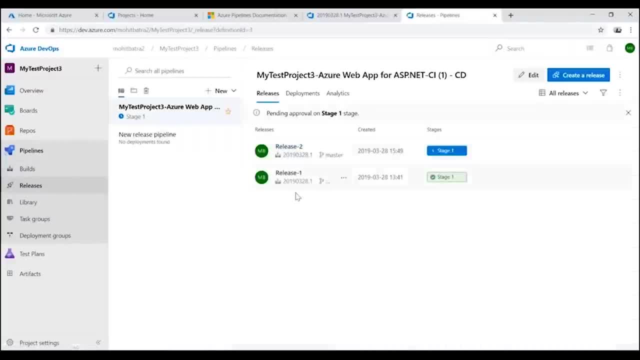 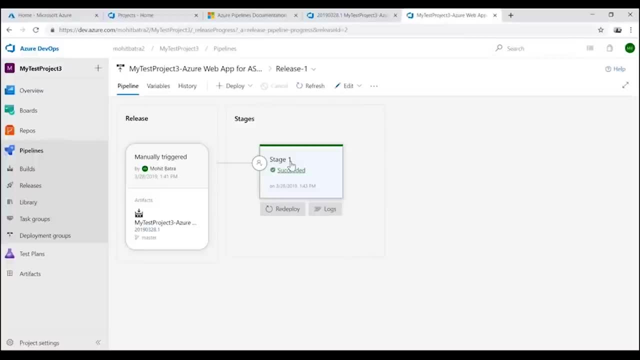 Just give me a second. Okay, so this one is already done. So what you will see here, after basically everything is done, or basically the release starts and it starts deploying- You can see the logs here If there is a failure in your pipeline. 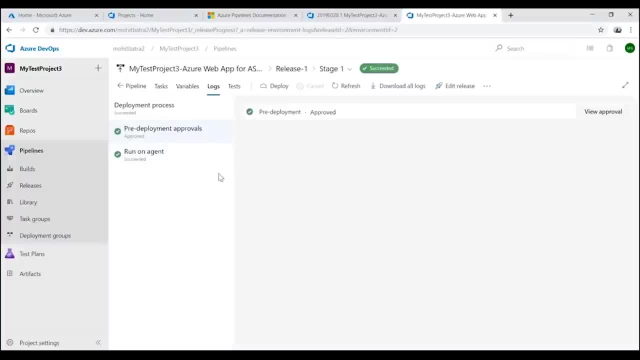 it is going to you know, inform you that there is a failure in the release, but you will get email so you can quickly act on that. Otherwise, it will download all your build artifacts. in our case, It was a web application. 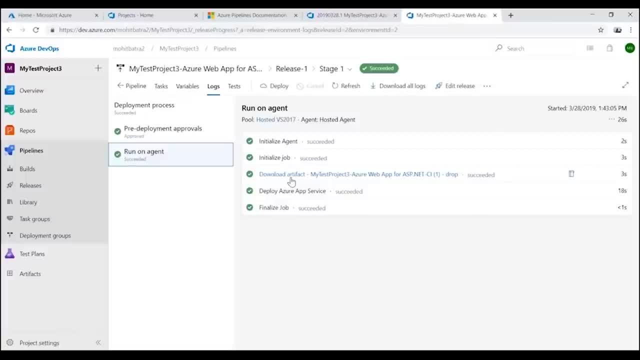 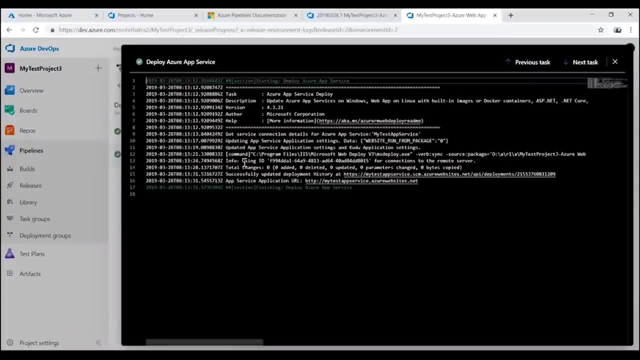 So it downloaded all the artifacts of my web application and then it is started deploying it to the Azure app service. Okay, so you can see all the logs. In fact, you can even write custom logs here that this is what we are doing as part. 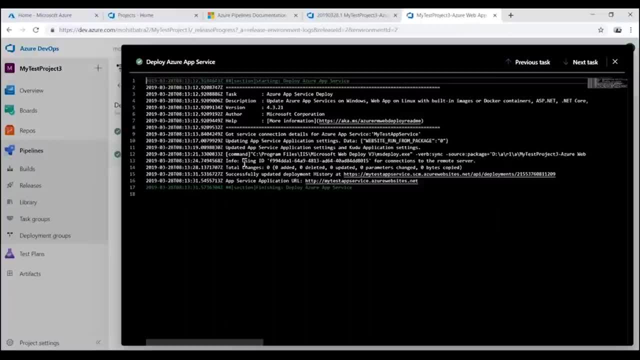 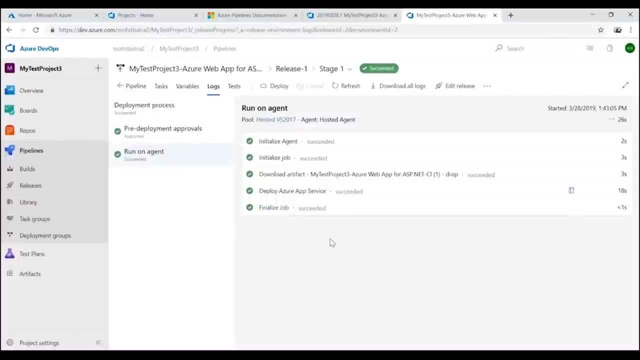 of the release: deployment on Azure app service. All right, so you can see here: successfully updated the deployment history. app service application is running at this particular URL and then you can use this URL Now, once this release completes, this means our code which we created, has been deployed into production. 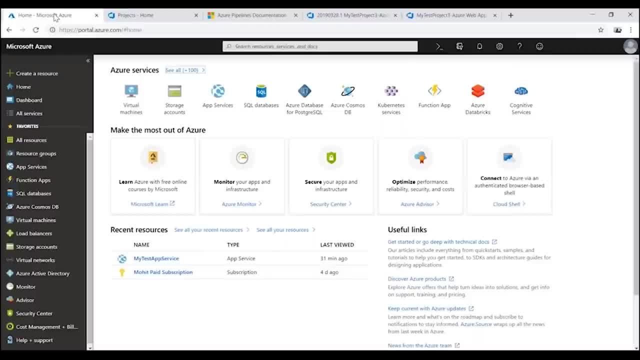 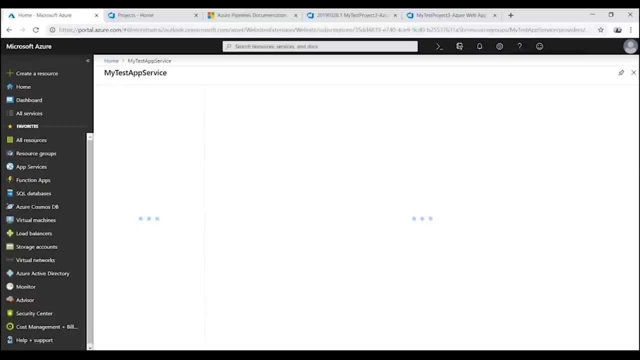 Let me go back to Azure now, Okay, and I'm right now into Azure portal, which you can get from portalazurecom. You can click on my test app service which we are using for deployment, And if I run this particular app service, 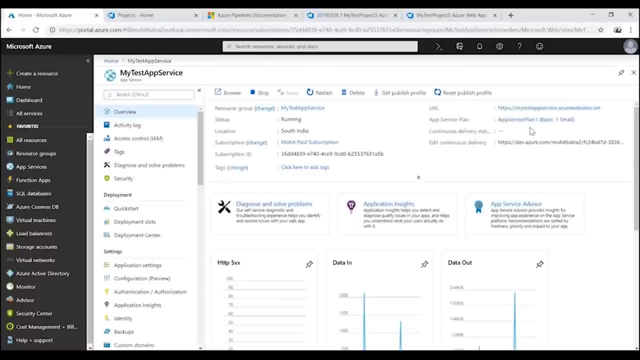 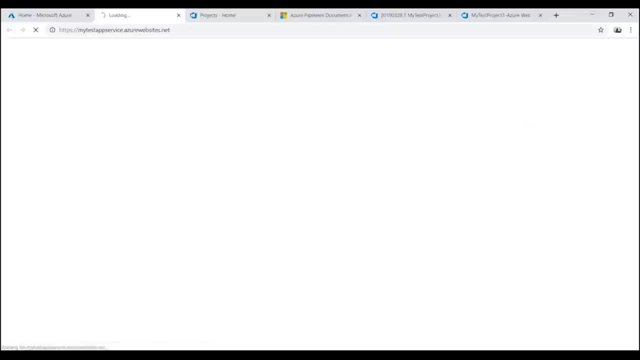 which is basically a platform for hosting the websites or, in fact, platform for hosting different websites, APIs, mobile applications- so I can click here and see my application is successfully deployed. So just to summarize all this stuff now you can see here: the application is ready. 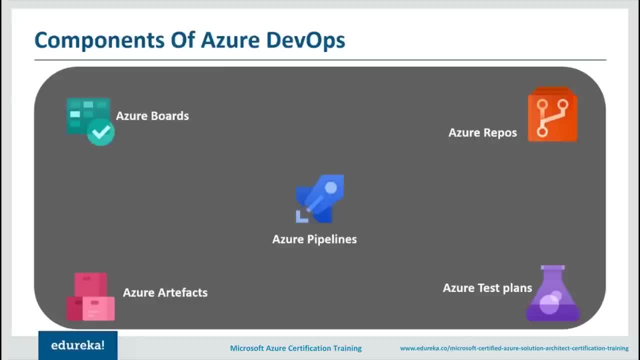 There are five components basically of the Azure DevOps, which means that we have got Azure boards in which you can manage your work items. You can manage the task, You can create either the scrum boards, Kanban boards or you can have the agile process. 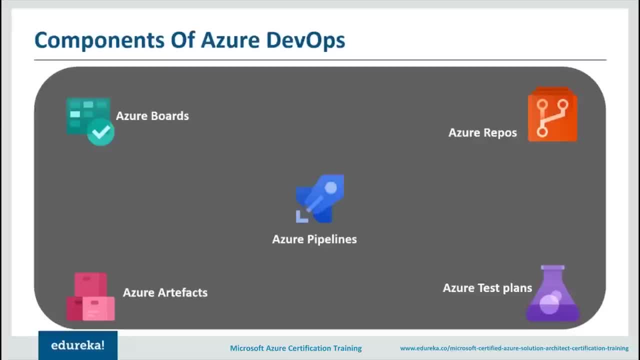 All this is being handled as part of the Azure boards. Now second thing is about as your repose, where we have got git and TFS, in which you can check in your code and you can manage all the branches. You can manage complete git functionality. 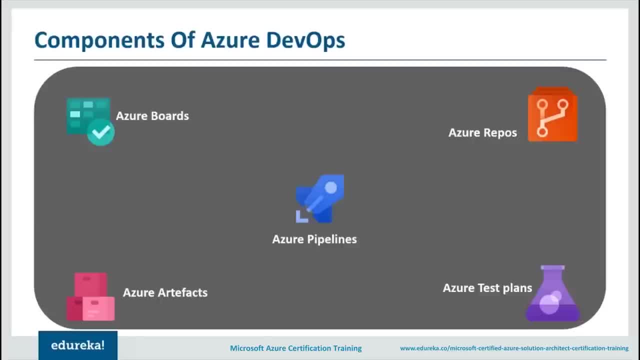 which is available as part of the Azure repose, so you can check in your source code there. The third thing is about as your pipelines, in which, after you have done the check-ins, you can build your solution and you can also release your solution in multiple environments like dev, pre prod. 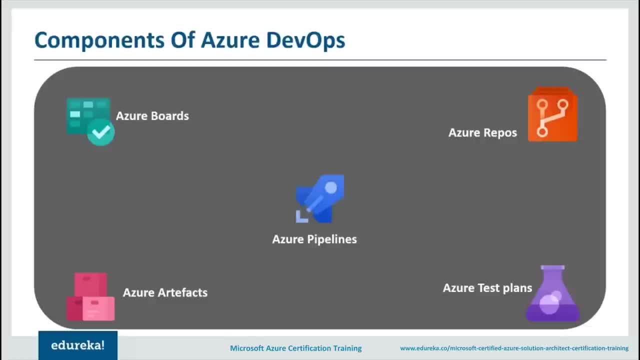 you at production, all that stuff. Next thing is about as your test plans, which we haven't covered. I just wanted to give you an idea of what is a test plan. So test plan is something where you can run your automated manual exploratory testing under as your test plans. 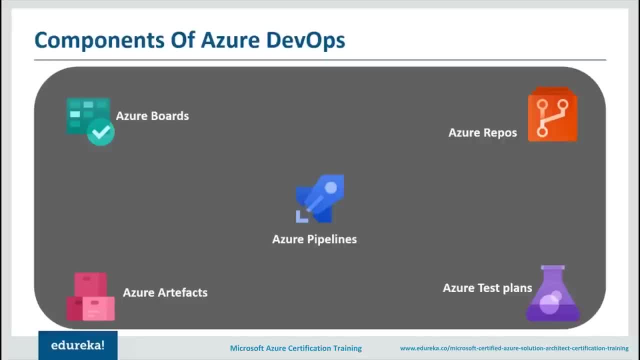 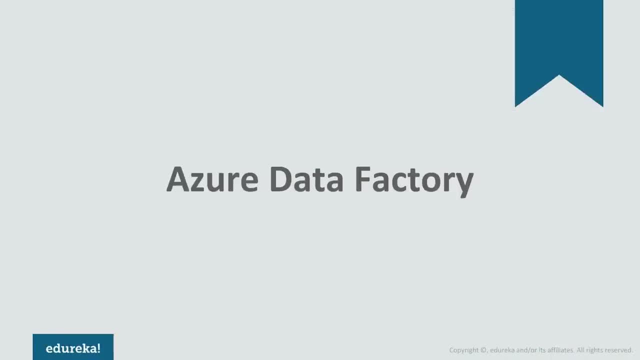 And finally you have the Azure artifacts, in which you can store some dependencies. So this is the overall picture of Azure DevOps. Today's topic of discussion is Azure Data Factory, which is very important from data integration and data management perspective. But before we do go ahead, 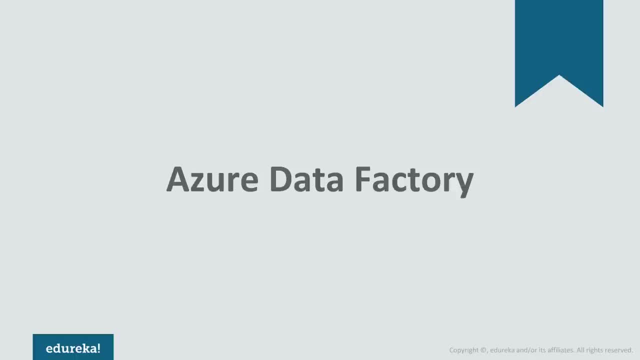 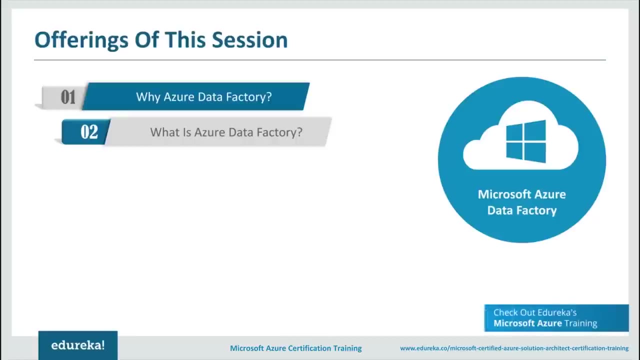 and dive into the concepts of this particular term. let's quickly start by taking a look at today's agenda. first, I would start things off by talking about why do we need Azure Data Factory and what it is exactly. then I would talk about various concepts that surround this particular term. 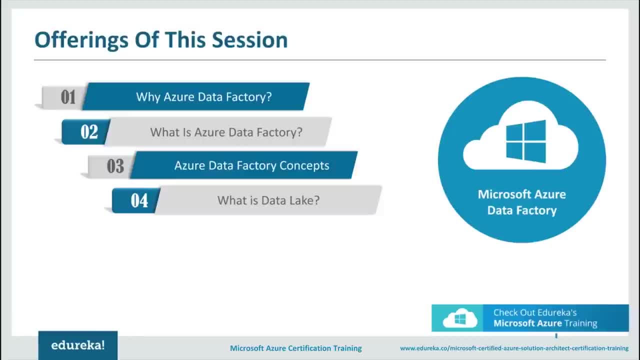 We would also understand something called as data lake- not into depth, but to some extent- and would also understand various concepts that surround this term as well. I would discuss two other terms, that is, data Lake and data warehouse, and what is the difference between these two terms. 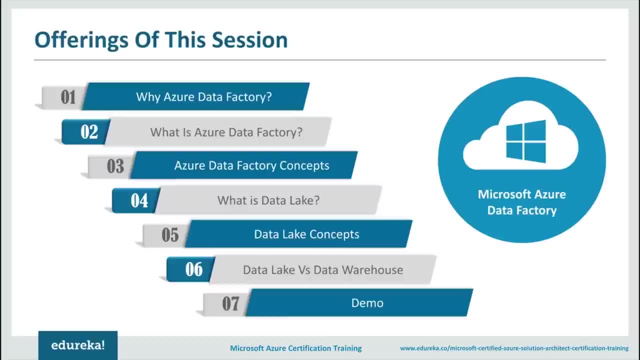 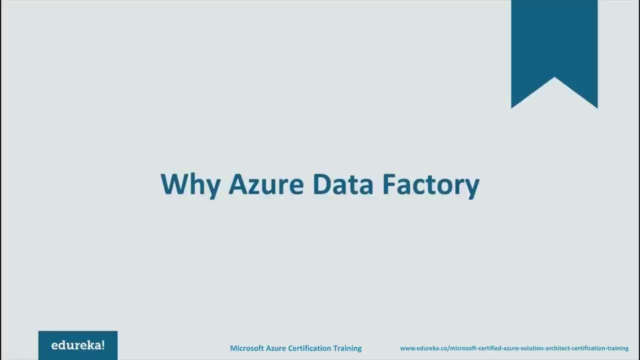 And finally, I would finish things off with the demo part. as far as this demo goes, I would be talking about creating a pipeline and moving data from one source to the other, but that is for the later part. Let's start with the first topic of discussion, that is, Azure Data Factory. 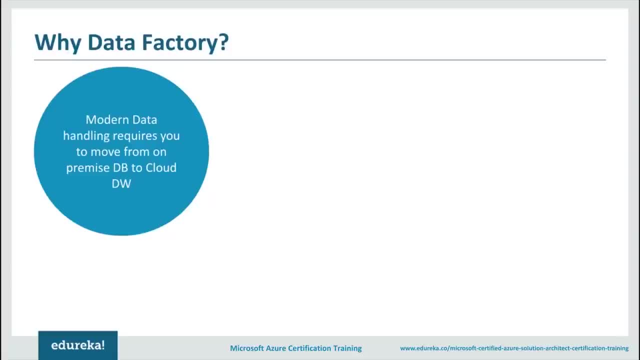 So why do we need Azure Data Factory? Well, first and foremost, we need to understand the fact that the amount of data that is being generated these days is huge, and this data comes from different sources. Now, when we move this particular data to cloud, 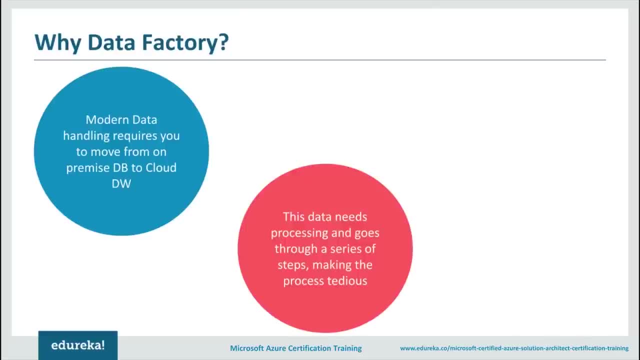 there are quite a few things that needs to be taken care of Now. this data. it can come in any form, because we are talking about different sources and these different sources would transfer or channelize this data in different ways, and it can be in different formats. 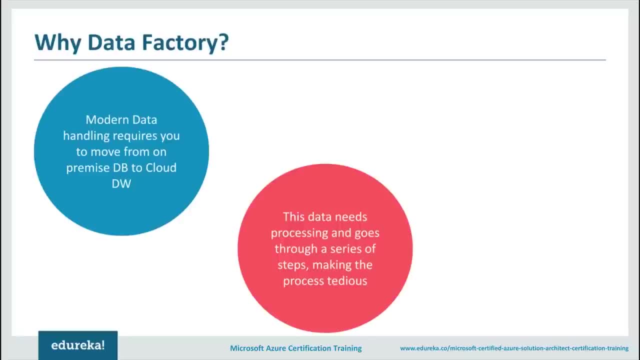 So, when you do decide to bring this data on cloud or at a particular storage place, you need to make sure that this data is well and truly managed. Now, what do I mean by this? Well, you need to transform this data. You need to delete unnecessary data. 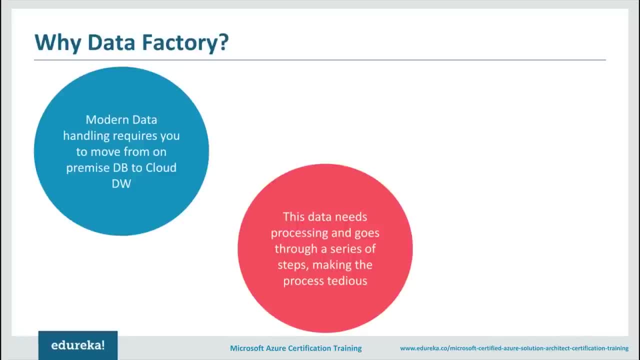 or get rid of all the things that is not needed Now. that is an after part or pre-processing part, But as far as moving this data is concerned, you need to make sure that you pick this data from different sources and bring it at one common place, then store it. 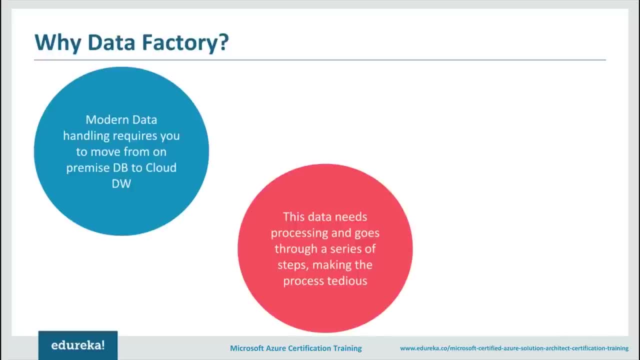 and, if required, you should be able to transform it into something more meaningful. Now, this is something that can be done by using traditional data warehouse as well, but then there are certain disadvantages. What happens is, at times, you are forced to go ahead and have custom applications. 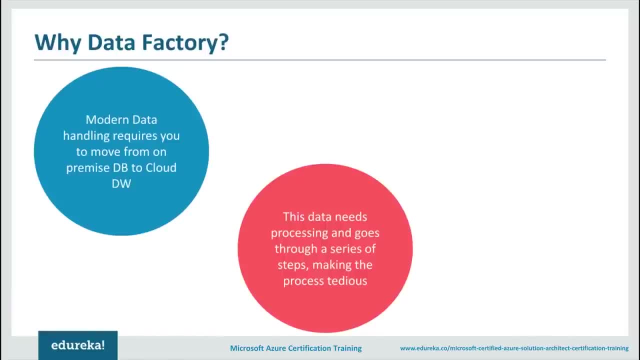 that deal with all these processes individually, and this can be time-consuming, and integrating all these sources can be a huge pain. Now, how do we solve this problem? Well, if there was a way to automate this process or create proper workflows, this burden would have been taken care of now. 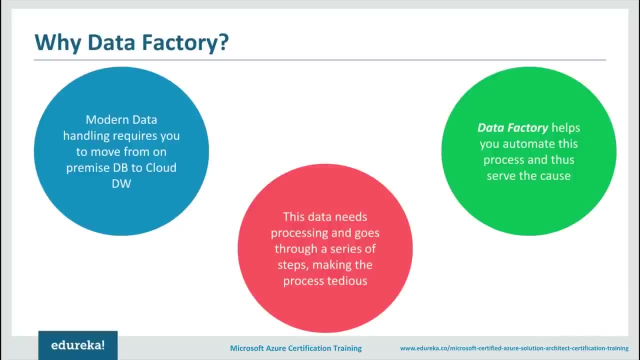 This is where data Factory steps in. what it does is it kind of helps you automate this complete process. instead of seeing automate, I would say it helps you orchestrate this process into more manageable or organizable manner. Now, that is something that is needed, and that is why we need something called as data Factory. 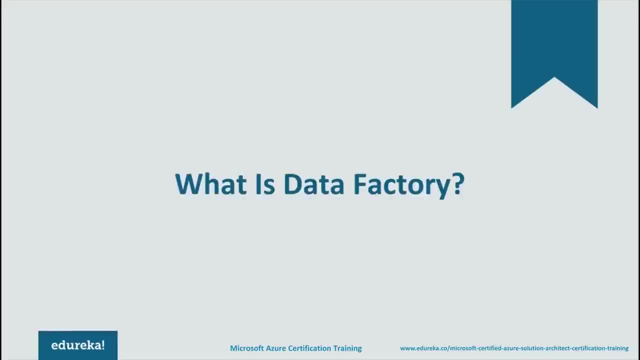 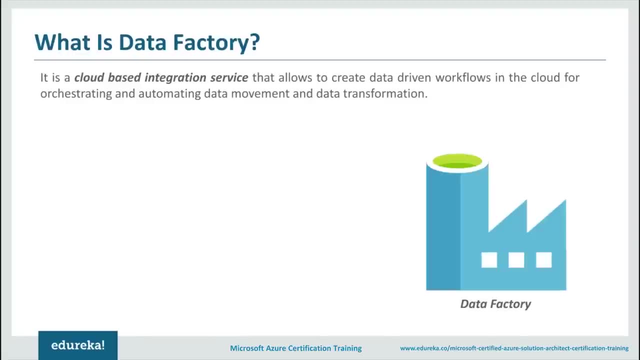 which lets you automate all these processes. Let us move further and try to understand exactly what data Factory is. So if I just go ahead and talk about its definition, I would say it is nothing but a cloud-based integration service which lets you do quite a few operations. 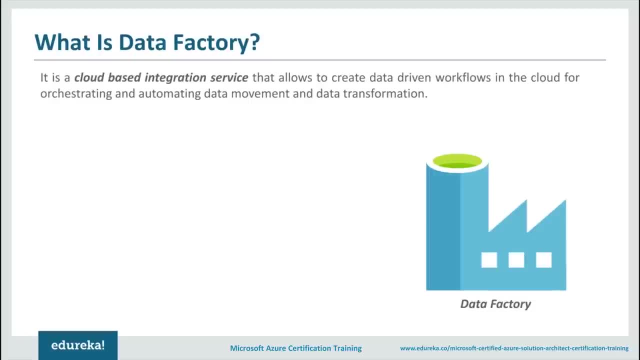 like create data-driven workflows, basically, and to go ahead and orchestrate all the sources that are there. But what exactly does it do? to name few common operations, what it does is it helps you create pipelines which are nothing, but you can think of it as a logical pipeline. 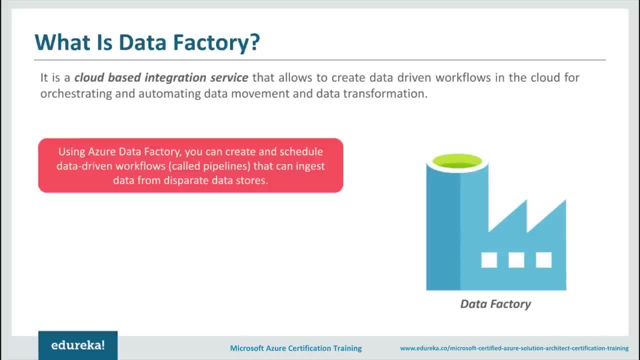 which supports various processes that happen. It lets you ingest data from different sources and then process it. when we are talking about processing it, It also helps you go ahead and do analytics, which is very important these days because we know that the amount of data that is being generated, it can be helpful. 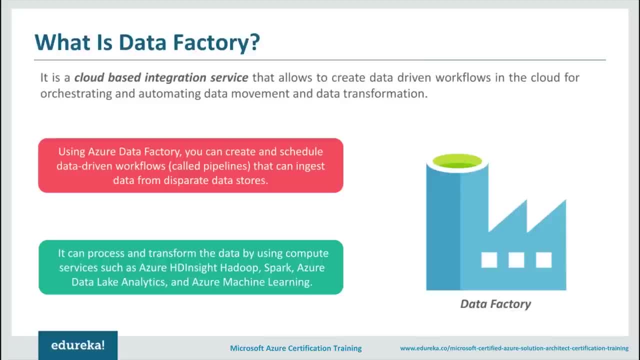 and it can help you take various good business decisions, And this is where analytics comes into picture. Now, what data Factory does is it lets you to transform this data and make it ready for something like data Lake, to use it. Now, data Lake is something. 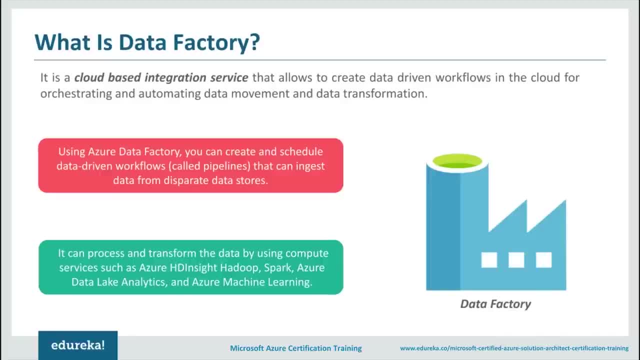 that lets you use various analytical tools or methods, like you have something called as Azure HD, insight, Maybe a Hadoop spa, Azure data like analytics and all these things. now, as we move further, I would be talking about these terms to some extent, but till then, you'll have to wait for now. 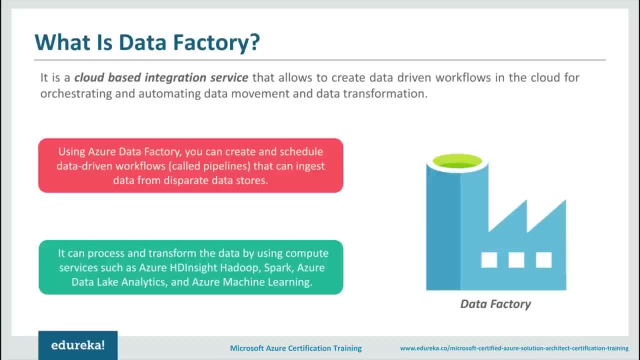 Just understand one thing: that these are nothing but platforms or tools which basically let you go ahead and do various analytical operations. So that is what data Factory lets you do. It lets you get in all the data, arrange it in a particular manner or order, and then supplied further for various processing. 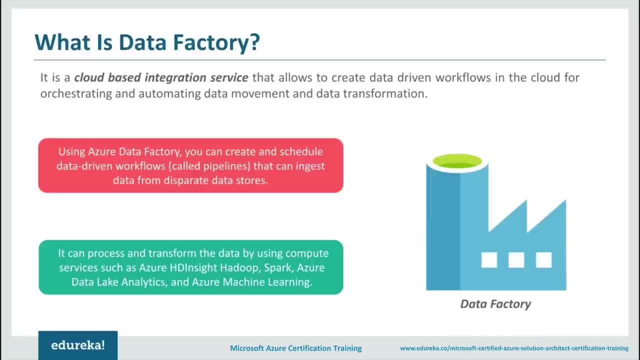 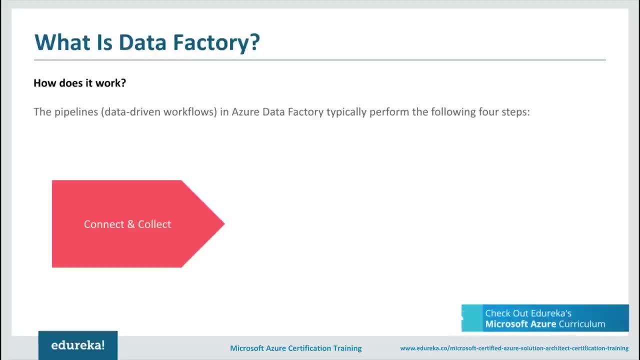 or various other things that can be done with that data. So, if you talk about particular steps, what does it do exactly? well, first and foremost, what it does is it helps you collect and connect data. Now, when I say connect, I'm talking about connecting. 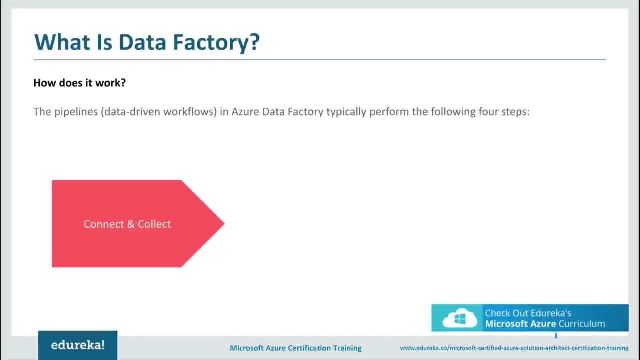 to various sources from which the data can come. now There are quite a few desperate sources from which the data can come. you can connect to all these resources by using your data Factory and then, once you have this data, you can collect it and store it at a central place. 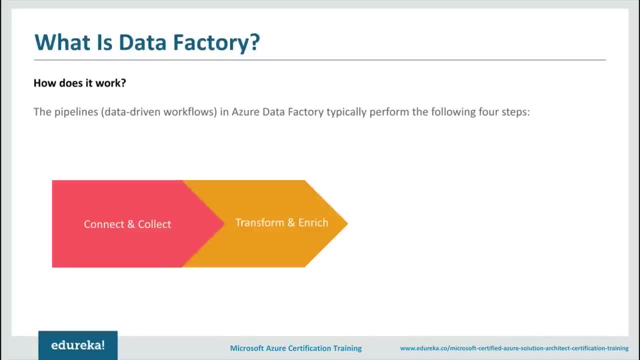 Say, for example, your data warehouse. then comes the process of transforming and enriching it. Now, when I say transforming it, I mean running various patterns on it, creating schemas and all those things. you can then actually go ahead and publish this data. Now, we all know. 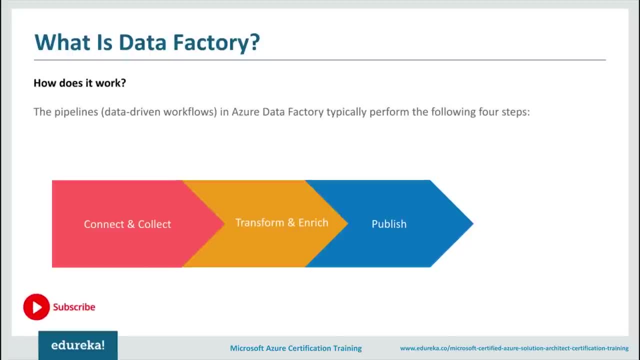 that Microsoft Azure supports various other tools as well. We have one more popular data visualization tool called as power bi, which is very good when you talk about data integration and various data visualization capabilities. what you can do is you can connect power bi to your Microsoft Azure. 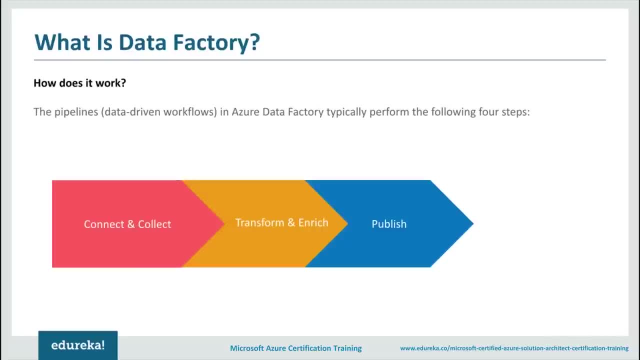 and publish this data, that is, create various dashboards and all those things. now, that can be very insightful when you talk about it from business intelligence perspective. So, yes, you can go ahead and do that as well, And then you can actually go ahead and monitor your data. 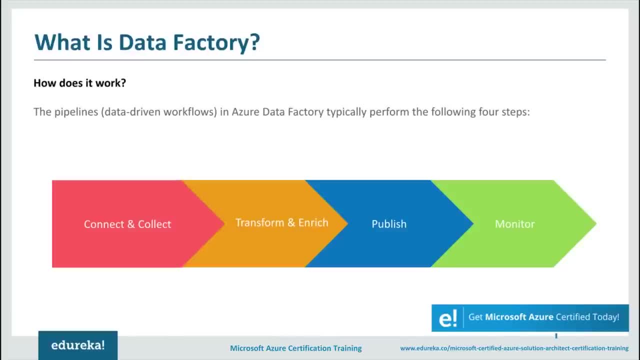 That means you can take a look at all the data that you have, and you can actually go ahead and analyze it in real time as well. So these are the processes which we are talking about. that is, connect and collect a data, transform and enrich it, publish it and monitor it. 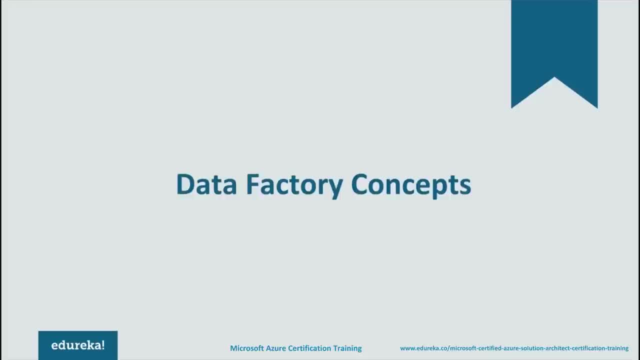 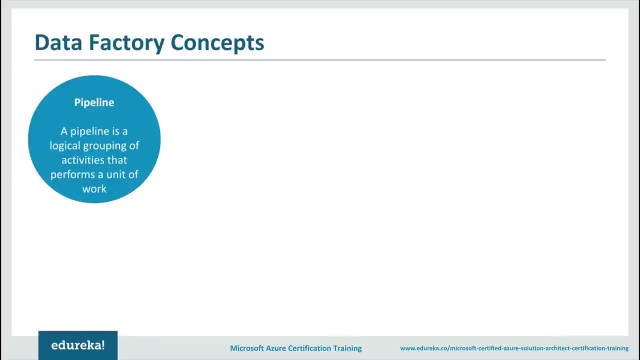 Now, that is what a data Factory lets you do. So what are the concepts that surround this particular term? So when we talk about data Factory Concepts, we have quite a few terms to discuss, like we have pipelines, data sets, activities and linked services. Let us try to understand these one by one first, 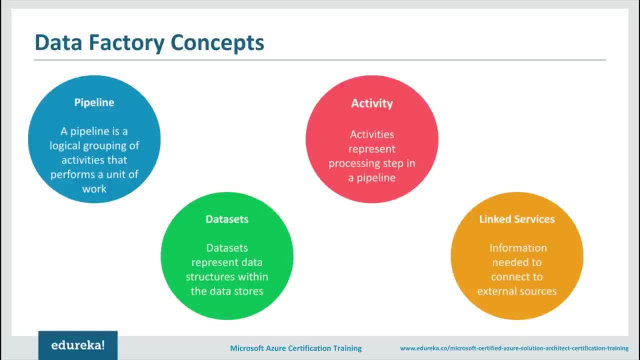 We will be talking about pipeline. now, pipeline is nothing, but think of it as a proper pipeline, That is, it is something which acts as a carrier, in which we have various processes taking place. Now, this individual process is nothing but an activity If you take a look at this side. 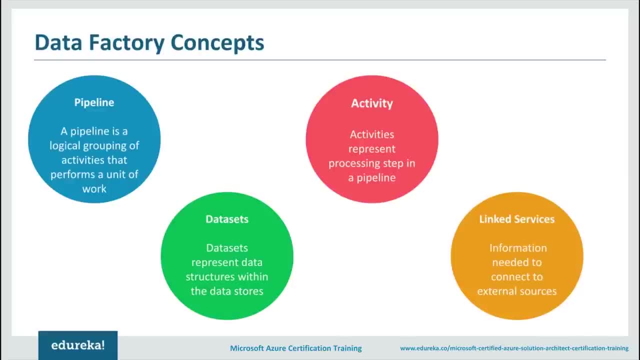 you would understand that activities represent processing step in a pipeline. That means your pipeline can have one or multiple activities. Now, when you talk about this activity, it can be anything. it can be a single process, like querying a particular data set, or it can be something like moving data. 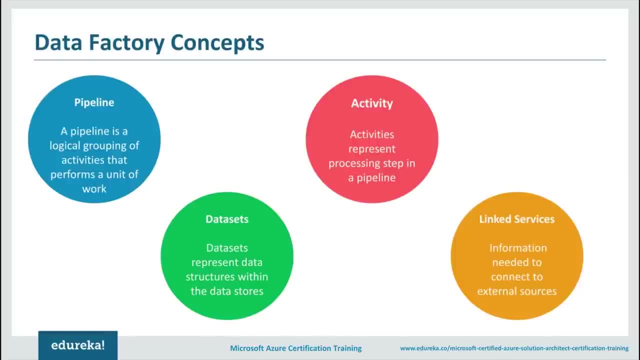 from one source to the other, then you have something called as data sets. now, data sets are nothing but sources of data. Say, for example, my data is stored at an end location and that end location is nothing but my data set. So in simple words, 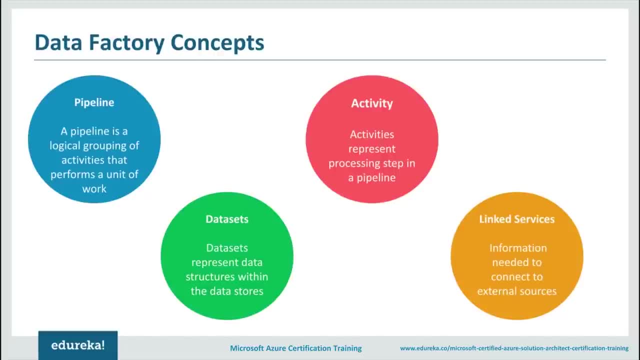 it is nothing but a data structure that holds my data Linked Services. now, this is nothing but a law. say, for example, I need to move my data from a particular database to a blob storage. They need to be something that connects these two things. 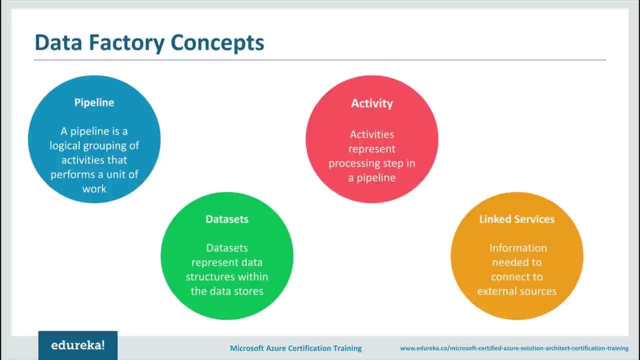 that is a law or some information that lets a database understand that it has to move the data to a particular data source. So that is what a linked service is. It is nothing but an information that tells your data factory that is, you need to connect to these particular sources. 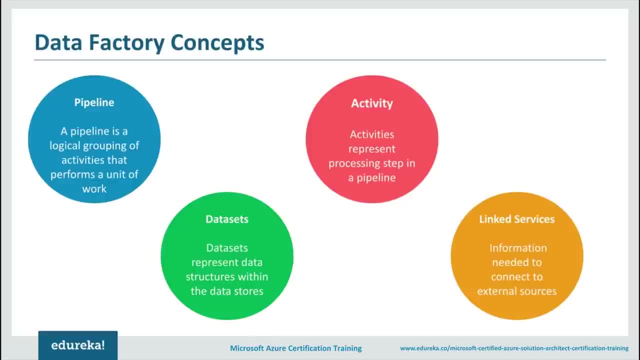 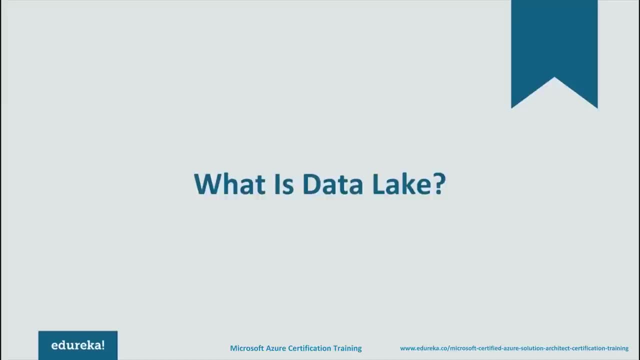 So these are some of the concepts that form a central part When you talk about a data factory Now. next, we are going to talk about something called as data links. Now, this is something that we won't be seeing in the demo part. 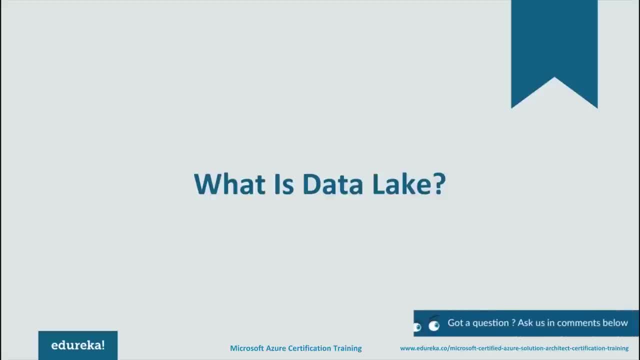 but it is important when we talk about data warehousing and I feel that when I move further or I create more sessions or videos as far as this topic is concerned, I would be talking about analytics and quite a few other terms as well, So this is a particular term. 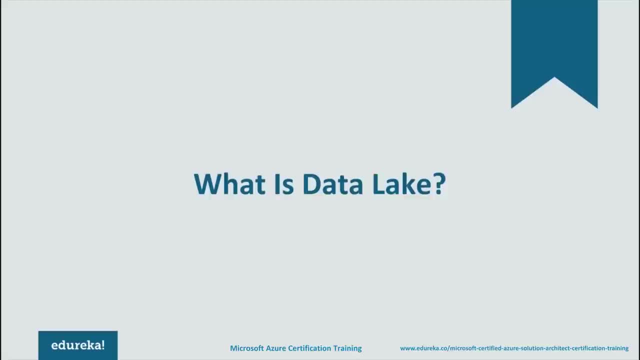 which is reserved for those sessions and videos. But for now, I would be giving you You an overview of this topic as well, because I feel that it is important. when we talk about data warehousing, we need to understand what data Lake is, first of all. 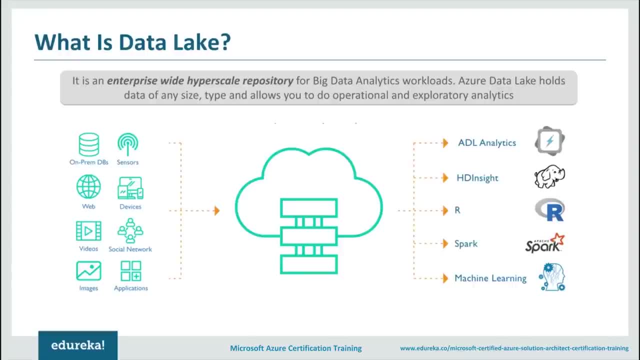 let's start by understanding what it is exactly now. Think of it as a container or basically a store. is that holds data? Yes, we already have databases. We have so many things. So how is your Azure data Lake different? Well, think of it as a hyperscale repository. 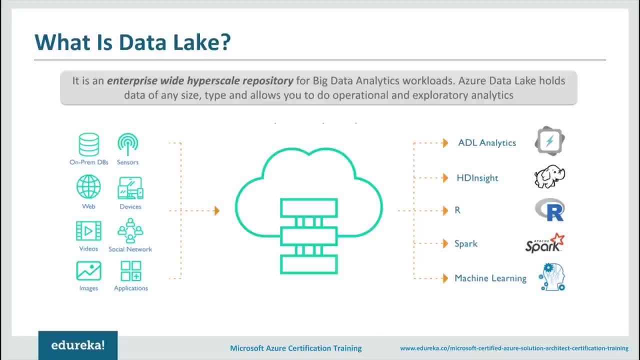 which lets you do quite a few other things. as I've already mentioned, analytics is something that is very important. now, when we talk about user mode of data, there quite a few things which you can do with it. You can use various analytical tools, to name of you. 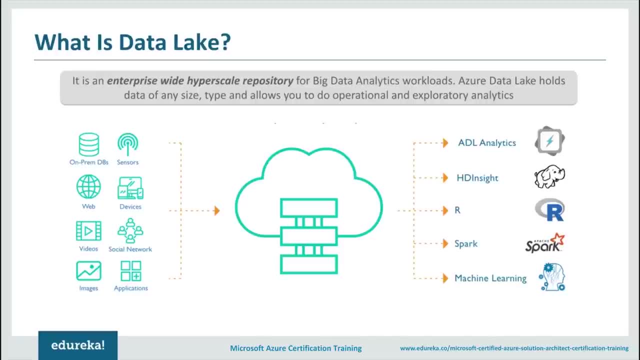 We have some here. We have our Azure data Lake analytics, We have HD. insights are spark and machine learning. Now, These are some of the commonly used and very popular tools which are there. what Azure data Lake does is it supports all these tools. 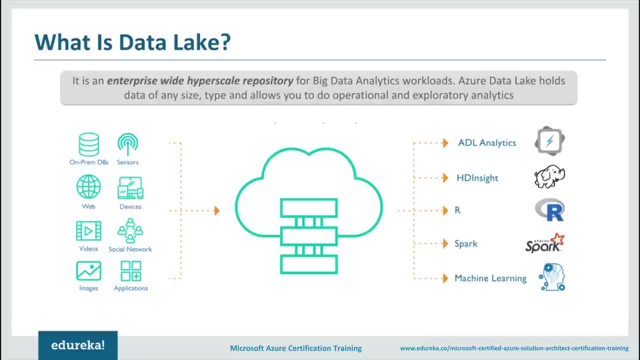 That means you can store data from any source and in any form at your Azure data Lake and then you can use these tools and terms to actually analyze this data. So that is two-in-one kind of an operation. In fact, it is multiple in one kind of an option. 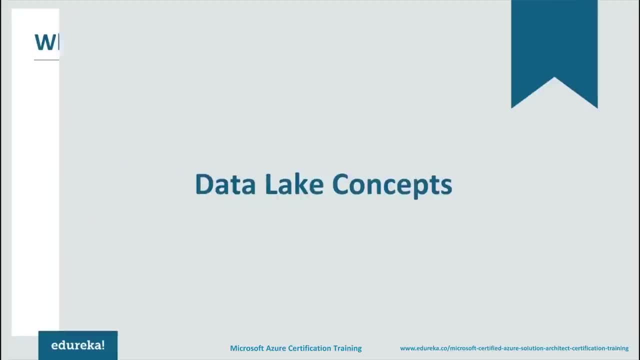 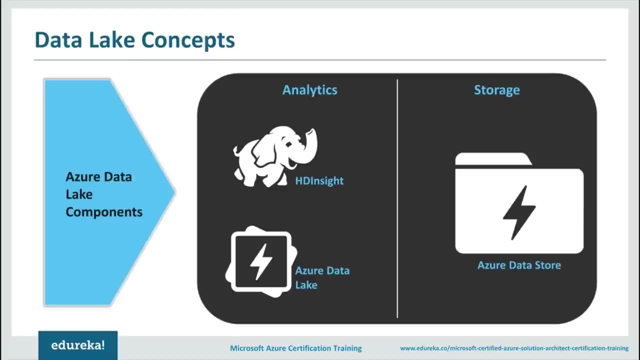 but basically because it lets you do so many other things. So what are some of the concepts that one should know? first, Let us try to understand some of the components. when we talk about this particular term, that is, your Azure data Lake, basically it forms of two parts. 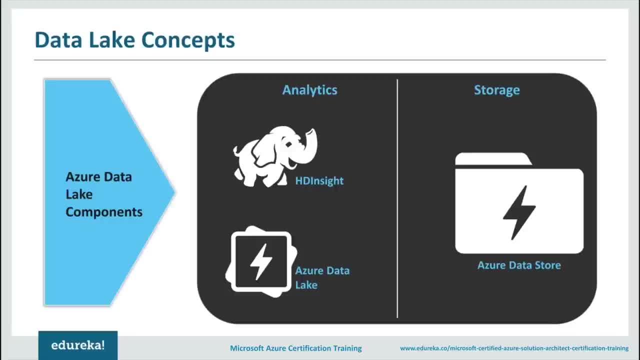 One is your analytical part and the other one is your storage part. I'm going to talk about the storage part. The best thing about your Azure data Lake is it does not have any particular schema. That means data from any form can be stored into this particular source. 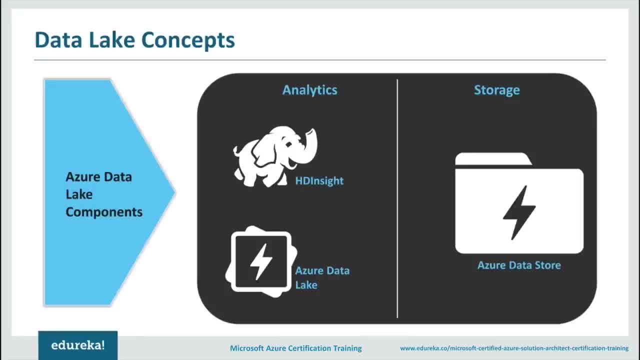 That is, it can come from different sources and it can come in different forms as well. And then you have something called as your analytics part, where you have something called as SD insight. It lets you form those Hadoop clusters. Now I won't get into the details of what a Hadoop cluster is. 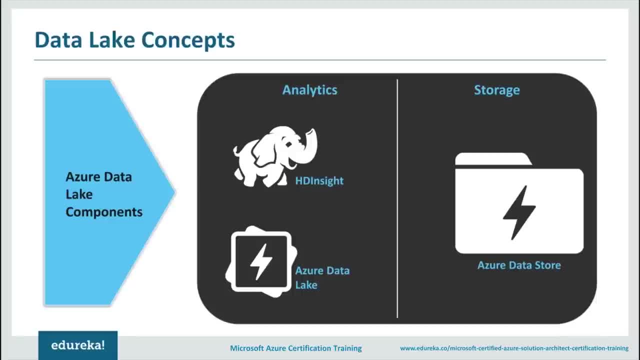 but it is a process or a way by which you can actually analyze data. So, yes, you can actually go ahead and create those Hadoop clusters, take that data in and then process it as well. You can also go ahead and use Azure data Lake Azure data. 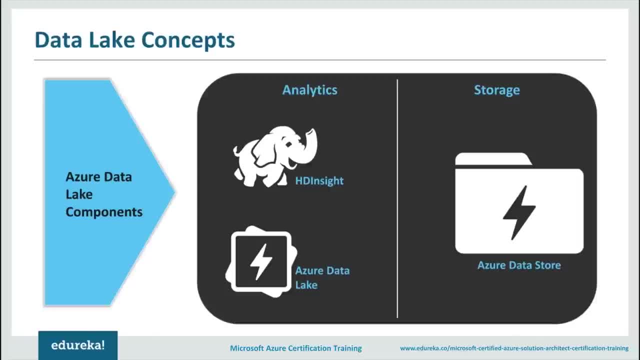 Like analytics, is something that is again used for various machine learning and other analytical process as well. So these are the two things which your analytics part will have, and apart from that you have something called as Apache spark, which is nothing but a fast computation processing thing. 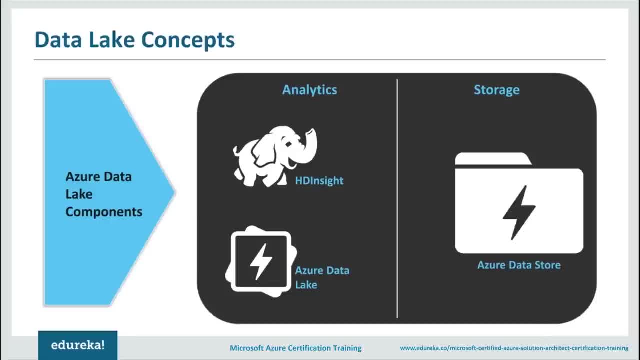 That is something that lets you process data parallelly and in huge amounts as well. So these are some of the basic concepts when we talk about your Azure data Lake, and how does it actually go ahead and process the data? Well, let's see that as well. 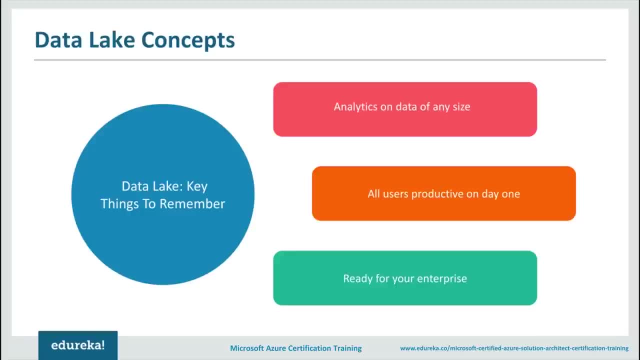 but there are certain key points which you need to understand when we talk about Azure data. Like, the first thing it does is it lets you store data in any size and of any kind, which is very important because what this does is it kind of takes away the barrier. 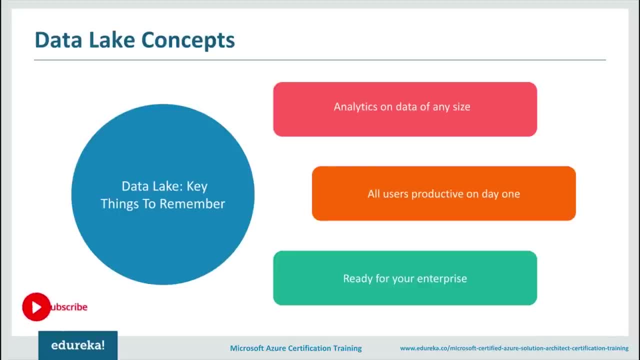 where people had to wait to go ahead and process that data. They had to take this data first, clean it, arrange it, organize it and then put it somewhere from where they could actually go ahead and use it. Now this is something you do not have to worry about here. 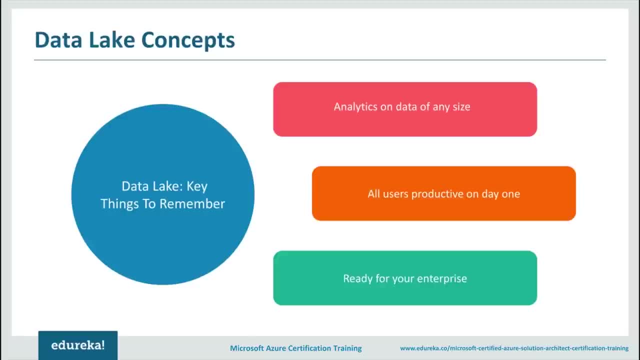 Why? because you can just go ahead and dump your data in your data Lake and then actually take a particular schema, pick that data and then start processing it. So it helps you save time and it lets you store data of any kind in any size. Now the second point is: all users productive on day one? 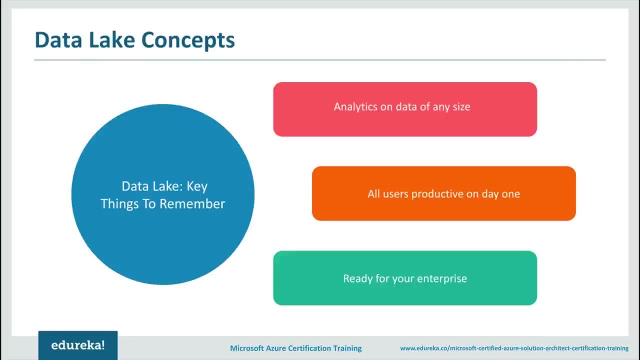 That is what I mean. That is, since the data of any type can be stored here, You're not restricted. You can just start working on it from the very first day, and it is ready for any kind of Enterprise. That means there is no restriction on what kind of tool. 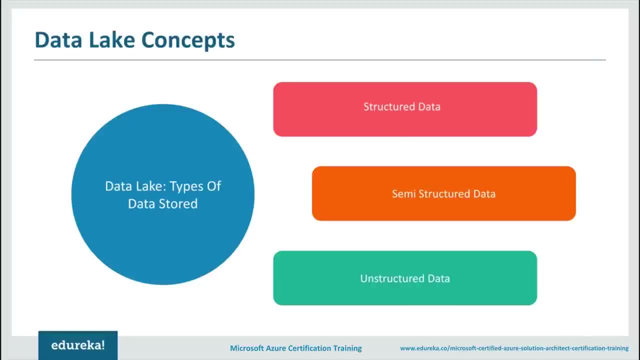 do you want to use and what kind of business problem are you dealing with? So what are the types of data that your data Lake stores? first and foremost, what it does is it stores structured data, semi-structured data and unstructured data. That means all the types of data that can possibly be there. 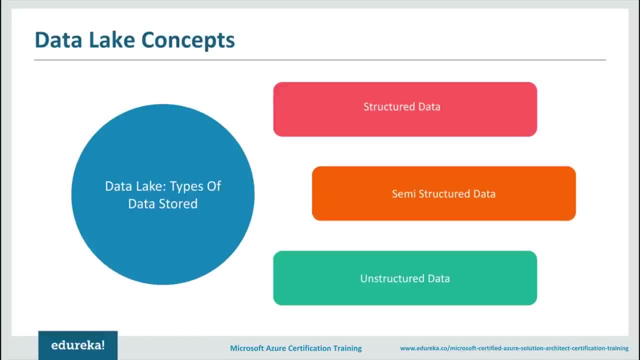 as far as storing is concerned, Everything is taken care of. now, when I talk about structured data, I'm talking about data that has a particular schema. then you have something called as your semi-structured data. Now, this is nothing but your JSON files. 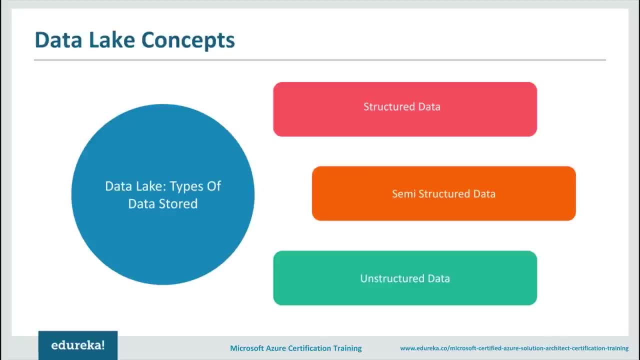 or maybe your XML data. even that kind of data can be handled. and when I'm talking about particular unstructured data, that is, data which can be in text files and has no schema or no pattern whatsoever, Even that kind of data can also be stored by your data Lake. 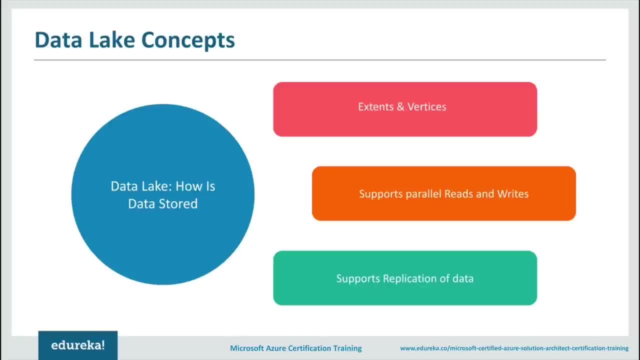 Now let us try to understand. how does it actually store data? If you all know how Hadoop stores data, this would be quite easy to understand. now We all know that what Hadoop does is: it takes our data, It divides it into chunks and then processes it parallelly. 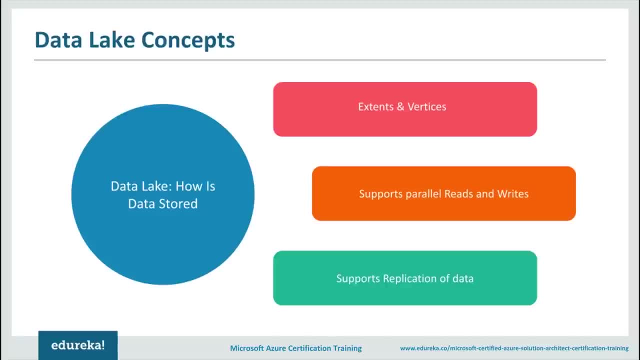 Now, this is what your data Lake also does. say, for example: you have a particular file which has some amount of data. now, as soon as the size of the data goes about 2 GB, It breaks this data into two chunks. say, for example: 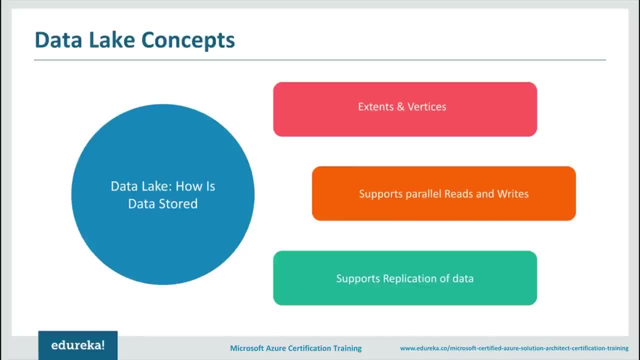 I have maybe 10 GB of data, So it would break my data into five chunks of 2 GB each and then it would replicate this data. That means three copies of this data would be made and it would be stored at three different locations or at same location as per the values or rules. the user asset. 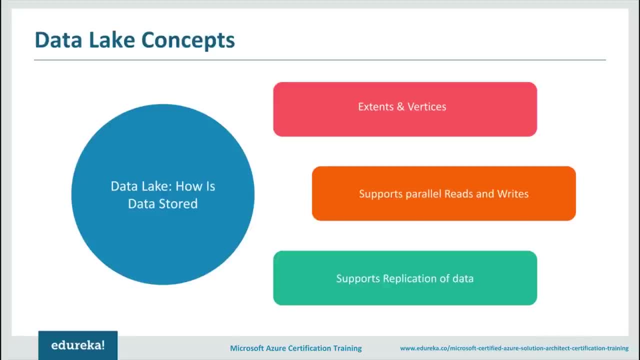 So when you store this data and replicate it at three different locations, what happens is, even if your data goes down at one place, it is still available at the other place to use it or to recover it. rather, now, when you talk about Particular data storage method, you can read something called 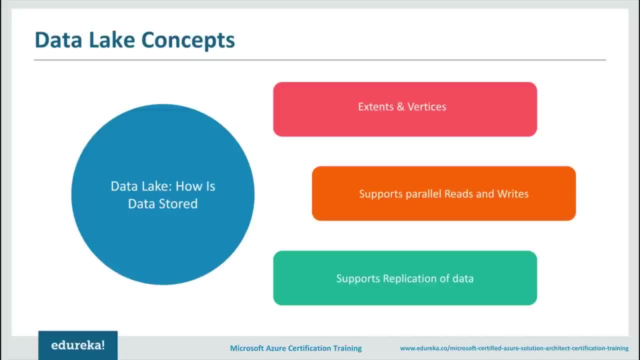 as extents in the slide. now, extents are nothing but these chunks, those two GB chunks which are there, and when you process this data using something called, as you, SQL, which is a language that your data Lake uses, it actually goes ahead and Maps various vertices, which lets you keep track of all this data that is there. 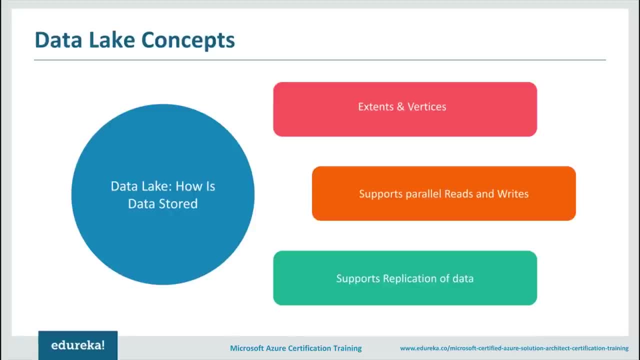 So, yeah, these are the terms, that is, extent and vertices. Now what happens here is, since you are replicating this data and you adding it into chunks, you can actually go ahead and process this data parallelly, Saving a lot of time and giving you high computation. 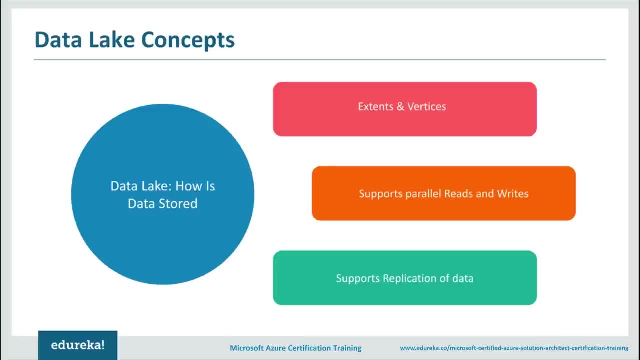 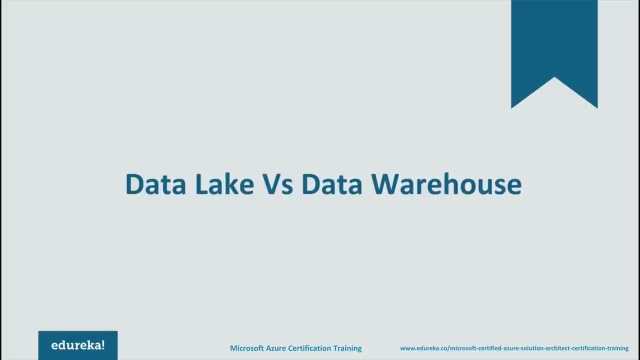 It also supports replication of data. This is something that I've already discussed, So I would just move further and try to talk about other concepts as well. Next, we are going to understand what the data Lake is and what the data Warehouse is now. 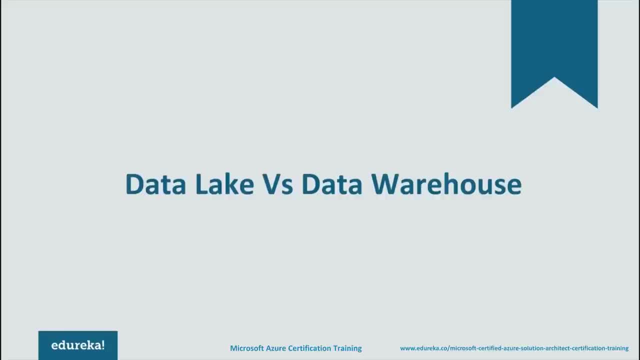 Why did I bring this topic up? Well, data Warehouse is something that is a traditional approach towards storing data, and it is still used widely. but then why do we need data Lake and why am I comparing these two terms? will quite a few people confuse these two terms? 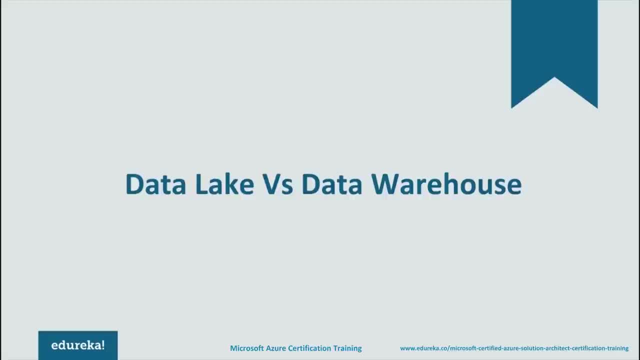 as in. what is the difference between them exactly? Well, they're quite similar to each other, but there are slight differences which are important, and I felt that we should have gone out and discuss those. That is why I put this slide here, So let's try to understand that as well. 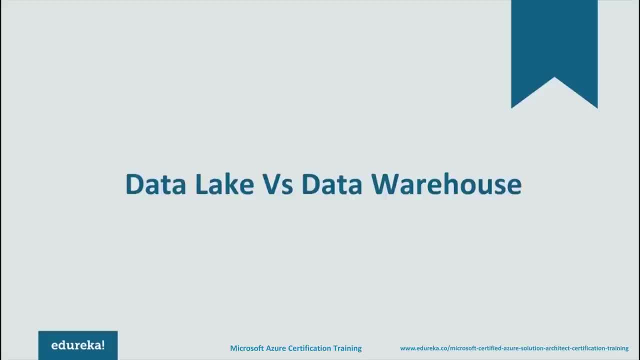 Well, this is a clear differentiation between these two things. not as. first of all, you need to understand that your data Lake is nothing but something that is complementary to data Warehouse. That means, if you have your data at a data Lake that can be stored. 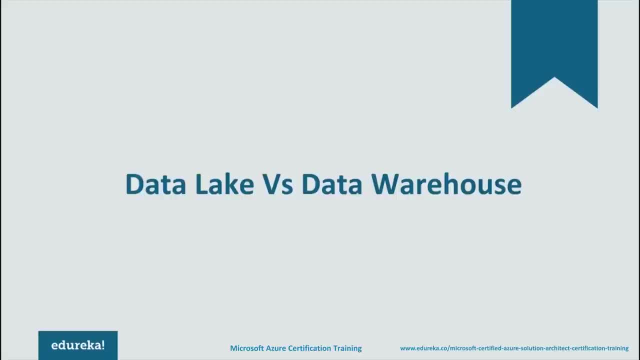 at data Warehouse as well, but there are certain rules that need to be followed. Now, when you talk about your data Warehouse, what happens is you can use again your data Lake to bring in data, But the main difference is when you talk about a data Lake. 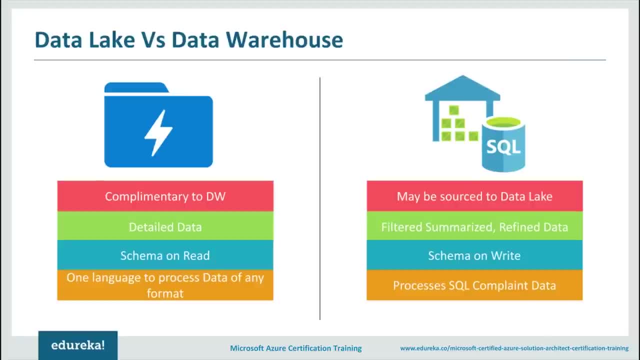 the data is detailed data or raw data. That means it can be in any particular form. You just need to take the data and dump it into your data Lake. That is not the case with your data Warehouse. here The data is filtered, summarized, refined. 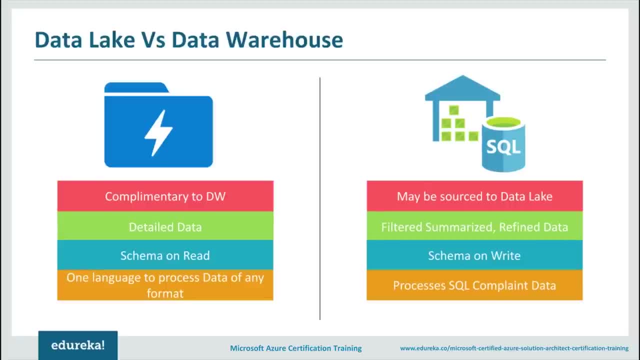 Now you might wonder that, okay, if everything is happening here at your data Warehouse, isn't it better in some situations? Yes, definitely It is better. But as I've already mentioned so many times in this video, the amount of data that is generated these days is huge. 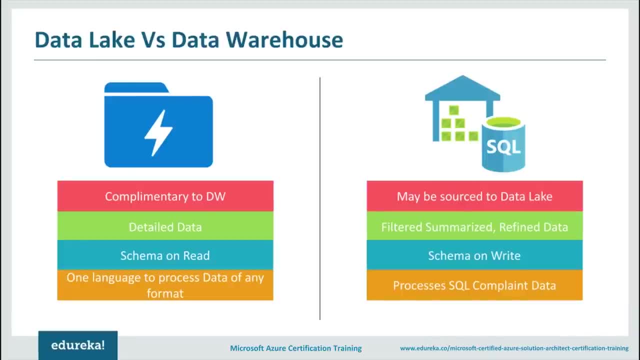 and it can come from any particular source. This might not be the best of options to deal with, why? well, your data Lake has something called as schema on read and your data Warehouse has a schema on right, kind of an approach. what this does is, if I talk about it, 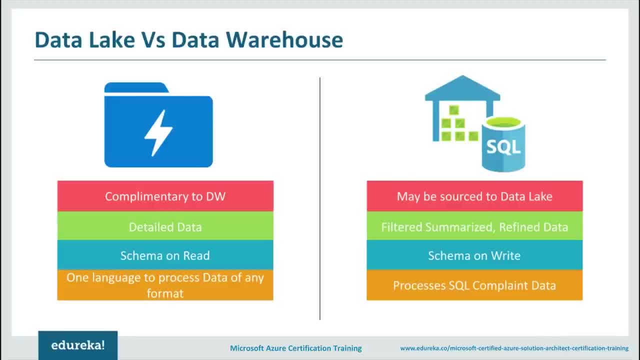 from a data Warehouse perspective where you have schema on right. That means when you're writing your data to your data Warehouse, it is written in a structured form or in a particular schema. So when I'm reading this data, I have to read it in that schema only. 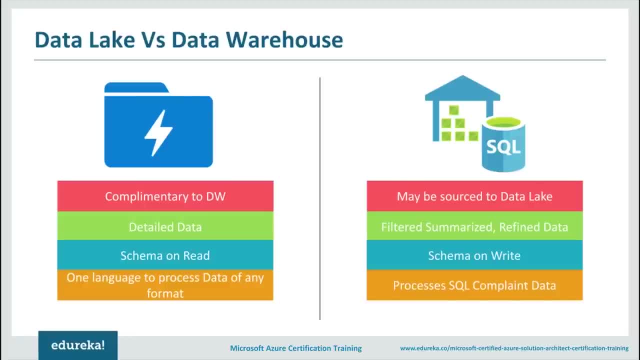 but when you talk about a data Lake here, you just dump your data. It is not structured. So when you are using this data, you are free to go ahead and define your schema in a number of ways as it suits your needs. So this is where the benefit lies, in that is, your data does not. 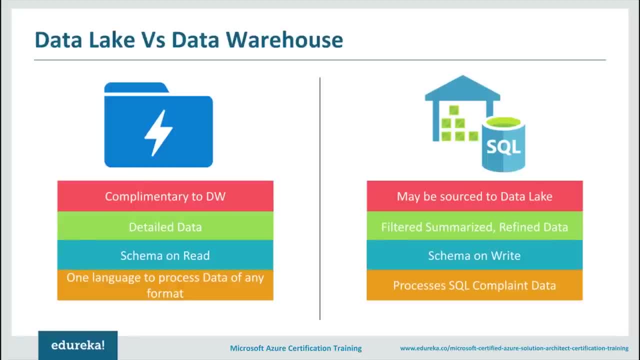 follow a particular schema. You can just go ahead and pick a schema for it. So that is a plus point again. one more point: your data Warehouse. Basically it works in SQL, That is, it uses SQL to choir or question your data. But when you talk about your data Lake, no matter the data comes. 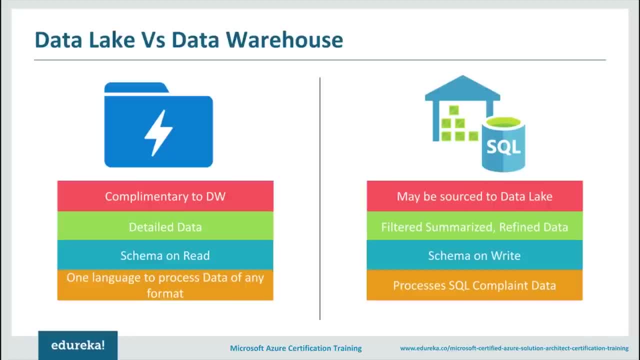 from different sources. it can be quiet by using one single language. That is your usql, and again, that actually helps you reduce various barriers because you're talking about different data sources, but still something that lets you access the data is one single programming language. 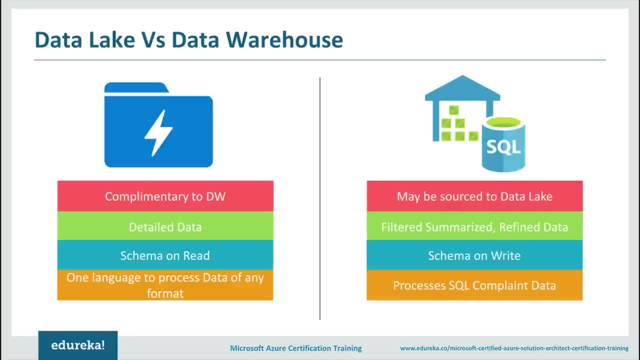 So these are some of the concepts I felt that you all should know. that is what a data Factory is and what a data Lake is. again, The reason I talked about data Lake was it is an important part when you talk about data warehousing and data integration. 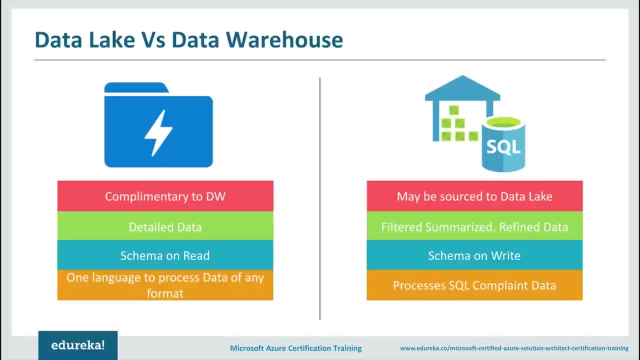 because all these topics would form a base when you talk about analytics and processing data, and that is why I wanted you all to know all these terminologies. now, since we started our session talking about data Factory, let us move back to data Factory and try to visualize all the concepts that we talked about. 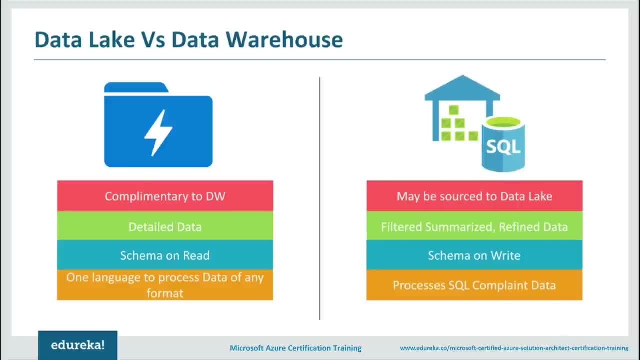 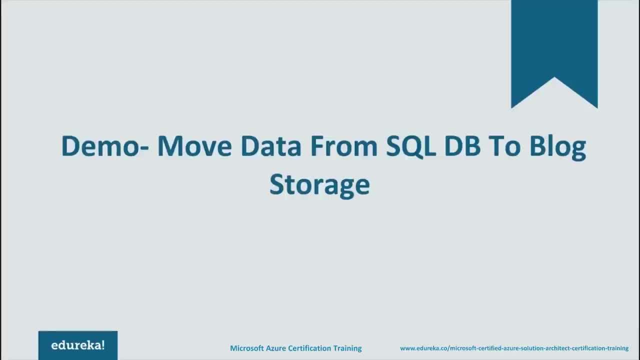 because I talked about something called as pipelines, activities and all those things. So what I'm going to do now is I'm going to go ahead and give you a demo where I'm going to actually go ahead and create a database, probably load a table in it. 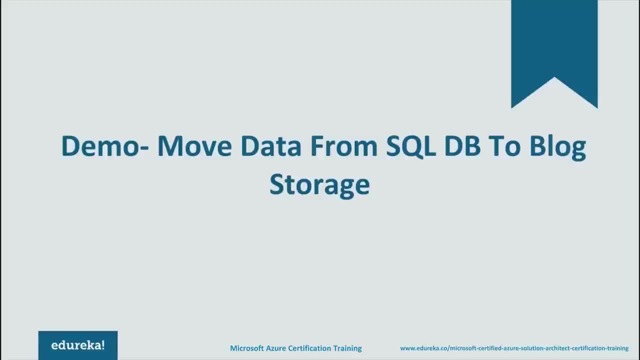 and then move that data from that particular source to a blob storage using a data Factory. So, yes, this might be a lengthy demo, but I'm sure that you all would like it and have something new to learn out of it. So let me quickly switch to my Azure. 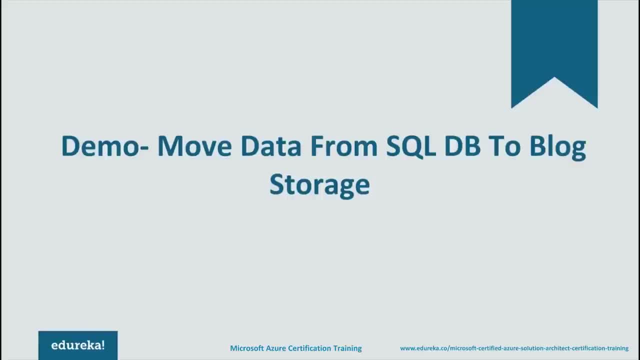 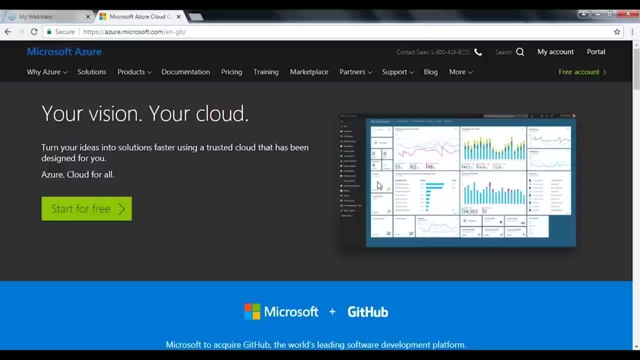 and we can actually go ahead and see how it works. Okay, So there you go. What I have done is I've gone ahead and I have blocked into my so-called Microsoft Azure portal. for people who are completely new to this term, That is Microsoft Azure. 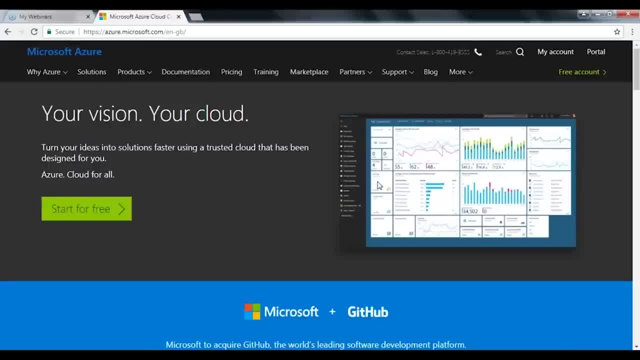 What you should do is you should go ahead and take a look at other videos, if possible. I've created quite a few videos in the series, and those videos talk about various concepts. as far as Microsoft Azure goes, there are certain basics as in how should you use it. 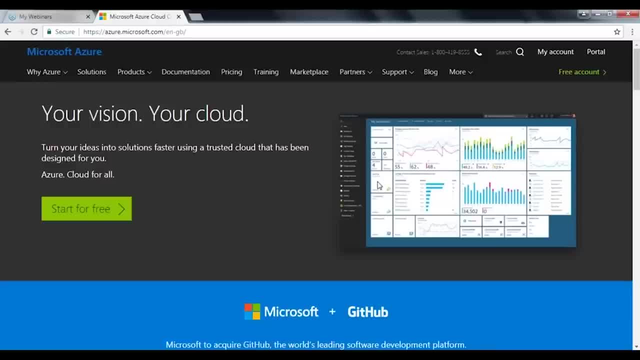 and what are the things that you need to do? One of the things that is there is creating a free account, which is very important. Now we are going to go ahead and use our free account for our subscribed account. What Microsoft Azure does is it lets you have a free account. 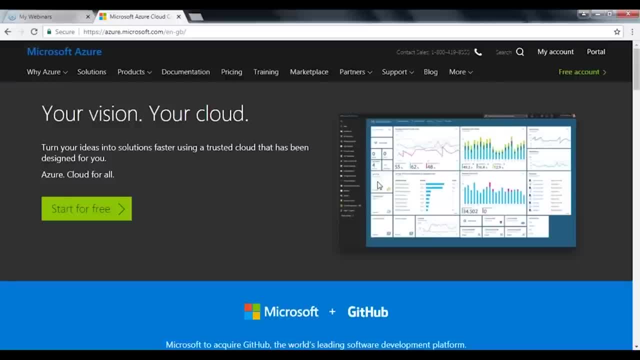 You need to just register for it and quite a few resources would be made available to you, and some credit is also given to you which you can use. that is, you would be charged for these resources, But since you are given certain credit, you can use that. 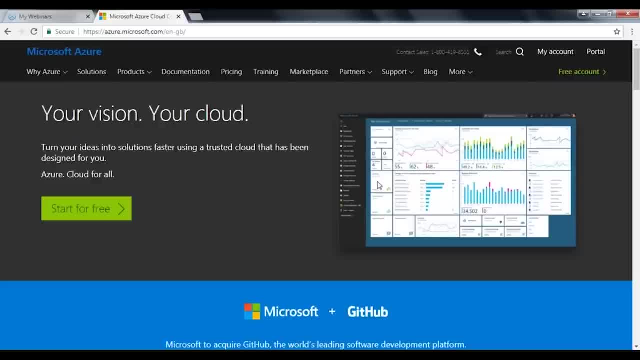 and that means the services are freely available to you. If you already have an account, then that is not a problem. We are just going to go ahead and take a look at the demo part. as far as this demo goes, what I'm going to do is I'm going 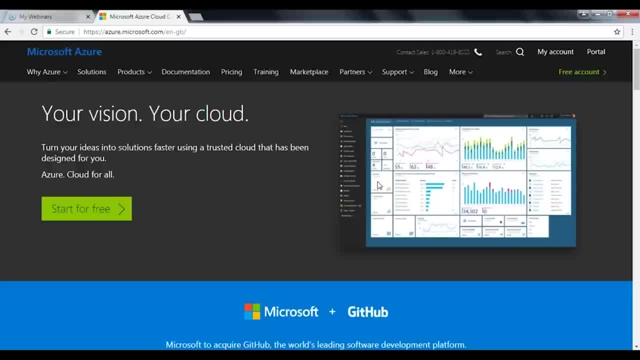 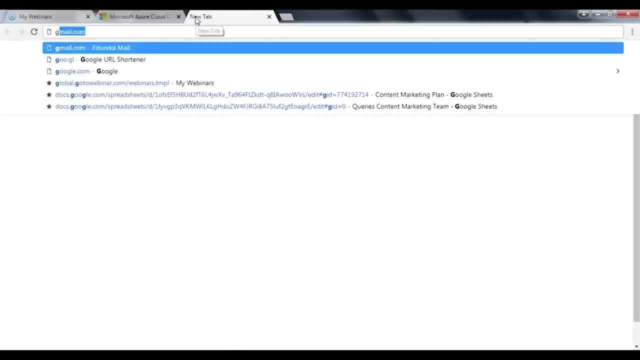 to go ahead and create a database. for that. I need something called SSMS. let us go ahead and try to understand what that is first. But if you do not have that thing, you need to go ahead and install it. So how do you do that? 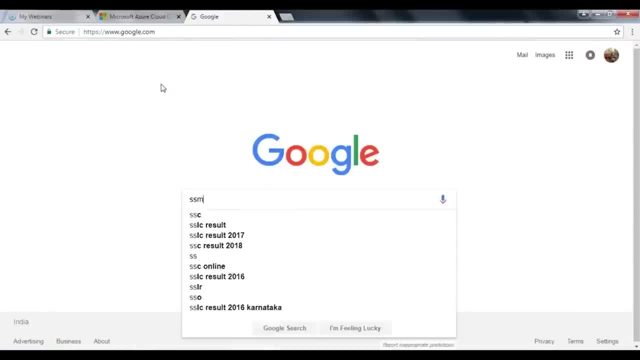 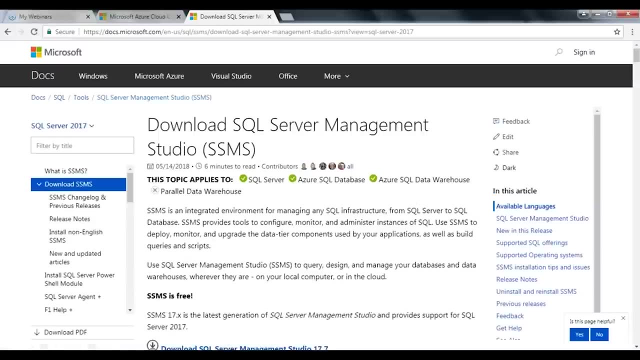 Just go to Google, basically, and type SSMS. This is the first link that you get and you open it. You have your SQL Server Management Studio. Now, this is something that we would be needing. you just come here and you click on it and it would start the setup download. 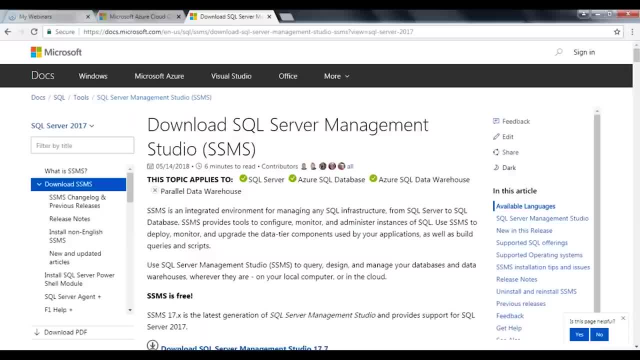 I guess it's getting downloaded twice. I don't need that. I've actually gone ahead and I've installed that thing on my system. I'm doing this for you people. What you need to do is you need to download this particular file. 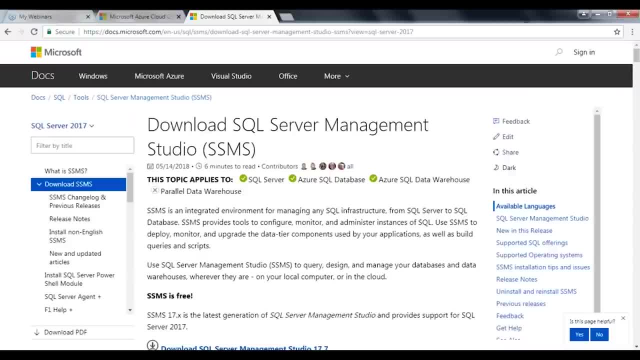 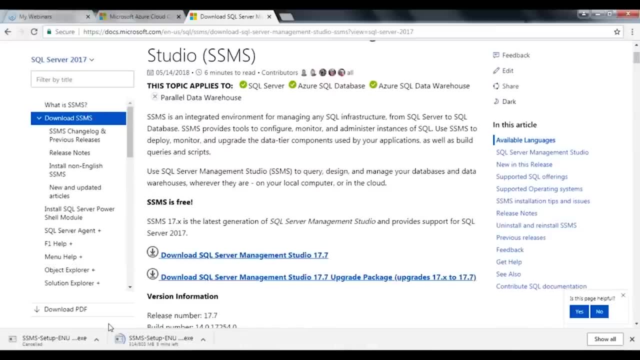 Now, as you can see, it is somewhere on 800 MBS. that is approximately equal to 1 GB. So you need to download that file And once you do go ahead and download that file, you need to install it in your system. The installation can be a lengthy process. 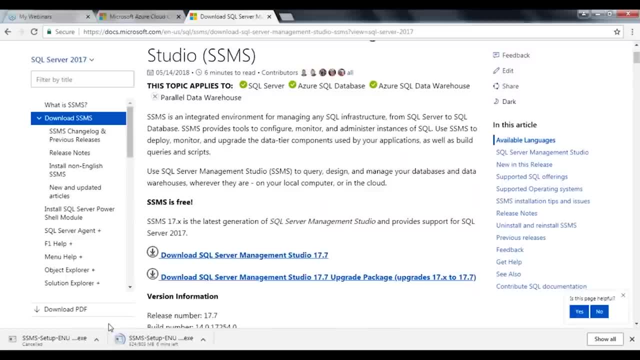 Now, when I say lengthy process, it can be time-consuming. It is not difficult to do. All you need to do is open this file and double click on it. It would give you an option to install it and just say yes. Once you do that, it takes care of all the processes. 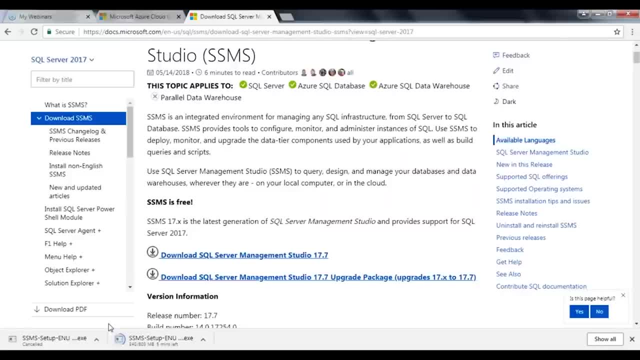 and once you do, go ahead and install that thing now. this is something that would help you have your own server and that is on your local device, basically. So this is something that we would be using in the later part, But what I would suggest is you come to this website. 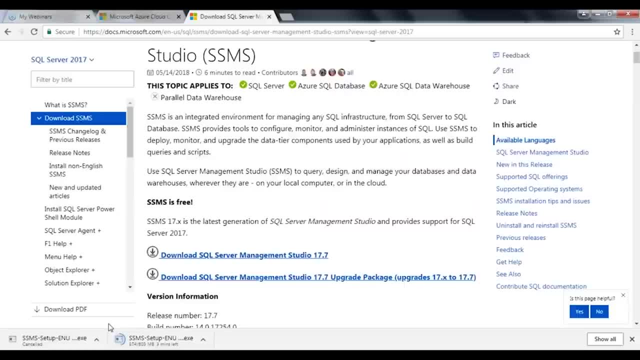 and download this particular thing. if you do not have it, and once you download it, I would suggest that you go ahead and install it as quickly as possible. again, Let me tell you, it might take some 10 to 15 minutes, depending on the processor you have and the internet speed that you have. 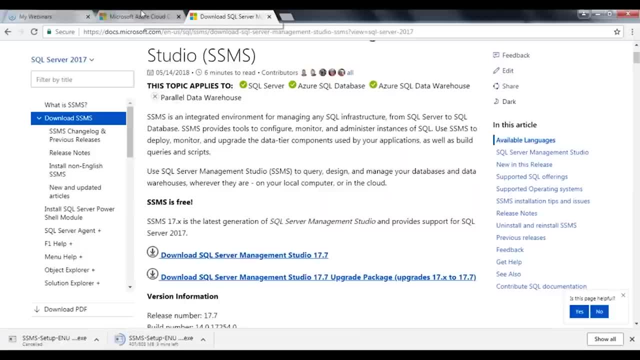 So yeah, once you're done with this, then what we do is we again switch back to our Microsoft Azure account. Now, what I'm going to do is I'm going to go ahead and create a database here. So how do we do that? 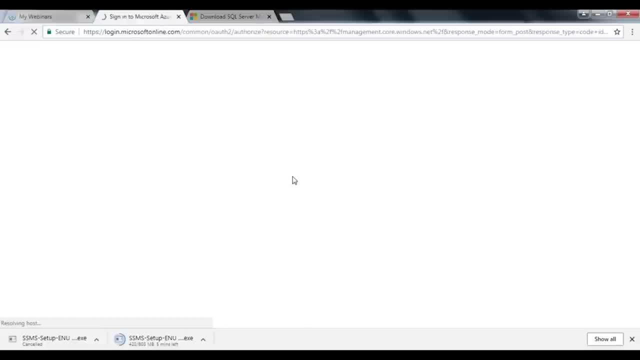 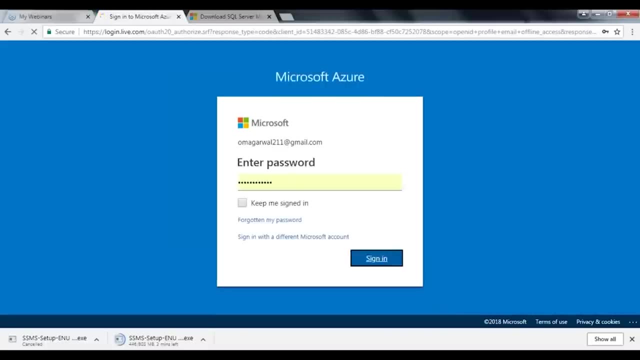 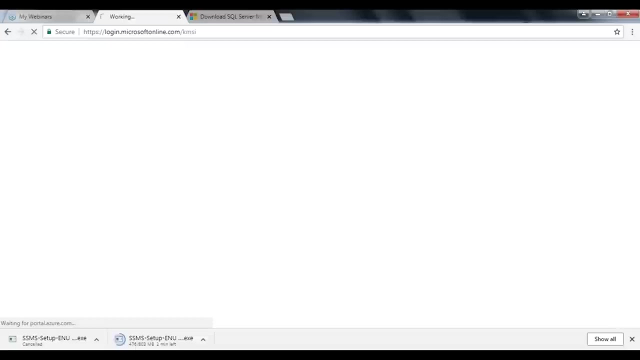 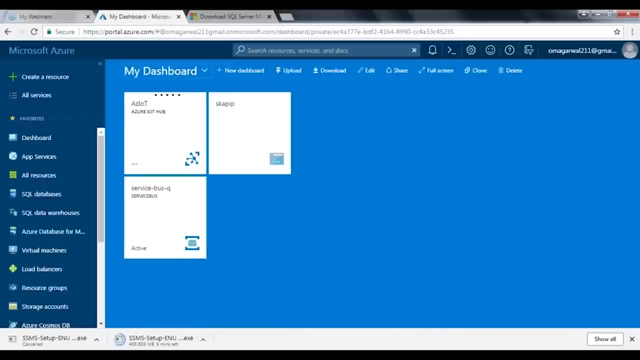 Well, you go to your portal, basically, And quickly log into your so-called account. My internet is fairly slow today, So, yep, it might take some time. So this is how your Microsoft portal looks like. you have quite a few things to select and choose from. you can just go. 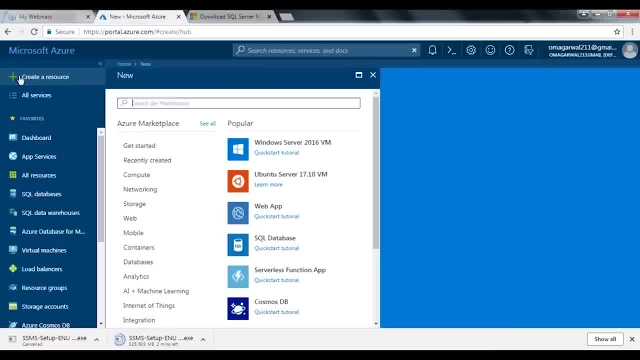 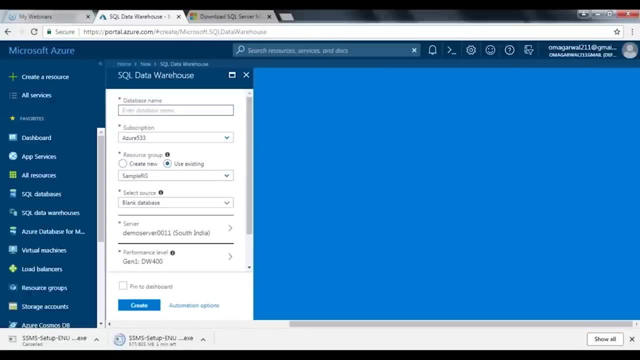 ahead and click on create a resource here and it gives you quite a few options to select from or instead. what you can do is you can just come here and look for your so-called databases and I select an SQL data warehouse. So it would ask for a database name. give it a proper name, say demo. 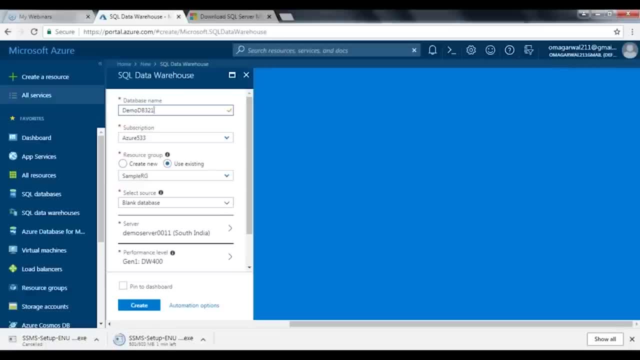 DB is what I would call it And, yes, the name is acceptable. My subscription is Azure 533.. I would be needing to create a resource group. for people who do not know what a resource group is, It is nothing but think of it as a place. 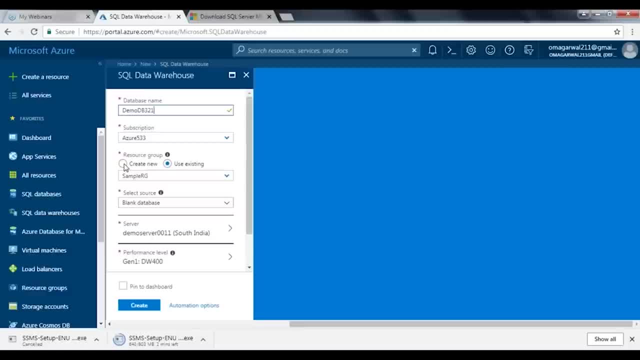 where you put in all your resources basically. So it is a group of resources Again. if you need to understand more about it, we do have a session on it which you can take a look at it on YouTube. So I say, create a new one, say I call it demo RG. 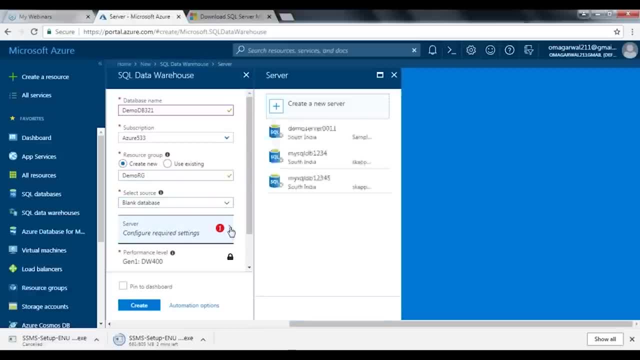 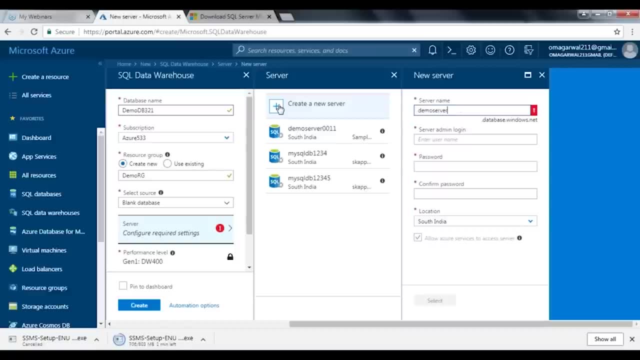 and let me just pick a blank database. I need to configure a server to it. So I would say: create a new one. Let's name it, say demo server, and I should give it some numbers. probably, yes, it is acceptable, and you need to create some login credentials. 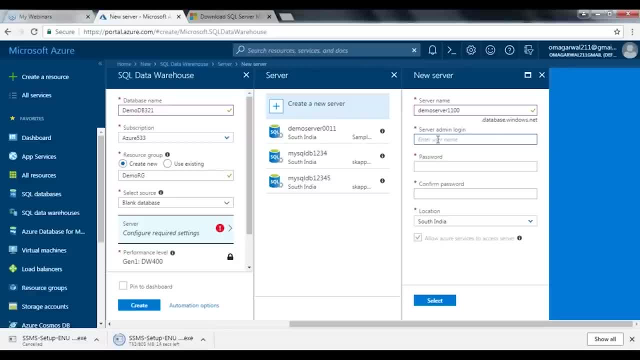 when you do log into the server. So let those credentials be, say, admin demo. Maybe there you go. And what password should I set? let it be strong and let it have a number and symbol. basically, Location: South India. that does not matter a lot. 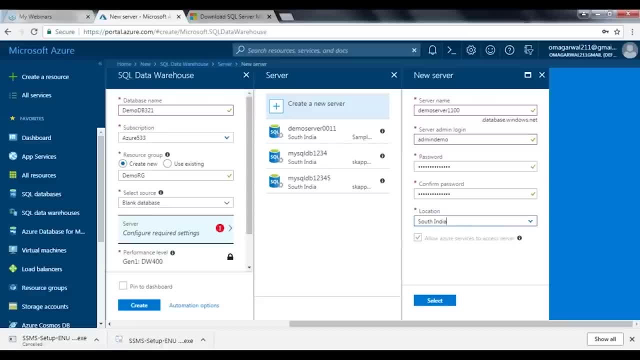 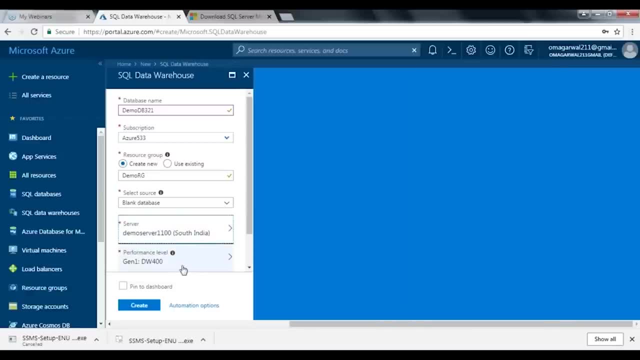 You can choose the location that is there in here. You have quite a few options. There you go. I would stick to what it is there and I would say select: Yes. so I have a demo server as well. performance level now it depends as per your need, as in how fast do you want it to work. 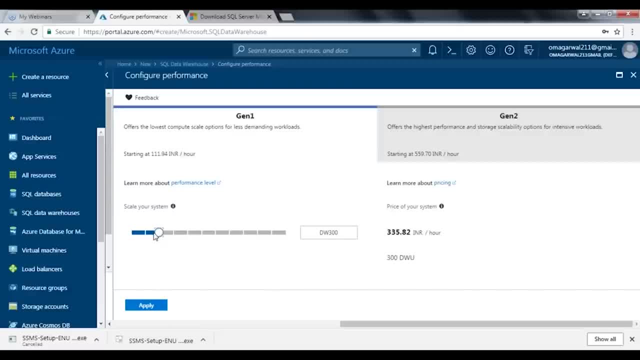 now, as far as my so-called demo is concerned, I do not need it to be very fast or something like that. Let me have it to this value now, based on the location where you've created your so-called resource, the prices would be given to you. 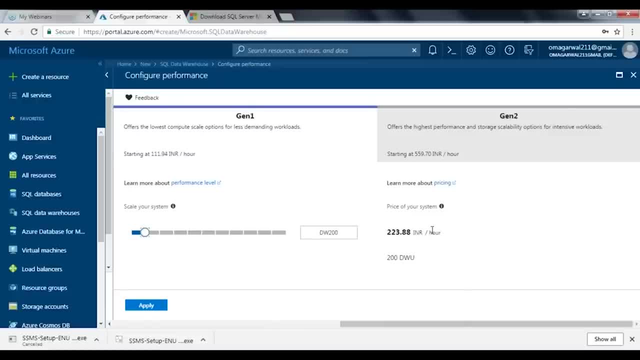 Now, This is something that I created in South India, So the price to me is an INR, that is, Indian rupees, and it is two to three Point eight, eight per hour. All I would do is I'll just go ahead and apply. 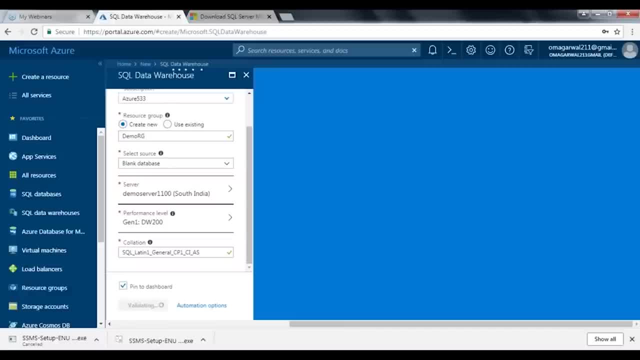 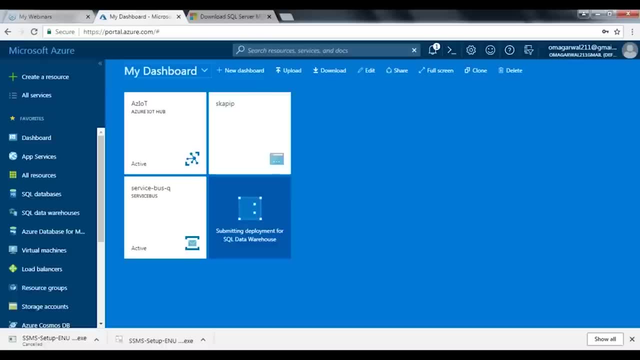 I would say pin to dashboard and I would say create Now. the deploying might take a little longer than normal because, yes, as I've already mentioned that it depends on the internet speed and even if your internet is faster at times, it might take a longer while for this thing to happen. 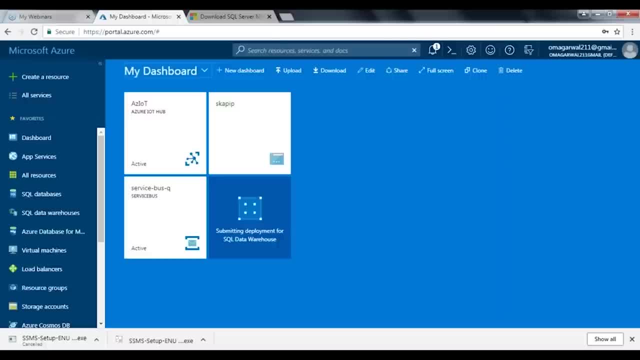 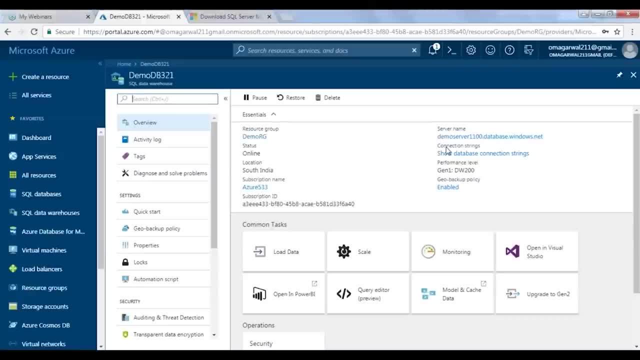 So what I'll do is I'll just pause the video for a minute and once the deployment is done, I'll get back to the demo part again. So yes, guys have gone ahead and I've done the process, that is, we have our so-called demo DB already. 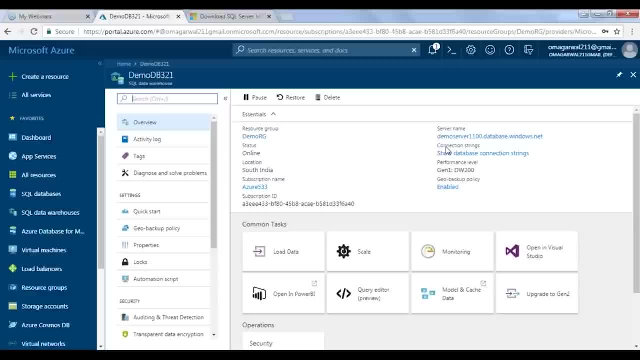 It took a while I actually went back and had a cup of coffee as well. It took that long. My internet is really slow today. So, yeah, let's move further and now try to go ahead and do the other thing that we are supposed to do. 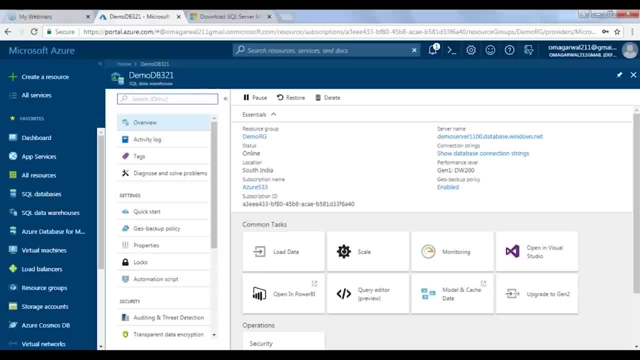 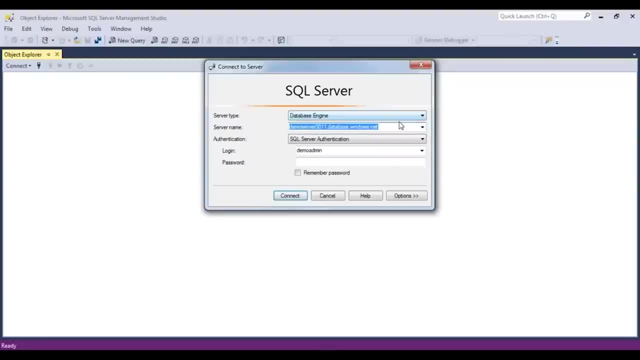 as I've already mentioned, you need to go ahead and install SSMS. if you do go ahead and install it, This is how it would look like. now, since we've already created a database, we can log into it. You can go ahead and given your credentials here, that is, I would be putting. 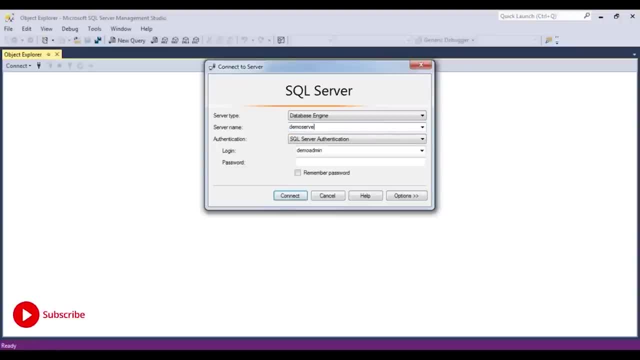 in the credentials which I've mentioned, that is demo server 1 1 0, 0 and then the extension. that is database, not Windows dotnet. Yes, and the name here is admin: demo. I can go to options here. connect to what database? 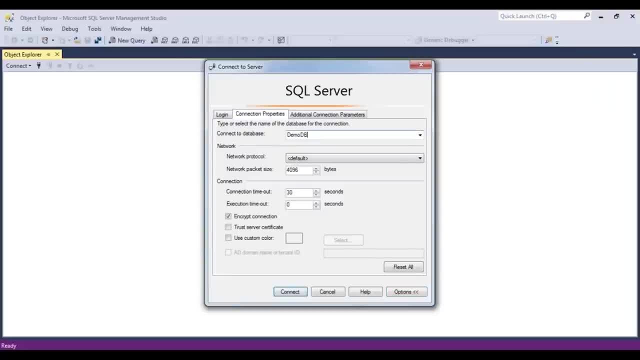 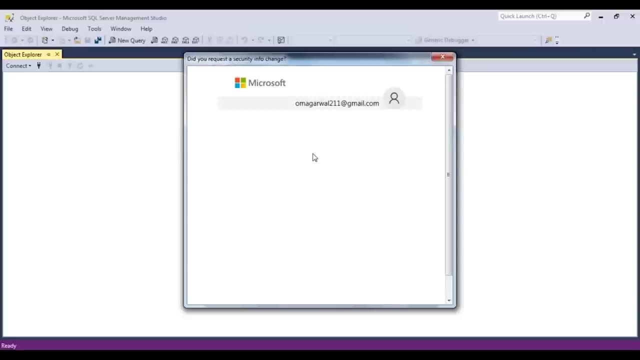 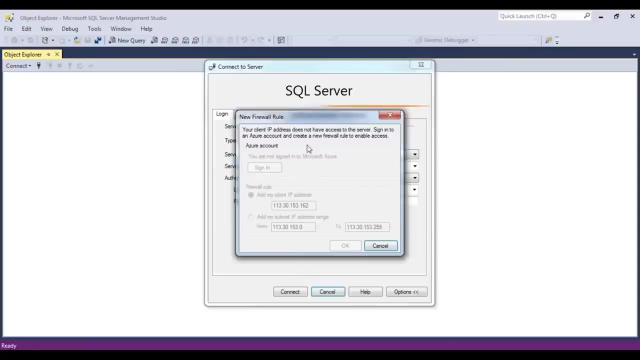 we have something called as demo DB and that is 321 TCP IP. I say connect. it wants me to sign into my so-called as your account. I hate this each time it happens because I've already logged in. I should have stayed signed in but I did not, and that is costing me now. 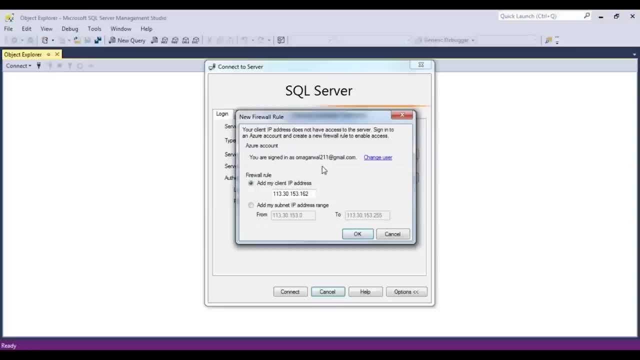 Yeah, one more thing. at times you would be logging in from your client user Or your client PC, and that times you might not be an administrator. So in that case you need to change the firewall rule and make your system accessible here. And there you go. 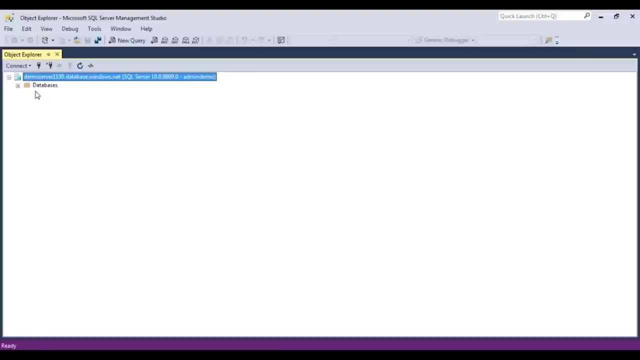 I've signed in, So we have our information here. That is, this is my server. I used to log in and if I click on databases, the schema is there. We have our database. that is demo DB 321.. Now what we can do is we can actually go ahead. 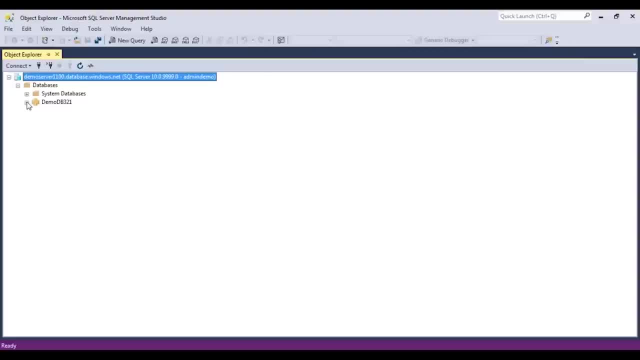 and add a table to it. Now, I'm not going to go ahead and create a table, a completely new table. instead, I'll just go ahead and maybe run a simple query, which lets me have two columns. So what query should I put in? 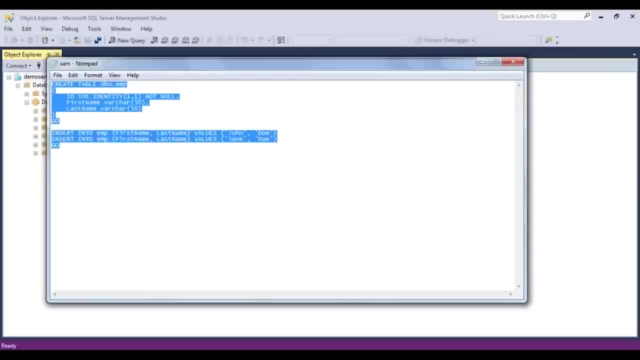 What table should I create? I'll just go ahead and pick up some query from Microsoft Azure website. Now, this is something that lets you create a table with this name and these are the so-called variables or column names That you are so called table will have. 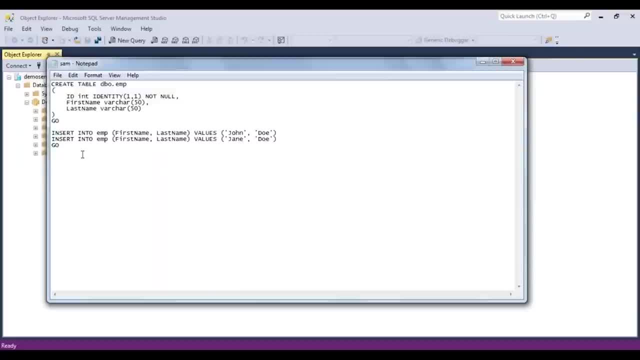 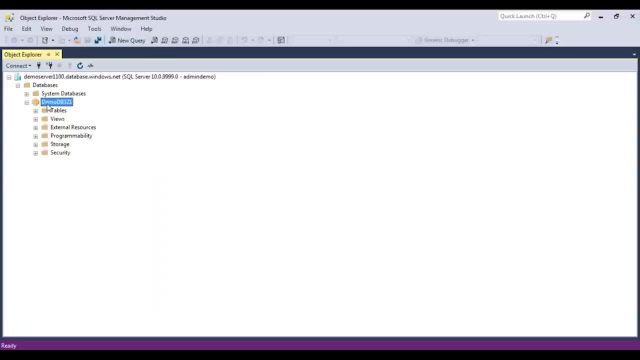 so I'm just going to copy this piece of code. If you wanted, you can go to Microsoft Azure website and you can have this piece of code as well. I'll share the link. do not worry So when I close this and I come here. 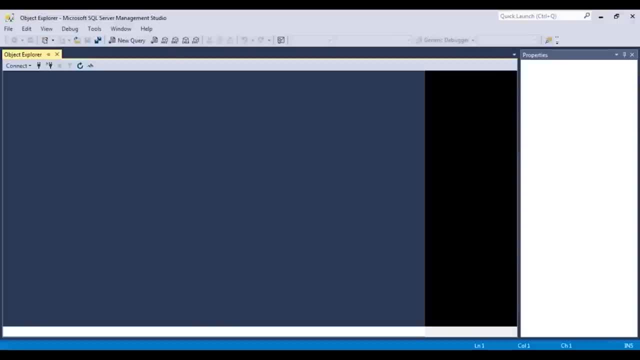 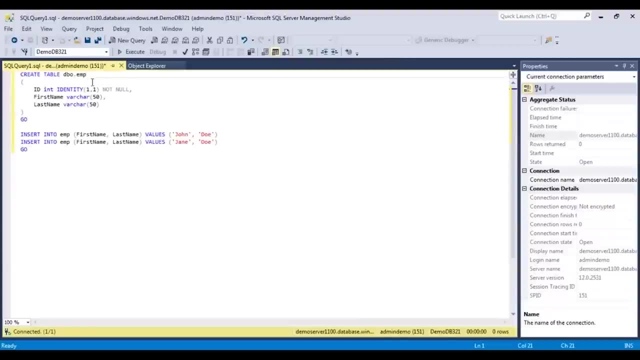 and I click on this, I say new query And I simply go ahead and paste this piece of code. Now I'll just make some changes to the name just to get rid of ambiguity. say to maybe three, and I would be inserting two records in it. 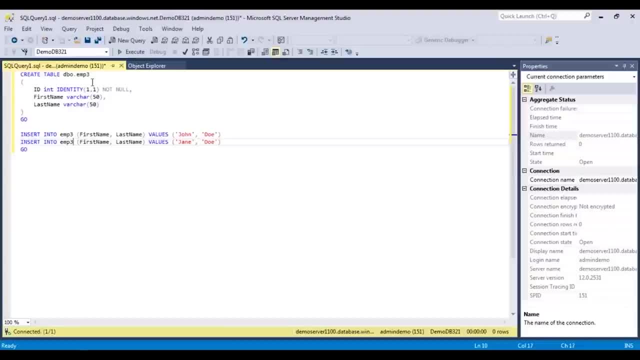 So this is the changes I make here, that is, insert into this so-called table, and to do that, I would say execute. Okay, this should not take this long, but it is now once it does happen. These are the two records that would be there. 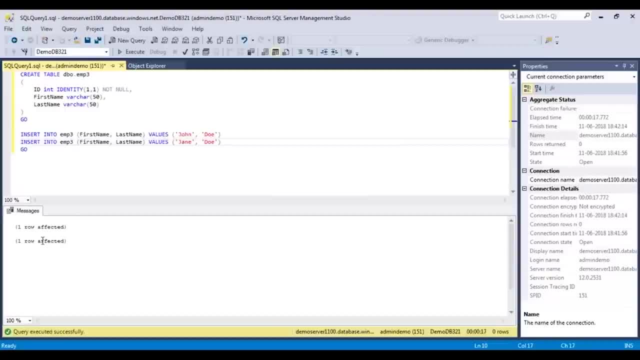 That is John Doe and Jane Doe. There you go. One row is affected is what it says. So we have actually gone ahead and logged into my SSMS and we have connected to our SQL Server and we've created a table there and as far as the table goes, it has these two records. 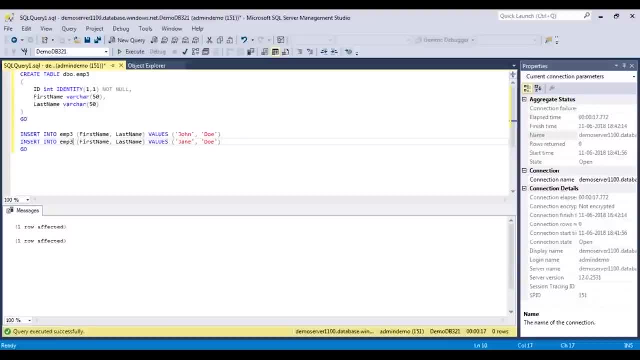 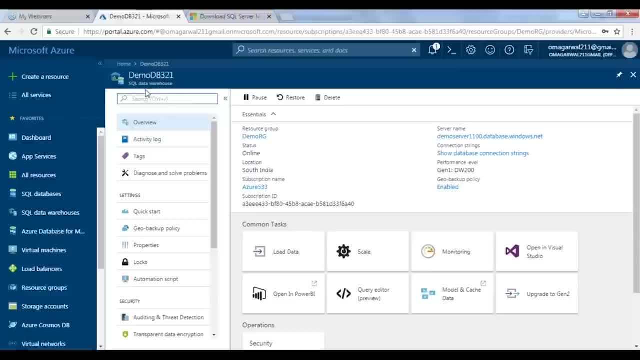 So what I'm going to do now is I'm going to again switch back into my so-called Azure Data Factory, that is, to my Azure account, and create a Azure Data Factory, basically. So how do we do that? first thing you need to understand is in order to have a resource group. 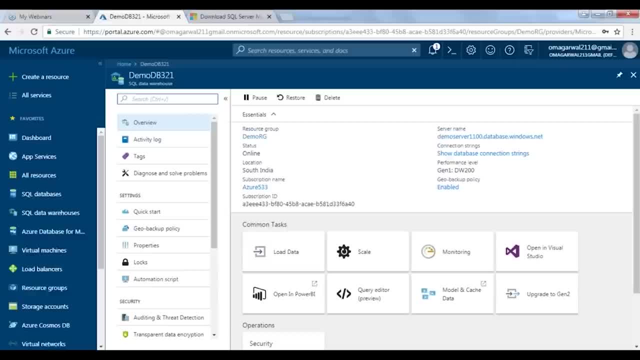 or have all these resources there on your system. You need to have a storage account. Now, this account is nothing but more or less a compliance or a law. basically, what that law does is: it lets you have your storage entities on Microsoft Azure. So let us go ahead and create that account first. 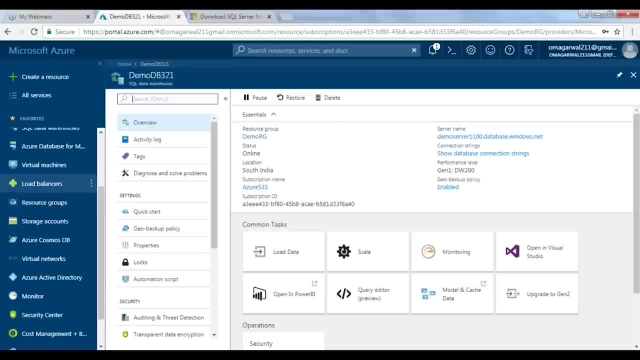 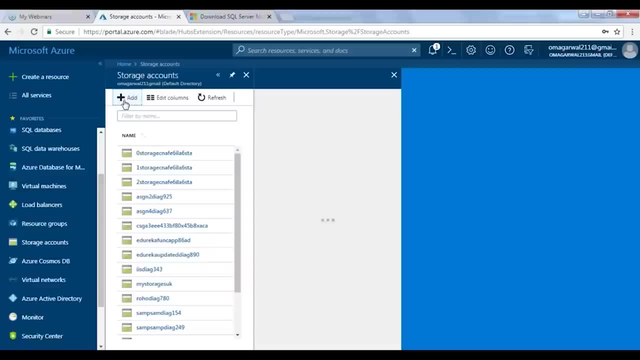 It is very easy. you come to this portal. Once you do that, you just scroll down and you see storage account share and I say add. when I say add, This window should appear and you need to enter in details. So what details should I give in for my storage account? 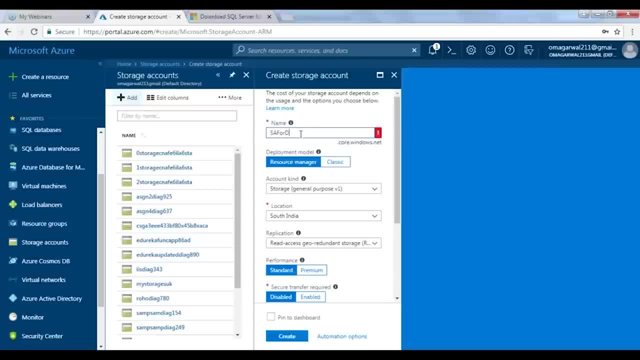 Let's call it, say essay for demo. now It is not accepting this name. Okay, it needs to be in lowercase. So I would say essay For demo and there you go, It is taken. resource manager is what I stick to and I say we to. location is South India. 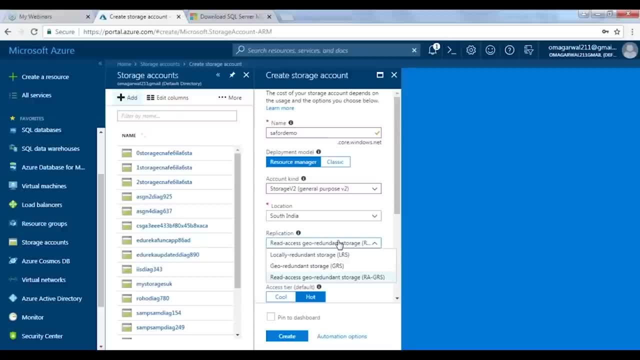 Now I've talked about your data getting replicated three times. that is, three copies are maintained, and when I talk about the replication, these are the types of applications that you have locally. redundant storage is which I'm selecting, which is the most affordable one. It is not very reliable. 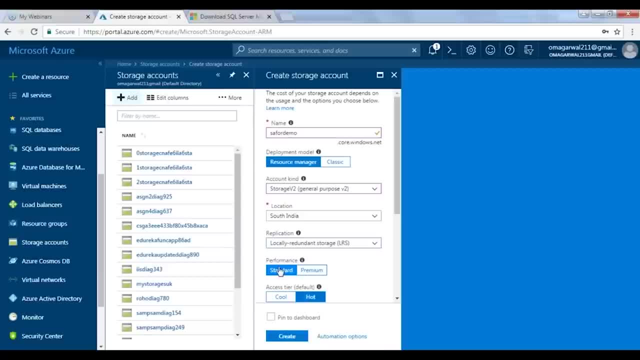 But since it is a small demo, I can use this. performance should be standard And if you see, by default the blob storage is always hot and when you talk about a resource group, let's go ahead and use the one that is already there. Our resource group was demo RG, if I'm not wrong. 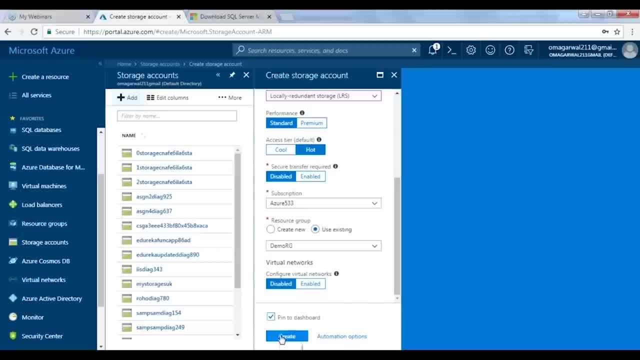 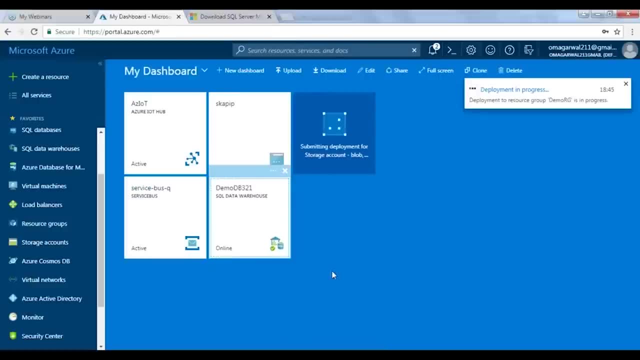 Yeah, let's select this. We need to dashboard and I say create and my storage account would be created. This should happen quickly. There you go. the deployment again might take a longer while. So, yeah, what we have done is we've gone ahead. 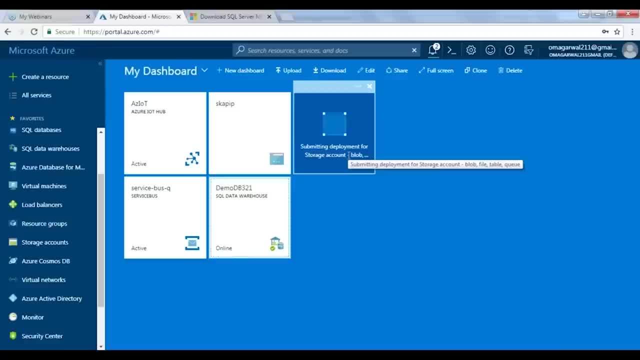 We've actually created a database. you've connected to a server, put a table there and now I've created a storage account. since I have a storage account, I can go ahead and create again containers and then I can use data Factory to basically move data between various sources. 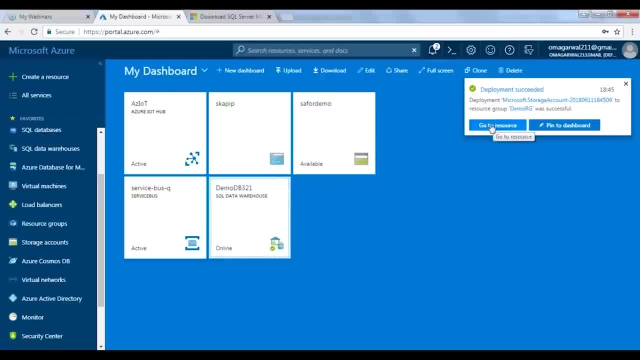 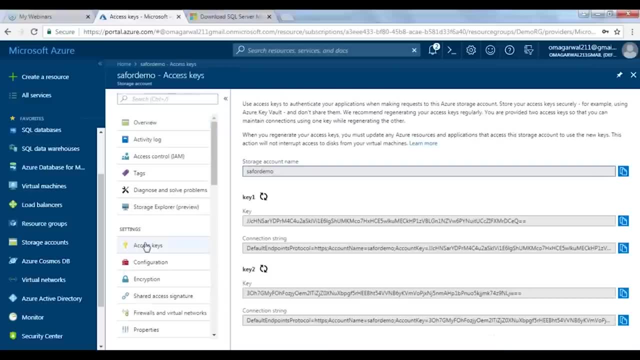 as you can see, it has been deployed. Do I want to go there? Yes, I do. Now, when you come here, you see this so-called app. here You have something called as access keys. What you can do is you can actually come here and copy some of the data that is here. 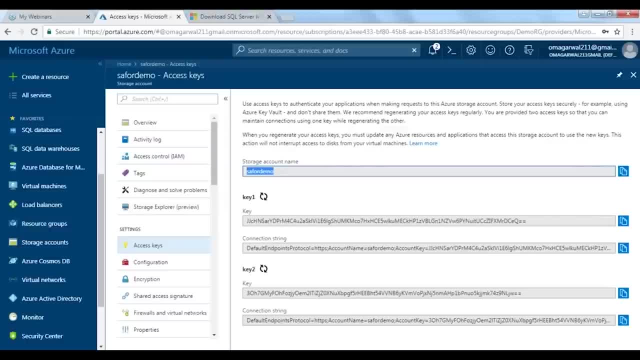 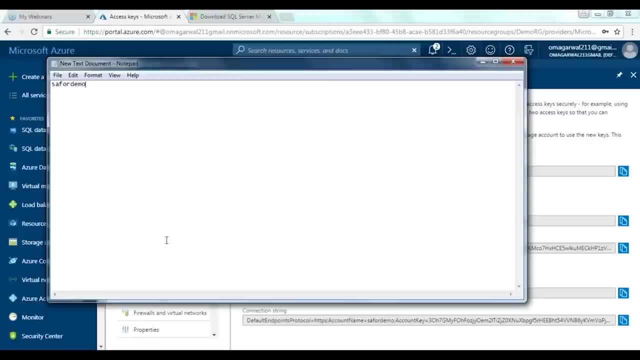 This is the name of your storage account, which you would be needing, and they're quite a few terminologies that you need to remember when you are using or going through this demo. Like I mentioned, you have created a database. You need to know its name or remember its name. 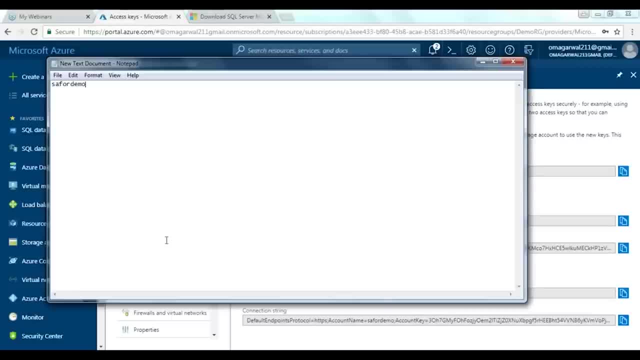 You need to know the server name, What is your server admin credentials, plus what is the name of your storage account, which is this, in this case, the key. I'm not sure whether we would be needing it or not, But if we do, I would still say that you copy this first key. 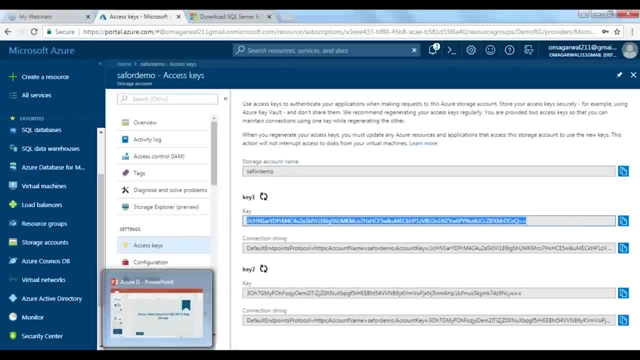 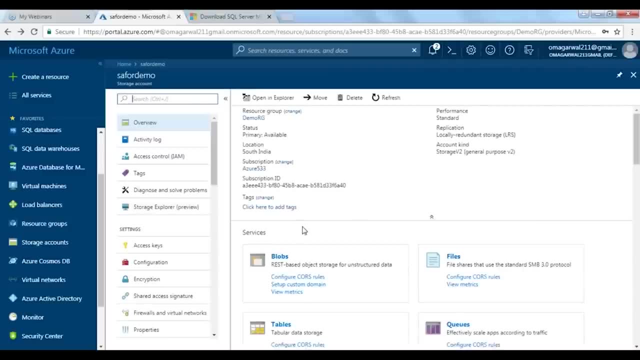 that is here I'm going to control a control C and I would just paste it there you go. Now, when you move back to this page, you have this option: here: blobs where we are going to go ahead and create a container. you can click on it. 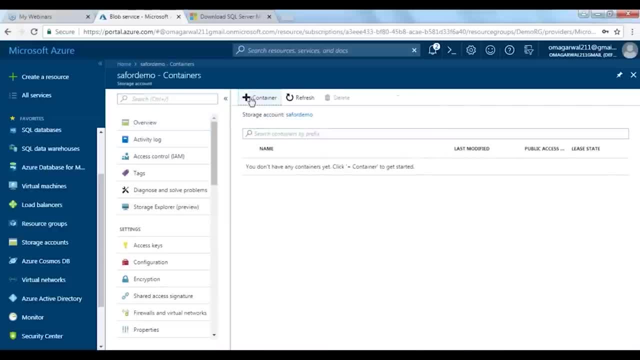 As you can see, there's no container here. So you click on this plus sign and you have an option to create a container. So what do we call this particular container here? Let's call it, say, blob. again, You need to use something small, that is. 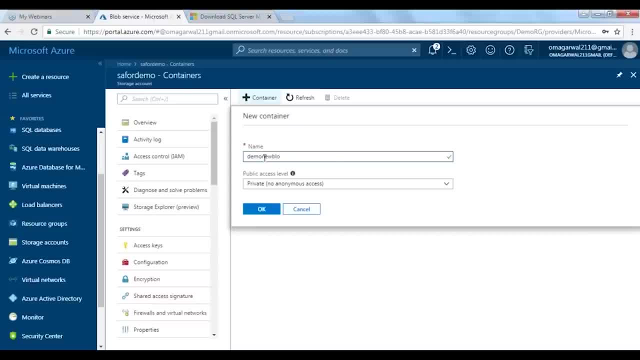 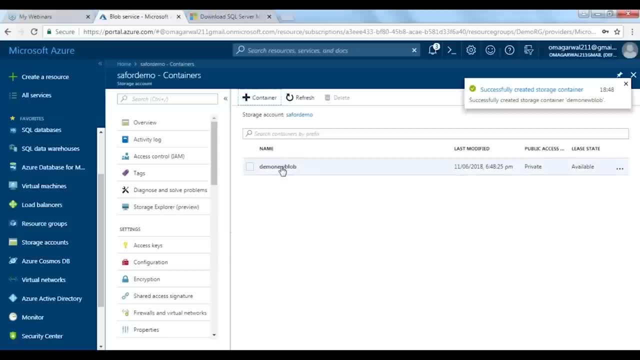 demo new blob, Maybe is what I'll name it, And I'll let the public access level be the way it is and I would say, okay, and my blob is created here. Now I won't be adding a destination folder or something here, because when you do go ahead, 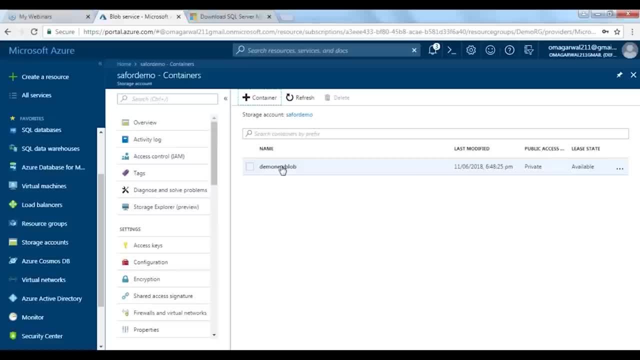 and move your data. destination folder is created automatically. So let's not do that. Let it be the way it is. So I have a blob storage or a container with me. now I need to go ahead and create a data factory here. So how do we do that? 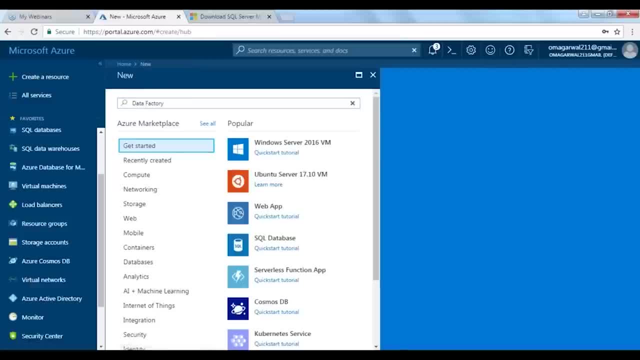 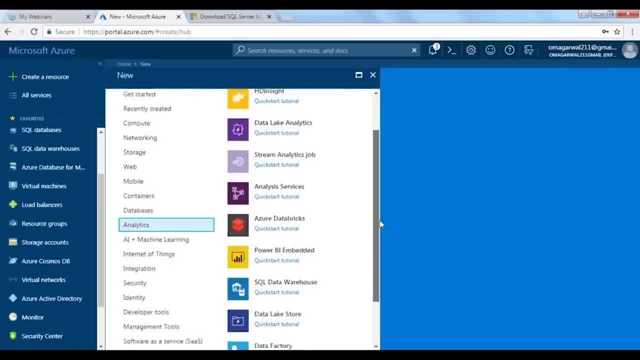 Come here, Let's search for data factory directly. There you go. No, this is not where I want it to be, So I close it. I click on analytics and here I have the option of data factory. I click on it. Yes, so I can create a new data factory. 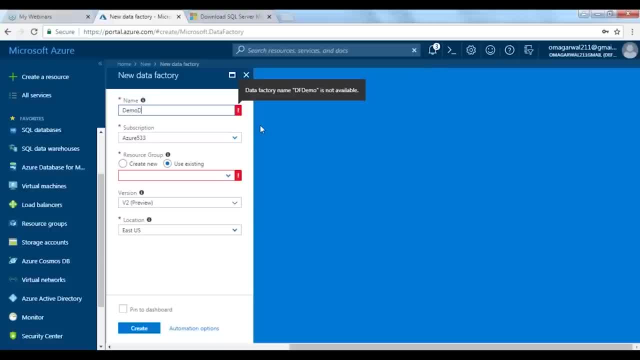 So what should I call this? Let's say demo DF. Okay, it's still not there. So that is surprising. Okay, Let me just try a few names And come back quickly. So this name is accepted now. So use an existing resource group. 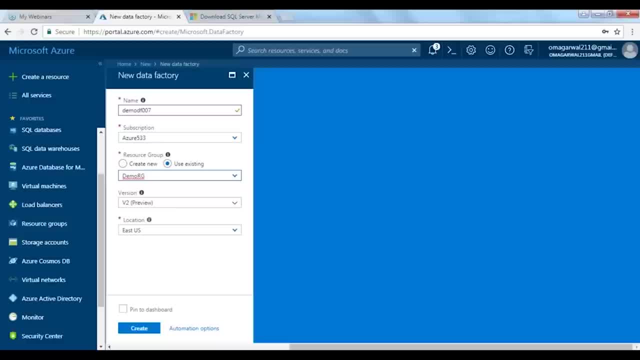 which resource group did we have? It was demo RG, If I'm not wrong. there you go. V2 is the latest version that we have, and do we need to bother about this thing? Let's say, okay, These are the areas that are there in the option. 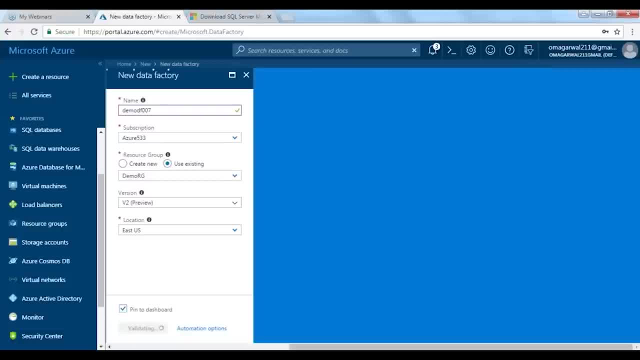 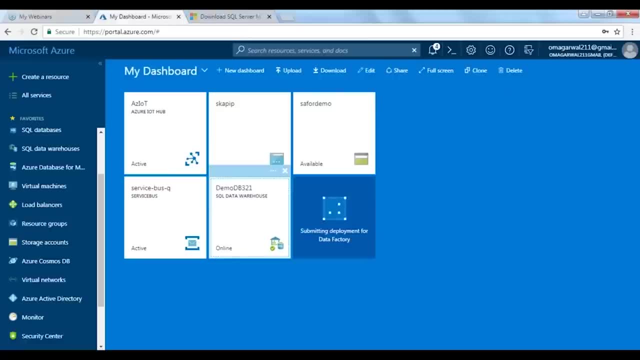 We select this into dashboard and I say create. and I have a data factory with me, So this might take a while, So let me again pause it and switch back to the time. No, I don't need to do that, It's created. 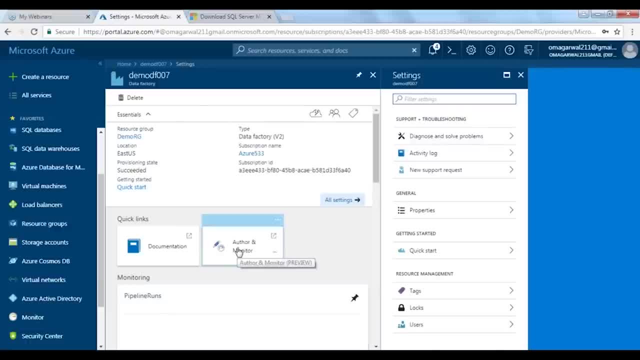 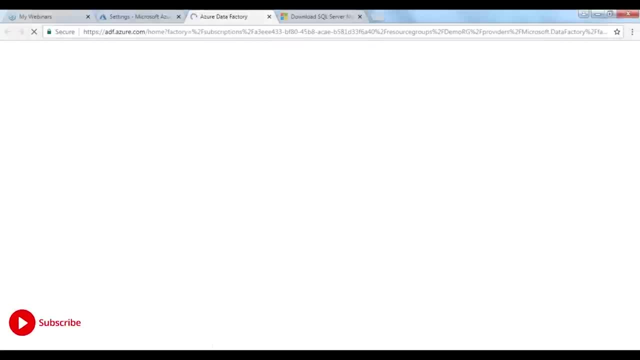 Okay, so I have a data factory with me. now I need to come here and click on this because I need to go ahead and move my data, So I come here. When I click on this thing, I would be given quite a few options to deal with. 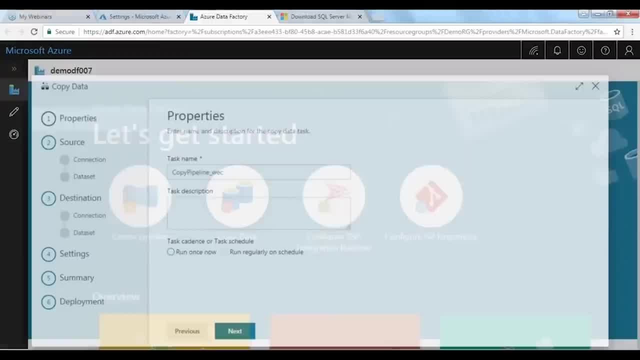 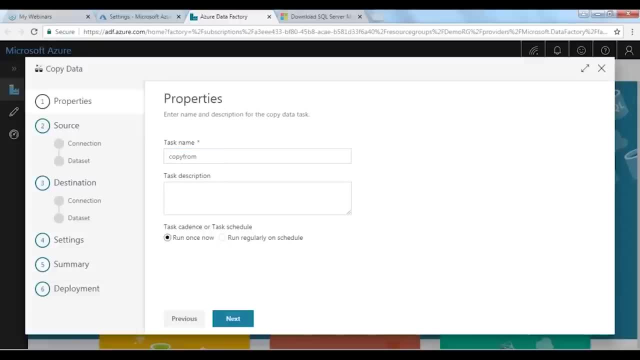 So I need to copy my data. So I click on this icon. There you go. I need to give a name to the task that is there. Let's call it say: copy from DB to blob And I go to next. I need to select an SQL Server here. 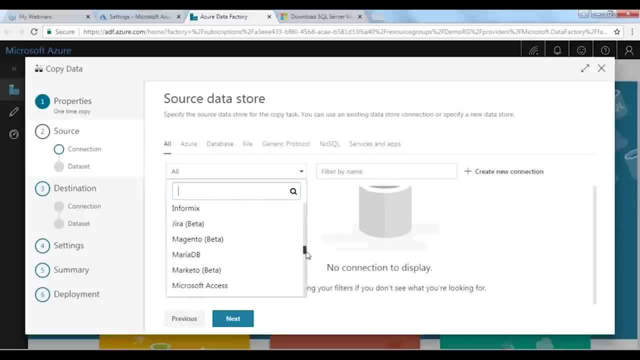 So I come here and I scroll down. now The interface might vary from different portal accounts. This is what it looks like as far as my so-called system goes: a skill server here, Here it is, I select it and I say create a new connection. 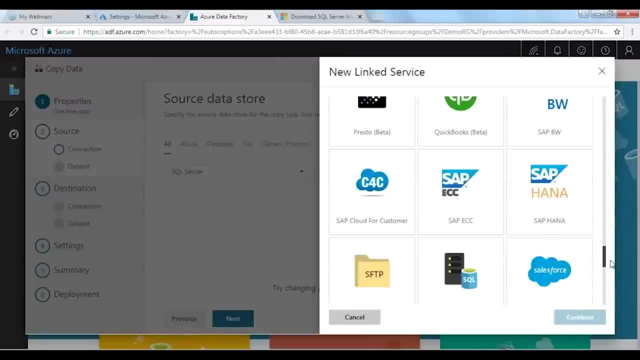 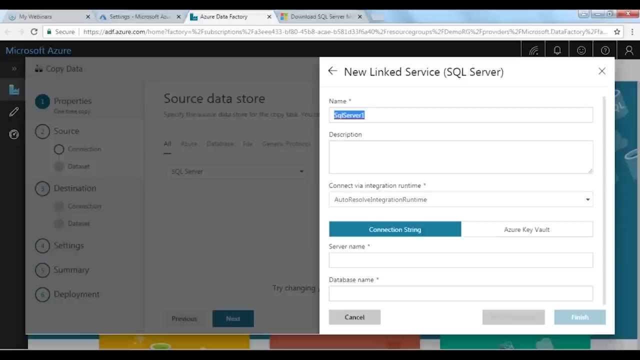 There you go. You'll have to scroll down right at the bottom, Skill server server server. Did I miss it somewhere? Yeah, here it is. You select it, say continue, and you need to give a name to your new linked service. Now, what name should you give it to you? 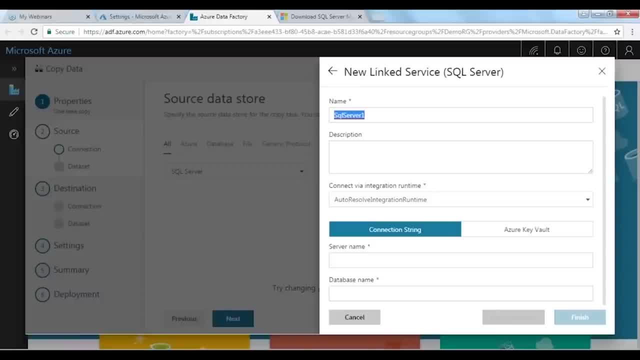 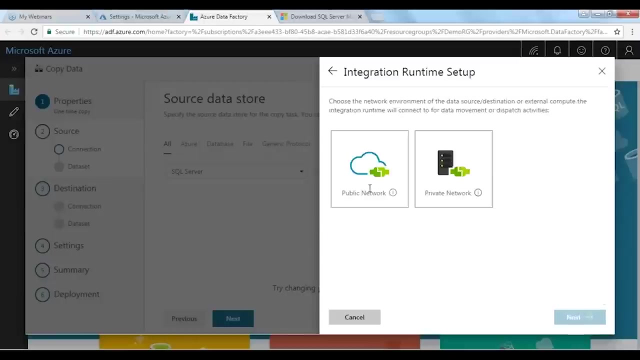 Say SQL Server demo link maybe, And I also need to go ahead and create an integration environment. So I come here and I click on this thing and I say create new Public Network. I see next. So what name should I give it to it? 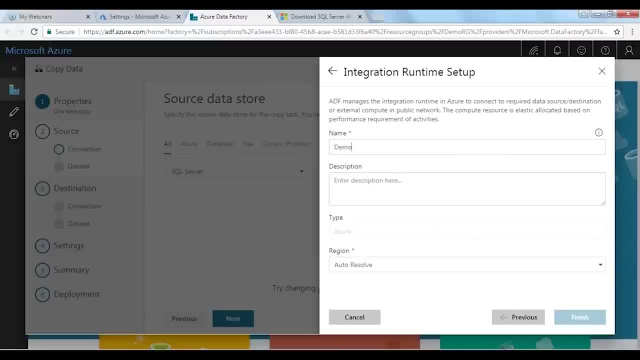 Let's call it said, demo integration maybe. And I say: finish Now, as you can see, what we've done here is I've gone ahead and I've been given in details for my so-called source. That is the place from where I'm going to go ahead. 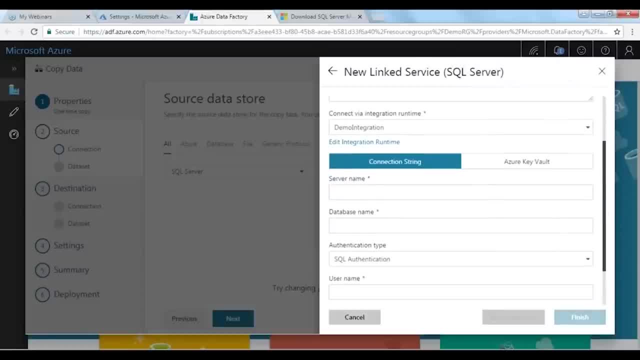 and use all the data. So I have this. so I need to go ahead and given my server credentials again. So, if I'm not wrong, the name was. I'm telling you you need to write everything down because you would be using all these names. 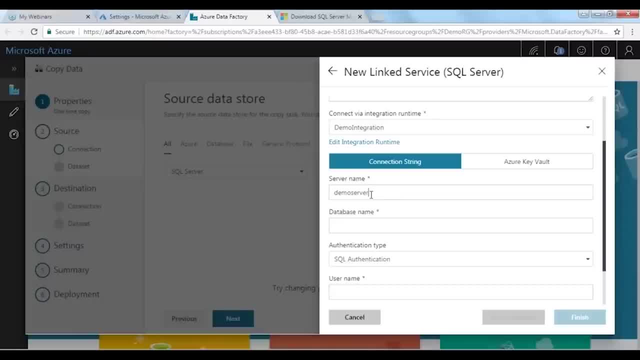 So a best practice would be: We're going to write everything down. So in my case it was something like demo server: 0 0 1, 1, if I'm not wrong. sorry, 1 1 0, 0. the extension is not database. 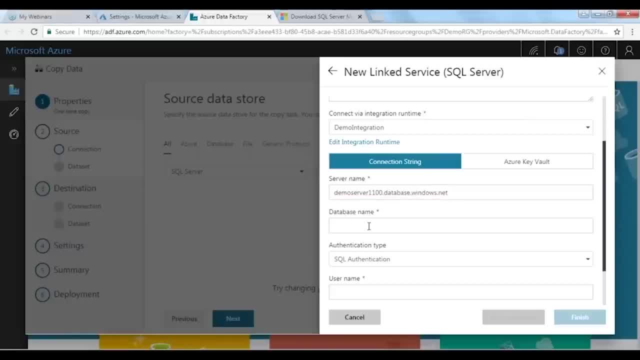 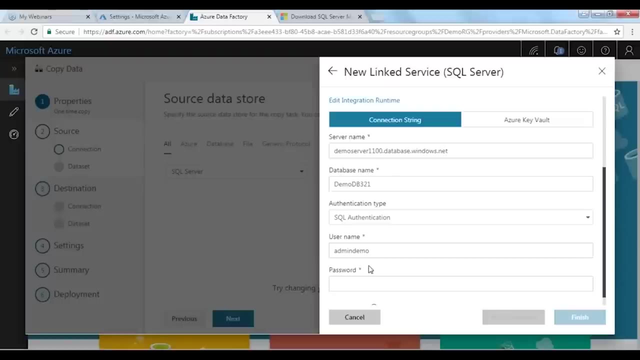 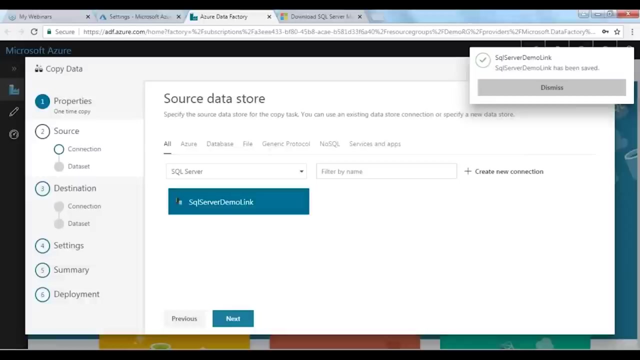 Dot windows dot net. There you go. The database name was demo: DB 3 2 1. SQL. authentication username was admin demo, If I'm not wrong. I scroll down and I enter the password that is, and I say finish. So yeah, my source details are given in already. 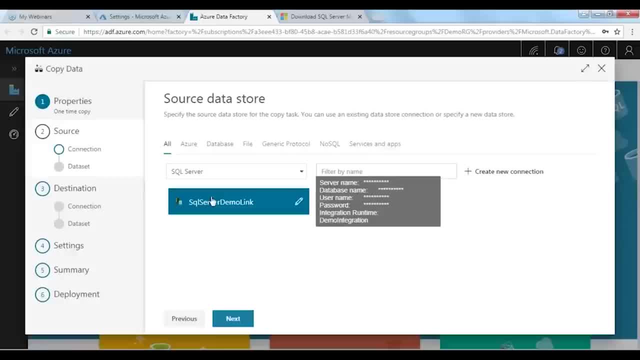 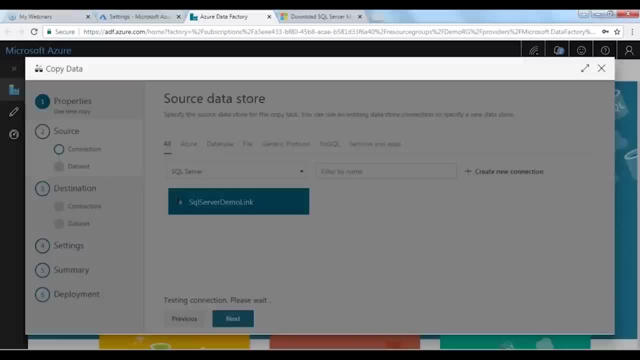 That is, this is my source data store and these are the informations, or this is the place from where I would be wanting to move in my data. So I go to next and then I enter the details about the destination now, But before that, what we do is I need to select a table. 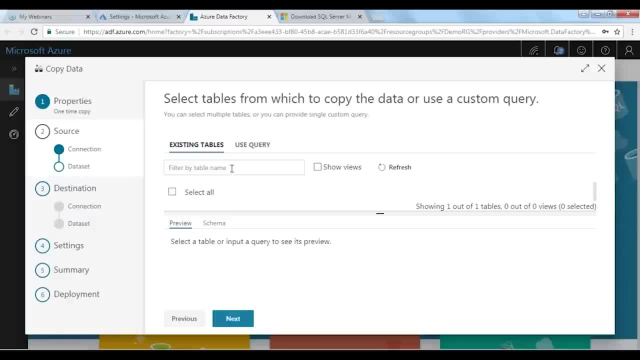 If you remember, we had run a small SQL query to give you the details. I do not remember the name It was. what was the name of the table? Was it EMP 3, was it? Yeah, let me just refresh it to see if the information is there or not. 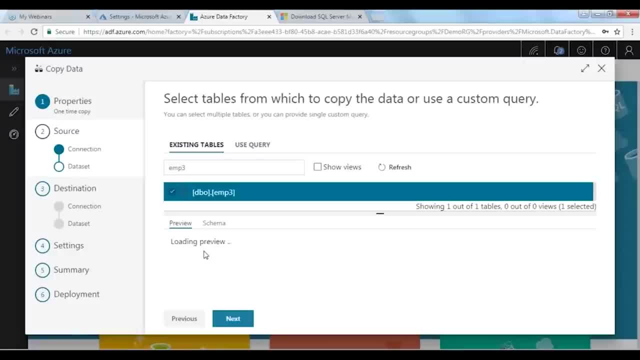 I scroll down and it is here, So I select it and it would load the preview saying that: okay, These are the records that are there. now, These were the records that we entered. so I say: next For my destination, I'll come here. 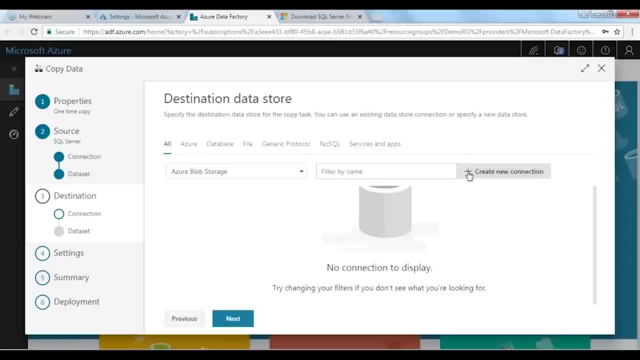 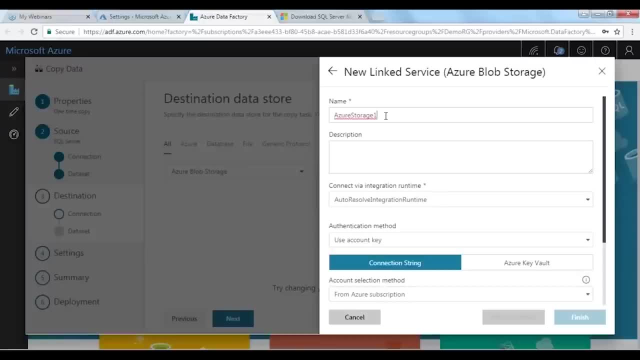 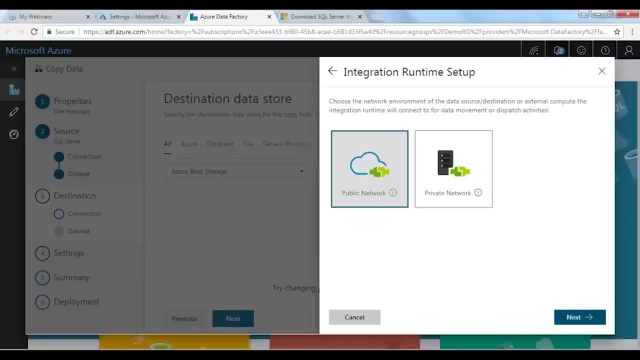 and I would select a blob storage. Now, there you go, create new Azure blob storage and I say continue. now I need to enter in details here as well. Let me just call it, say, as your storage demo link. Let me just do this thing again quickly. 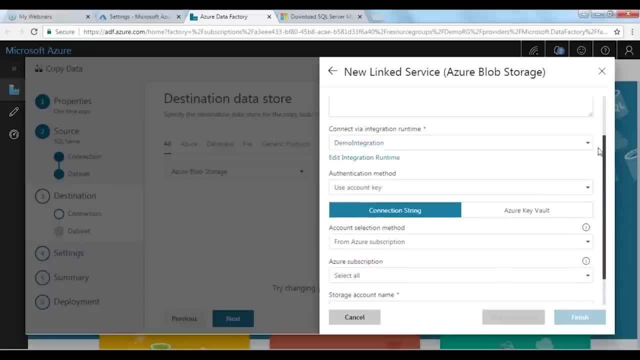 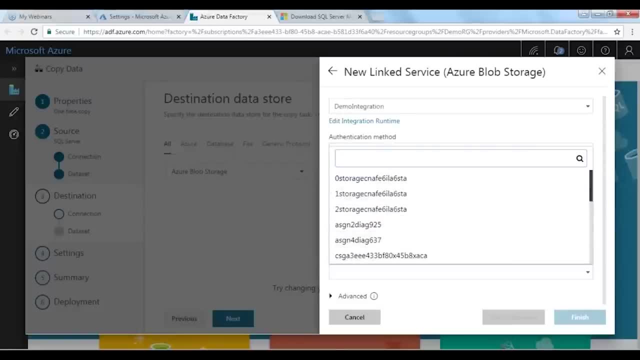 Now we need to select a storage account name as well, because we've gone ahead and created a storage account here which was for the demo part. What was the storage account? I forgot the name of it. It was storage account for demo, if I'm not wrong. 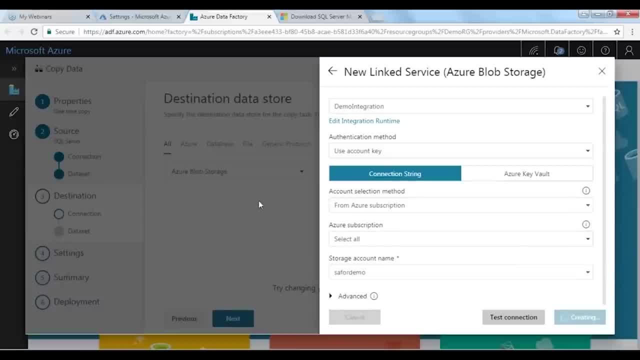 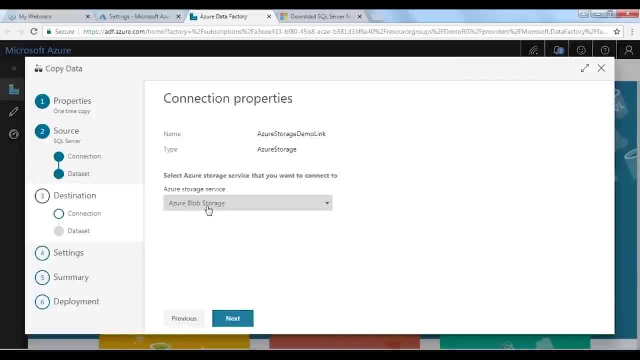 and I've selected that, and then I say finish, I click on next, Now, this is the service that I wanted to connect to. I say next, now I have to enter the so-called details. for that I would be actually needing the name of my blob. 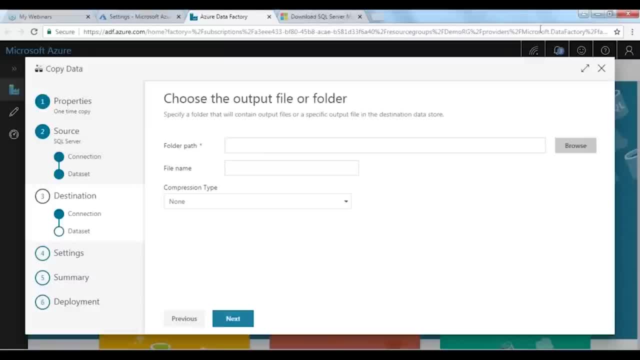 which I think I've forgotten, So let me just go ahead and get the details of that as well. It was something like this: that is demo blob and the file name was EMP3.. If I'm not wrong, I say next, I say next, next again and I say next. 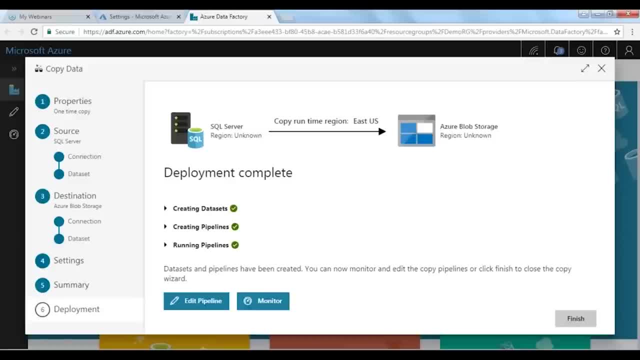 And there you can see the data has been deployed. that is, I've actually connected my skill server and I've gone ahead and I've moved the data to my so-called blob storage, which you can actually also do. then you can go ahead and edit the pipeline if you want, as you want. 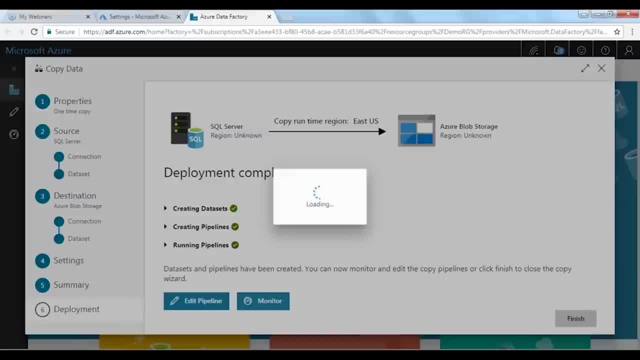 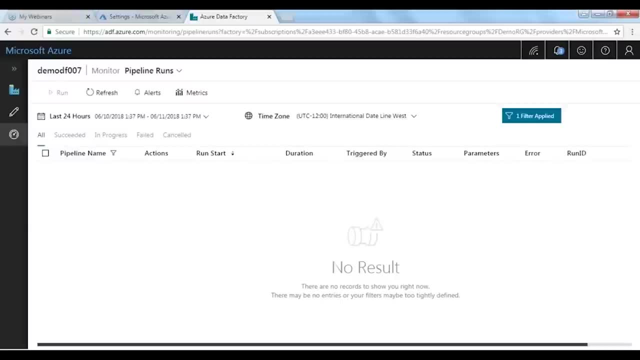 or you can just go ahead and monitor this data as well. It depends on your needs, as in what do you want to do. You can go ahead and do quite a few things with it. That is, you can go ahead and move this data to your so-called power bi. 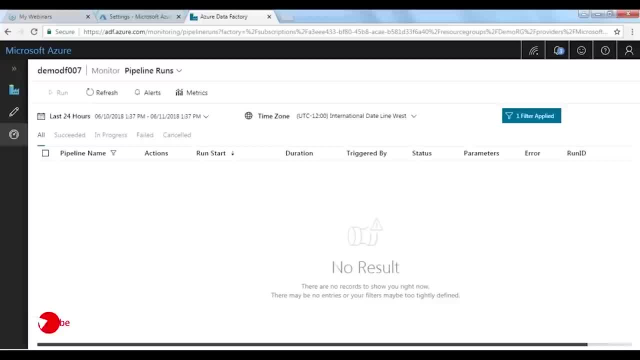 and implement various other things on it as well. when we did go ahead and create our so-called blob storage- that is, blob container- You can actually go ahead and keep that part or that so-called window open, because when you do go ahead and deploy this data, 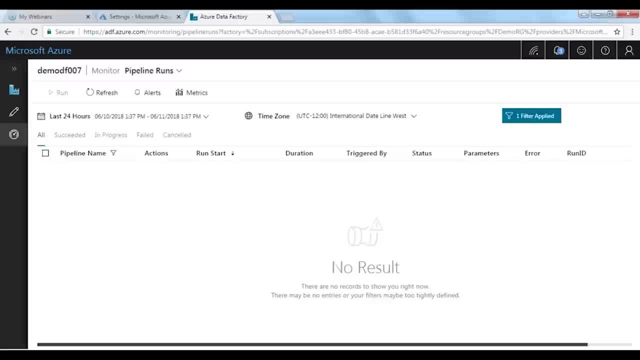 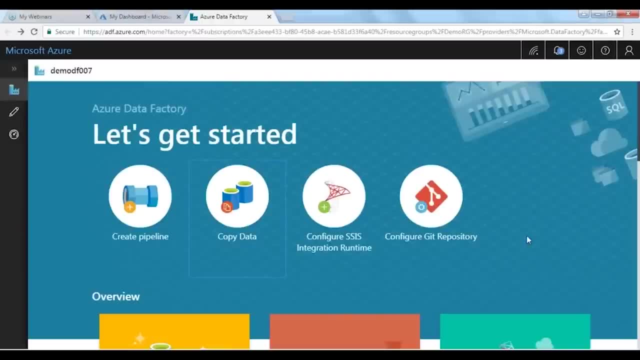 you can see all the details, not as what has just happened and how has it happened, all those things. So, yes, what we've done is we've gone ahead and we've moved our data from a so-called database to our blob storage. now I actually accidentally went back. 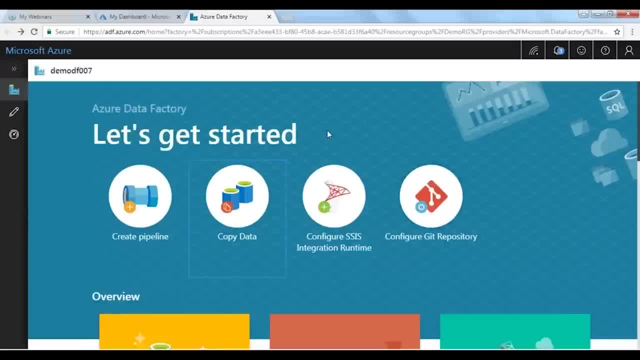 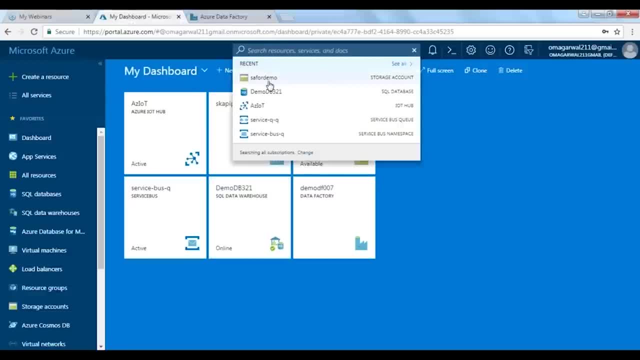 and did not go through that step where we see the deployment. but do not worry, We can just go back to our dashboard and take a look at that thing as well. So how do we do that? I have this so-called storage account here now inside. 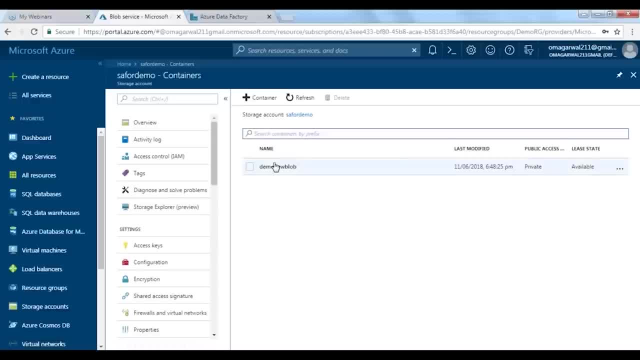 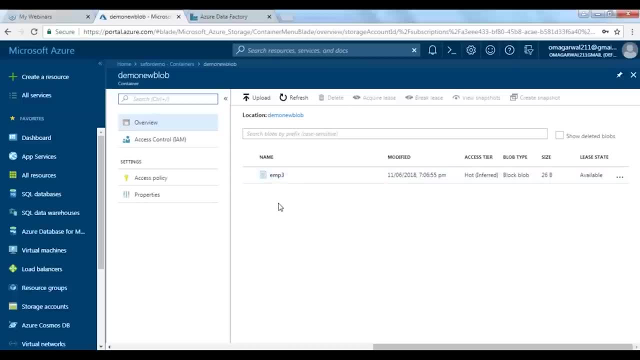 that storage account. We have our blobs where we moved a file. Now this was the blob where we moved the file and then this was the file that we moved. So yeah, our deployment has succeeded, That is, we've moved our data from a so-called database. 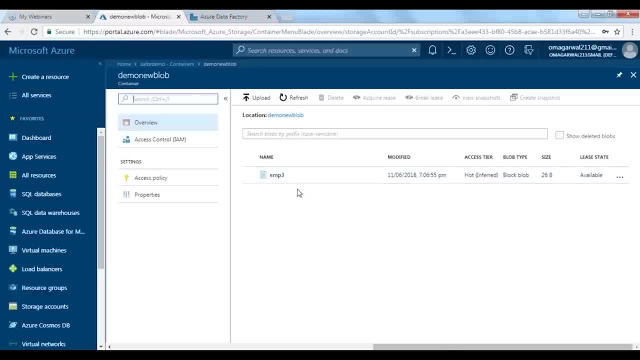 to our show called blob storage And, as far as this demo goes, that is what our aim was. So I hope that I did throw a sufficient light on following Concepts: that is, our data Factory, and how do you go ahead and create a data Factory and use it as a pipeline, basically. 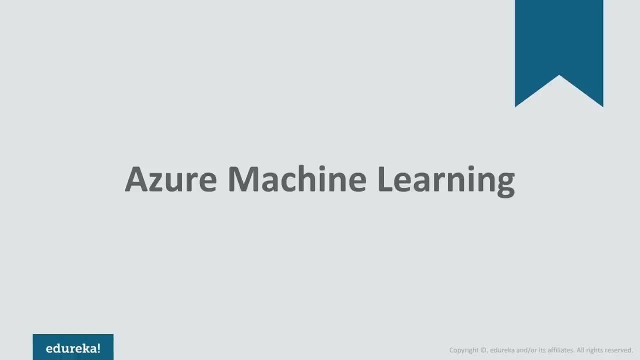 Today we're going to go ahead and talk about machine learning and to implement machine learning models. We would be using Microsoft Azure. before we do get into the details of these topics, Let's take a look at the agenda of today's session first. So, first and foremost, 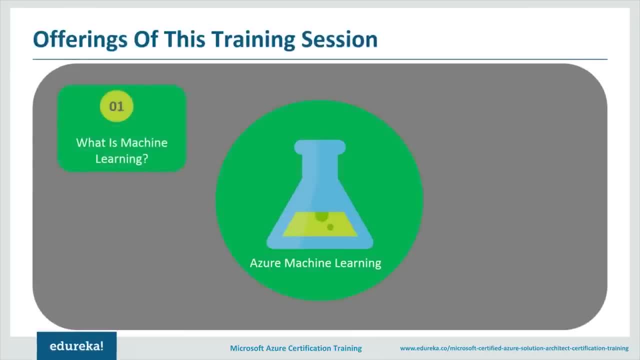 I would be introducing you to machine learning now, it being a very vast topic. We would be first taking a look at some of its fundamentals, and then we would be switching to Microsoft Azure and we'd be seeing how machine learning can be implemented by using Microsoft Azure. 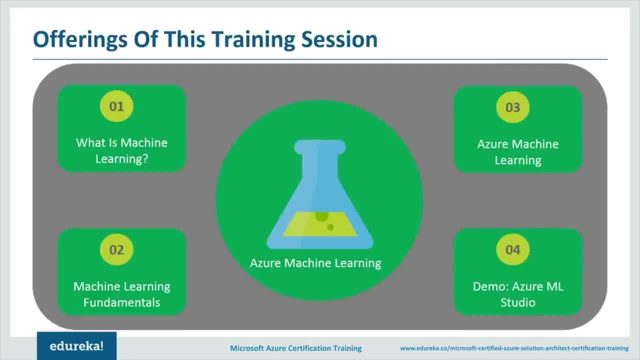 Finally, I would finish things off with a demo part where I would be talking about Azure ML Studio that lets us carry out machine learning processor. I hope this agenda is clear to you guys. So let's move further and get started with the first topic of discussion. 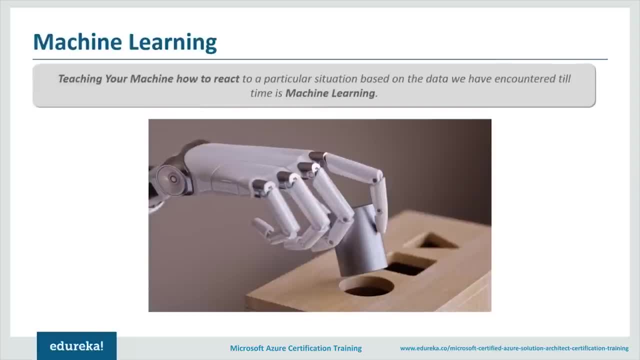 That is what is machine learning. Well, if you go by the definition, it is nothing but the process where you teach a machine to take in some data, analyze it or understand it and, based on that data, given some valuable outputs. Now, this is a very generic definition. 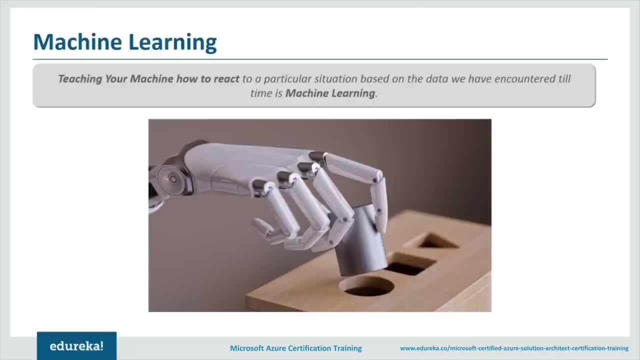 but to give you more simpler an example, I would say that it is something similar to how we human beings learn. I mean, when we are born, we have no idea about anything that happens around us, right? I mean, we do not know what shapes are, what colors are. 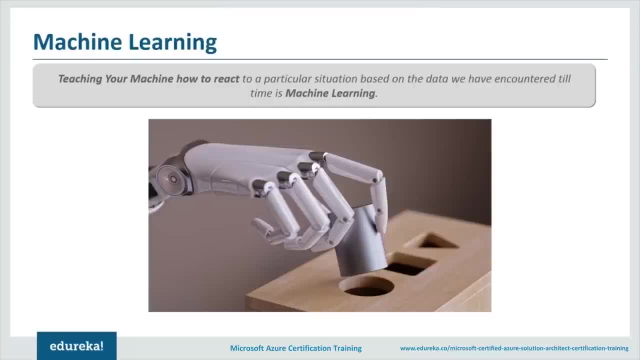 but as time progresses and as we hear people talk, we see stuff happening. when we learn to write, we actually go ahead and understand these things as in what shapes are, what colors are, what people are and all those things. So a machine learning process is very similar to this. 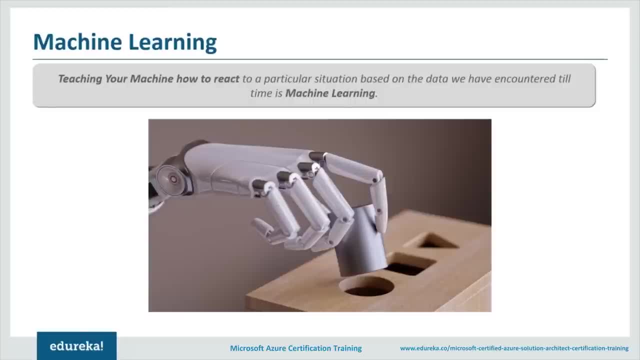 I mean. what happens here as well is you provide in some valuable data to your machine and you train your machine with that data again and again, again and again, or with new data as well. Now your machine takes in this data and it builds in a pattern or an algorithm using 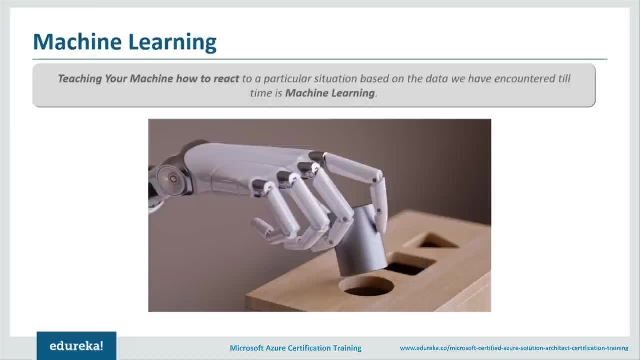 which, if similar data is given to that machine, it would be in a situation where it can probably classify this data or predict something or collaborate this data into something else. So this whole process is machine learning. now, as I've already mentioned, machine learning is a very vast domain. 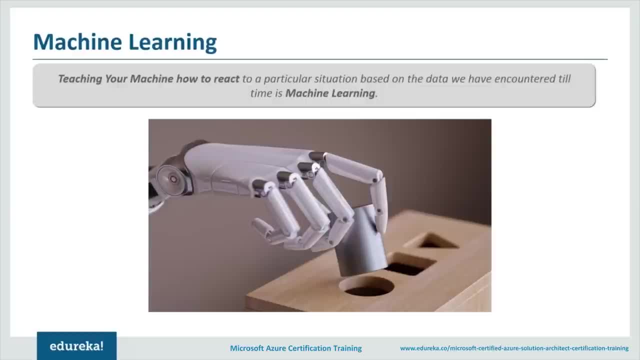 as we move further, we would be discussing these terminologies, as in classification and all those things, but for now, in simple words, it is nothing but the process where you're given some kind of data to your machine. It understands that data and, based on the data, 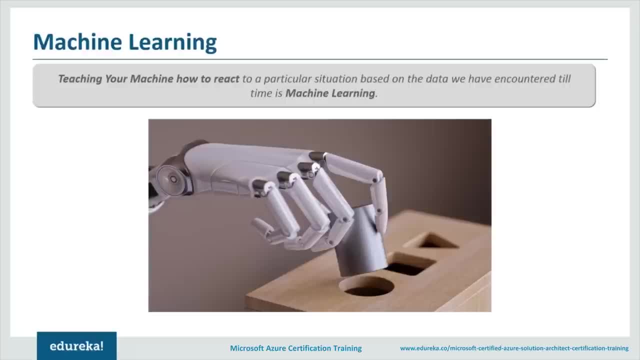 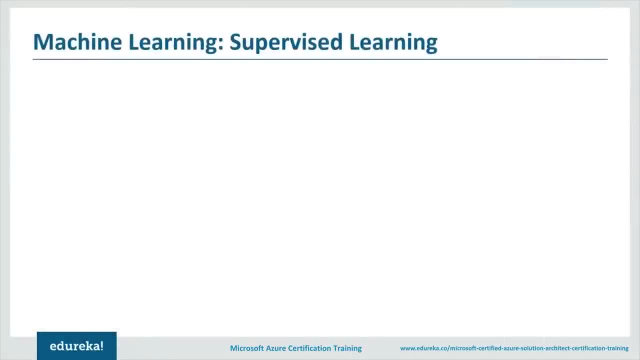 It helps you take better decisions. So let's move further and try to explore or understand some other topics as well. So what do we have next? Let's take a look at some of its fundamentals. If you talk about machine learning, we need to consider two important points. 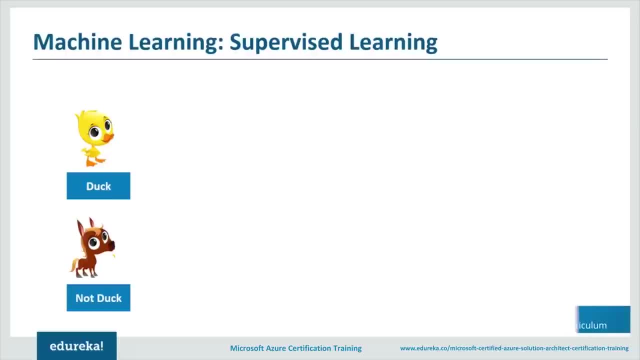 That is supervised learning and unsupervised learning. Now, these are two important classifications. If you talk about machine learning, we also have something called as iterative learning as well, but we won't be getting into the details of that. as far as this session goes, we would be sticking. 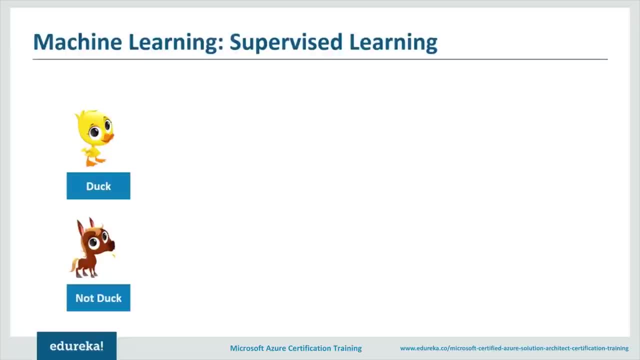 to supervised learning and unsupervised learning. So when you talk about supervised learning, it is nothing but a process where you actually go ahead and teach a machine to predict something based on the information that you already have, or you at least know the target variable. 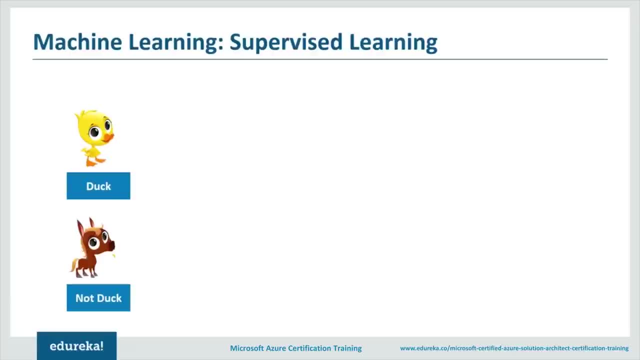 to be more precise. Now, what do I mean by this? Well, in this case, you actually know what your final outcome should be like, or you at least have the parameters that help you govern your final output. when you talk about unsupervised learning, that is something you do not know. 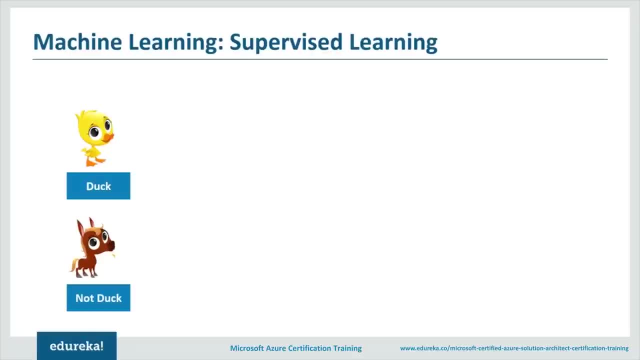 Let's stick to supervised learning for now and consider this example. Suppose you have some data set where you have information, as in. you have some data where you know that certain values or certain records are for ducks and certain values are not for ducks. So what you do is you pass in this data to one 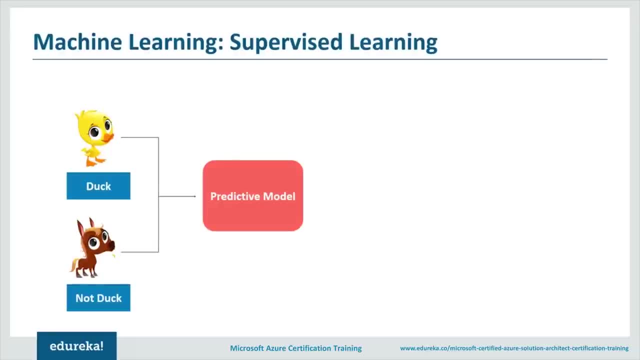 of your machine learning algorithms, rebuild a model around this data and when you pass in a new value to this so-called model, that model should be able to predict whether that value is for duck or it is not for duck. Now, in this case, this value is not meant for ducks. 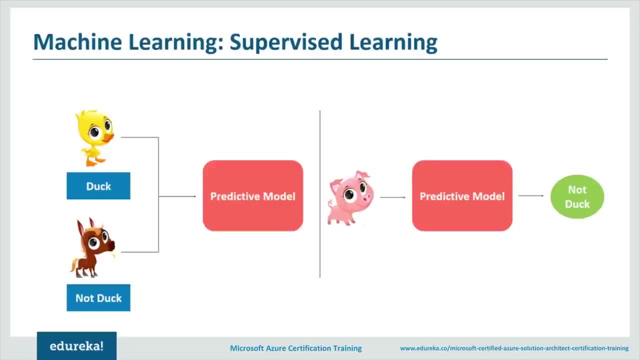 So the answer should be not that, because we can clearly see from the image, It is a piglet, So that cannot be a duck. Now, this is a very simple example of supervised learning. What we are doing here is: we know that. what kind of output are we expecting? 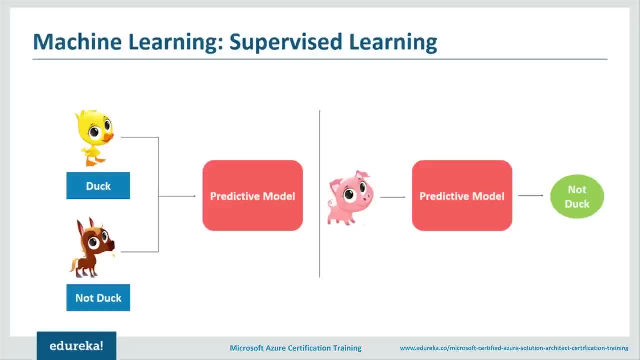 We are expecting an output where we know either it's duck or it's not duck, So our target variable is fixed. I mean we know what we are researching for or what we are analyzing the data for. now These kind of algorithms are called. 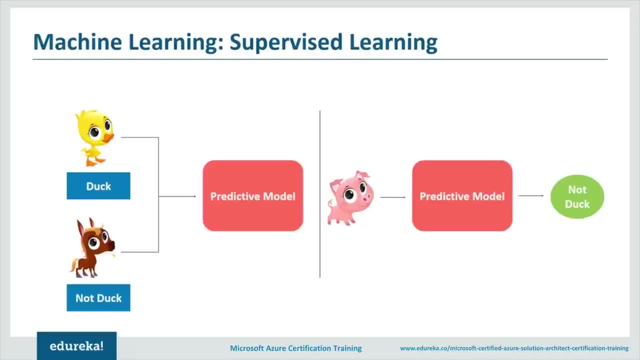 as supervised learning algorithms, or this process is called as supervised learning. So this is a part of machine learning. now, important point to note here is: your data is labeled. now. That is what I mean by the target variable which I just talked about, you know. 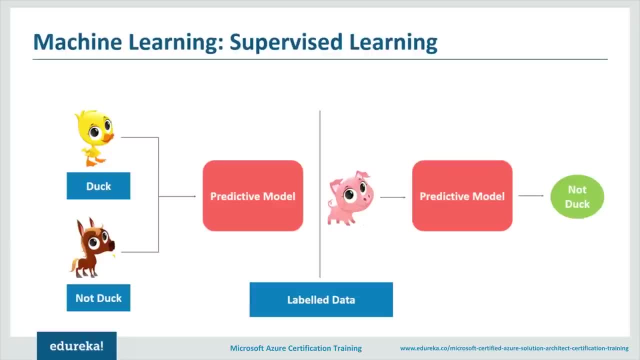 what your final value is, and that is why your data is labeled. you know what you are trying to predict or what your final outcome is. So this is a very important point to consider. your data here is labeled and you know your final goal, as in: 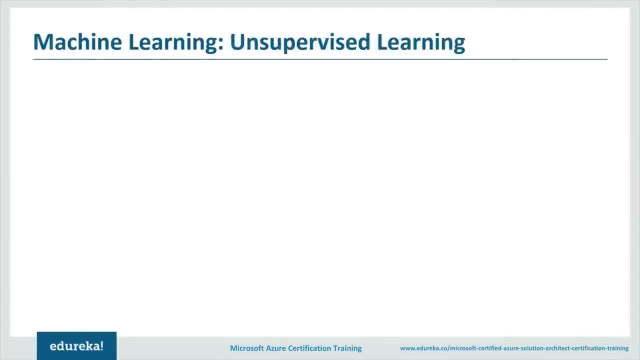 what are you trying to achieve if you talk about the next method or next approach, that is, unsupervised learning? here, You do not have labeled data. That means you do not have a final target variable, in this case, your final target variable or attribute. 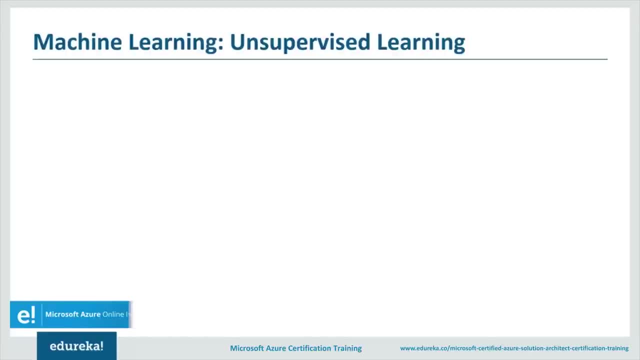 It can be random, or it can vary, or once your model ends, You would be reaching there, but that is something which is not consistent. that can vary depending upon the needs that you have. Let's take an example to understand this a little more. as you can see, we have some pictures. 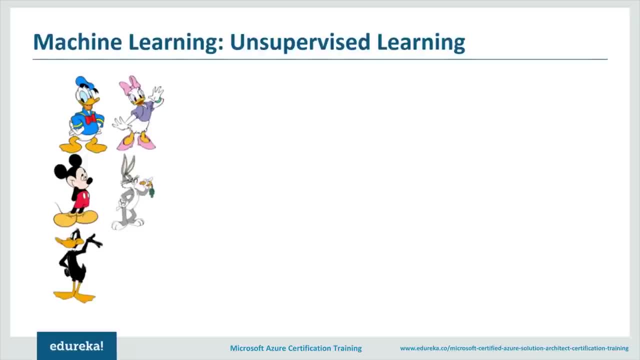 or on the screen You can see certain species of animals and birds. So if I want an algorithm to classify these pictures, or this records into their clusters, this would be more or less an unsupervised algorithm. Let's take a look at it first. 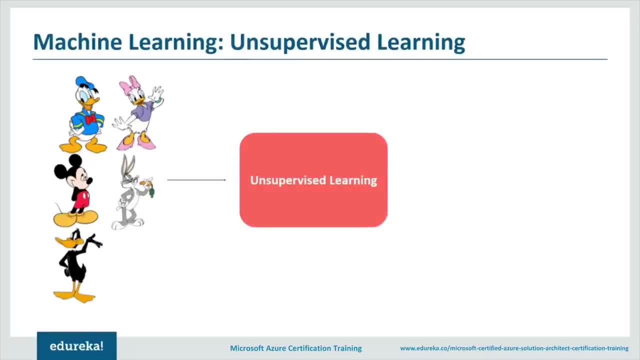 So, as you can see, we can pass in this data to our unsupervised learning model or build a model around this data. Once that is done, it should be able to classify my data into different clusters. Now, as you can take a look at the clusters, 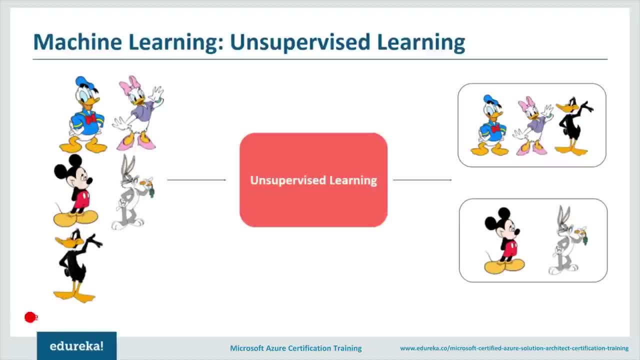 you can see that it has classified my data into ducks and something that is not ducks. Now you might wonder as in? okay, this is similar to what happened in supervised learning, right, But in supervised learning, that is what my target was. I knew that. I wanted to predict whether it's a duck or not. 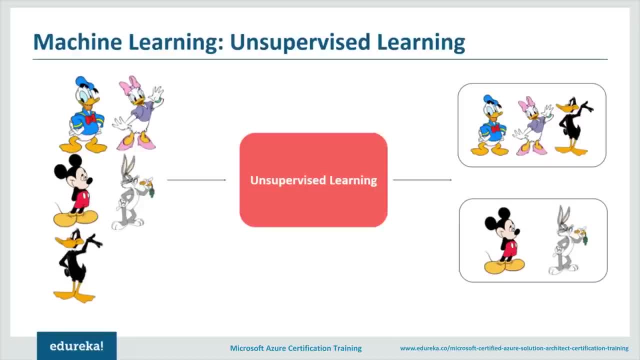 in this case, that might not be the case because, say, for example, I have this data where I have animals and birds and I do not know what animals and what birds are there. They might not be ducks in it right, They might be just mice. 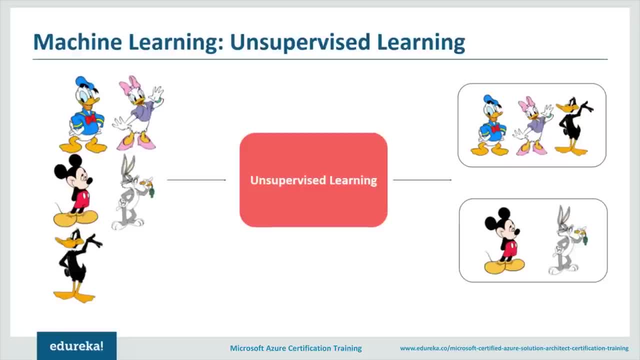 They might be just rabbits and all these things, or you might want some extra clusters as well. For example, I want to aggregate birds, I want to segregate animals. now, in this case, My final output is varying. it can differ, right. I mean I might expect different outputs out of it. 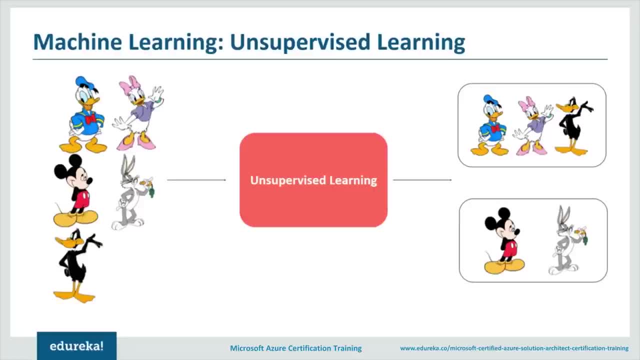 So, since I do not know what my final output is, I do not know what clusters are getting formed here. So that is why this kind of algorithm is called as unsupervised learning, where this is more or less similar to your black box testing kind of a process. 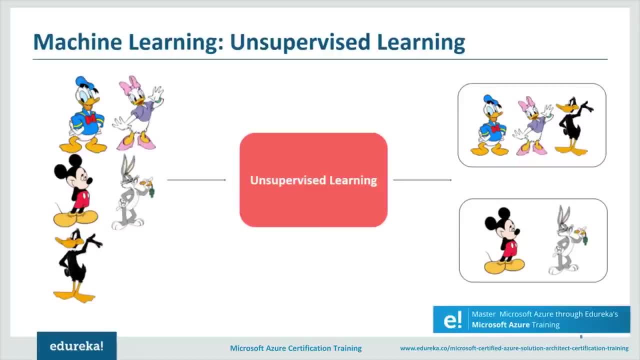 where you do not know what your final output is, but you do run in your algorithm and then you expect a more organized output. that would lead you to better decision-making. and important point to note here is: the data here is unlabeled. I hope these algorithms are clear to you guys. 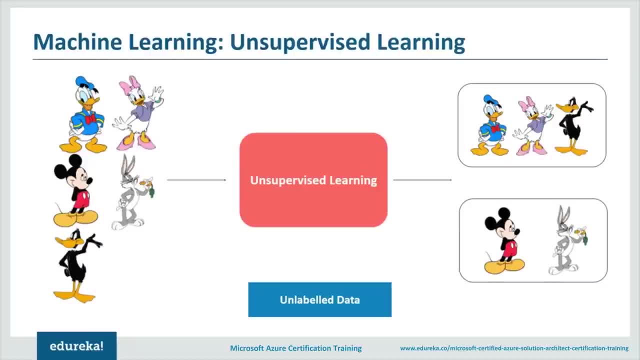 If you do have any doubts, do let me know about those as well. We would be getting back to you on those doubts as well. But in simple words, this is what supervised and unsupervised learning is. now Let's move further and try to understand some other things as well. 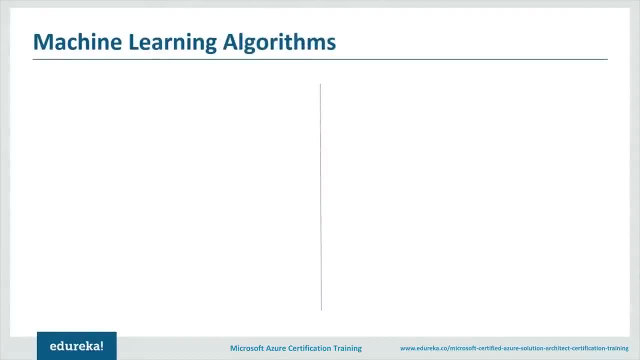 If you talk about different machine learning algorithms, you have these classifications here. first, We have supervised learning, and in that we have something called as regression and classification. Now these are two of the most popular algorithms, or two popular branches of machine learning algorithms. 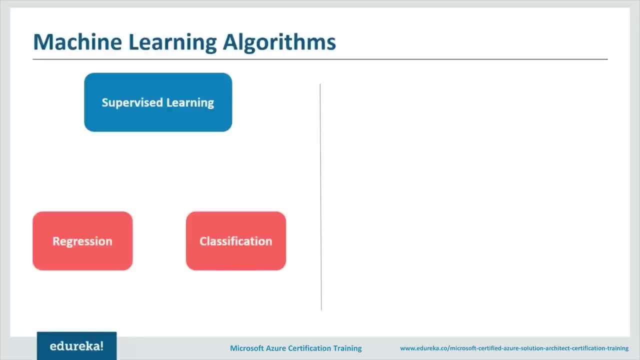 If you talk about regression, it is a process where you try to find out relationship between two or more variables. Suppose I have to detect as in: if I smoke would I be having cancer or what is the probability of me having a cancer now this is an example of regression. 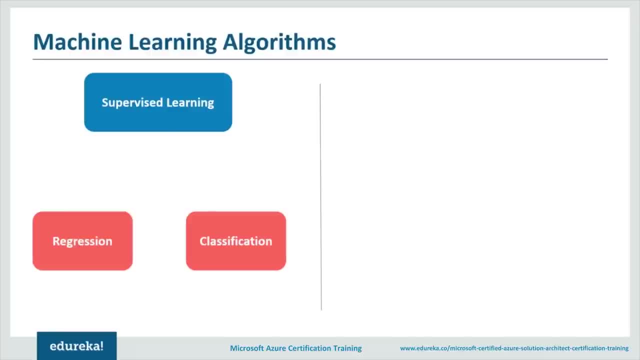 because I'm trying to compare cancer with smoking, right? So I'm trying to find out a relationship between these two. So these kind of algorithms are called as your regression algorithms, and then you have something called as classification. Now, in classification, you basically classify your data into groups. consider this example: 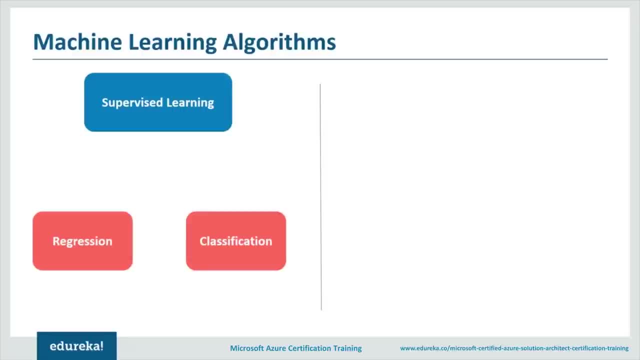 I need to classify my particular data set or information into different segregations or into different parts like male population, female population and all those kind of stuff. So these kind of algorithms are called as classification algorithms, And if you talk about regression and classification, you have quite a few advanced algorithms as well. 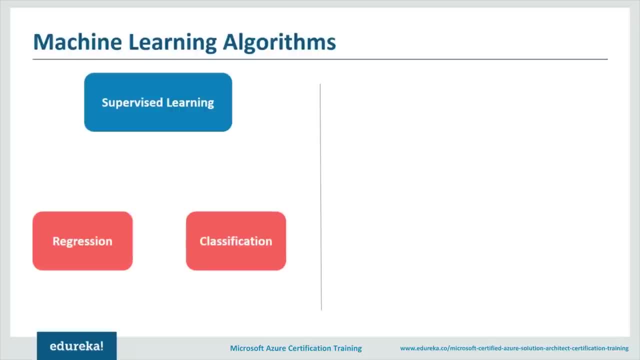 Say, for example, you have random boost, XG boost, and these kind of algorithms are not random boost or a random forests. So you have these kind of algorithms which are advanced level algorithms. Now we won't be getting into the details of those algorithms. 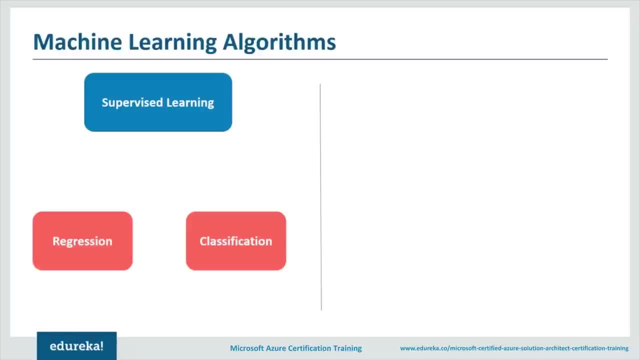 but those are important as well. So once you are thorough with what regression is, what classification is, I would suggest that you do go ahead and explore those algorithms as well. moving further and talking about unsupervised learning, We have algorithms like clustering. the example which I gave you in the unsupervised learning slide was: 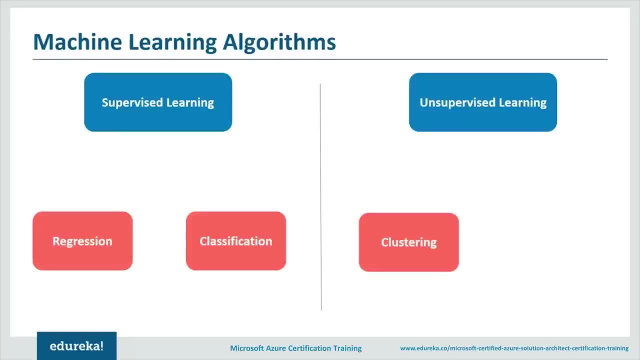 of clustering. So that is one method or one type of algorithm that unsupervised learning supports. Then you have something called as Association. Now we all go to supermarkets, right, We buy stuff. probably we go to buy some breakfast stuff. in that case you would be buying breads, butter, maybe milk, right, 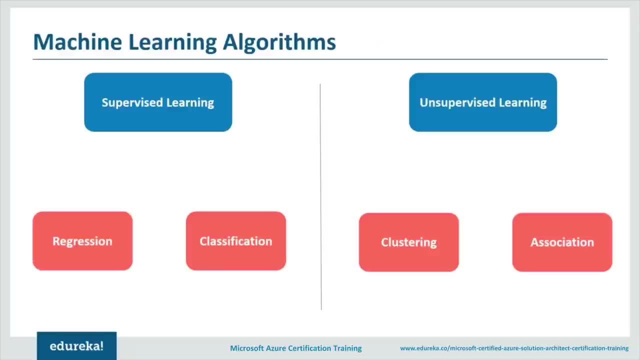 So what shopkeepers do is, or what supermarkets do is then normally place in products That people might buy in bunches or in groups, and this kind of process is called as collaborative filtering, or implementing Association laws, rather. So what these Association algorithms do is they help you predict. 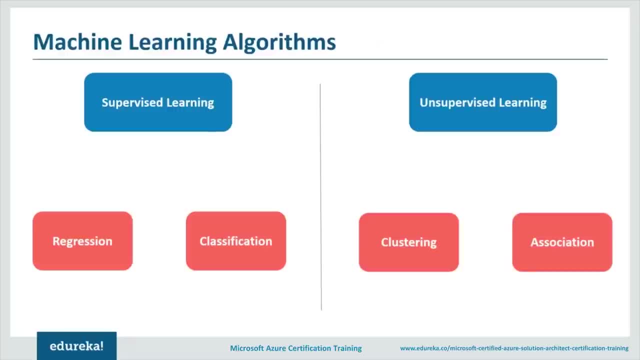 as in what is the probability of people buying certain products combined with other products, because it is understandable for people who are buying breakfast up. there is more probability that if you buy milk, you would be buying bread with it as well. So, yes, this is something that falls under Association. 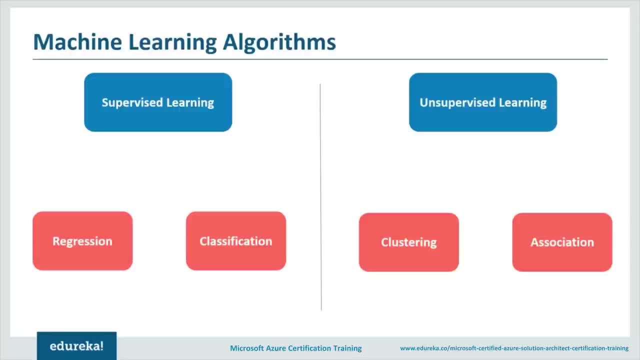 and Association laws, but that is a topic for some other time. I just wanted you to give you an introduction of what supervised learning is and what unsupervised learning is. I believe the idea is clear now, So let's move further and talk about something else. 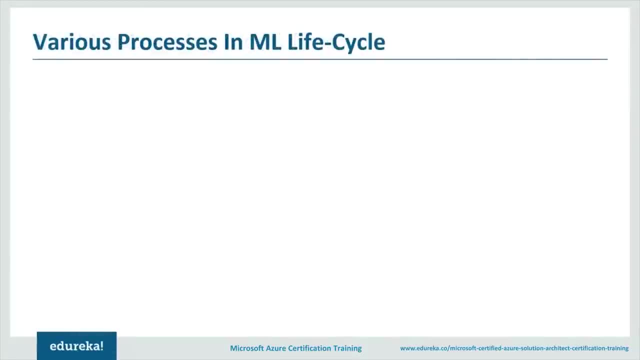 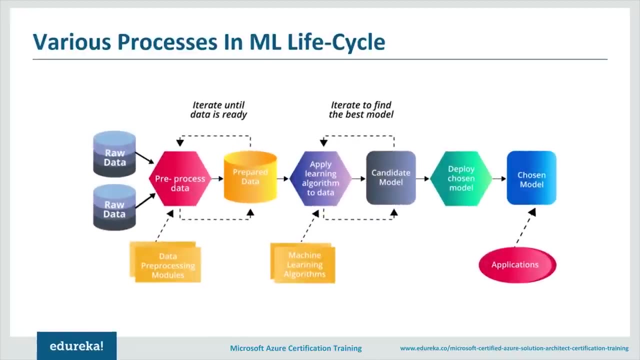 Yeah, So now we've talked about what machine learning is and what different kind of machine learning algorithms that are there. now I would like to brief you through the process of how machine learning works actually- and this is pretty much common for most of the algorithms- 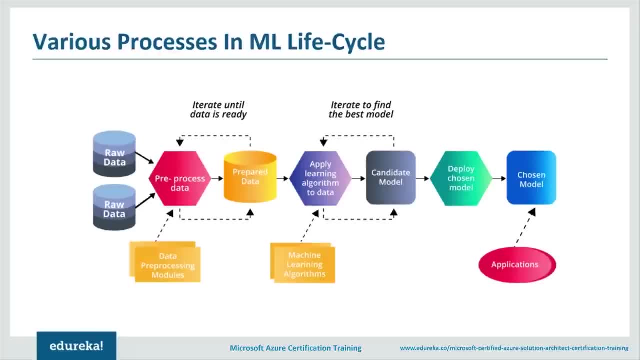 that you're going to implement. first and foremost, You would be needing data. Now, I've already talked about the point that data is centric to machine learning. If you do not have data, you cannot make any predictions, and more the data, the better it is for you. 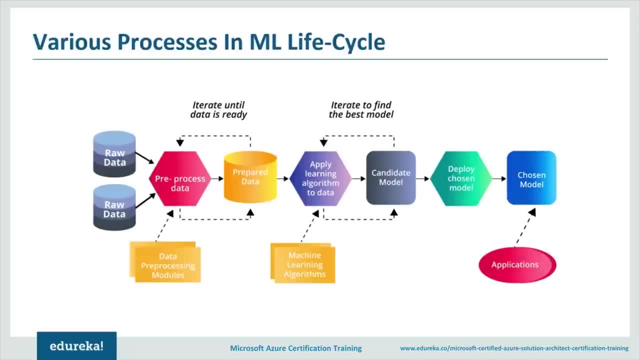 So the first part is having data and once you have the data, the next point you need to confirm or make sure is the data is appropriate for machine learning, and this is where pre-processing steps and what pre-processing does is it helps you process the data that you have and prepare it for machine learning. 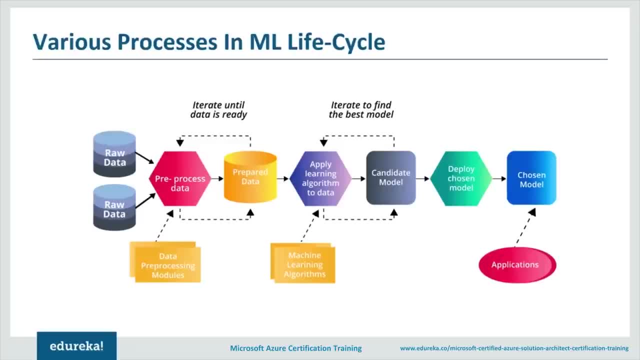 I mean your data might not always be clean. There might be some missing values, some repetitive values which you do not want in your data when it is getting processed right. So in this case, we filter out this data, We clean it, we fill in certain values. 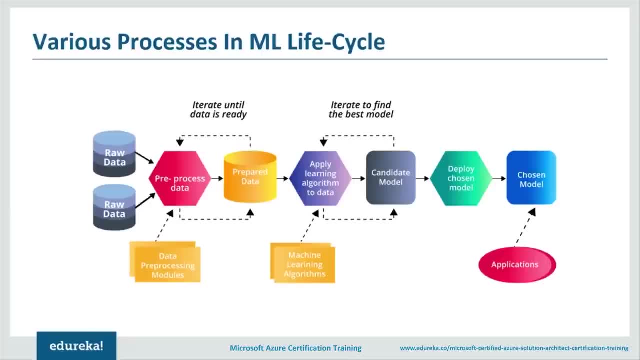 We predict certain values and we put in those values there, and once this data is up and ready for working, then we pass it on further and then we provide a particular machine learning algorithm to it. this again is a trial and error kind of method where it seems simple at times. 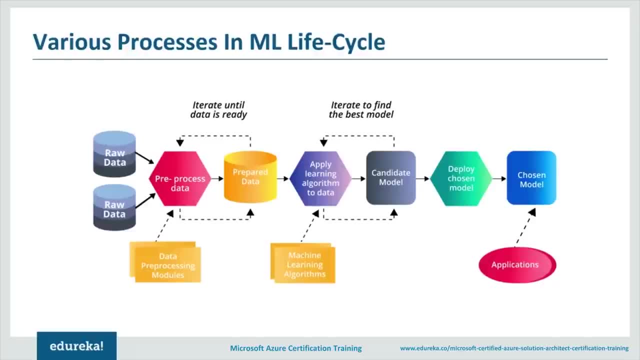 because we have discussed all those machine learning algorithms, right. So to naked eye or to naked man, basically, we might think in this direction where we would think that, okay, this is the kind of problem I'm dealing with, So this is the algorithm I might use. 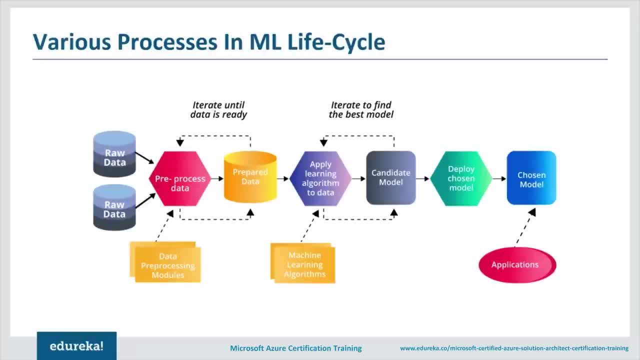 but that is not the case. at times, The data is misleading. We are not sure what kind of algorithm I want to use, what kind of data I want to pass and how much data I want to pass. in that case, What we do is we first a lot of particular algorithm, use it. 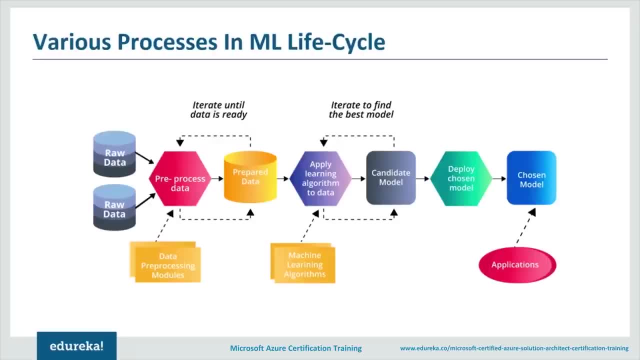 implemented, then we test the values, then we try out some other algorithms as well, and then we come to a conclusion as an: okay, This is the best algorithm and using which I have generated a model which is best to meet my needs, and while doing that, there are quite a few processes. 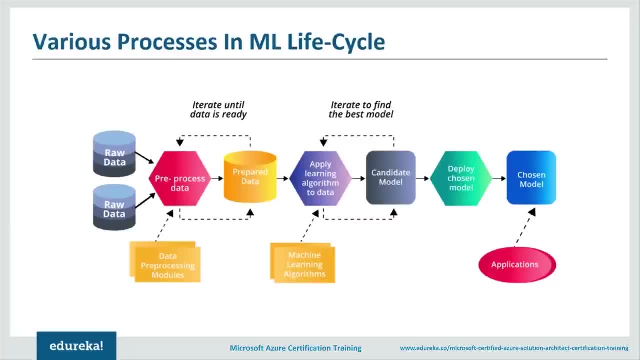 that happen. processes like training, testing, validating, where you pass certain, certain amount of data. you build the model, you train the model and then again you pass or keep some data behind which you later pass to test these models as in are they working properly or not. So this is an iterative process. 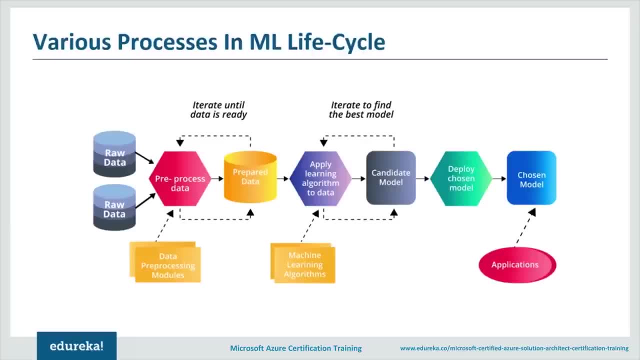 and this might take in more than one iterations to actually go ahead and jot down or settle down on to a particular point. So once your algorithm is selected, once your machine learning model is built, you can actually go ahead and deploy this model into your environment. 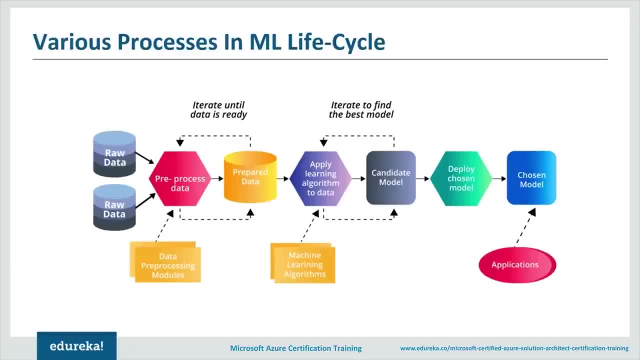 or real-time working, where it would be able to predict the real-time data or the data you provide to your so-called algorithm, right? So this is how the whole process of machine learning works. Now the processes which I talked about: pre-processing, then implementing various algorithms, training, testing. 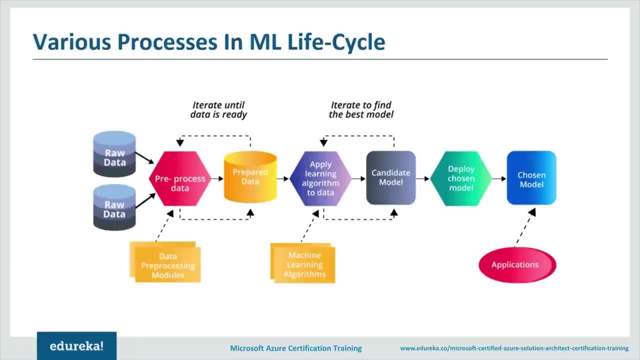 your data. now this again. they look simple or when you listen to them they seem pretty easy, as in training the data and all those things. But once you start implementing these things, it is fairly difficult. ask any data scientist and that person would tell you. 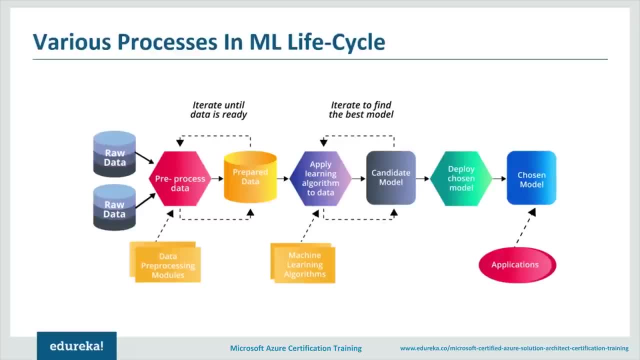 that pre-processing is something that is very difficult to deal with, and mostly 60 to 70 percent of the work is done in these phases Only. so what if we had something that could actually help us here? Wouldn't that be easy? I mean, if we could just speed up this process. 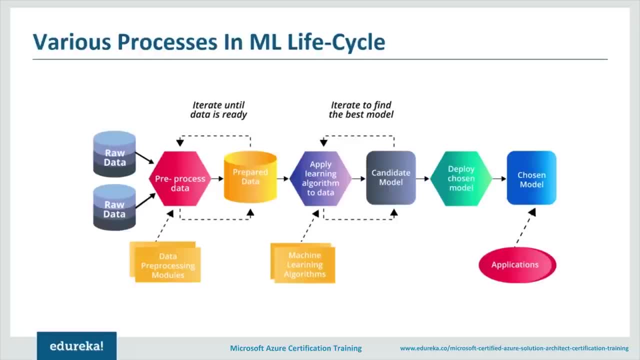 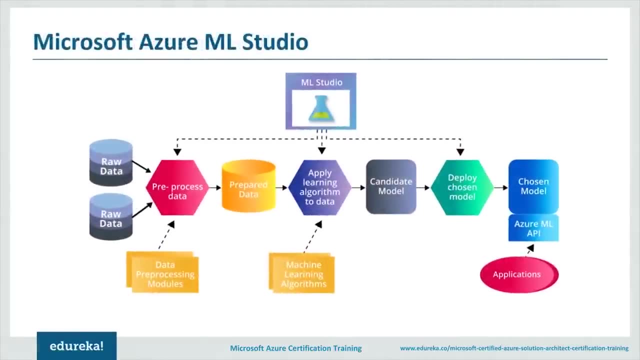 of pre-processing, algorithm selection, training and testing data, instead of doing these manually. can we do all these things automatically? The answer is yes. This is where your Azure machine learning steps in. what Azure machine learning does is it helps you carry out the whole process. 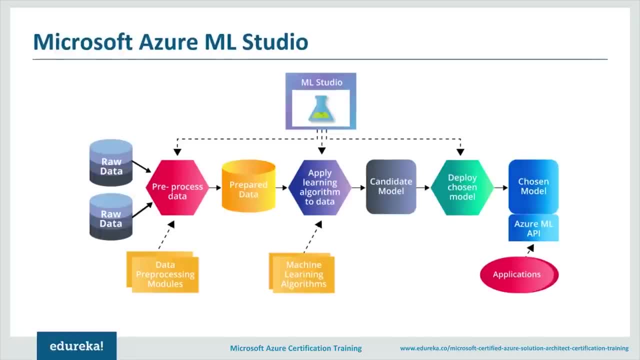 But, as you can see, we have something called as ML studio and it focuses on your pre-processing application of algorithms and deployment processes. So bulk of the task, where which can be repetitive or which can require you to put in more efforts to implement manually, It actually helps you automate or speed up that process. 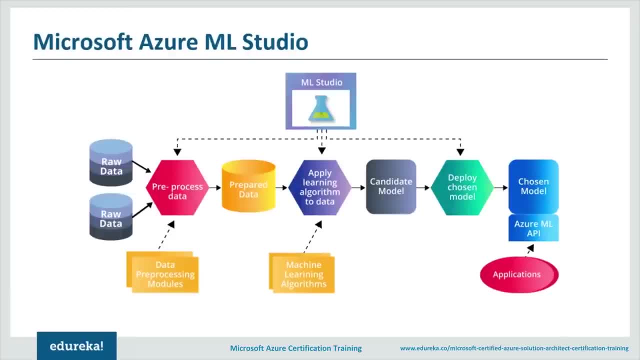 So that is what ML studio is basically. it is a studio or a service in a very popular cloud service provider that is Microsoft Azure, which lets you implement various machine learning algorithms, and it carries out the bulk of task or the bulk processes which you would otherwise not want to do now. 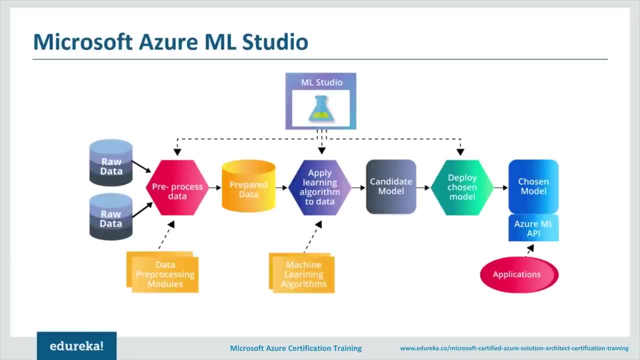 This is not something that actually is used to replace data scientists. You cannot do that, So no offense to any data centers. who is listening to this video or going through this video? It is more or less complimentary to data scientists. You would be needing statistical knowledge. 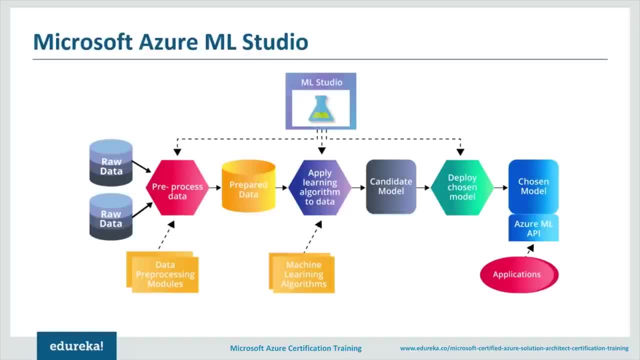 and hence we talked about machine learning a little, because, even if you build models using Azure or any platform, you would be required to have proper statistical acumen or knowledge about data science, something that would help you understand the output of the models that you've built. 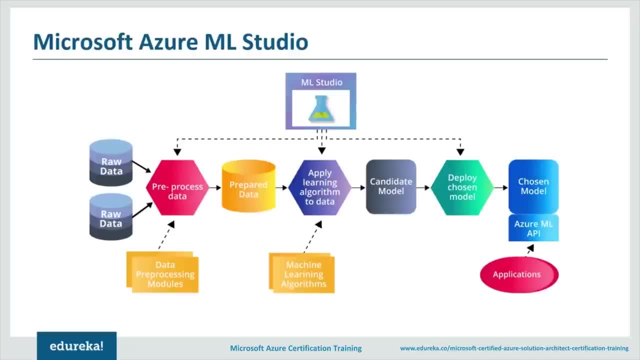 So, yes, some statistical knowledge would always help- and you cannot replace that, but definitely if you are working on machine learning and you need to speed up this process or make it more efficient than Microsoft Azure, and ML studio in particular, is a very important resource for you to have. 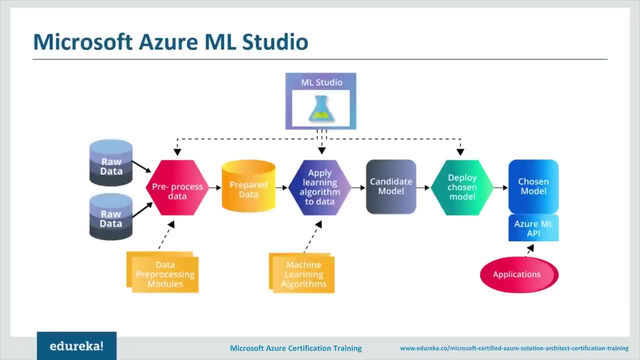 So what I'm going to do now is I'm going to switch into the demo part and we would be building a model so that we can discuss some of this stuff that I've already talked about and we also get to see how Microsoft Azure works in real time, right? 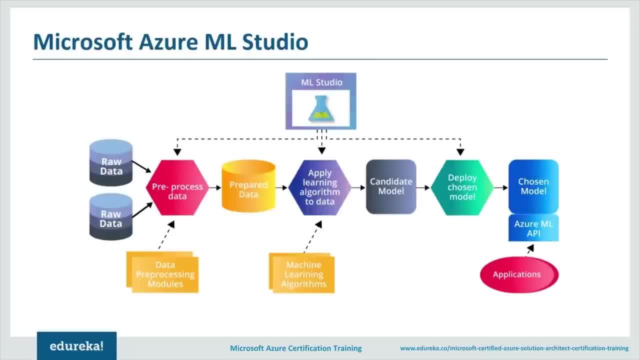 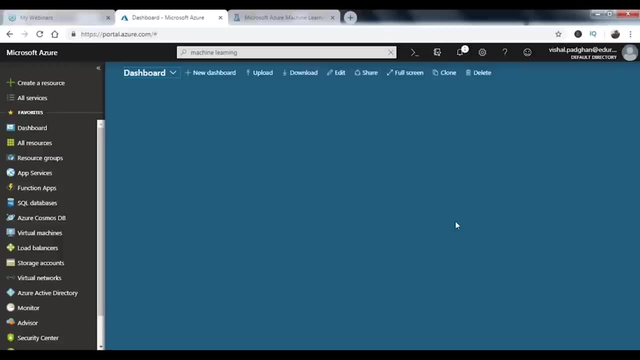 So let me just switch to the Azure portal or console that we have at our disposal. So, guys, what I've done is I've gone ahead and I've switched into my Microsoft Azure portal. for people who are completely new to Microsoft Azure, You can actually avail certain services. 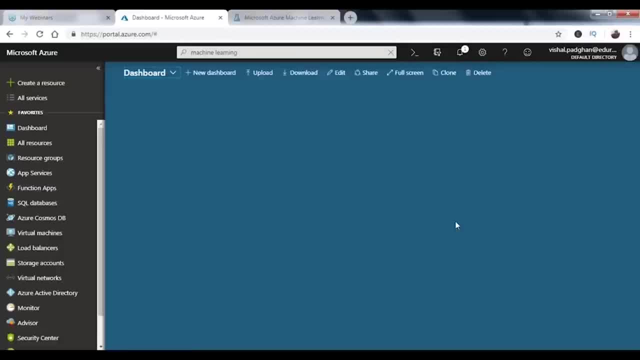 that Microsoft Azure offers you for free for one month Now. during this period, you can avail certain credit for US citizens or people who have an account in US region. They can actually available to $200 of usage where you can use certain services. Now these services are chargeable. 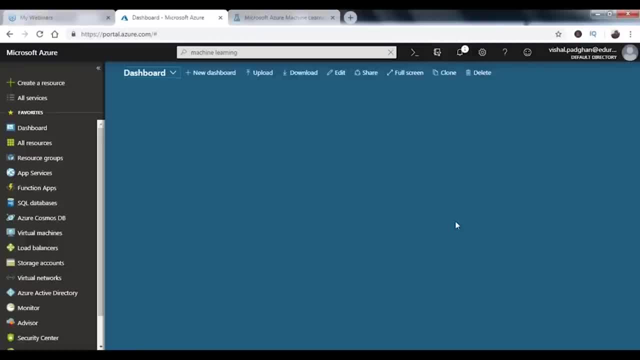 That is why the free credit that is made available to you, So which I believe is more than enough for one month's practice- So if you're somebody who's new to these platforms out says- is that you go through or sign up for Microsoft Azure. 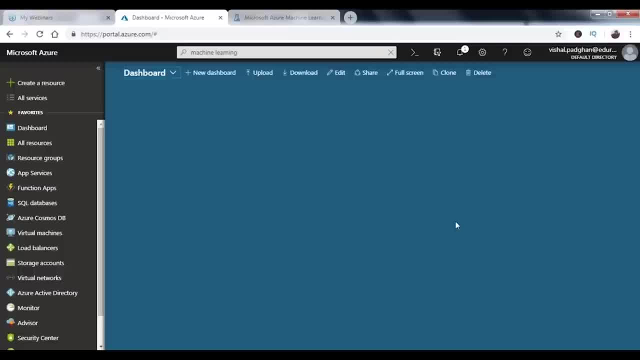 and you can avail those services now, since I am from India, We have Indian rupees as our currency and for our usage We are given somewhere around 13,300 INR or Indian rupees, which is a very big amount if you talk. 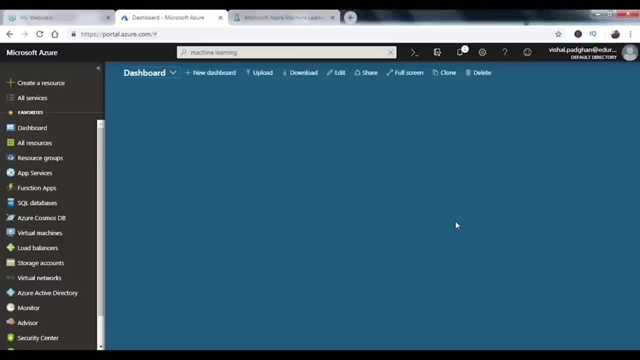 about using a service for a month's time, So it actually serves my purpose. I have been using it for a long time. That is this particular account. I've had a couple of accounts, but this one is something I created some 15 days back. 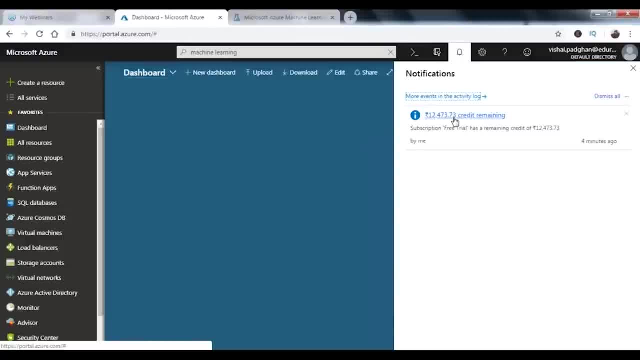 And, as you can see, I still have like 12,400 something, something which I can use, and we would be not needing this much today, somewhere Maybe 10, 20 rupees to the max. So, yes, you can go ahead and create this account. 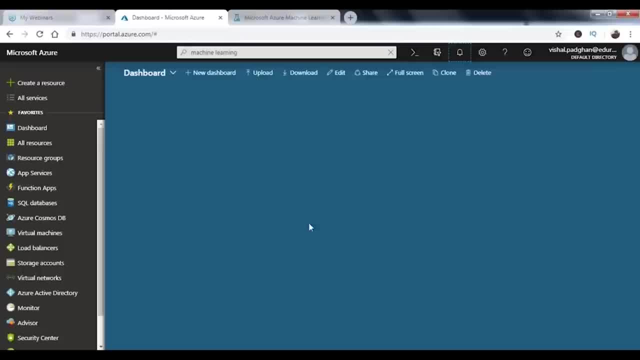 Once you do have this account, then you'd be having access to all the services that Microsoft Azure has to offer to you. You can go ahead and create all the resources you can have or utilize its compute services, database services and all the services that it has to provide to you. 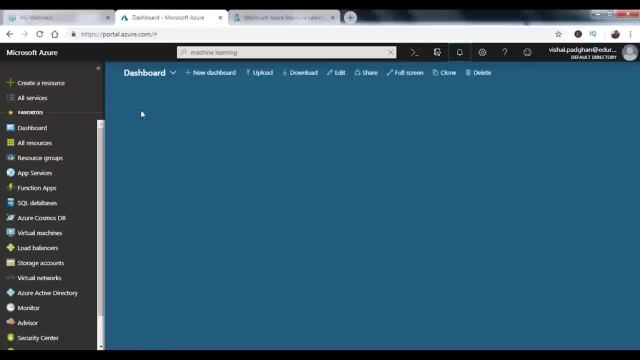 But since we are talking about machine learning, we would be sticking to those applications as well. So, in order to use your Azure machine learning, you need to create a workspace where you can actually go ahead and put in all your data. And once you create your workspace, 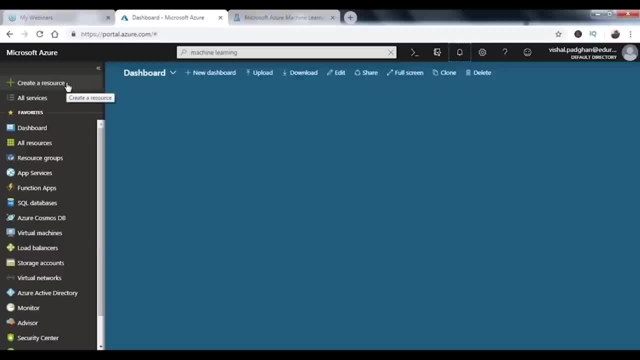 you actually need to go ahead and sign into the Microsoft Azure ML studio, which is an interface or IDE where you can actually go ahead and create all those models. So, in order to go ahead and create a workspace, you just need to come here and type machine learning. 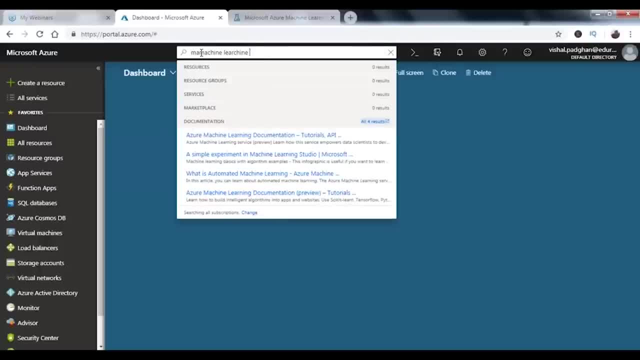 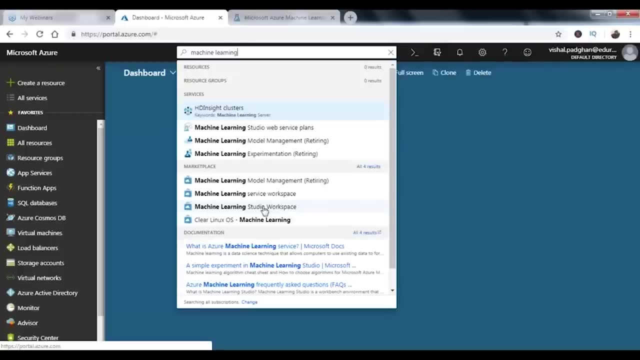 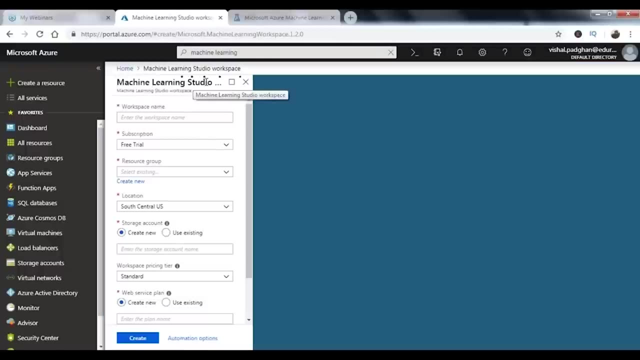 and you might be having that thing. in the suggestion It was already typed, I believe, machine learning- and you have this place where it says machine learning, studio workspace or service workspace. You can click on these. the studio workspace is something I've clicked on and you need to put in some details. 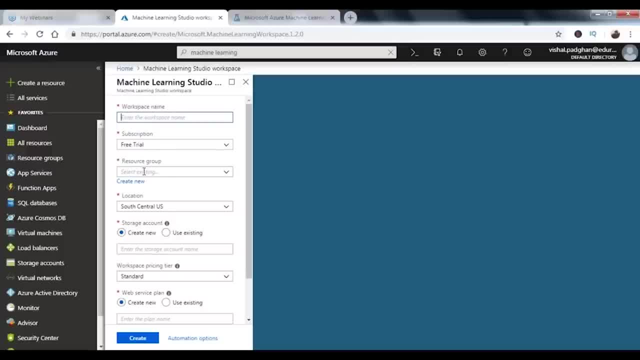 as in: what is the name of your workspace? What subscription are you using? resource group: You can use the one If you already have one. if not, you can create one, just given some name. Our resource group is something that holds in details. 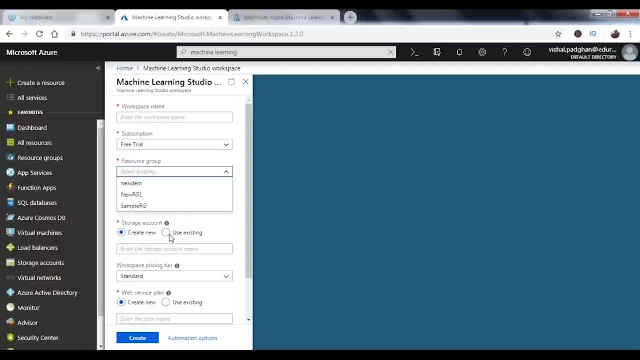 about your resources that you're using and then what kind of storage account you are using. You can create a storage account as well. It's not a big deal, It is nothing, but think of it as a storage place where you can store in your data. 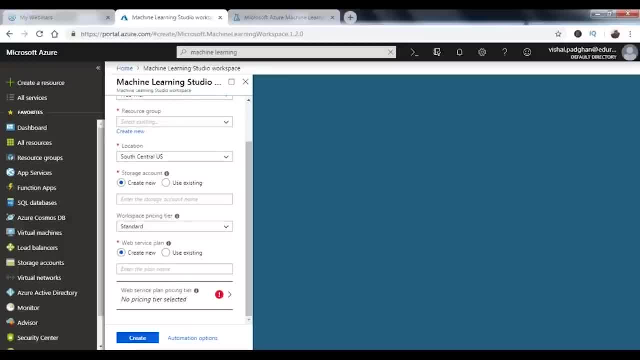 That's it. So you do go ahead and put in these details and then you say create. before that, you have to put in what pricing tier are you using, and you'd be entering the region where you want your workspace to reside. Now, what cloud does is: 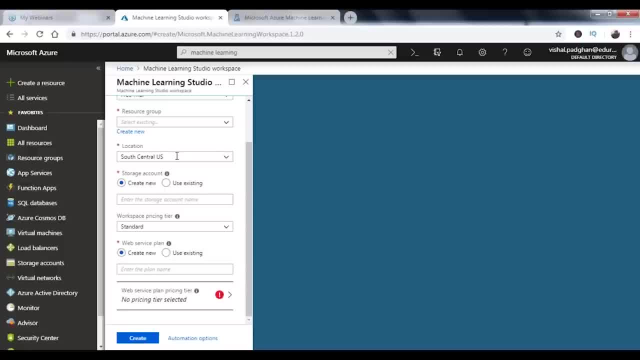 it stores a data in particular locations on the globe, right, So you can choose the location that is closer to you or closer to your business, depending upon your needs. for now, I'm going to stick to the basic one that is here, because we are just creating a simple demo. 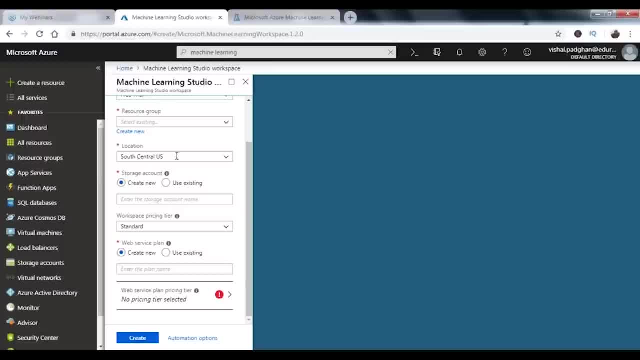 In fact, I'm not going to go ahead and create a workspace because I already have my own workspace, but you, I would suggest that you put in these details and create one. once this workspace is created, You can actually just open it and at the bottom you would be seeing an option called. 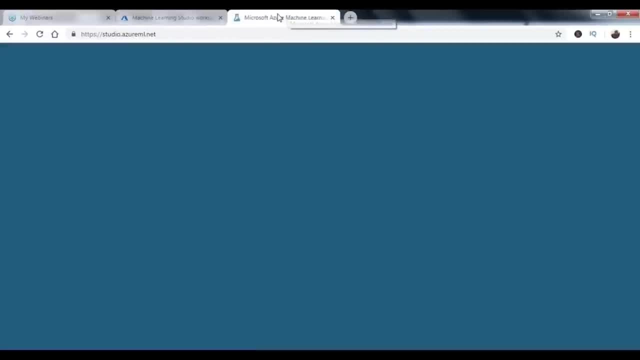 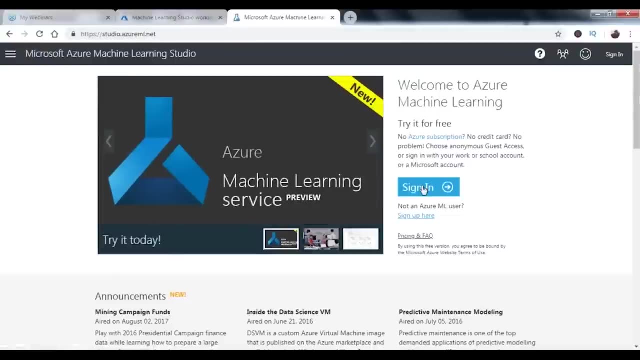 as machine learning studio. else, What you can do is you can type in this URL and you would be redirected to this page where you have to sign in with your Microsoft Azure portal account, and once you do that, you would be redirected to the ML studio that I'm talking about. 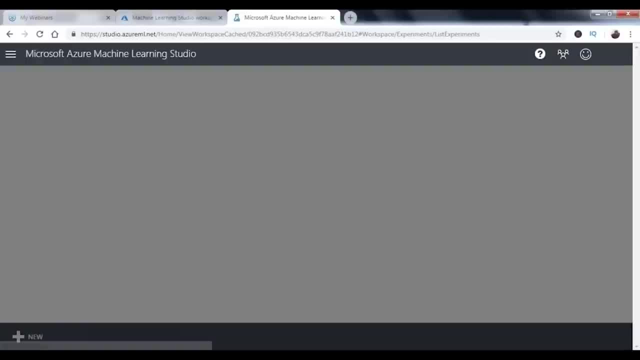 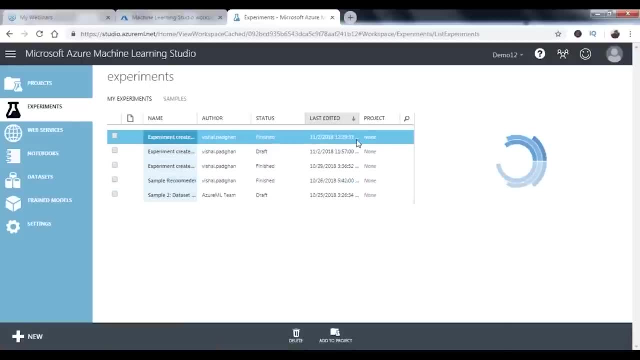 So the workspace would be created. once the workspace is there, you log into your Azure ML studio, And once you do that, this is what you'd be having at your disposal Now. these are some of the experiments that I might have worked out or worked on in last week or so. 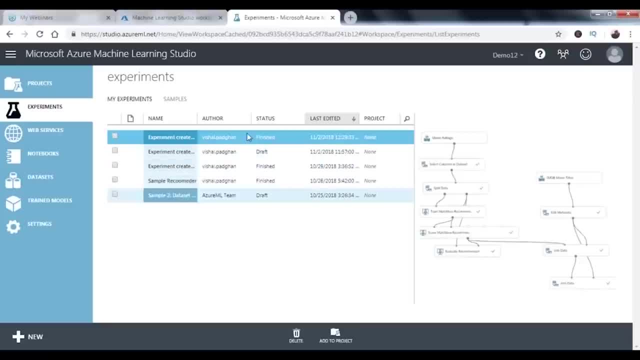 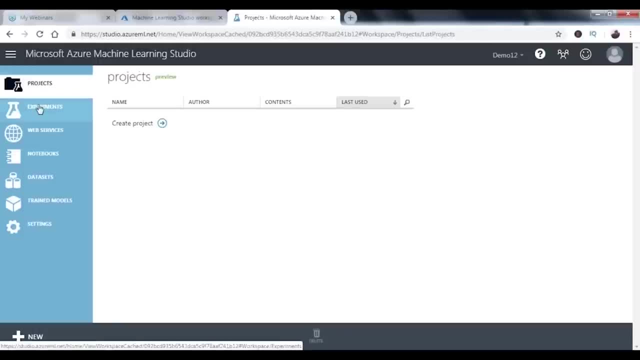 Some of them are finished, some are still in drafts, So you can actually go ahead and create these workflows. are these kind of workflows? Now you have so many options here? What are the projects that you create? experiments, which we just saw, different web services. 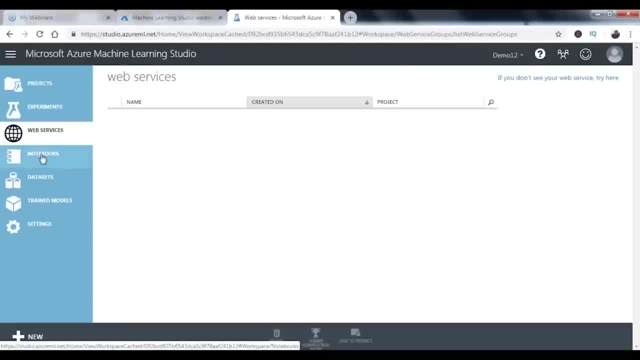 that are made available to you. You can actually go ahead and create web services as well. You have your notebooks now. you might not always go ahead and start from the scratch right. You might have your code written in maybe our or some other language like Python. 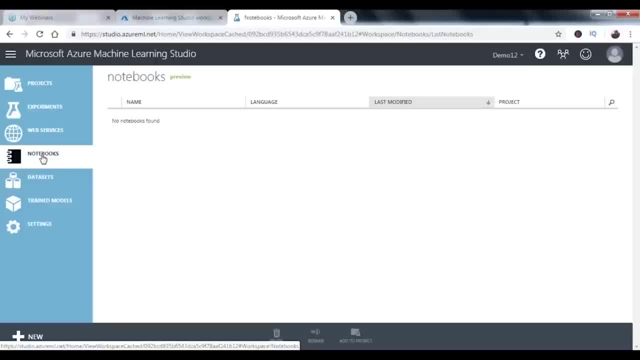 So you want to import that code? you can do that as well, or you can use the existing notebooks with Microsoft Azure has offered to you where you have ready to use codes or ready to use models as well, And then we have data sets. now again. 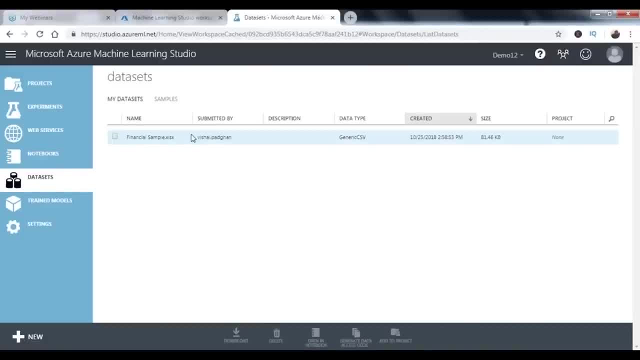 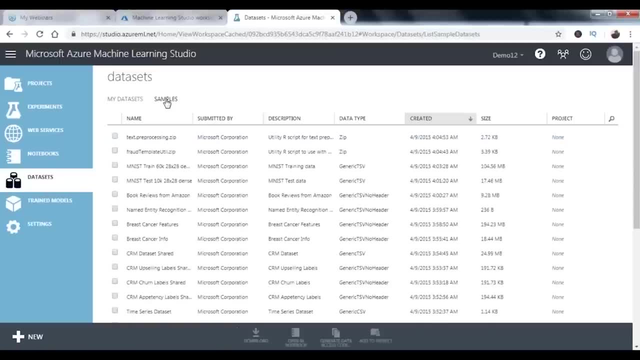 you can import your data sets that you have. There was one financial sample data set which I imported recently. You can actually go ahead and use sample data sets as well. Now you can see there are quite a few data sets that are made available here. 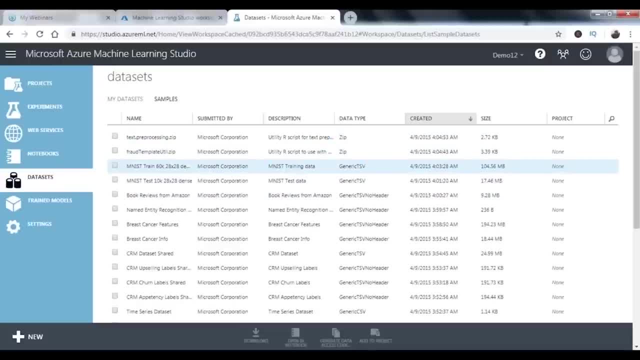 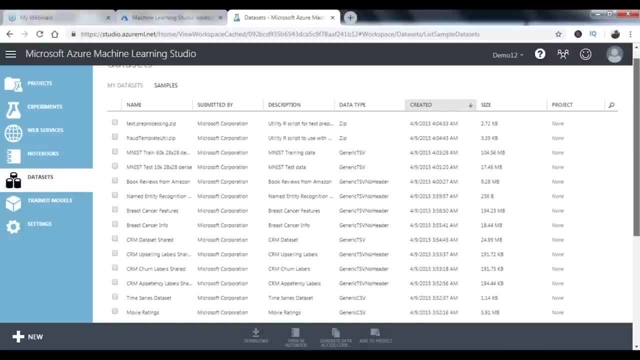 which you can use and implement your own algorithms or implement the algorithms that Microsoft Azure has to offer to you, right? So you can do that as well. So it pretty much depends upon what do you want to do And what kind of processing do you want to do. as you can see, 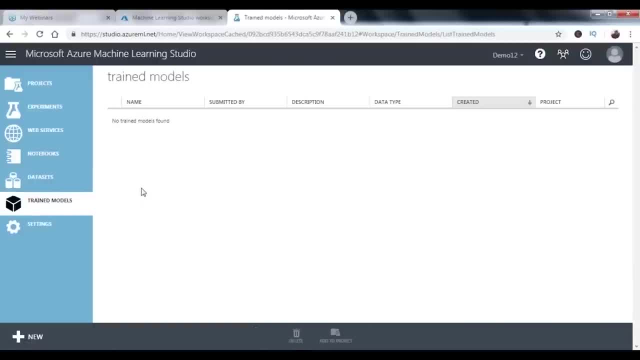 if you come here, you have some. this is somewhere you can see your train models, as well as in the work you've done or some models that you've implemented, So you can have that here. in this case, We are going to go ahead and implement one of the algorithms. 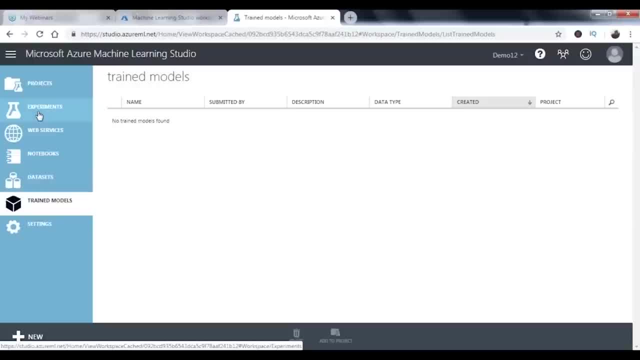 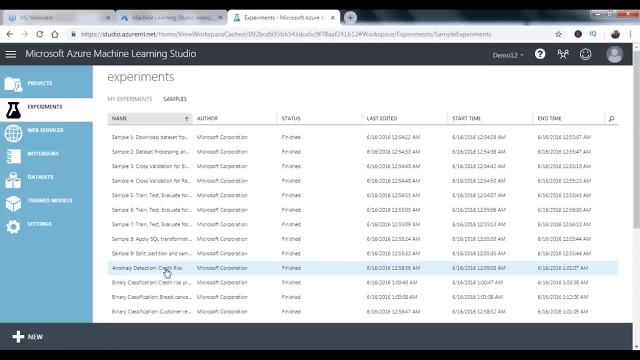 or algorithms that are implemented by Microsoft Azure. So if I come here to experiment and I go to samples, you can see that we have so many implementations. So we would be taking a look at one of these and then we would be implementing that on our own, do not worry. 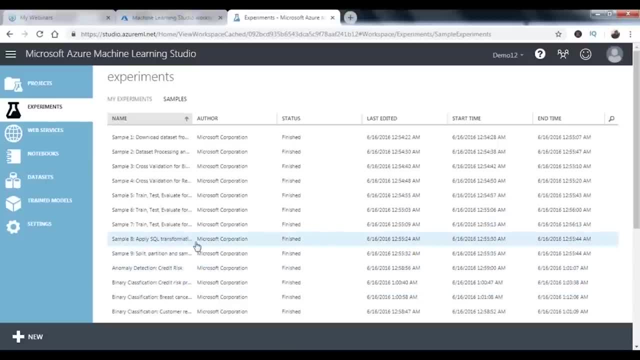 We won't be copying it right away, So we have quite a few options here, as you can see. Okay, let's just go ahead and do one thing. Let's build our own model here. So for that we need to go to experiments. 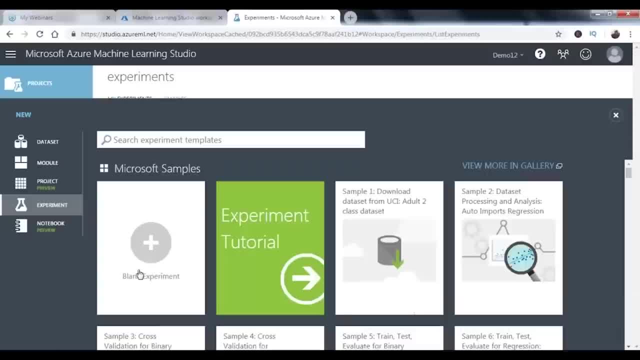 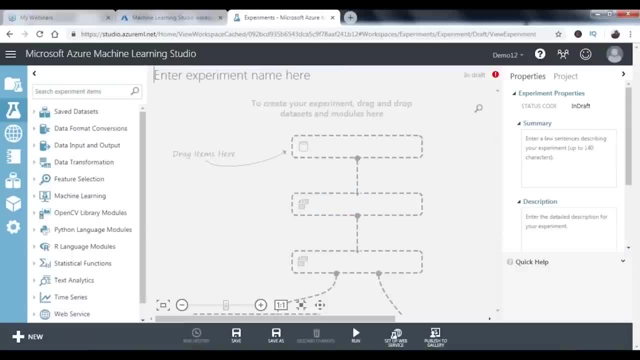 or rather we can come down here and say new and I say: add a blank experiment. Let's just go ahead and try to build a recommender system or something like that. So to do that, let's call it, say my recommender. There you go and save it. 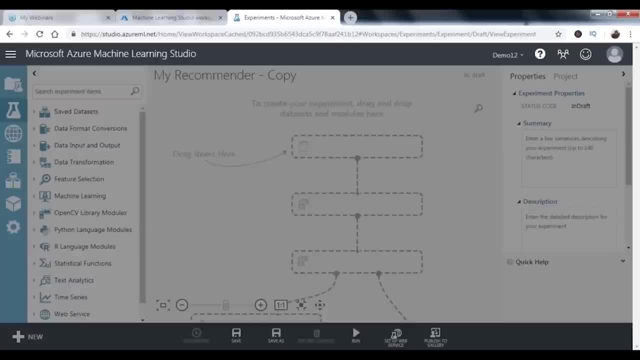 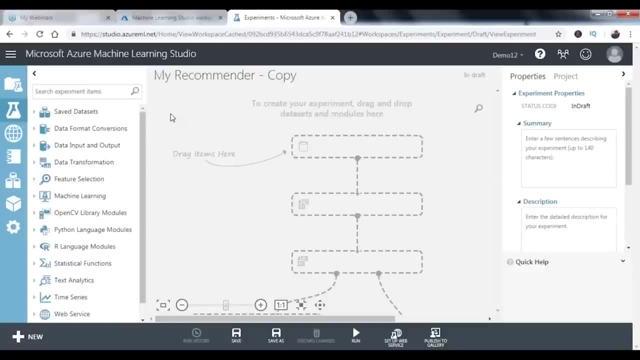 There are no models, so you cannot save it. So first, let's get started now, in order to create a recommender for people who do not know what a recommender is. It is nothing, but you pass in certain data and it might suggest, or the model might suggest you. 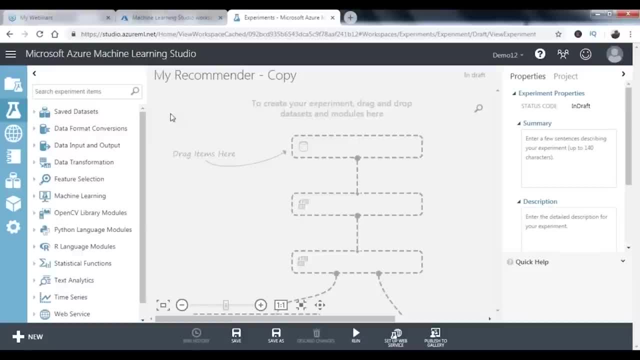 as in what you might like or what you might want to do. Say, for example, when you shop on Amazon or any other website that is there, you normally have some suggestions, right? I mean, you may like this, you may like that same. as with YouTube. 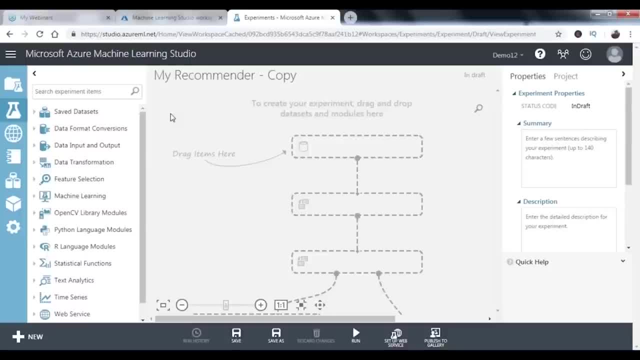 you go through certain videos and it gives you suggestions as in: you preferably might like these videos as well. So that is a recommender system. So let's go ahead and create one recommender system. Let's create one for movies. So let's just go ahead and practice or play. 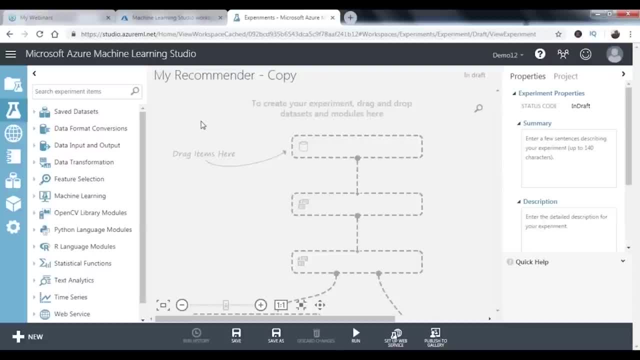 with the data that we have. for that, We would be needing a data set first. right now, if you talk about ML studio, it is very simple. You just drag and drop stuff, just like creating workflows. It is as simple as that. now, in order to use a particular data set, 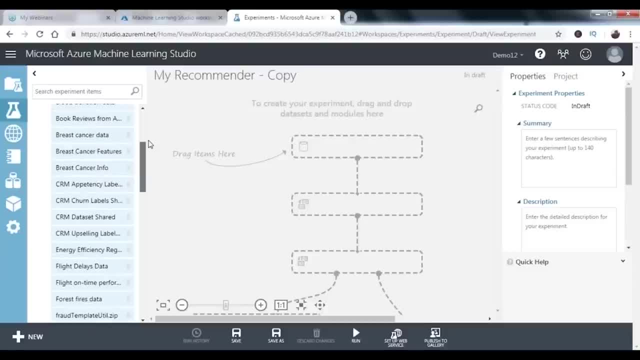 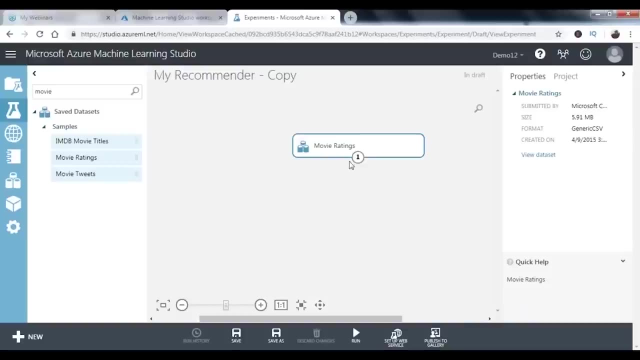 We have these saved data sets here, samples. Let's make a recommender. systems for movie, movies, movie, Yep, So movies. do I have something in movie? Yeah, there you go. movie ratings. So we would be using this data set. now, Once you put in this data set, it is available. 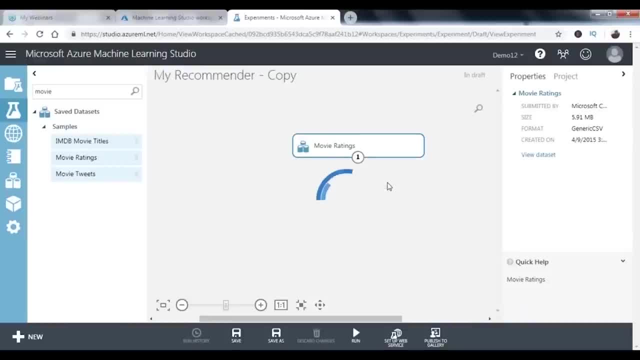 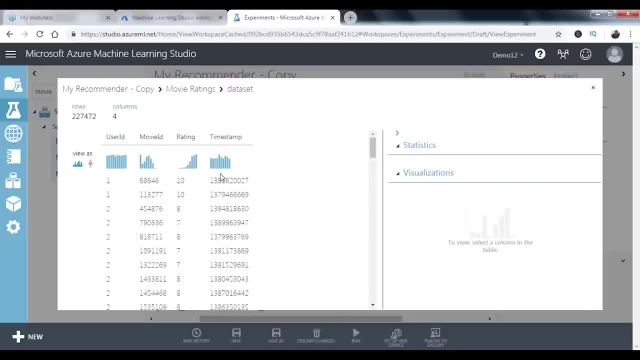 You can just go ahead and take a look at it. So let's just visualize this data And, as you can see, the information is here. It has certain values like user ID, movie ID, ratings and timestamp. timestamp is something that people do not use frequently. 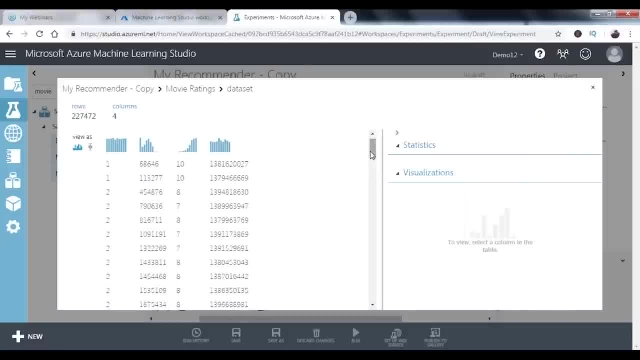 But yeah, these are things that are important to us. We have factors like your ID, that is, your movie ID, user ID and rating. It's somewhere around up to 10.. So I believe it has started from 0 or 1 maybe. so we have ratings from 1 to 10, which we would be using. 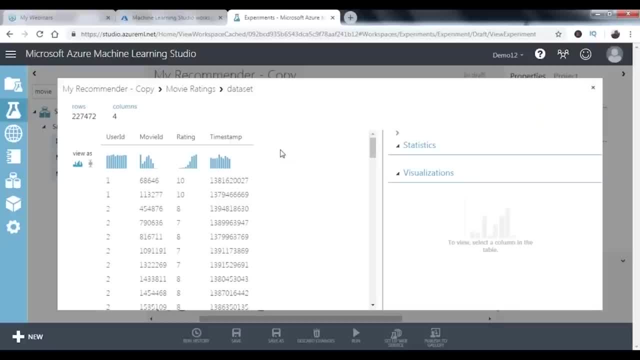 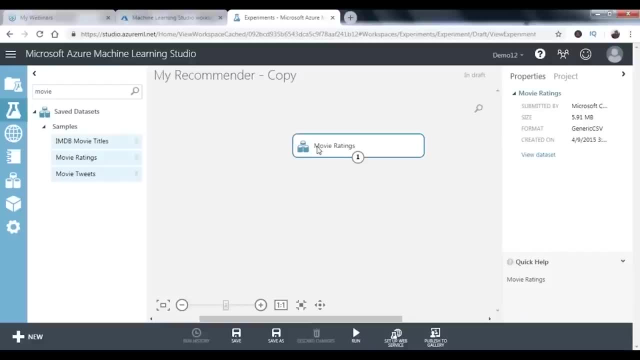 So this is the data that we've just visualized, but at times this data is not as simple and as managed. It might have some missing values and you might be required to play with it or make some changes to it. You can actually go ahead and put in some factors here as well. 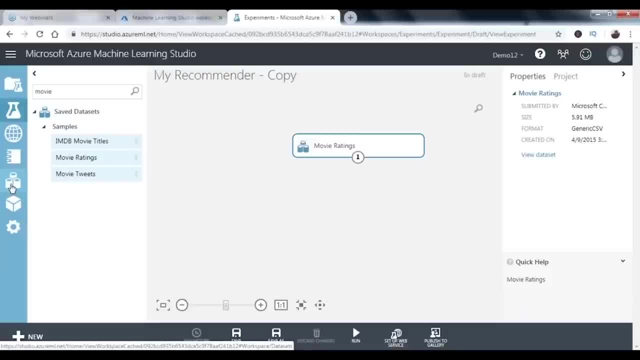 Now, here you have so many options that are made available to you, right? So you can actually go ahead and process your data a little, manipulate your data little like. you can take a look at Statistical analysis and all those things, but this, being a clean data, will not need to do that. 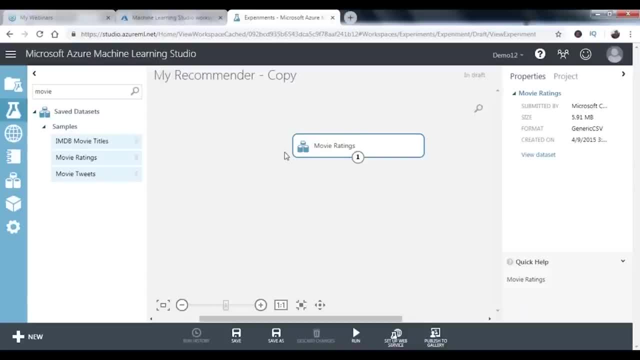 So we're just going to stick to the recommender system part here. So we have the data set. now I need to select the columns that I want to use, So I'm going to project certain columns out of it. So for that we have a module here called as project columns. 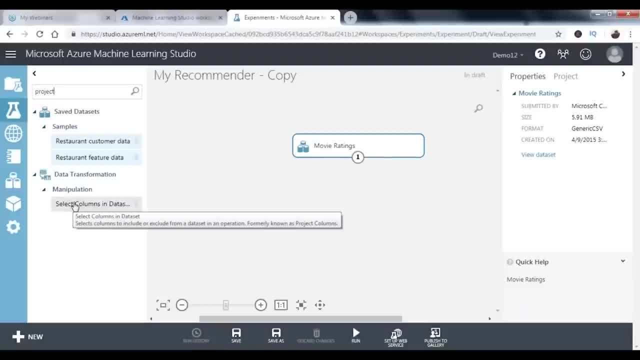 Okay, I don't see it here. I believe they've changed the name: select columns. Okay, So this is the one. they've changed the name. It's called a select columns in data set, So we drag it and paste it here and we hold on to the circle that is there on the previous module. 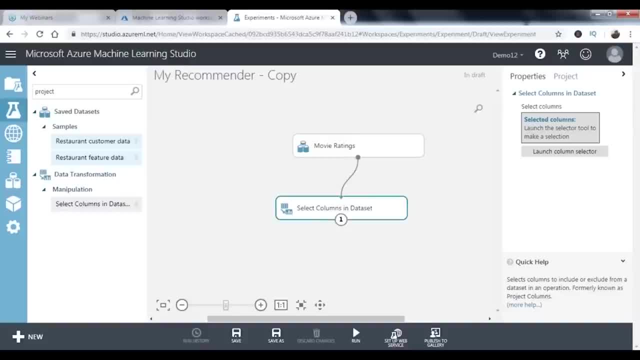 or the tab we had, and we pull it down so we can connect these two and they are connected and but since I've connected them, there's an error here. It says value required. now I need to pass in some values, as in what are the columns I need to focus on right. 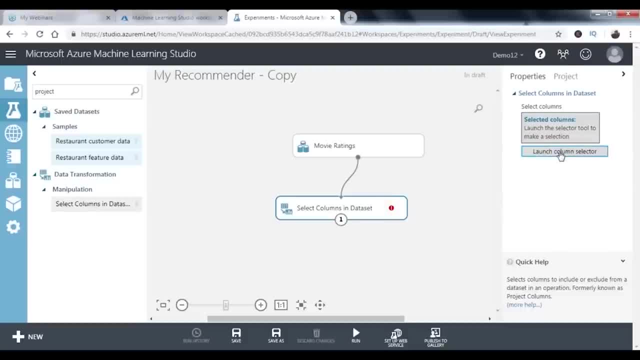 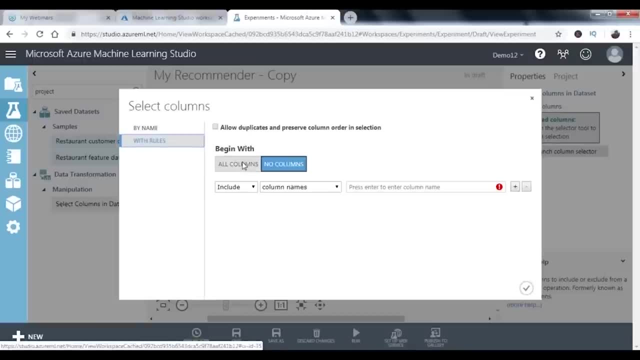 So I would be clicking on this icon here or tab which says launch column selector, and it gives me options. So I'm going to put in certain rules. Now, what are the columns that I want? first, I would say that get in all columns. 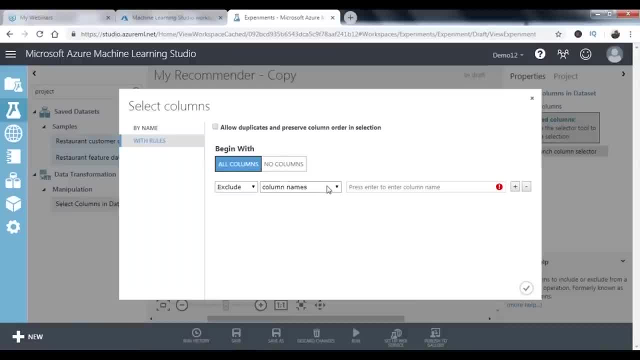 and just exclude the ones that I don't want. So what are the columns that are not on timestamp? for something that won't be very handy. So I'm going to remove that. so I would be excluding that and I would be seeing. okay, Once you do that, the error is gone. 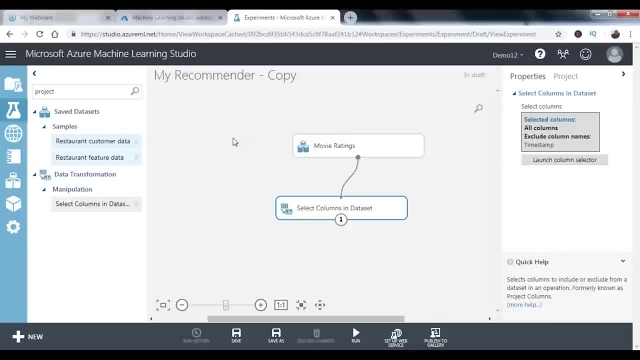 So we have the data set, we've selected the columns. now next phases. I need to go ahead and pre-process the data, but data is already pre-processed So I don't need to do that either. So in this case I would be going ahead. 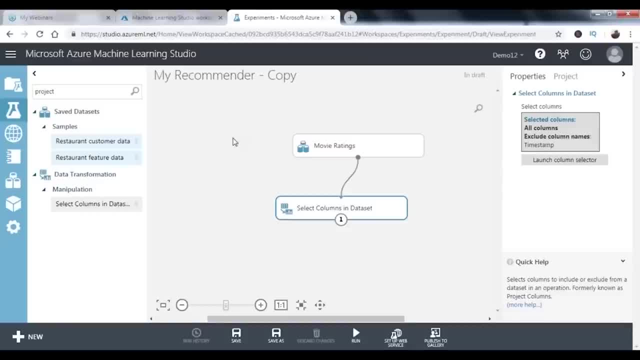 and splitting my data into two parts: my training data and my testing data. training data is something that we would be passing on to the model and we would be training a model based on the data, and test data is something that we would be holding back and then we would be using that testing data. 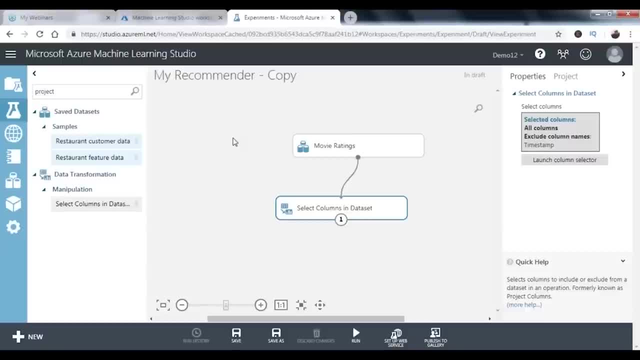 to test our models, or to predict the outcome, or to see whether the model is working fine or not. So to do that, we need to split our data. So come here. this process is easy. Just go ahead and type in the words that you need to do. 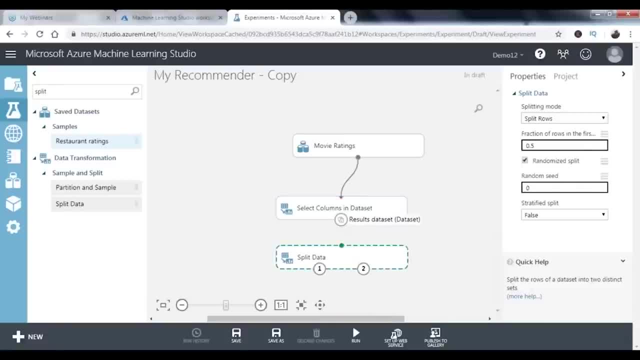 and it gives you modules to do that. So, split data: I just passing the data, So I've gone ahead and I've created or I've pulled this split data module or tab into my workflow. So, yes, the data would be split and it would be split in this fraction, 0.5.. 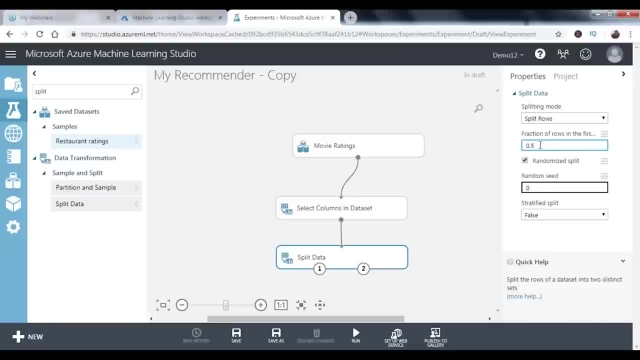 That is, we would be using 0.5 percent data to test. that is half of the data to test and half of the data to train our models. So there you go. I won't be tinkering with these factors. Those are good enough for me. 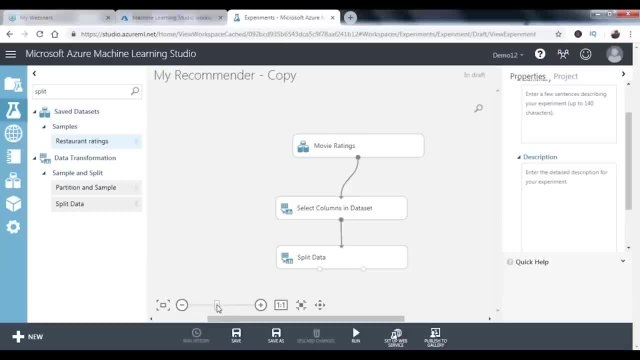 So let's just move further. now There's an option here where you can zoom in or zoom out your model to fit in the screen. So the data is split. now next job is to train your data, So train your recommender system. Do we have option to? yeah, 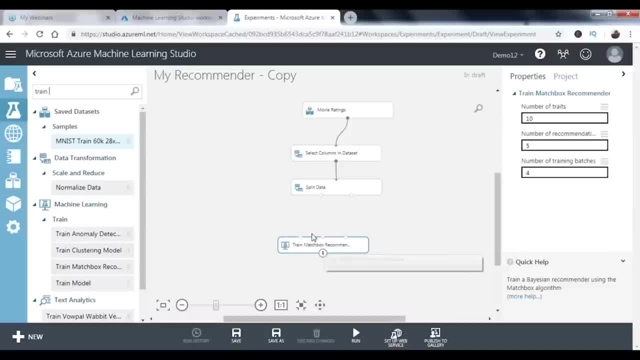 train matchbox recommender. So we select this and pull it here. Now what we do is we pass in one of these branches here, First one, and the split data is passed on to this training module or tab. Now, I'm not too good with the nomenclature. 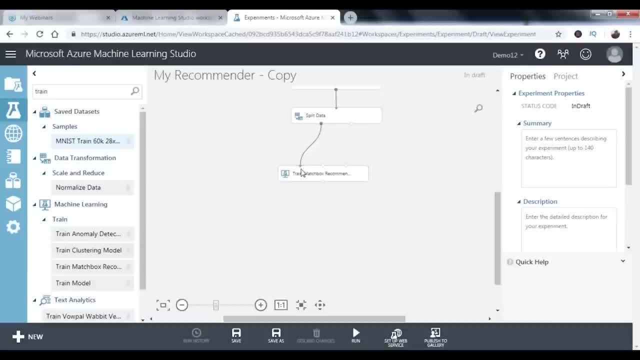 That is why this confusion. let's call it tab. So yes, so I've pulled in this data into the tab. So this is something that would get trained here, and I need to score it as well. So once I come here, I select this first and it shows me the details as an okay. 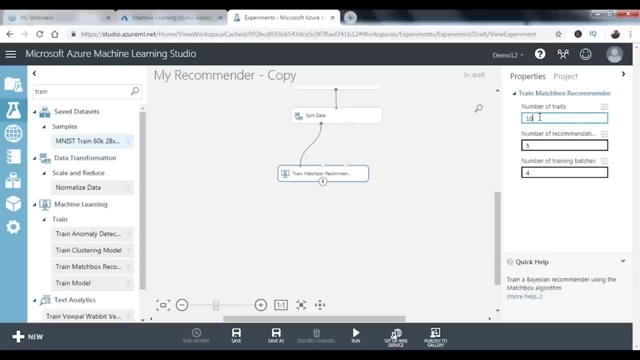 how many traits of the data that I have that I want to use to build this recommender system. Let's just say 10.. Okay, 10 is fine. I don't see too many problems with it. Maybe let's do it 20. number of recommendations. 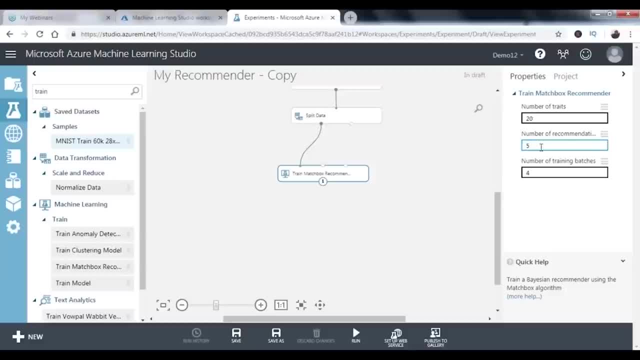 I want to know. this can also stay to five, No problem, training batches for is fine. So we just move further. and next what we do is we just go ahead and score the data that we have. So I say score and I pick in this thing. 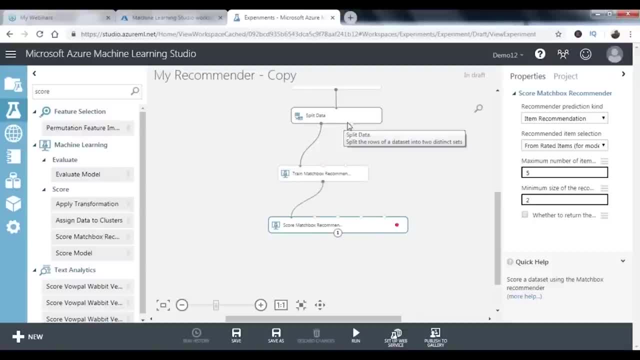 So, again to this, I would be passing in my training data here and I would also be passing in my split data. that is, the testing data. There you go. So the data that has been trained, that would come here and also the testing data would be here. 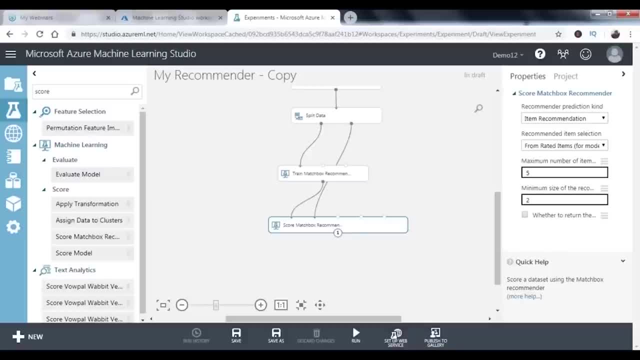 So I have this score where I need to give in the details, as in: what are the predictions that I'm looking for now? I basically want prediction where I would be wanting related items, right? If I watch this movie, what kind of movie I need to watch, right? 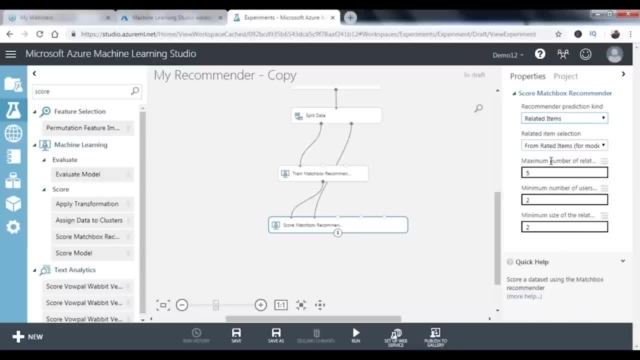 So this is what I would be entering here. So once I enter related items, it says: what are the maximum number of related items to find from an item that you have? Let's say, I want just one item. There you go, And so it would give me one related item to the movie. 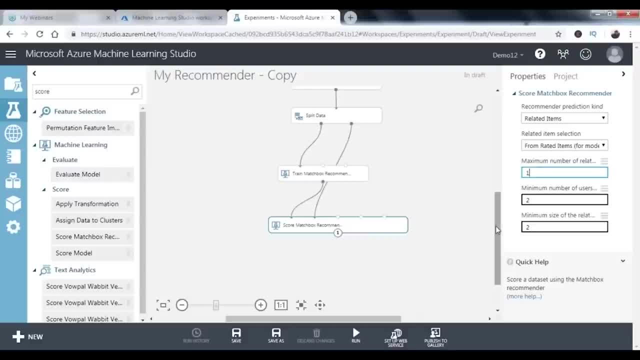 So if I pass in a particular movie to this recommender, it should suggest one movie that I might like watching. So that is what I'm talking about here. So one related movie, you can have more than one as well. So that is up to you. 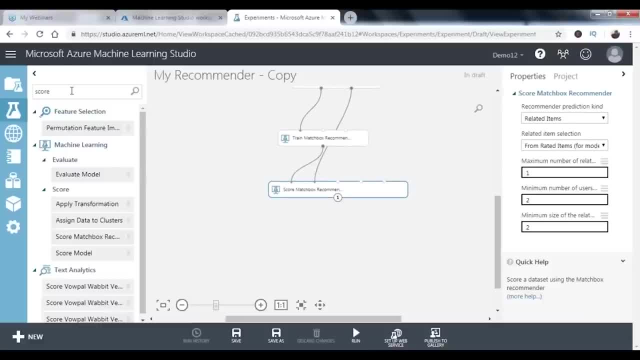 So we have done this. now next is I build a model, or I've actually gone ahead and put in a tab for training and scoring. next I need to evaluate this data right. So I say evaluate or test rather. so it says: evaluate your recommender. you get in here. 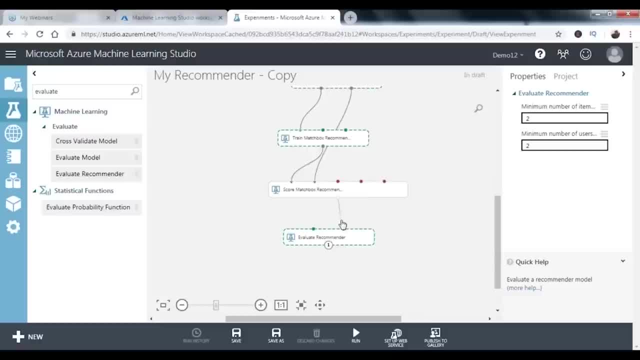 and this time you take in this value, That is your score and you put it here in this column. We passed in one of these threads here. Next is we take in the split data and we enter it here. There you go. This is fine. 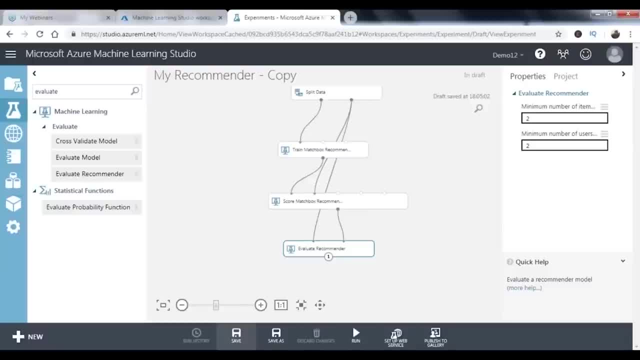 I would be saving it here, just to be safe, Once you save this data. okay guys, So the connections that we pass in these are important. in which port are you passing in what value So this might hold? And this is more or less an experimental kind of a stuff. 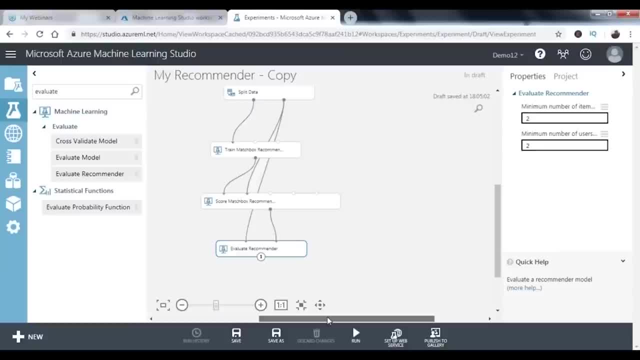 where you might actually go ahead and put in some wrong connections and you might get in some errors. So you actually need to go ahead and troubleshoot some of those at times- not always. So we've actually gone ahead and we've almost built a model. 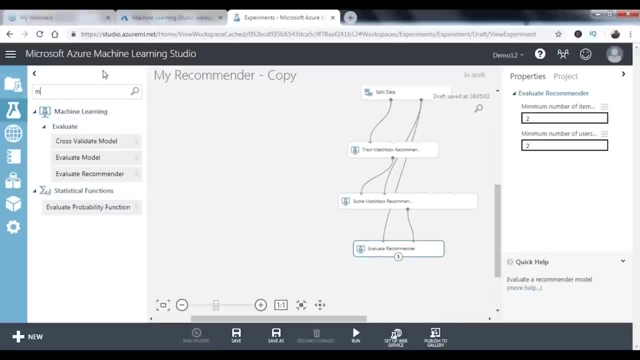 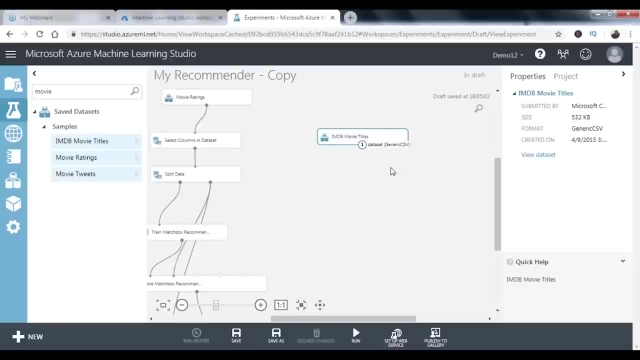 Now We need one more table here or one more data set. That is movie. I am DB titles. Let's place it here. It has gone somewhere, So I place it here. they go, and whenever we have a new data set, we always visualize it to understand what it has. 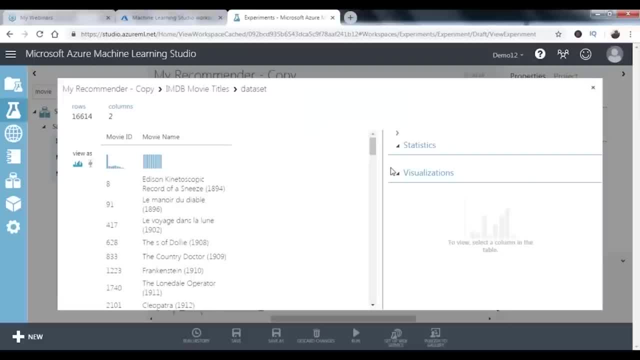 Okay, this should not take this long, but for some reason it is so I have this data set where I have movie ID and movie name. So I would be using this data set for my recommender, where it has some IMDb titles which is not the actual IMDb that website which we have it. 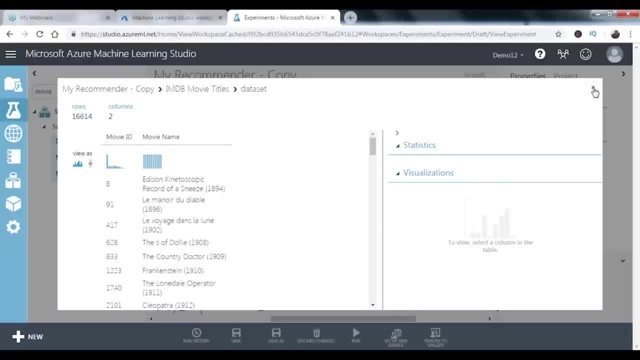 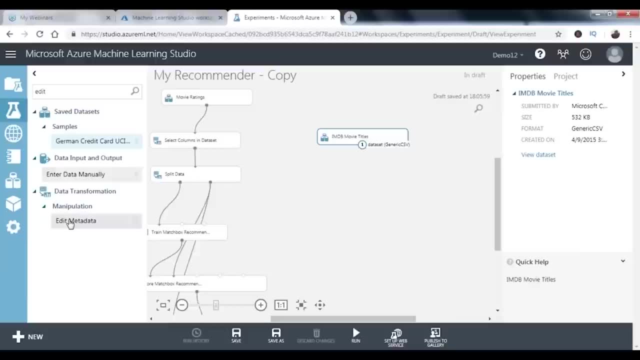 as a sample data set that is created. So we have this data set here. now that we've seen the data, I'm going to go ahead and use a command called as edit metadata and I'm going to place it here and, as usual, I'm going to go ahead and put this thing in here. 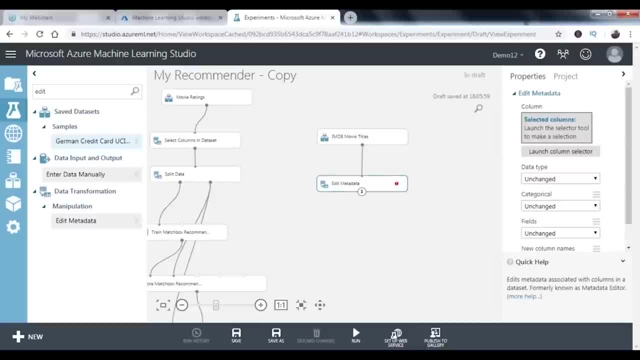 Now, if I come here, as you can see, there's this column here which says: select certain columns which you want to use. So what are the columns that I want to pass to my metadata basically, or what is the metadata that I want to use? 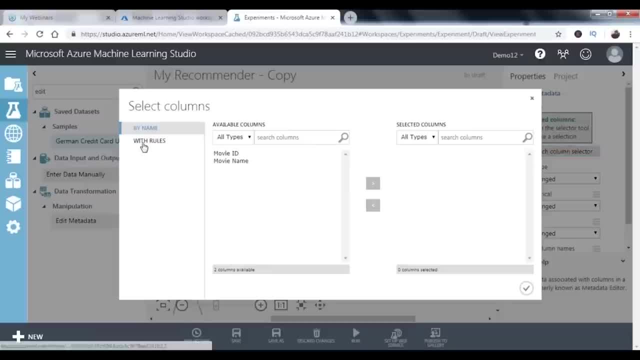 So I'm going to go ahead and click on launch column selector and in this case, with rules, I would start with no columns and I would say include. So what are the columns I need? first is I need item, So you have to hit the enter button. 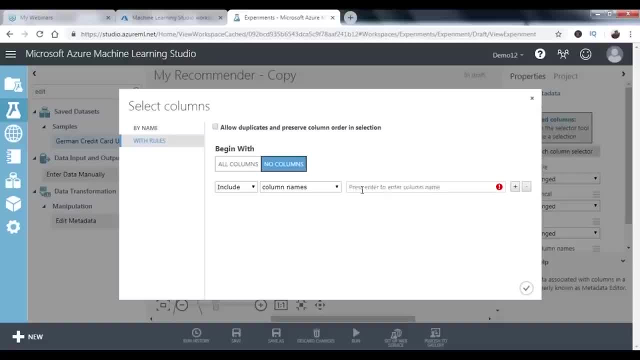 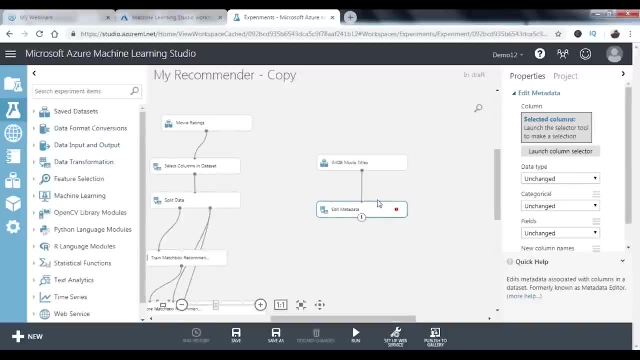 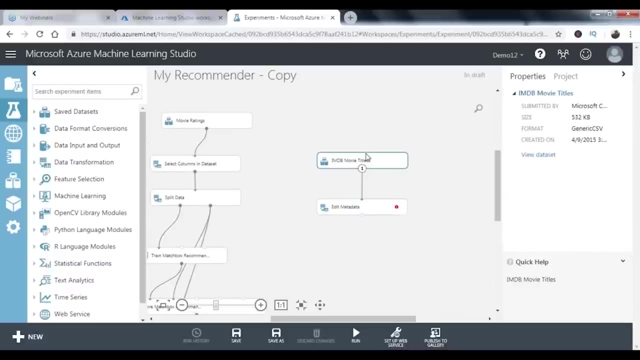 You won't be given a suggestion here. For some reason, it is not taking in this value. Let me see what is wrong. We need to pass in first values to this so-called metadata. before that, we won't be able to deal with items. because we just took a look at this data set. 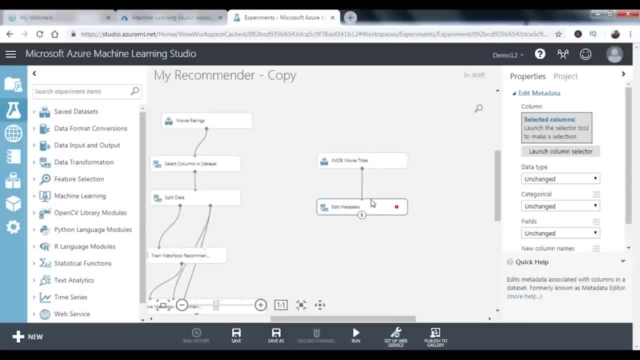 and it does not have item value. That is why we are not able to pass in that value. So let's pass in other values to it, Values that are more relevant to this data set. So we'd be coming here and we'd be selecting some other values now. 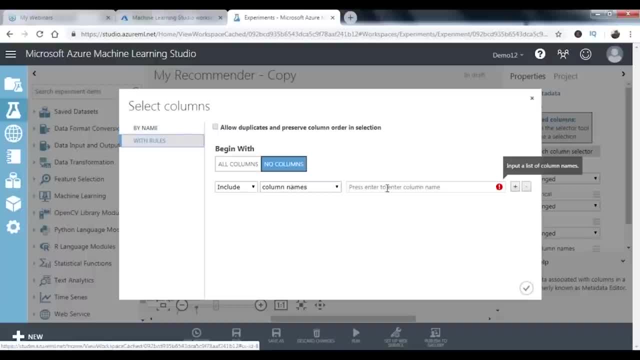 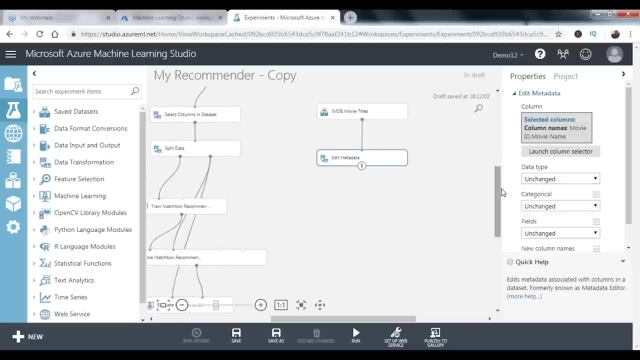 you can see that we have these values that available, So let's just go ahead and select those. There you go And I say, okay, so there is gone now. Now we have a metadata which is made available to us, and I have a model which is up and running here. 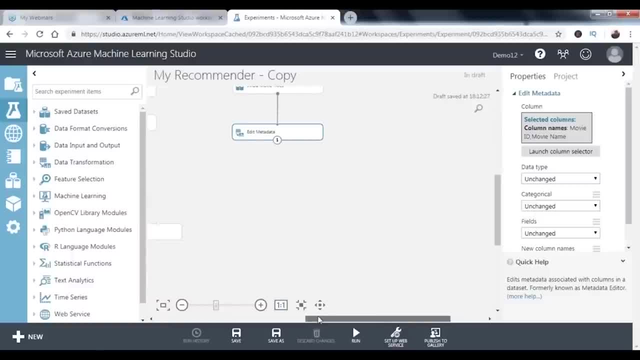 Now I need to put in joints here. Now, if you all know what joints do is, they basically help you select data from one table to the other. So we have two tables here, or two data sets, So I want to combine the data that these two tables have now. 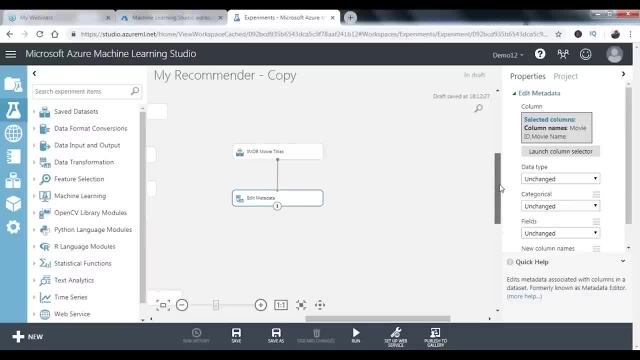 I won't be getting into the details of joints and all those things, but we would be using them here for the general reference sake. So I have these two data sets here and I want to predict or compare the table with the table that is here. 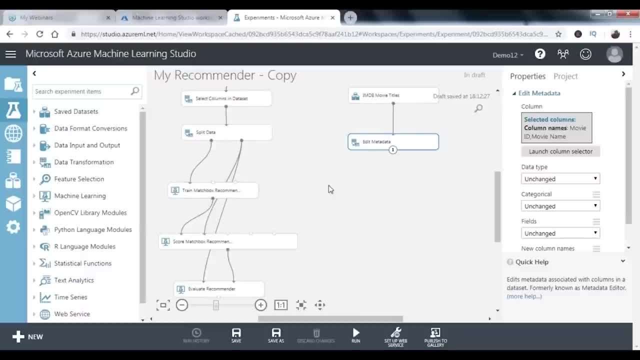 So what I'm going to do is I'm going to build a model or create a joint that lets me compare the movie names from one data set with the other or give me recommendations from one of the two data sets. right? So for that I would be needing: 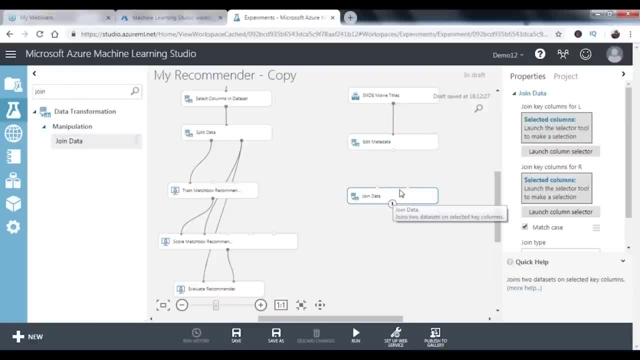 a join here, So let's just come here and say join. Okay, before we get into this thing, There is one more important point. my edit metadata data type. It has to be string. they go. now. I need to pass in values to this tab as well. 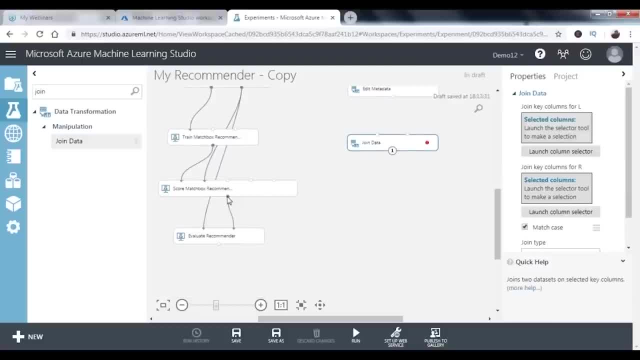 So for that I would be needing a score from here. So I would be taking this and I would be placing it here. There you go, and one from the metadata to this joint. Now, what are the values that I want to pass in here now? 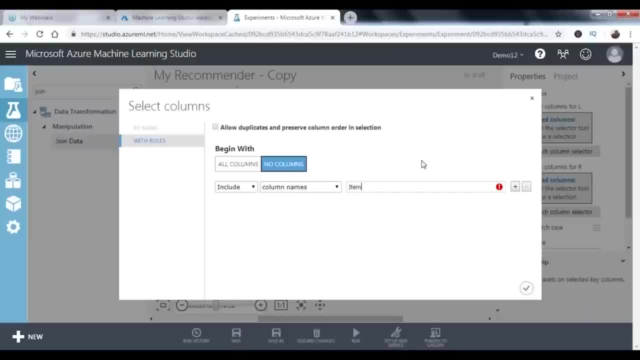 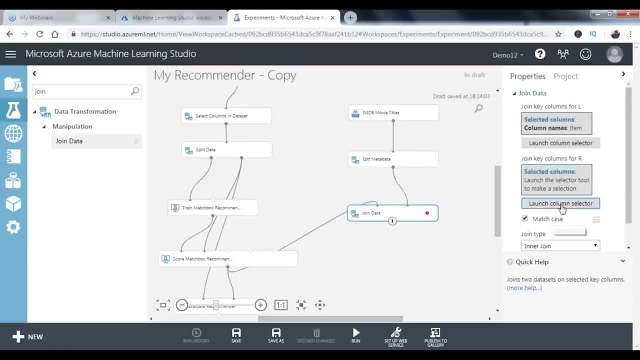 It should be item, I believe. So, as I've said, hit the enter button. there you go and you say: okay, and columns from our or the other table. What do you want from here? I would be seeing, maybe movie ID. There you go. 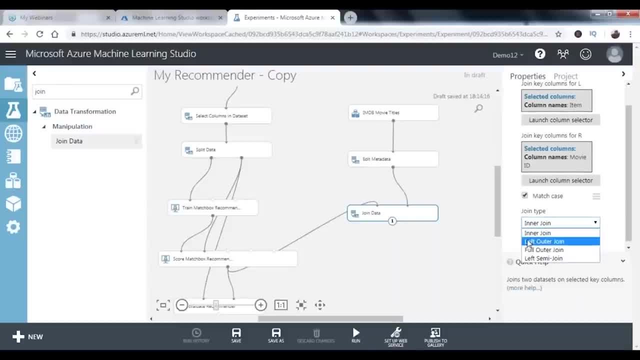 I say, okay, what kind of joint do I want? I want left out to join now again. I won't be getting into the details of these joints. don't keep the right key columns, because that is the reason I'm using this joint. 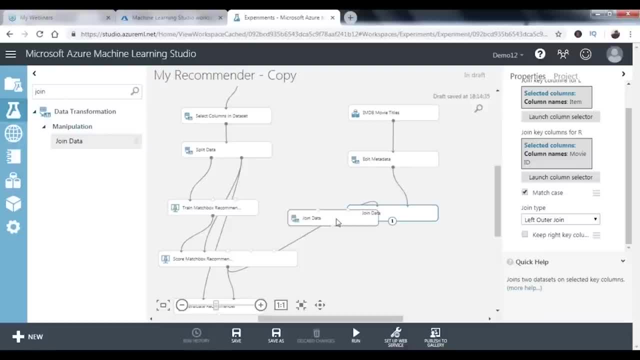 There you go. I would be needing one more join here and I would be pulling it here because the first join would just give me the movie ID. but I just don't want the idea. I want the movie name as well, right, So come here at pull in this thing. 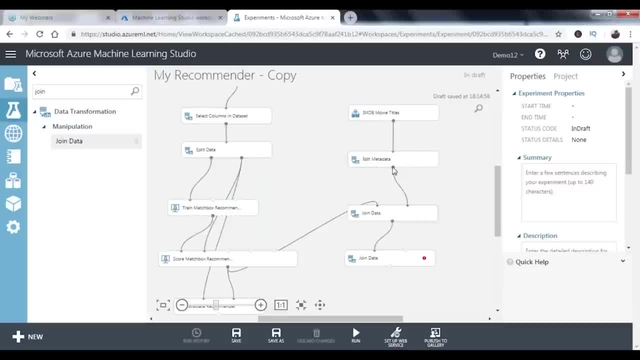 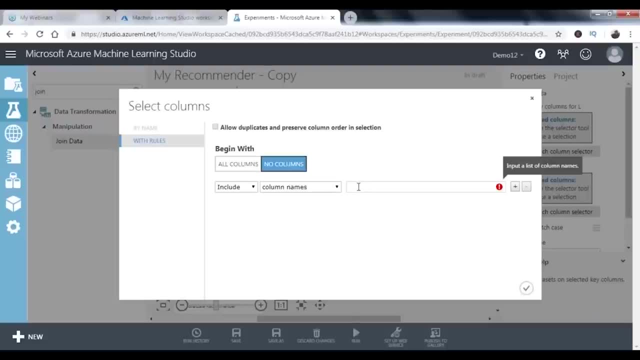 and I would pass it to this data set and edit metadata. There you go again. If I come here, it would ask me for values. I would say: give me related items if you have any. Sure The movie name, Let's say save if you missed out on one thing. 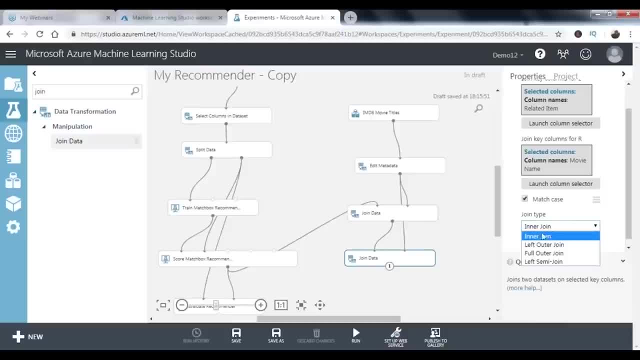 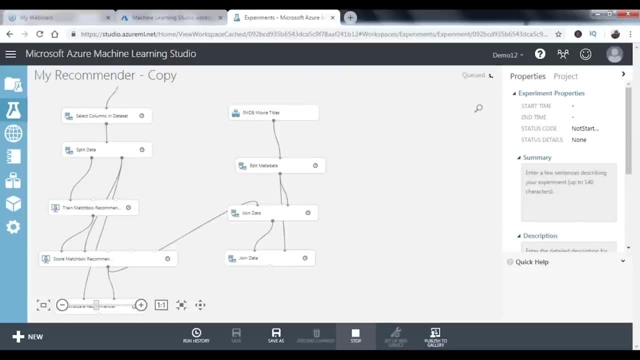 We need to come here first and remove this left outer joint and now save. we are bound to have some errors, guys, So stay tuned. Now this thing runs. it would run it tab by tab or module by module, and then everything would be executed, So this might take a couple of minutes. 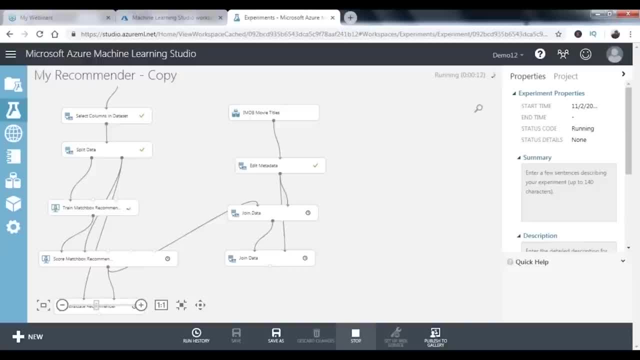 Once the model or the tab is executed, It shows a green tick on it. as you can see here, We have ticks here in here. This might take a longer because we have increased the number of iterations to 20 in the slide or in the tab when we were working on it. 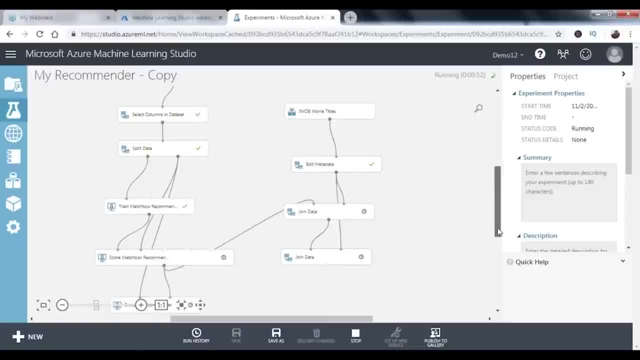 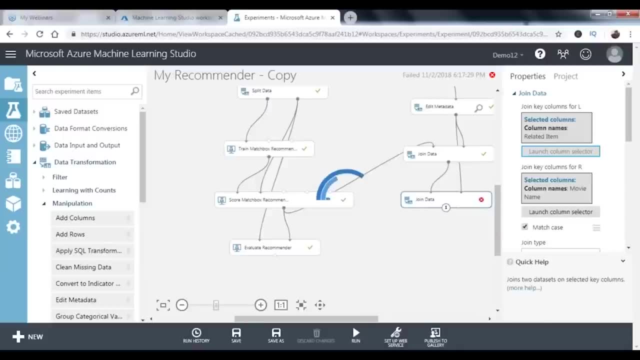 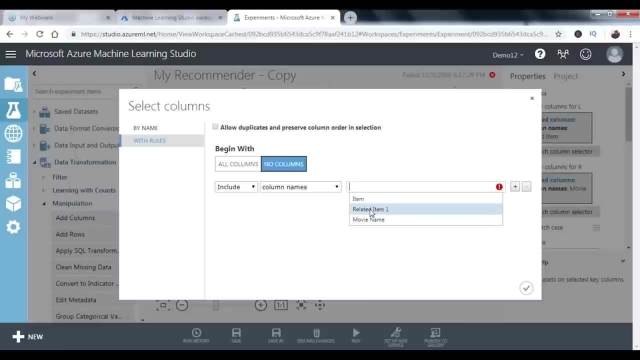 So the whole processing might take a little longer than normal. Okay, it says related item not found. Let's see Why is that happening. Launch recommend the selector. Yeah, this is the one that is the related item one. probably. there is no related item variable in the data set that we generated now. 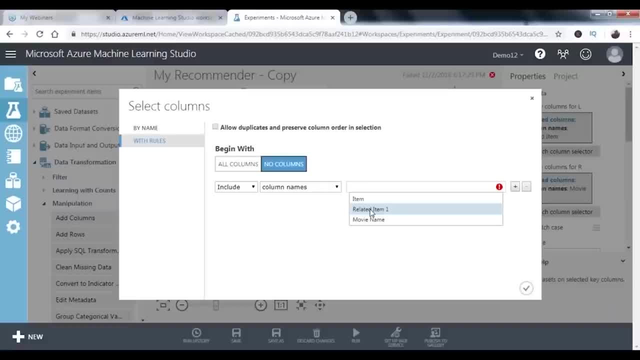 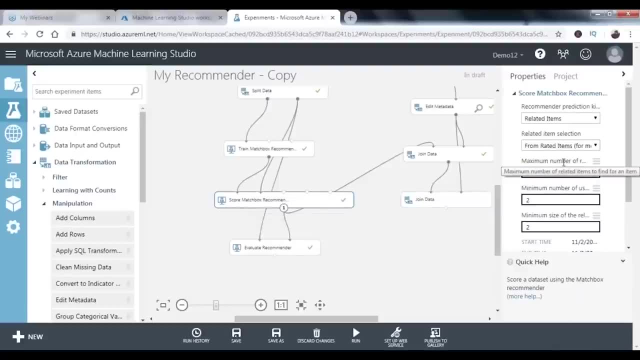 as I've told you in the first model. I'll show you where. first Let me select this for now And let me say okay here. in the score matchbox I had passed in number of related items. right, It was one. 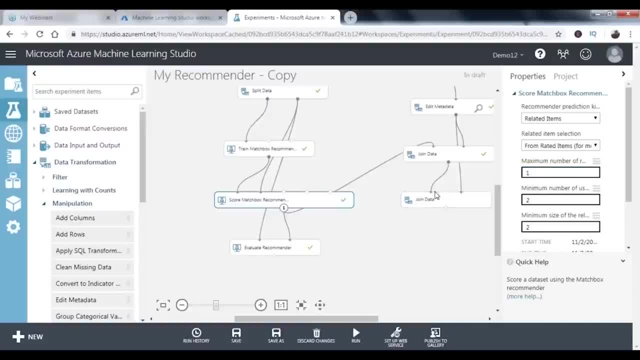 So, by default, it was given a name called as related items one. So that is something which we are passing in here or something that we would be displaying. So there you go. So what we've done is we've actually gone ahead and put in all the stuff that we wanted to. let's just see. 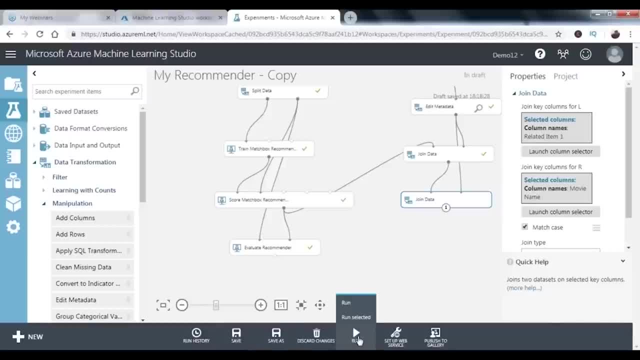 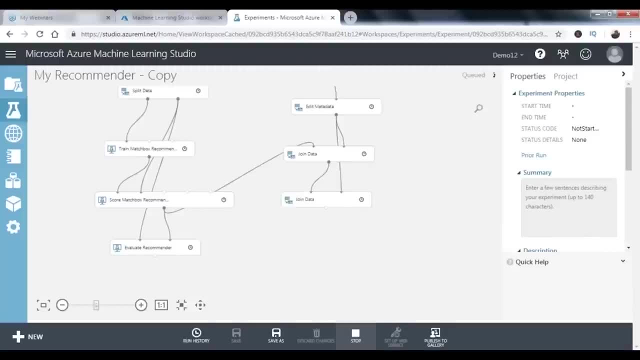 whether it runs, and once it runs, I would be explaining this again to you people. So do not worry, first Let's run it Now. this time around it should happen quicker, because most of the stuff is done. We just have the error in the last tab or the last module. 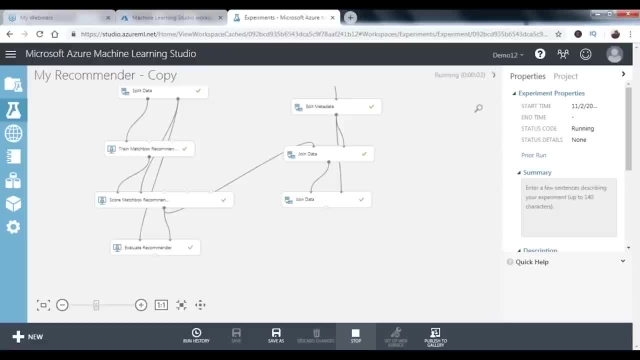 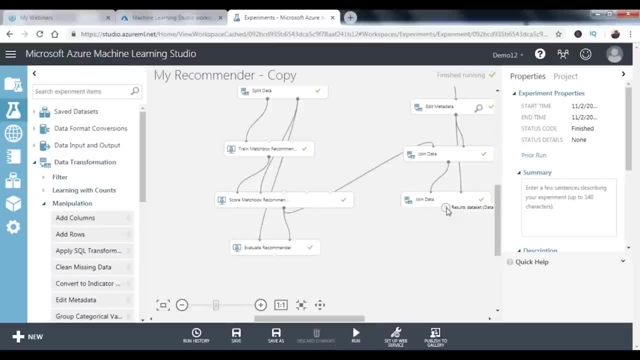 So the other part should be done quicker, as you can see, and now the last one would be implemented, and it is done already. So, guys, are model is up and running. Let's just go ahead and check. So when I click on this icon and I say visualize, you should give me some values, see. 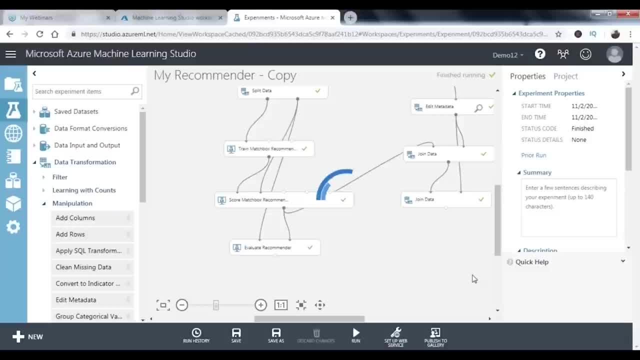 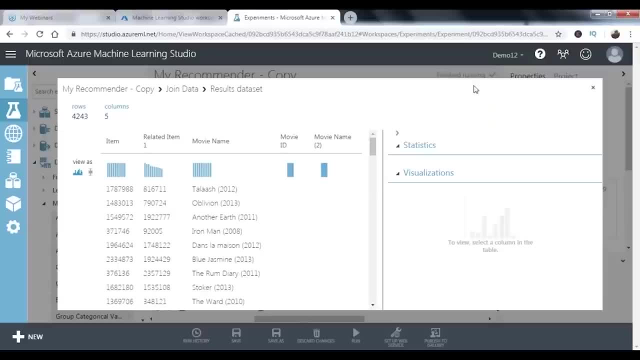 how relevant values these are. Let's just verify it Now. this being a model, It might not be that accurate, but let's hope it gives some values. It is not giving me the movie name and movie ID for the other section or the related item. 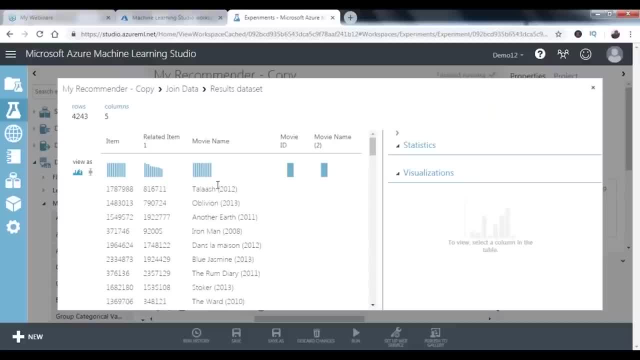 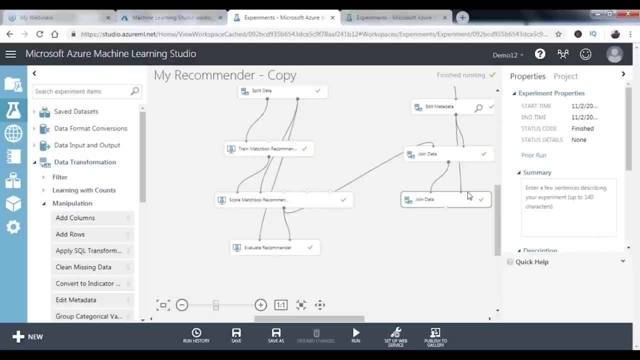 Let's see Why is that the case? but it says: if you have seen this movie, you might like this movie, but we do not have that movie. So let us see where we have gone wrong first. So there is some error here or here. 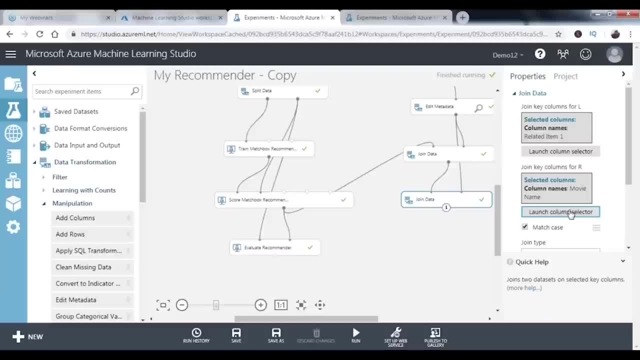 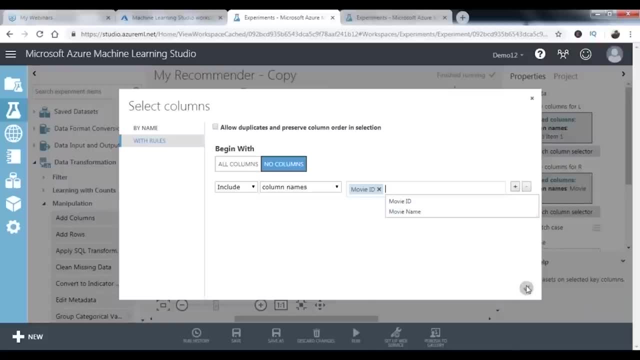 We have a movie idea. So let's just come here and see: Okay, so we can just match ID to ID or map ID to ID. So let's remove this for now and say movie ID and then see whether we get the output. 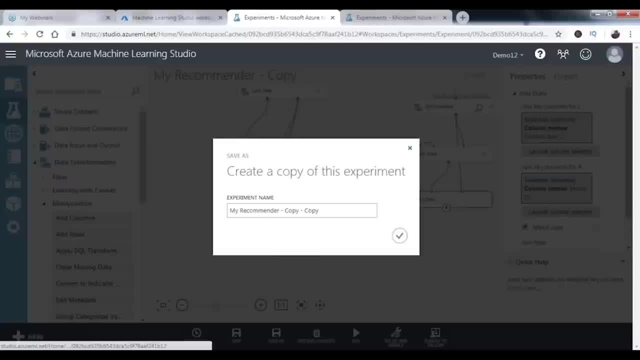 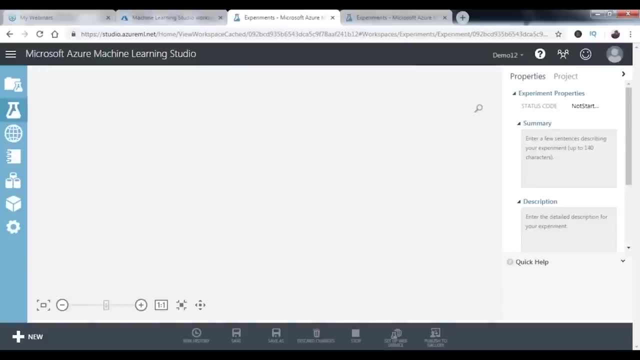 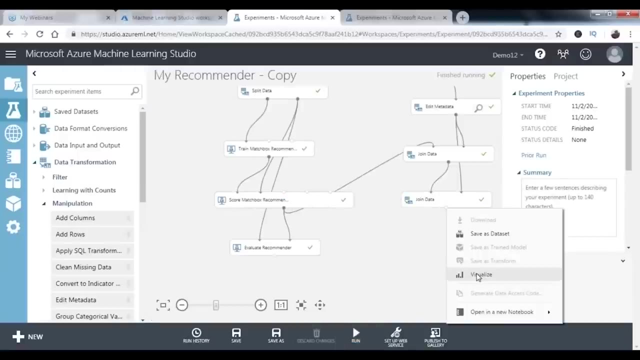 So I say save, not save, as I would say save and I would run this. So again it should run quicker than the last time They go. now let's just see what is the output that we get. So I say: visualize. And there you go, guys. 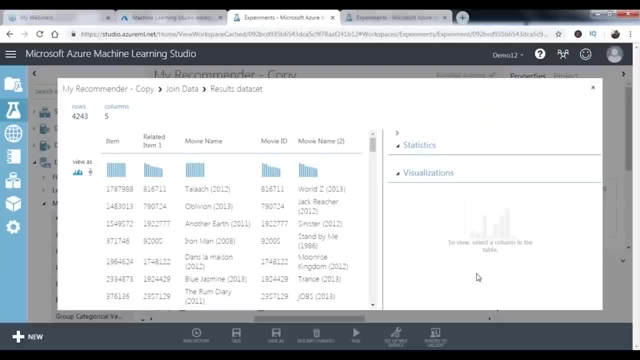 It's as simple as this. I mean, we put in, or pulled in, some values and we've edited certain values. It is, and we have the result here Now. this is an Indian movie called as the last and it says that, if you like this: 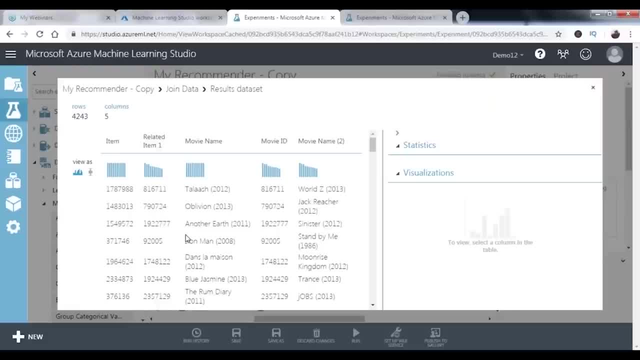 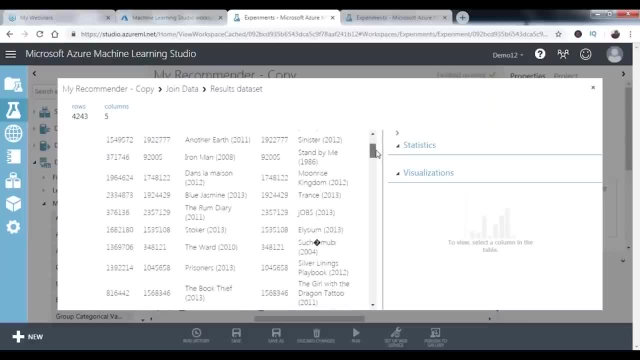 you might like this oblivion, probably Jack Reacher. I haven't seen either of this Iron Man, You might like. stand by me So I don't think this recommender is that accurate, but probably I'm sure that there would be some movies in it which are more relatable. 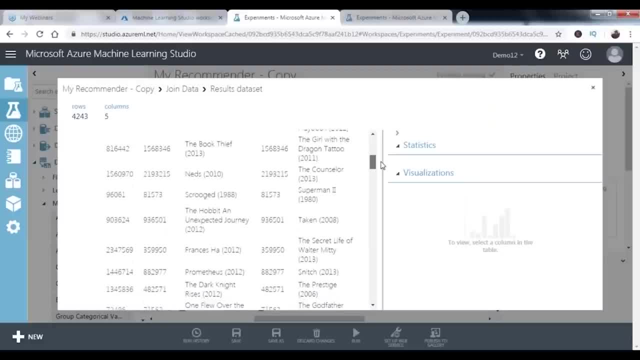 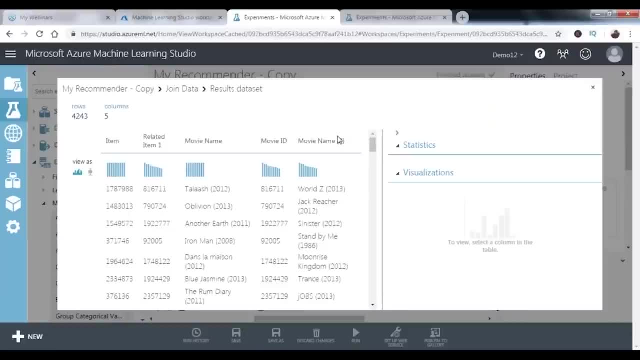 So, and for people who are big movie fans, they probably would be able to relate a lot more to the movies that are here. So again, you can actually go ahead and select the number of related items that you want to select, and you might actually go ahead and tinker. 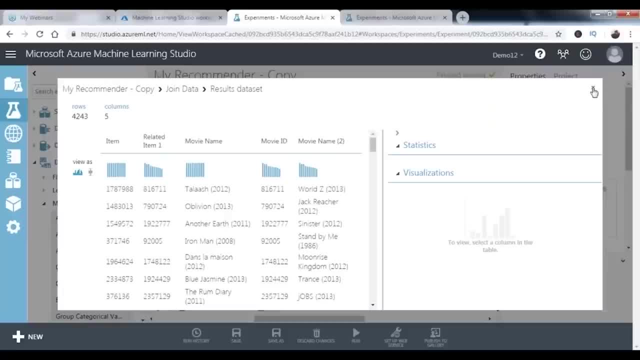 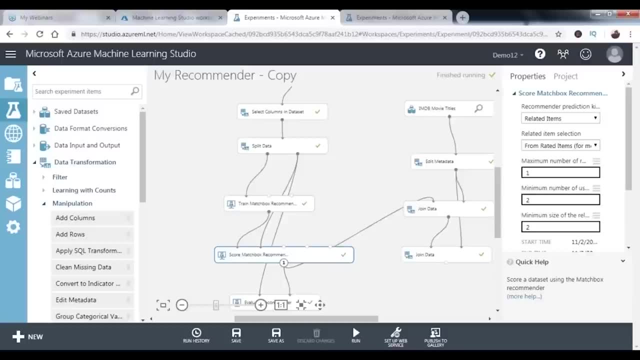 and tailor your algorithm a little more. for that You have to play with the values that are there, You have in this algorithm. You can just come here and switch in these details and probably the answer might be depending upon the inputs that you pass to this algorithm. 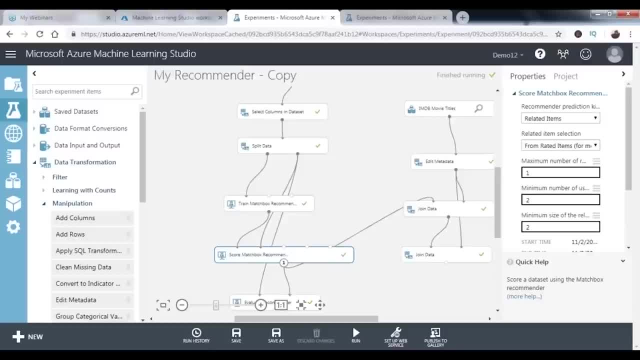 So this was my basic aim: I wanted you to get some hands-on on Azure machine learning studio and nothing more than that. But as far as this model goes, or this particular session goes, we've actually gone ahead and taken into data sets. We've actually gone ahead and build a model, trained it, tested. 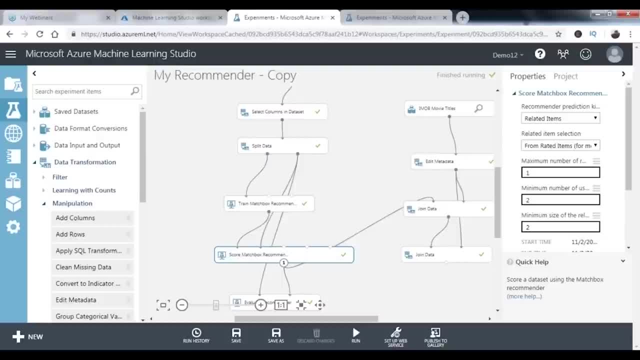 and we've used a joint to actually go ahead and see what would be the possible movie that you might want to watch if you liked one of those movies. So again, as I've already mentioned, it might not be that accurate. You are free to go ahead and play a little more with it. 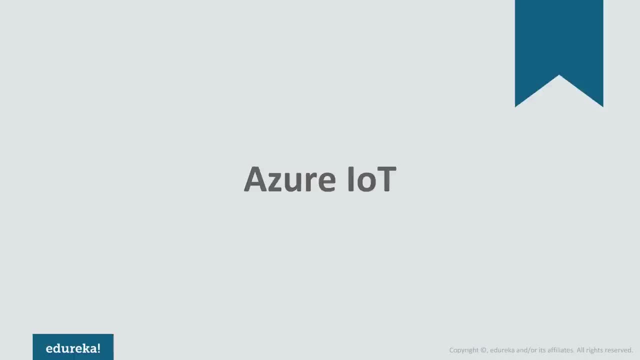 You can pass in your own data sets as well. In today's session, we would be discussing yet another interesting topic that touches up on cloud computing domain. Today's topic of discussion is Azure IOT. before we move any further, Let us take a look at the agenda. 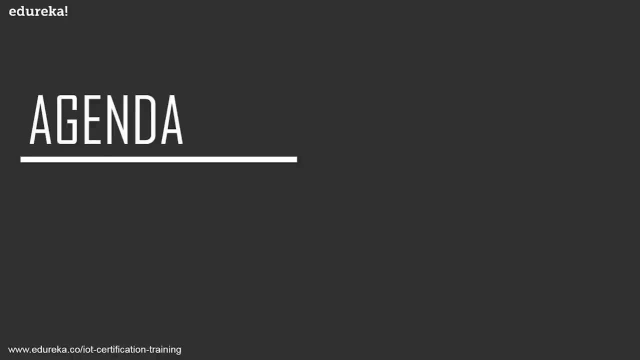 or the offerings of today's session first. So I would start this session by talking about what is IOT, that is, Internet of Things. moving further would understand what is IOT on as your. that is, a cloud platform. Then we'll talk about Azure IOT components and their users. 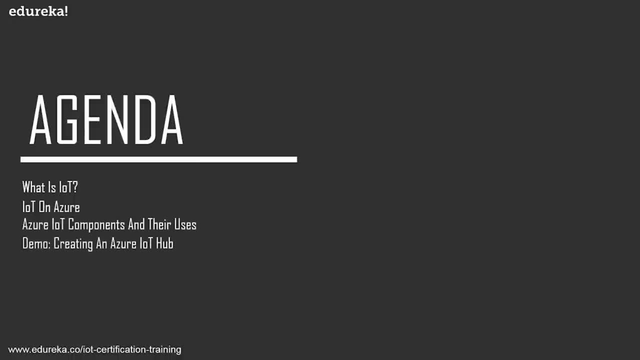 And finally, I would finish this session by discussing or giving you a slight or a smaller demo. I believe this agenda is clear to you guys, So let's not waste any time and quickly get started. So what exactly is IOT? now, IOT has many definitions. 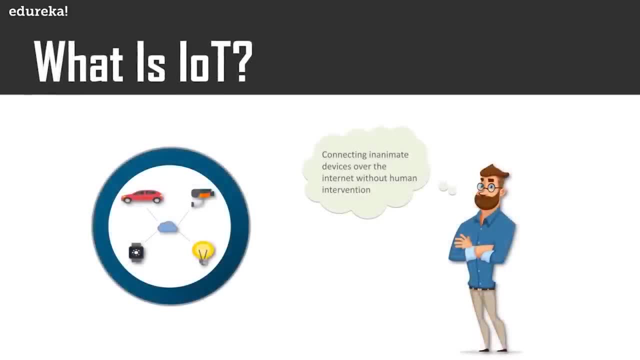 I mean because the domain is so wide, or I should say there are so many things that you can do with IOT, that to define it in one single way would not make a lot of sense. I mean you can think of it as an approach that lets you collect data. 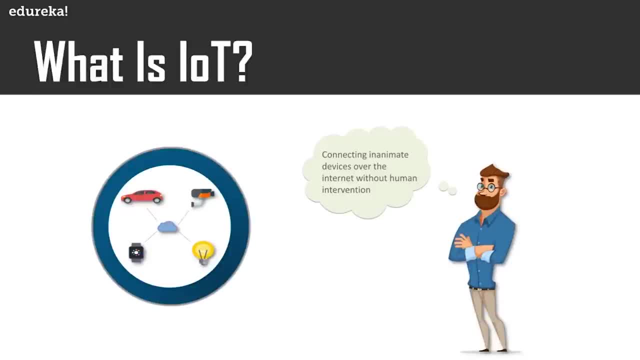 It is an approach that makes your devices smarter. It is an approach that basically helps you connect devices. now, to keep it simple, We all are social beings, or most of us are definitely. I mean, we need some social contact, Right. So what we do is we basically communicate with people. 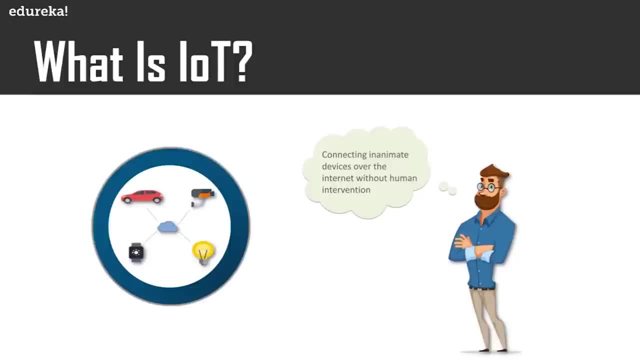 We tell them what we feel like or what is happening in our day-to-day life, or we take in inputs from them in similar manner, right? So in a way, we are actually exchanging information, We are actually exchanging data. What about devices? I mean devices do store data. 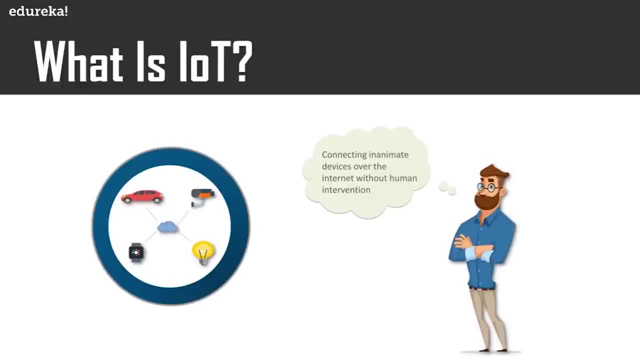 They do have information that might be useful to human beings. But how do you collect this data? How do you make use of this data? Well, yes, you have devices that let you collect data for you. There are devices that are smart and they do a lot of things that you'd want them to do. 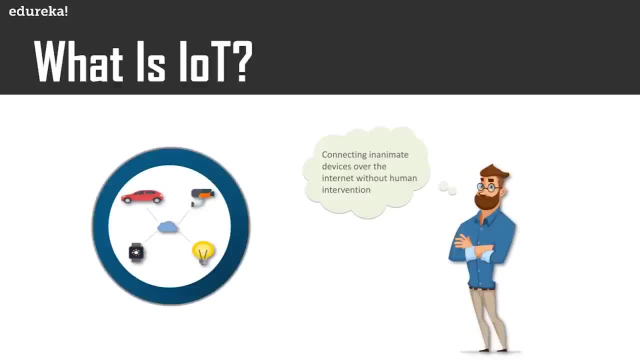 But what internet has done is it has enabled you to connect these devices with each other, and that has actually simplified the process of collecting data and also making these devices interactive and social in one way or the other. I'm sure this is not making a lot of sense for now. 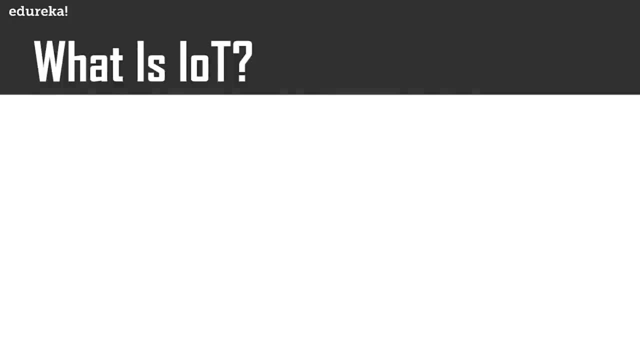 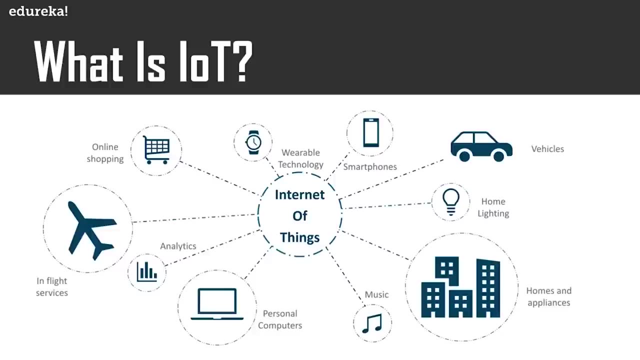 Let us move further and try to understand this topic a little more. now. when you talk about the rise of internet, what you would notice us these days: There is a lot of data that is generated online. I mean the amount of cell phones being used these days. 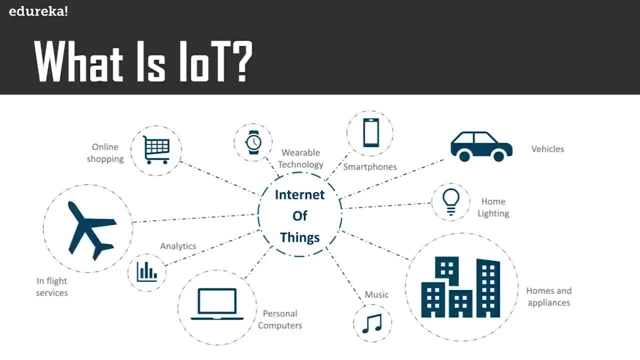 the amount of applications that run on these cell phones, the shopping you do, the food you order, the remaining stuff, the browsing and stuff like that you do and the amount of work that you do here. I mean it generates huge amount of data of this data can be very useful. 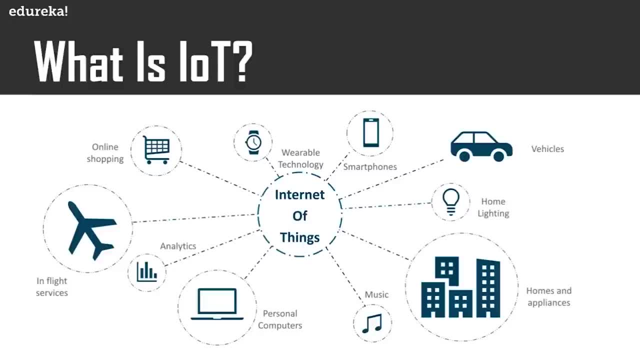 I mean, you also have analytics, data science in the market these days, and what it does is it basically lets you collect this data and use this data in n number of ways to serve the customers better, to basically make better medicines, to make better machinery and stuff like that right. 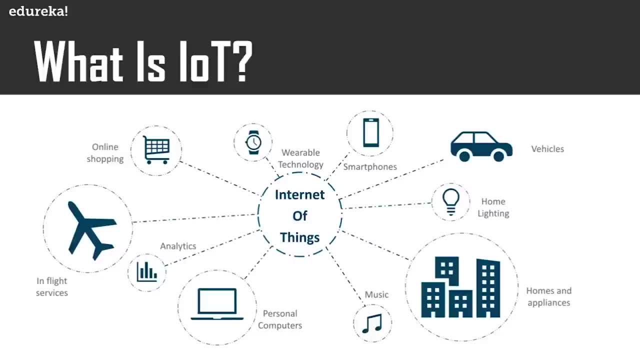 So that is what data science has done and that is what internet has done, But what this also means is a burden on human beings to collect this data. I mean, you need some way or the other to collect this data. and when it comes to human beings, 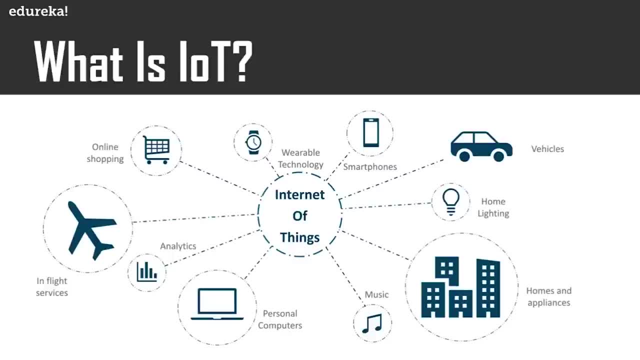 Yes, we are the sharpest beings on the earth, But the problem here is the human accuracy. at times it can go down or it cannot be as accurate as the machine is. so you need to create machines that let you collect this data. So what internet has done here is if this data is huge. 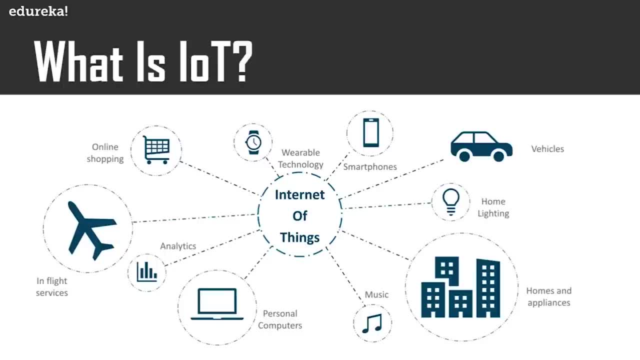 and the amount of data that is being generated is huge because of internet. it has also given you a solution. The solution is Internet of Things. What it does is it lets you connect different devices together and by doing that, these devices are smart enough and they can collect this data for you. 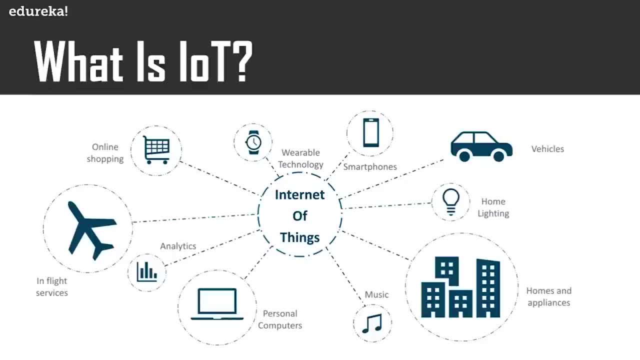 so that your only job is to go through this data or use this data, And that is why these devices are being, or becoming more smarter day by day. not to give you a very simple example, If I go home and basically what I do is I remove my wallet. 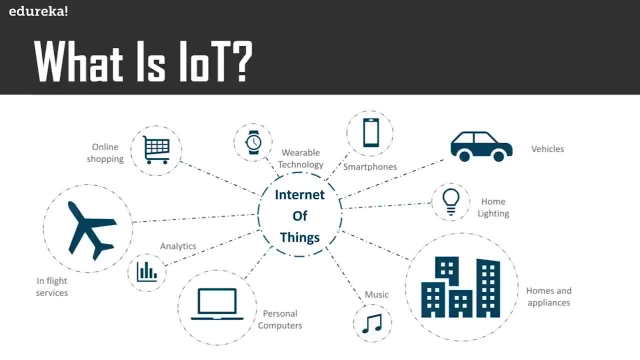 I remove my bike or car key and I keep it on the desk that is close to my door, or I rather hang it on the hanger that is there. So what mostly happens is when I leave my home, There are chances that I forget my key. 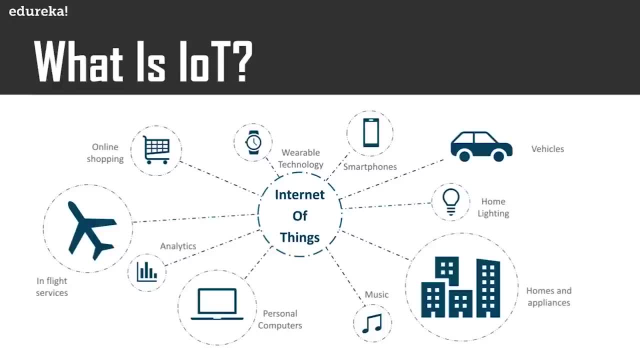 I forget my wallet right. What if there were smart devices that would tell me that I have forgotten my key Once I leave the door? wouldn't that be nice? so that can be done. I mean, you have sensors. these days, you can have sensors. 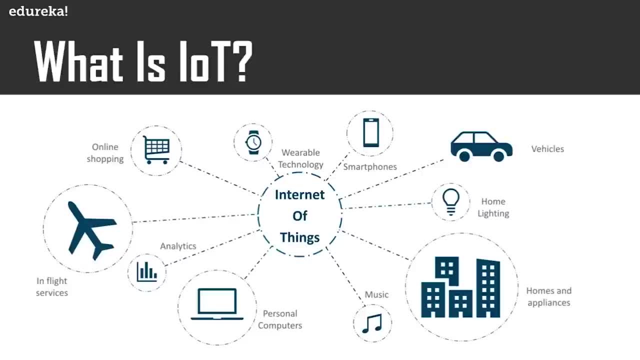 on these devices, on the keys, on the wallets that you work on or on the wallet that you have. So, basically, what these devices would do is they would basically sense the fact that you have moved out of the house And once you cross a particular range, probably. 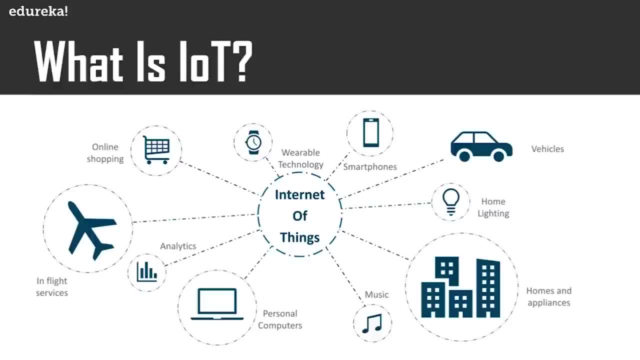 what it would do is they would throw in an alarm with some device that you have with you. So now this seems little impractical, but or seems little complicated to do. but the simple achievement out of this is you get notified. no sooner You miss out certain things at home. 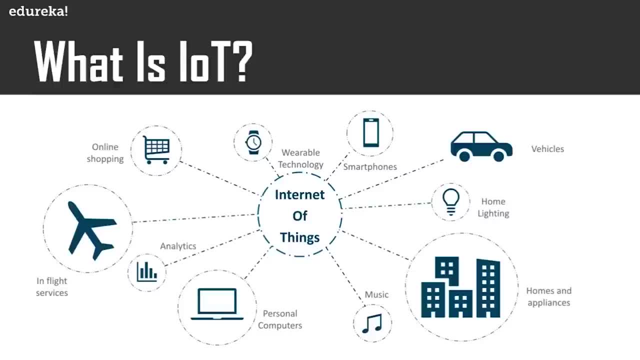 and this application can be used on the longer run to solve different kinds of problems. Now, this is one of the applications of IOT. internet can be used here. different sensors can be used here. different devices can be used to connect with each other. Now, this was about hardware. devices, basically, can connect applications. 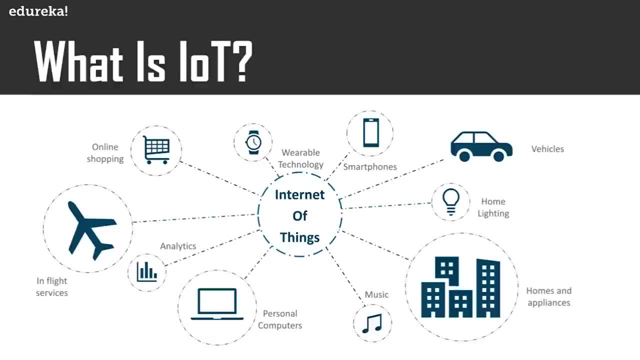 with each other, which reside on particular hardware. So this is one very basic application. There are a lot of things that you can do with IOT. So, as you can see in the image, what IOT is doing is. it is basically helping you connect different applications. 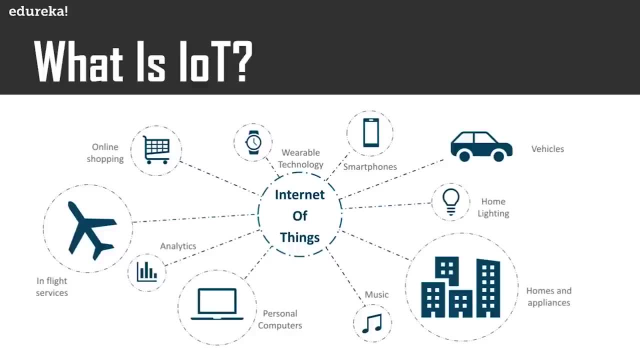 different businesses, different services together and the fact that all these things are connecting with each other. there is live data with you and that would help you solve a lot of problems. I mean, you can do better with the predictions with IOT. You can do better traffic predictions with IOT. 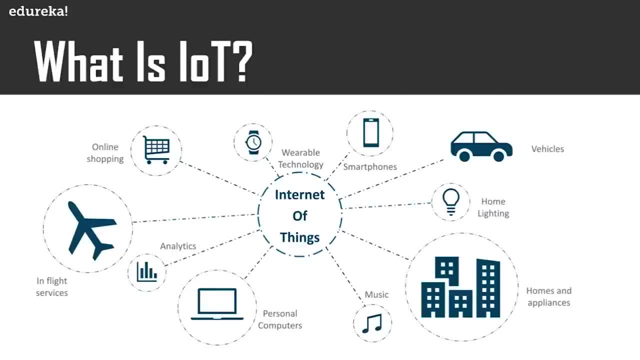 You can better figure out, as in what kind of data a person is using, you can figure out what kind of exercise routines a person follows. So all these things can be dealt with. with IOT You can prepare better medicines. You can gauge how basically medicines are administers. 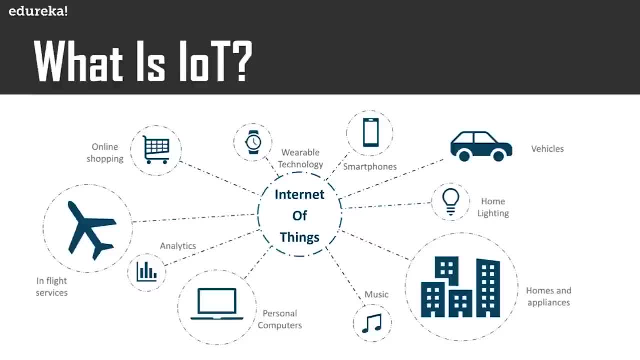 and what administered and what kind of effect are they having on that particular individual. So IOT is a great boon for humankind if used wisely. So that is what IOT is. I believe by now you've understood what IOT is. Let us move further and try to understand the other topics. 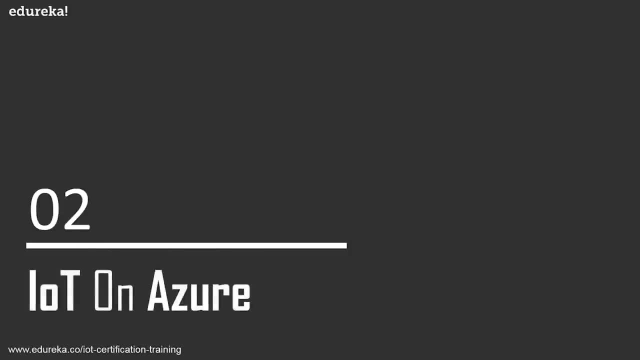 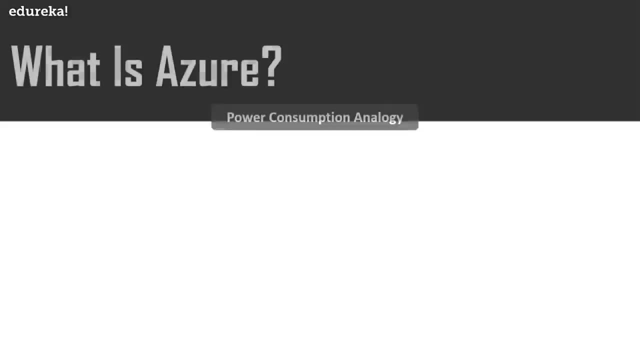 that we mentioned in the agenda. So, guys, next on this list is IOT on Azure. I mean, why should you use IOT, or Internet of Things, on a platform like Microsoft Azure? First, let us try to understand Azure in a bit. 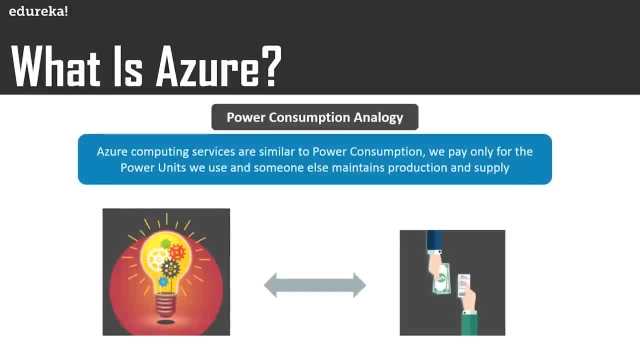 Now, when you talk about Azure, I can think of this power consumption analogy and normally use these in my sessions, So let me just throw in some light on these topics so that we can understand what Azure is. So, basically, think of Azure as a platform. 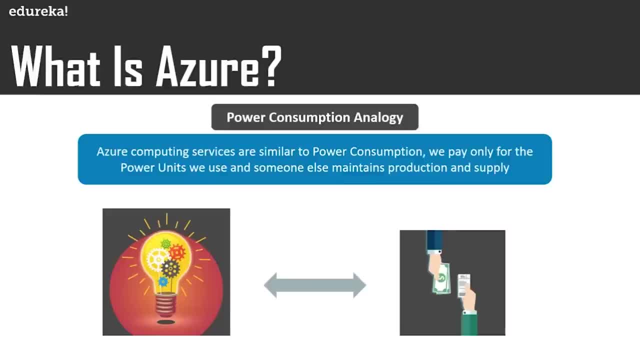 that basically provides you with services that help you solve various computation, storage and application development issues. How does it do that? If you take a look at this power consumption analogy, what you would notice is when electricity flows into your house, you basically consume the electricity. 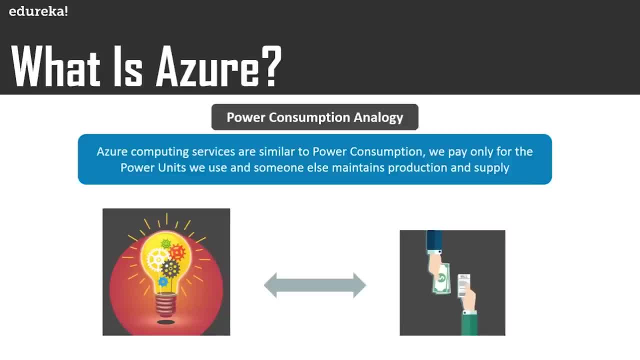 and at the end of the month you pay the bill for the units of electricity that you've consumed, right? You do not have to worry about how does this electricity flow in, who manages it? and once this electricity goes down, all you have to do is you have to call the power suppliers. 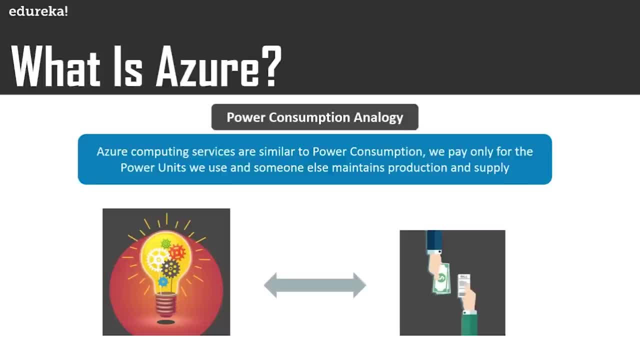 and they take care of it right. You do not have to worry about managing the units you've consumed. All you have to do is take a look at the bill and pay the bill. So, basically, what is happening is someone else is taking care of all the things. 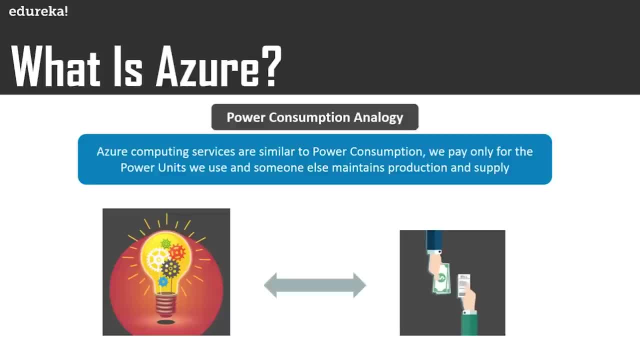 that are related to power consumption. All you do is you outsource this work to someone else. You use the services and pay for the services that you've used. It is very simple and very realistic in real life When you talk about software development. 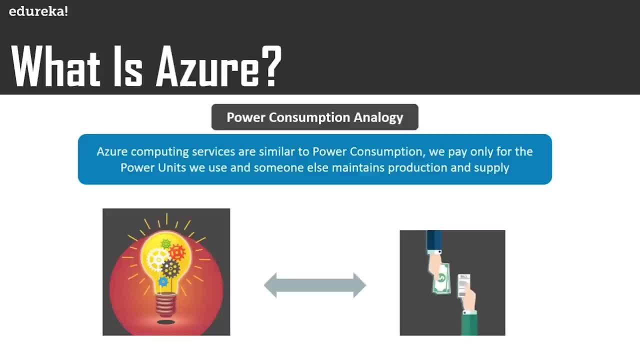 there are a lot of constraints that one has to face. I mean buying servers, hosting applications, maintaining, monitoring those applications. What if you were given solutions ready to use, solutions where you had to worry about just the data that you have and take or deal with better business insights? 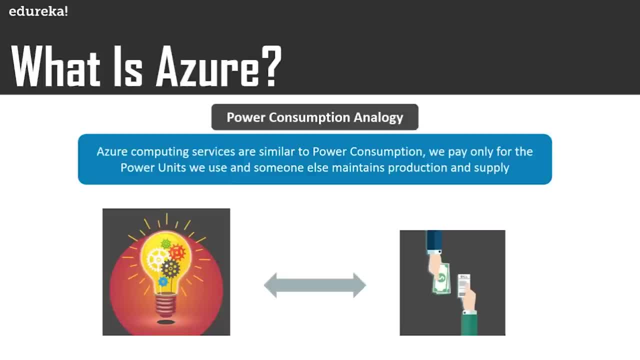 and stop worrying about all these issues. Wouldn't that be nice? when you talk about Microsoft Azure, it does exactly that for you. It provides you with cloud computing solutions, or it provides you the platform that solves various issues that are related to your software development. 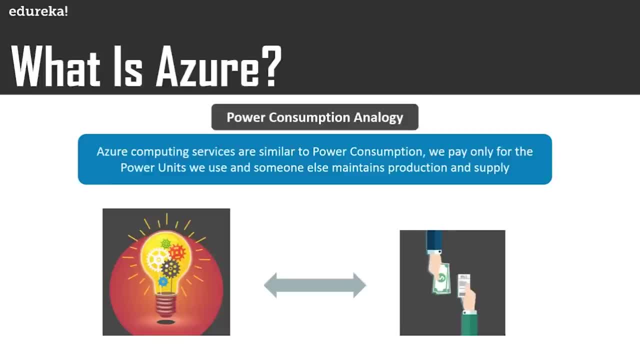 So it is similar to the power consumption. I believe it is making some sense. in this case, Your Azure is basically your electricity provider. in terms of software services, right? So that is what Microsoft Azure is. It is a cloud platform that provides you with various services. 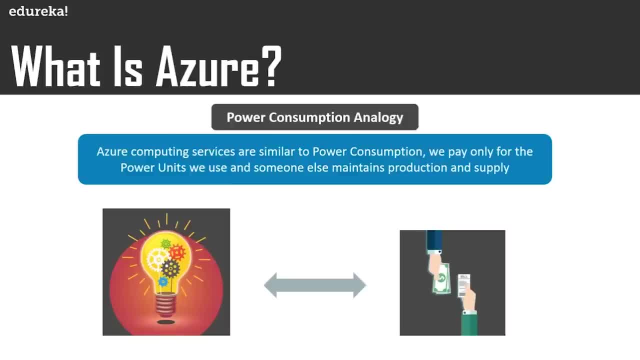 that concern computing and software development, and you can actually go ahead and rent these services and use them for a particular time duration when you want to use them, and you can get rid or release those services once you are done using them. So this is what Azure is, and why should you use IOT on Azure? 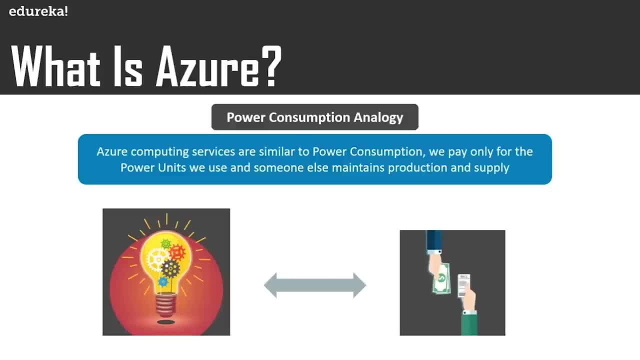 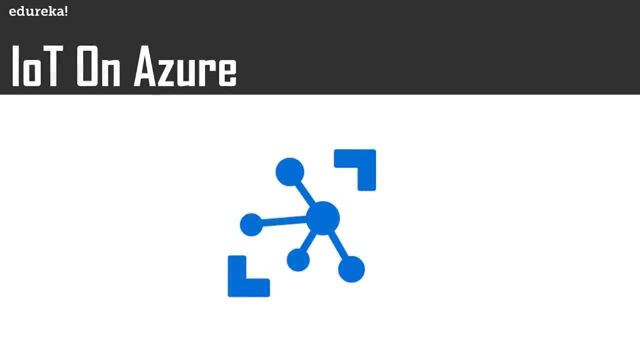 Well, Azure is one of the leading cloud service providers and that is why, when you talk about Azure, what it does is it basically provides you with various integrations, various services that would help you implement IOT services on top of it, and with ease. to give you a simple example: 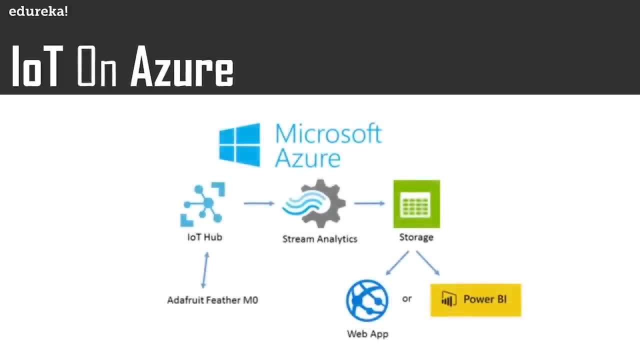 Now, this is an image I directly picked up from Microsoft Azure's website, If I'm not wrong. I would be giving credit to them, Do not worry about that, But this is a very simple example and this is what it demonstrates. 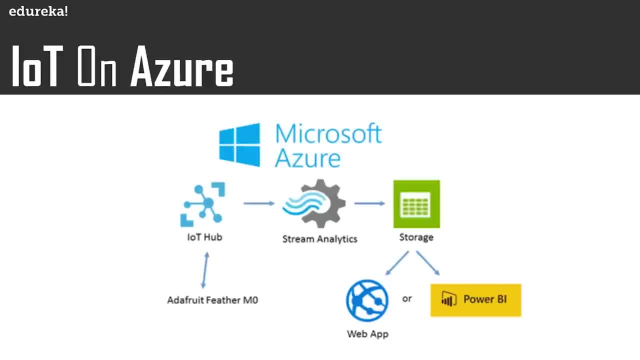 I mean, you have an IOT hub, which is an IOT service that is basically giving data to your stream analytics which can be visualized by using different Azure tools. Now, when you talk about Azure services, there are services for everything for your data visualization. 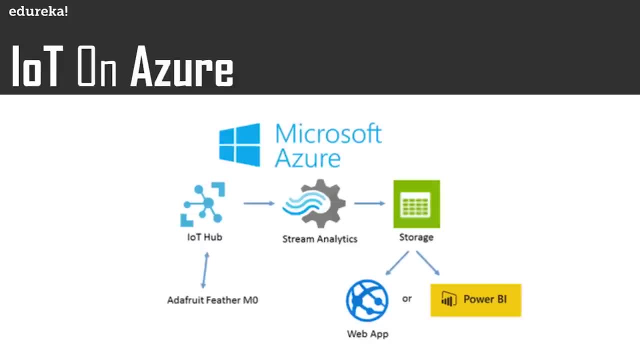 machine learning, data warehousing, data lakes. You have application creation, past service creation, instance or virtual machine creation, storage, security, and everything is taken care by Azure. So basically, if you have applications that run on Microsoft Azure, you can actually go ahead and apply Internet of Things to it to make them more smarter. 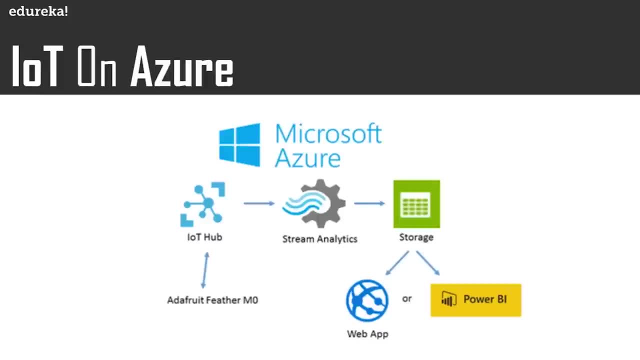 And if you do not have applications on Azure, you can actually go ahead and create those using Microsoft Azure, and you can again use IOT on top of it. So, yes, if you talk about IOT and Azure, it is a very good choice. 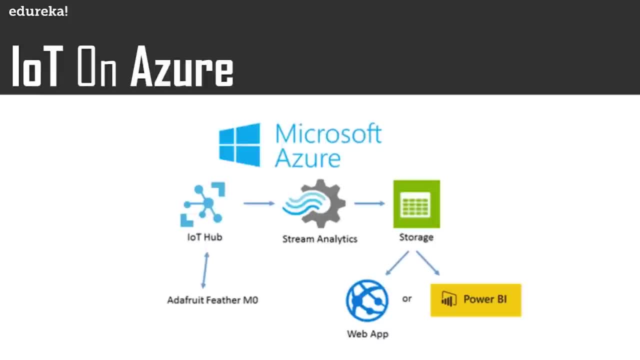 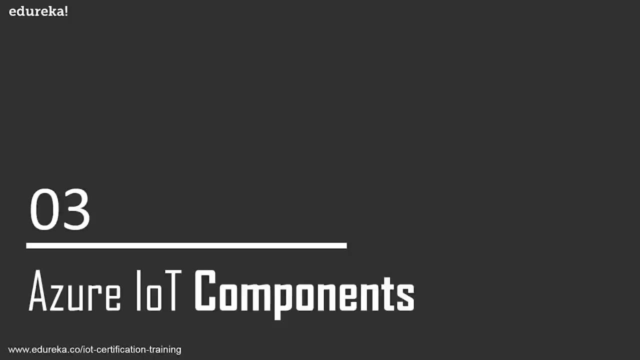 and a very good option that people can opt for. what all can you do with IOT and Azure? Let us take a look at some of the important IOT components on Microsoft Azure. Now, when I say components, you can think of these as services that cater the need of Internet of Things on top. 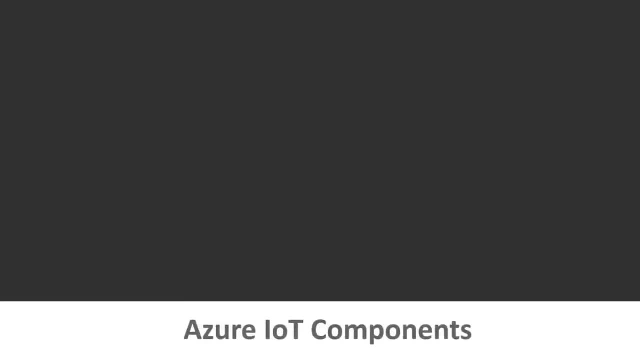 of Azure platform. Let us try to understand those. So, guys, first and foremost, you have your Azure and IOT central. now, when you talk about Microsoft Azure, as I've already mentioned, it is a cloud platform. So, if you've learned, cloud platform to some extent. 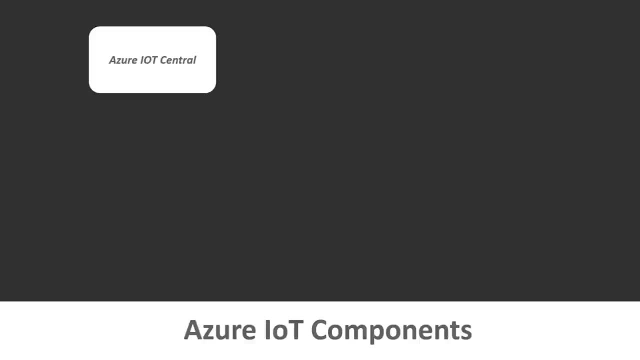 you have three services. you have infrastructure as a service, platform as a service and software as a service. now, as you progress with these services, IAS is basically a service that provides you with basic infrastructure, on top of which you can choose everything that you want to do. 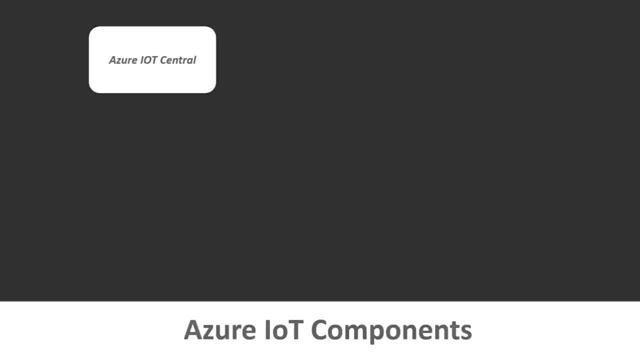 That means you can basically have a basic layer on top of this. You can choose what operating system you want to use, what binaries to use, what applications to run, what programming languages to use. So it is a basic infrastructure that you can have. when you talk about pass, 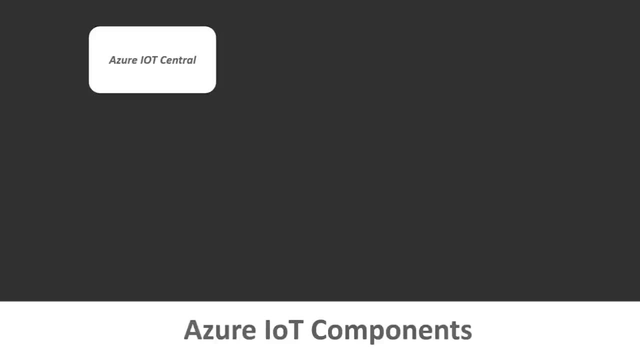 It is basically platform as a service, where a platform is given to use, where you have ready to use, templatized applications. And when you talk about SAS, it is software as a service, where a complete software is given to you on rent which you can use, say, for example, Gmail. 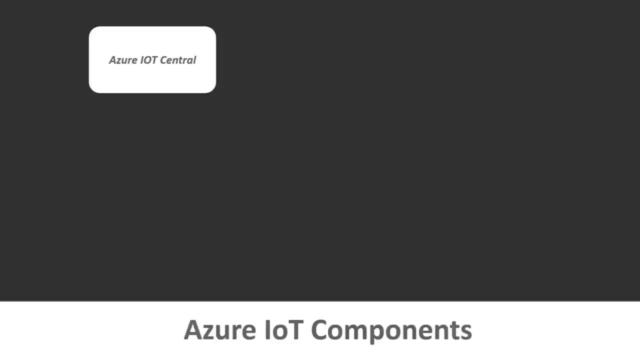 I mean, you do not have to sit and code Gmail right. It is a ready-to-use application, You do not worry about it. It's security, its management, It's maintenance- Everything is taken care by someone else. So cloud provides you with these kind of services now. 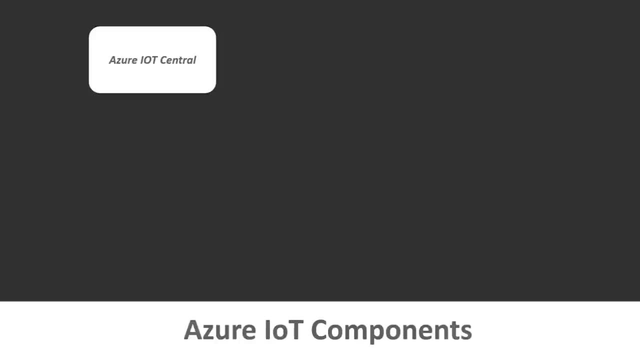 when you talk about as your IOT Central, think of it as a SAS kind of a service. I mentioned Gmail, right? So what it does is it provides you similar services, or it provides you a service that basically lets you create a similar software as a service, kind of applications for IOT platforms. 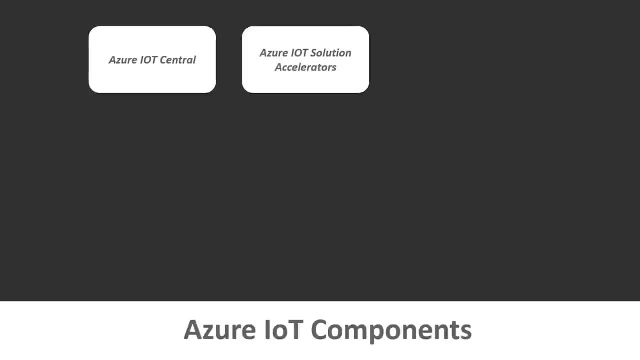 So that is what Azure Central is when you talk about Azure IOT it is. it is more of a pass kind of a service that lets you create templatized applications or templatized IOT applications, which you can use to create ready-to-use IOT services. 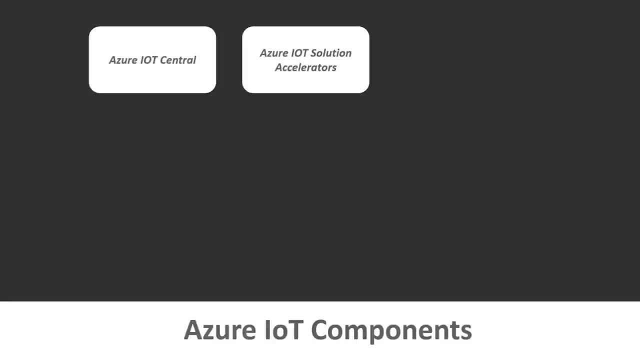 Now, what is the difference between these two? the major differences. now, as your IOT is a SAS service, That means it would require you to put in lesser efforts. I mean, it is more ready-to-use kind of a service, just like your Gmail. 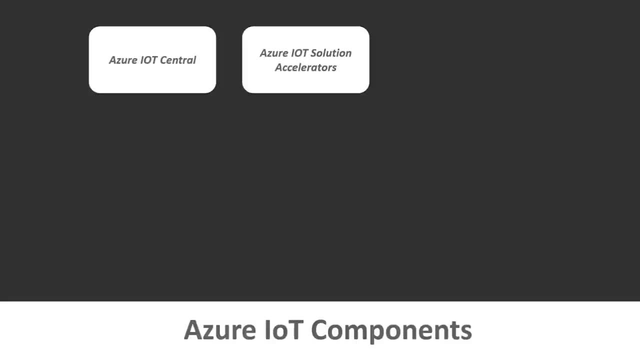 So it is easy to create. but the disadvantage of this service is it does not give you a lot of customizations. I mean, you cannot go to Gmail and decide to hard code it again. right, You can't. but when you talk about as your IOT accelerators, 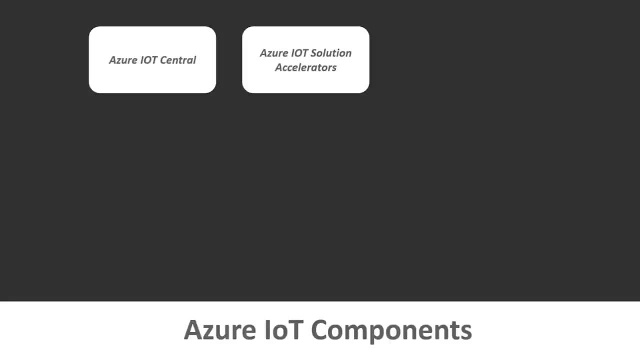 it again provides you with templates to create applications, but it is platform as a service. That means it gives you a platform. So this platform, it forms a way or paves a way on which you can actually go ahead and put in your applications, decide what kind of platform. 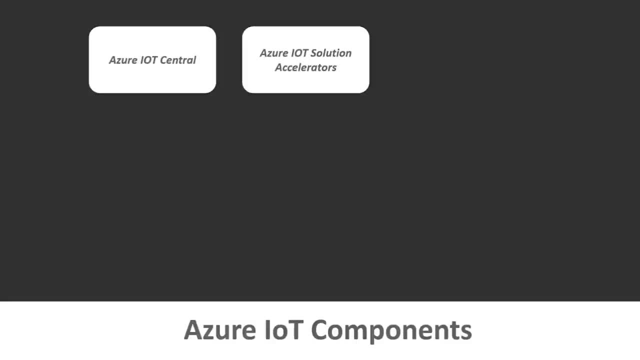 what kind of software you want to run on top of it. So it gives you more flexibility. So it would require more efforts, So it is not easier, but it gives you more flexibility. So, yes, these both services basically focus on templatized applications. third on this list: 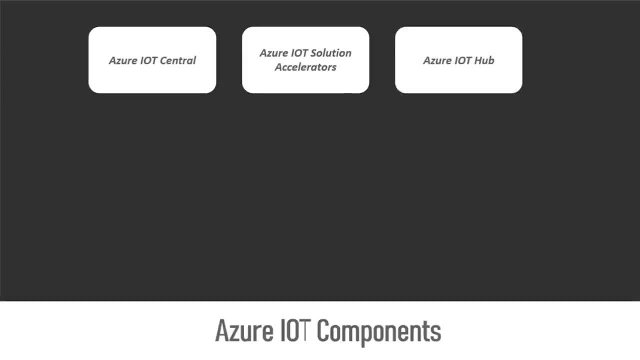 You have as your IOT hub. now, as your IOT hub is a very important service Basically water does is, it lets you connect other services and applications, So it forms a central point of communication for all these applications. So when you talk about the first two services, 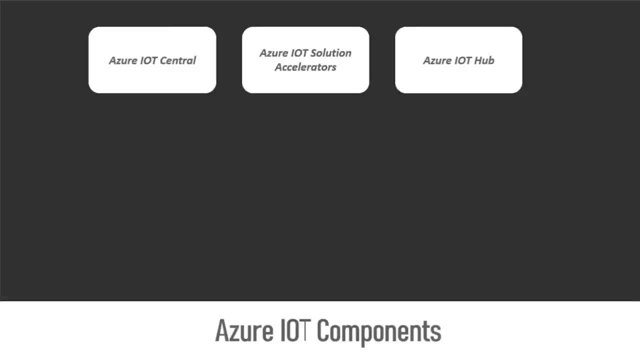 they are kind of dependent on Microsoft as your IOT hub to some extent. the other way around is not true. That means, as your IOT hub is a fairly independent service. what it does, as I've already mentioned, it lets you communicate with other applications and other services it forms. 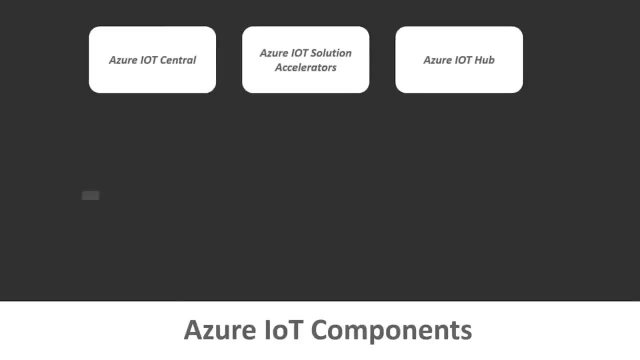 that hub where applications communicate. then you have Azure, digital twins and, as your time series, insights Now these services. basically what they do. is they let you create models? Yes, they let you create models. And when you talk about digital twins, Yes, it works in that way. when you talk, 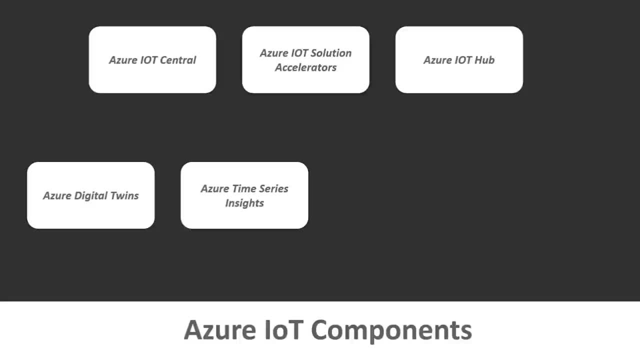 about Azure time series insights. basically, if you've learned analytics, you know you're talking about time series. That means how data varies from time to time, like your stock markets, right? I mean, the graph is not constant. It might go up, it might come down. 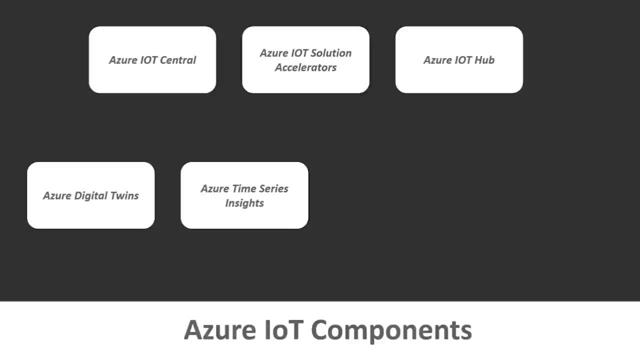 So, basically, a series of information that varies as per time is called as time series analysis. I'm going to talk about Azure time series insights. What it does is it gives you insights or let's you build applications that helps you collect real-time data and generate insights out of it. 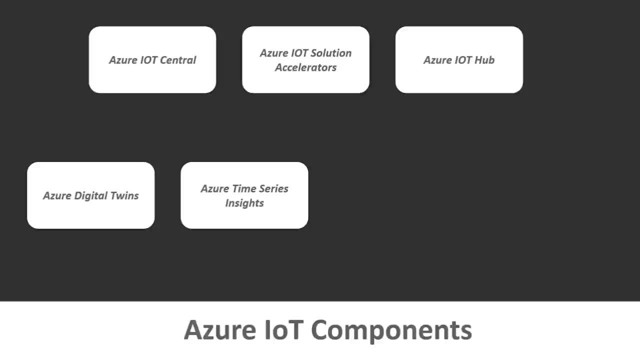 So it is an analytics kind of an application. when you talk about Azure IOT, it helps you in data visualization and for various analytic approaches, as well as your spear and as your Maps. now, when you talk about Azure spear, basically what it does is it lets you create devices. 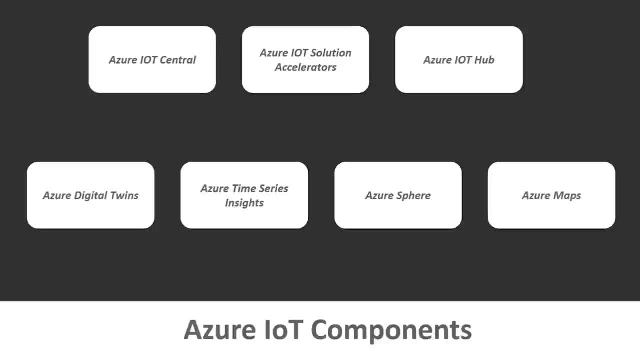 Those are Hardware heavy. I'm not sure whether this is a right term to use. now, when you talk about IOT, you also are talking about Hardware devices that let you connect different sources, And when you talk about Azure spear, it has a set of devices or classifications. 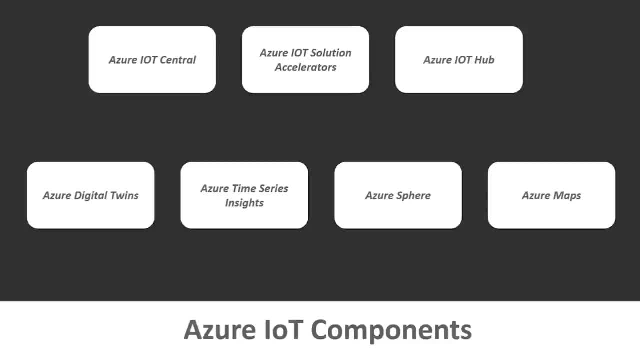 which lets you do a lot of IOT things like: basically it has its sets of MC user micro controlling units. basically that helps you in better IOT services. And when you talk about Azure Maps, I've mentioned an application called as knowing the traffic at different locations, tracking your cars and stuff like that. 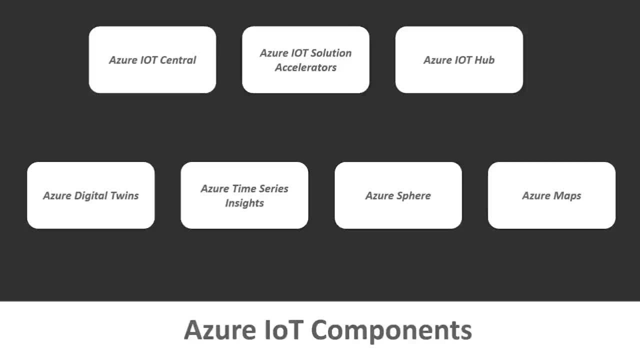 So for that you need the location of the device and, as your Maps, will help you in that aspect of IOT as well. So, guys, these are most of the services that Azure IOT has to offer to you. We won't be getting into the details of all these services today. 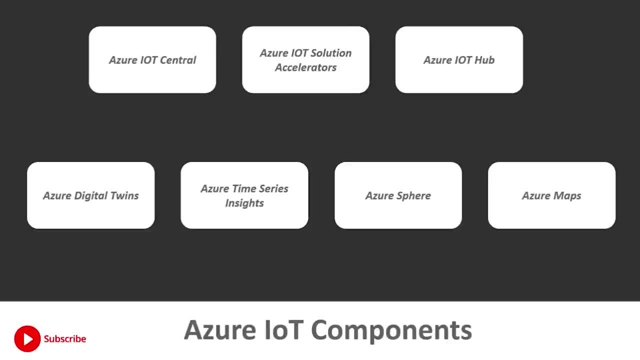 as we move further and we have more sessions on this topic, That is, Azure IOT. Probably I would be focusing on all these services individually and in a lot more detail. for now, Let us just quickly move to the demo part. What I'm going to do is I'm going to quickly switch. 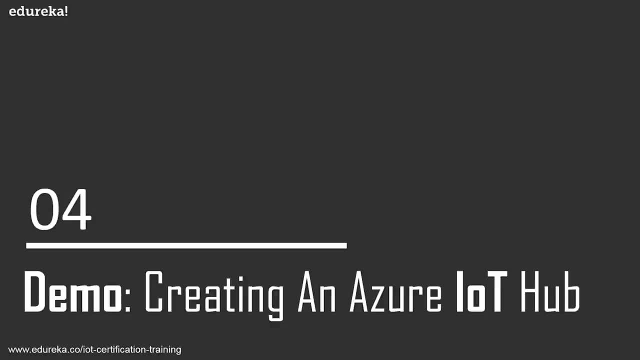 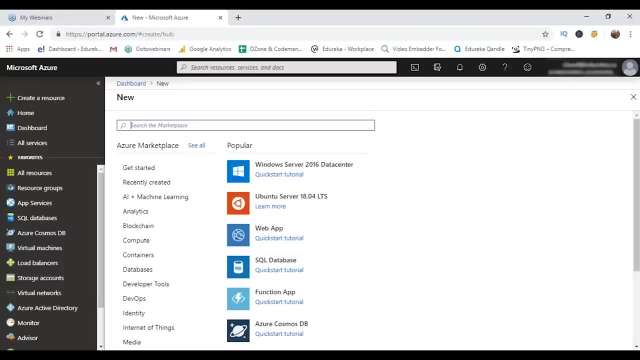 into the Azure console and we are going to go ahead and kind of create a simple Azure IOT hub. So, guys, when you talk about Azure IOT or when you talk about Azure in general, now you have your Azure portal. it provides you with free as your services for a limited amount of time. 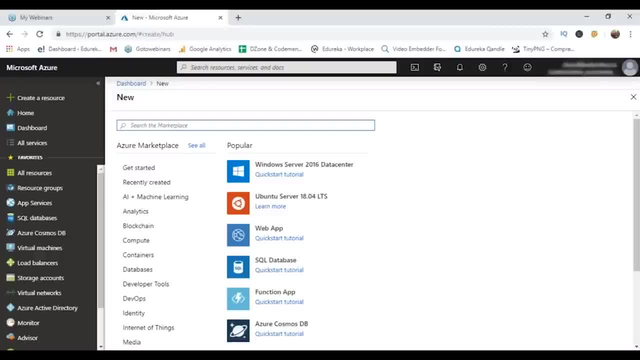 If you are completely new to Azure, I would suggest that you actually go ahead and create a free tier account. All you have to do is given certain details- your credit card or debit card details- and you're good to go. You can have that free tier account. 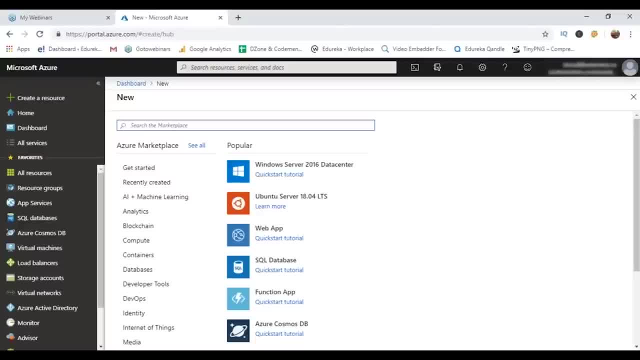 in which you have certain free credits. That means you can use these credits to use these services. I mean, these are paid services, so you can use those free credits to practice these services on your own. I would suggest that, if you do not have a free tier account, 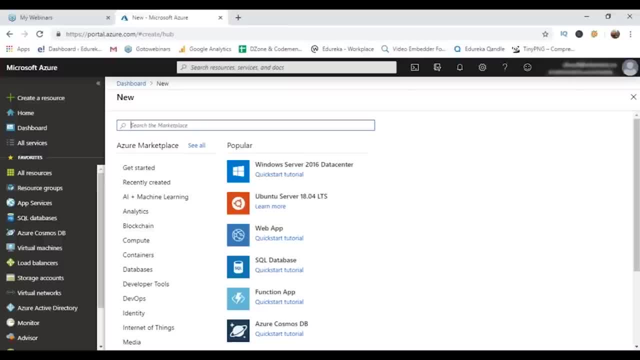 you actually go ahead and create one now. in my case, This is a paid account, So I am kind of restricted to using these applications. So let us just go ahead and create a simple Azure IOT hub first. So, guys, this is the console. 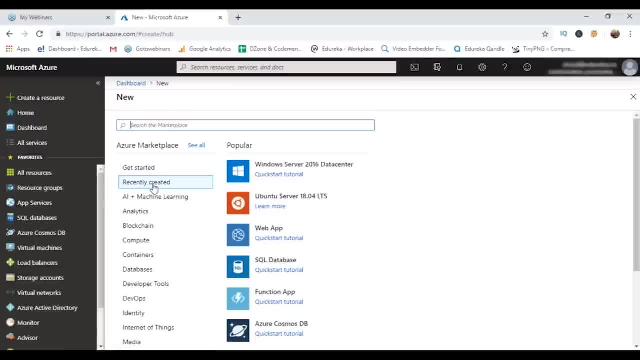 I mean, you have a number of services, whether you talk about your recently created services, whether you are machine learning, analytics, blockchain, compute, containers. Now, these are different domains that Azure touches upon. our concern Today is Internet of Things, So let's just click on this icon and go to Azure IOT hub. 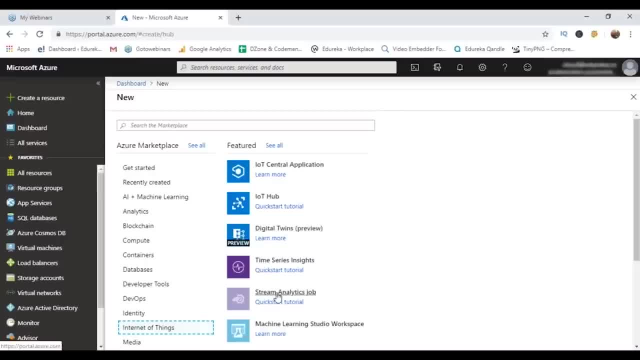 If you move to these different services, you can actually go ahead and learn a lot about them. This is quick start tutorial one for IOT hub as well, So you can know what you can do with all these things or all these services. So when you talk about Microsoft Azure, 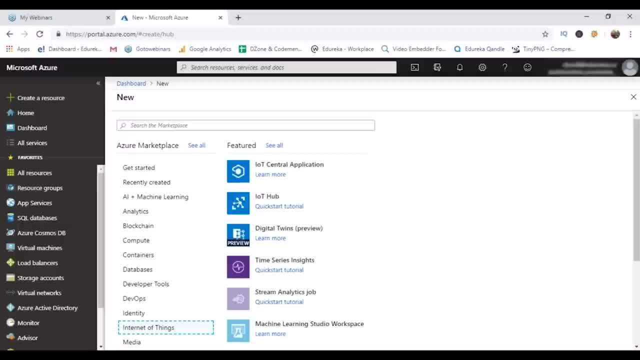 there are a lot of documentations or a lot of documents that Azure provides you for free, So you can use those documents to understand these services to a lot more detail. So I would suggest that you actually visit their website and take a look at those services as well. 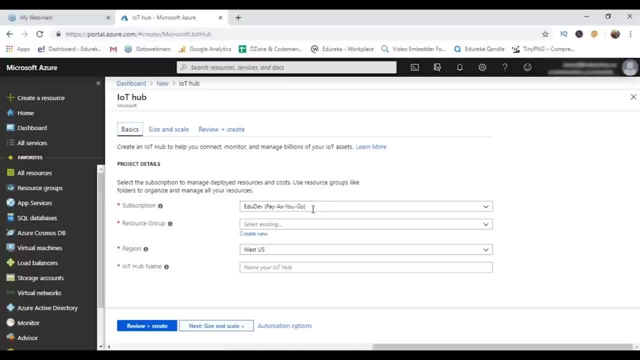 Meanwhile, I've moved to the service. as you can see, the subscription is a direct a subscription here, resource group. I can create one or I can use the existing one. So let us create one As your IOT demo. 1, 2, 3, 4, 5, guys. 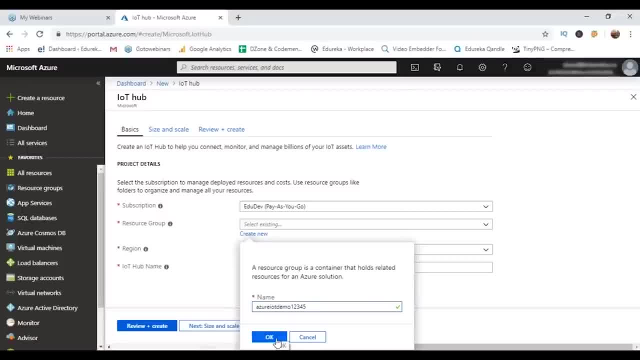 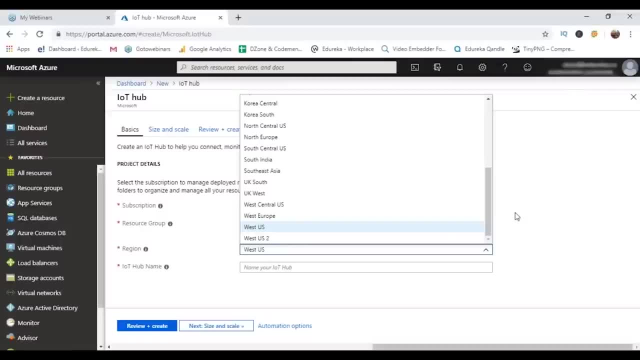 These are unique names, So probably you might be forced to give longer names. Let's just say: okay, you can choose the location where you want to create this IOT hub. when I say location, what does your does is? it has a data centers in different parts of the world. 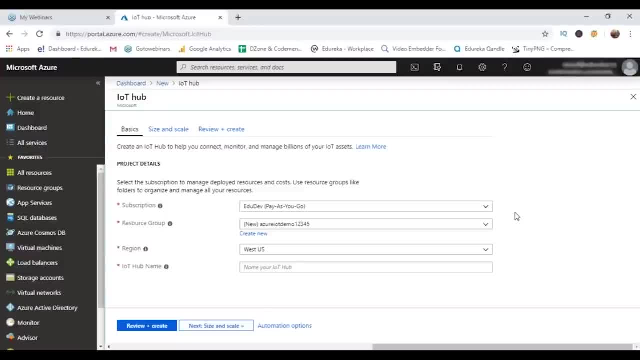 So you can choose the data center that is close to you, or you can choose the data center that is close to your business and accordingly, you can take a call on which reason do you want your data to based in? based on that, You can choose a region. 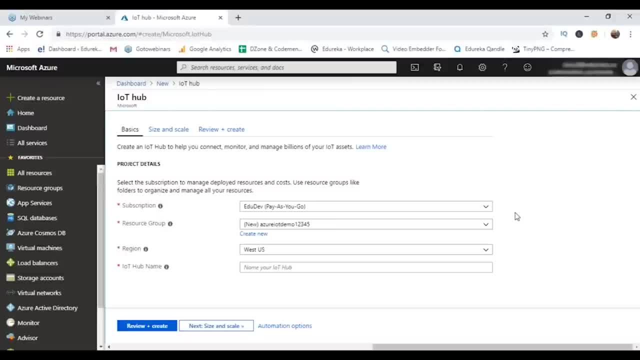 There are certain services for which all regions are not available, So you would want to visit those particular services and decide accordingly. in this case, I'm going to stick to West us. I mean, it's a simple application, So I do not want to put in too much effort or time into it. 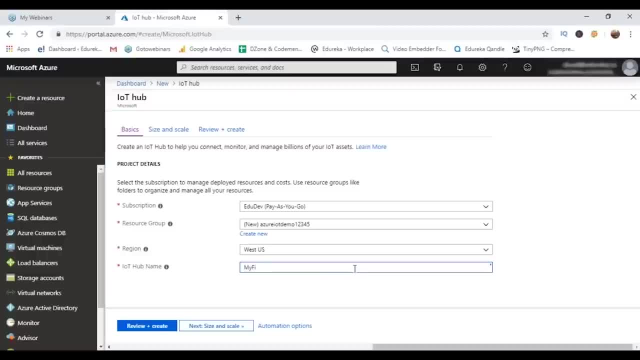 Let's just name our application, as in my first IOT hub. It's not available is what it says. Let's say 1, 3, 4, 4, 2, 2, 2, 1.. Yep, Now it is available, So you can just review it first, right? 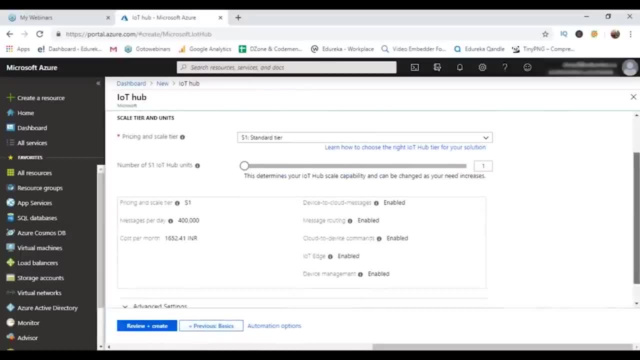 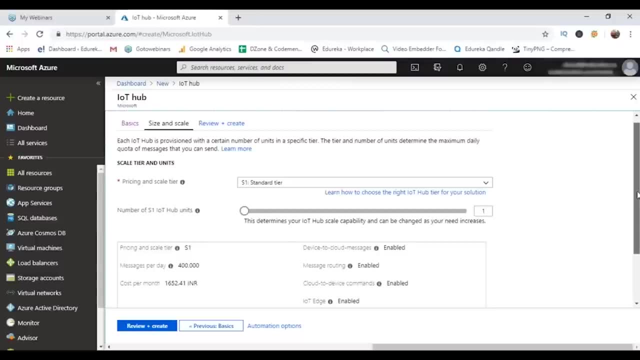 You can go to previous. actually you can take a look at this size and the details you want to enter. pricing tier: It is s1 for me, That is standard one. I won't be getting into the details of pricing. Let's ignore that for now. cost for month. 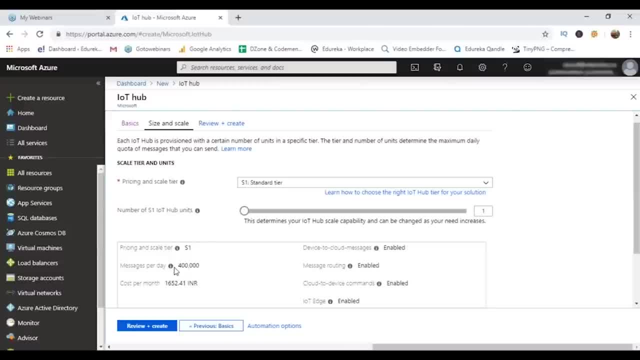 for this device is 1652 INR, that is Indian rupees, and it supports 400 messages. Basically, number of units for the hub- for now Let it be one. you can change it accordingly and you can actually go ahead and decide what year you want to use again. 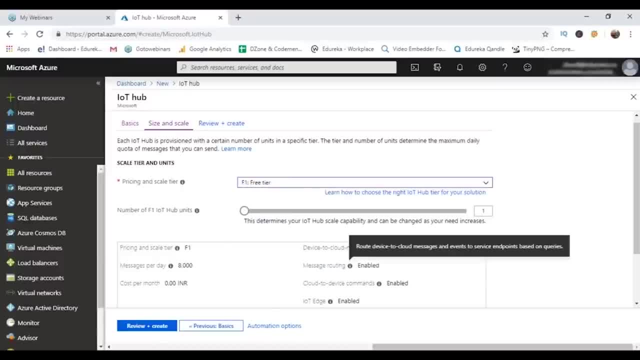 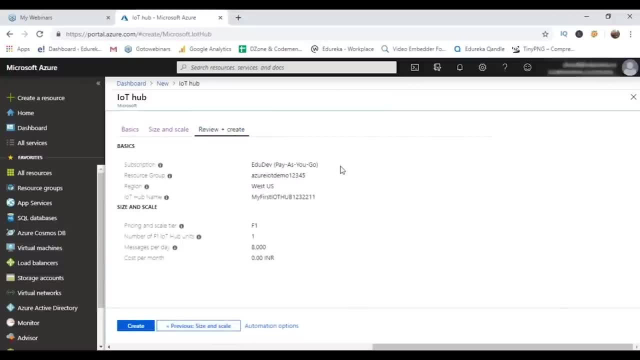 So let's just move to free tier for now, so that we don't get charged a lot, and let us just move ahead and say review and create. So this is the information. This is the subscription. Mine is pay as you go. This is the name, region and the name. 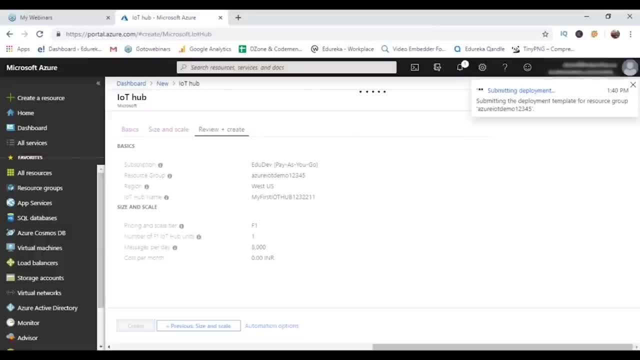 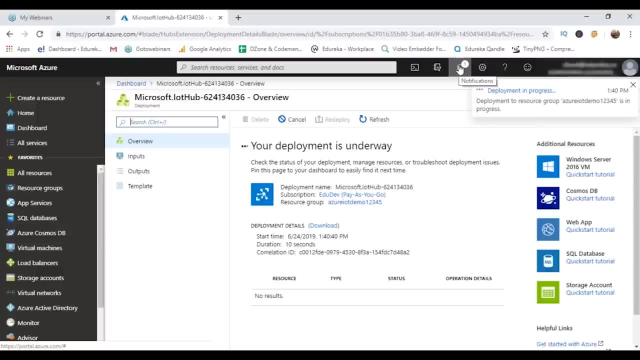 I just go ahead and say: create. So, guys, creation at times might take a while, not long, but a minute or two. So there you go, The deployment is in progress already. It is giving you all the information that you need, and once it is done, you can avail information. 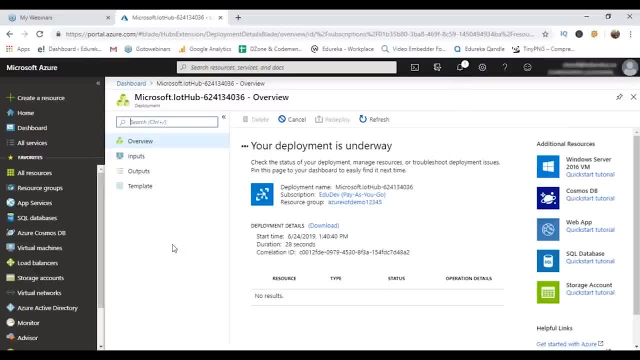 on other things as well. Also, guys, if you are new to edureka or to our YouTube videos, I would suggest that we do a lot of stuff. I mean, we have a live sessions, mostly on Tuesdays, Wednesdays, Thursdays. we have our podcast sessions as well. 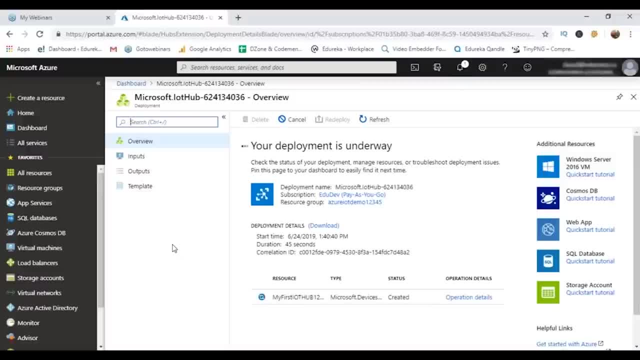 You can actually go ahead and visit our podcast channel where one of our Associates- he- works on great sessions. Then you have live sessions, which I've already mentioned, and there are quite a few other channels like these own medium channels, on IG TV and other places as well. 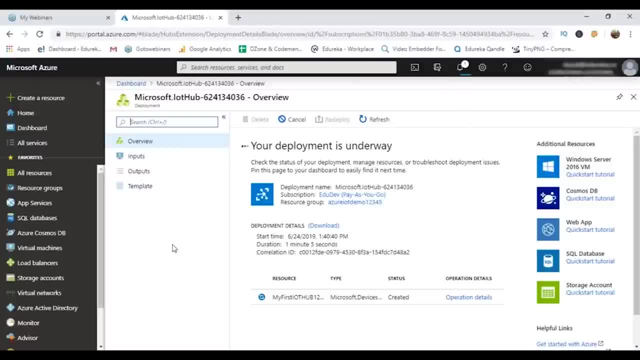 So our presence on social media is huge. you can stay connected to all these media to learn about new technologies. I mean, we upload content on all these platforms every day and especially we started with YouTube. So if you are looking for such content on YouTube, like on regular basis, 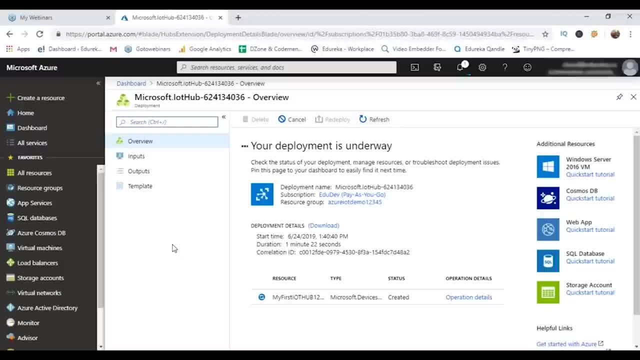 you can actually go ahead and subscribe to our YouTube channel so that you can avail these videos like every day, and also make sure that you click on the bell icon so that you get notified to these videos on regular basis, because there are a lot of resources that I believe would help you in a lot. 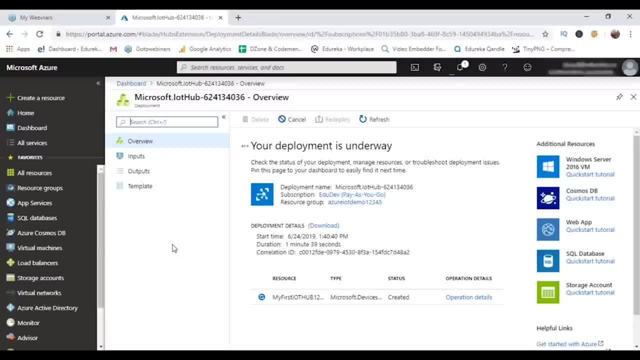 of ways, I would be dropping in the links for the other channels that I mentioned in the description, so that you can actually go ahead and probably sign into those channels as well, like telegram, D zone, IG, TV medium, Etc. As far as this application goes, the process is still underway. 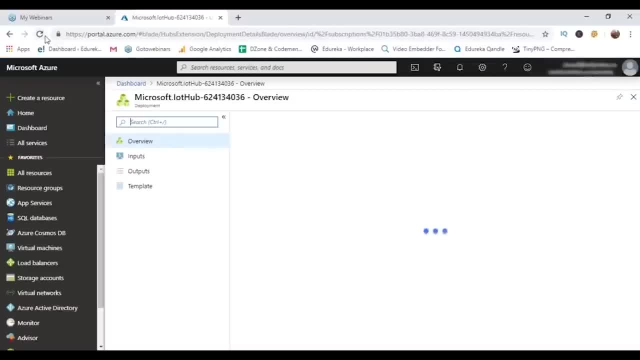 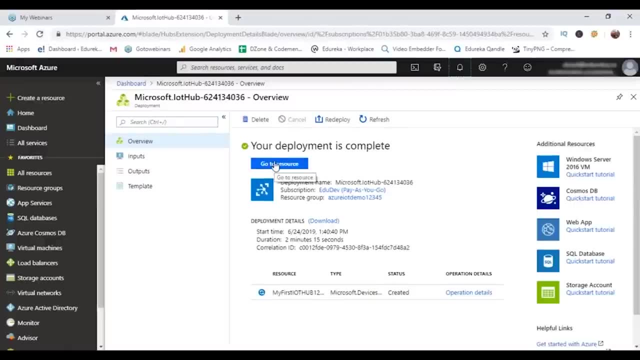 Let us just quickly refresh it and see whether the application is created, whether it's up and ready. No, it's still underway. So there you go, guys: the resources created. you can click on this icon. You can see the information is here, That is, you can have your operation details. 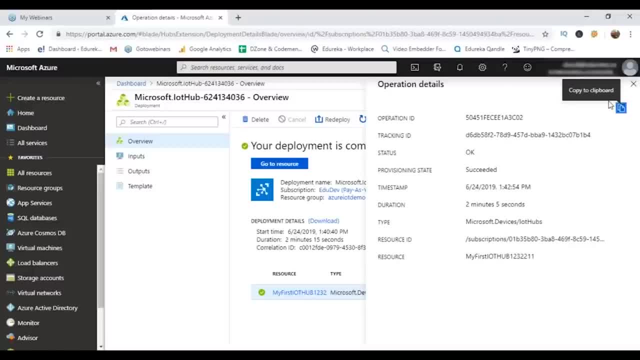 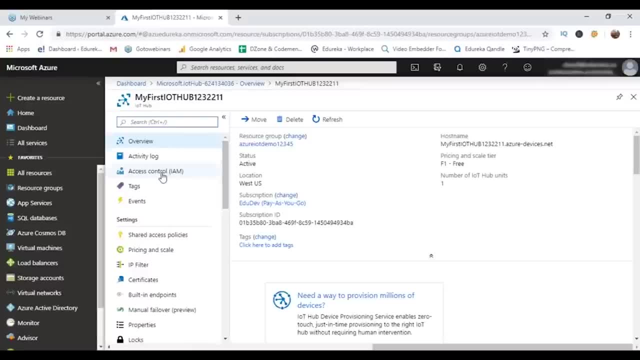 by clicking on this thing and you can get the details about it. You can copy the details as well, You can go to the resource as well, which is here, and, based on this information, you can actually go ahead and decide what kind of access. 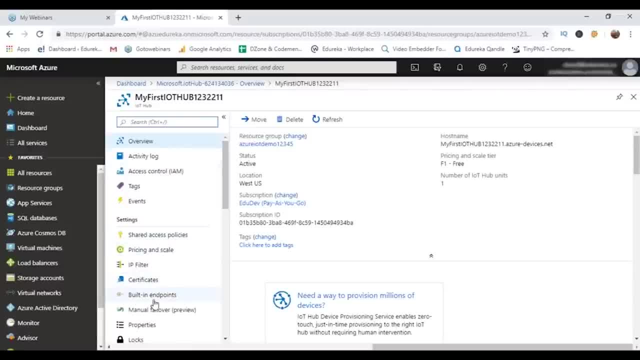 do you want this device to have pricing and scaling? all these things can be taken care of. other information that you need need a way to provision millions of devices. go ahead and see how these things work. So, guys, this is how you actually go ahead and create a basic IOT hub. 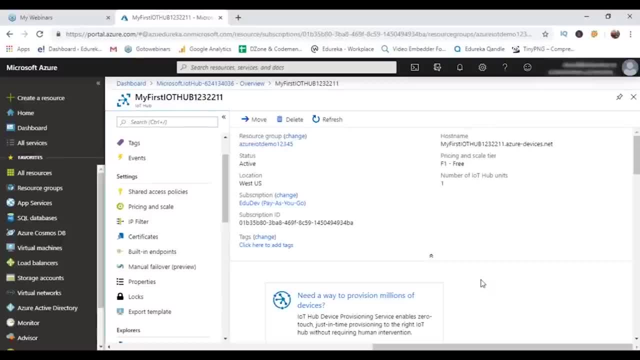 in the following sessions that follow the session probably will be creating a lot more content related to these topics, and I believe these topics would help you a lot more. as far as this session goes, guys, I probably believe this is the end of it before that. 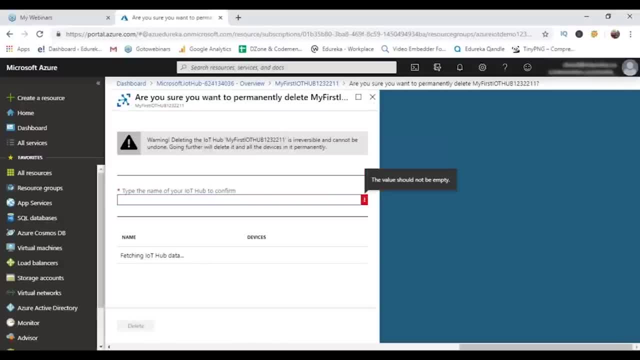 I would suggest that you actually go ahead and delete the resources that you have. you'd have to enter the name of the app that you've created, So let me just go ahead and do that. hub 1, 2, 3.. I've given it a fairly long name. 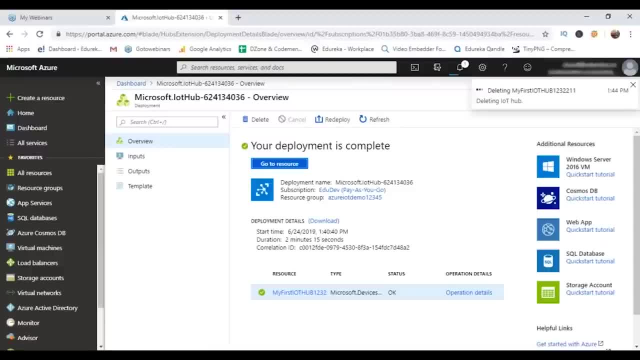 So there you go. There you go, guys. The reason I'm asking you to delete these services is now: this was under the free tier, but probably there are services that would cost you a lot more and say, for example, if you launch a server and keep it running. 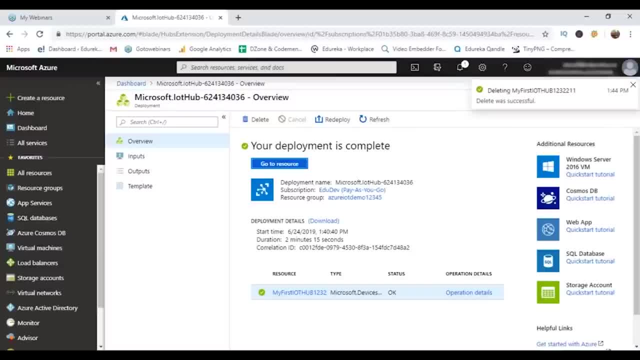 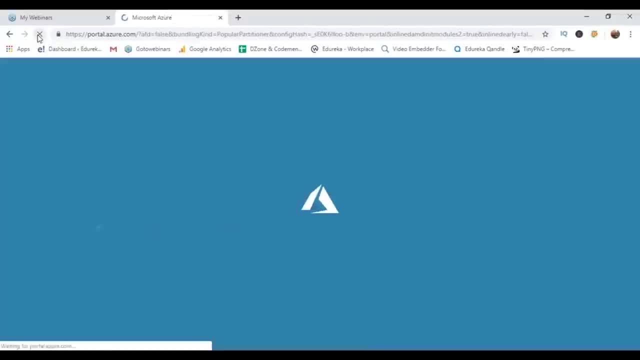 So probably you'd be paying a lot of money, and I don't want that to happen. So it says, is that you always follow this practice where you delete the resources that you've created, and once you do that, it is certain that you won't be charged. 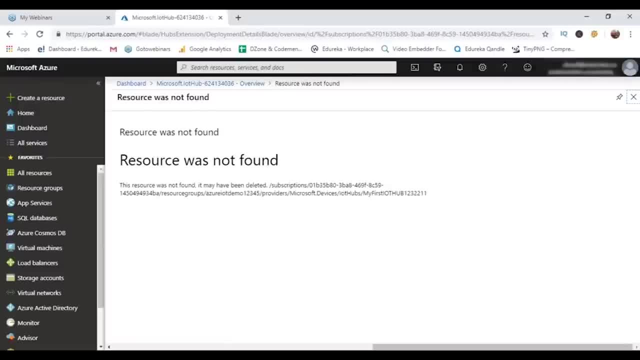 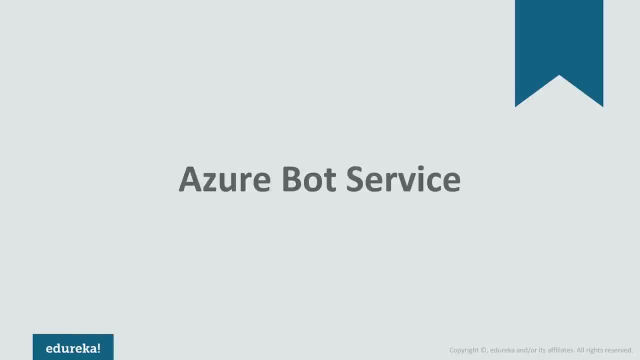 Now you can see that if you go to this deployment, the resource won't be on, because I have deleted it already. Today we are going to discuss Azure chatbots. Can we create chatbots using these cloud platforms? So, yes, we can create chatbots by using cloud computing platforms. 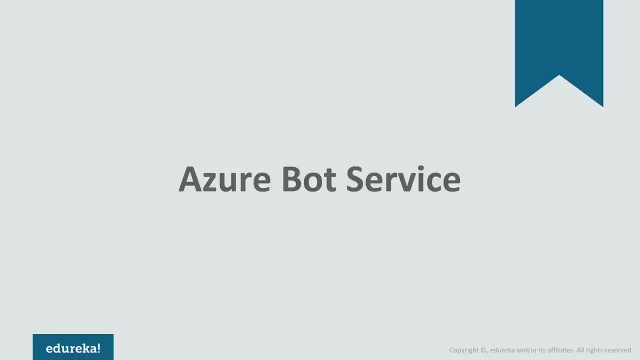 If you talk about AWS, you have a service called as Lex, and if you talk about Azure, it is Azure bot service. So this time around, I thought of using a different cloud platform, and that is why I went ahead with Azure. Let's continue with this session. 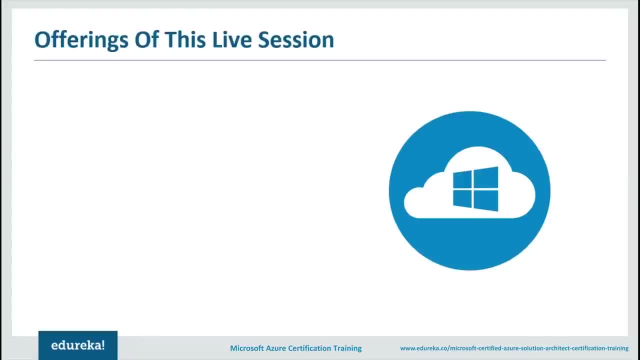 and take a look at the agenda for today's session. Well, as far as this session goes, following are the offerings. we would start by understanding what are chatbots. next, we would understand what is Azure bot service and how can you use it to create a chatbot. 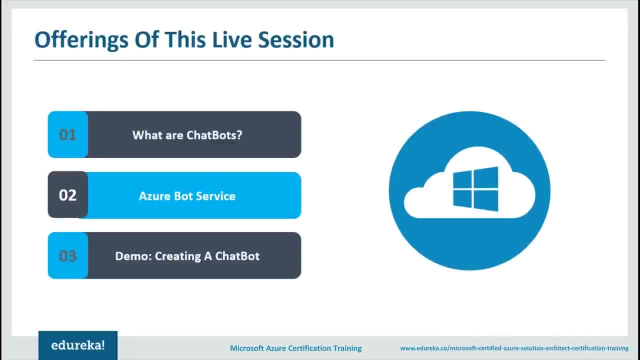 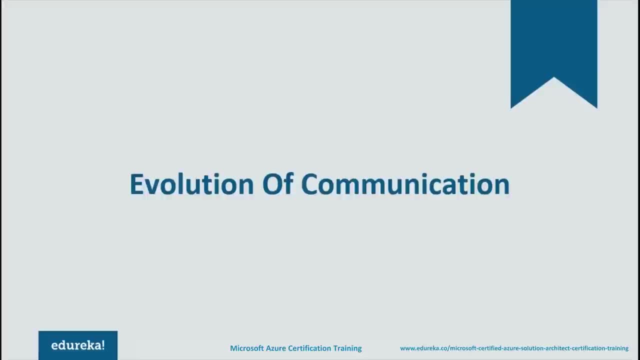 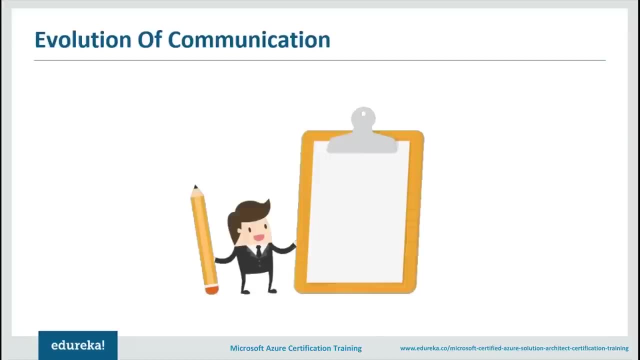 There's a lot more to offer. as we move further, everything would unfold. So let's jump into the first topic of discussion then. First, we need to understand how communication has evolved with time. Now, if you talk about times when I was little, I remember my father writing letters to his relatives. 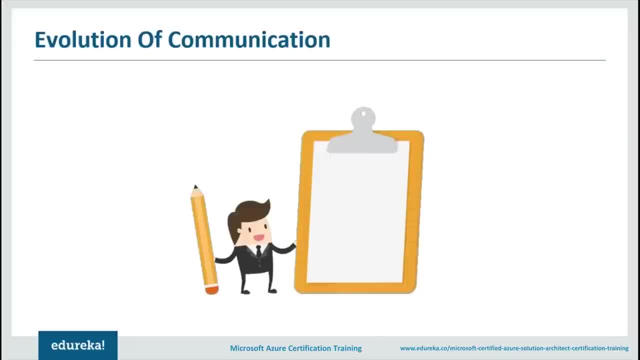 or my grandparents rather. So in order to send these mails or letters, we had to attach those postcards, go to the post office, put the letters there and then that postman would take that letter to the respective party and that party would reply in the same manner. 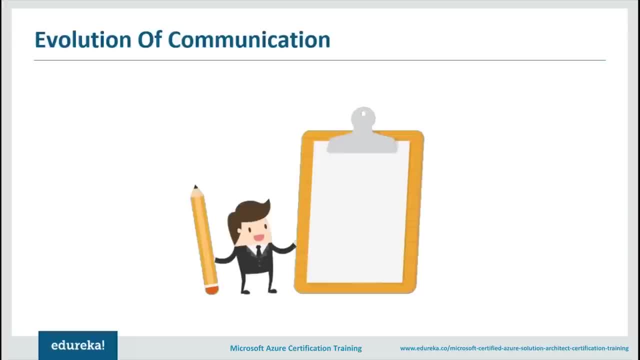 So this process would take days, isn't it? it had its own fun, But if you talk about current times, the technology has evolved a lot and with that The way we communicate with people has changed to. nowadays We have something called as mobile phones right where, if we do have to go ahead, 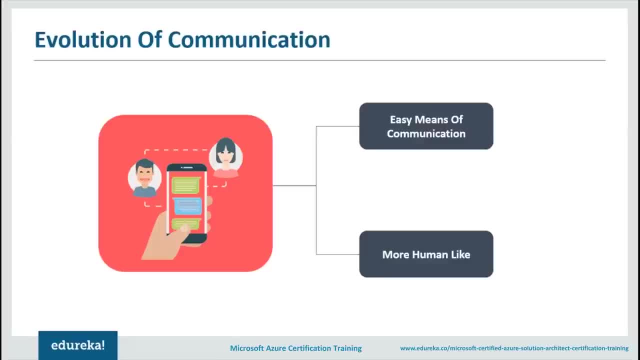 and communicate something to people. all we do is we just go ahead and type in a particular message and it gets delivered to that person within seconds. That is how communication has evolved. and what has this part done? Well, what it has done is it has made communication one easy. 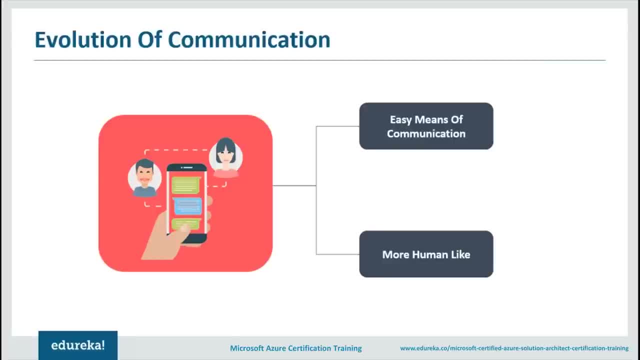 and two more human like. what do I mean by more human like now? I've been in the age of chatting as well And I know that. how do we chat? It's very simple. whatever we have to say, We just type it right, unlike the formalities that we do in other ways of communication. 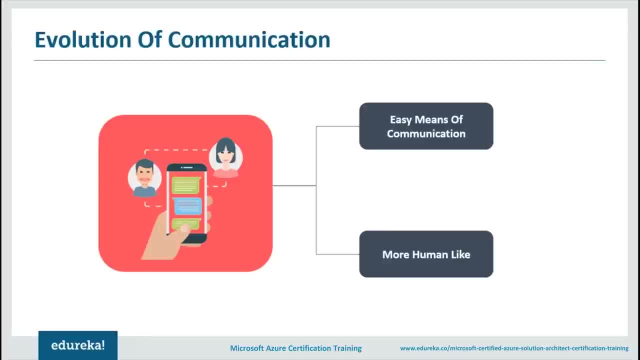 Say, for example: suppose if I have to apply for a leave, what would I do? I would go ahead and type an email, right. in that case I would be putting in the details, as in who it is to be sent to, what is the subject. then I would put: 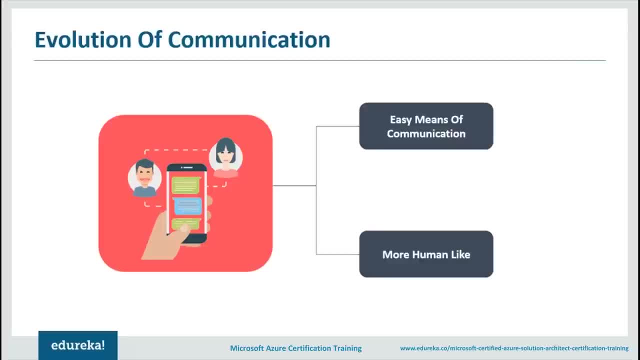 in the details, then I would ask for a leave and all those things I mean. this also is pretty much organized, but then it is too complex, isn't it? If you talk about chatting, it's very simple. I'm not well, I won't be coming today. as simple as that. 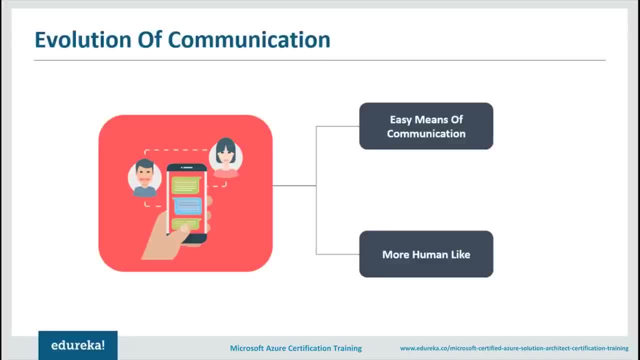 Imagine if we could just go ahead and do this in every aspect of our life. Wouldn't that be easy. Can that be done? Definitely it can be done. nowadays, What people are doing is they are trying to attach communication or implement communication everywhere in such a manner. 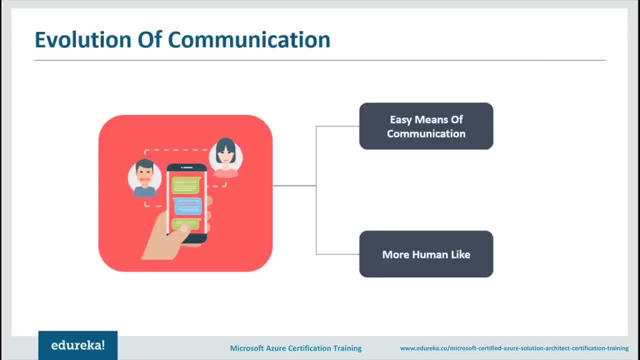 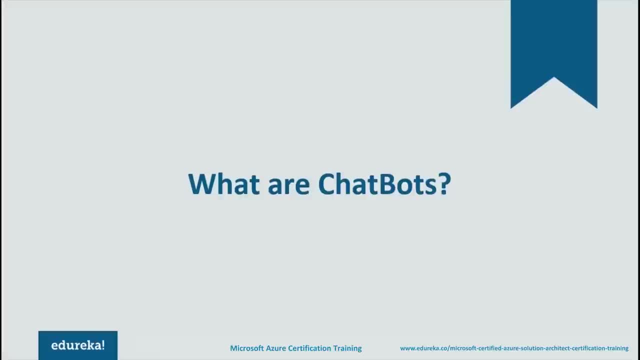 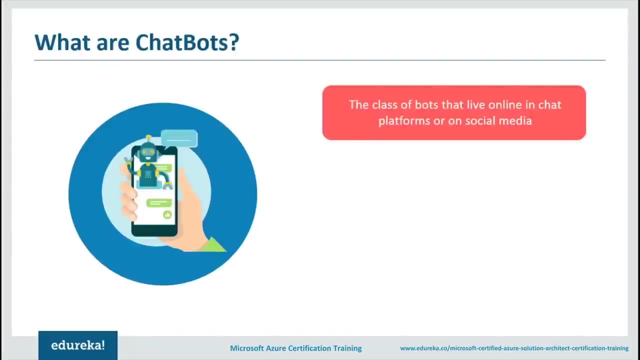 that you can easily communicate with people or with different resources and get the desired result out of it. One of the ways to do it is chatbots. Let's try to understand what chatbots are and how do they contribute to this concept. Well, if I were to define chatbot, 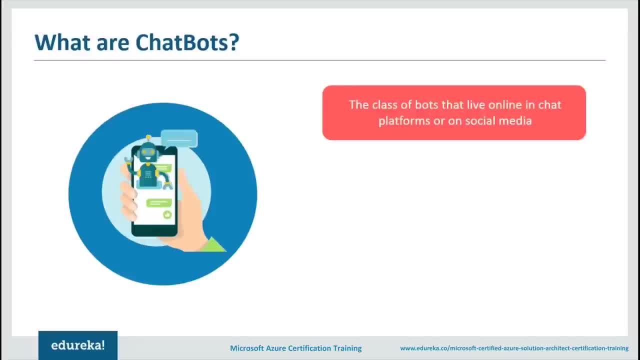 it is nothing but a software that lets me communicate with a human. Now suppose I am an individual and I have certain requirements. Suppose I visit a website. What happens there? a pop-up comes in right saying that: how can we help you? What is the possibility that it is not about? in 90% of the cases it is. 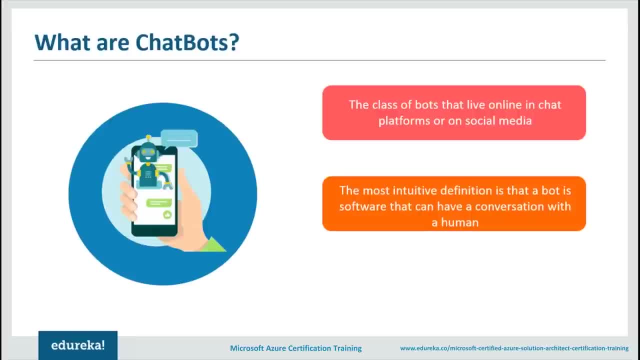 So that is what a chatbot is in more formal ways. It is nothing but a bot or a software that can have a conversation with a human being. Now, there are types of this chatbot. You have the standard chatbots and the self-learning chatbots as well. 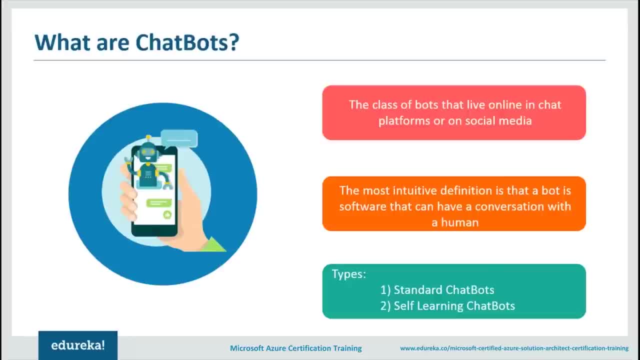 Now, if you talk about a standard chatbot, think of it as a device or a software that learns, not learns, that takes in the data that is given to it, And if a query is thrown at this bot, the machine or the software, I would reply to that individual. 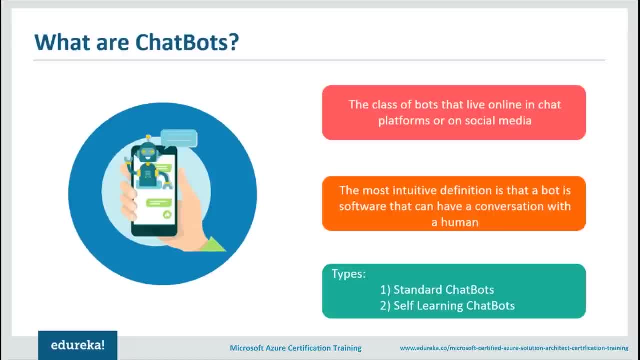 It does not go ahead and make any modification on its own. This is where the second option comes into picture. You have something called as self-learning chatbots. Now, These are the bots that actually take in the data, understand the data and then adapt to that data. in my previous session, 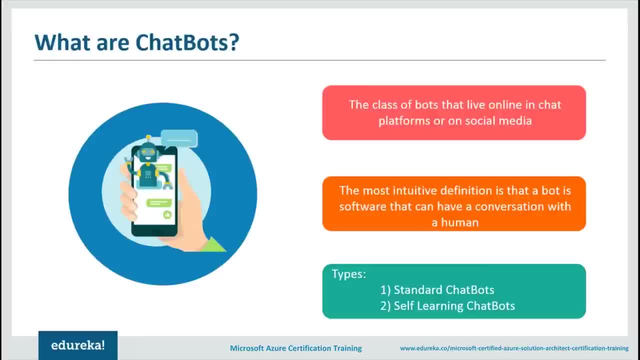 I talked about recommender systems. right, for people who are completely new to the system, Let me tell you what it is now. Basically, recommender systems are nothing, but those are devices, or softwares, rather, that give you suggestions. Now these suggestions are given based on the inputs that you provide. think of it. 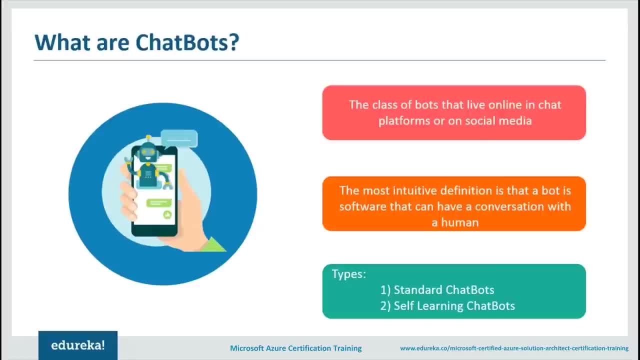 as your YouTube channel, right? I mean where you put in a particular song and you play that song when you do play that song. If you take a look at the suggestions suggestions list, you'd be having a song that either relates to the song that you played or the song that you might have played previously. 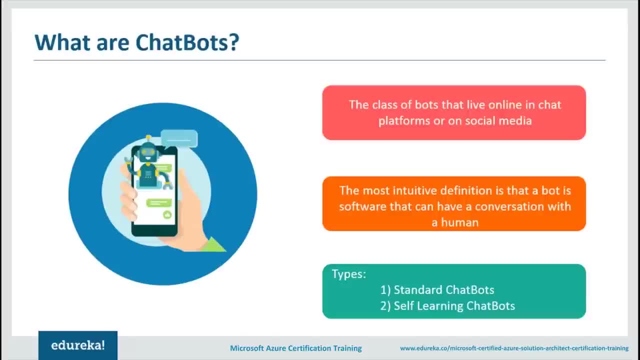 So what has happened here is your so-called recommender system, or the software. it has learned from the preferences that you have given or the browsing history that you have. It also takes into consideration the preferences of other people who chose similar data and, based on that, it gives you an input right. saying that, okay. 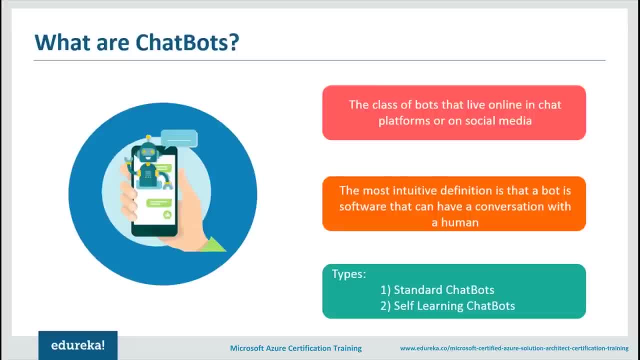 These are the songs that you might like as well. Similar is the case with a self-learning chatbot. What it does is, given the data you provide to it, It learns and it makes the discussion more interactive. to give you another example, Suppose you are. 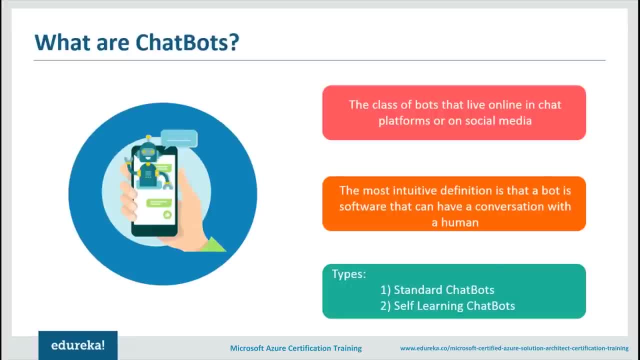 A policyholder and let's assume that there is a criteria that unless you are 18 years of age, you cannot buy a policy at that particular place. Now also imagine that you have this imaginary child or a kid who has turned 18 this year. 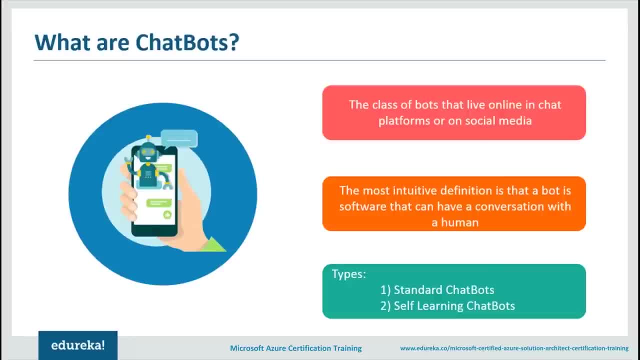 Now, if your data is with this chatbot or with this organization, that chatbot would understand what your data is and next time, if you try to converse with it, it might give you a suggestion saying that: okay, your son recently turned 18.. Would you like to buy a policy policy for him as well? 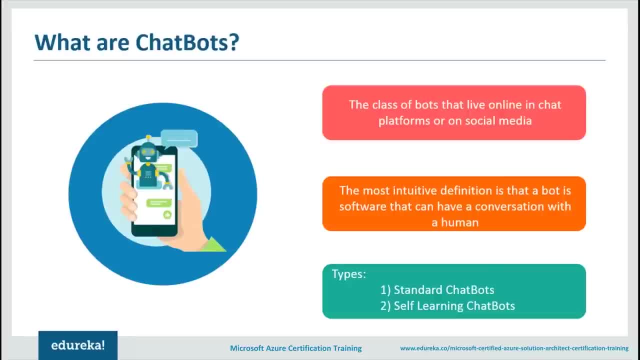 So that is what a self-learning chatbot does. it basically goes ahead, It understands the data and it adapts to the data and, based on this adapt adaptation, It rather gives you a suggestion saying that, okay, This is what would you like to do, this as well. 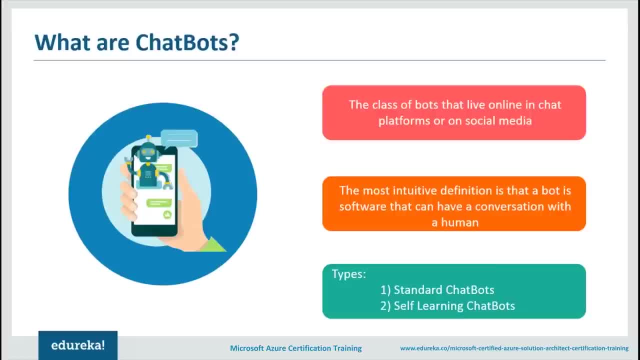 The aim here is to go ahead and make the interaction little more interactive than what it is already. That is why- the reason why this is happening is because, as an individual, we like to have discussion with people. that is how we human beings are: we like to communicate, and the aim 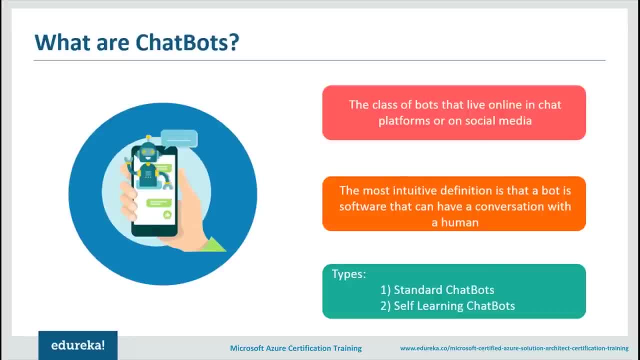 Of chatbots or these softwares is to make the conversation as interactive as possible. Plus the fact that we have chatbots everywhere, what companies are trying to do these days is they're trying to make their working lot more easier instead of just giving you information. 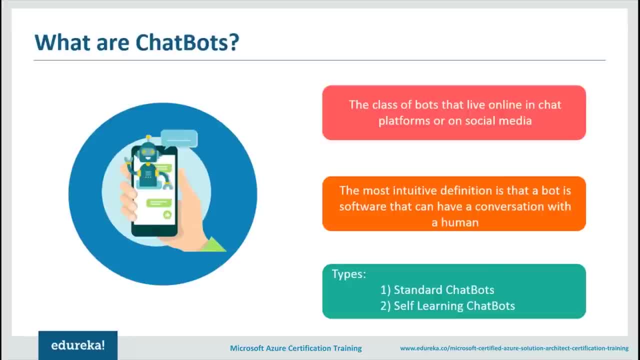 They're trying to understand your requirements and, accordingly, give you solutions, So you do not have to go through the documentation and all those processes. So this is what chatbots are basically. those are nothing but softwares that try to understand the data that is given to them. 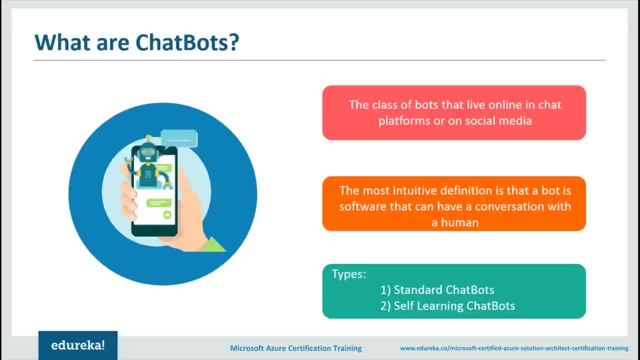 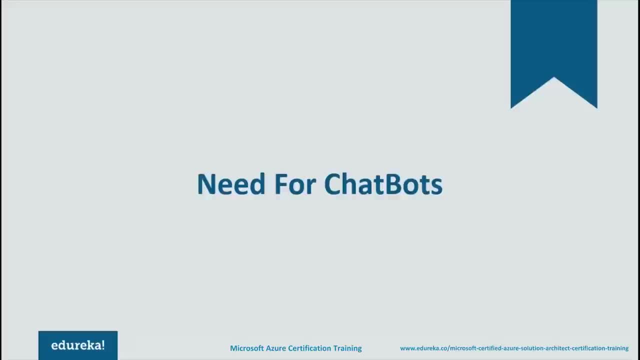 And based on that, they would either give you an answer or a solution to the problem that you have. Let's try to understand chatbots and the concepts that surround it a little more. So what is the need of chatbots now? I've already discussed quite a few reasons as in why do you need chatbots? 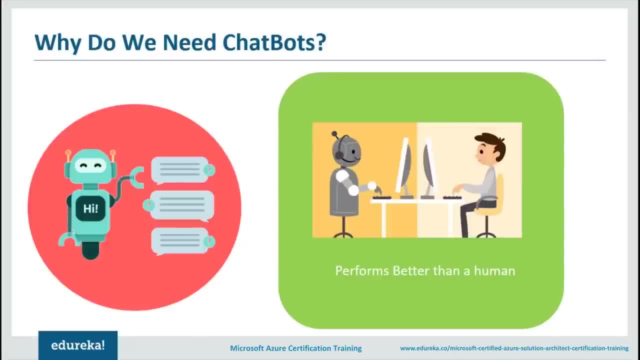 but there are some other reasons as well. Most important reason is, when you compare it with a human being, a chatbot performs better. How is that? now There's no computation to no competition to human brain, Right, I mean? we all know that it's a great thing. 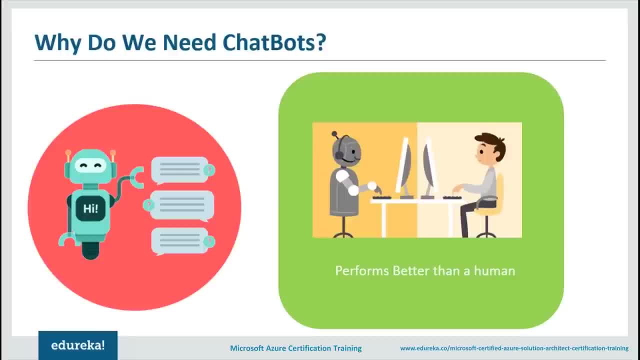 and it is the thing that actually created your chatbot. But if you talk about precision and performance, if you have a software that has been trained that could actually give you better application and better throughput, How is that? Let me give you one more scenario. the next point that is easy to replicate: 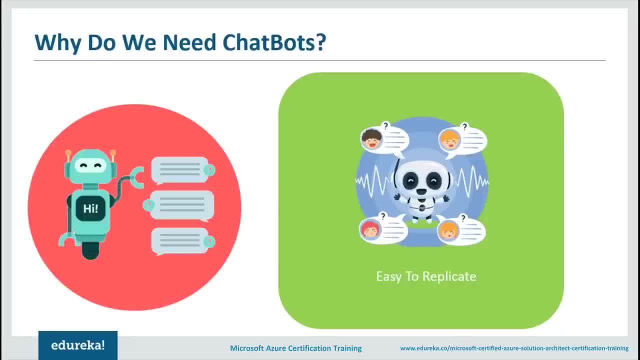 What do I mean by this? now Suppose I have a human being who is setting and answering certain queries. no matter how great or how brilliant That individual is, if I throw like 20 queries parallelly to him, He probably would be able to answer four to five queries right. 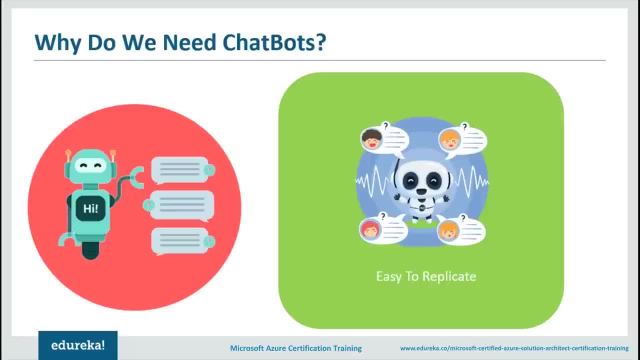 So this is where a chatbot is different. I mean, I can train, I can create one chatbot, I can program it in one way and then I can train it for 20 different services. So when 20 different queries come in, I have 20 chatbots that can actually do the job that is needed. 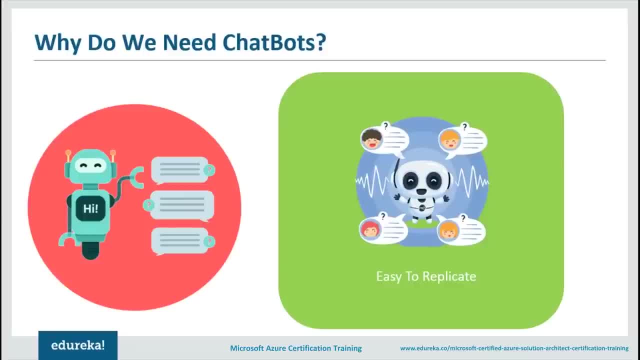 So, when you talk about parallelization, this is where chatbots come into picture. So these are some of the needs. apart from that, the major need is to make interactions lot more interactive than what they are. So, yeah, this is what chatbots are and we are going to go ahead. 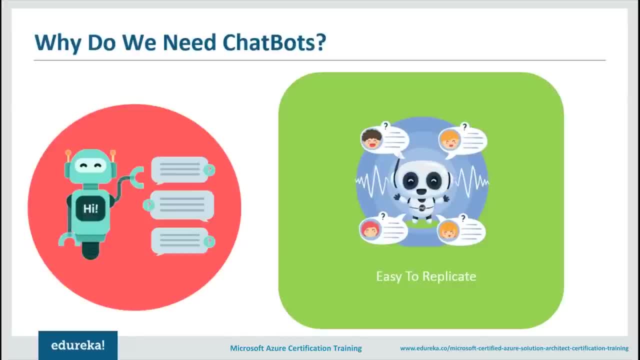 and implement chatbots by using Microsoft Azure, and in that we would be using a service called as Azure bot service. So let's try to understand what Microsoft Azure is, and then we can move into the demo part, where I would be talking about the bot service. 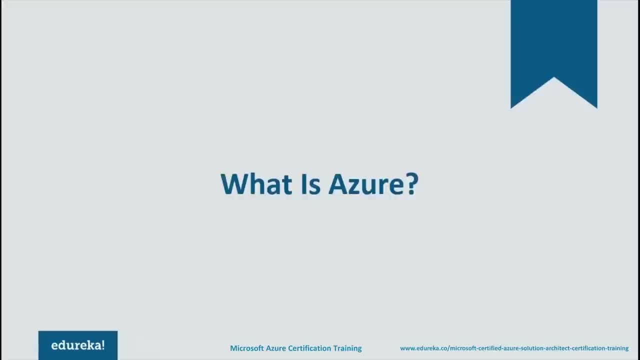 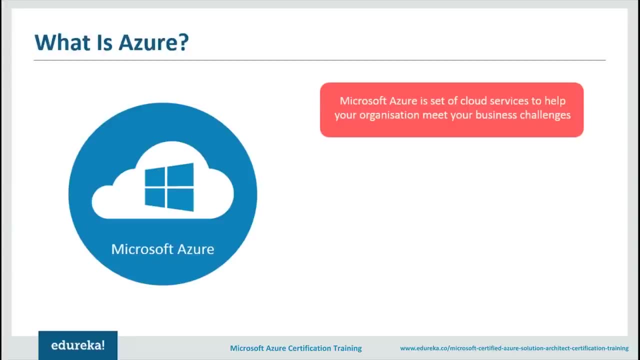 and how to build a chatbot. So what is Azure? Well, Azure is nothing but a cloud service Provider. now, if you compare it with Amazon Web Services, it again is a great cloud service provider, just like Amazon Web Services, and it has a plethora of services to offer to you, whether you talk about your storage services, 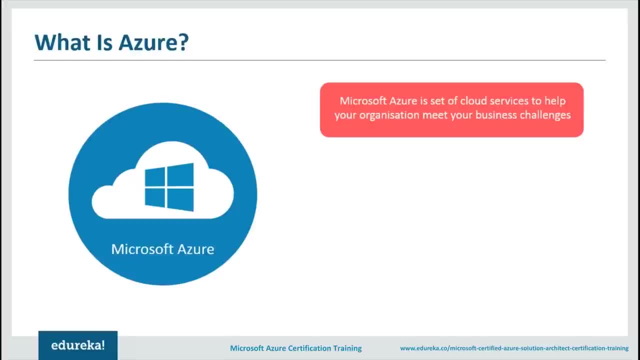 compute services, security services, whatever service it is- everything is taken care by Microsoft Azure, and what it does is it lets you create applications, deploy them, maintain them, monitor them and also keep them secure. The best thing about Microsoft Azure is it is a Microsoft product now. 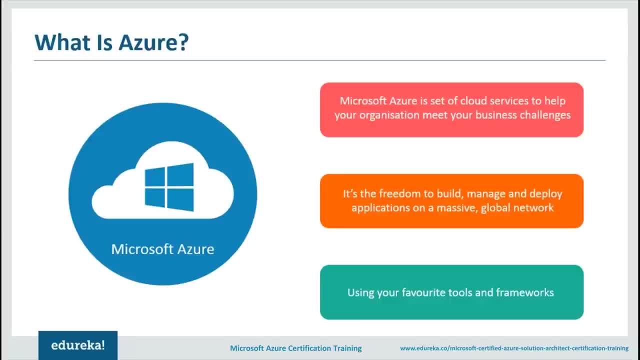 When you talk about Microsoft, we all know that the plethora of applications or the Microsoft stack of products that is there, We all know that it is huge and what that means is there might be some software in your life which you are using and that has something to do with Microsoft Azure. 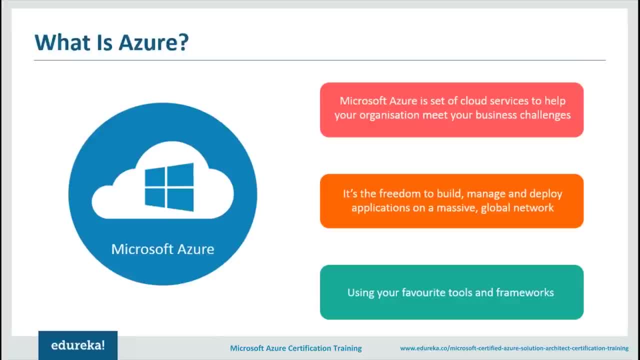 So if you are moving to cloud, you would want to use, or have the ability to move your so-called application, or have the freedom to implement your applications that are there in Microsoft onto your cloud platform, isn't it So if you are using Microsoft Azure? 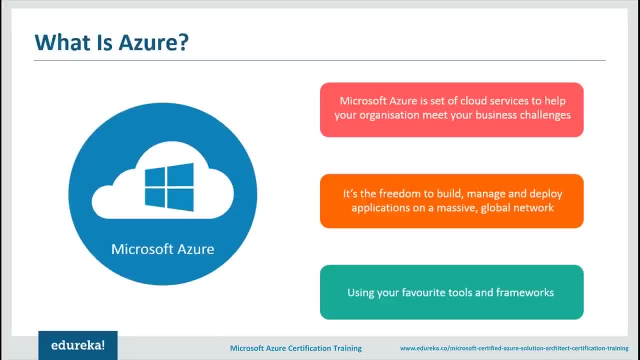 it becomes easy Here to migrate all these applications or integrate these applications to Microsoft Azure, So it actually gives you a freedom of using your favorite tool or your Frameworks on Microsoft Azure. So yeah, that is what Microsoft Azure is and, as I've already mentioned, it is a very popular cloud service provider. 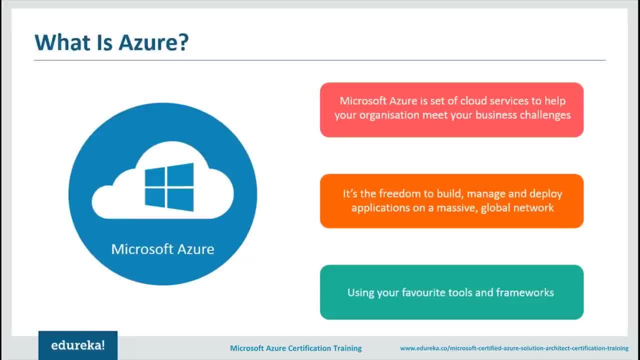 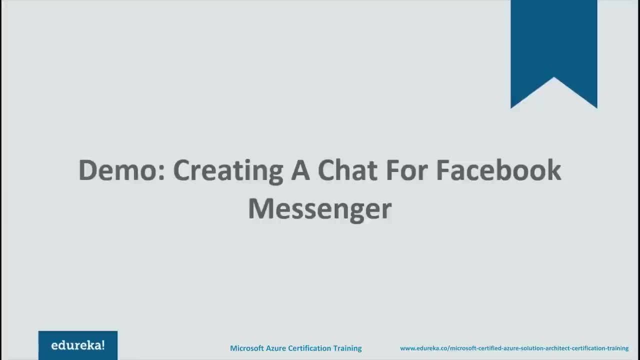 in this case, We would be using Microsoft Azure bot service in particular, and using that we are going to go ahead and create a chat bot. So that is what we have for the demo part. Let's just switch into the console of Microsoft Azure and let's take the discussion forward there. 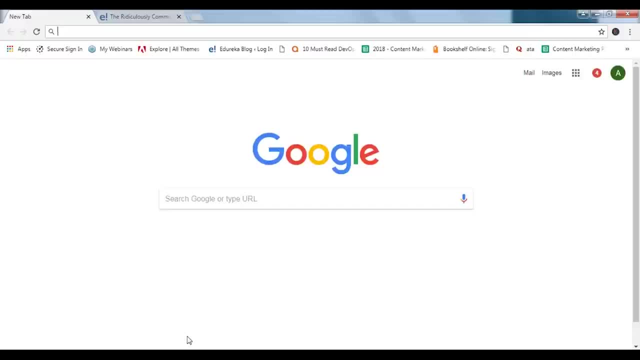 So yeah, guys, let me first give you a scenario as in what are we going to do now. now, when I talk about creating a chat bot, what is going to happen here is: first, I need to create a chat bot and in order for that chat box to work, 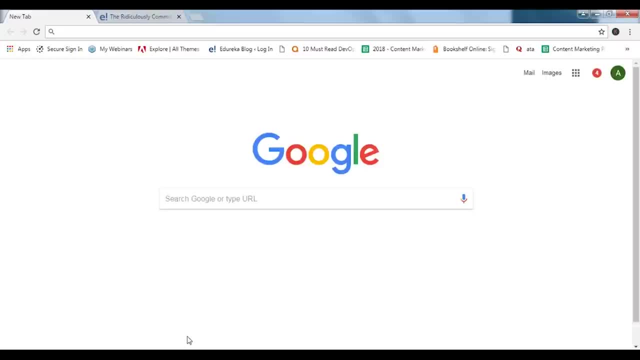 What I'll have to do is I'll have to go ahead and create A source or some data source from which my chat bot would learn, Isn't it? I mean, it needs some data, right? So for that we need to create something called as knowledge base. 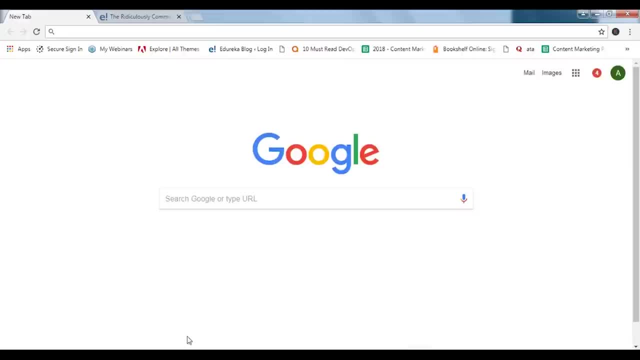 Now your knowledge base is nothing but basically a set of information. It can be achieved from anywhere, Maybe a URL that has pages or two where the information is given, or it is a document that you own, So we will be using that document or that URL and using that URL. 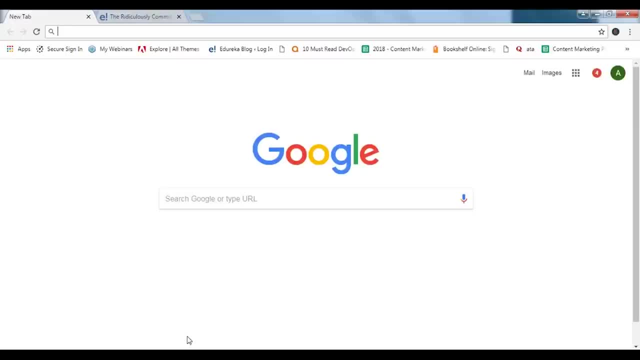 We will take in the data and we would create a knowledge base. once the knowledge base is Ready, we would go ahead and switch into Microsoft Azure portal and there we would be creating A chat bot. Now, what we would be doing is we would be giving that chat bot that information. 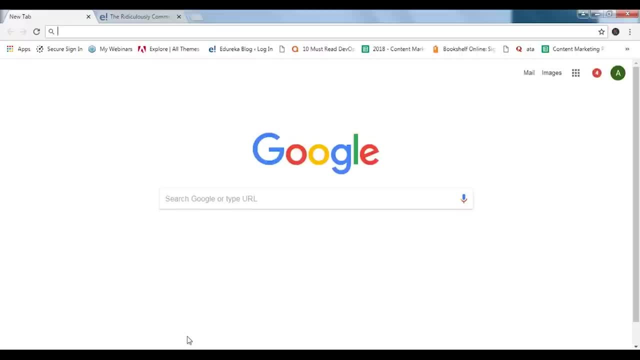 and then we would test our chat bot as in whether it works perfectly or not. Once we are done with this, I'm going to take it a step further, where I would be going ahead and integrating my chat bot with my Facebook Messenger app. So stay tuned and let's implement all these things one by one, first and foremost, 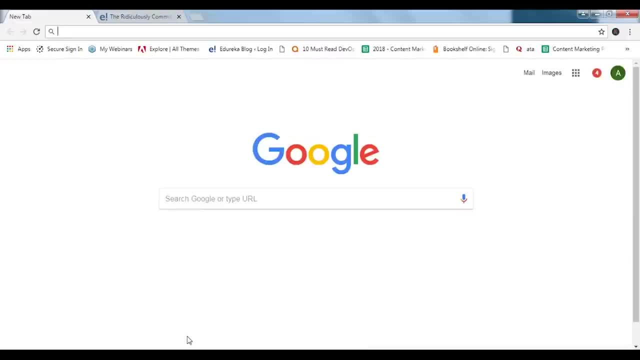 Let's start by creating our Knowledge base. for that We have to go to this URL. that is QnA maker. Bear with me, guys, If my internet is little slow, it might take a little longer than normal. So this is what we have here. 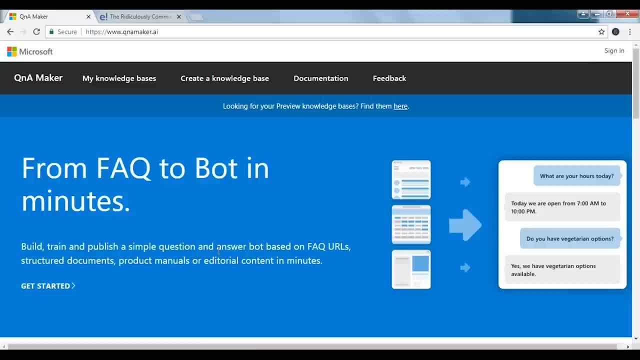 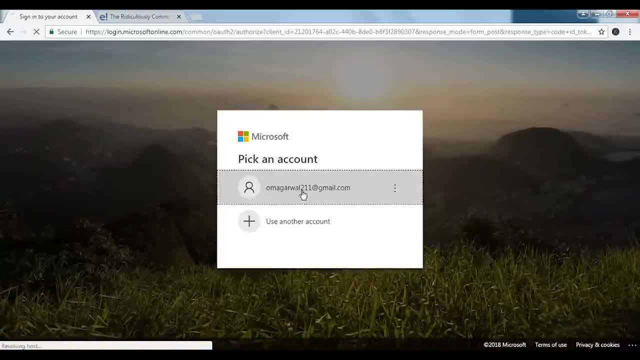 That is wwwqnamakerai. Now, if you come here, you can create your knowledge base. If you click on this icon, it would say create a knowledge base. Okay, I have to sign in every now and then. that can be irritating. 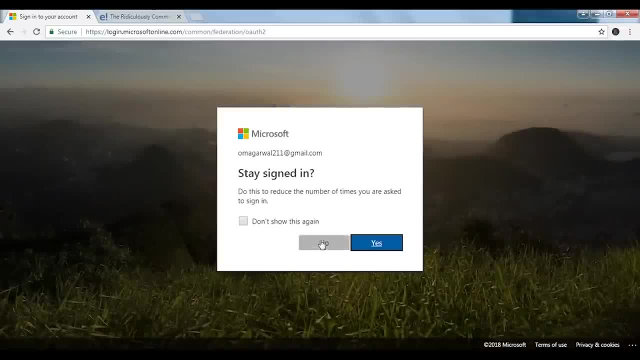 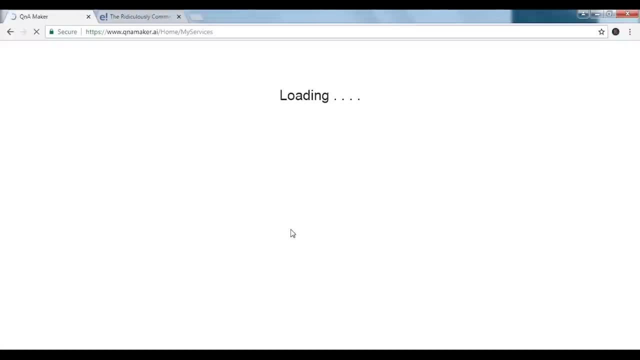 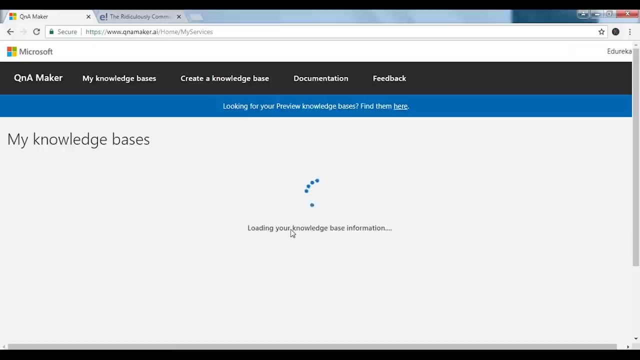 Why say sign in? No, I don't keep it signed and that is why it asks me every now and then, but that way I feel it's safer. There you go. might take a minute or two, Probably lesser than that. First, it would check whether I have any knowledge bases that are there with me already. 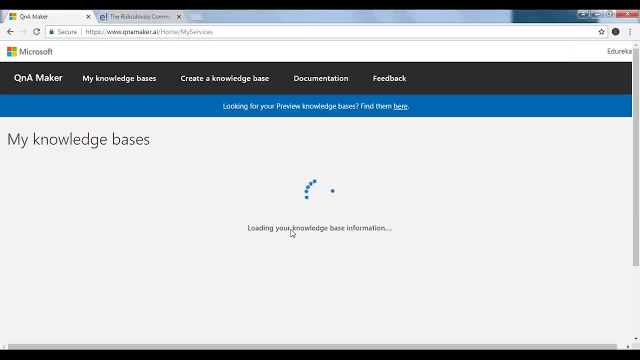 If not, it would ask me to create a newer one. So that is how it works, guys. Microsoft Azure at times takes a little longer time to load. that depends on various sources. I won't get into the details of that. So if that, 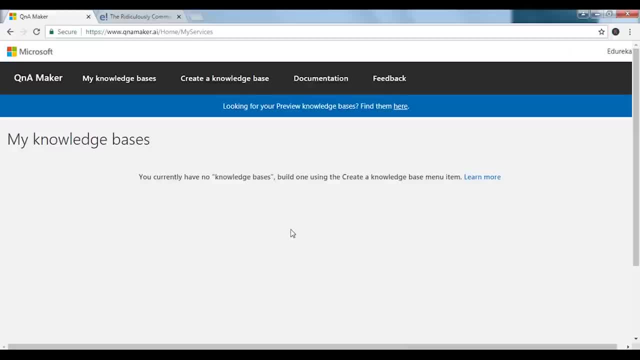 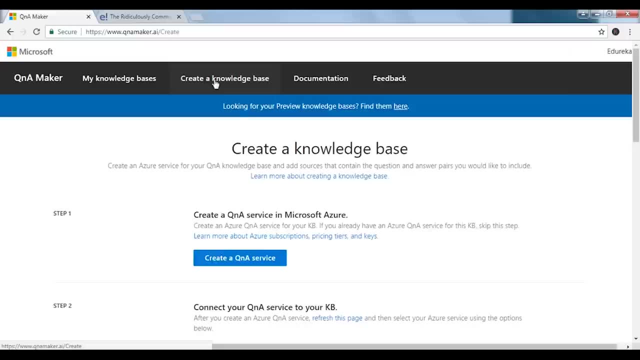 happens, don't worry, I would be keeping keeping you engaged and we'll be discussing something Meanwhile. so there you go, We have this thing here. I say: create a knowledge base. Okay. so, guys, we are creating a knowledge base, right? 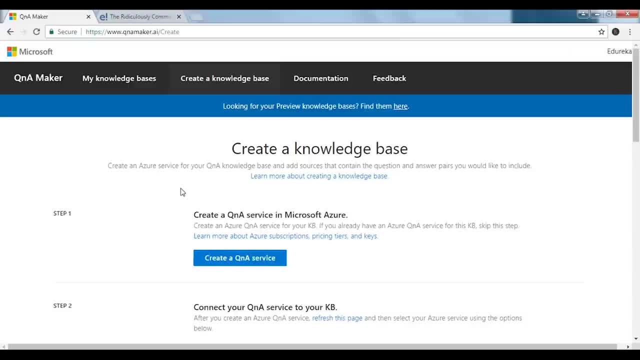 So, since we would be putting it on Microsoft Azure, we would be needing a service that is there on the platform that can attain to this knowledge base right? So for that we have to create a Q&A service as well. So let's go ahead and create that service here. 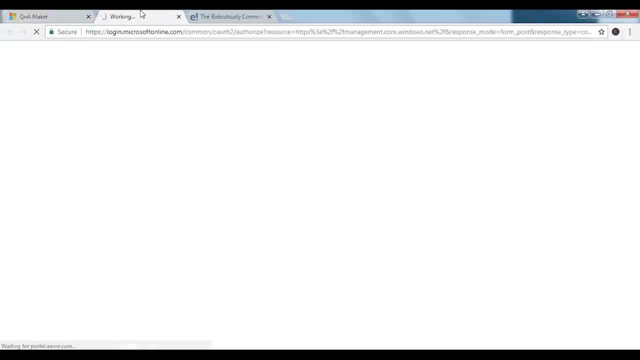 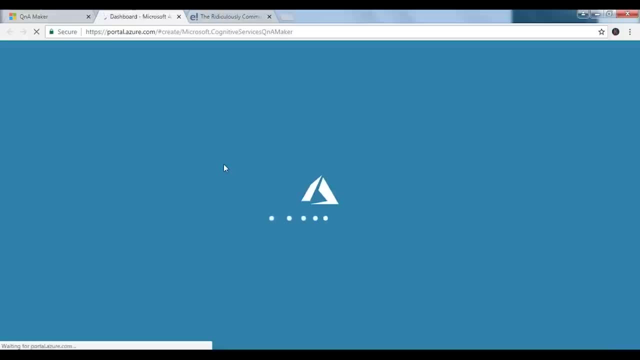 If I click on this icon, it navigates me to Microsoft Azure account. Now, I've already signed in, So it would directly take me to the portal and it would open that tab where we can just go ahead and create this so-called Q&A maker. 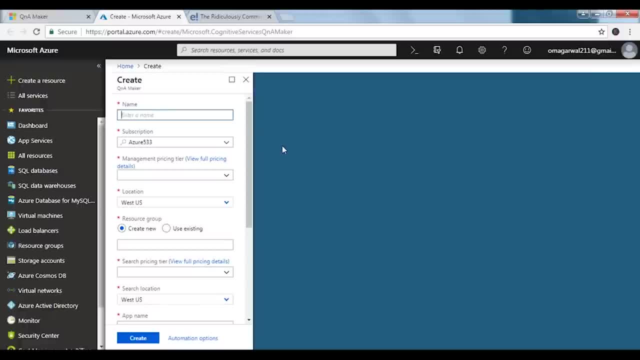 If you want to visit the website first or the portal first and then open this thing, you can type your Q&A maker and it would take you to this page where you can click on create and then this would appear. So this is the Microsoft Azure dashboard. 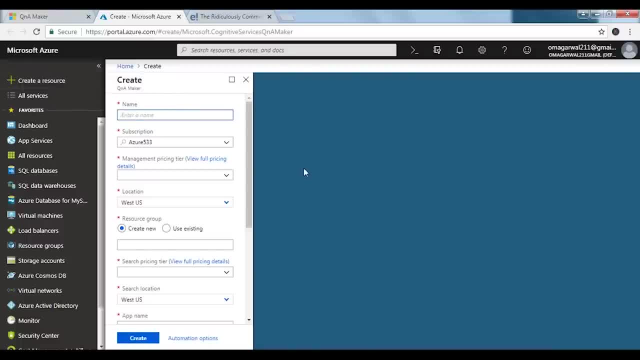 We will be talking about it, Do not worry. So we are going to go ahead and create this Q&A maker service. Let's call it, say, demo: 1, 2, 3, 4, 5. 1 1. subscription. It's Azure 533 standard. 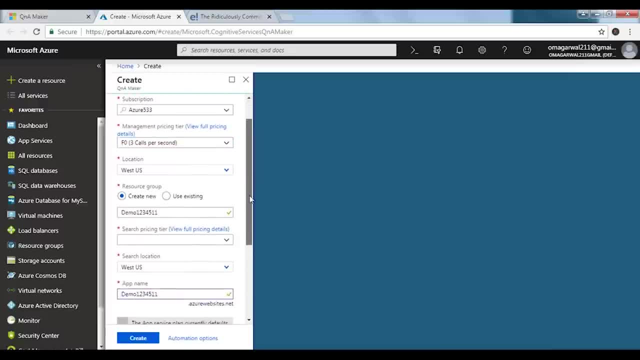 What is the payment here? I want keep it standard again, and location is West US. Let me prefer that now. your chatbot service is not available everywhere, So you would be wanting to be careful while you select the regions. Okay guys, resource group. now it by default takes the name. 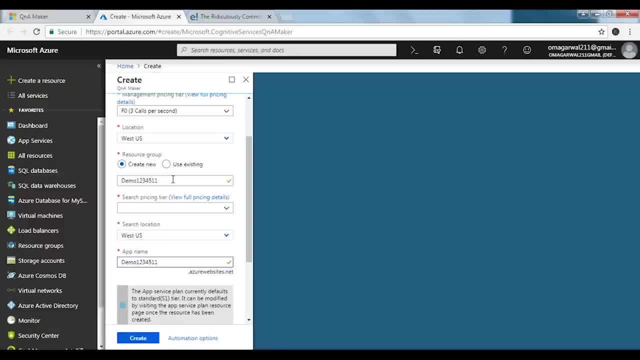 Of my Q&A maker name and it replicates the name. You can actually go ahead and use an existing resource group If you have one. if not, let it create one. So what is a resource group? Basically, it is nothing but think of it as a container where certain resources are put in by Microsoft. 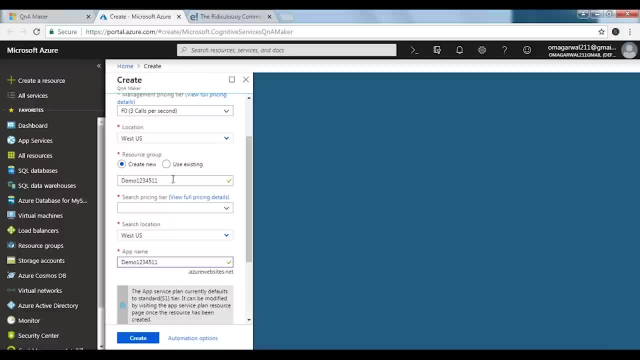 Azure. So when you do create a service, along with it it has to have a resource group attached to it. So each time you have a service, either create a new resource group or use the one that you already have and that suits your needs. in this case, 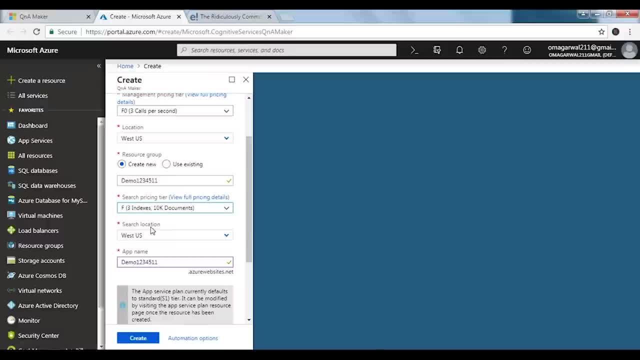 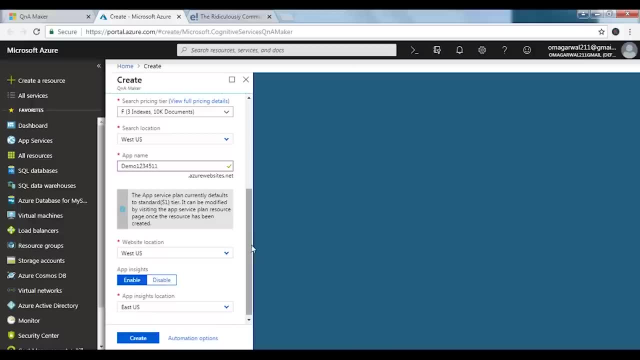 We would be creating one. Once you do that, come here and select this thing: demo 1, 2, 3, 4, 5.. Everything is okay. West US is the region. West US is the region again. So, guys, everything is pretty much in line. 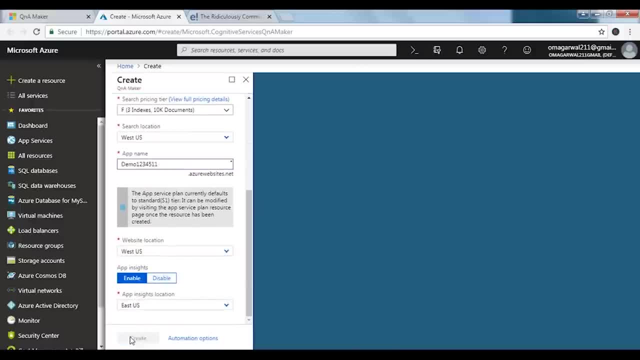 There's nothing that we need to discuss here. Let me just go ahead and say create. Yeah, so it would just go ahead and create this thing. once this thing is created, we can actually go back and then select this: Okay, it's deploying. 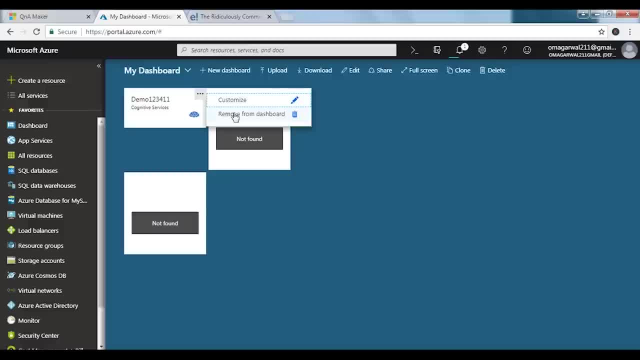 Now, These are some of the applications that I created in the past. I do not need them right now, So I'm just going to go ahead and remove these. Meanwhile, my application gets created here Service. rather Okay, it's deploying. 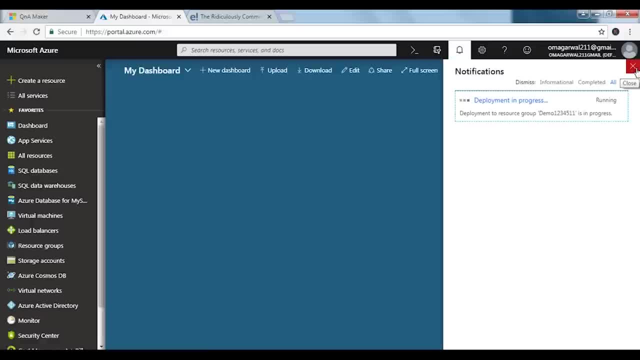 So, guys, as I've already mentioned, at times it takes a longer while. So, yep, this is what might happen here. might take a minute or two, or half a minute if we are lucky enough. So once we do that, you're going to come back here. select all the resources. 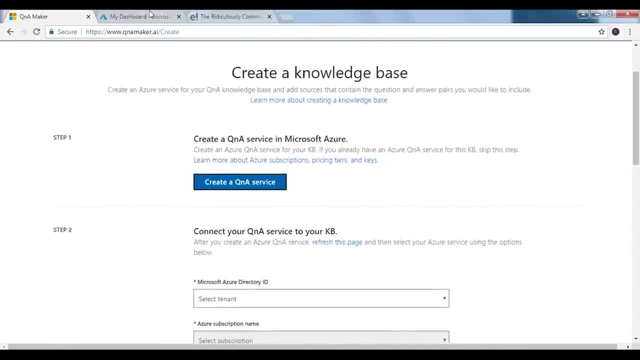 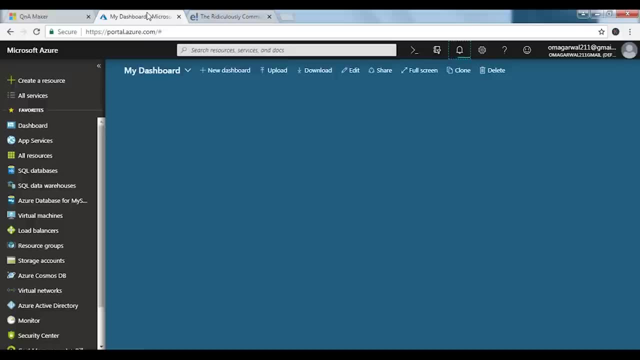 and then we are going to create a knowledge base. Now, what happens here, When you do create that knowledge base, basically what your Microsoft Azure does is- or your QA maker does- is it fetches the data from the source that we are generating or the source that we are giving. 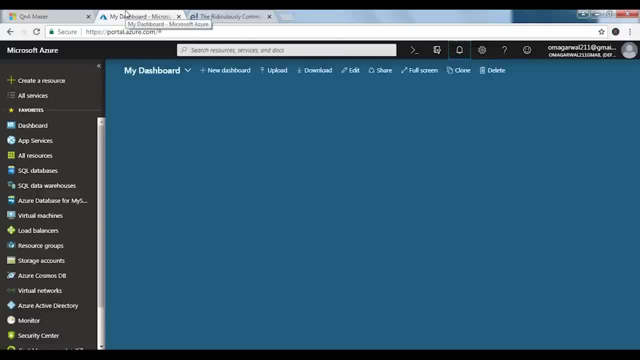 now, as I've already mentioned, you can either go ahead and probably given a document or you can select certain URL. in this case, I'm going to go ahead and select a URL. So what kind of data would we like? if we have some FAQs, that would be better, right. 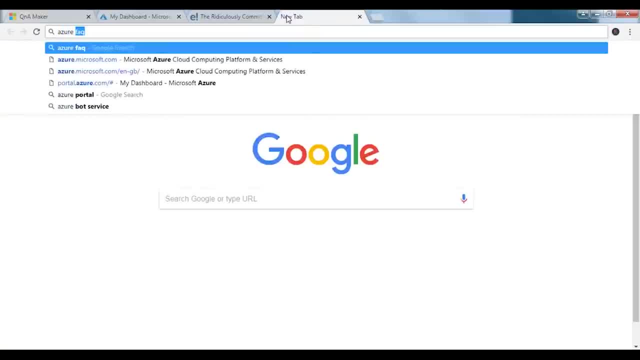 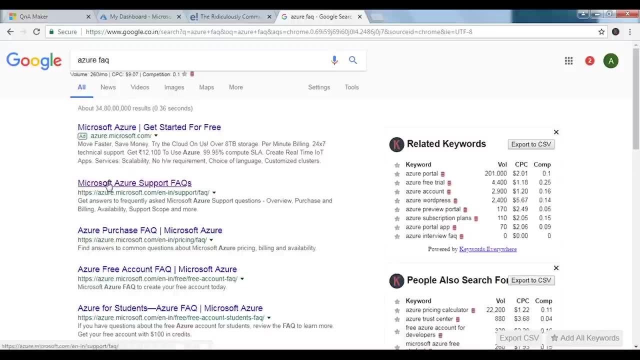 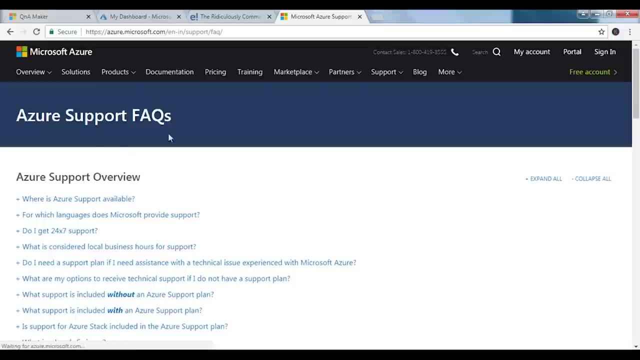 So let's go ahead and select some FAQs. Let me just go ahead and search for as your FAQs and we'll select the first one that is there. Now, this is an ad. let's not select this, Let's select this thing. So, guys, this probably has some Azure support FAQs. 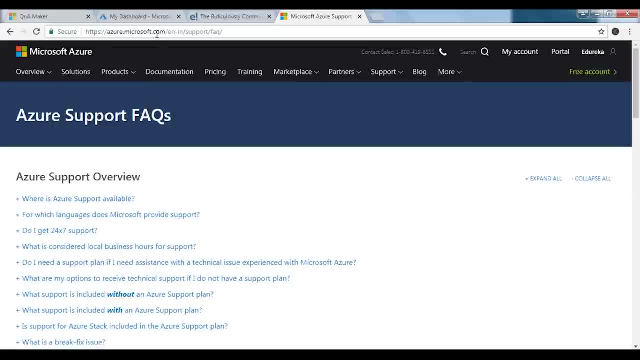 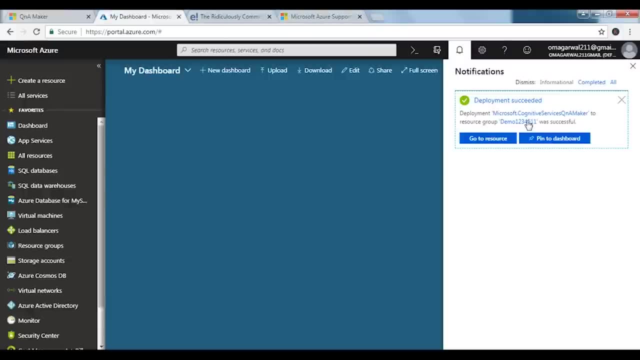 So some questions asked and some data given, so this would be one of the best data sets to use here. So let's copy This link and, as you can see that our service is created, Let me just pin it to the dashboard So it becomes easier to use. 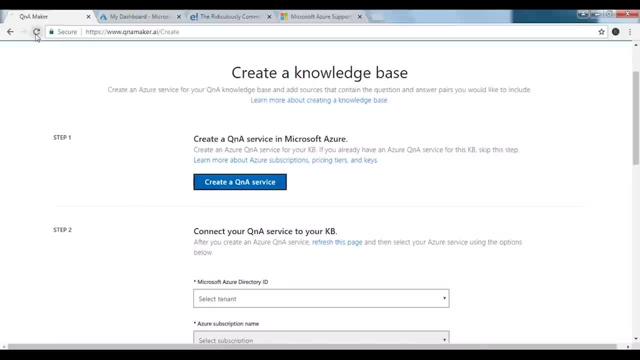 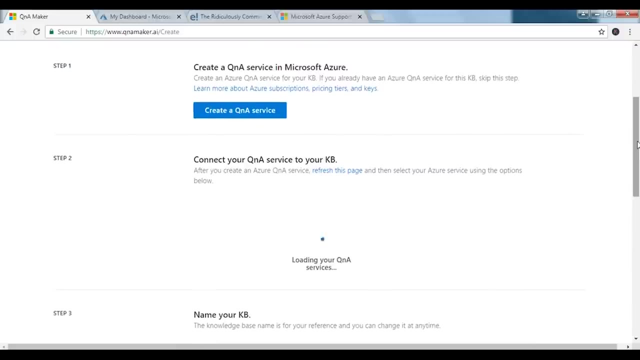 It has been pinned. now I go back to QA maker and I refresh it. guys, You need to refresh it once, because else your so-called service won't be displayed here. Okay, loading your QA services. Please do that for me. Okay, so it has been refreshed. 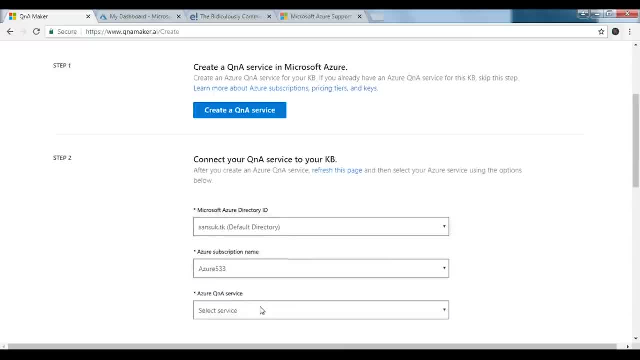 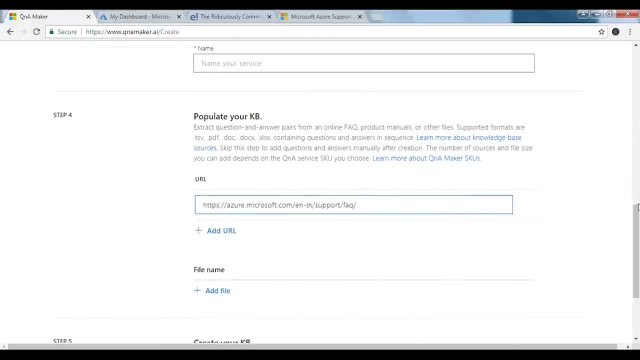 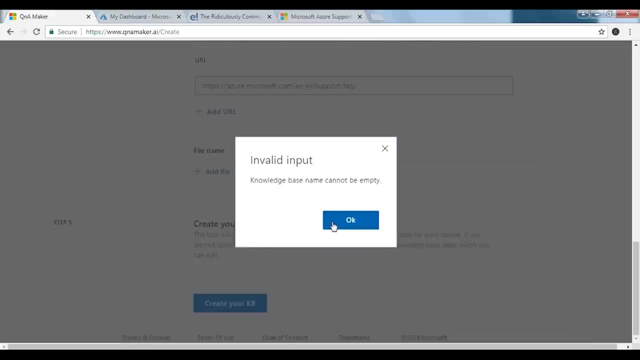 Now let me select the by default account that I have, my subscription name and the service which I just created URL. I paste it here and then I say: create knowledge based name cannot be empty. Okay, I forgot to enter in the name. Let it be the same as we've already entered. 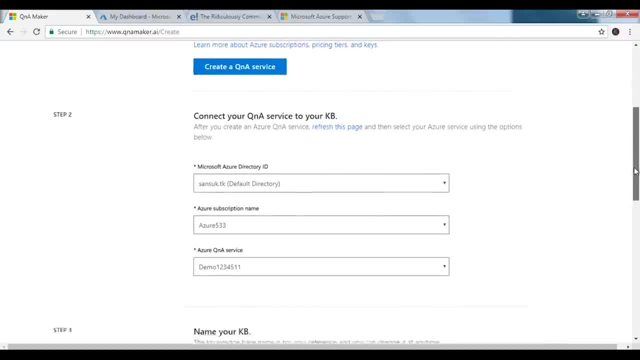 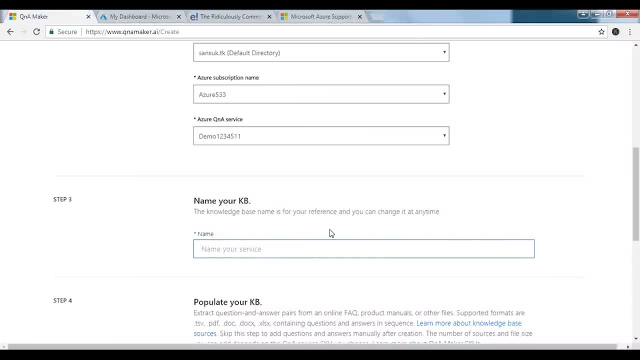 It has nothing. but what was the name? Okay, let's call it, say: let's come here first. It's demo 1 2 3, 4, 5. 1 1, right, So let me just give in that name. I like to have it ambiguous, guys, at times. 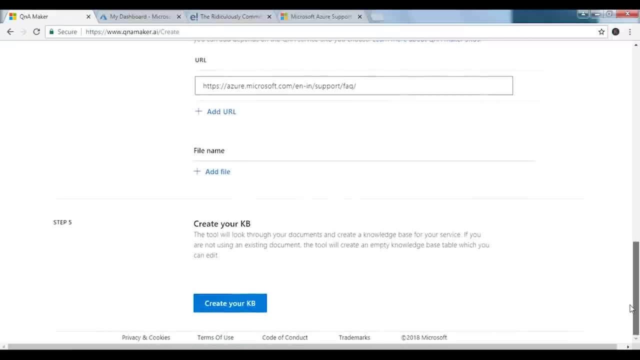 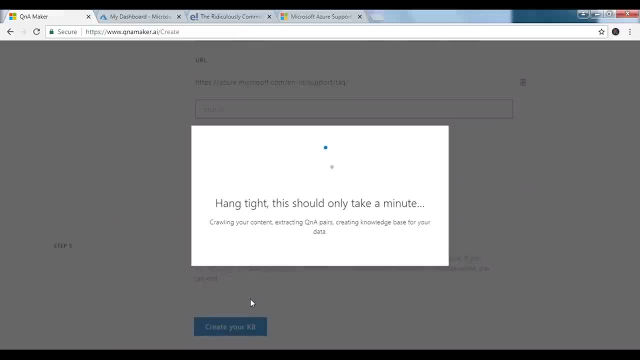 It's simpler to remember same names or use one name throughout the application, So ambiguity is good at times. So there you go. Let's hope it's get it gets created this time around, Okay, So my Take half a minute here and once it's done, it would fetch in all the data and it would create a knowledge base which we can use. now, guys, once the knowledge base is created, it would be created based on the data that we've entered, but that is not how I would start the communication right instead. 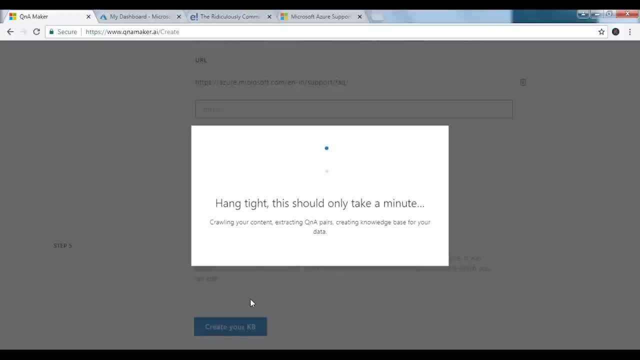 What I would do is I would start by saying maybe hello, or how are you, or something like that. So when I say hello, I need an appropriate reply from the chat bot, right? So we would go ahead and use this knowledge base, but we would also go ahead and add a couple of comments or a couple of starters or endpoints. 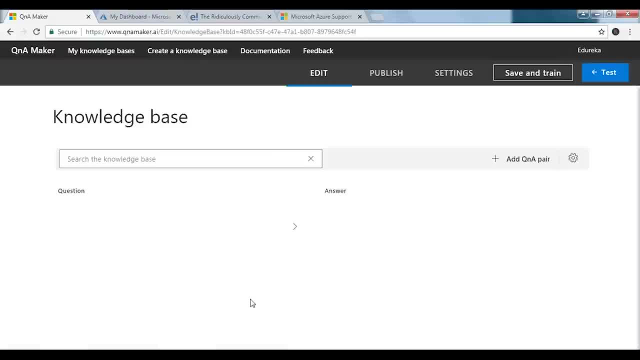 For this discussion. So there you go, The knowledge base has been created. I would like to train it a little more by adding a Q&A pair or two. So in case, if I just go ahead and say, hi, I want my chat bot to reply something like this: 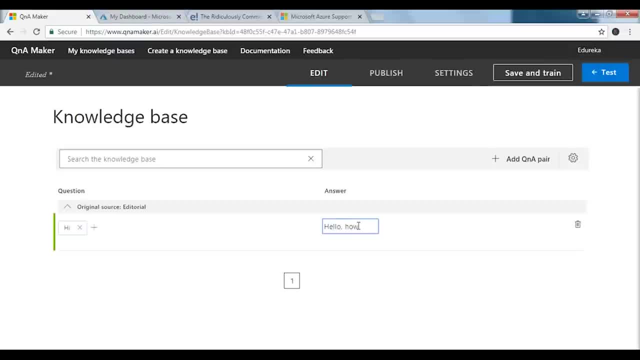 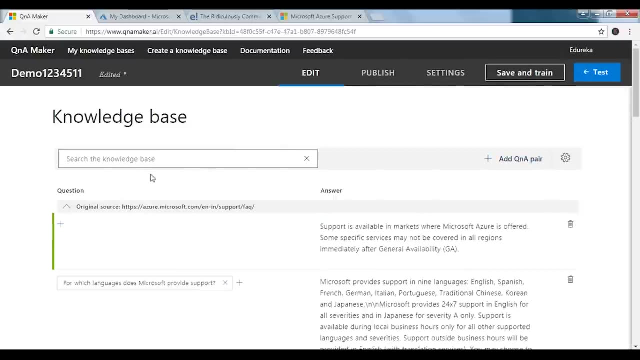 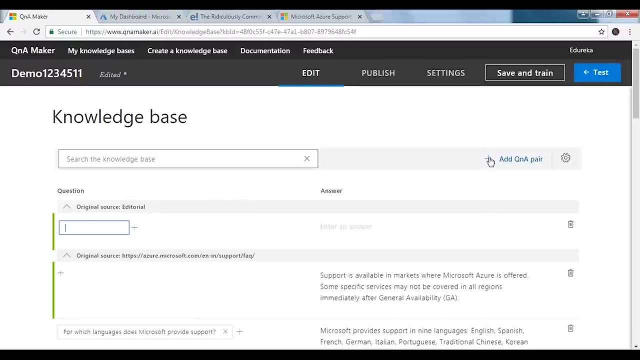 Hello, How Maybe help you. There you go. So, and let me add one more Q&A pair. this time, What I'm going to do is I'm going to what just happened. Okay, there you go. Let me just say thank you and on this, let it say glad we could help you. 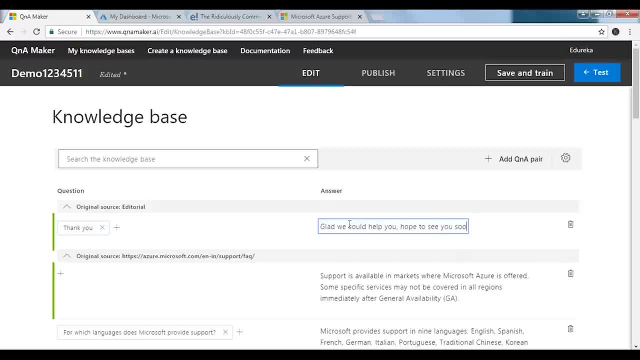 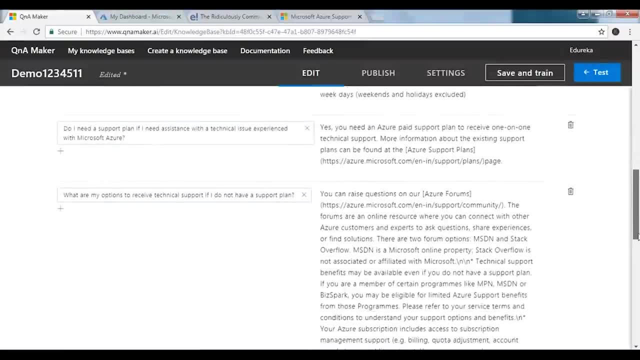 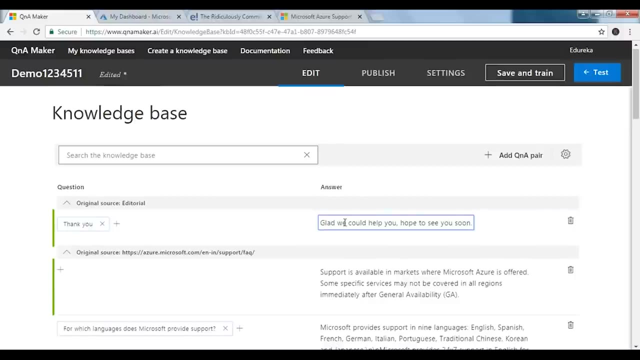 Hope to see you Soon. There you go Some. I'm not sure whether I added that high thing, So if that is not added here, probably will just use this thing to test, as in if we say: thank you, This is the output that we need, right? 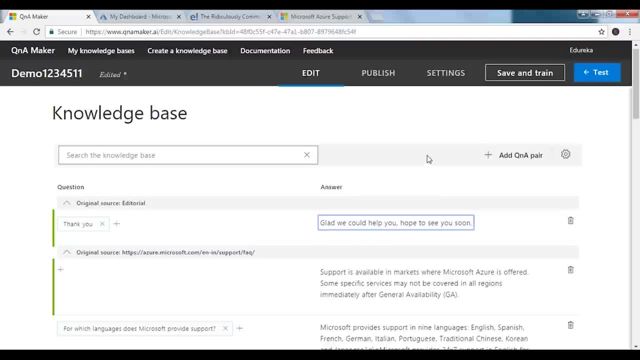 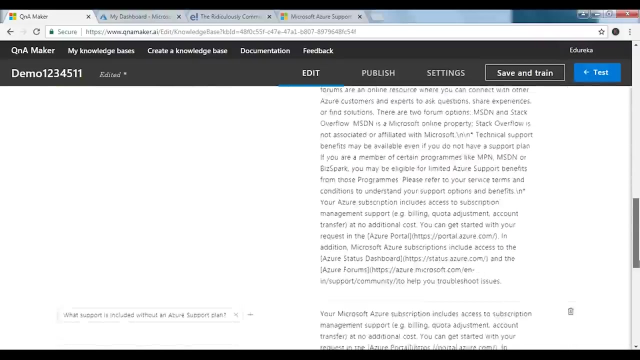 Or if we type some of these keywords, this is the data that should be displayed. So let's just say: save and train. One pair cannot be empty. So which pair is empty right now? Okay, Is there something that is empty here? 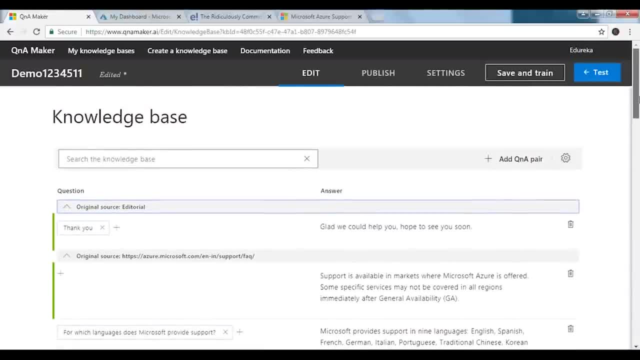 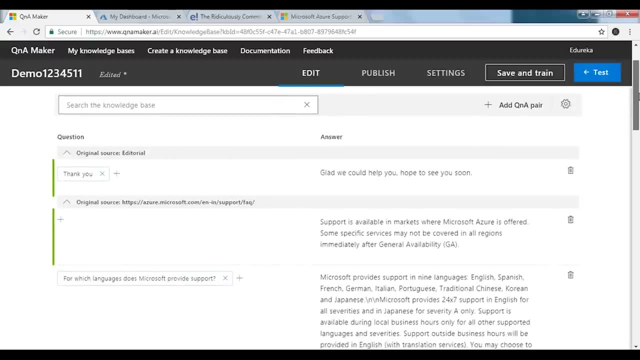 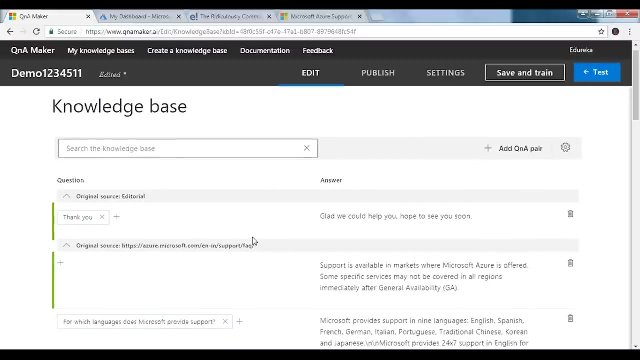 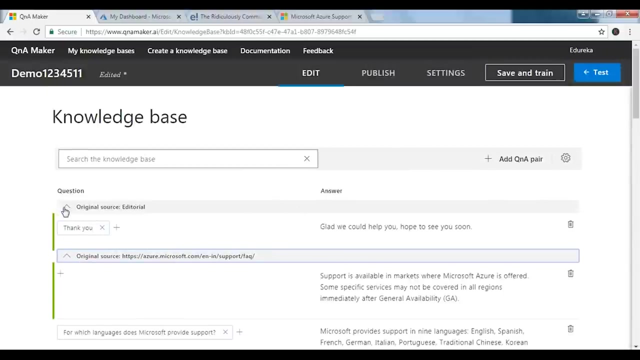 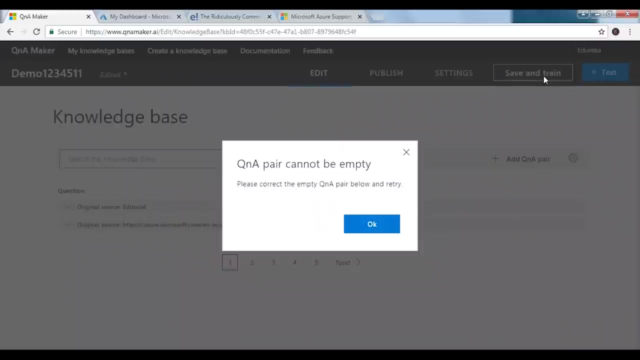 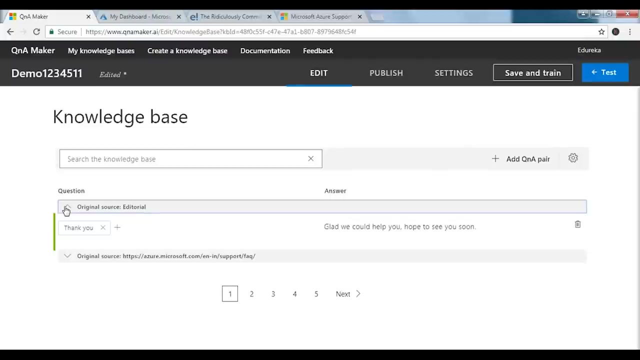 I cannot see anything that is empty. What just happened? The problem is we added Hi and hello, right, I just cannot see where did it go? or could not see where it go. Okay, it's saying that some key pair is empty. 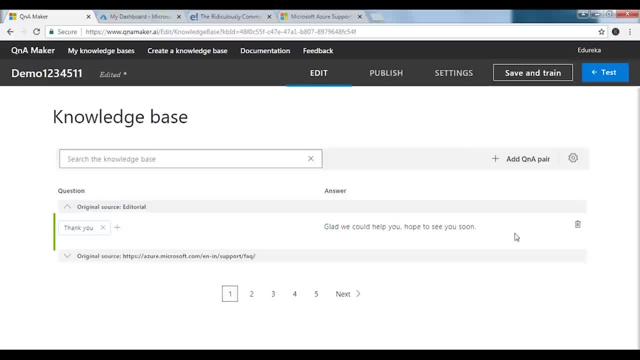 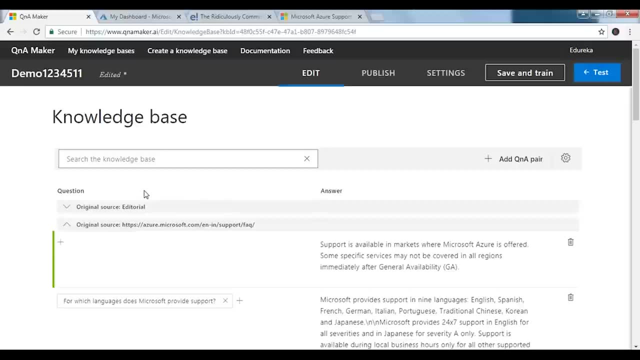 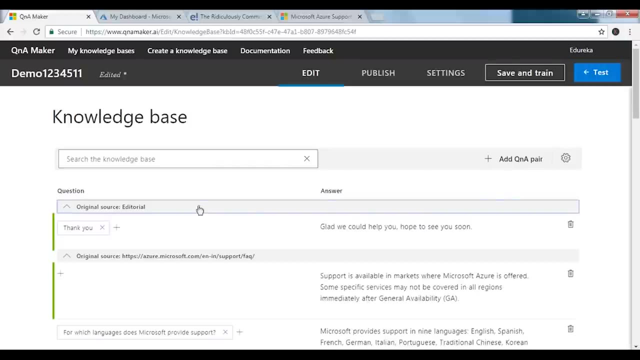 There is thank you here And there is a plus here, So this is fine. This is what we have. Do we have anything else that we need to focus on? Okay, this is the part- Let me just refresh it, guys- that we probably would be able to edit it better. 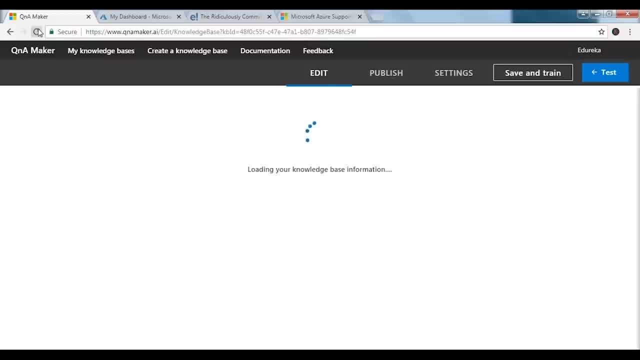 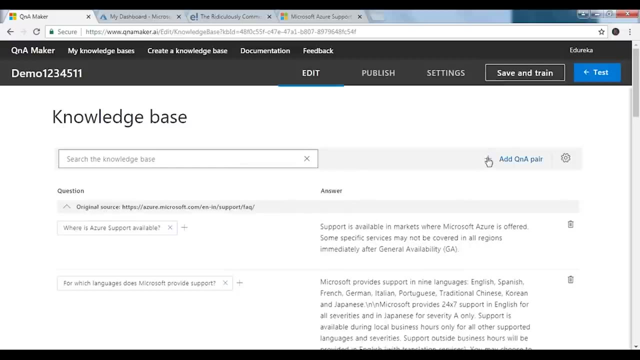 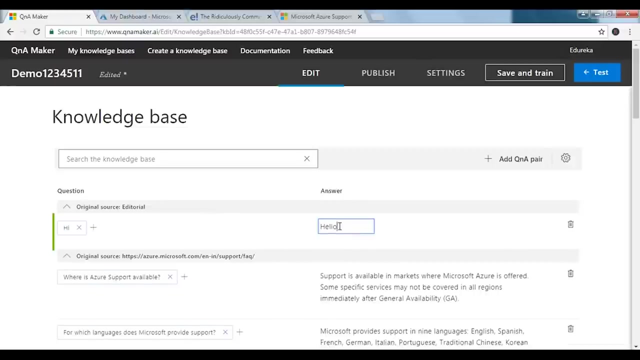 Again, the waiting time. That is something that I hate a lot when you work with these things. Add a Q&A pair, Let's say hi and let's just say hello. How can we help? Question mark and let's see whether we can save it now. 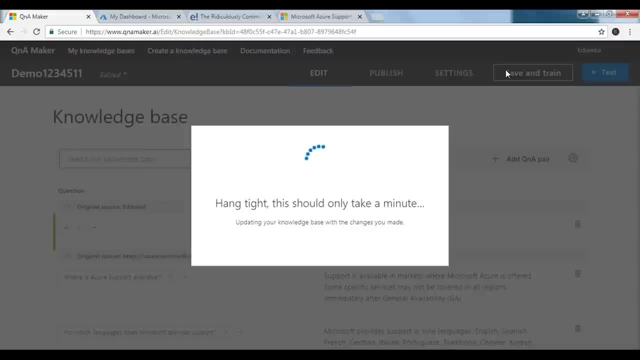 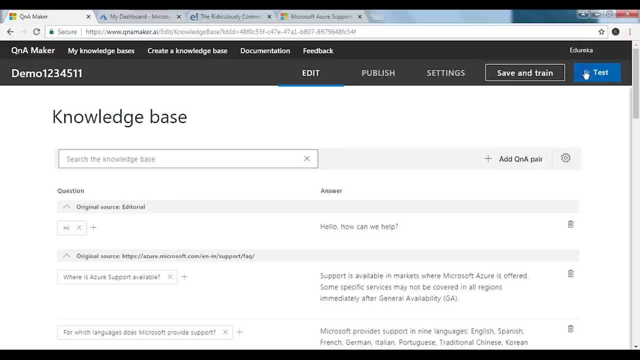 Okay, Now there shouldn't be any problem here. So hi and hello has been added, So I believe we can test our so-called knowledge base based on the data that we've entered here. right? Yep, It has been added successfully, So let's test it guys. 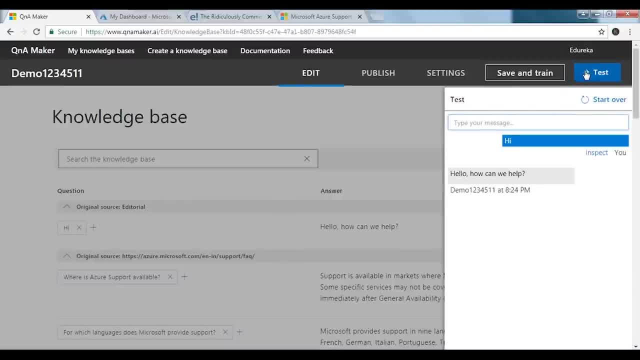 I say hi and I hit the enter button. There you go, We have the reply. How hello, How can we help? you can ask other questions as well, like: do you provide support? So if it can actually go ahead and pass this data, or rather segregate this data, it would give you an answer. 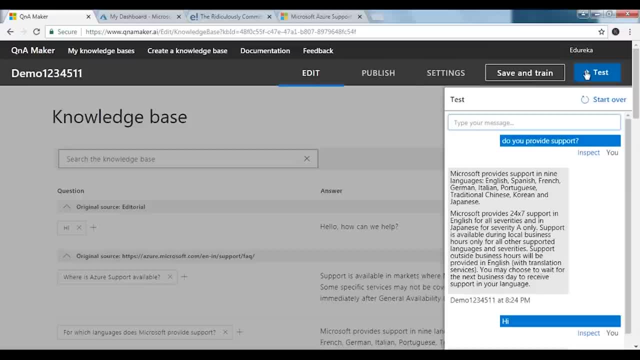 There you go, It has the answer, It has used the database that is there and it has given in the answer that suits in best for this keyword. So, guys, test is complete now. Now let's just go back and publish this knowledge base. 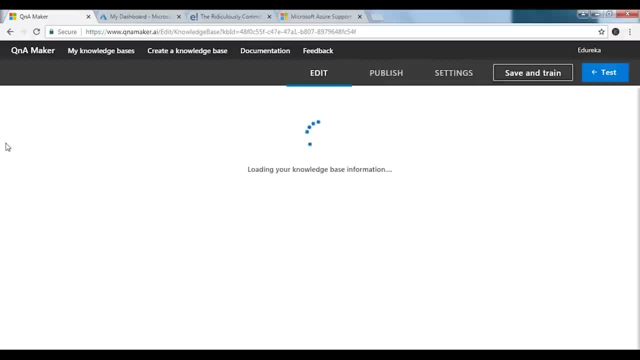 For that I would need to refresh it once, and once it gets refreshed I can just go ahead and publish it. So, guys, once we are done publishing this thing- Okay, we have this option here- publish, Okay. so it might take half a minute. 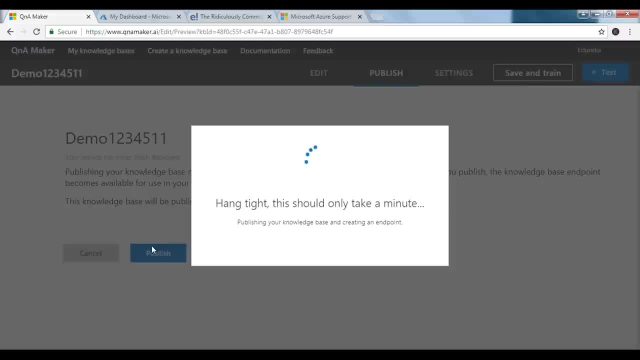 So once it gets published, now we are going to go ahead and create a chat bot and we are going to integrate or we are going to give this Knowledge base to a chat bot. So if we again taste test it and put in certain queries, it would give us the reply for the questions that we've asked. 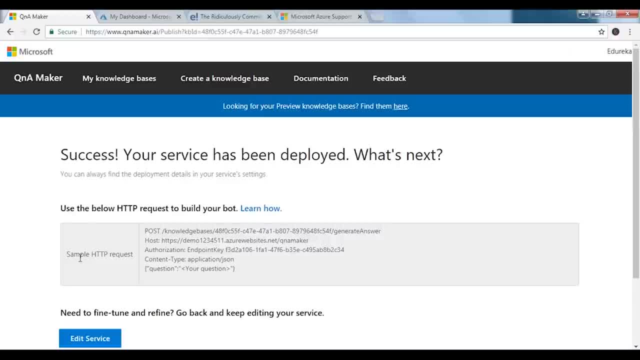 So there you go. Now, this is something that we would be needing. It is nothing but sample HTTP request. That means, once I try to connect with my chat bot, there are certain credentials that I might be required to enter, like the host ID or the authorization endpoint and all those things. 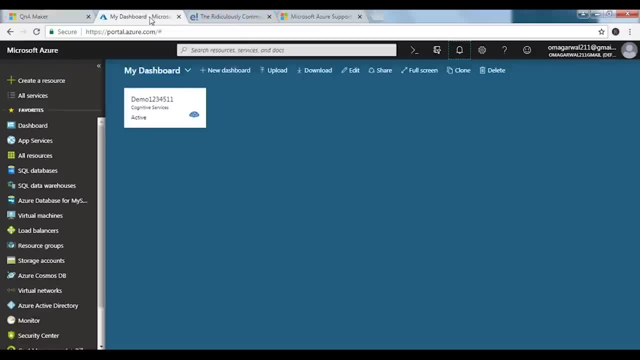 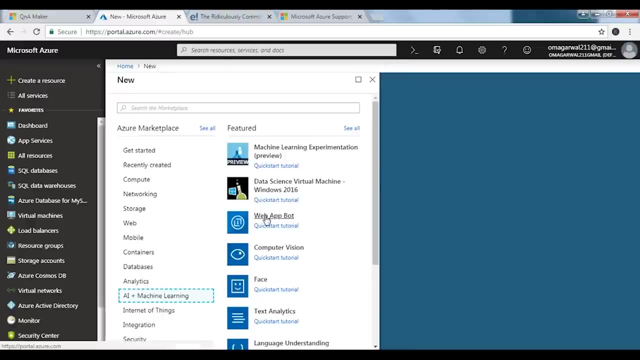 So let's let this thing be open and let's just switch to the dashboard part. Now, here I can create my chat bot. for that I need to click on create a resource. There you go. I say AI plus machine learning and I get this option where I say web app bot. 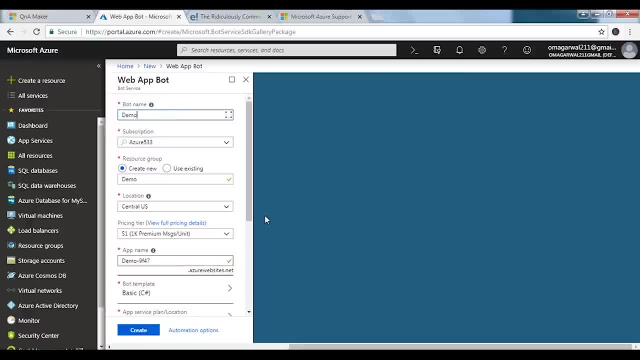 There you go. So let's create something called as demo: 1, 2, 3, 4, 5, 6, 1 1 Again. subscription is Azure 533.. It has created a resource group Central. No, no, no. 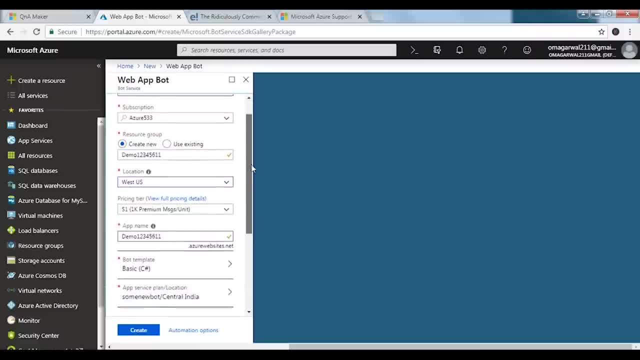 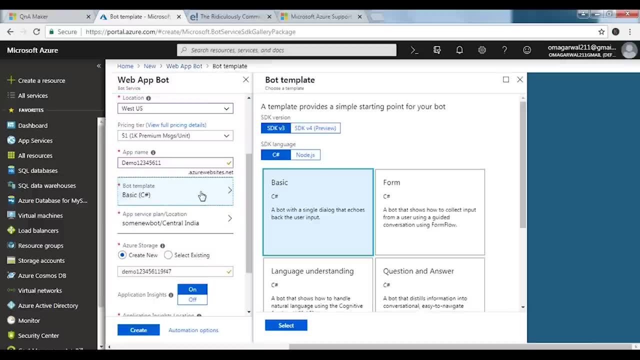 I want West us want West us. I scroll down What is the bot template? Well, it is built in basic C. sharp, I would click on this thing and select Q&A. that is question and answer form, and I say select. There you go. 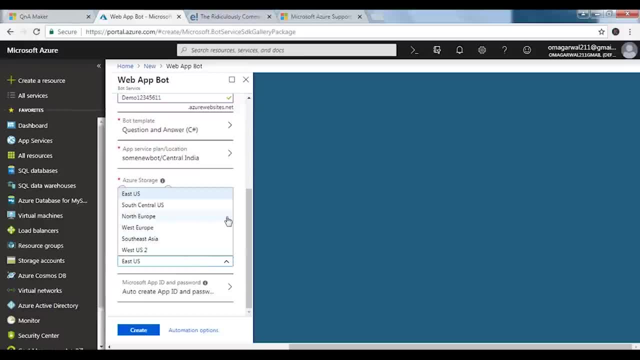 I scroll down East us again, I want West us, maybe West us 2, and I say create. So, guys, this thing takes a while. It takes a minute for my chat bot to get created. Now, once the chat bot gets created, next job is to take this chat bot and connect it to. 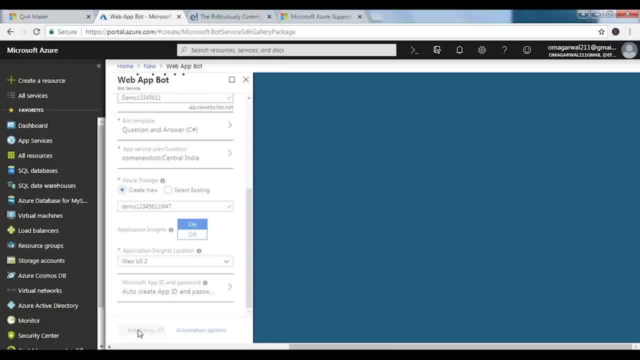 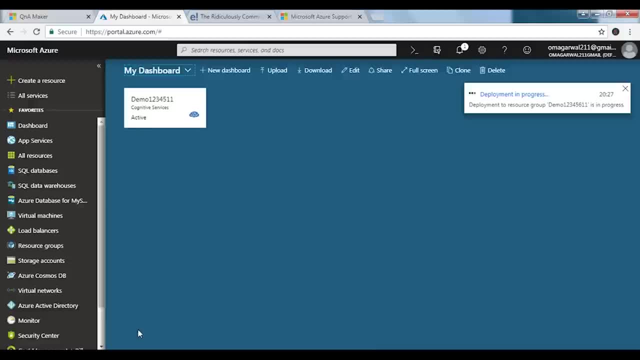 the knowledge base and move the whole thing to my Facebook Messenger. Now this is where I would be asking the questions, that is, I would be creating an application on my Facebook Messenger and on that I would be putting in this chat box. So if I do throw in these queries, my Facebook Messenger would reply. 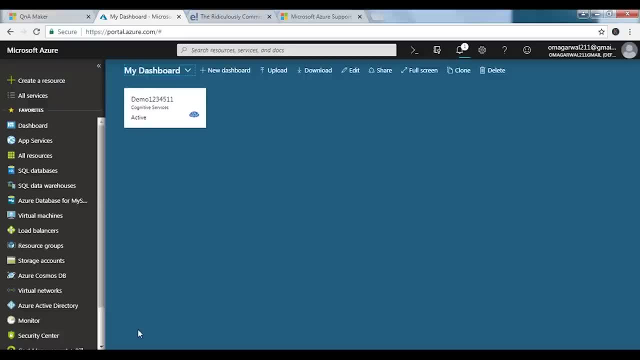 That means the chat bot would reply using my Facebook Messenger. for that We need to integrate our chat bot with the Facebook Messenger. So how do we do that? for that We need a Facebook account. while this thing works out, Let's do that. 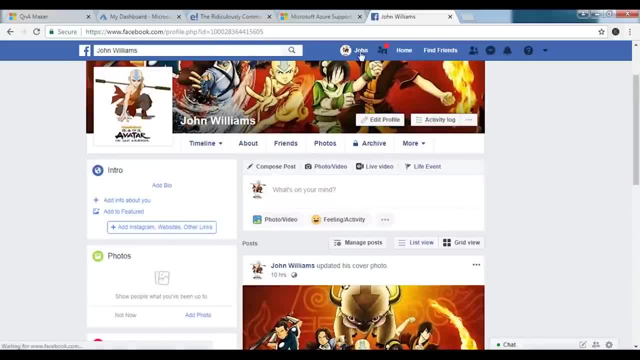 Now this is a sample account that I've created. This is an anime which I used to watch once, So I've taken this template. this basically deals with different vendors who can bend different elements. Now you don't need to get into the details of what those elements are. 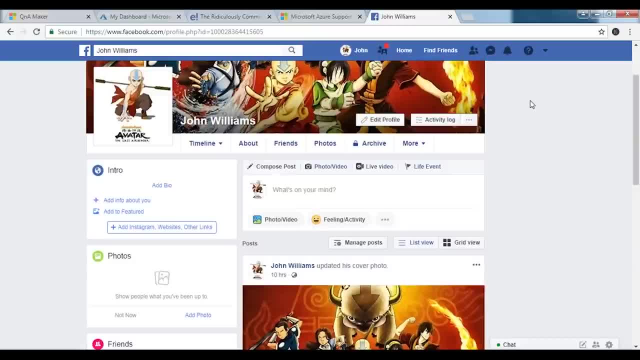 I've just used this theme and, based on that, I would be creating a page to which I want my chat bot to react to, and I would also be going ahead and creating an application as well. Why are we creating all these things? Once the bot is ready, you would understand all the stuff as in why we are here and what. 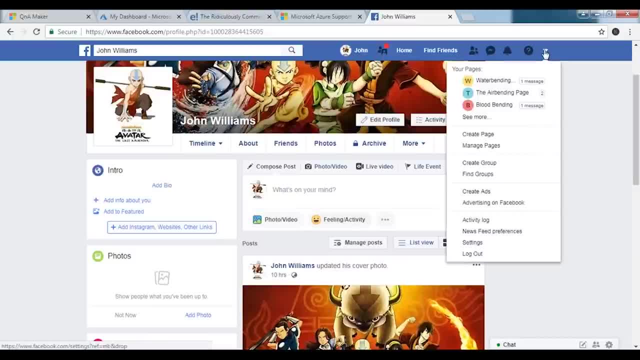 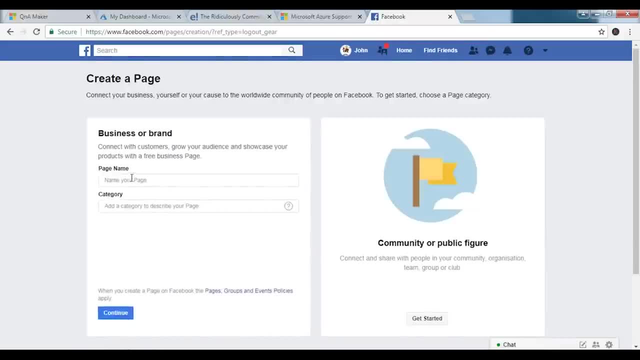 are we doing here Meanwhile? just create a page first. Let's say create and let's call it. say Okay, Let it be business brand, call It's a metal bending. Don't get into the details of what this title is. 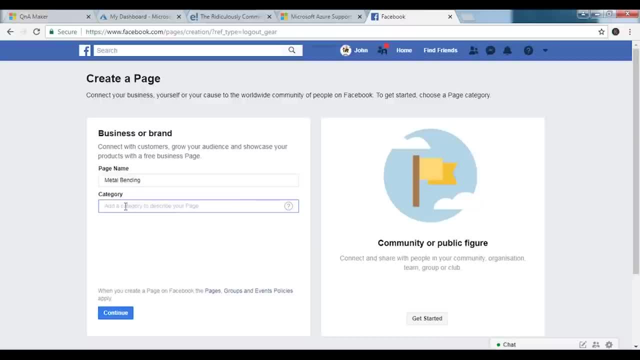 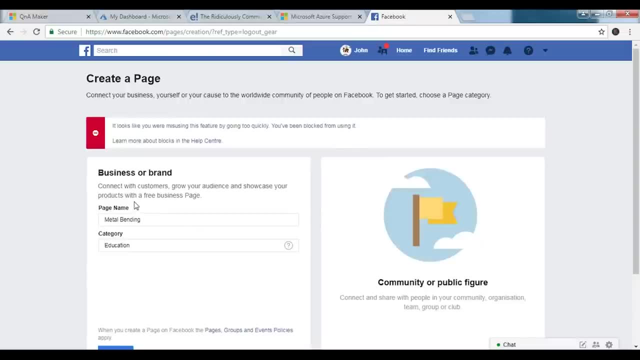 It's a random title and category. We are here for education, So let's stick to that. I say continue, Okay. it says I have been blocked for some reason. The thing is, I happen to create this thing twice today. That is why probably, they blocked me as in for creating this page. 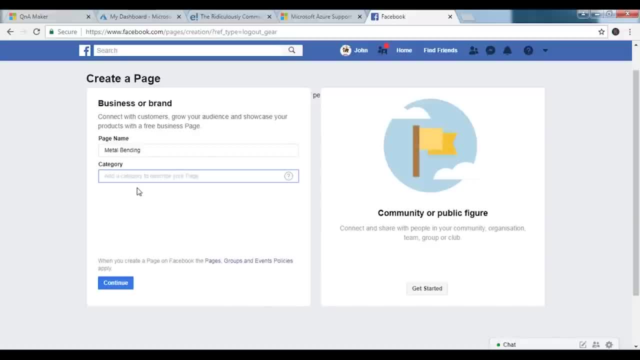 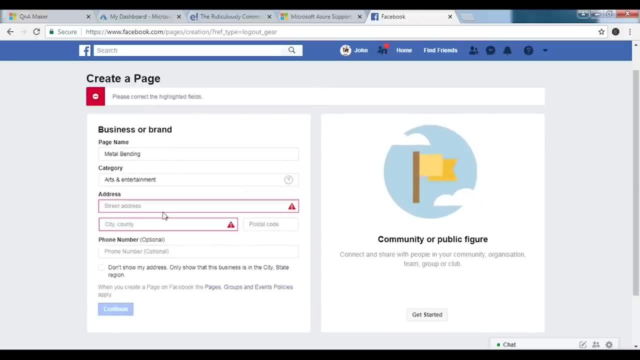 Let's see if we can choose some other category and see whether they allow us to create a page here: Arts and entertainment, Maybe. now, Okay, they need other details as well. So let's skip. Let's try something else. Say it's a beauty salon again. 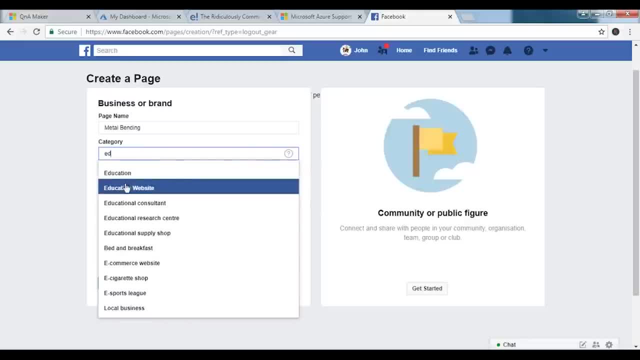 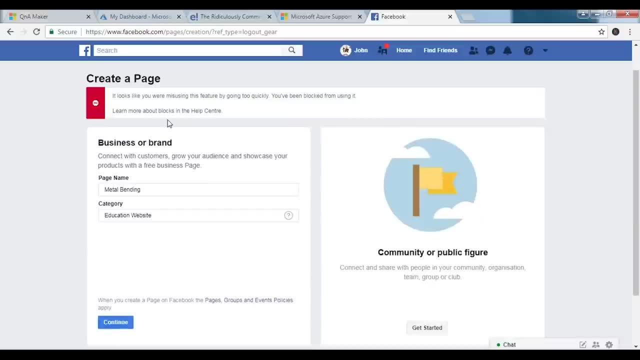 They need in the details. If I put in education, that is when they don't ask anything else. Okay, education website, Let's say continue and let's hope that they let us create one. Okay, No, I have been blocked, So I doubt that I would be able to use this thing. 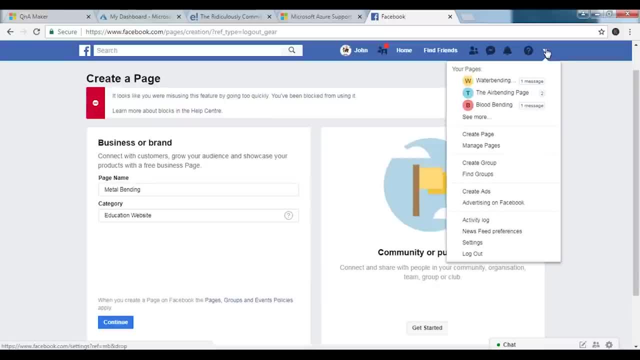 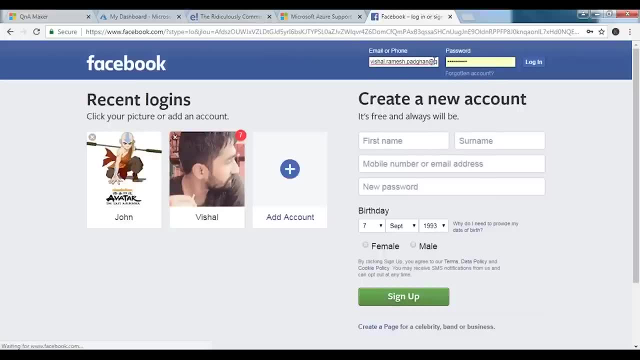 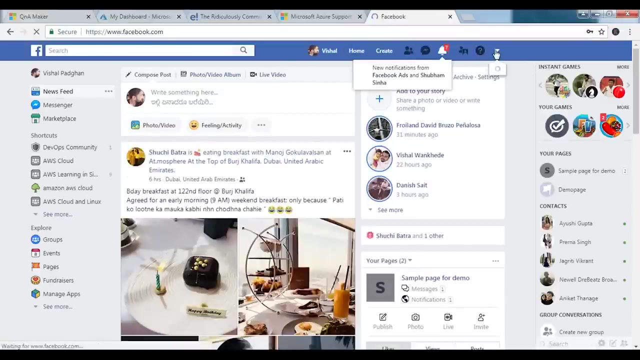 Let me just quickly switch into some other account and see whether I can go ahead and try to do it with some other account. Let's try to create a page Now. let's hope that it lets us create a page here. I say create. 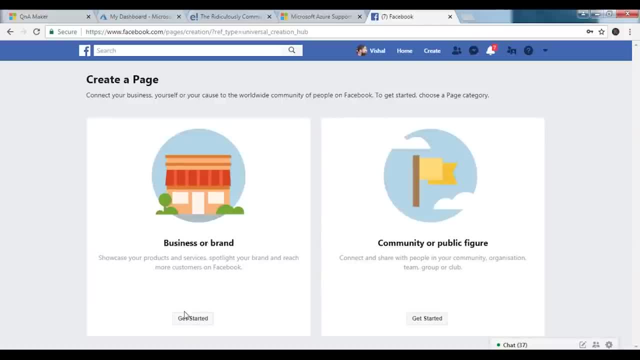 Nice, I create a page, Let's call it. say, If it allows me, will, and good. if not, then we'll have to switch to something else. Probably it is letting me create one, So that's a good sign. We can go ahead and use this thing. 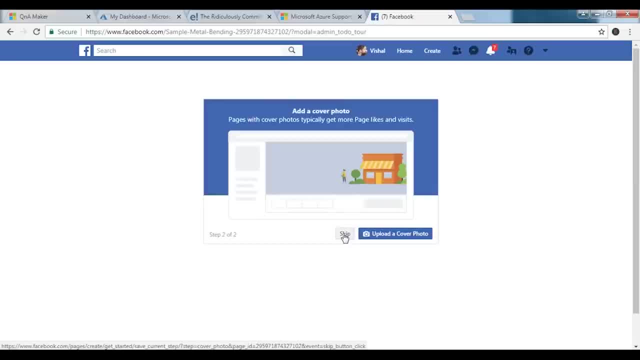 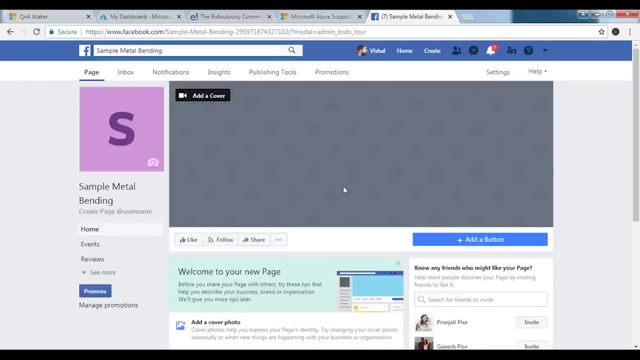 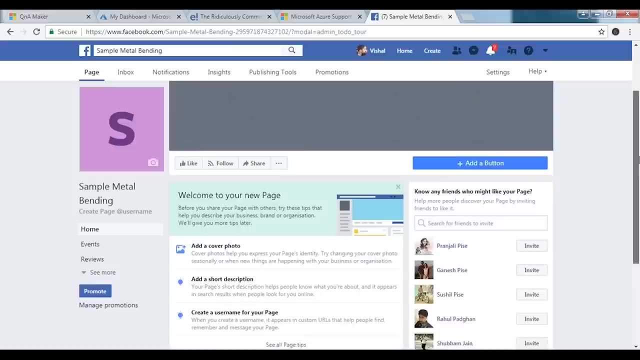 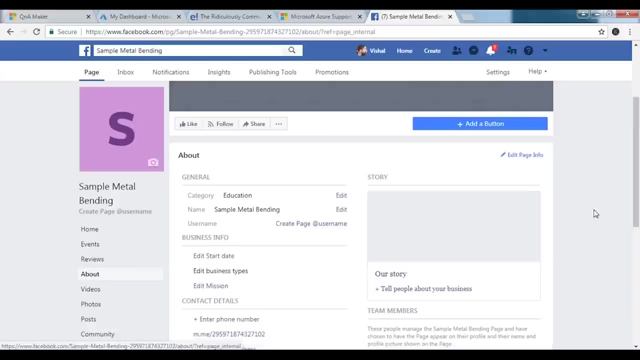 Skip And I say skip. There, you guys, we have a page here. Now, once we have this page, next what we have to do is we have to go ahead and take a look at certain other details that are needed. Like, if I click on this about page, I would be having an ID here which I would be using. 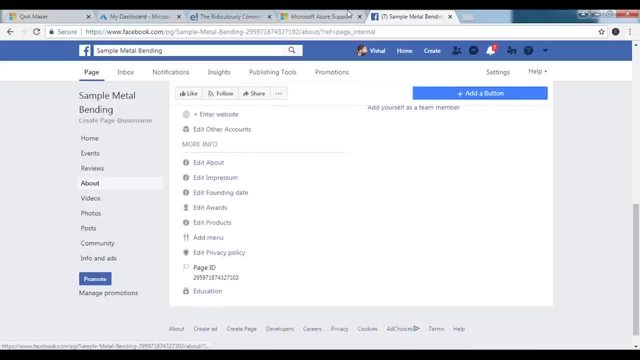 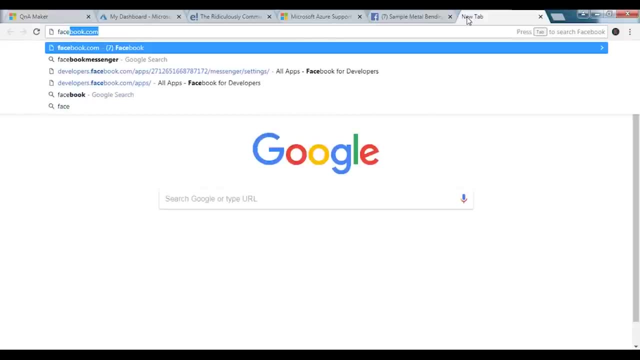 now, This is my page ID that I would be needing. Okay, so we have a sample page and we are going to use this to test our application. apart from that, I would be going to this Facebook Developers, where I would be going ahead and creating an application as well. 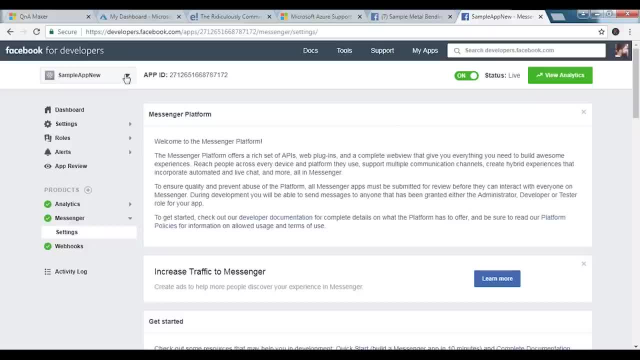 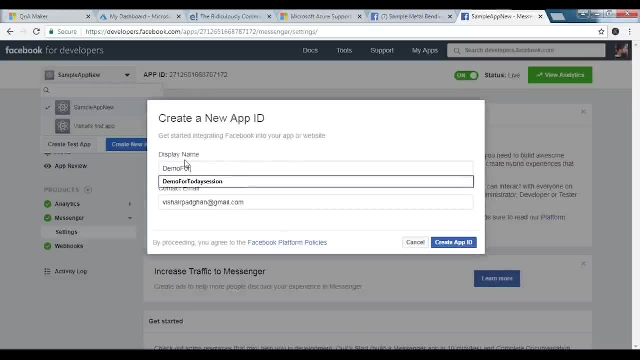 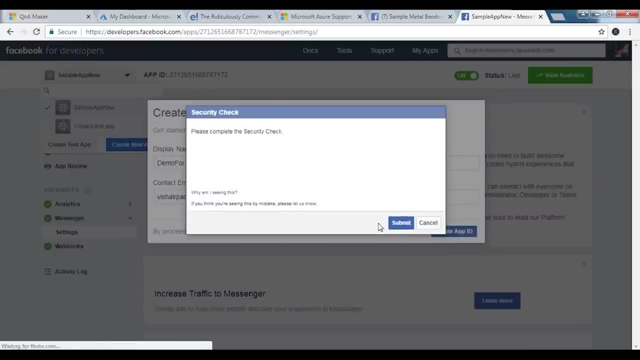 Now I am basically signed in as Vishal here, So that is good. Let me just go ahead and create one more app. Let's call it, say, Demo for today. There you go And I see Create. Am I a robot? 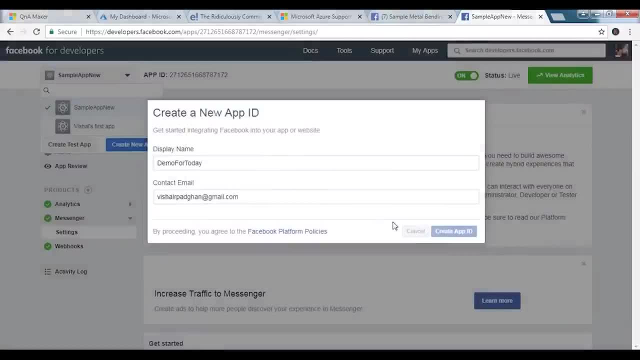 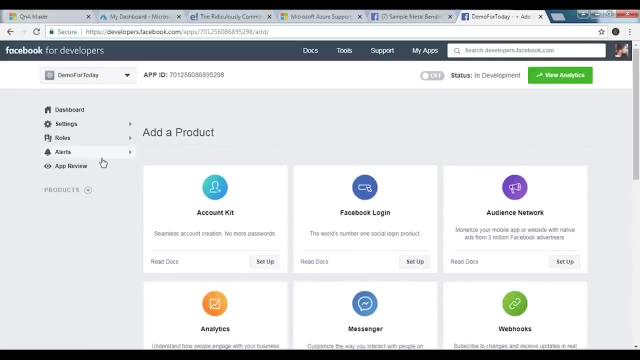 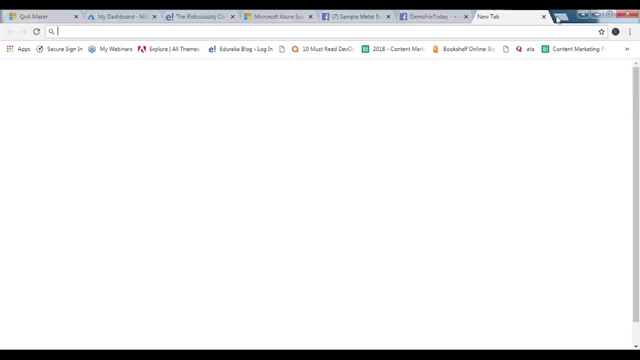 No, I'm not Submit. So, guys, an application would be created here, So we would be using this application and we would be attaching a messenger to it and we would be attaching the chatbot to this messenger. Let me just quickly go ahead and check one more thing, because I do not want any more. 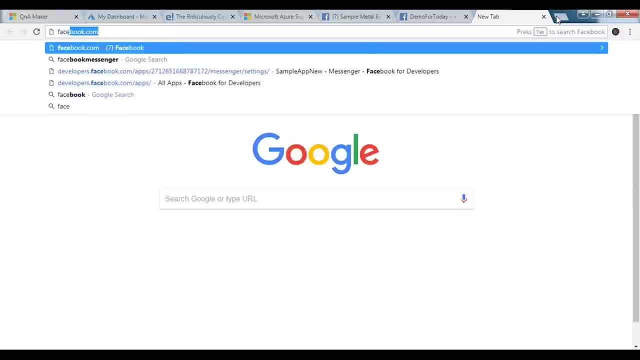 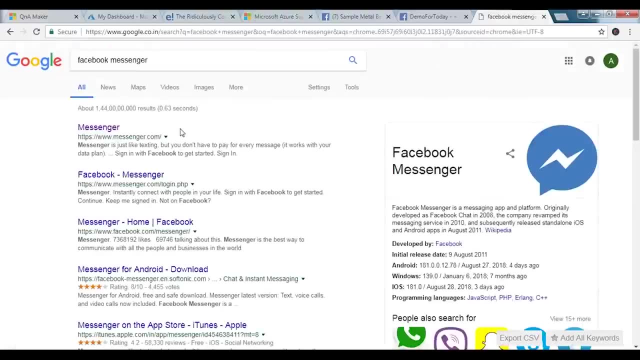 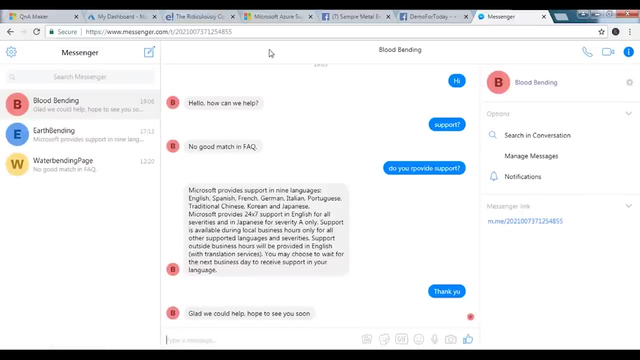 problems in this session. So let's just quickly say Facebook Messenger. If I open the messenger, let me just see What is the messenger that I have by default here. So, as you can see, I have this thing, which I do not want. 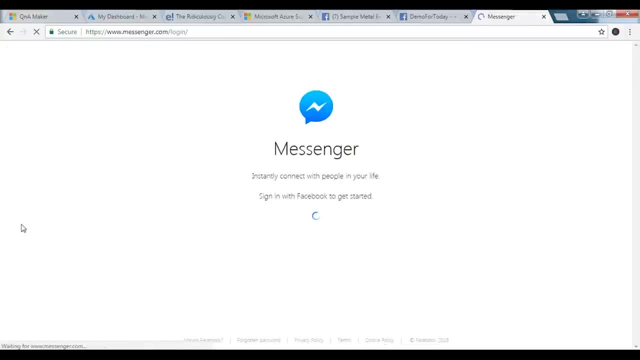 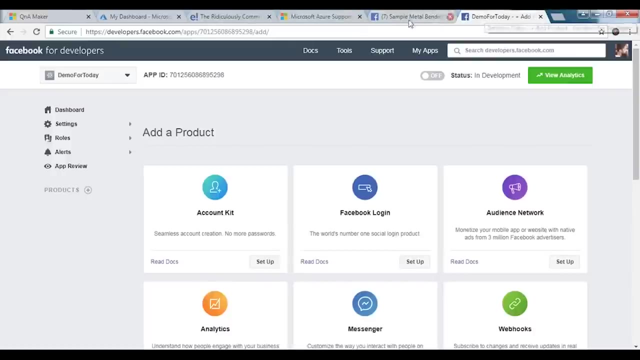 I would rather go out and log out from here. So, guys, Yeah, on the continuous, we shall put them. Yep, There you go. Now we should be good to go. So, yep, we are here. and, guys, by the time our- I believe our- application is up and. 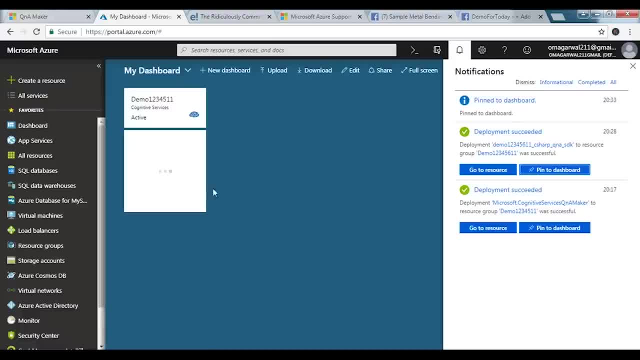 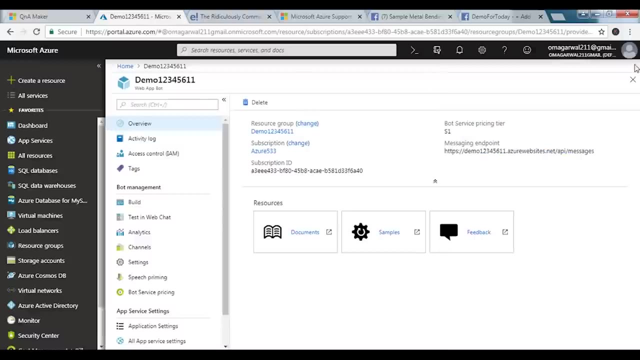 ready, Pin it to the dashboard. Now, guys, we have an application on Facebook, We have a page on Facebook and we have our demo bot up and running which we can use. So let's just open this thing and see what it has to offer to us. now, guys, 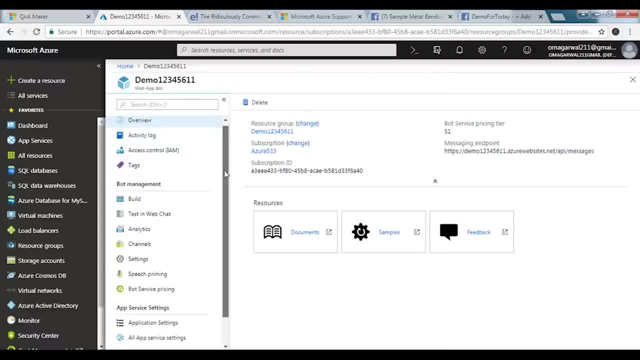 These are the resources that we have at our disposal and apart from that, we have quite a few other things that we can do. we can test our web chat here. We can take a look at the analytics that is there and what are the different channels that we can use. 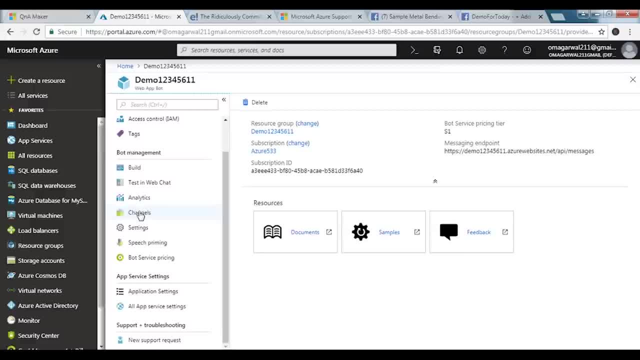 To use this chat bot. So we are going to take a look at all these one by one, but, first and foremost, what I'm going to do now is I'm going to go ahead and connect the knowledge base to my chat bot. How do we do that? 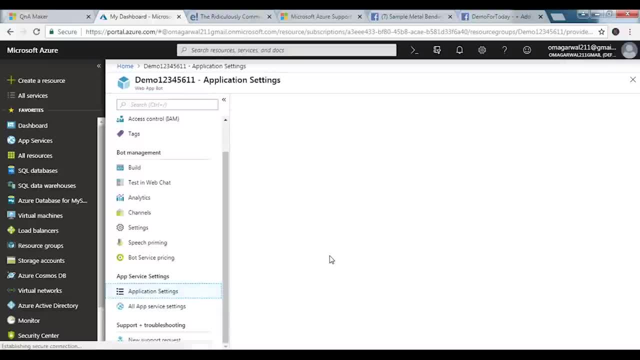 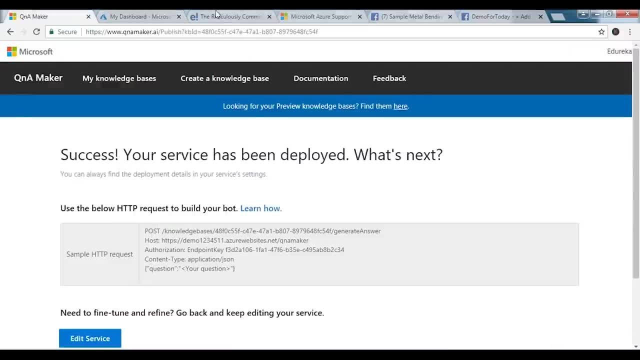 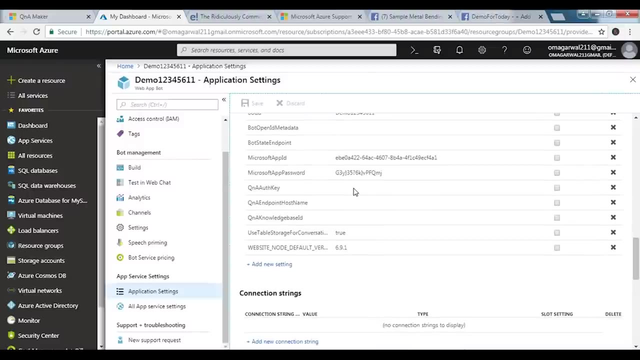 We come here and we click on application settings. Once I open that, I would be entering the details that we have here. the connections are the endpoints. There you go, So I have to scroll down And these are the three fields that I need to enter here. 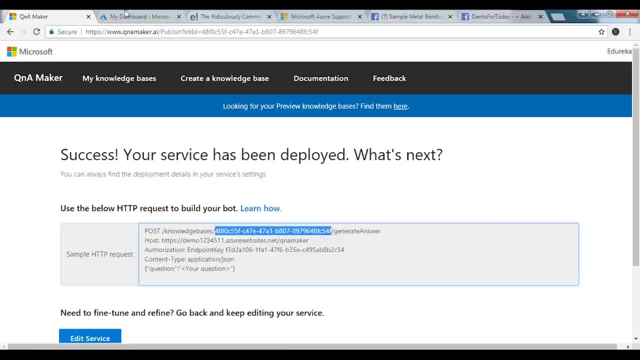 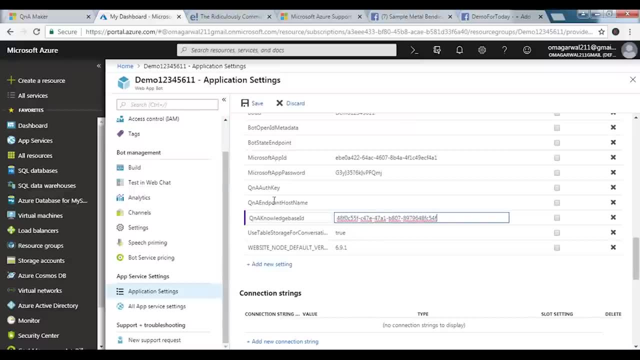 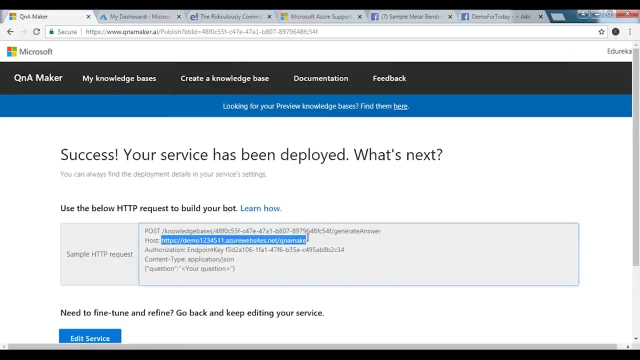 So I copy this first. that is now. this is my ID, which I would be entering here. The first place where I enter this thing is this: Okay, I also need the host name, which in this case, is this: Okay, and apart from that, we have this data. 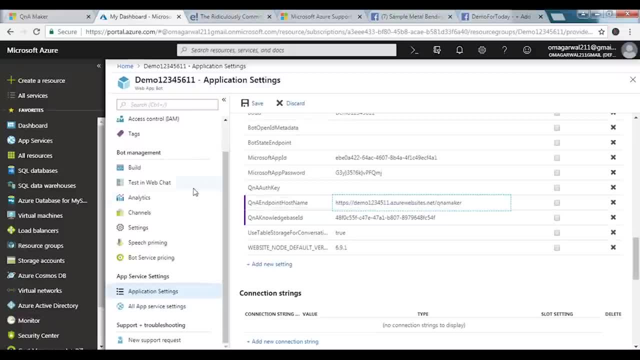 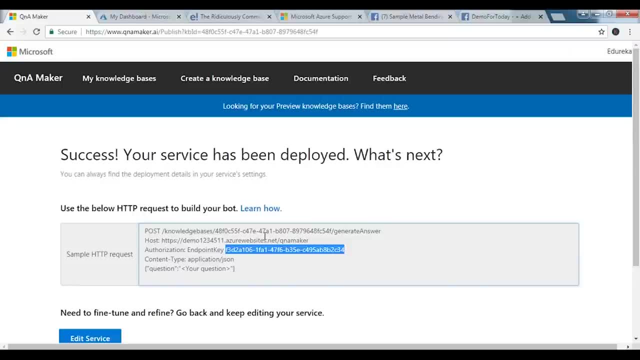 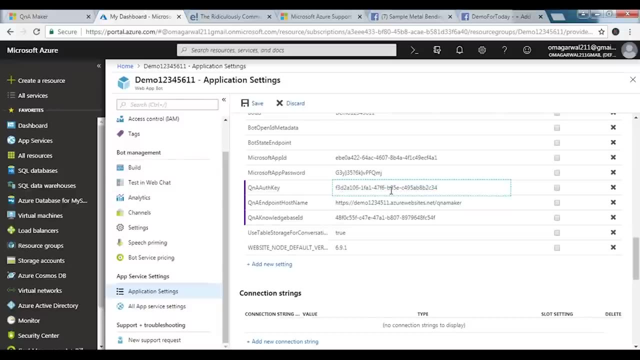 This is my authorization key, Okay, so let's just verify it. We have the knowledge base ID, which is correct, host name is correct and the authorization key is also there, So let's just save it. Yes, so it has successfully updated this thing, so I can just come here and I can say test. 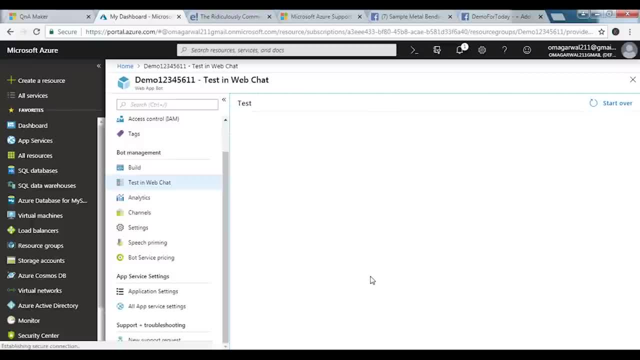 it in chat box. So if I just say hi, you should give me a reply. It's still sending the data. So, okay, how can we help? So yes, it has been integrated or connected to my chat bot. Now next job is to connect this chat bot to my messenger app. right, 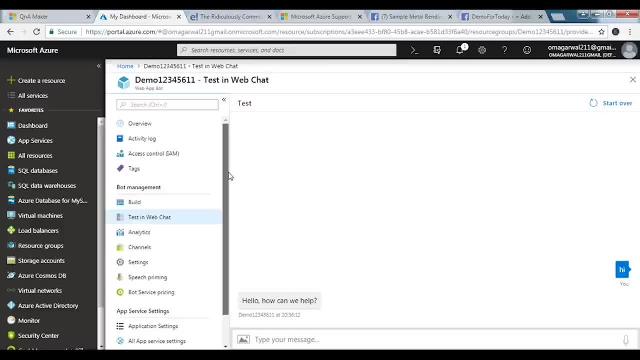 So how do we do that? To do that, I would have to come here to channels, and I have some channels that are made available which I can connect to. first, I would just come down and select Facebook Messenger, The one which I want to connect to. 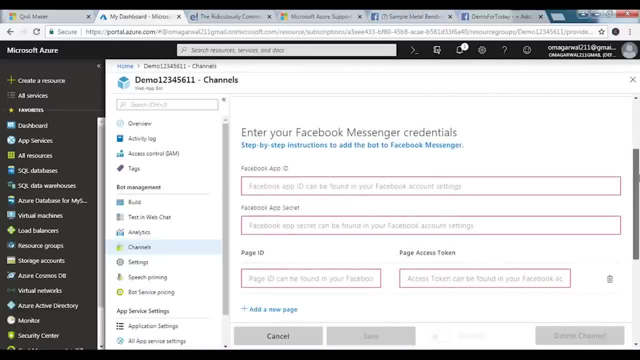 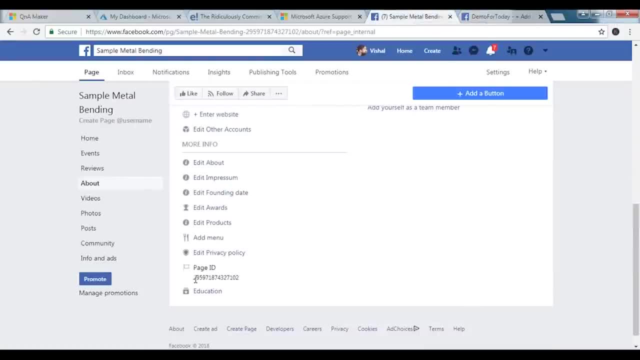 And, as you can see, this is the reason we created the app and all those things, because we need to fill in these details as well. for that, I would come here To my page and I would copy this page ID. Guys, there's too much to and fro of information here. 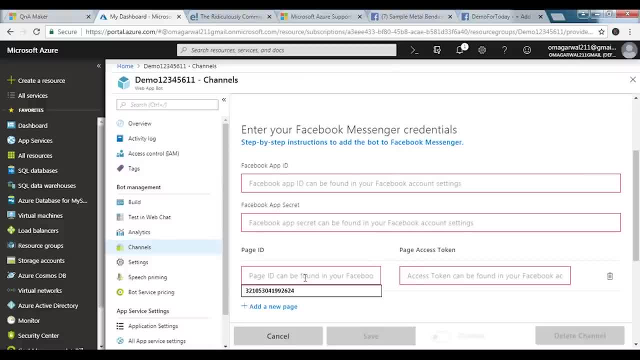 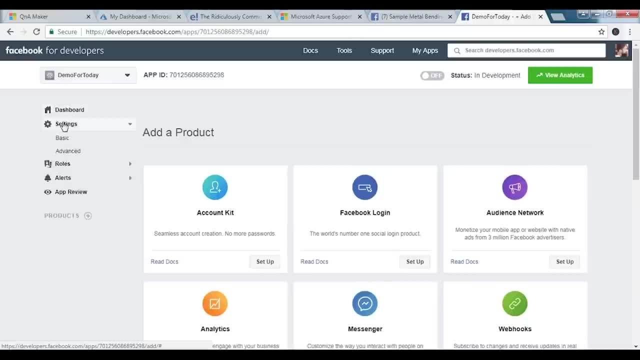 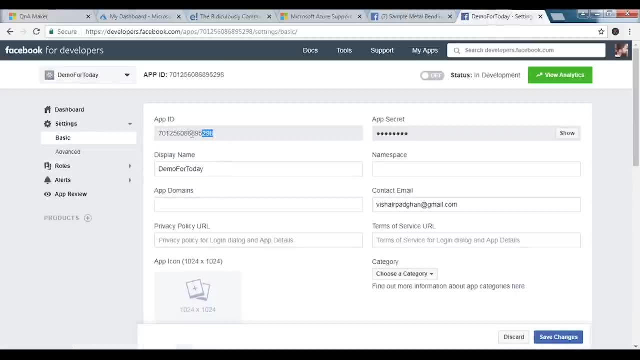 So keep an eye on that, as in what I'm copying, where this is the page ID As I move further, I have this application here. So in that if I go to settings, I have the basic settings option, I need to copy this ID as well. 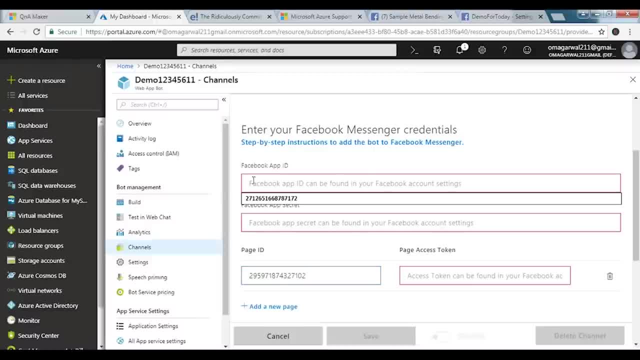 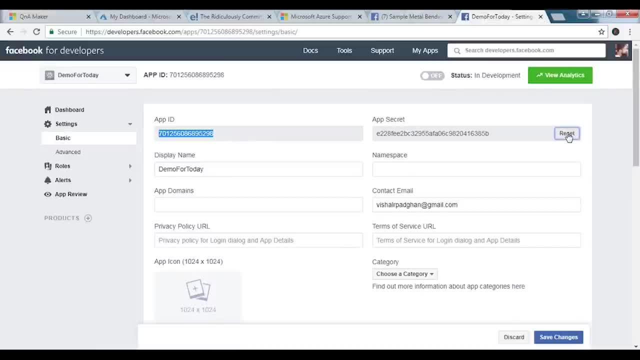 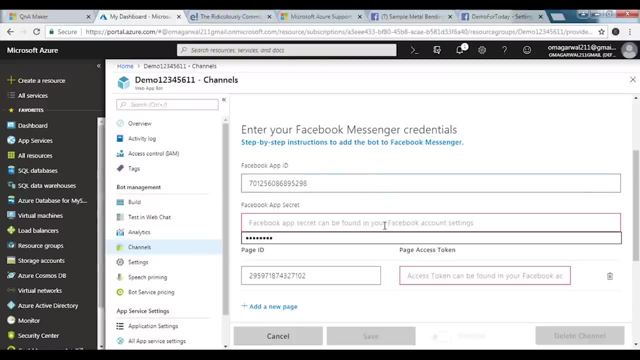 Now, this is my application ID, which I would be copying here. Control V and guys. Lastly, we need the secret key, which is here. I need to copy this as well. control C and I paste it here. Okay, So, guys, we also need something called as page access token, but that is something that 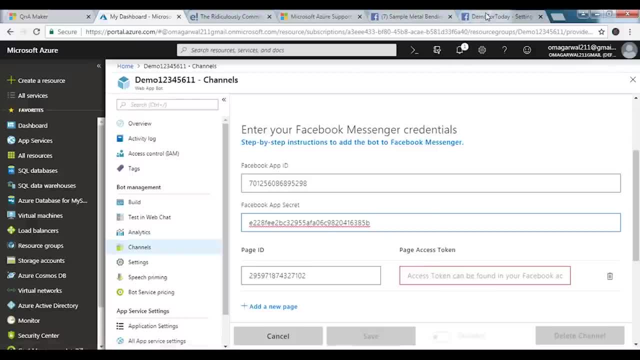 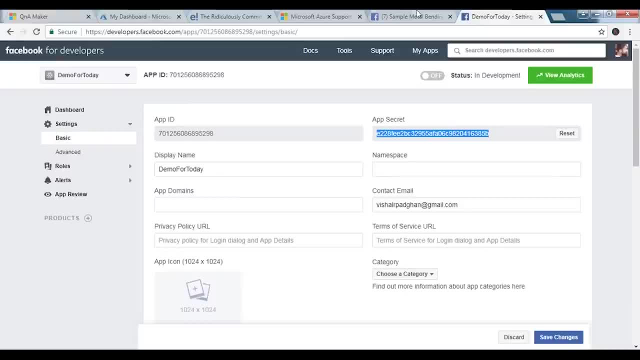 would be given to us once we move further. I tell you how to generate that as well, Do not worry. Yeah, so, guys, now we are at our application. one small change that we need to make here as well, as we move to the advanced setting. 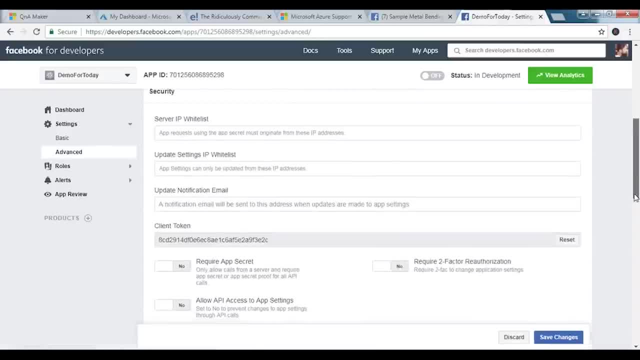 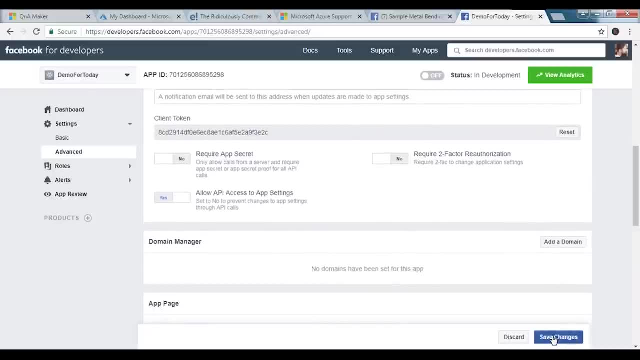 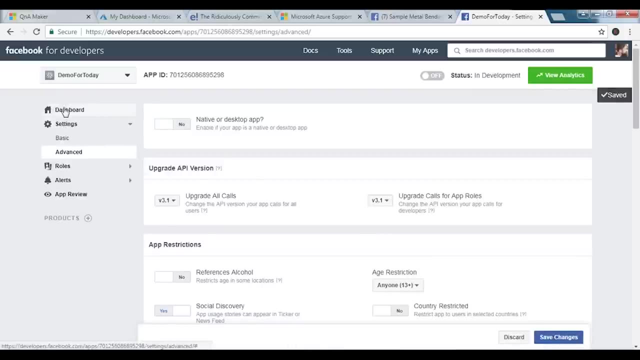 And in that we say yes to this thing. At the bottom we have allow API access. I say yes And I say save changes. There you go. next We move to the dashboard and now we configure our messenger to with the chat box. 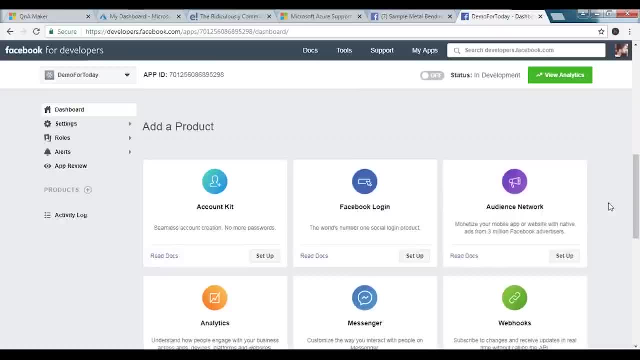 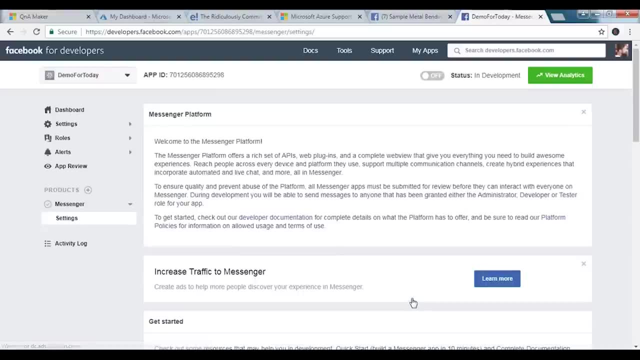 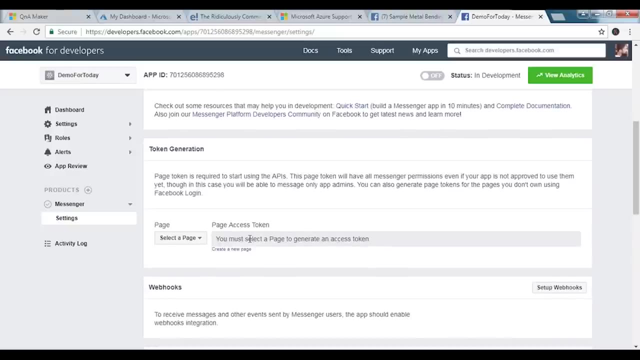 And how do we do that? We scroll down here on the dashboard and we select this option: Setup. Okay, so there are certain things that I need to take care of. I need a page access token as well If I come to app review guys. 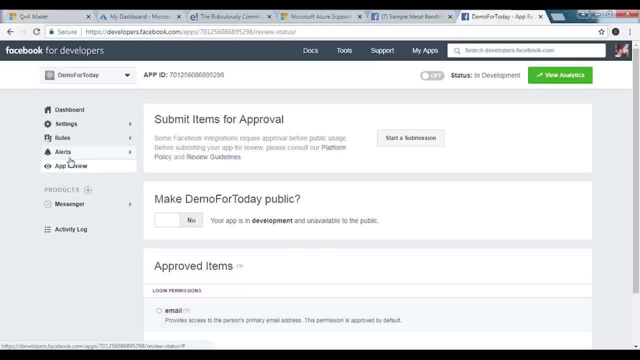 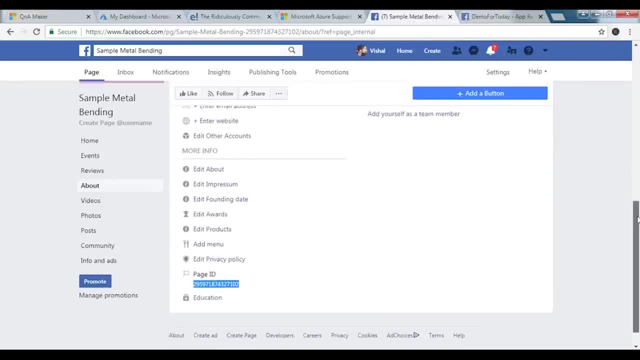 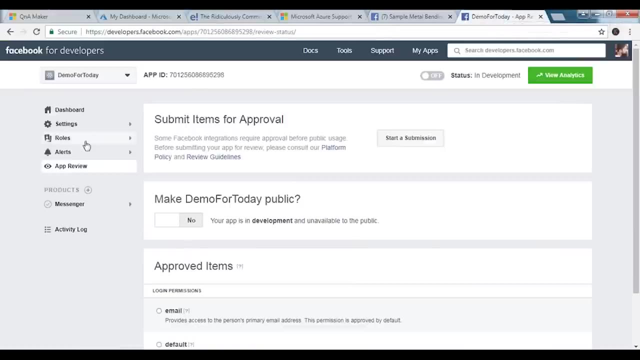 There are certain things that I would be needing to review, and before that I would be needing to enter in few details. We would be taking a look at those as well, one by one. Do not worry about it. Okay, So when you come here, first thing you do is again go back to settings. 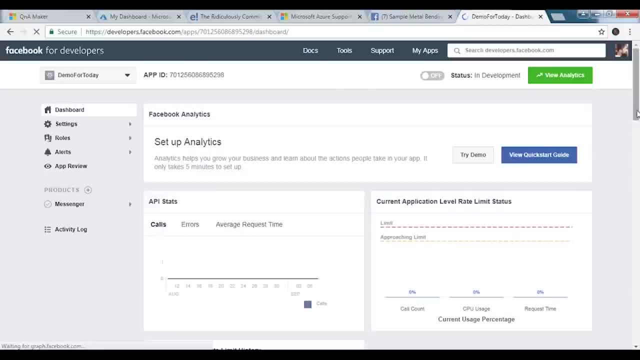 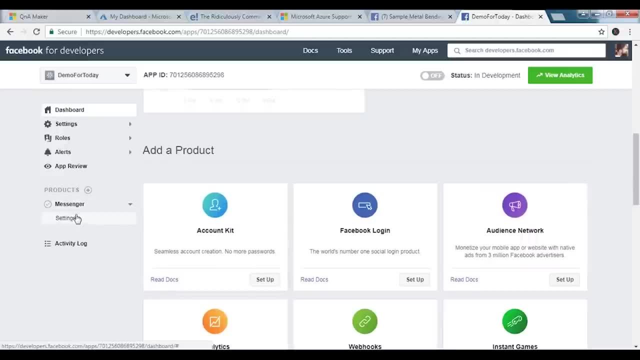 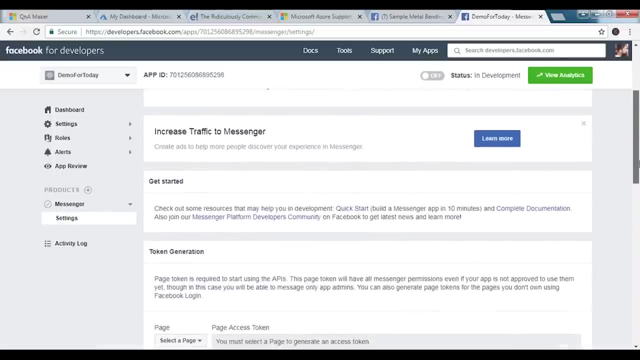 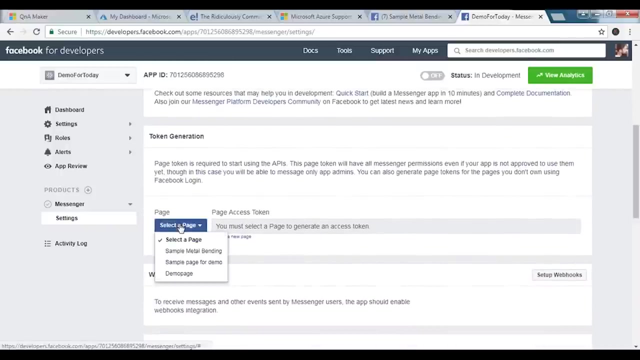 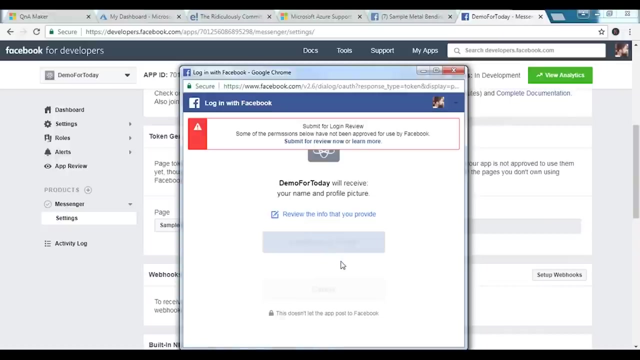 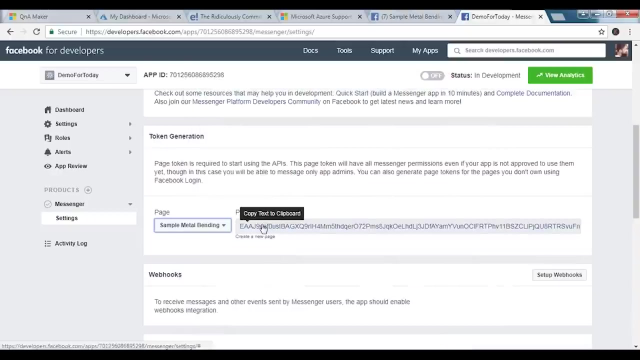 Sorry, dashboard, Yeah, So what is the page that I want to refer? it as sample metal bending, if I'm not wrong. Yep, It would ask me for access. I would say yes And I would say okay, Give access. it would generate a token which I need to copy. 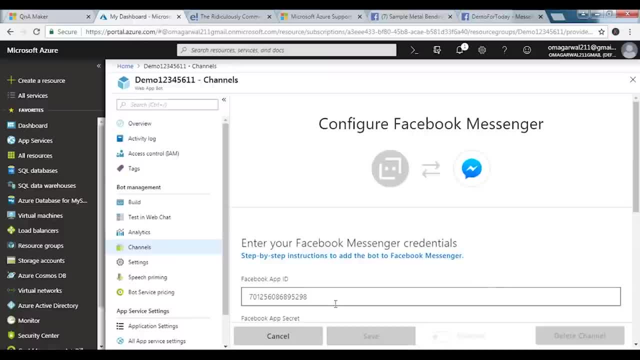 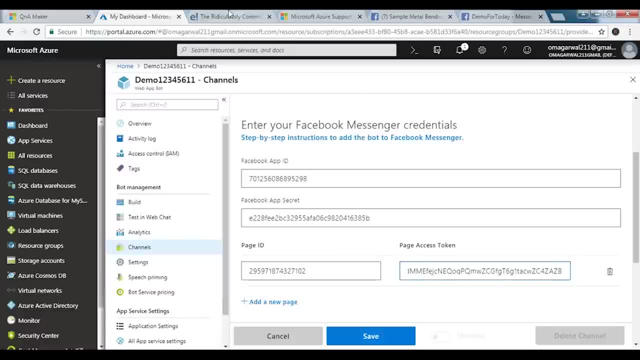 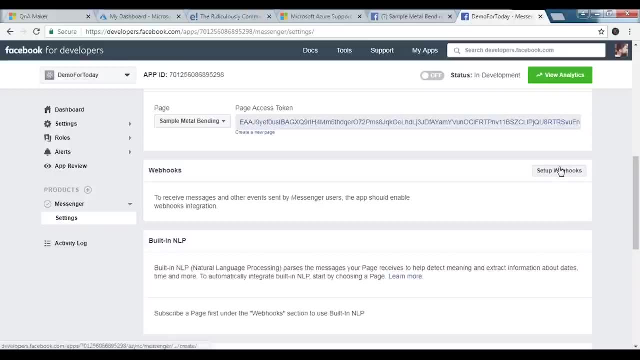 Once it's copied, you would come back to the dashboard of your Microsoft Azure and you would paste it here Like this: and this thing is more than ready to go. now I come back here again. Okay, guys, So I need an API through which I can actually communicate the messages. that is through and 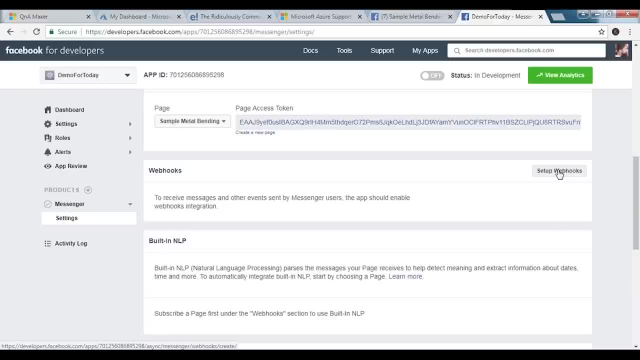 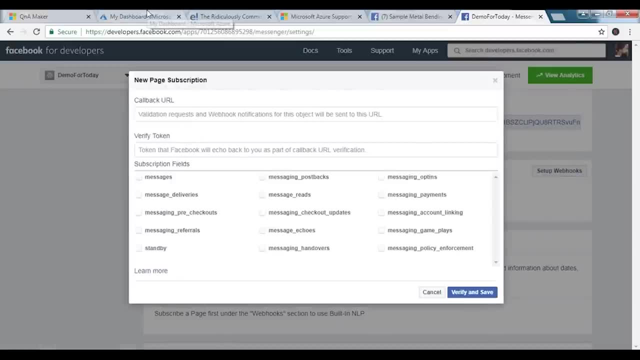 to and fro. So how do I do that? I have something called as webhooks. I won't get into the details of it, but it helps me in better communication rather. So I would be needing to enter in these details here. These are available here on my dashboard. 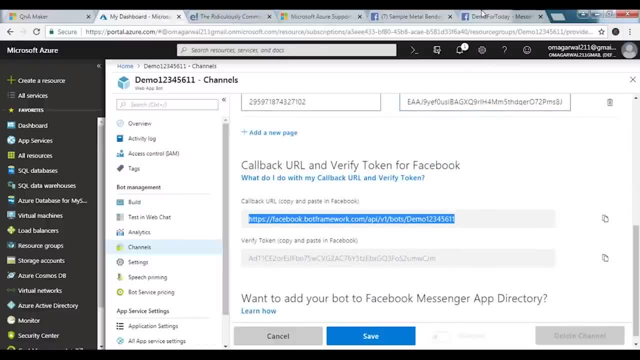 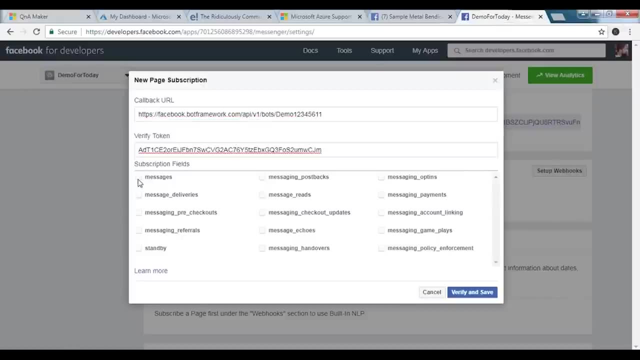 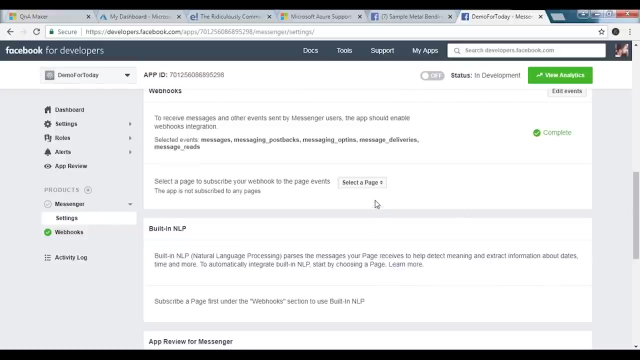 If I scroll down, I need this thing one copy, I paste it here. Copy again, I paste it here. And these are the subscript And fields that I need to respond. So I say verify and save. There you go, Select a pager again. sample metal bending subscribe. 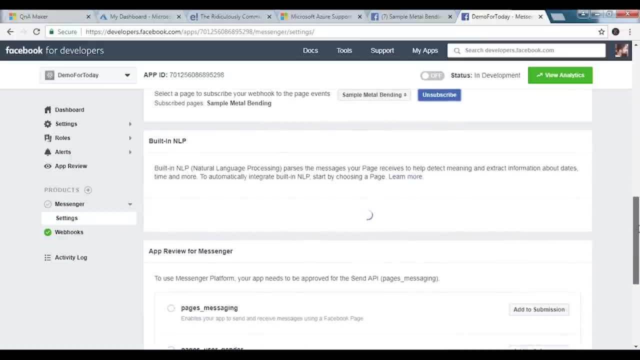 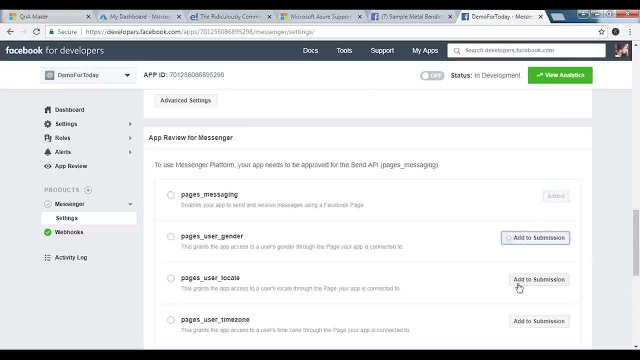 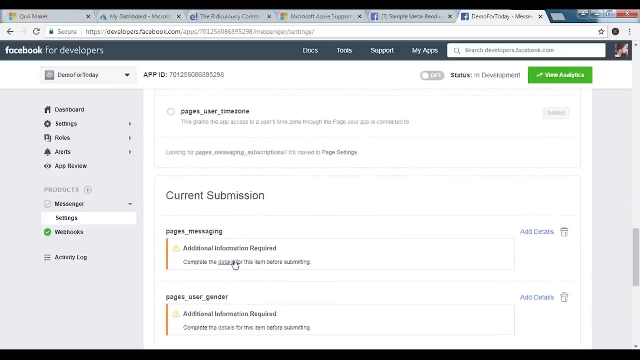 So my webhooks are done. now My next job is NLP Sample metal bending. I say yes And add all these two submission. There are certain details that you need to enter. one is as: in what kind of communication would you like to have your first? select the page. 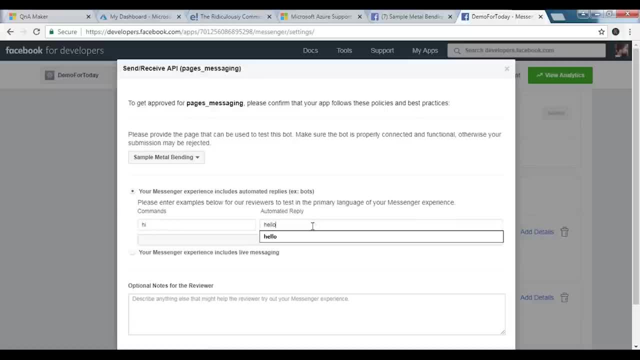 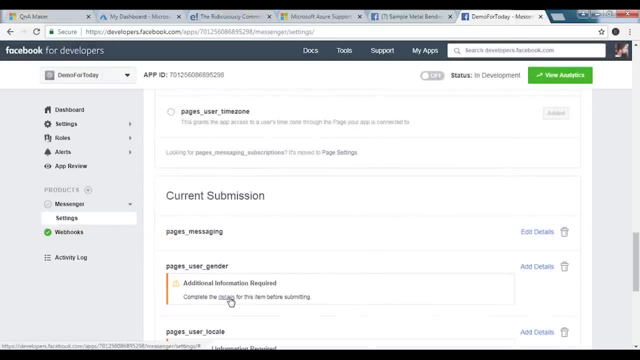 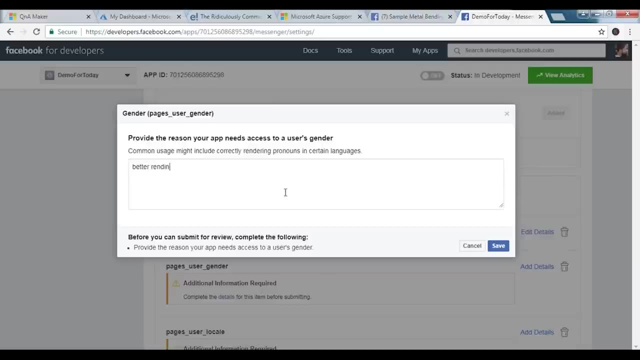 I see, if I say hi, give me a reply saying hello, Okay, and I just scroll down here and I say save, There you go. Next is this for better rendering guys, Do not worry about this thing, This is just a basic input. 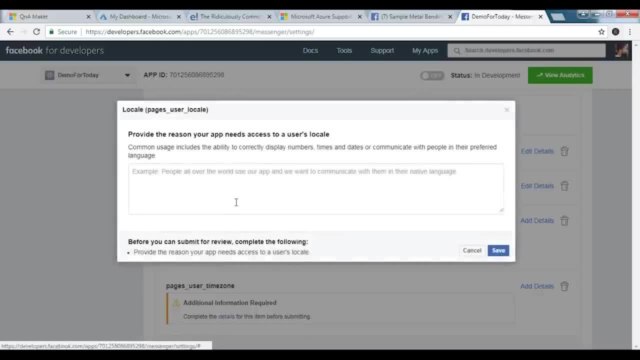 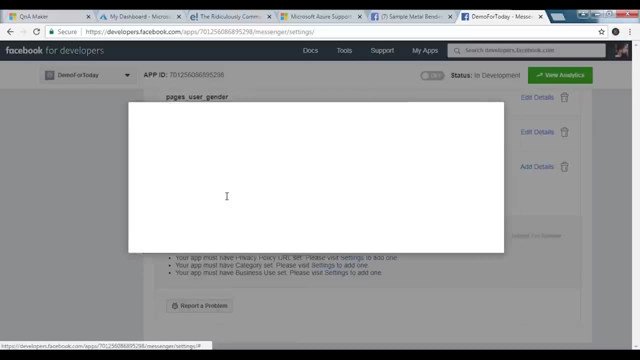 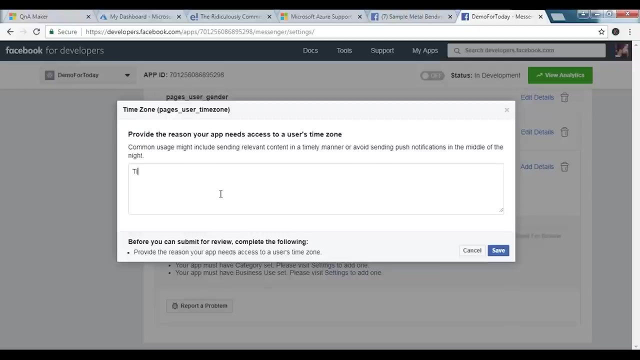 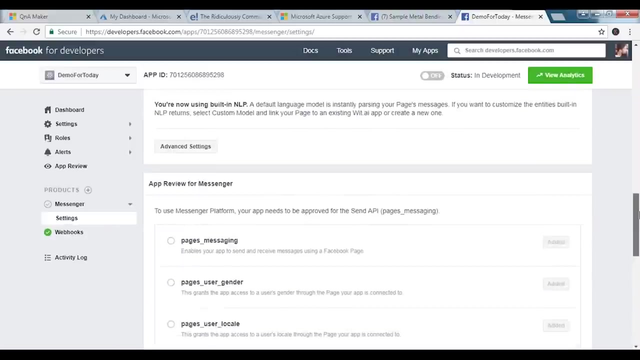 Okay, Hmm, Why do I need to access apps? local, better communication. I say save. And, lastly, I have this thing. Okay, now for better time management, maybe. Okay, I say see, There you go, guys. So this has been saved and almost everything is done and I believe you're good to go. 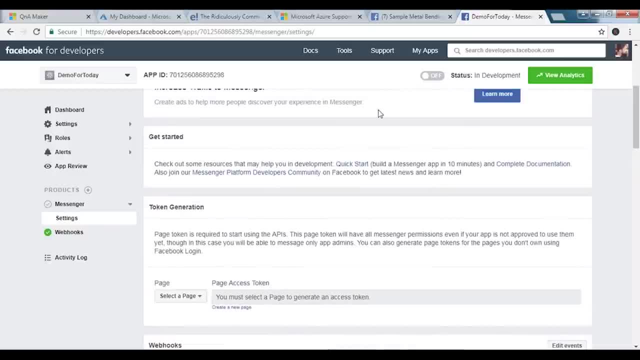 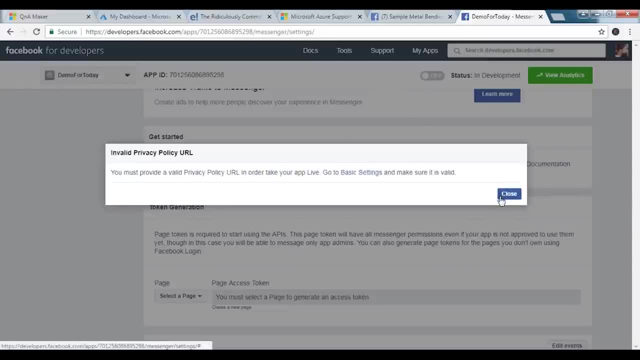 So this information has been entered in properly. before I do that, I need to set this thing live. It would give me an error here, I'm sure. Okay, you must provide a value- It's a valid policy or a URL policy- in order to make your application life. 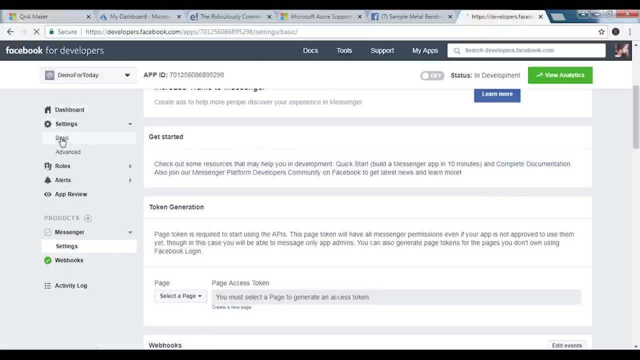 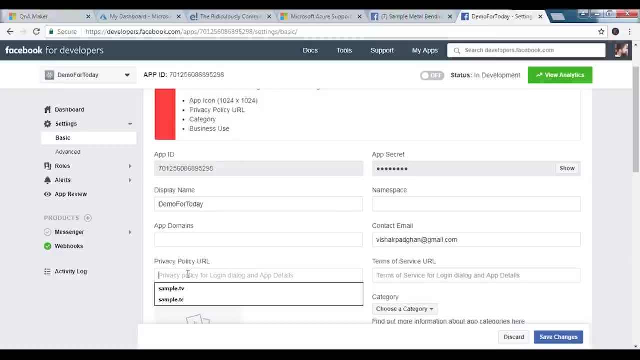 How do we do that? It has to be there somewhere in the setting part. So there you go. Private URL policy. We enter it here. Let's use sample dot TV movie and I say: save the changes. Now can I set it live? 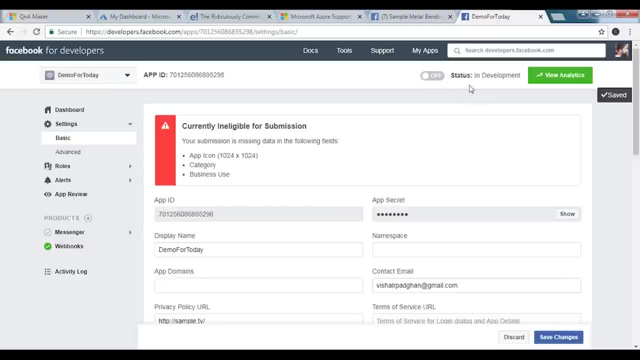 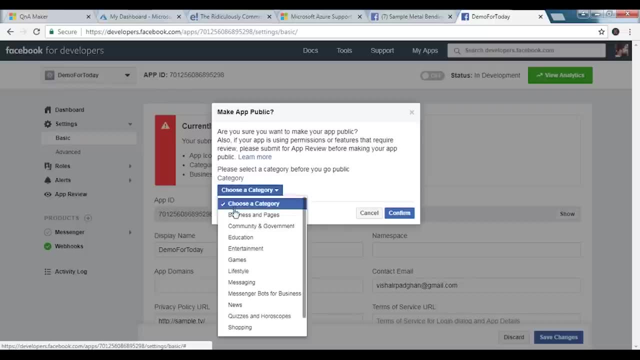 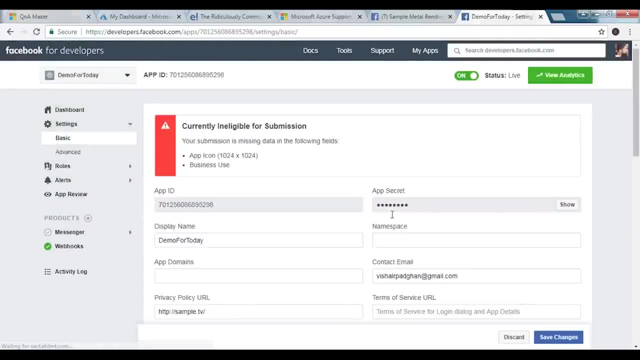 Definitely I can set it live now. So I said set it live. It would say: select a domain first. Which domain do you want to target? It's a education and I say: confirm, There you go. So this is done. Let me just go back to app review. 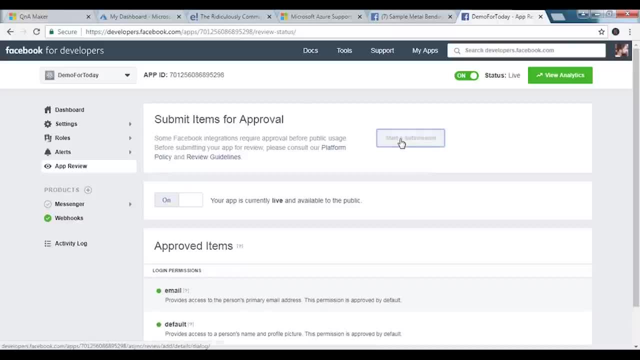 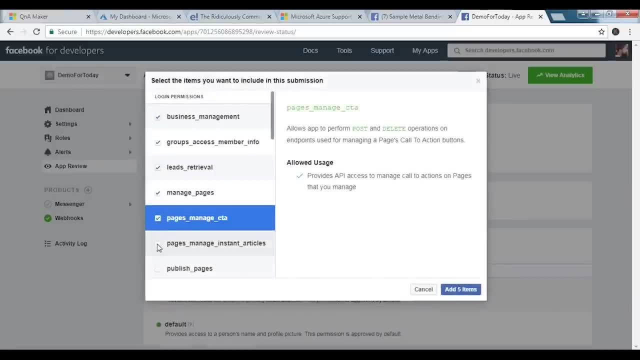 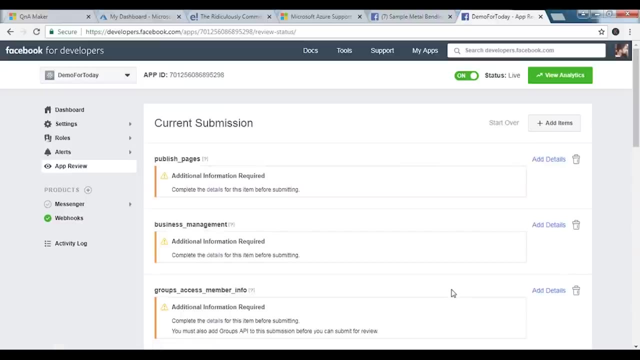 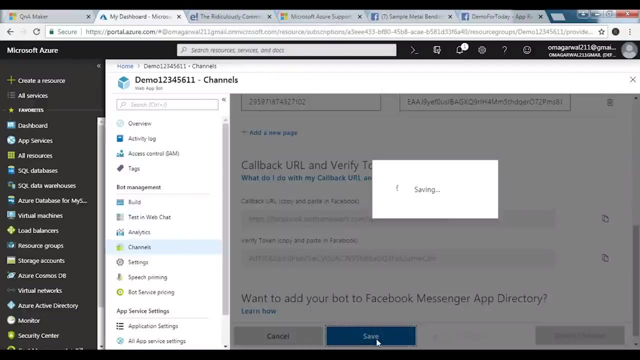 My app has been set live. Start a submission for approval. Yes, please select all these fields And I say add seven items. There you go. So this has been done, guys, and our app is good to go now. So I would just go ahead and save this thing. 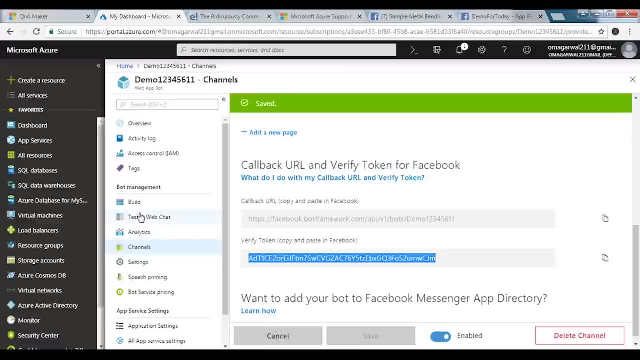 Okay. so if we just go back to the channels, we would see that our Facebook Messenger has been added. So if I do put photo query, that would be replied into my Facebook Messenger or my account would reply. That is, my chatbot would reply using my account. 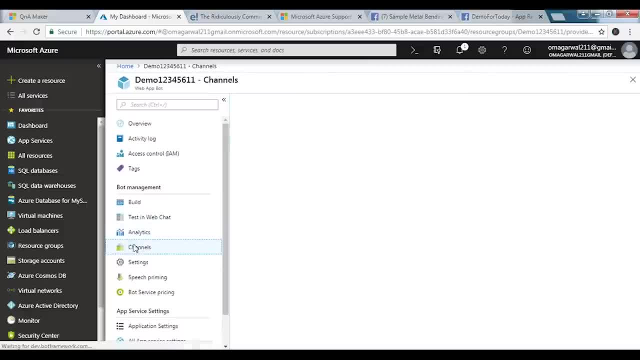 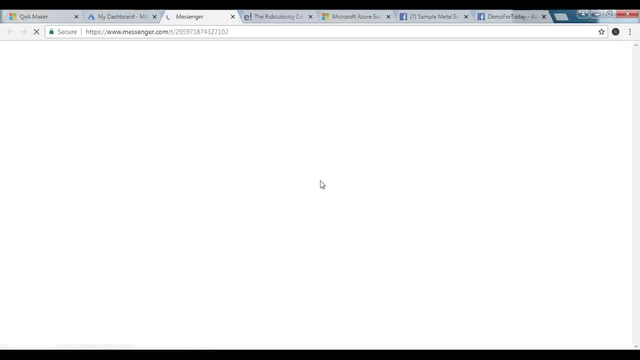 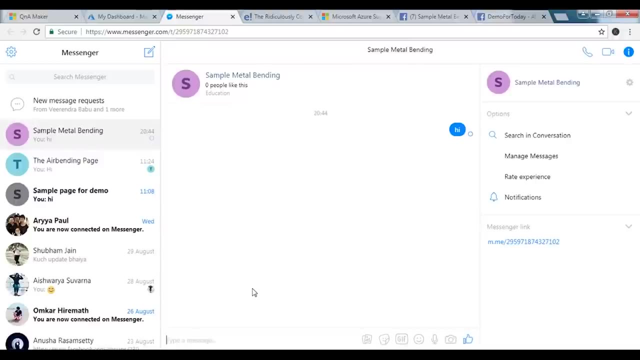 So for that, okay. this refreshing takes a while at times, So we should see the messenger app here. There you go. If I click on it, I get this at my disposal, And if I type hi, this time around I should get a reply. 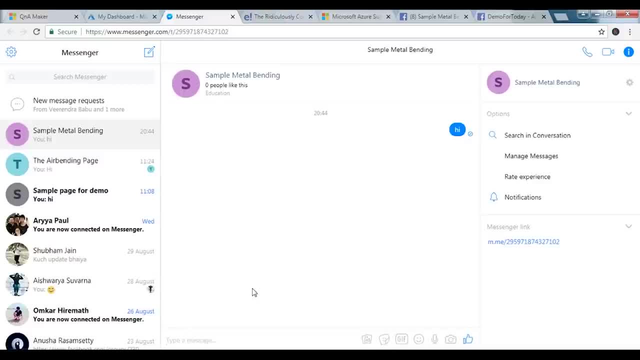 How can we help? Do you provide support? So there you guys, we've successfully gone ahead and we've actually integrated our so-called application with our application on Facebook. That means our chatbot Is replying using our Facebook application. So that is a plus and that is what I wanted you all guys to see. 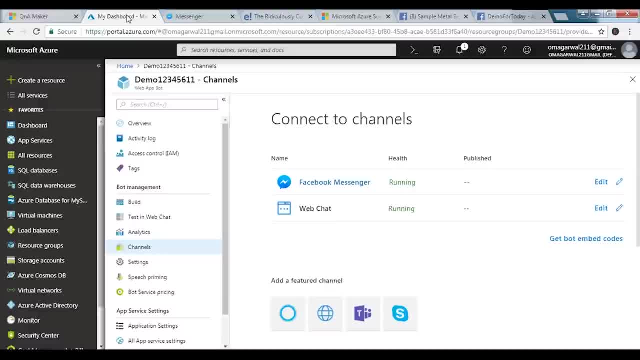 So what we've done is we've gone ahead and created a chatbot, We've created an application on Facebook and we've combined these two so that if I can throw in queries onto my Facebook, or if somebody comes in and throws in a query, my chatbot would reply on that page as well. 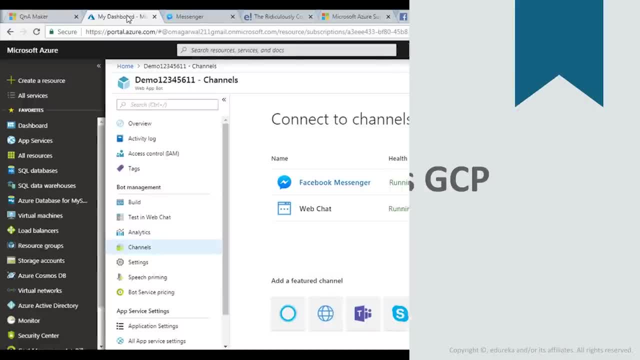 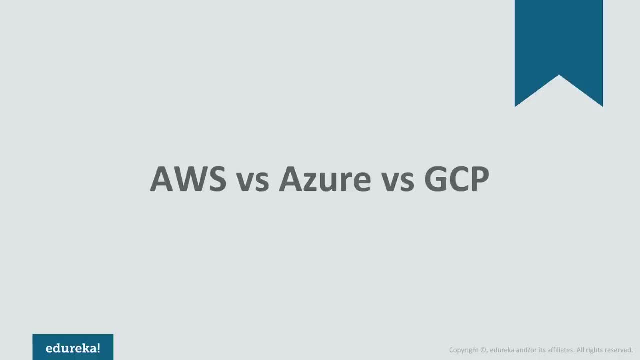 So we've successfully done that, and this was the aim of the session. Today, We'll be comparing these three powerful cloud platforms and see how they stack up against each other. So let's get started before we dig in. Here's the quick intro. 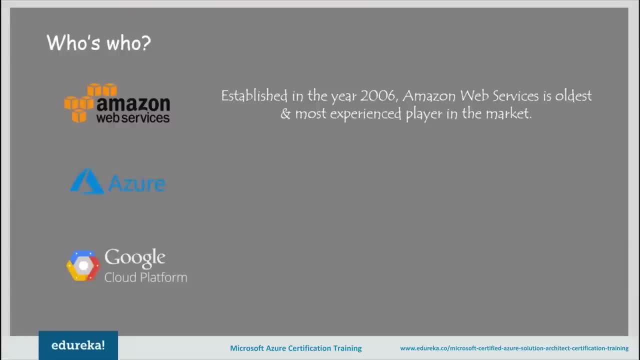 Amazon Web Services was established in year 2006. with 12 years of experience, It's the most popular player in the market. It offers wide range of services across storage, compute, analytics, database and many other fields and, like six to seven years after AWS, Azure was launched by Microsoft though. It's very anger. compared to AWS, It has quickly built a reputation for itself in the market and, just like AWS, It offers complete set of cloud services, and in the same year as Microsoft Azure, Google cloud platform was launched as well. The main reason of introducing GCP was to power their own services like YouTube and Google search, but later on the built Enterprise cloud services as well. 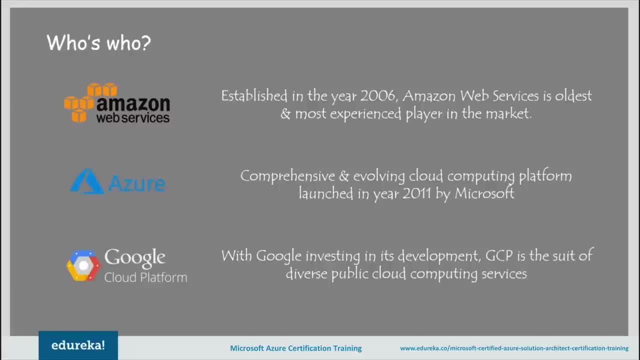 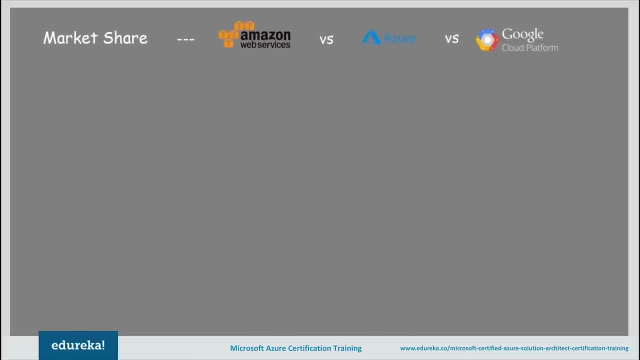 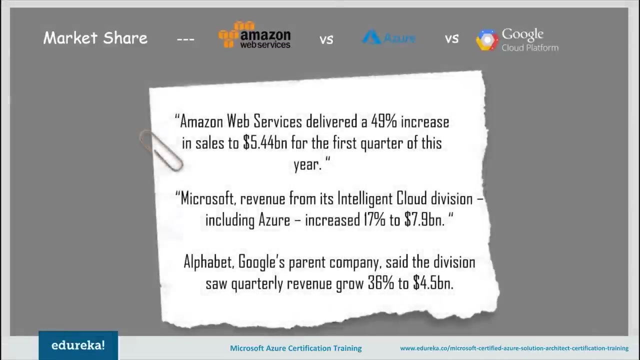 So you can say that Google cloud platform is still an evolving cloud computing platform. Now that we have an idea of the foundation of these cloud providers, Let's see where they stand in terms of market share. So here's the snippet of media interpretation, and you need to keep in mind that this information is with respect to first quarter of 2018.. 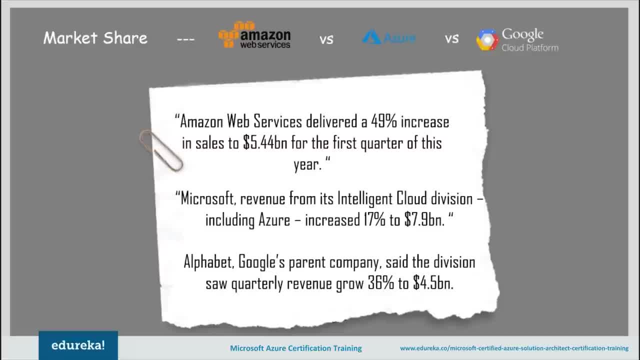 So Amazon Web Services delivered a 49% increase in sales, that is, up to 5.44 billion dollars. Then Microsoft Azure showed a increase of 17%, that's up to 7.9 billion dollars, and alphabet, Google's parent company, said that the division which had GCP, along with other. 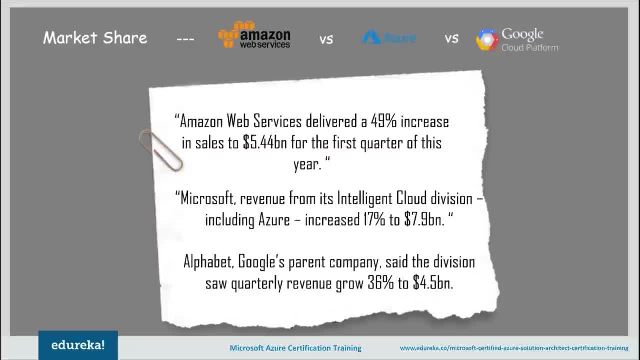 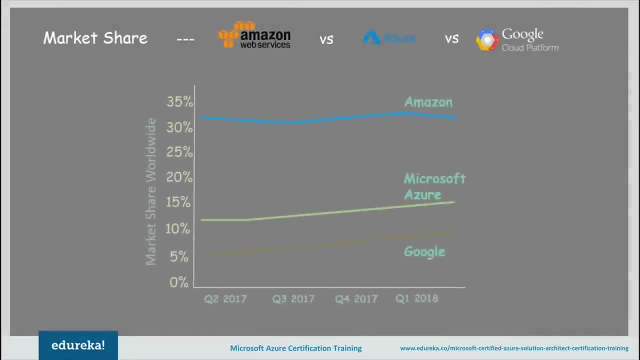 services Like Google Hardware and Google App Store saw a revenue growth of 36%, that's up to 4.5 billion dollars, and with all this stats, I can confidently say that Amazon Web Services is still in the lead and holds line share of Market. 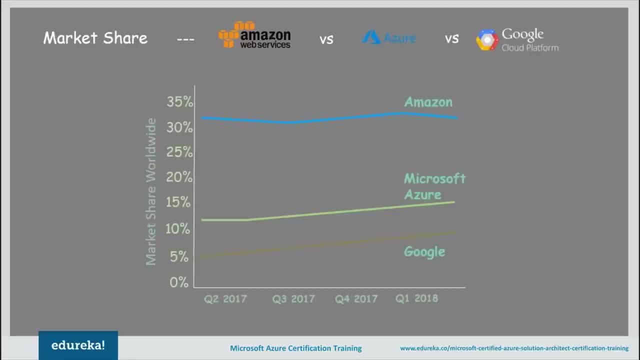 So if I have to tell that in form of numbers, then Amazon holds 33%, that's almost about one third of the total market. Then we have Microsoft, which holds about 13%, and finally Google, which holds about 6%. so to conclude, Amazon Web Services. 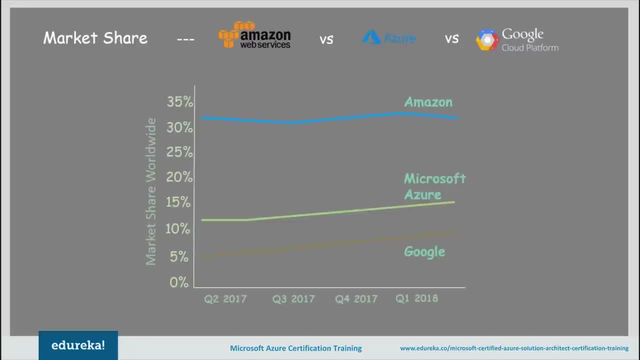 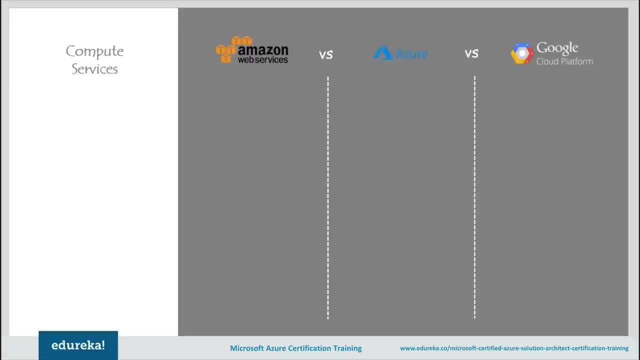 Market share is bigger than its next two largest competitors combined together. Now that we know who leads the market, Let's compare these cloud providers based on the services they offer. So first let's consider compute services. The compute services offered by all these three cloud providers are equally powerful and yet unique in their own way. 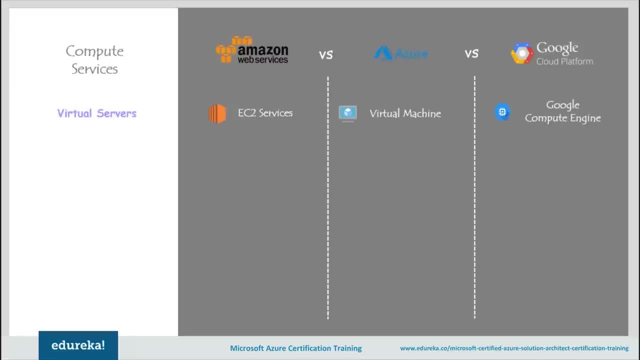 Amazon's primary compute service is easy to, which is elastic cloud compute. as for the Microsoft, its primary compute service is known as virtual machine. Unlike Amazon's easy to, this virtual machine provides enhanced security, hybrid cloud capabilities and integrated support for Microsoft software similar to Amazon's easy to and Microsoft Azure's virtual machine. Google cloud platform offers compute engine. 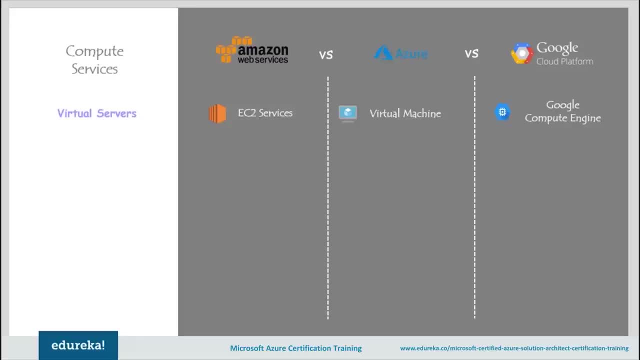 This compute engine offers automatic price discounts and it runs on an infrastructure that uses half the energy of typical data center. Well, that's about the primary compute services. Now let's take a look at additional Compute services. I'm sure you know that all this cloud providers provide a combination of IRS, pass and SAS services. 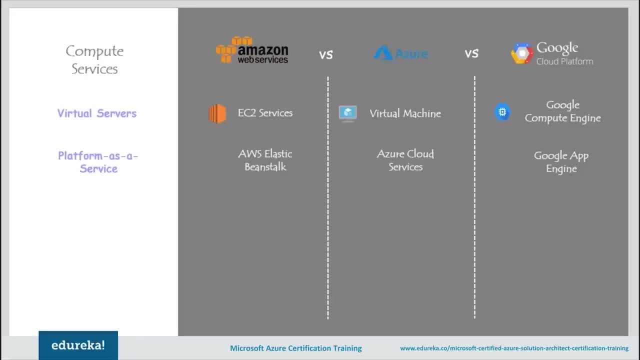 But to say, platform as a service is strong suit of Microsoft. So Microsoft Azure offers Azure cloud services using which you can easily deploy, scale and run an application on cloud. Amazon's elastic beanstalk and Google's Google App Engine are similar to this Azure cloud services. 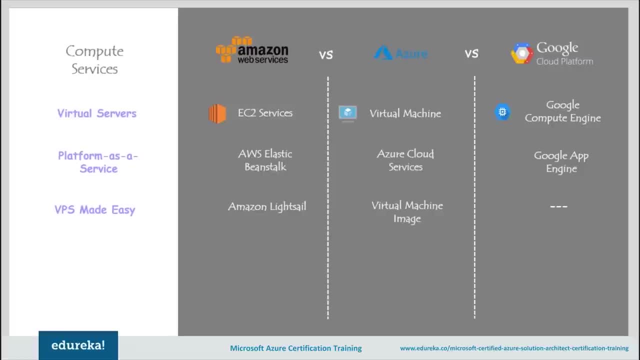 Moving on. Let's say you want to deploy A virtual private server without bothering about the underlying infrastructure, Then Amazon light sale is the best option. similar to Amazon light sale, Microsoft Azure offers virtual machine engine and Google cloud platform is yet to launch one such similar service. 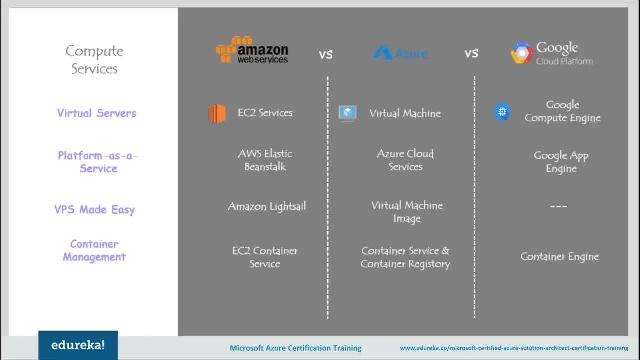 So all this cloud providers also support container platform and they offer their own unique serverless computing services as well. to conclude, in terms of compute, all the three cloud providers offer equally powerful compute services, and yet I can say that Google cloud platform is still lagging behind in some areas. 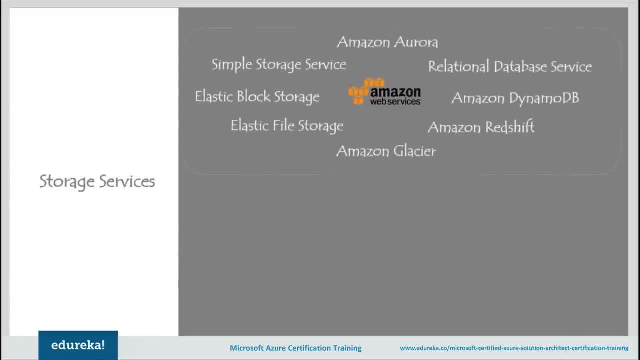 Now moving on to storage services. AWS offers a long list of storage services. to name some, it offers simple storage service, elastic block storage and elastic file storage. talking about database options, at offers Amazon Aurora, a high-performance relational database, Amazon RDS and DynamoDB managed NoSQL database. AWS also offers a cloud-based data warehouse, which is also a cloud-based data warehouse. 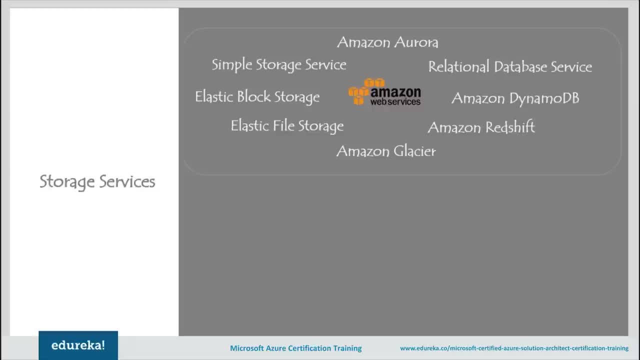 We know as Amazon redshift. though It doesn't offer a backup service per se, it offers Amazon Glacier for long-term archival storage at very low rates. Then, talking about Microsoft Azure, it offers way more storage services than compared to AWS, and just for the basic storage. 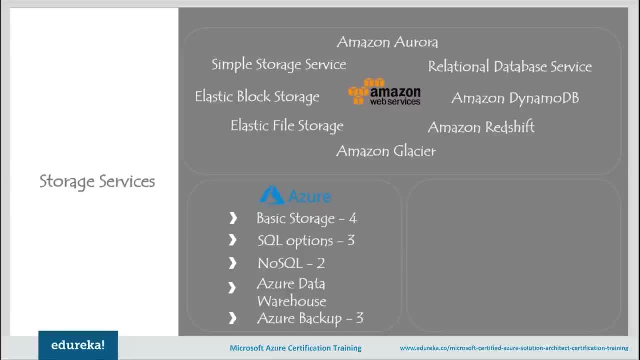 It offers four options and for database, It offers six to five options and, like AWS, It also offers cloud-based data warehouse, which we call Azure data warehouse, and, unlike AWS, Microsoft, It offers an actual backup service called Azure backup. in addition to this Azure backup, 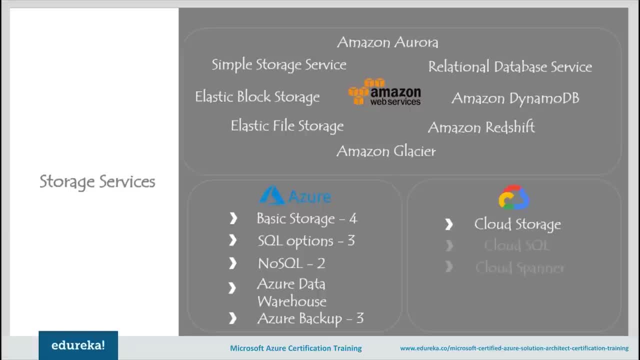 It also offers site recovery and archival storage. a final contender, Google cloud platform. when compared to AWS and Microsoft Azure, offers less number of storage services, but the storage services like cloud Spanner and cloud Bigtable are quite popular and it doesn't offer backup or any archival storage service. 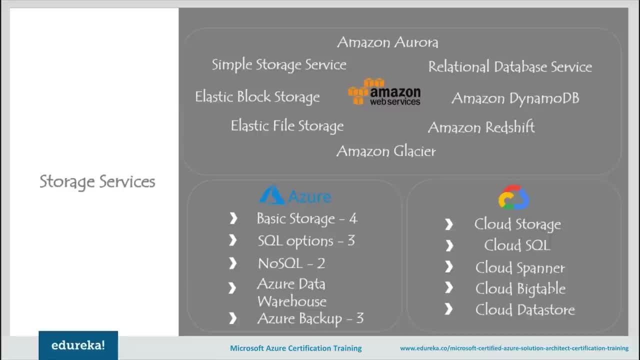 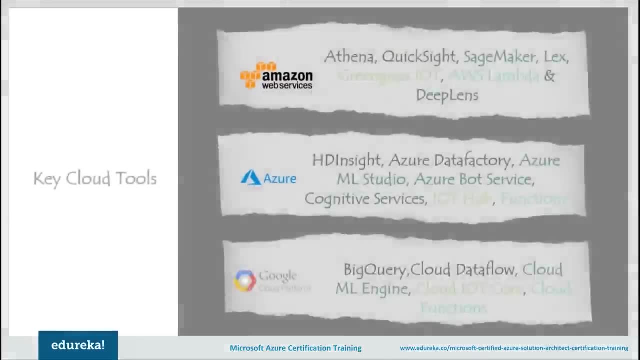 So, in terms of storage, Amazon web services and Microsoft Azure stand neck-to-neck, whereas Google cloud, Our platform, has still long way to catch up with Amazon and Azure. All these vendors are actively launching services aimed at cutting at Technologies like serverless computing, machine learning, analytics and IOT. 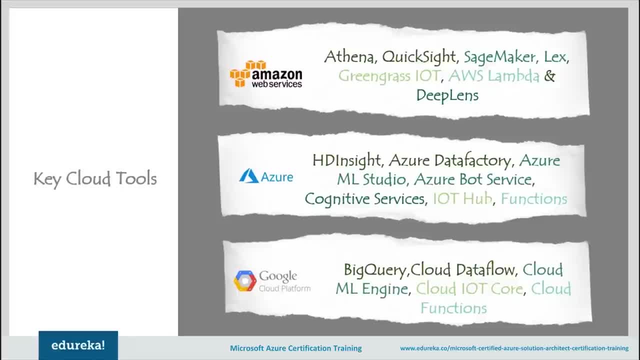 If you're talking about Amazon web services, it offers Athena and QuickSight, using which you can get data insights. It also offers a machine learning service called SageMaker and Lex, using which you can build voice and text chatbots. And as for the IOT devices, it offers green gas IOT messaging app. 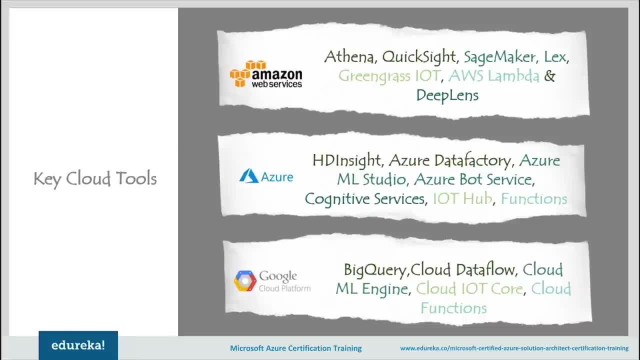 And as for Microsoft, it has invested heavily in artificial intelligence and it offers a machine learning service called ML Studio and a bot service called Azure bot service. In addition to this, it also offers cognitive services like Bing search API, text analysis, VPI, computer vision API and many other services. and then Google- Google cloud platform, as known for its analytical background. 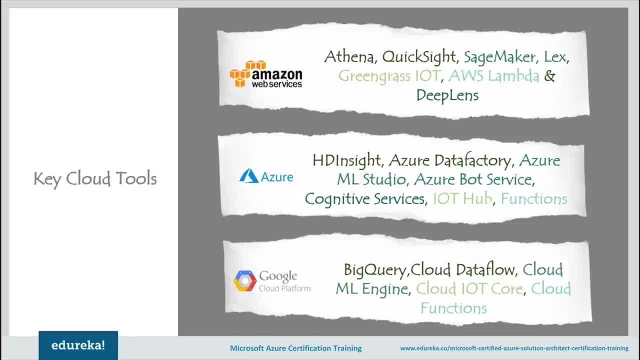 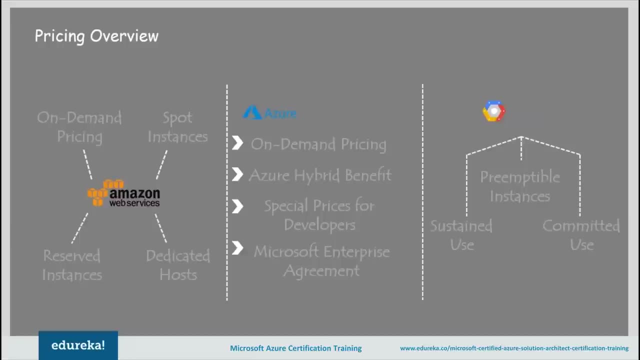 I'm sure you might have heard of a service called BigQuery that enables interactive analysis of massively large data sets. In addition to all this, it also offers IOT and serverless computing services, but still there in beta version, though. One of the major benefits of most cloud providers is that competitive pricing strategies- and all this three cloud providers- follow pay-as-you-go model. 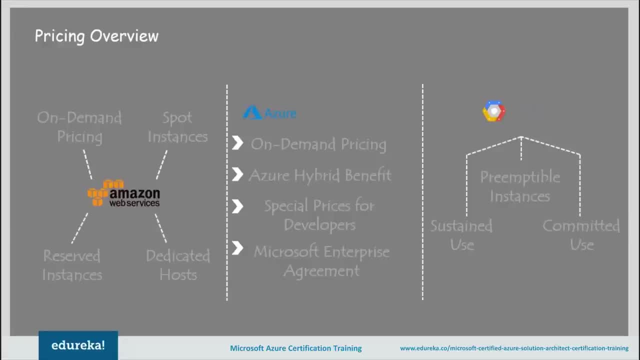 It means you need to pay on the basis of usage. Where an Amazon charges you on hourly basis, Microsoft Azure and Google cloud platform charge you on minute basis, And All these three cloud providers offer you on-demand pricing. That is the standard price you pay when you access their services. 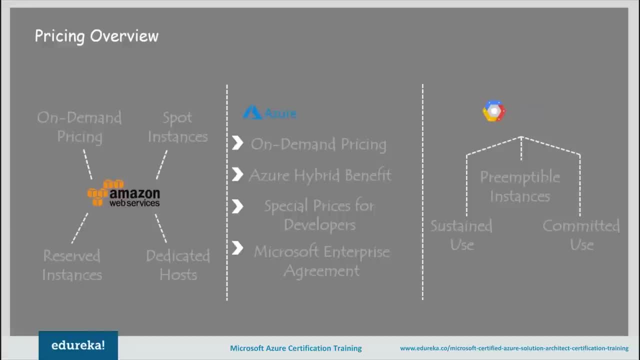 And then, in addition to that, Amazon also offers you spot instances, reserved instances and dedicated host where you are liable to get certain discounts based on some conditions, Then, as for sure, it offers special price for developers and something called Azure hybrid benefit. Suppose your organization runs some sort of Microsoft software on its own data center. then, using this Azure hybrid benefit, 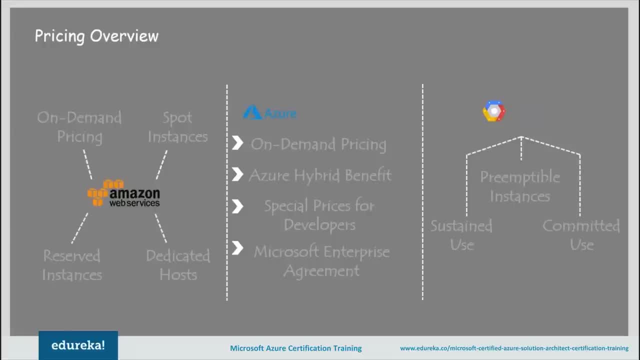 You can get 40% discount, depending on the type of Microsoft software you use it, and as for Google, it offers customer-friendly pricing compared to Azure and Amazon web services. It offers different type of discounts. to name some, you have sustained use discount. These type of discounts usually kick in automatically when you keep using same instance for most part of the month. 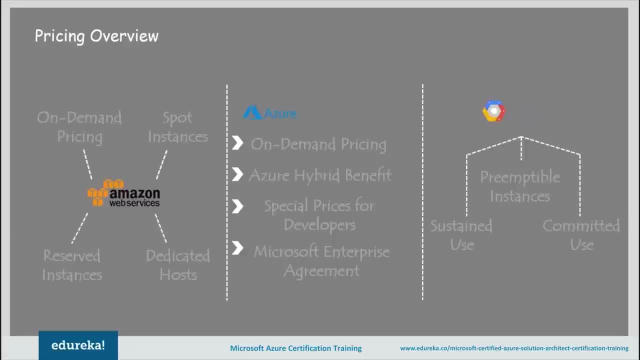 Then you have preemptible instances, which is similar to Amazon spot instances, And one more thing is that all this three cloud providers offer you long-term discounts. So if I have to conclude, Google cloud platform is almost always the lowest class provider. Then you have a shot. the second least expensive and its prices are usually close to Amazon's, and if you are looking for long-term discounts as an Amazon web services as the best option. 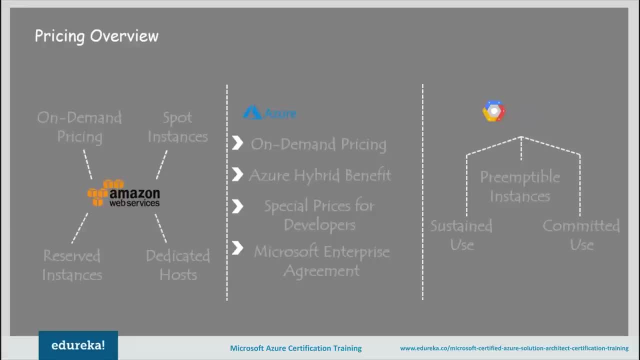 The big takeaway here is that you won't know which vendors least expensive until you know what you need with this cloud providers. So now that we've looked at the features and pricing, let's see which one of this cloud providers are easy to get started with. 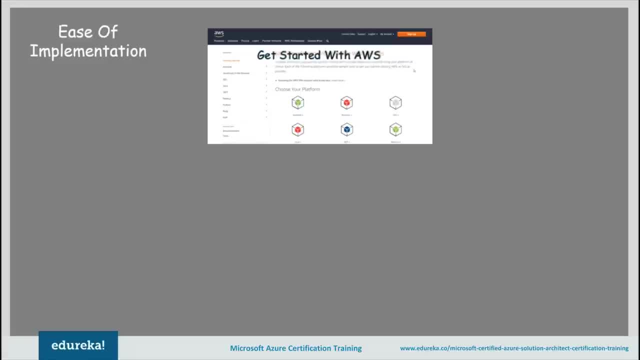 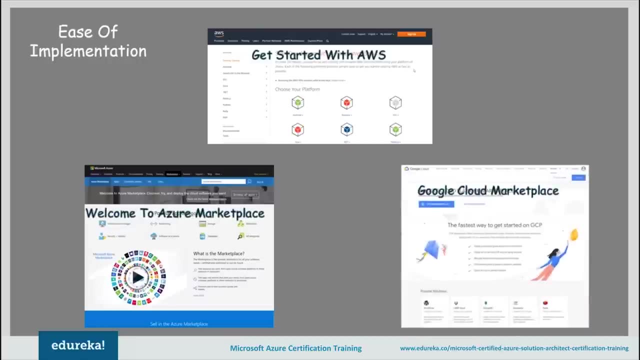 So any guesses? Well, if you're guessing AWS, it's right. AWS provides this nice and easy page to start using their services. You can see that the break it down by platform you want to work on. So, whether you're making an iOS app or writing in PHP, they provide you some sample code so that you can easily get started with. 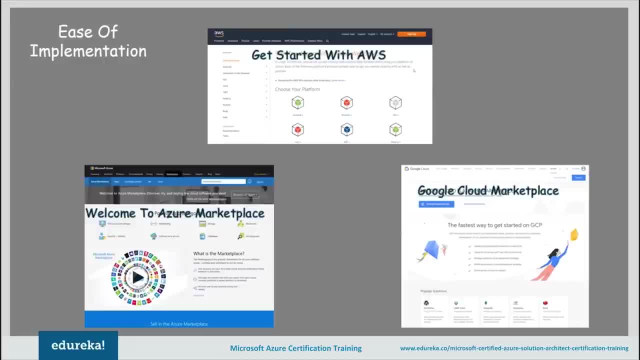 And as for Microsoft Azure and Google cloud platform, the segregation of services here is not that great when compared to AWS. That's mostly because they are less experienced, So you need some guesses Getting used to before you feel comfortable to start using their services. 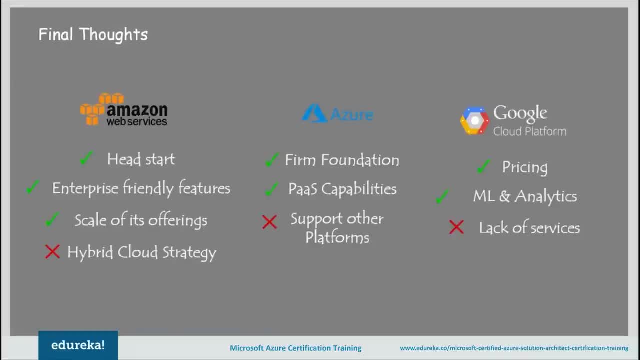 So there you go, guys. We've compared all these cloud providers based on their market share, features, pricing and implementation. to conclude, Amazon web services still remains to be the most popular cloud provider, Mostly because of the seven years head start It has over its competitors, and AWS services are far more evolved and functionally rich when compared to other services. 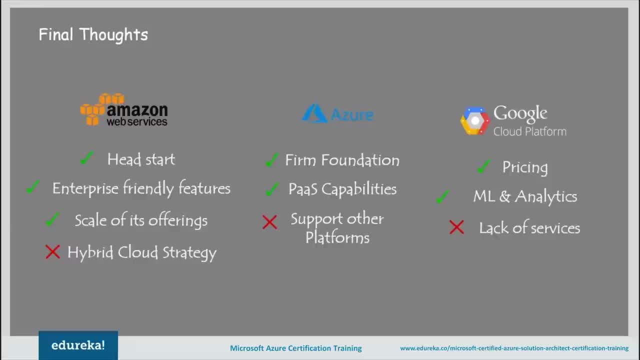 It has its weak points as well. It doesn't support hybrid cloud strategy and its counterpart, Microsoft Azure. though It was launched several years after AWS, It's doing fairly well in the market. It has its firm foundation and is actively competing against Amazon web services. 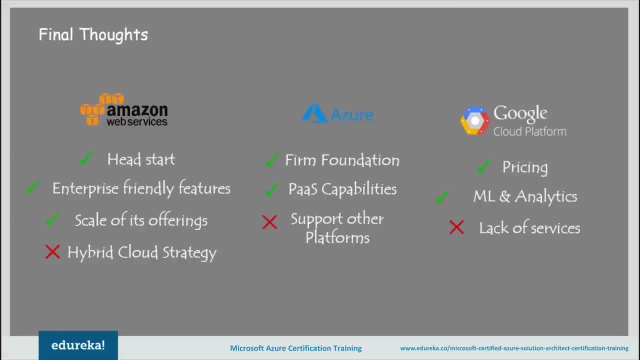 You shouldn't be surprised if it overtakes Amazon web services in near future. And then our final contender, Google cloud platform. when compared to AWS and Microsoft Azure, is still not that popular, but it's known for its pricing strategies and machine learning and article tools it offers. 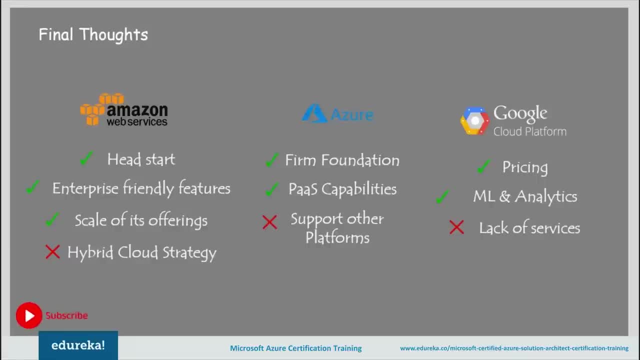 But other than that, it has a long way to meet up Amazon web services in Azure. So, guys, every cloud computing platform has its ups and downs, but the best cloud computing platform, or the one that's suitable for you, Julie, depends on what you expect from these cloud providers or what kind of services you need from these cloud providers, these cloud providers, or what kind of services you need from these cloud providers. 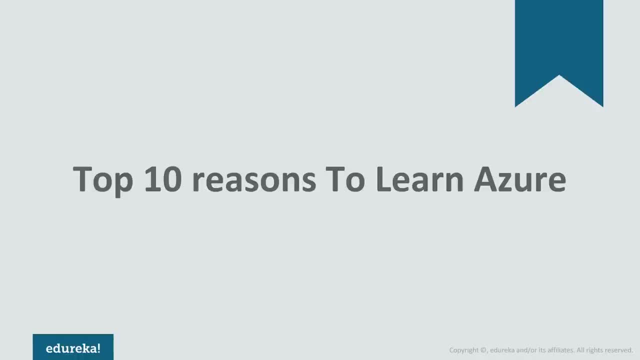 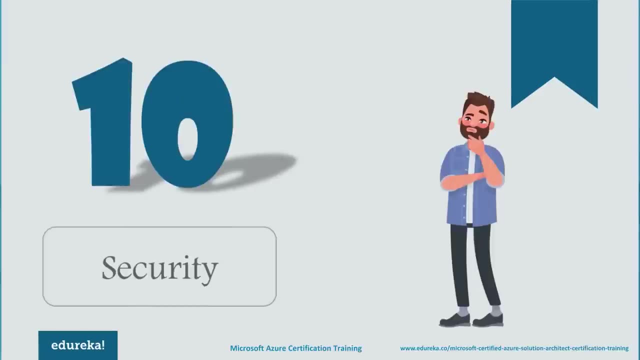 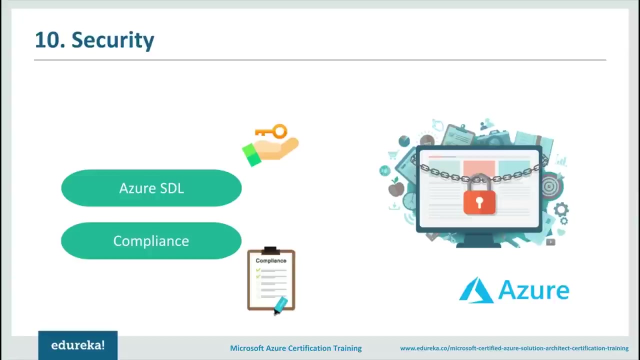 Today, I'm going to give you top 10 reasons as to why one should go ahead. and then Microsoft Azure. So let's not waste any time and quickly get started. The first reason on my list is security. Now, when you talk about cloud service providers, people normally have the doubts whether these platforms are secure enough or not. 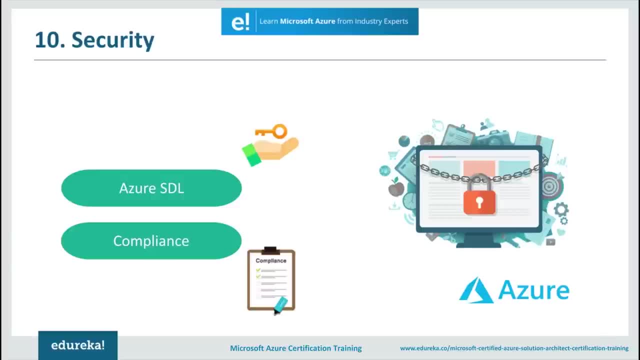 but Microsoft Azure puts all these debates to rest. it uses something called a security development life cycle. This ensures security even from the operations perspective and also from the customers perspective. plus, they have more than 50 compliance programs which ensure that all these stringent policies are implemented. 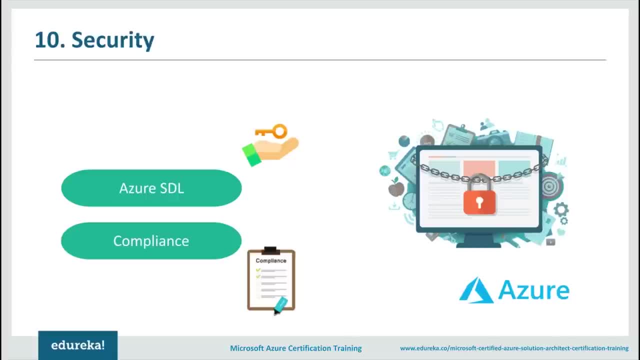 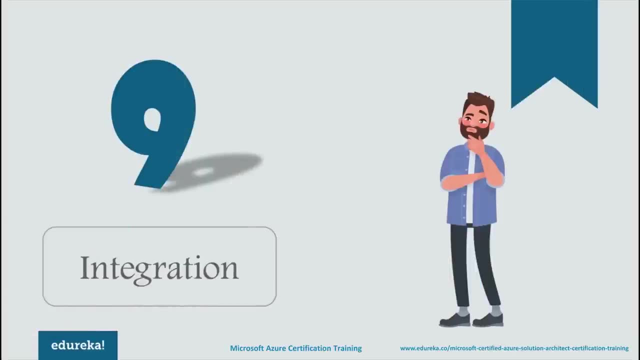 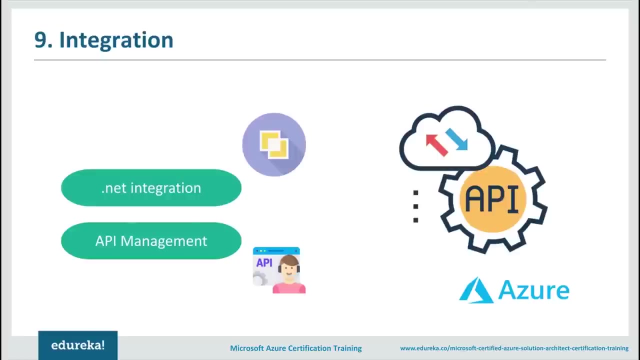 and they're thoroughly taken care of. So if you are worried about security, do not. Microsoft Azure will definitely take care of all your security. concerns Integration, since people want to move their data to cloud. We would be talking about a lot of applications. and when you talk about a lot of applications, 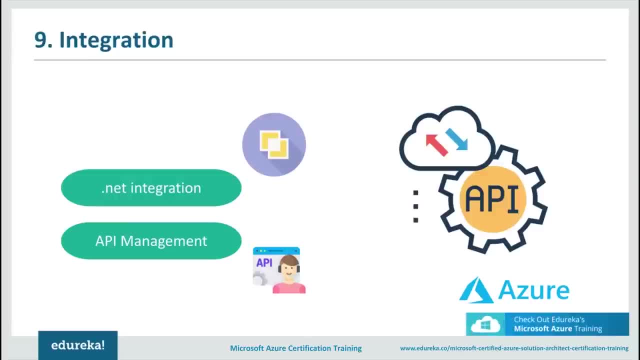 you need to be able to integrate these applications with your service provider. That is why you need to have good integration and apis. What Microsoft Azure does is it first of all provides you with dotnet integration. now, we all know that dotnet is a very popular language. 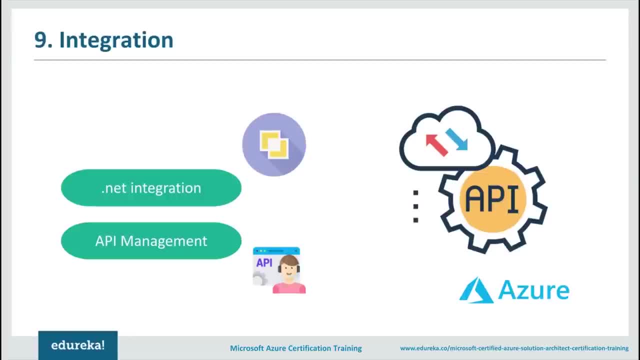 and if you are able to incorporate or use Microsoft dotnet with Microsoft Azure, it would be a big plus, and Microsoft Azure exactly does that. apart from that, if you do want to go ahead and use other applications or maybe other Technologies, you are free to do that as well. 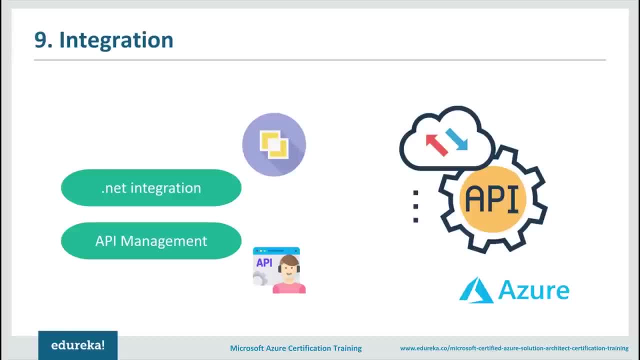 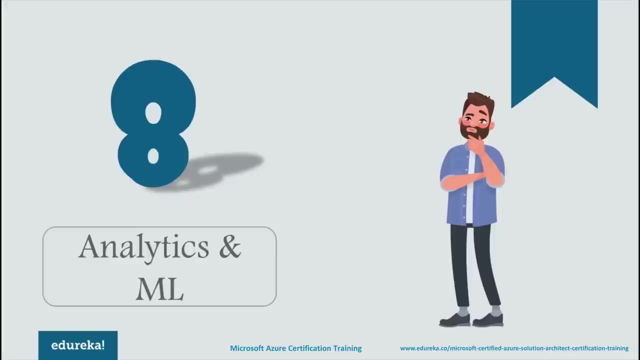 because it has something called as API management, which ensures integration or collaboration of various applications with Microsoft Azure. So, again, integration is something that can be done very easily by using Microsoft Azure Analytics and machine learning. now, when you talk about analytics or machine learning, you know that you would be dealing with huge amount of data. 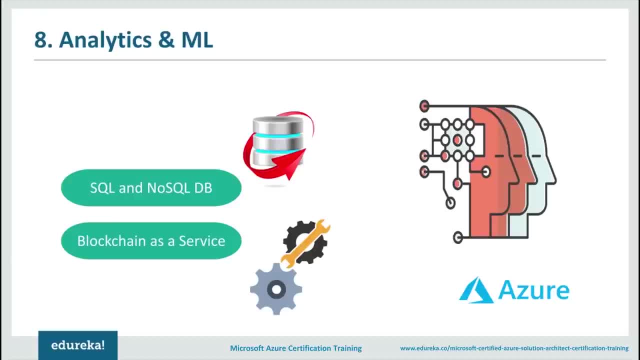 Now, in that case, you need databases that can deal with both SQL kind of queries and no SQL kind of queries. That means both structured and unstructured data. Microsoft Azure makes arrangements for these type of queries and databases as well. It also supports blockchain as a service. 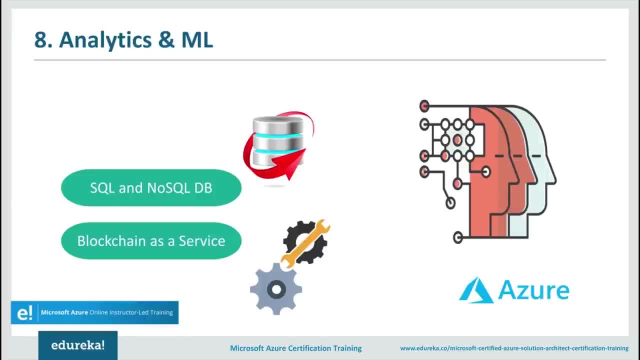 and various other algorithms, like your machine learning algorithms, your artificial intelligence algorithms and a lot of things that you can do in machine learning and data science. basically, and we all know that these Technologies and terms are very popular in recent times and they are here to stay, and Microsoft Azure will ensure that it takes care. 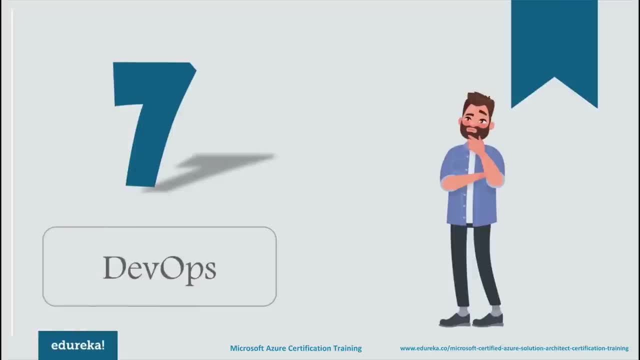 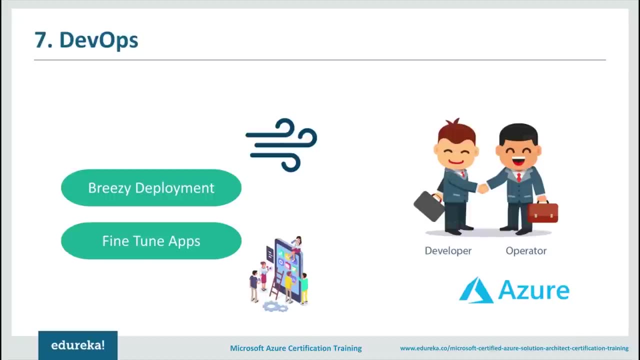 of all these Technologies and approaches as well. DevOps: this is another approach which is very popular. What it does is it brings in developers and operators together. when you talk about software development Now, it has various phases, and these two teams play a very important role in it. 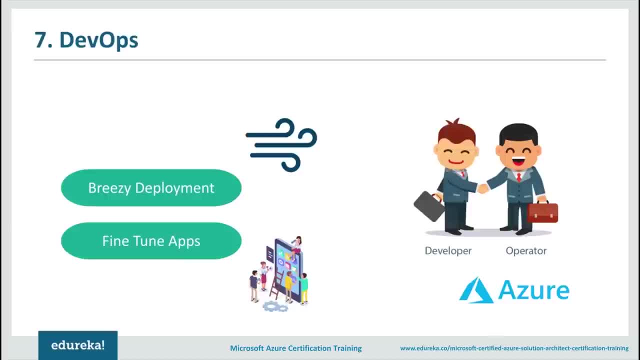 And they normally have a conflict because they share similar interests but they deal in different environments. What DevOps does is it brings these two teams together, and that ensures breezy development, and it also ensures fine-tuning of various applications. Microsoft Azure also incorporates this approach. 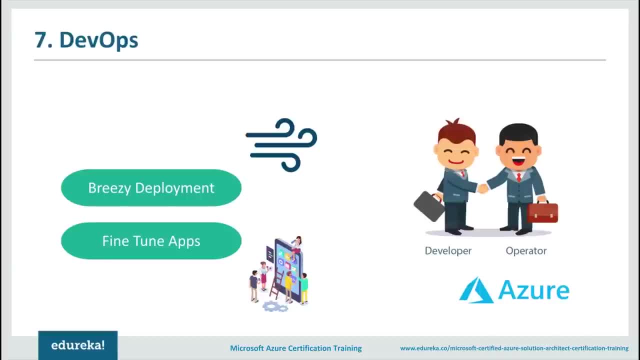 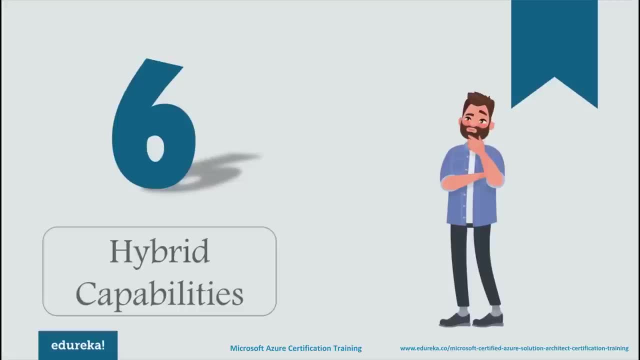 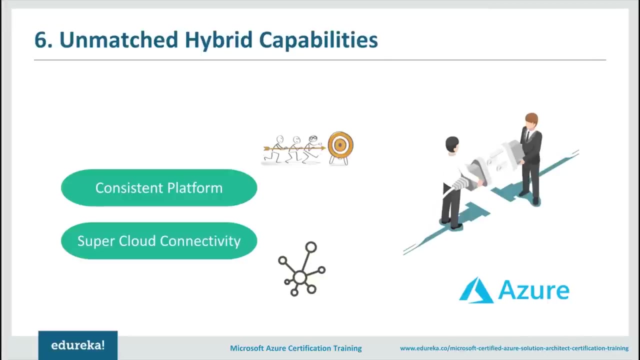 So if you are interested in DevOps, Microsoft Azure will let you do that as well. Sixth on this list is hybrid capabilities, or, in simple words, Customization. you need to have a platform that is highly consistent, because you are talking about different applications coming together. Microsoft Azure provides. 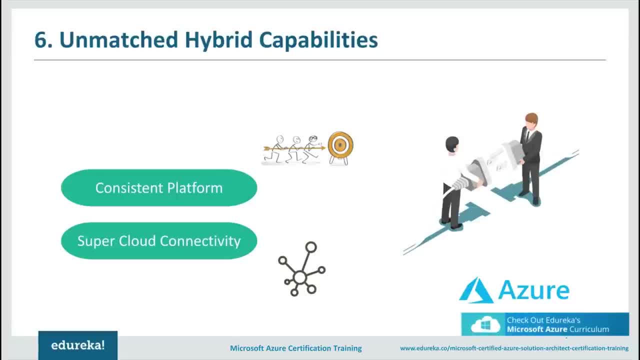 with that kind of a platform. Plus, it also ensures high level of connectivity. It uses something called as CDNs, that is, content delivery networks and VPNs or these things ensure static movement of data and applications, and that is a very healthy point to have when you're talking about hybridization. 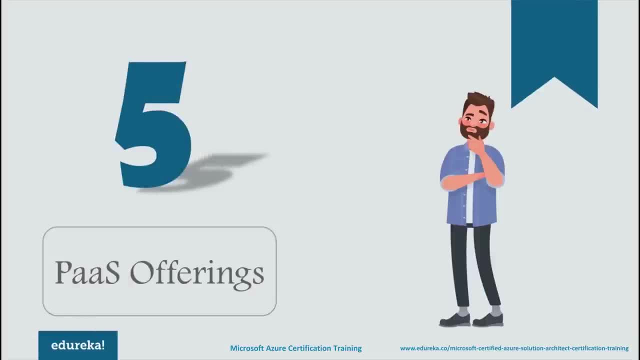 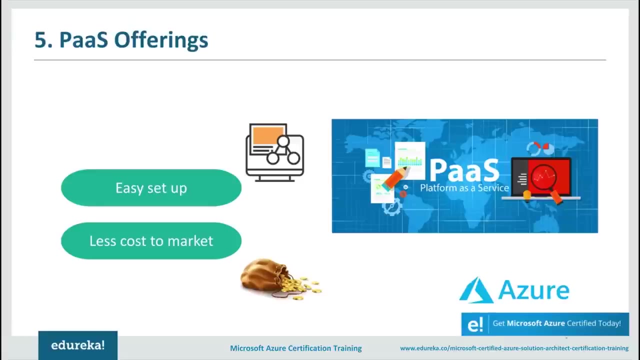 or customization of your applications. Fifth on this list, We have pass offerings. pass stands for platform as a service. what Microsoft Azure does is it provides you with a platform where you can easily set up your applications. That means you can build them, you can manage them. 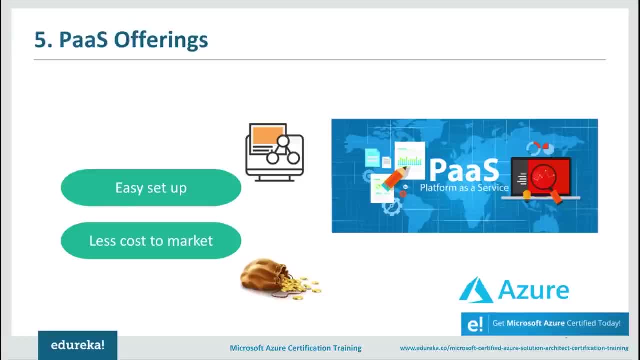 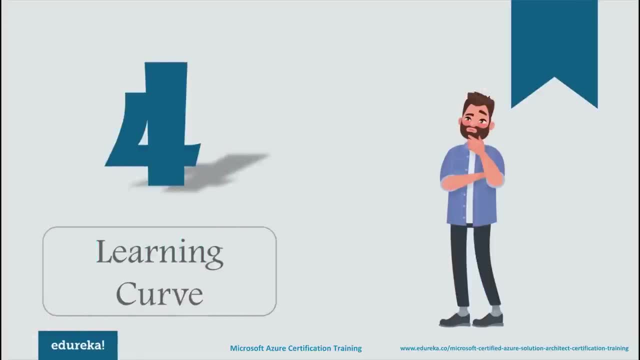 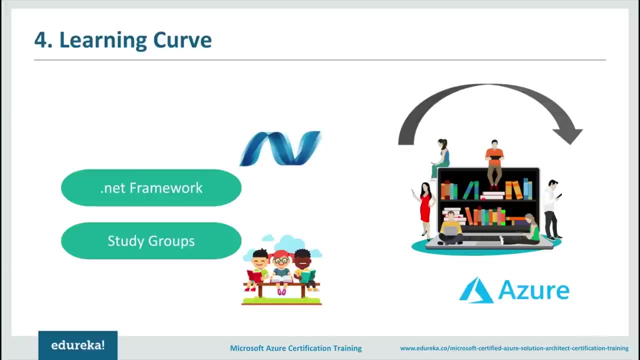 You can monitor them and also take care of all the security issues as well. And also all these things happen at a very low cost. That means your cost to set up is very less. Fourth on this list: We have learning curve if you wish to incorporate a particular technology. 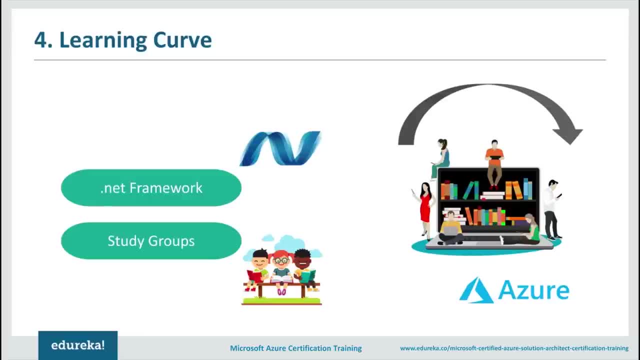 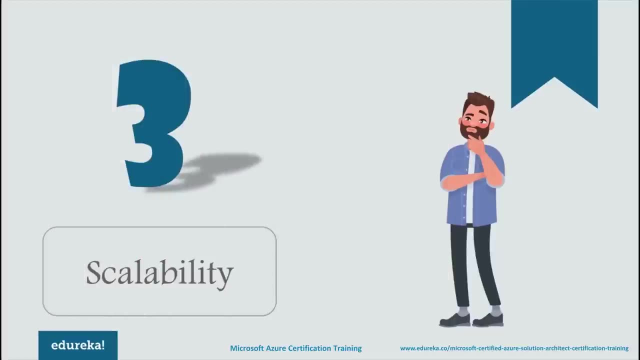 or a service provider. it should be easy to learn, and that is the case with Microsoft Azure. It is fairly easy to pick up and understand. plus, we have a lot of documentations and study groups that let you go ahead and learn Microsoft Azure. The next point on this list is scalability. 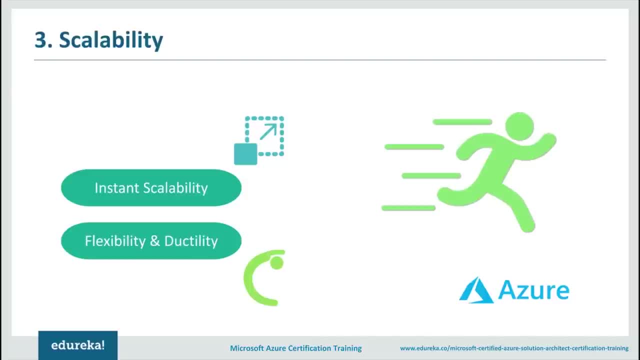 This is often the problem with cloud services. The reason why cloud came into existence was it wanted to overtake or overcome this problem of scalability, because it was difficult to pre decide how many servers or space you are going to use. so people move to cloud, and Microsoft Azure definitely takes care of this issue. 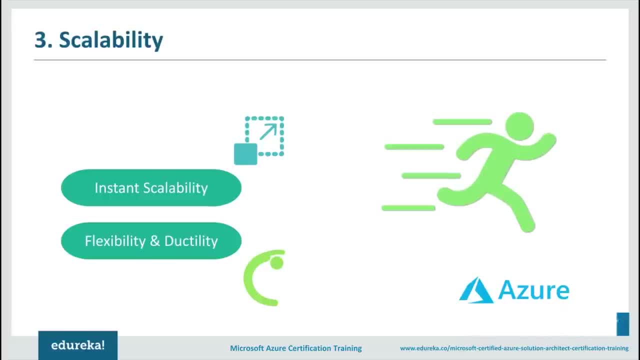 because it enables granular scaling and it lets you scale up and down as per your need. This makes the system very flexible and easy to make changes. That is, if you want to have a completely serverless application, you can do that as well. 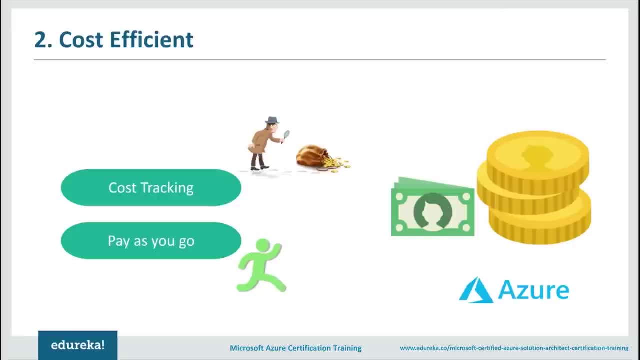 Cost efficiency. now, this is a very important point, because when you talk about money, people normally tend to look at businesses where they can save a lot of money and yet end up making a lot more money than what they've invested. Microsoft Azure ensures that you use a model called as pay-as-you-go. 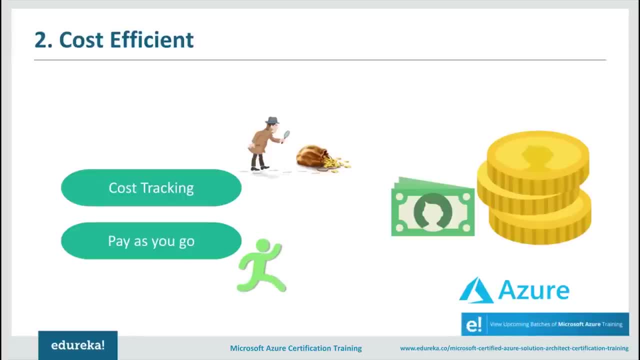 That means you would be paying only for those services that you use and only for the time duration You are using them. plus, you can also go ahead and keep track of all the costs and the money that you would be investing or you have already invested. 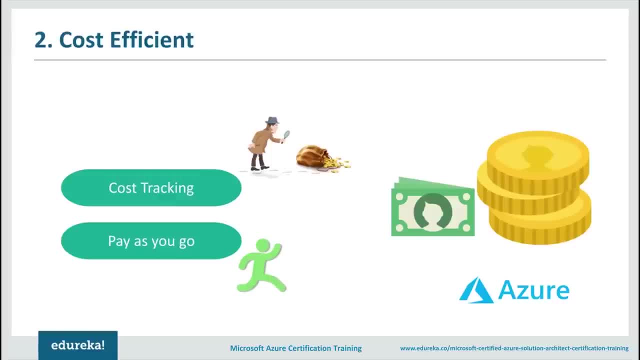 That means you have ready-to-use metrics which tell you as an if you use these services for this longer period of time, you would be charged this much, so you can keep a perfect track of how much money you would be Investing or you are using right now. 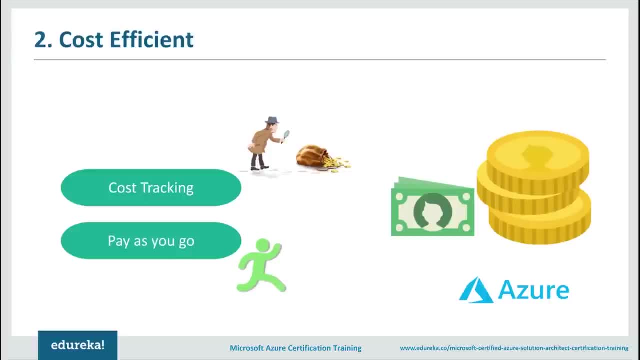 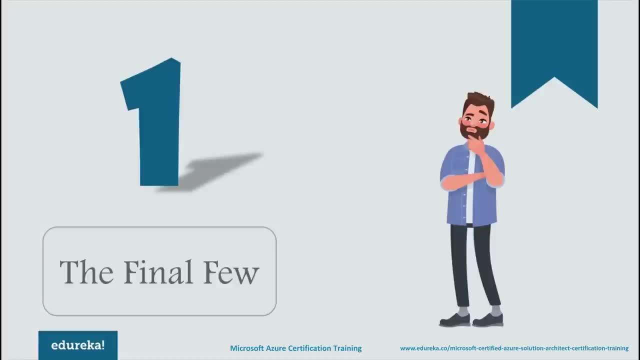 So if cost efficiency is something that is there in your mind, Microsoft Azure will definitely make sure that you pay very less money. The final few now. when I was jotting these points down, I realized that I had more than 10 points, So I just went ahead and jotted few points. 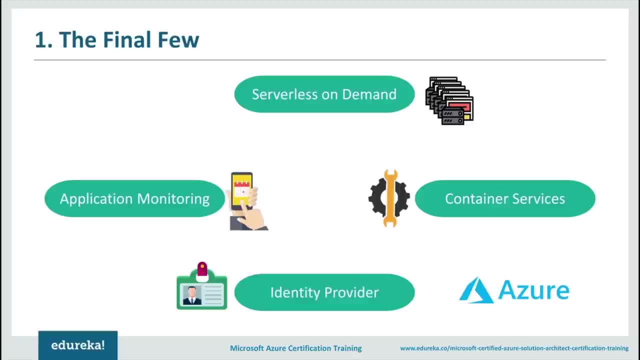 for my last point: serverless on-demand. I believe I just discussed this point. That means while you create your applications, you would not want to get into affairs where you have to deal with your servers or at least maintain or monitor them. What Microsoft Azure does is it maintains your servers. 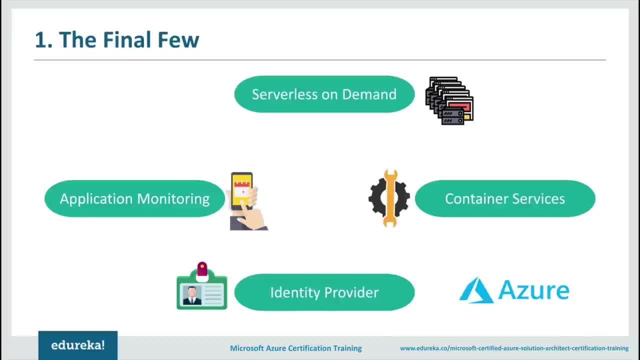 and softwares for you, So you can focus on your business problems and create applications independently. So it is truly serverless on-demand container services. Now, this is nothing but an approach. again, This lets you have containerization, or rather virtualization, at the operating system level. 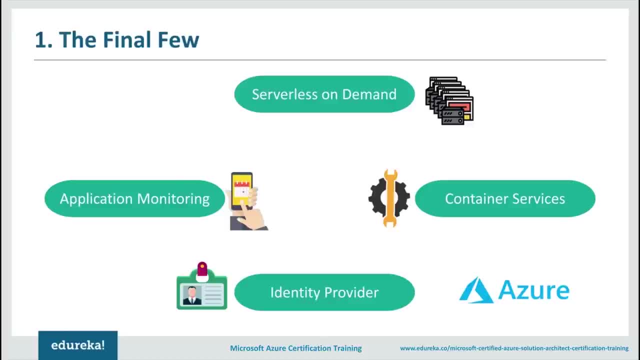 which ensures that you can go ahead and build your applications with much more ease. Now there is a containerization technique called as Kubernetes, and what Microsoft Azure does is it lets you use Kubernetes. That means you can simplify your process of building applications again. identity provider. 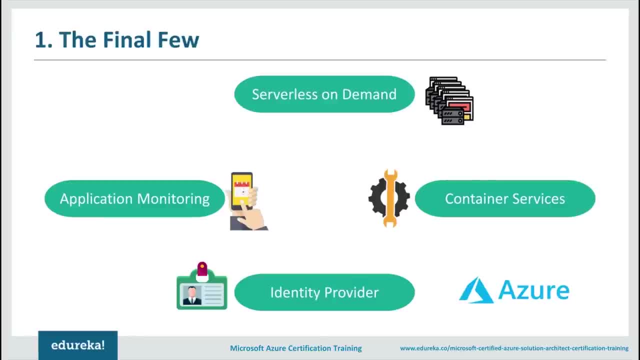 This is an important point as well. Now, when you're talking about a lot of applications, you will have to go ahead and sign in for every application identity provider. What it does is it lets you have a single sign, So you do not have to worry about going ahead. 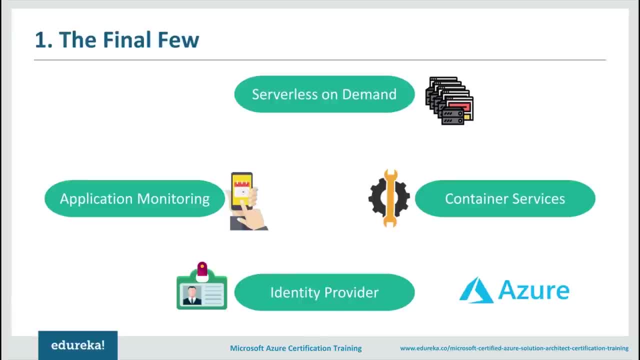 and signing in again and again. and this brings us to the last point, that is, application monitoring. since you are dealing with so many applications again, you want to be in a situation where you have all the metrics or all the data that is moving around and you would want to keep a track of all this data. 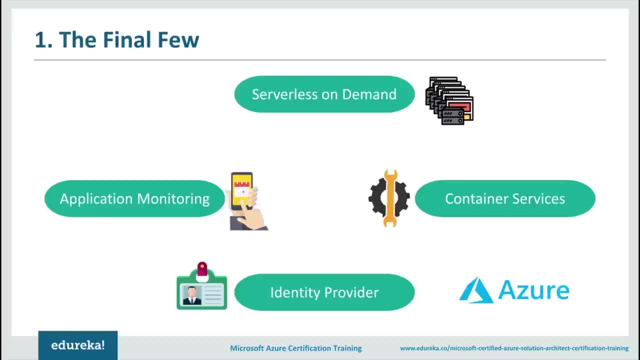 What application monitoring does is. it provides you with a feature called as insight management, which gives you a matrix at a single click and you can have all the information that you want to have. So these are some of the points I feel which are very important, and I feel that these were the top points. 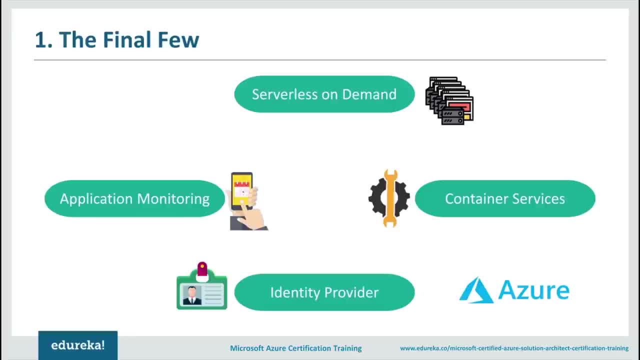 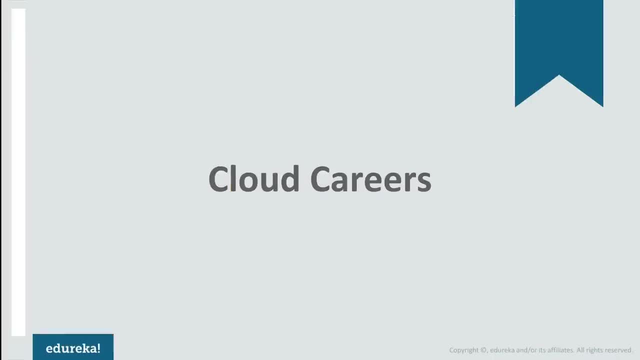 that I wanted to discuss with you people. If you people do have any different suggestions or you feel that there are certain other points which are more important than these, you can definitely share those points. in the comment section below We will talk about few Azure interview questions. 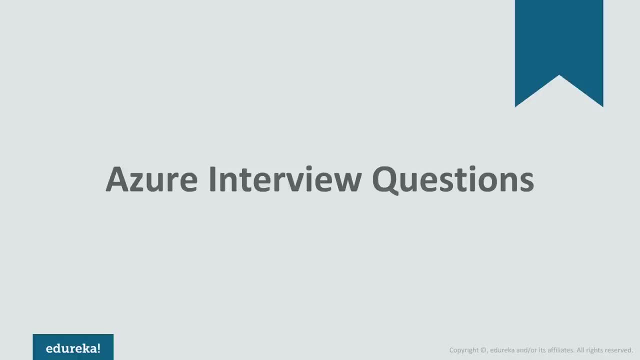 So, first of all, we need to understand what exactly Azure is and what's the reason behind us understanding and talking about these interview questions. So Azure is a pretty hot topic these days. It's a part of Microsoft Cloud- A lot of people who are listening to this particular webcast. 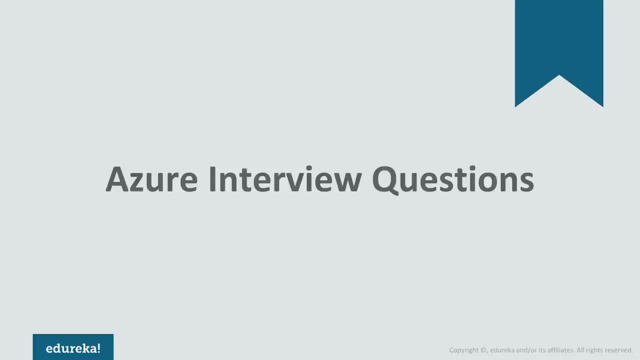 would have been heard of. I mean, might have heard of AWS- is there? then we talk about Google Cloud. is there? there's one from Microsoft which we are talking about. So there's a huge potential as far as cloud is concerned and the market is huge. 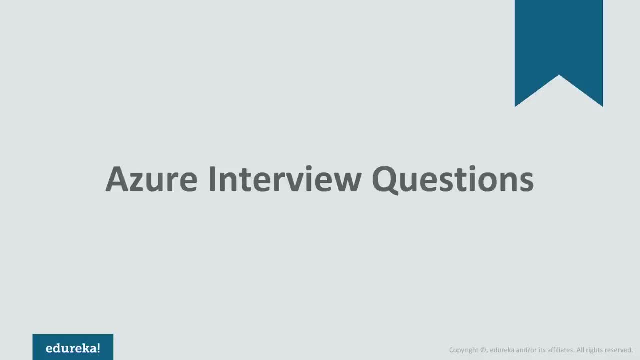 The market is hot these days and I will share a few of my experiences as far as the interview is concerned and the questions relevant to Azure. So if you talk about this particular interview session, I mean the question and answer session. I would say rather, or interview. 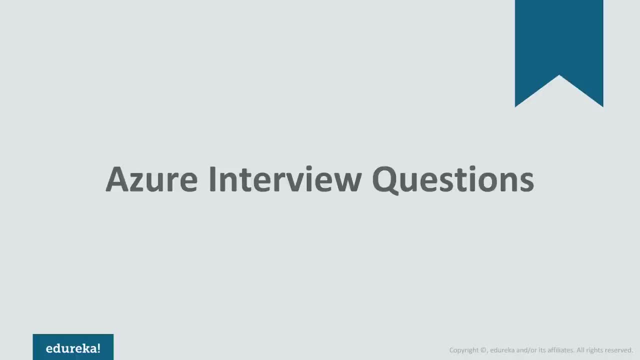 So this covers two major courses in Azure. One is 533 and one is 534.. So 533 is for admins and 534 is for architects. So when you talk about admins- the people who are responsible for managing and doing the run and maintain every day on Azure- 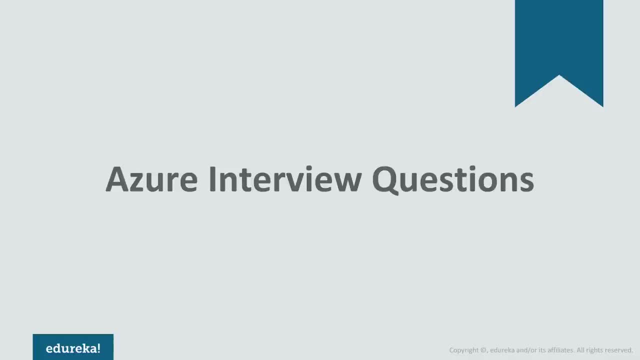 So the questions in this particular slide would focus on that and, at the same time, few things related to the architecting part, right? So there is another course, also from Microsoft itself, which is 532.. We will not focus much on 532. 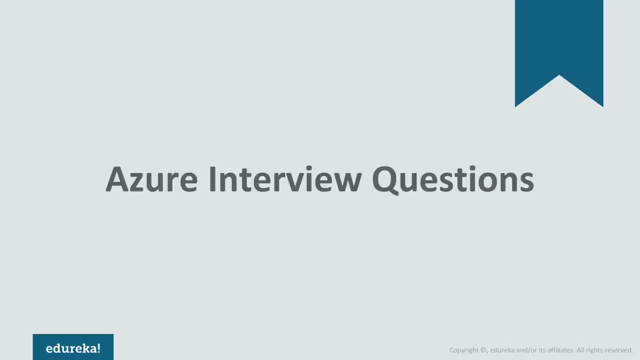 because that talks about, I would say, programming. So how do you use Azure- I would say services- in order to put your services, I would say your applications, on Azure? So that basically focuses on that. So we would not talk much in terms of that. 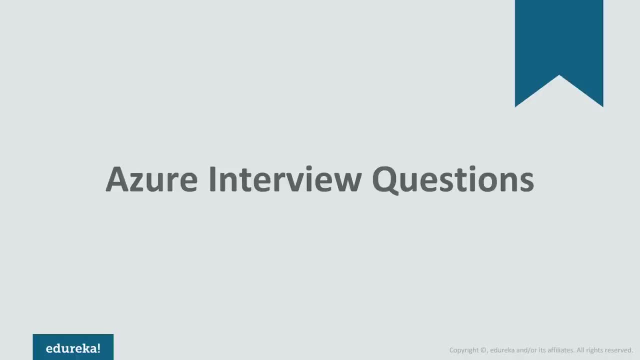 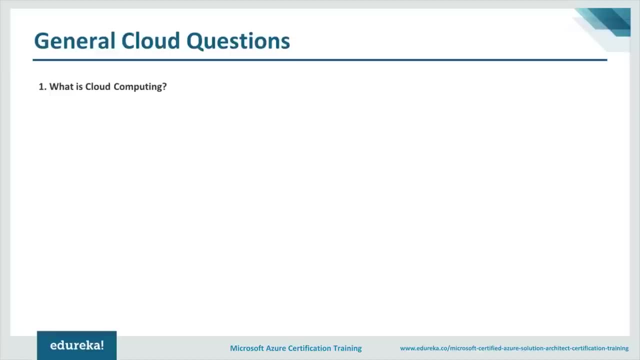 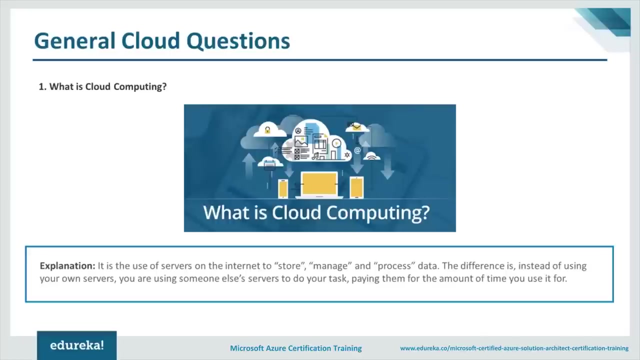 So this will again focus on 533 and 534.. So let's just start with the interview questions. So now, when you talk about cloud computing, a lot of different people have different definitions of cloud computing. So now cloud computing is something which is not very new technology, I would say. 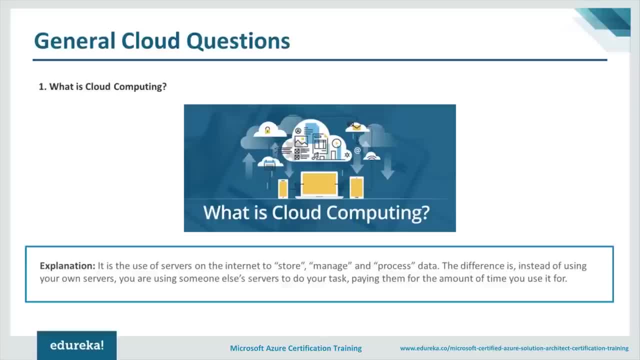 I mean, the technology is new, but the technology is not. The first product I would say which was talking about cloud was my Hotmail, which was designed and developed by Sabir Bhatia, So I'm sure a lot of people listening to this webinar. 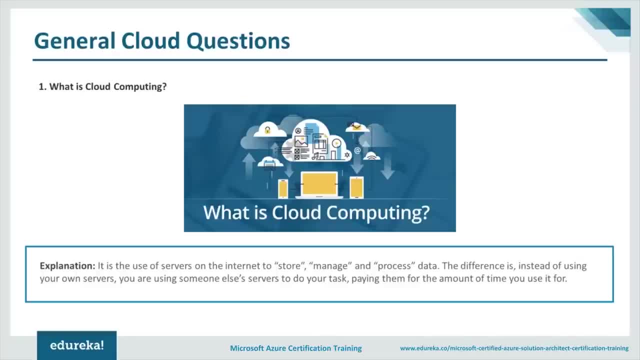 would be aware of that particular name. So what he did was he designed a mail server. So in that particular mail server I used to go in and access my mails, right, So that mail server was in the cloud, and then I was connecting to that mail server remotely. 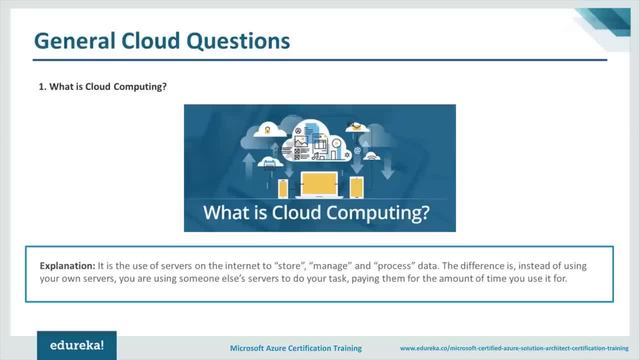 to access my mails. So that makes it a cloud product, Right. So now when you talk about cloud computing these days, the definition has changed, But as far as the working is concerned, it remains pretty much the same. So now when you talk about this, 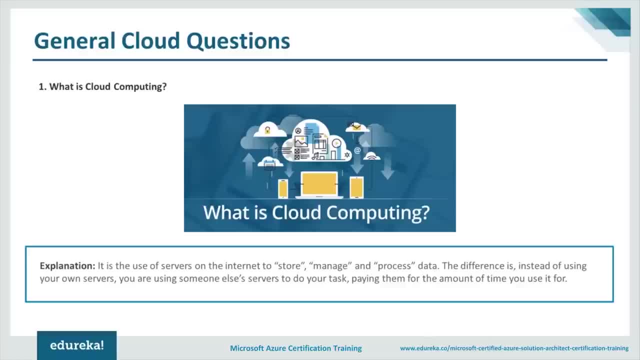 we talk about that. we use and pay right. So pay-per-use is the kind of model of what we talk about. So we basically use and then pay only for that amount of- I would not say data, but I would say- services which we use. 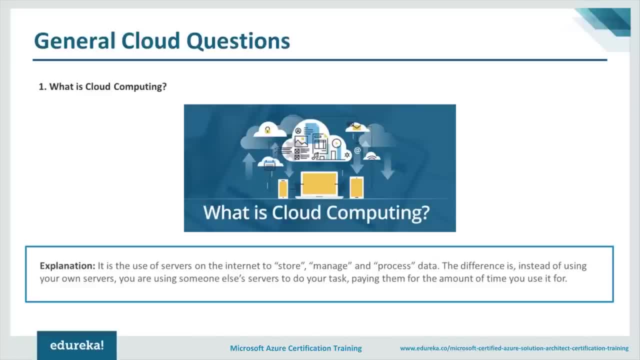 So there's an explanation down there in the slide. It talks about it is the use of servers on the internet to store, manage and process data. The difference is, instead of using your own servers, you're using somebody else's server to do the task. 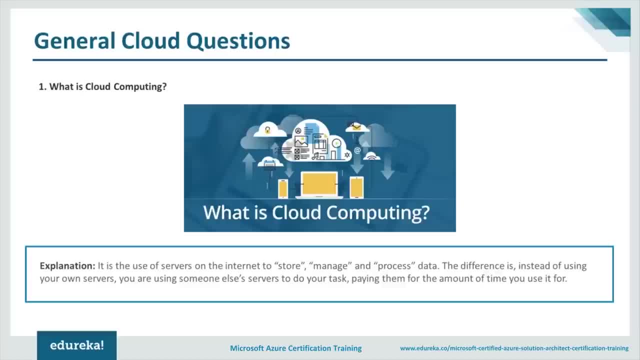 and pay them for the amount of time for which you use them, right? So this is what the idea is. So pay-per-use is the model which we focus on when we talk about cloud computing these days. right, So this is what cloud is. 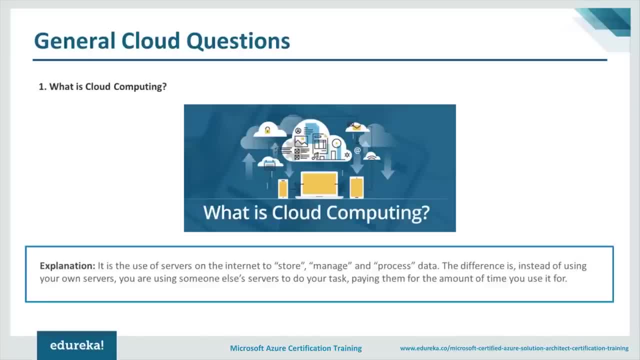 This is what a basic definition of cloud is. If you search the internet, you will have more than, I guess, 100, 100 plus definitions on cloud. Now, as far as definitions on cloud are concerned, it's up to you which one you would like to adapt. 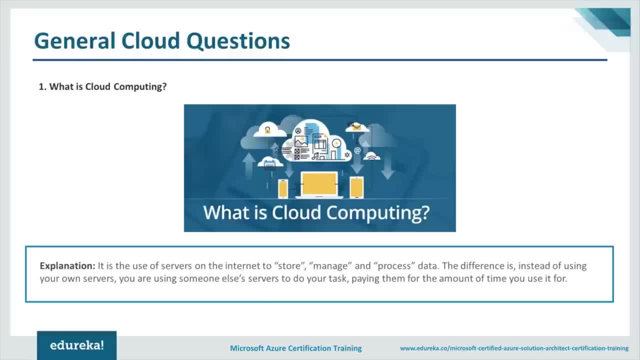 and which one you would like to go with. but then it works with a single model which is pay-per-use. So when you use, you pay, If you don't use, you don't pay, And end of day, you're using somebody else's resources. 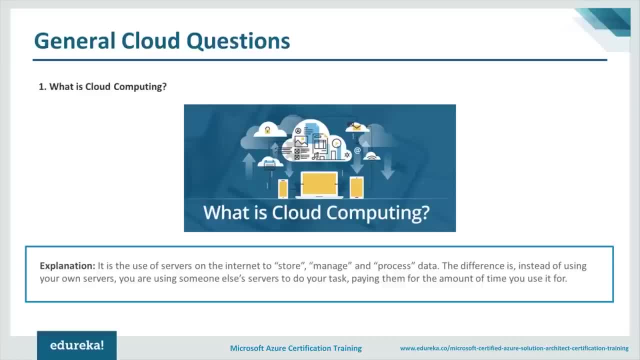 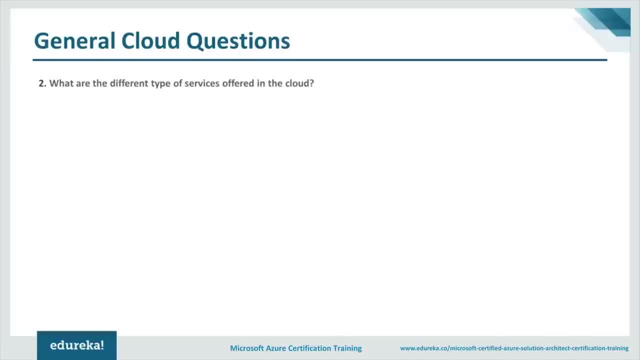 You're not using your own resources and you're only paying for their resources, what you use. Okay, now talking about different types of services, which we talk about as far as my cloud is concerned. so there are three major things: what we talk about. 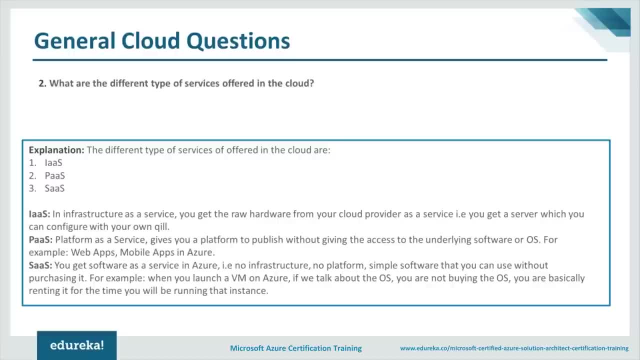 which is IaaS, PaaS and SaaS, And there are other things like somebody has talked about the AaaS database as a service, then you talk about SaaS. So that is for my mails, but then majorly we categorize these into three types. 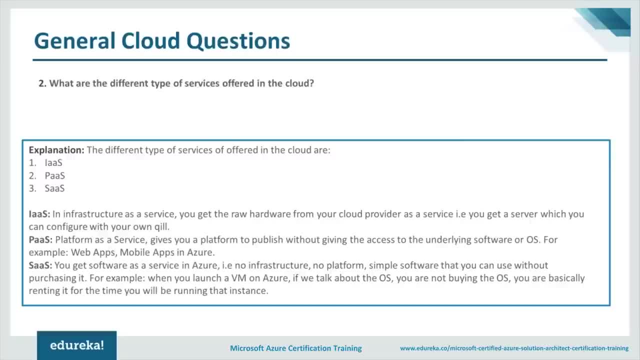 One is IaaS, PaaS and SaaS. So IaaS talks about infrastructure as a service and you get the hardware in that from the cloud provider as a service. So say, for example, you want to go ahead and deploy a machine, deploy a server. 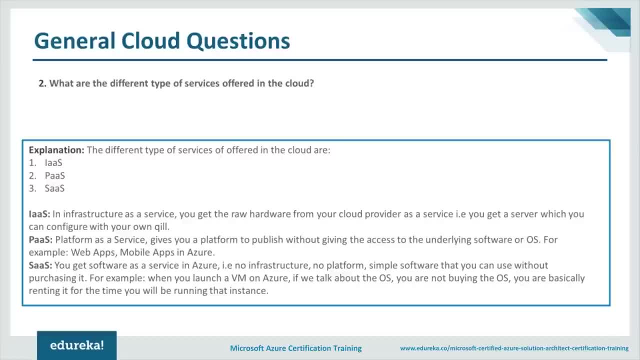 So basically, when you talk about that particular scenario, you are basically putting a server in IaaS, which is my infrastructure as a service, So you get complete control on a virtual machine which is there in the cloud, hosted by Microsoft, Google or AWS, and then you can just go ahead. 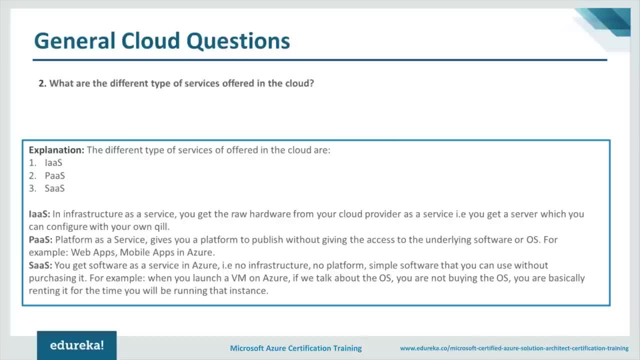 and put in your resources onto that particular machine. So this is how it works, right, Simple enough. Then you talk about PaaS platform as a service. So in this you don't get access to your machine, or in other words, 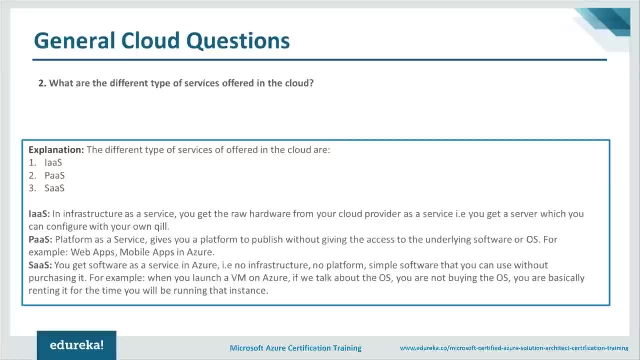 you can say you don't get access to the underlying layer, but you get complete access to the resources or the services right? So it's more like my platform on which you publish your applications or you put your application. There are a few examples. 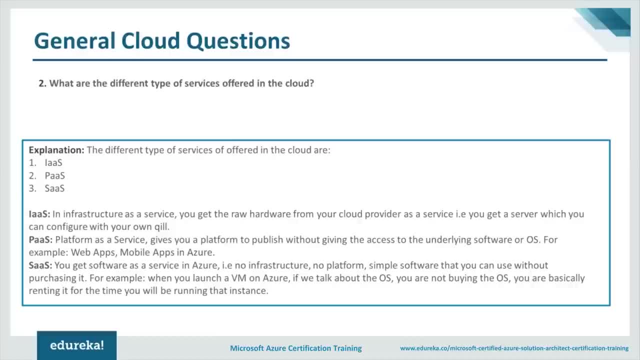 So I talk about my web apps, my mobile apps, which are in Azure. Then you talk about the last type of service offered in cloud. So this is my SaaS. So when you talk about SaaS, you get software as a service in Azure. 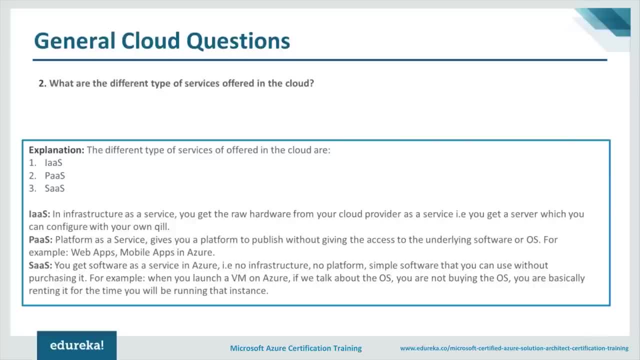 So you don't need to worry about infrastructure, You don't need to worry about platform. So you basically are getting the end product which may be running on the infrastructure which may be running on the platform. So, for example, when you launch a VM on Azure. 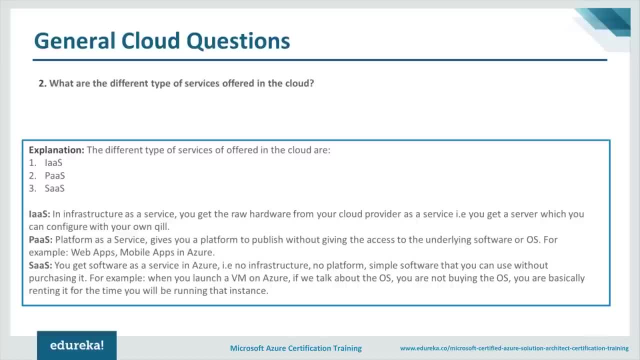 if you talk about OS, you're not buying the OS, And if you talk about PaaS, you're not buying the service. So you're just basically paying for the software which is running on either IaaS or either PaaS. So this is what we get. 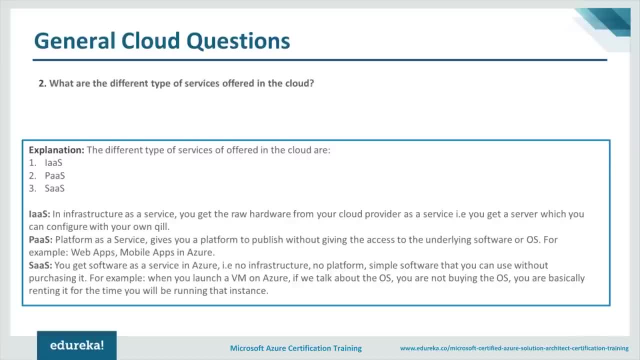 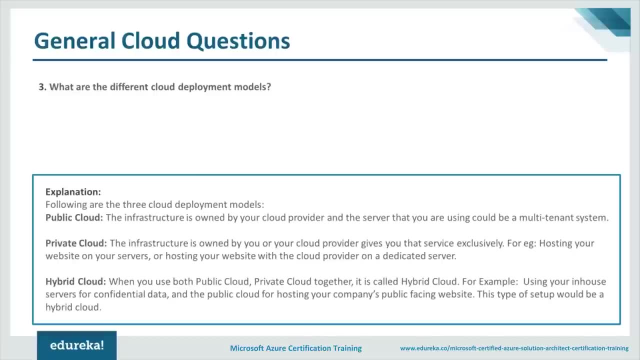 as far as my types of cloud is concerned. Now let's just jump on to another question. Now, what are the different cloud deployment models? So explanation talks about three models which we have. One is my public cloud, one is my private cloud. 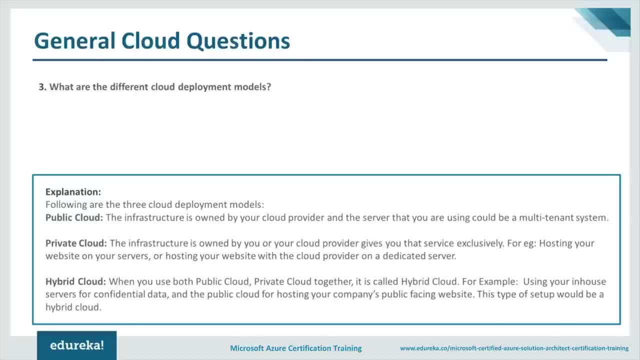 and one is my hybrid cloud. So let's just take this with examples. So I am a general user, I am a home user, I want to go ahead and put a website, So I decide that my website will be hosted on my cloud, right? 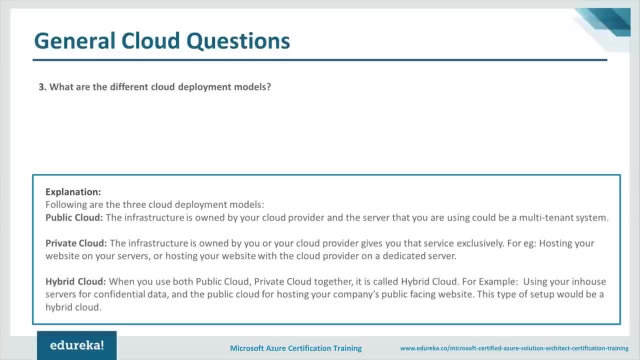 So I want to go ahead and deploy a VM on the cloud and I want to put my website over there. So I go to Microsoft website, Azure website, I sign up there and then I- maybe you can say- provision a machine. 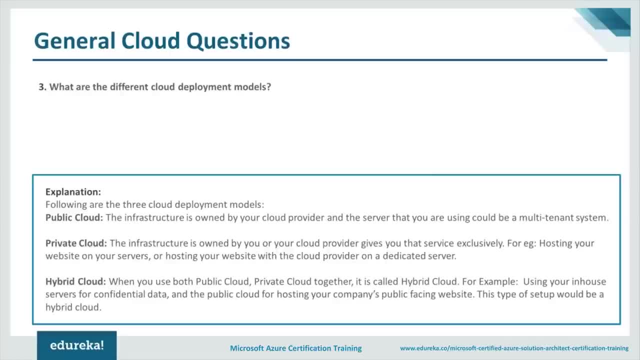 Once I provision a machine, I put IaaS on top of it. Once I put IaaS on top of it, I will just go ahead and move my resources. When I say move my resources, move my application on the cloud. So what I'm trying to say is a general, basic end user. 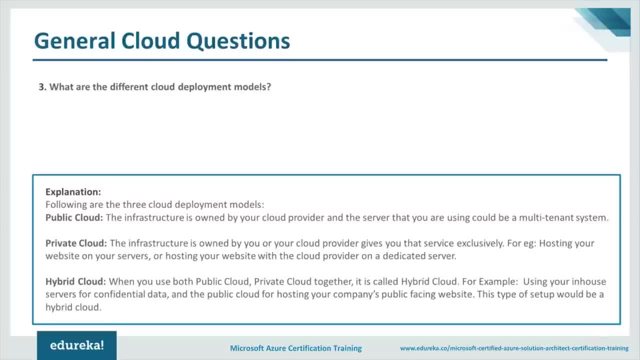 who is sitting at home can log into the cloud, get a machine and then use the machine, right? This is what my public cloud is, So it's available for the public, right? Then you talk about the private cloud. Now, as far as private cloud is concerned, 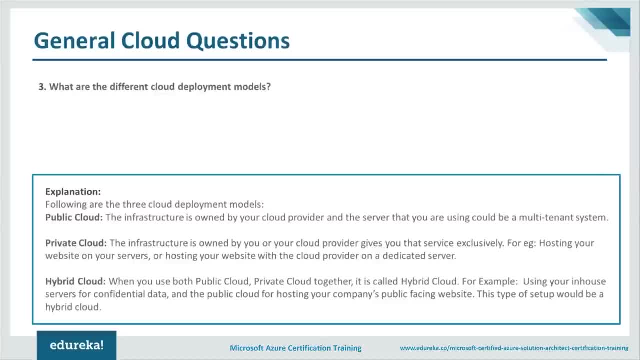 it's owned by the enterprise, okay, And only enterprise people will have access to it. So organizations like Accenture or maybe Wipro or maybe Capgemini, Cognizant, So all these people own a private cloud, right. 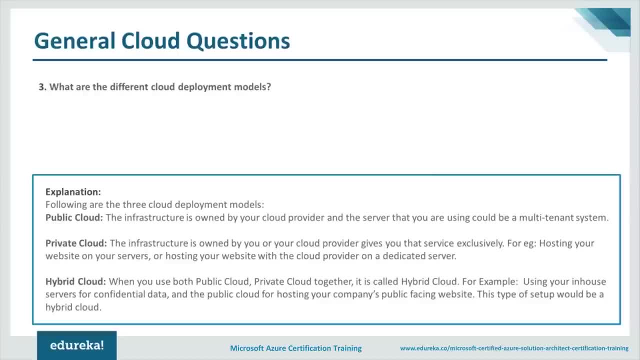 So the idea is that the resources are owned by them and hence their people are the ones who will go ahead and access that, And then, at times, what happens is they give access to their private cloud for their customers also. Now you might have a question. 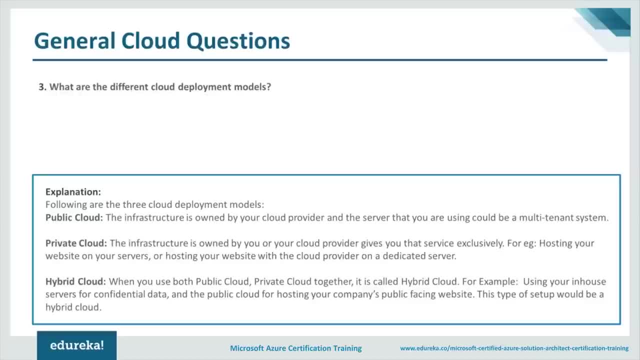 that. why do I build a private cloud? Because, end of day, I'm spending a lot of money on infrastructure. I'm spending a lot of money on air conditioning, electricity and I'm spending a lot of money on licensing also, So why can't I just go ahead and work on public cloud? 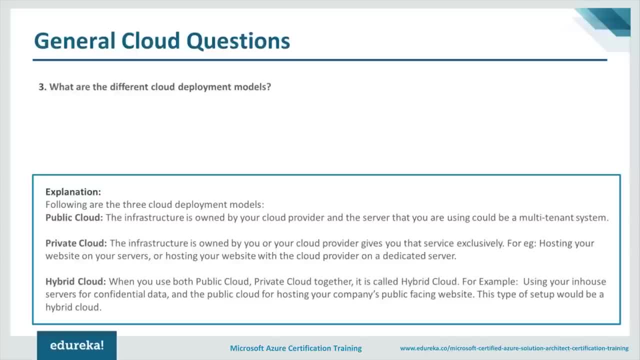 Why do I need to go ahead and implement a private cloud? Now, basically, when you talk about a private cloud, private cloud is built for automation. That is one of the most important things, And the second important part when we talk about is that, when you talk about private cloud, 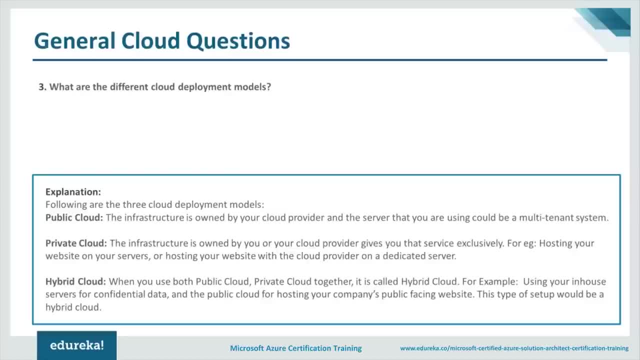 it gives me more control over the resources, Whereas when you talk about public cloud, I do not have control over the resources because everything is owned by the vendor. right Now talking about hybrid clouds, so I'll give you an example for this also. 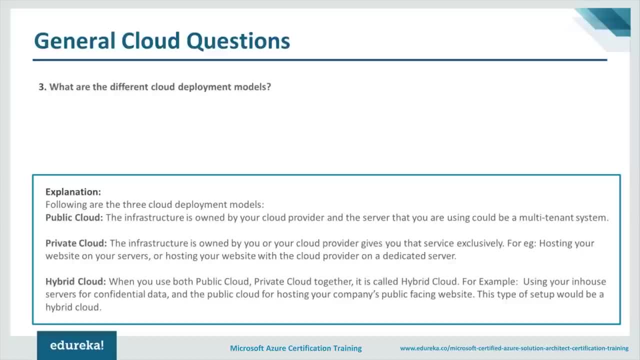 I go to Amazon and Amazon is my public cloud provider And I tell them that I need a private cloud. so would it be possible for you to host a private cloud for me? Amazon says yes, and they dedicate a list of resources for me, only for me, only for my organization. 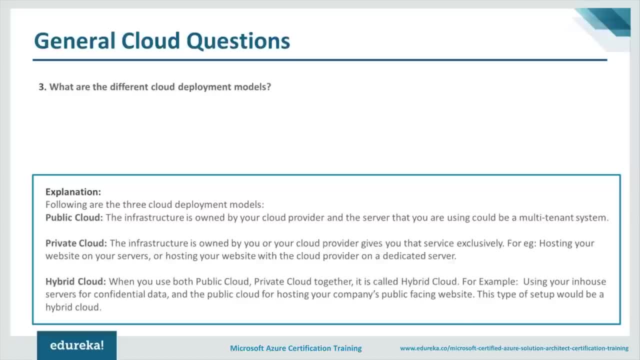 So now, when you talk about Amazon, Amazon is hosting a public cloud, but then they also are capable enough of hosting a private cloud for my organization, So that makes it a hybrid cloud. So this is what hybrid cloud means. So these are three different ways. 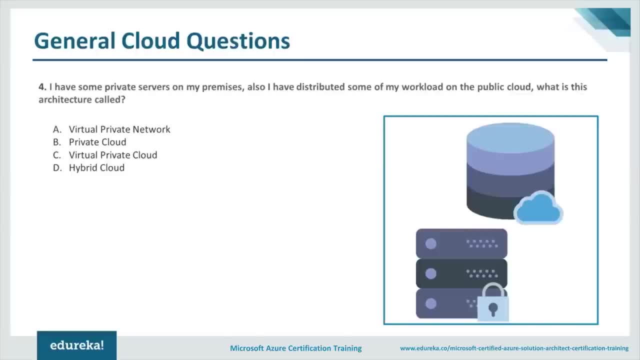 of how I categorize these cloud models. Now a few other questions. Now. the question says I have some private servers on my premises. Also, I have distributed some of my workloads on the public cloud. What is the architecture called When you talk about this kind of scenario? 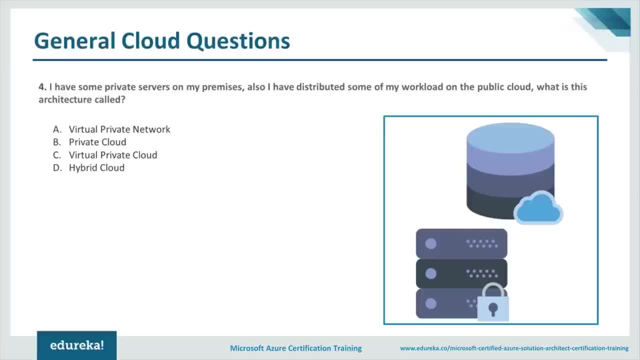 so we talk about my virtual private network. So these are my options, basically: virtual private network, Then we talk about private cloud, Then we talk about my virtual private cloud, And then you have hybrid cloud. okay Again, so just read the question carefully. 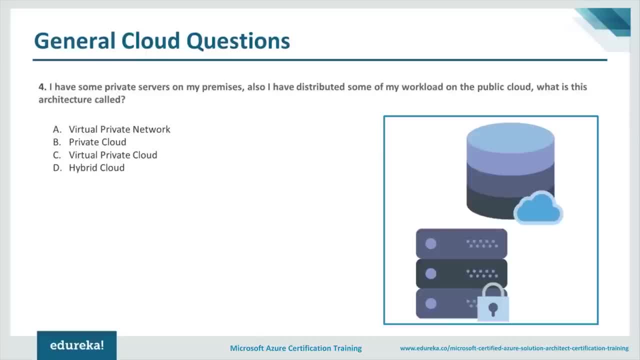 and then probably I'll just jump onto the next slide and we will talk about the answer and the explanation. So again, I would say I have some private servers on my premises. Also, I have distributed some of my workloads on the public cloud. 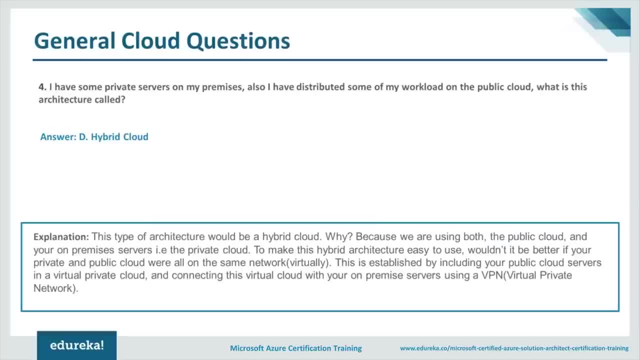 What is this architecture called? okay, So now it says hybrid cloud. So when you talk about this, this type of architecture would be on a hybrid cloud. Why? Because we use both public cloud and the on-premise server, which is on the private cloud. 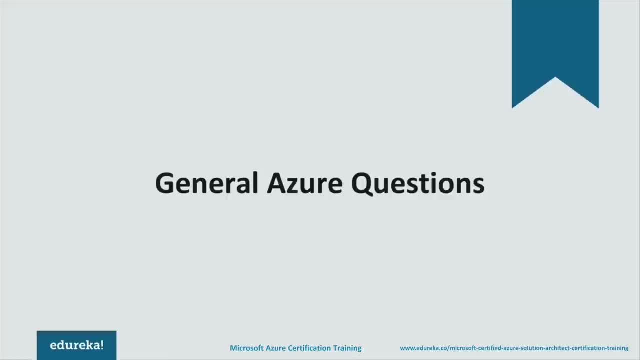 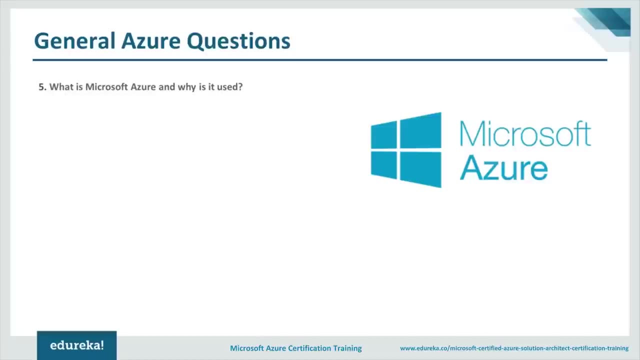 Now let's just jump onto the next question. So we have a few general Azure questions. Now these are Azure specific. The questions which we didn't talk about previously were just general cloud questions, right? So if you are giving an interview for maybe Azure, 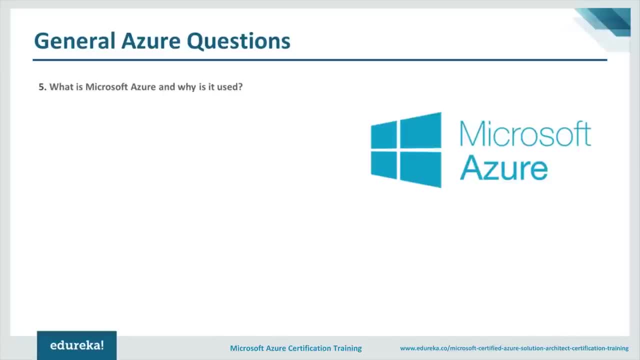 maybe AWS or maybe Google. so those four questions are something which you, I would say, go with any of these scenarios, any of the interviews which you would do. okay, Now, these are specific, general Azure questions. So when I say specific general Azure questions, 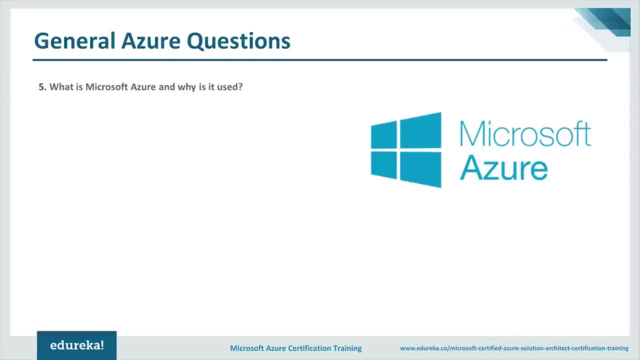 so we talk about only Azure in here, okay, So the first question talks about what is Microsoft Azure and why is it used? okay, So, as I initially said, that Azure is my public cloud from Microsoft, So let's just see how it works. 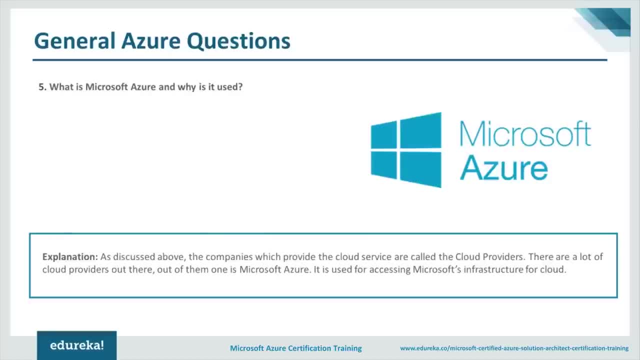 So we have our definition on the next slide. okay, So, as discussed above, the companies which provide cloud services are called cloud providers And of course, I did explain you this in the previous slide, I mean the first slide which we talked about. 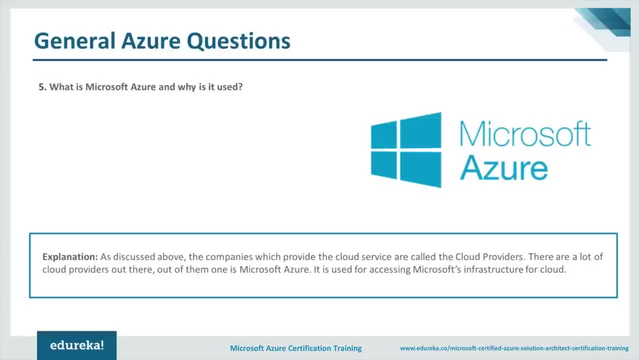 So I explained to you about Google- so that is a cloud provider. I explained to you about AWS- that is a cloud provider. And then I talked about Azure, which is a cloud provider. So now Azure is from Microsoft And the idea behind this is: 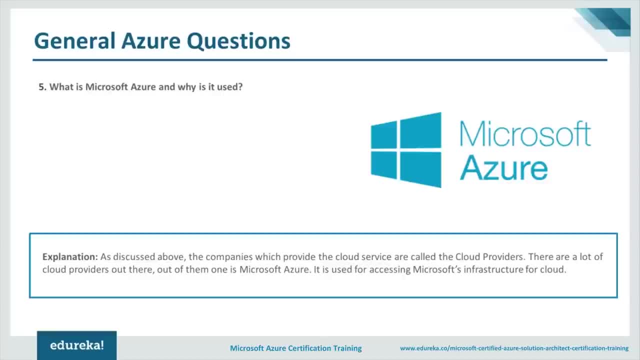 it's more like my public cloud. so you can go to Azure, you can log on to Azure, create a machine and then start working with that. So this is one of the cloud providers. So Microsoft is one of the cloud providers. 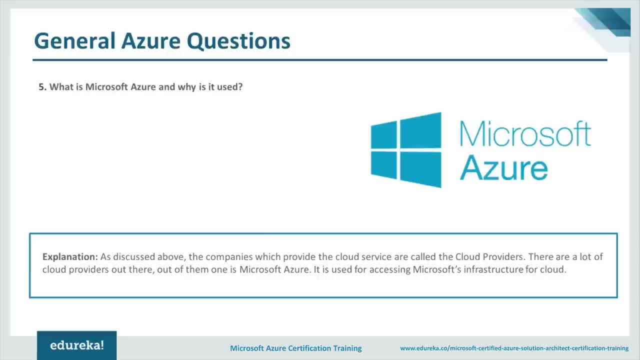 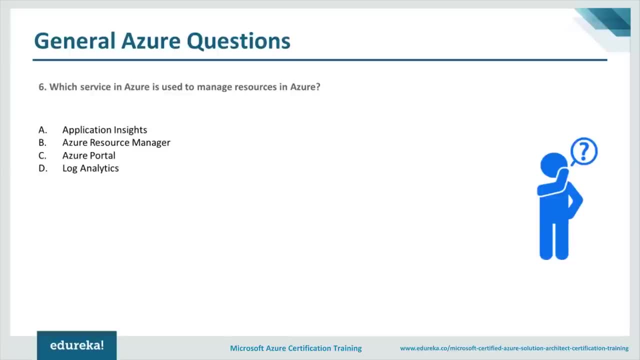 one of the major cloud providers these days, right? So this is what my Azure is Now talking about. which services in Azure is used to manage resources in Azure. So we have few options. I have my application insight. I have my ARM. 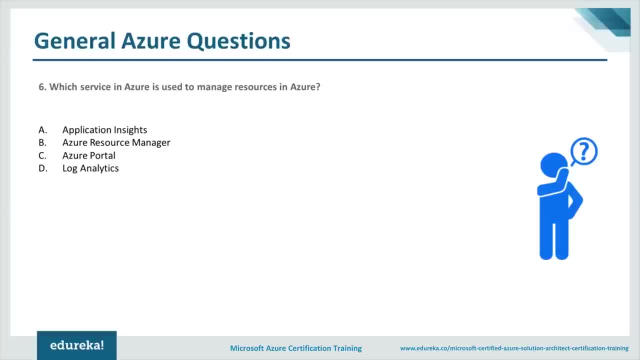 which is my Azure resource manager, Then you have my Azure portal, Then you have my log analytics, okay, So, as far as this is concerned, so we talk about my ARM, So this is a service which is basically on the newer portal, right? 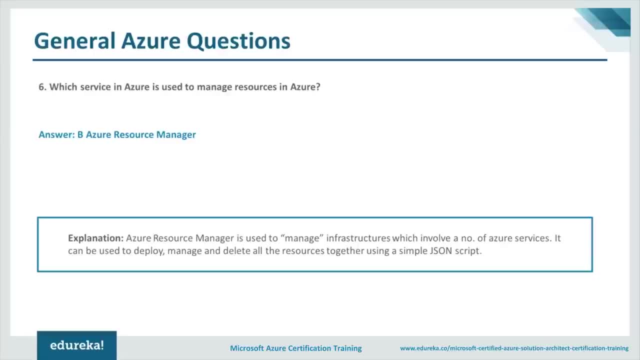 So now, when you talk about these services, which is on the newer portal, so it is used to manage the infrastructure which involves a number of Azure services, It's basically my fabric, So I'm not sure how many people are aware of what is an Azure fabric. 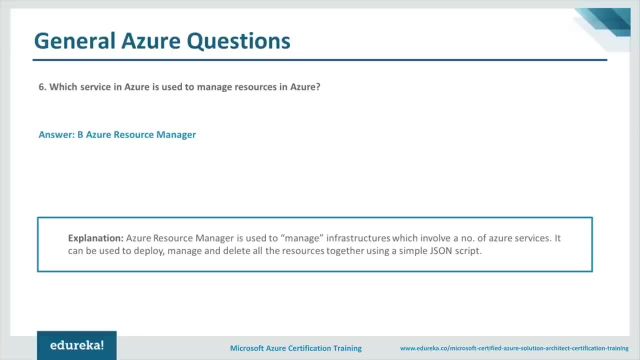 but then the idea behind this is that when you talk about my Azure fabric, Azure fabric now runs on something called ARM. Previously, in version one of Azure, it was using the service management model, So now this is a new thing, right? So when you talk about managing the resources in Azure, 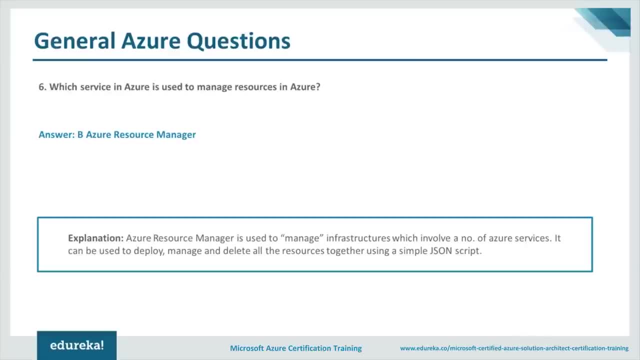 so we basically talk about my resource manager model and then how our services run on it, how they work and how they interact with each other. There are a lot of things which you need to work on and which you need to learn. as far as my ARM is, 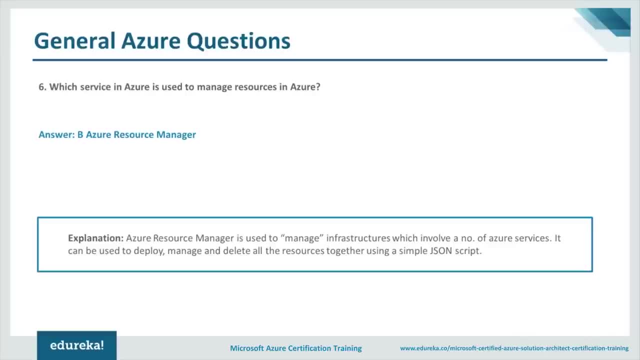 But for the time being, you just need to remember that we talk about my Azure resource manager, So this is something which runs everything and takes care of a lot of different things as far as my Azure is concerned. So when ARM came, a lot of different came. 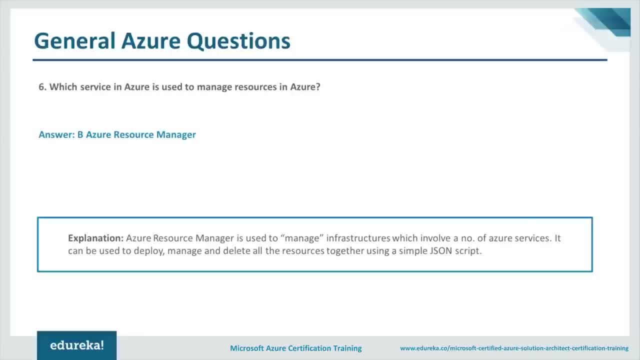 A lot of different things started coming in, So tag was one of them. Resource groups was another one. If you are familiar with resource group, great. If you're familiar with tags, great, If you're not just go to Google and search for it. 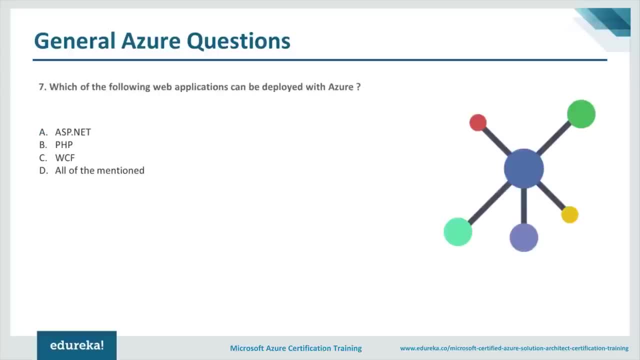 and you'll find your answers. Then we have a few questions. Which of the following web applications can be deployed with Azure? So we can, of course, put ASPNET applications in Azure. Now you might have a question Where exactly I can use these applications. 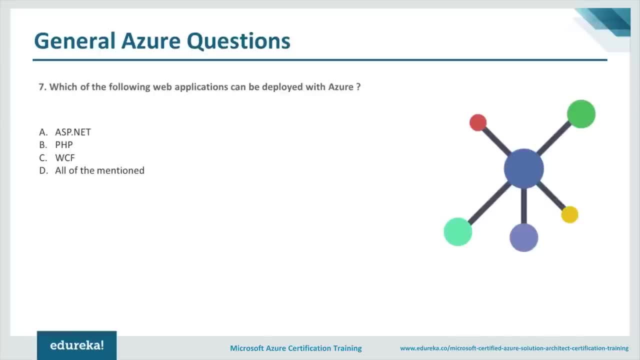 or where exactly I can deploy the applications. So, to answer that, you can deploy it either in IaaS or you can deploy it either in PE, So you can, of course, deploy ASPNET, You can deploy PHP, You can deploy WCF. 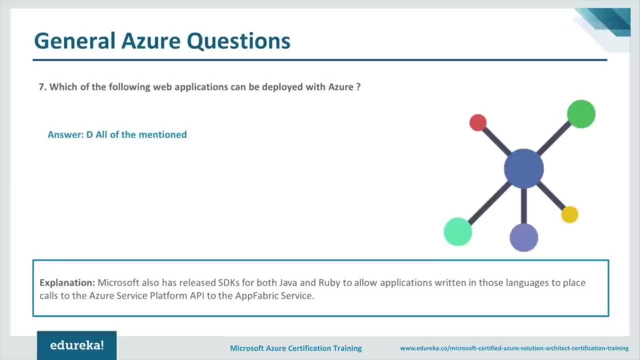 So the answer is all of the above, But then it's very important for you to understand that if there is an application which is on Java, so that may have few problems when you deploy it on Azure, Because of course, Azure is majorly designed. 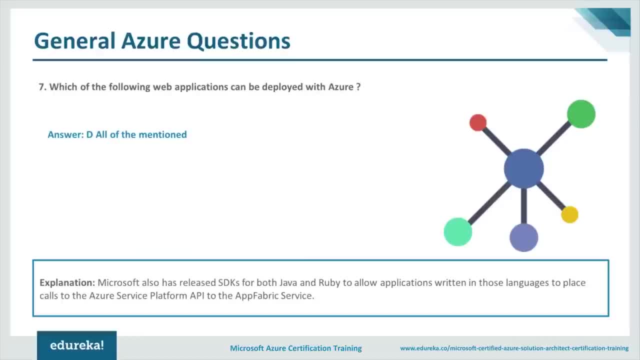 for Microsoft services. When you talk about these Microsoft services, Java is not a Microsoft product, So it's more like it's not that friendly when you compare it with other services which we are running in the cloud, Specific to Microsoft cloud, of course, I would say 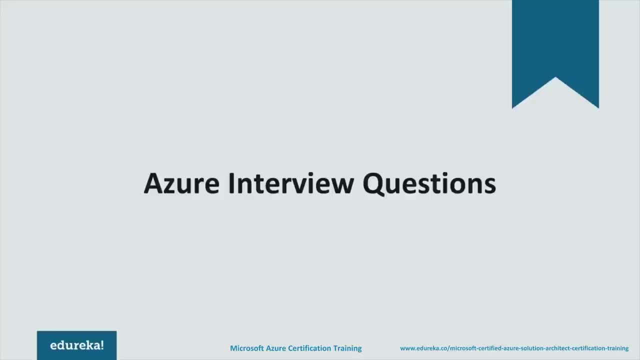 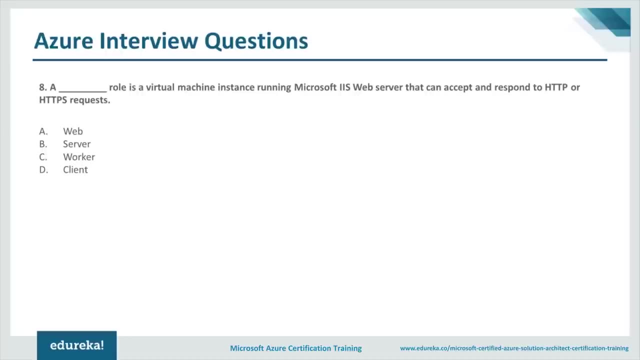 Okay, jumping on to the next one, Then a few other questions, So these are my fill in the blanks. A Dash role is a virtual machine instance running Microsoft IaaS web services that can accept and respond to HTTP or HTTP request. Okay, 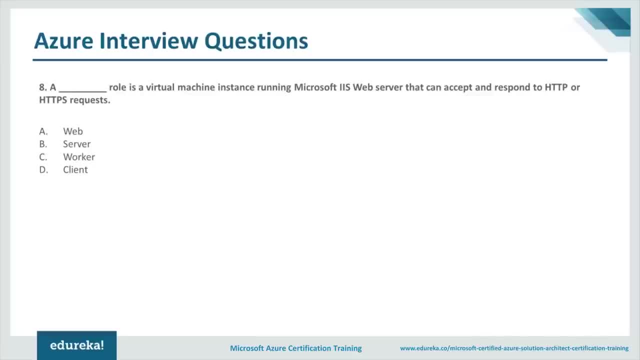 So we have four options in here: One is my web, One is my server, One is my worker And one is my client. Okay, Now, when you talk about this, the answer to that is: web. role is something which is basically hosted on a virtual machine. 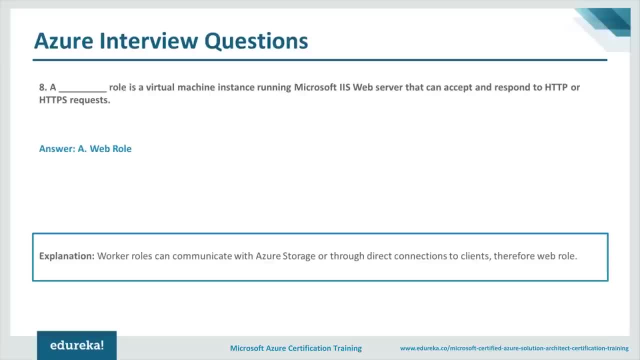 and is running on Microsoft IaaS web server and that is capable of accepting HTTP and HTTPS request. So basically, on the web role, what you do is you can upload your website and your website runs on top of it, And then, of course, you know that my website works on HTTP and HTTPS. 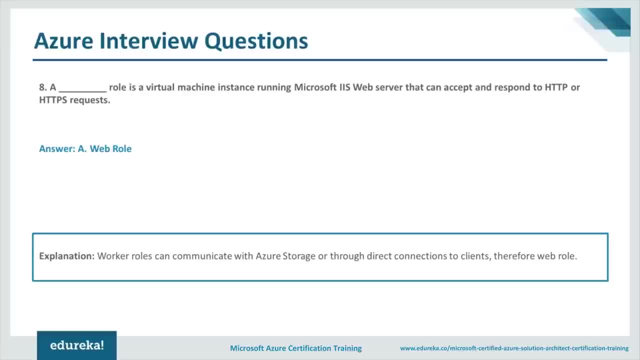 So hence, my web role is the one which is capable enough of running that particular maybe application or software or web services. Okay, The other question what we talk about is what is the use of roles in Microsoft Azure? So when you talk about what is the use of roles, 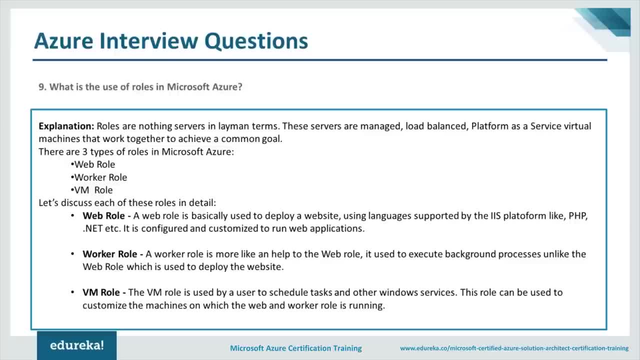 we talk about three roles: One is my web role, One is my worker role And one is my VM role. Okay, So now, when you talk about my web role- web role basically is for hosting and deploying my websites. Okay, The worker role is the one which basically helps. 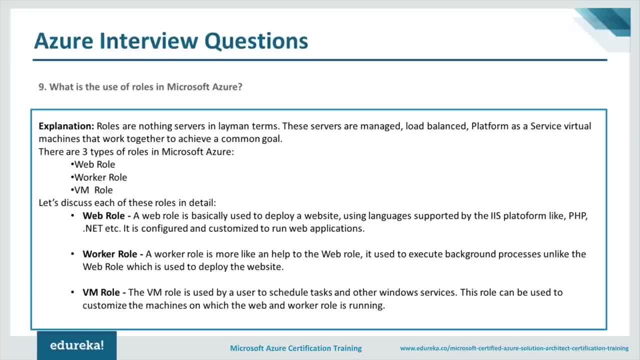 the web role to execute the background processes. The example I can give you is my web jobs. I'm not sure how many people are aware of web jobs, but if you want, you can again search on the internet. So my web role is residing on worker role. 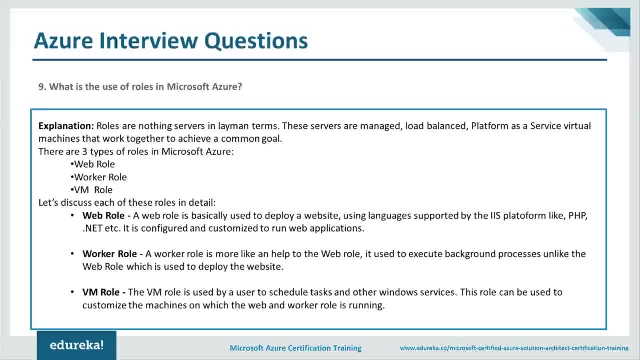 Worker role is the one which supports my web role, And the worker role is the one which actually resides on my VM role. Okay, So this is the one which talks to the underlying layer. It's more like a framework. It acts as a framework. 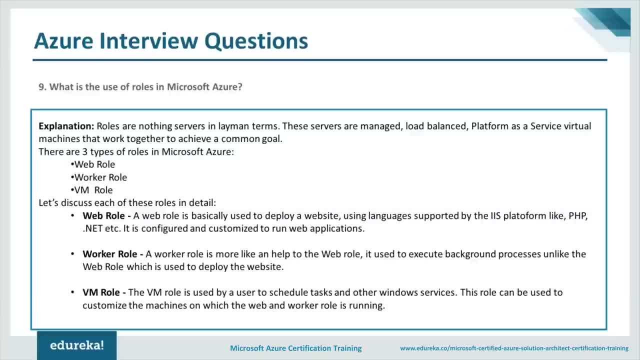 So that means on the operating system I have my worker role, On top of it I have my web role. So my web role is the one which will host my services- I would not say services, but the applications, rather. Okay. 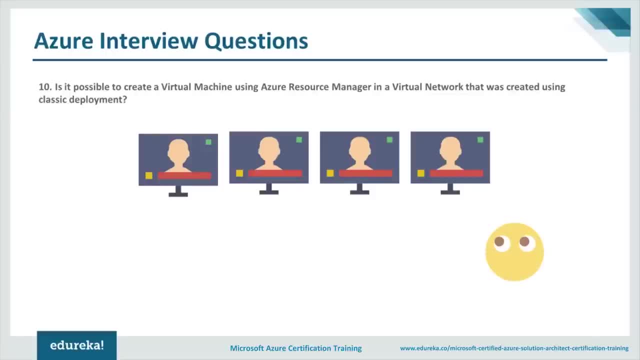 So, jumping on to the next one. Now the question says: is it possible to create virtual machines using ARM in a virtual network that was created using classic deployment? And of course I don't think so. it's possible. So let's just see. 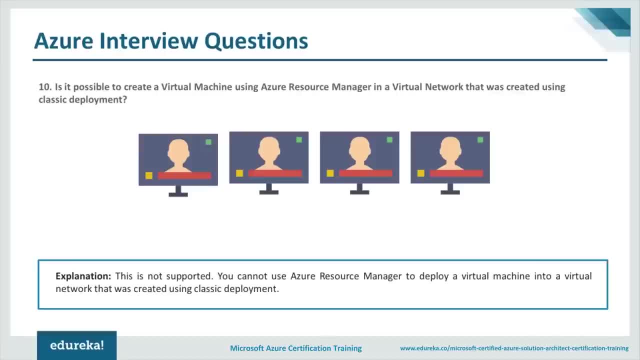 This is not supported, as I said, because ARM is something different And previously the classic portal was using a different model of deployment, So it used my classic model of deployment, which was basically for service management. And, if you see, if you're aware of the two portals, 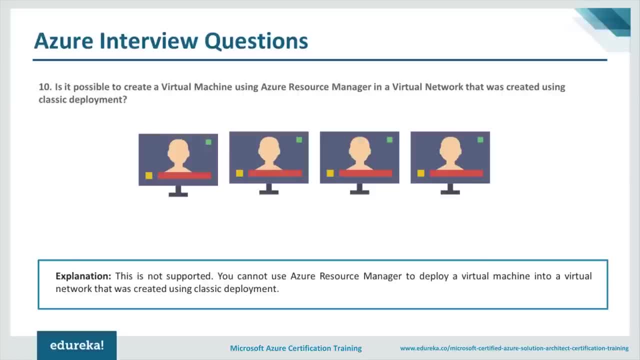 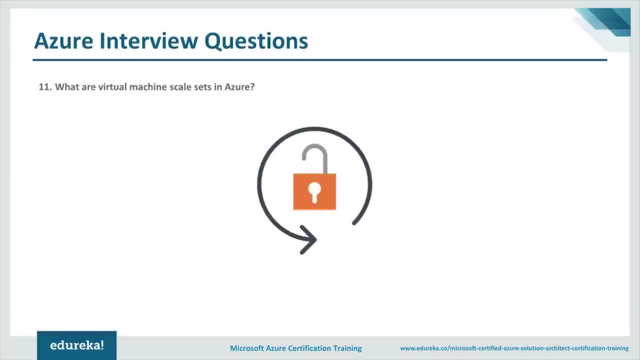 you'll see, there's a huge difference in how classic portal was and how the new portal is, So there's a huge difference in terms of that also. So it's not possible. Jumping on to the next question: What are virtual machine skill sets? 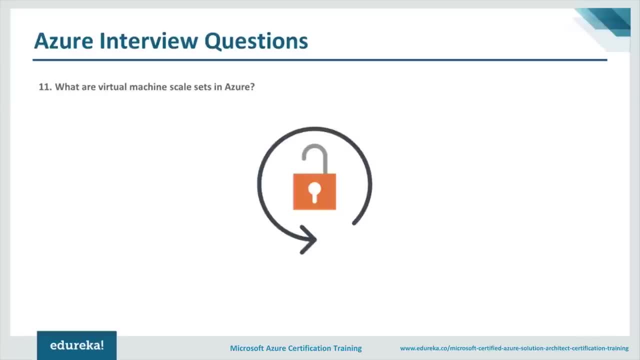 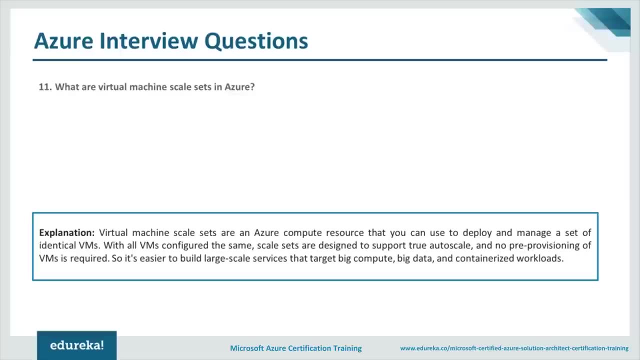 So, scaling up, scaling down. So, if you're not aware, if I have more number of requests coming in, my virtual machines have the capacity and capability to scale up and scale down based upon schedule and performance. Okay, So in other words, 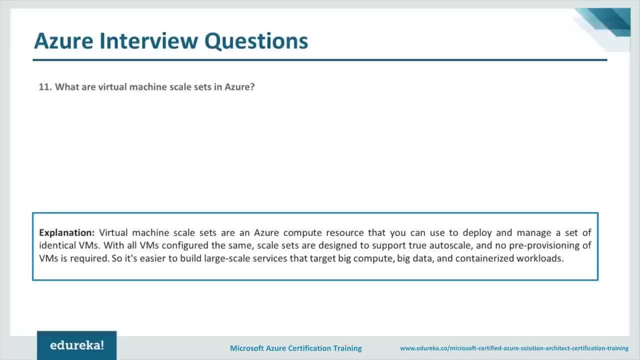 what I can say is if my CPU is spiking to 100% or not 100%, I would cap it to 90.. So if my CPU is spiking to 90 and my requests are still coming in for accessing that portal, the web portal, maybe you can say. 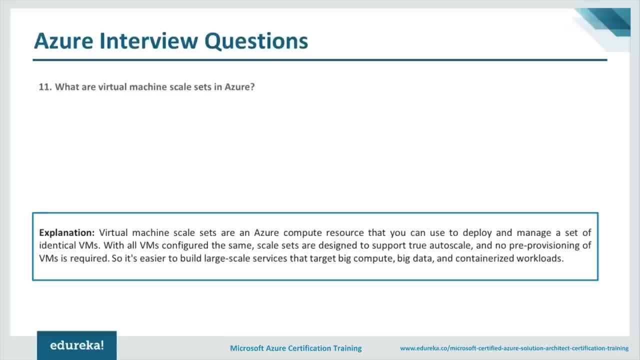 which is running on this particular machine. So my skill set is intelligent enough to scale one more instance and then load balance the traffic between the two instances which are now deployed running the same set of application. Okay, So this is what my skill set does. 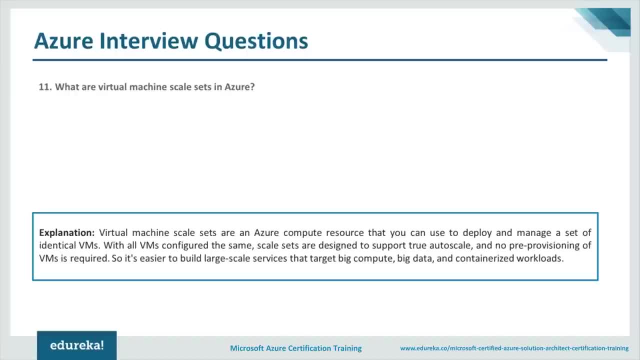 It automatically auto scales, I would say rather the workloads right, Based upon the performance and the schedule. Now how this schedule thing works. So say, for example, if starting from morning nine to evening nine, you have more number of visitors on the website. 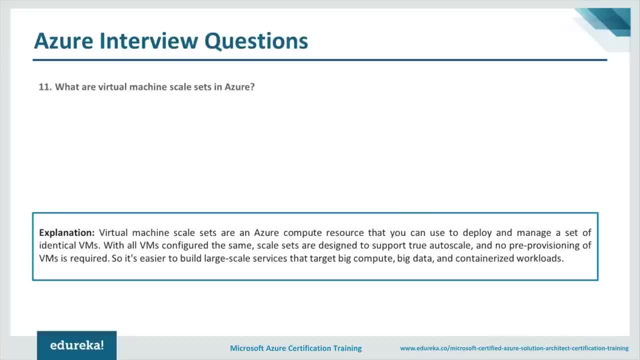 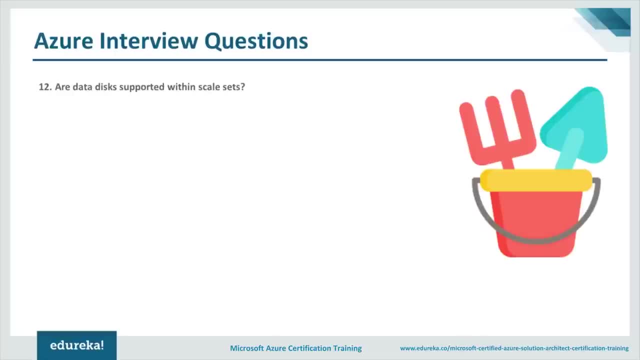 so you can scale more number of instances for your website, And after 9 pm at night, you can minimize the number of instances. right? So this is how my skill set works. Okay, Jumping on to next question. Are data disks supported within skill set? 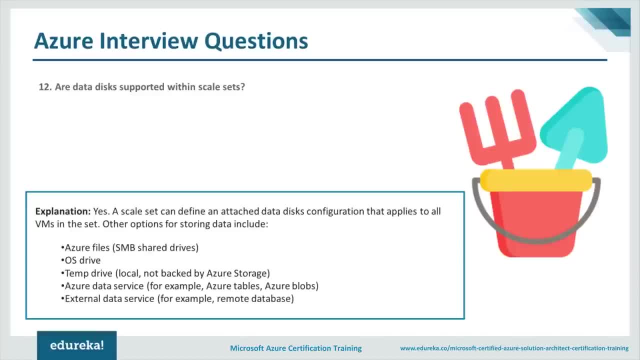 So now, first of all, when you talk about this, yes, of course, my data disks are supported in skill set. Okay, So when you talk about this, a skill set can be defined as attached data disk configuration that applies to all VMs in the set. 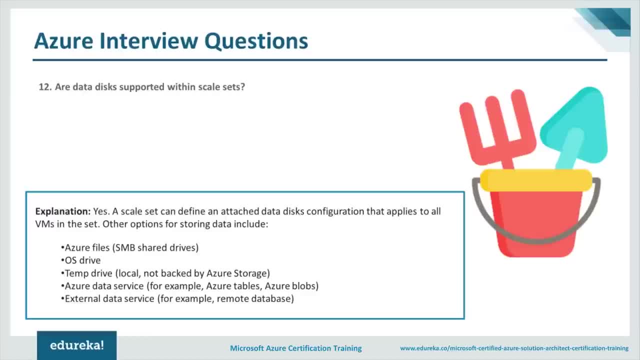 So there are a few types of data disk examples which I've given over there. So one is of course my Azure files, which is my SMB shared disk, And then you have my OS drives, Then you have my dev drives, Then you have my Azure data services. 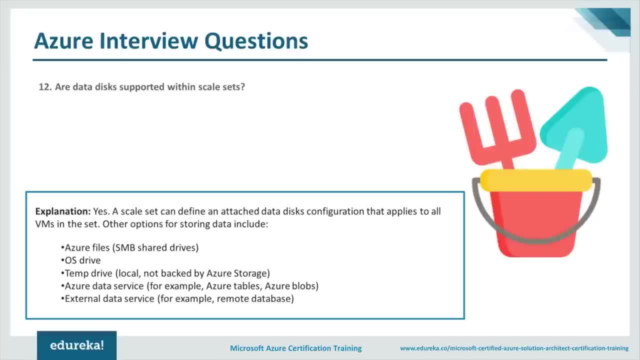 like the blogs are there and tables are there and cubes are there, And then you have my external data services, such as remote databases. So all of these are supported. All of the disks are supported which you see over there Talking about availability set. 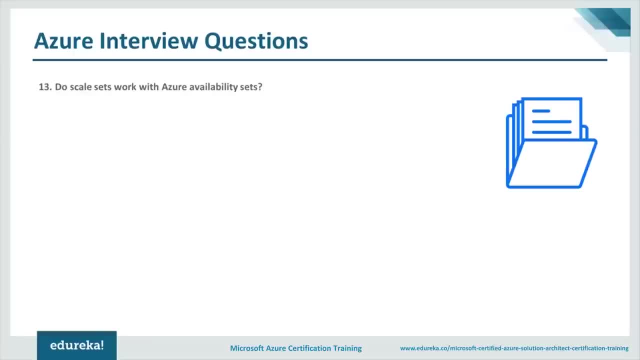 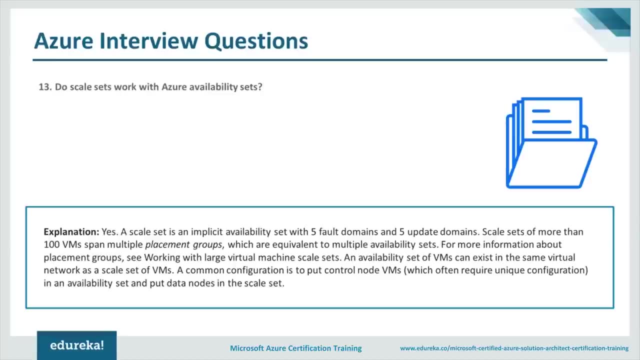 so do skill sets work with Azure availability set? Now, first of all, you need to understand what is an availability set. Availability set is basically grouping of servers so that I can load, balance the information among those servers, So that is done for high availability. 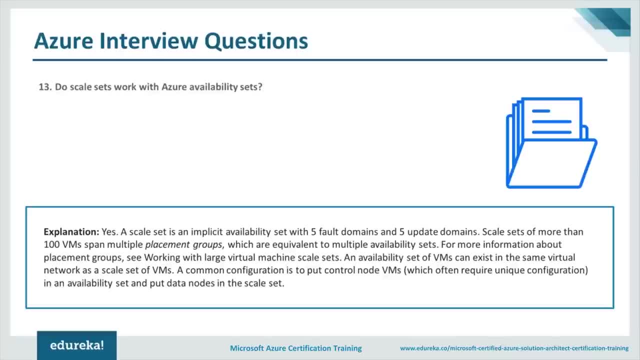 And there is something called fall domain and update domain as far as high availability is concerned. So fall domain, say, is that if I have two VMs in same availability set, both the VMs will share the common power source and common network. okay, 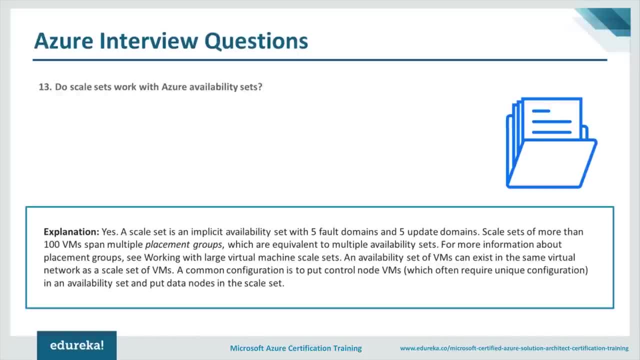 As far as update domain is concerned. so update domain talks about that if I have, say, for example, 10 VMs and I will keep the value of update domain to two, so I will have sets of two to each right, So I'll have a group of two to each right. 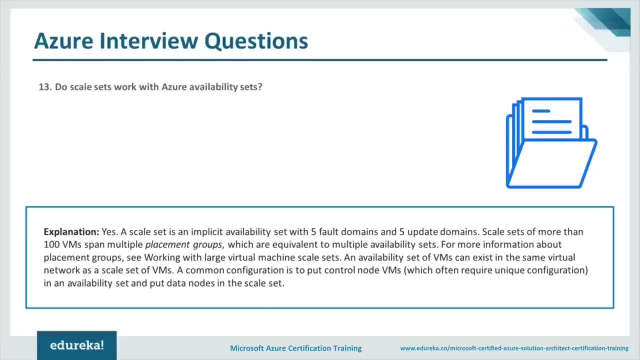 And at a given point in time. if Microsoft needs to perform a planned maintenance, only one update domain will go down at a given point. So this is what my update domain means. So now, does it support my availability set? The scale set supports my availability set. yes, 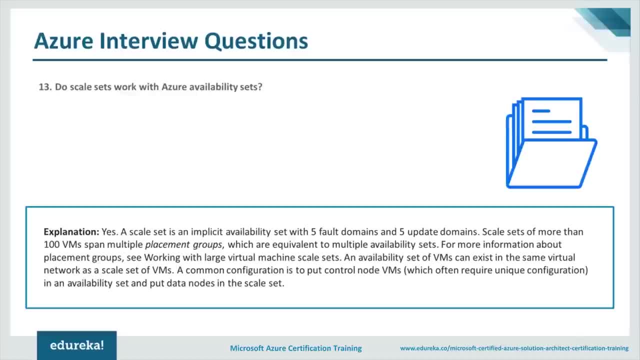 The scale set supports my availability set and you can just go ahead and fetch some information about the availability set if you're not very much well-versed with availability sets. as far as my Azure is concerned, okay, And there is a small description also over there. 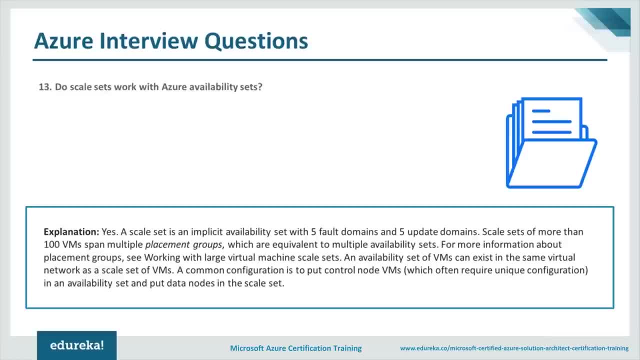 So I'll just read that for you: Yes, a scale set is an implicit availability set with five fault domains and five update domains. okay. Scale sets of more than 100 VM span multiple placement groups which are equivalent to multiple availability sets. okay. 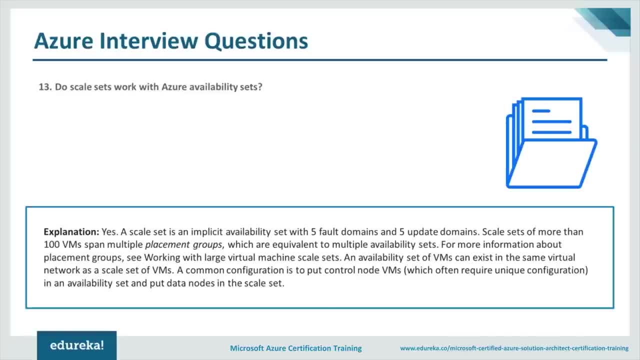 So this is what it means, and then I will just skip the other part, because I've given you enough explanation for this, and I would definitely recommend that you read the availability set. Okay, now the question is: what is a break-fix issue? 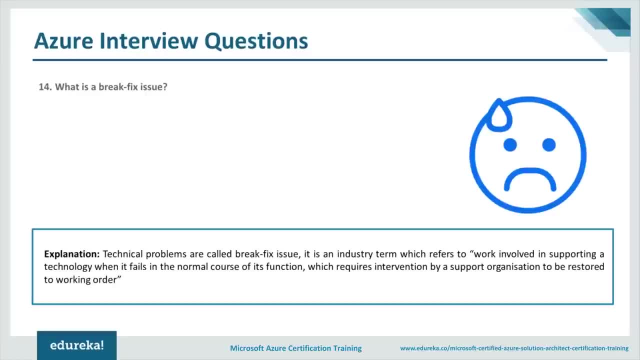 Break-fix issue is a technical problem which is like your environment is running and then all of a sudden a problem comes right. That is a break, and then fixing that particular problem is my fix right. So technical problems are called break-fix issues. 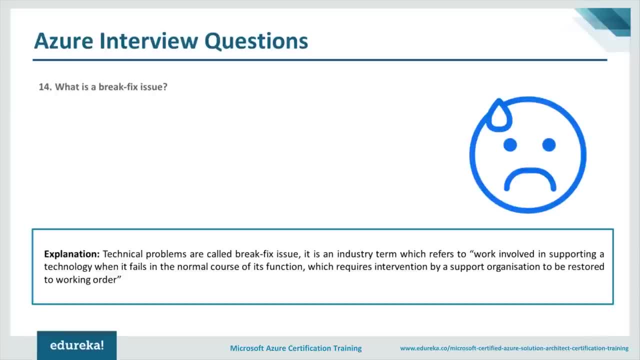 It is the industry term which refers to work involved in supporting a technology when it fails in the normal course of function, which requires intervention by a support organization to restore the service. okay, So this is what break-fix is. Now. it's not specific to Azure, actually. 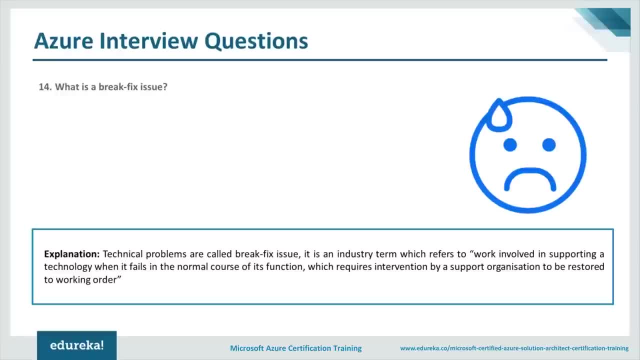 It's just a common term, what we use as far as my services are concerned. So even if I talk about on-prem, on-premise networks, so we still talk about break-fix issues, right? So I'm not sure how many people. 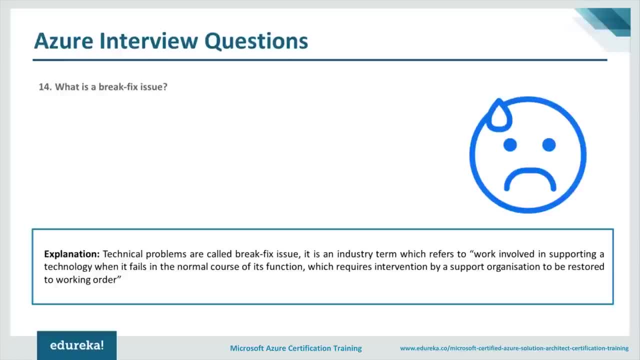 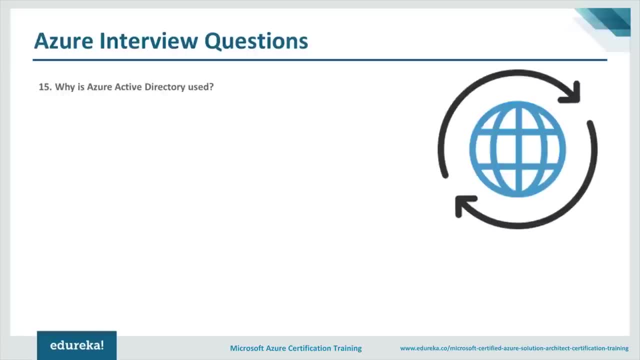 have got a chance to call Microsoft and open a support case in case you have issues with any of the things in your environment, So those issues are basically my break-fix issues. Jumping on to the next question: why is Azure Active Directory used? 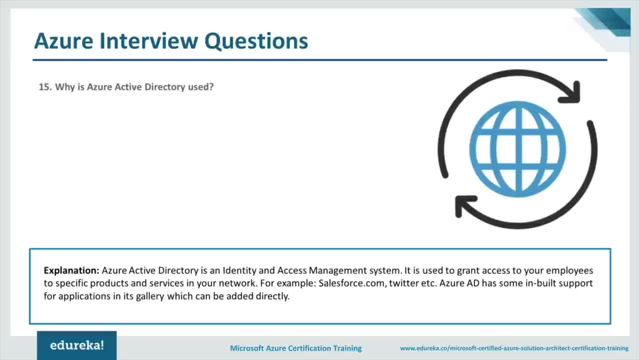 Now, when you talk about Azure Active Directory, Active Directory is used for identity and access management, first of all, And it's a PaaS-based service. Azure Active Directory is a PaaS-based service. Now it is used to grant access to employees. 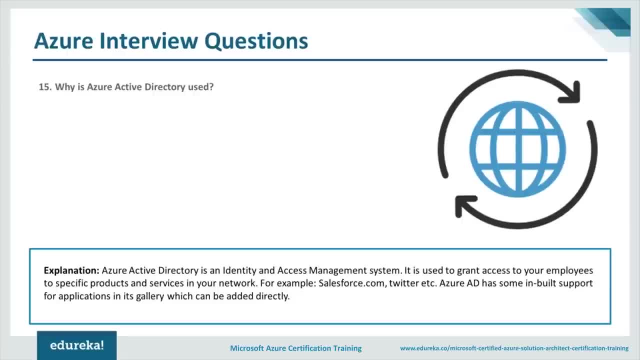 to specific products and services in your network. So there are a lot of examples: Salesforcecom, Twitter, right. I can give you a few more examples: Office 365, Intune, which are two different products from Microsoft, So they work with Azure Active Directory right. 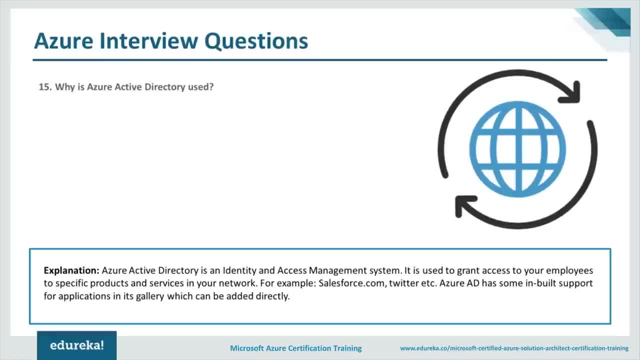 Now Azure AD has some inbuilt support for applications in the gallery which can be added directly. okay, So there is a gallery and then you can just go ahead and add support for Azure Active Directory to any application which is available in the gallery. 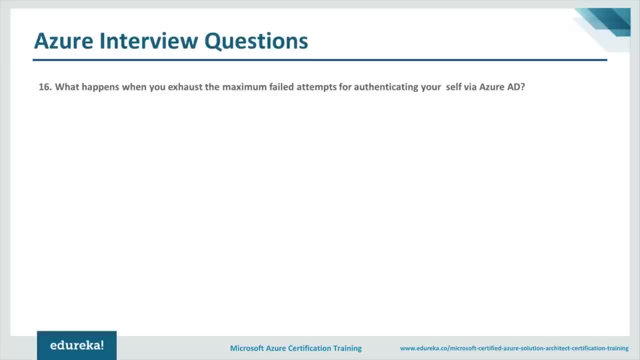 Okay, talking about a few other questions regarding Azure AD, what happens when you exhaust the maximum failed attempts for authenticating yourself via Azure AD? okay, So we have a more sophisticated strategy to account lockout, which is based on IP of the request. 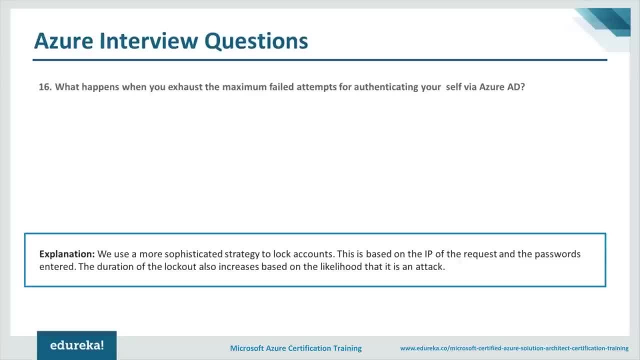 and the password entered, okay. So now when you talk about on-prem, we talk about account lockouts. So if you enter into your account incorrect passwords more than three times, so your account is locked out and it will be unlocked after maybe 15 minutes. 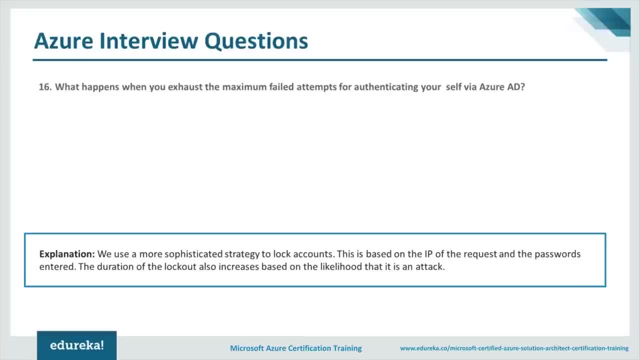 or half an hour, or one hour, based upon how your administrator has configured it. Now the same thing happens in Azure AD, but then it happens based upon the IP address. okay, So it will go ahead and track the IP address of the request and the password entered. 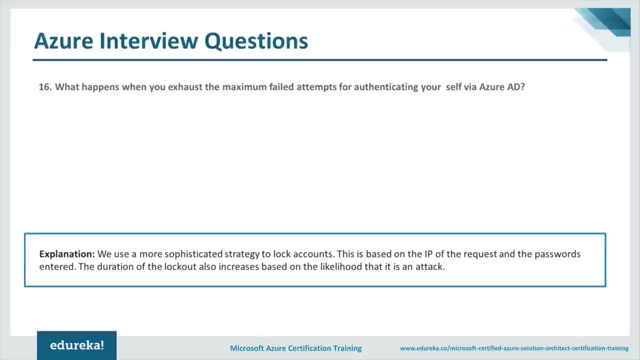 and the duration of the lockout also increases based upon the likelihood that is in the attack. Okay, so this is how it works when we talk about maximum failed attempts for authenticating yourself. Okay, jumping onto the next question: Where can I find a list of applications? 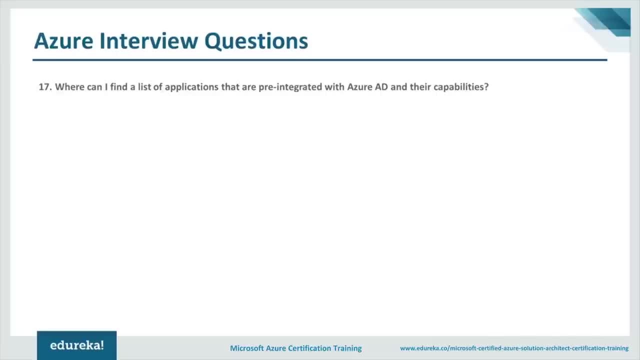 that are pre-integrated with Azure AD and their capabilities. So, when you talk about this, my Azure AD has around 2,600 pre-integrated applications, and all pre-integrated applications support single sign-on. Single sign-on lets your organization credentials 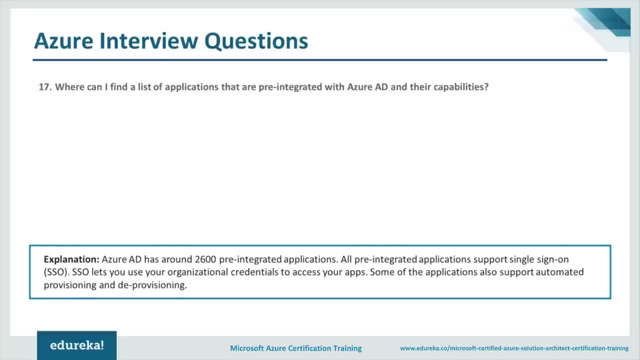 to access your apps. Some of the applications also support automated provisioning and deprovisioning, So there's a gallery. you can just go to the gallery and then you can get a list of applications which are available for using my Azure AD. 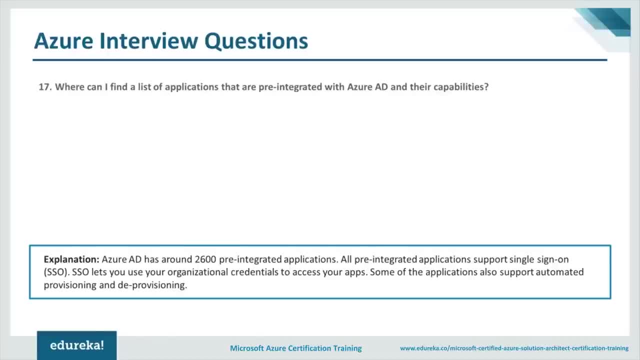 But of course, that is not the complete list of applications which are available which you can use. as far as this is concerned, There are a huge number of applications which are supported by Azure AD. okay, Of course, single sign-on is one of the components. 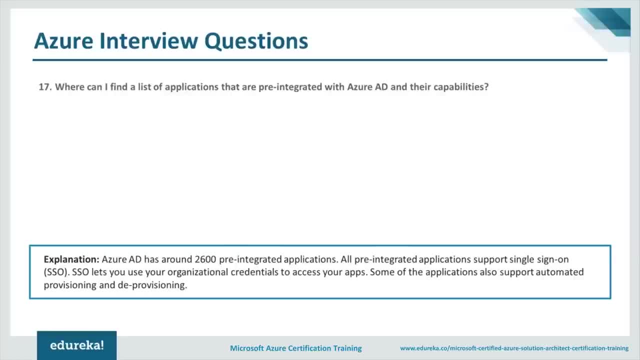 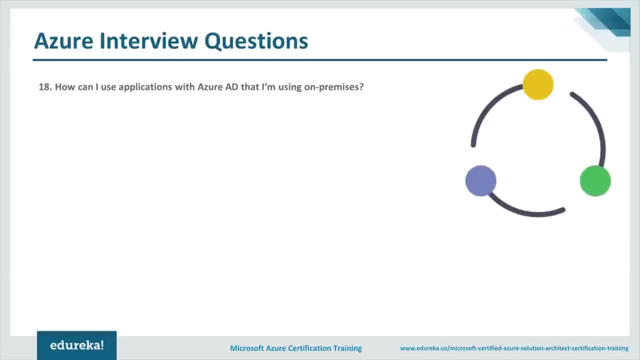 of Azure AD. so probably, in case you're not aware of single sign-on, you can just go ahead and do some research on that. Now, talking about the next question: how can I use applications with Azure AD that I'm using on-prem? 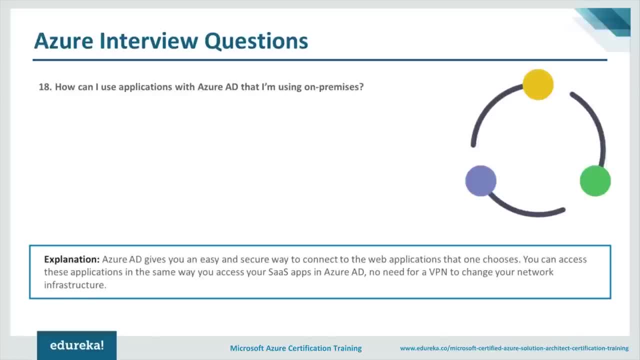 Of course you can do that. Now. Azure AD gives you an easy and secure way to connect to the web app that you choose. You can access these applications in a way. you can access your SaaS-based applications in Azure AD, So you don't need to have a VPN installed, okay. 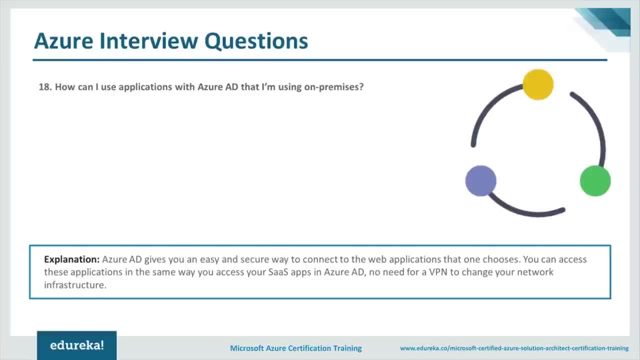 You can just go ahead and install a component and then you are ready to go. You can use the applications which are there on-prem. A few examples I can give you is: you can use your SharePoint. You can use your web apps, for which the servers 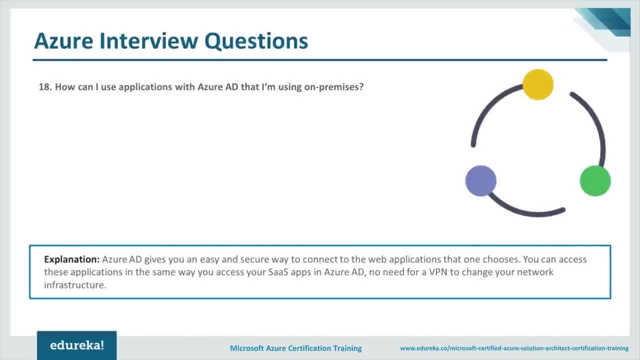 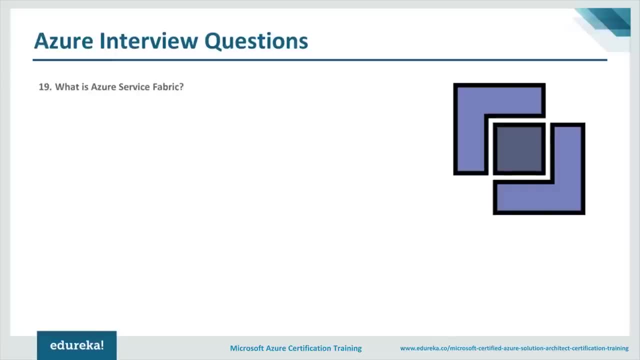 are installed on your premises and you would like to use Azure AD for authentication, So you can do that for sure. Now the question: important question, very important question: what is the Azure Fabric, Service Fabric? So when you talk about that, my Azure Service Fabric? 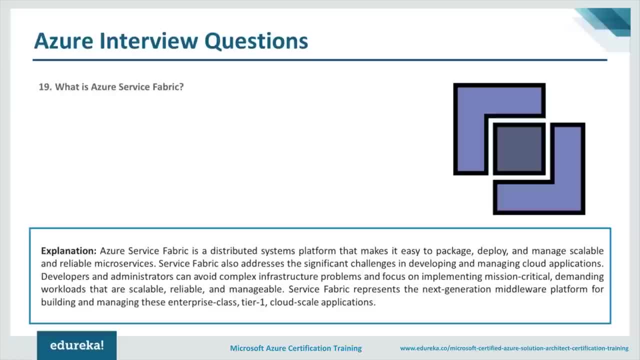 is a distributed system platform that makes it easy to package, deploy and manage scalable and reliable microservices. okay, So this is the guy which actually controls your network, your storage and your compute. okay, Which are basically the most critical components. 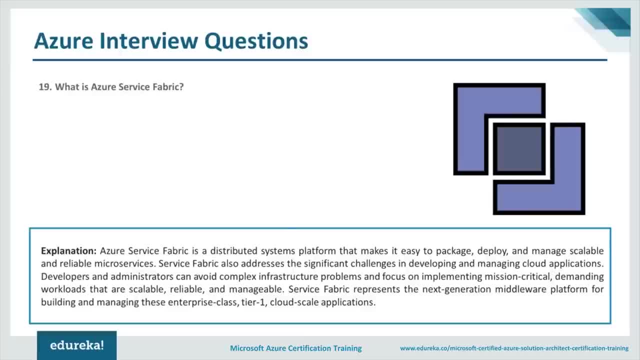 of my cloud. So if my Fabric will not be running in the backend, so nobody will be assigning IP addresses, nobody will be assigning the resources and nobody will be assigning the storage. okay, So this is the guy which actually runs everything. 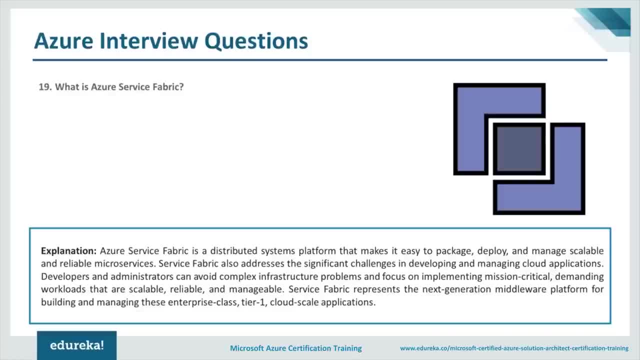 I would say in the cloud infrastructure. right, Okay, let's go further. Service Fabric also addresses the significant challenges in developing and managing cloud applications. Developers and administrators can avoid complex infrastructure problems and focus on implementing mission-critical, demanding workloads that are scalable, reliable. 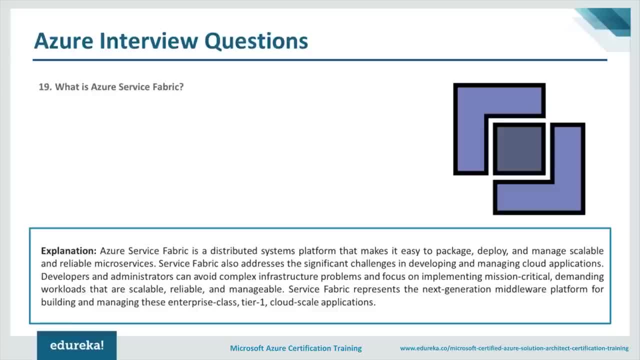 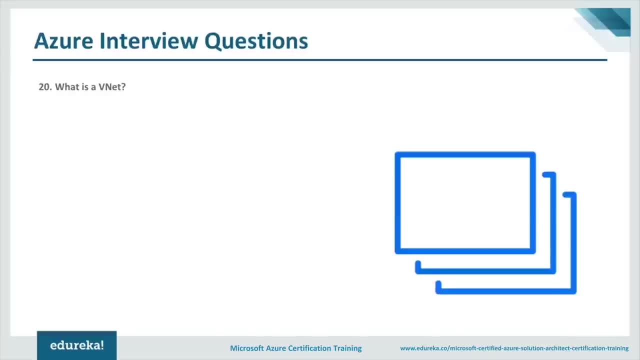 and manageable. Now my Service Fabric represents the next-generation middleware platform for building and managing these enterprise-class tier-one cloud-based applications. okay, Now, what is VNet? VNet is basically nothing but my virtual network, So VNet is a representation of your own network. 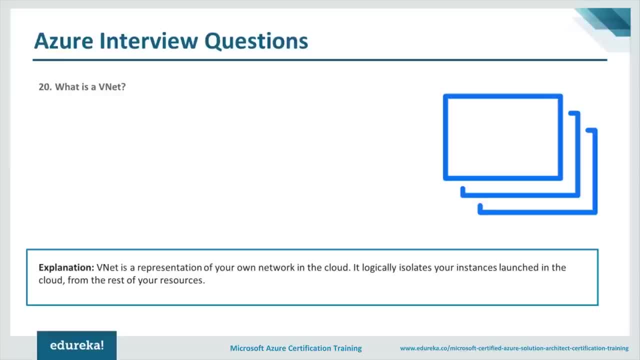 in the cloud. It logically isolates your instances launched in the cloud from rest of the resources which you have in the cloud. So this is my whole network, based on which my configuration of machines depend, I mean the subnets. the address space depends on right. 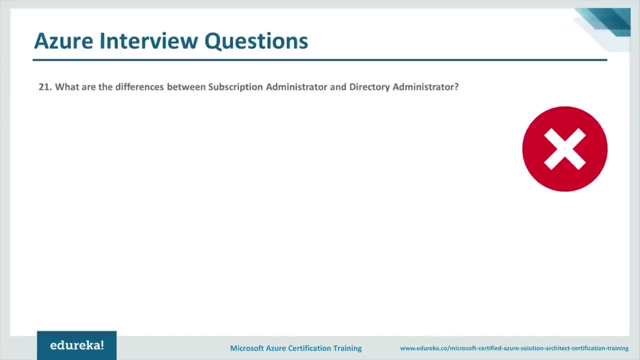 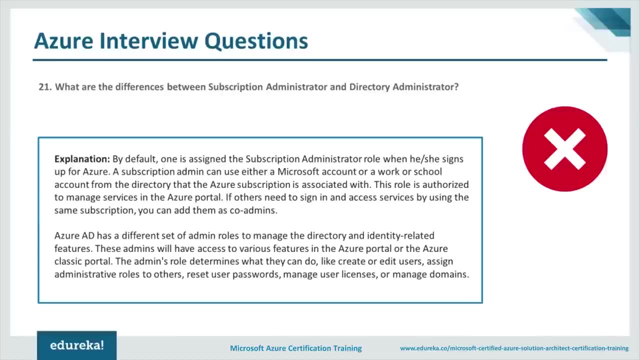 Talking about a few other things. what are the differences between subscription administrator and directory administrator? So when you talk about the subscription administrator, the subscription administrator is the one which is responsible for the complete subscription. Now, by default, only one subscription administrator role. 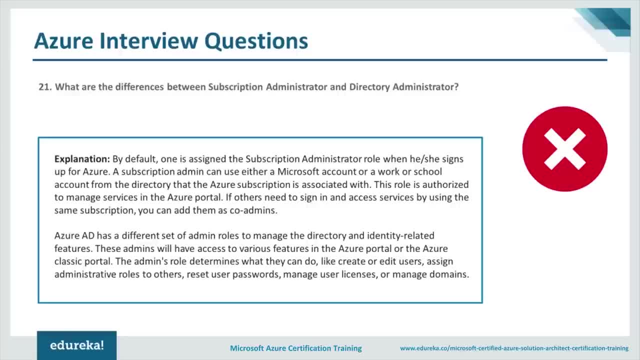 is assigned in Azure. A subscription administrator can either be a Microsoft account, or either can be your work account, and that guy has control over the complete Azure portal and the services which run on that. okay, If you want, you can just go ahead and sign up more accounts. 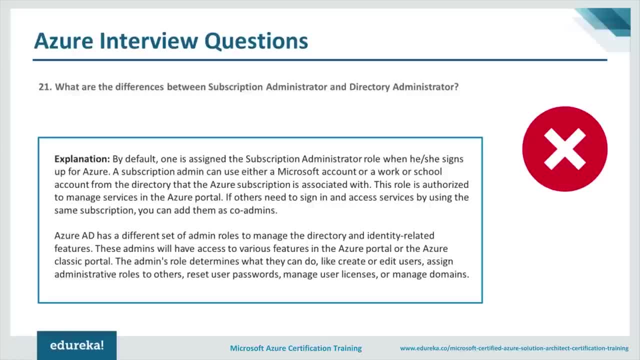 which are basically subscription administrators, And these people are my co-admins. Now, as far as the Azure AD is concerned, so the account which we set up over there for identity and access management, so we talk about my Azure AD administrator, the directory administrator. 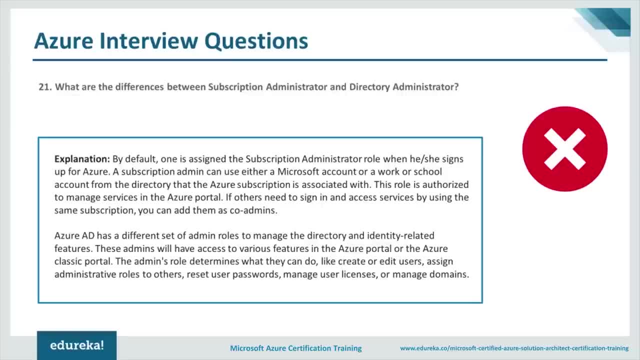 So let's just read this: Azure AD has a different set of admin roles to manage the directory and identity related features. These admins will have access to various features in Azure portal or the Azure classic portal and the admin rules determine what they can do. 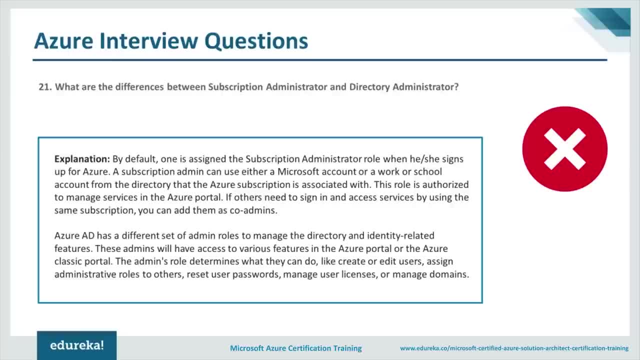 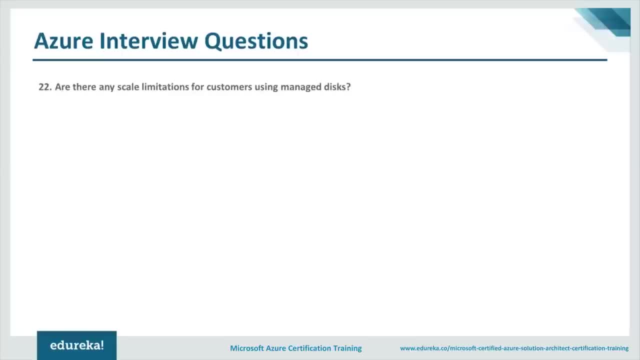 like create or edit users, assign administrative roles to others, and so on. So this is what my Azure AD administrator does. Are there any scale limits for customers using Managed Disk? Managed Disk eliminates the limit associated with storage accounts. Now, first of all, you need to understand. 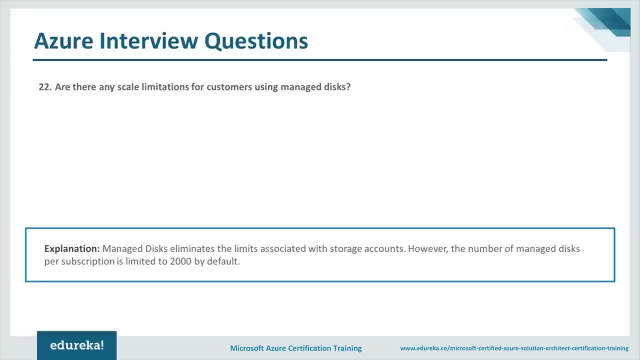 what is a Managed Disk right? When you create a machine now these days you will have an option over there that you want to use Managed Disk or Unmanaged Disk right. So when you select Managed Disk, Microsoft manages. I would not say Microsoft. 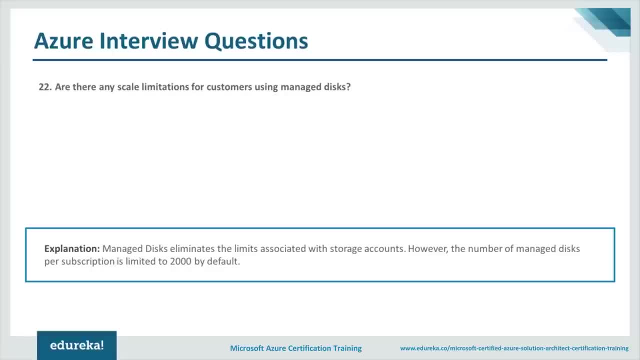 but then the Azure fabric manages all your disk right. So a disk which is assigned to VM will be managed by Azure. okay, So this is what my Managed Disk is Now. using my Managed Disk, I basically eliminate the limit associated with my storage account. 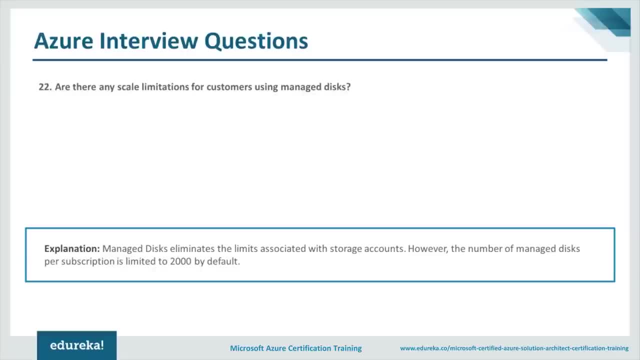 However, the number of Managed Disk per subscription is limited to 2,000 by default. okay, So you can have 2,000 Managed Disk in Azure subscription. Now talking about what is the difference between service bus queues and storage queues. 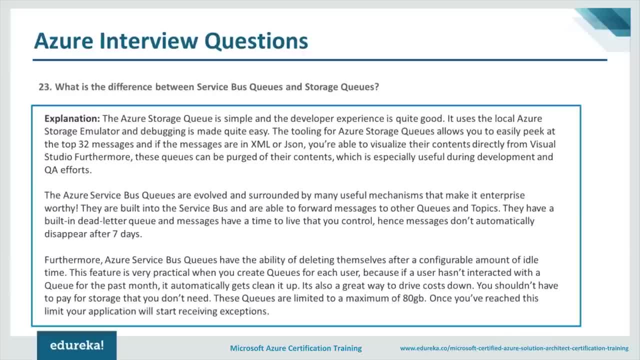 Now the Azure storage queue is simple and the developer experience is quite good. It uses the local Azure storage emulator and debugging is made quite easy. The tool for Azure storage queue allows you to easily peek at the top 32 messages and if the messages are in XML or JSON. 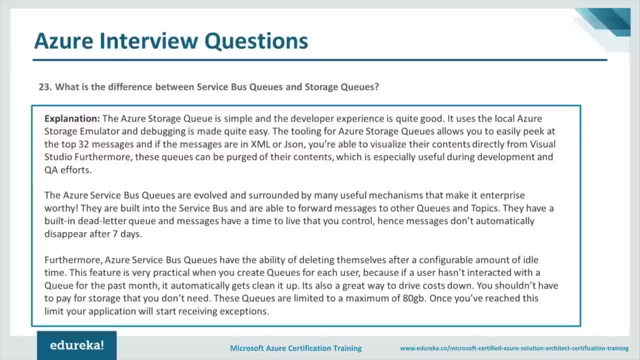 you'll be able to visualize their content directly with the Visual Studio. Furthermore, these queues can be purged of their content, which is especially useful during the development process. the queue efforts, basically, And as far as my service bus is concerned, so the Azure service bus queues are evolved. 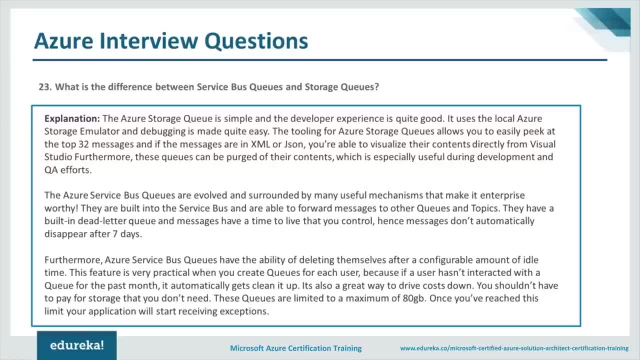 and surrounded by many useful mechanisms that make it enterprise-worthy. They are built into service bus and are able to forward messages to other queues and topics, and they have built-in header message queue and messages that are timed to live. that has control, hence messages don't automatically 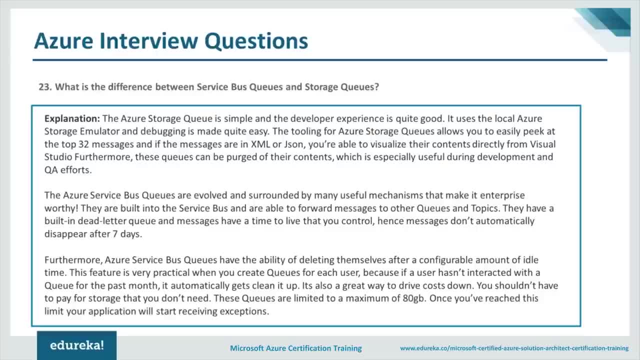 disappear after seven days. So if you talk about this, probably you'll have to go ahead and read about what is a service bus queue and my storage queues. So I talk about my storage queues, which are a part of my storage itself, If you're not aware of storage. 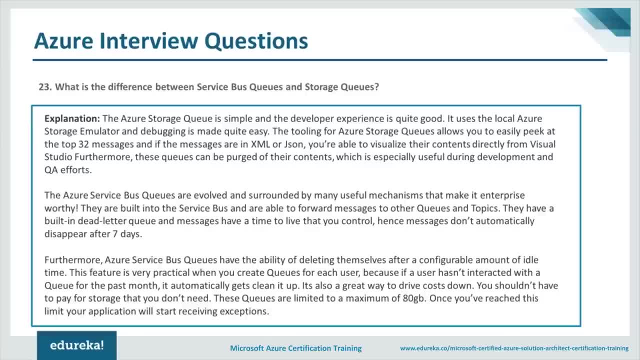 storage has four types of storage: One is my blog, one is my files, one is my queues and one is my tables right. So I need to have more information of what my storage queues is. Okay, now talking about what is Azure Redis cache? 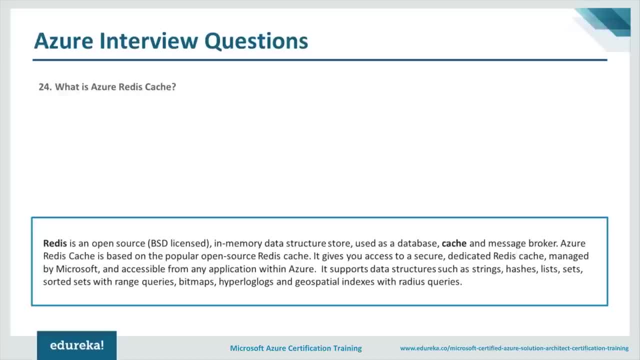 So Redis is an open source in-memory data structure store used as a database. And then you talk about cache and a message broker. So when you talk about my Azure Redis cache, that is based on the popular open source Redis cache. It gives you access to secure, dedicated Redis cache. 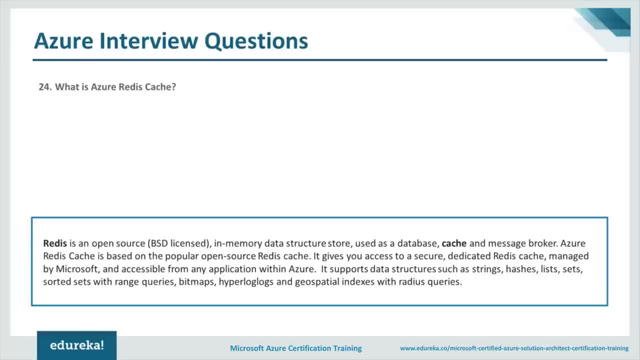 managed by Microsoft and accessible from any application within Azure. It supports data structures such as strings, hashes, lists, sets, sorted sets with a big range of queries, bitmaps, hyperlogs and indexes with radius queries. Okay, Another question we talk about is: 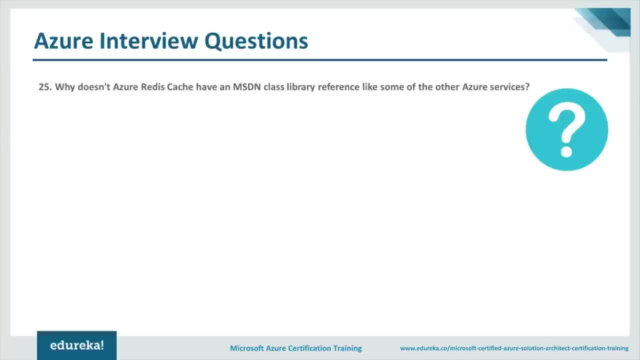 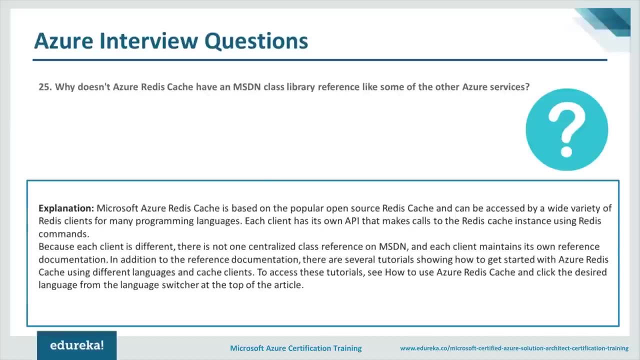 why does not Microsoft Redis cache have an MSDN plus library reference, like some of the other Azure services? Now, of course, when you talk about this, this is an open source. one very important thing Now my Microsoft Redis cache is based on. 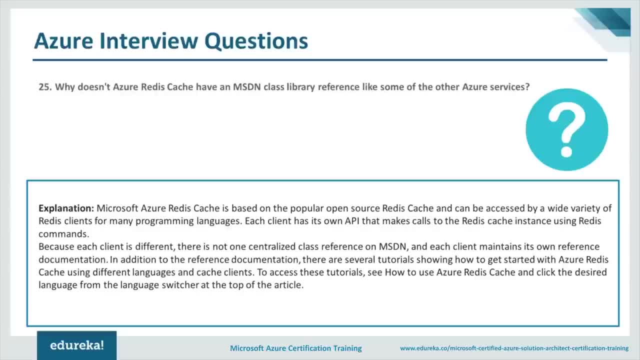 the popular open source Redis cache and can be accessible by a wide range of Redis clients, And that is the reason we cannot just go ahead and import it into MSDN. okay, So simple enough. just remember that, Because each client is different. 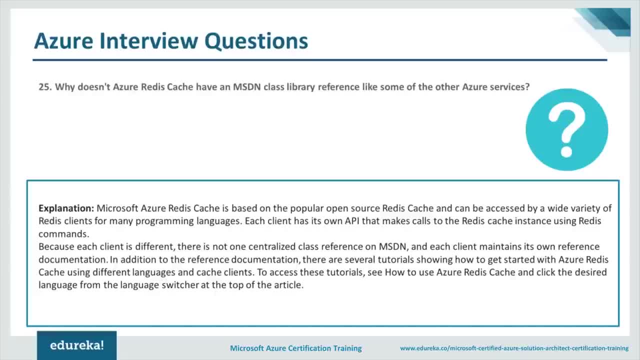 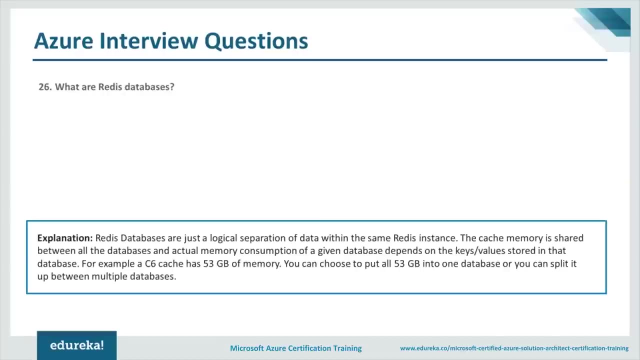 there is not one centralized class reference on MSDN, So we cannot just restrict it. maybe you can say right. So this is the reason we do not have any MSDN class library for my Redis cache. What is my Redis databases? So Redis databases are just a logical separation. 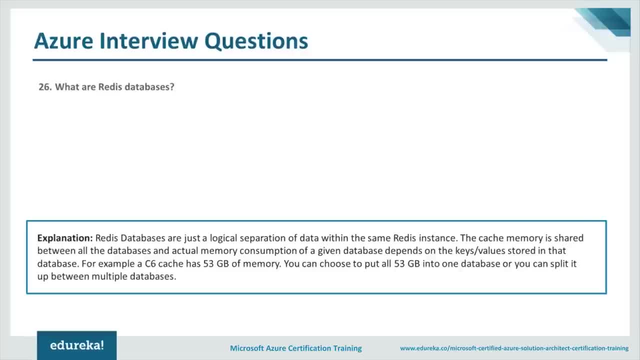 of data. within some Redis instances, The cache memory is shared between all the databases and actual memory consumption depends on the key values stored in the database. For example, a C6 cache has 53 GB of memory and you can choose to put all 53 GB into one database. 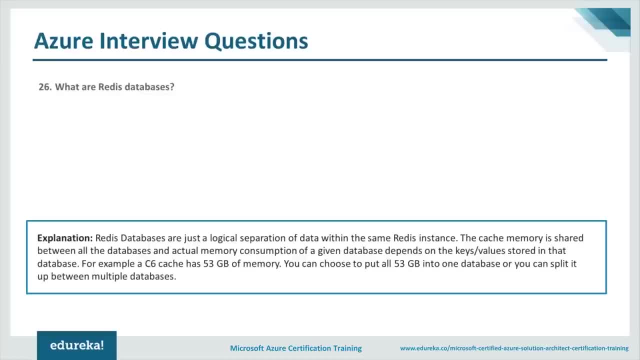 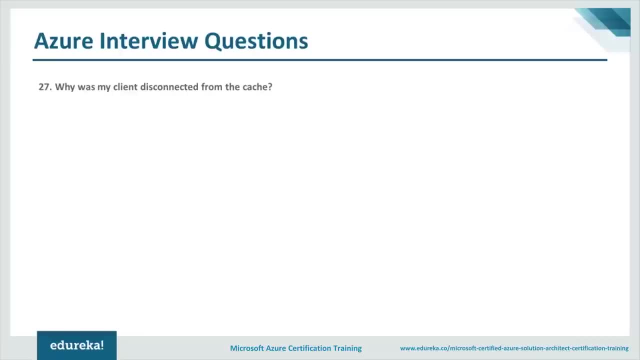 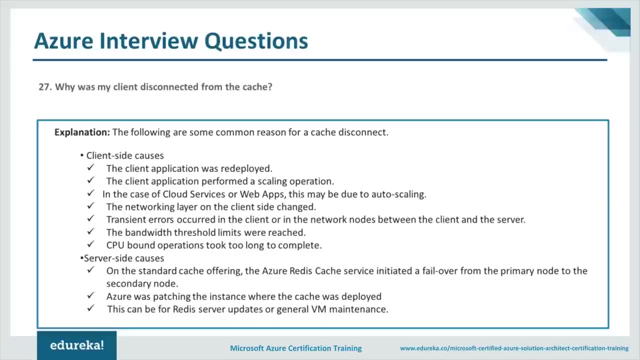 or you can split it into a multiple set of databases. Then you have another question: why was my client disconnected from the cache? Okay, Now, when you talk about this, the following are some common reasons for cache disconnect. Now, my client side causes the client side. 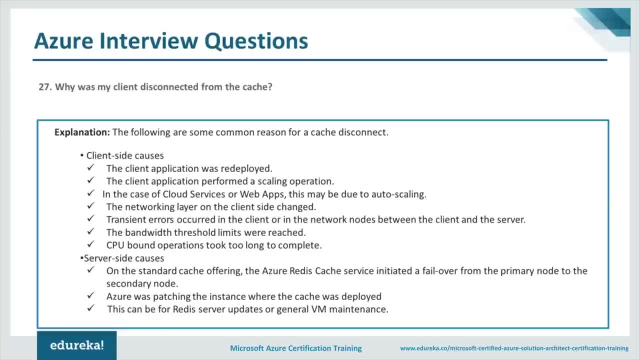 of the server issues. The client application was redeployed. The client application performed a scaling operation. In the case of cloud services or web apps, this may be due to auto scaling. The networking layer of the client side changed. Then you have transient errors occurred in the client. 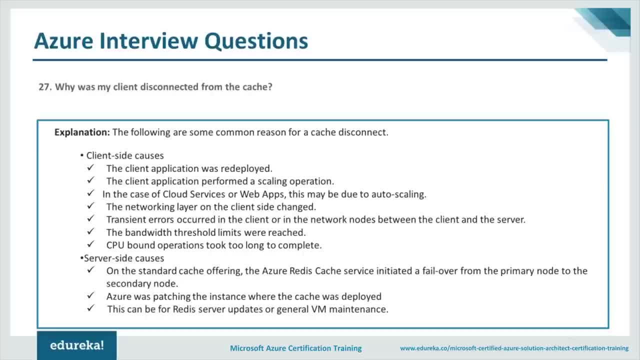 or in the network node because of the client and the server. The bandwidth threshold limits were reached. CPU bound operations took more long to complete, And then you have my server side issues also. few of these server side issues also On the stand cache offering. 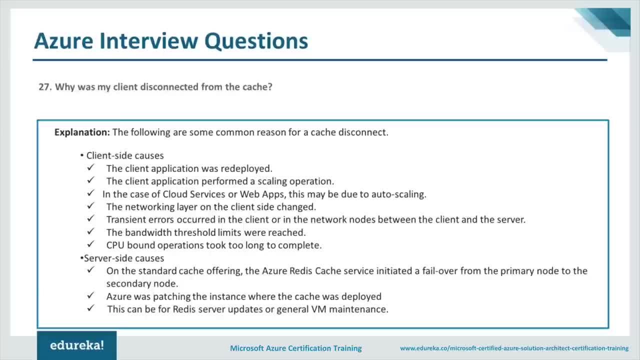 the Azure Redis cache service initiates a failover from the primary node to the secondary node. Now Azure was patching the instances where the cache was deployed, and this can be the Redis server updates or general VM maintenance. Then you have what is Azure Search? 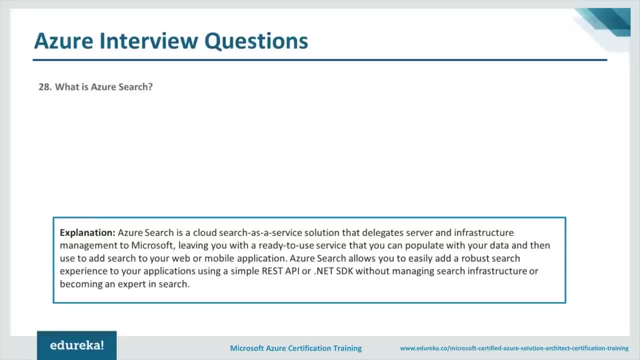 So simple enough. Azure Search is a cloud search as a service solution that delegates server and infrastructure management to Microsoft, leaving you with a ready to use service that can populate with all your data and then used to add search to your web or the mobile application. 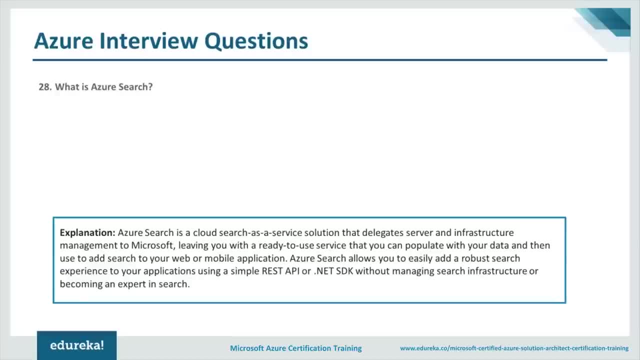 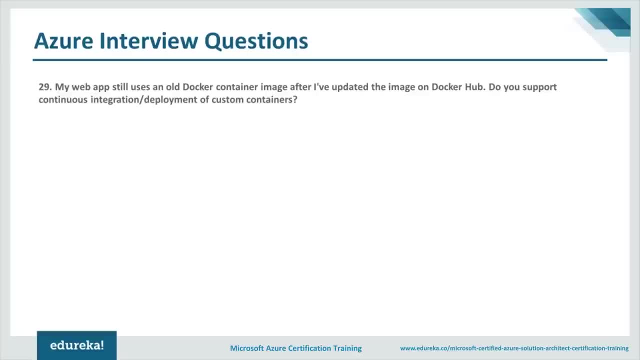 So it works with REST API or NET SDKs. of course, Few other questions. My web app still uses an old Docker container image and I have updated the image on Docker Hub, which is basically the new portal, what we talked about. So we are basically talking about container services. 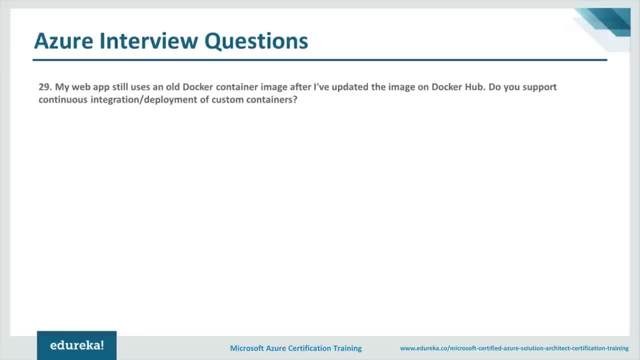 Do you support continuous integration deployment of custom containers? Now, first of all, for private registries. you can refresh the container by stopping and starting the web app, or you can change or add a dummy application setting to a force and refresh of your container. 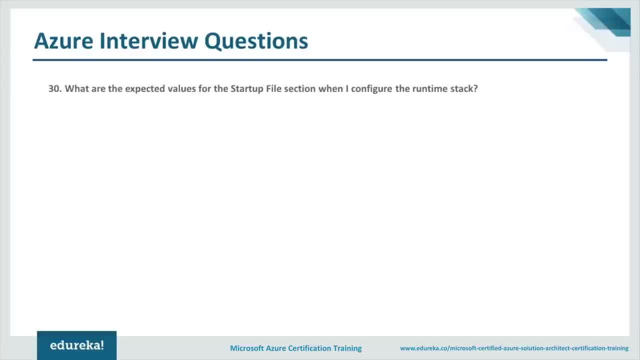 So this is what you can do. Now, talking about few things, what are the expected values for startup file section and I configure the runtime stack. Now for JS nodes: you specify a PM2 configuration file or your script file For NET code. 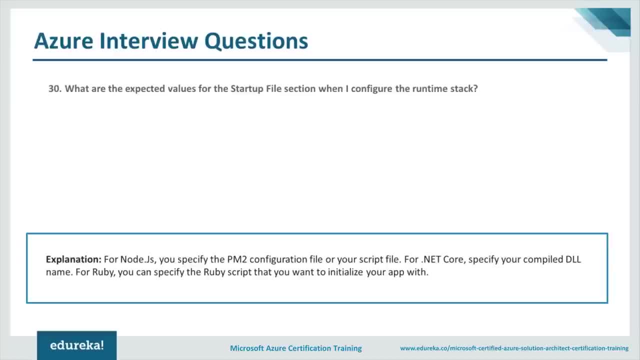 specify your compiled DLL name For Ruby. you can specify this and specify the Ruby script that you want to initialize with your app. Okay, How is your marketplace? subscription is priced. So we have these models. One is monthly fee, So pay as you go, kind of thing. 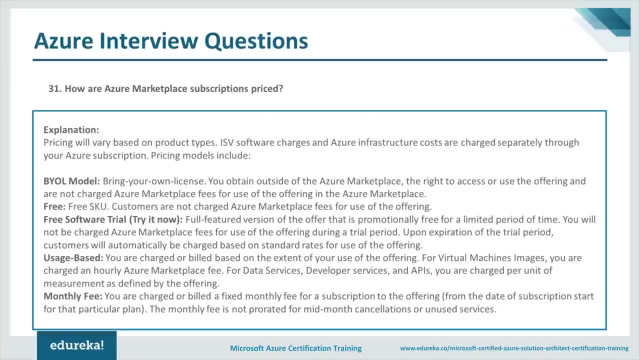 Usage based. Then you have free software. So Microsoft gives you a free subscription. So free subscription is valid for a period of one month and you get approximately $200 in that, So you can use that. Then you have the free. So this is for the customers. 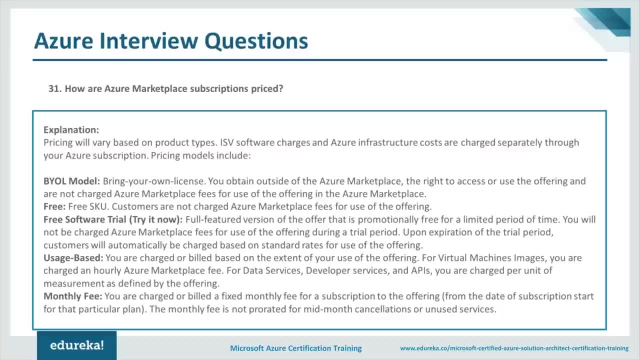 who are not charged marketplace fee for use of the offerings, the Microsoft offerings, And you have BYOL. bring your own license. Okay, So these are the subscription models, Basically how these are priced, you can say So, jumping on to the next one, 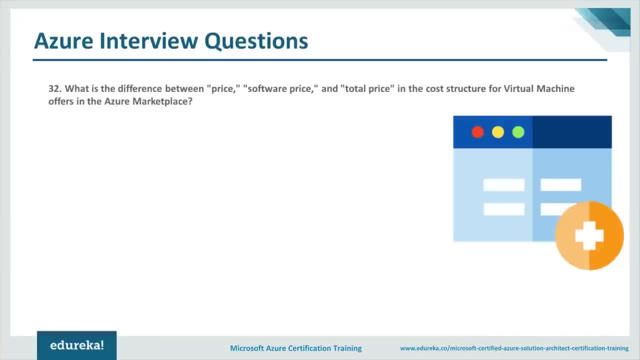 What is the difference between price, software price, total price and the cost structure for virtual machine offerings and virtual machines? So let's just see. Price refers to the cost of Azure virtual machine to run the software Software. price refers to the cost to the publisher software. 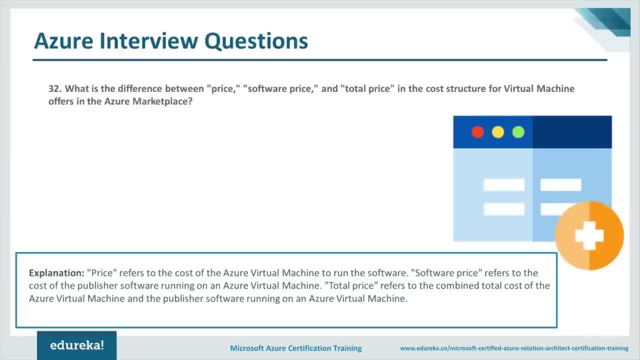 running on the virtual machine. Total price refers to the combined cost of these two. Simple enough? I don't think so. You need to get more details of this, because it's very simple. Price of VM: software price, total price. Total price is equal to price of VM. 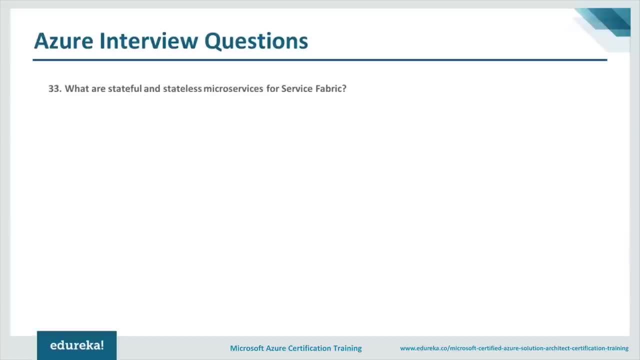 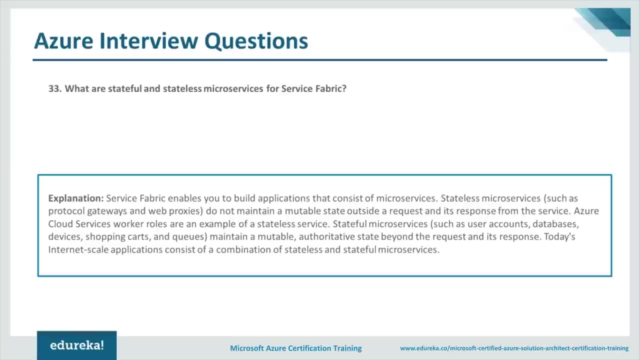 plus software price. Now the other question talks about what are stateful and stateless microservices for service fabric. So service fabric enables you to build applications that consists of microservices. So stateless microservices such as protocol gateway and web proxy do not maintain mutual state outside a request. 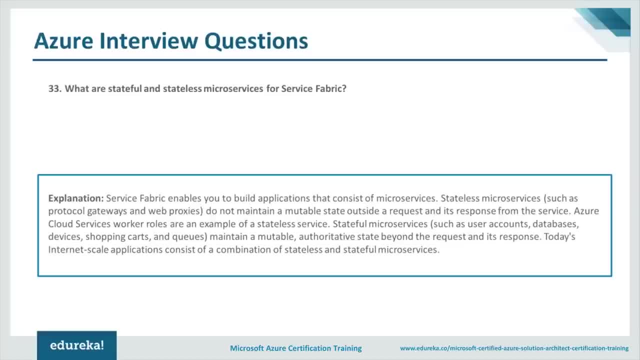 and its response from the service. Now, my Azure cloud service worker role is an example of a stateless service, and my stateful microservices, such as user accounts, databases, devices, shopping carts and queues, maintain a mutual authoritative state beyond the request and its response. 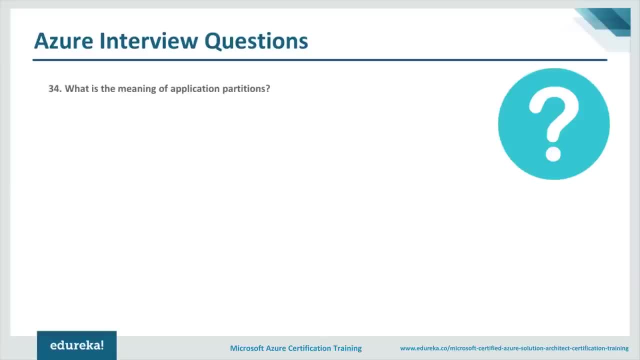 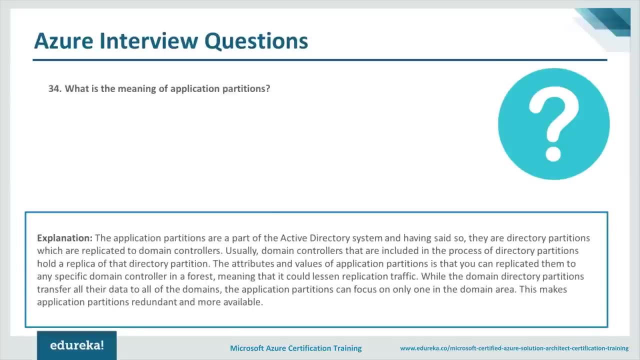 So this is how it works. Now, what is an application Application partition? Okay, Now, when you talk about the application partition, the application partition are a part of active directory system and, having said so, there are directory partitions which are replicated to domain controllers. 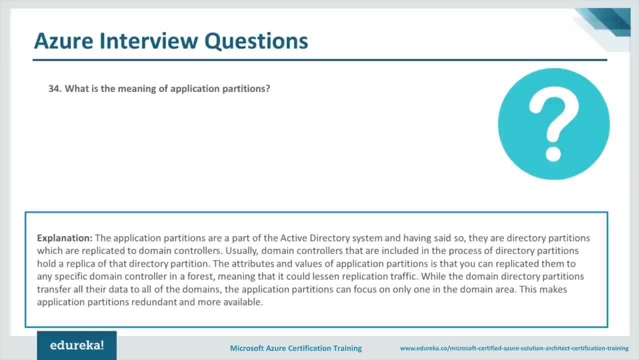 So usually domain controllers that are included in process of directory partition hold a replica of the directory partition. Now maybe you can read some more information. My domain controller has four types of partition. One is configuration, One is schema, One is my domain partition. 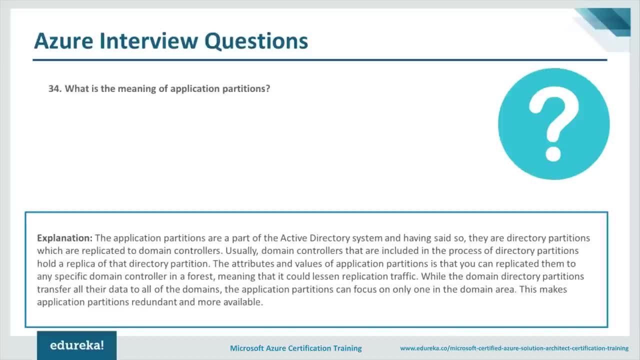 and the next one. you have my application partition, So all the information related to the application goes in the application partition. So it actually again has nothing to do with the cloud, but then it's always good to know, because if you're designing and developing an application on the cloud, 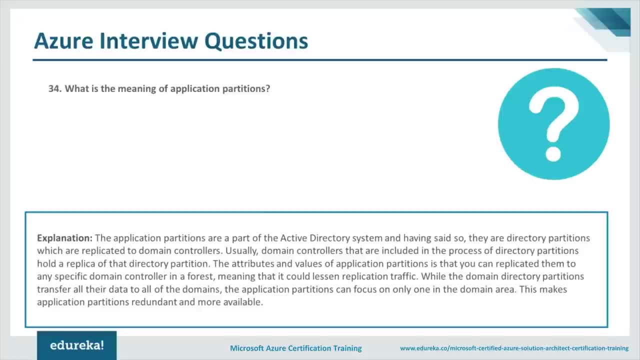 you can just go ahead and put that information in the application partition on the active directory server, But then it's very important for you to understand that we should have an active directory server up and running fine in the cloud. Okay, So these were a few of the questions. 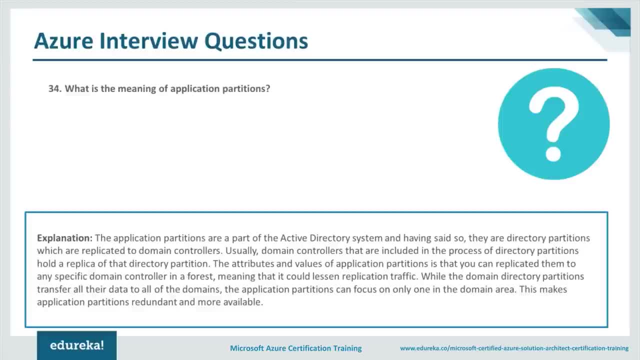 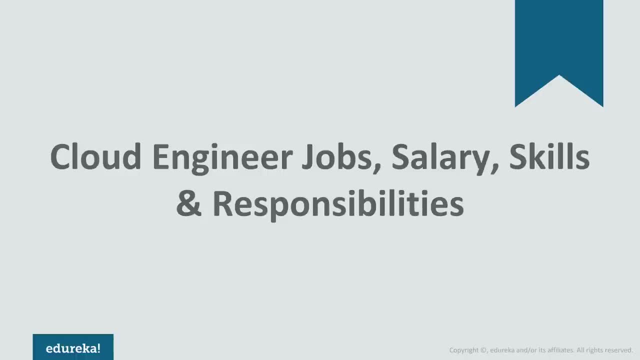 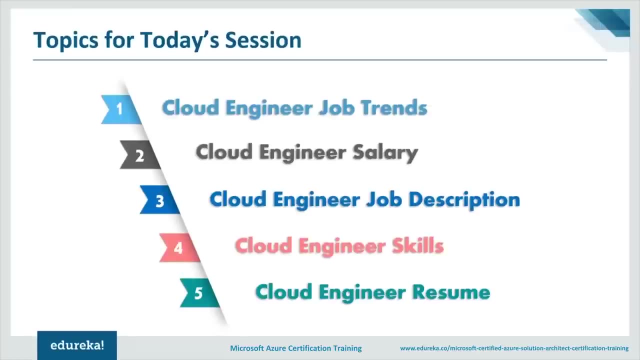 what we talked about as far as my interview questions are. So, first and foremost, I would start by talking about different job trends that are there in the current market. If you talk about cloud engineering, we would also discuss certain parameters that affect a cloud engineers salary. 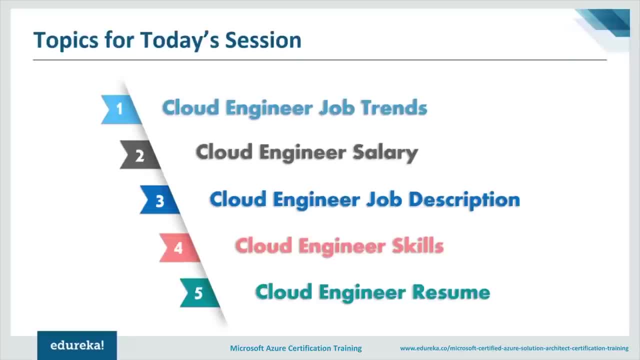 Then we would get into the details of job descriptions that are there in the market that different companies require in order to hire a cloud engineer. Moving further, I would also talk about what skills you should possess and how should you actually go ahead and shape your resume. 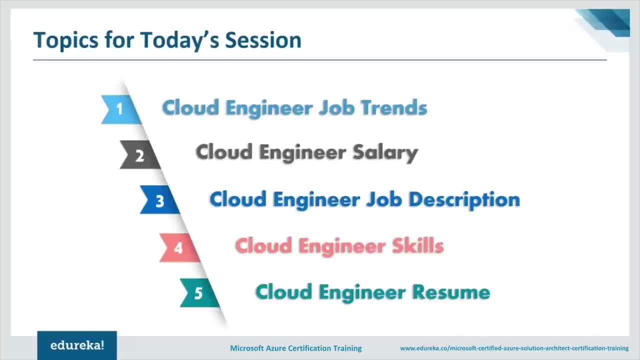 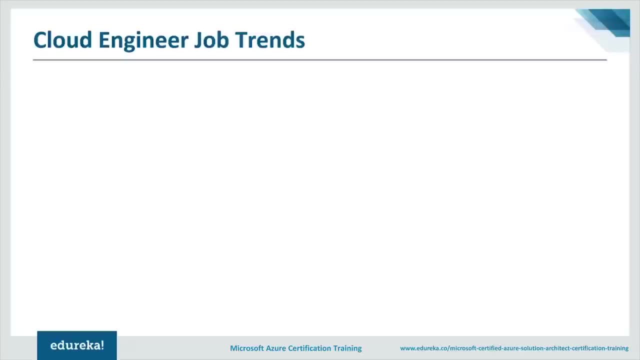 in order to apply for certain companies. having said that, guys, let's just move further and take a look at some of the job tents. now. guys, What I've done is I've actually gone out and jotted down certain figures for job vacancies in US and in India. 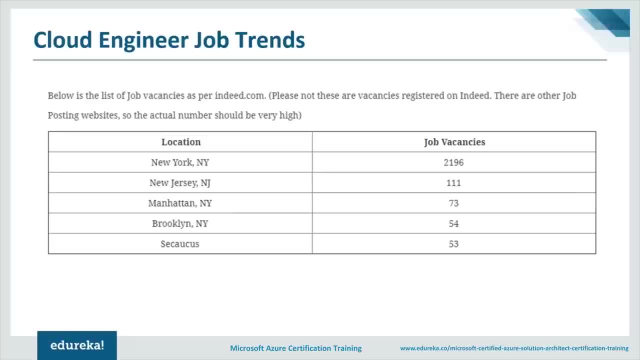 which tell the number as in: okay, These are the vacancies. now, These numbers are specific to, indeed, which is a popular job portal. They're quite a few other portals, So this number might not be consistent, It might vary, but as far as indeed is concerned, 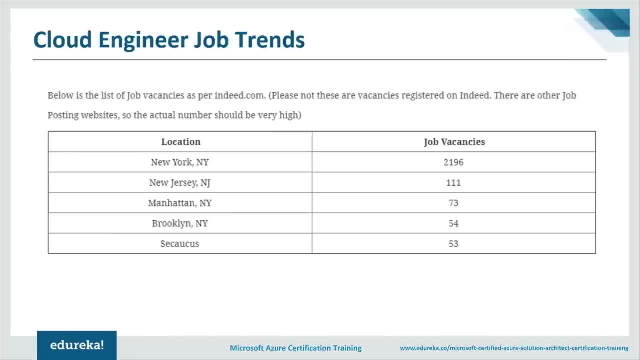 These are the numbers and these are the vacancies. So, guys, now these are certain factors here. I would like to lay stress on quite a few other pointers as well. to do that, What I've done is, recently I've written an article on this particular topic. 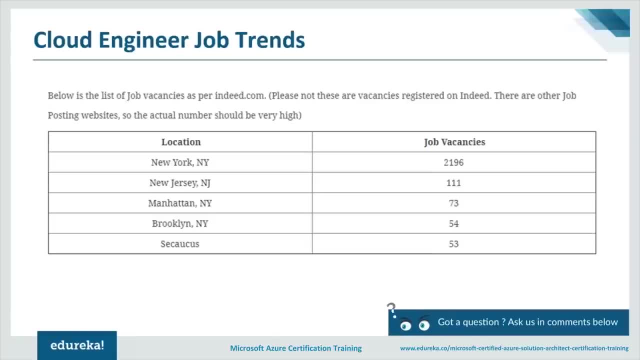 which talks about job trends and salaries in particular. So I would like to refer that blog and walk you through that blog so that we can discuss some of these pointers in little more detail. So let me just quickly Switch to the blog part. So yeah, guys. 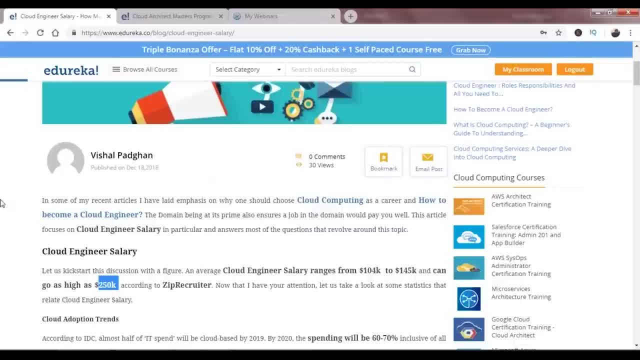 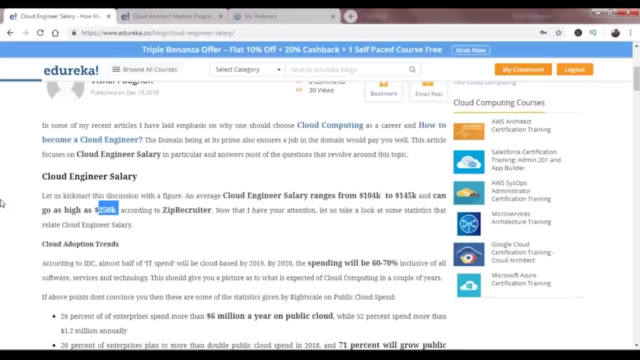 this is the article that I've written recently. If you take a look at it, there are certain factors here. now, zip recruiter: They gave in a number of, or the average salary of, a cloud engineer and they state that it is in the range of some around 104 K. 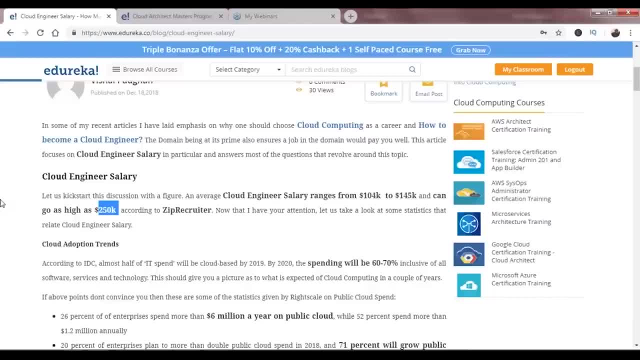 to 145 K dollars. Now that is a huge amount if you talk about US dollars and even if you talk about the salary in India. now, the fact that I'm recording this session from India, I believe I should give the number of Indian rupees as well. And the currency states that are the figure state that the amount is somewhere in the range of 15 to 20 lakhs for a mid-level ranged experienced person. even for a fresher, the amount is fairly high but it actually depends on the skill set that you have having. 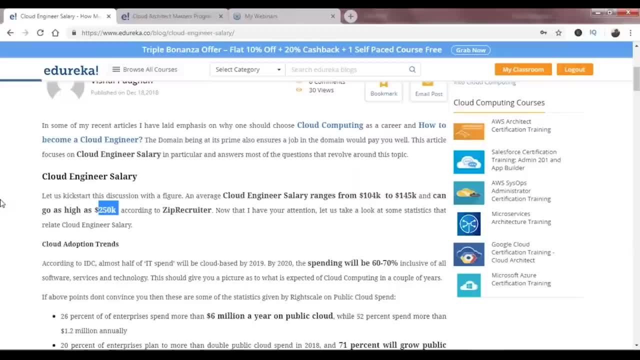 said that it also states that is zip recruiter, that it goes as high as somewhere around 250 K US dollars, which is a very big number right, And if you can actually go ahead and pick up right amount of skills, you would be getting a high amount of salaries. all I can say. 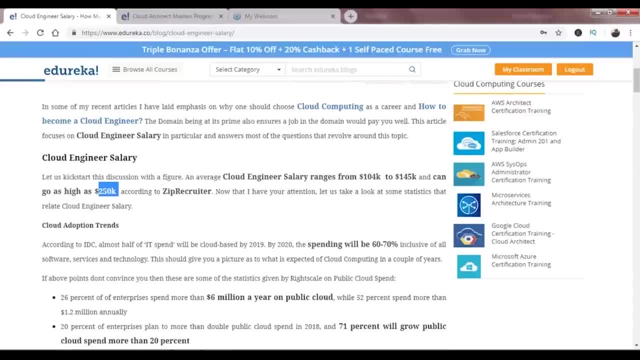 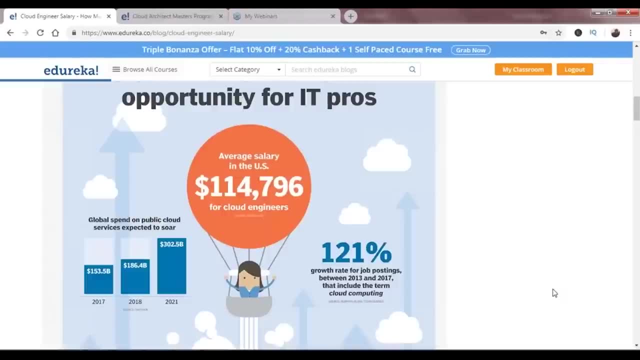 Having said that, let's just move further and take a look at some of the other trends that are there in the market Now. this is another interesting image which is given by Tech Target. Now they have put in certain stats in front of you. 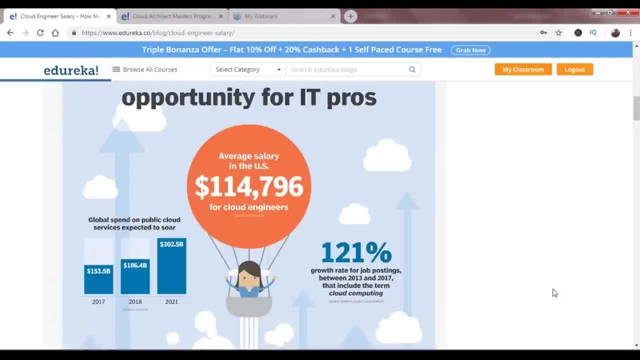 Now, if you take a look at it, they say that the average salary in USA is somewhere around 115,000.. Now, guys, this number might vary depending upon the number of data you take in, because different people refer to different websites and they pick up data from different sources. 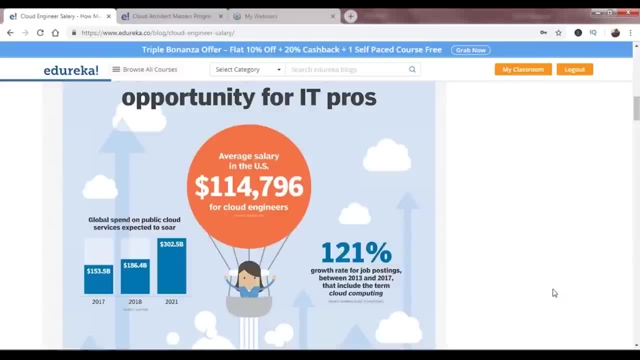 So, based on that data set, this number might vary a little. as I've already told you, it is somewhere in the range of 105 to 145 K US dollars. again, if you put in or take in data from other sources, that might vary a little, but that is more or less. 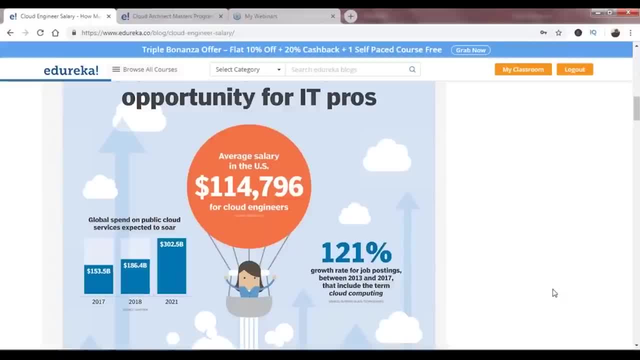 what this salary that you can expect. another important pointer here is that you can expect a lot of growth rate in cloud computing in recent or in near future. If you take a look at it, it says that it's a 1 21% growth rate. 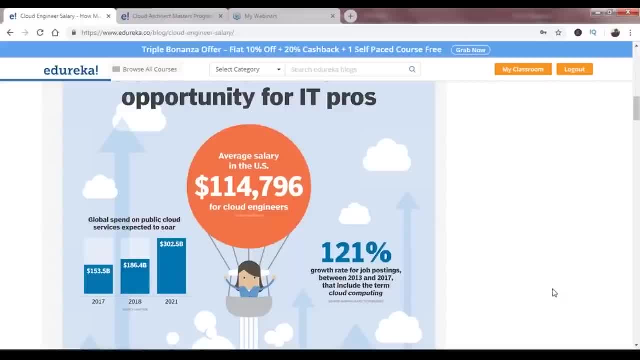 for job postings between 2013 to 17.. So these are the number of job postings that are there in the current market. are these are the numbers that have actually taken a rise in recent times? and, guys, this number is going to rise. Why? take a look at the number of global spend. 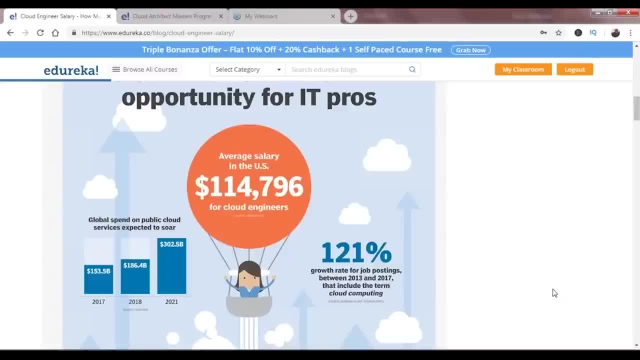 These companies are doing these days. when you talk about cloud computing in particular 2017, it was somewhere on 153.5 billion, then it moved to 186.4 billion and by 2021 it is expected to go somewhere on 302,. 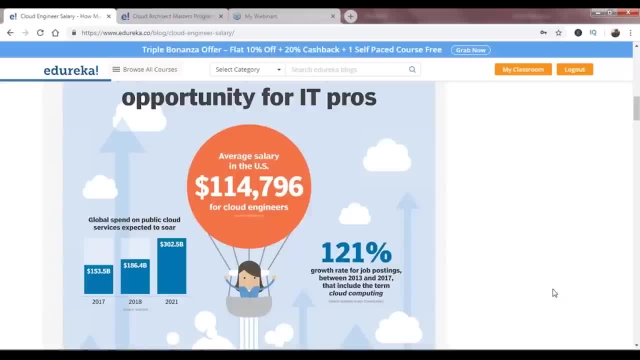 which is almost the double that you had in 2017, guys. So the fact, or this fact in particular, States that companies are ready to invest in this particular domain, and that means they would be requiring people who have skills in this particular domain, and hence the need for this kind of a role. 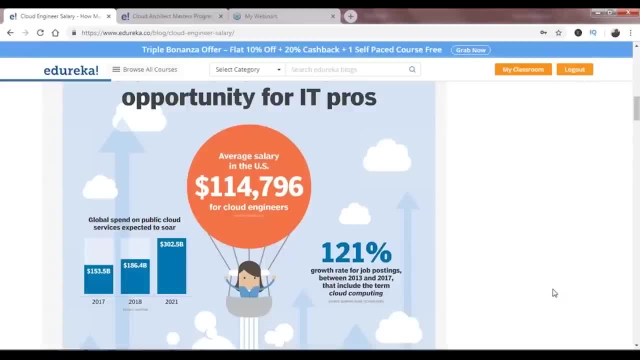 So if you talk about job Trends, salary, cloud computing is something that is booming and it is going to boom in near future as well, So you can expect good pay scale. You can expect good kind of life If you talk about a career in this particular domain. 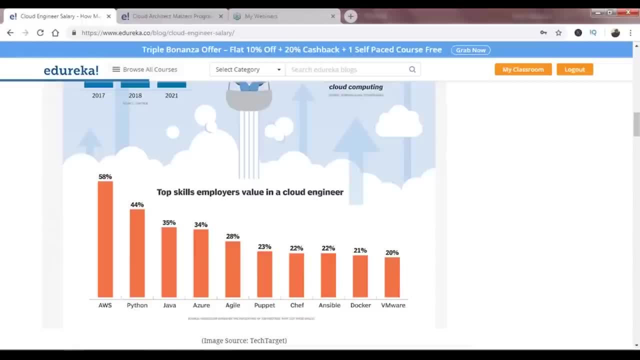 there's one more fact here, guys. These are some of the skills that employers normally demand a lot. as you can see, Python is something that is trending. if you talk about programming languages, everybody knows how important Python is because it's making news everywhere. people even claim 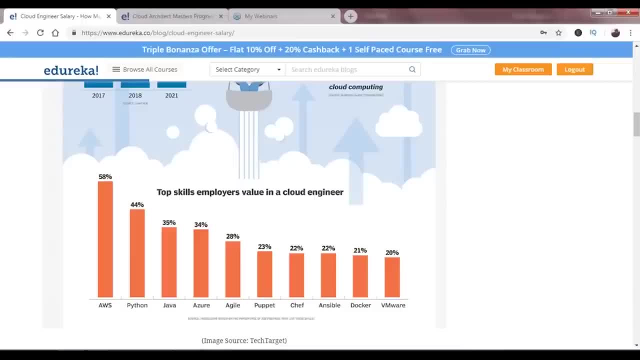 that it has dethrone Java. I do not know whether it's true or not. I don't get into those kind of debates. The reason people are claiming that is because it has actually changed the way programming happens these days, and that is why the popularity 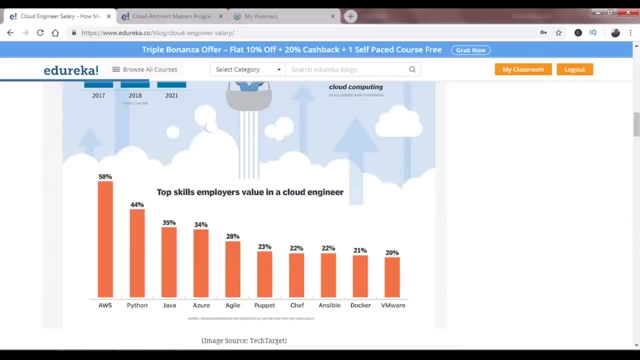 and one more factor that I would like to state here is if you take a look at its predecessor- not predecessor, but the one that follows before Python in this chart, it is AWS. It says 50% or 58% of people normally demand the skill. 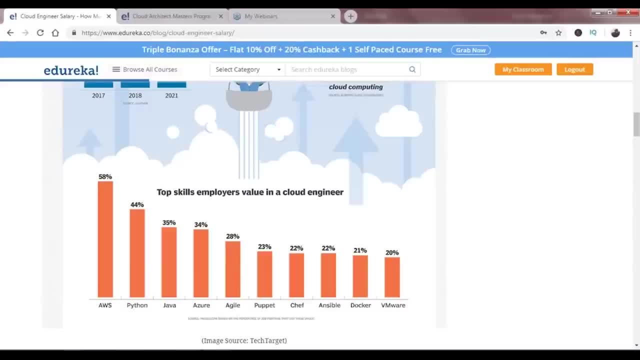 in the market. So, yes, you can gauge by it, as in how popular AWS has become. It is a popular cloud platform. So the fact that AWS goes well with all the programming languages or all the tools that follow in this chart, you can make sure that, or you can assume how popular AWS 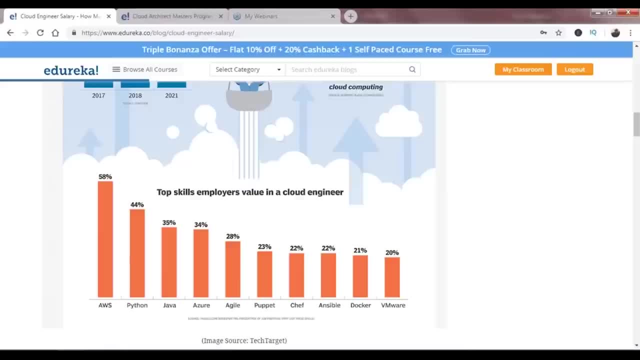 or cloud platform has become. So again, this stat states that if you try to make a career in this domain, it is going to be a good option for you or it's going to be a bliss for you is all I can say. Let's move further, guys. 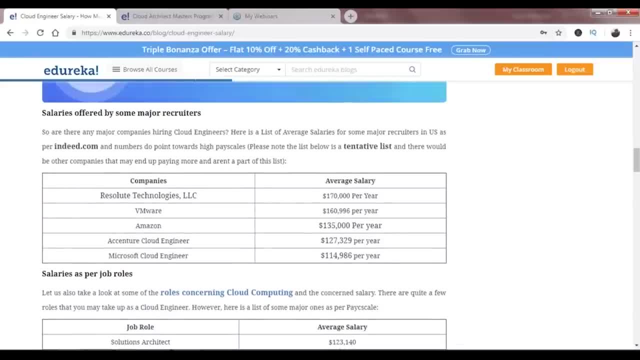 and take a look at some of the other factors as well. Now let's jump into the salary part, which follows our pattern in the agenda, which I discussed. So when you talk about different parameters that affect salary, one of them is: what are the companies? 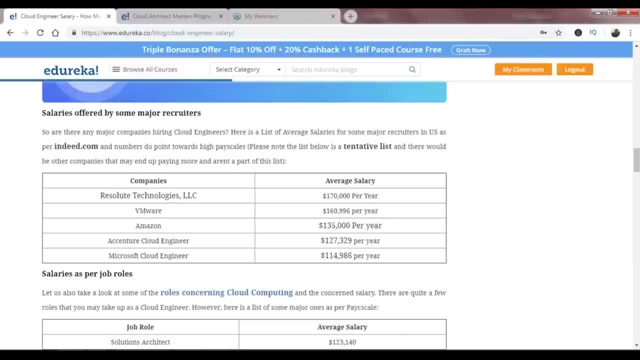 that are trying to hire cloud engineers, and what is the salary they're offering? now, guys, we take a look at some of the numbers here. Resolute Technologies, VMware, Amazon, Accenture, Microsoft- Now, these are popular companies, guys, and on an average, they're paying you somewhere on 170. 160 thousand US dollars, which is a huge amount. and again, if you ask me about the companies that are going to hire for cloud engineering, almost all the major companies that deal with computing or data processing. they are going to switch to cloud in near future companies. 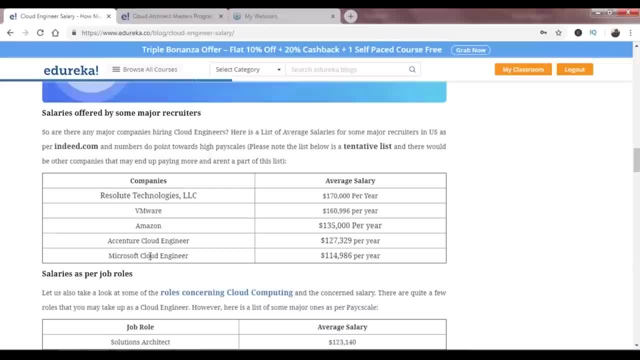 like GE General Electricals, They've actually gone ahead and move to cloud already, which is a big company, and quite a few other companies. now, if you talk about Amazon, if you talk about Google, Microsoft, they themselves are marketing cloud computing. They have their own service providers. 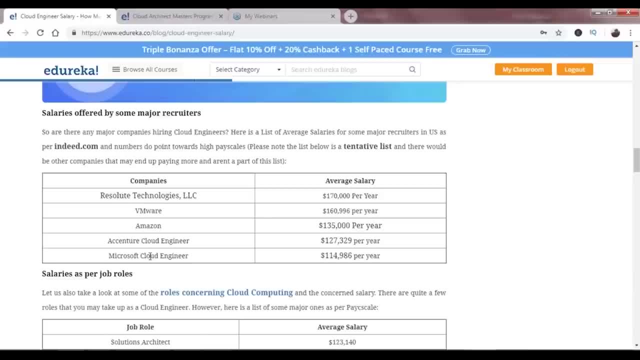 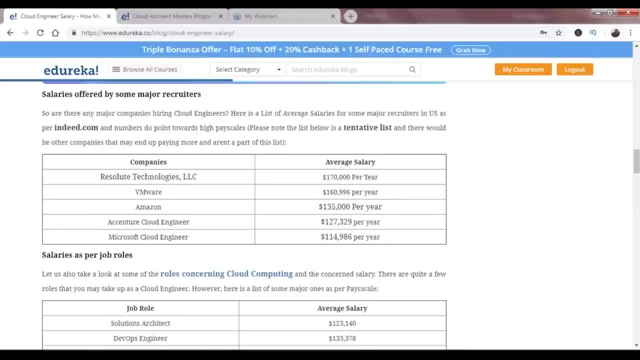 that actually act as vendors in providing He is cloud computing services. So, yes, major companies are going to move to cloud and they're going to hire you as a cloud engineer. having said that, let's take a look at some of the other factors that concern a salary of a cloud engineer. now, guys, 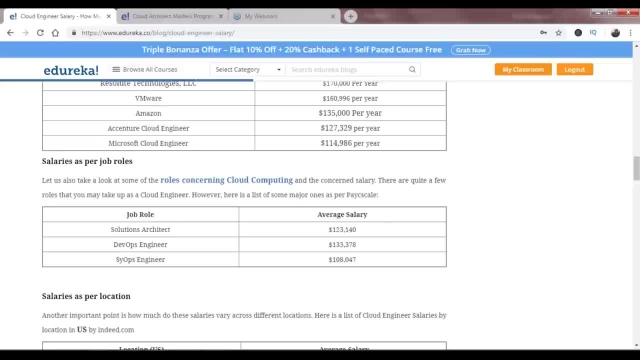 if you take a look at salary is based on the job roles. Now these are the three major job rules, that is, a solutions architect, a devops engineer and a sysops engineer, and these are the average salaries. I do not agree with these numbers that much. numbers can be deceiving. 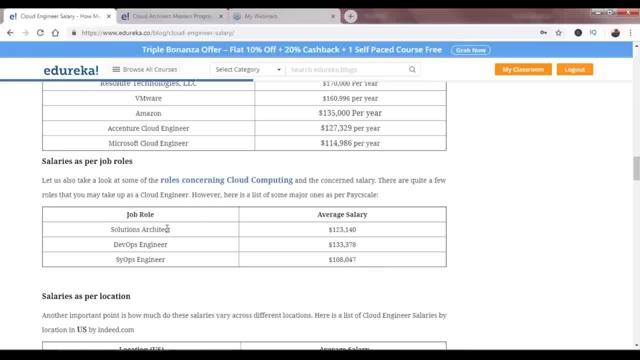 at times probably, solutions Architect is one of the most demanded cloud jobs. I mean, it is the most popular cloud certification. no matter what vendor you talk about, solutions architect is something that people demand a lot. So these are some of the job roles now apart. 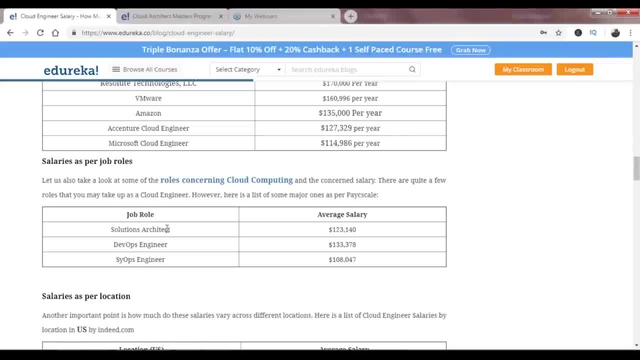 from these job roles. There are various other job roles as well, but more or less they follow this particular category or these three categories. as you move further, We would be talking about these job roles. do not worry about that, But these are some of the numbers. 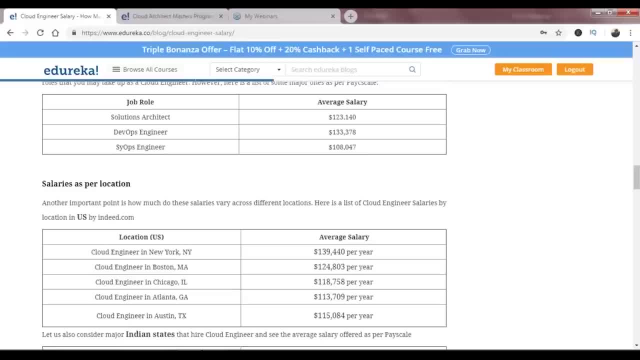 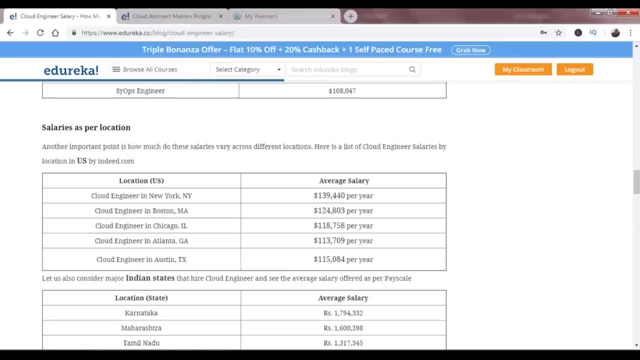 I want you to take a note of again, guys, based on the location, your salary might vary, and these are some of the positive numbers that are there again, I've used, indeed, as a source here, if I'm not wrong, because most of the data that I've picked- 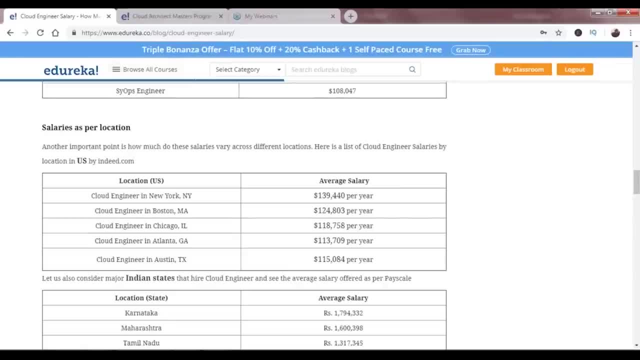 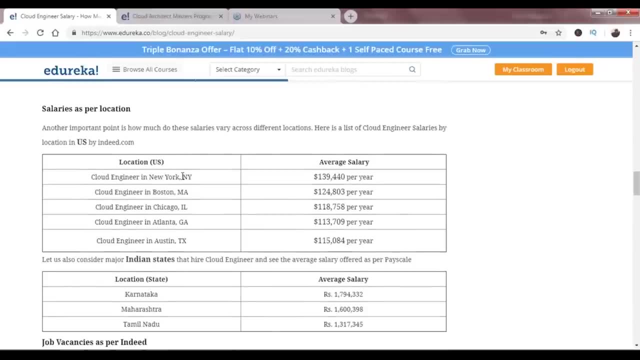 from. it is a combination of, indeed, pay scale and a couple of other websites that are popular when you talk about job trends. So, yes, when you talk about- indeed, these are the numbers that they've given as in based on these states or the location in USA. 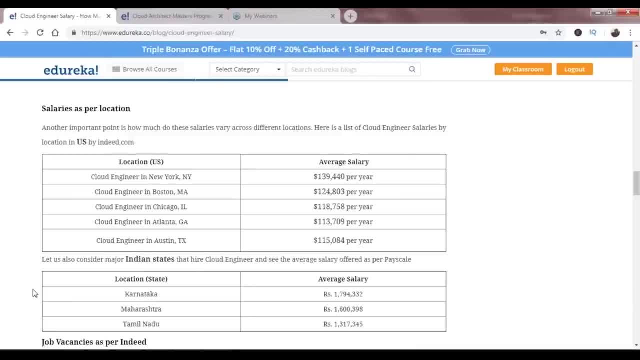 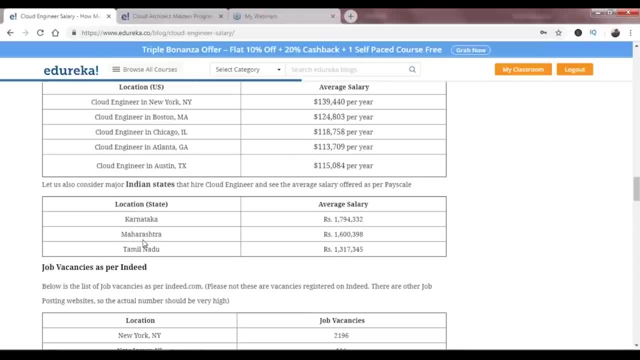 These are the salaries of its people can claim on an average. You have numbers for India as well. Now these are three of the major states that recruit. I know Delhi is one more state, but their numbers are similar to Maharashtra mostly. So yep, you can take that into consideration as well. 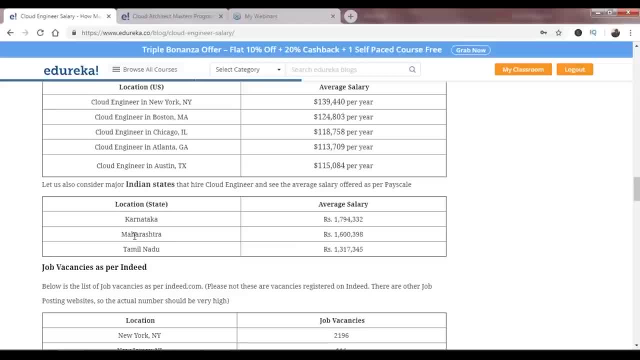 And I'm sorry, Delhi is not a straight city which popularly hires a lot of engineers as well. Delhi, Gurgaon- in that domain, or in that region in particular, the salaries are similar to what you get for Maharashtra guys. So, yep, these are the three states. 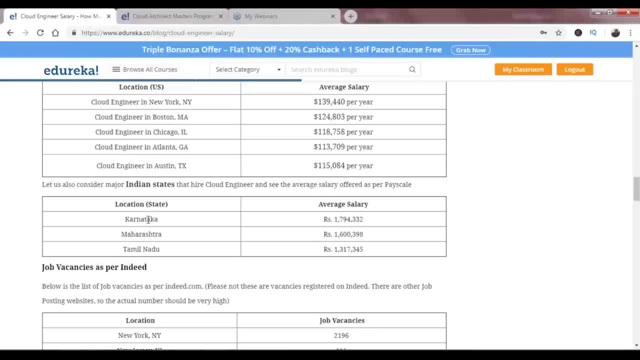 that the website shows numbers for guys and Karnataka, which is the ID hub of India. You can see the salary goes as high as this. This is the average salary, Maharashtra in particular. This is what which is very closely followed or follows very closely to Karnataka. Tamil Nadu to has a lot. 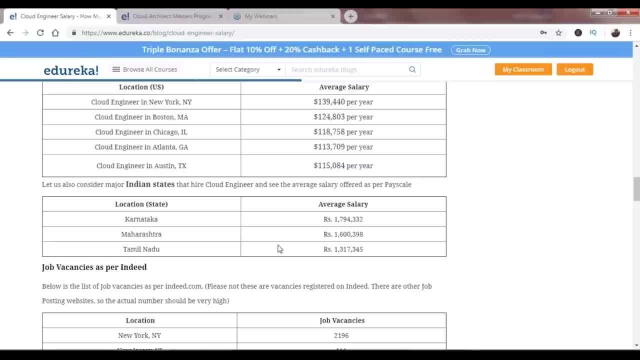 of requirements for cloud engineers And, as I've already mentioned, if you go to the Delhi part of the country, yes, there to, people are looking for these skills as well. It's not that the other parts of the country are not looking for people with these skills. 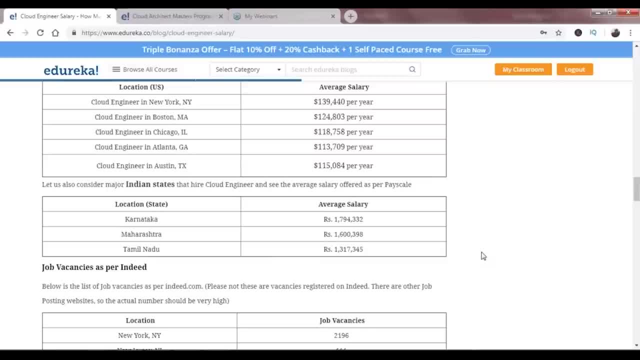 It's just that these are the major hubs and they come into the reckoning when you talk about the stats or the data. there are other regions and states where people are normally hiring cloud engineers there as well. I constantly go through or do market research a lot. when you talk, 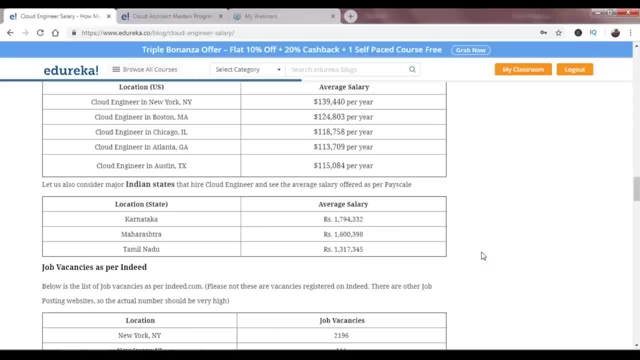 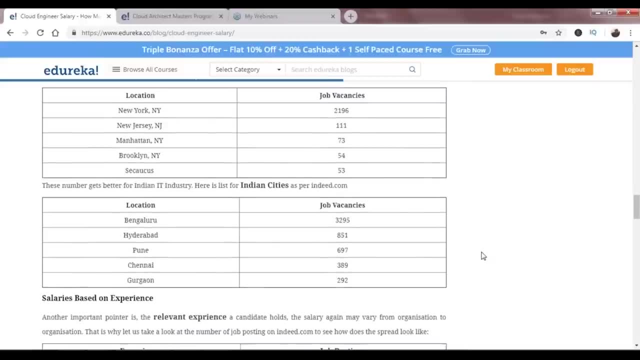 about cloud engineering in particular, and, yes, I've seen requirements in other states as well. again, guys, These are the number of job vacancies which you saw in the presentation. So, guys, yes, these are certain numbers that are there and, again, the numbers are based on. indeed, guys, 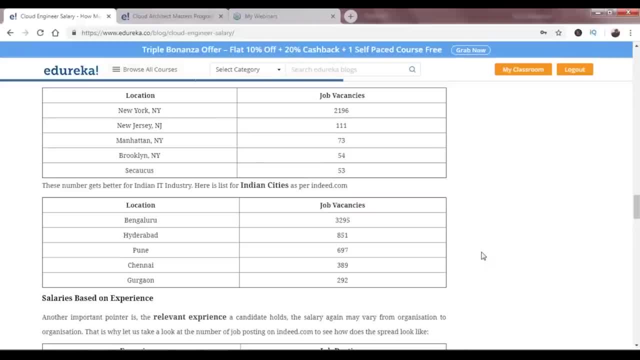 If you take a look at the other websites as well, you might find more numbers. So again, this is just a parameter, guys, and, to be honest, there are a lot more vacancies than what these numbers state. The problem here is people are not skilled enough. to actually go ahead and get these jobs. So yes, if you are rightly skilled, definitely these jobs would be yours. salaries based on experience: again, you can see mid-level has the most number of salaries, guys. Why is that? because cloud engineering mostly is a branch. 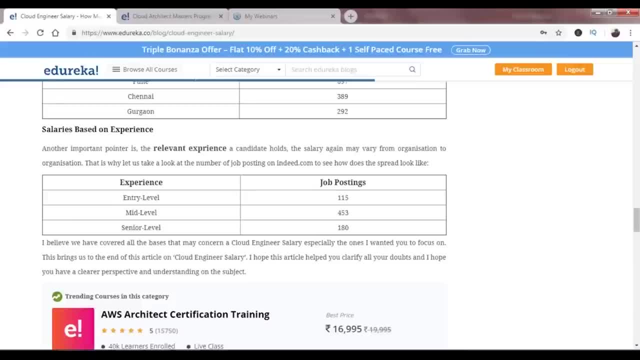 where you would be expected to have certain skills that you've learned while you worked. So an experience of three to four years is the best place or the best time for you to move to cloud. even two years is what I would say. It's not that pressure should not move into this role. they can. 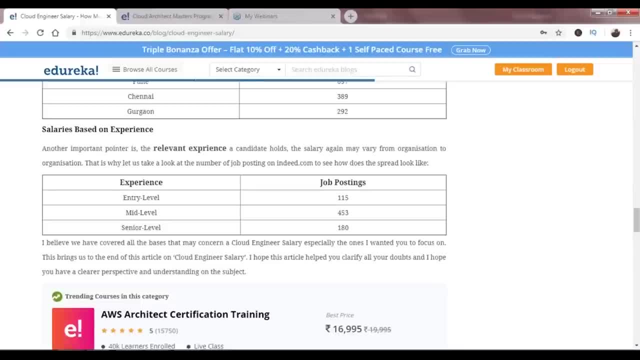 but again the number of placements that happen and pressures is lesser. Why? because the chances of them getting picked as a cloud engineer mostly happens through campuses. I would be talking about this factor as well. Do not worry. Once we talk about the resume part. 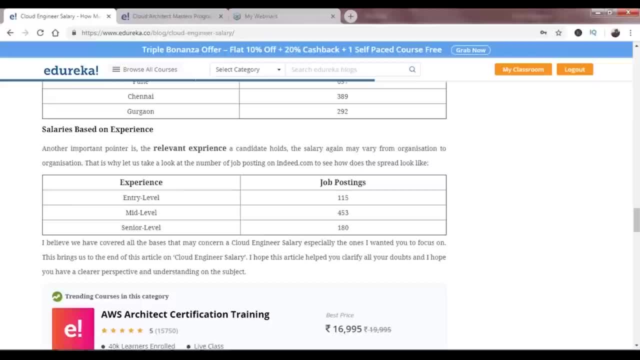 I would help you, even if you are an entry-level person, a mid-level or mid skill person or a senior person. I'd be talking about these pointers. I'm just taking certain numbers here. So entry-level people normally find it little difficult. The most expected part is mid-level. 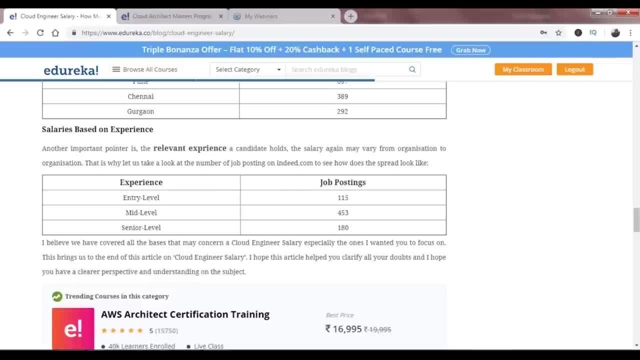 Why? because salary is something that companies can bargain on and these people are rightly skilled, senior level to people. higher These people. but what happens is, since you are very experienced, you normally would be expecting managerial kind of positions, right, So you cannot have too many manager positions. 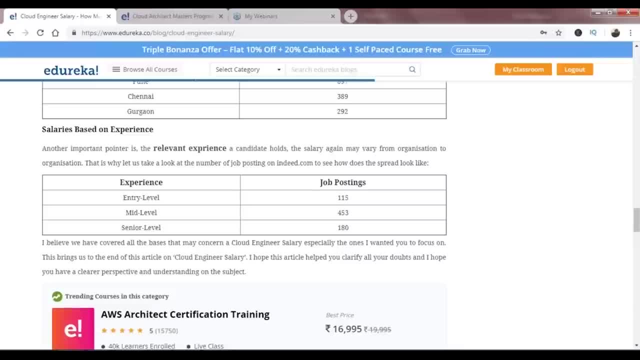 So it is understandable The number is not that high, but considering that as well, 180 on an average is a good number. So, guys, these were some of the parameters. I wanted to talk about salaries and certain job trends. I hope I've discussed enough. 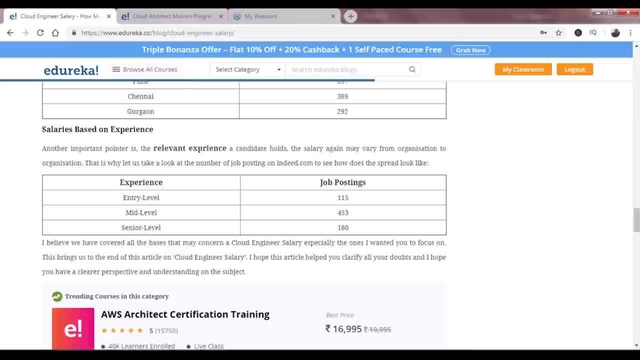 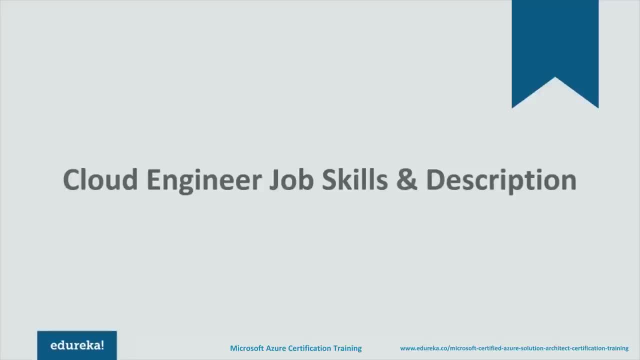 So, guys, let's just move further and switch to the presentation part, where I would be discussing certain other pointers that concern cloud engineer. So, guys, let's just move further and talk about cloud engineer skills and also the job description. now, guys, I've actually clubbed two topics from the agenda here. 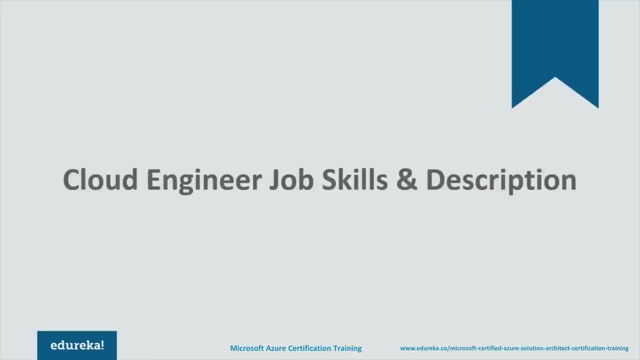 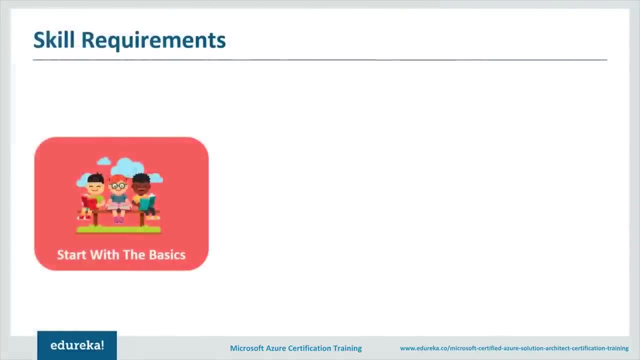 and I would be actually going to and forth while discussing these pointers, because I feel they are very intellect or very connected to each other. So let's talk about these pointers first and foremost. Let's talk about certain skill requirements If you want to become a cloud engineer. 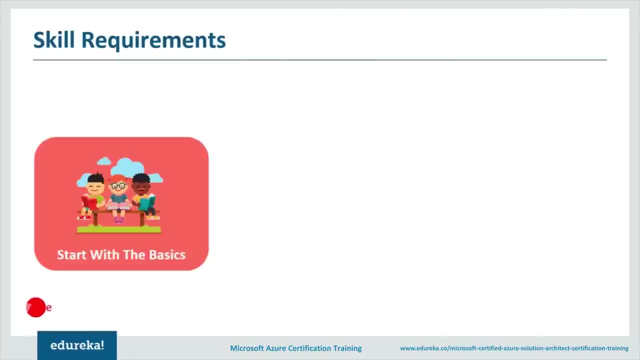 what are the stuff that you should know now, guys? for people who have experience, you probably might know some of these pointers already, but I am wanting to take everyone on the similar page and while doing that, I would be talking it from the very basic part as well. 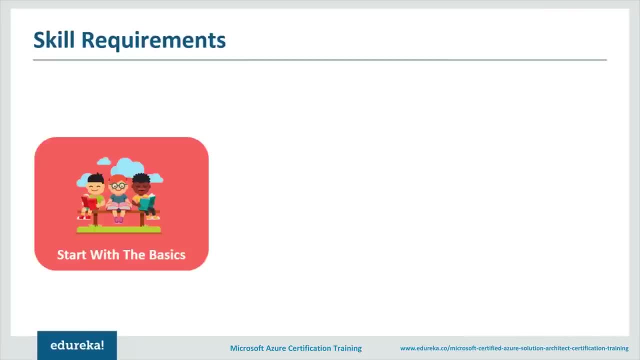 So let's get started with the basics first, as in what are the skills or knowledge set that you have in order to becoming a cloud engineer. So you need to have an understanding of why do you need cloud computing and what are the different domains that impact cloud computing. 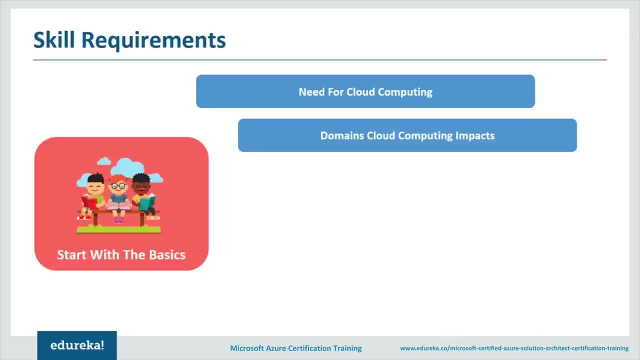 because, based on that, you would be able to decide as in: okay, what do you want to do with cloud computing? It is a very vast domain and it has various services that are there or that are made available to you, using which you can do so many things. 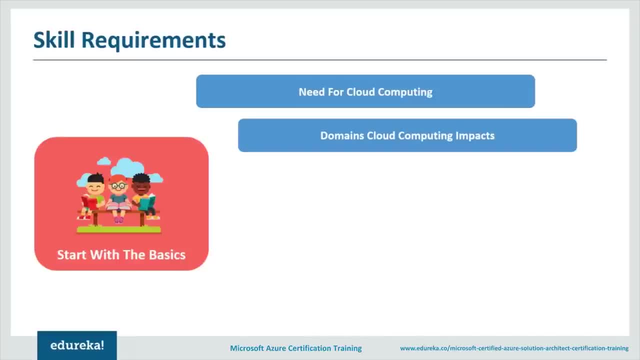 You can focus on marketing proper software development architectural part. for that You need to understand why do you need cloud computing, What are the different domains that it affects, and once you do that, probably you would be in a better state to decide how do you want to use cloud computing. 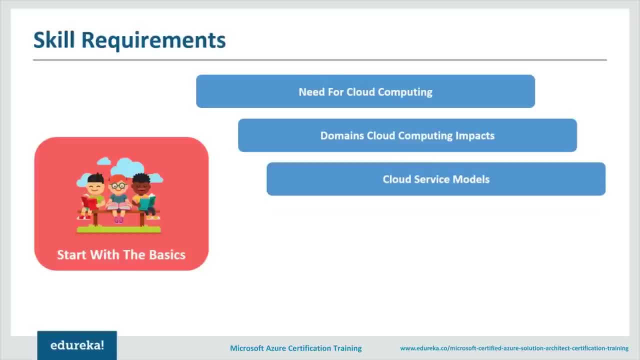 for your own benefit. moving further, You would also be required to have knowledge about different cloud service models, as in. these are something that tell you how can you use your applications or how can you build your applications using cloud computing. That is why understanding of this topic is important. 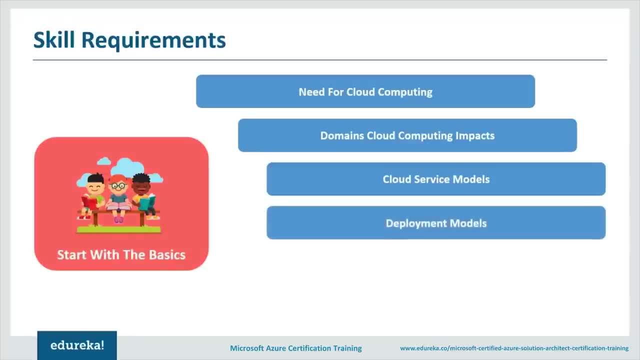 You need to have an understanding of different deployment models, which again is similar to or related to cloud service models as well. It is the way cloud services are provided to you by your cloud vendor. That is where understanding of different deployment models is also important. 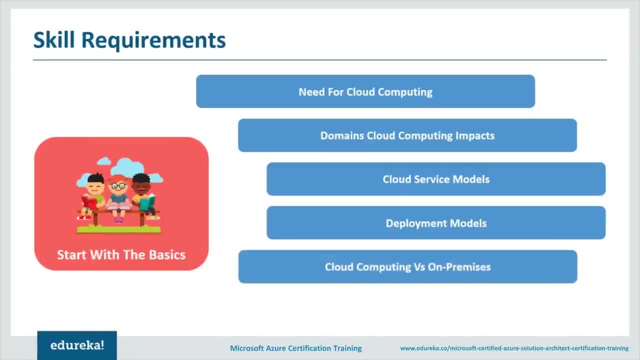 You should understand Why do you need to move to cloud computing and why is it different from an on-premise architecture or an infrastructure? rather finally, you need to have an understanding of different cloud service providers or vendors in the market, because having an understanding and thorough knowledge of at least one cloud service 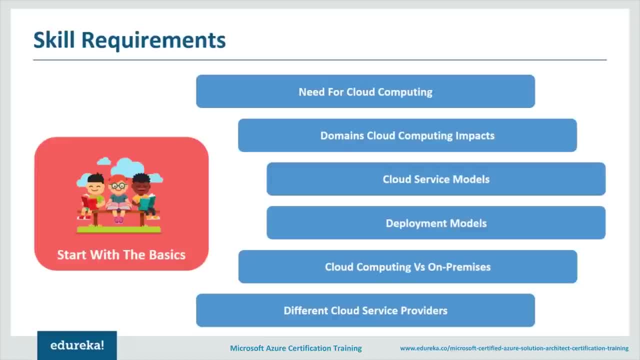 provider is very important and, guys, when I say a cloud service provider, it is very important to understand that there are various in the market, but preferably people normally start with AWS and they gradually move to Azure, which are two of the most popular cloud service providers. 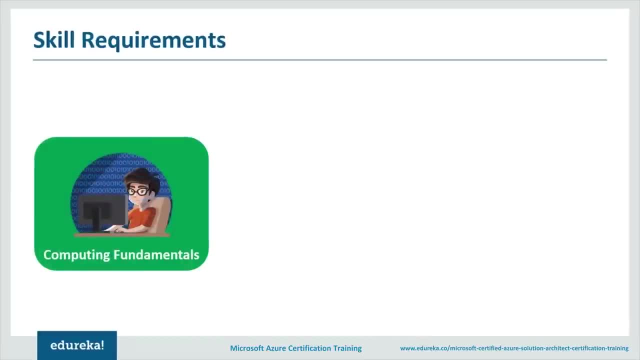 So what are the computing fundamentals that you need to have now as a cloud engineer? guys? I won't lie to you. I won't say that you don't need any prior programming experience or anything like that as a cloud engineer, guys, you need to have understanding. 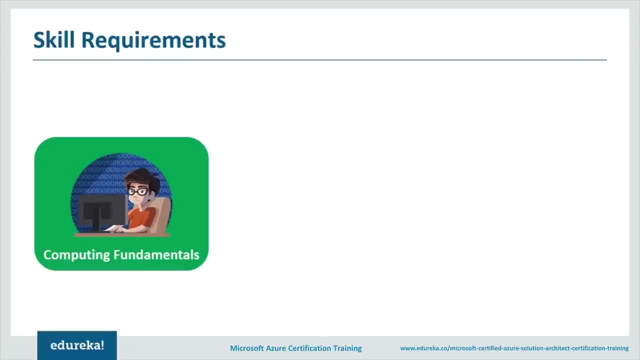 of computing fundamentals and it is very important in becoming a good cloud engineer. What should you know? networking is very important, guys. Now it is not that much into programming, but understanding of computing. it starts with networking. You need to understand how routing works. 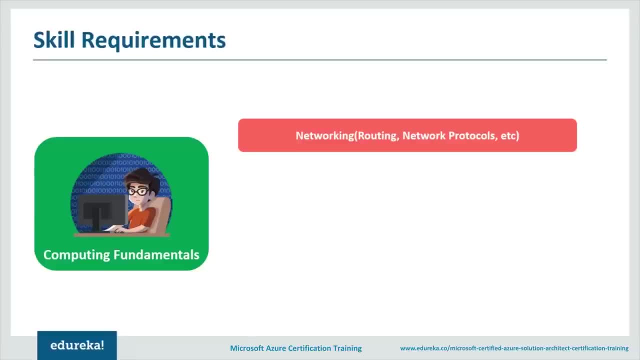 What are different network protocols, What are different networking layers, Etc. And how do you use networking for an organization? because it is very important. You would be talking about a lot of applications, lot of data, lot of scalability, application building and stuff like that. 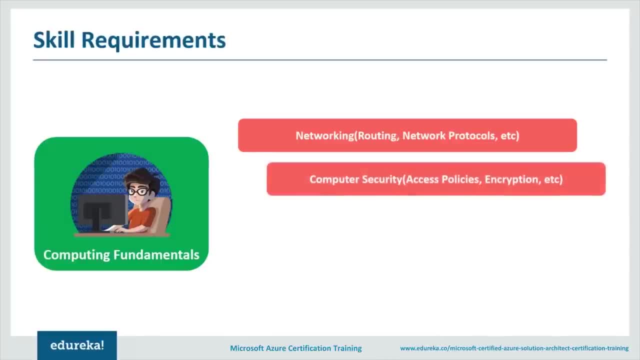 So for that networking becomes very important. Computer security guys. Now, when you talk about cloud, the first question people ask is: is it secure? most of the people do not know what cloud computing does or how it ensures security. Let me give you a fact. 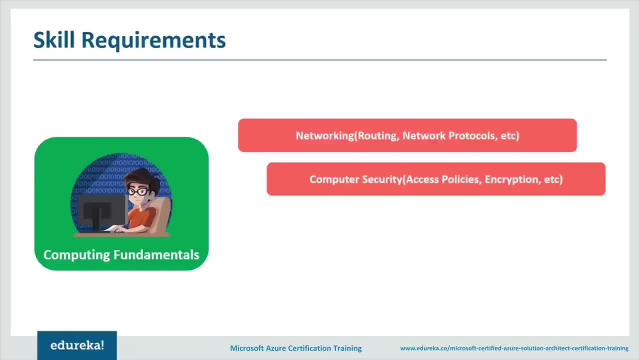 They use shared security model. what it is? I won't be getting into the details, but you and your cloud vendor, you actually go ahead and decide certain security principles and those are implemented. So if you are working on a cloud platform and if you are into the security part, 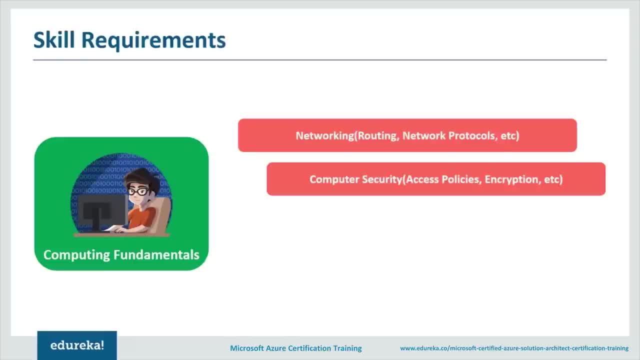 you need to ensure quite a few things as in how to make your application secure, What are the protocols that you should follow and stuff like that, And for that you need knowledge about access policies, encryption, Etc. understanding of systems is very important, guys, where you need to know what are the different design principles. 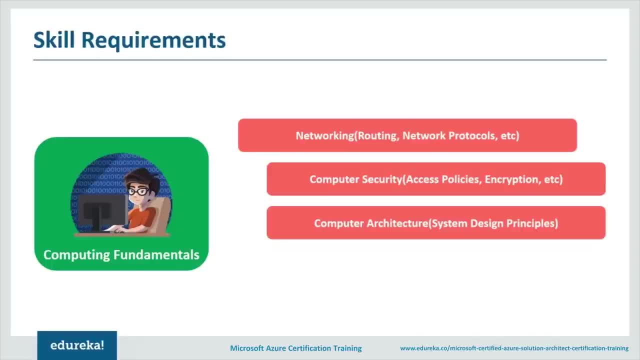 What kind of methodology are you using and where do you get the knowledge for these things? your computer architecture. You need to have an understanding of databases. You need to learn SQL, which is very important because you are going to deal with a lot of data and guys. 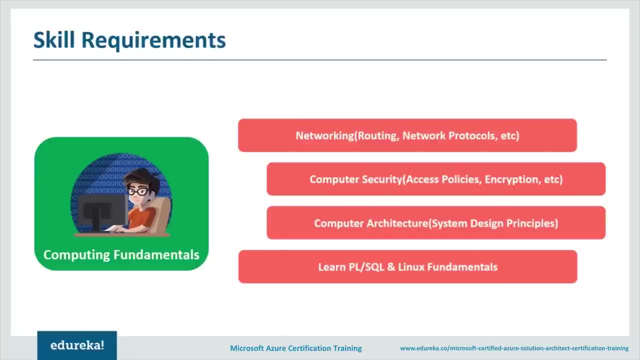 since you're talking about cloud platform, you would be dealing with different kinds of instances or virtual environments, and for that, understanding of Linux fundamentals is very important. So these are some of the basics, guys, which you should understand, and I would suggest that if you are completely new. 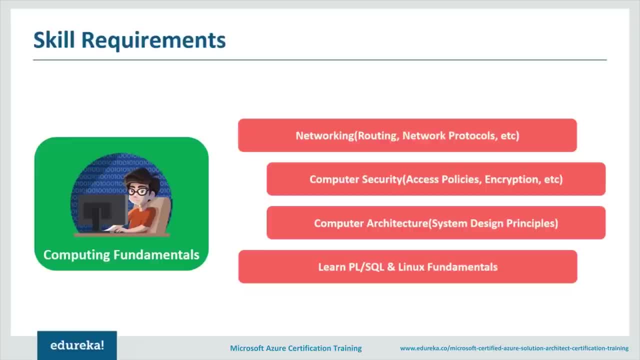 to cloud computing. focus on these pointers as well. So these are some of the basic skills that you needed to have. now let's just go ahead and take a look at certain job roles and, based on those job roles, What are the skills that you should pick up? guys, now again, 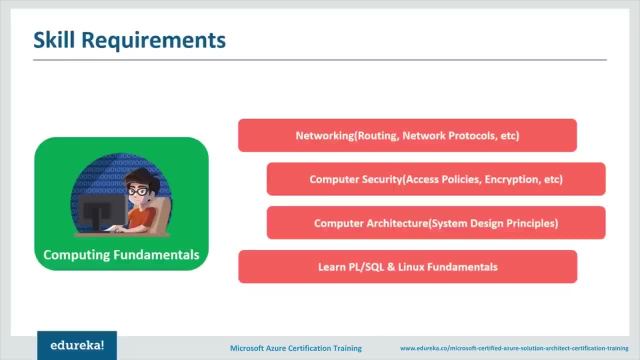 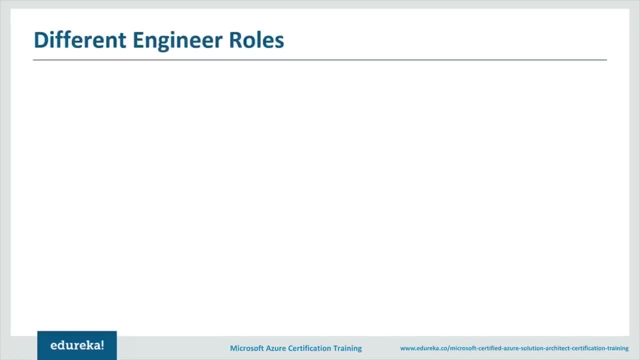 these are the responsibilities that even major companies would be expecting from you. So when I said I would be talking about job description, now these are certain roles and the pointers that I'm going to talk about. the responsibilities, Those are the skill sets that major companies expect from you. 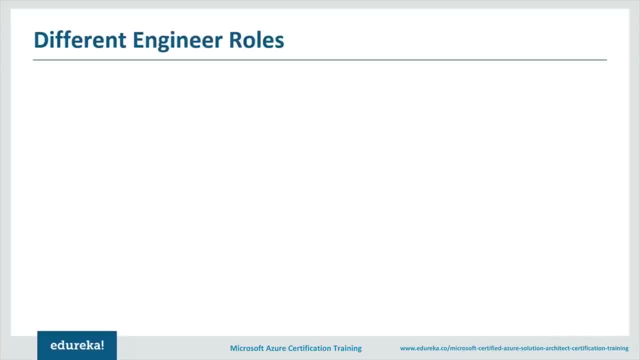 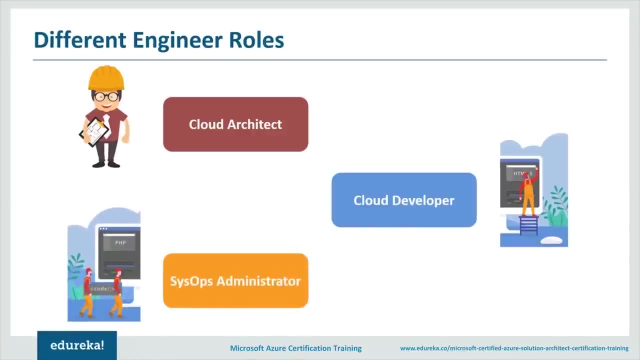 when you actually do go ahead and try to apply for cloud engineering jobs. So, first and foremost, we have an cloud architect, cloud developer, and an admin sysops. admin is nothing but system operations administrator. So, guys, let's try to talk about these roles in detail, guys. 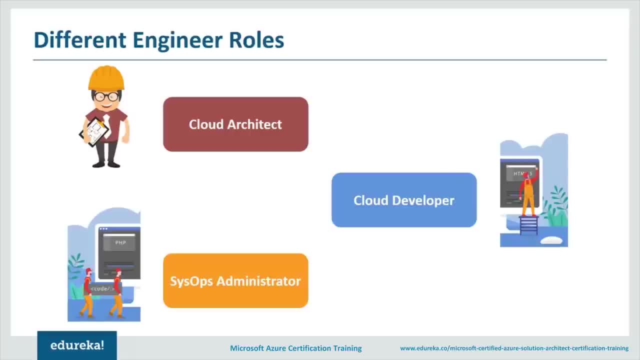 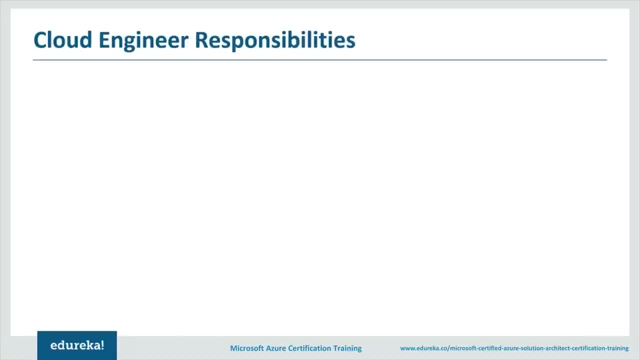 I won't be getting into the definition part. I would be sticking to what I've experienced till time when you talk about cloud engineering. So my definitions are going to be very general and basic so that everybody can understand. So if you talk about the cloud architect, 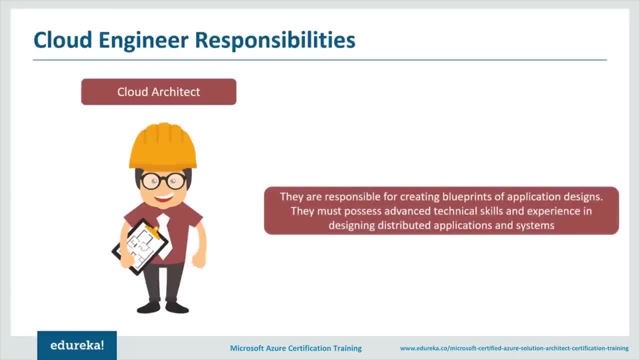 these are the people who are responsible for drawing the blueprint. I mean, they actually design your application as in. this is how it looks. so their part is designing planning stuff. like okay, when I actually go ahead and build an application, This is how much I might be expected to probably scale. 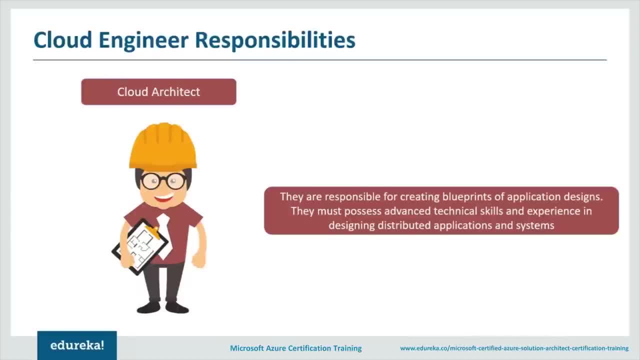 or these are the current softwares or these are the current programming languages that I would be needing. They also take into consideration, when it comes to migrating your application, which already exists on-premise. So they need to understand what are the parameters that affect the current application on-premises. 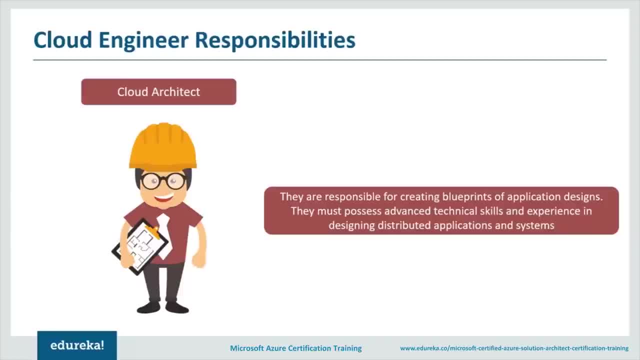 and, based on that, decide as an: okay, These are the changes that we need to make when we move this application to cloud. So this is what a cloud engineer does: They actually help you design a flow for your application to actually go ahead and work on cloud. 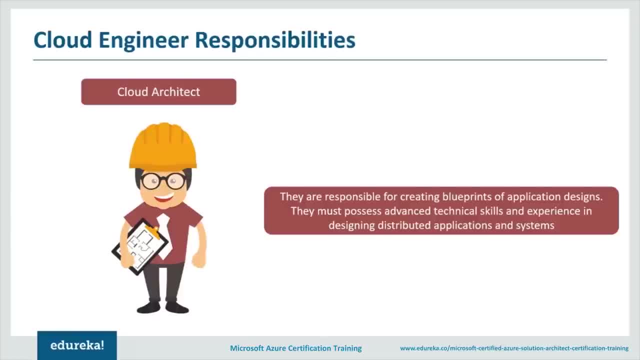 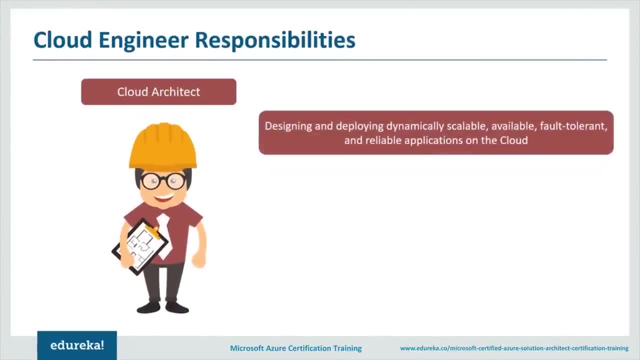 Let's just move further and take a look at some of the common responsibilities that a cloud engineer or a cloud architect is actually responsible for. they actually responsible for designing and deploying dynamically scalable, available, fault-tolerant and reliable applications, something I talked about while going through the definition part. 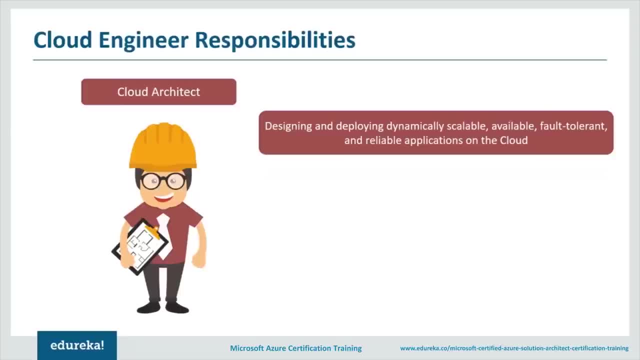 They actually design and deploy applications. Now, these are some of the pointers that concern an application, like how available it is, how easily can scale, how fault-tolerant it is. Let's not get into the details of that. I'm sure nobody wants to get into the details of that. 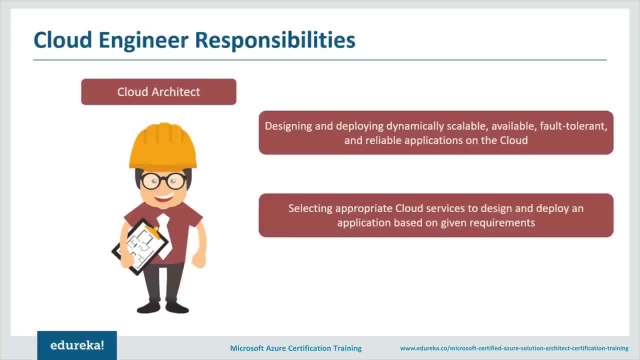 You should be able to select an appropriate cloud service to design and deploy for your applications. I mean, you would be dealing with different cloud vendors, So you should know, okay, if I have real-time data, what kind of an application do I use if it's static? 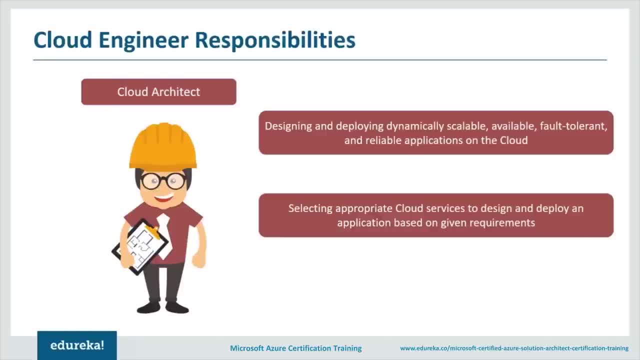 What kind of application do I use? so having an understanding of these things is also very important for an architect. again, I talked about migration. What are the factors they need to consider while migrating an application to cloud? again, you are expected to design and deploy enterprise-wide scalable operations. 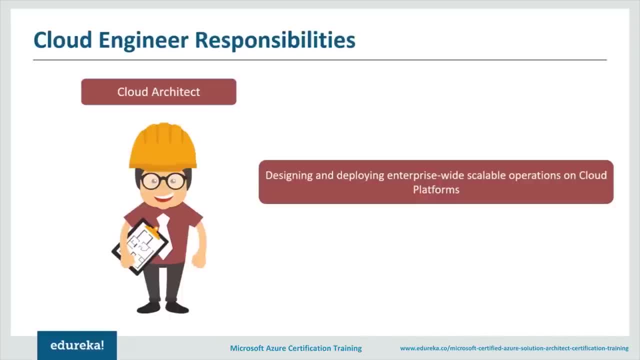 Now, again, it sounds similar to the point which I discussed, right, but again, you also need to have an understanding of operations that are performed while your application is working. Now, this is something that is important when you talk about the deployment process and dealing with the customers part. 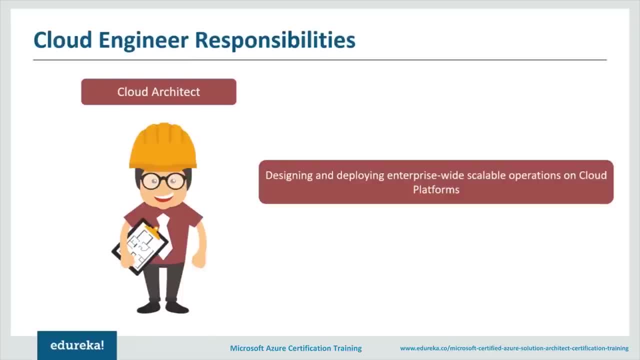 because, based on that, your operations team has to put in certain inputs and it is designed properly at the beginning. Your workload gets reduced here. So this is where cloud architect again comes into picture. implement cost control strategies to ensure maximum cost optimization money. This is something that is very important. 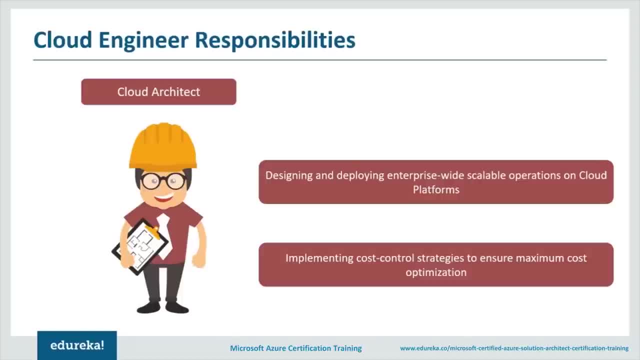 And if you plan your applications properly as an okay in case of using a particular kind of a service, if I use the other one, would it be cost effective? This is the decision again, your cloud architect should be able to take. Okay, moving further, 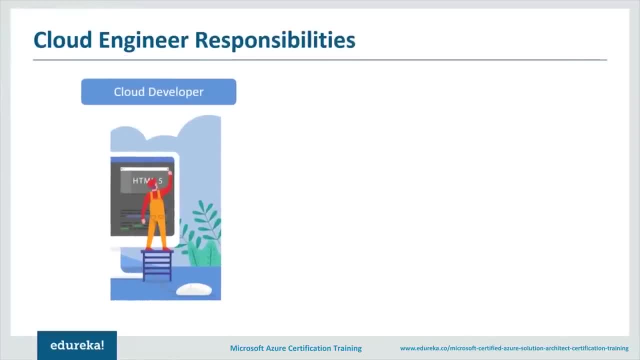 We have the cloud developer. now We have already designed our application with the help of an architect. next is building an application. Who does that? your developer. so they need to have strong understanding of programming. apart from that, Let's move further and take a look at some of the pointers. 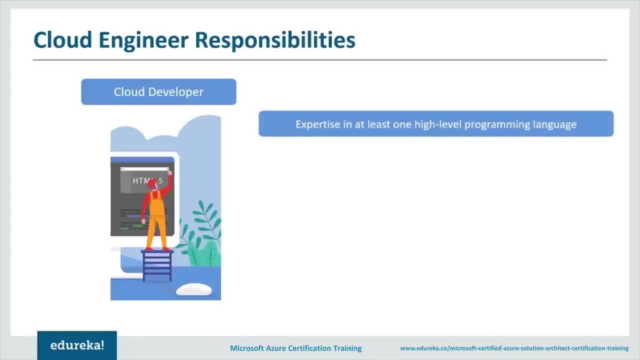 and what are the other things? they need to be concerned with expertise in at least one high-level programming language. I'm sure it's more than one, but yeah, you should know the basic programming fundamentals so that you can understand how the coding works. skills for developing, deploying and debugging cloud applications API. 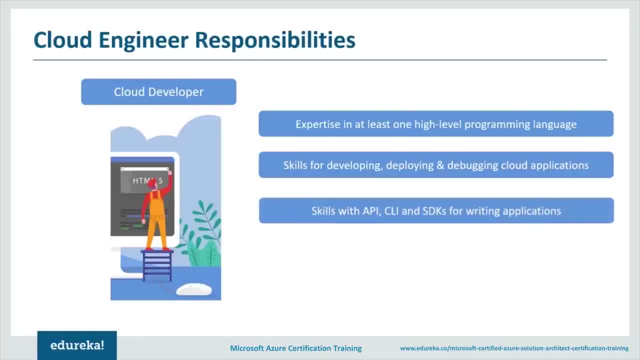 CLI SDK is. it is very important, guys, because you would be integrating a lot of applications and for that, understanding of how application protocol interfaces work is very important. now, command-line interfaces are something that you would be working on with a lot as well, So having an understanding of those also helps application. 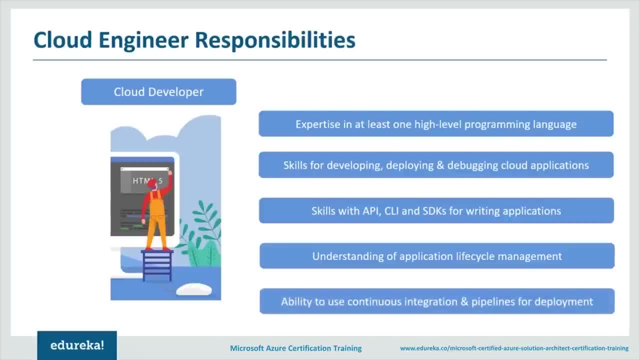 lifecycle management, which is very important, ability to use continuous integration. and pipelines for deployment. Now, this is something both developers and the admins to, so you need to have an understanding of how these pipelines are created, how they work and how do you deploy your data continuously. 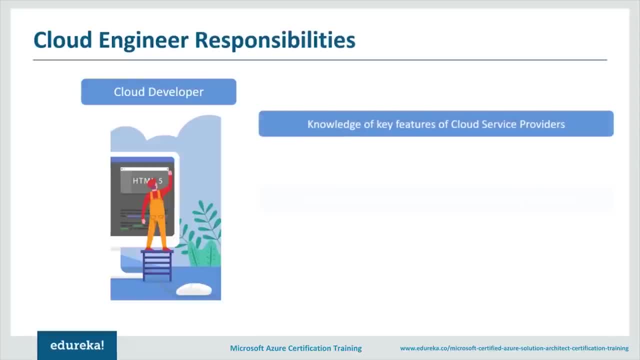 You should have the knowledge or the understanding of key features of service providers, guys, because, again, if you're building an application on cloud guys, you should know how these service providers work, because you would be using a particular service to go ahead and actually build a particular part of your application. 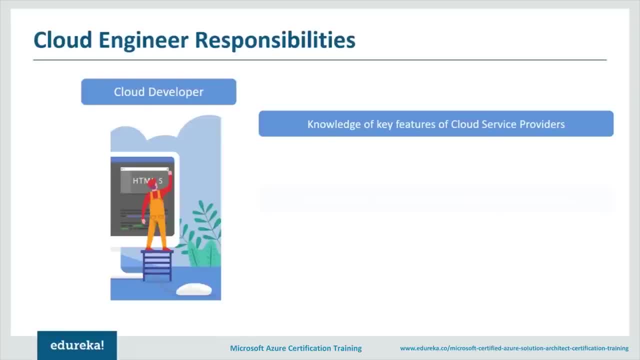 So an understanding of different cloud service providers is very important. You should be able to code and also make sure that you are thorough with the security essentials: skills in writing and correcting and debugging code. again, testing and building is something that goes parallelly. serverless applications. 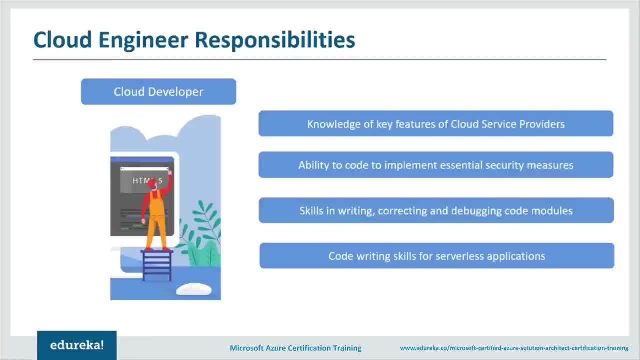 cloud computing supports serverless computing, and that is where you should know what serverless applications are and how should you use containers- containers, or something, that are trending in the market, and you need to have an understanding of those as well. If you take a look at the resumes, 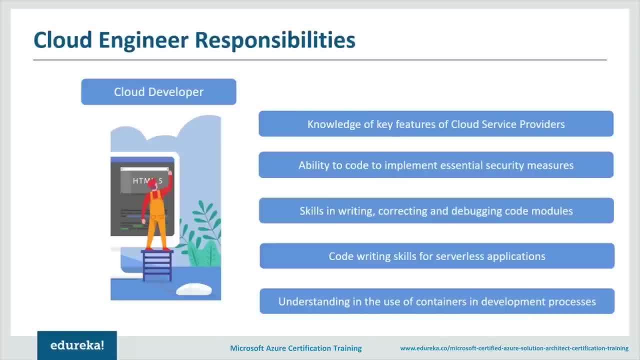 or the job descriptions in the market. people expect you to have understanding of different service providers, understanding of different APIs. at least one programming language- and they have this thing mentioned there, as in a knowledge in Kubernetes or Docker- would be an add-on. So that means they consider these skills as well. 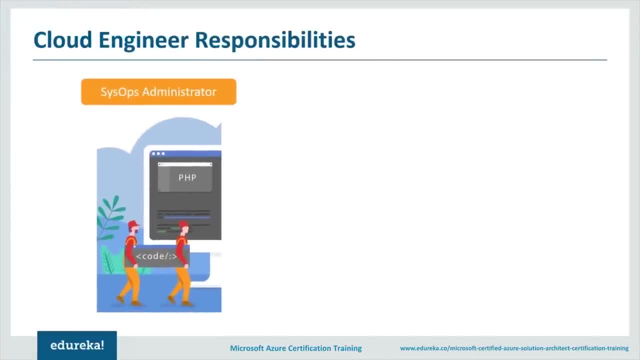 Then we have the admin guys. now our application has been designed and it has been developed how it needs to be maintained by someone, or monitored by someone. who better than an administrator? So their job is to actually go ahead and make sure that the application runs perfectly. 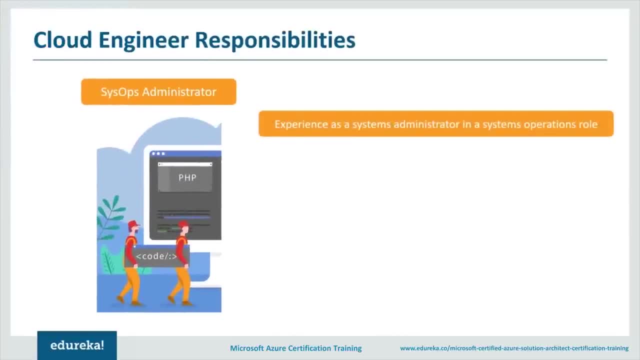 in the production environment. What do they do? They need to have an experience as a system admin, and they should be able to understand how virtualization works, something which is very important for scaling your application in case of peak times. monitor and audit your applications again. 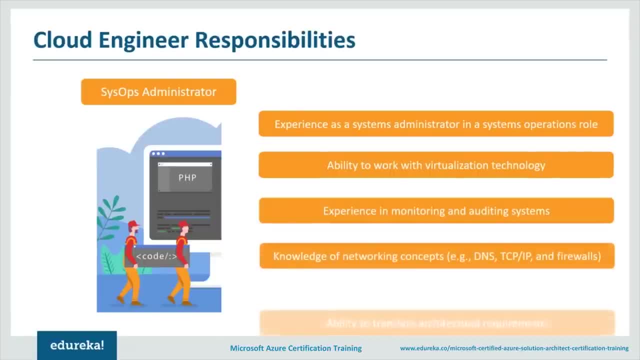 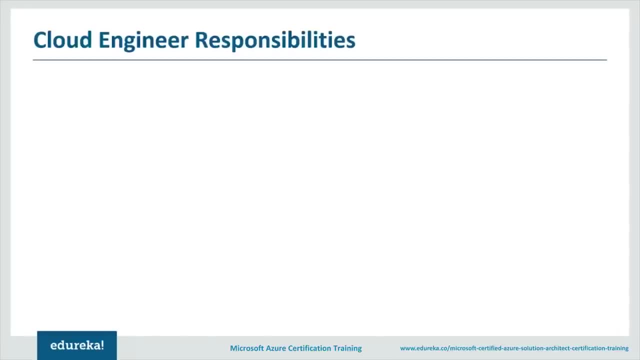 have understanding of networking, which is very core for an admin role, and to translate architectural requirements, because they are the ones who take care of it in the production atmosphere or the environment. they should be able to actually go ahead and control the data flow because, again, if something goes wrong somewhere, that is during the process of CICD. 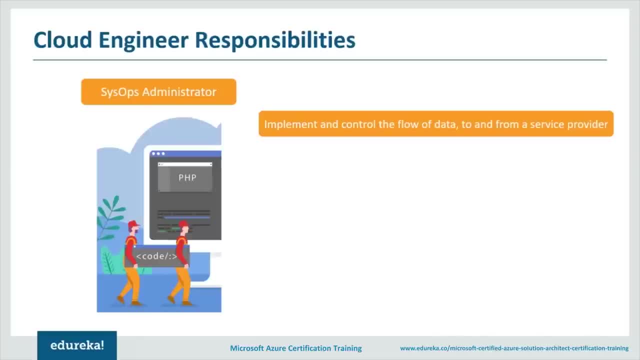 They should be able to detect that and get in touch with the developers team as well. appropriate service-based. They should also have the knowledge of security. if something goes down, how should they actually go ahead and take care of it again? optimization is something that is not the concern to a greater extent as far. 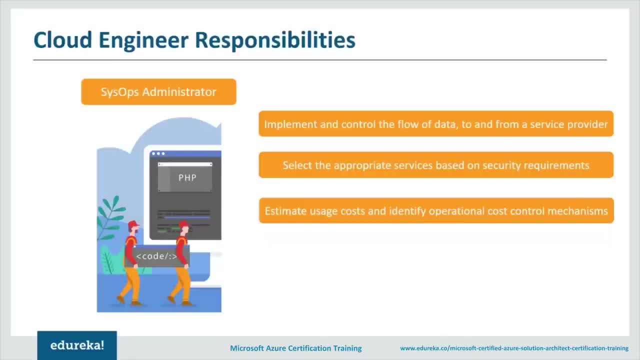 as your architects are concerned, administrators have lesser responsibility in it. Okay, networking is something that has repeated, I believe, but yeah, we've discussed that already- and migration is something they are also concerned with, because I've already talked about the fact that they deal with the production environment. 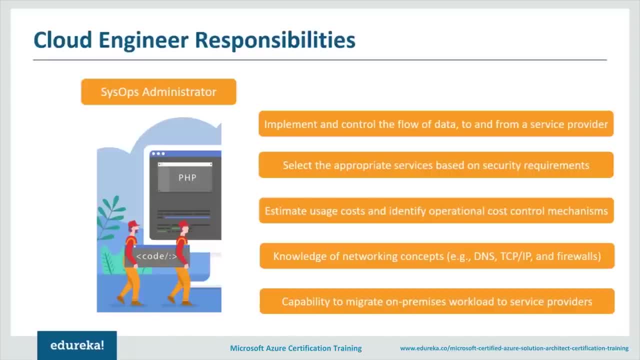 So, guys, these are some of the responsibilities that different cloud engineers take care of, and these are some of the responsibilities that companies would be expecting you to be skilled in. So these are some of the pointers I wanted to talk about. that is, about the job description. 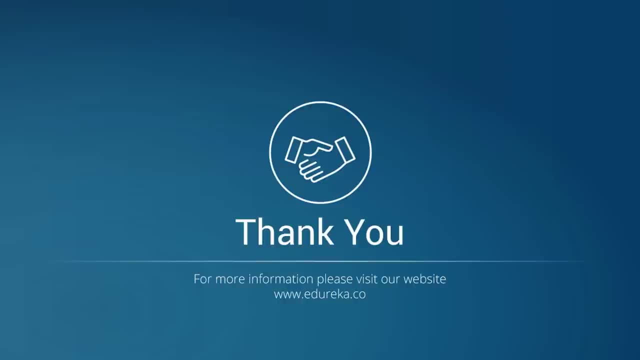 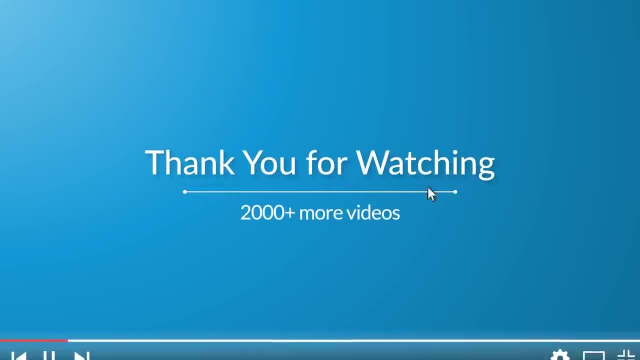 and the rules and responsibilities of a cloud engineer. having said that, as far as this particular session goes, guys, I would be resting it here in here. Thank you, Bye, Bye. I hope you have enjoyed listening to this video. Please be kind enough to like it.